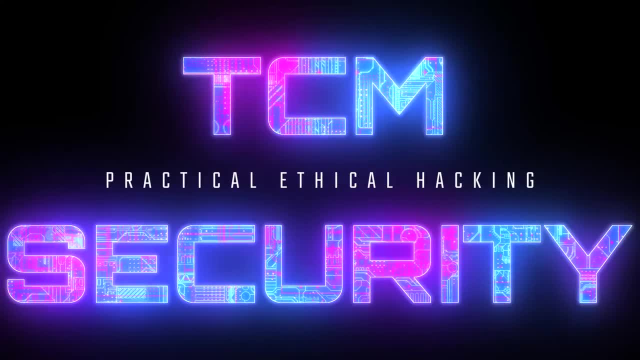 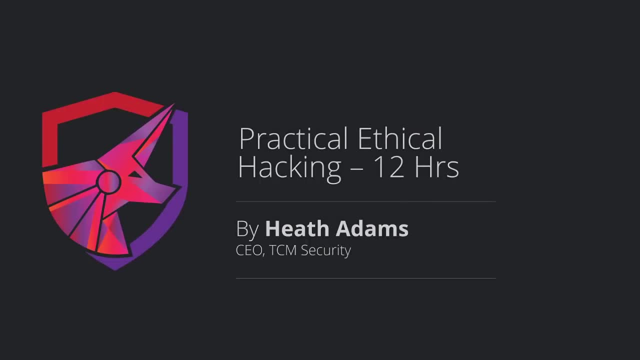 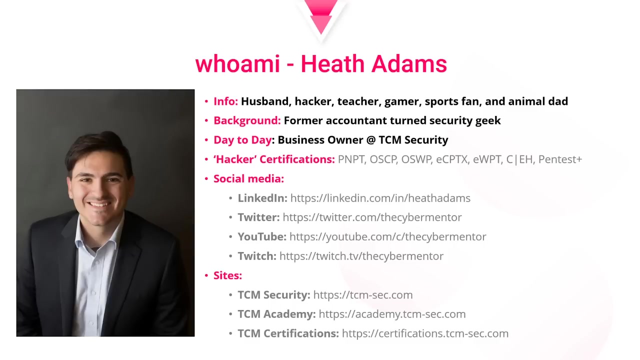 Hello everybody and welcome to this 12-hour edition of Practical Ethical Hacking. My name is Heath Adams and I'm going to be your instructor for this course. A really quick, who am I? I am a husband, ethical hacker teacher, and when I have time, 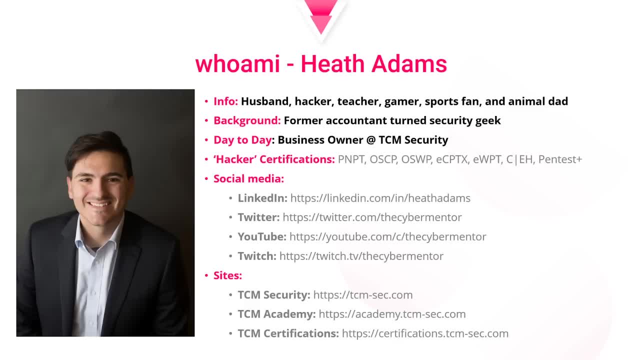 gamer, sports fan and animal dad. I am the business owner at TCM Security. We are a cybersecurity consulting and education firm. I do what is called ethical hacking, meaning companies pay us to attempt to break into them. It could be through a network, wireless network, a web. 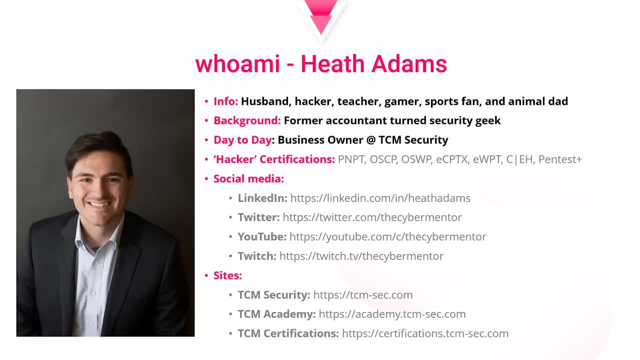 application, even physical pen testing like a building, Anything that they want us to try to hack into. we're happy to do it, And there's careers out here that involve physical pen testing, like a building, anything that they want us to try to hack into. 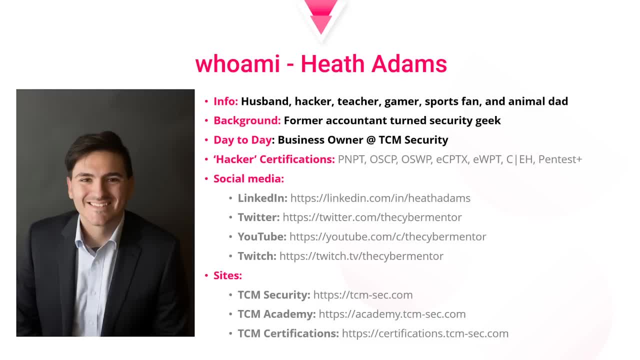 ethical hacking. It's actually a booming industry right now and a lot of people are coming into this industry from unique backgrounds. For example, I was an accountant and I ended up in this industry and I've seen doctors, dentists, lawyers- all kinds of random backgrounds that have just come. 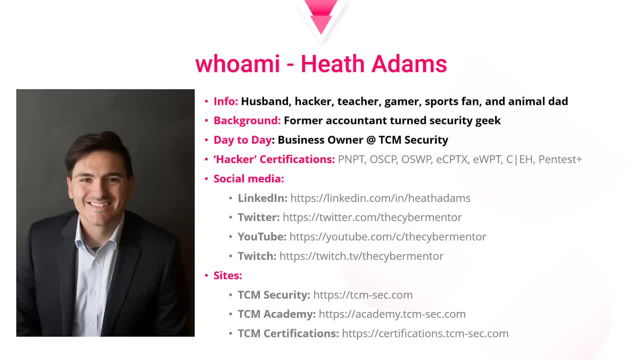 to this industry and found homes here. So if you're interested in ethical hacking, this course is designed for you: to brush you into the basics, help you understand what an ethical hacker does and some of the techniques, And it's going to be all hands on. I am not a PowerPoint person. 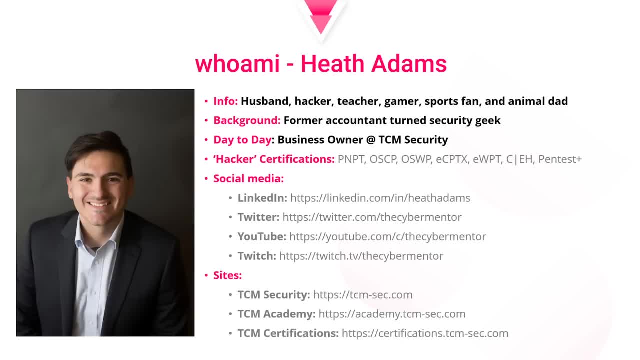 whatsoever. So this is the little bit of PowerPoint that you're going to get at the beginning of the course, And then we're going to get into heavy hands on techniques. So if you're interested in finding more out about me, I am very approachable. You can find me on LinkedIn, on Twitter, here, on 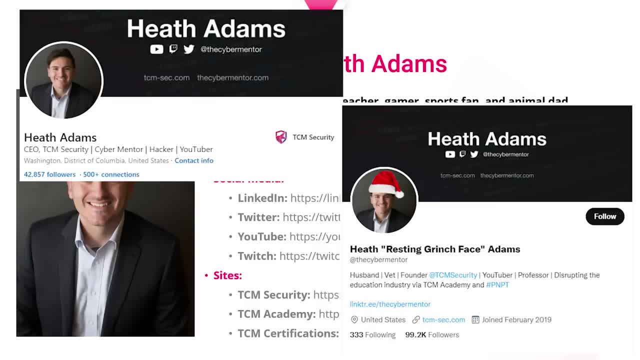 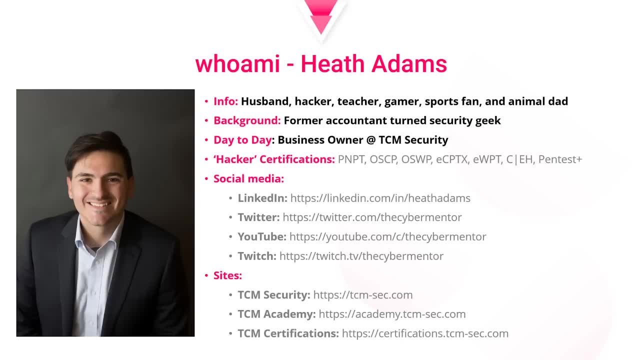 YouTube. I would love if you hit the subscribe button. comment, hit the like, let me know how you enjoyed the course. And of course, you can find me on Twitch as well. We do a lot of stuff on live streaming: some ethical hacking streams, some Q&A, et cetera, et cetera Down below. 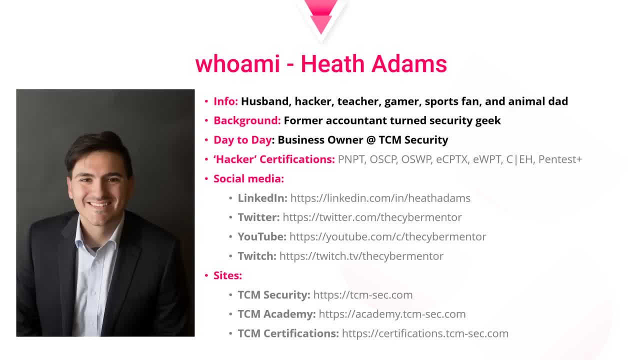 you see sites. TCM security is the consulting side of the business, The academy is the educational side and the certification side is the certification side. So I'm going to cover that really quick and what this course is and what we're going to do in this course. 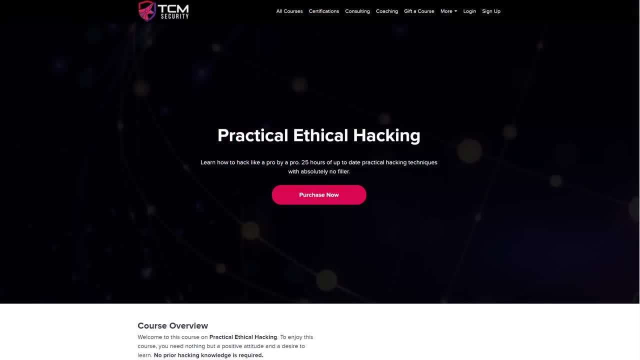 Okay, so welcome to Practical Ethical Hacking. This is 12 hours of 25 hours of a course, So full disclosure. this is not the complete course, though. This is a course that takes you through the first half and gets you to a good stopping point. So, reviewing the curriculum. 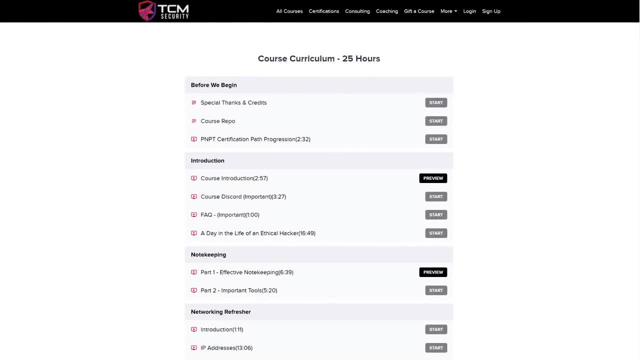 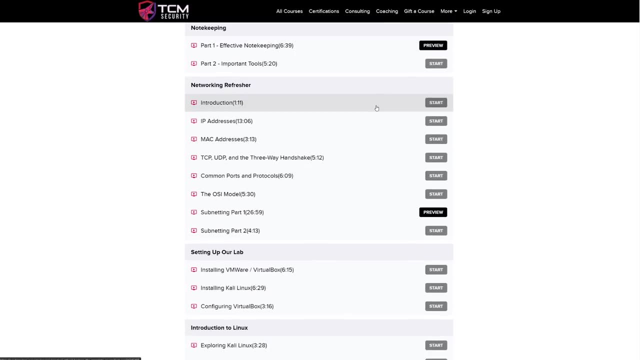 I'm going to scroll down here and I'm going to link everything in the description as well. We're going to cover a few things in this course. We're going to talk about note keeping, We're going to go over computer networking and also Python. So if you've never used Python or 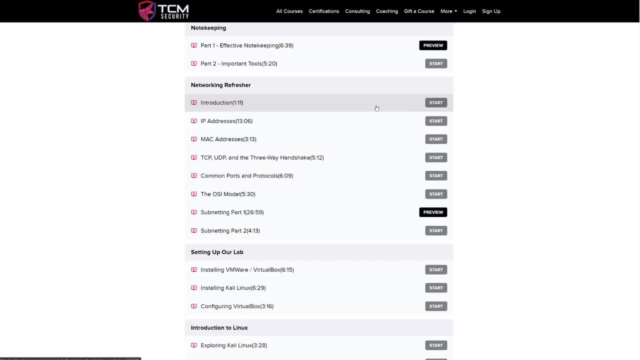 if you've never done anything with computer networking. we're going to kind of cover that, And so we'll cover some of the things that we're going to cover in this course. So let's get started foundational skills before we get into ethical hacking, And that does include note keeping and 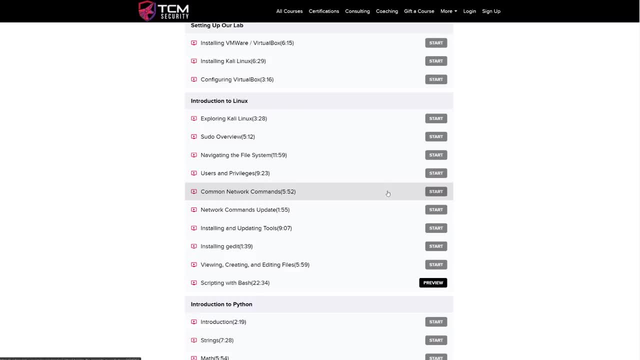 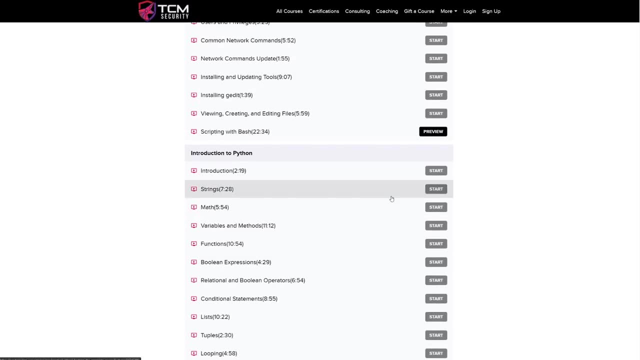 setting up a lab and installing Linux and running through Linux as well. So we built all the foundations in this course before we start getting into ethical hacking. So once we get through Linux and Python and we get through our computer networking, we start getting into the 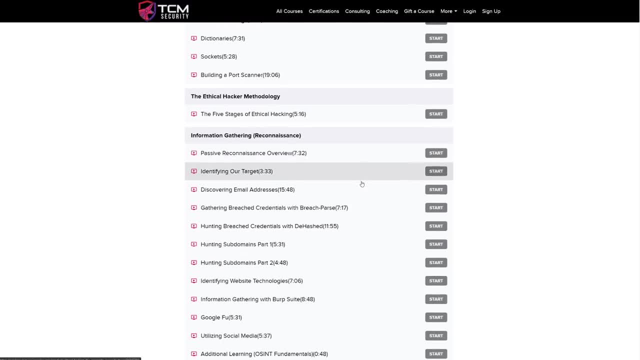 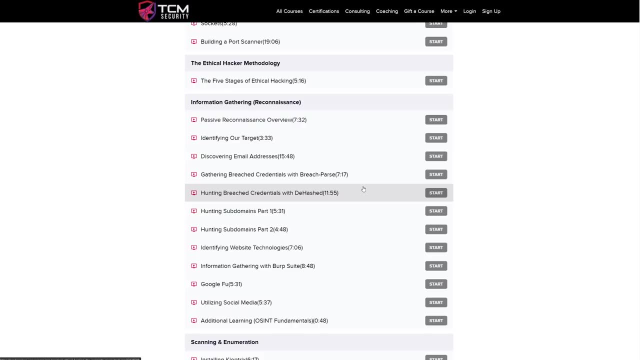 ethical hacker methodology. we talk about the five stages of ethical hacking And then we start getting into information gathering. What information can we gather about our target? We can look at social media. we can look at finding email addresses, finding intelligence about these companies or individuals or whoever it is that we are paid to target, And we'll do that. 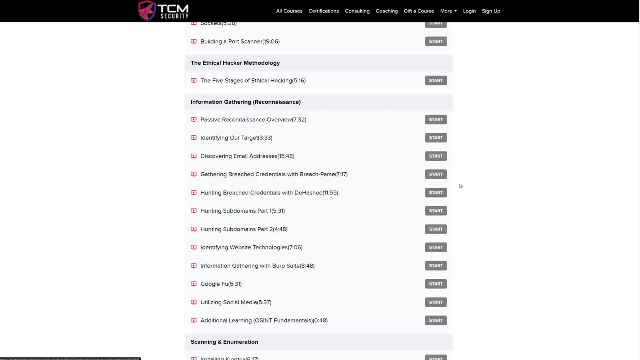 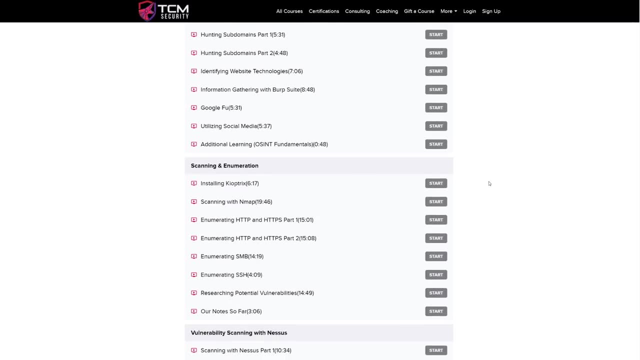 through information gathering and reconnaissance. There's a bunch of different techniques that we can do. Then we'll move into the next phase, which is scanning and enumeration. we're going to have a intentionally vulnerable machine that's presented to us. we're going to scan that with tools that you 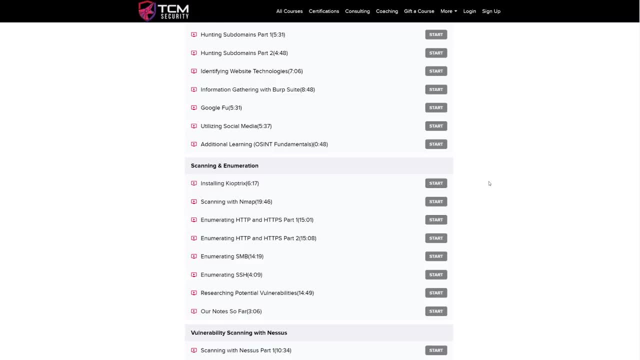 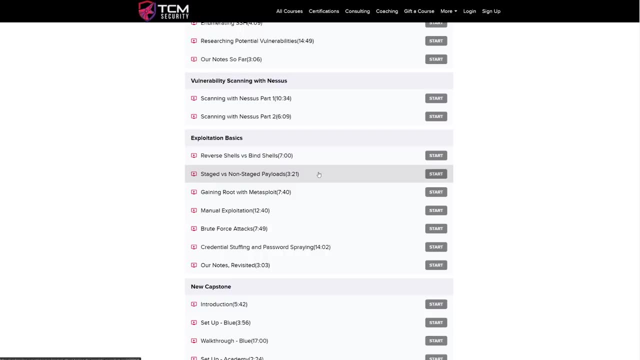 learn throughout the course, Identify what vulnerabilities might exist within the machine, And then we're going to eventually start hacking it. So we'll get into exploitation and talk about how we can hack a machine, understand the basics of exploitation and then eventually hack a machine. 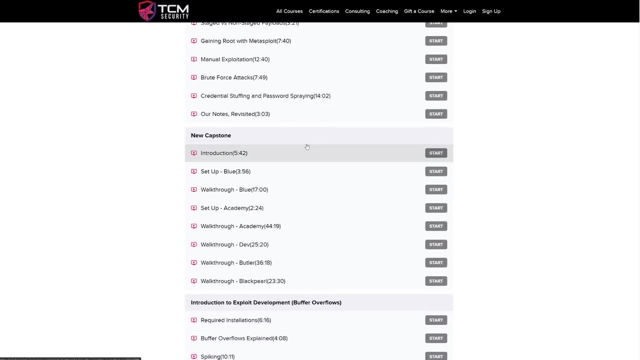 Once that has all been said and done, we're going to go ahead and move into a capstone. So we have four to five boxes- actually five boxes that we have built ourselves- and we're allowed to use them in a few different ways. So we're going to go ahead and start hacking it And 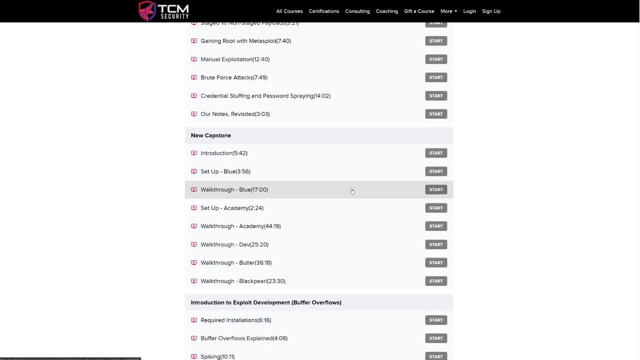 you to download those. you run through those and you try to attack those, And your goal is to hack into these machines. So you go through all these and that is your capstone, your end to your 12 hours of your course. Now, this is the only time I'm going to try to sell you. anything is going to. 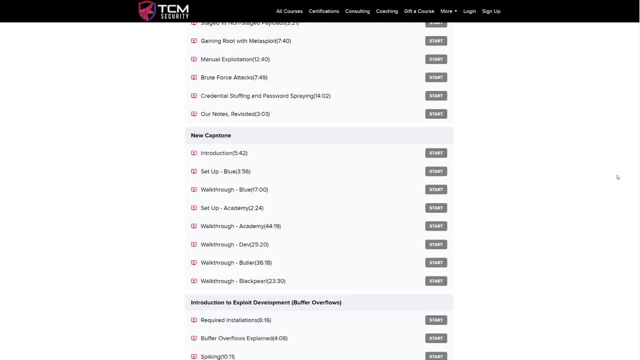 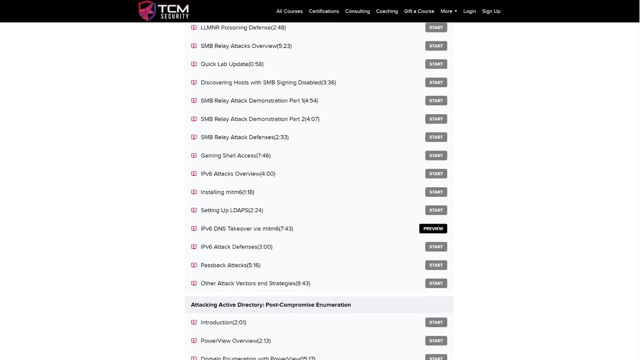 be the next 30 seconds to a minute If you are interested in continuing on with the course. it does cover exploit development, active directory, which is probably the coolest thing ever. It's my favorite thing to teach and how to hack into active directory, which you can see. 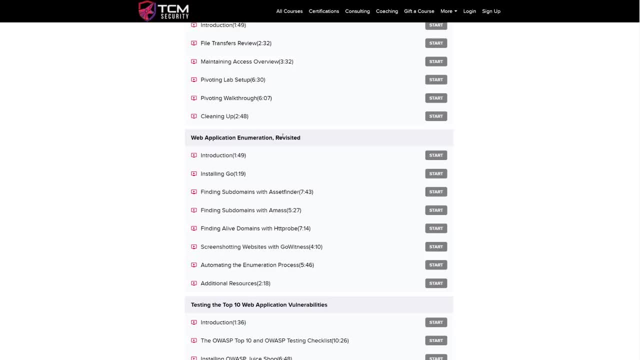 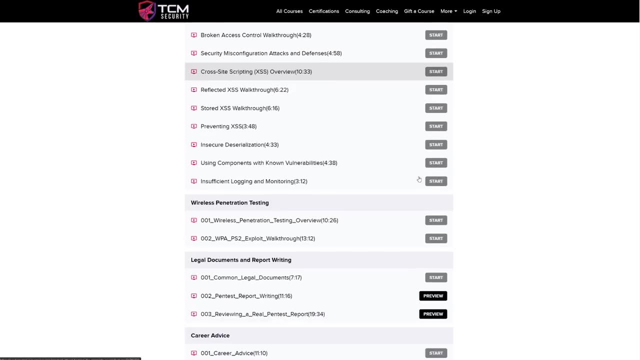 there's a lot of active directory attacks here. We go into post exploitation, we go into web application enumeration and the OWASP top 10 web application attacks. We do a little bit of wireless pen testing, legal documentation, report writing and career advice And we do sell all of. 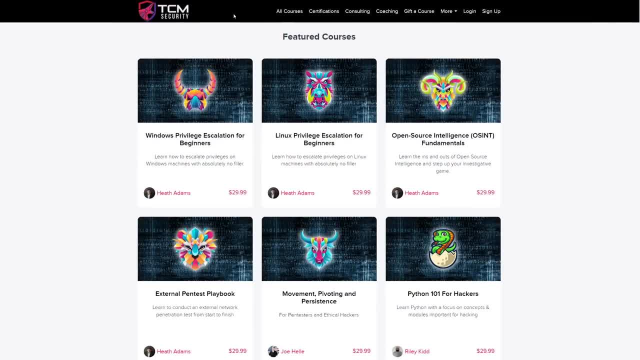 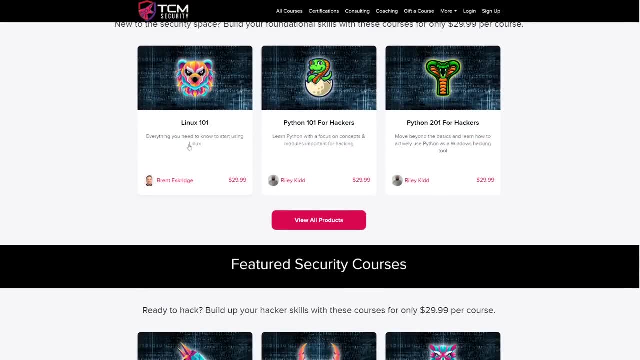 our courses for $30.. Full disclosure. we have about 12 courses at the time of this recording. If we go to the homepage, we could see all of our courses Here. So we've got everything from Linux and Python all the way down to open source. 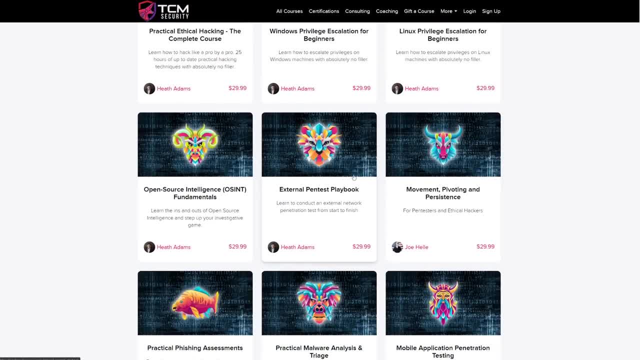 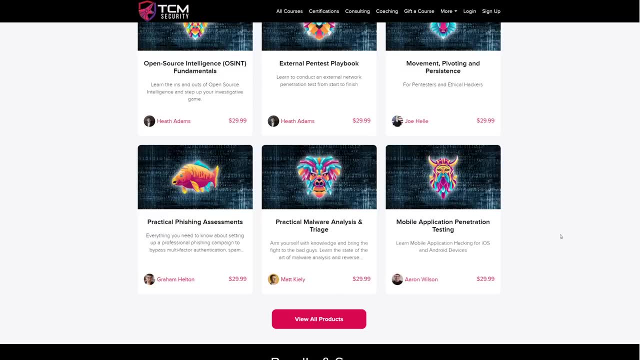 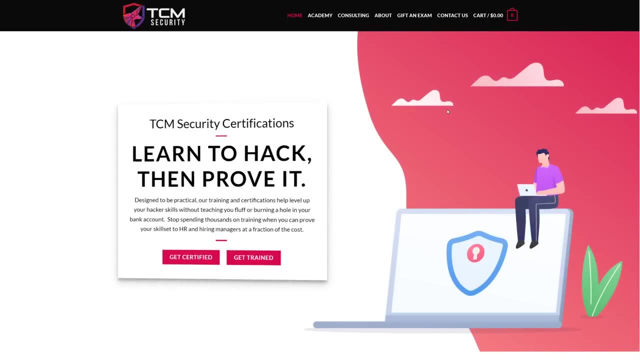 intelligence, different types of pen testing and advanced pen testing, mobile pen testing, malware analysis, phishing- everything is no more than $30.. And that is the only time I'm going to sell you on anything again. So, last but not least, we do have a certification side of. 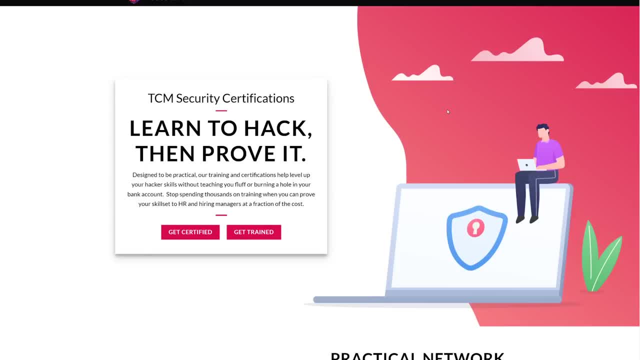 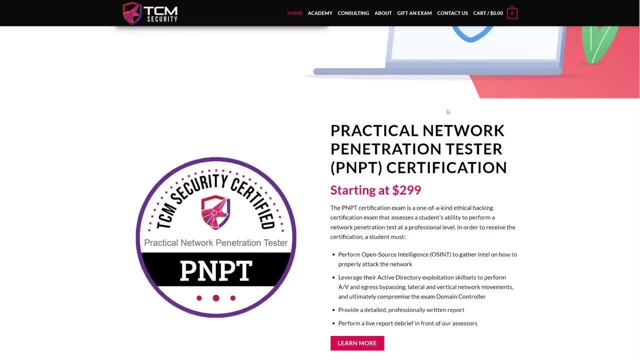 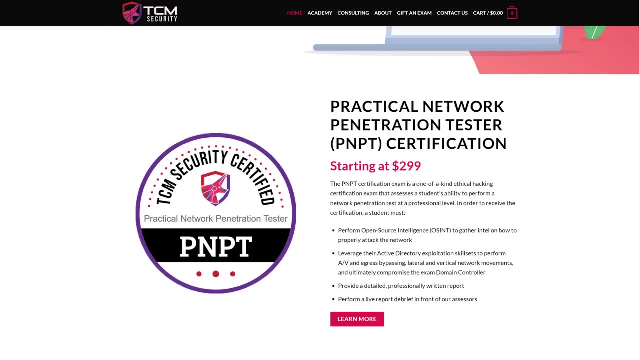 things. If you're interested in the certification this course, it leads to the network penetration tester certification. If you want to find out more about that and why that's cool and industry changing, feel free to go to certificationstcm-seccom. And with that being, 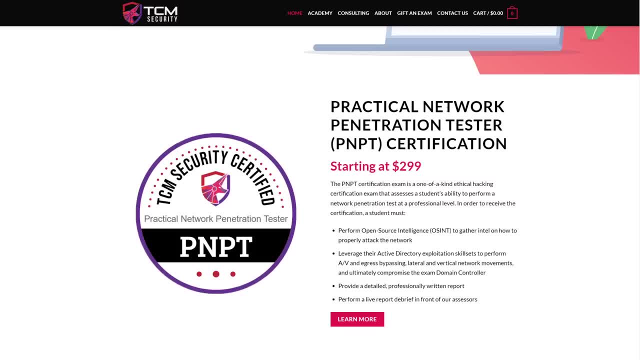 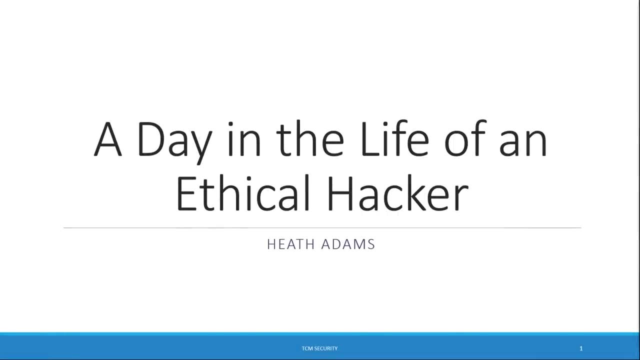 said: I am done pitching you, selling you anything for the rest of this time being. Let's get into 12 hours of free material and start covering how to become an ethical hacker. Let's go ahead and get this course started. I want to talk about a day in the life of an ethical hacker And I want to talk about why I 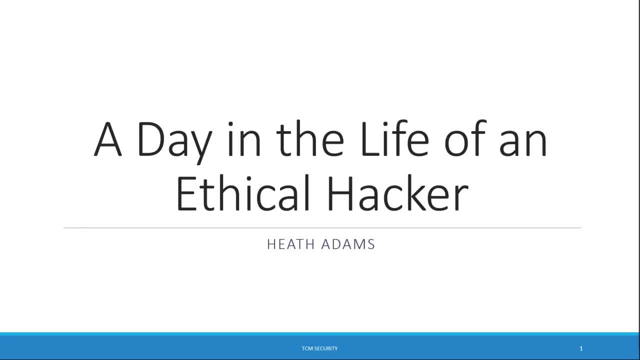 love ethical hacking or penetration testing, And what I do on a day to day basis, what kind of engagements you might find yourself in as an ethical hacker, and then the soft skills and technical skills I think that you should have in order to be successful in this field. So let's go. 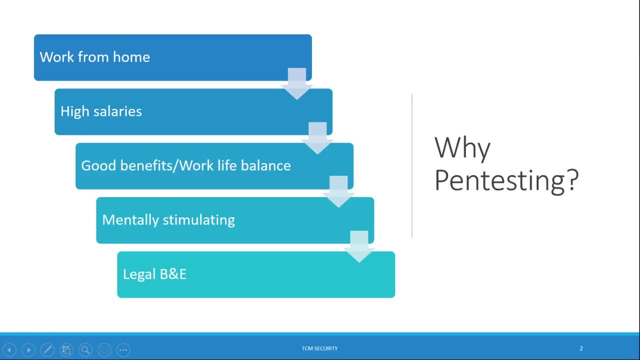 ahead and first look at why pen testing. So why pen testing? Why for me? Well, I work from home. I roll out of bed at like 755 in the morning. I'll get my coffee ready, I'll go to my desk, I'll make it there by eight And I am ready to go. I don't have to sit in traffic. I. 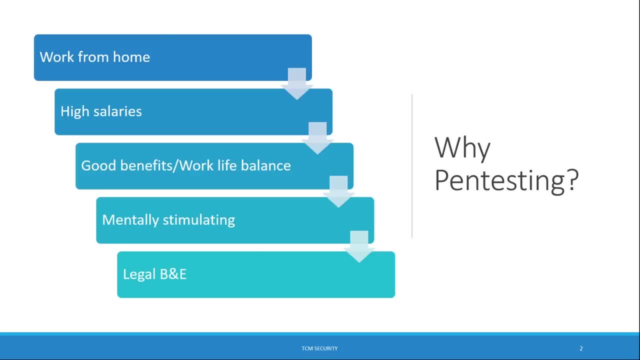 don't have to drive to work. I you know I save so much time out of my life just by working from home. It's a great luxury. I love the lifestyle. It's not for everybody, But a lot of penetration testing nowadays is working from home. And another great thing about pen testing: 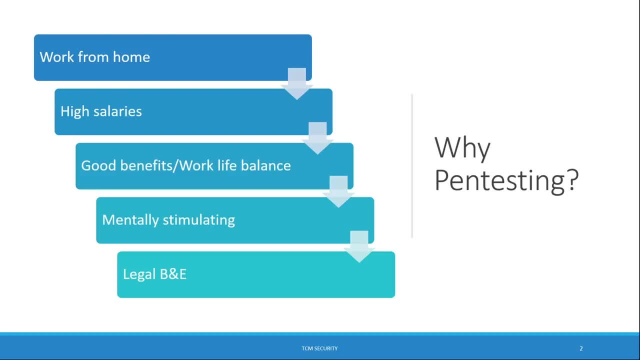 is the salaries are incredibly high. My first job in the field was over six figures, meaning over $100,000 in this field as a- you know- first year pen tester. So it's incredible money And it's very lucrative. moving up anywhere from a senior pen tester can make $150,000. a manager can make. 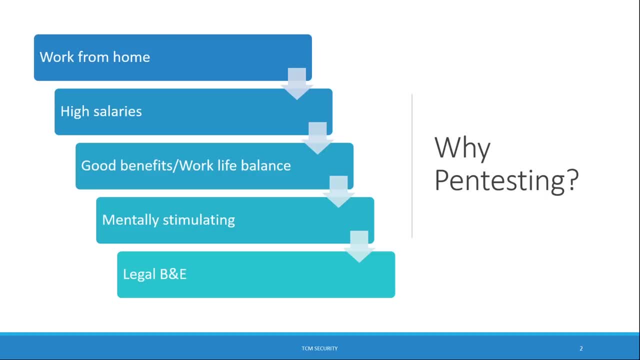 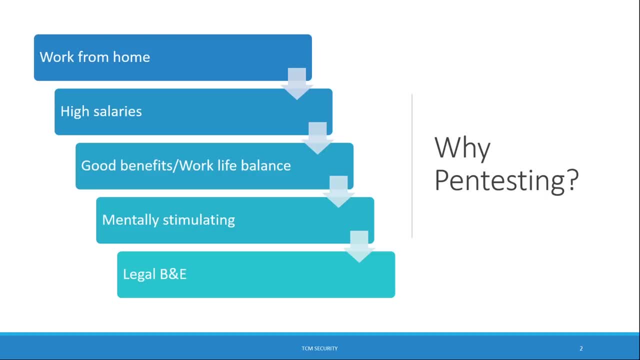 especially if you go out and you do your own business or your own consulting. The salaries are very, very high, because this is a very technical field And there there is a job shortage or people shortage. right now we need- we have- more jobs than we have- people, So that 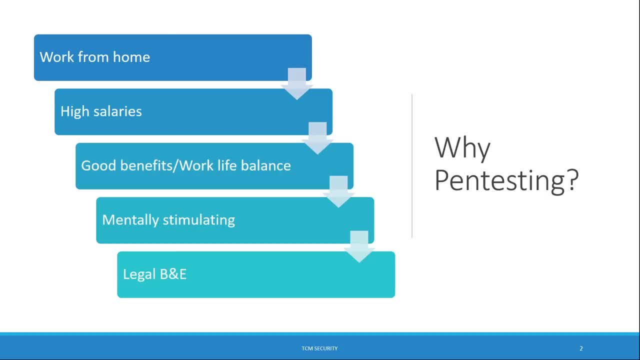 relates to high salaries as well. On top of that, the benefits are great. The work life balance is great. Again, this boils down to where you work. But for for me personally- you know I'm working 40 hour weeks- my benefits are have been fantastic through and through. 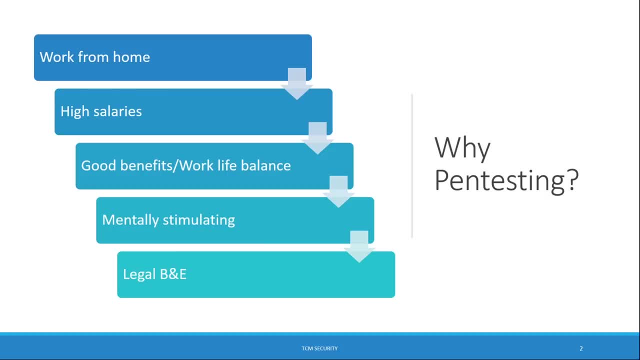 And I just, I love the lifestyle right, That work from home, that 40 hours a week. I was an accountant before I got into penetration testing And let me tell you, I was working 60 hour weeks, 70 hour weeks. I was in the office at all the time And I was, you know, I was going in when. 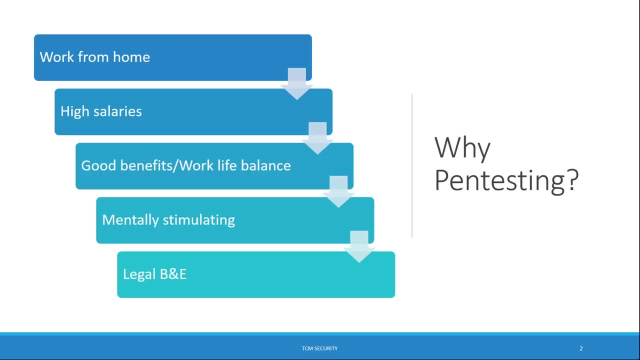 it was dark and I was coming home when it was dark And it just, you know, can easily lead to depression doing that. I've not experienced any of that in penetration testing And I'm really, really happy for it. So, on top of all this, it is mentally stimulating. This is one. 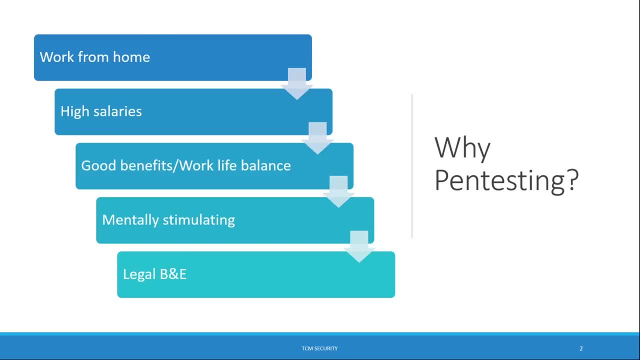 of the best fields. I am what I consider a lifelong learner. I like to learn, I'm nonstop learning right And I have that personality type And you're going to find that if you enjoy this field, it's never going to feel like work to you. I could sit here and I can pen test for 80 hours And it. 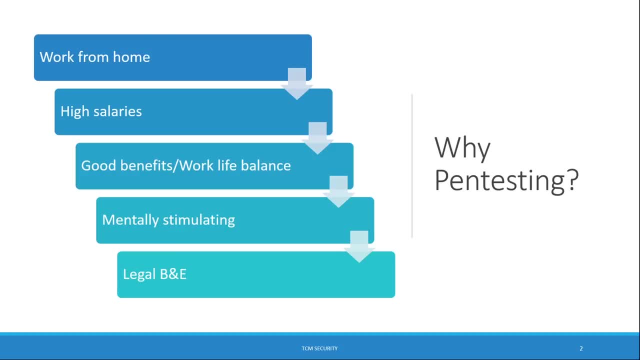 is just mentally stimulating. It's a puzzle. there's always something new to learn, there's always a new attack out And there's always a new defense out as well. So somebody is always trying to block your attacks, And it's this cat and mouse game. And if you do not stay up to date or on top, 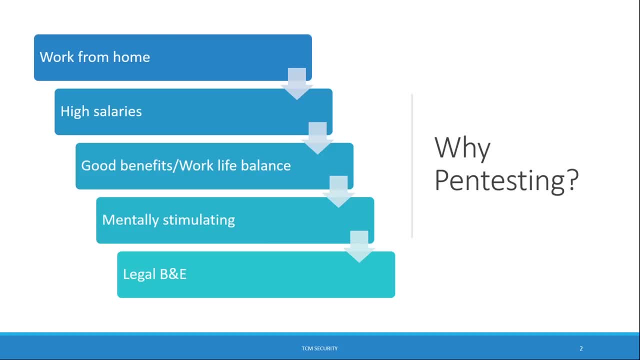 of things you're going to get left behind. So you have to have that mentality in this field, where you're always willing to learn and you like learning And that's really like for me. that's what I'm testing, because I enjoy that. And lastly, of course, it's legal breaking and entering who. 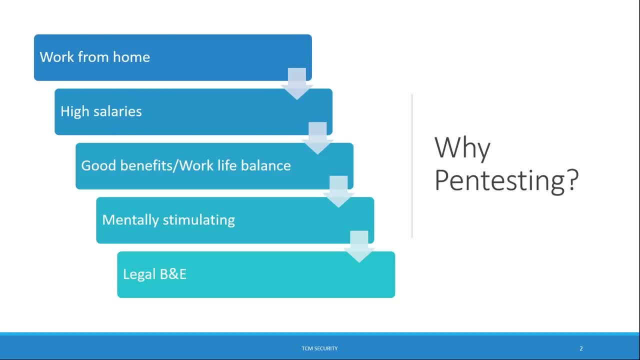 doesn't like that. I get to break into buildings, I get to break into websites, into networks, and people pay me to do it. I cannot believe that this is a job. when I first heard about it, I was like No way hackers. hackers are bad guys, right, But hackers can be good guys too, And we 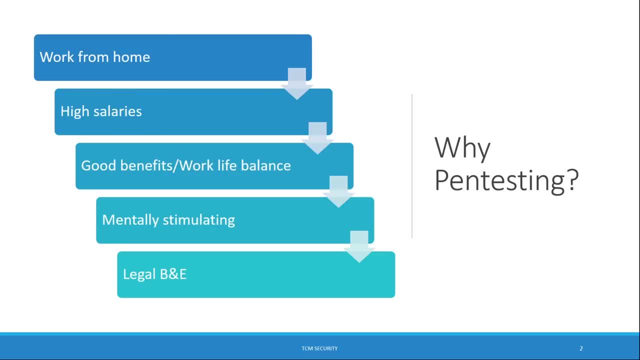 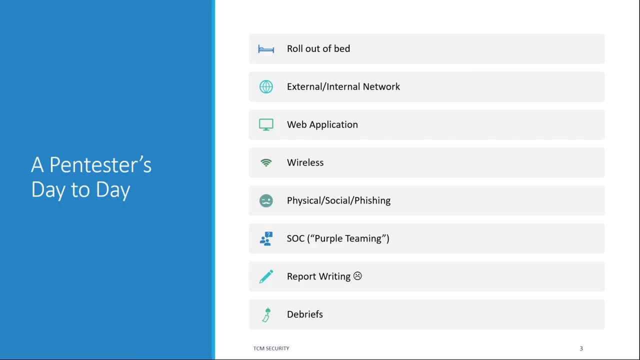 can get paid very lucrative salaries. So from here let's talk about a day to day lifestyle. Day to day here, What's guaranteed- most basically should be guaranteed- is that I roll out of bed. I'm still relatively young And I have several different types of assessments that I can do, And 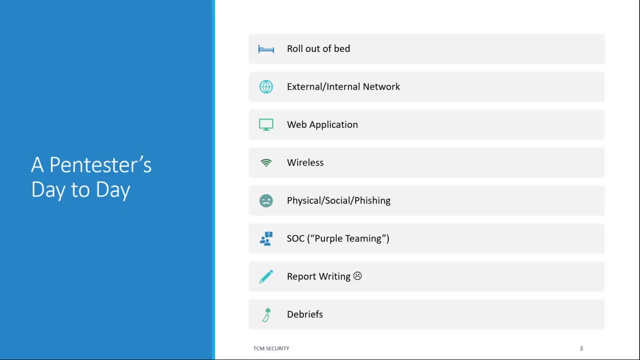 this really isn't all of them, But this is the ones that I do the most. Now I have what is an external or internal network assessment, And we're going to cover those quite a bit in this course. But when we're talking external network assessment, that means that I'm evaluating a network from the 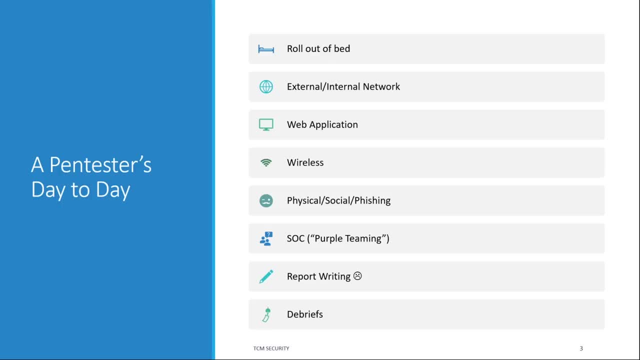 inside. I can be in China, I can be the United States, I can be in Russia. it doesn't matter where I'm attacking from right. I can be in any country at any time attacking this network. So I'm on the outside. looking in the internal is different. We assume at this point that we have 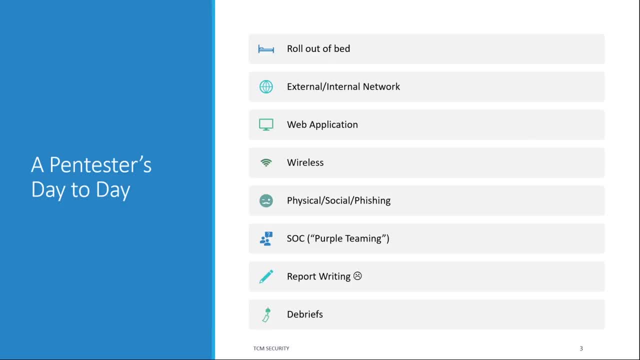 breached the network. we have a Dropbox, we've got some sort of code execution on their network. we logged into their VPN. it doesn't matter. somehow, some way we're on that network. What can we do once we're inside the network? And what that means is we're going to be talking a lot about active 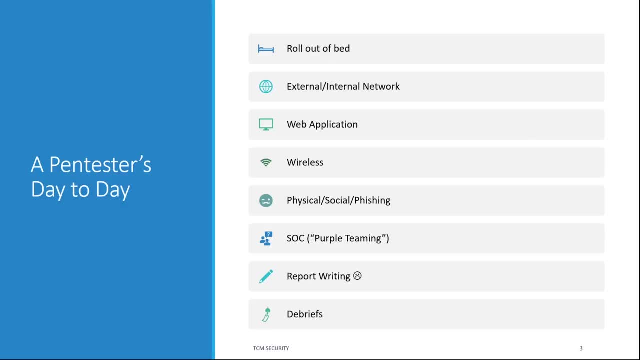 directory pen testing And that's really what it corresponds to, And this course is going to hit very, very heavy on active directory because of this And this. so you have two different types of network pen tests and they, the methodology is very similar. the attacks and tool sets are. 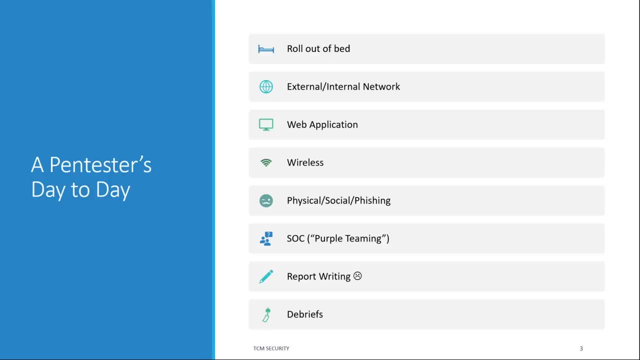 very different So they can almost be split apart into their own subsections. But you will have external pen tests, internal pen tests. on the network side You may be asked to do web application penetration testing. So that is assessing a website, right, you have a website or an application that is given to you And you want to see if you can. 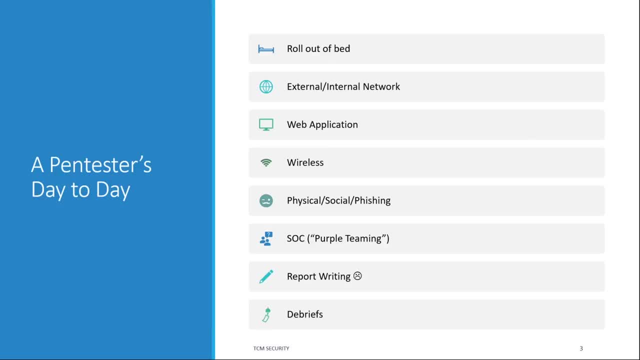 break that website if you can log in as an administrator or get somewhere that you you shouldn't be able to get to and you just want to evaluate the security posture of that website. So there are a lot of tools and methodologies out there for that And we're going to cover. 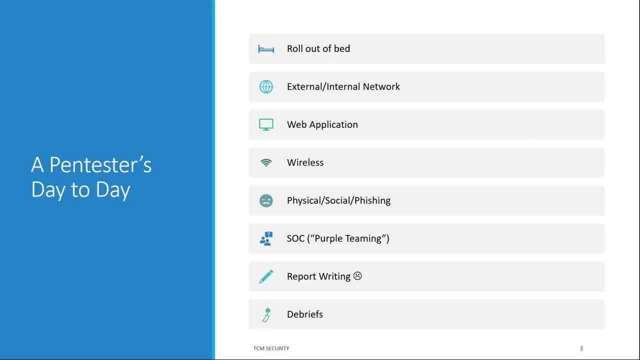 the OWASP top 10 in this course when we talk about that, which is big when it comes to testing web applications. So from there we also have what is called wireless penetration testing, That is, the evaluation of a wireless network. So we'll go on site, we'll try to hack into the. 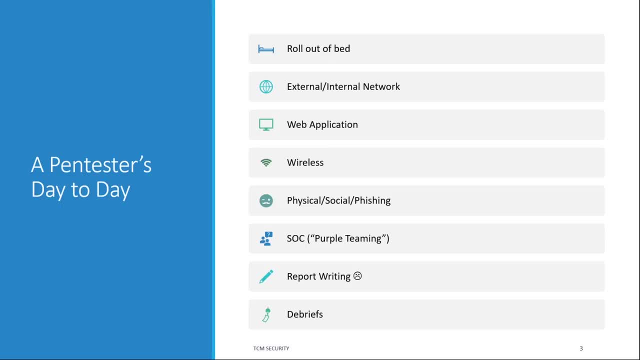 wireless. we'll look at the guest network and see if there's any segmentation or not. Should a guest be able to sign in and access the same network that somebody who is logged in as an employee should access? The answer is no, but it happens quite a bit. We'll also look for rogue devices and 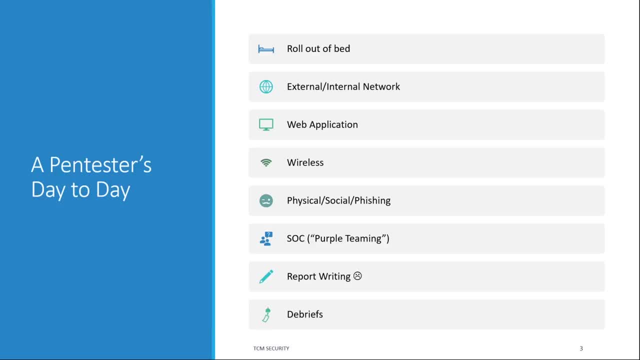 see, you know what might be out there that is interesting to us. We'll talk more about all these different assessments when we get into their respective sections. Now there's also what is called physical or social, or phishing. There are three different types, but they fall into social. 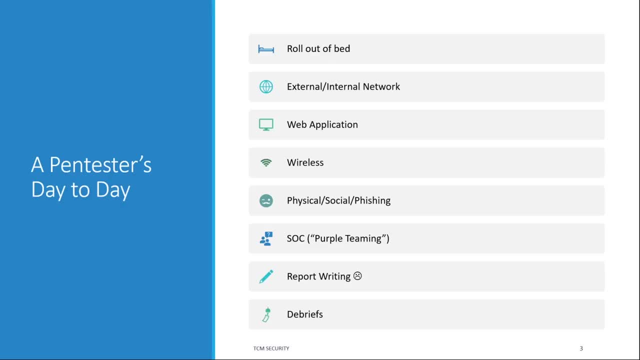 engineering. Now, physical assessment is where you go on site and you try to break into a building. you have a destination in mind. maybe it's a server closet, or you know some, some critical location, the building that they don't want you to get into. And then you can also look at the. 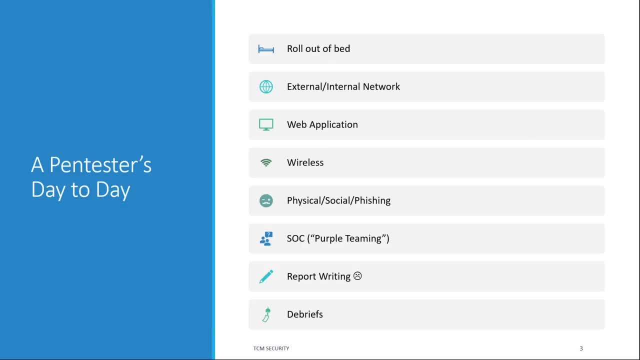 building that they don't want you to get into. This could involve picking locks, social engineering a lot of the time, cloning badges, you know, and just making your way into this building through whatever methodology you can. Now social engineering and phishing. 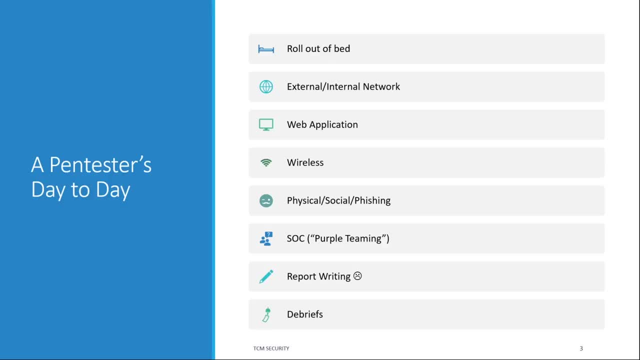 those are, you know, kind of hand in hand. you'll do a phishing campaign or social engineering campaign or even a vishing, where you're calling on the phone and you're trying to get information And you're just after. you know what kind of credentials can I get? Who clicks on my links? 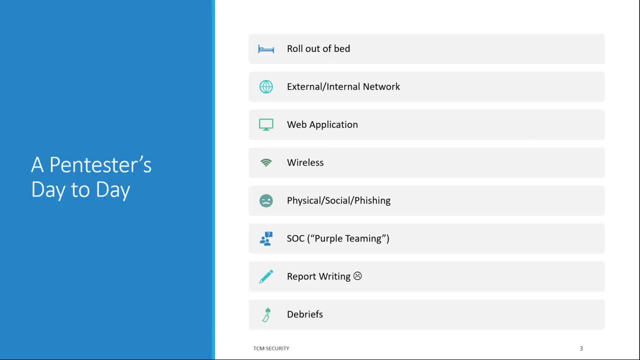 What kind of passwords do I get, etc. We also have what is called SoC assessment. So a SoC assessment is also known as purple teaming, And purple teaming is when you combine red and blue. So as a penetration tester or ethical hacker, you're often known as red. 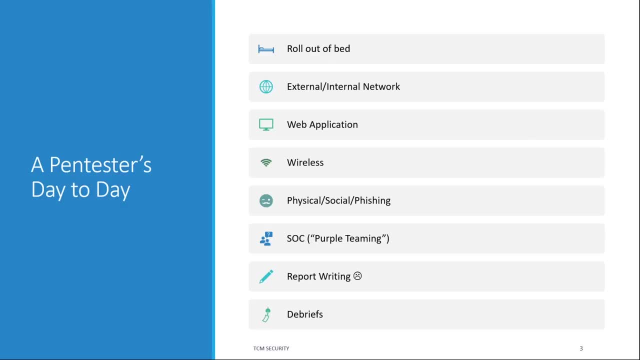 and a defender is often known as blue, So you combine those and that makes purple, And what that means is we'll sit down with a blue team as an offensive team will sit down with a blue team and we'll say: Hey, what attacks do you want us to try? 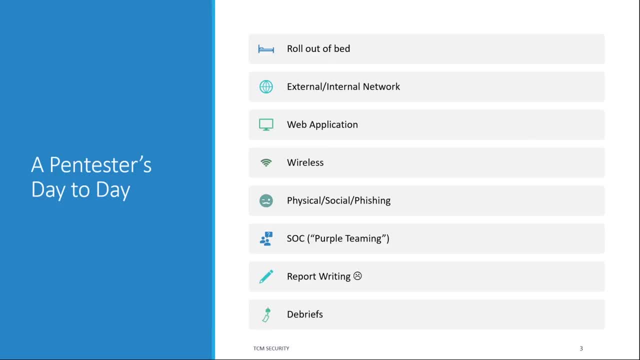 to run, Or we're going to run these attacks And I want to know if you pick it up So I might run a specific attack and see if the blue team detects it. I might go plug into their network and see if it prevents me from plugging into their network. Do they get an alert on that? If not, how can we? 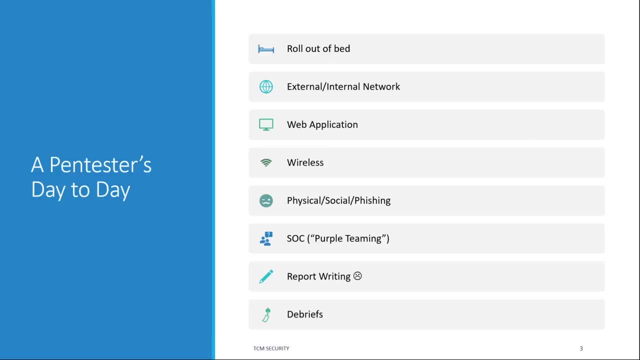 help them baseline this attack, to get this alert. So I think purple teaming assessments are some of the best assessments that are out there, Because not only do they learn from you and what attacks are out there, but you learn from them on how to defend against these and how to bypass these two. 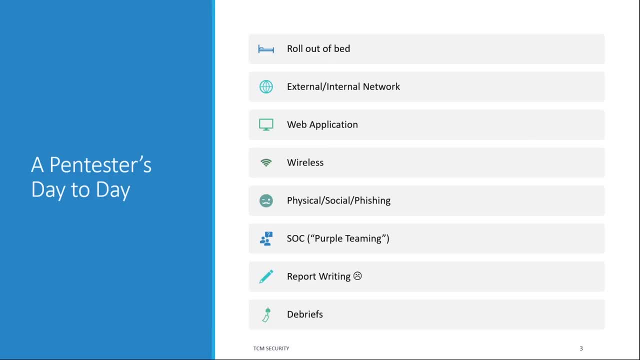 because maybe your first attempt does get blocked And you're like, Hey, maybe I should, you know, run a different attack and see if you catch that. And it's a great way to have that cat and mouse game again. So once we do these types of assessments, we have to write a report, we have to 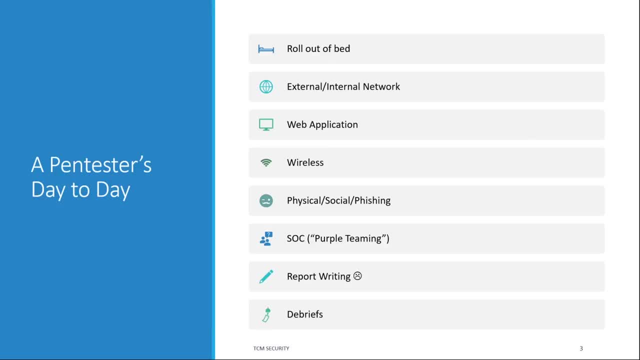 report back on what we saw and tell the client about- And I put a little sad face there because you know not everybody likes writing reports, but it is absolutely part of the job. you have to be well written in this field to be successful. 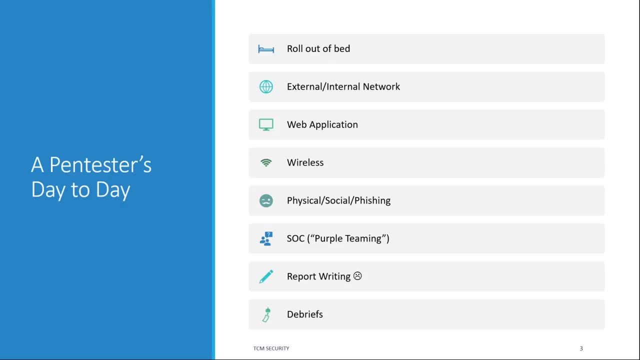 So you know you write this report and you're going to have to present this report to a client, And that's what is the debrief. Now, debrief is where you take the report and you give it to a client and you walk through it with the client and say: here's what's wrong, Here's why it's wrong. 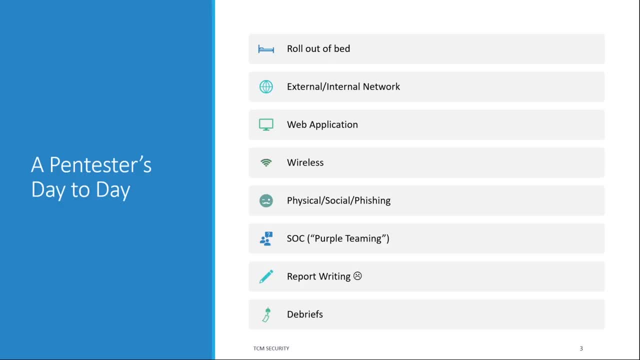 And here's how we can fix that for you. Or here's how you can fix that for you, Right? And so you have to have this technical skill set as a penetration tester, And you have to have this well written skill set. you have to be able to write well. you also have to be able to talk in. 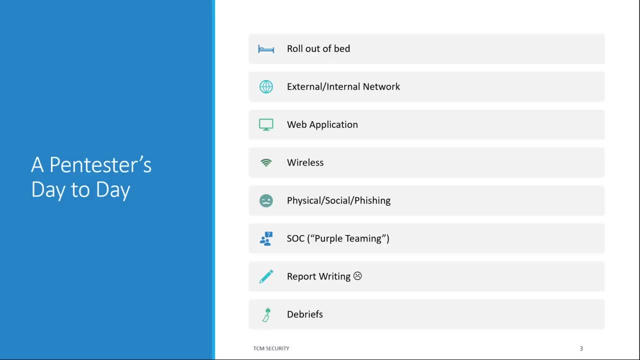 front of people, when it comes to doing debriefs and talk to people. That doesn't mean you have to be an extrovert by any means. you can be an introvert- I am very introverted- But you have to be able to put that personality on when you're on site. Same thing with the physicals, by the way. 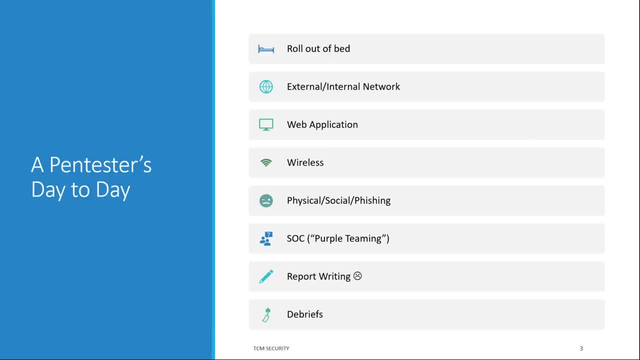 if you're on site for a physical, you do not have to be an introvert, You have to be an introvert, have to be an extrovert to be successful. I know plenty of good physical pen testers that are actually introverts and do just fine, as long as you're able to get into that mindset for that. 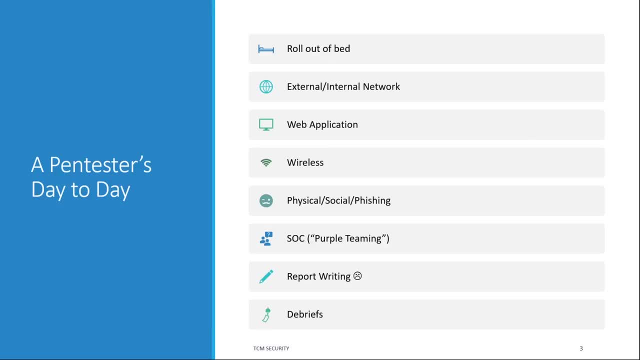 temporary time period. So, anywhere from all these different assessments that you could end up doing at any given time, you'd be well rounded there. you're going to be writing reports and you're going to be presenting reports to clients. Now let's talk about the technical skills that you 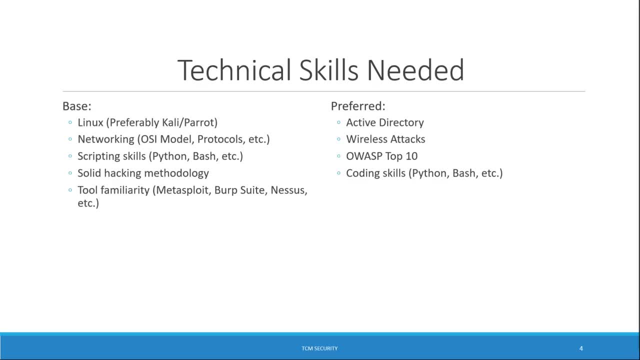 are going to need And our course here is going to cover the technical skills that you are going to cover a lot of these. So at a base level you really do need to know Linux, preferably Kali Linux or what another type was called parrot. There is networking that you should know, you should be. 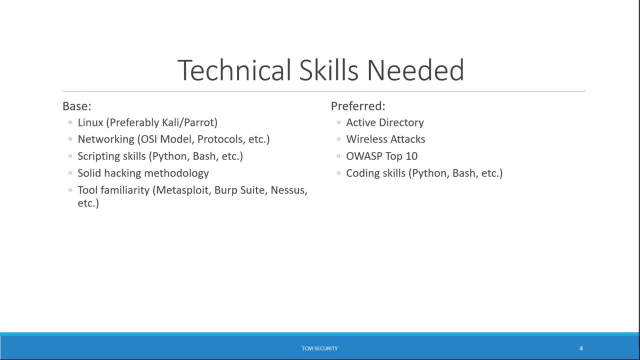 familiar with the OSI model, certain protocols like TCP, UDP, HTTP, etc. You should have good scripting skills, whether it be Python scripting or bash scripting, etc. There and you should have a solid hacking methodology, And this is going to cover a lot of these. So, at a base level, you really 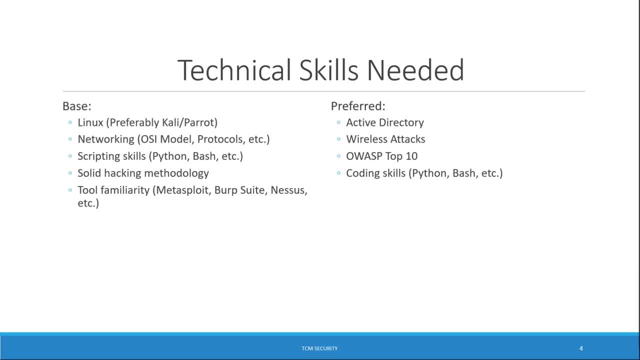 This is all what you'd want as a base for an interview. you should have also tool familiarity: right meta supply, burp, suite Ness's. If all this sounds like a foreign language to you, that's fine. Come back and watch this video again once you've gone through the whole course. 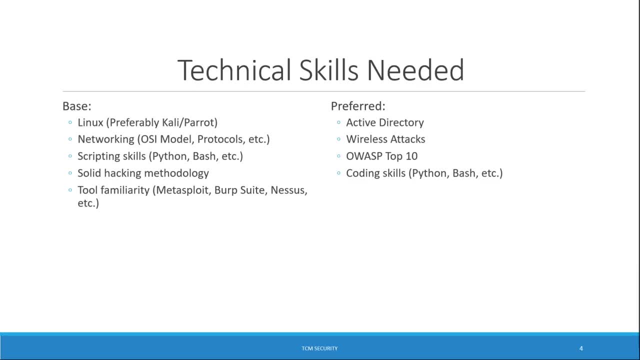 and it's going to all click for you And you're going to say, Hey, I know a lot of this And on the preferred side, Active Directory is huge. If you know Active Directory, you're going to be ahead of the game. Most people when I interviewed them, they have a good base, but 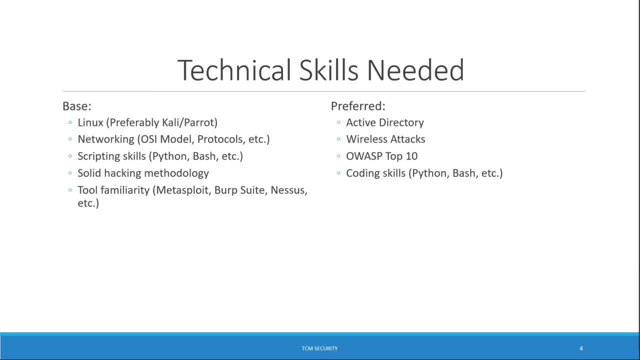 that good preferred side And we like, we like the preferred column a lot. Okay, So active directory: super important wireless attacks, important to know, the OWASP top 10.. Also important to know that is related to web application penetration testing And, lastly, coding skills, So scripting. 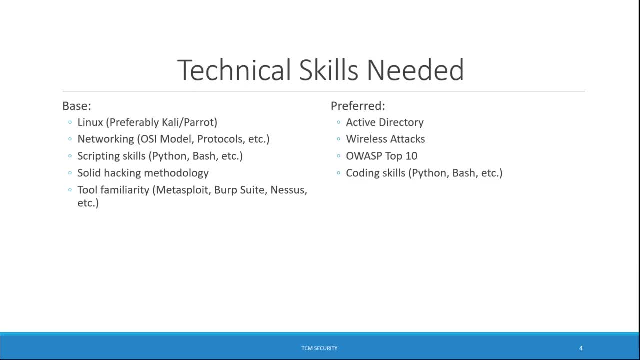 and coding a little bit different. scripting is what you'll be using, primarily coding. you don't have to be a coder to be successful in this field at all. By the way, if you only script for the rest of your life in this field, you'll still find plenty of success. However, you can code. 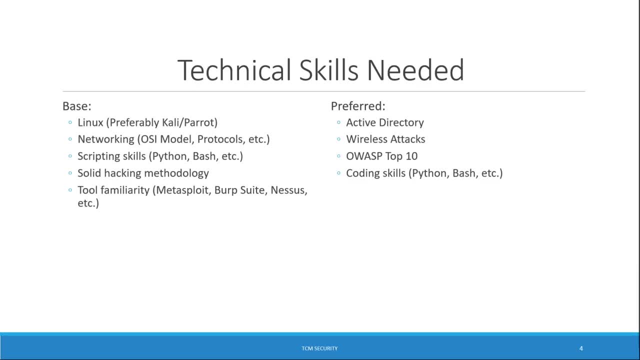 new tools, things you know contribute to the community with it. We'll talk about that here in a second as well, But just know that the base is possibly potentially can get you into a job to prefer. it will definitely get you into a job if you have strong knowledge on that side. 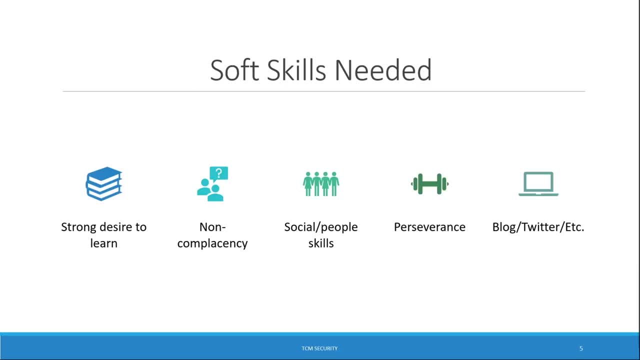 along with the base knowledge. Lastly, something that is not covered much is the soft skills area, And that is the soft skills area, And that is the soft skills area, And that is the soft skills that you need to be a pen tester. So, yeah, it's great to be technical And we already talked about 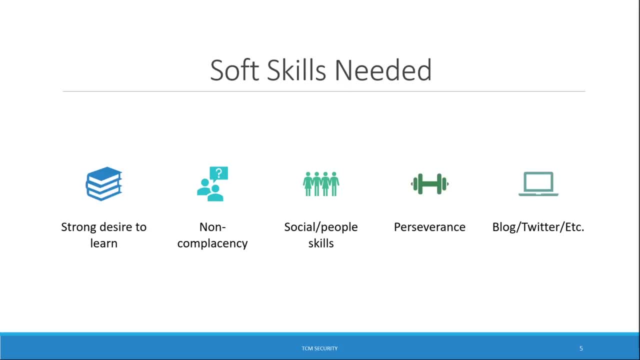 the, the social people skills- right, Because you're going to be doing that debriefing, you might be doing social engineering, etc. And you're gonna have to have that well written ability to you as well. But let's talk about some of these other ones. You need a strong desire to learn, you. 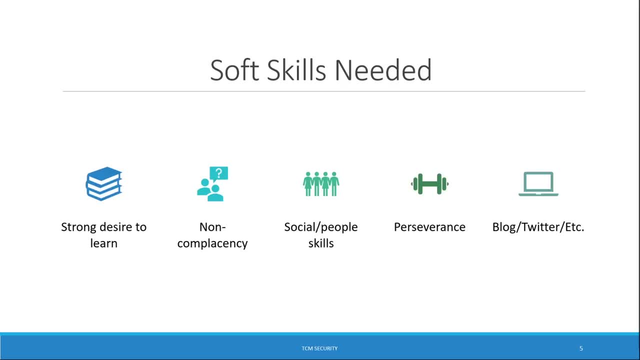 should be the type of person or that personality type that always wants to learn, and we talked about it right where you should be: the guy or girl that wants to go home and study and you find this fascinating and you that desire to learn is going to benefit you because of that. 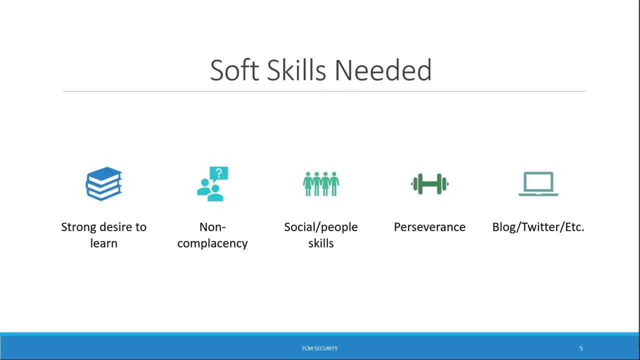 cat and mouse game because you know something that you knew yesterday might not be an exploit today. You know patches are coming out all the time and you have to stay ahead of the game because of this cat mouse game. So that strong desire to learn, super important if you do not stick up with. 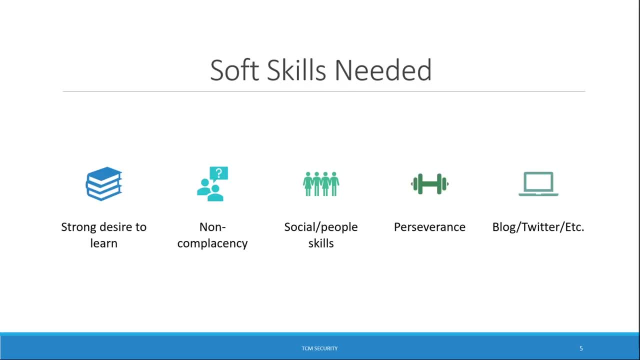 your studies, you're going to get left behind. And most people have this desire to be in the field of ethical hacking because they think it's sexy, It sounds cool and is cool. But if you do not have that desire to learn, you do not have that that perseverance which we're going to talk about. 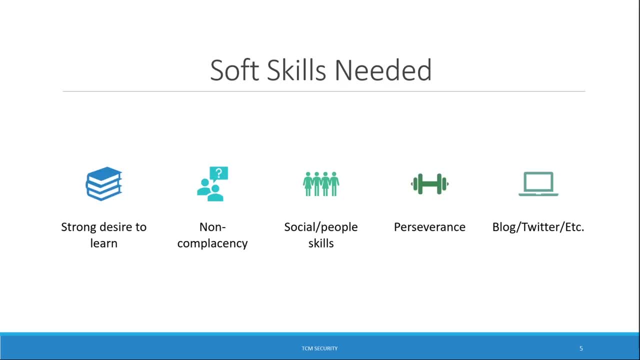 you're going to get left behind in this field and you're not going to be successful. So let's move over to perseverance. You have to have this perseverance mindset, not with just that desire to learn, but also that ability to not give up, because the answer is not always there in front. 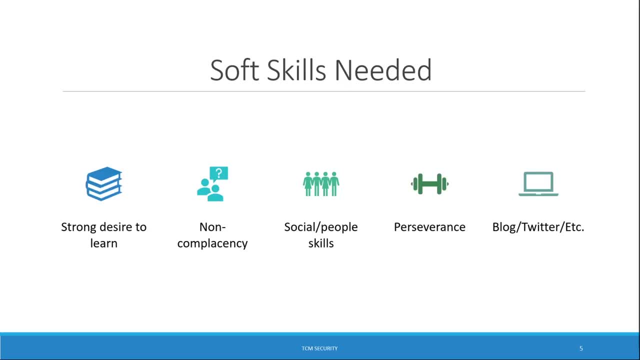 of you And you're going to see this as we go through the course. It's not cut and dry, It's not. Hey, I scan for this. I see an exploit, I go, exploit it. you might have to do a. 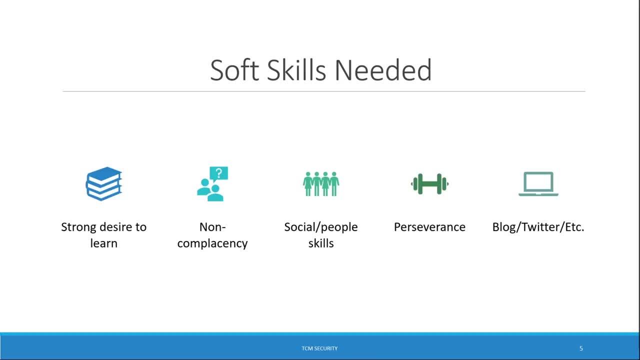 lot of research. it might look like the machine that you're attacking. it has no exploits available to it And you have to be able to put in that persistence To be able to persevere. you have to have that mindset where I'm not going to give up. I'm going to keep trying at this until I have. 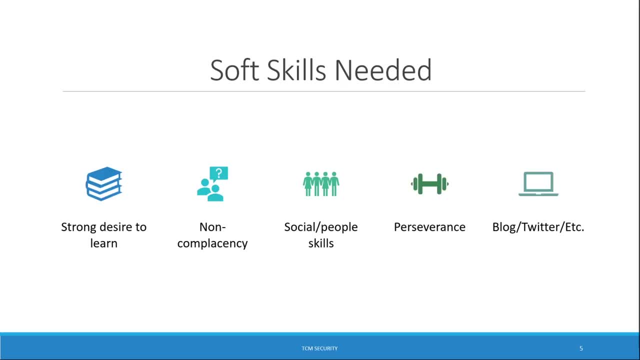 exhausted all my potential resources. That is what makes a good hacker. Okay, that that mindset of I'm not going to quit really makes a good hacker. Okay, that mindset of I'm not going to quit really makes a good hacker. Okay, that that mindset of I'm not going to quit really makes a good hacker. Okay. 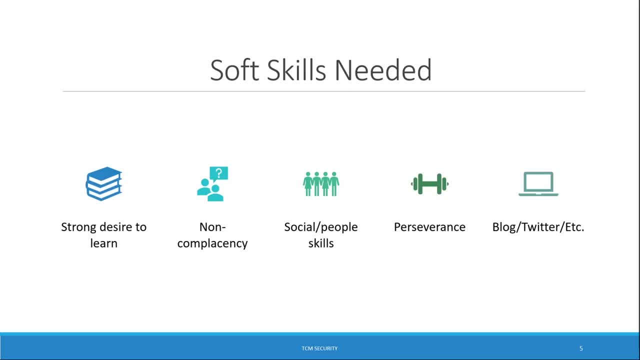 makes a good hacker. Now, on top of that non complacency, this kind of falls into that strong desire to learn. Now I've had co workers that are completely happy. when I was working help desk, when I was working in networking, plenty of co workers who are happy with their. 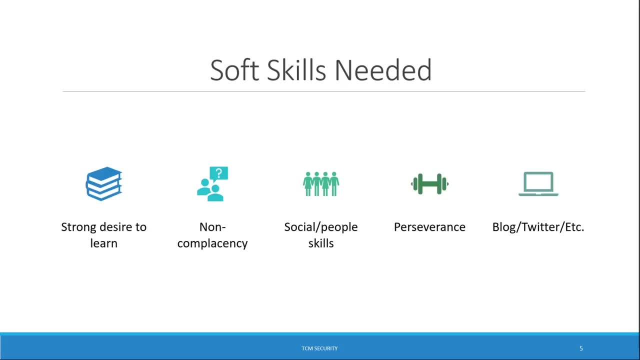 jobs. they've been in the same position for five years, 10 years. you cannot be that person. If you want to be a pen tester, you always want to learn more, you always want to move up, you want to, you want the most out of yourself. okay, Don't be. 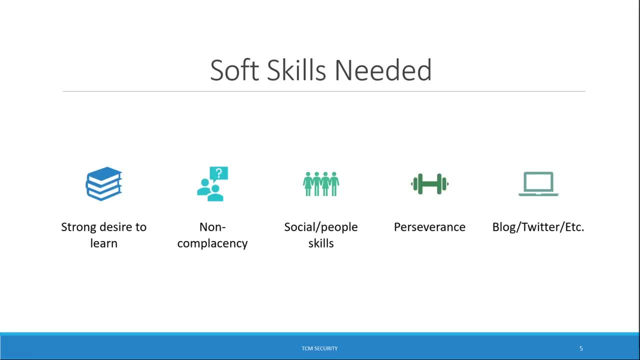 complacent. If you're complacent, you're going to get left behind. Just, I'm beating the dead horse here, But it really is true that you're going to get left behind if you're not constantly studying And if you stay complacent. Lastly, you should have a blog or Twitter or GitHub or something. 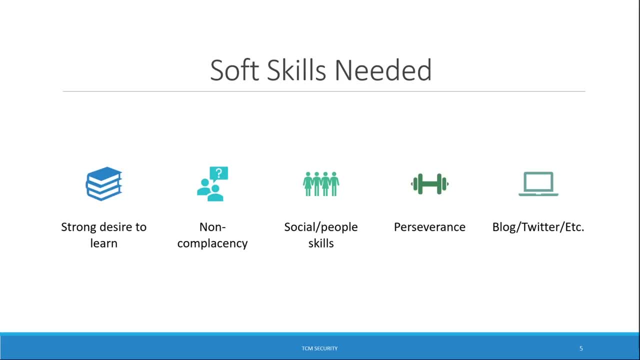 that you contribute back to the community with. it could be a YouTube channel or Twitch stream or however you want to do it right. You should give back to the community when I see that somebody's giving back to the community on their resume- Even if it's a blog post or Twitter, whatever it really helps And things that you're going to get. 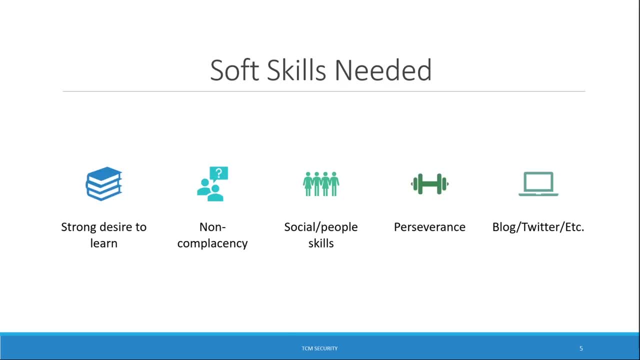 asked an interview, include where you get your news from, or and how do you, you know? do you have a blog? you're going to be asked that you know, and Twitter is a great place to get get news, And a blog is a great place to give back And Twitter is a great place to give back to. So make sure. 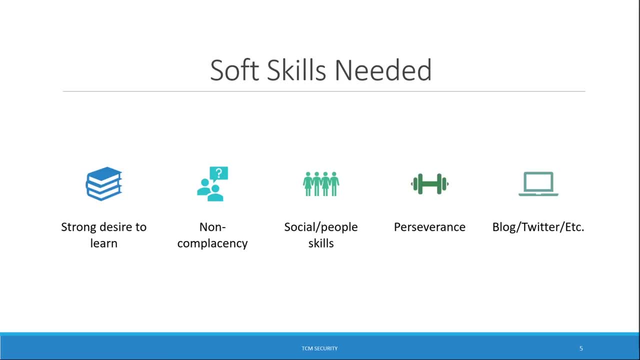 you're contributing to your community. it'll really help you in the long run And you don't have to reinvent the wheel. it could be a blog that somebody's posted before, or 20 people have posted before. as long as you're posting it in your, it helps you learn and it helps. 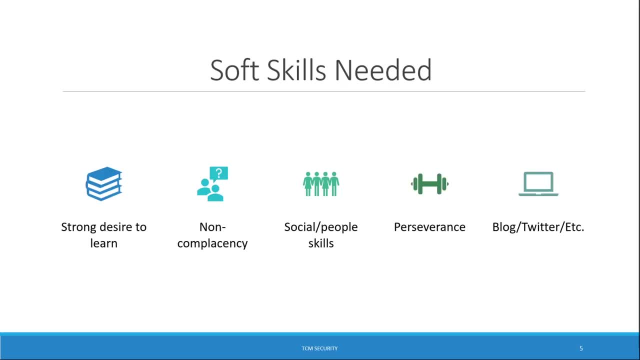 your style might be something that helps somebody else learn as well, compared to the other blog posts where maybe people didn't like that writing style or they didn't like that you know commentary or however it is, So you never know how your content is going to help somebody else. 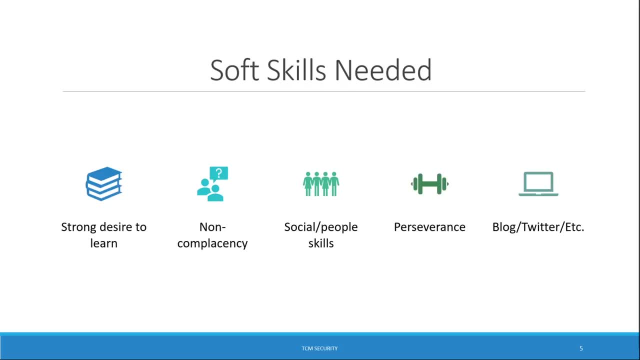 So I always encourage people to go out there and make their own content. So that's it, And I know this is a long video. this is going to be longer than most of the videos, but I want to make sure that you guys have a great day And I'll see you guys in the next video. Bye for now. 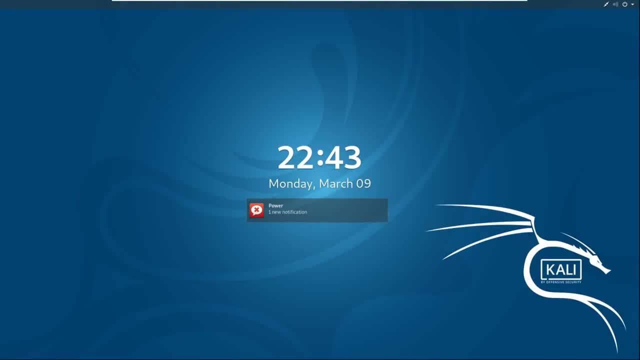 So, before we begin in this course and we really start to dive in, it's important to cover one of the topics that I'm going to harp on the most, which is effective note keeping. If you're going to be successful in your career, and you're going to be successful in this course, you really need 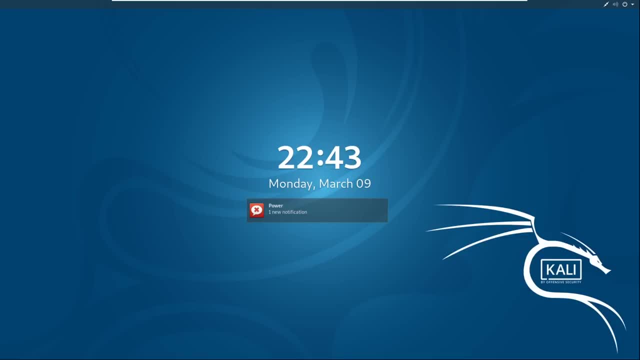 to take good notes. Now, in this first video I'm going to show you what my notebook kind of looks like- not only for my personal notebook, but as a notebook for an assessment, and how I might take notes for an assessment, And then I'll also show you some note keeping applications that I prefer, or 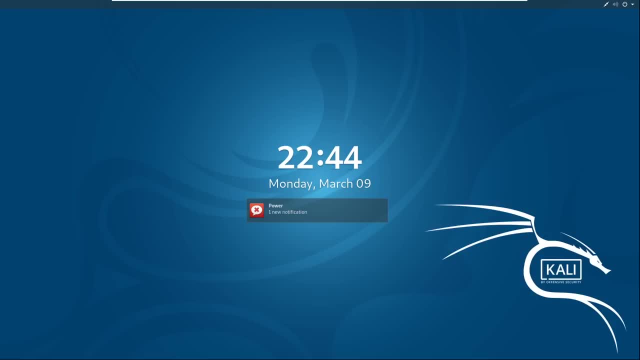 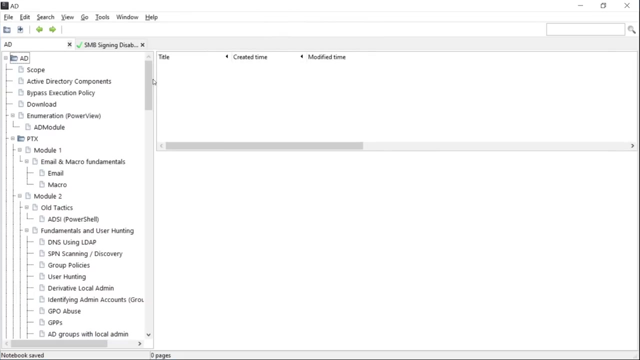 I've heard students prefer. In the second video we're going to cover how to install one of the applications and another cool application used for taking screenshots. So let's take a look at my notebook first. So here is my notebook And actually let's click over here. So this is my 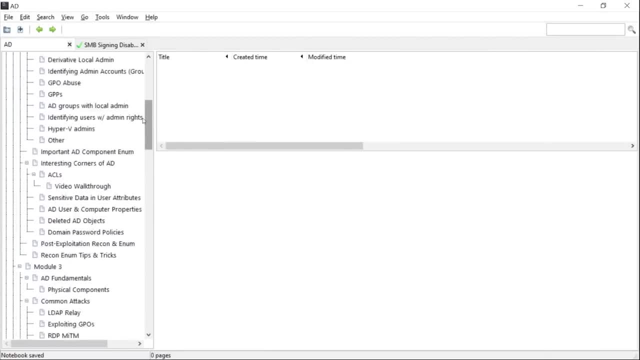 notebook And you can see it's really long. it's got all kinds of stuff in here And it's just something that I build upon. This one in particular is actually only geared towards Active Directory. So I have a few different notebooks. this one is Active Directory And it's actually a few different courses that I've taken in. 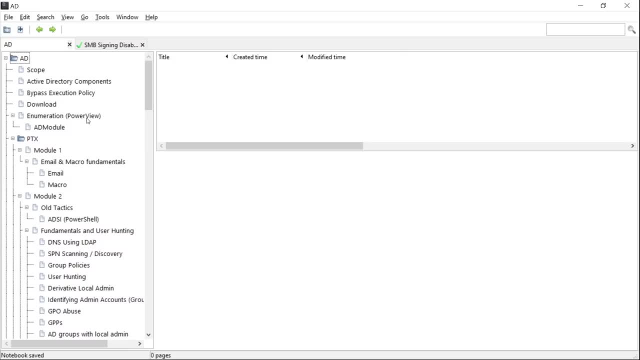 the past that I've kind of put together And then just for assessment work etc. I just kind of have a little cheat sheet here. So I wanted to show you this one in particular, because these were built off of courses and you're going to be working through a course, So kind of just get an idea of 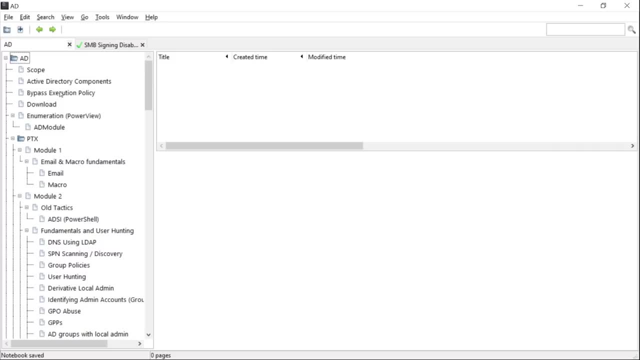 how maybe to structure it. So here you can see I structured it. So we've got different modules here where, okay, module one might have had this email macro fundamentals. module two, two here has all these different components to them, right, And we have 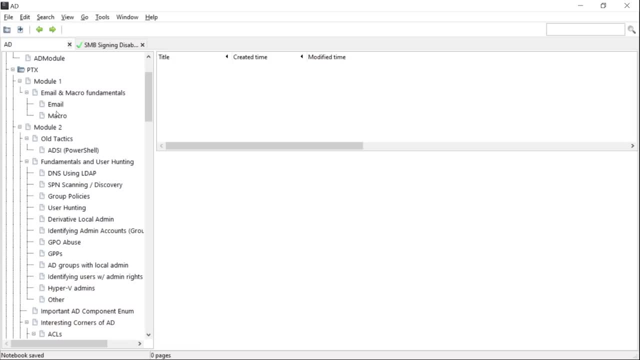 we have other notes, then we have child notes and even sub children to those child notes, And I'll show you how to create that here in a second. But let's say, for example, enumeration, which is one of the most important things that you're going to cover in hacking, And we take a look at enumeration. 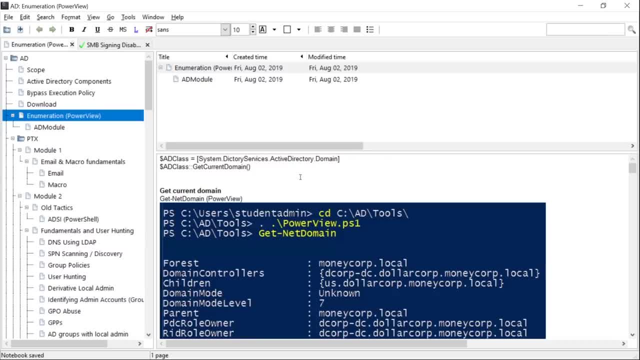 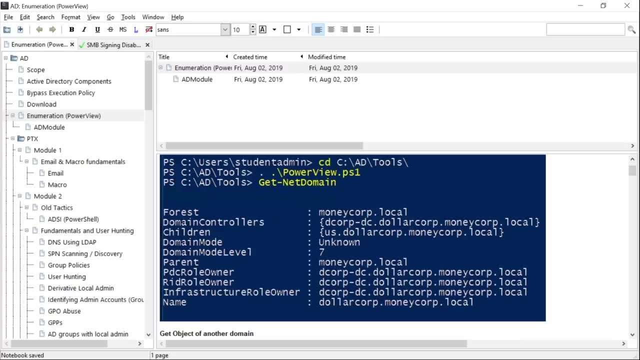 you don't have to understand what any of this means. here You could see if I want to look at a domain and I want to get the current domain that I'm on. here's the command I run And here is a picture of what it looks like And here's what comes back. 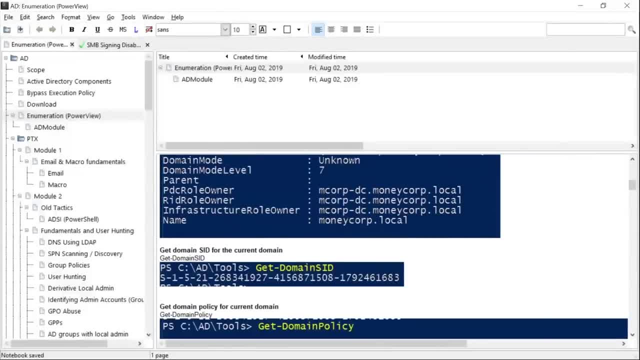 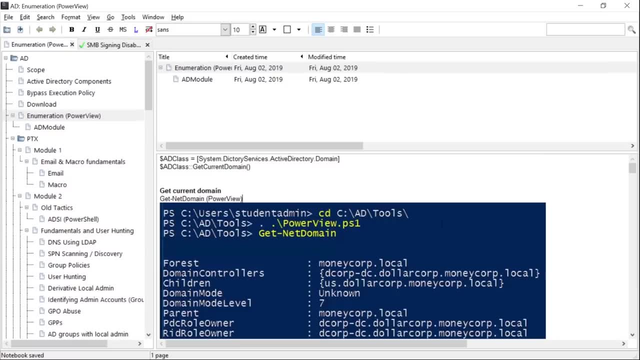 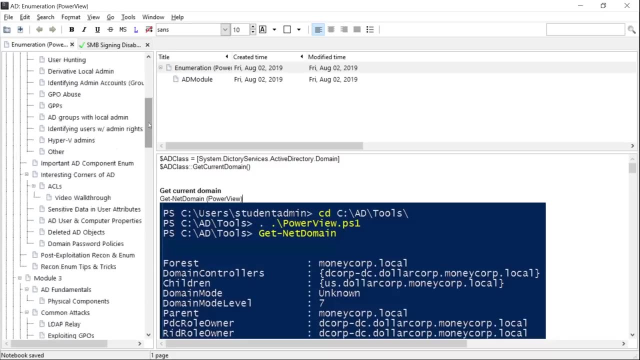 when you run that command. That's great. That's what I want to see, And I have a whole list of commands for all these in here, right? So if I'm confused on a assessment and I want to go and find a command that I'm not sure of, I can go to my little cheat sheet here. Now again, this is: 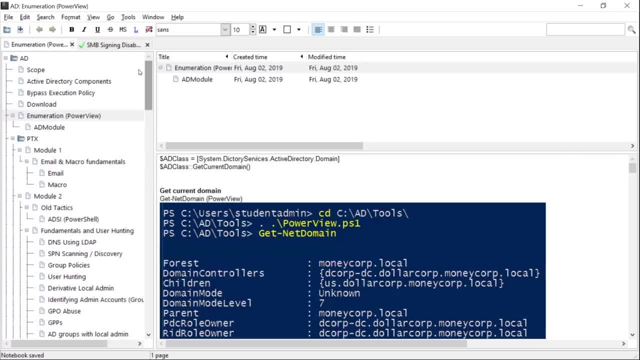 really long. You have to create your notes the way it really helps you for a course. I think it's good to write it all out step by step, like this, and then go back and make a cheat sheet. I don't need this pictures anymore. I've been doing this for a while, So maybe I just say, Hey, get. current domain is. 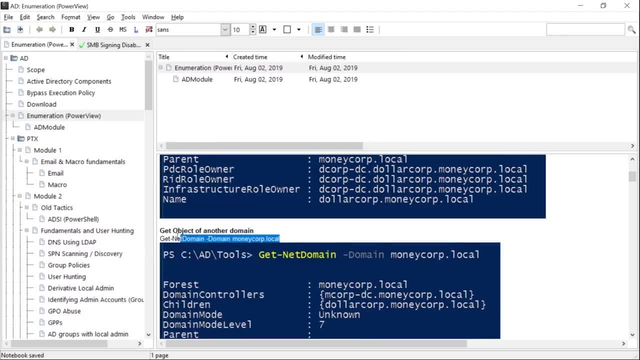 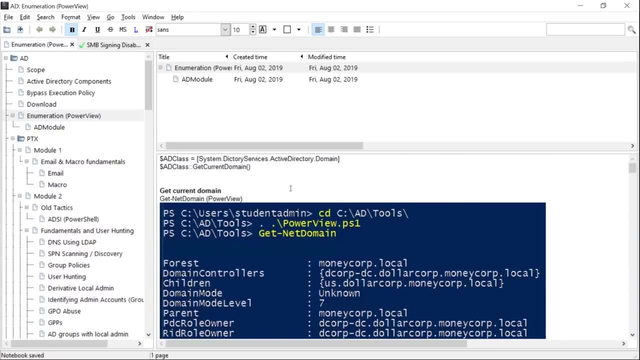 getting that domain And then I say, Hey, okay, get object of another domain. Here's an example of it. I don't need the pictures because it makes it really long, But as an example, and over time you learn with the pictures as well, at least I do. 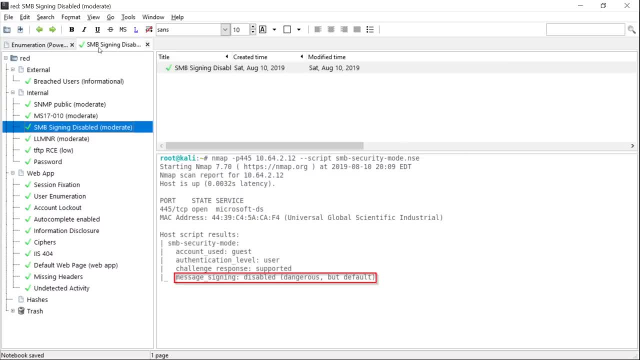 So let's build from that. Here is an example of an actual assessment that I did for a client, And you can see how I did this. Now I did an external, internal and web application assessment for this client And these were the findings. Now I'm only going to show you what is, master obfuscated. 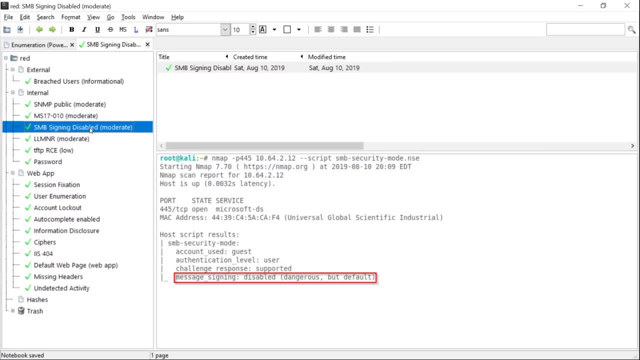 already or doesn't reveal client information. But as you can see here, one example is on the internal. they had something called SMB signing disabled. you don't need to worry about it. But here in my picture I've got a nice picture. The picture has highlighted. it says Hey message. 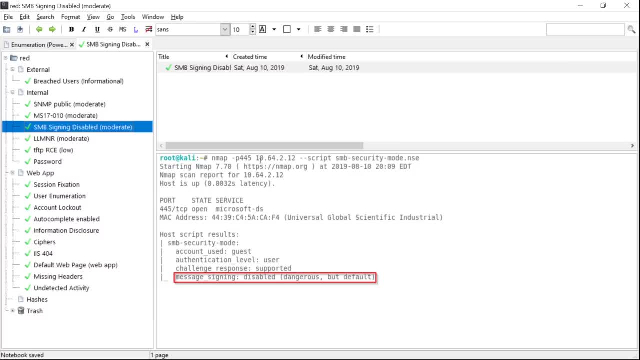 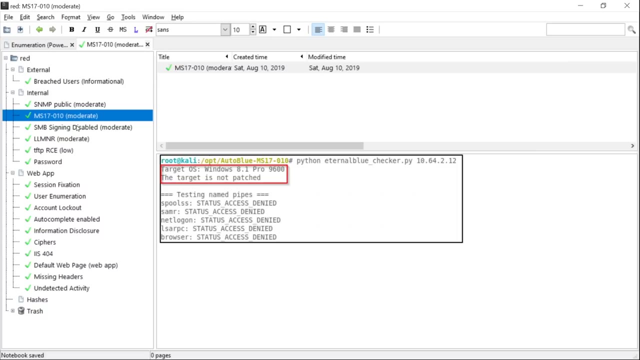 signing disabled. that signifies SMB signings disabled And it has the IP address. So we identified the machine And we give proof of concept that this SMB signing is disabled here. Another example, ms 17010.. These are both internal exploits that you're going to encounter in this. 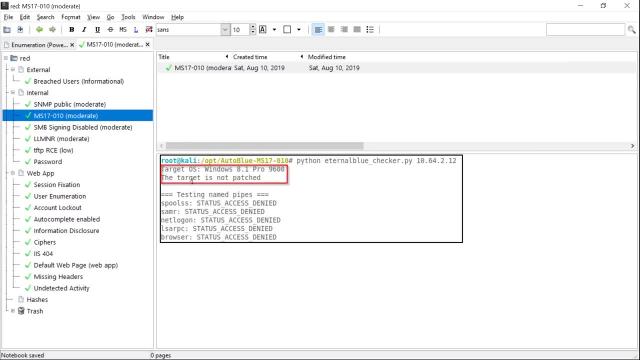 course. Here's one. I checked this machine. it says, Hey, this targets not patched. Now, this is one I didn't exploit, But it shows that it's actually vulnerable to this attack. So these are a couple screenshots that I'll put Now. your notes could be different than mine. How I organize is I take. 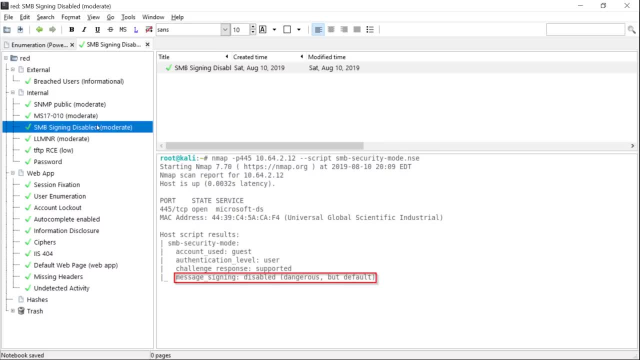 a screenshot, I put it in here and then I make sure that I have at least the IP address and the screenshot for reference, because I'll remember it. But if you need to go in here and take detailed notes, that's absolutely fine as well. You always want good notes for your assessments because you 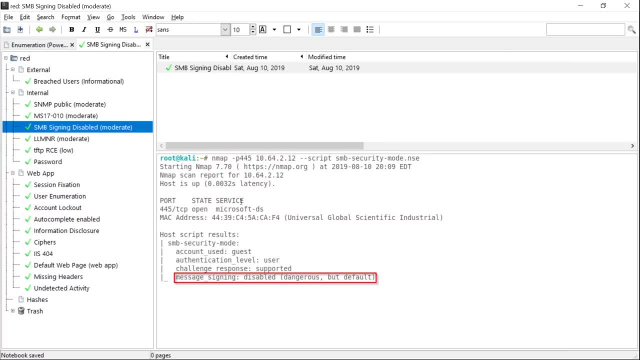 never know if a client's going to come back in six months or even a year and say: Hey, what was that here? And if you go back to your notes you say: Oh, you know, I did this. And some people get down. 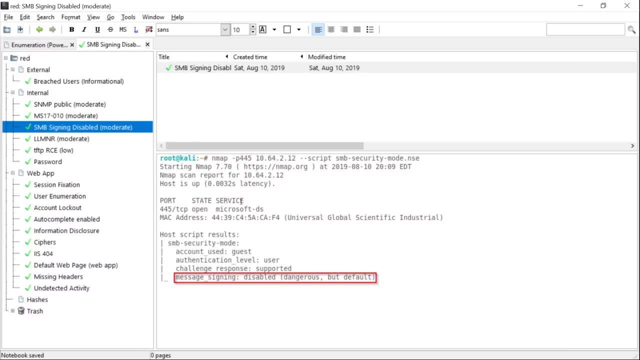 really into the weeds. they have dates, times, everything for step by step, what they do on an assessment, And that's completely up to you and how well you take your notes. This is kind of how I lay it out And then you see the green check marks next to it. I add those green check marks. 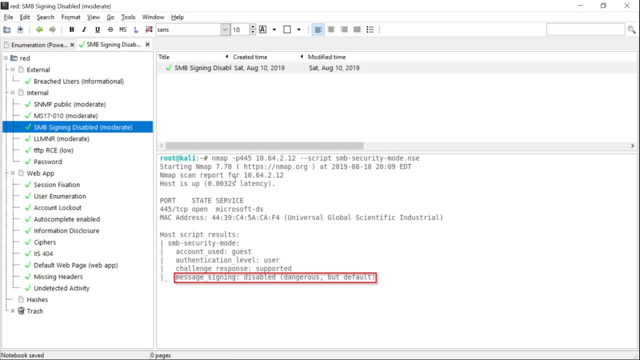 when I'm doing my report. So as I'm building my report out and I cover something in the report, I'll just go ahead and right click and I'll change the note icon to a checkmark, meaning that I've written that part of the report for that finding And we just kind of go through over. 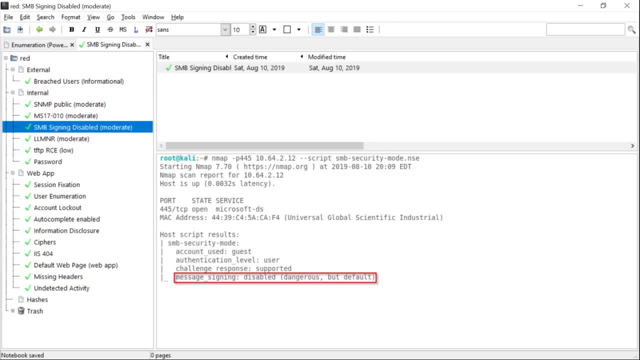 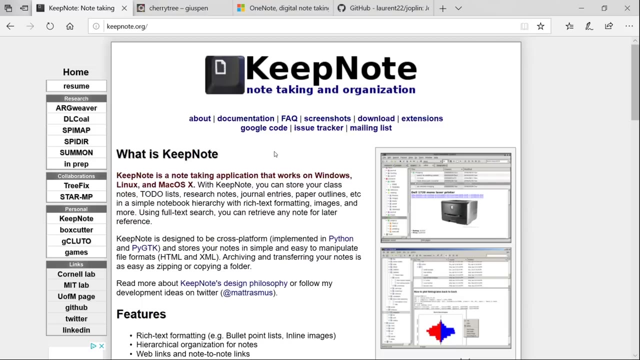 time. So, with that being said, I do want to show you some decent applications. The one that I'm using here and that you see is called keep note. Now I run on Windows as a base, So keep noteorg- That's how you get keep note. It is for Linux, it is for Mac OS X, But this is totally a preference. 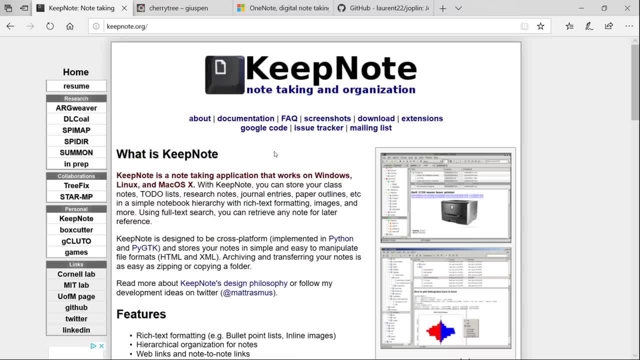 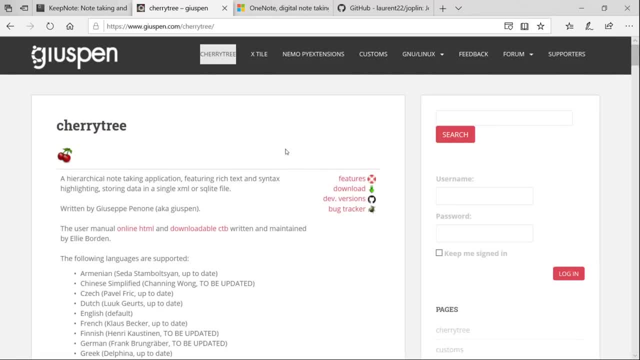 thing Me I prefer. I've been using it for a long time. Some people don't like it, Okay, so I'm going to offer some alternatives as well. cherry tree comes built into Kali Linux, as you're going to see here in just a little bit worth looking at, worth trying seeing if you like it. One notes: 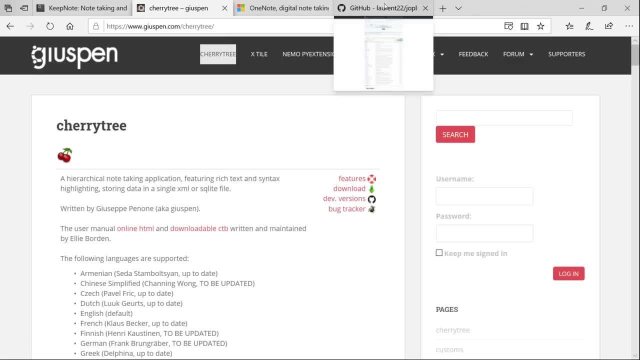 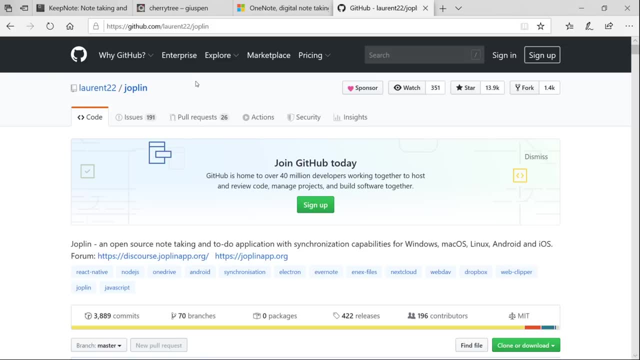 another example: if you use Microsoft and if you're a Mac user. a lot of students have told me that Joplin is really good. Now, I've never used this, but I keep hearing great things about it. So what I'm going to do is I'm going to put all of these into the course resources and you'll be 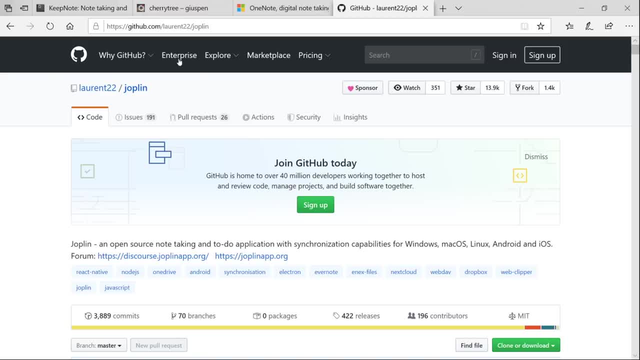 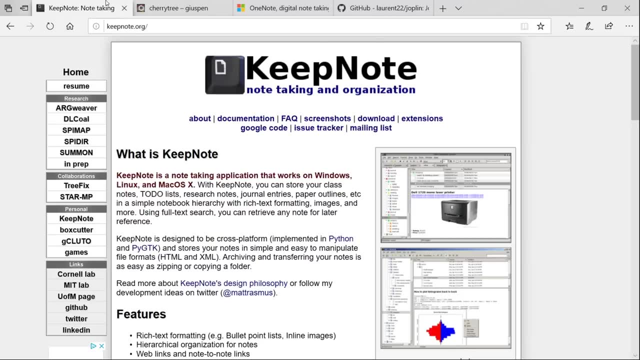 able to look at them, download them, decide on your own. Now, you're not limited to these four note keeping applications. by any means, feel free to use whatever you like to take notes. If you want pen and paper, that's great as well. 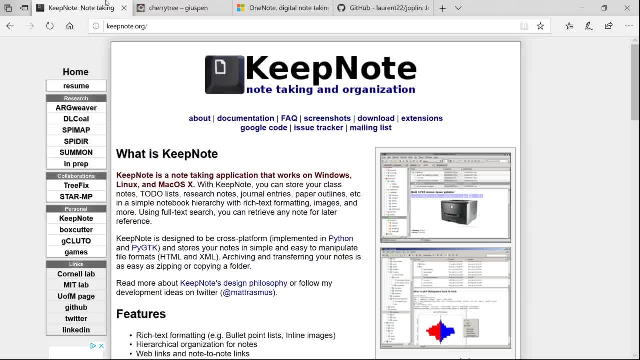 And so just make sure that you're taking good notes, And we're going to, we're going to harp on this throughout the entire course, over and over and over again. So make sure you're taking good notes. So, from here, what we're going to do is we're going to install. keep note in the next video. 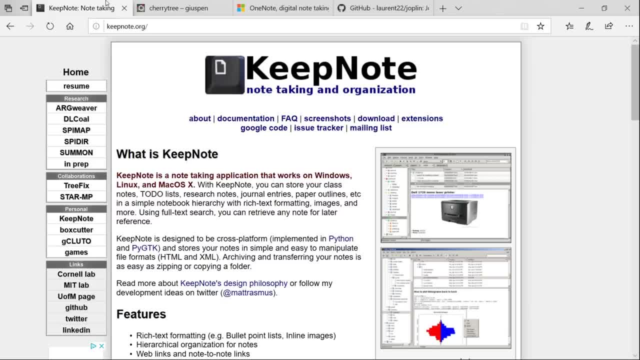 And we're going to install an awesome tool called green shot. I'm going to show you what green shot does And why it's so cool And I cannot live on any assessment without it. So let's catch you over in the next video when we work on installing those tools. 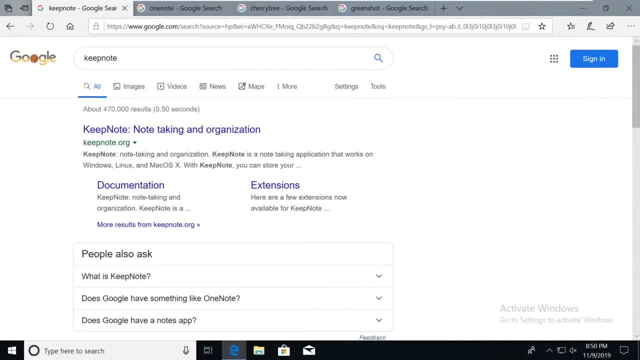 Alright. so in that example in the last video we talked about using keep note. So if you go to Google and you type in keep note, all you got to do is come here and keep note. works on Windows, Linux and Mac OS X. So great, great tools. 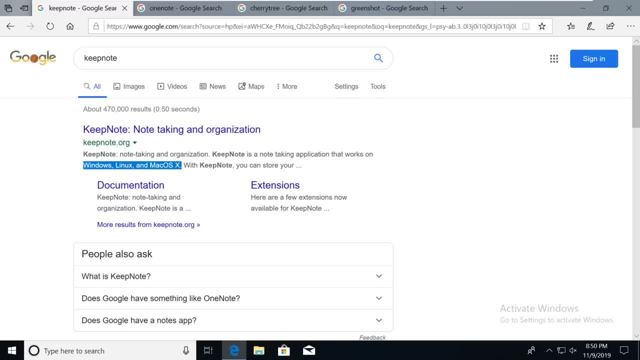 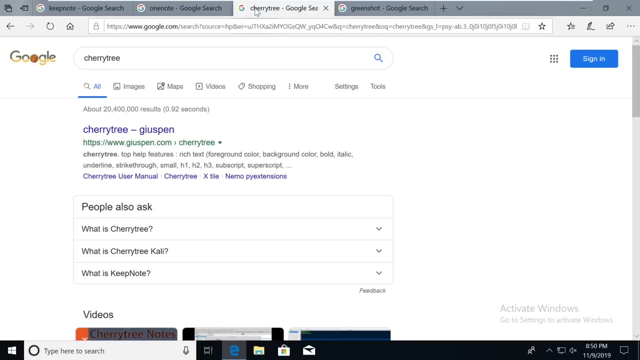 tool. the only issue with this tool is it has not been updated in a long time. some people find issue with that. if you're one of those people- i'm actually not- you can use other tools. one note is an option: cherry tree is also an option. you can also find other options out there for you if you. 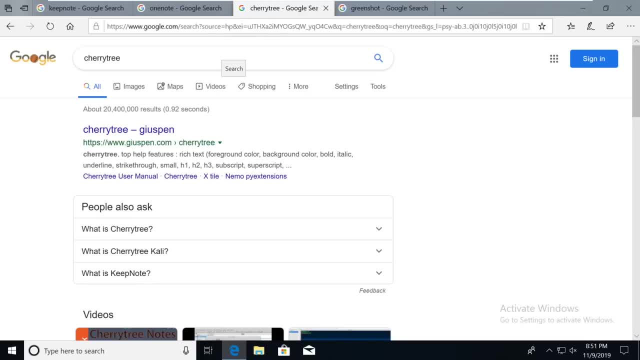 have a favorite note taking tool already. that's absolutely fine as well. just make sure to take good notes, especially during this course, and make the most of it. learn all the things that you can and incorporate that. so i will show you quickly how to install. keep note here. and another thing: 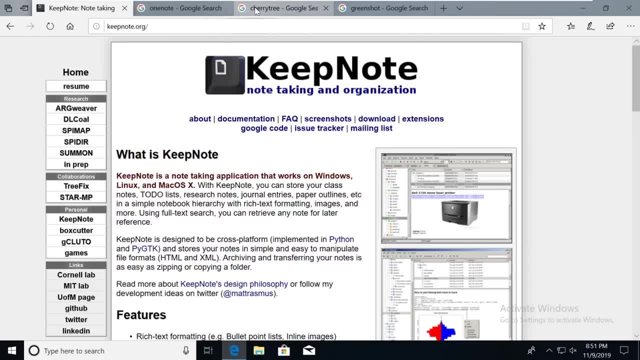 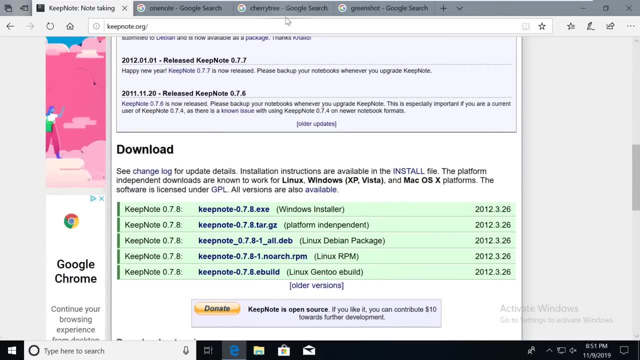 note too is, while we do this is cherry tree is available on cali linux. we're going to install cali linux here very soon. so once we install cali linux and we get into the introductory linux and we explore it, i'll show you a little bit more of cherry tree and what that looks like and we'll 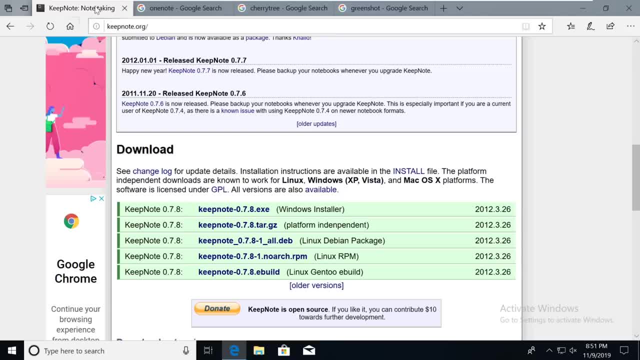 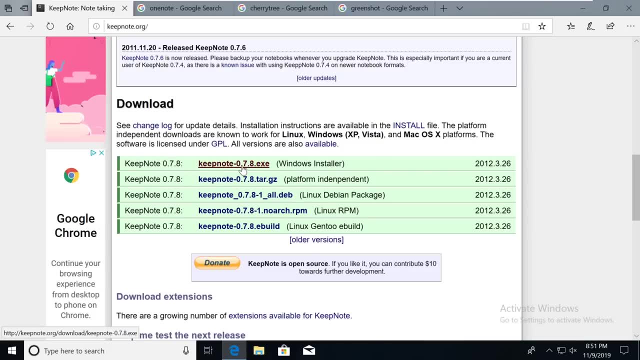 talk pros and cons of cherry tree when we get there. so here we go. if you are on windows, you can follow along, or you download your appropriate one here, you depending if you're on linux or if you need mac as well. so i'm going to go ahead and install the. 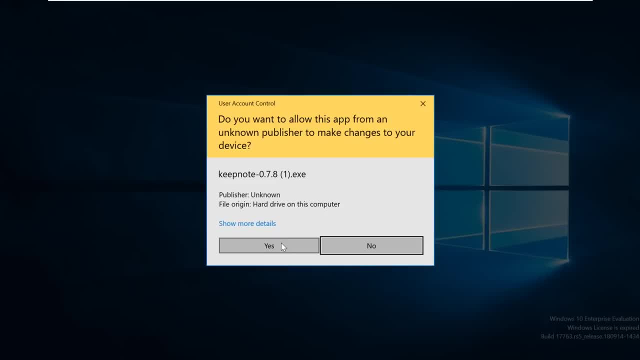 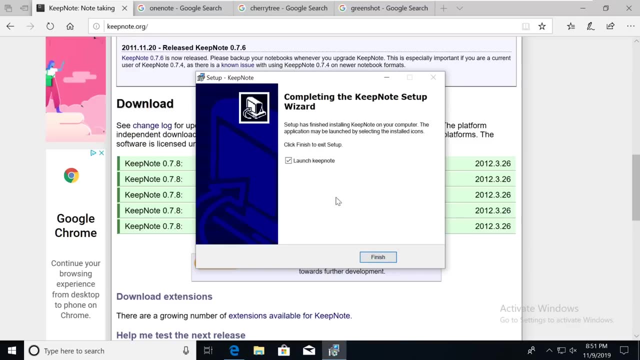 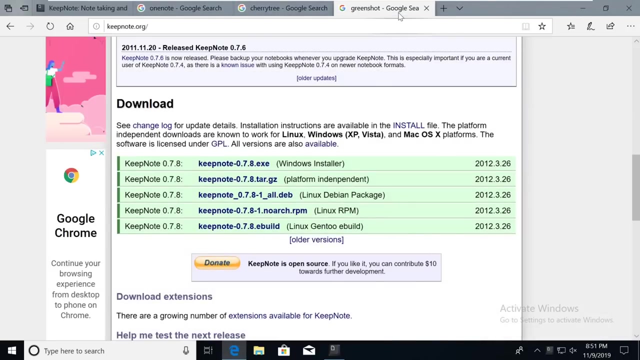 exe, and i'm just going to actually run this, we're just going to say yes, and i'm going to say next, next install, and that's it. that i mean it's, it's that quick, and then we just launch: keep note. and here you go, we've got keep note. so the other tool, the really cool tool that i love, this one is 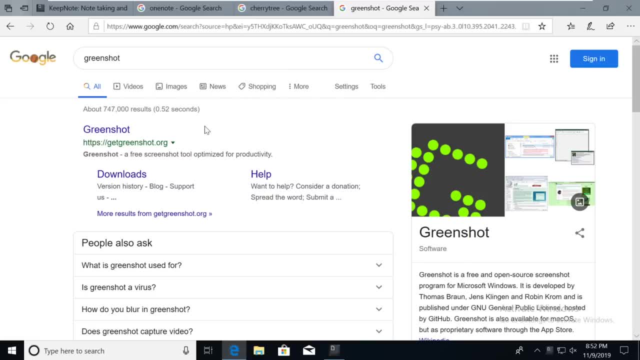 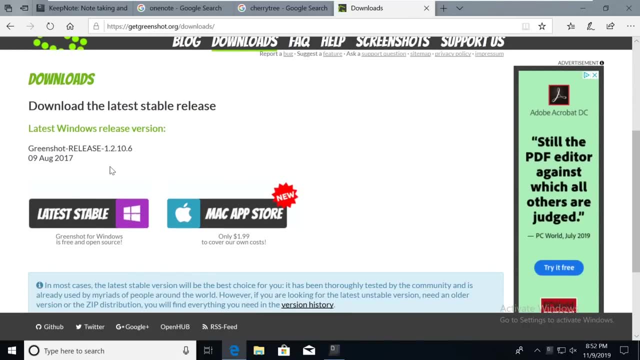 called green shot. now this is a screenshot capturing tool, so let's go to downloads here. on green shot, if you are running on something other than windows, you're going or windows or mac, so basically linux. you're going to need a different tool, the recommended tool that i've 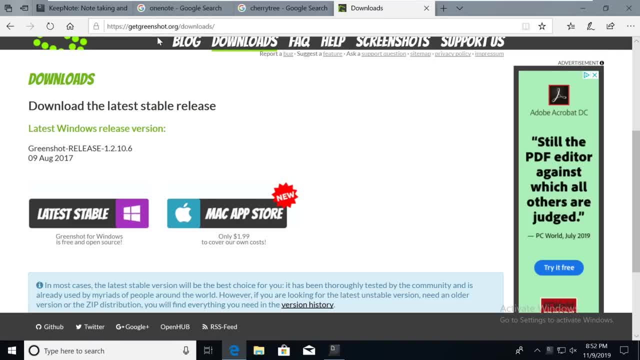 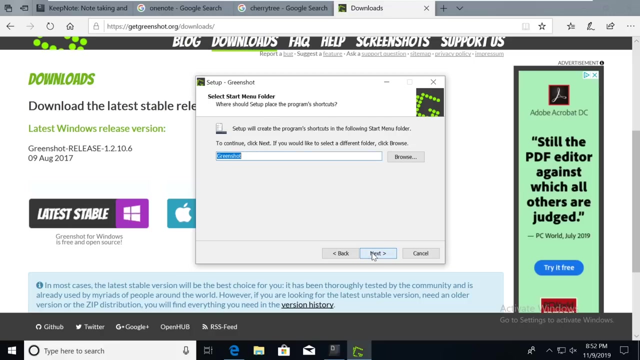 heard out there is called flame shot f-l-a-m-e. though i have no experience with it, i've heard it is identical to green shot. so here i'm going to download the latest stable. i'm going to select: run, yes, okay, accept the agreement. give away our firstborn. next, next, next, place it, however you. 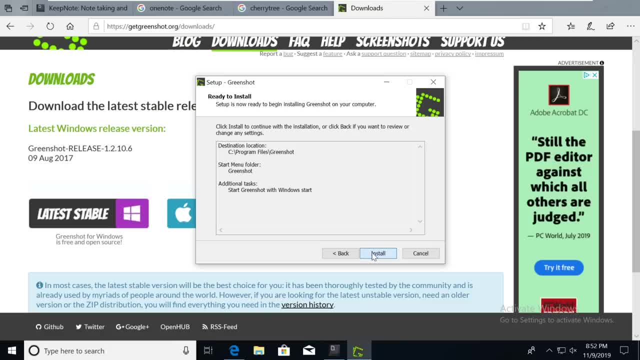 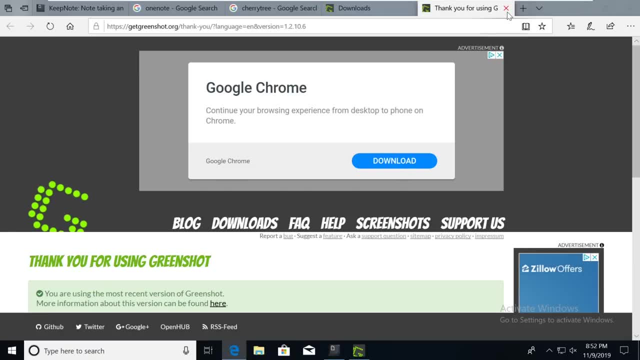 want. i'm just going to next through everything and i'm going to start green shot with windows start. that is my preference. i love this tool again. so it's finished, all right, let's take a look at it. so it should be running. let's start green shot now. okay, now you see it running down. 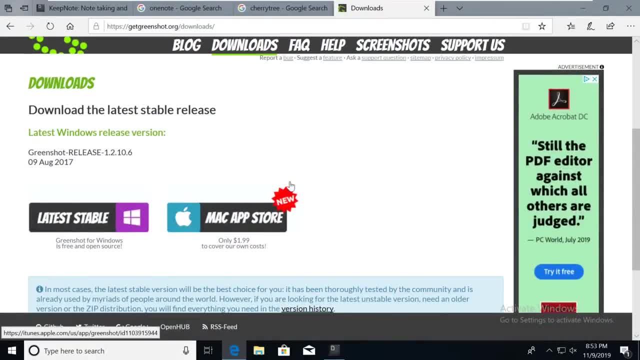 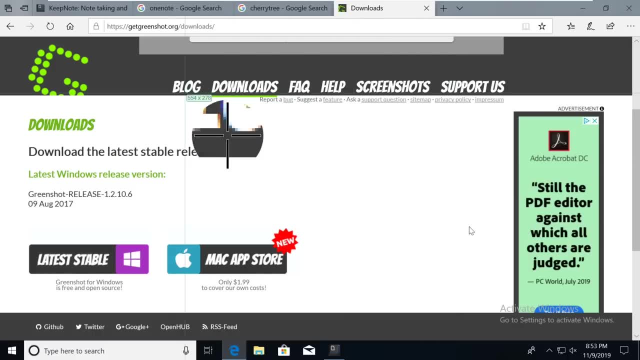 here on the bottom. okay, let's, let's go. let's open up a web page. let's say we want to take a screenshot of something. now you just hit your print screen button and this nice cursor gets brought up here. and let's say we want to. 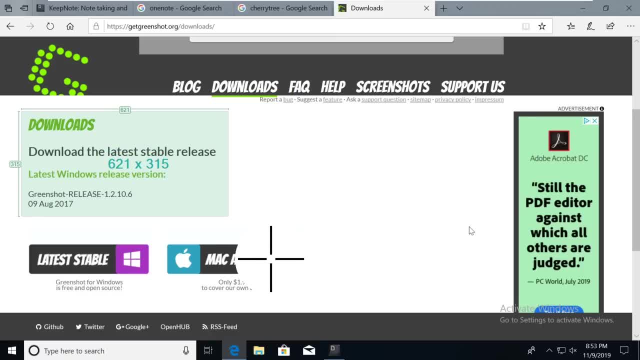 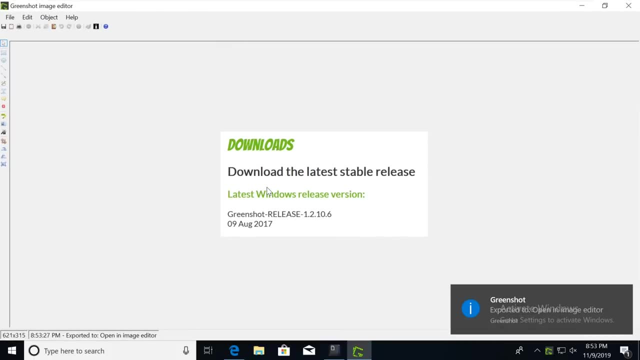 take this downloads part right here. we're just going to capture this and now we have choices. we can just save the image that we just grabbed, or my favorite is that we can actually open in an image editor. right, so let's open this in their image editor. look at this, okay. so here's the 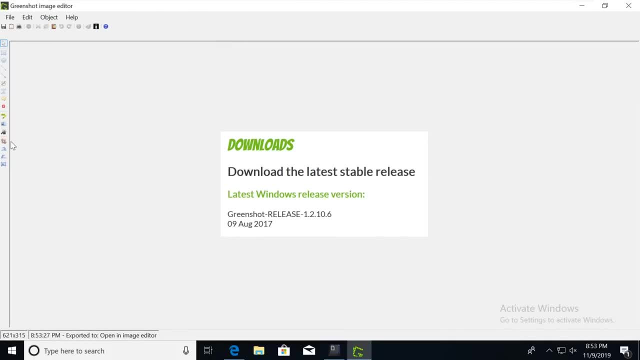 picture we just grabbed. right on top of this, we're going to take a screenshot of something like a meaningful Lorlin, etc. and we can see right above it that we're going to take those potential photos out of the tab that it says our image, that we 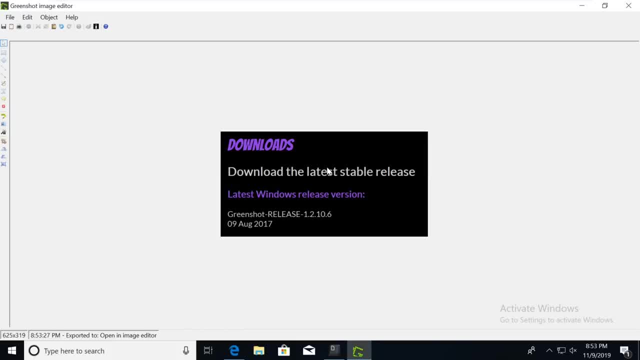 animated. that's how everything should be created, from where we get our material done zu, and then this is what we're going to do. what you can do here is we're going to go down here and go back here over there. oh, and this is where we're going to put our visual environment into the 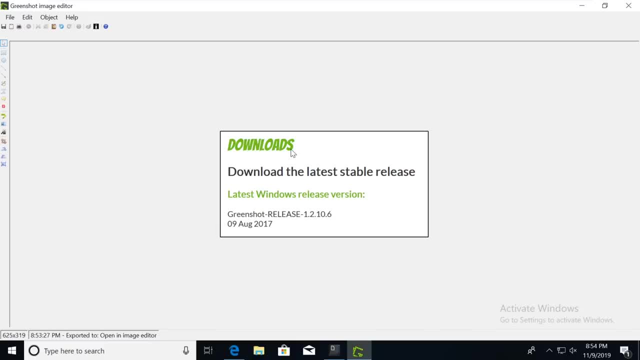 small image editor. we're going to do a passive cloud display, highlight a very powerful一点 and we hear that and we're not even off the toolkit. like I said, this is just wounded, massing, feeling nice on a report and when we get into the reporting you'll kind of see what that looks like. 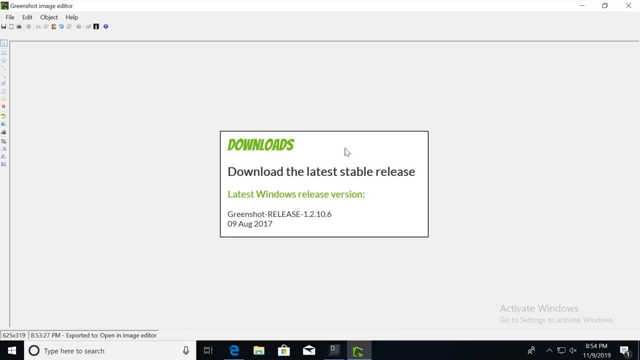 but i like a nice clean background. it saves on ink as well, if they were to print it, and it's just nice and neat when you give it to a client. so i always invert my images if i need to. you've got the black border here. another thing is: let's say you want to point something out. you saw in my keep. 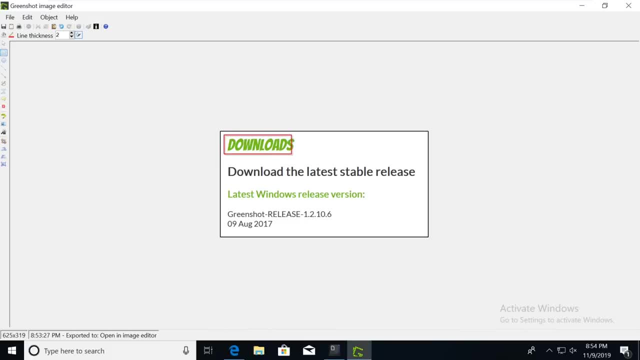 note notebook that i had a highlight. you can just click that button up here and just highlight something like: right here, great. another tool that's in here is this office gate. so let's say that there's like a password or something really sensitive in here, that that you don't want the. 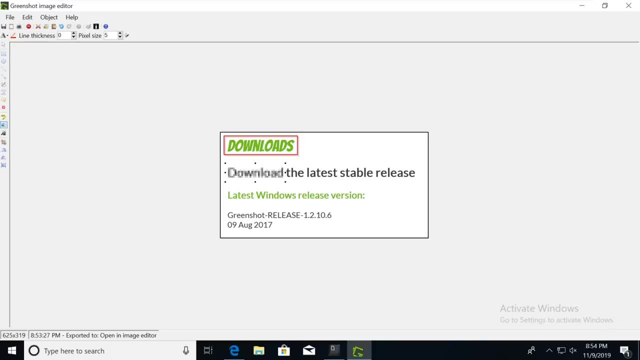 client to see or you don't want to be reveal on a final report. you can do that and then you can just like up the pixel size on this and make it really blurry, you know um. so it's a really really great tool and then, when you're done, you can copy it to your clipboard. you can save the file. 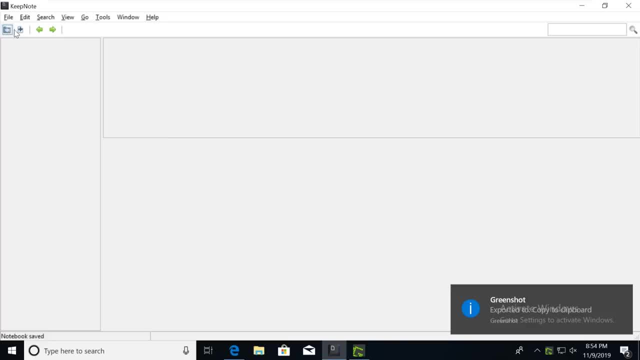 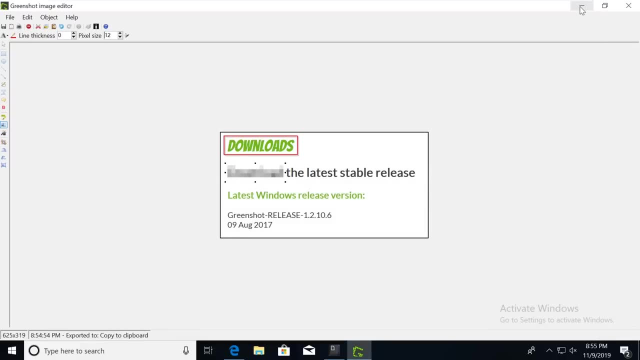 i just usually like copy this and if i want to go paste it, like know, make a new notebook or whatever, i'll just paste it in my keep note and just kind of go from there. so again, fantastic tool, awesome to use. if i had two recommendations for your note, keeping it's. 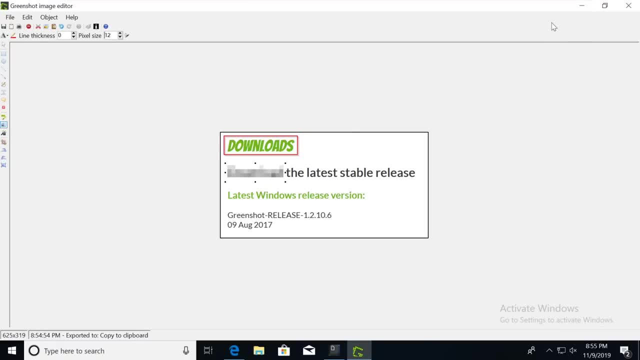 keep note and green shot. if i had to make one recommendation out of the two, it's absolutely green shot. you can be flexible on your note keeping tool. so again, hopefully this helps you. again, again, again. please do take good notes through this course you're going to find yourself. 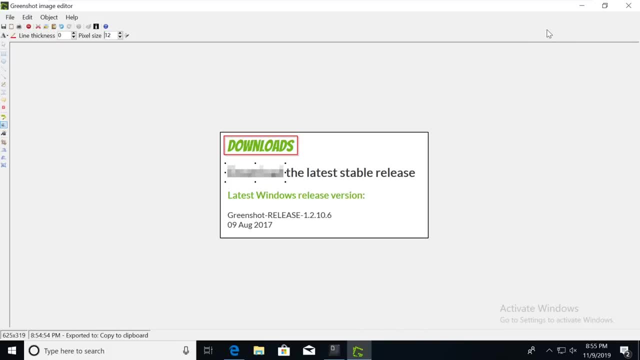 wanting to know, hey, what was that command, i ran again and because we're going to go through so much stuff by the time this is all said and done that you're gonna want to remember it, so please take good notes. so from here, let's go ahead and move. 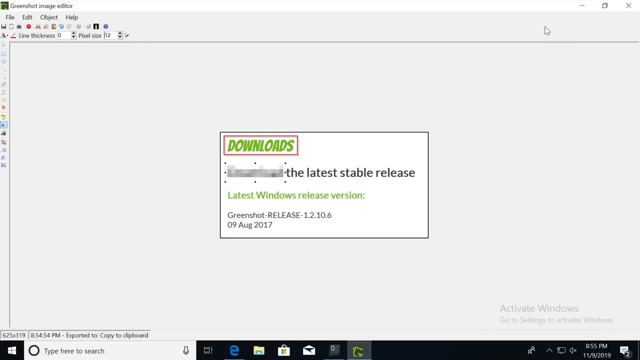 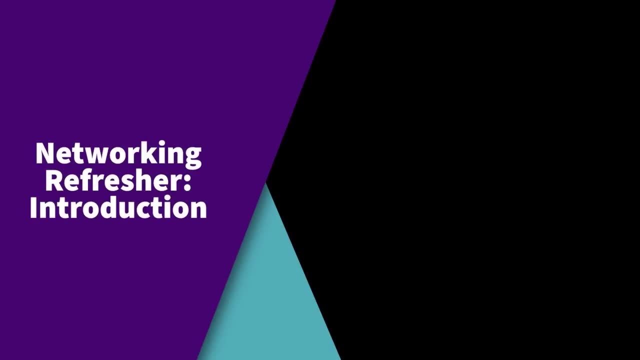 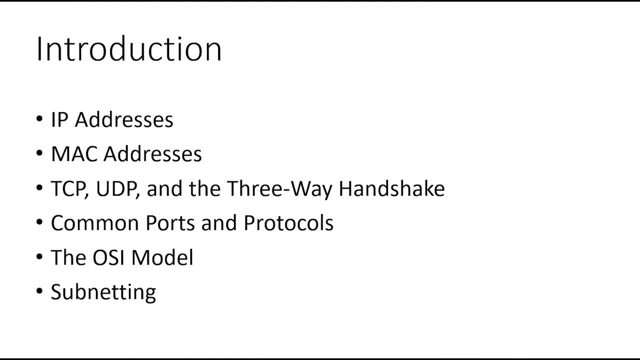 on into our networking refresher and we'll, uh, catch you in the next video. hello everyone and welcome to this section on networking. so this section is titled networking refresher, meaning that some of you are a little strange in the networking background, and if you're looking at this list, that's on the 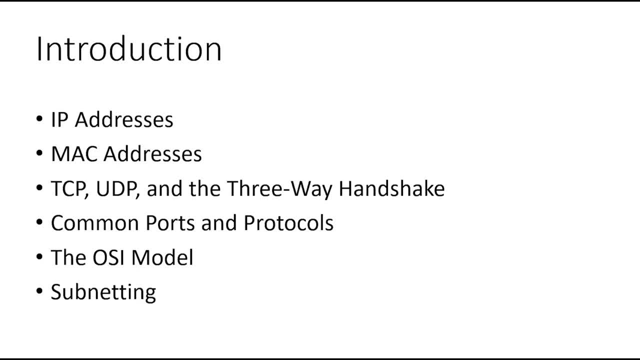 screen and you go down the list and you say, yep, i know all those. you can feel free to skip this section. if you've taken some of these in the past and you just might want a little bit of a refresher on them, then this section is for you. we're going to cover these topics- not totally- in. 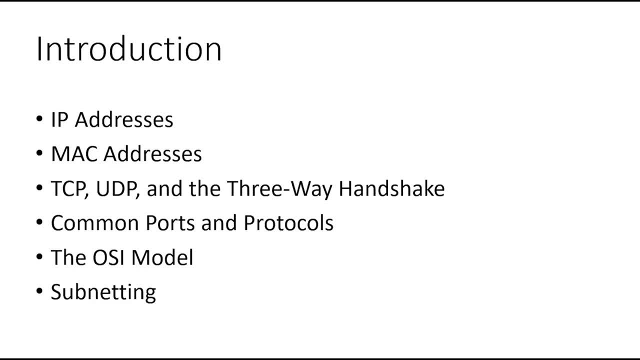 depth, but we're going to use it as a way to brush up and then we'll hit on networking again when we get into introductory linux. so if you are unfamiliar with things like that, then these three actions will help you meet in the like TCP, UDP and the three-way handshake, or if your subnetting is a little shaky or you don't. 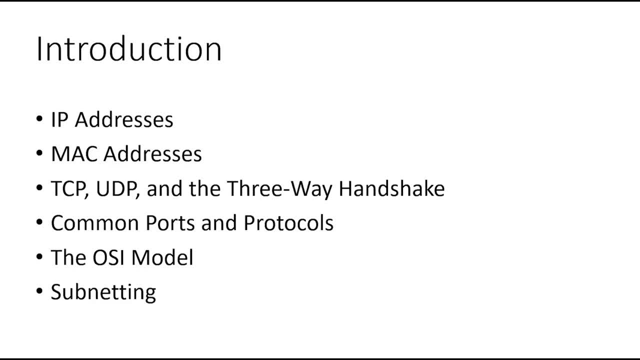 know what the OSI model is, chances are you should probably stick around and just click through this series, watch it and build that foundation. Remember we talked about one of the core foundations of pen testing being a strong networking background. This is a good way to. 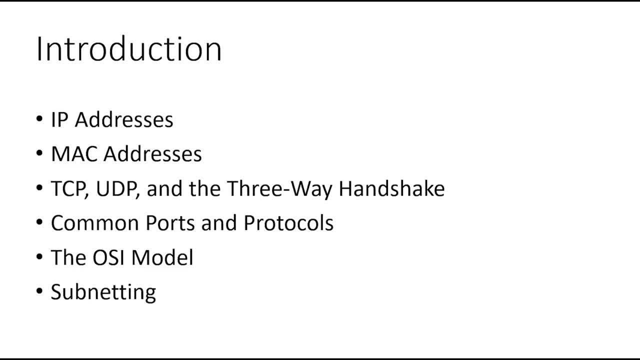 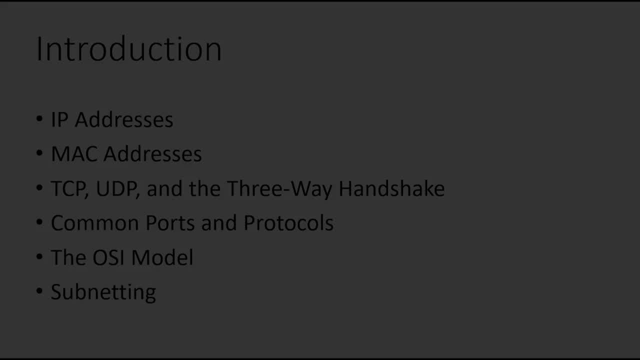 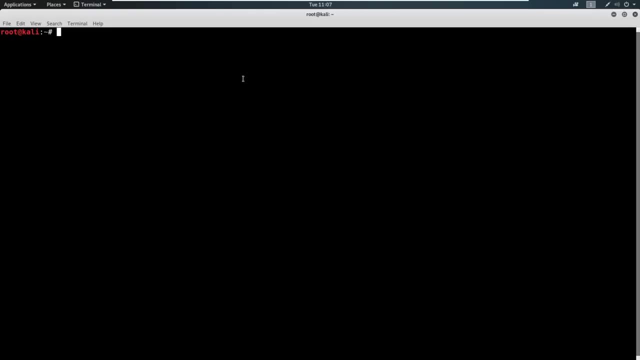 build it up, remember what you might have forgotten and go from there. So let's go ahead and just jump right into the first video, which is going to be IP addresses. What's up, everybody? So I'm going to preface this video really quick. with that it is. 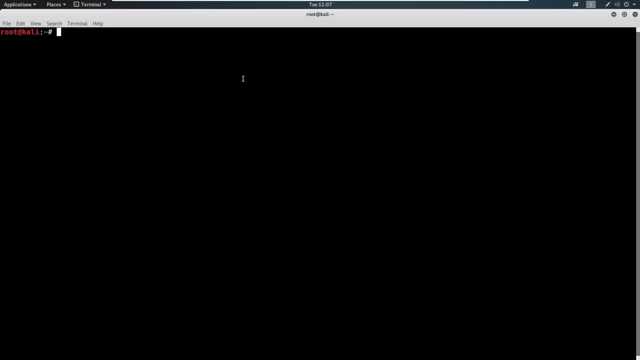 raining pretty hard here, So if the soothing sounds of the rain puts you to sleep during this video and you can hear it, I'm very, very sorry, But the show must go on. So what we're going to be doing today is we're going to be talking about IP addresses. Now, if you've ever 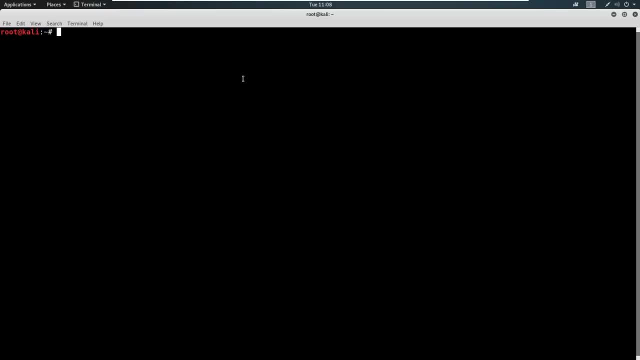 used IP addresses, you're probably familiar with the IP addresses. So if you've ever used IP addresses, you're probably familiar with the IP addresses. So if you've ever used IP addresses computer before and you're any any what familiar with it, you probably know what an IP. 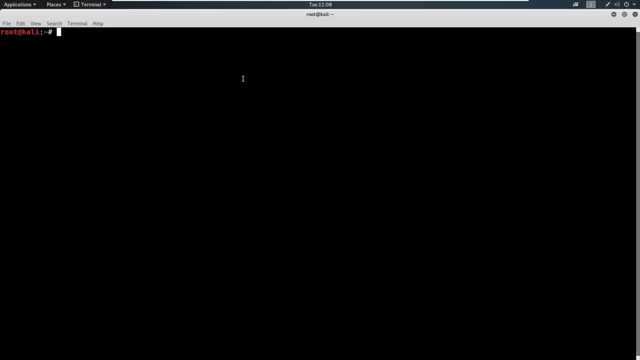 address is. But I want to take this a little bit deeper in in theory, on why we use IP addresses, what types of IP addresses are out there, and talk more about protocols and how IP addresses are actually designed and made up. So I'm here in a Kali terminal And I'm just going to type 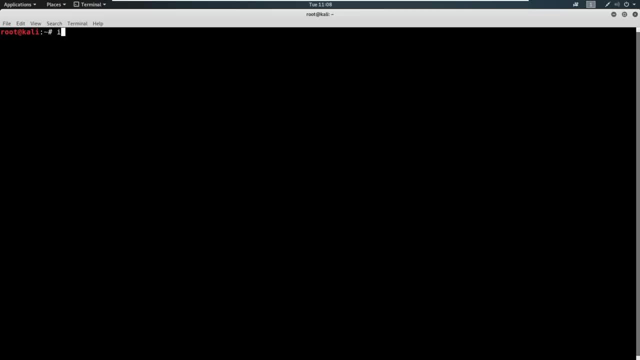 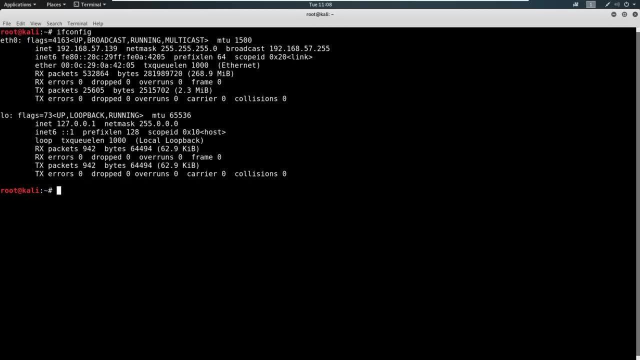 in a simple command, And that command is if config. Now, if you've used IP addresses, you probably know what an IP address is. If you've used Linux before, this might be familiar to you. If you use Windows, it's similar to IP config. all I'm trying to do is bring up my IP address, So what? 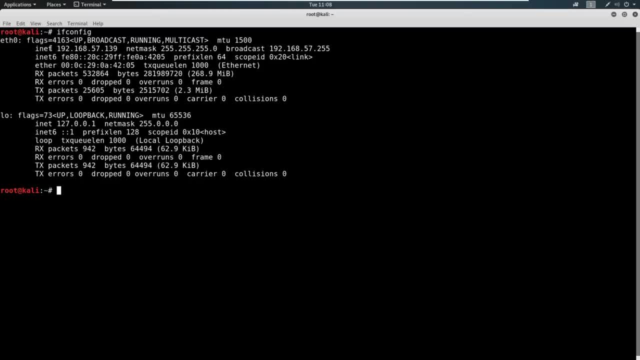 we can see here is that we have an IP address which is our INET. This is my IP address here. I also have another IP address, this INET six. this is what's called an IP v six address. So we've got this INET, which is considered an IP v four, in this INET six, which is considered an IP v. 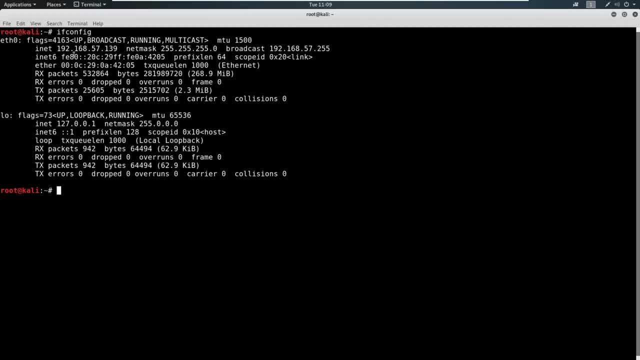 six. Now you can notice right away that there's two different types of notations for these. This INET here is in a decimal notation And the IP v six is in a hexadecimal notation. we'll get to the importance of that in just a second. So when it comes to IP addresses, this looks probably pretty. 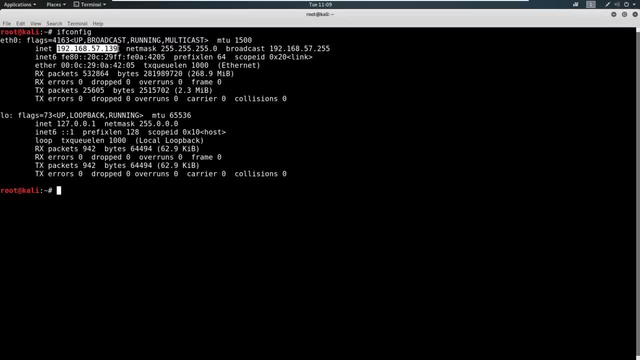 familiar to us. This is an IP address. This is how we communicate. we communicate over layer three, And you're going to hear me talking about layers repeatedly throughout the course, or at least throughout this part of the course, so that we can get familiar with how we're actually doing this. So I want you to be familiar. 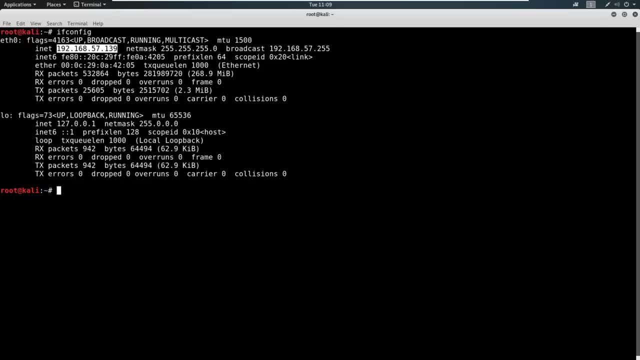 with troubleshooting these layers. And these layers all refer to something called the OSI model. So when we we talk about layers, we think about the OSI model, and I'll introduce the OSI model here in a few videos And it should all click once I introduce the OSI model. So if I 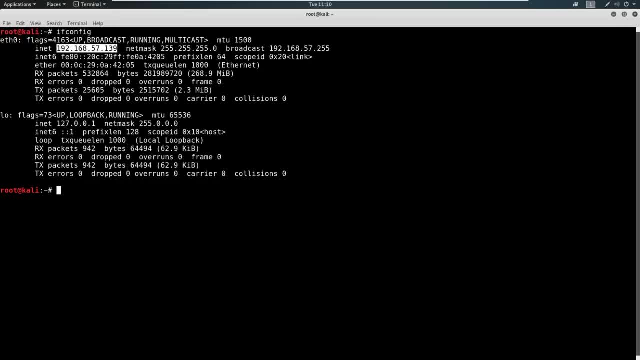 brought in the OSI model up front. it might be boring, might not make sense, So I'm going to introduce the OSI model near the end And you're gonna say, Hey, yeah, that all makes sense. So what we've got here is we've got this IP v four address, And this is the most. 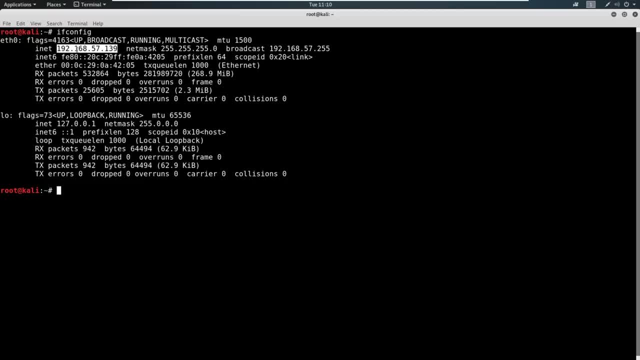 commonly used format that we use today. right, we use IP v four for mostly everything And, again, this isn't that decimal notation. So when we see this decimal notation, it's just a realistically, a bunch of ones and zeros that are put together so that we have this human readable format. 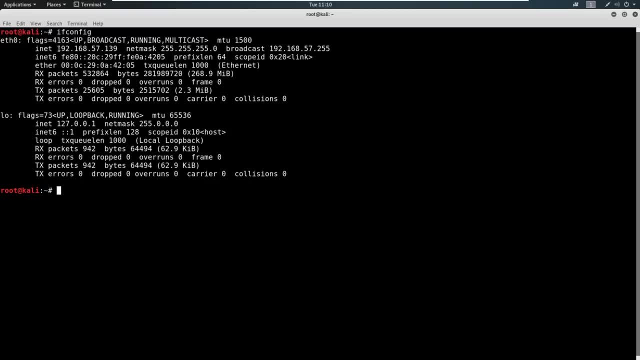 Realistically, all we're seeing here with 192, this first, this first section here, this first octet, is actually just a bunch of ones and zeros, eight bits. So we've got a range of eight ones and zeros here. we've got another eight here. 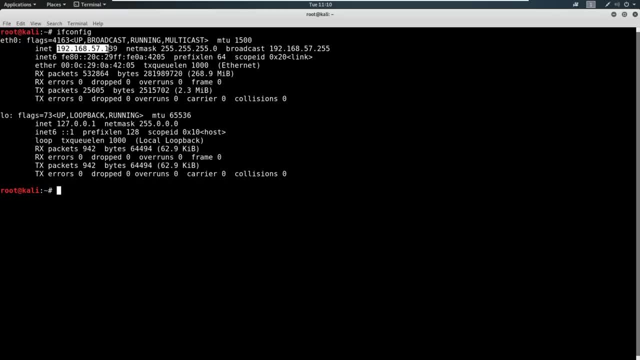 eight here and eight here. So when it's all said and done, this INET or this IP v four is made up of 32 bits, eight plus eight plus eight plus eight here, and which equals four bytes. So another way to think about that is to think about the IP v four, which is the IP v four, which is the IP v four. 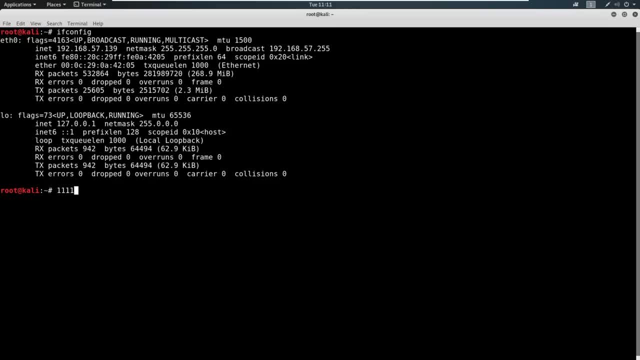 and then we can think about it as, say, something like this: 12345678. Period. Okay, that is one section there, So we've got eight ones that can make up this, and then we'd have another eight, etc. I'm not going to beat a dead horse here, But I do want to give you guys another example. 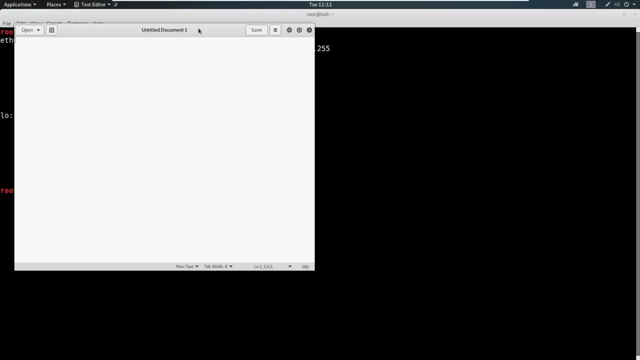 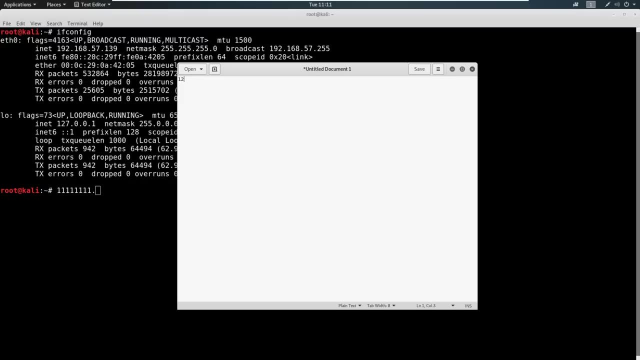 So if we go into our applications and we go to a text editor really quick, So the way this looks is something like this: we start with a number like 128.. I'm going to try to space this out as best as possible And all I like to do is think of 128 as 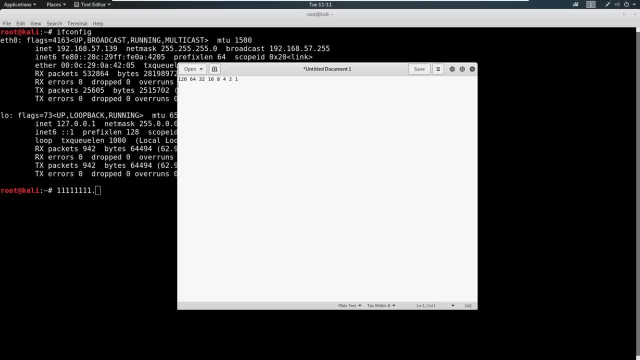 my base, And this will make a lot more sense when we get into the subnetting. So please, if you're confused by this, don't worry. this is all theory right now. When we get into subnetting and we get hands on, it'll make a lot more sense, I promise you. So let's say we have ones and zeros. 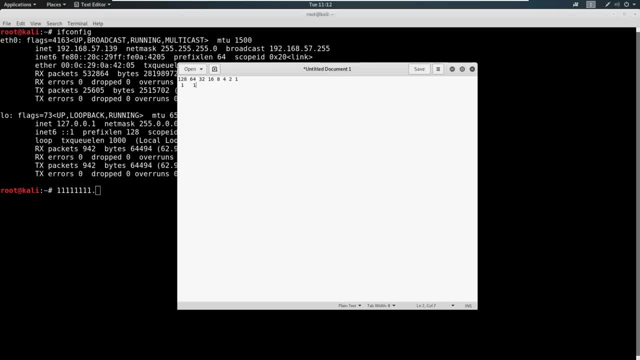 here. If we have a one for each of these sections. I'm going to space this out again as best as possible. It's not pretty, So let's have a one for each of the sections- Again, as best as possible. 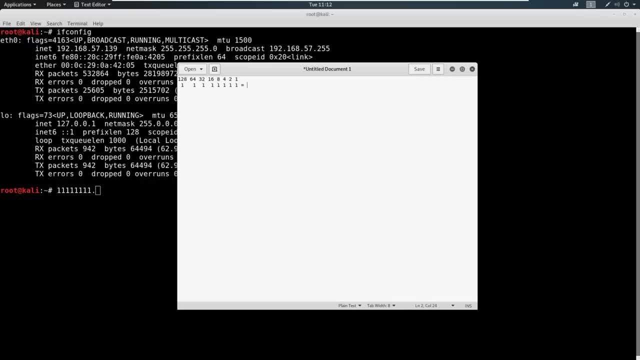 It's not pretty, But if we want to make it a little more easy than that, we can do that here. So so we'll. it's not pretty, But if we have a one for all these, this equals 255.. Why does this equal 255?? 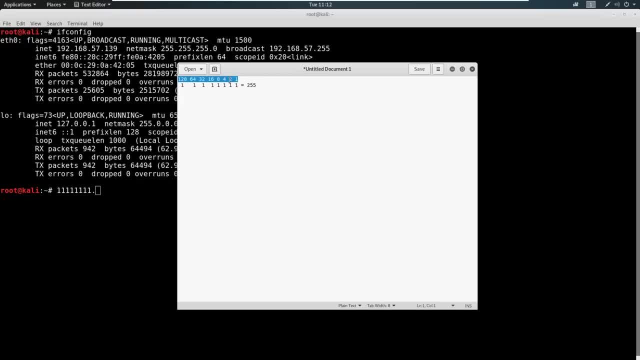 Well, you take this and all these numbers add up one plus two plus four plus eight, all this adds up to 255.. So let's say, if we didn't have all the ones and zeros, we had just some ones enabled, like these last three here. Okay, well, this would equal seven. 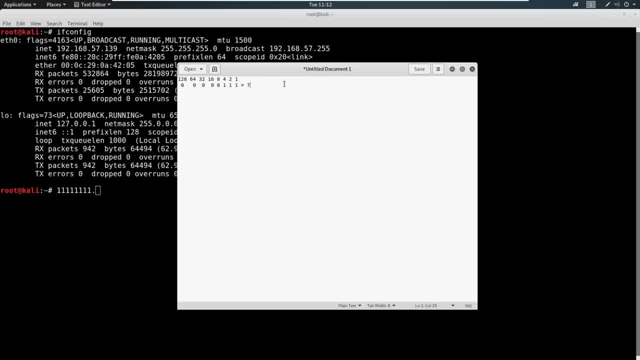 Because we have four plus two plus one equals seven. So our first number, or whatever number this applied to in the octet, would be seven. So if we had 7.7.7.7, it would just be this: numbers repeating over and over, these numbers repeating over and over, right. So 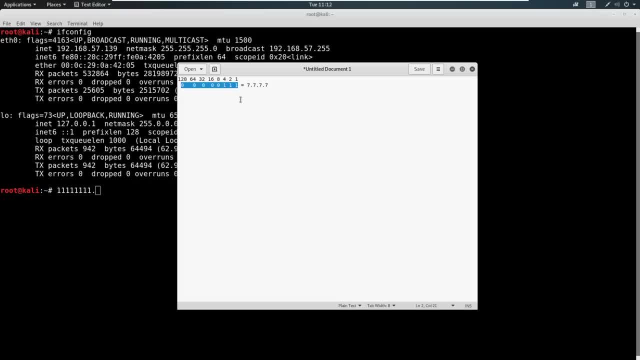 be 0000111.0000111, and so forth. So this is kind of what it looks like behind the scenes, because we have all these numbers and we have all these numbers, and we have all these numbers because, again, a computer is just ones and zeros. we're all binary. So what we're going to do is: 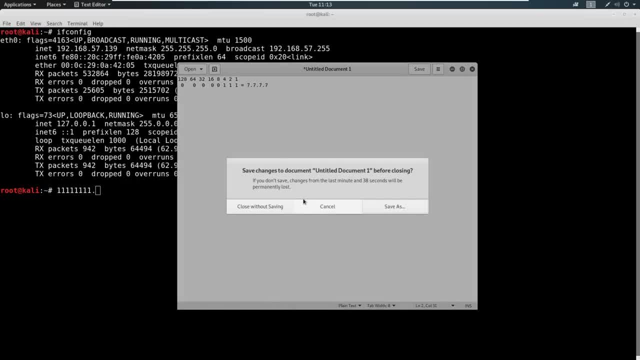 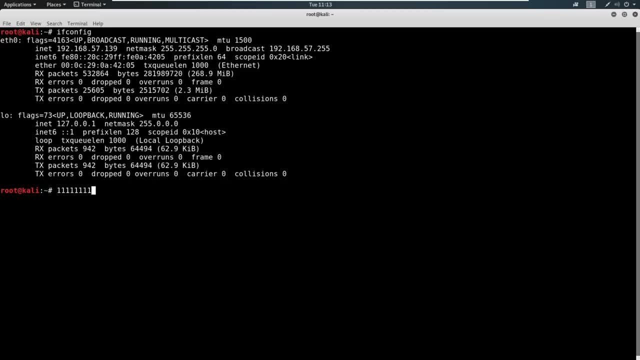 we're going to close this out. we're gonna talk a little bit of other theory when it comes to this and why I net or IPv6. And why IPv4. So let's close this and let's talk about IPv4. So I'm 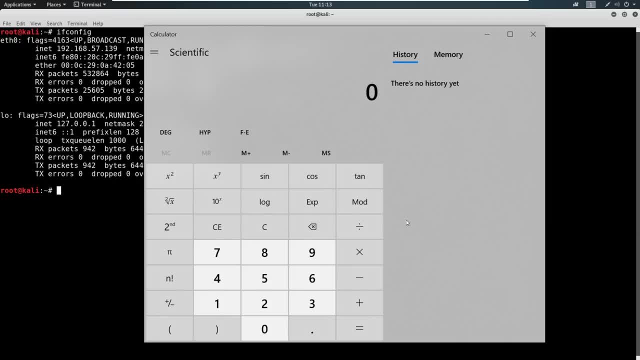 gonna bring up a calculator And with IPv4, we have these 32 bits. So what we can do is we could take two to the 32nd power And this is the possible amount of IP addresses that we could have. So we have somewhere in the 4 billion range of IP. 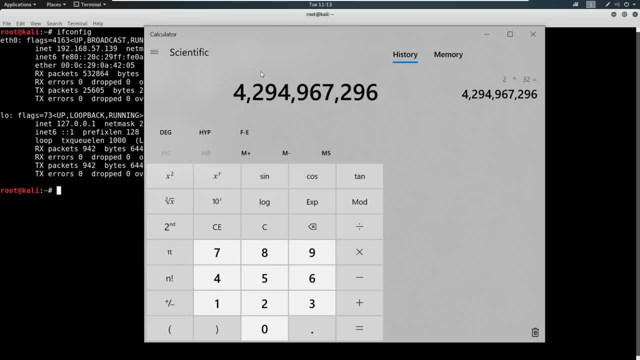 addresses. Well, spoiler alert, we don't have only 4 billion people on earth, right, We're up to seven something billion at this point, And all these IP address spaces are gone. So IPv4 has been around since 1981.. Nobody thought we were ever going to use all these addresses Computers. 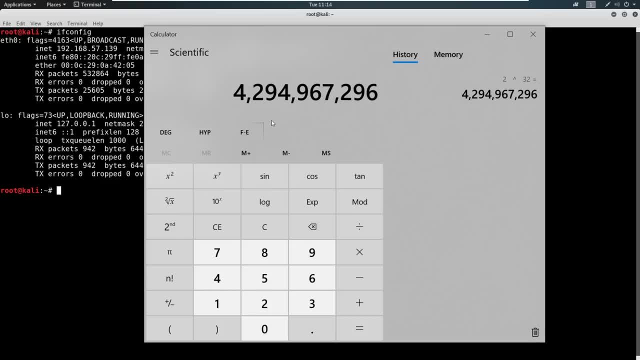 weren't really a thing. Who knew that we were going to want all these addresses? And you know, these companies started buying them up and they started buying them up in large chunks And then they sold those to ISPs. and then ISPs sell those to you And so these IP addresses have. 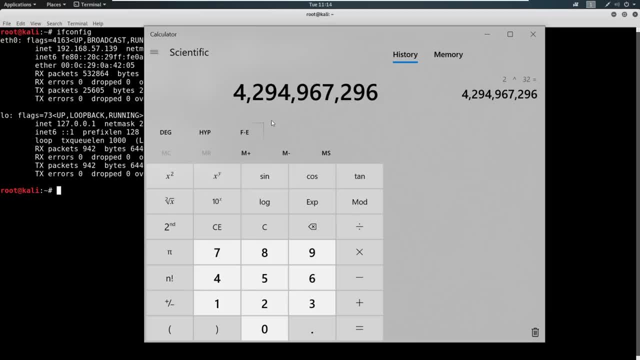 been gone for a very, very long time And chances are when you, when you have an IP address and you get this IPv4, you're only going to get one. if your corporation you might buy it more, but we've run out of IP address space. there's just not enough to go around. So the theory is: 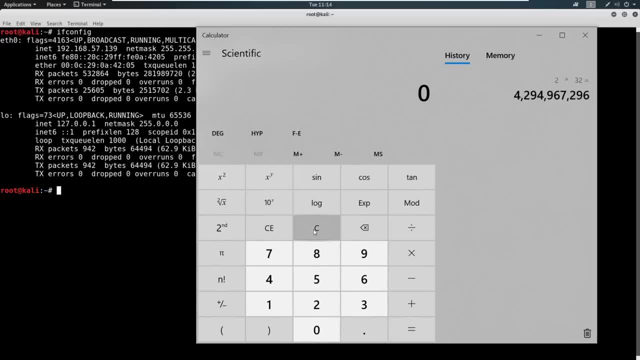 okay, let's come up with something different. Let's come up with IPv6.. Now this hexadecimal is actually in 128 bits, which makes things just a little bit longer and adds quite a bit. So let's take this two to the 128 power And we get a number that I cannot tell you how to say, not even. 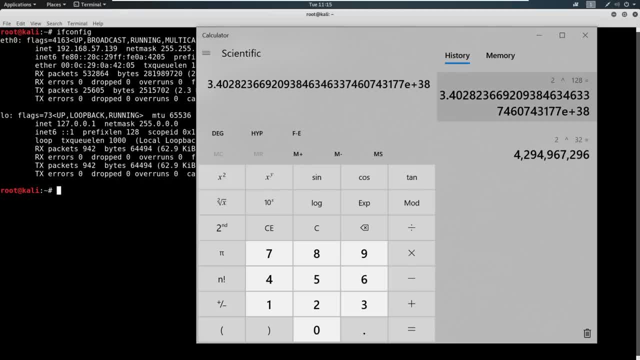 going to try, But I can guarantee you that in our lifetime we will never use this address space. So we've come up with a solution of IPv6.. But nobody really uses it. IPv6 is just a thing, that's, that's there. But when we get IPv6 addresses a sign. but still to this day, everybody's using. 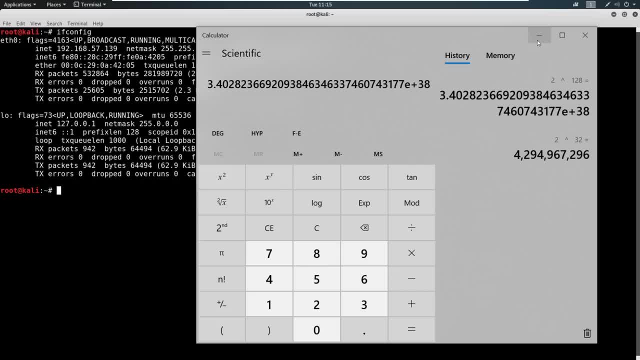 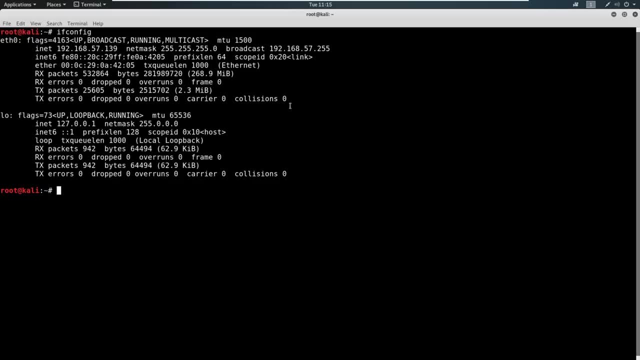 IPv4.. Well, how? how is that possible if we're using IPv4, but we're out of address space? Well, think about this. we're using something called NAT, which is network address translation. Now, let's think about your network address translation. Now, let's think about your network. 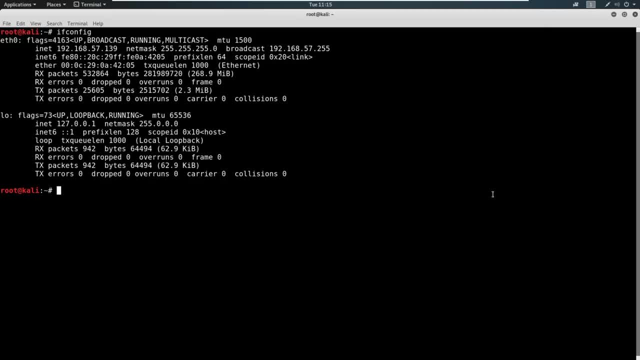 address translation. Now let's think about your network. So you might have a cell phone or computer or multiple devices. my network has at least 20 devices on it. I've got. I've got cameras, I've got multiple cell phones, smart TVs- everything that connects to my internet gets an. 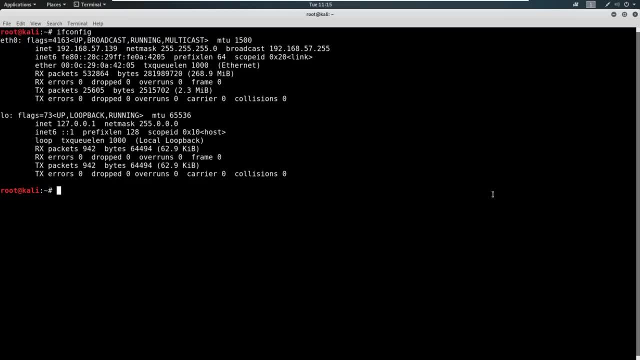 IP address And that's 20 IP addresses, right there, right? So let's say I have 20 devices, that's 20 IP addresses. Am I taking up 20 IP addresses out of that 4 billion? No, we're actually. 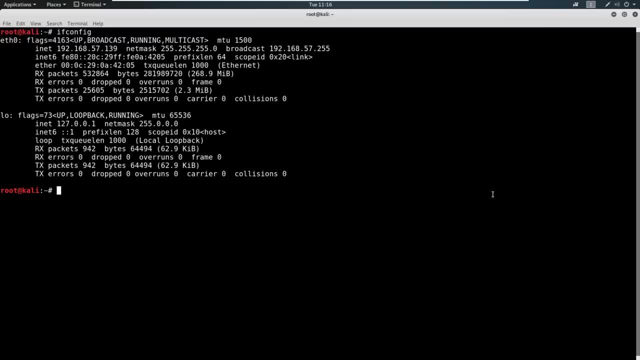 something called network address translation, or it's called NAT for short, And we'll talk about this again when we we set up our actual lab. But with NAT, what we're doing is we're assigned these private IP address spaces. So we've got this: 192.168.57.139.. Now, if you've ever seen a IP, 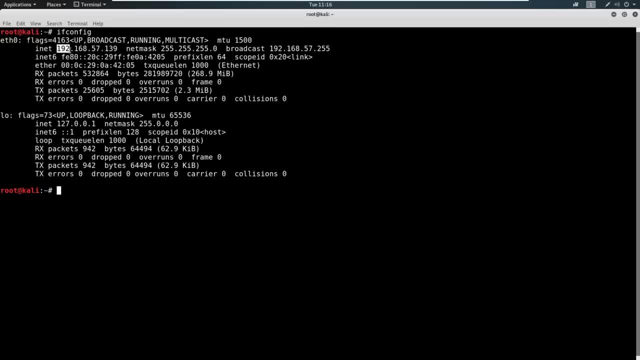 address before and you've been on a network, good chances are probably started with 192. Or maybe it was a 10 dot or something along those lines, And that's because those are private IP addresses. So anything that starts with 192.168 is not an IP address that is going to be out in the 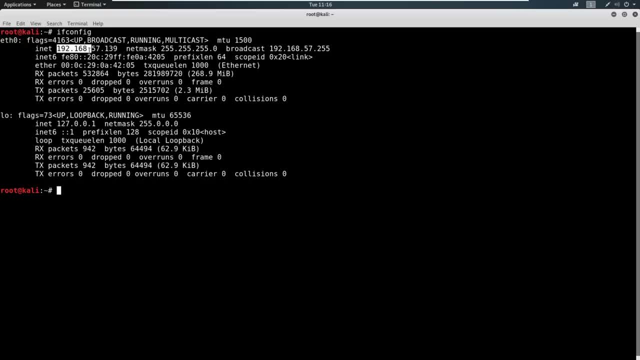 the interwebs, it is going to be an IP address that is only known to you. These are called private IP addresses. So because we use these private IP addresses, we can pass them out through what is called a public IP address. Now, to make better use of this, let's go out to Firefox. 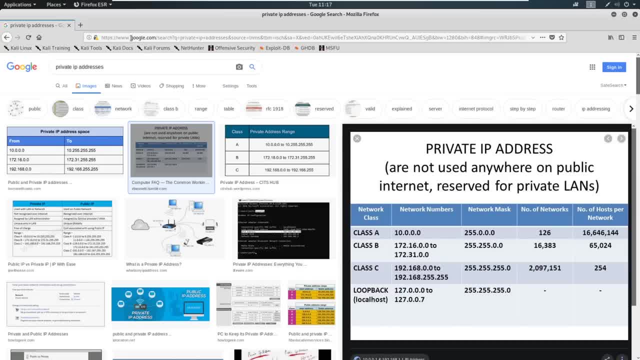 I've already got a tab open. So I went to Google and I just said private IP addresses And I clicked the second image here because I think it's a great image. So if we look at this, there are classes of IP addresses: private IP addresses. Now there is a class D and E. we're not going. 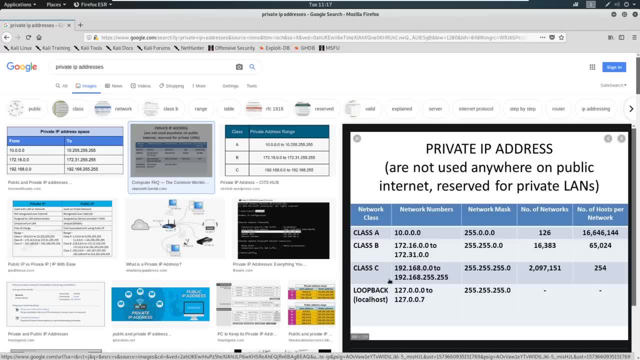 to worry about those. The big three are class A, B and C. If you know these, you are good to go. So if we look at class C, this is what the most common household and small business use- We see it starts with the 192.168.0.0.. So the 192.168 are constant. If you see a 192.168 address. 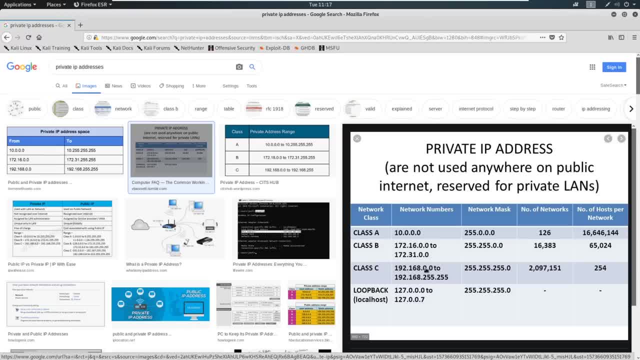 you can guarantee yourself that that is a private IP address space. And then we have the range of changing this number between zero and 255. And this number between zero and 255.. Y, zero to 255.. Well, that'll all make sense when we get into subnetting. 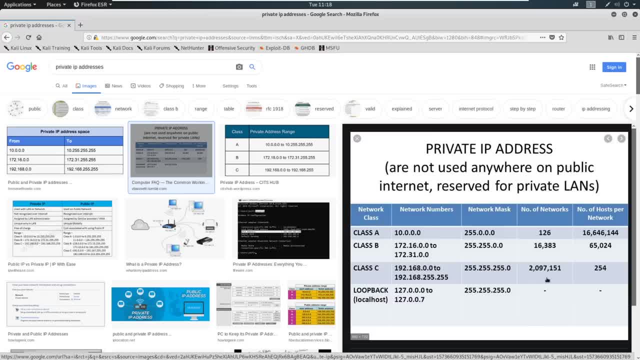 But what that allows us to do is have a large number of networks here and a small amount of hosts. But for a regular user like you or I, or a small business, 254 hosts is pretty good. I mean, I'm only using like 20 in my household, So the most common. 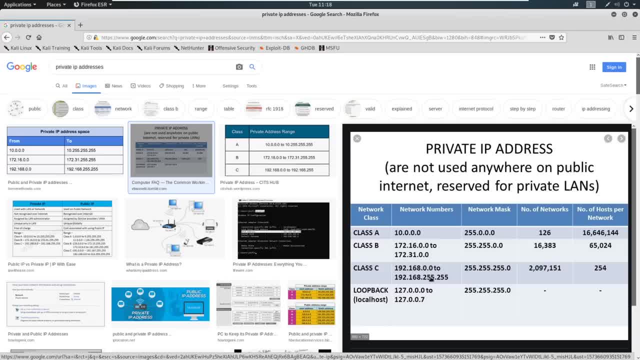 household is probably using this 192 address. But what about a big, big business, right? Something huge? Okay, well, they might use a 10 address, Because a 10 address frees you up to anything after this. 10 is private. So 10.1, 10.1.1.1, whatever you want to put in here, up to 255 on. 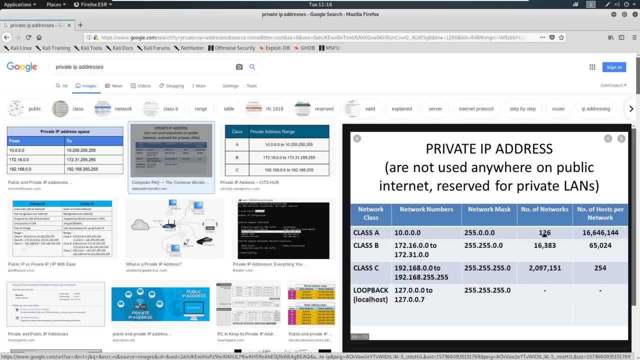 each octet makes for a small amount of networks but a large amount of hosts. Okay, and don't worry about the host versus network thing Again. subnetting, we'll talk about that, It'll all make sense. But just imagine the amount of amount of hosts that you can put in here with this wide 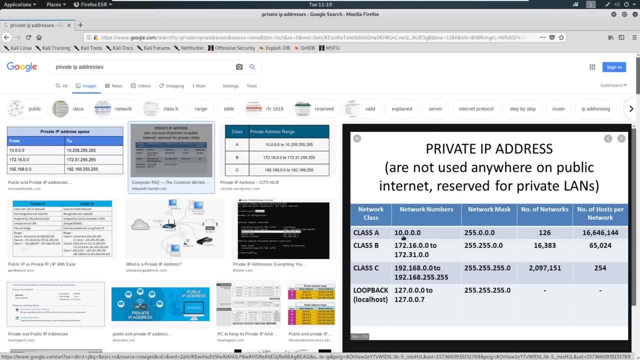 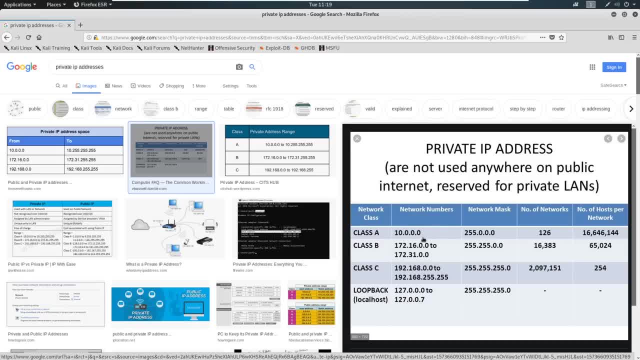 10 addresses The. the matter of fact is, as long as you have this private IP address, you're good to communicate across your network. So any IP address outside of these and the loopback here are free game. for the public address space, they're probably already owned And you purchase. 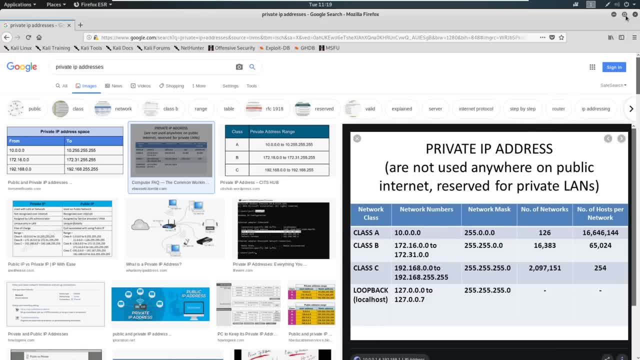 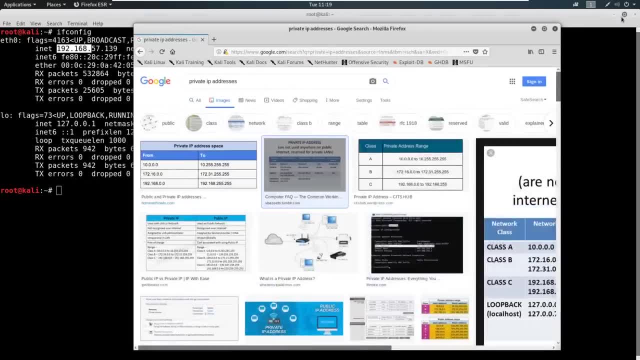 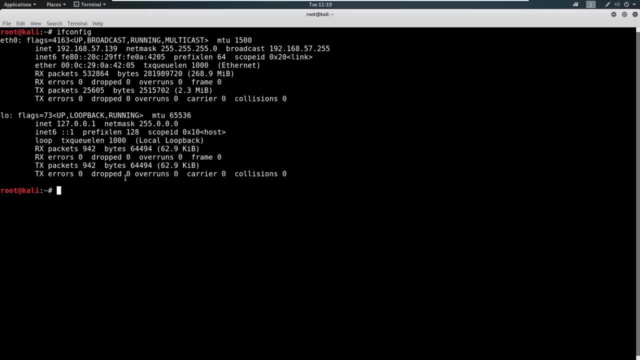 those or rent those really from your ISP, your internet service provider. So, going back to this thought we have a Class C address, my network's Class C, 192, 168, 57, 139 here, So it falls into that Class C. I've got all these devices on this 192 168 network. all these devices are 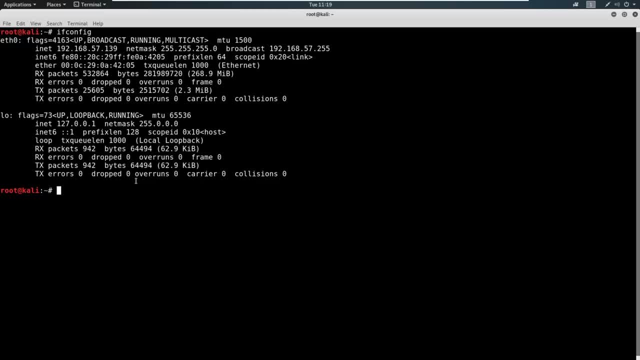 talking out of one IP address. that is my public IP address, That is what I rent from my ISP And all this network traffic goes out one IP. So this is how we have achieved or solve the issue of running out of address space without having to use IP v six, not that there's anything wrong with. 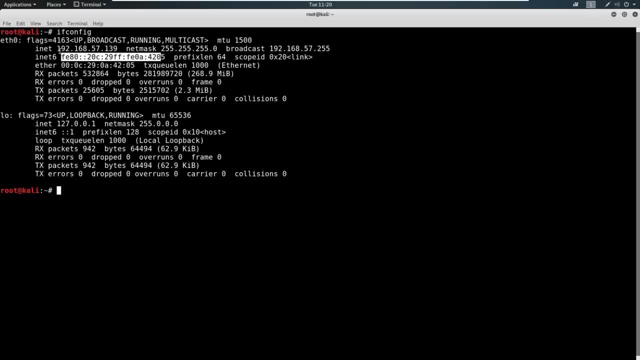 IP v six. It's not pretty. I mean, it's way easier to type this stuff in then it would be to type something like this in: But, at the same time, this is how we've solved it, we've, we're able. 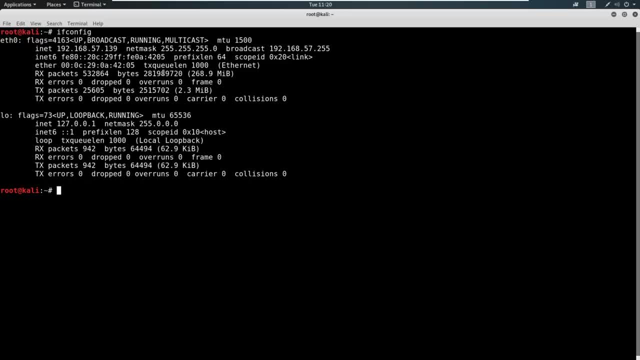 to still use IP before in mostly all networks And we are able to communicate out with this- quote unquote, IP address shortage. So hopefully that makes sense. We're going to build upon these concepts Again. IP v four, IP v six, IP addresses are layer three. 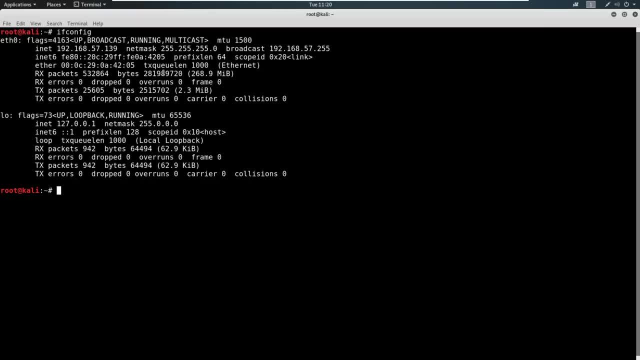 protocols. Layer three is a router. So when we route traffic, we route via an IP address. So we're going to build upon that as well as we go in. Hopefully this is all just a refresher to you. So that is it for this video. I'll go ahead and catch you over in the next one. 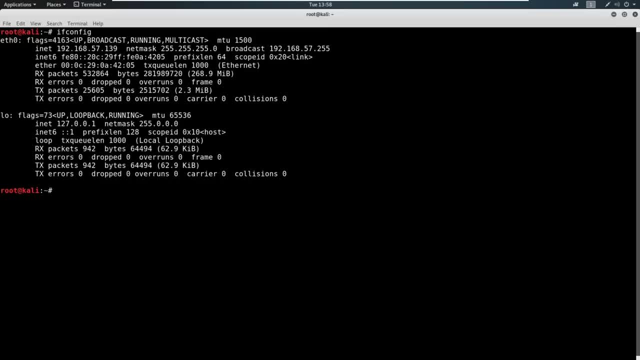 All right, so we're going to move down, Down a layer here and talk about layer two. So remember IP v four, IP v six, IP addresses as a whole. that is layer three. we're talking about routing Here. in layer two we're going to be 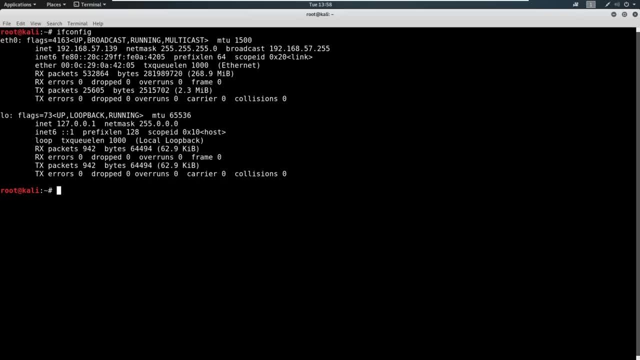 talking about a MAC address or a physical address. Now, MAC stands for media access control And that is identified here in our if config as this ether here. So we can think of this as our physical address and a way that we communicate when we are using switches. 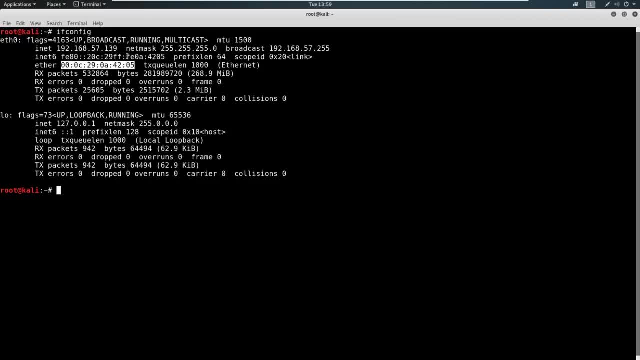 So we just communicate over this physical address. This is kind of how they know what device is what. So what we say here is: if we have a device- say you just built a computer and you're installing your network interface card or your NIC, you're going to plug that in and you're going to have 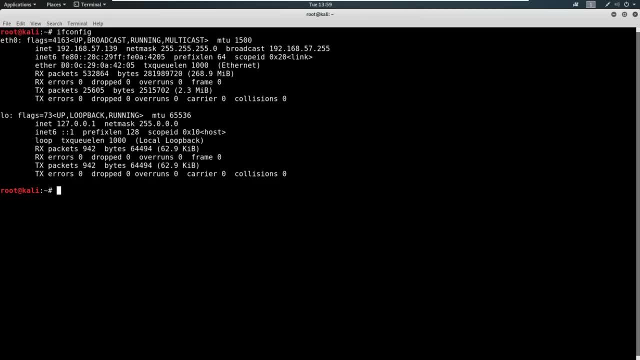 a MAC address for that NIC. your cell phone, that's going to have a MAC address. anything that's using a network interface is going to have a MAC address. So these MAC addresses are very important because they utilize layer two or switching, And they are how we communicate over. 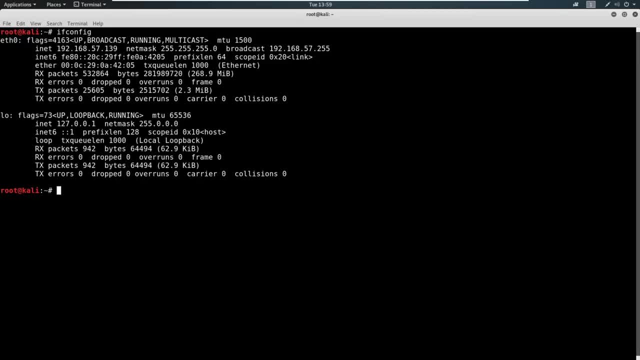 switches. Now there's something to be noted briefly about MAC addresses. Now, MAC addresses have identifiers. So, as you can see here, this MAC address has six different pairs of two, right, And what we can do is we could take the first three pairs And we can just copy this And we can go. 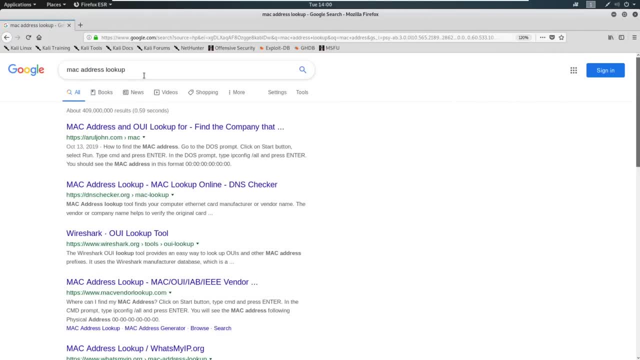 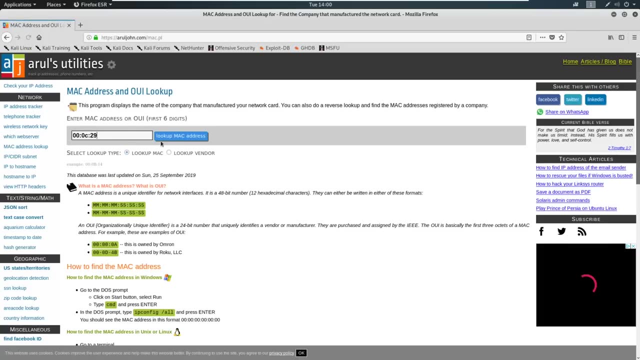 out and we can try to put it into a MAC address. Look up Now for this one. this is just going to be VMware. I'm not sure if it's actually going to come up, But I'm going to go ahead and paste it and see what happens, And you can see that the 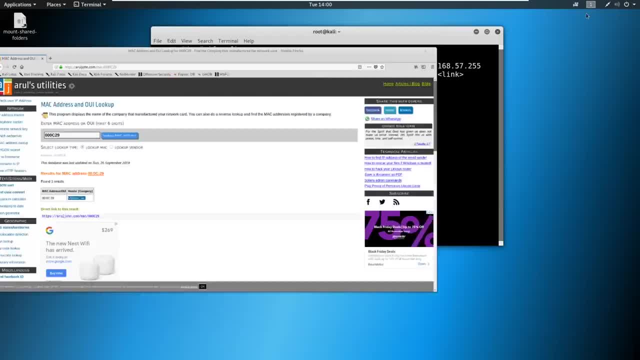 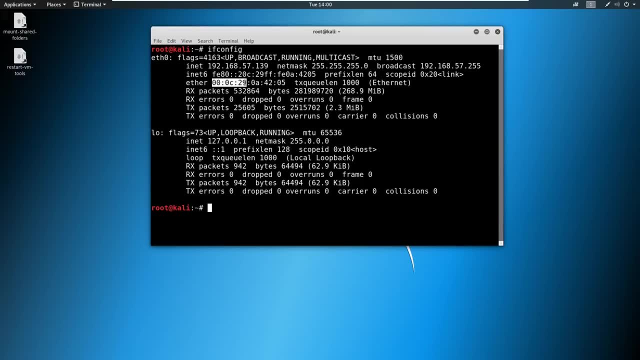 vendor actually shows up as VMware. So the first three pairs here are identifiers And we can identify what we're up against. If you've ever looked in your house and you've looked at your network and you you're trying to find a device and you see the IP address. 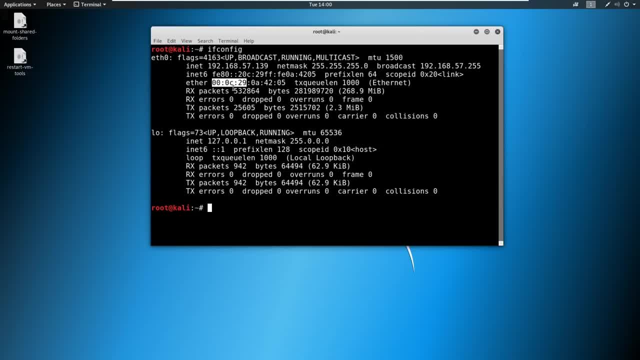 but the IP address doesn't really help you identify it. you might see something along the lines of a MAC address, because your, your home device, say your, your router, might also be what's called a layer two, slash, layer three device, meaning it's doing switching and routing for you And 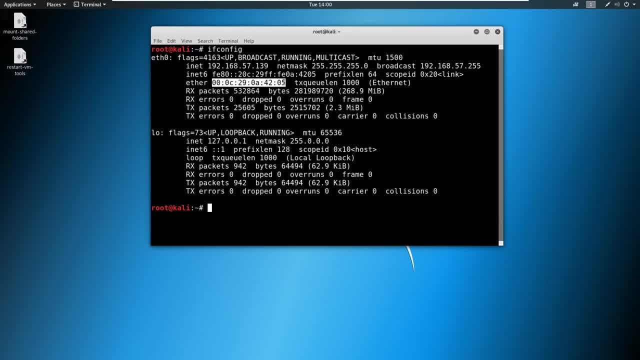 it'll also know the MAC address of that device. So you can take the first three pairs here, put those into the Google machine and see if you can identify what that device is. So if I was unsure and have a host name or device name and I could just reach out and say, Okay, well, let me look. 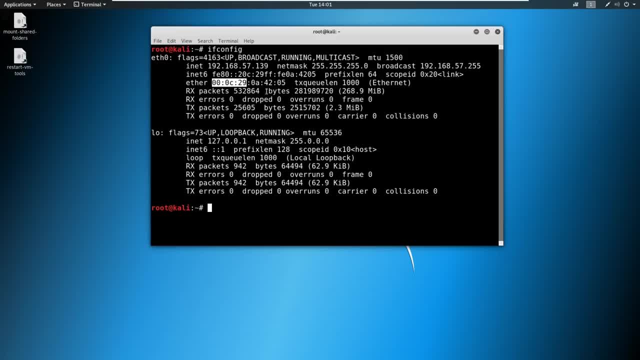 these up. maybe it'll give me an ink link. it's not going to tell me the exact device, But if I know it's running VMware then I can say: Oh, you know, that's my host machine running. Or if it's 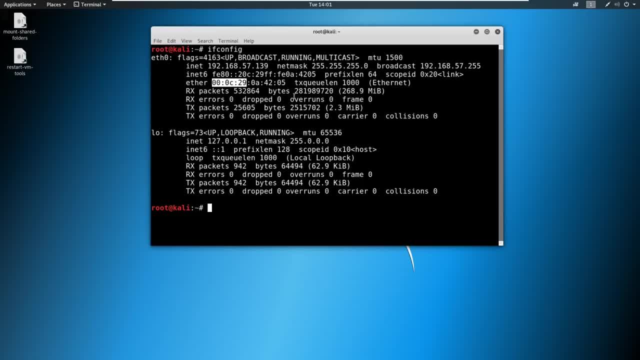 related to like Texas instruments or something maybe. I know that device in my house, So this is just a quick way to look up devices and know about them. The other option or other thing that you need to know here is just that again. MAC addresses. 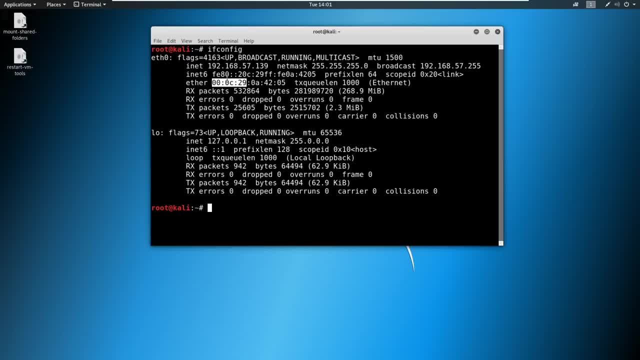 layer two related to switching. I'm just trying to repeat this and get this into your head. So that's all we need to know from this lesson And we're going to go ahead and I'll catch you over in the next lesson. 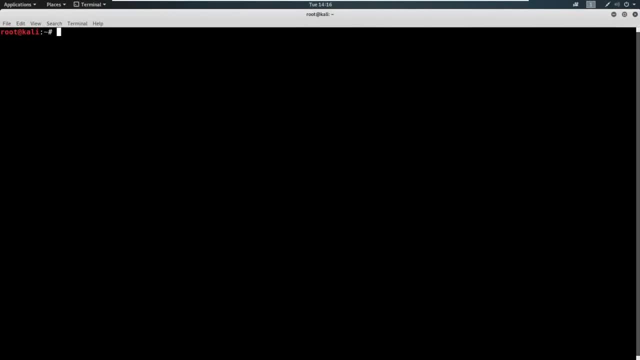 Alright. so now we're moving into layer four, which is the transport layer of the OSI model, And we're going to talk about what is TCP and what is UDP. So we'll type that in here And then we're going to type in TCP versus UDP. So TCP is what is known as the transmission control protocol, And 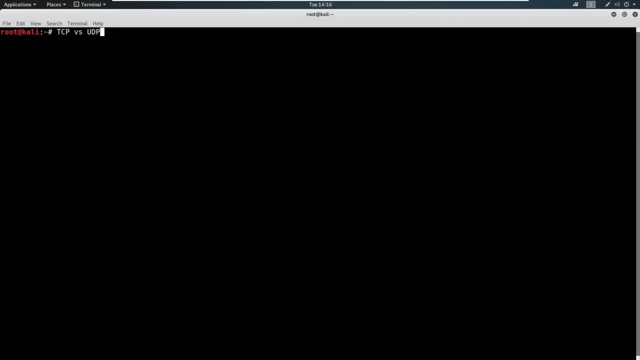 you could think of that as a connection oriented protocol. And we also have UDP, which is the user datagram protocol, And this is a connection less protocol. So when we have these two protocols, one is best suited when it comes to high reliability, That's TCP. TCP is connection oriented. we want to 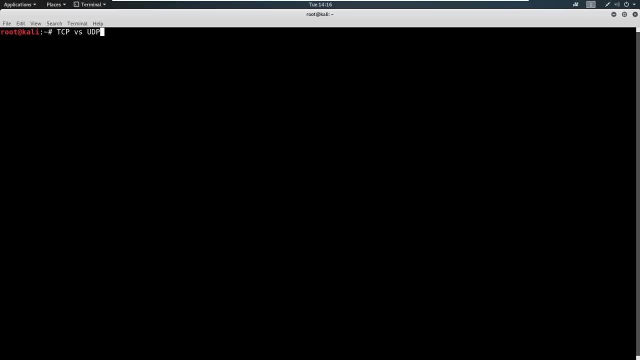 make a connection oriented protocol. So we want to make a connection oriented protocol. So when we need a connection, we need high reliability. So you can think of something like a website which is HTTP or HTTPS. Or you can think of something like SSH or FTP, the file transfer protocol, those all 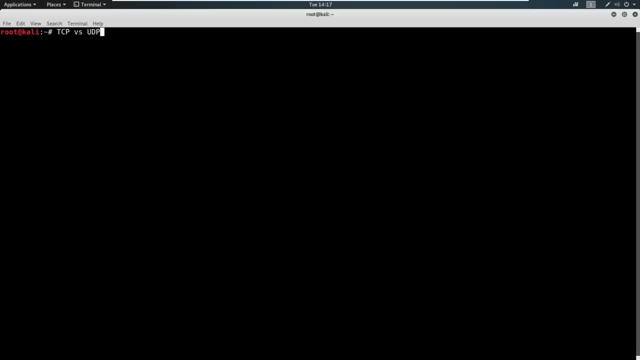 utilize TCP. When you think about UDP, you might think about something like a streaming service that's connectionless, or DNS is connectionless or voice over IP is connectionless. And when this comes into the importance of scanning, scanning is super important. And when you think about 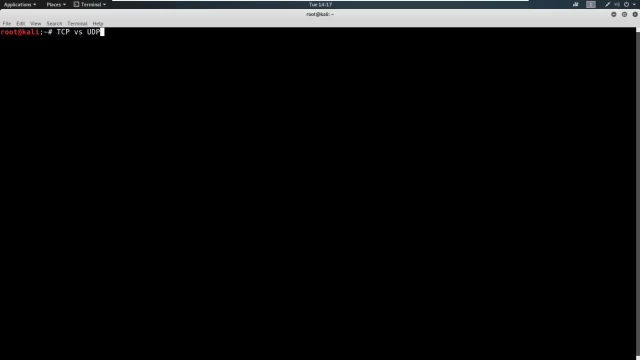 TCP, you might think of something like a UDP. So we're going to be scanning both TCP and UDP as a penetration tester, And don't worry about scanning. this is going to help you a lot, But you want to make sure that you're not using these two. 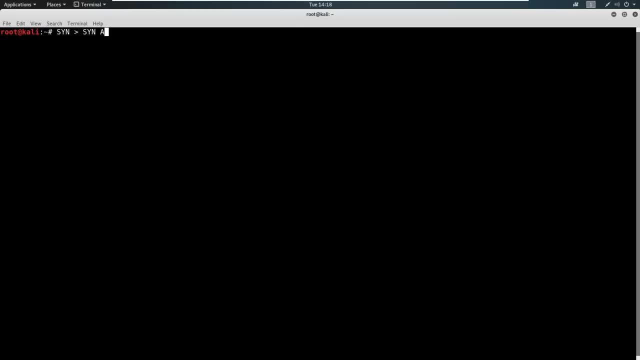 and not using the same thing. But once you've got all of these two, we'll send out a SYN packet, and then we're going to receive back a SYN ACK packet And finally, we're going to send an ACK packet. Now, how does this work? Now, you can think of this as an interaction. So let's say you have a 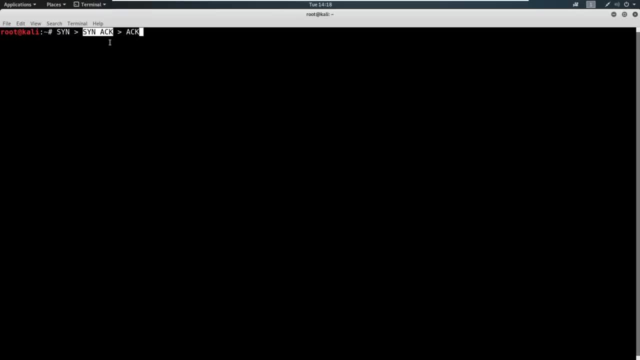 friend or a neighbor and you go to your neighbor and you say: hello, that's a SYN. Now SYN ACK is going to be the response that's going to say: Hey, SYN, I acknowledge you, that's your neighbor waving acknowledgement. now, when we think about this in the terms of ports- now, port is a item that can- 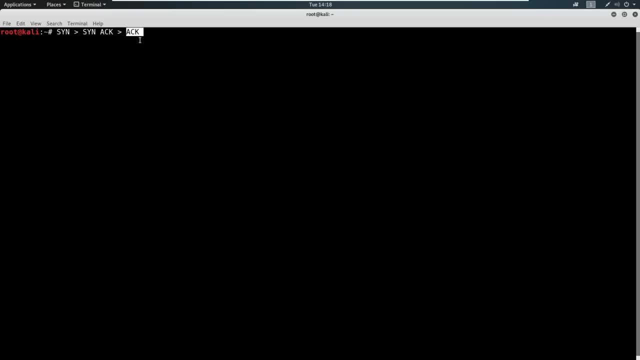 be open on a machine. it's a way to communicate with certain protocols. for example, if you think about http, that's over port 80.. if you think about https, that's over port 443. there's a lot of different protocols and there are 65 000 plus ports that can utilize these protocols. so everything. 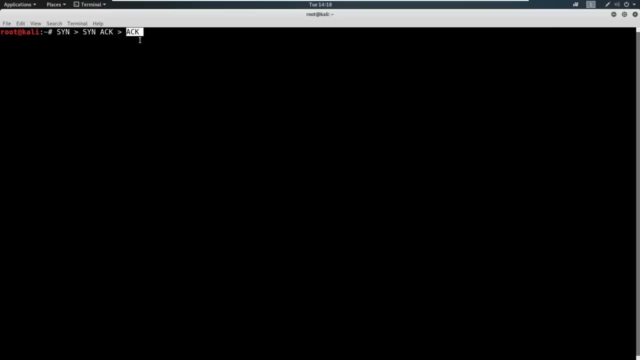 related here is has to do with these ports. now, let's say that you want to connect to port 443 on a website. you're going to send out a syn packet to that website. you're going to say: hey, i want to connect to you on port 443 and if 443 is open and available for connection, 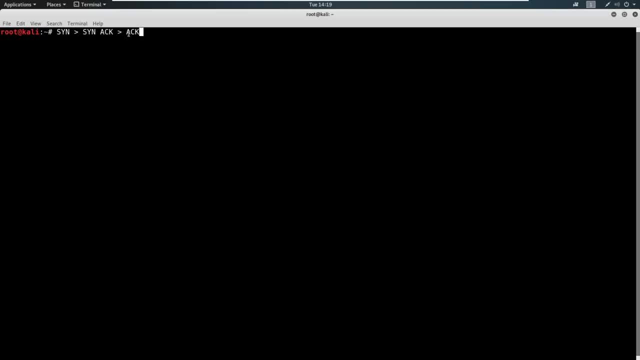 they're going to say: hey, you can go ahead and connect to me, and when you want to actually establish that connection, you're going to send that acknowledgement packet back. now let's make more sense of this. let's go ahead and open up a tool called wireshark. so this is built into kali linux. i'm just going to type in: 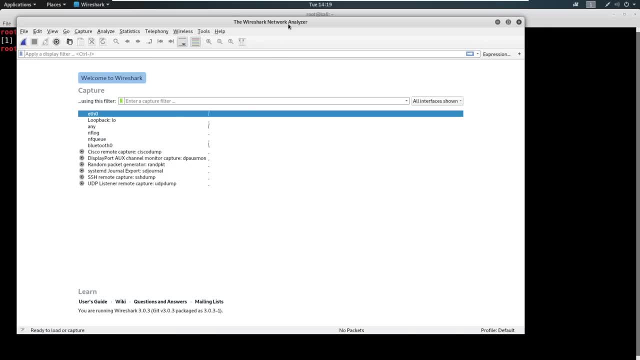 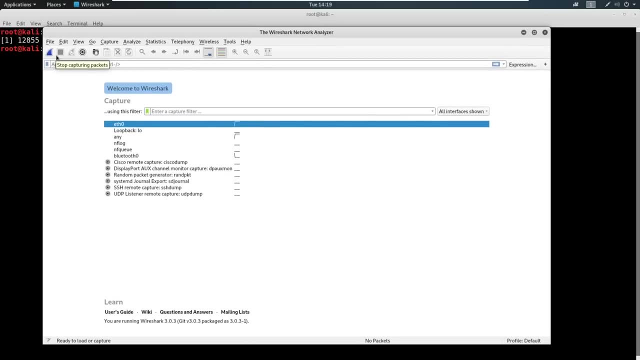 wireshark and i'm going to provide an ampersand here just so i have shell access if i need it in the background, and all i'm going to do is capture packet data. so this is going to be listening in on my nick and it's going to say: hey, what's he doing? let's capture all that data. so we're going to. 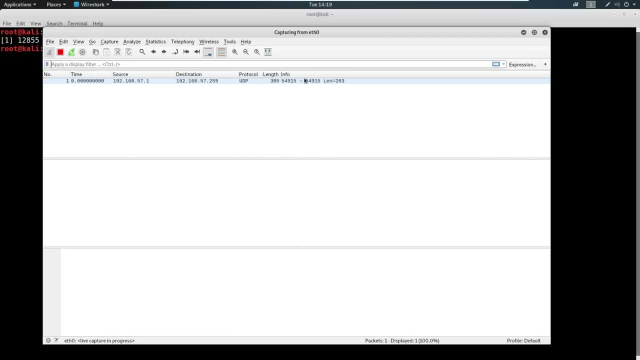 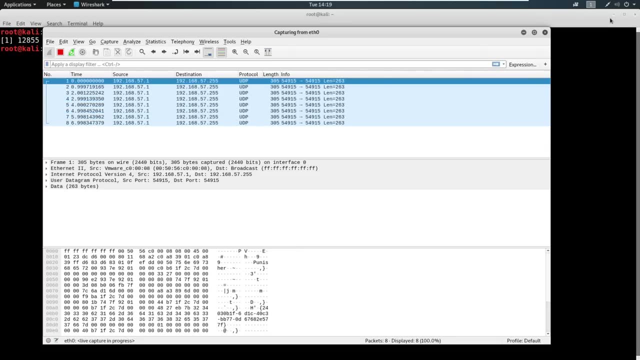 capture that. i'm going to start a capture here. you're going to start to see a bunch of traffic coming through. you can see the different protocols here. you can see udps coming through right now, but we're going to go establish a tcp connection. so let's go out to the world wide web, and i've got google up. i'm just going to refresh google. 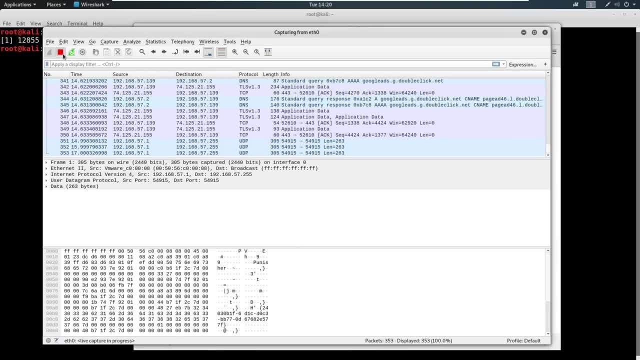 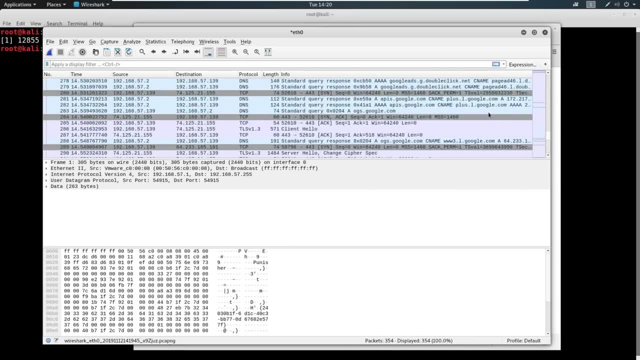 you're going to see a lot of traffic start coming through, so i'm going to go ahead and just stop this right here. look at all the data packets that get sent when you're using your computer. this is what's going on in the background. you don't even think about it. so we could. 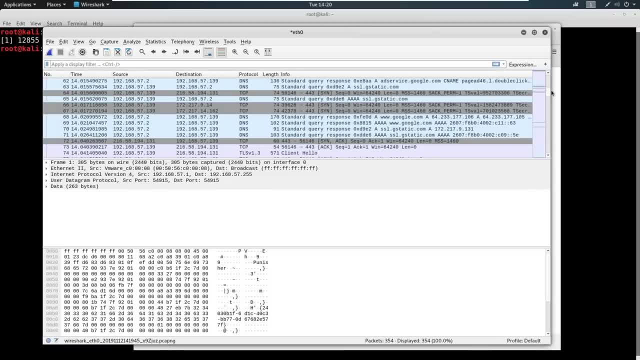 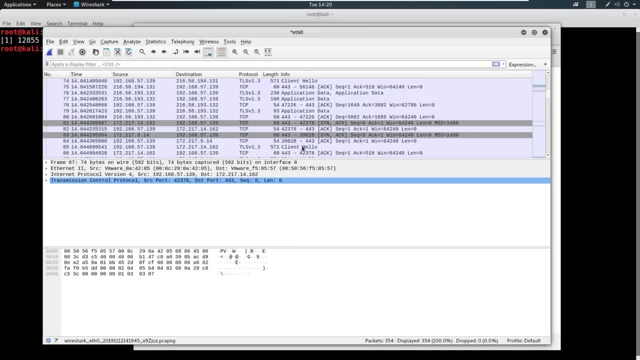 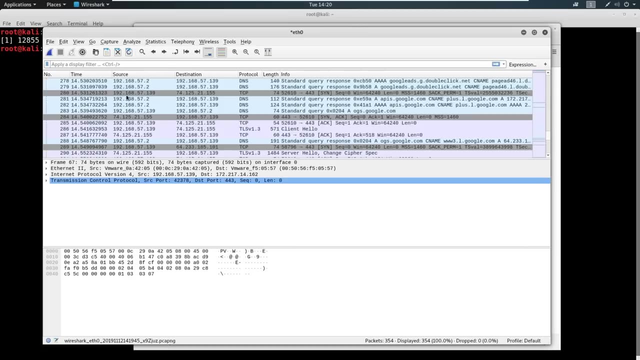 see some sins and acts there. those are in the gray. let's see if we could find a good one. okay, so here is one right here. um, so what we're going to do, actually, let's find a better one. so we're going to come down to here and we're going to say, okay, so here we are, we're our source ip. this is 192 168. 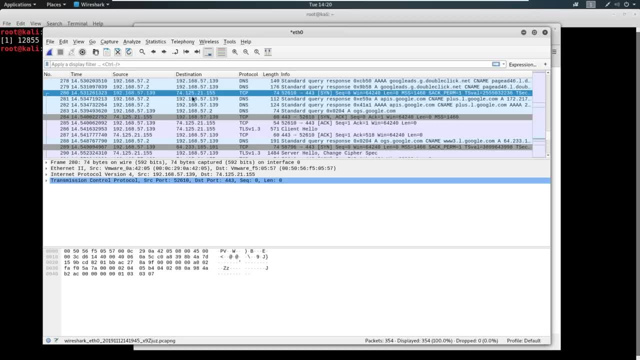 57 139. we're going out to destination of 74, 125, 21, 155. we're saying, hey, i've got this port here. i want to connect to your port, so port 443. this is a web page. we're sending a sin packet. 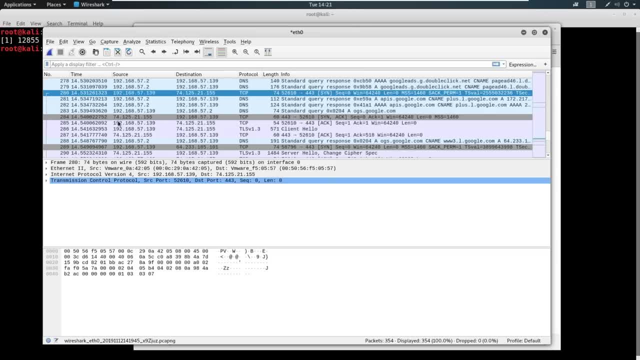 port is open and available for connection and communication. what's going to happen back is that ip address is going to say: hey, here i am, i'll allow you to connect on this port and if we make that final connection, we're going to go ahead and send the act packet back. 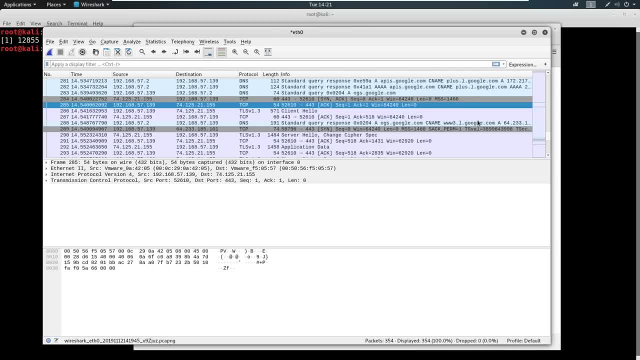 which is right here. it's going to say ac. so that is the three-way handshake, please do remember. this is going to come back into play when we get into scanning and we'll talk about stealth scanning and how we modify the three-way handshake to actually do some scanning. 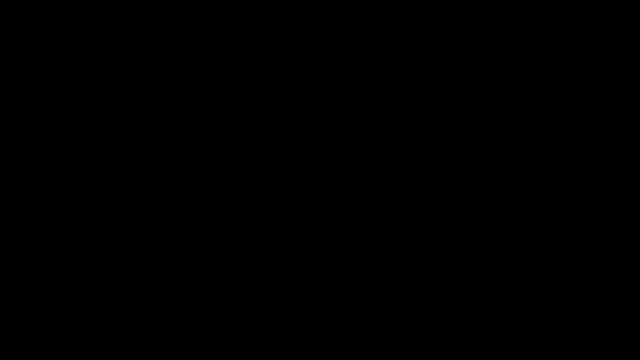 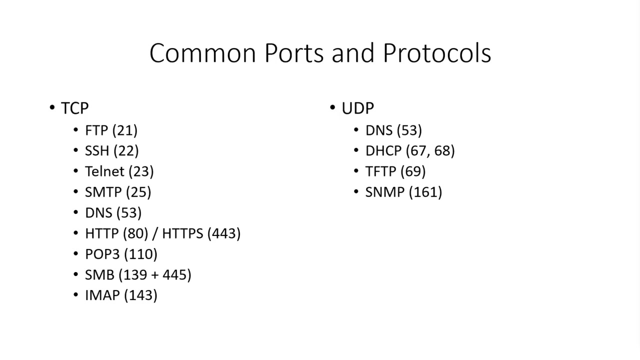 so that is it for this lesson. i will catch you over in the next one. all right, so before we go into the osi model, i do want to talk about some common ports and protocols. since this is a refresher. most of these should be pretty familiar to you. 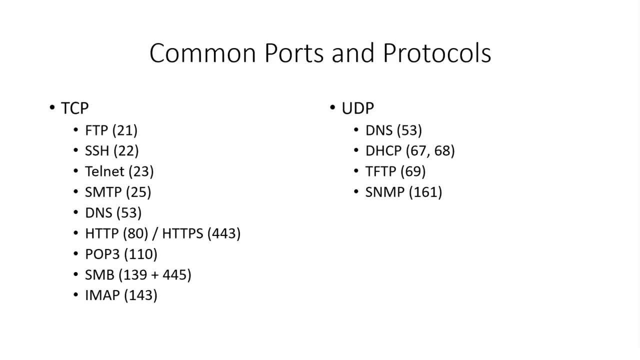 i'm going to run through them pretty quickly and just talk about them briefly on each of these common ports, and the reason i've listed these is because they are things that we'll see quite often in the future, but they're just a little bit more common and i want to start off by saying that. 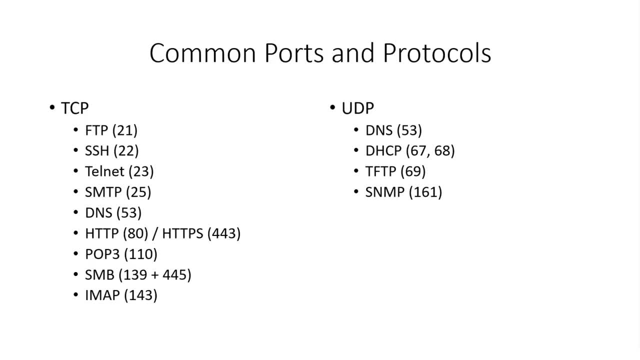 it's a pretty common port, or port 80. i'm a penetration tester and it's just something that, as we're going through the course, if one of these show up, it's something that just rings a bell and you see, you see a scan, it comes back and you see port 21. you just think, ah, yes, ftp, or you. 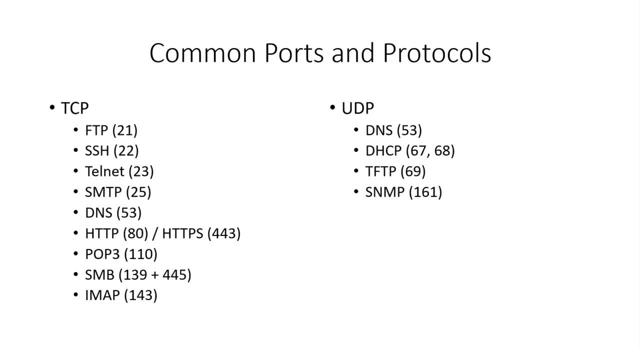 see port 80, you think, ah, yes, http, so you got to start training your mind to memorize in these ports. so when we get into our scanning- which again we haven't covered scanning- but when we get there and we see what ports are open on a machine, we're going to be able to have these common ports. 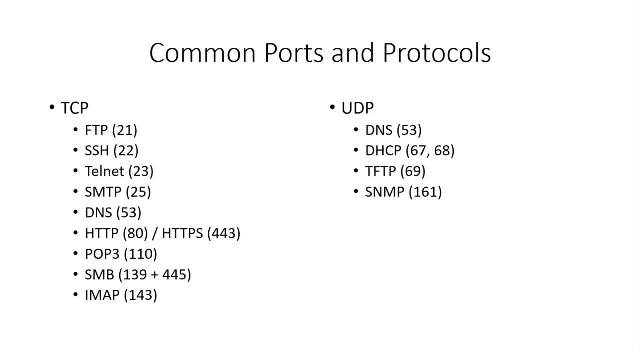 the TCP side we've got FTP. FTP is the file transfer protocol. You're going to see this in some assessments. You're going to see this a lot when we do something called capture the flag. we run through some test machines. you'll see FTP open quite a bit. So FTP file transfer protocol. 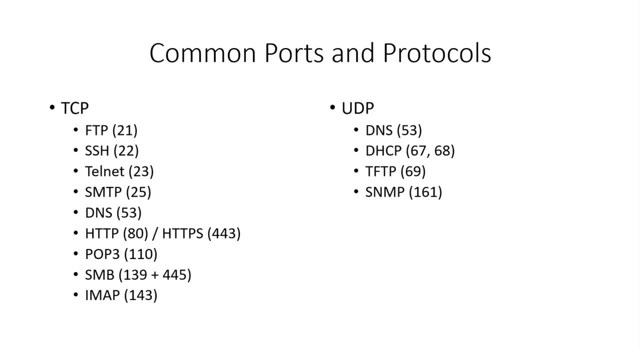 all that means is we can log into this server, we can put a file or we can get a file off the server. Now SSH and telnet kind of play hand in hand. telnet is the ability to log into a machine remotely. Now SSH does the same thing. The only difference is SSH is the encrypted version of 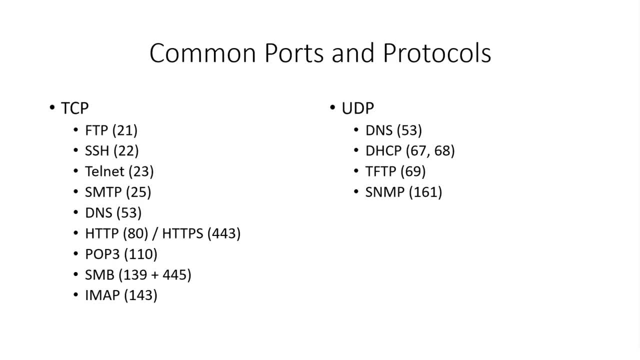 that. So with telnet you are in clear text And with SSH you are encrypted. Now SMTP, pop three and IMAP all relate to mail. we're not going to worry too much about mail in this course, but you might see it come back up at some point. So just remember your 25, 110 and 143 DNS. So DNS. 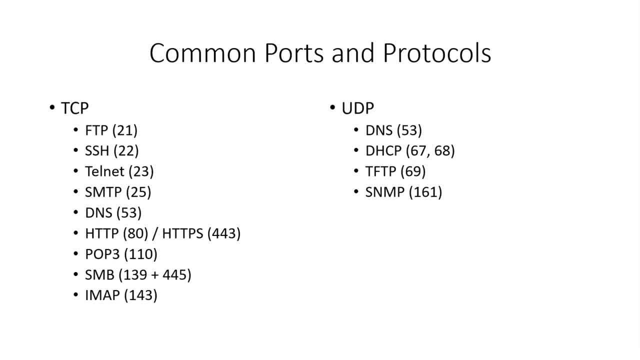 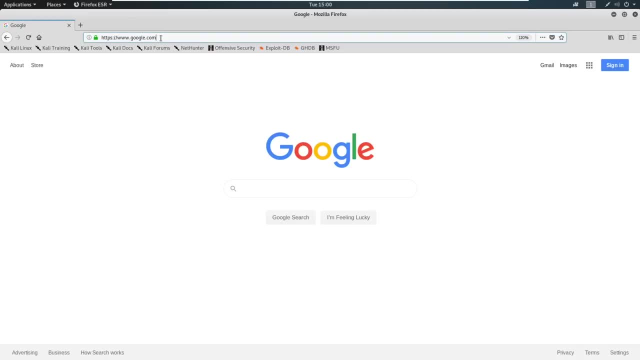 is a way to resolve IP addresses to names, And we can take a quick look at that if we go back to our Kali machine And say we're at Google, here we've got Google up, but the computer doesn't really know what Google is. the computer is just using nice texts like googlecom for us, the humans. 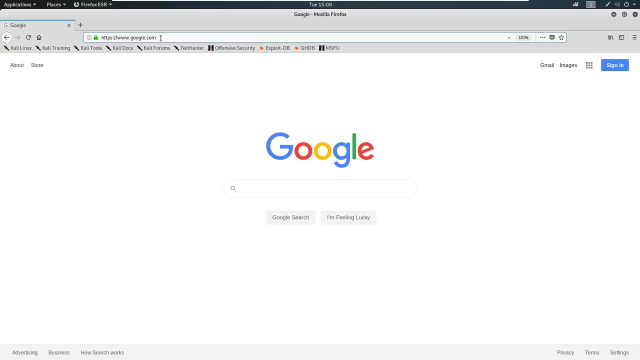 what's going on on the back end is Google actually resolves to an IP address. Now, the IP address is how the computer knows to get back and forth, Because we don't want to sit there and type it in the back end. we're going to go back to the computer and we're going to type it in the back. 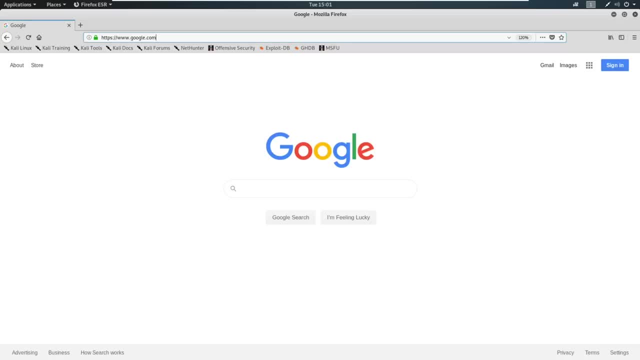 end we're going to type in IP addresses. this DNS or domain name system has been implemented for us, So we type in googlecom on the back end. it knows, hey, I want to go out to 179, 1022, 34,. 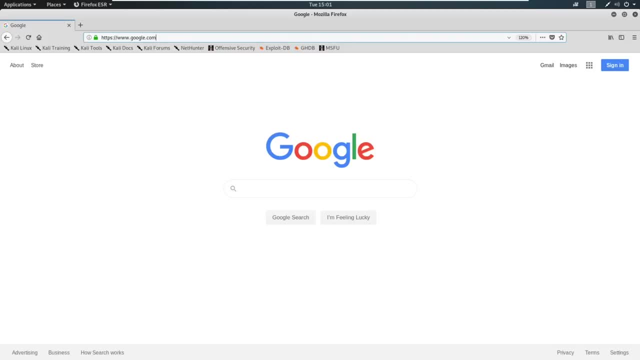 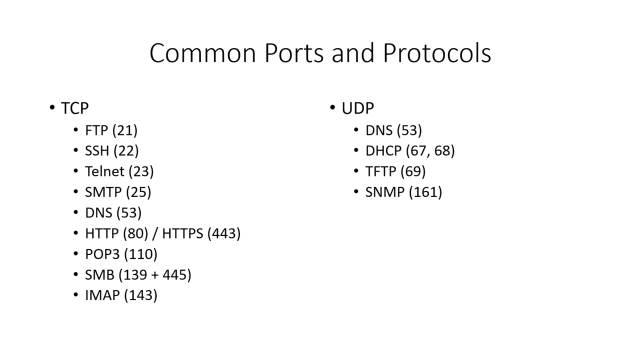 whatever it is in reality, But this is just a quick way for the computer to relate to a human and the human, to you know, have easily readable access to some of this stuff. So, going back to our PowerPoint, we have HTTP and HTTPS. That is a website, just what you saw there. Mostly everything is on 443. 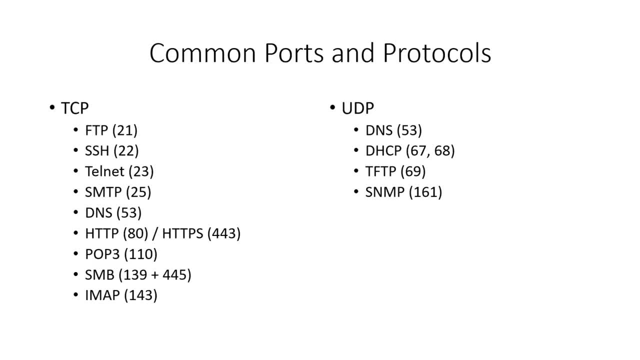 now, or HTTPS, The HTTP on port 80. You'll see, sometimes remember that is the non secure version of the protocol. So HTTPS is encrypted, HTTP is not encrypted and not secure. So, lastly, SMB ports 139 and 445.. Originally it was just. 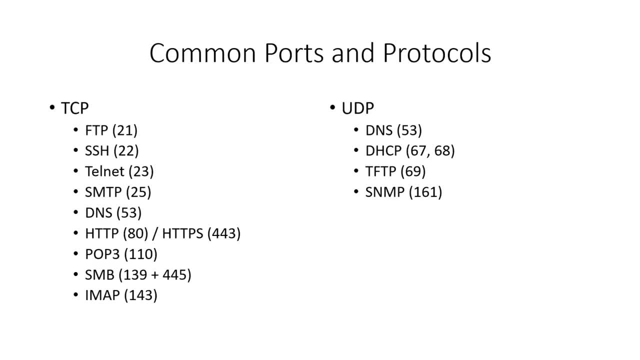 139. in the later versions of Windows they put on 445,. you're going to see these ports a lot. this is probably the most common port you're going to see as a pen tester. These relate to file shares. you might also hear this called Samba, So there are a few names for it, But when 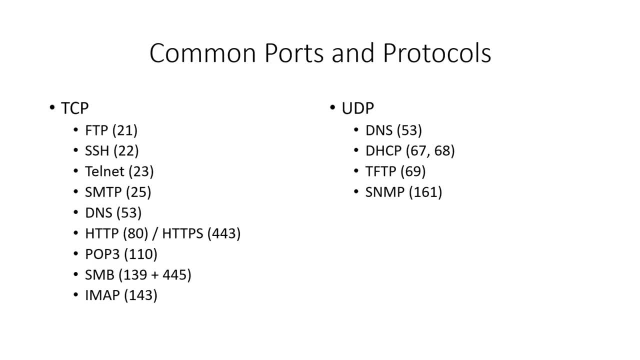 you think of SMB and you see 139 or 445, think of file shares And, as a pen tester perspective, you got to think about all the crazy exploits we've had regarding SMB. the recent one, as of this course, was the WannaCry virus. Right, So you had the WannaCry virus is. 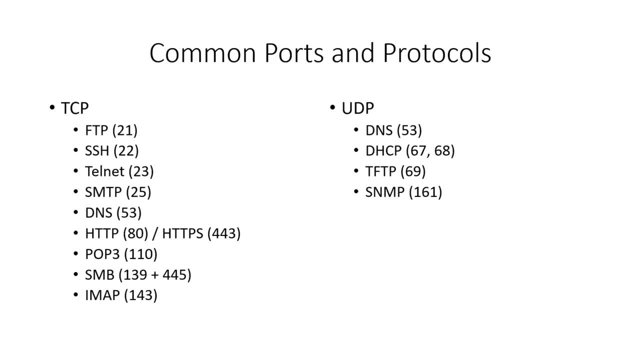 also known as eternal blue, was what it was built off of, or Ms 17 010 was the official term of that exploit. that exploit utilized an SMB exploit to navigate through networks. So it became very vicious very quick because SMB is opened so frequently on networks. Now on the UDP side, we also have DNS over this, but we haven't. we don't know where it's coming from. Let's go ahead and go ahead and hit the play button. So let's go ahead and go ahead and click the play button. Okay, that's one of the great features of the network. So we did a couple of things. Let's close. 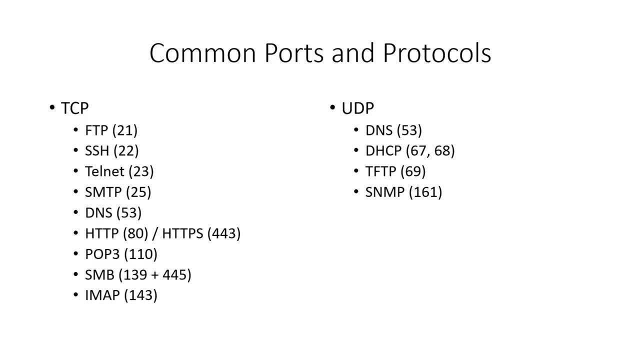 up. Let's go ahead and go ahead and click the play button. So if you want to log in over here, DNS is both ATCP and UDP protocol. We also have DHCP Now when it comes to IP addresses. DHCP associates you with an IP address kind of at random. Now you could have the opposite of that. 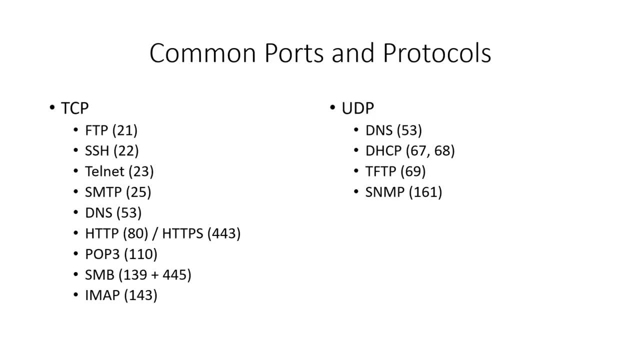 is what is a static IP address. So with DHCP you plug into your network, say your home network, and the internet just fires up Guess what? Probably DHCP on the back end. It just picks a number between a range, says hey, here's your IP address. I'm going to let you lease that out for 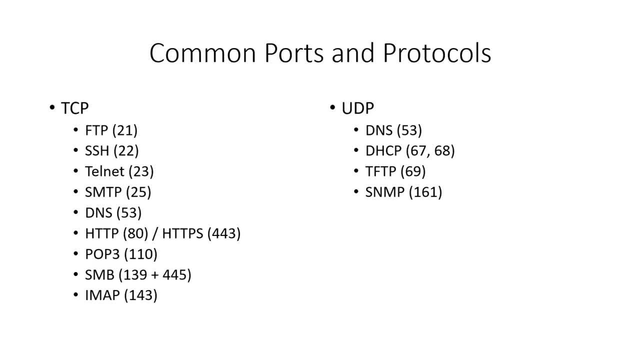 eight hours or a day or a week or however long the timing is set for, And that IP address is yours. Now the opposite of that, again, is static. So you could say, hey, I want a static IP address And anytime I plug in with this specific computer, go ahead and give it this IP address. So how are 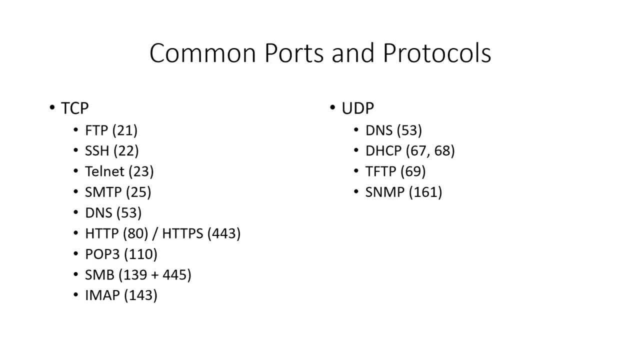 we going to know that? Most likely the MAC address, right. So from layer two it's going to know layer three and how to assign it. So again, DHCP is a static IP address. So you could say, hey, I want a static IP address And anytime I plug in. 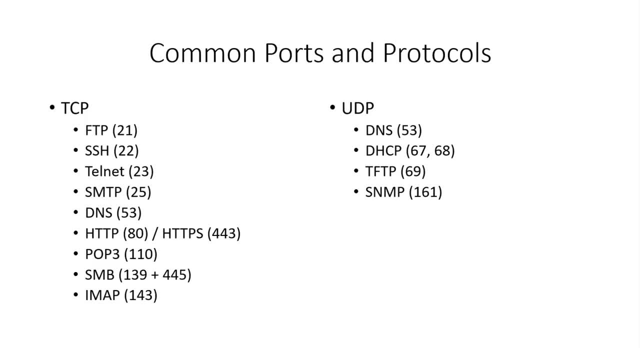 with DHCP. it should be pretty familiar to you. We've also got TFTP on port 69,, which is the trivial FTP, and it utilizes UDP instead of TCP. And we also have SNMP, which is the simple network management protocol. So you will encounter SNMP occasionally on networks, not always. 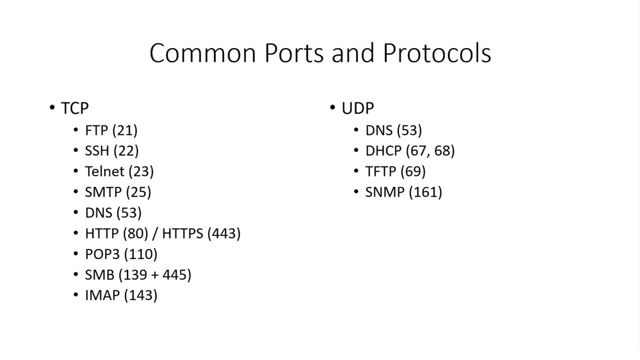 but when we do encounter it, there may be some information to be gathered, especially if there are strings being used that are community or public strings. So you could say, hey, I want a static IP address And we'll worry about that when we encounter it. but you will probably see it. 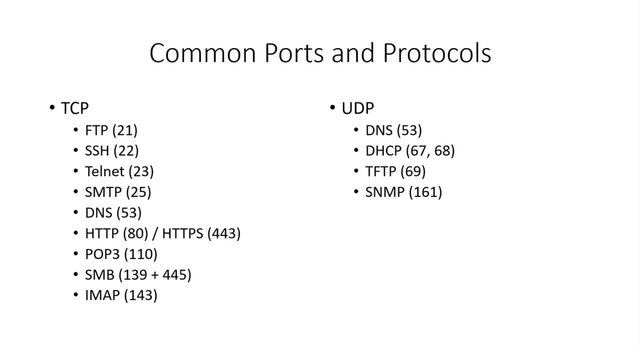 again in this course. So that is it. In this video we're going to go ahead and move on to the OSI model and tie all this together. Then we'll get into a little bit of subnetting And we'll end this with a refresher on networking. a final video on networking. So I'll see you over in the next. 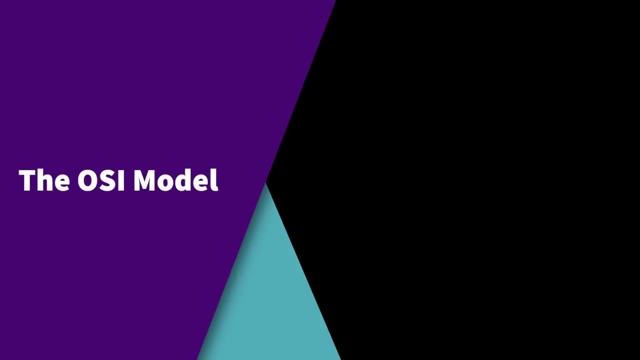 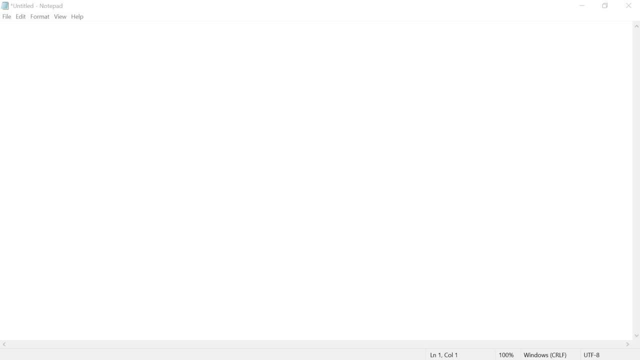 video. All right. so this whole time we've been talking about the OSI model and we've been talking about the OSI model and we've been talking, we've been talking about networking and I've been throwing terms at you And I every. 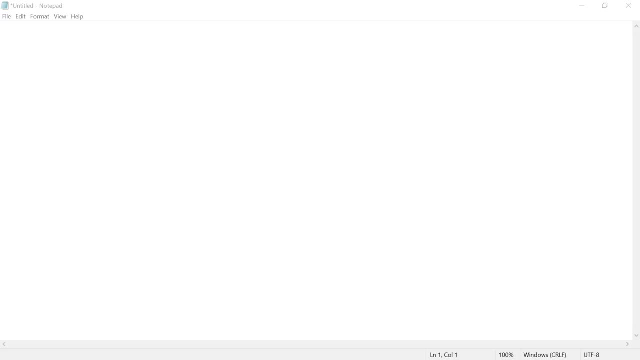 time I throw a term at you, I try to use the respective layer for it. So you've heard me say layer two, layer three, layer four, And those all correspond with what is called the OSI model. Now, if you're ever in a network interview or if you're ever talking to somebody who has 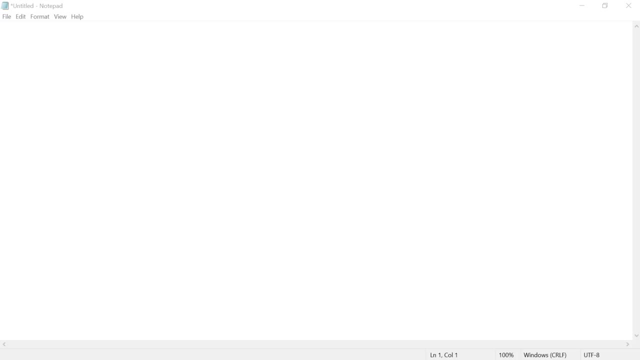 experience in networking, or even if you're on the help desk taking tickets, knowing the OSI model is incredibly helpful, And people will just throw layers at you, especially the people who have been in the field for quite some time might just say layer two. 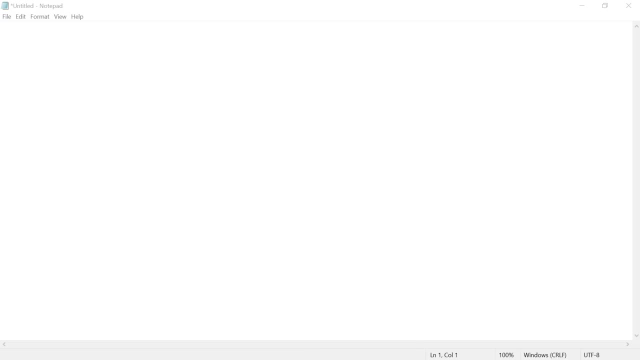 instead of a switch, or they might say layer three instead of a router. So I'm going to discuss the OSI model really quickly, give you a mnemonic on how to remember it and just talk about some of the concepts within it and how to troubleshoot down as well. So I picked this up. 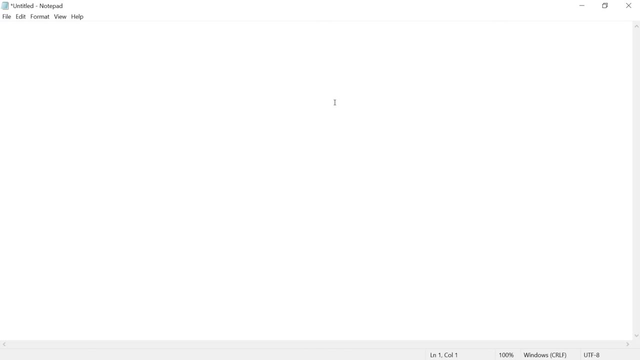 from Keith Barker a long time ago And he said: I'm going to talk about how to troubleshoot down a long time ago- Great trainer, by the way, And this is the mnemonic. So we're going to go P, D, N, T, S, P A, And this stands in my head, for please do not throw sausage pizza away. 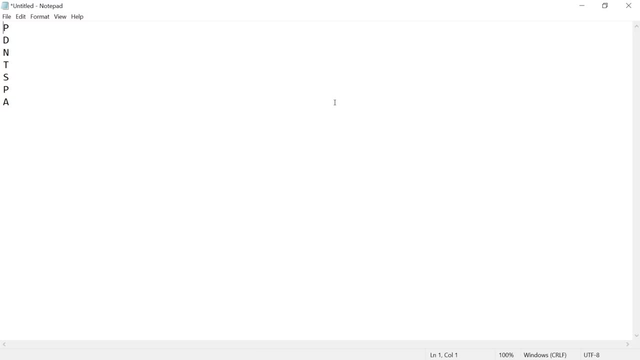 Again, that is, please do not throw sausage pizza away. So I'm going to put numbers corresponding to the layers in front of it here And we're going to go ahead and type these out one by one. So on the first layer here we've got what is called the physical layer. 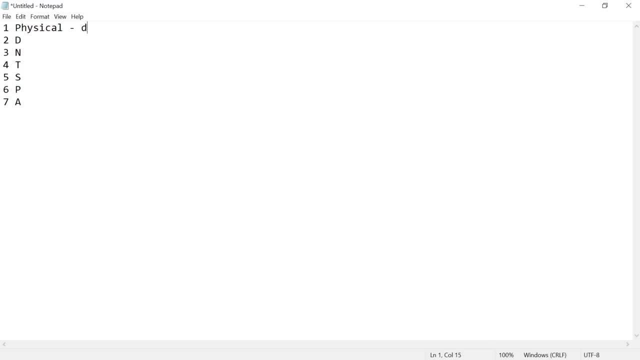 And you could think of your physical layer as like data cables or like your cat six cables, stuff like that, something you might, you might plug in right, That is the physical layer, And we've already talked about layer two quite a bit. Layer two is the data layer And that is our. 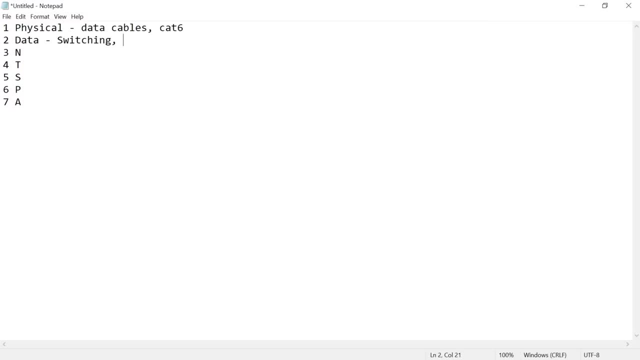 switching Right And we're going to go ahead and type in the data layer And we're going to go ahead and type in our session And also our MAC addresses Going down the list. we've got the network layer, which is IP addresses Also routing. The fourth layer is the transport layer. 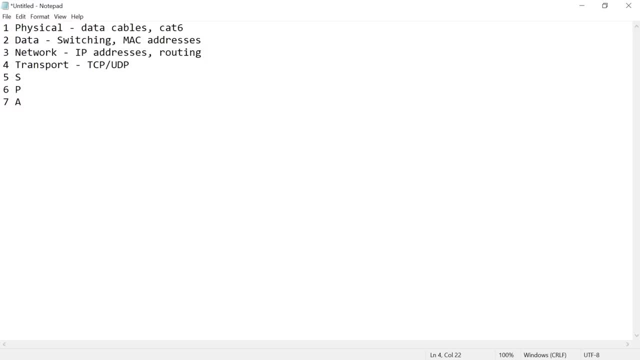 which is TCP, UDP, which we have talked about as well, And the last few. So the session layer. we've got the session layer, which is just session management. you don't really have to too much about this. one Six is the presentation layer. Now, this should be familiar to you because 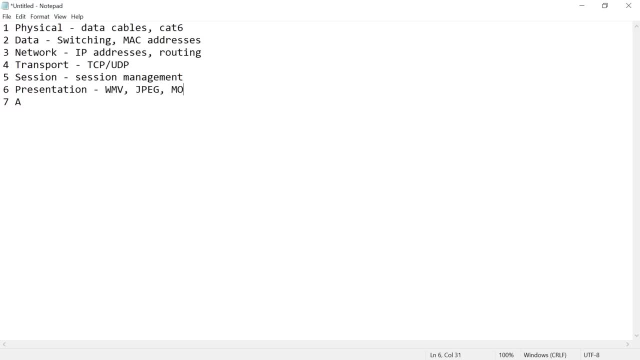 think about WMV, JPEG movie files. that's what your presentation layer is, So media. And then, lastly, we've got the application layer, which is like HTTP, SMTP, your applications that you utilize, right. So we've got this laid out here And you might be asking: why is this important? 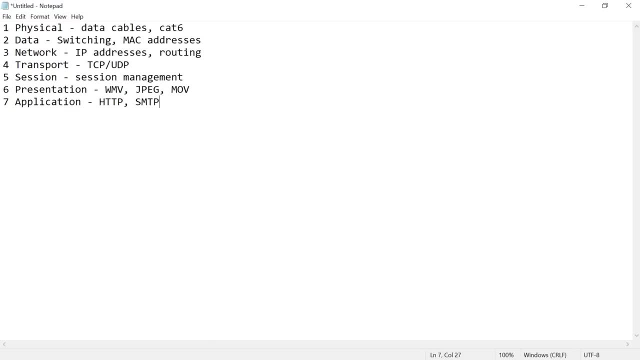 Well, again, when we say something like my home router is a layer two, three, So that means it does. It does switching and it does routing right, You might think of this in another way as well. you might be asked to troubleshoot- And something to talk about too- with the, with the. 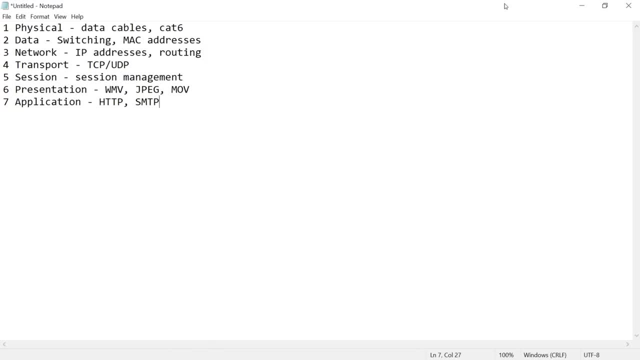 OSI model is: when we receive data data, we receive data down this physical layer all the way down to the application. When we transmit data, it goes out the application layer down to the physical. When we're troubleshooting this, it is always best to start with the physical and go down to the application level. Okay so. 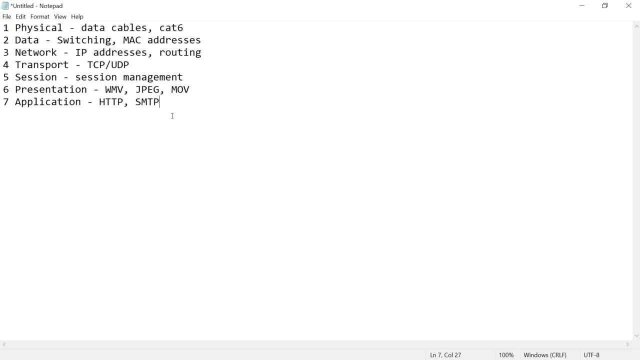 say, you get your working help desk and you get a phone call and somebody says: you know my internet's not working, help me. Well, what's the first thing you're going to do? Are you going to ask them application? 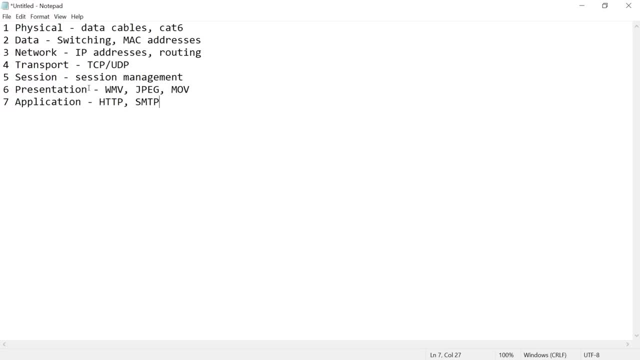 Level questions. Yeah, probably not. You might say, Hey, can you look at the back of the computer? Do you see a? the cable plugged in? Oh, the cables plugged in. Okay, well, do you? do you see the the? 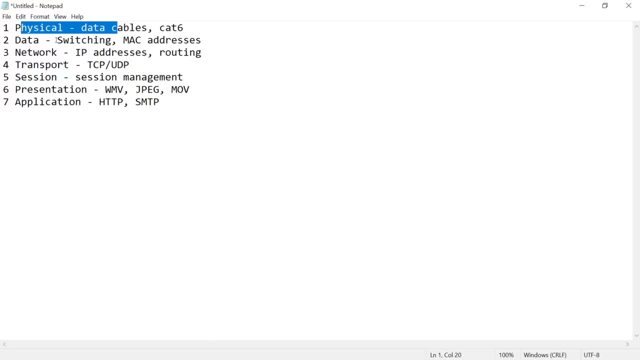 where the cables plugged in. Is there a blinking light? Is that blinking like green by chance? Okay, we're checking the NIC right And then we might ask them to you know, do they have an IP address? What's going on all the way down and then we troubleshoot all the way down to layer. 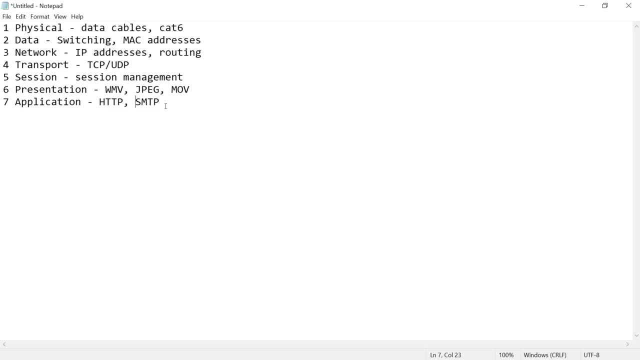 seven, So we wouldn't start on layer seven. So we wouldn't start on layer seven. So we wouldn't start on layer seven, right, we would start from the basics and move down. So it's important to know this. This isn't a help desk course by any means, But it's super important to know this especially. 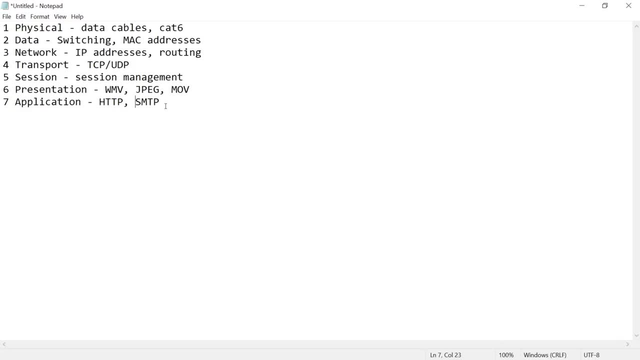 if it's been a while since you've seen this network stuff, or even if this is new to you that the OSI model is commonly referred to. even as a pen tester, I get all kinds of layer two, layer three talk and you will be sitting in meetings with network engineers. 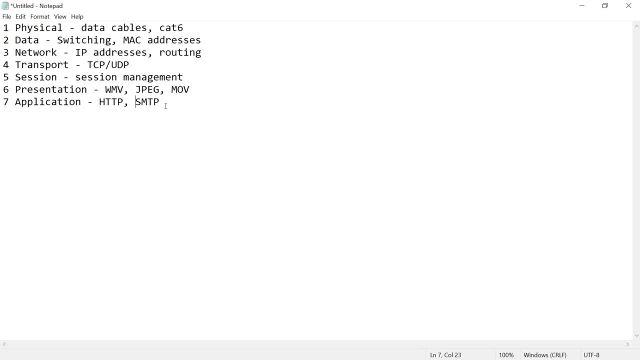 with people who are very, very smart about this stuff And they're going to throw all this link go at you. So, if you know, this lingo really, really benefits you, or else you're just going to sit there and wonder what the heck they're talking about. So hopefully this is a quick. 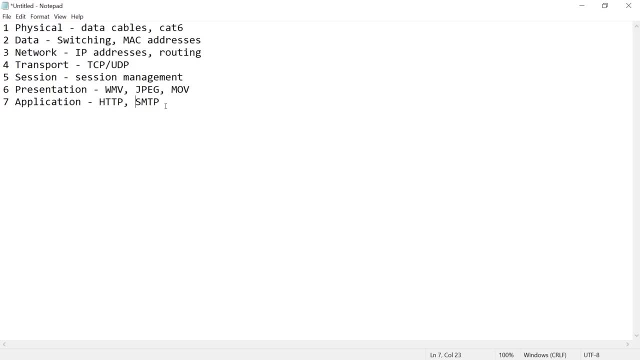 informative method for you. And again, remember, please do not throw sausage pizza away. That's the easiest way that I remember it. You can make up your own mnemonics if you want. People have other things as well. If you've got a, you got a favorite mnemonic. please feel free to comment down below. 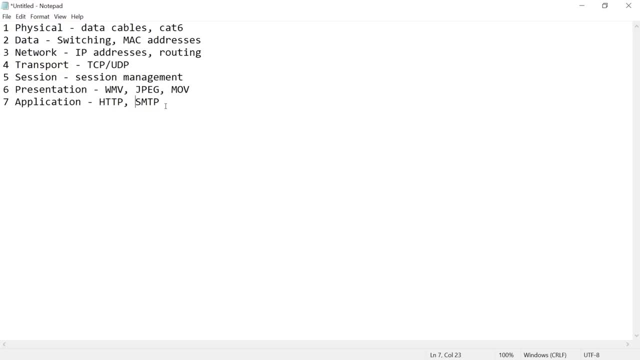 and tell me your mnemonic as well. So I'd love to hear some of these other ones. So let's get started, Let's get started. So, let's get started, So, let's get started, So, let's get started, Let's go ahead and move on into subnetting, And then we'll we'll start moving into other fun parts. 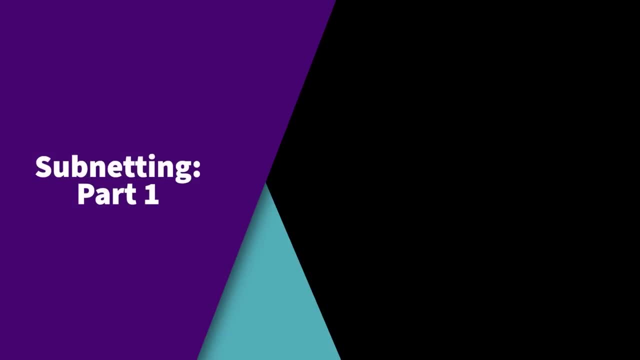 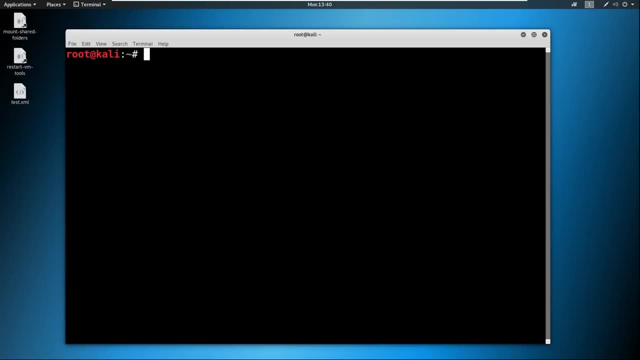 of the course. Let's talk about subnetting. So subnetting is important in networking. you hear about it all the time. you hear even people perhaps freaking out. I know I freaked out when I heard that I had to do it for exams like network plus or CCNA And I feel like there are a 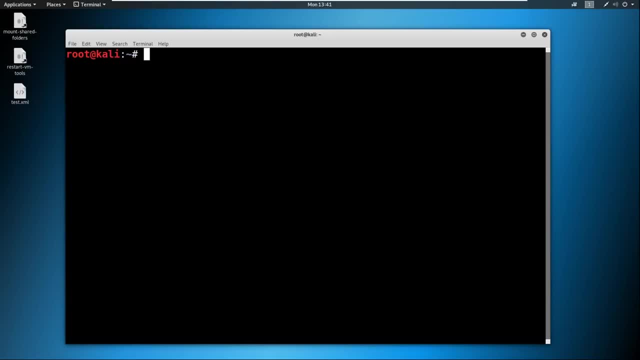 lot of complicated methods out there for subnetting, But there was a method that was shown to me middle of my career And it just blew my mind. It's really, really fast subnetting method And I really want to break down for you what subnetting is, why we do it, and then show you the methodology. 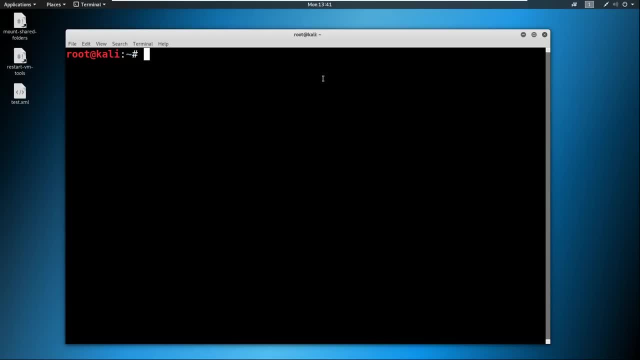 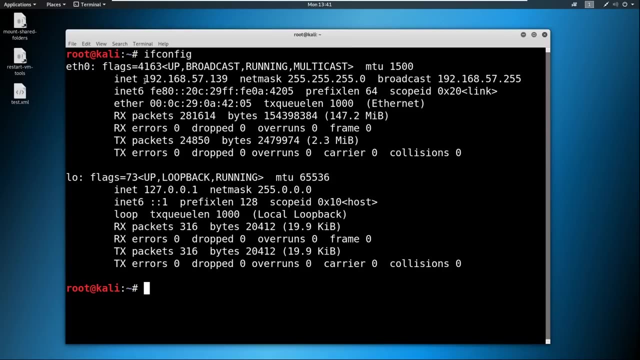 behind it. So if we want to talk about subnetting, if we just come in here and just do an if config and we look at our IP address, right, we have our I net, which is our IP v5, four, And you can see, here too we have this net mask. this is also known as a subnet mask or a. 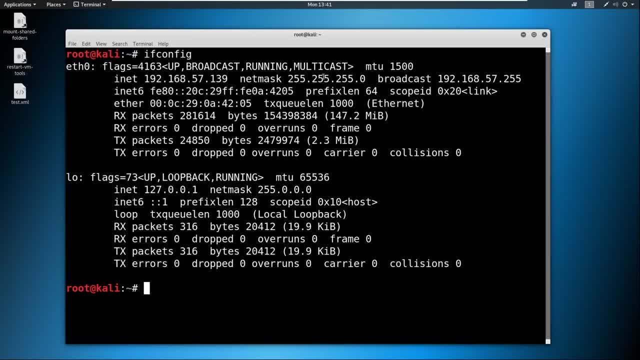 subnet And it just says 255, 255, 255.0 doesn't really tell us a lot if we don't know much about it, But this is what a subnet looks like, And we can think of subnets in ones and zeros. It's all. 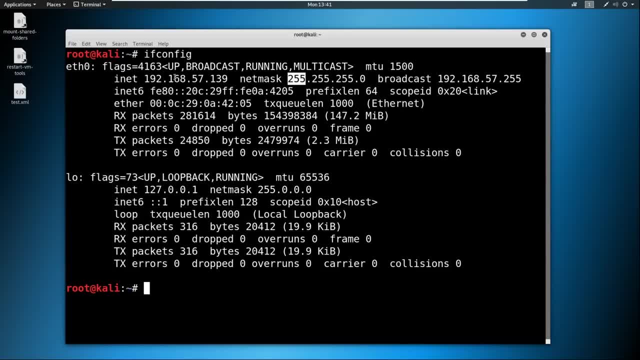 bits, right. So we've got eight bits here, just like an IP address, IP before, same thing. eight bits, eight bits, eight bits and another eight bits, And we've got ones and zeros. if all the ones are switched on, we've got 255.. If none of the ones, 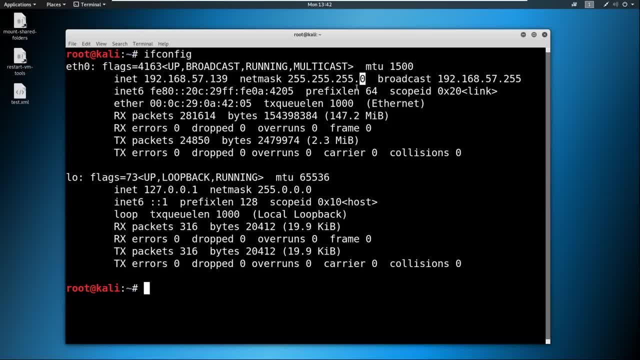 are switched on, we've got zero, And depending on how those ones and zeros are switched on or off determines a lot of things for us, And that's why this net mask is important. Now, attached to your resources for this course, I've created an Excel sheet that I think will be useful. So if we look 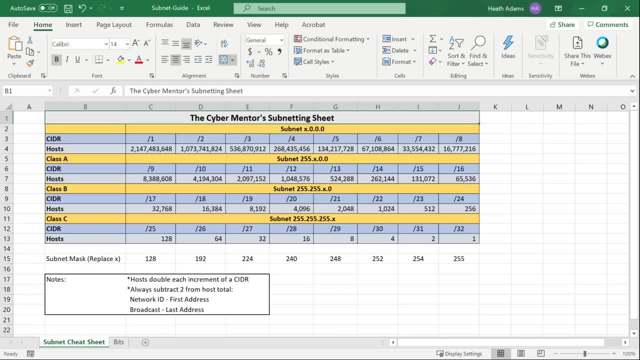 at the Excel sheet. here is the cyber mentors subnetting sheet And let's talk through this. a bunch of numbers and might look crazy for you And we're going to talk about how this breaks down, how the bits break down, and then how I would write this short handed for an exam or tests or just 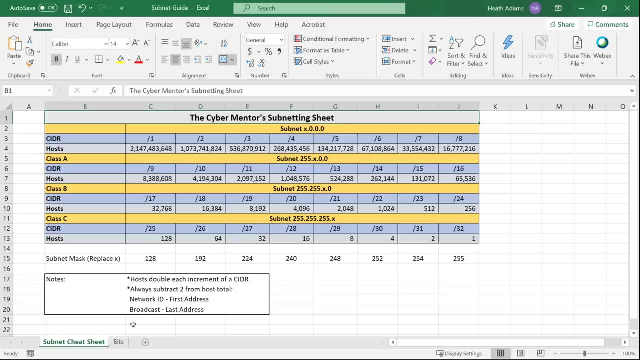 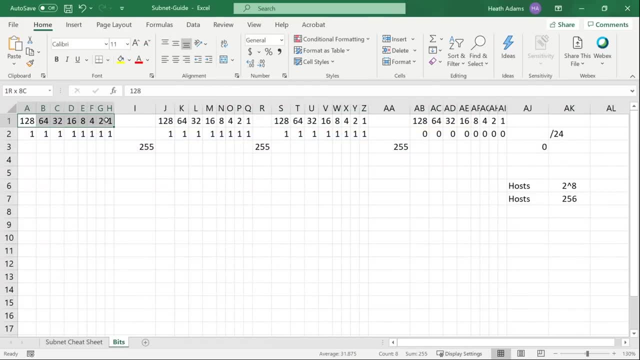 something that I do on a day to day basis. So first let's talk about the bit. So come to the Bits tab here And we have our eight bits right. we can count this across And there's eight here on the count You can see that and it starts with 128 and descends down to one. you just keep cutting. 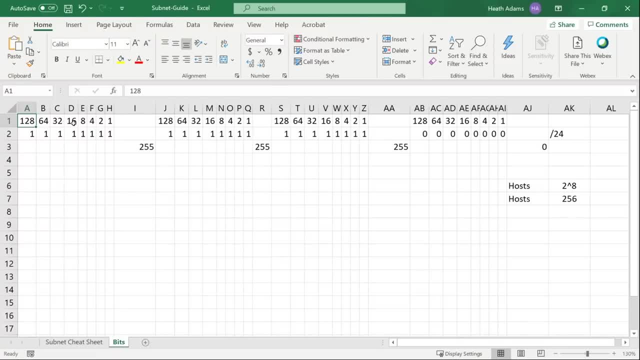 it in half right. So 28,, 64,, 32,, 16,, 8, whatever. What's more important is why we get to these numbers. So if we have a one switched on here, it adds to the value. When all the ones are switched on, it equals to 255. 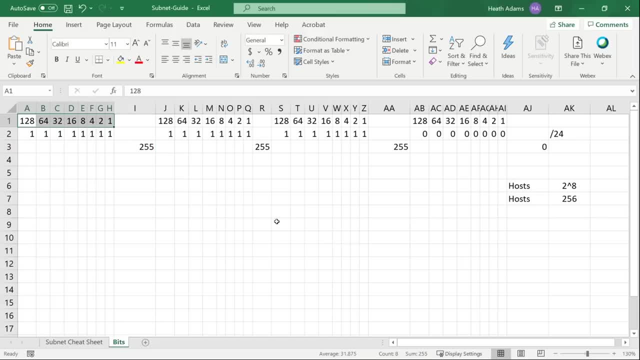 You see all the ones switched on here. If we were to highlight over all this, come down to the sum, you see the sum is 255.. That's all this formula is doing here. So if we were to come through and you see all the zeros here, nothing's flipped on to actually turn any value on here. How this? 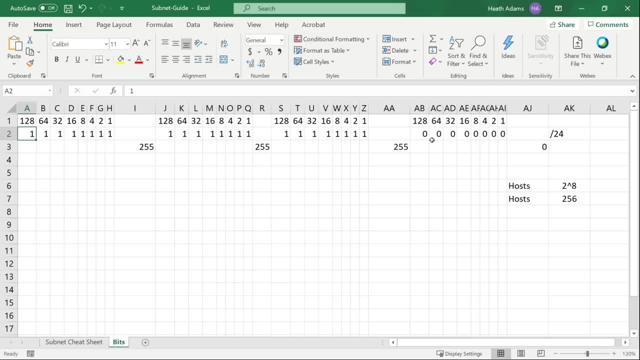 actually works is the switch has to be on in order, right? So if we were to switch on another bit, we'd have to switch it on here And we'd have to switch another one on here. We couldn't just come down here and switch it on here. It wouldn't make sense. It doesn't work that way, not with. 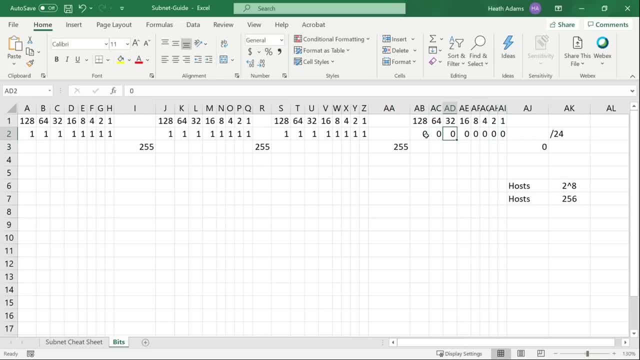 subnetting. So we're going to take these back off and just show zeros again. But you see how the values change If, for example, we had this network and you saw the default. and I'm showing you the 255, 255, 255. 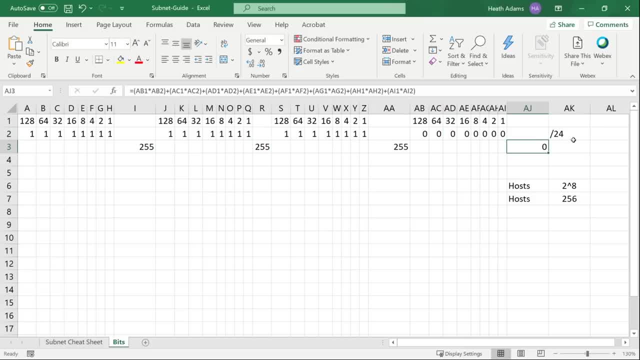 zero the standard here, because that is what's known as a slash 24 network. that's very, very common, And it's very common because it's used mostly in households and small businesses, And it's done this way because of the amount of hosts that it allows. Now, if we talk about the host, 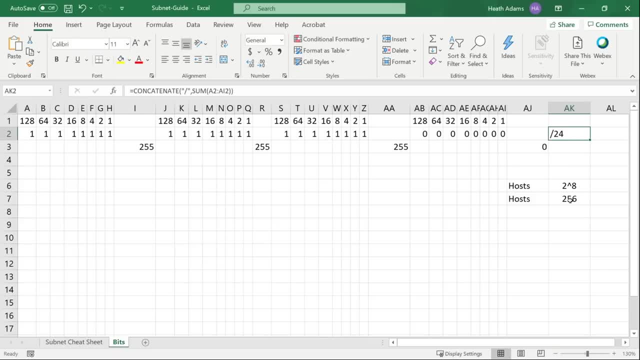 you can see that I have here two to the eighth power. Why do I have that? Well, we actually go by how many bits are switched off or how many hosts are available to us. So if a host here, a bit, was switched on, then we lose the amount of hosts we have available to us. and 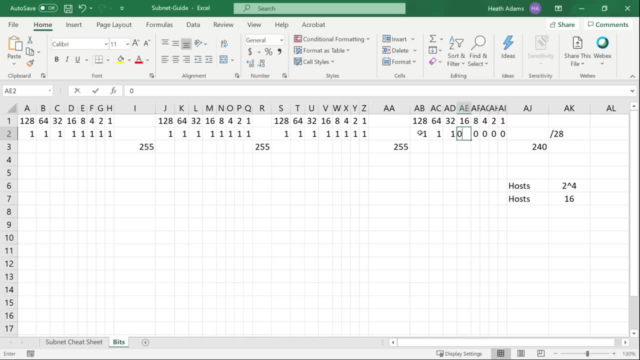 the subnet gets smaller and smaller. Now don't worry too much about the ones and zeros, it's going to make a lot more sense. And we stopped talking in these binary terms. I just kind of want to break down the math behind it first before we make it really, really simplistic. So again, we've 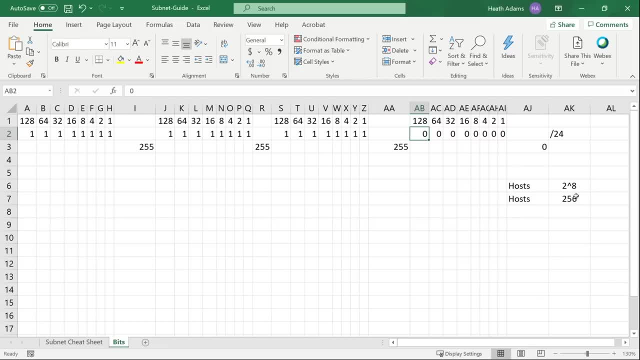 a WAC 24 network And it's so standard because of the host, again 256. think of all the devices in your house. you have cell phones. you probably have computers, you might have like a Roku or Amazon Fire or something along those lines. you might have smart TVs or smart watches or something. 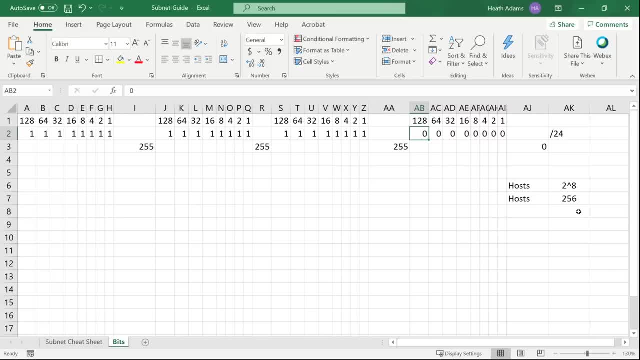 that connects to the internet. Well, again, they're all connecting through NAT right and going out. But the amount of hosts that you can have on your private network really depends on this subnet mask and how you set it. So we have this class C that you saw before, the 192, 168 dot one or dot. 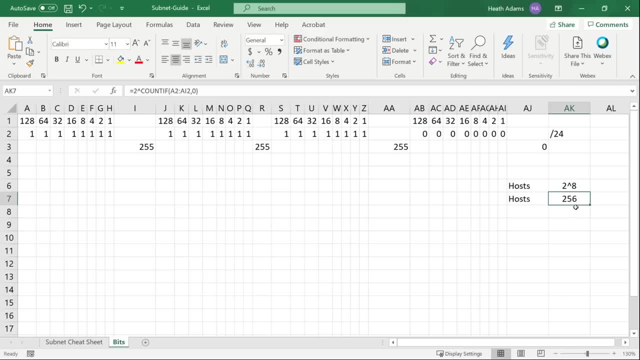 zero or however you want to have it right. Well, it allows us to have 256 when we have a subnet of slash 24.. So that's very common for a household. It's also common for a small business. maybe there's a printer, some few devices in there, but they're never going to get over this 256 hosts. 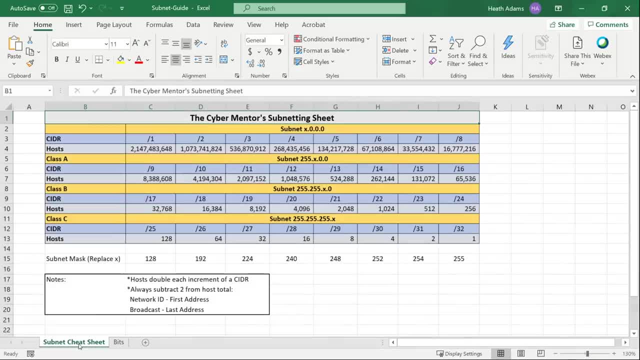 Okay. so when we come to the subnet cheat sheet, let's bring this down a little bit differently. So we have our host here. let's start with the slash 24. we just were and you saw that there is 256 available host as we start turning off bits. Okay, we turn. 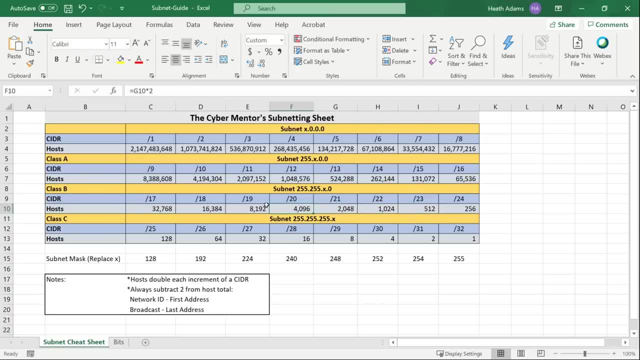 off a bit. here. we turn off a bit, keep going down the list, the host start getting bigger And that just corresponds. here we have a slash 24.. And the only reason I'm saying 24 is I'm counting the ones. 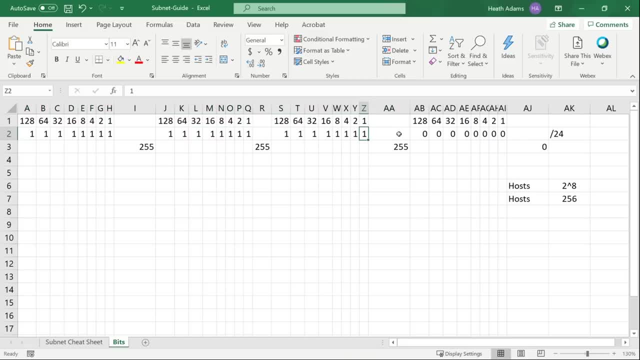 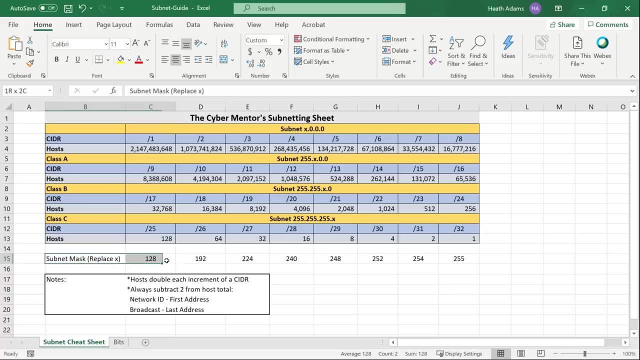 across, right? So we've got 24 bits switched on. if we had 23,? okay, it gets bigger and bigger and bigger. Now Let's stay away from the ones and zeros. I think it's a little bit complicated. The better way to think about this is to look at the subnet mass down. 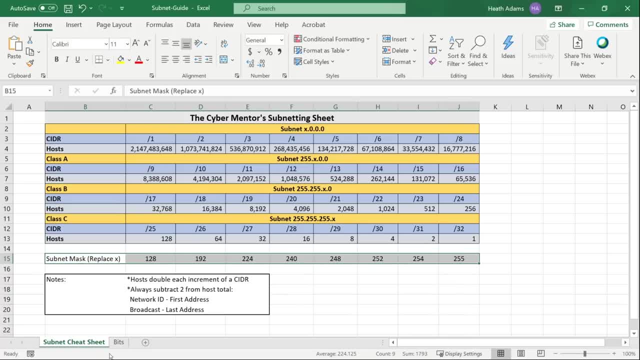 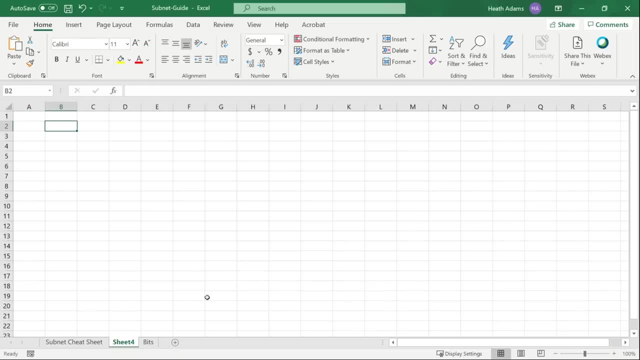 here And I'm going to replicate this and then we're going to come back to it. So what I do here is we can have a possibility of 32 bits switched on right. So I'm just making a new tab And I'm 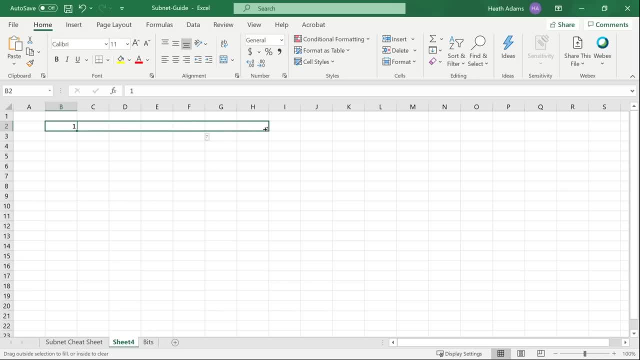 just going to go over here and I'm going to hit Control and drag this across. it hits eight, Okay, and then I'm gonna do the same thing with nine. I'm gonna drag it across. all I'm doing is just making really quickly 32 placeholders And I'm just emulating here. 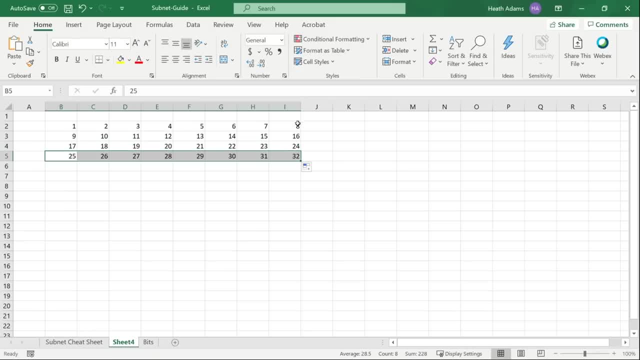 If we had the possibility of 32 different switched on bits. So imagine one bit is switched on. Imagine all 32 bits are switched on. That's the possibilities here, right? So always for sure, we're going to have an amount of hosts And we're going to have a subnet mask, Okay. 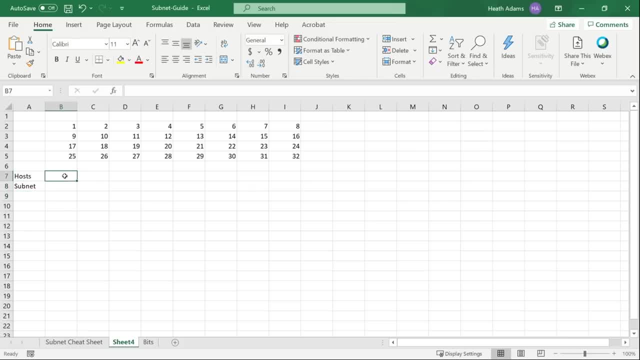 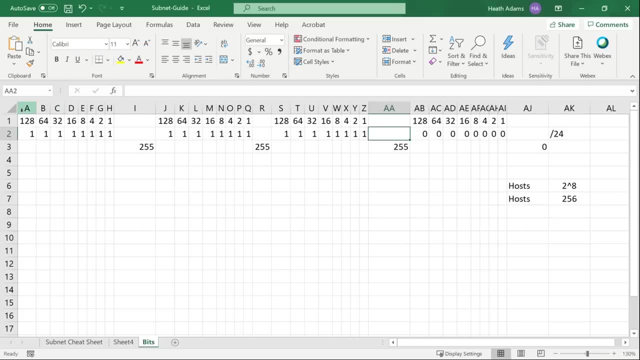 so we'll just call it subnet there. We always start here with 128.. Just like the bits that you saw. you saw the 128 start on the bits. Let's just start also with 128.. Now, as you saw, every bit. 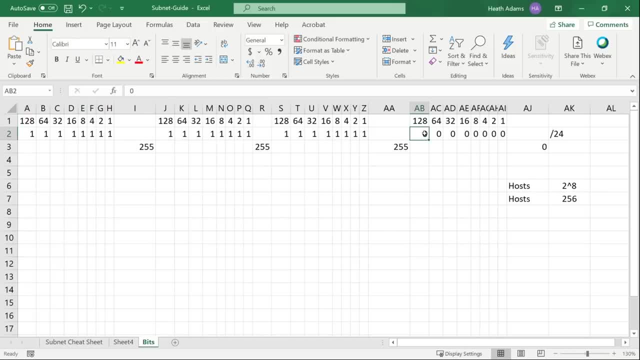 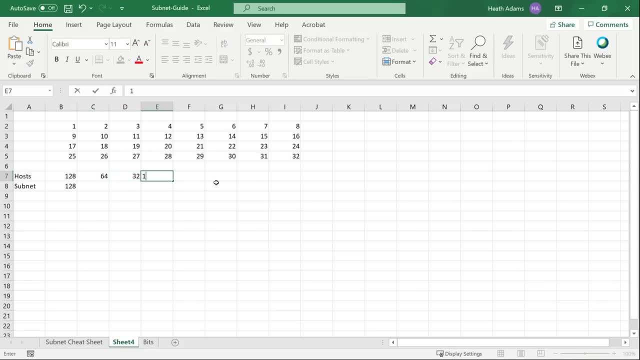 that switched on. remember, when we switch a bit on over here, it starts decreasing. So we're going to decrease for the bits that are switched on: 64.. 32, 168421.. You come over here And what I like to actually do is I like to just add these numbers. 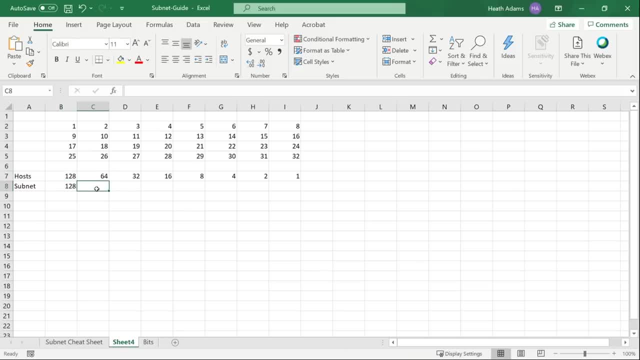 together And you can see 128 and 64 is 192. And then you can add these two together So you get 192, 32, you just add diagonally is the way I actually always do it. So 224, 240, 248, 252, 254. 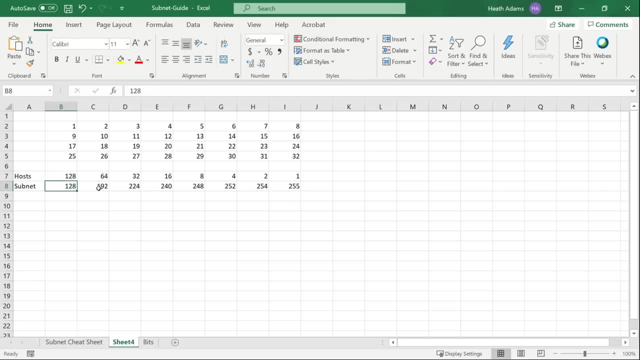 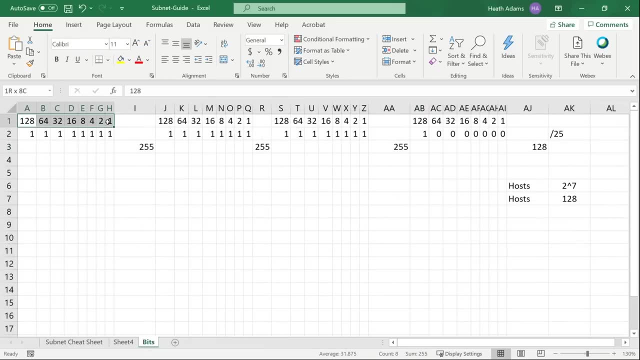 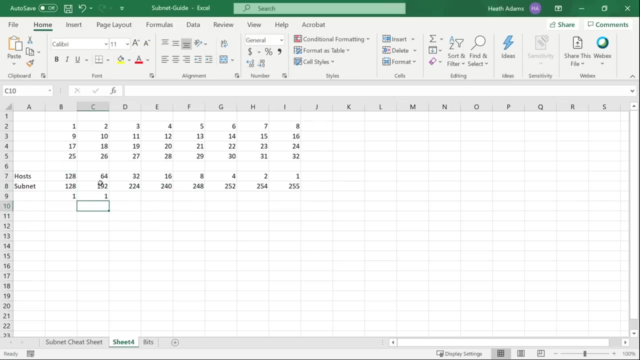 255.. Now, what does that correspond to? It corresponds to the possibilities of the bits being flipped on Right. So this looks just like what you see here: Same deal. And if you had a one underneath of it, okay, then you got 128.. If you've got another one underneath of it, 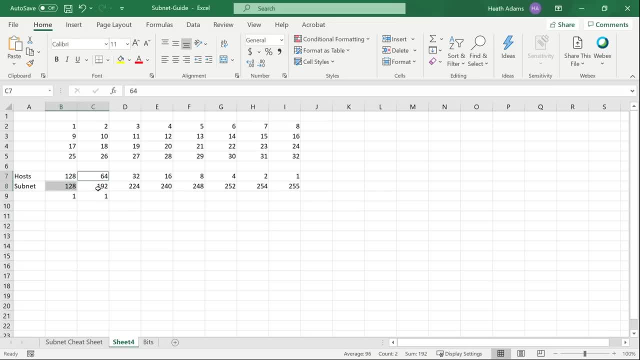 well, guess what? you've got 128 plus 64, which is 192.. And this number keeps growing. Why is this important? This is still all ones and zeros, right? Well, let's start thinking about it. We have a slash 24 network. we've got 24 bits turned on. our subnet mask is 255, 255, 255.0.. If we 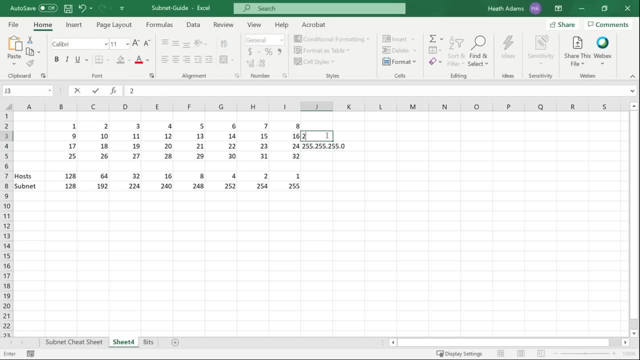 had a slash 16, it becomes 255- 255.0.0.. Why? Where are these changes coming from? Let me show you this. Okay, for a slash eight. I'm just tying this into just this right here. Well, this is coming from. 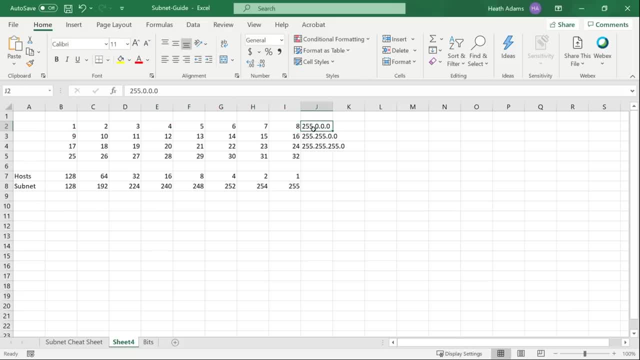 the subnet. And if you look at the subnet you can see that we've got eight bits turned on. eight bits turned on, we've got 255, and the rest are zeros. you got another eight bits turned on: 255, 255, the rest are zeros. come down to the slash 24, which is that really common subnet that you. 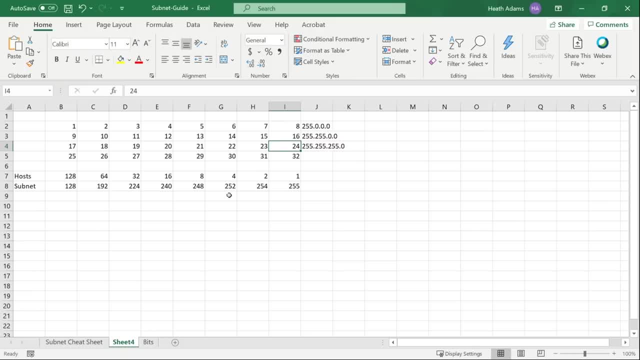 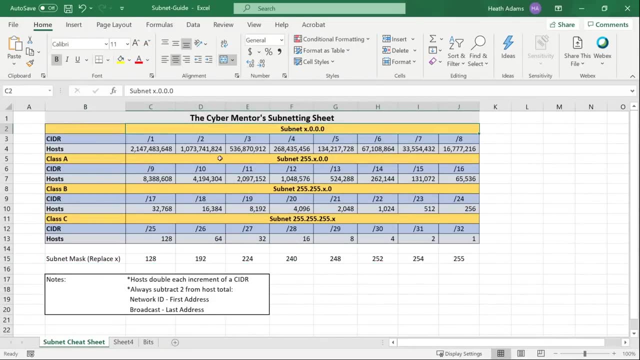 see, And you've got 255, 255, 255.0.. Now, this is very common. Okay, let's go back to the cheat sheet now, And you can see that I've got X as a placeholder in the subnet. I've got a slash one. Well, for this whole area here, from one to eight, 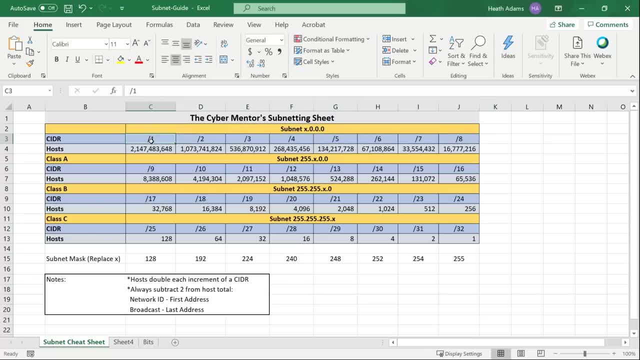 the placeholder is going to hold in place of this x. So for a slash one, if I've got 128, then guess what? it's going to become 128.0.0.0.. Because that's how it would be, And if you would, 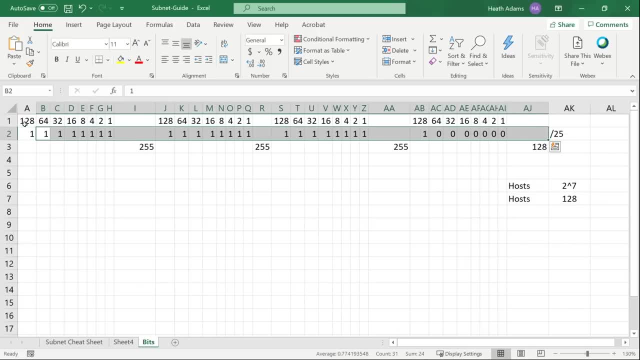 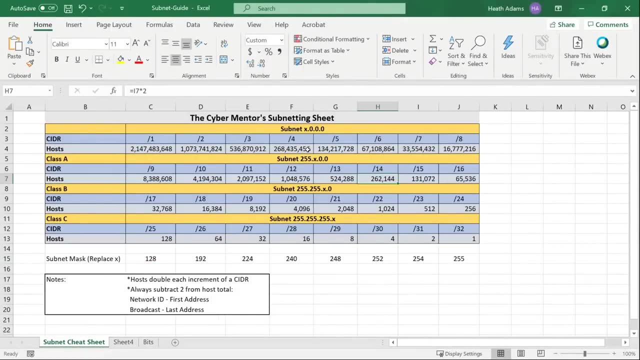 turn on just one bit here and made all of these zeros. guess what just the 128 would be on. the rest would be zeros. Okay, if we had a slash 14,? okay, so 255 automatically flipped on. you have a slash eight already passed through it. Okay, so you're starting on the second iteration. 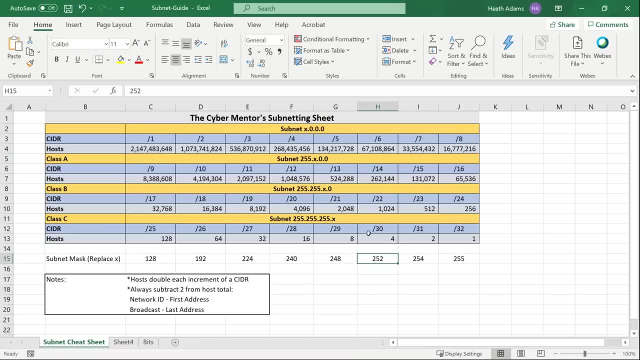 here, slash 14 corresponds down here to 252.. So you'd have a 255- 252.0.0.. So all this is is placeholders. Let's go back to the sheet here. So I make this quick and dirty list. 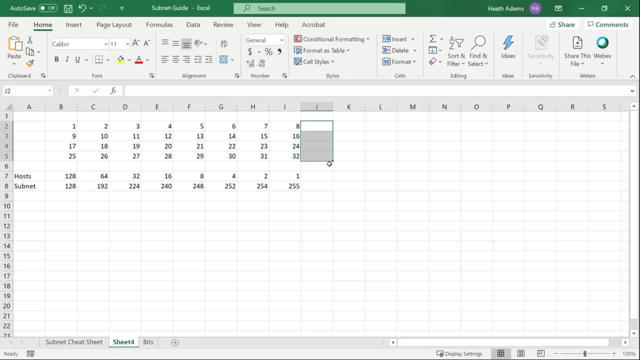 This is what I write out when I'm just writing out something quick for an exam. I'll write out one through 32.. I'll put the host here and I'll put the subnet here. So again, if we know that once we cross through 816, 2432, that we has a 255 in front of it, 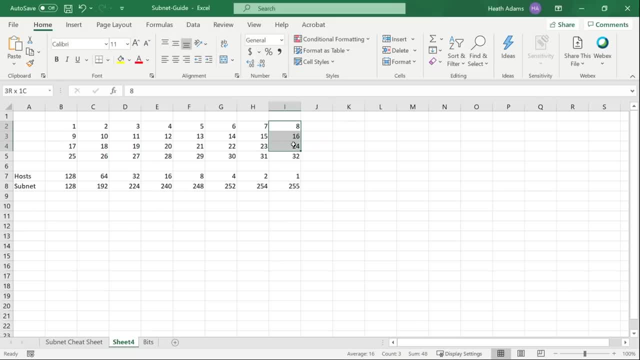 all we've got to do then is we'll say slash 27.. Well, we've come through three columns. then I know for sure that we've got 255, 255, 255, got something right. you see, the slash 27,. you come down here, the subnet would be 224.. Say 28.. Okay, 255, 255, 255.. Look at the 28,. 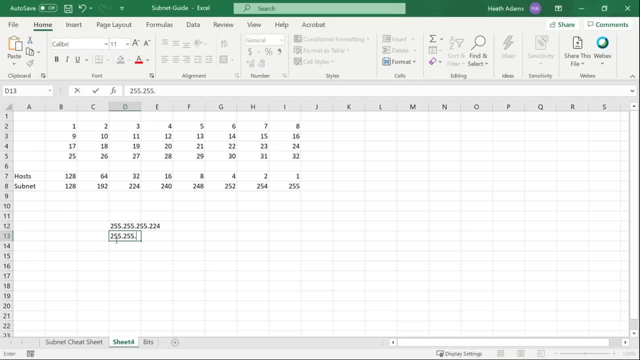 you've got a dot 240. And this is going to be confusing. This is: subnetting is not necessarily easy. Once you get the chart down, it makes a lot more sense. So let's start piecing some more things together. When I say that I've got hosts, Now the host I'm showing you only correspond to: 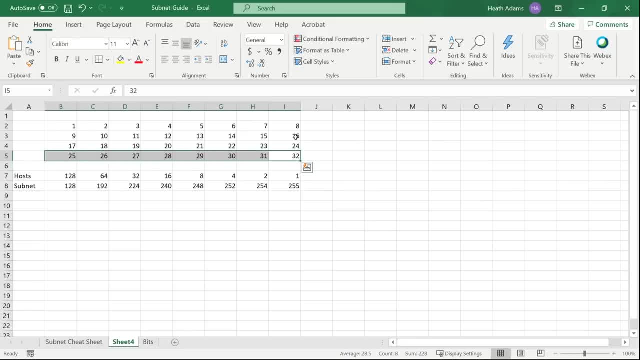 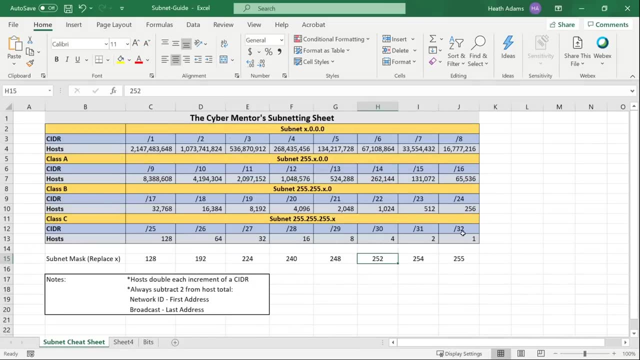 these first rows, But it's very common or very useful just to know this number right off the bat. Now, if you look at the cheat sheet, what you can do here is you just know that you start with a one 28, you go down, but every time you go up you're doubling. And why are we doubling? Do you remember? 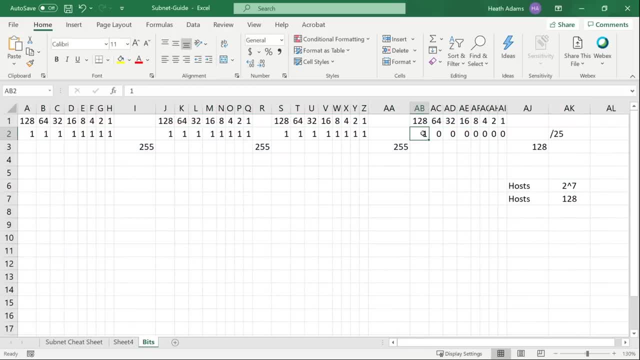 from the bits part. Every time a bit is turned off. So as we go up a number we take it to the next power. So we've got eight bits turned off, we take two to the eighth power. it's 256.. Well, 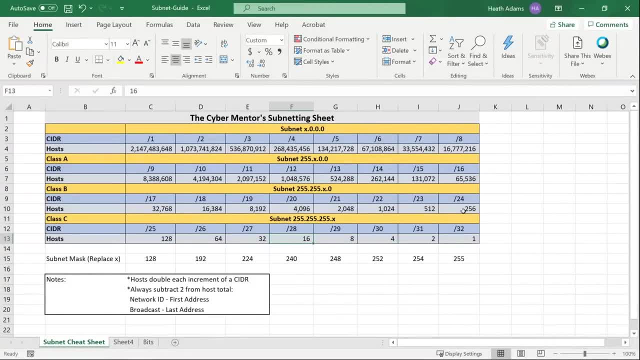 here you go, Look, come through here to 56.. We go to the ninth power- 512, to the 10th power- 1024.. It just keeps doubling. Okay, that's all you got to think about in your mind is. it keeps doubling. 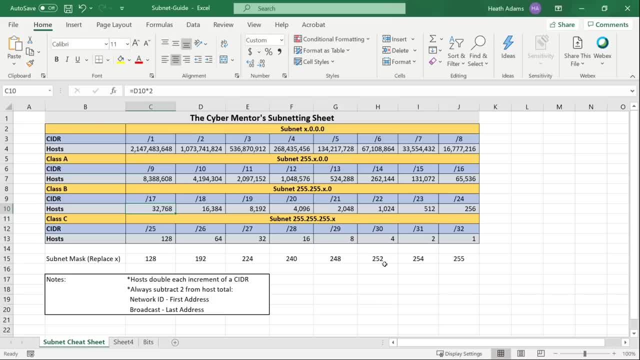 So on an exam, for example, you might have something like what meant how many hosts could be potentially in a slash 20 network, And you come to your cheat sheet that you made, or you have in your head, and you say, Well, 496.. And then we'll get to this in a minute, but we have to subtract. 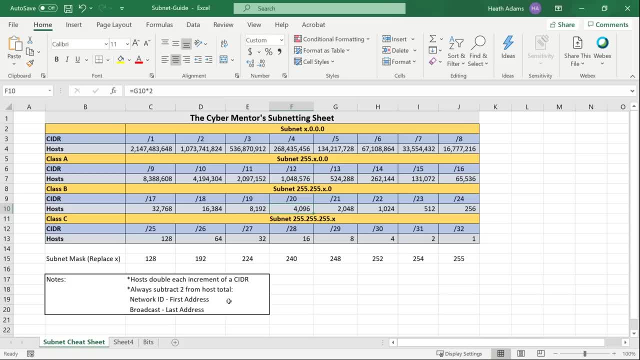 two, So 494 potential. And why is this all important? What do we even care about any of this? Why am I rambling on? Well, you need to know. based on the network. okay, the slash 24 is great for a small office home. 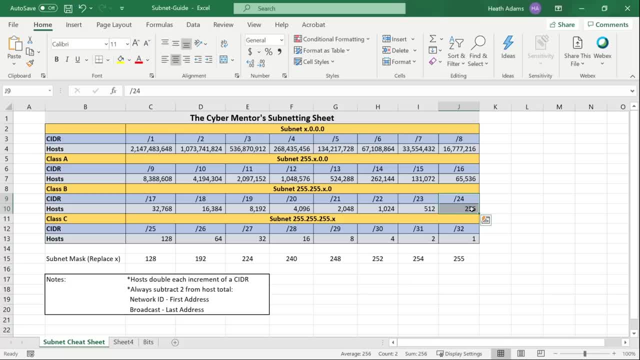 network however you want to have it. But what if you're a large enterprise? Maybe you have 1000s of devices. okay, maybe you want to slash 16 network. that might make more sense for you. Or you even see some with a slash eight network. It just depends on how big the company is. the larger the 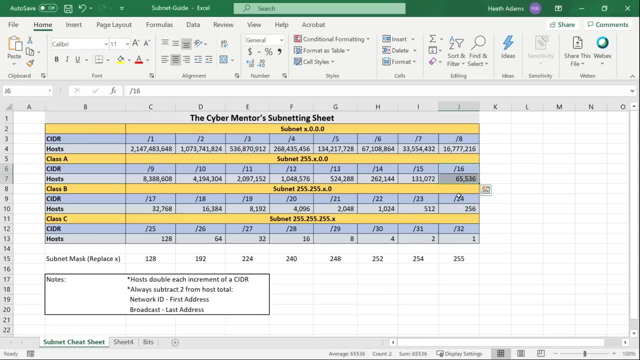 company, the greater chance that you're going to see that they're not using slash 24.. Or they could even have sub netted segments of their network where, say, they have just telephones and they've got 500 employees and 500 telephones. they might just have one slash 23 network for nothing. but. 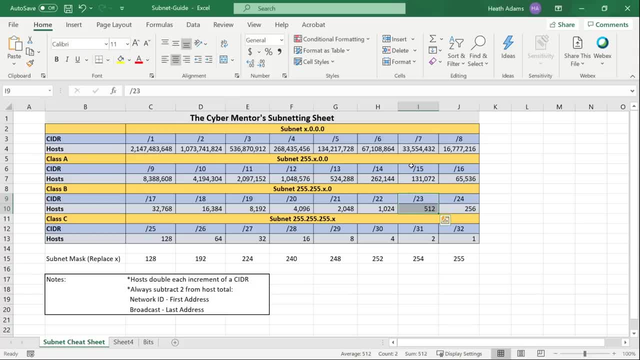 telephones, because that's the amount of hosts that fit in there. So what we're after with submitting is: how many hosts can we fit And what is the mask that's behind it? So those are questions you might be asked in the exam And these are questions that you're just going to see. 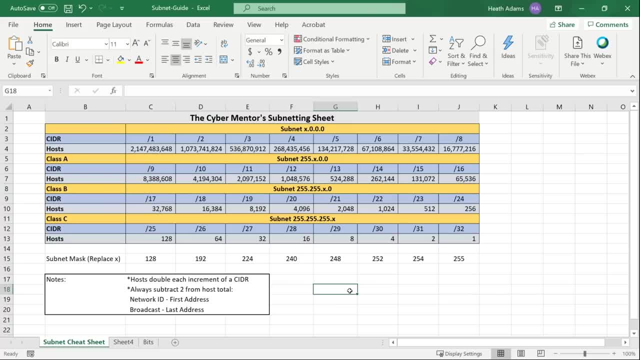 And when you're given addresses- say you're doing a pen test for a client- you might be given something like this: you might be given an IP address: 192.168.1.0, slash 24.. Okay, and immediately in your head you're like: Oh, slash 24.. That's standard. there could be up to 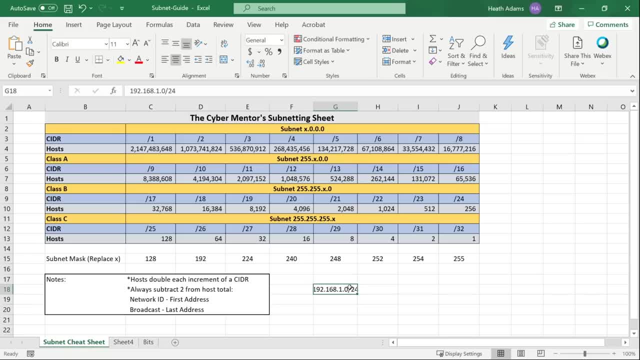 256 hosts or 254 hosts or devices in this network. But if they gave you something like 192.168.1.0 slash 20, then you might look at your little chart and say 4094 hosts. remember, we're going to. subtract to 4094 hosts and then you might look at your little chart and say: 4094 hosts. remember, we're going to subtract to 4094 hosts. and then you might look at your little chart and say 4094 hosts. 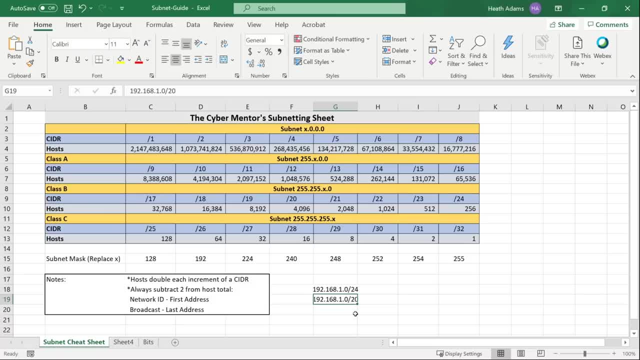 in this network. Now I know if I'm scanning this, I'm up against a lot more devices potentially than I am in this. Okay, so when a client gives you your subnets, they might just write it out like this And, depending how big your client is, might depend on how big their subnets are for you. 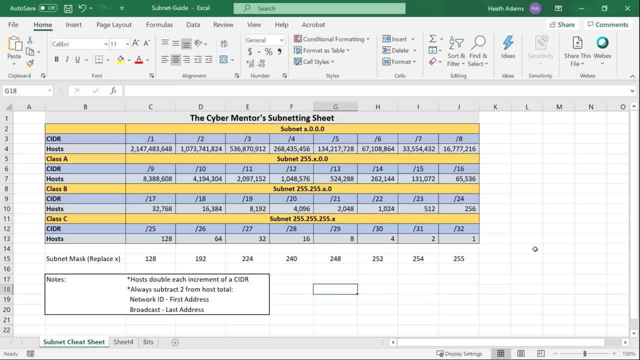 For example, I just pen tested a client that was a slash 16 all the way across and it looks something like 10.1.0.0, slash 16.. Okay, and your subnet mass for that would be something like 255255.0.0.. And how does this come into play? Well, every time you have a 255,. 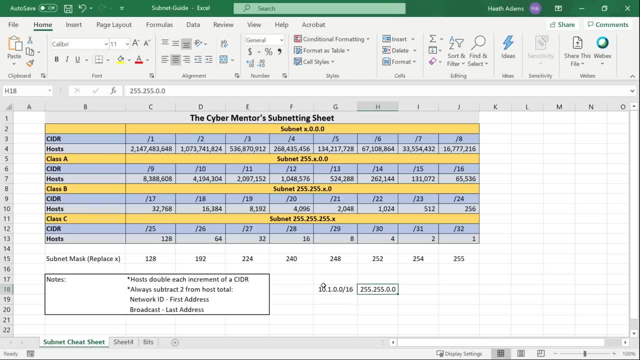 that number is locked in place. That's another way to think about this, So that 10 is always locked down. This one is always locked down. The rest of the bits are fair game, meaning we could have 10.1.1.0.1.2.3,. we could actually have a zero here, 0.1.2.3.4.. And that's how this number 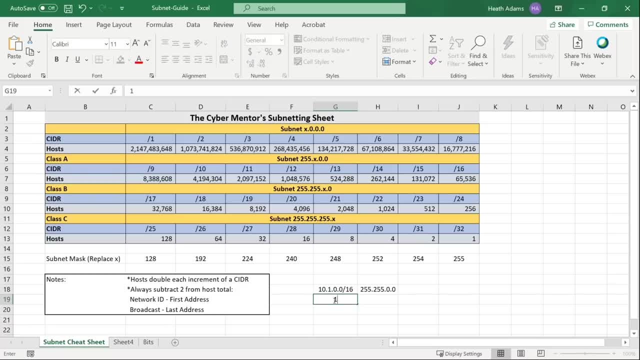 for like a slash 16 gets so big because you have 10.1.0.0 through 255 on the possibilities, which equals 256 hosts. okay, for one range you get 256.. Well, imagine you have to do that 255. 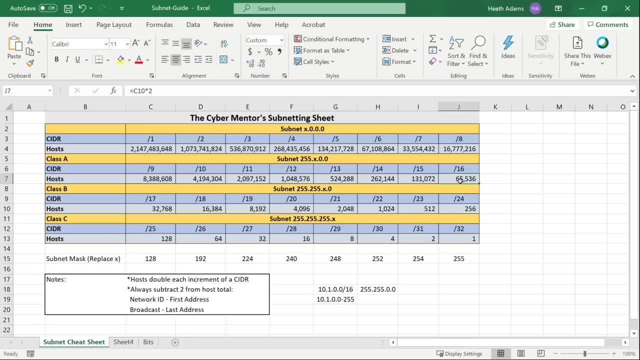 other times right, And that number gets substantially bigger here And then, if you were to have a slash eight, then of course it gets bigger and bigger. So what you need to realize are a few things. here we have these addresses. 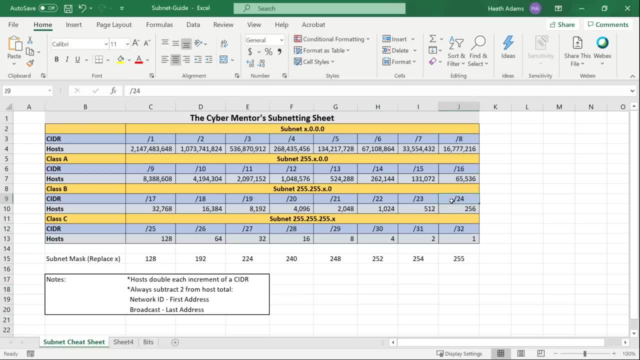 and you see the slash one, slash eight. again, we call them wax. WAC 24 is going to be very common. I would say wax 16 is probably your next common. you might see some weird submitted networks like this, sub netted networks like this, But typically it's slash 24, slash 16.. Now your network ID is: 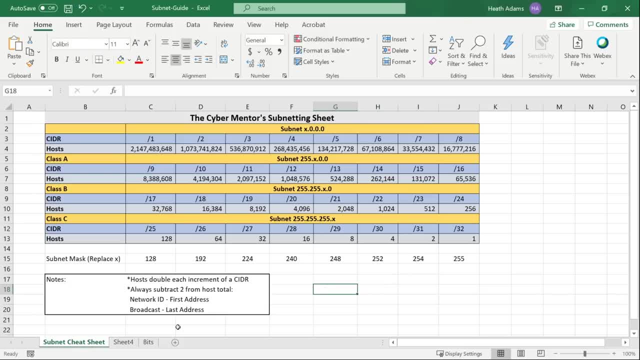 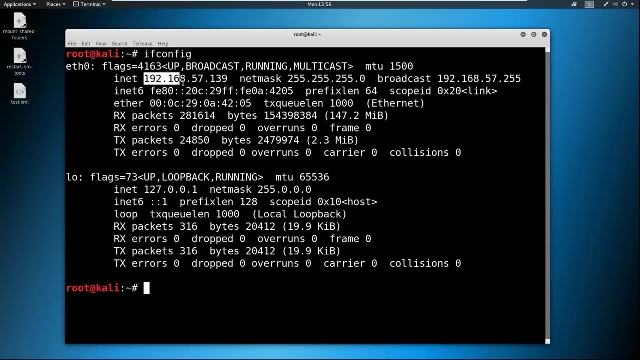 typically what is known as your first address and your broadcast ID ID is known as your last address. This is not always the case, but it is very common And let me log back into this Kali machine here And I'll show you. So we have our IP address: 192.168.57.139.. And we've got a net mask of 255.255.2550. 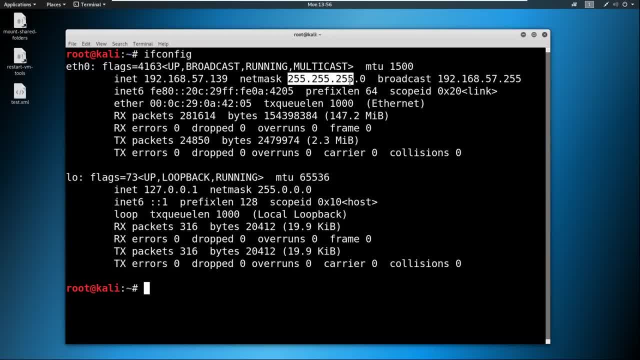 What does that tell you from what we just learned? That tells you we have a slash 24 network. Okay, this is a common network. there are potentially 254 hosts. why have I keep saying that? Why do I keep subtracting true? Well, we've got a network ID and a broadcast ID, or broadcast? 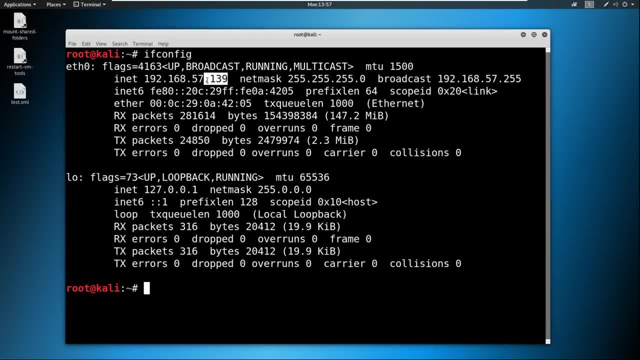 IP here. Well, what we need to know is we are dot 139,. we could be anywhere from dot one to dot 254 within this network. That's our 254 possibilities. This zero means we have the flexibility to be any IP address range from one to 254.. Usually, usually a dot zero for this IP here and a dot. 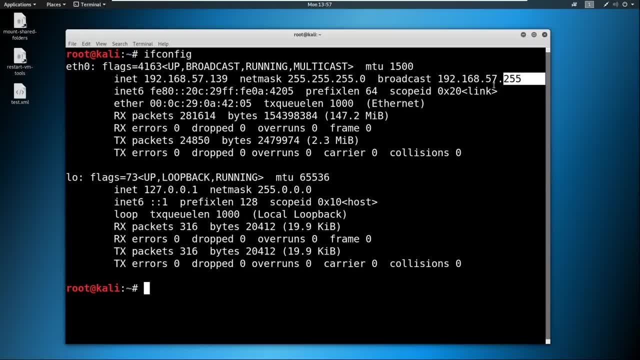 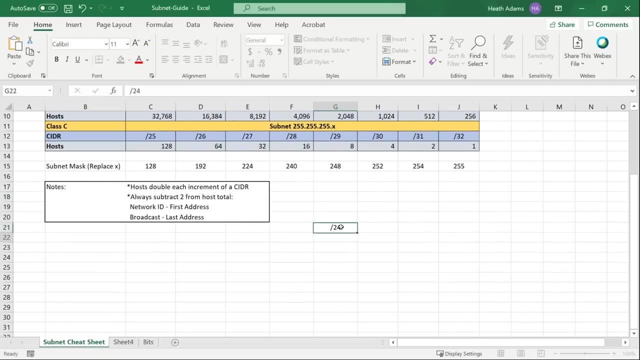 255 make up your network ID and your broadcast IP. Okay, usually. so if we were to say something along the lines of: let's go back to this Excel document. And we were to say something along the lines of this: let's say that we have a slash 24 network And we want to know how many hosts 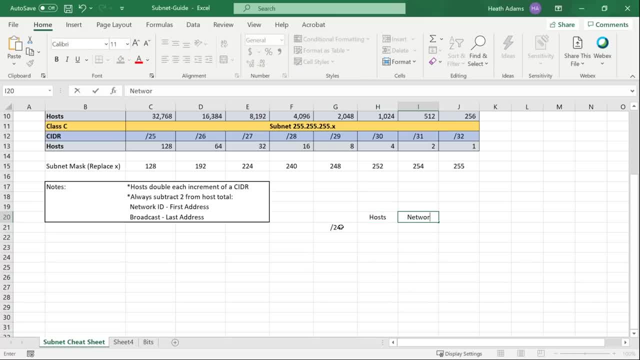 we want to know how, what our network ideas and what our broadcast ideas for IP is okay, we would, Okay and we'll. we'll give it one more. we'll say it's a slash 24.. And the IP starts with 192, 168.1.0.. 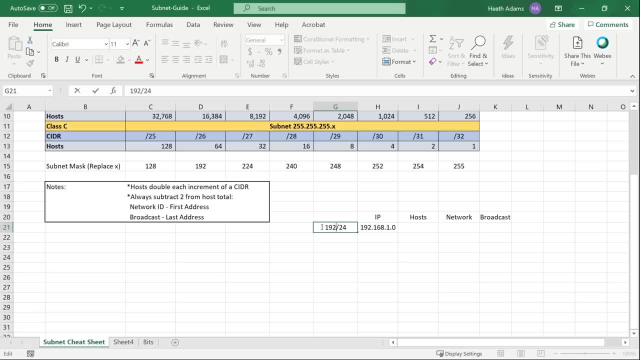 Okay, or we can even write it like this: 192, 168, 1.0, slash 24,. delete this And we'll say what's our subnet mask, What's our host, What's our network, What's our broadcast. So, subnet, you come to your. 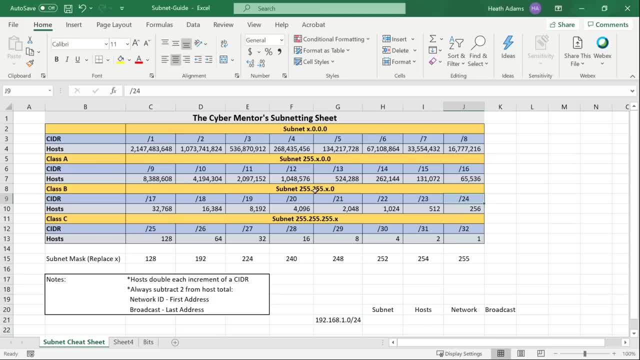 cheat sheet. you say, Okay, let's go to our broadcast, So subnet. you come to your cheat sheet. you say, Okay, let's go to our broadcast, So subnet. you come to your cheat sheet. you say, Okay, slash 24,. I already know that I need to be filling in this area here on the x, So I'm just 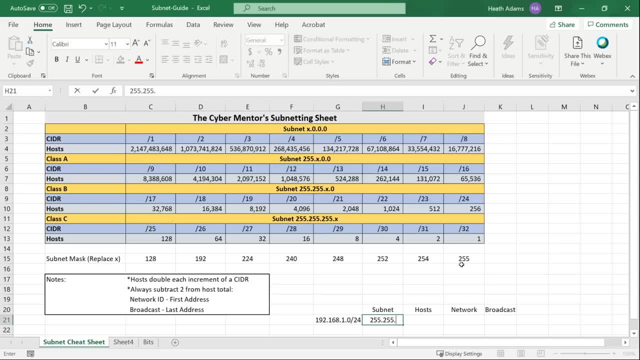 gonna come in 255, 255.. What's the x? Well, we know to come down this row to 255 here. dot zero, Okay. and then we've got hosts. I'm just gonna expand this a little bit. We've got the hosts, Okay. 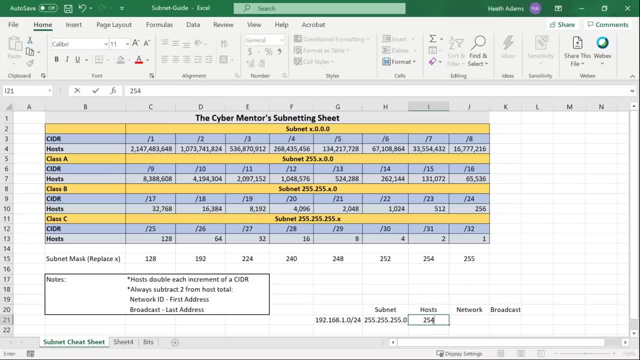 dosa right here: 256 host, potentially 254, though, because we always subtract two from the host total. So our network ID we're going to use in this whole thing. We're going to drag and drop, sort of like, the first address available to us, which is 192.168.1.0.. The broadcast is 192.168.1.255,. 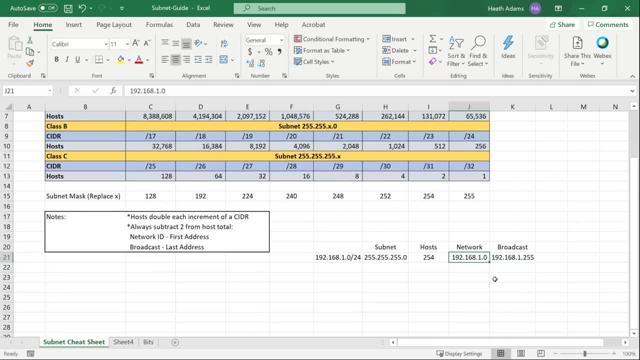 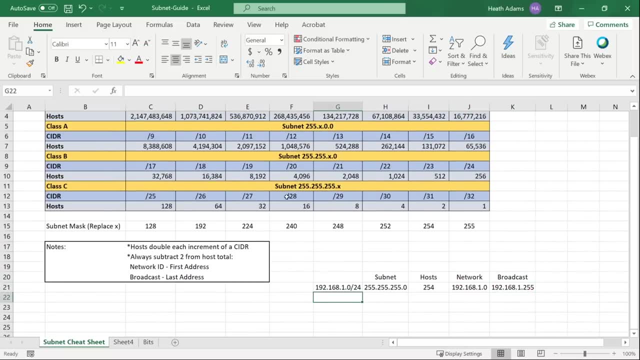 meaning available to us is anything from .1 to .254.. Let's take a look at something else. That's a basic example. Let's do like a slash 28.. Let's say we got 192.168.1.0.28.. Now what? Well, 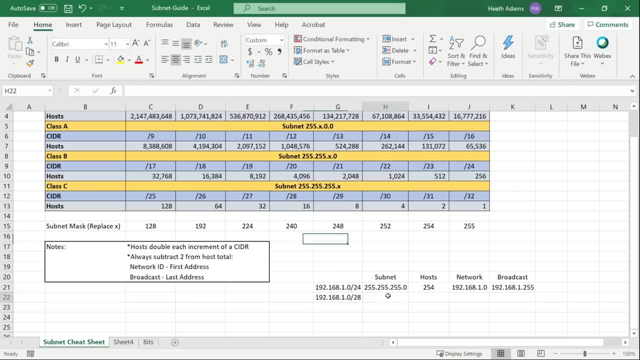 we've got 16 hosts here. Okay, so our subnet is then going to fill in 255.255.255.x. right, because we're in this row. Slash 28 says it's going to be a 240 when we drop down to the subnet. 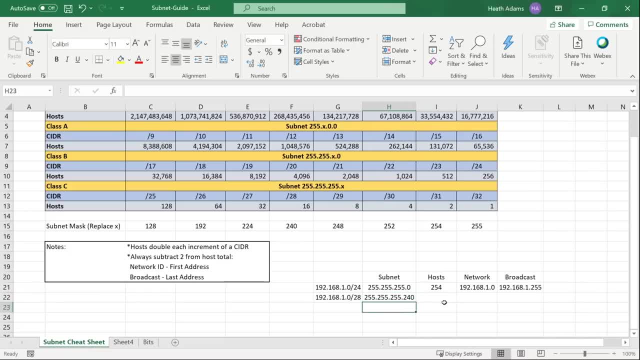 mask. I'm going to make this a little bigger. How many hosts? 16 minus 2.. We have 14 hosts. Okay, so the first non host would be 192.168.1.0.. Again, still the same thing. First address, Last address is going to be what? 192.168.1.15. 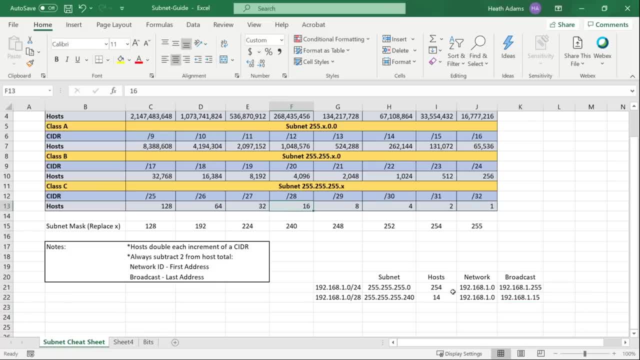 Does that make sense? 0 to 15 is 16. addresses Usable space is 14, because we take out the network and the broadcast. Now you could see something like this And then guess what? You're segmented. So because you're only using this little bit of space, you can then in turn have 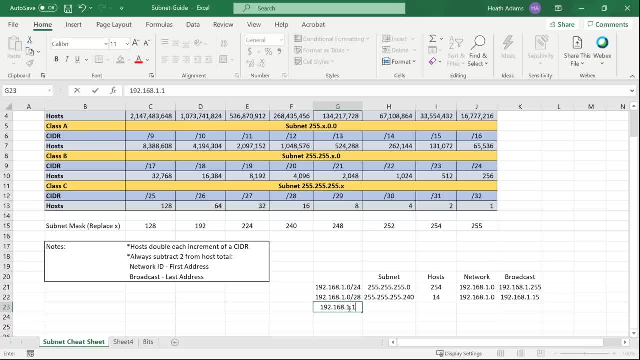 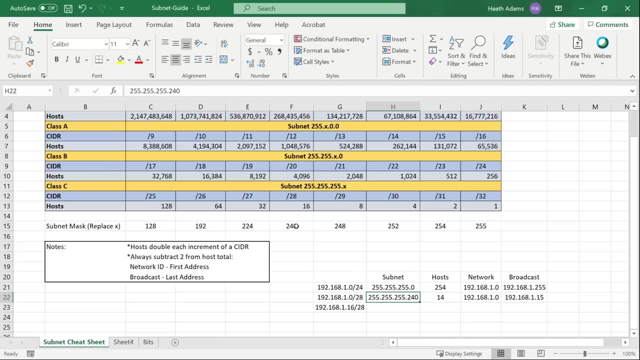 something like this: 192.168.1.16.28.. And then it starts the same way. Your subnet mask is actually the same because you're using a slash 28.. You come through. you can just copy and paste that. the hosts are still. 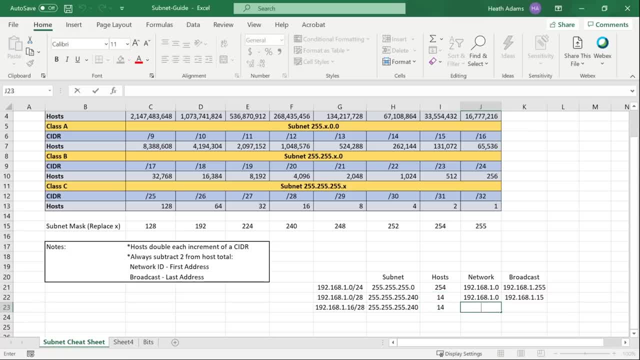 the same. What changes here? Well, your first address, 192.168.1.16.. And then your last address, which is 192.168.1.31.. So because this is smaller on the slash- 28 side- we can actually have multiple networks within, like, say, a dot 1.0. 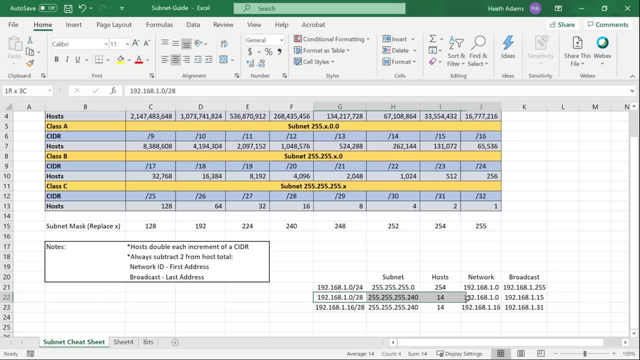 dot 1.16.1.32.. You get a multiple little networks here with only a small amount of hosts. So maybe you have a just a few servers in this range And you have like servers A, B and C. they go in a. 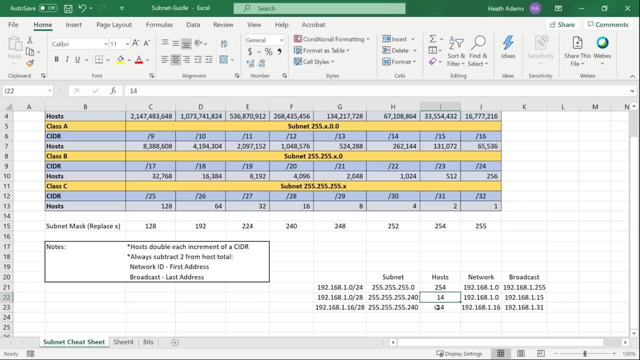 slash 28.. And then you have another one of servers- DC and E or D, D, E and F, however you want to say it, And you have more in that range. Okay, so you can subnet this out into different things. And when we see subnets, we see all kinds. 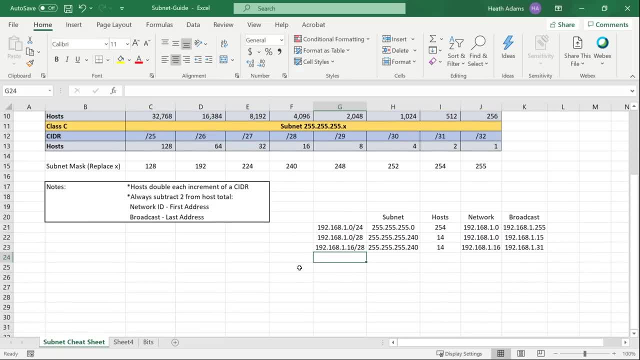 of stuff. We could see phones, servers, user computers, wireless, all different sort of things. Some companies get really specific with their subnetting. Now let's try one more. Let's say we have a slash 23.. Now I want to put in 192.168.1.0, slash 23.. But that would be wrong. 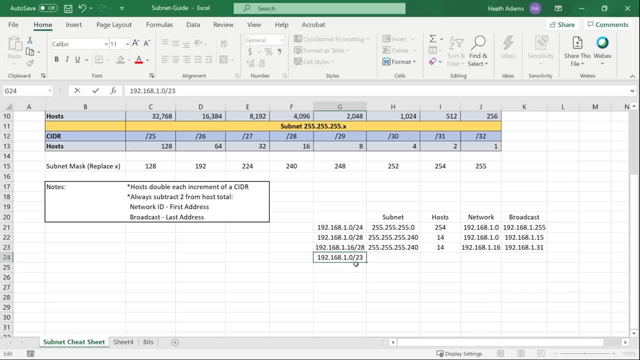 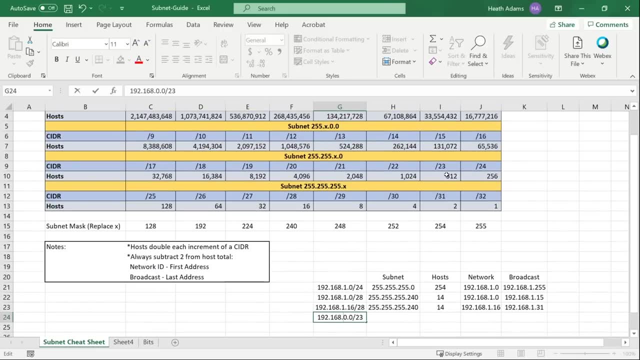 Why would this be wrong? This is actually going to be a zero, and I'll show you why in a second. Okay, so we're no longer locking in the this, this number anymore. right, When we get below the slash 24, the 255 all the way across for three of them, guess what? we're now have the ability to change. 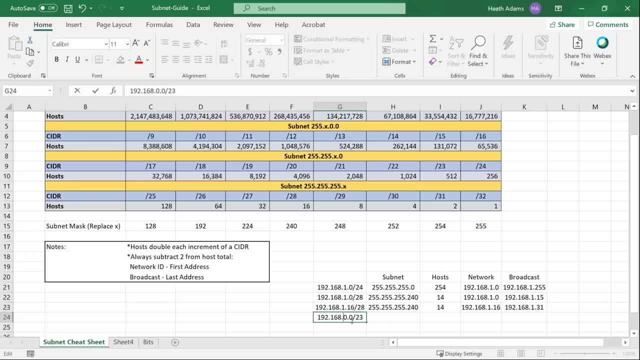 this number other than what's locked in. So let's do a dot zero. we'll talk about why it's hit. enter here, So subnet on a slash 23.. Well, we're going to do a 254, which is going to be the placeholder. 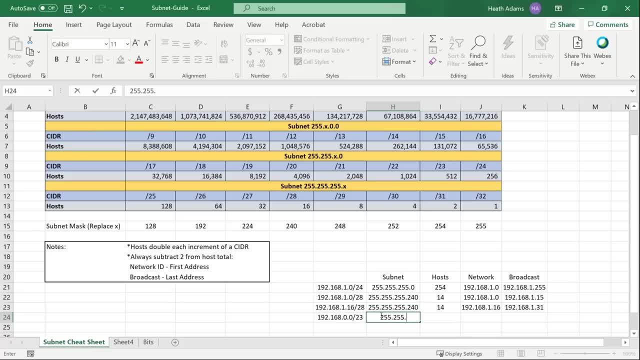 of the x here we're going to come in and say 255,, 255,, 254.0.. And now again we're not locked in. So remember, this 255 would lock in this dot one. that doesn't happen anymore. So we've got 255,, 255,, 254.0.. We're actually going to start. 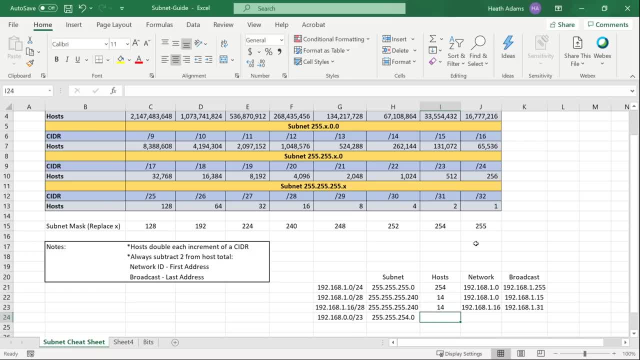 at zero here, And we're going to say the number of hosts that are possible. It's 510.. Okay, 512 minus two, we'll say our network ID is 192.168.0.0.. And our broadcast would then be. 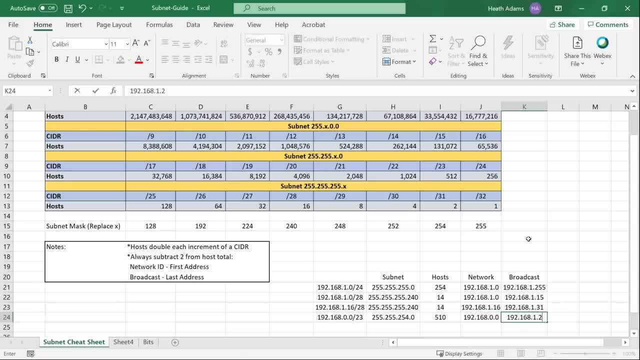 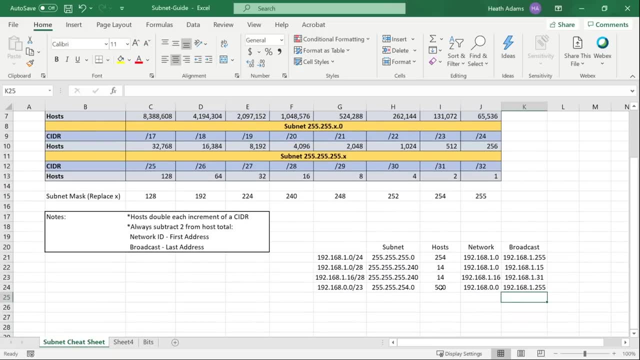 192.168.1.255.. Why, Okay, so we have the possibility now that we're spanning two ranges. we've got 510 hosts in this network, Okay, and we have the ability to go between zero and one. we've got two options now: zero and one. So if we were to say another network, 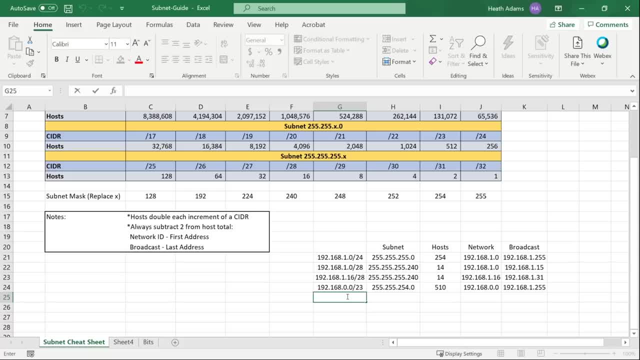 if we wanted to get to like a two, we'd actually have to say 192.168.2.0.23.. It would be the same subnet mask, same number of hosts, but then this would be 192.168.2.0.192.168.3.255.. Again. 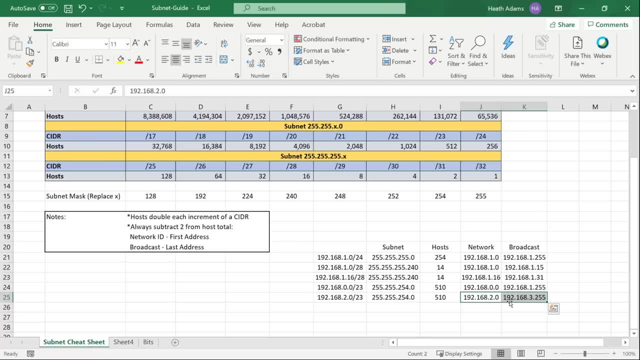 there's 510 possible hosts in between this right, Because you've got to think 0.1,, 0.2,, 0.3, all the way through 254.. And again, 1.1,, 1.2, all the way through 254.. 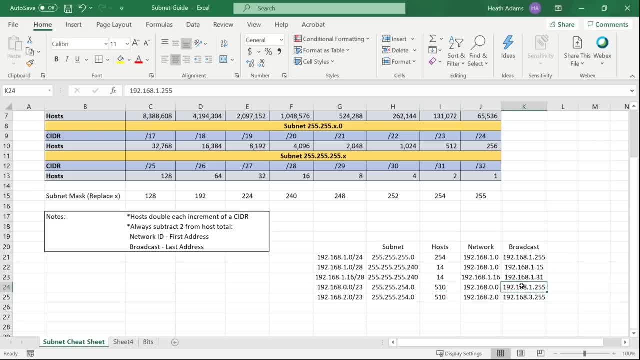 So that equals 510.. Once you've hit that maximum, that 1.255,, then guess what? You start at two. you have a whole new network here. Just like these smaller segments, you get whole new networks on the bigger side as well. So what you need to know is that if I were to put something like a 192.168.1.. 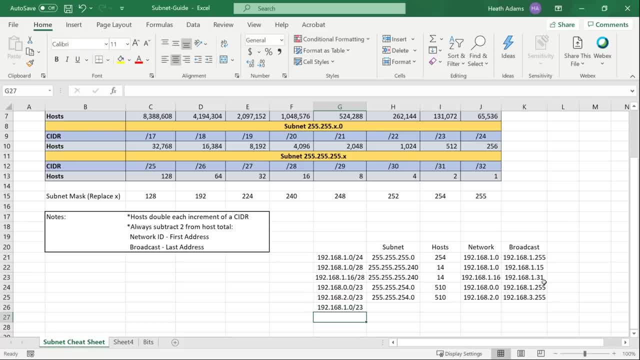 0.23, that would have fallen into line with the one and the zero in our actual network ID still would have been 0.0.. And a 1.255 would have been the broadcast here And you can double check this anytime you're confused. you can double check your cider notation. So I'm going to bring over a. 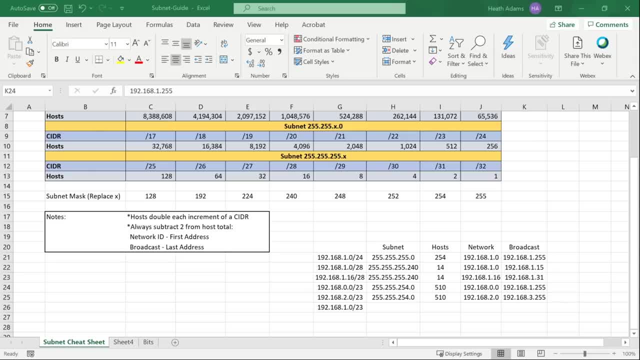 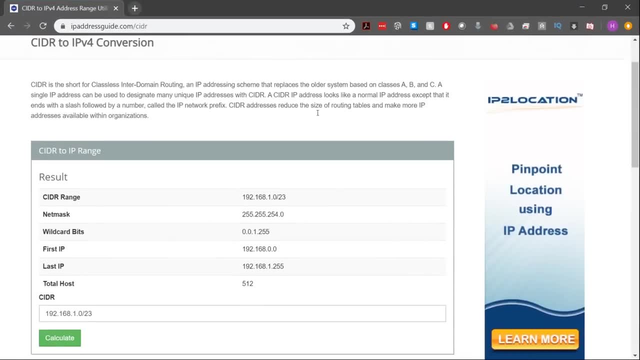 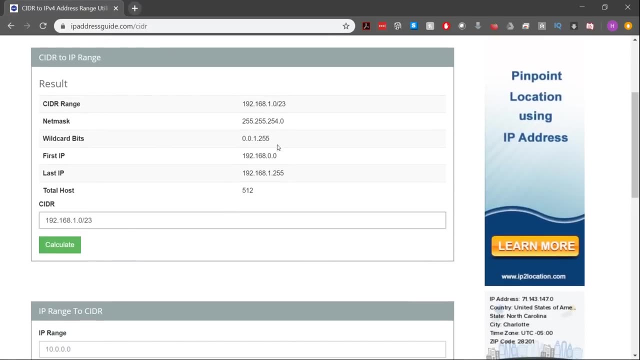 website that I will show you here, And this is just an IP addressing guide. It's called ipaddressguidecom. You bring this over and you scroll down just a little bit and I just put in 192.168.1.0.23 and you can see that it actually corrects me and 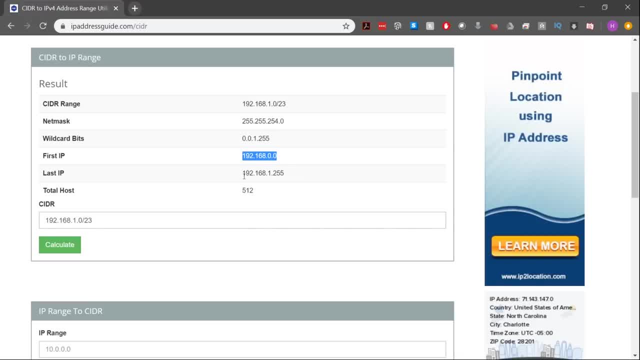 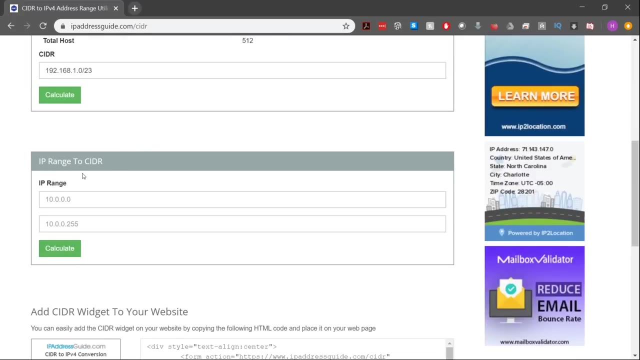 says the first bit is 192.168.0.0. the last one's, 192.168.1.255. total host is 512 minus 2. shows you that again. first IP, last IP. you got your net mask very easy to use a CIDR calculator here or an IP. 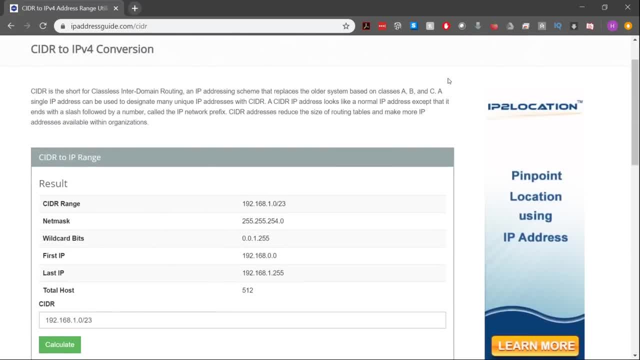 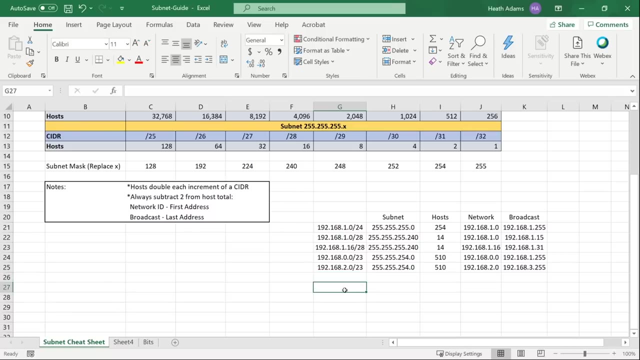 range to convert to CIDR as well. so very useful calculators, but if you're not allowed to use these for like an exam purpose or something along those lines, then using the cheat sheet that I've shown you is super useful. now what I want to do is I want to try three more subnets. okay, I'm going. 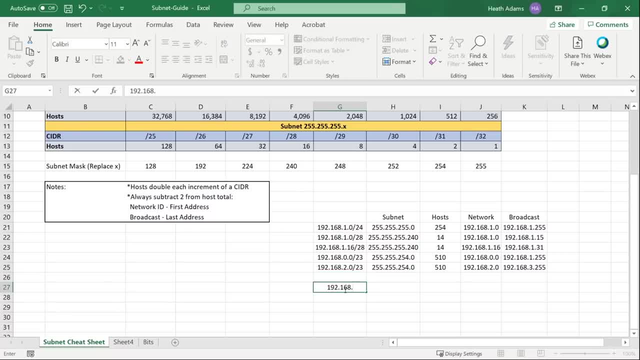 to write these out. I'm going to say 192.168.0.0.22, 192.168.1.0.26 and 192.168.1.0.27. I want you to solve these for me. tell me the subnet mask, the host network and. 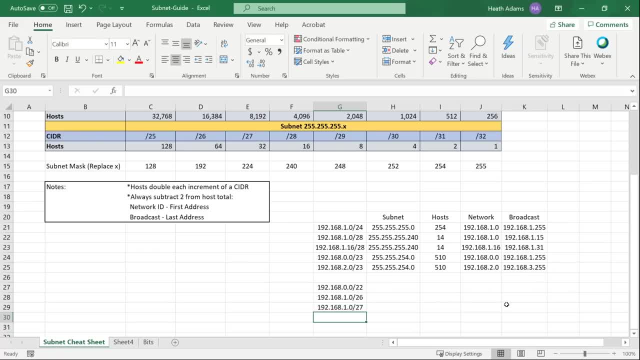 broadcast and, with that being said, this again is a very complicated topic. I did not pick this up the first time or the second time that I got it. if you're running confused right now- perfectly normal- you can go back and watch this video again. try to pick up more topics. try to understand it. 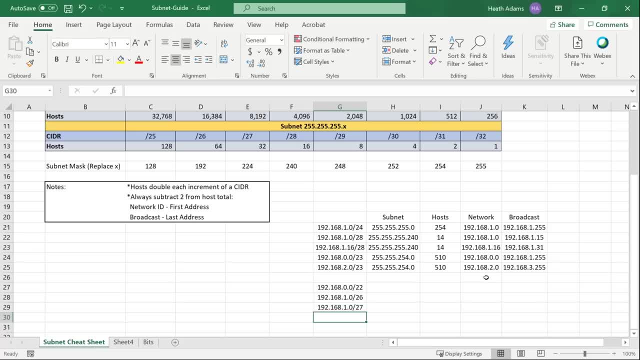 maybe I'm not the right instructor for this either. I do recommend you to go back and watch, looking at other resources to completely fill in your knowledge gap, if there is one that exists. another resource that I'll link down is what is called seven second subnetting. it is very useful. 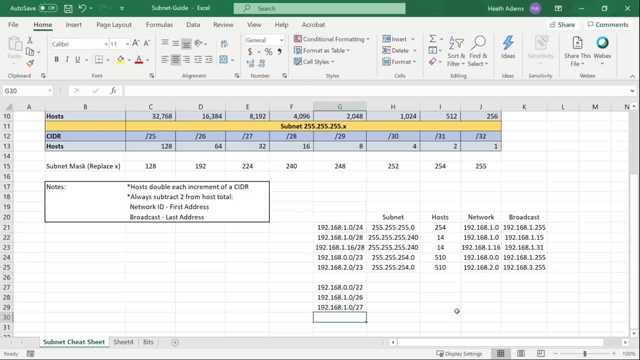 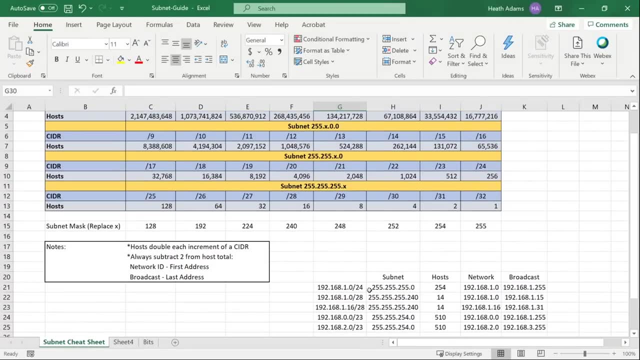 a lot of students have recommended it to me. I'm going to push it forward as well. so go ahead and try to solve this. understand that. what you're after here is just understanding what a subnet is okay when you see something like this: if a client sends you 192.168.1.0.24, you're going to. 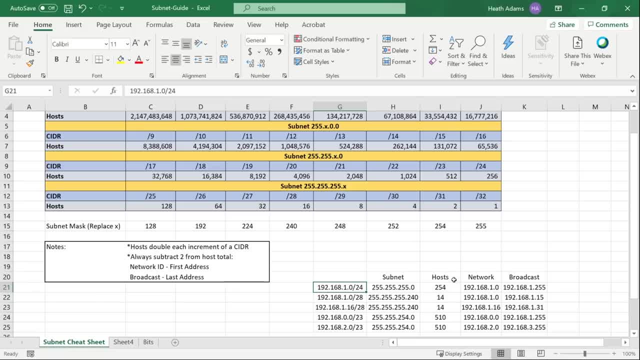 say, hey, okay, I know that there's probably two 154 hosts in that network and I know what I'm working with. if you see this 255.255.255.0 again, you know that you're working with a slash 24 network, very standard stuff. that's what we're. 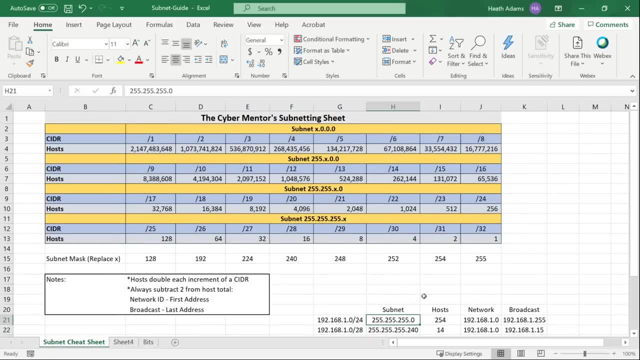 after. I don't expect you to ever memorize this. I don't have this memorized, like I don't come in here and say: you know, a slash 18 is a 255.255.192.0 network and it's got 16,384 hosts. I don't do that. 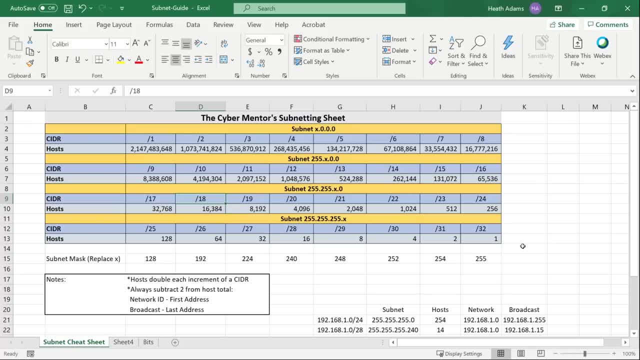 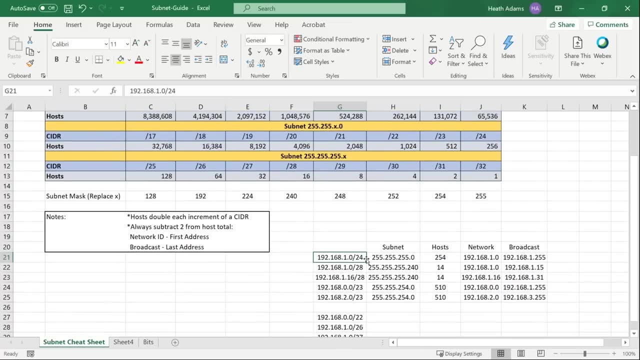 okay, I have a cheat sheet. I'll use a website if I need to. the most part, what you need to understand is 254 hosts for a slash 24. if that number has gone up to like a slash 28, you know you're dealing with less. if that number is lower, like a slash 16, you know. 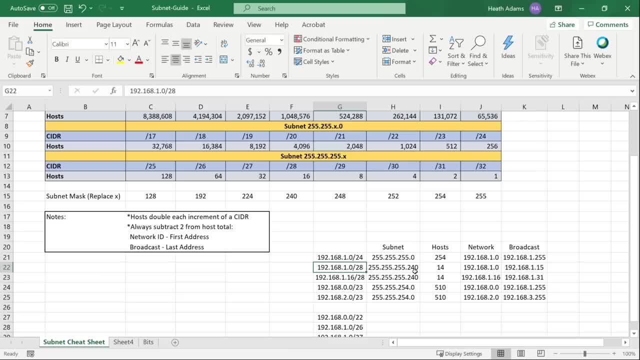 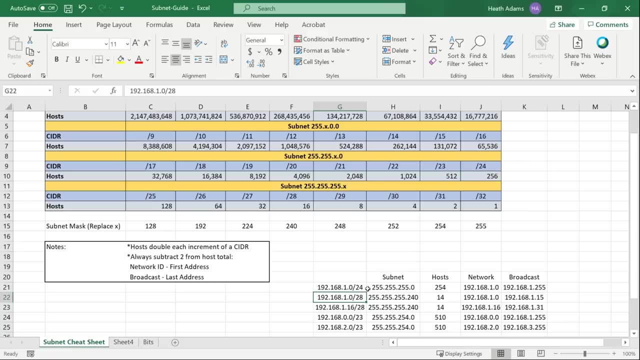 you're doing with a bigger network. that's really what it comes down to, unless you are working in networking and then these become more important. but as a pen tester, understanding how to read this, understanding what the subnet is and just identifying it with very basic measures, this is. 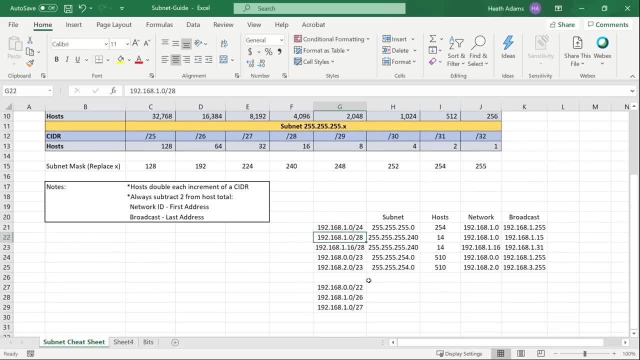 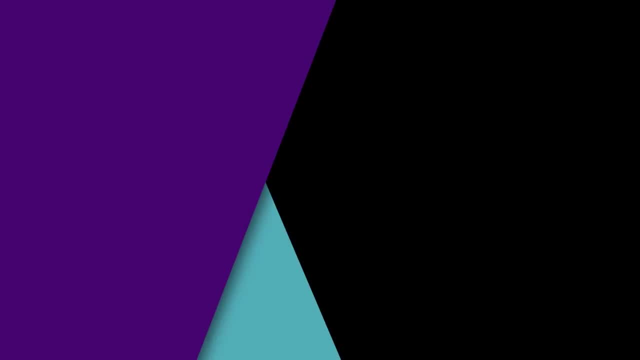 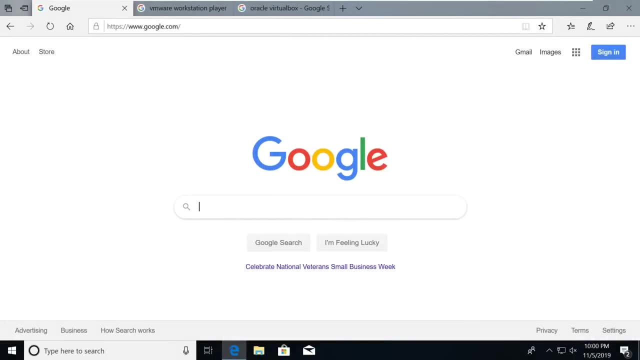 extremely useful. so I will catch you over in the next video, and I'll see you in the next video when we talk about solving these challenges, and hopefully we got them all right. so I'll see you over there in the next one. all right, so in order to be successful in this course, we are going to 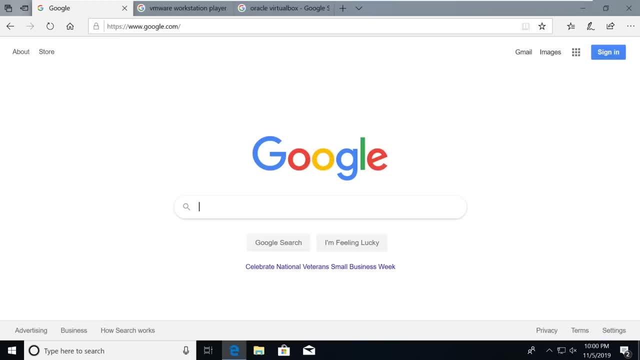 be utilizing what is called a virtual machine. now, virtual machines are known as VMs for short, and a VM is just a machine on top of a machine and, to give you an example, I'm actually running this instance that you see here on top of my Windows 10 instance. so here you can see if I scroll up. 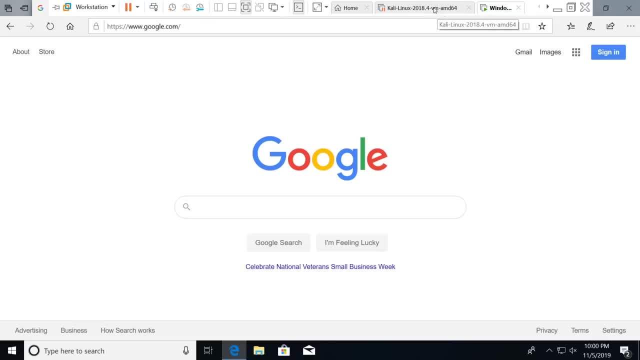 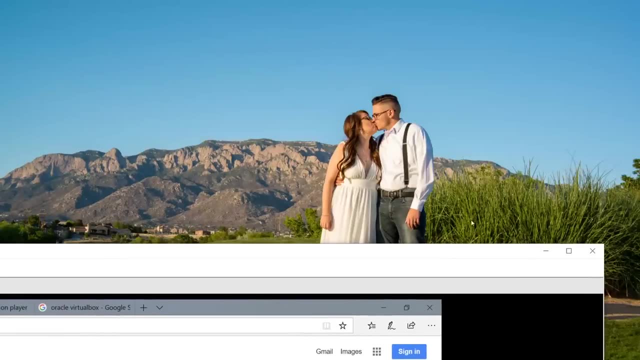 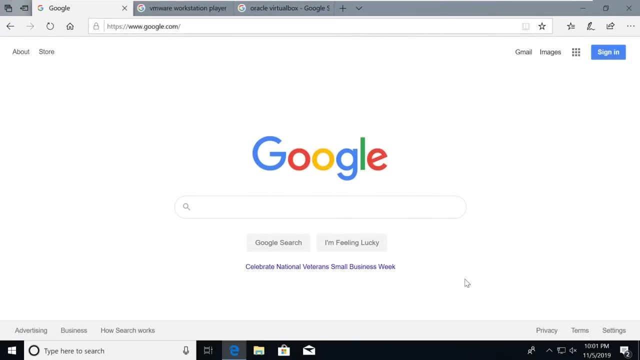 that I have a Windows 10 machine. I also have a Linux machine sitting here. if I were to D maximize this, you can see that I'm actually running here a Windows machine in the back. this is my wife and I, and when you come through here, we just blow it back up and we're back inside of our machine. so 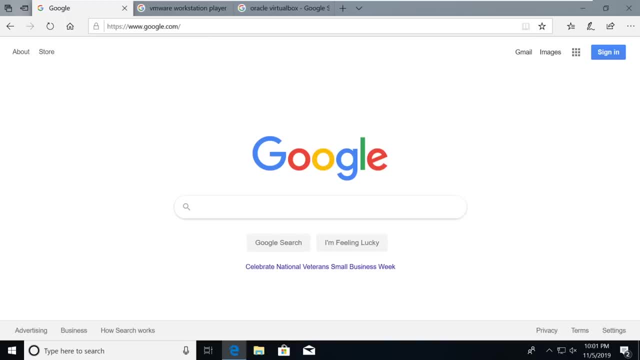 a virtual machine is just a machine inside of a machine. so what we're going to be doing is we're going to be utilizing this to build out labs. that way, we don't have to actually have a bunch of hardware. we can just use this for our our course and run what we need to on top of our. 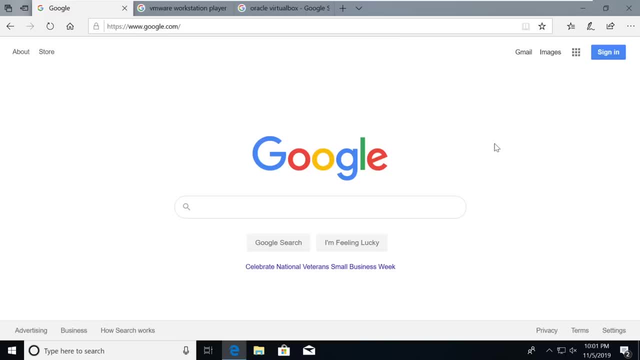 own machine already now. this can get resource intensive. so if you are only utilizing something like 8 gigabytes of RAM, then you might have some issues with this, but you can still follow along. when we get into the Active Directory portion, you might run into issues if you do not have at least. 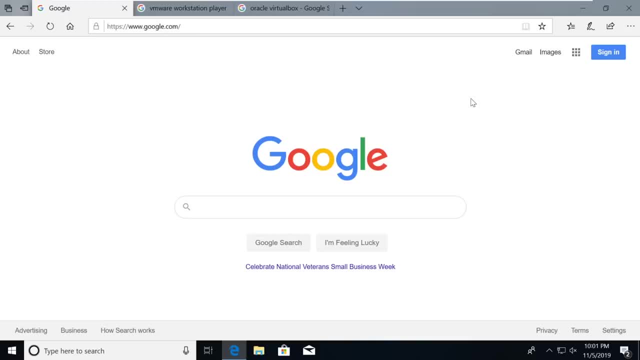 16 gigabytes of RAM to utilize. if you don't have at least 16 gigabytes of RAM to utilize. if you do utilize- but we'll worry about that when we get there- there are still plenty of ways to follow along throughout this whole course. so another thing to note is that I use VMs every single day. 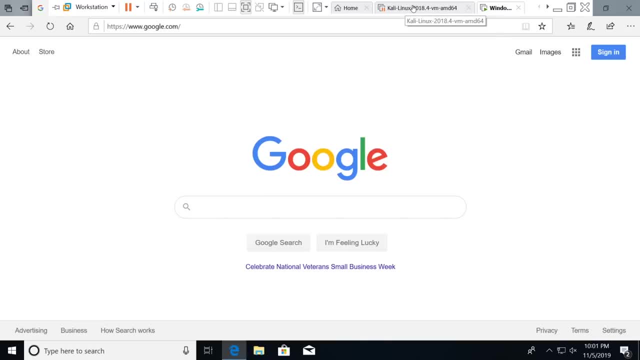 this machine that you see here is actually my day-to-day pen testing machine. so I run a Kali Linux instance on top of my Windows machine and utilize that to do penetration testing. so I'm going to demonstrate that to you and how we're going to build out our labs with that and a lot. 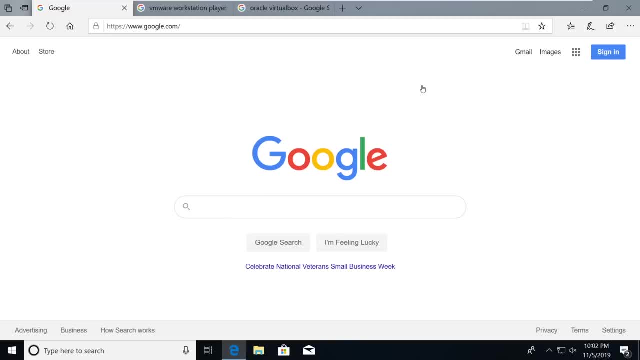 of us in the industry run through VMs as opposed to running it directly on metal or on a machine. so in order to utilize virtual machines, we first need some sort of virtual machine software to play these. so there are two different ways that we can do this. if you are on a Windows machine or a Linux machine, you 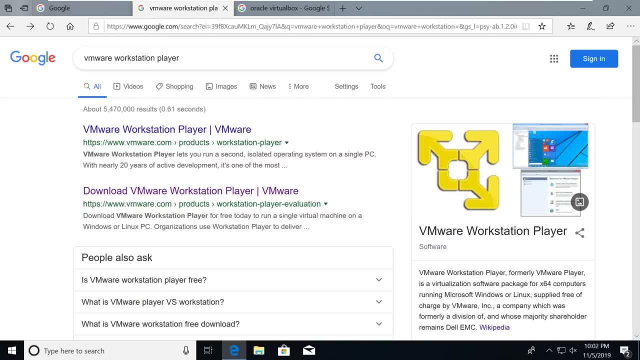 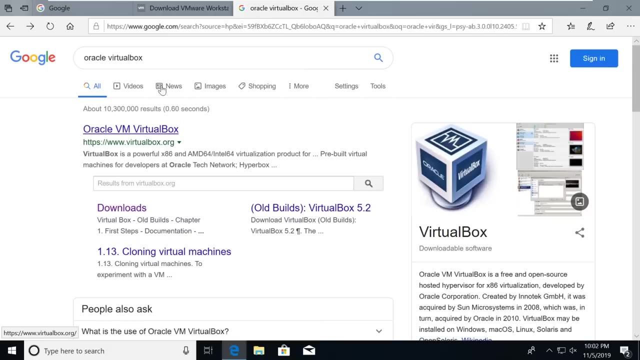 can utilize VMware workstation player. now, if you type in VMware workstation player in Google- the first one here that says download VMware workstation player- you just click on that and if you are in a Mac environment, you're going to be utilizing Oracle Virtual Box. so if you type 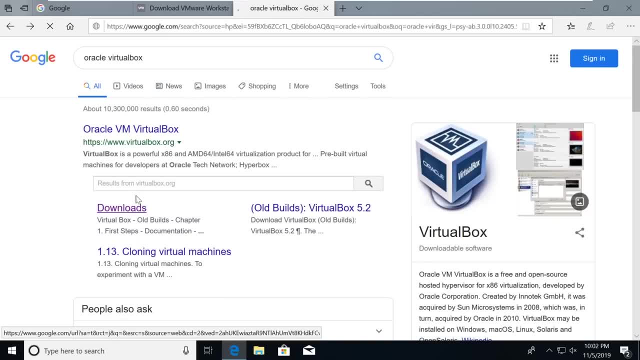 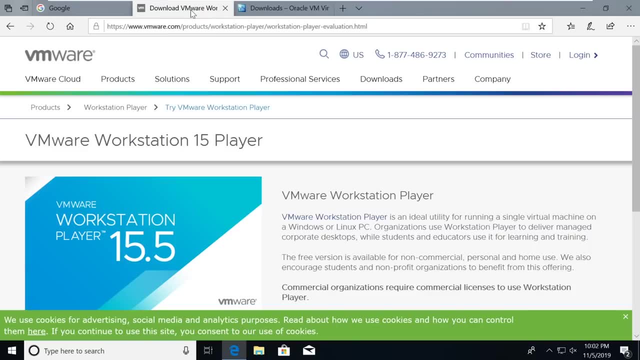 in Oracle Virtual Box. you come here and you go to downloads. you have your option there as well. so in this course I will be using VMware workstation player. I'm going to be running it on top of Windows. if you are using Mac, that is absolutely fine. you're going to be following. 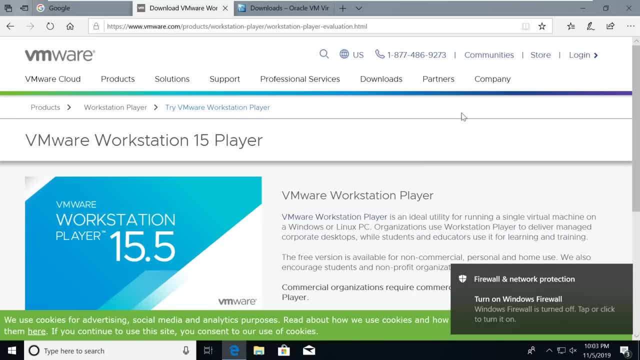 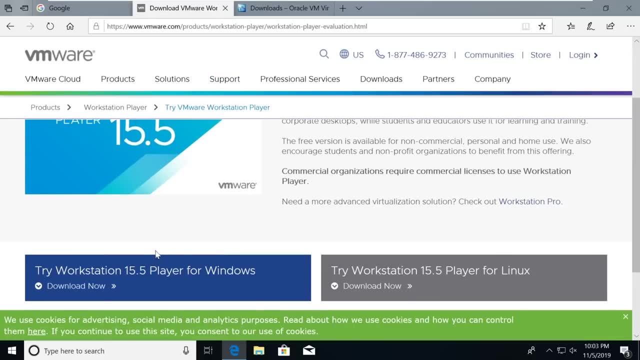 along just the same. all you need to be able to do is follow the same instructions that I give you and it will be a-okay. so if you scroll down here, you can see try workstation player for Windows or try a workstation player for Linux. go ahead and just select download now. that should bring up a. 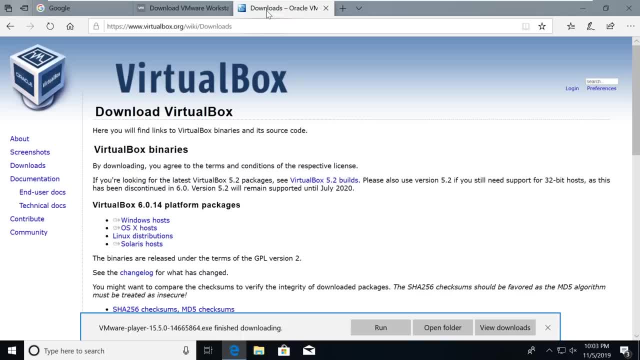 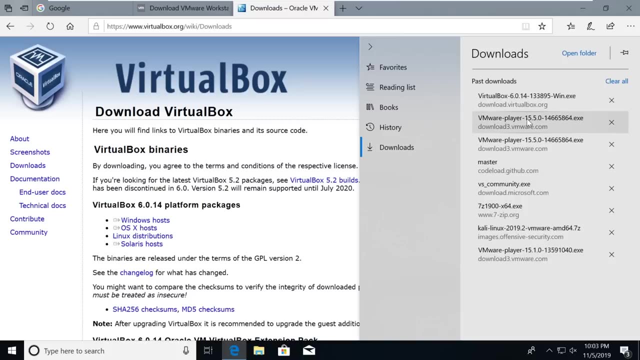 download and go ahead and save it. if you're doing Virtual Box, go ahead and download. for OSX, I will download the Windows version just so that we can- uh, we can- see what that looks like as well, so I'll save both of these. so let's view our downloads. and we've got VMware workstation player. 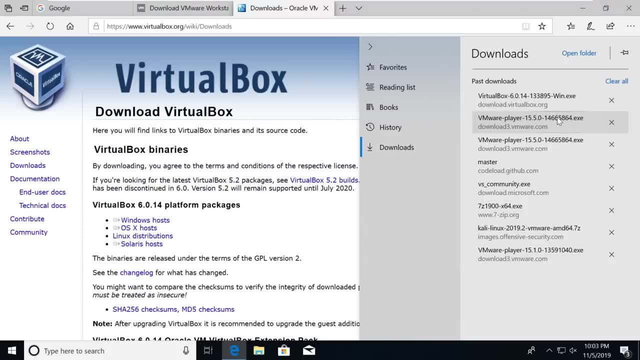 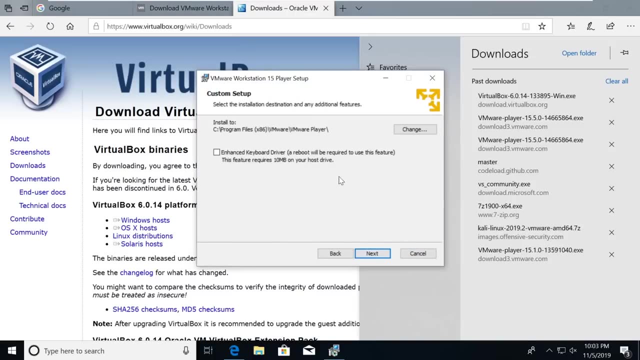 here. I'm going to go ahead and open this one and we're going to install this, and this will be very point and click. so next, accept the agreement, possibly give away our first child. uh, yeah, we should go ahead and install the enhanced keyboard driver while we have this. 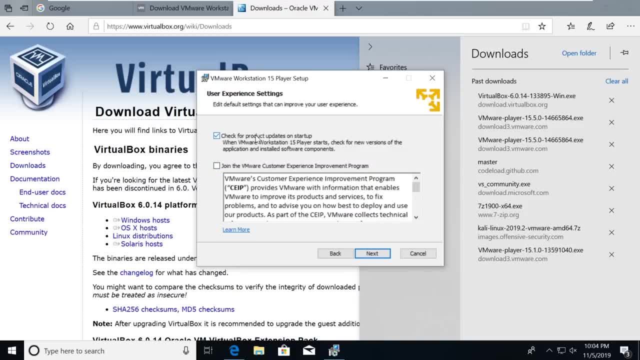 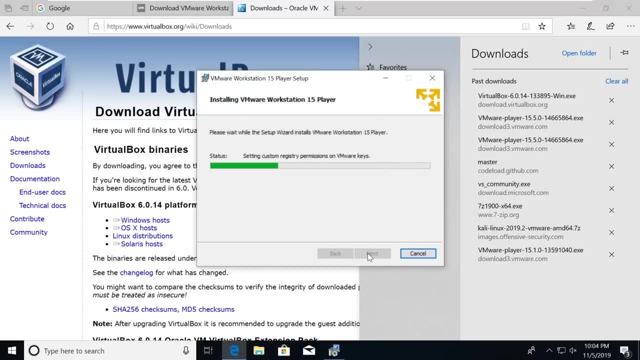 and then we don't need to enjoy, join any improvement programs or check for product update. that's okay, we will install desktop start menu. you check. check your preferences as you like it. I'm just going to install this and this should just finish here in just a second. okay, then you'll be brought. 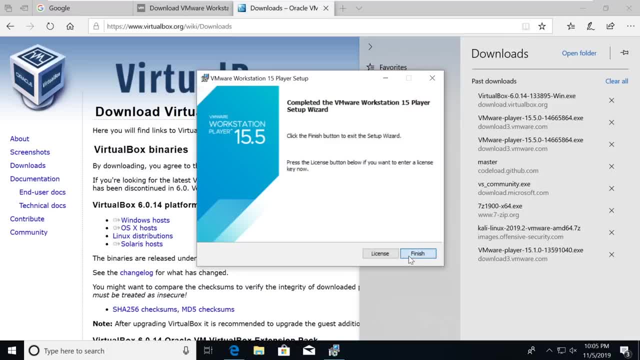 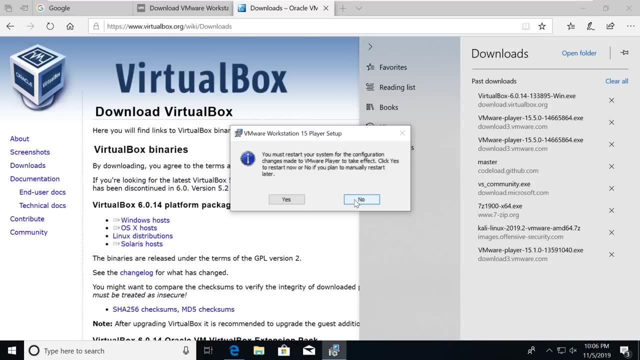 to this screen once everything's done. it should take about a minute or two and we're going to go ahead and hit finish and it's going to want a restart to take effect. you can go ahead and restart your system. I'm going to say no right now. let's go ahead and install Virtual Box, if you are. 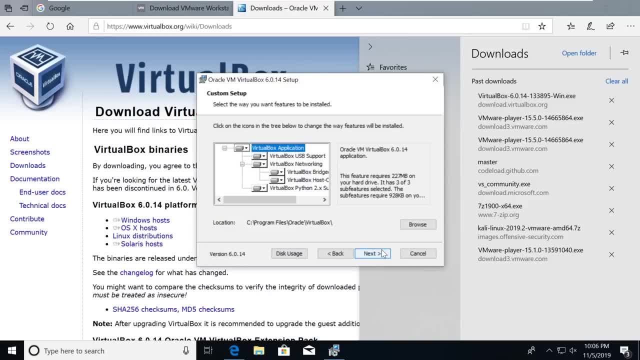 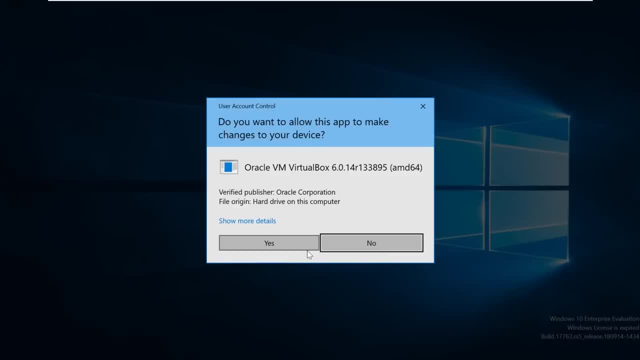 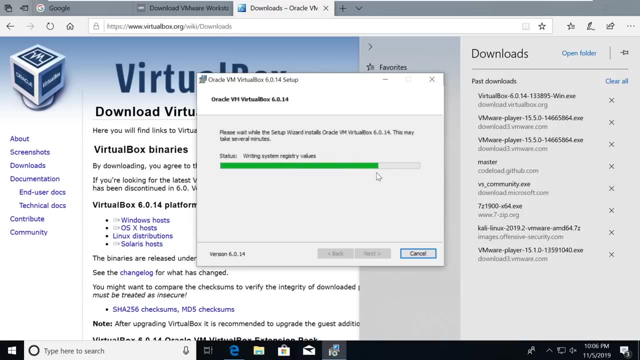 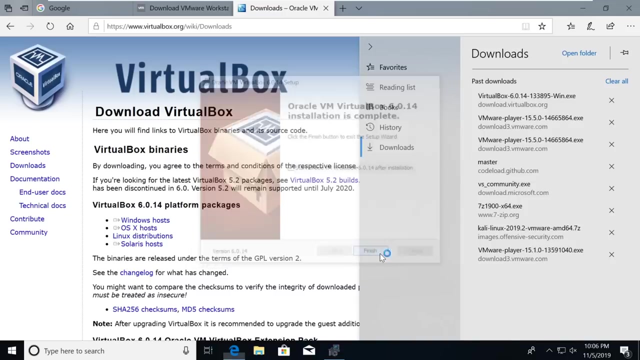 a Mac user, we'll hit next, next here, next and yes and install. accept and again very point and click with the installation, select install and any options that do pop up, and then we can start Oracle VM. if we want, let's go ahead and just start that. this is what Oracle VM looks like. 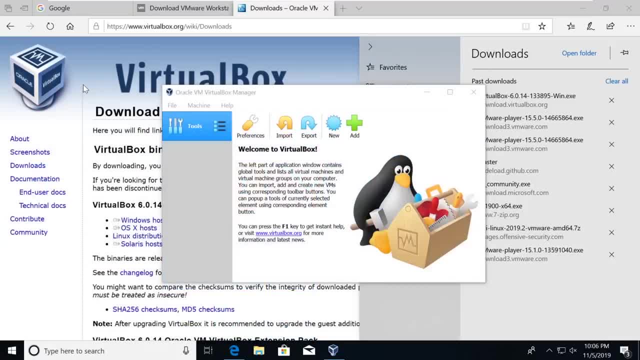 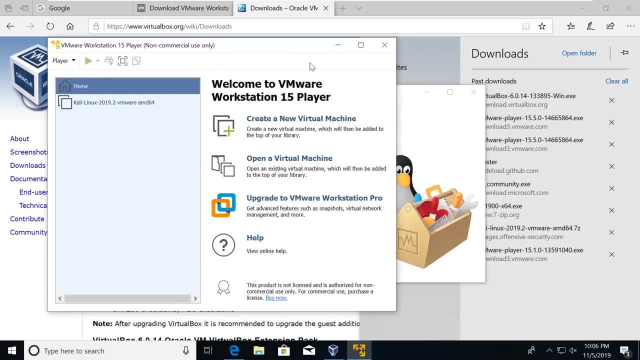 and let's see if we can start the VM player here even though we need to restart, And this is what VMware workstation player looks like. So here you can see that we have virtual machines. we can create new virtual machines, open ones, etc. We'll get into that in the next video. So again, if you're using Windows or Linux, 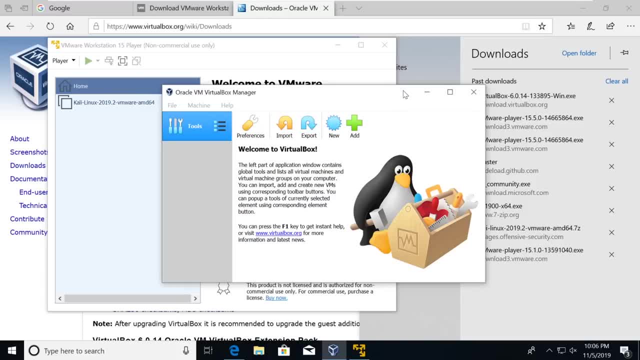 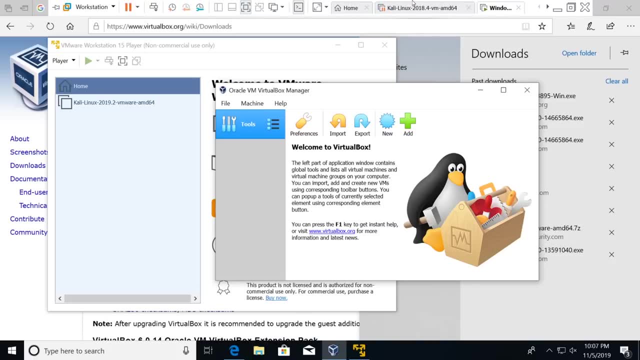 this is probably what your view is going to look like for the rest of the time. If you're using Oracle on a Mac, this is what your view is going to look like. Another side pro tip here is that I am using workstation pro And I might utilize this in. 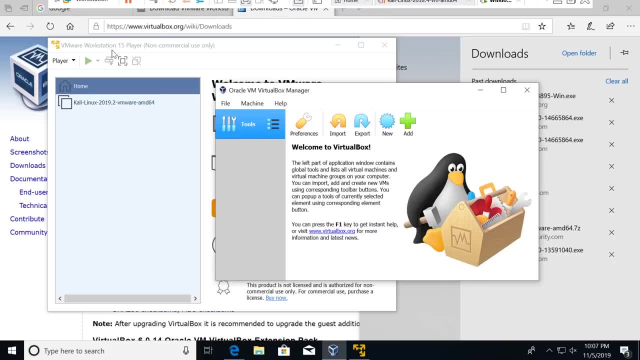 some instances throughout the course. Other instances I'll be utilizing the workstation player. they are not much of a difference, especially in the beginning, when we get into the active directory portion. it might actually be worth it for you all to download the VMware. 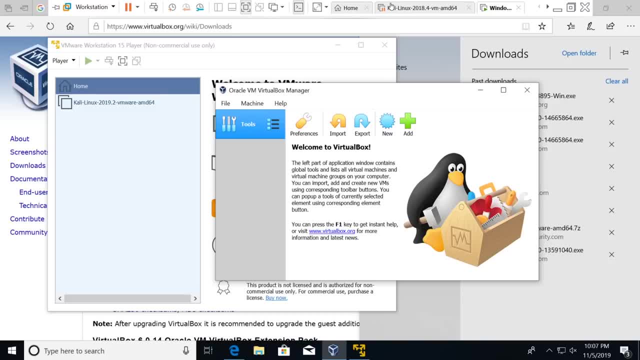 pro trial because the trials 30 days and you can utilize that to get through some sections and actually have nice little windows here, to to be comfortable, clean and just have a pro edition. you can do everything that I'm going to show you in the 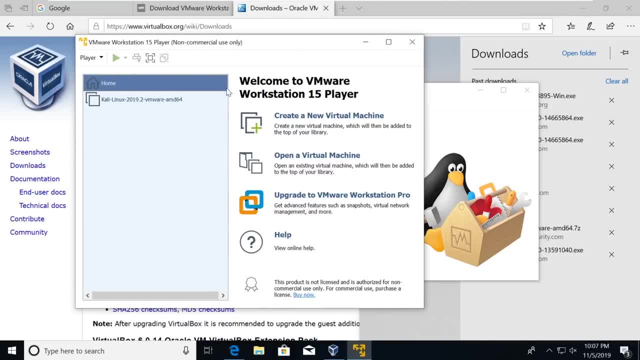 course on the player. it just is that you have to open if you want to run more than one machine. you'll just have to reopen the VMware workstation player several times to run multiple machines. but that's okay. it just won't look like this nice clean layout where you can transfer between 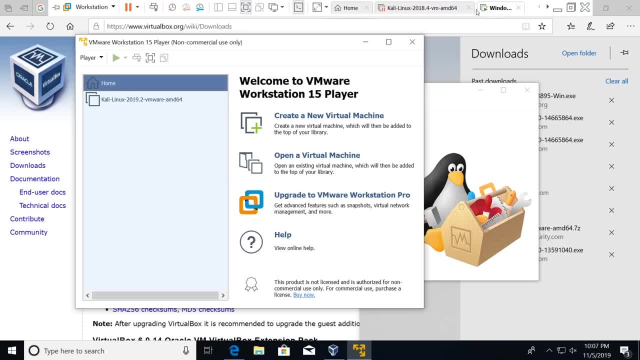 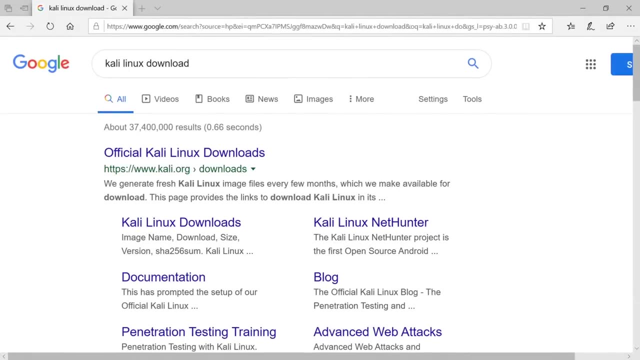 machines like I can do just here. So, with that being said, let's go ahead and move on to the next video. we're going to be installing Kali Linux onto our VMware workstation player. All right, so now that we have our VMware player installed, we're going to need to put a VM on top of. 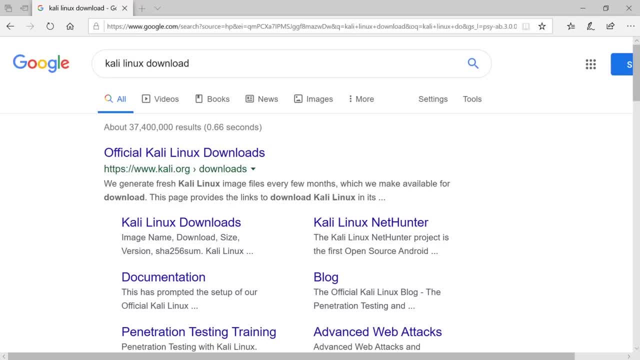 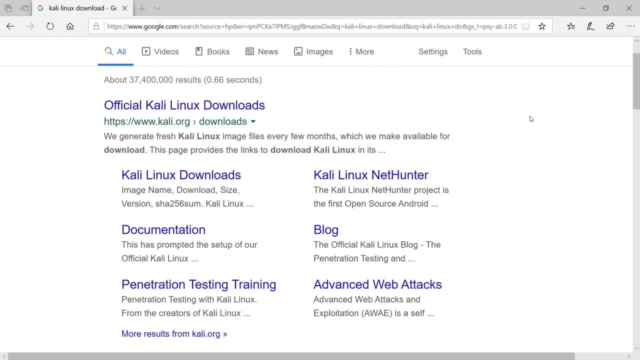 that. So throughout this course, we're going to be utilizing Linux. More specifically, we're going to be utilizing a Linux called Kali Linux. Now, if you've never used Linux before, that's absolutely okay. we have a section coming up on introductory Linux and we'll get you completely up to speed. 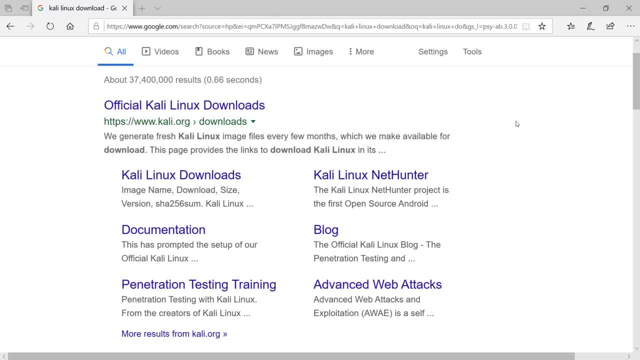 But for now, we're going to be using Kali Linux And we're going to be using Kali Linux and we're going to be using Kali Linux. So for now, we need to be able to install Linux so that we can use it. 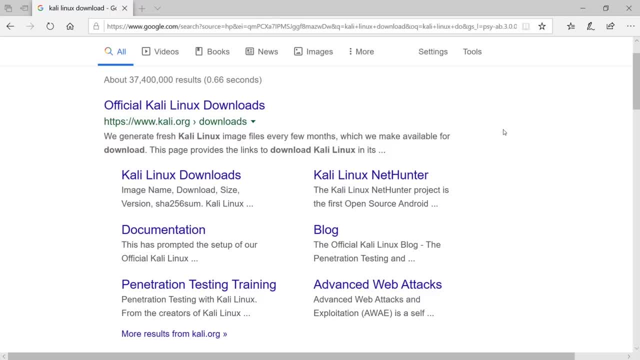 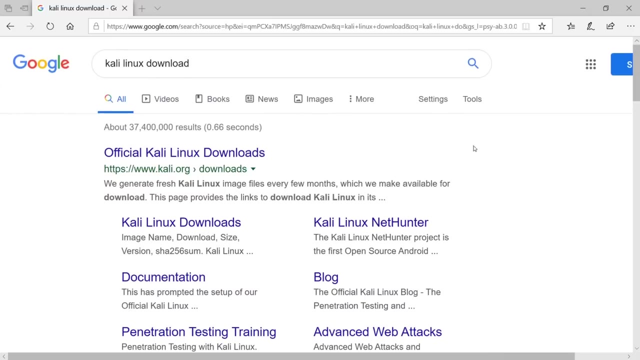 And Kali Linux is a Debian based version of Linux And it is a pen tester Linux, So this is completely built for ethical hacking, as you're going to see once we dive into it. So I've gone ahead and just went to Google and typed in Kali Linux download And if we scroll down, we're going to skip this. 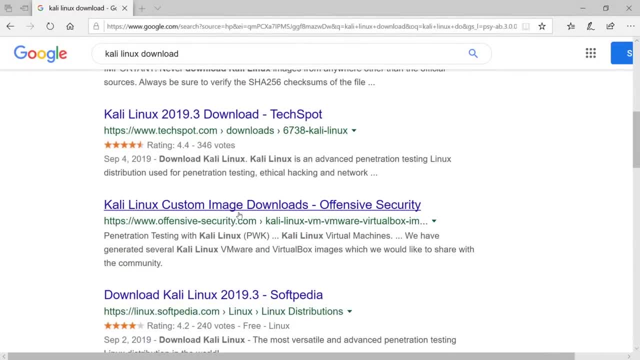 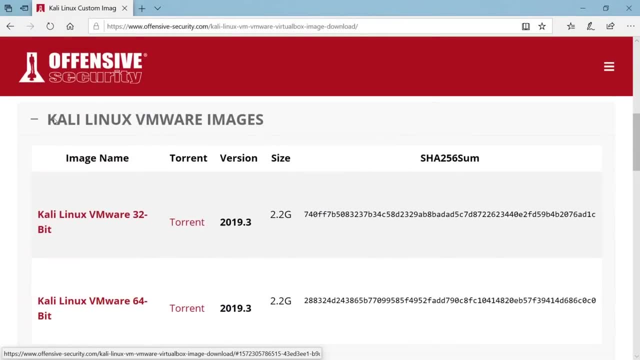 first section here. let's scroll down to this. Kali Linux custom image downloads from offensive security. We're going to go ahead and type in Kali Linux download And if we scroll down, we're going to click on this link And we're going to scroll down a bit And you can see that there are Kali. 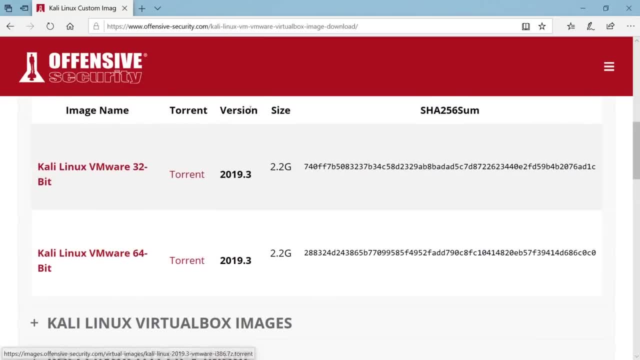 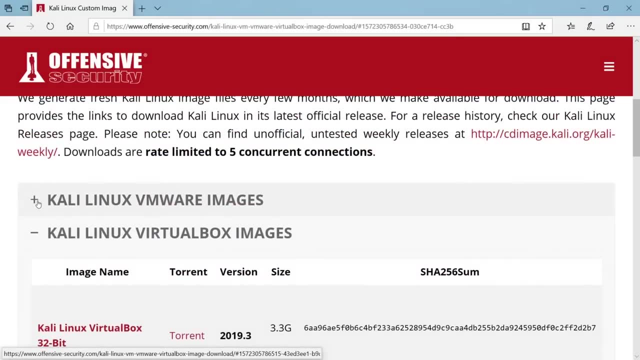 Linux VMware images. Now, if you're utilizing VMware, this is exactly what you're going to use here, And if you're using VirtualBox, then you're going to use this down here. Since we are using VMware, I'm going to go ahead and select the 64 bit download here. So we're going to download 64. 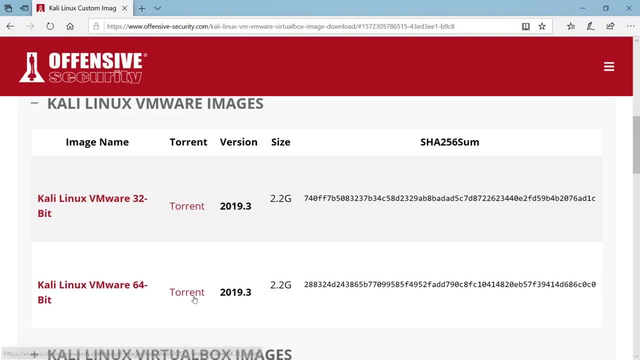 bit. you can either download it just by clicking or you can download the torrent as well. So this is going to download a seven zip file. I'm going to go ahead and type in Kali Linux download And just hit download and save, And this is going to take a second. this is 2.2 gigs, So go ahead and 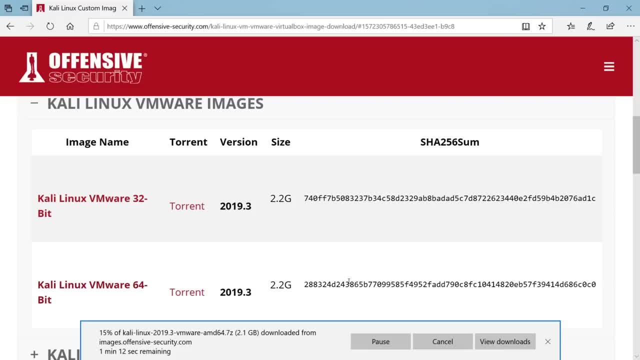 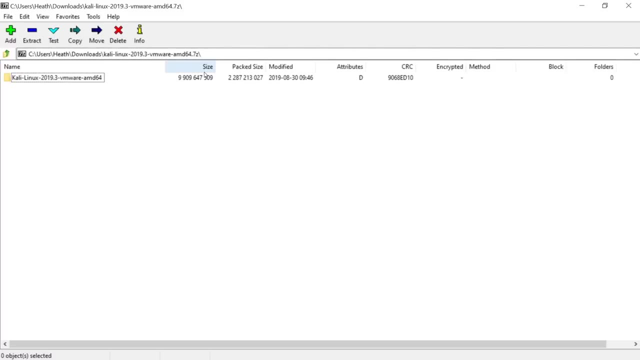 pause the video. Once your download is complete, We'll go ahead and start from there. Okay, so the download has finished And I'm going to go ahead and select open. Now, if you do not have a seven zip installed on your machine, you're going to need to install seven zip So you can go out to. 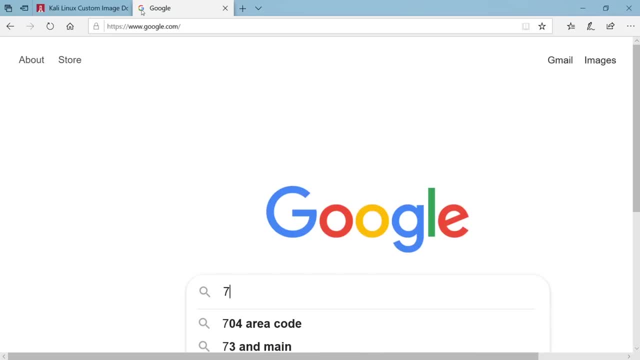 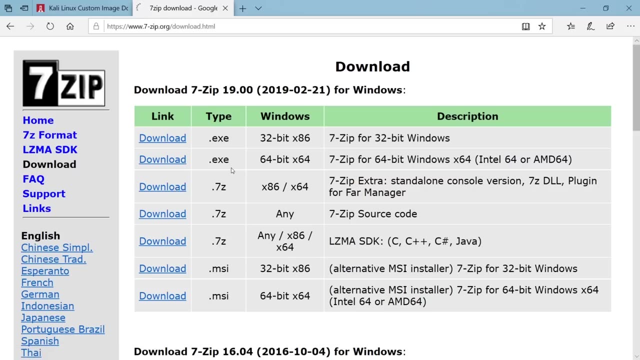 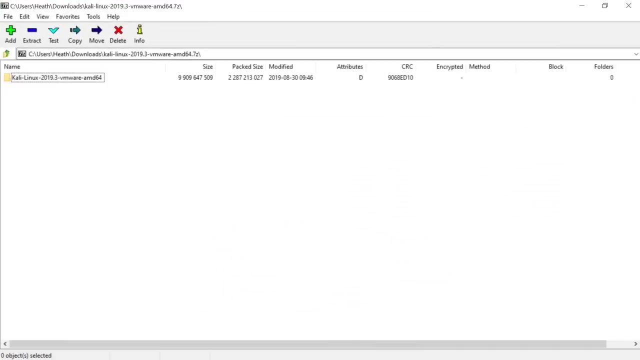 Google and just say seven zip download. And if you go to download seven zip right here, download the appropriate one for you. Here is the executable 64 bit for Windows. So go ahead and download this one, install it again, point and click, and you'll have seven zip on your machine. So once you have, 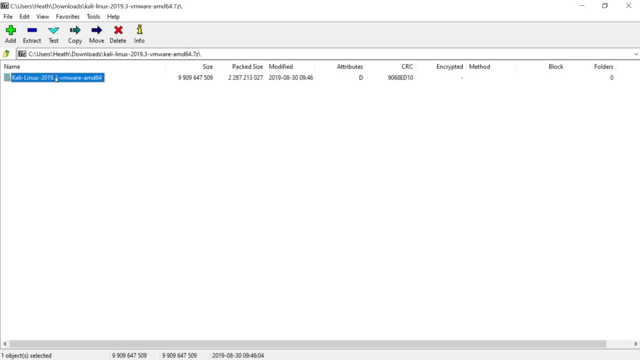 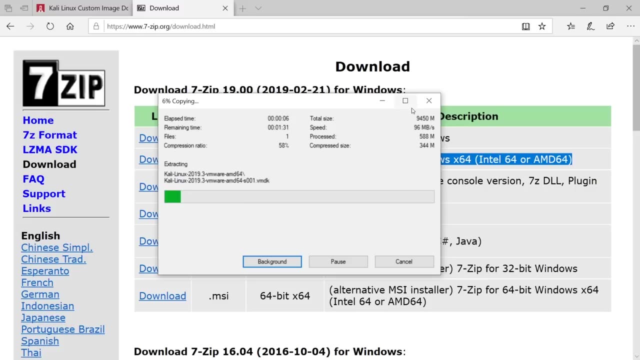 that come back here and we're going to need to extract this. So go ahead and get your file extracted. I'm going to do that really quick And I'm dragging this over just to show you it's going to take some time. I'm just putting it in my downloads folder. So, again, we're just dealing. 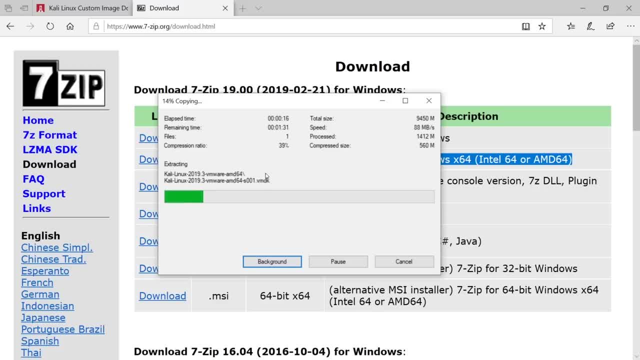 with a lot of data compressed- I think it's 2.2 gigs uncompressed, around nine or 10 gigs- So make sure you have the space as well when you do extract this. So once this is done extracting your machine, go ahead and unpause the video and come back and then we'll actually get Kali Linux up and 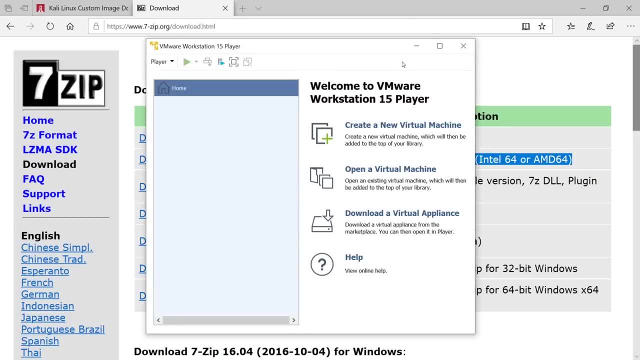 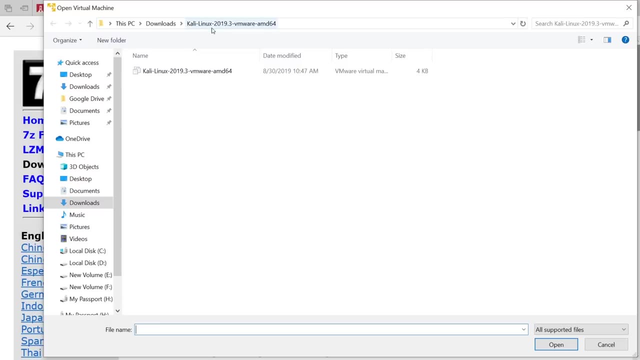 running Okay. so now I've got my VMware Workstation player open, our files are extracted. I'm going to go ahead and just select open a virtual machine, And I've navigated to the folder that I needed to get to, which is just my downloads folder, with this Kali 2019.3.. I'm going to go ahead and open that. 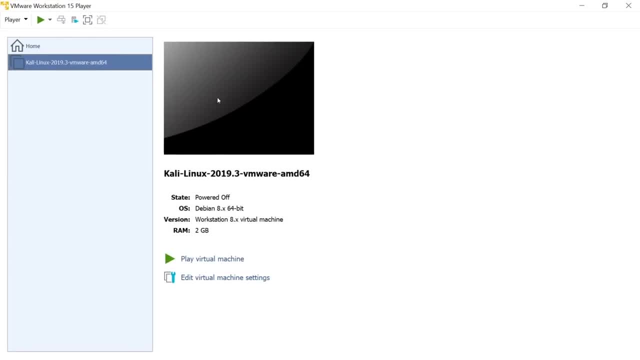 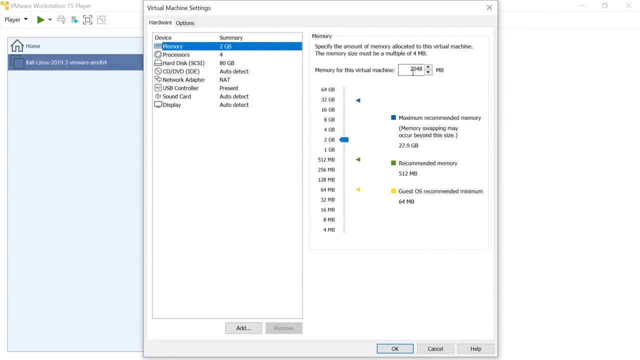 And now you should see the files open. Before we go ahead and do this, let's go ahead and just select open a virtual machine settings, And there's a couple things that we need to talk about in here. So the amount of memory that you allocate depends on the amount of memory that you have. So here it. 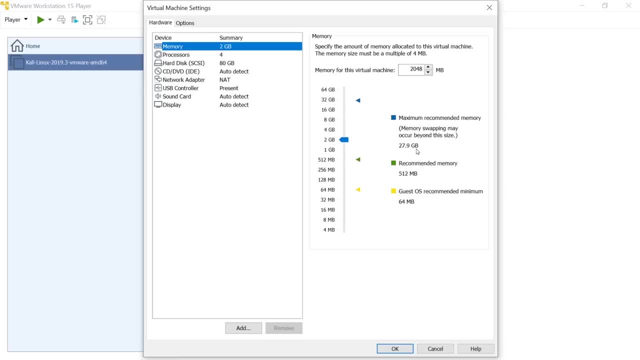 tells you the recommended amount and the amount that you have maximum available. So for my system, for example, I have 32 gigabytes of RAM. Now I would probably give this machine somewhere between four and maybe eight gigabytes. I would say four gigabytes. 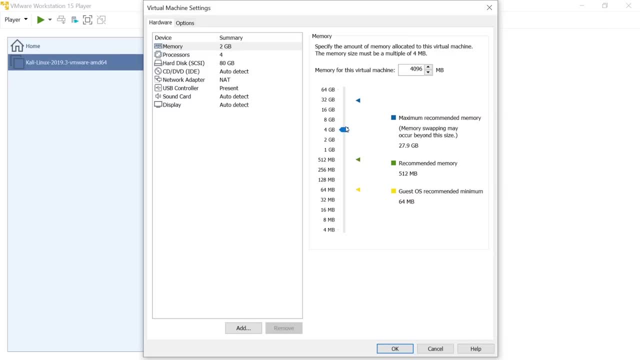 I would say five gigabytes. So if you have a little bit of RAM or you do not have a lot of RAM, go ahead and leave it at two gigabytes. Two gigabytes is fine. you might notice a tiny bit of slowness. 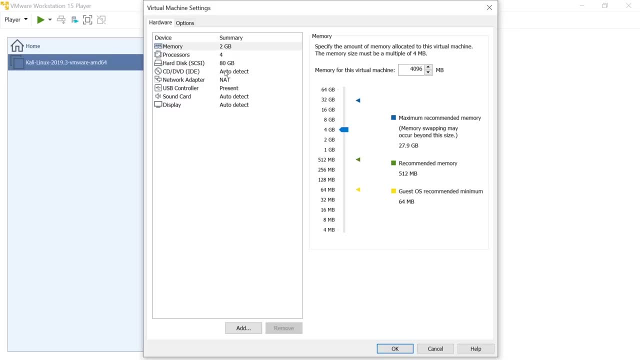 but it's nothing that's going to keep you behind by any means. So I'm going to bump this one up to 4096, which is four gigabytes, And I'm also going to take a look at the network adapter. Now we 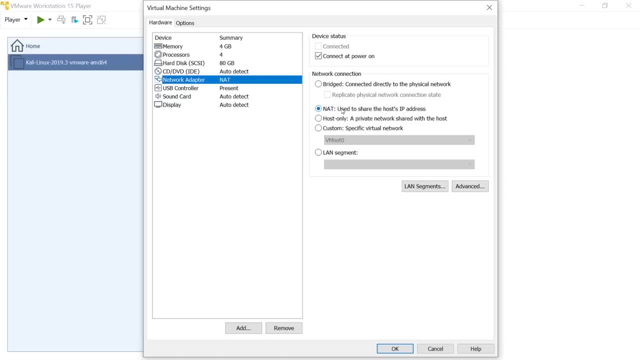 haven't gotten into networking yet, But we're going to cover some of these topics. So nat or we can use Bridge, Go ahead and leave it for now at NAT. If we need to change it to Bridge later, we will. NAT should be perfectly fine. If you don't know what NAT is, that's okay, We're. 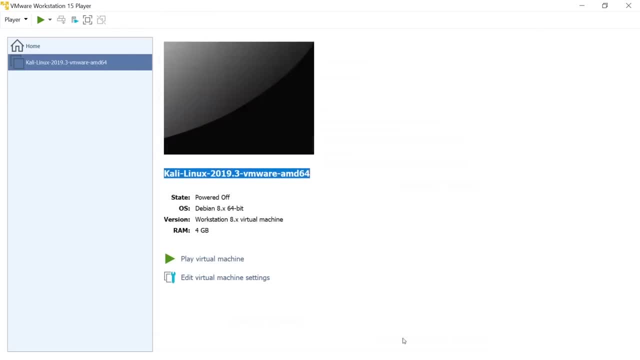 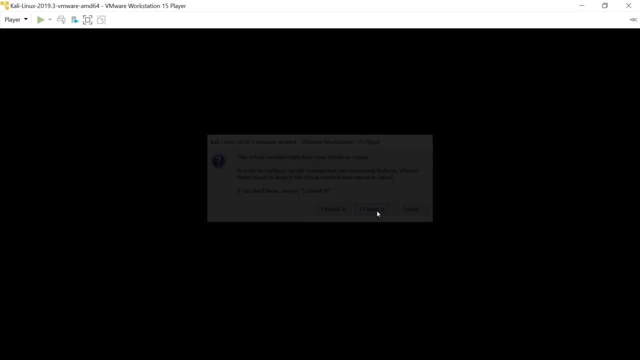 going to cover that here in a little bit. So we'll select OK and we're just going to hit Power On. And when you get this prompt, all you have to say is: I copied it and it's going to boot up your Kali Linux machine. Now, this is the first time booting it Sometimes. 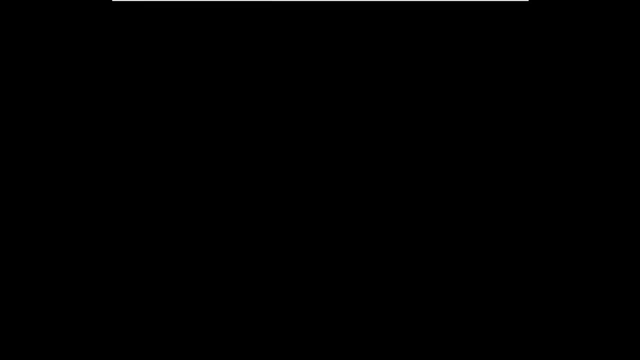 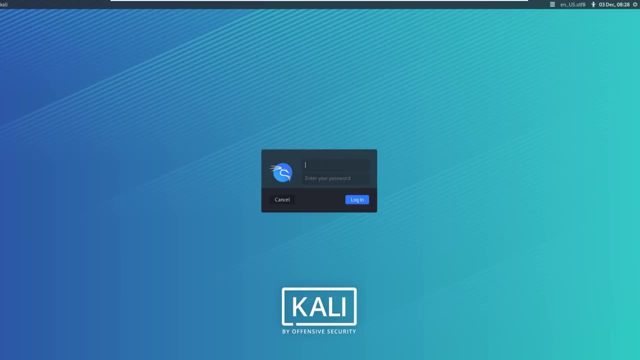 you can full screen it. sometimes you can't. As of right now, we just tried to full screen. it doesn't work yet, So go ahead and let this boot up. it shouldn't take but just a second. Okay, and now we're going to be brought to this login screen here And the password is going to 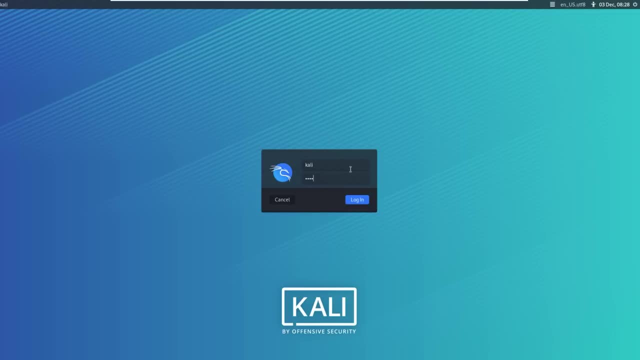 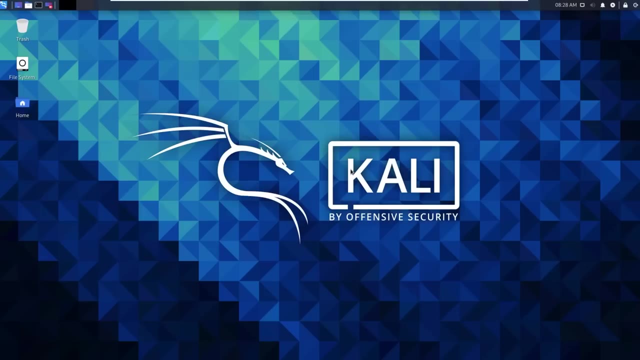 be, or the user is going to be Kali, password is going to be Kali And you just log in. might take a second to log in on the first. go Now. you'll be brought to this screen Now. what you may or may have not noticed is that 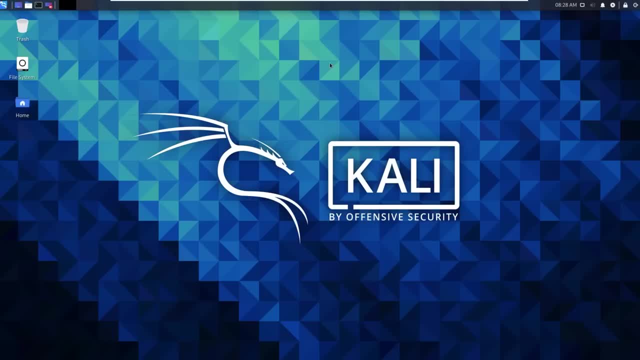 this is a perhaps different version of Kali that you're running. Things do change as the videos go on. What you're hearing on this video is actually an update from where we were at As you saw me installing. I was installing 2019.3.. As we are working through the course, 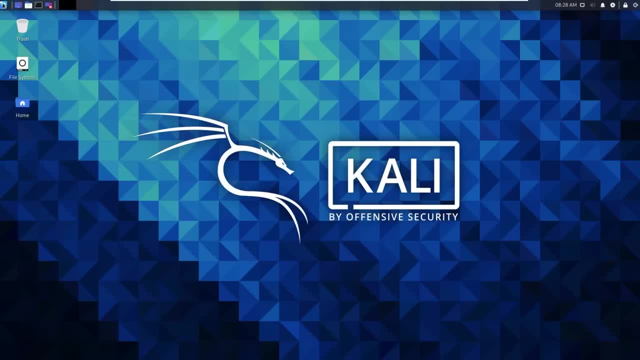 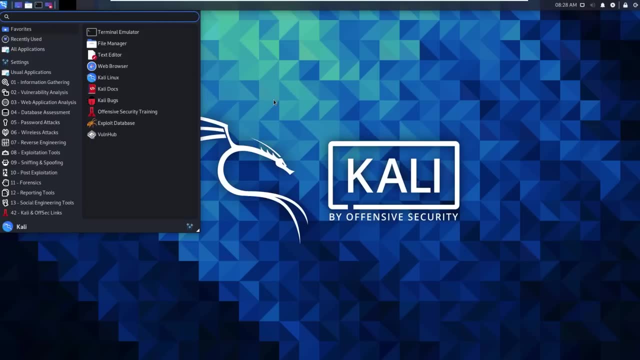 I'm actually going ahead and doing updates. So this is now 2020.4.. And we are adding updates to the course. So the notes that I have for you before we move into Linux section is: if you're installing Kali and it looks a little bit different, that's okay. These versions do change. 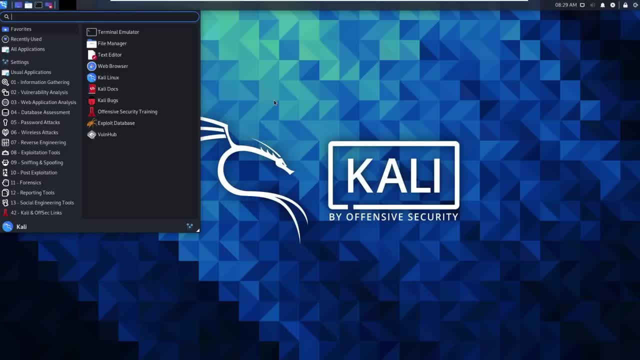 over time. Sometimes they do get major updates. When that happens, I update the course. Here we are on the latest and greatest as of right now. So this is kind of what it looks like, but don't be to worried if your image or background or things look a little bit different. Everything that. 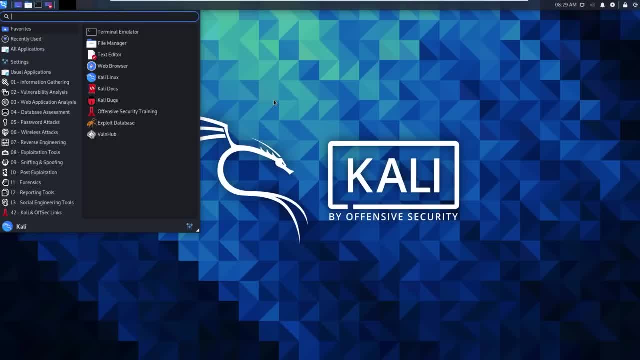 you're going to learn is 95% the same for the most part. So let's go ahead and move forward. We're going to go and move to the next section. We start talking about Kali Linux and we start talking about an you- what Kali Linux is and how to navigate around it, And we'll talk about Linux and Linux commands. 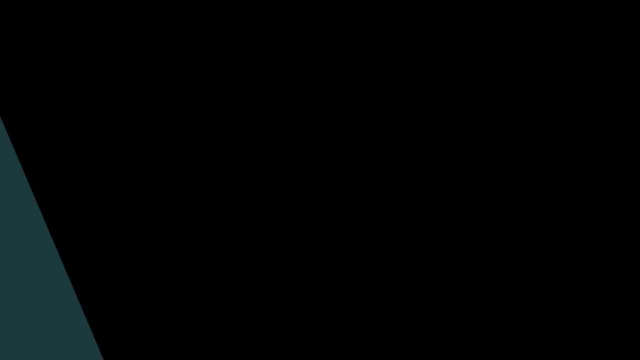 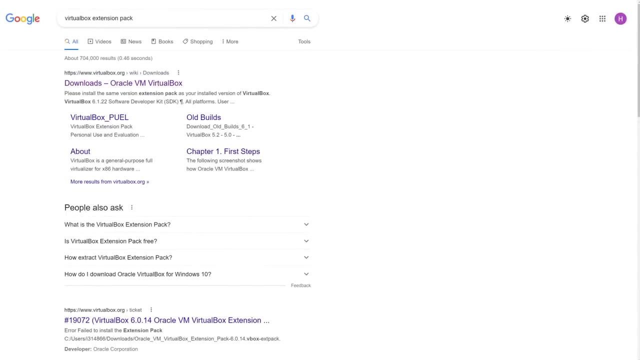 as well, So I look forward to seeing you in the next section. Okay, so this video pertains to some updates we need to make to VirtualBox for quality of life. So if you're not using VirtualBox, you can go ahead and skip this video. If you are, buckle in. we just need to do a couple. 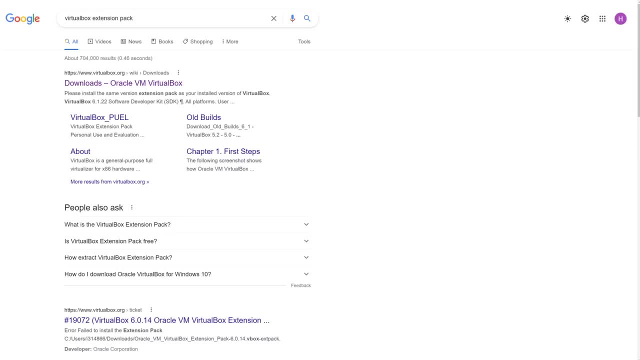 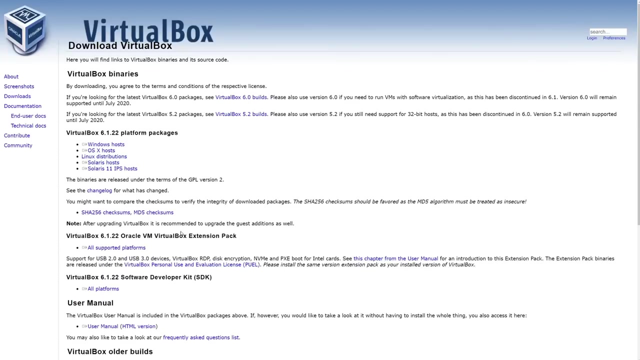 of quick updates and then we should be good for the rest of the course. So go ahead and go out to Google and Google VirtualBox extension pack. what it's going to bring up is just the downloads page of VirtualBox. So we're going to want to go here And on this page. if you look kind of towards the 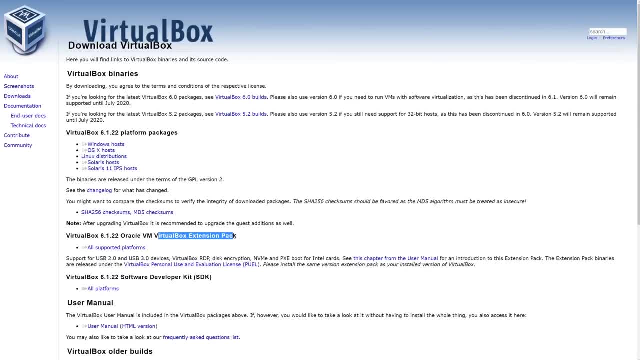 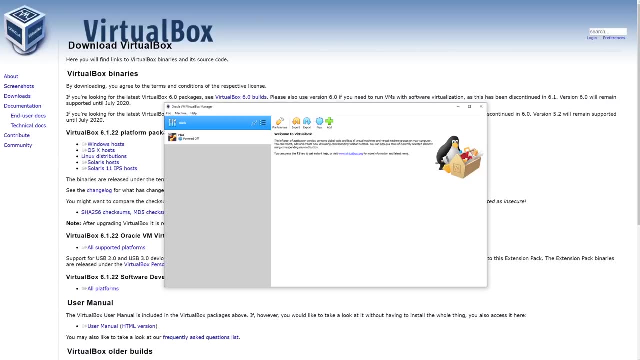 middle you'll see that there is a VirtualBox extension pack. here we're going to just click all supported platforms and that will automatically download the file that we need. So once that is downloaded and pause if you need to go ahead and open VirtualBox And you can come. 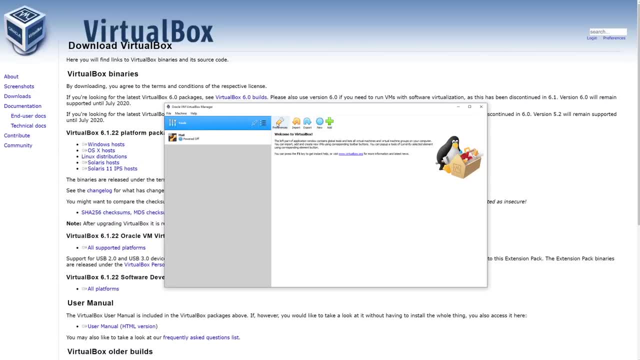 in here And up at the top we're going to go ahead and click on preferences, And from here we are interested in extensions. see extensions right here. go ahead and click on that. There's a little plus sign. we're going to go ahead and click on that And then you should have your. 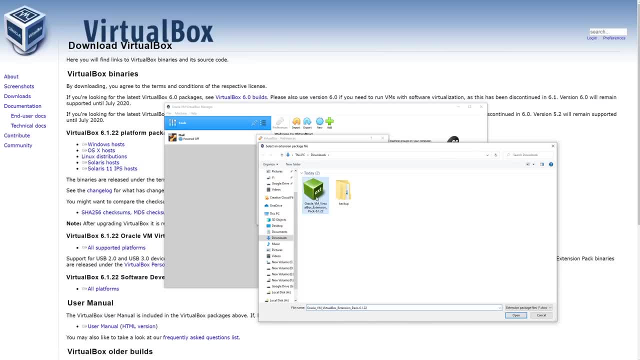 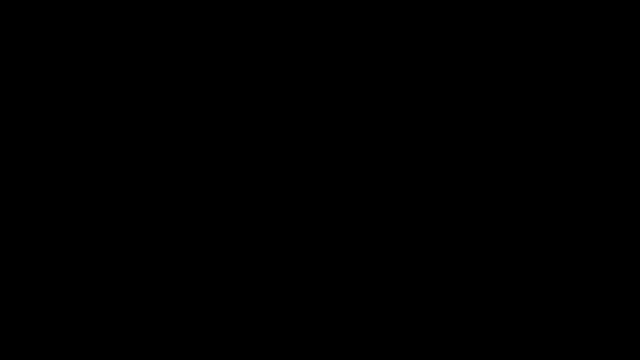 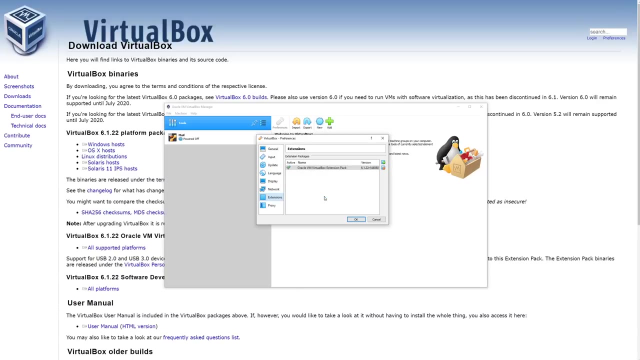 downloads right here. So we're going to take the downloads and just go ahead and install that. hit install, Read this, give away your firstborn, accept all the terms and you should be good. very quick install, Okay. The second thing we need to do is we need to come to the one tab up here above. 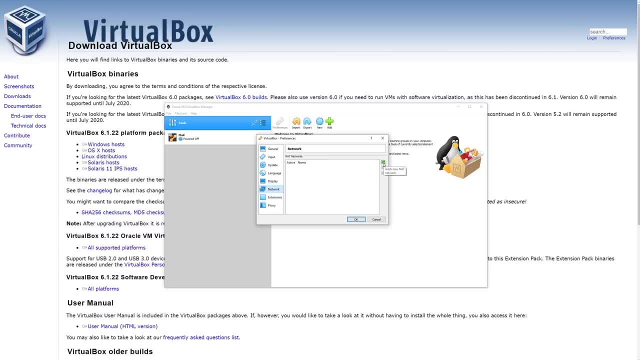 which is network. we're gonna go ahead and hit the network button or this Add button, and we're going to add what is called a NAT network. Okay, and we're going to come in here and we're going to double click And you can go ahead and keep the. 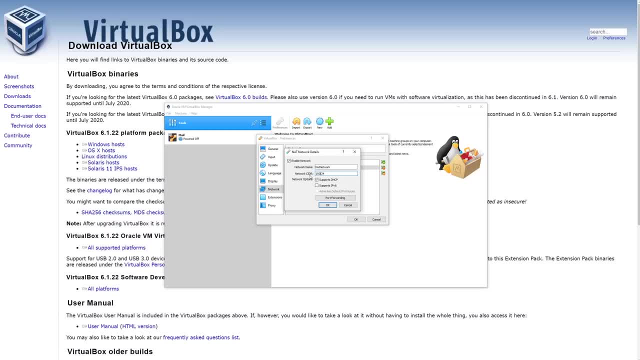 ones in these defaults. I'm going to actually change them to 1920, 168 dot. 57.0.. Because that's what's going to be used through the rest of the course And that is what the cider notation of my Kali machine and my key objects, which you'll see later, etc. all fell into this 57.0.. So we're. 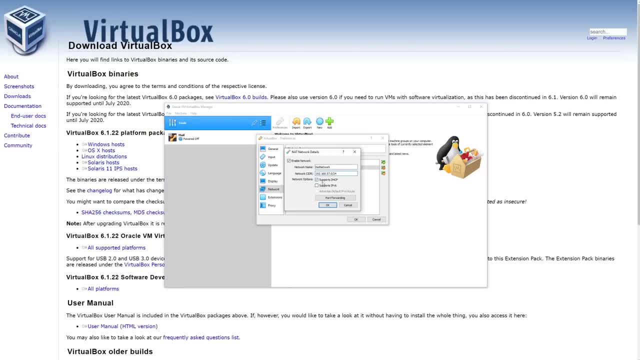 going to go ahead and keep it on this NAT network. make sure you support the HCP. go ahead and just hit okay, hit OK. And then for a machine And make sure any that you use again, any machine that you use in this course, make sure you set it to NAT network. 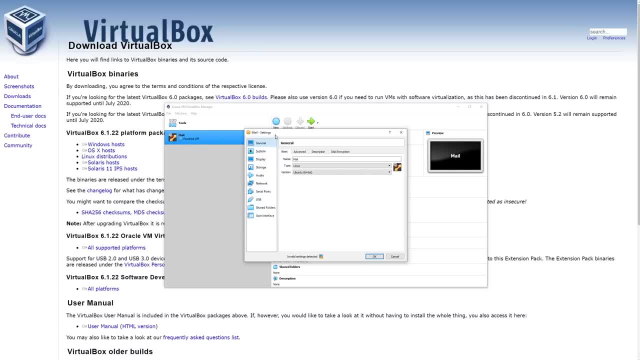 if you're using VirtualBox So you can come in here, click on a machine like this mail machine I have here. you can just click on that settings, go to network And then you can go ahead and just go to NAT network. All right, And that name. right here you see. name: NAT network. that's all we're. 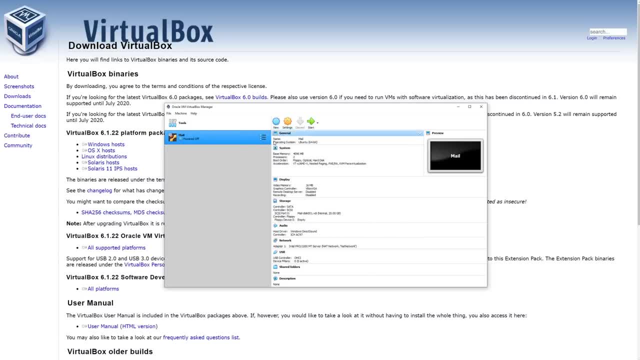 going to use, that'll automatically set it up. So when you have a Kali machine running later and you have key optics or another box running, or even when we build out an active directory lab, you need to make sure that you're running that NAT network so that all the machines are on the same. 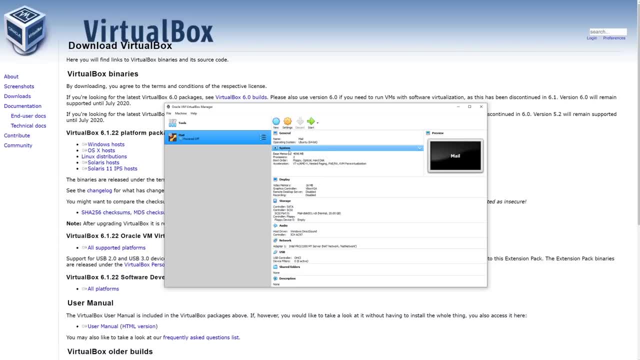 subnet. If you don't, you might run into a situation where the same IP comes up for the same machine and then they're conflicting with each other or you get on different networks and some weird stuff happens. So make sure again that it's imperative that you're setting. 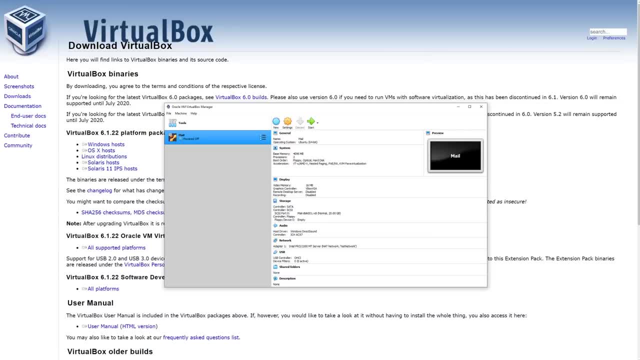 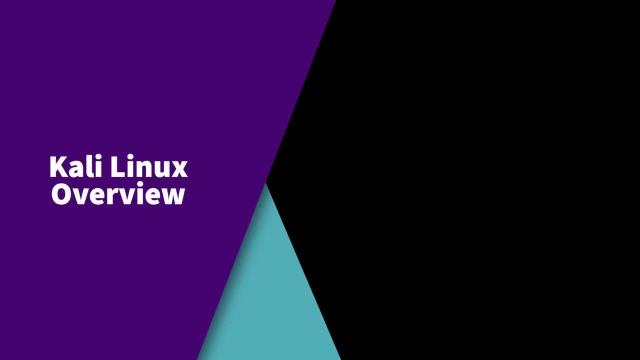 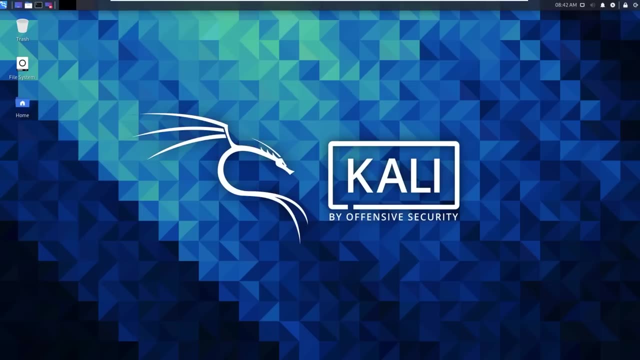 that NAT network for every single machine that you're setting up. So, with that said, we're gonna go ahead and move on to the next video in this section. The first thing I'd like to do before we get started with any commands or anything like that: 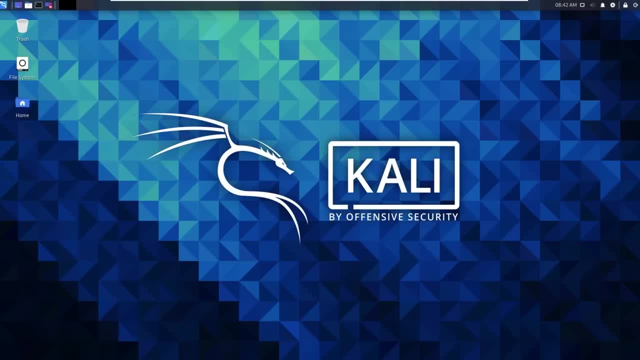 is: just take a look around Kali Linux and kind of demonstrate why a pen tester, ethical hacker, might use this distribution of Linux. Now, throughout the course, as stated in the last video, you might see a different version of Kali Linux. So if you're using Kali Linux, you might see a different version. 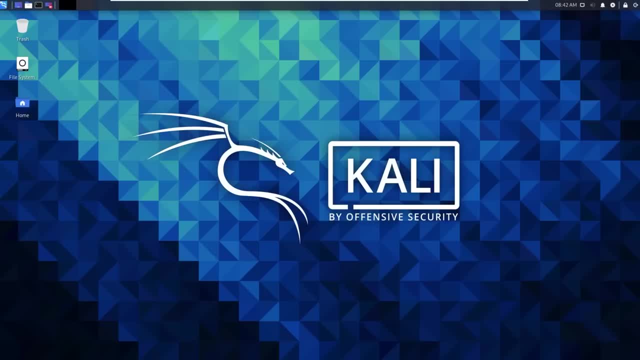 of Kali Linux. So if you're using Kali Linux, you might see a different version of Kali Linux And you might see a different version of this pop up. as I recorded videos on some of the older versions, everything should still work just as is. you just might see a different look and feel to some of the 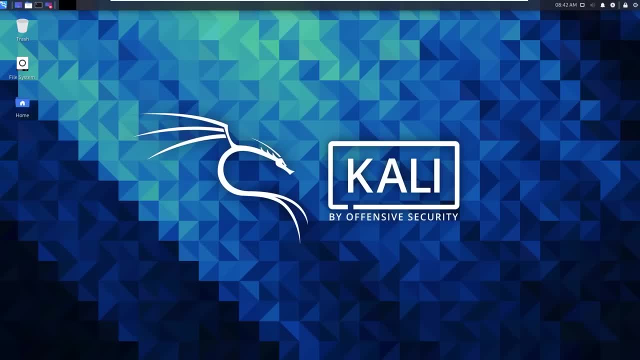 Kali interface, But all the commands I'm going to show you, everything that we do, is going to be the same. So let's take a look and just explore Kali Linux just for a bit. So if we come up here into the corner and we just click on the little Kali logo, you can see that we have nice things broken. out for us. So we've got these favorites of Linux, and then we have a little bit of Warwick, and then we have, And then we have a little bit of Kali Linux, And then we have a little bit of Kali Linux, And then we have. 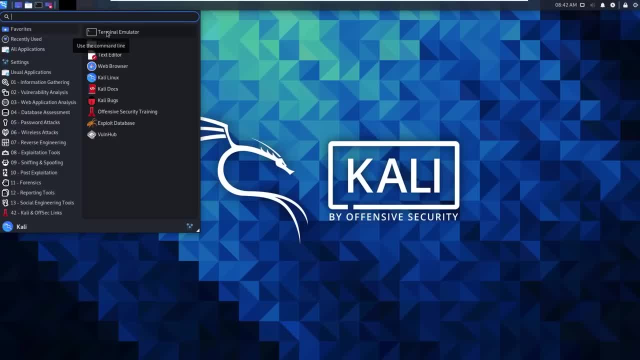 here which we have our terminal, which we're going to be living in. essentially, we've got a text editor, we've got a web browser, which is basically firefox. we've got some other tools down here: docs, etc. the other thing that we can come scroll through is we can see that we have different. 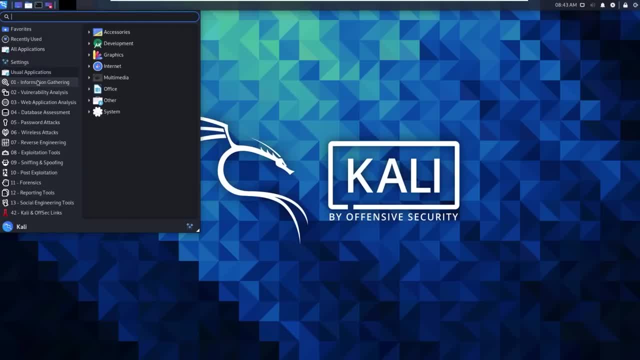 applications in here. if we look at the different sections, these kind of go in order which we haven't covered quite yet, but in the order of how a hack might go down. so information gathering is usually the first step. you can come in here, look through this and here's a bunch of tools related. 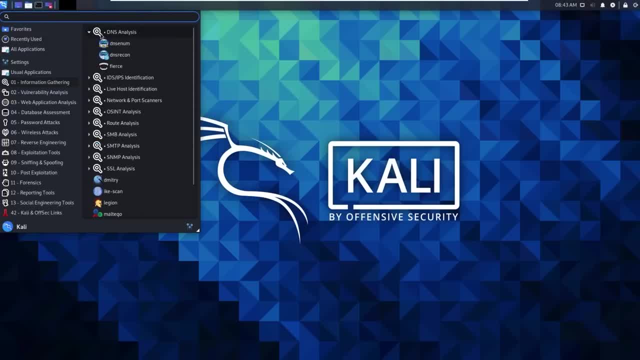 to information gathering. you can even click into these and go deeper if you wanted to, related to specific things. so dns or smb or open source intelligence, all of this that's in here. this is just built in tools. so let's say we're coming in here, we want to do a wireless attack. well, we. 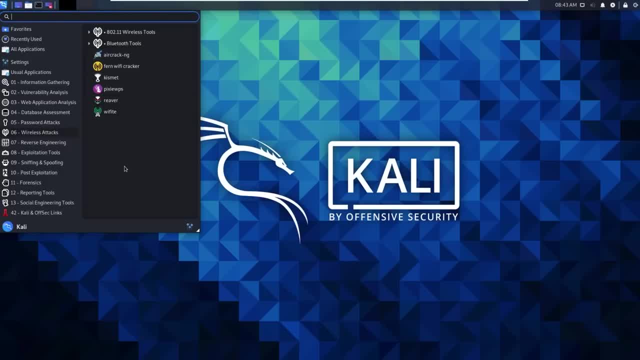 go to wireless attacks. got a bunch of tools already built in, so kali linux is just essentially a ethical hacking distribution of linux, and it's built on debian. so if you've ever used something like ubuntu or anything along those lines of a debian distribution, this is all going to feel. 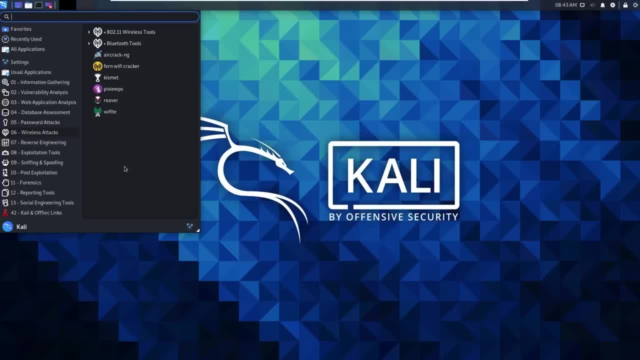 really familiar to you, with just a bunch of tools built in on top of it, so fairly straightforward. they do have some nice tools in here. you can come through and utilize these. a lot of this is already built in and we're going to take a look at that as we go. okay, so the 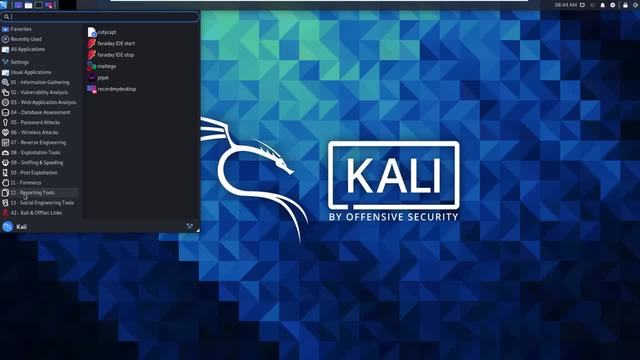 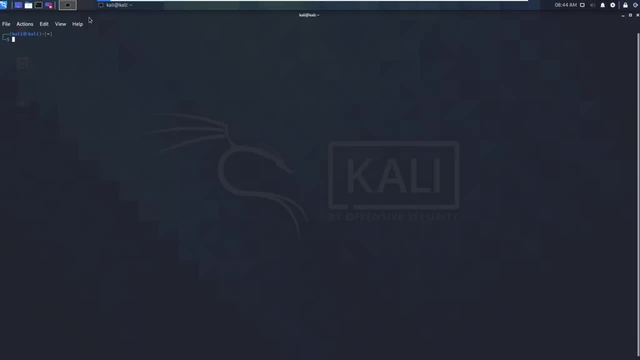 next thing that we're going to do is- and throughout the rest of this course- is start looking at the terminal. so if you come up here, you'll see that we have a terminal now. mostly everything that we do is going to be done in this terminal here now. this is almost like accessing the command line. so 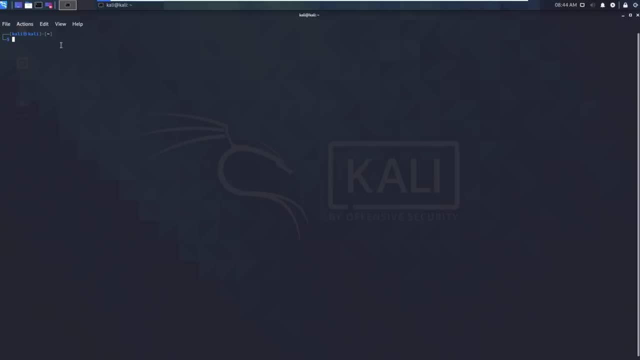 if you're using a command line, like in windows, for example, if you ever use a command line. if not, that's okay. but we do a lot of this from this interface as opposed to maybe utilizing a gui based interface where, if we clicked a folder, this might look more familiar to you if you're a windows. 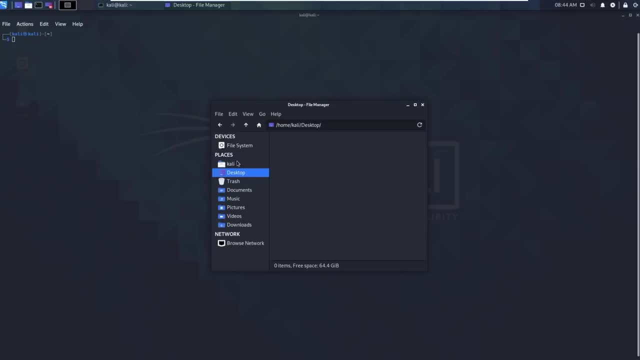 or mac user. we come in here and we're going to go to the command line and we're going to go to the command line. here. you have this kind of area, yeah. yeah, we can do that and sometimes we'll utilize this, but a lot of times we're going to be living right here, okay, so, as we move forward, we're going. 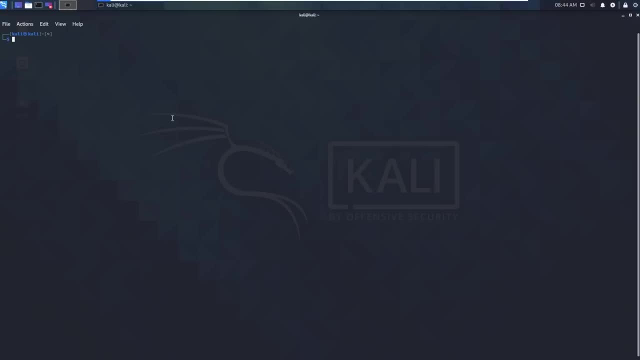 to start talking about this command line, how we can utilize it and use it to our advantage, and then we'll do some tips and tricks and hopefully learn some pretty neat stuff as we go. so in the next video i'm going to cover the sudo feature, which i think is important. it's something that 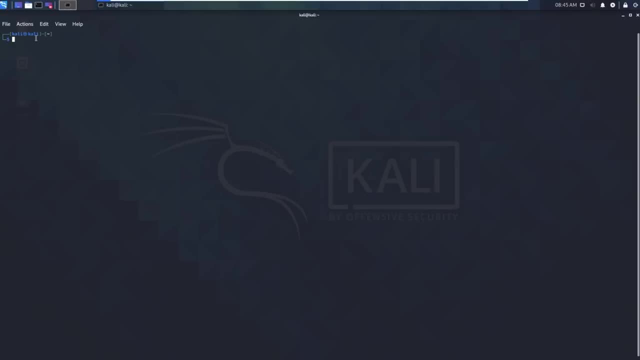 was brought in now. originally we had something called a root permission and we'll talk about that in a little bit, but the root permission has changed since 2020.1. moving forward, so we're introducing that into this course and we'll talk options that you have. so let's go ahead and move. 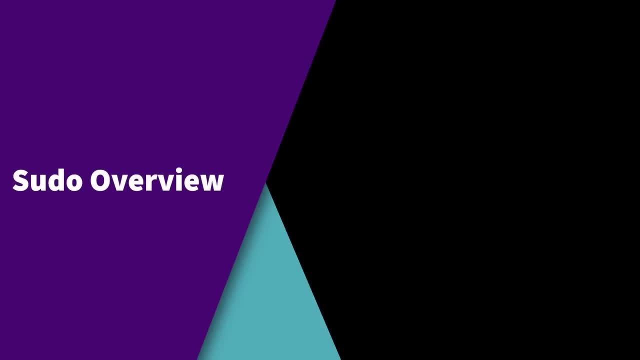 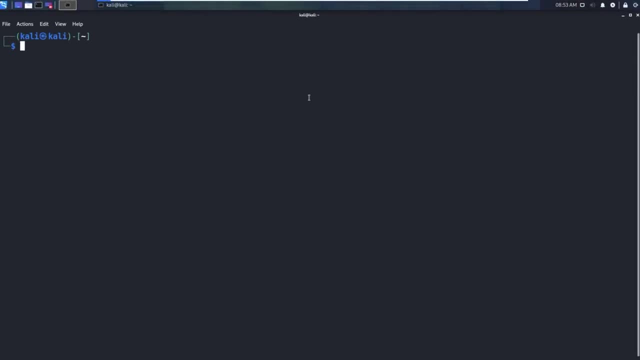 to the next video, where we talk about the sudo feature. all right, so before we look at any commands or learn any command line, we have to talk about sudo. sudo is very important, and what had happened previously, the earlier versions of kali linux, we ran as a user called root. root is the ultimate user. you. 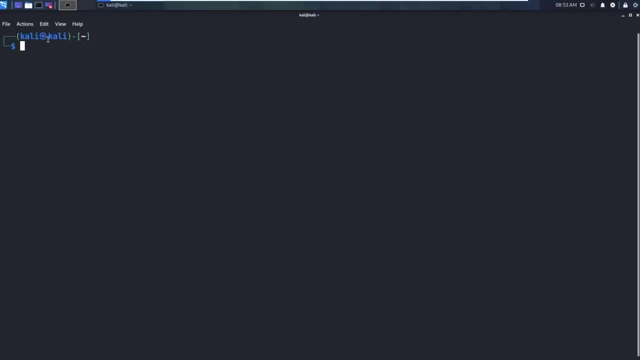 could think of it as the administrator of the machine. now we're running as a user called kali, so we don't have root privileges directly. this is as an improved security feature, because we should be running only certain commands when we need to as the root user. so what we're going to. 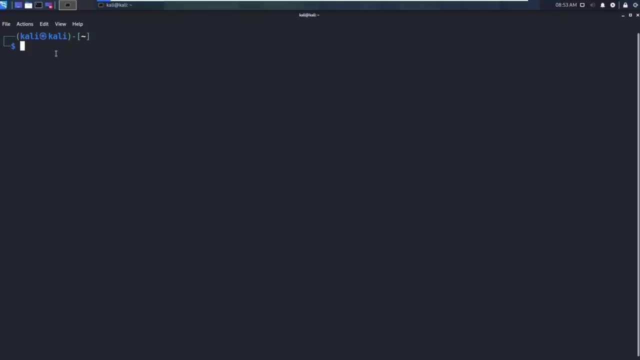 see is we're going to see how we can run commands as an elevated privilege, and we're going to do that with sudo, which stands for super user. do they just kind of shortened it so we just have sudo now? okay, now with sudo, what we're doing is we're saying, hey, i want to run a command. 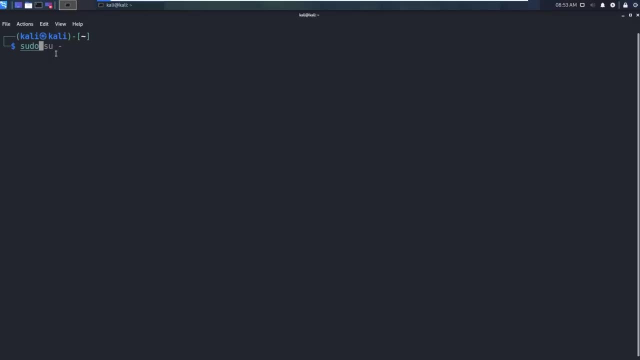 elevated. i want to run this as a higher user. in this instance, we can say: i want to run the command as root. why is that important? well, let's take a look at an example. let's say that i wanted to look at a very sensitive file. now, one sensitive file in our system is the etsy shadow file. you can 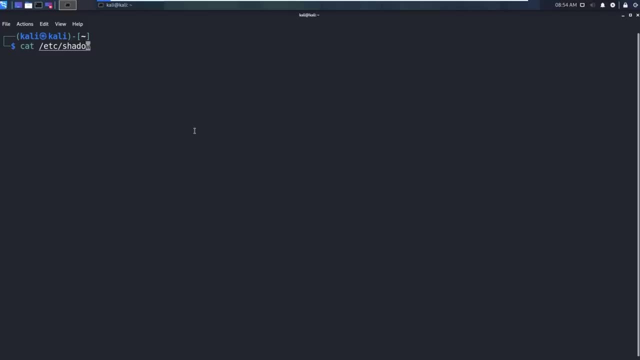 see cat etsy, like this etsy shadow, and you don't have to follow along right now, you don't have to really understand what's going on if you've never seen linux. all i'm doing is saying, hey, i want to print out this file, i want to look at it, okay, and for here i can't see it. it says permission. 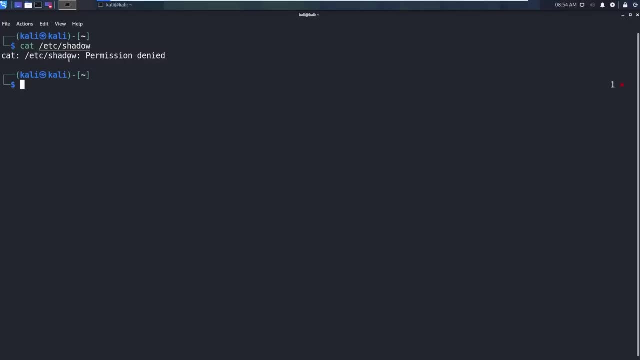 denied. you don't have the access to see this file. that's a good thing, but if i was the root user or somebody that had elevated privileges, i could see it. so i could say: sudo, cat, etsy, shadow, like this, okay, and it's going to say: what is your password for kali? i'm going to go. 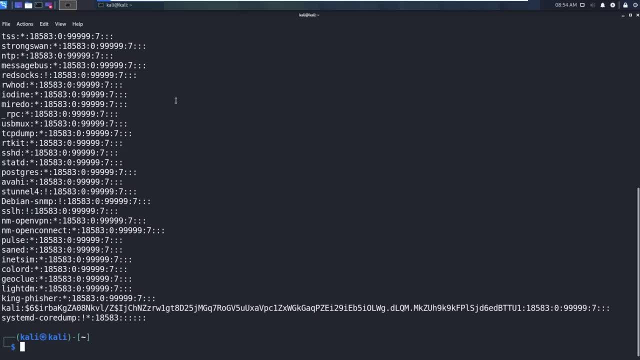 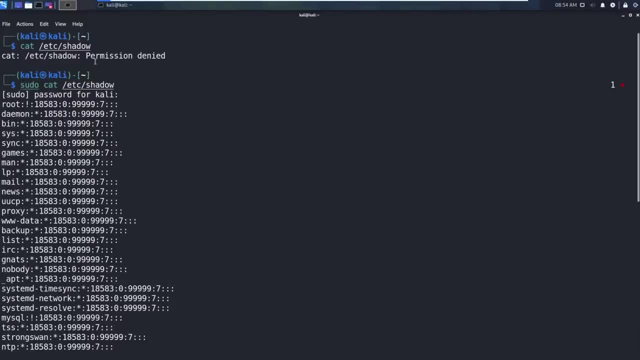 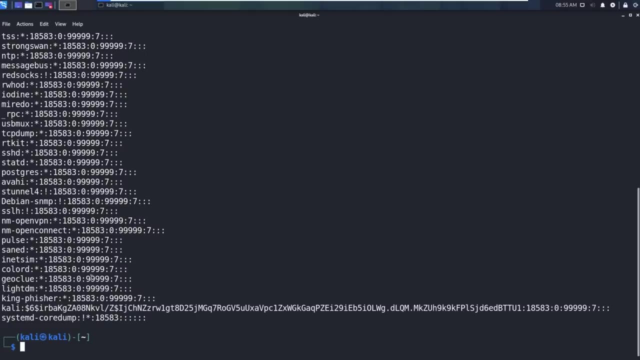 ahead and say kali k-a-l-i, hit enter and now i can see that i have access to this file and this file is very sensitive- we'll talk about this later on in the course, but sensitive file okay. so when we're looking at it, i ran that command specifically as the root user. as the root user. 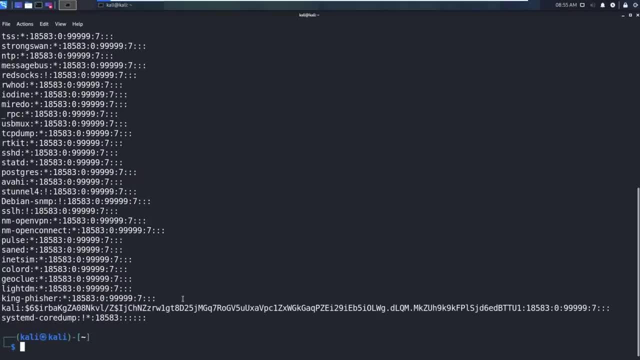 i'm able to see, okay, this file. now why, or what's going on here? well, we're running that specific command right and we're still staying as kali. we're doing this in a kind of one-off scenario. so there will be times where something that you run in this course might require sudo or 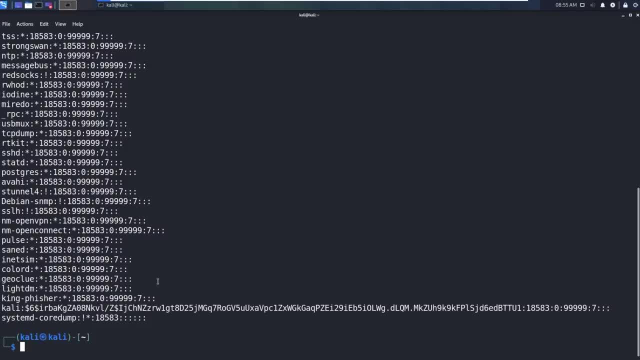 you can run the command without sudo but you notice something doesn't work. so best practice for this is saying, hey, let's go ahead and just run mostly everything you want to run. that I'm showing you command wise in this course. that's not best practice overall. usually you should run things just as a regular user, if you get. 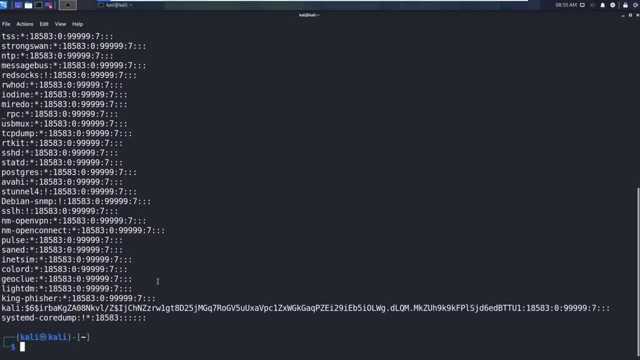 permissions blocked, then run it as sudo as necessary. now the other thing to point out- and we'll talk about this again and later on in the course- but why can we do this? is because this user is part of what's called a sudoers file, meaning we can have this permission. not any user can come in here say we made a. 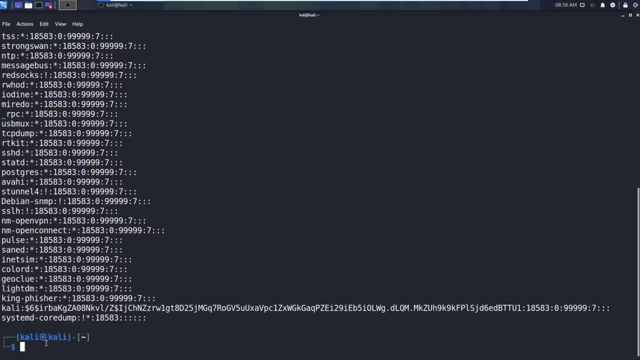 new user and we just called the user John. we can't just take John and just go ahead and just run these commands as root. no, John has to have the permission to do this. so you can think of Cali as being an administrator, but only when we 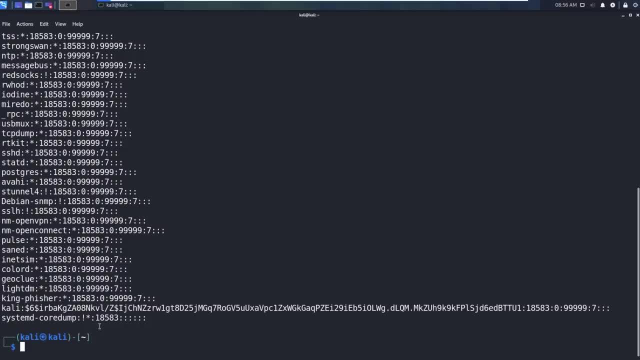 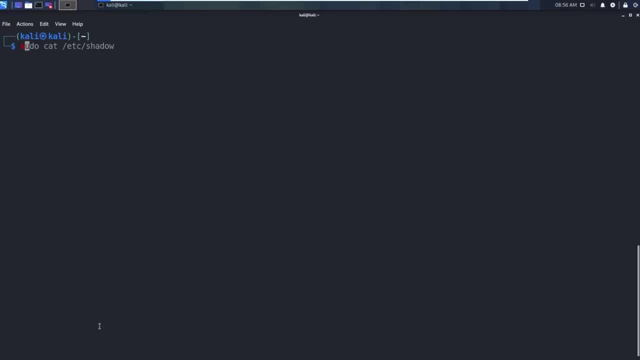 utilize that access or that privilege, okay. the other thing I want to show you, though, is that we can switch over to root if we want to. we can come in here and we can say sudo, switch user dash, just like that, and then I'll put us into. 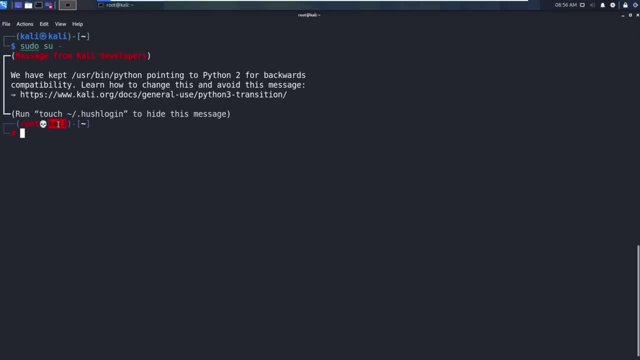 root. now you can see that we have the permission to do this, so we can come in here and see: okay, we're running root at Cali and that's only for this instance. you can, if you want. I'm not going to demonstrate how to do this, but you can. 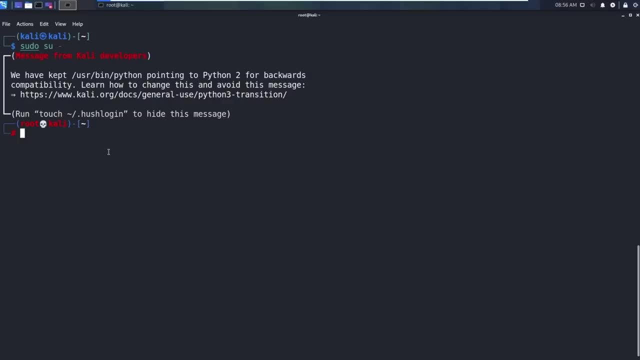 if you want change the root password, log out and log back in as root and run through this course as root again. that's not best security practice, but that feature is available to you if you are a Linux user that is comfortable with Linux, comfortable with running as root, and you want the easy path. otherwise I 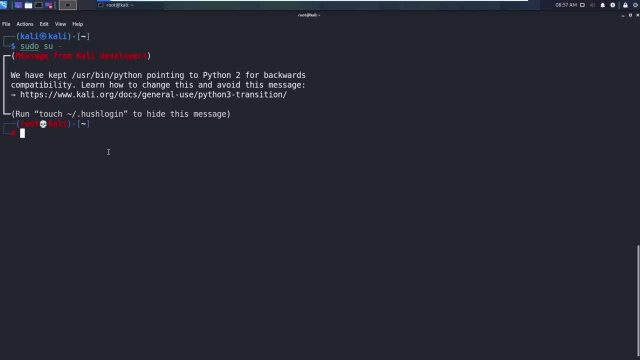 highly recommend just staying as Cali, running as sudo privileges as you need it and then moving forward. but this is a quick way to switch into root if you need to. sometimes even running sudo causes some issues, so switching to root to run a command is okay. what we can do. 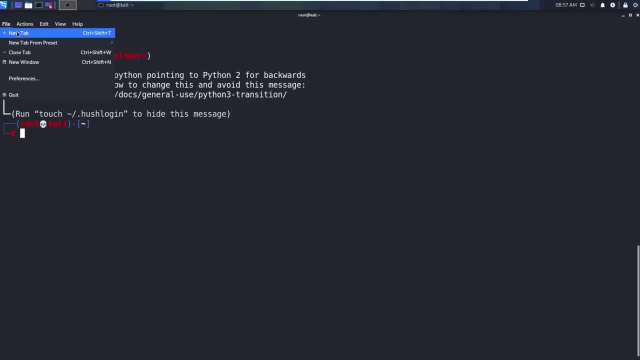 here too is the demonstration is we can go file new tab and look at a new instance and you'll see that this instance of root is only good for this tab. here, once we start a new tab, we're going to be brought back right back to Cali Cali. you can see that from the top line in the tab. 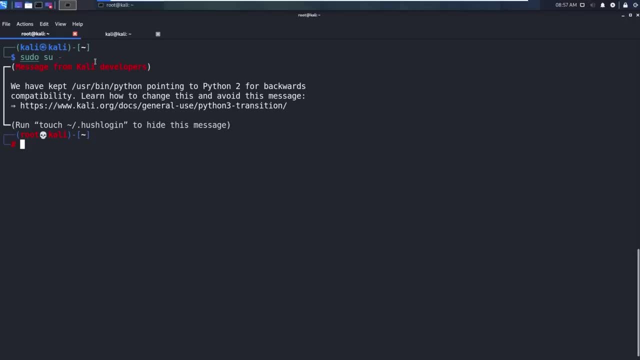 the tab as well. that's the first thing to going to run a command, cause we're going to be as well, so just keep note of this when you're running commands in this course. if you see something again, try running it with sudo. if it's not working or if 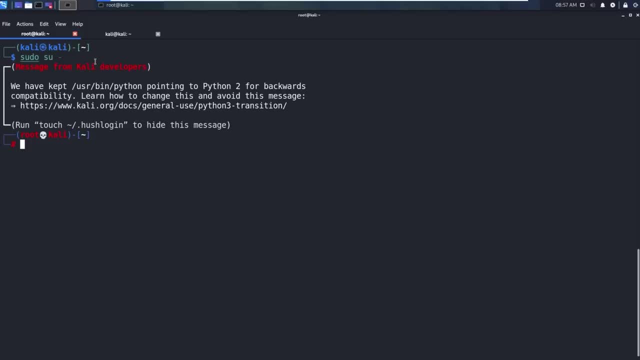 it says access denied, then you know, hey, I need to run sudo. very, very, very important. okay, I'm trying to drive that in into your brains right now. so from here we're gonna move on. we're gonna start looking at how to navigate around the file system, taking a look at everything from a bigger picture and 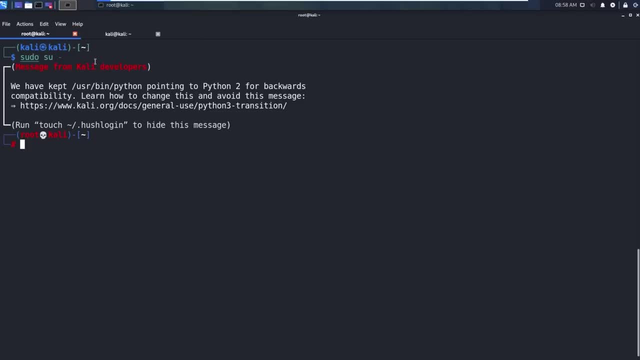 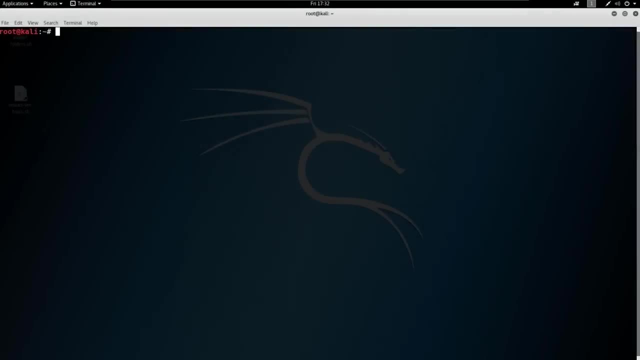 diving into terminal, so I will see you over in the next video. okay, so now our first lesson in Linux terminology is going to be navigating the file system. so if you're a Windows user, you're used to navigating your file system probably through folders, through a GUI, so a graphical user interface. 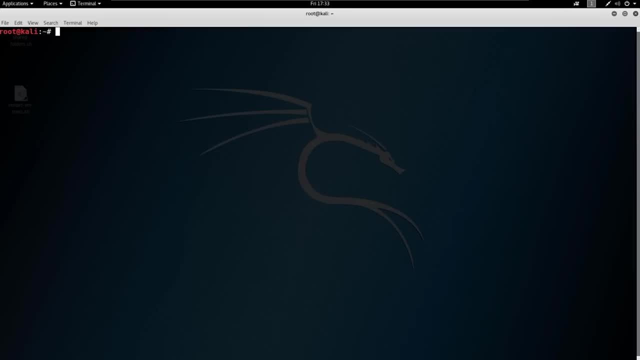 well, in Linux we can do that, but the majority of time we're going to live in this world of code, so we're going to be using a lot of code and we're going to be using this terminal here, so we really need to know how to get around. so the 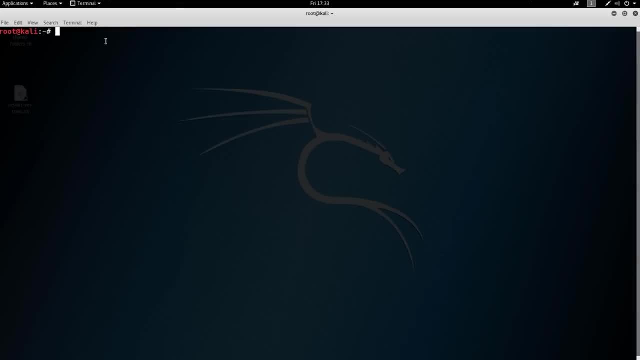 first thing we can do here is we can say, hey, where are we at? and that's PWD, so that stands for present working directory. so you type that in, you hit enter and it says, okay, we're in the root folder. so we know that we're in the. 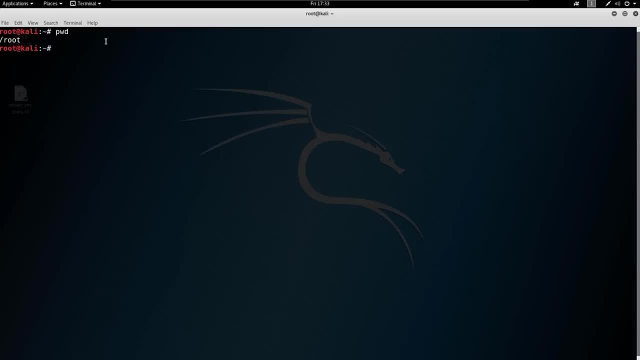 root folder. but how do we get out of the root folder? we can use a command called CD and that stands for change directory. so if we want to change directory backwards, we just type in two dots here and now we can say, ok, where are we at? so we're in a slash, so we're. 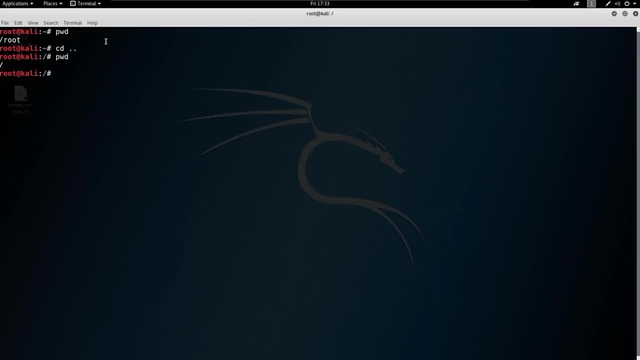 just in a home folder here or just there, our generic slash folder, right? so what we can do is: well, how do we know? can we go backwards from here? let's keep trying so we do PWD again? no, we can't. this is our base folder, right? so you have to think of this as the the lowest you can go. 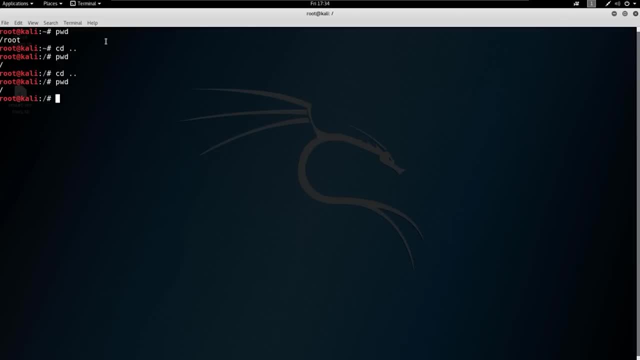 so now, how do we move around? how do we know how to go forwards again? well, we don't know what's in our directories, right? so we're sitting in this, the slash folder, and how do we look around? so there's a command called ls that lists everything that's in the folder. 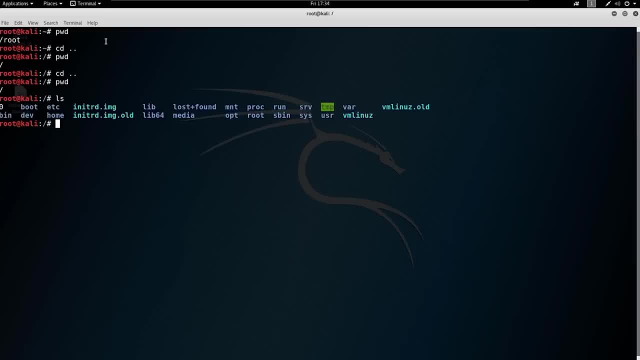 so if we say ls, we kind of see this color coordinated here and the color coordination it just depends on if it's a folder, if the folders read right, you know there's permission settings, which we're going to get into later, but the majority of these here are folders. okay, well, 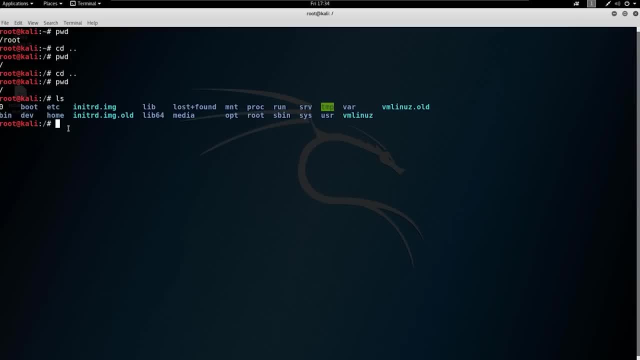 we know we just came out of root so we can go back into root. now how do we do that so we can say change directory root and we can actually hit tab to auto-complete? I don't know if you caught that, but there's no r any folder besides root, so at r I can just hit tab. 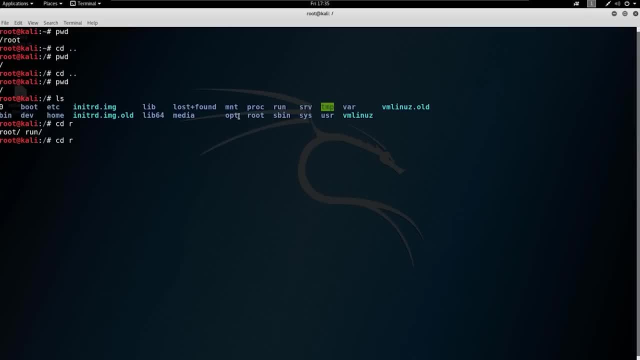 and it should type it out for me. oh, I lied, there is a run in here somewhere, but it's hidden. we're going to cover that soon as well. so ro, hit tab auto complete can change directory into root. so let's ls and root and see what's in here. okay, this is more like our home folder, right? 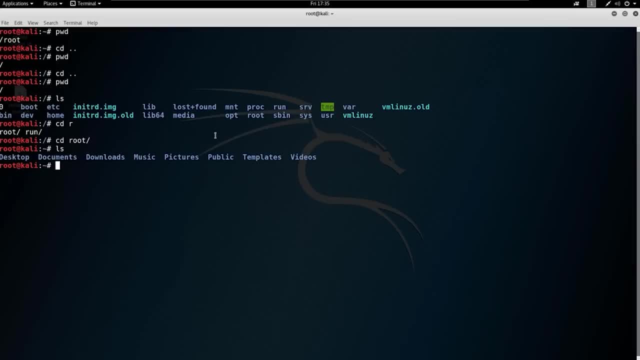 so we've got desktop documents downloads. this is kind of what applies to the root user. so what if we're sitting in this root folder here and we wanted to access instead this etsy folder? well, could we do the same etsy command here? well, I'm hitting tab and nothing's happening. 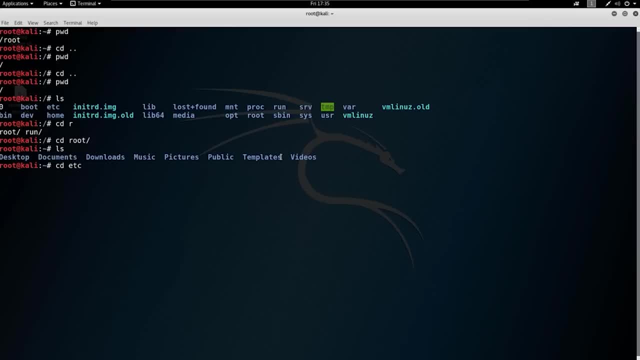 well, because etsy doesn't belong in this area, right. but if we put a forward slash in front of it, because this is the base and then we hit etsy there, now we can navigate to the etsy folder and we can actually double tab and see what's all in the etsy folder, like an ls say no, another way to. 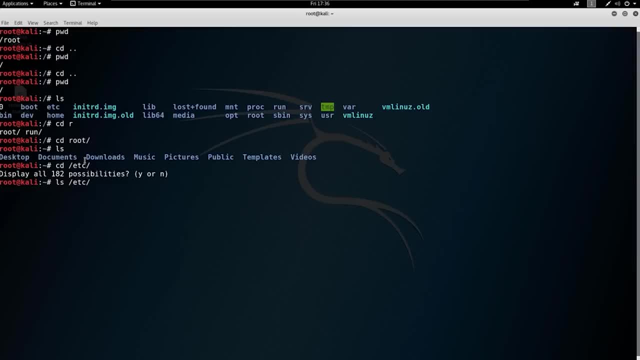 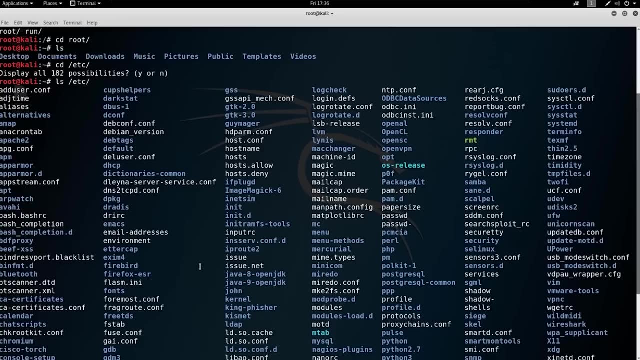 do. that is, if we wanted to ls what's in the etsy folder without navigating to it, we could just type ls- etsy and you can see everything that's in here. so there's some some tricks that we can do right, so we don't have to actually navigate to the folder to know what's in there. again, if we ls. 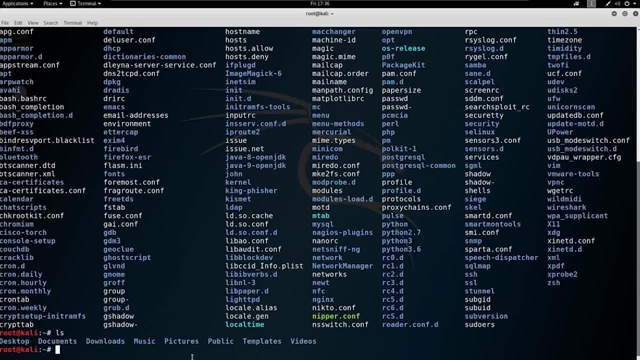 and we want to know how we're on here. right here we're on the right, the file, we're on there and we left the class bold what's sitting in videos? or even, let's say what's sitting in desktop for our folder. Well, if we start typing desktop and hit tab, we can't do that either. 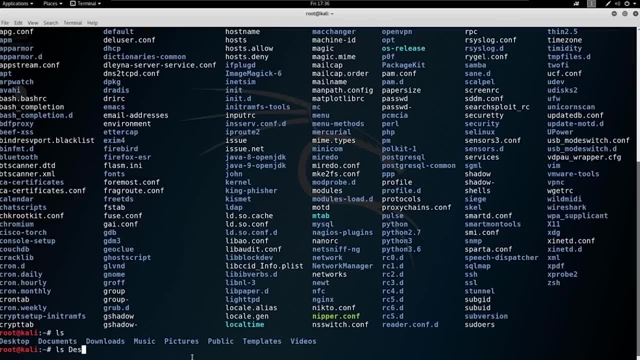 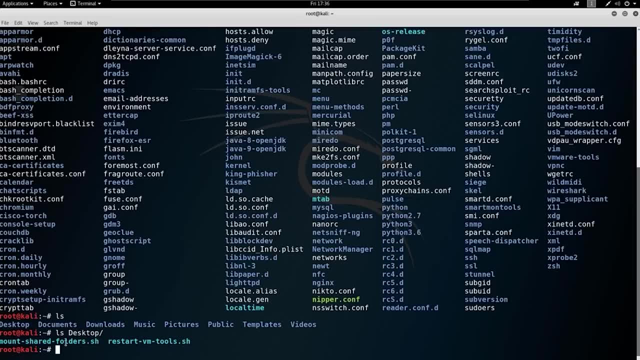 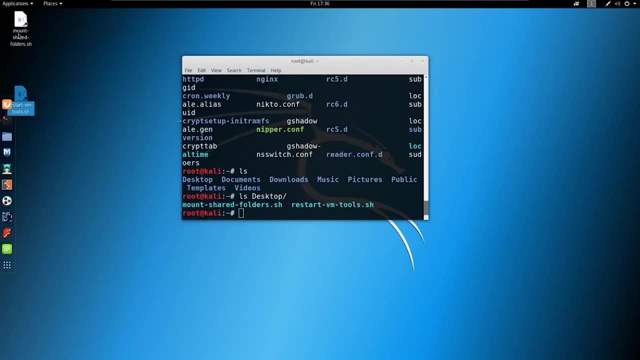 because everything in Linux is case sensitive. So if we start typing desktop and then hit tab, now we can LS and see what's in there. So our VMware came with a couple of shell scripts here that are automatically placed on our desktop. If we wanted to confirm that, you could see that they're both right here. 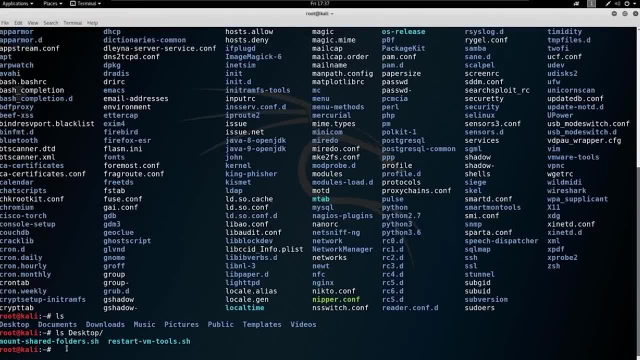 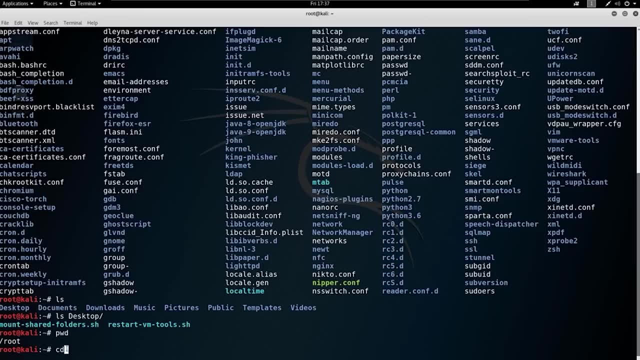 So, as of right now, we are just sitting in our root home folder and we know how to navigate around. So if we wanted to go to desktop, we could. We could hit LS now and see what's in there. If we wanted to go backwards, we could. 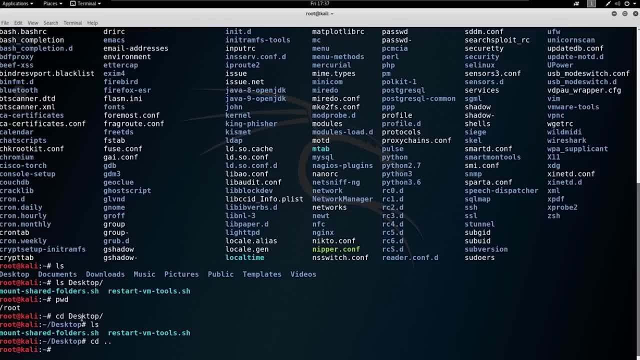 Okay, now we're back in our root folder And you can also tell where you're at. Your present working directory sits right here, right? So this little at tilde is actually your home folder and you can see that it's sitting in our root home folder. 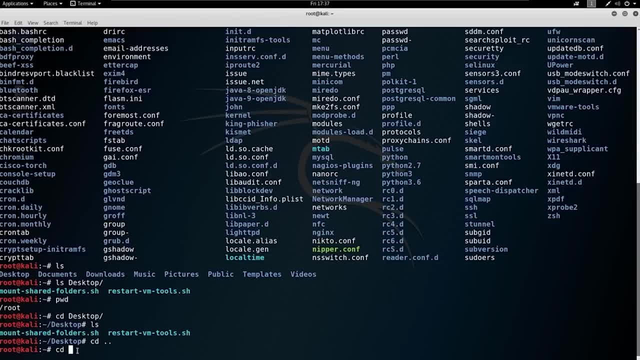 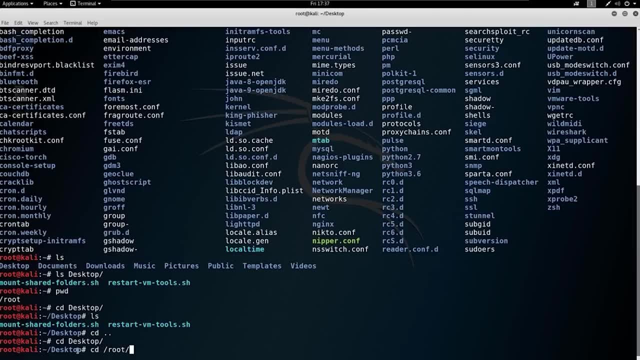 And you can see that we're in desktop. So if we wanted to go back into our desktop instead of typing, say you wanted to go to music from your desktop instead of going root music, which will work- you could also just say: I want to go music. 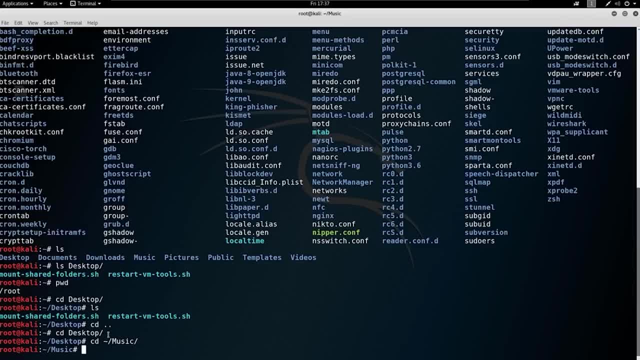 And that'll put you there as well. And notice you don't need the leading forward slash when you use the at tilde. So just some couple interesting tricks that you'll kind of pick up along the way. Tab is definitely going to be your best friend. 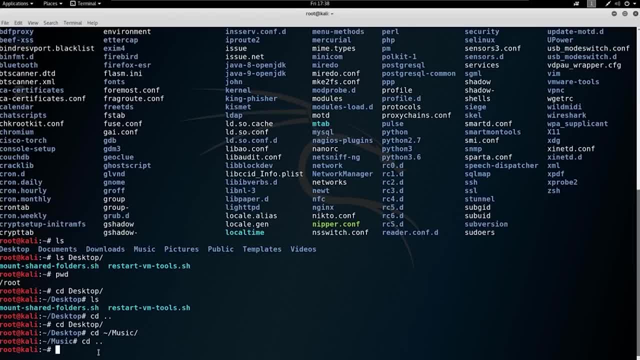 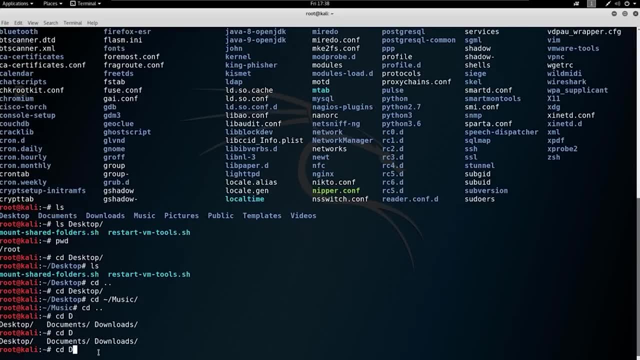 If you run into something with multiple options, say you're trying to CD and you say I want to go to my desktop and you're tabbing and it's not working, you can hit double tab and then it'll show you: okay, well, there's desktop documents downloads. 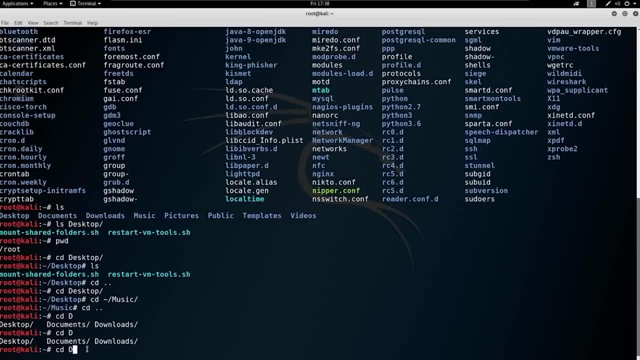 Those are your three options that start with a- D. So now you kind of have an idea as to how to kind of move around, But let's do a little bit more. So what if we want to make our own folder? Well, there's something called make directory M-K-D-I-R. 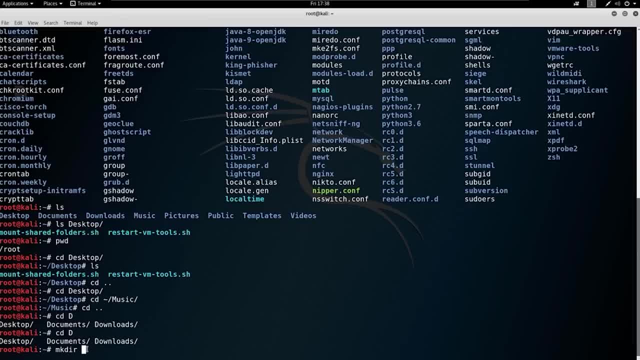 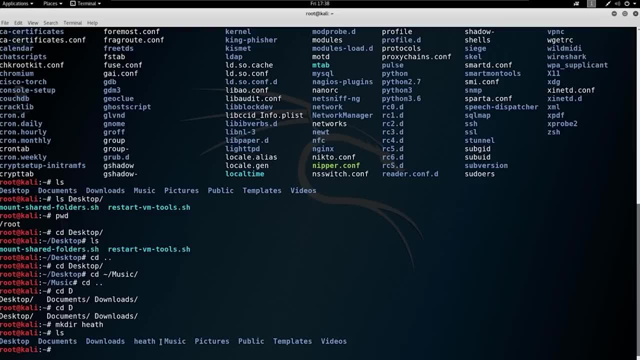 So if we say make directory, we'll say I'm just going to use my name Heath. So now, if we L-S, we can see that this Heath folder is now here, We can go into the Heath folder and there should be nothing in it, right? 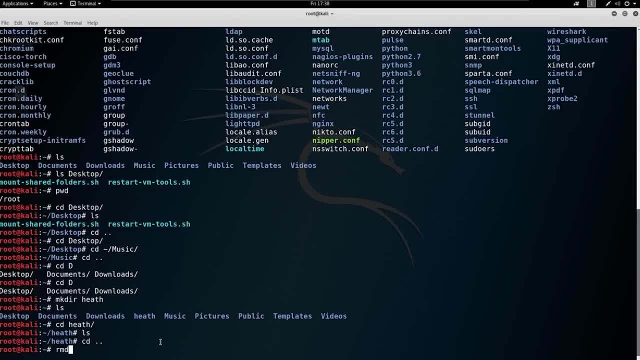 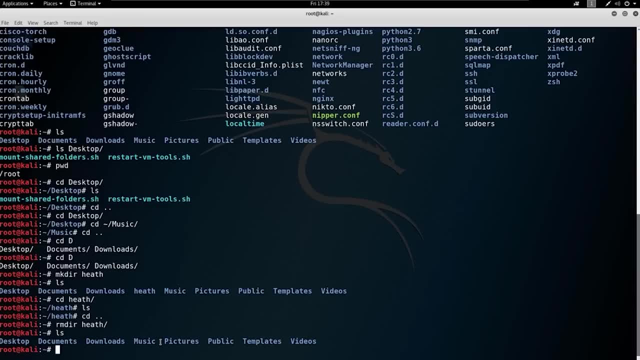 So we can go back and we can also get rid of the Heath folder. remove directory Heath. If we L-S again, it's gone. So now, what else can we do? Well, we can also look for hidden folders. So we can say: L-S dash, L-A. 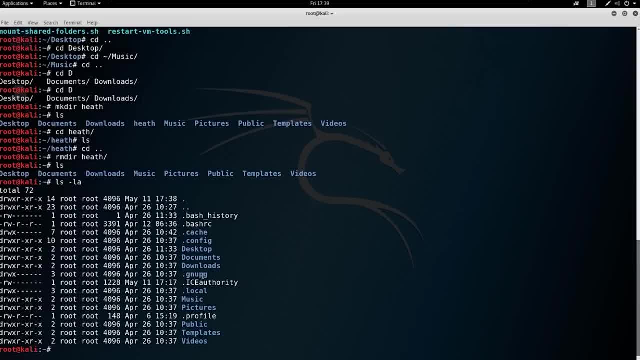 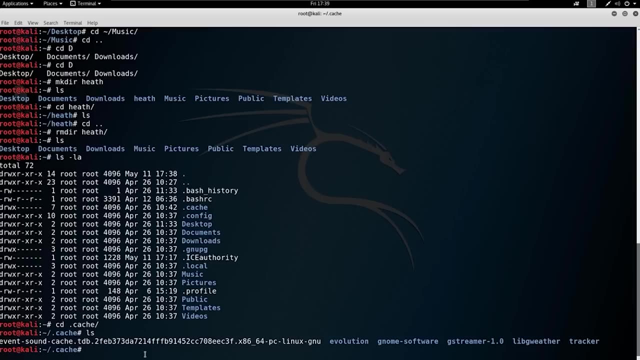 And we can look for hidden files and folders here. Remember the color coordination. So this dot cache, right, that in theory is a hidden folder. So if we say CD dot cache, we can go into there, We L-S and there's actually some information in there. 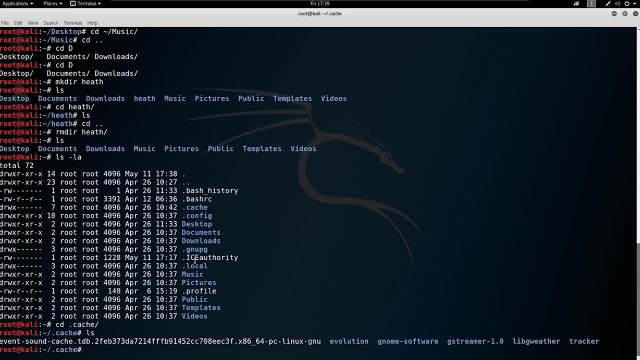 But when you saw it originally you didn't see that We're going to cover more on this. I just kind of want to show you that trick. As you see, over on the left side there's file permissions and properties. So be aware that just because it looks like something's not there doesn't mean it's not there. 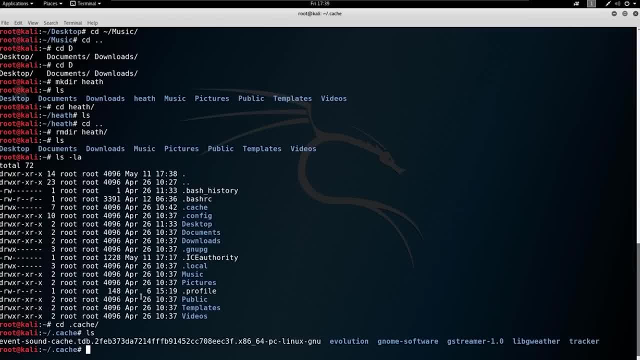 It might just actually be hidden, similar to Windows, where you have hidden files and folders. So just a quick trick to show you that. So another thing we can do. So let's go back And don't worry about what I'm doing here. 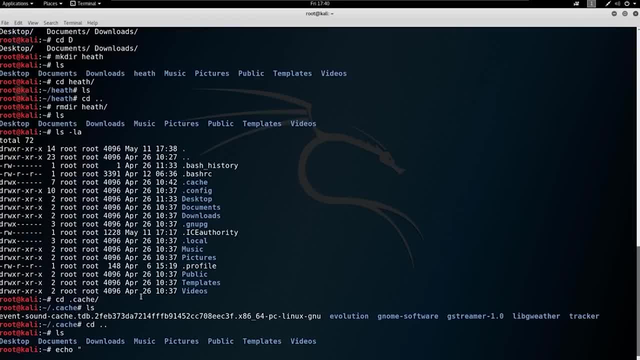 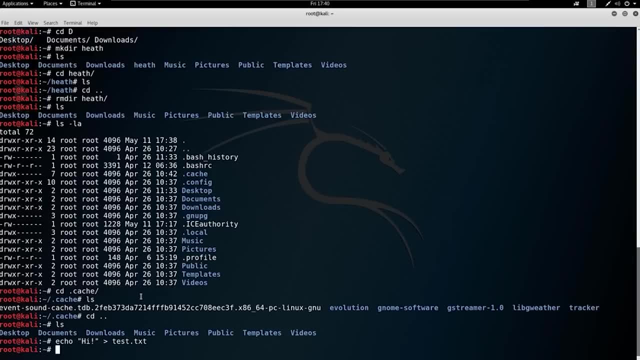 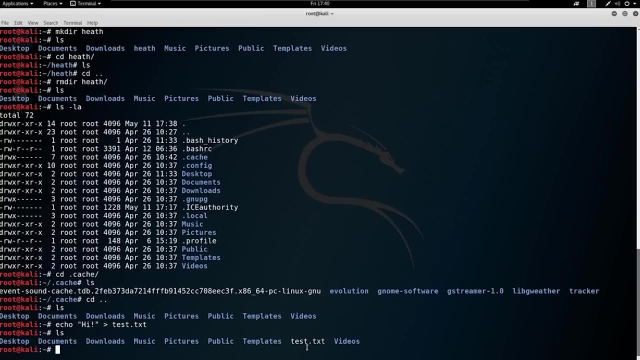 You're going to cover these commands in a little bit. I'm just going to echo hi and we're going to put that in a test dot text folder. So now, if we L-S, you could see that test dot text is here. So if we want to actually copy this file, we can copy this file to another location. 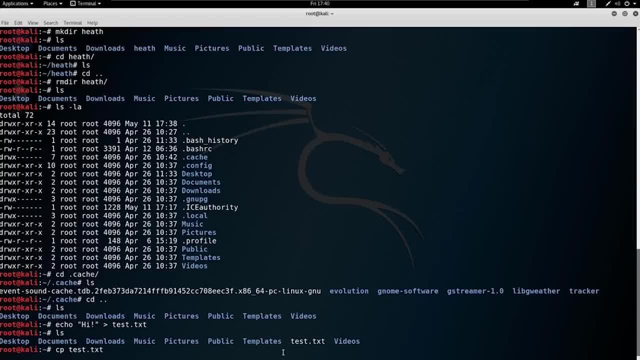 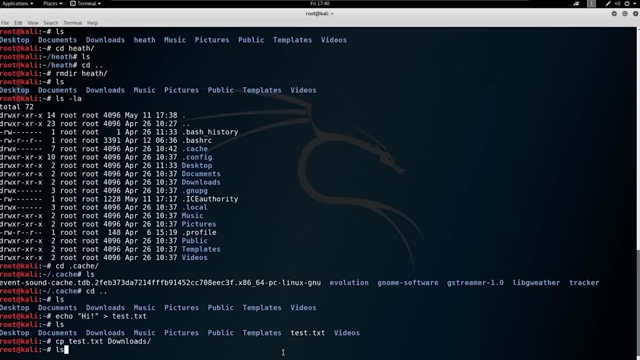 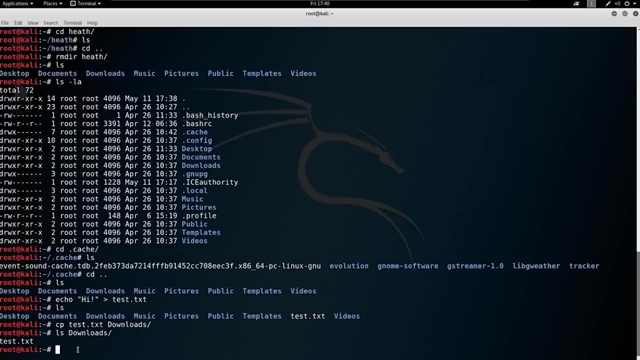 So we can say, hey, I've got this test dot text, but I actually want to move it to download. And if we go L-S to downloads you could see that test dot text is actually sitting in there And if we wanted to remove it, we can just say remove from downloads or test dot text. 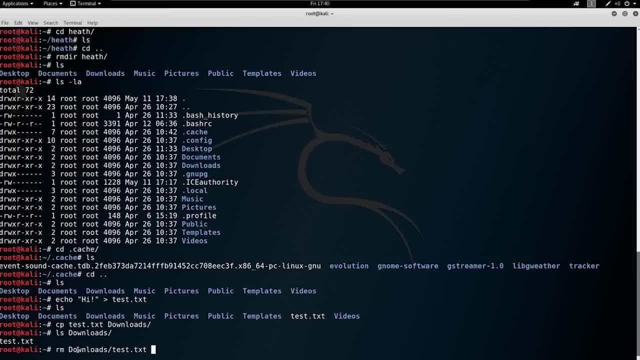 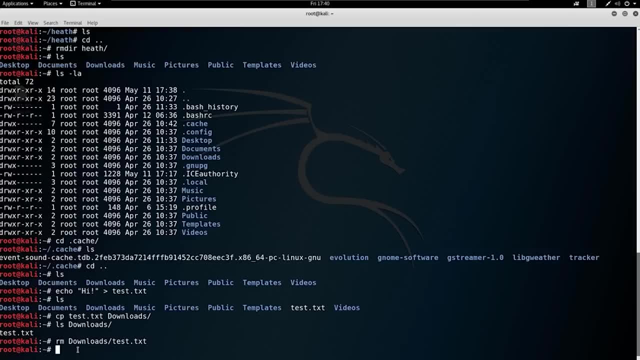 Actually sorry. remove downloads test dot text. We don't have to transition into that directory if we don't want to. So another trick: Say, we want to see now that it's gone and we want to L-S, but we don't want to keep typing this out. If you hit the up arrow now you can just see your. 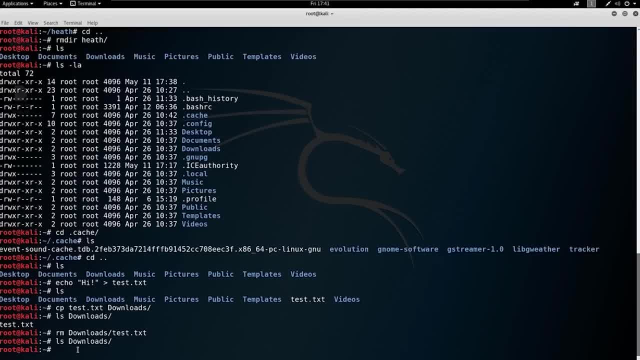 old commands. So if you keep typing a command over and over, you can see what's going on. So LS shows that there's nothing in downloads. Now we're able to successfully remove that file. So another thing that we can do is we can actually move. So say we wanted to move test dot txt. 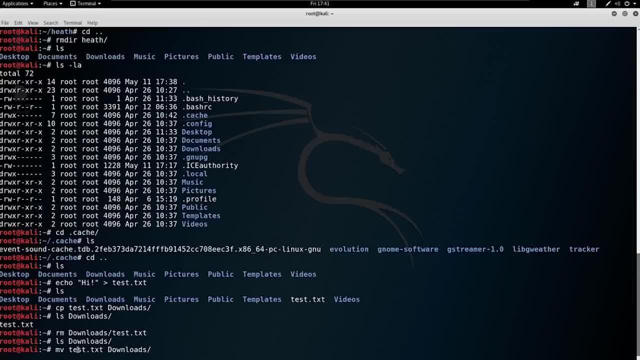 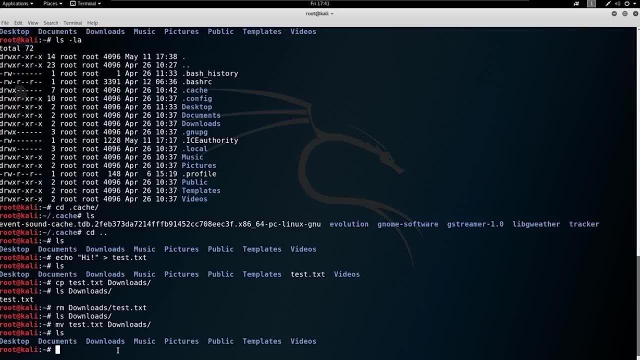 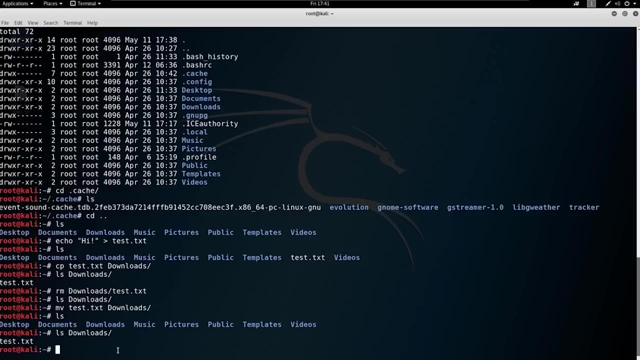 and we wanted to put that into downloads. Okay, now if we LS, test dot txt is now gone from this folder because we've moved it. we haven't made a copy, we've actually physically moved it away. So now if we LS, actually, let's just tab up. you can see that test dot txt is now in there And I'm 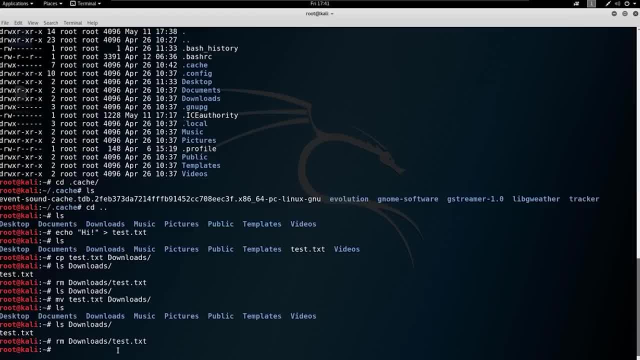 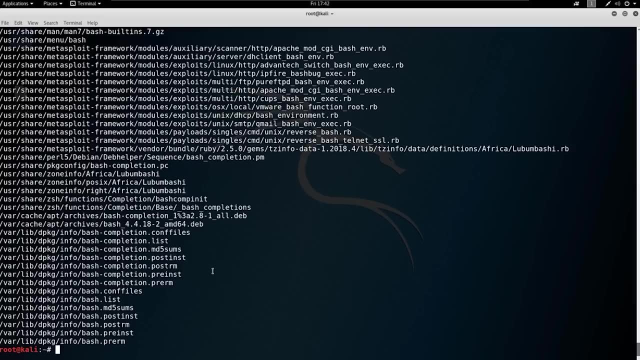 going to remove that here. Okay, and now, the last thing I want to show you is the locate feature. Okay, so if we wanted to locate a file- say I wanted to locate bash, let's see. So we're looking for a. 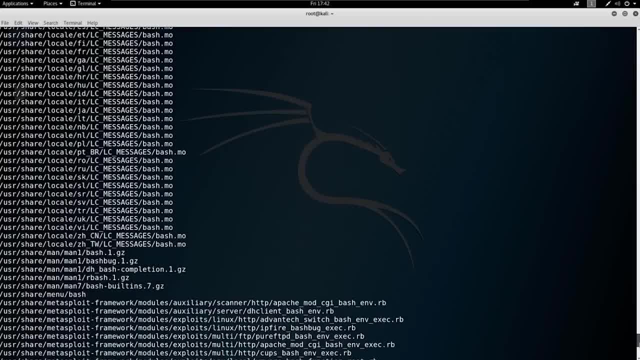 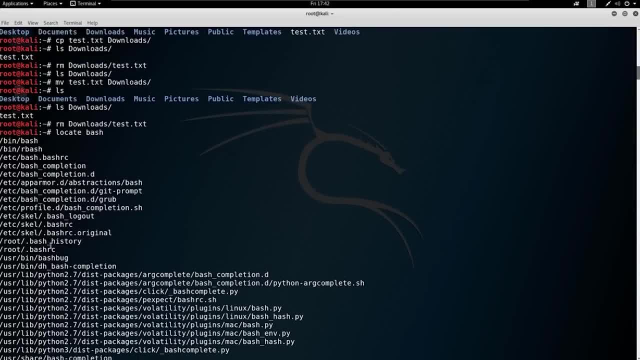 file, and we're going to get more specific along the way. But if you type in locate, you can kind of look through a system to see if you can find it. Now I'm looking for, say, any type of bin bash or bin R bash. that's fine, That's really what I wanted. But it shows you everything with bash in. 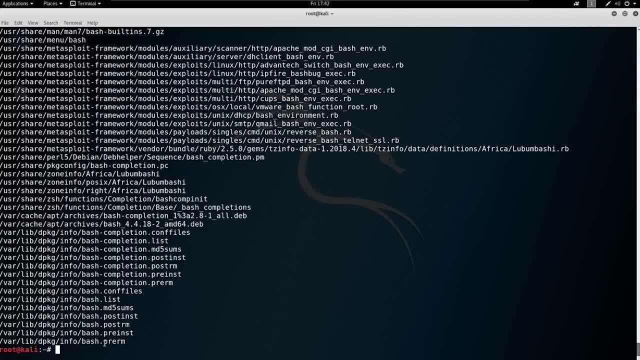 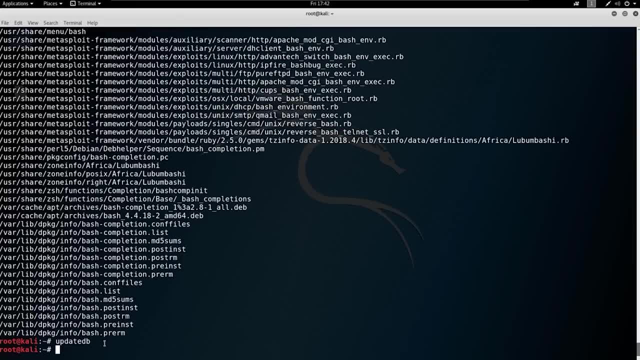 it Now. this might not work Right away. what you might need to do is update the database. So you type in update DB, it updates everything for you And then you can use locate again. So it has to build that database of the. 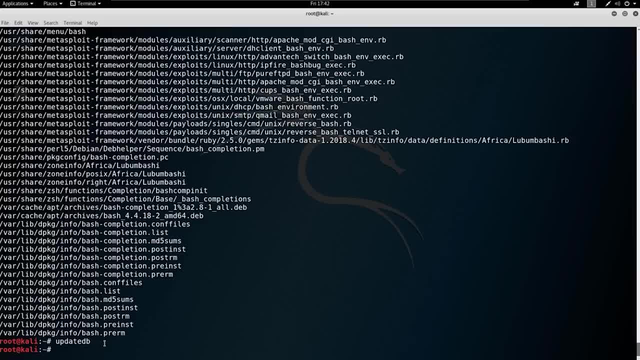 information that it's finding in order to locate what you're searching for. So make sure that you use Update DB sort of frequently. Okay, so two more things I want to show you, and then we'll close out this video and move on to the next one. So an important thing you want to do with your new. 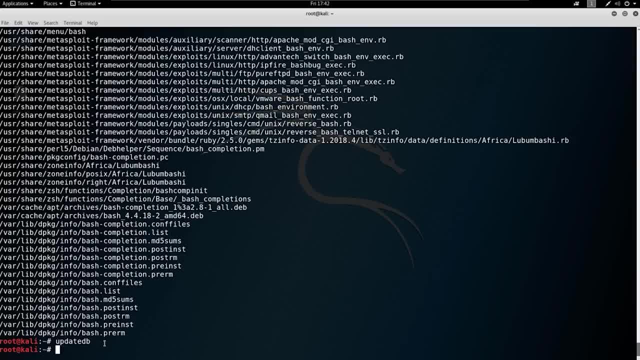 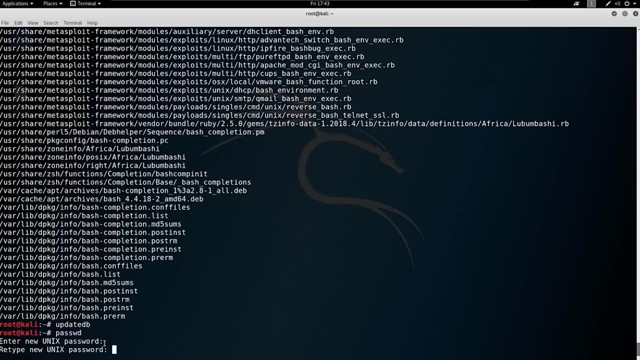 account is we're using a default password and that's not very secure. so to change a password for our user, we can just type in PA SSW D, and now it's going to ask us for a new password. so instead of using Tor, we can use something else. I'm going to type in the very secure 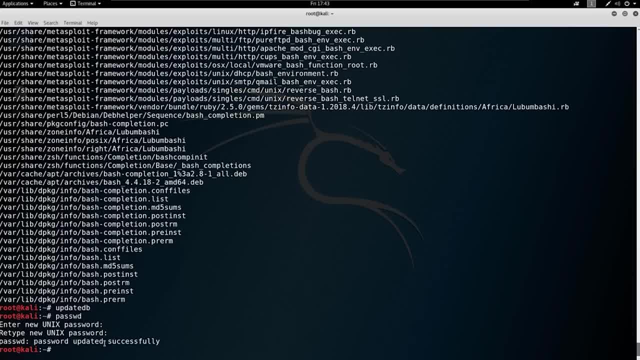 password as my password for an example here. but if you plan on using this machine for a future reference, you can type in a secure password and kind of keep it. so lastly, I want to show you is something called man, so man pages- man pages are your instructions for any command that you're running. most, 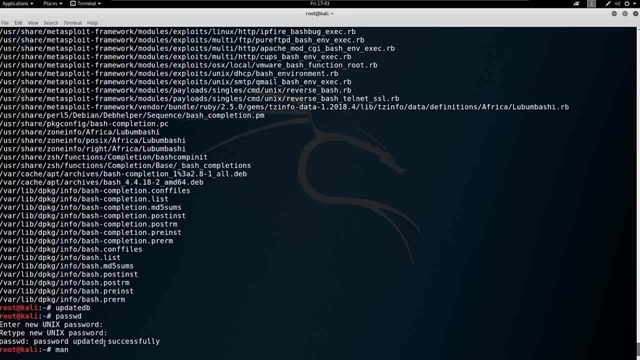 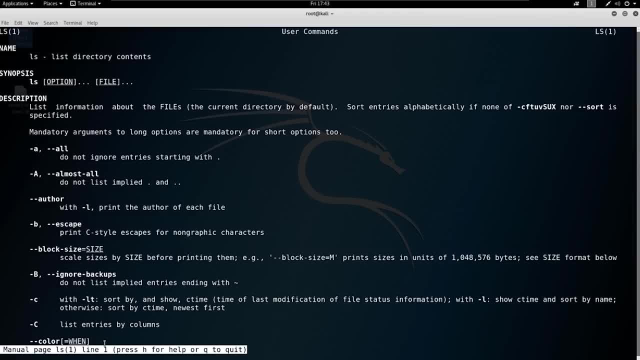 commands come with a man page. so let's say we want to look at LS, we can say man LS and then it's going to give us all this information here about LS. so if you see it says LS is list directory contents- awesome. and then it gives you. 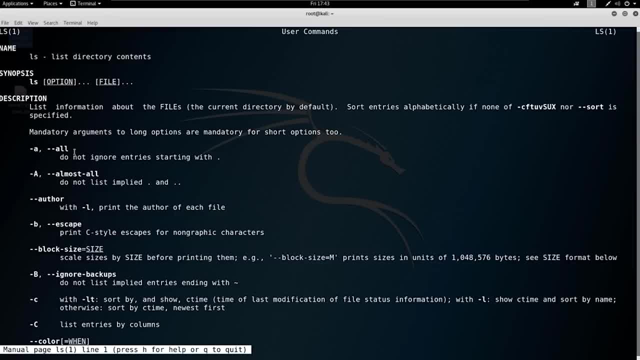 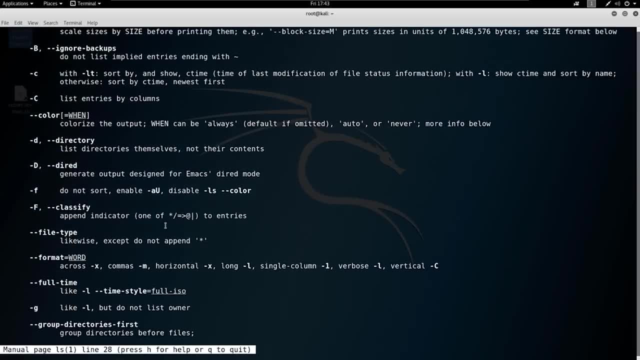 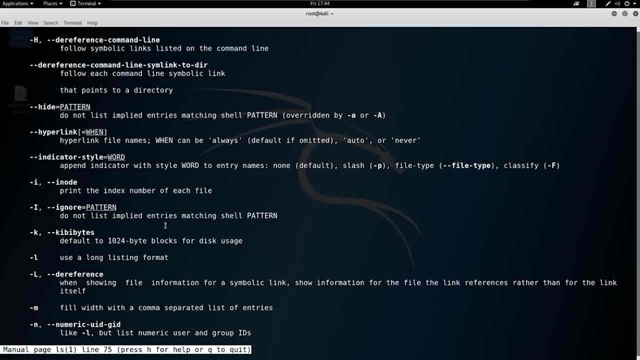 what options we can do. well, we can do a dash a for all which you saw earlier, and you can kind of scroll through here and just see exactly what it has to offer, and that's kind of it. so when you go through here, you can kind of you know if you're struggling to like. 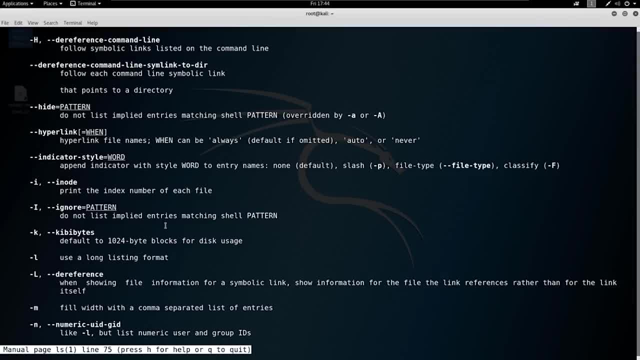 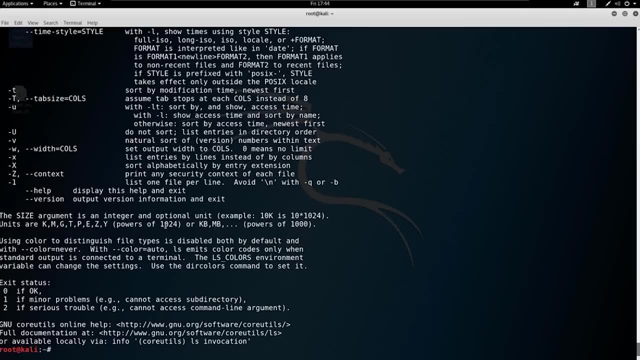 you know there's a command in there, but you're not sure exactly what the command is. you can type in man and search it, and sometimes you can do LS. I don't know if this is gonna work, but dash, dash help and you get some information as well it. 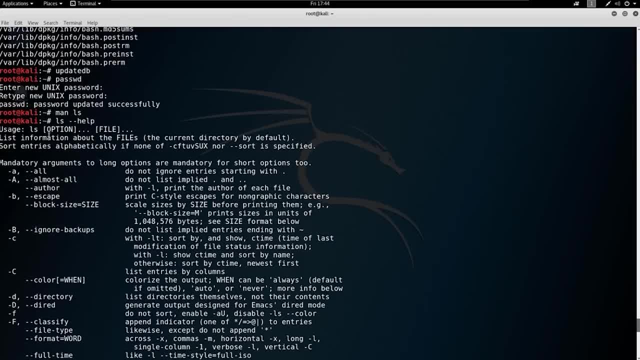 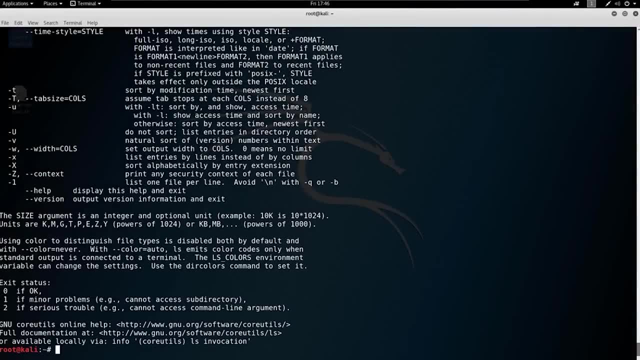 provides you the full man pages, but it provides you something pretty close, so that's kind of just your way around if you ever get stuck something to look for. okay, so that's it for this lesson. next we're going to move on to users and privileges: how to add users and how to, how to change some pseudos and some. 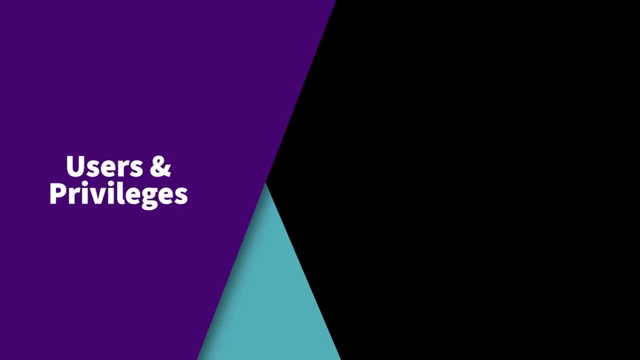 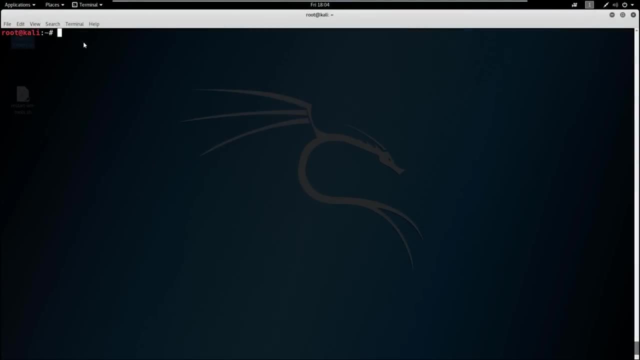 modifications to our file permissions. okay, so now we're going to cover users and privileges. So in the last video we touched a little bit on privileges with our ls dash la, And we touched a little bit on users by changing the password of our root account. So now we'll cover a few more. 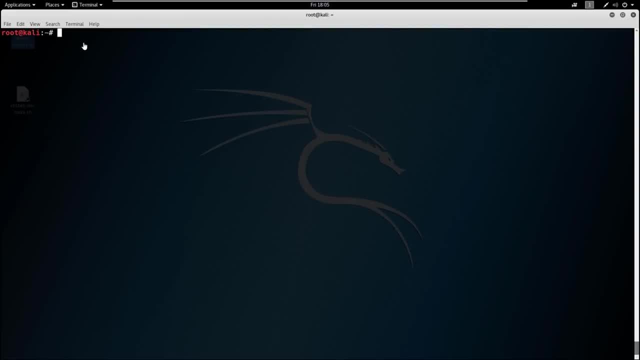 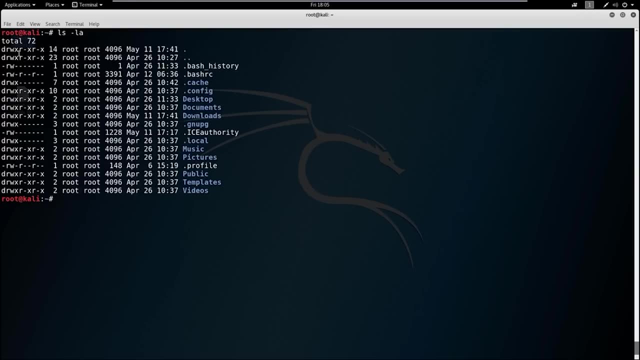 commands regarding those. So if we look again at ls, dash, la, you could see all this crazy jumbled wordage over here, right? So it actually means something. So we look at the first line here. if we see a dash like this, a hyphen, that means it's a file. If we see a D, that means it's. 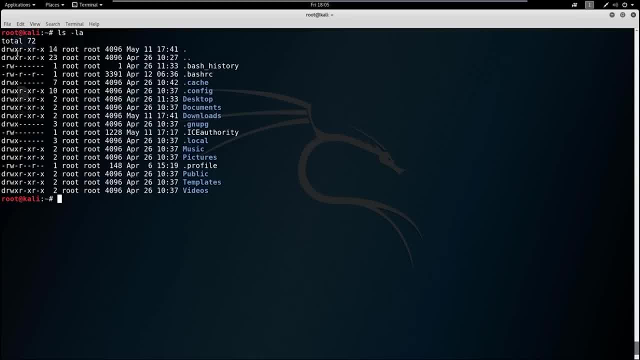 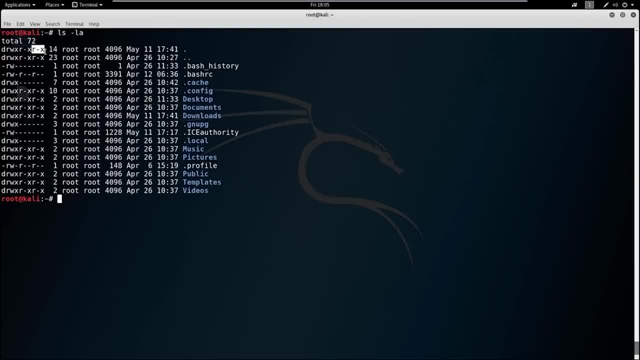 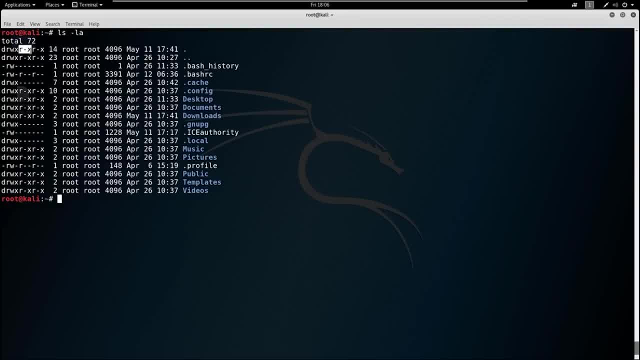 actually the permissions for the members of the group that own the file. So this is a group ownership as opposed to actual ownership here. So the for the people that are in the group, the group that has access to this file- they can only read and execute, they can't write to it. now, 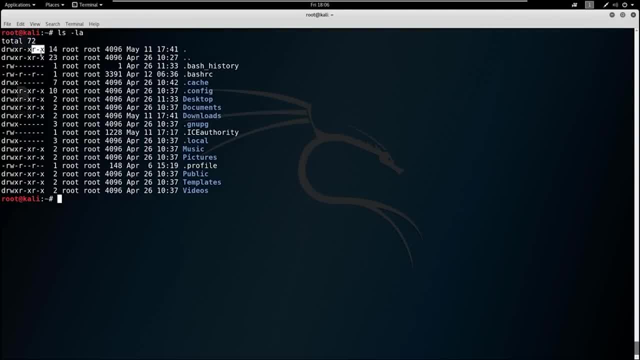 for the last one. this is just all of their users, so any common user here can actually just read and execute. they can't write the document. so that comes into play, especially when we get into penetration testing, because with penetration testing we're looking to have full access right. 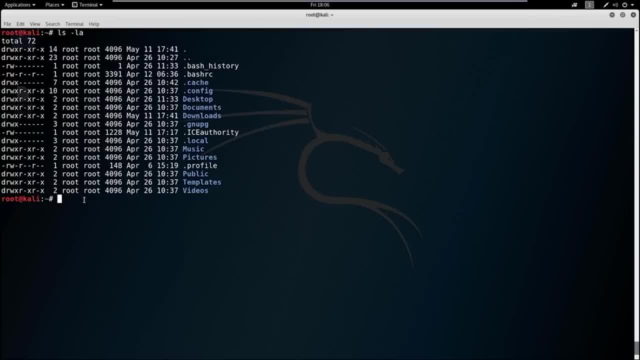 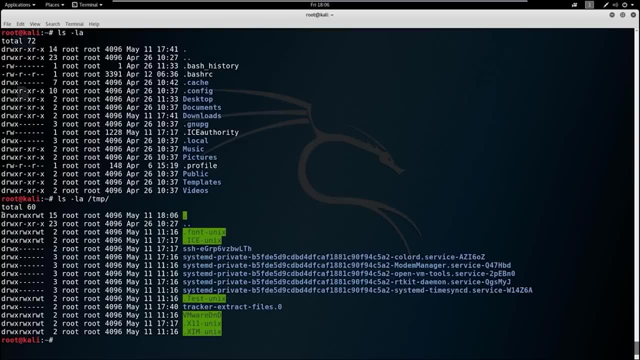 so we're always going to be looking for that folder that has full read write. typically if we look at temp, that's our temp folder. a lot of times you see the temp folder has full read write- execute. so when we're doing penetration testing, we're trying to upload some sort of exploit. we 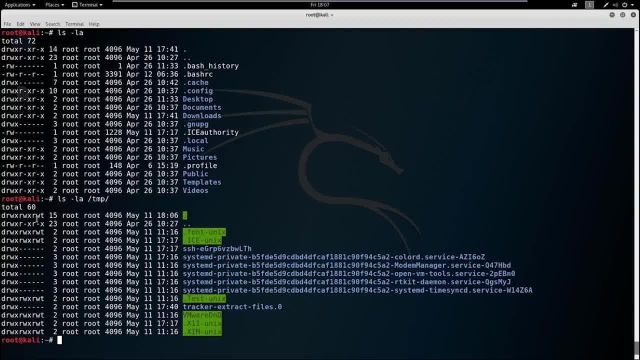 might actually upload it into the temp folder, because that's where we can execute those those files. however, we could also be looking for other full read write execute files where we need to modify them and give us root access to a system. so it's all about insecure configurations and we're going to 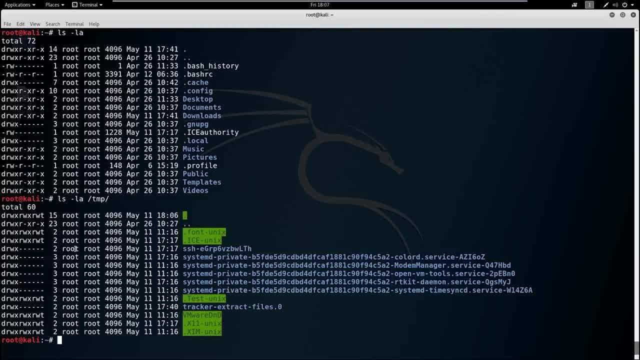 cover that more once we get into the actual penetration testing part of the course. so for the Linux essentials part of the course, all we need to worry about is these file permissions. another important feature of that is, if we were to create a script, our scripts not going to be. 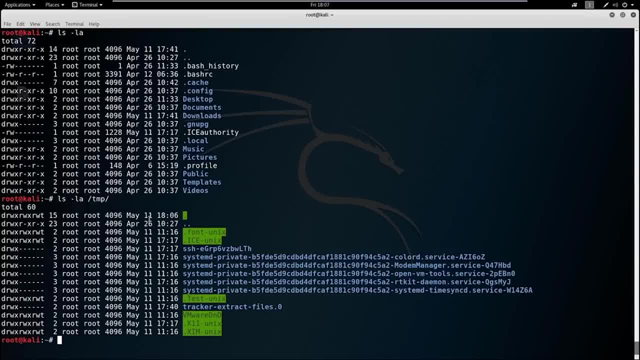 able to run until it has full access. so how do we change access here? so let's make a file, a I'm just going to make, we'll just echo another text document, right? so we'll just say hello, and actually I type that in backwards so hello, and we'll call it hello dot text. so if we LS here, 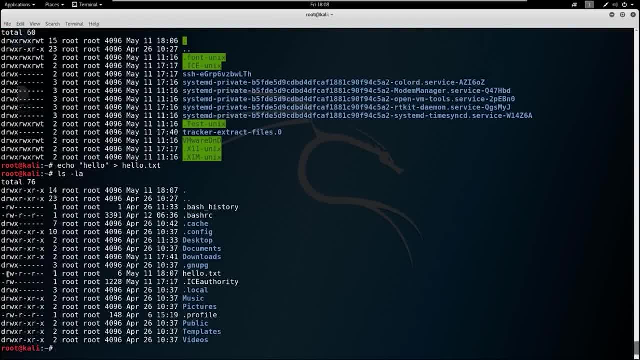 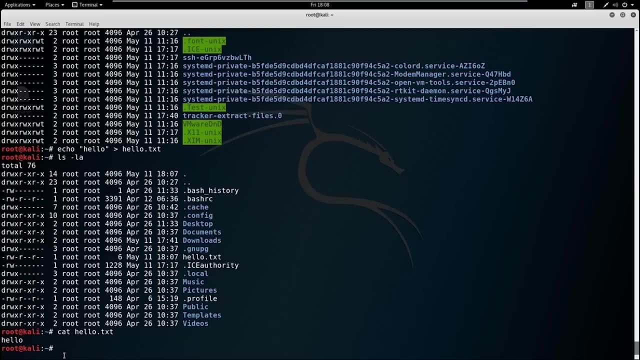 by default, we only have read, write and then read access for everybody else, meaning, if we wanted to read it, we could say cat, which we're going to get into later- cat, hello dot text. it just says hello. so what can we do here? well, we can use something called. 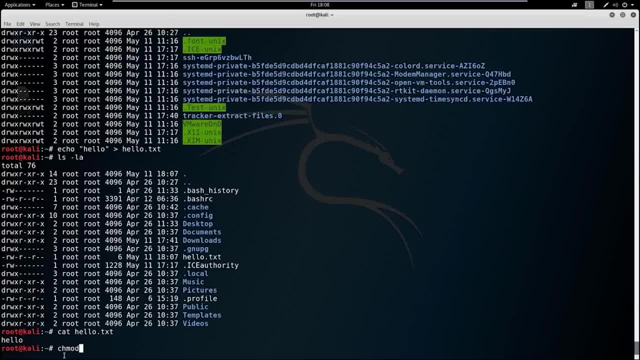 change mode. in changing mode is ch mod and we have a couple options here so we can do a plus right and we could say: well, we want read, write, execute or we just want execute. but another way I like doing it is you have another way I like doing it is you can do it any given time. so let's. 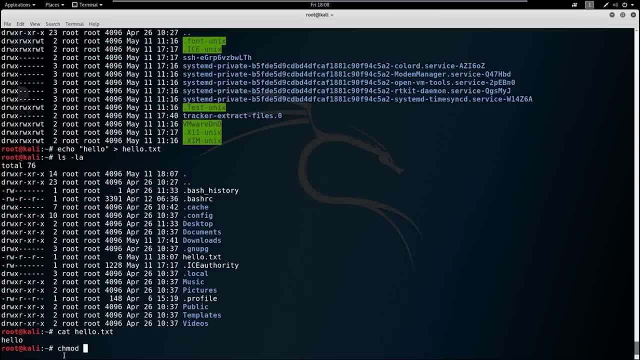 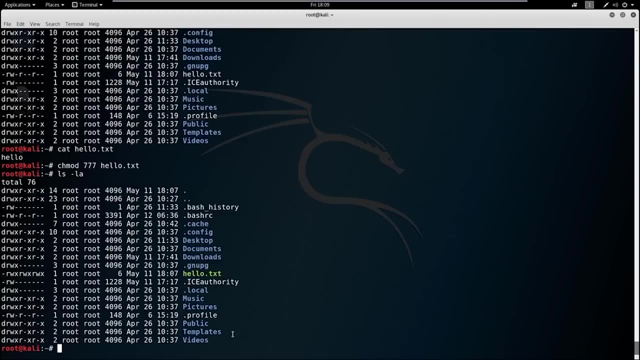 number feature. So the one you really need to know is all sevens. Sevens gives you full rewrite access across the board. So if we say chmod 777, hellotxt, now we ls la And you notice that hellotxt turns green, That means it is full rewrite. And here you go, We've got the dash here. 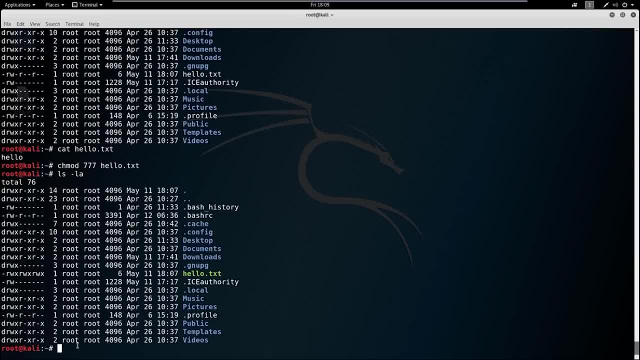 saying it's a file And we've got read, write, execute across the board. So this is how we change file permissions. You don't need to necessarily know about the other numbers in terms of penetration testing. It becomes more in terms of configuration and security management of files if 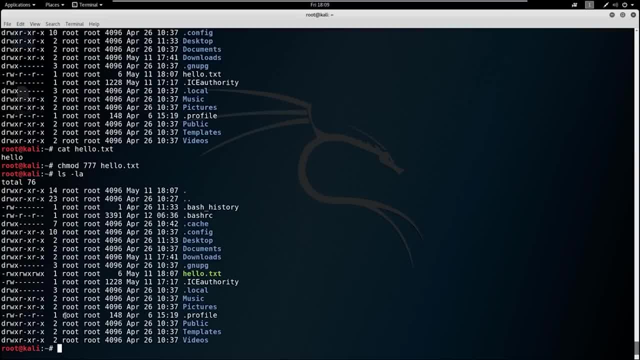 you were to get down that path. So to stay on the easiest path, just remember 777 or plus x will work as well. So changing the mode is critical And we're going to cover it time and time again throughout the course Once we get a little bit deeper. So a couple more things we need to talk about. Say we wanted to add: 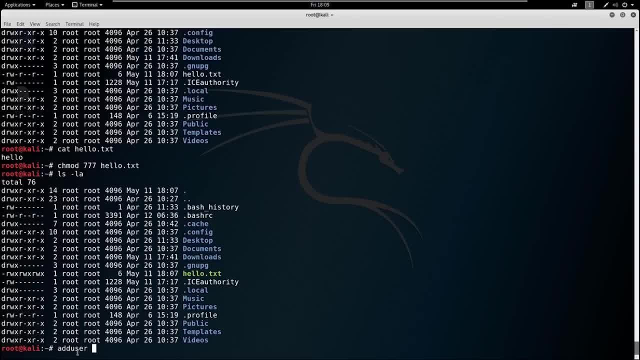 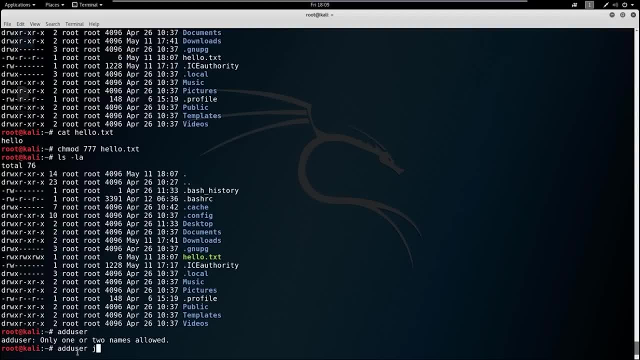 a new user. Well, there's a feature called add user. So we say add user And one or two names is allowed. So we need to add user. say john, Okay, so it made something for john, let's give him a. 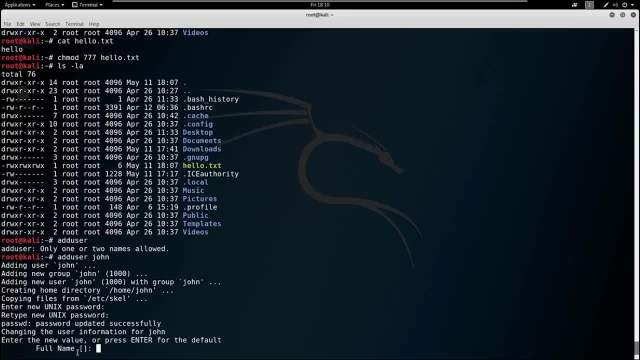 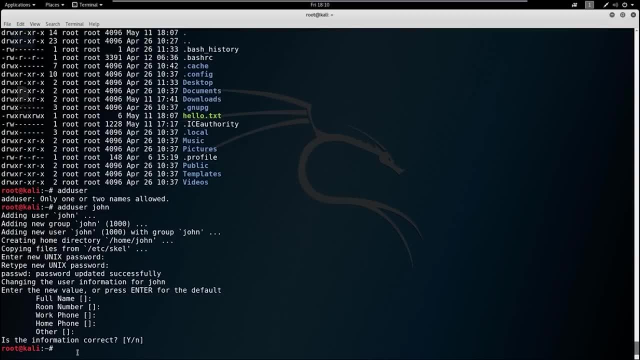 password. Give him a password again And we'll just hit enter for the default And we'll just hit enter for the default And we'll just hit enter for the default. It's all correct. Okay, so we now have a username, john, And we can confirm that we can actually cat. 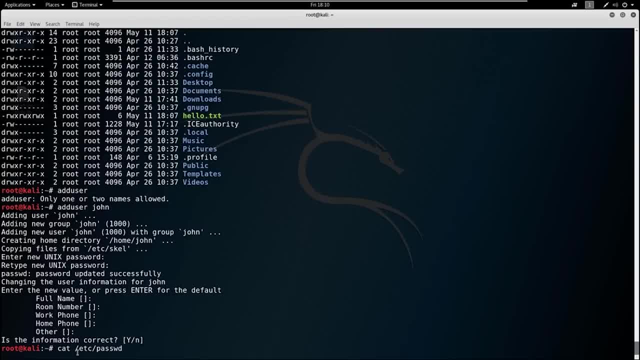 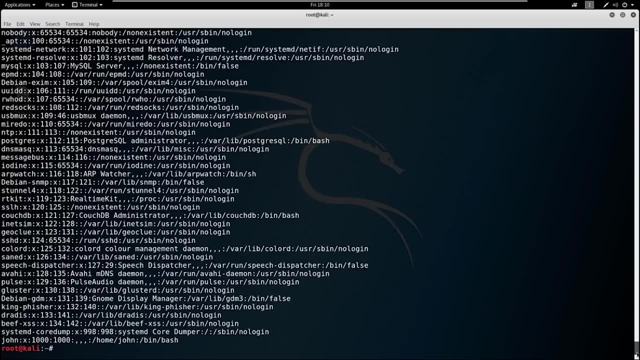 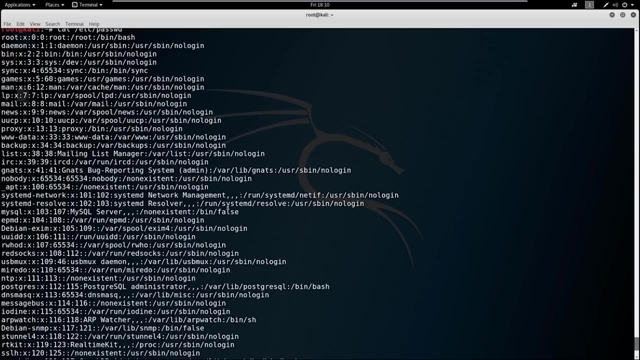 the Etsy password file here And you see down at the very bottom we have this user, john. So this Etsy password file you're going to become very familiar with because it shows you all the users. Now this will. there's a lot of times where you're doing penetration testing. you're going to have 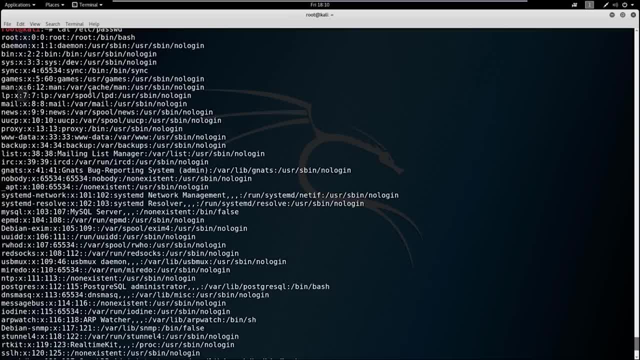 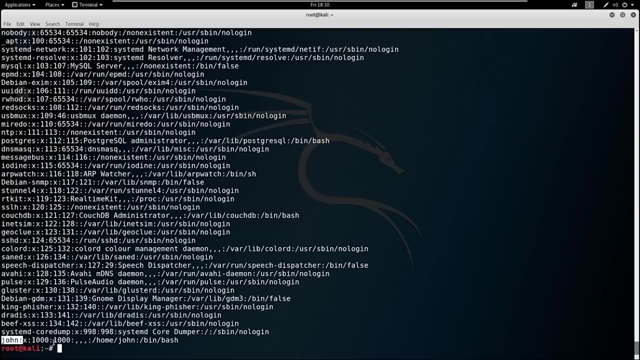 access to this Etsy password file because it doesn't provide the password anymore. it used to a long time ago. passwords are now in the shadow file, So you actually have a little bit of access and information disclosure here at the hands of poor configuration. So you see that I've created a user, john. well, that gives us a little bit of. 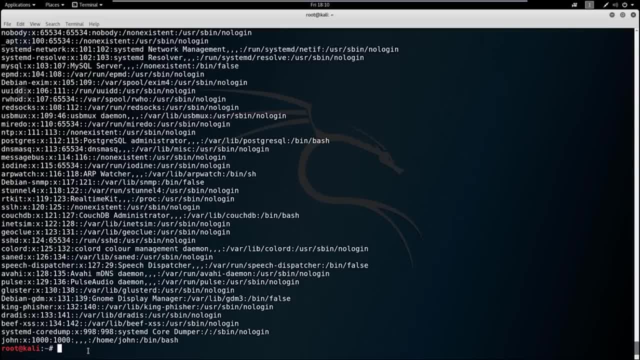 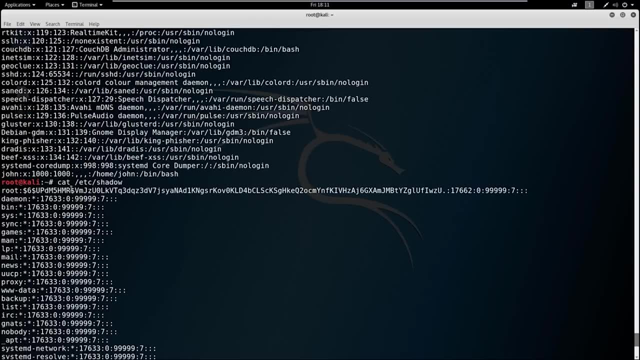 information. say there's SSH on a machine or something else, we can use that username of john to try to break into the machine. So we'll cover that again later. But if we wanted to see what the Etsy shadow file looks like, Now we come in here and you've got these, these jumbled stuff here. 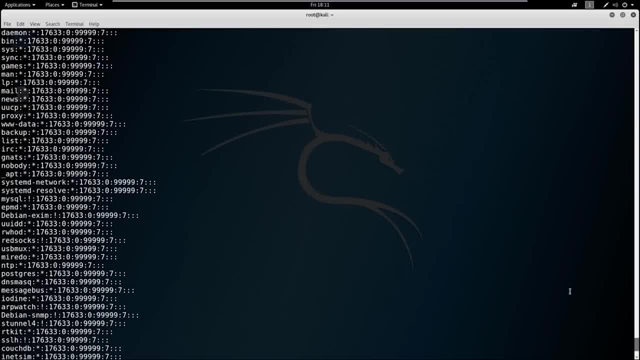 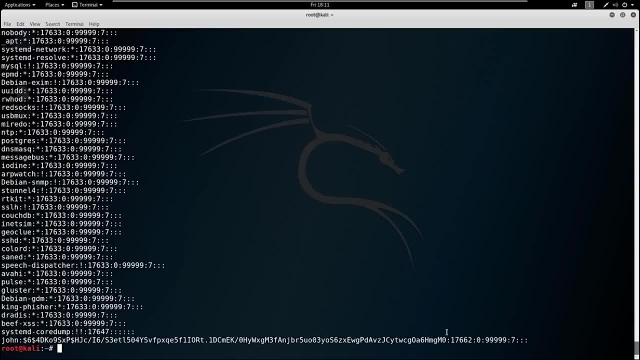 right. So it's just a hashing format. So what we're doing is we can actually use a tool like hashcat to break this down and crack these passwords. Now, a password, a password, will be very easy, But just know that if you have access to the Etsy shadow file, you have a good chance of cracking a password. 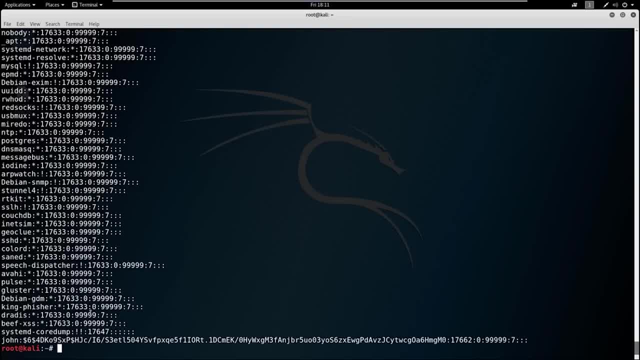 depending on your capabilities and depending on the strength of the password that allow you access to a machine. So something to think about there. Okay, so now we have our user john, let's go ahead and switch to him, So we can use something called su, which stands for switch user, and we'll 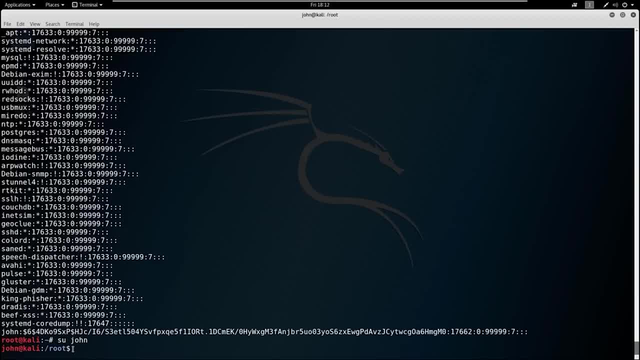 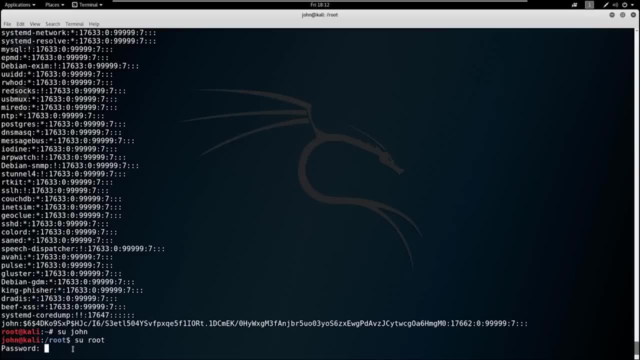 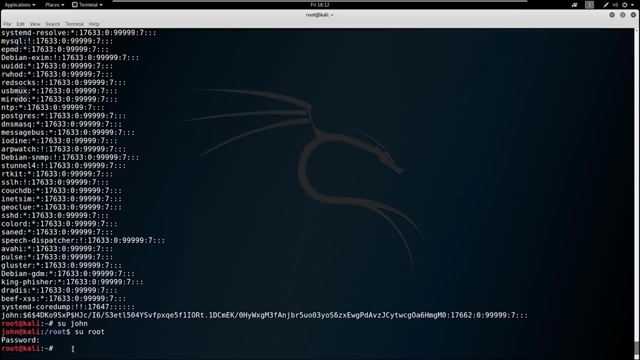 say, switch user john? Okay, so automatically gave us john here. let's see if we could switch back to root. Okay, we can't just switch back to root because we need roots password. Right, so we can type in password and that works. But if we didn't know the password, then we'd be 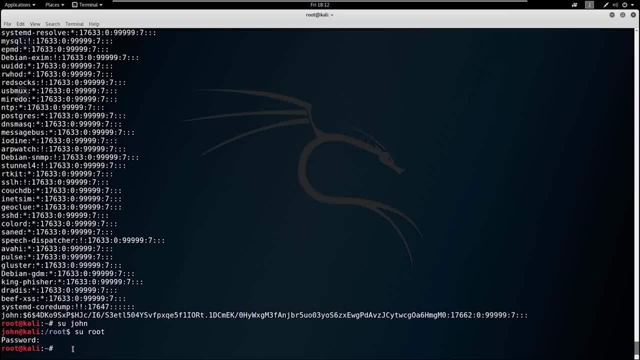 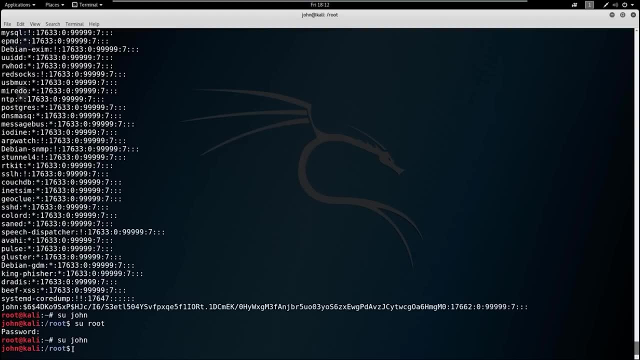 stuck on john. we are able to access john because we were already rude, So this comes into play in terms of users. So let's go back to john here Now. if you're a user, you have to be able to do certain things. You need permission to do certain things. I should say right, So root has full. 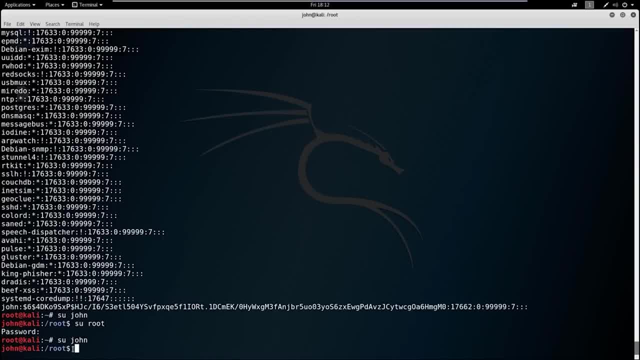 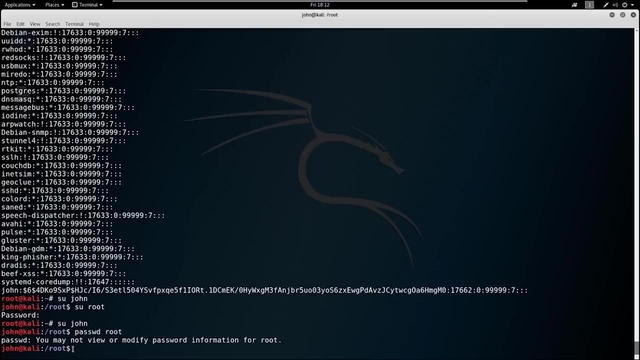 access and permission to do everything. But john- we just created john- john have any sort of access. so if we wanted to, if we wanted to change the password, say we want to change the password for for root, I can't modify the password information because I don't have. 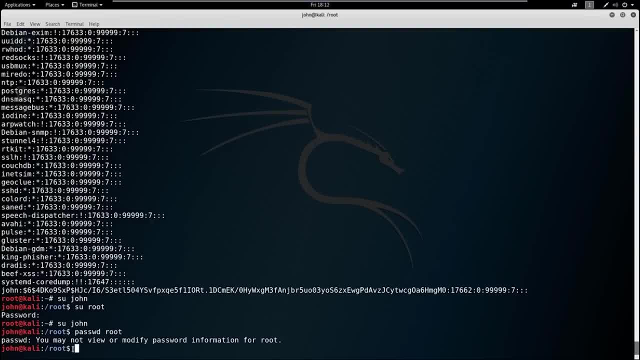 that kind of access. now there is something called a pseudo, which would provide John that access if we gave it to him. so it's called a pseudorus file and basically anybody in that pseudorus file can change permissions given if they are a pseudo user, right? so we would type in pseudo password. 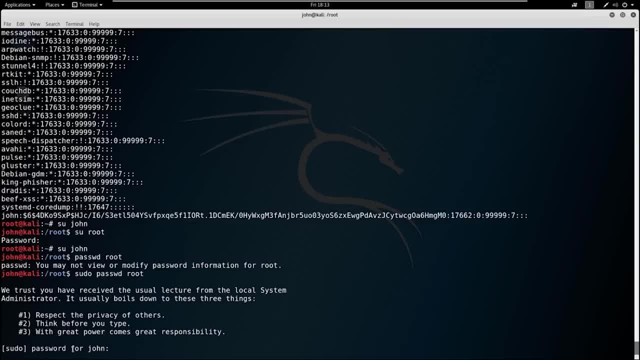 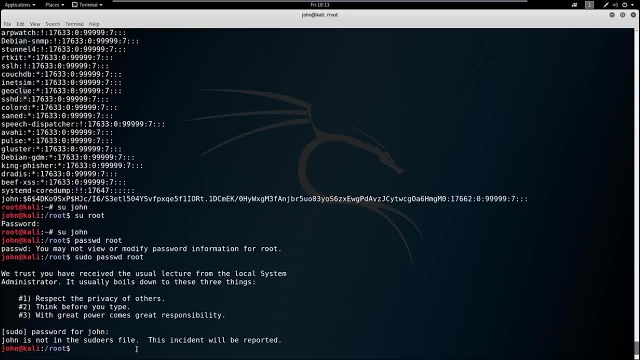 root and it's going to ask for the password for John. but you're going to notice, hey, John's not in the pseudorus file, John can't do this. so John has base permissions right, and we're going to counter that a lot of times in penetration testing where, if we get in, we'll get something called. 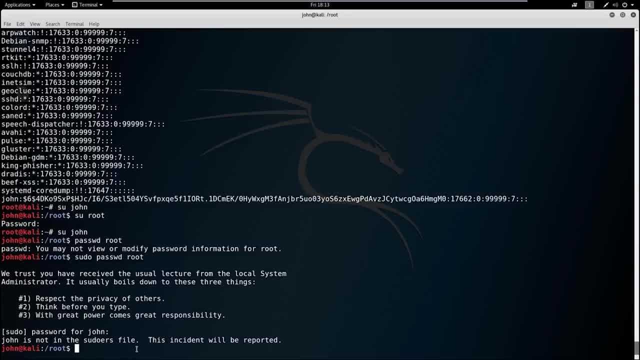 lower privilege and we'll get an account like John and we're going to try to ask, escalate into root, but we just can't do it. you know the chances of doing a doing that and having a John in a pseudorus file is just not high. it's possible but it's not likely. so for now, just know. 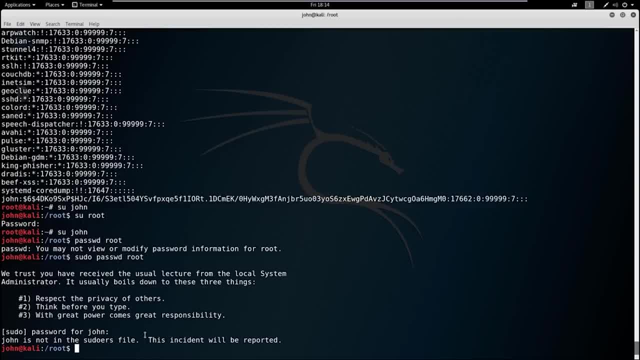 that if you want a user other than root to have access to file permissions, you need to have them in the pseudorus file. that becomes useful to in penetration testing, because you can look at the sewers file if you have access, to see what users have pseudo privileges. okay, so that is it for this. 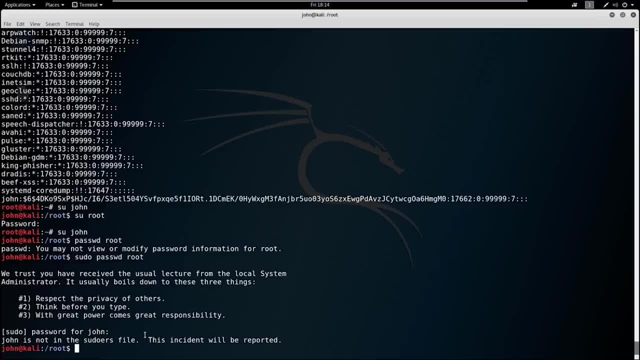 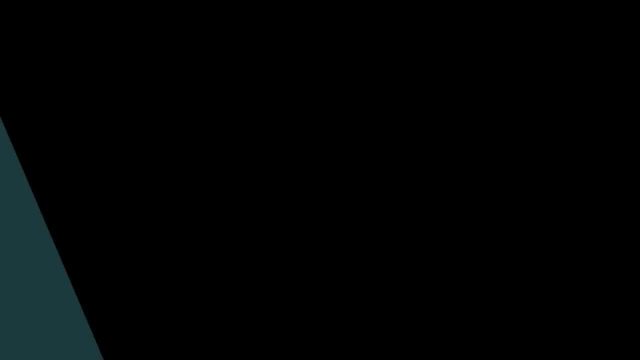 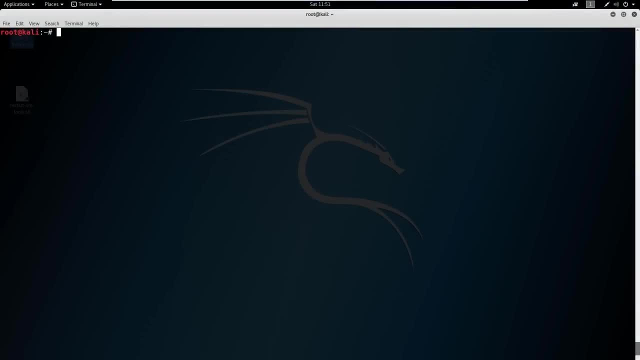 lesson. in the next lesson we're going to be covering network commands and moving on gradually towards scripting. so let's go ahead and get there, and I will see you when we get over there. okay, so now let's cover network commands. so the first command I want to cover is if config. so you. 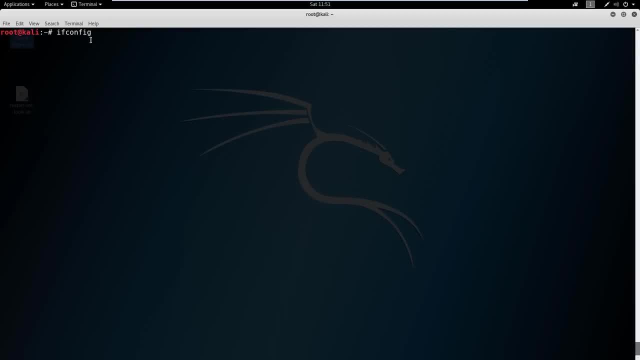 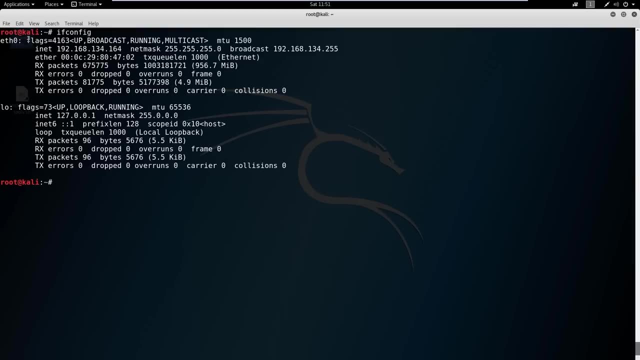 may be familiar with the Windows version of this, which is IP config, and they pretty much do the same thing. so it shows you the IP configuration and the IP configuration and the IP configuration. sehe that at the motion interactions also one more with all these fine Visual Leaf comes back. you can just memorize your. 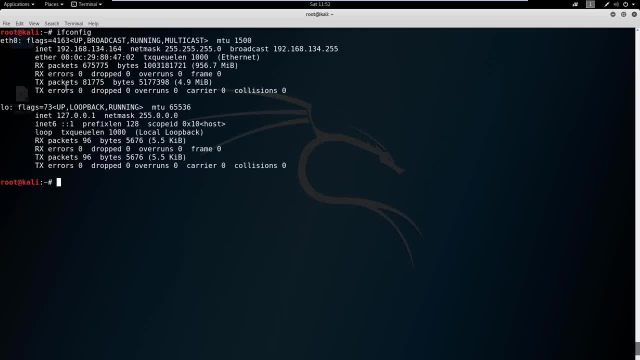 own JavaScript. it'll change the configuration later. absolutely, it also starts. everybody can capazes at that very same time. so that's it for this videoので. I hope you enjoyed it. that's very, please do, uh, if you still not on my site, I´d be glad if you did. did that in the comment section. 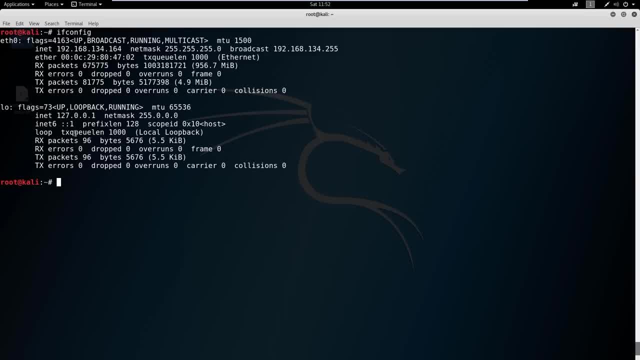 below, uh, in the live chat that is supported right here and it shows you here your different interface types and the IP address associated with them. so eat 0 here. Ethernet 0 has an IP address of 192.1, 68.132.164 or at some point you want to do wireless penetration testing, you're going to need 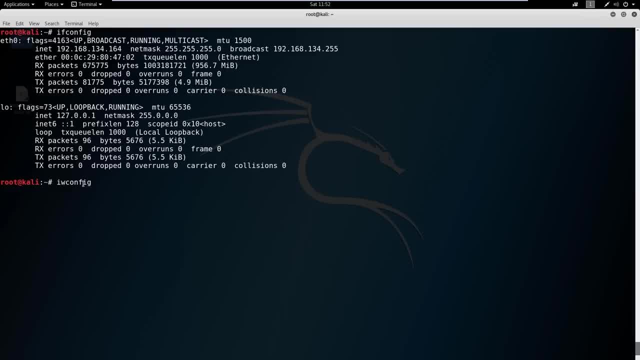 iwconfig, and you should not expect to see anything on this at the moment, unless you're using a laptop. then you actually might see a configuration down here for it. if you would see something under iwconfig, you would see like a wlan1, wlan0, something along those lines. okay, and another common command. 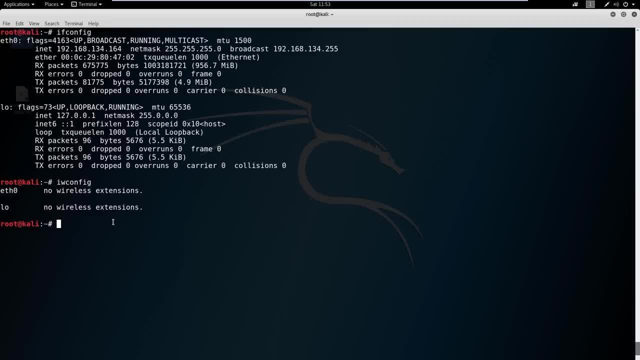 that we're going to see is going to be the ping command, so we can just type in ping and the address that we're trying to talk to. so, for example, I'm going to try to ping my home router and I get talking back. so if I tried to ping, 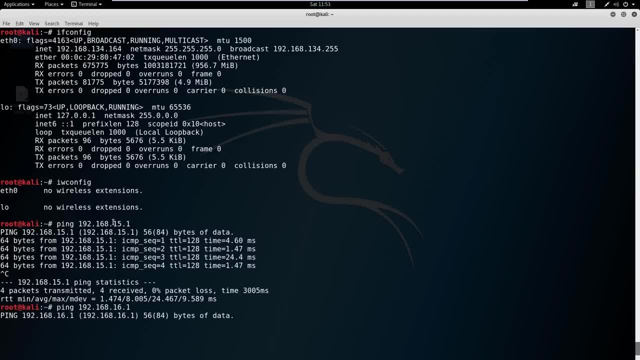 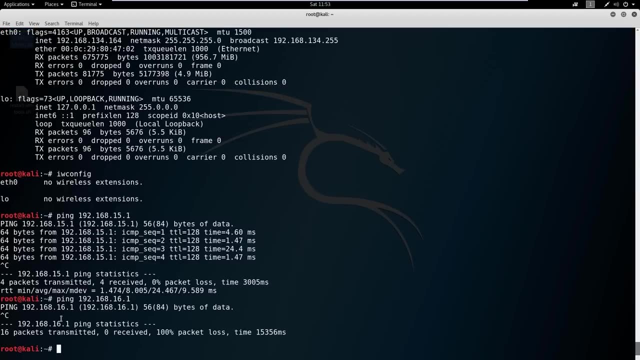 something that wasn't in my network, like a 16.1, you're going to see the results change. so with ping here, ping is going to be endless until we hit something like ctrl C to stop it. it'll ping forever. so I'm going to hit ctrl C again and kind of show you the difference. so you see that we 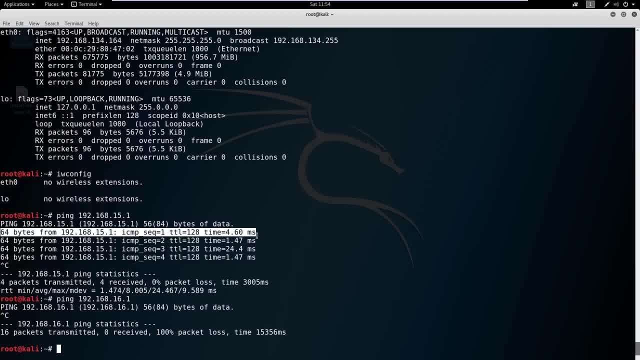 attempted to ping here and we got replies, we got information back. well, that's good, that means we're talking to the other machine. it says, hey, are you there? it says, yeah, I'm there, and we try to ping this machine here, but this machines not talking back. it could mean that the machine is on the network or 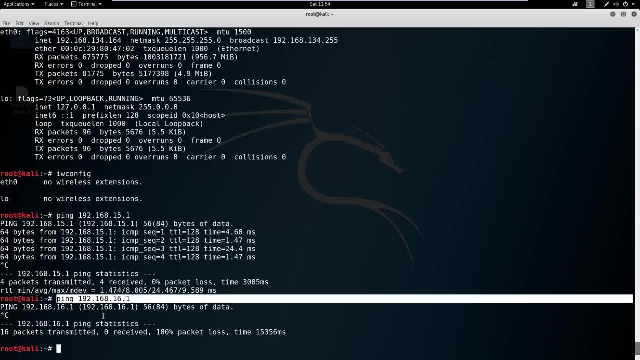 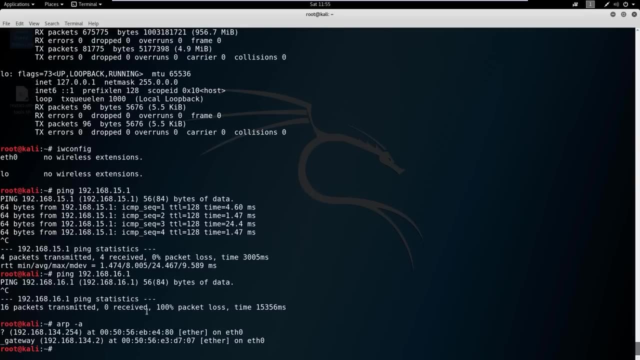 that the machine is just blocking ICMP traffic. I seen is a another word for régging. so, moving on to the next command i want to show you are so the best in it. Uh, just going to show you mac addresses that it talks to and the IP address. 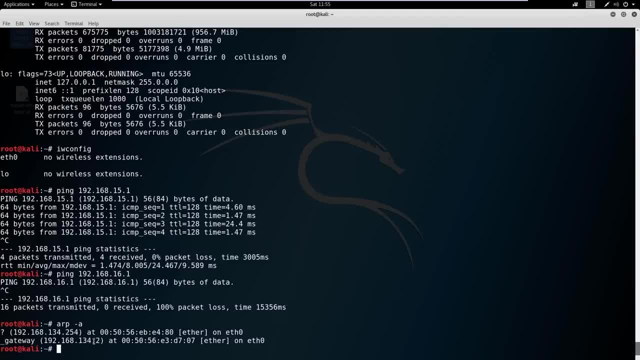 actually I said that backwards is gonna show you the IP addresses talks to you and the mac addresses and MAC address associated with it. so if an IP address reaches out, say 192, 168, 15.1, talked out to this machine, it's gonna say, okay, hey, who are you? it's gonna send. 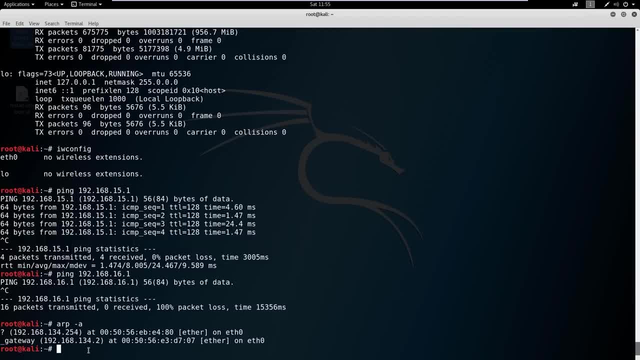 a broadcast message out to say who has this IP address, and then the IP address will respond. it says: hey, I do, and this is my MAC address. so ARP is just a way of associating IP addresses with MAC addresses and once you know that you can also look at net stat. so net stat dash a and L is another one of my favorite. 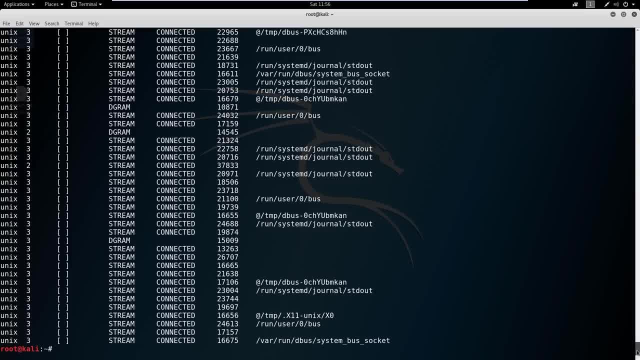 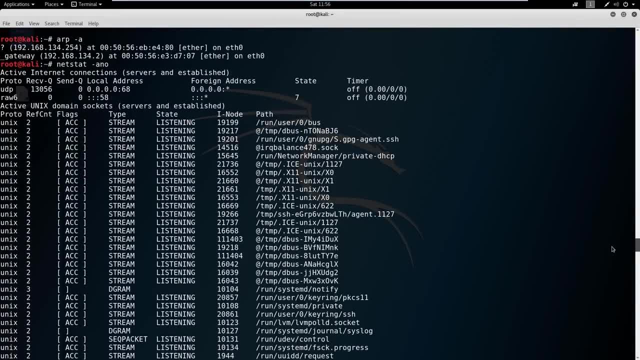 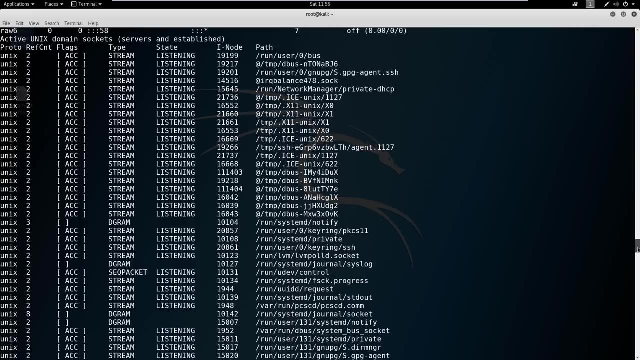 commands and this shows you just the active connections that are running on your machine. so if we scroll way up and you can just kind of see what's open and where it. what's talking here and where this really comes in handy on a penetration test is to see if a machine 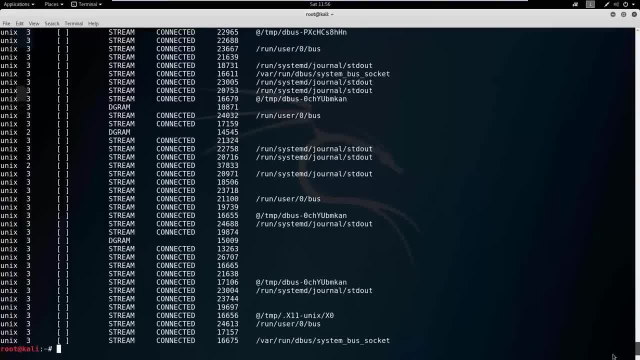 is talking to somebody else. same thing with ARP. you want to know what that machine is associated with. and is it talking to something on a port? so this is more just internal right now, but it's still good to know. so, for example, if I were to open up a Firefox page and connect out to the Internet, then I went. 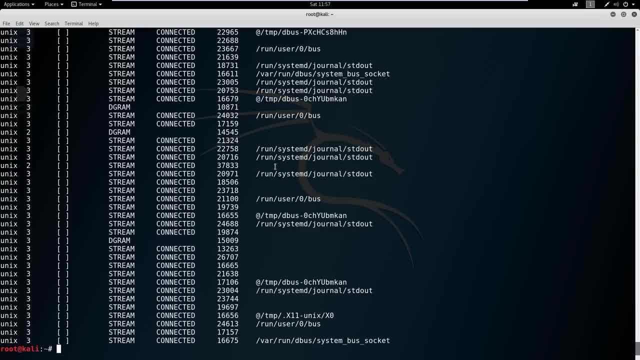 and I did a net stat again. I would see information about the internet and then I would see the internet and then I would see about that port being open and and that I am going out with it. so just kind of keep that in mind. these are not commands that you really need to know in depth. 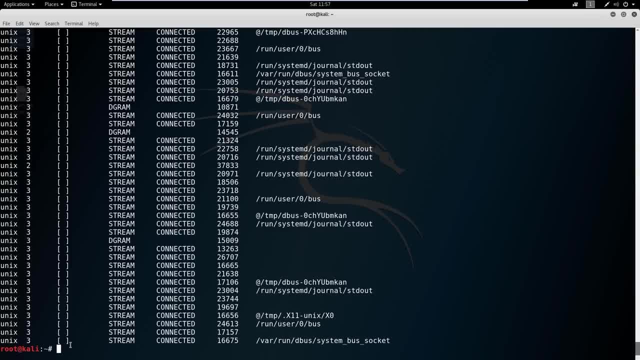 right now. network B does come into play when you are doing penetration testing. but we're gonna cover these commands time and time and again. I just wanted to give you a very brief introduction to them. okay, in the last command that I have for you today is route. so if you type in a route, that's gonna print your routing table in the 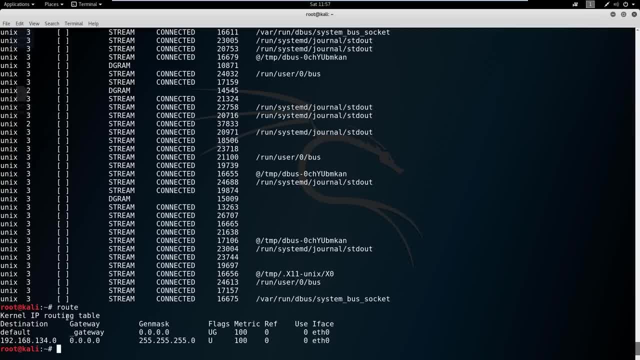 routing table is important because it tells you where your traffic exits. essentially. so, for this VM, my traffic is exiting on one, nine, two, one, six, eight, one, three, four, naught, zero. so any traffic goes out of this zero, dot, zero, dot, zero, zero, zero gateway in this range, right. so when it goes out this gateway, 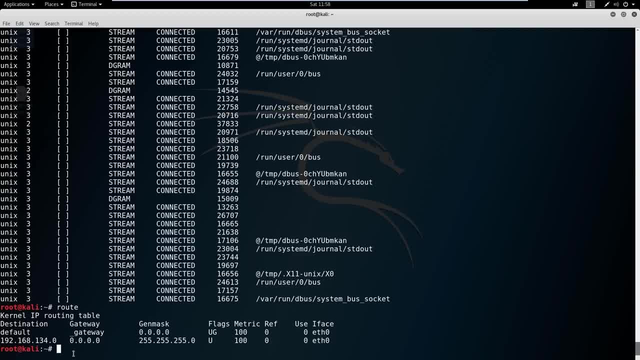 gateway. it's doing nat, so network address translation, and it's running off my computer. so the best examples aren't here. but it's important to know route as well, because there could be a machine that you're attacking that has multiple routes. so you might see a 134 and a 135 because 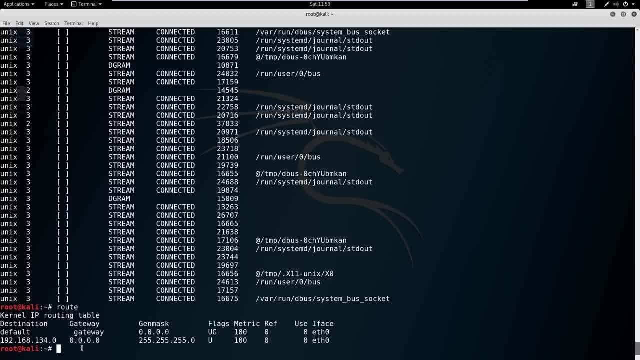 it has a dual home nick, the meaning it has two nicks inside of it. so it's actually talking to a completely different network that you didn't know existed. so you might have been attacking one network and the 134 range, and then 135 is just out there and this computer can talk to both. 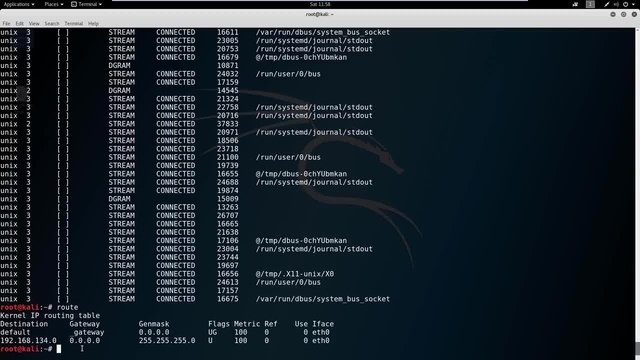 and until that point you had no idea. and that's the idea of called pivoting when you switch a network from one to the other but you're using a machine. so that's it for this lesson. in the next lesson we're going to talk about viewing, creating and editing files. 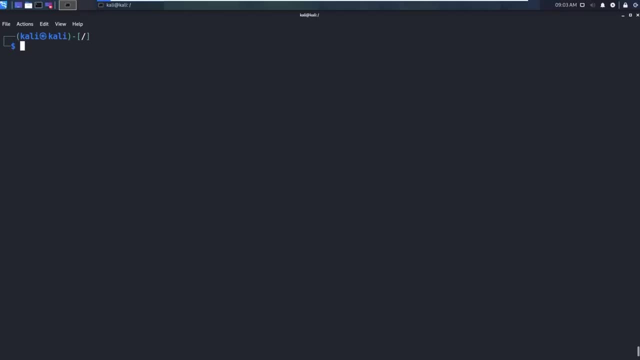 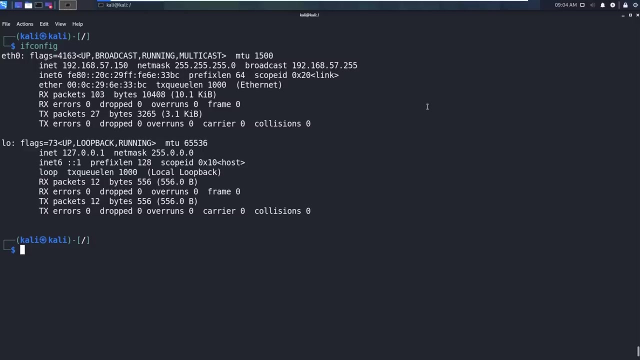 so in the last video we took a look at different networking commands. in this video i want to show you some updates to those commands. now we were running ip or ifconfig, so we were doing ifconfig and that works and that's fine, although it is becoming deprecated. 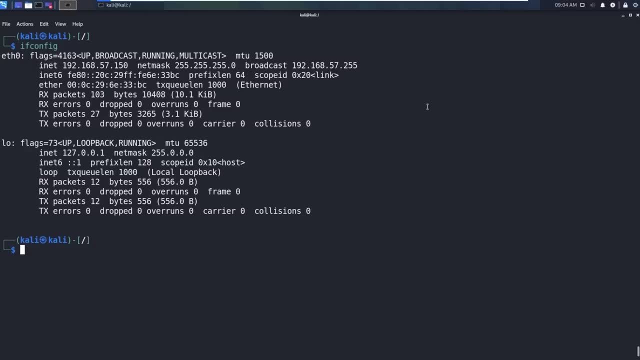 so it is still my go-to, if i'm being honest with you, because i like to stay old school. but i do need to show you the new and improved version of ifconfig. so if we take a look, i'm just going to clear my screen here. so the command is ifconfig. so if we take a look, i'm just going to clear my. 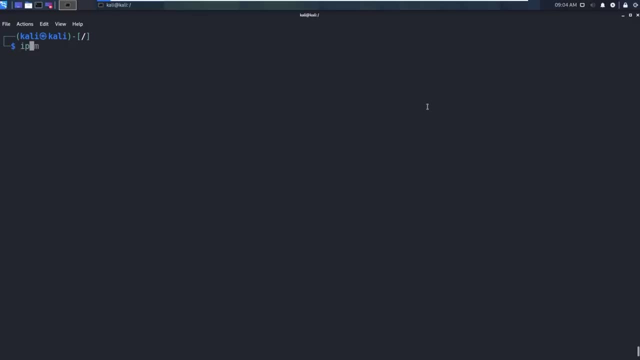 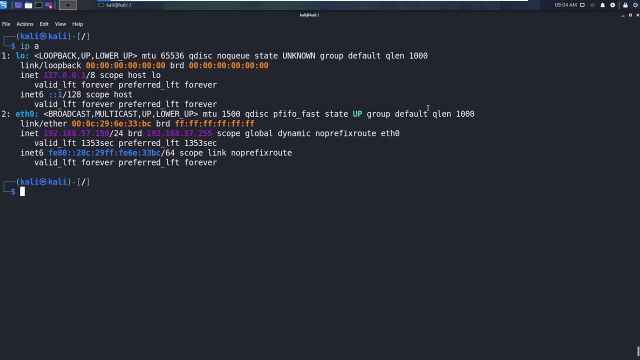 screen here. so the command is ifconfig. so if we take a look- i'm just going to clear my screen here now- we can say ipa and we can look at that, and that says ip address. and what do we get here? well, we get our loopback and we get our ethernet and we still get to see. 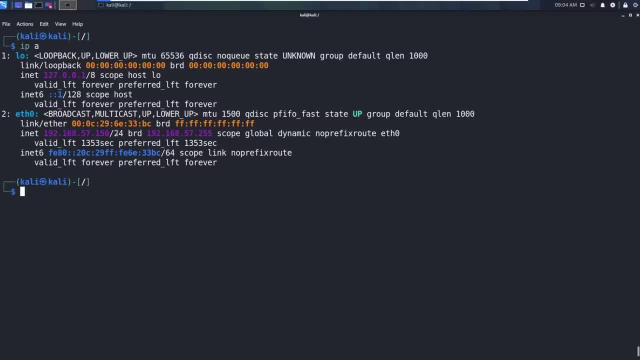 what our ip address is. we get to see what our subnet mask is. here as well, we get to see our broadcast address. so there's a lot of information here that is provided, which is good. we can also take a look at some of the stuff that i was showing you before. so say, we want to look at the 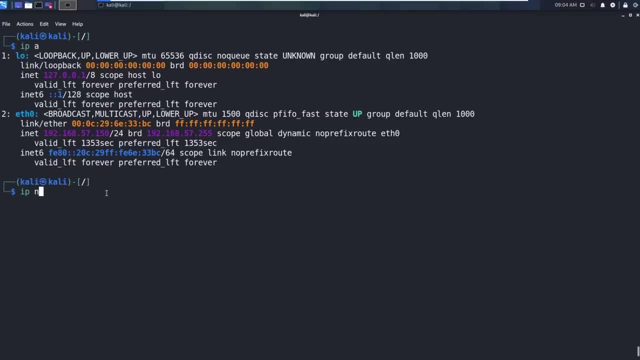 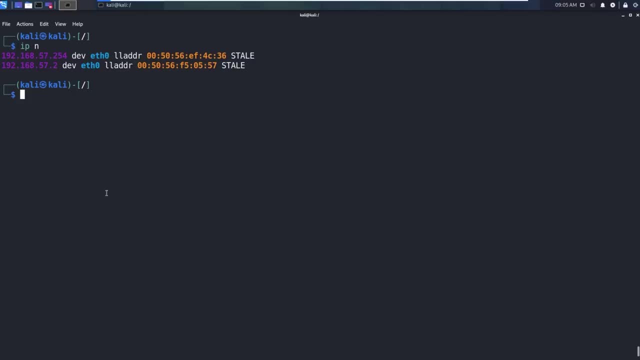 arp table. we can say ipn, which stands for neighbor, and clear this: and here's our arp table. okay, so very similar. and we want to look at routing tables. we can just do ipr. so instead of having to remember: okay, arp, or we're having a look at route. okay, we can do. 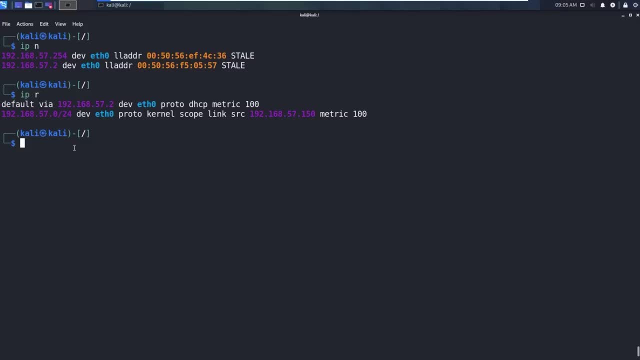 all of this through one command, which is the ip command. so i just wanted to add this updated video to kind of show you that there is this command out there. this is where the industry is moving. this is something that you should know, but it is perfectly fine in my book if you still want. 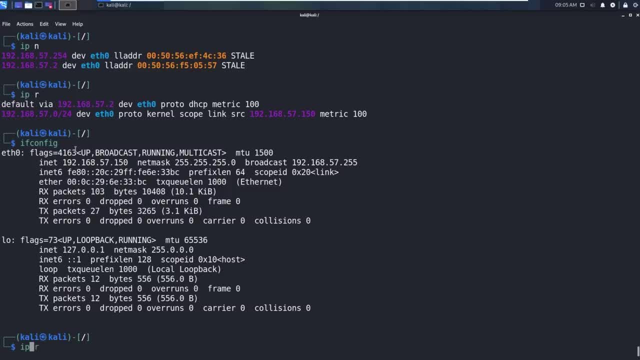 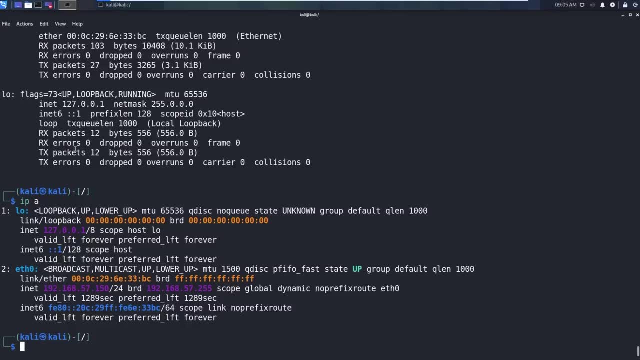 to use ifconfig. nothing wrong with ifconfig, nothing wrong with using ipa. both are fine, okay. so just another command for your repertoire and for your tool belt and something to keep in your back pocket. so, with that being said, we're going to go ahead and move on to the next video. 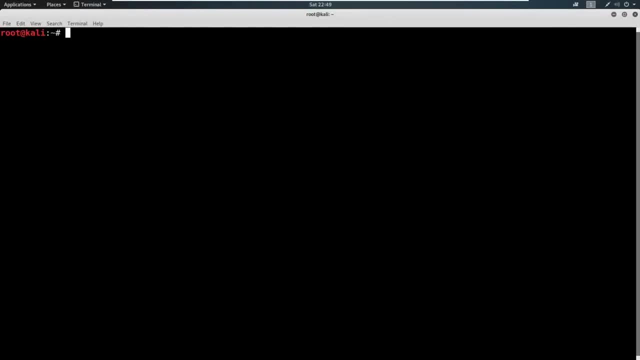 all right. so second to last video here in our linux series, and this one is a very important one. so we're going to cover a few things. i want to cover how to install files, how to install updates and how to get files from github. all these are going to be. 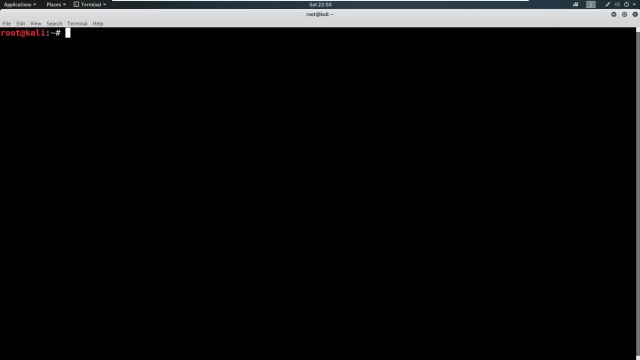 very important and things that you're going to encounter as a pen tester all the time. so from a linux perspective, let's say that you want to update your system and you're in the terminal. what you can do is you can say something along the lines of apt update and we'll say also apt upgrade when you're done with that. 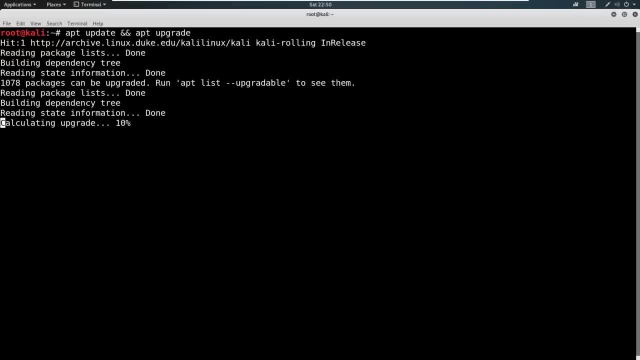 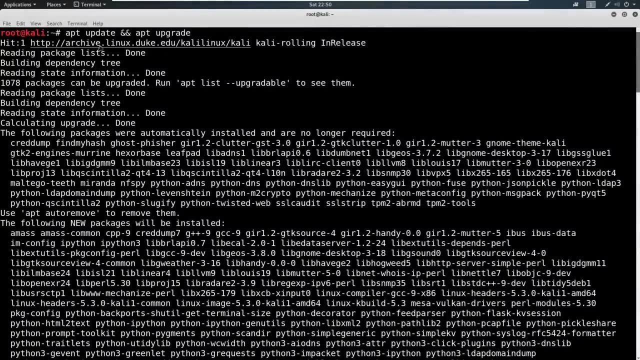 so what this is going to do is: this is going to go out and you can see these archiveslinux- i'll scroll back up here- and all these tools need to be installed, but this archivelinuxedu. so this is what's called a repository. so we're going out to 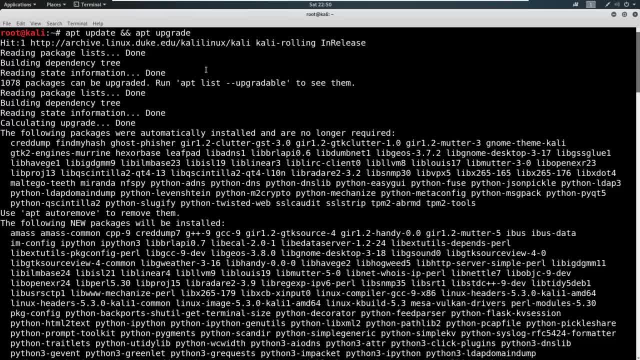 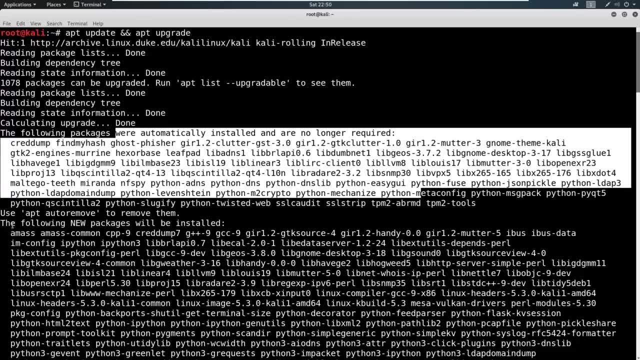 these repositories and we're saying, hey, what's been updated lately and what do we need to download? and we're going to say, okay, these packages that are automatically installed no longer required. we can auto remove them if we need to. and then we have all these new packages that need to be. 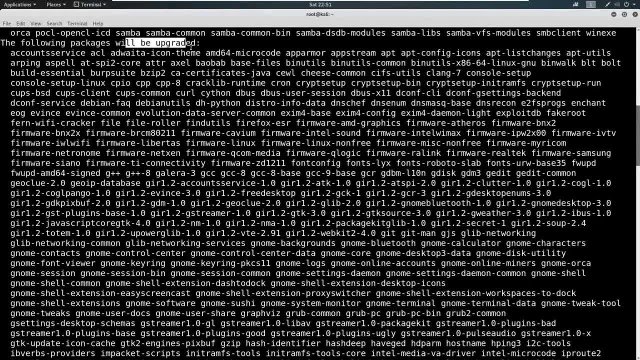 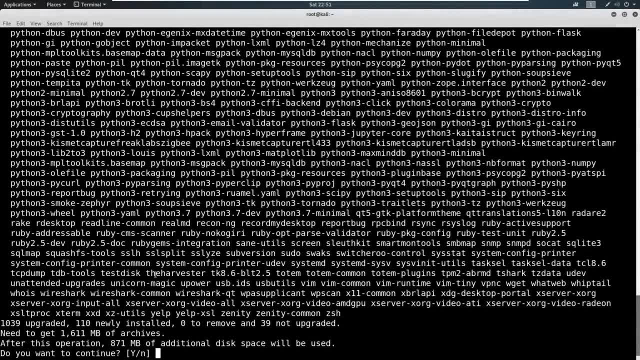 installed. if you look through the list, it's quite a bit, and then we've got the- the packages that will also be upgraded through here as well. so we have all these updates, upgrades, etc. if we want to perform this, it's going to take up 871 megabytes of additional disk space and it will probably take. 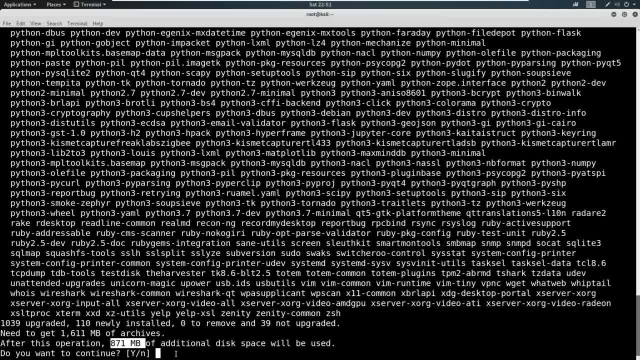 a little bit of time to download, upgrade etc. so if you want to do this, go ahead and push your update. you absolutely don't have to to be successful in the course, but just to provide clarification and understanding of how it's done and what it's doing. just wanted to point that out. now let's say we just wanted. 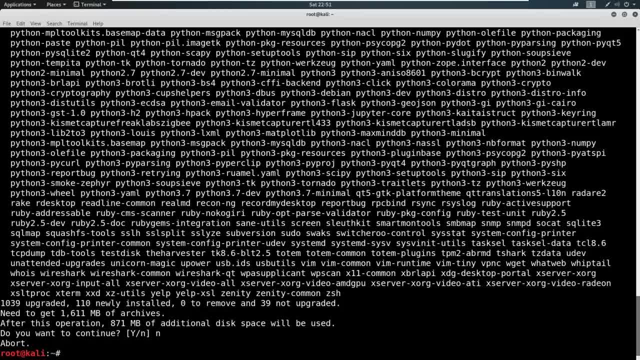 a tool, a specific tool. you see all these things in here. a lot of them are related, like python, which is interesting, because i do want to install a python tool. so let's install a tool called pip. so what we're going to do is we're going to say apt. 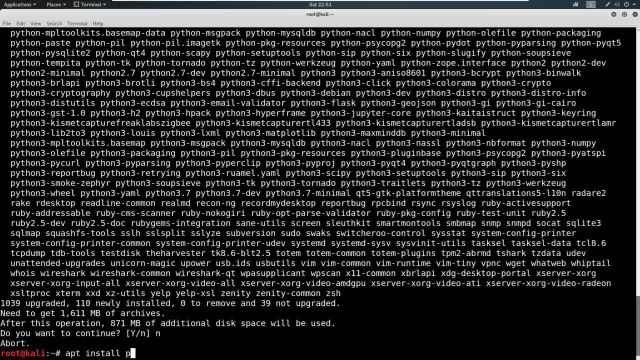 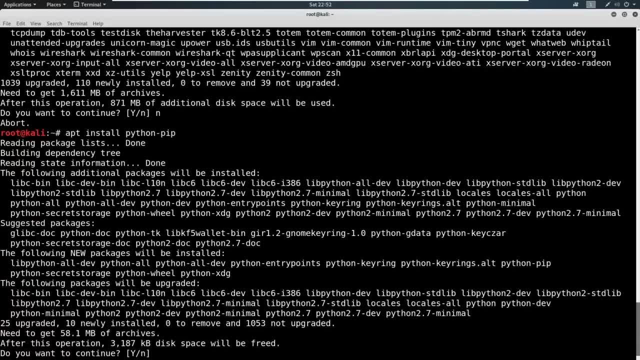 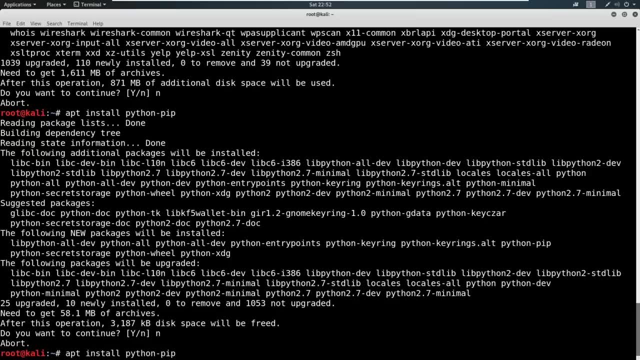 install and then the tool is called pip, but it is python-pip like this. so type that in hit enter. it's going to go check for it, it's going to look for it and it found it, which is great. if it were weren't to find it, it would say something a little different. we can show you, like say: 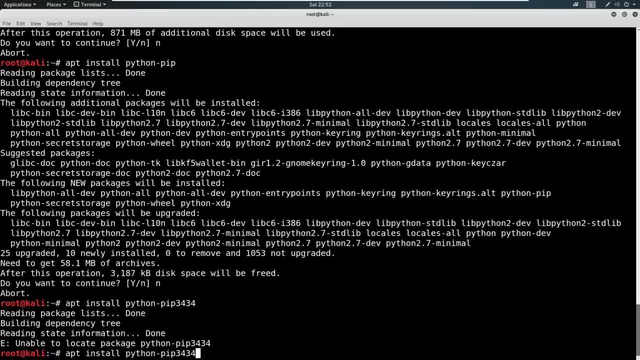 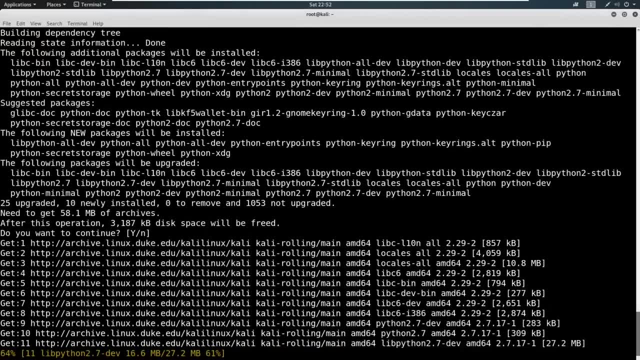 just hit some numbers in there, say unable to locate that package. so you'll know you're on the right track with the package name here. so i'm going to go ahead and actually hit yes to install this. it's going to go out and download it and then we're going to go ahead and install it and then 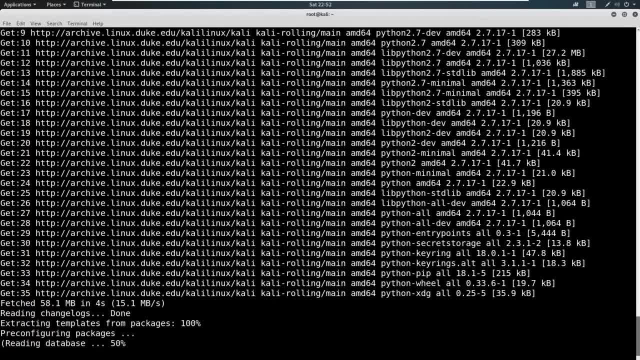 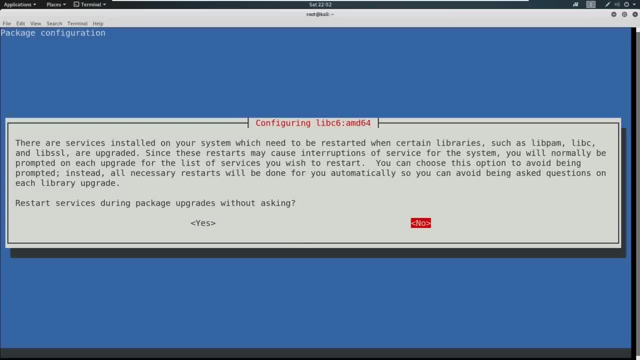 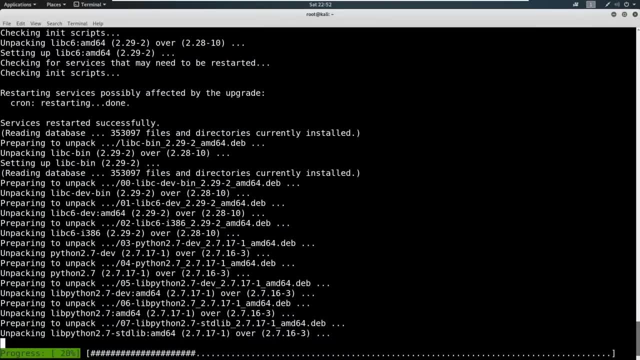 we're going to go ahead and download everything we need for pip and you're going to see why pip is important here. so there is pip and there's pip3. now both of those go out and do some installs for us and we're going to go ahead and just say: yes, and those installs are related to python, so we're. 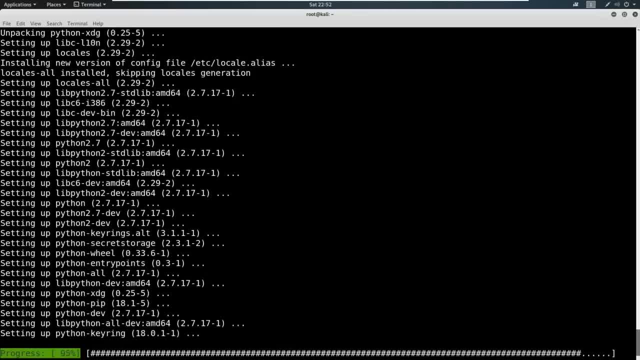 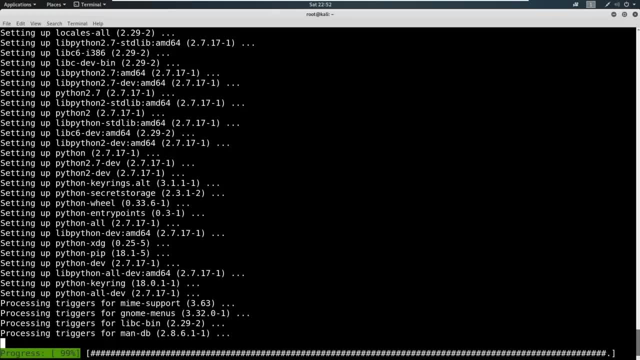 going to use a lot of tools in this course that are related to python, and it's going to install those tools for us. so pip is for for python. pip3 is for python3. now python3 is for python3. python3 is the latest and greatest. python2 is actually being deprecated in 2020 or end of. 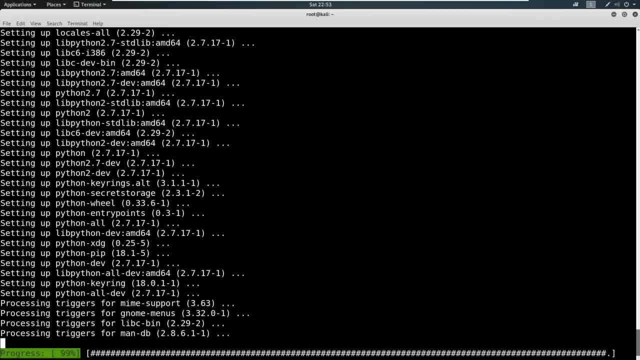 service in 2020. so a lot of things are actually moving away from that now. so when we get into the python section of the course, we're actually going to be working completely in python3, for this reason solely. so, while we wait for this, let's go ahead and go out to the interwebs. 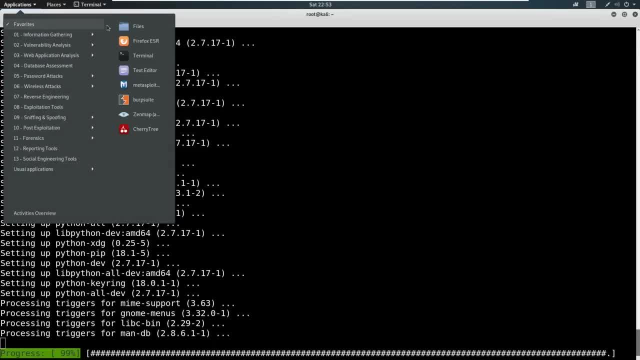 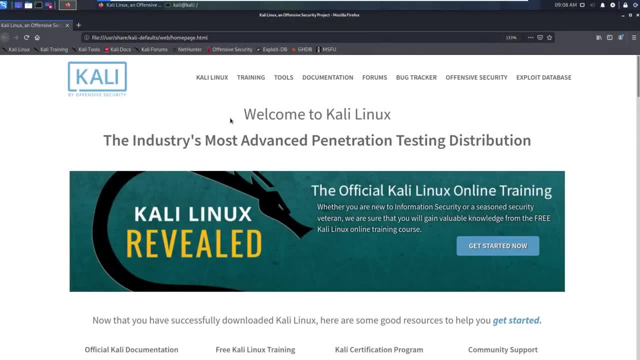 and i'm just going to applications up here and then firefox terminal from here. as an update to the course, i want to introduce a tool and teach you also how to install a tool. so this is kind of serving two purposes here. so i want to go out. 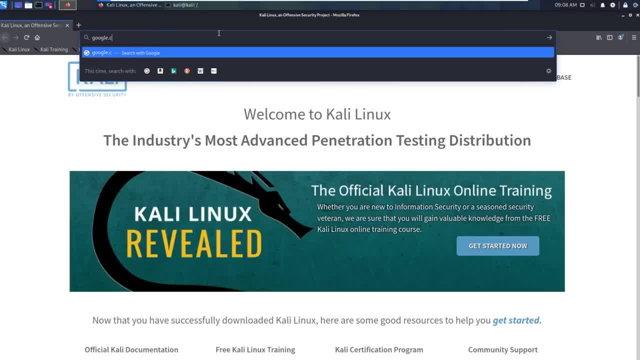 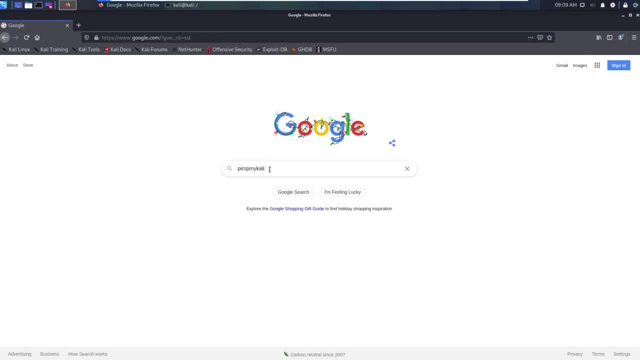 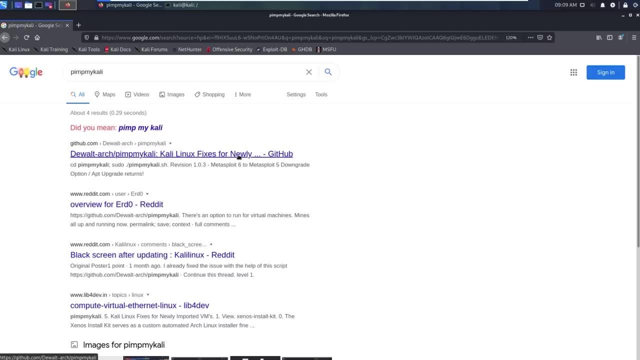 to google, and what we're going to do is we're going to look for a tool called pimp my cali, p-i-m-p my cali, just like that. now, this is written by a guy named dewalt. he is a Windows Cloud Unit outside of google, and uh, well, what's the word we use? and then we'll talk. 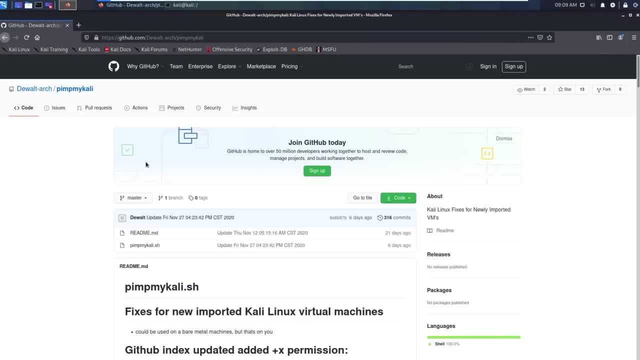 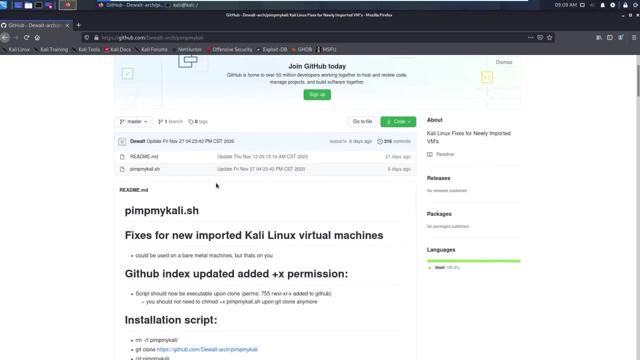 about pimp my cali with much more depth in that later, because he has a pretty good wanted to all of those issues. okay, so we don't have to go through and troubleshoot a lot of things throughout the course. this script just kind of goes in and fixes a. 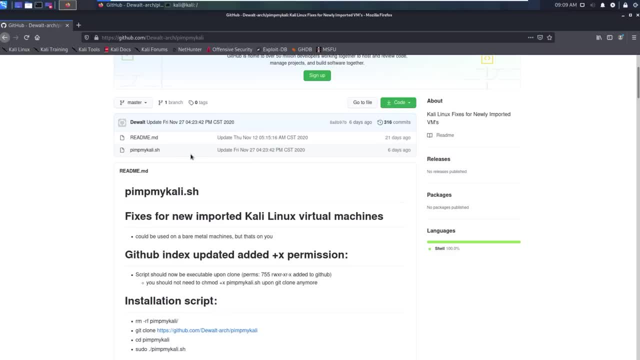 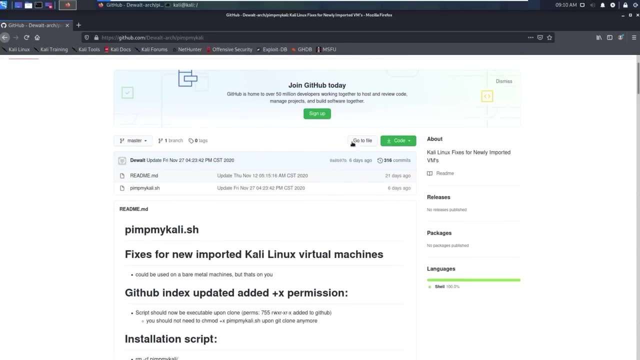 lot of things that were wrong, so I really am appreciative of this script, because it has fantastic. what we can do is learn from this as well, though, so what we can do is we could take this code and we could just copy it here. okay, we can hit ctrl a, ctrl C, or you can hit copy on the clipboard what I want you to. 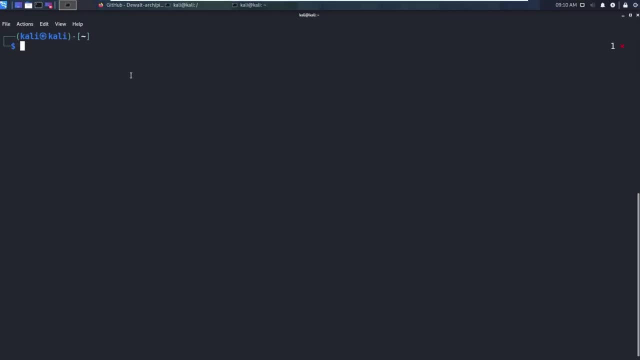 do is I want you to go out to a terminal. we're gonna go ahead and just sudo, switch user, okay, and enter in our password. now we're going to install something from github. so what we're doing- and this is very common, by the way- you're gonna see this happen throughout the course. we're gonna put this into a. 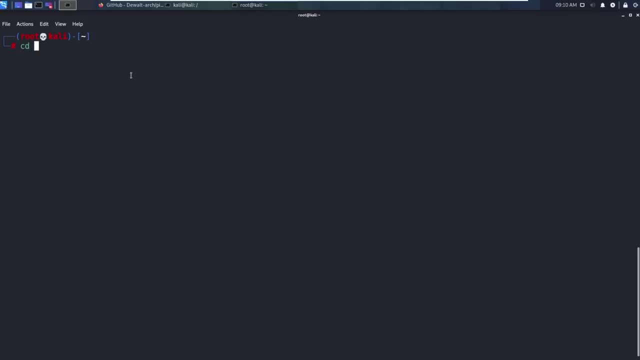 folder. so what I want to do is change directories to a folder called opt opt, just like this, and hit enter and we're going to put our file here. now. this is very common. a lot of people tend to put their their downloads or installs into the out folder. it's just a place to 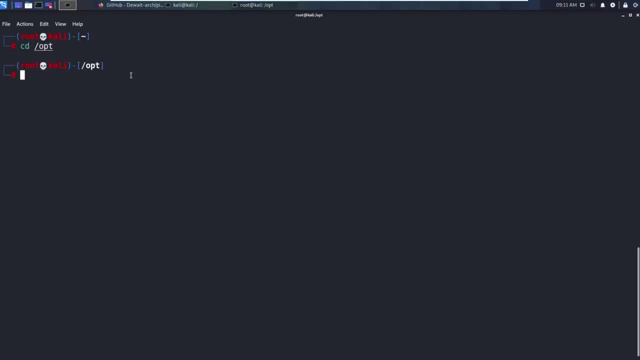 keep all these. so this is a common thing to do and a good practice to get into. if you've never done this before, so now what we're gonna do is we're just going to type in git clone and then we're gonna paste it so you can do control. 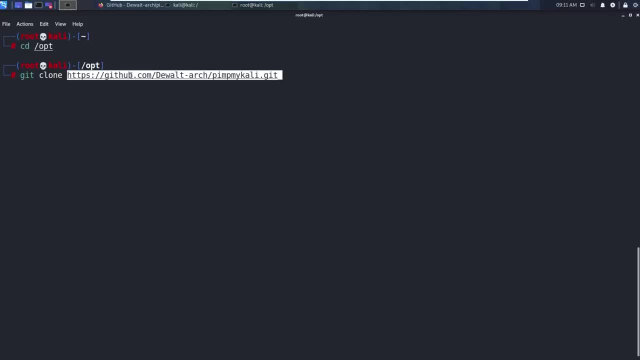 shift V as a shortcut, or right click and paste, hit enter and you can see it started cloning. now, once it's done cloning, all you have to do is change directory into the file name right here or the folder name, so CD, we'll just type in: pimp my Cali tab, hit enter, okay, and from here we can just do. 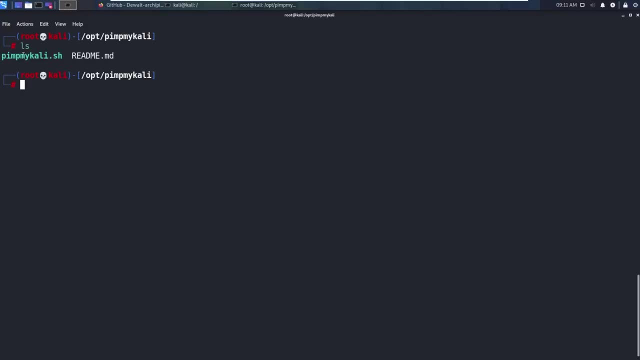 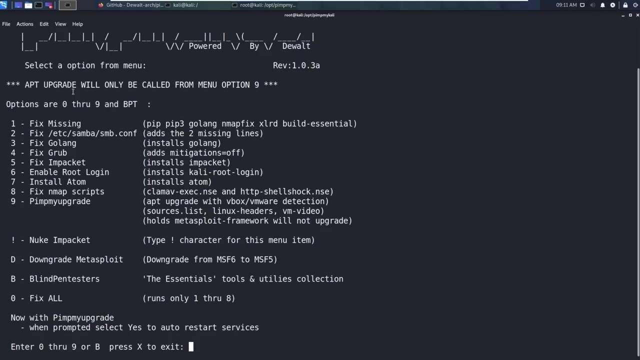 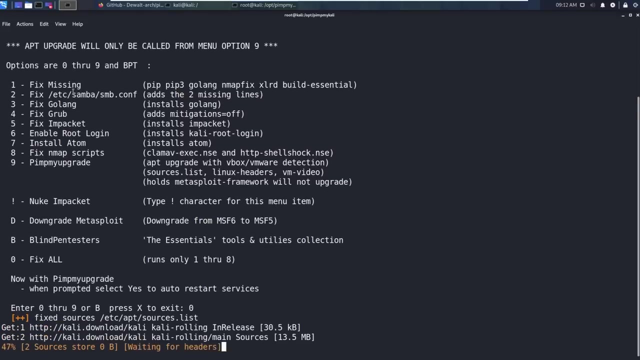 LS. look what's in here. okay, so you can see it. pimp my Cali sh. we're gonna go ahead and just run that. so dot forward, slash, pimp my Cali sh, just like that. hit enter, alright, and we're going to run zero here. okay, and this is going to take a minute, so it's gonna go through and run all. 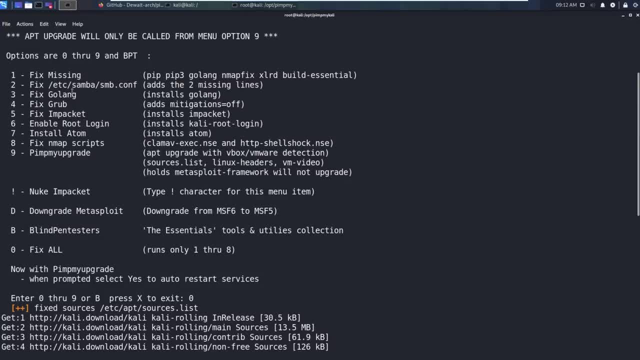 these upgrades that you see here. so what it's doing is it's fixing some of the issues that we have. so we're fixing go and we have to install go later. we're fixing impact it, which has some issues on its own in 2020, point one and later. 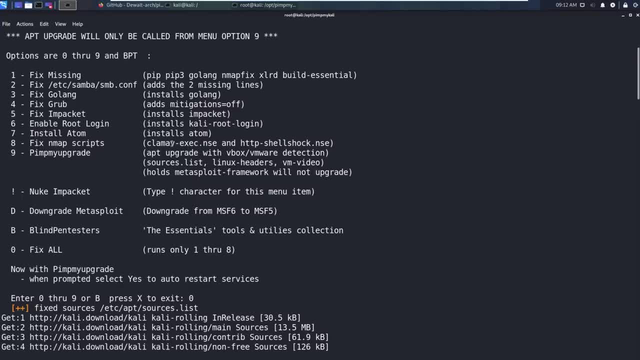 and we're also enabling root login. so there's a lot of things that we're doing here that help us out throughout the course and is just a nice overall upgrade. there are some other features that we're going to be looking at as we go through the course. so, as you'll see, we 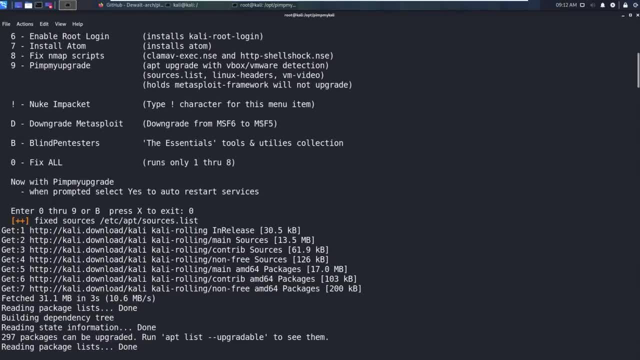 have the ability to downgrade from Metasploit 6, so if you do encounter issues in the course, you can come back and downgrade to Metasploit 5, which is what we are currently doing. but as you go through the course, Metasploit 6 might. 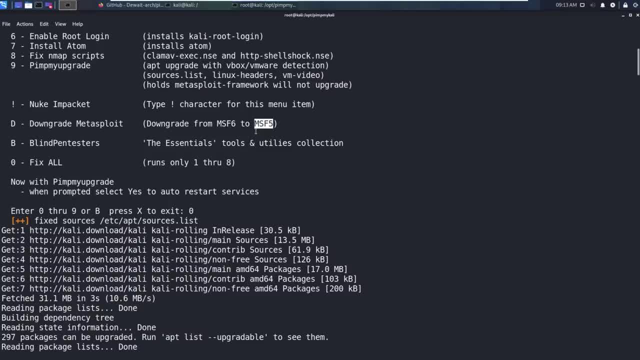 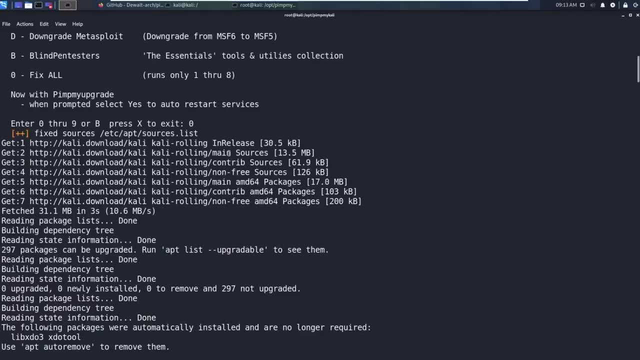 be working or more functional as these tools upgrade and things go on. you know you have to kind of evaluate what's working, what's not working and take it from there. so, as the script gets updated constantly, be on the lookout for these things as they get added or removed. 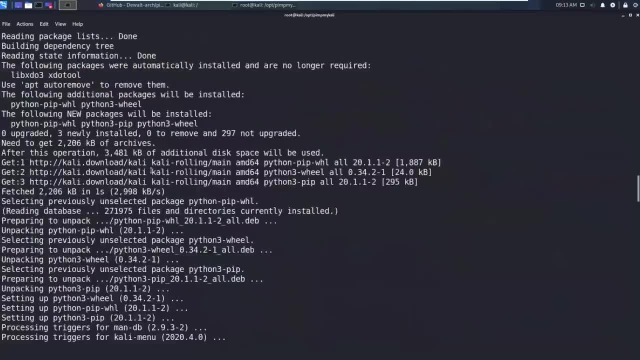 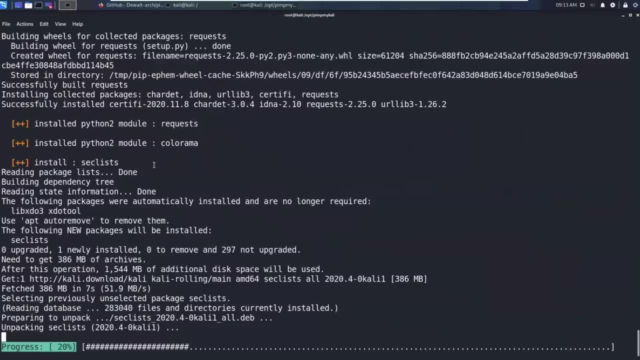 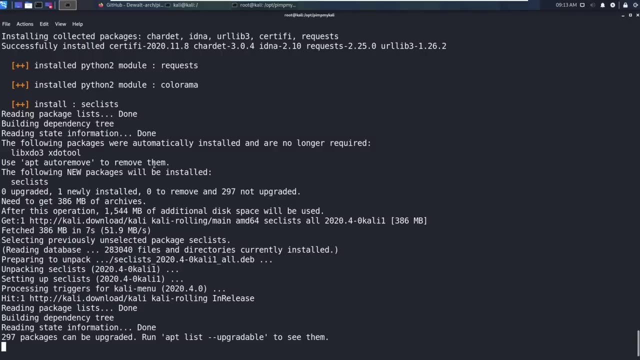 but for now, we're just running the zero, we're going through and just adding all these different tools in. you should see it scrolling along like this and should function pretty, pretty straightforward. so go ahead and let this install the big takeaway here and once, once you're done, go ahead. we're going to move on to the next video. 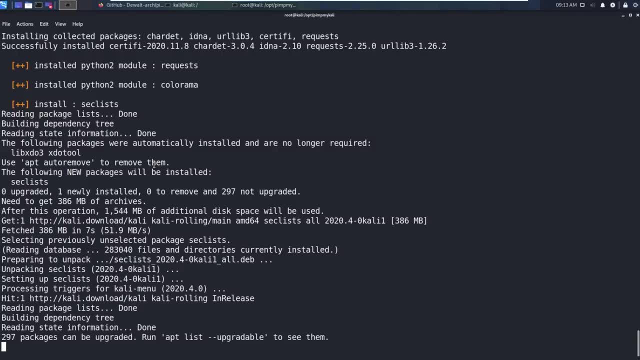 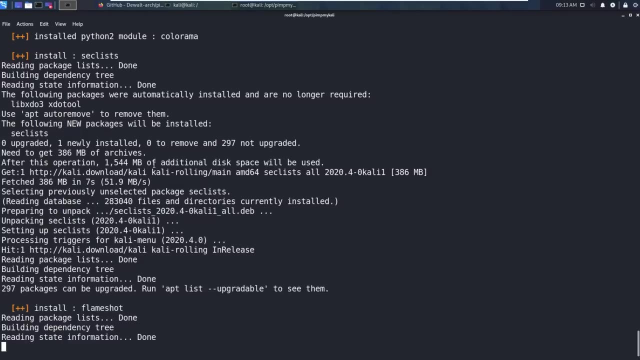 but the big takeaway here is that you should be comfortable with using the apt package to go out and download tools. you should be able comfortable with upgrading your system through apt and you should be comfortable now with going out to the web- github at least- and going and. 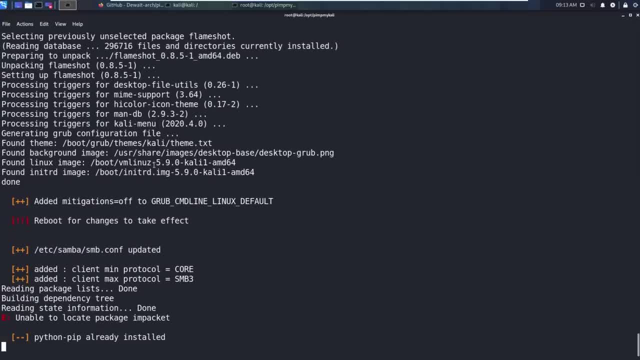 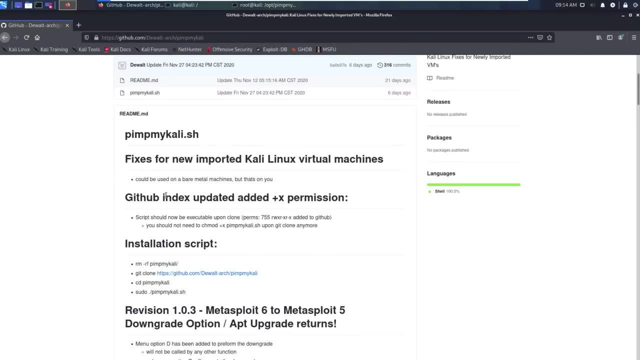 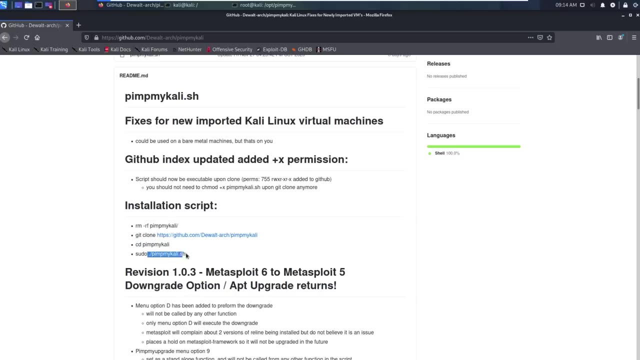 downloading a folder or cloning a repository off of github and installing it on your own. it's very straightforward. if the github is good, the github will tell you: hey, here's how you install it. and it'll say these are your instructions. like right here. it says here: git clone cd into it, dot forward. 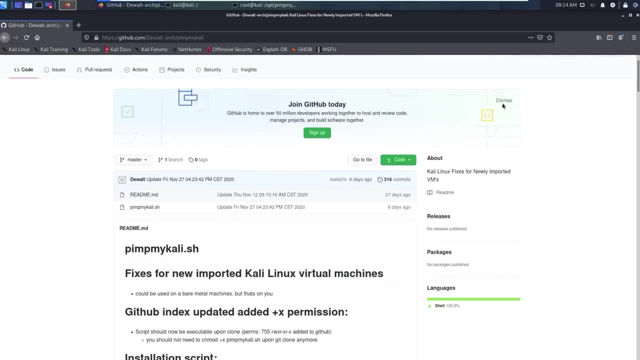 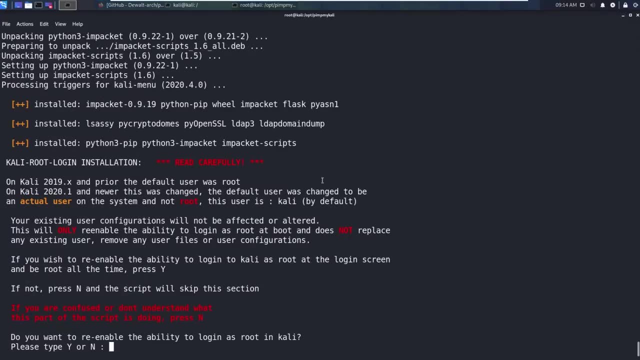 slash. put my Cali straightforward, and most, most githubs are like this. so as we download tools in the course you're going to get more practice with this and understand it better, but from here you're going to just take it and go, and here you can see. something that we talked about is that we 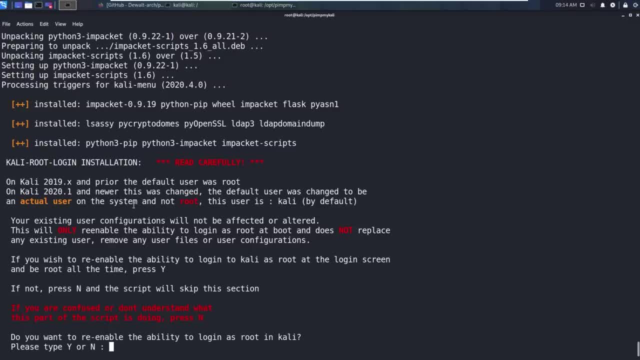 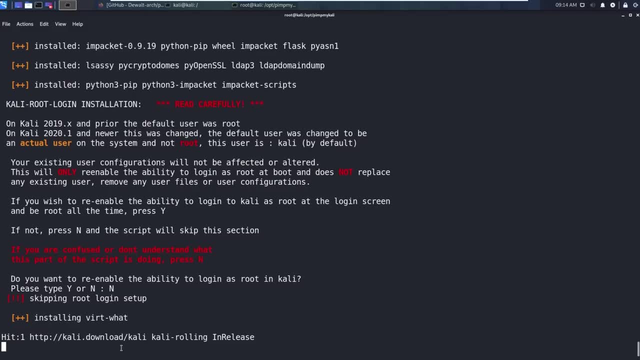 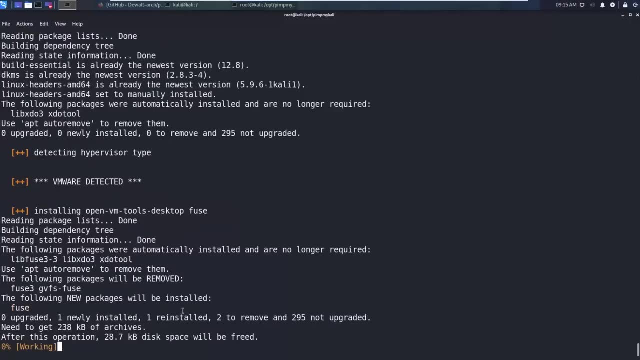 are lost the ability in 2020.1 to use root. this will allow you to run root in Cali, if you want. here we're just going to type in no. unless you know what you're doing, you could type in yes, but again, as stated in the pseudo video, if you are not familiar with Linux, it's best practice just to. 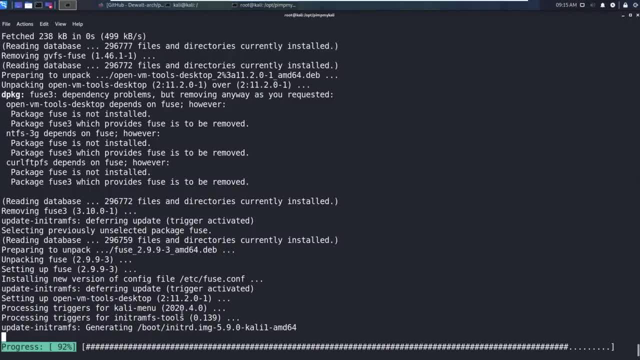 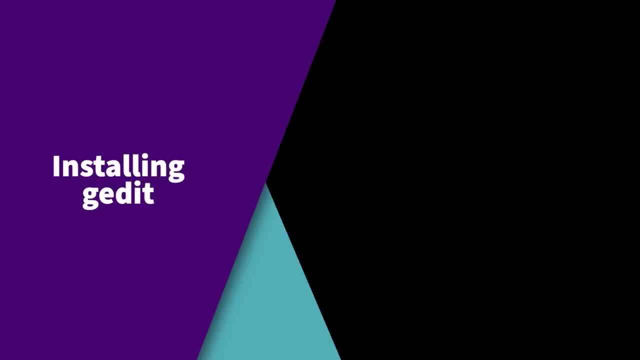 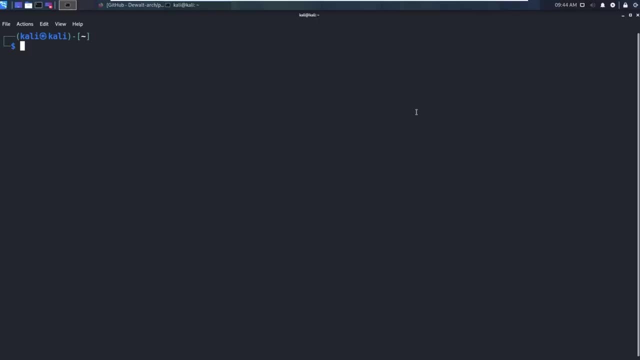 keep hanging out in pseudo and utilizing it that way as a low-level user. and again, we're just going to let this run and I will catch you over in the next video. so there's one more tool I want to install because I use it quite a bit throughout the course as my go-to note editor, and I'll talk some alternatives as well. 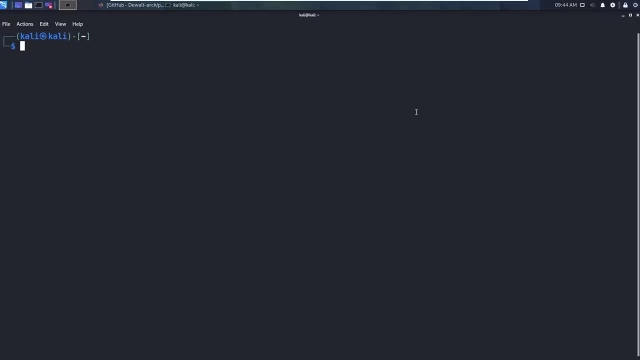 but I just want to make sure that you have it installed and you have it at your disposal if you want to use it. it's not the only text editor in Linux and I'll show you those options. but that tool is going to be called gedit. so if you just do apt install gedit like this, actually let's do a pseudo apt install. 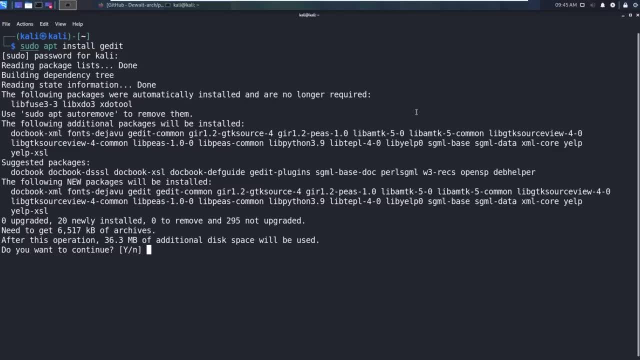 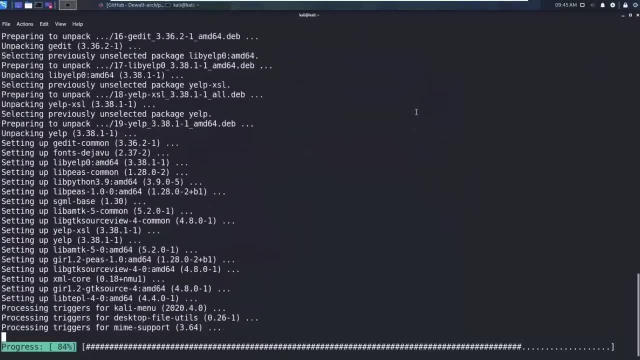 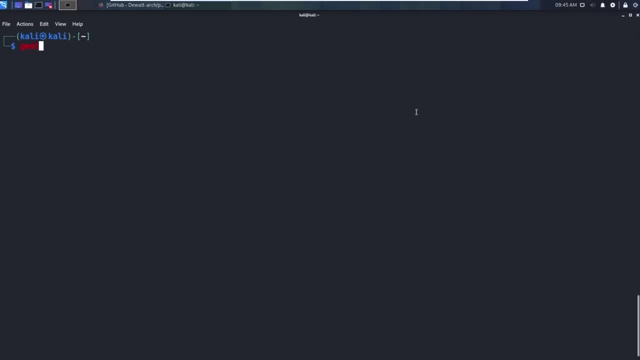 like that: enter in our password and then go ahead and just hit enter, for yes, we're going to let this install and it should be pretty quick. now, what this is going to allow us to do is just have a text editor option. you're going to see this in use in the next video, but we get to say gedit, testtxt. 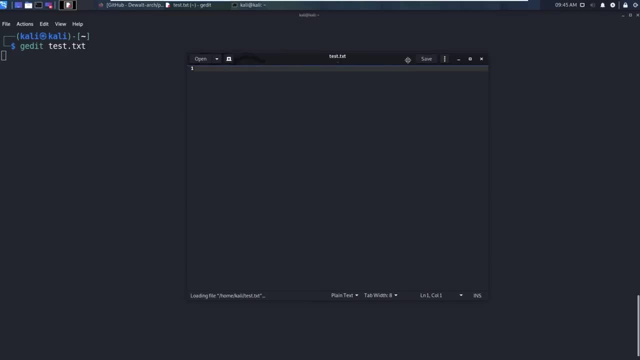 as an example, and it'll bring up this text editor. plain and simple. that's all it is. now you'll get some warnings like this: if you see a warning, just ignore it, don't even worry about it, as long as you're able to get into the text editor. 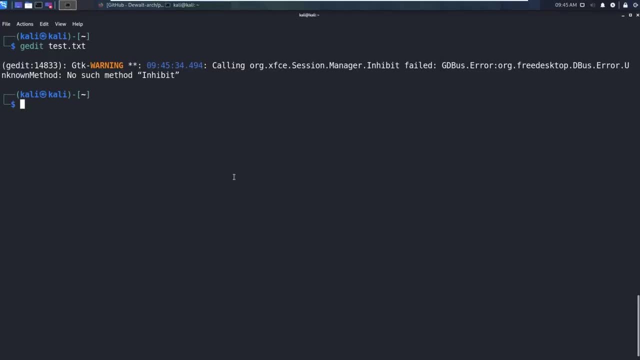 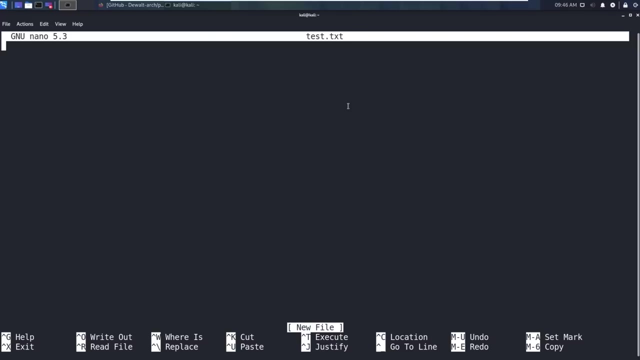 and edit, that's fine. I'm going to close this out without saving. another thing that you can do is you can use mouse pad and just say testtxt, that's fine. and you can use nano testtxt- same thing, and you'll see these throughout the course, so don't worry about having to memorize them right now. but 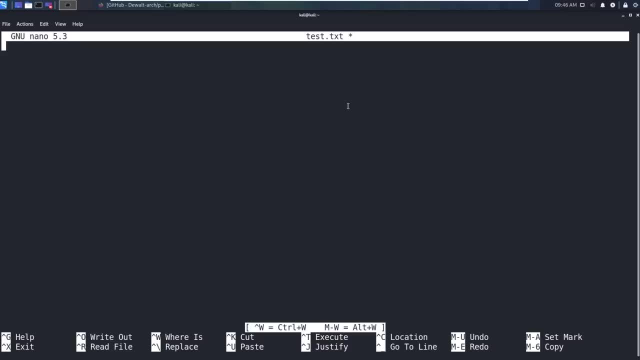 there's a few different text editing options. I just wanted to install gedit and show you gedit because I use it so much throughout the course, and they removed it from Kali Linux in 2020.1 I believe. so I just want you to be familiar with it and know how to use it if you want to. so that's it, we're. 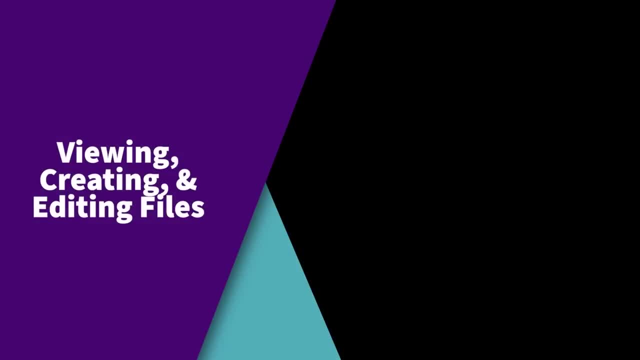 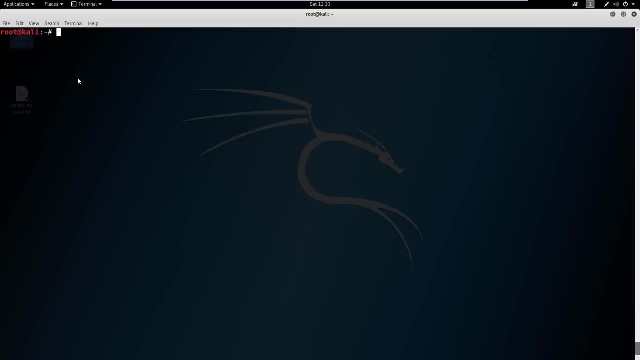 going to go ahead and move on to the next video. okay, so this is my second time recording this video. I'm going to turn my microphone on and performed for my cat, so she approved of it. let's see if you approve of it the second time around, now that I have a little bit of practice. so we're going to. 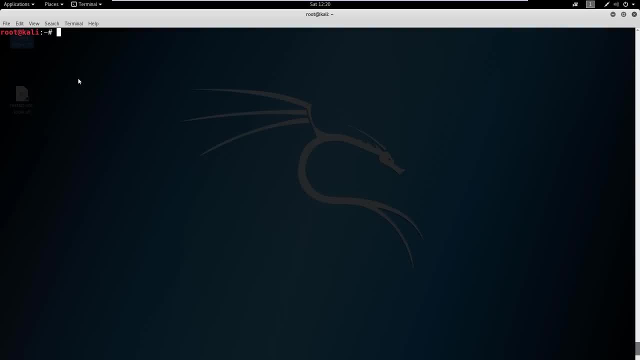 be talking today is we're going to be talking about viewing, creating and editing files. so I've already showed you the echo command. if you recall, we used echo to create a file. right, we created a hellotxt and we can just echo hello out to the terminal. we could say echo hello and I'll say: 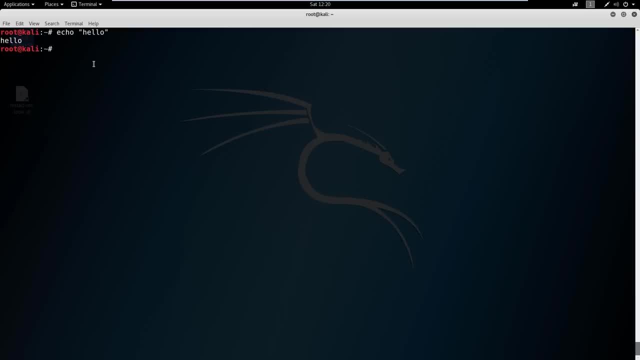 hello. so what we can do with echo is we can use it to write to a file. so if we were to say echo hey, and then we write it to hey text, well we can look and see that hey dot text is here and you can see my files from the previous one. so I'm trying to come up with more ways of saying hello. 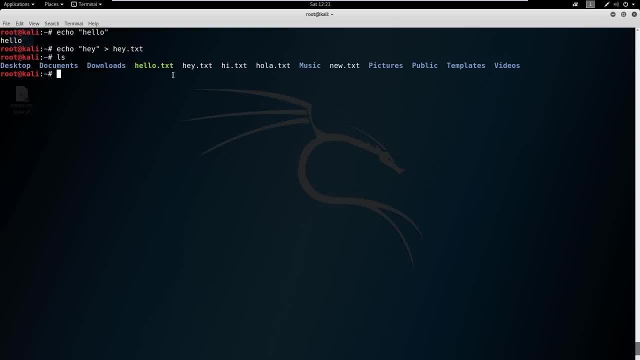 but we're going to use echo in this case. I'm going to use echo hey dot text and I'm going to hey dot text here. so if we cat hey dot text, a all cat does is print out to the screen what is in a file. it says hey, okay. so let's say we want to append cat. 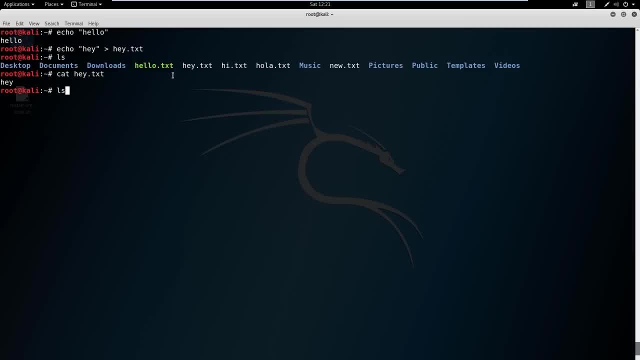 or we want to append hey dot text. well, we can tab up here. what if we just say hey again? we've got this greater than symbol here and we're just putting it into the hey dot text file. well, that didn't work, we didn't append it. we. 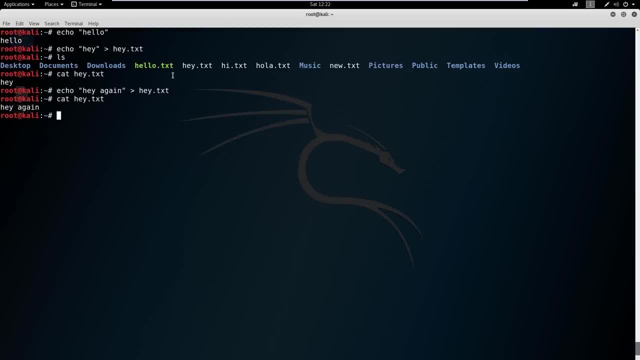 actually overwrote it. so what if? what can we use to actually over append this here? what we can do is we could say: hey, again, again, right, just to give us something different, and we can add a second greater than symbol here. so now, if we cat the file, you can see that we actually 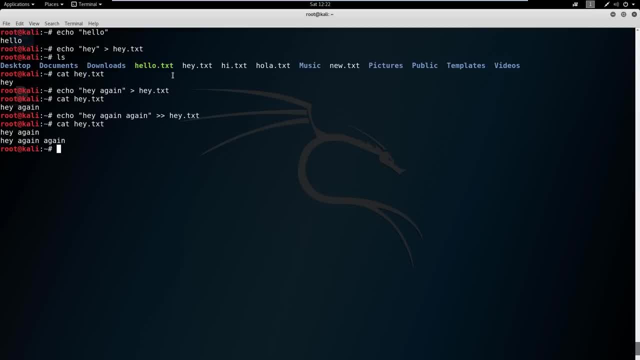 appended to the end of it. so this becomes incredibly useful when we are either adding stuff to a list- say, we're gathering IP addresses and we just want to combine our lists- or when we're creating a series of commands and we're going to use those commands to send all at once. we're going to cover that later. 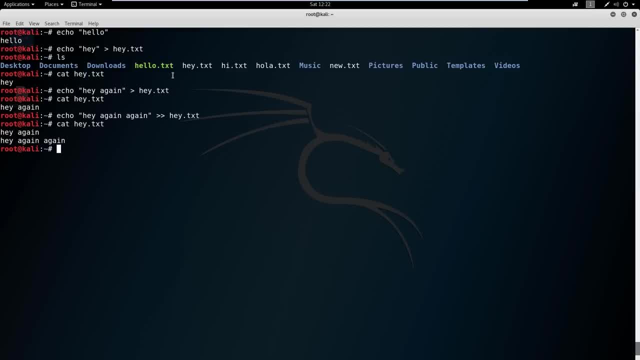 when we're talking about file transfers in the penetration testing section, where we use a set of commands like this on a Windows machine to actually transfer files via FTP. it's just so much easier than typing them all in one by one. we can create a little document and run the document. so this becomes useful when we have a 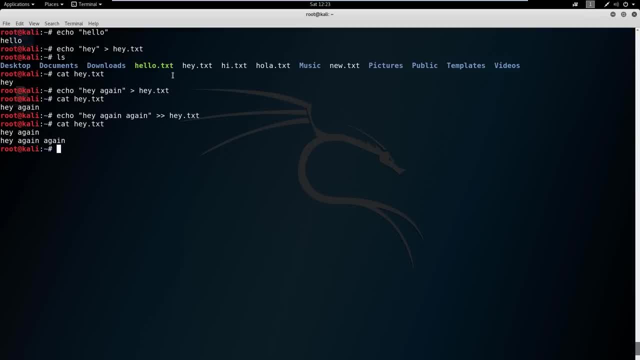 series of commands, and for other reasons as well, as you'll learn as you go on in your Linux career. so we've talked about echo and we've talked about cat, so let's talk about some other ways to create a file. we can use something called touch. 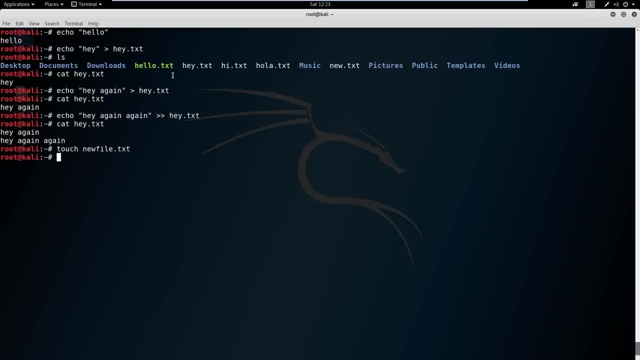 and to say: new file, that text, and if we LS, you could see that new file, that Texas here. but if we cat new file, there's nothing in there because they have a put anything in there yet. so there's a few things that we can do. we could use echo and append the file, right. we can also. 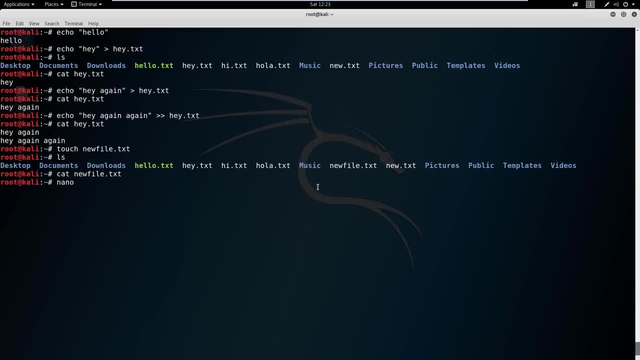 use a tool called nano. nano is a terminal text editor. there are other terminal text editors, like by in Vim. I don't prefer those. personally, I like now the most. some people have their preferences, so I encourage you to play around with any of them as you wish. 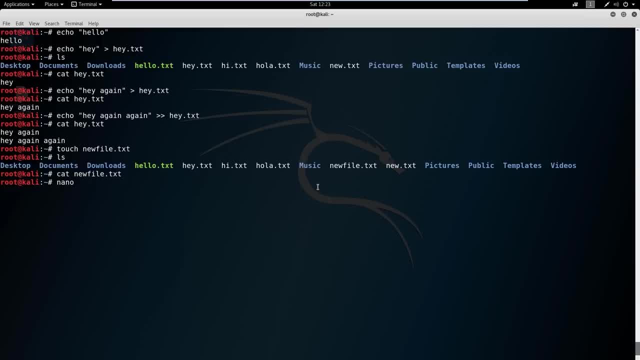 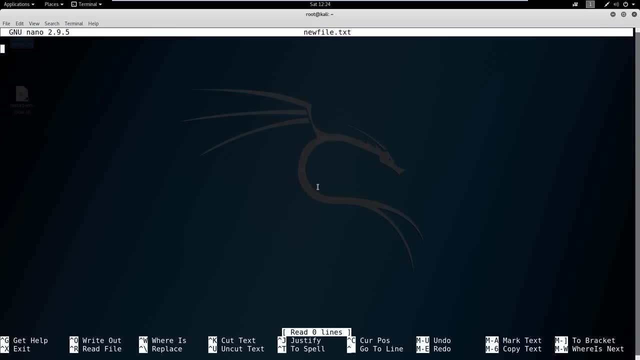 by, and Vim are the other two. but for this course we're going to be using nano. so if I say nano, new file, dot text, I could type whatever I want in here. and we're going to be using a lot to create scripts, to create Python scripts and to 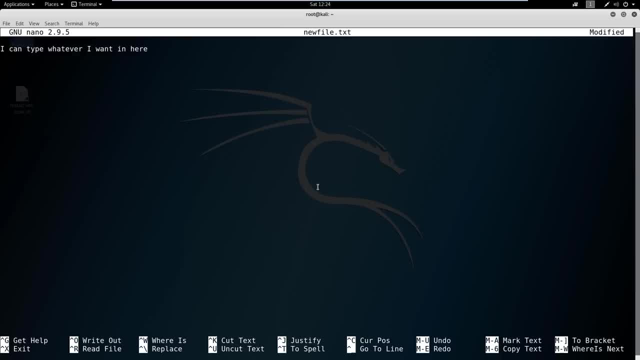 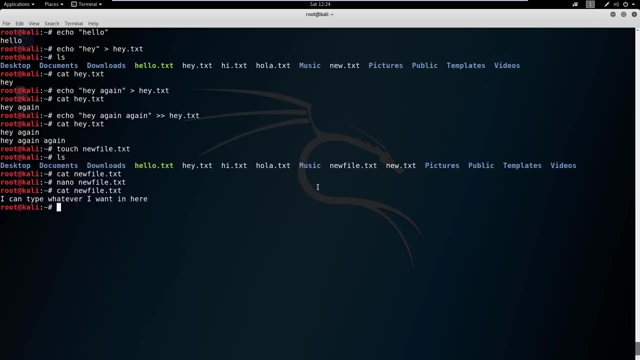 edit shellcode as we get into a little bit exploit development. so I'm gonna hit control X, I'm gonna hit Y for saving and then we'll save it to new file. that text, if we cat this now, it says: hey, I could type whatever I want in here. so that's one way of editing it. 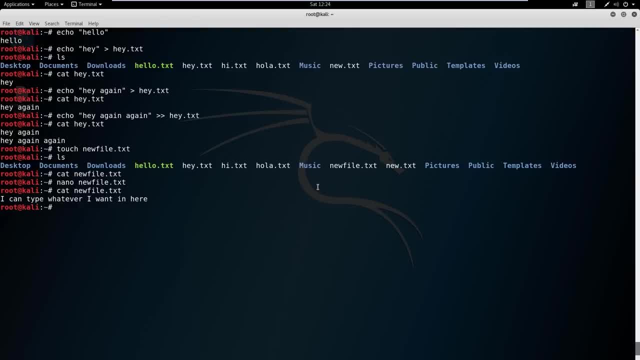 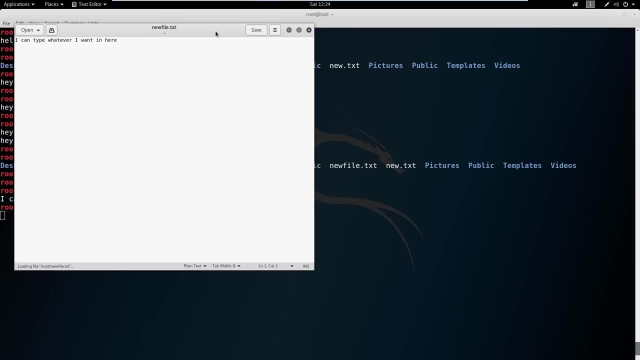 another way of editing. it is using a graphical interface. so we can use G edit and say new file. and if you don't like using a terminal, you're more than welcome to use G edit here. just type in new line here and save it. and I like using G edit. it's a lot cleaner because I can, you know, highlight and 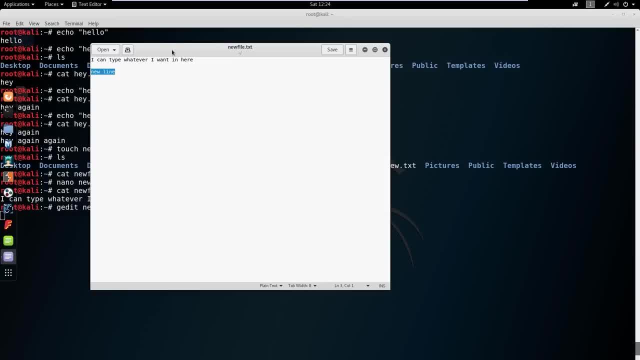 delete. I don't have to use my keyboard and navigate around like I do in the terminal. so if you have the option to use G, edit for sure. but sometimes you're going to be on another machine that's not your own or is headless and doesn't. 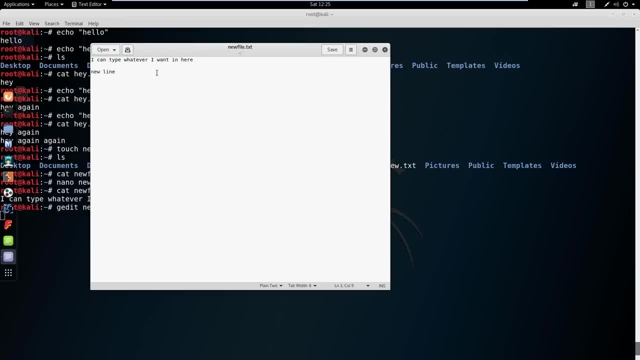 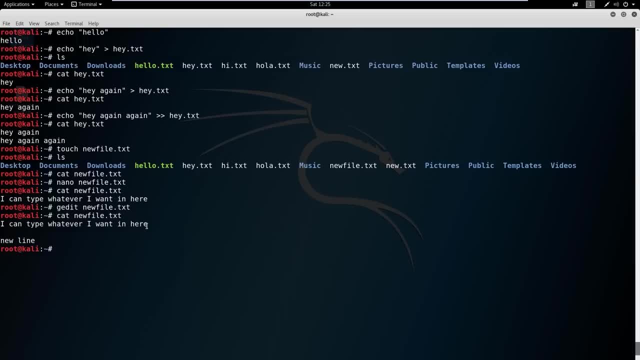 have a GUI that you're going to have to use nano, so get comfortable using both. so we save this. let's go ahead and cat it out and see what happens. ok, you can see that the new line is in there. so really, that's the overall overview that I wanted to cover. so just know that you can create files pretty. 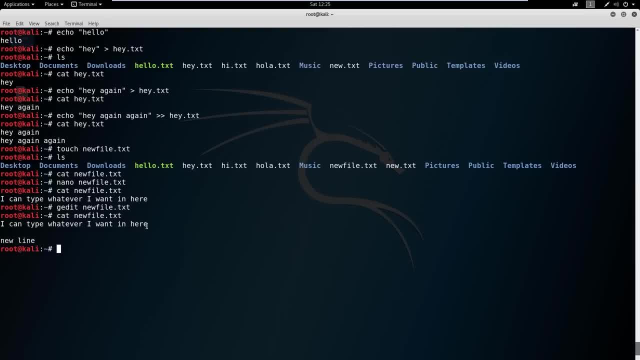 much using echo touch and actually you can create files using nano as well. if you say nano, this is new dot text, I'll just say hello, ctrl X, save it. you, LS. you can see this is new dot Texas right here, so you can use all of these tools in. 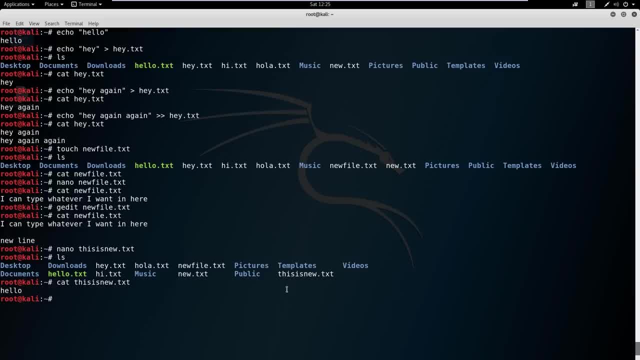 different ways to create a new file. so I'm going to go ahead and create a new file here. so I'm going to go ahead and create a new file here so you can see files. that's completely up to you how you want to do it. personally, what I'm 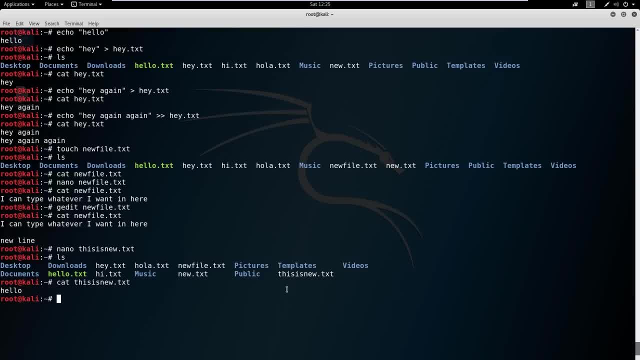 creating a file. I use nano and I just create a new shell script, Python script text document. that way you could also do it using G edit as well. so just know that we're going to be using these a lot and try to get comfortable with these, and from here we're going to be moving into controlling Cali services, so we're 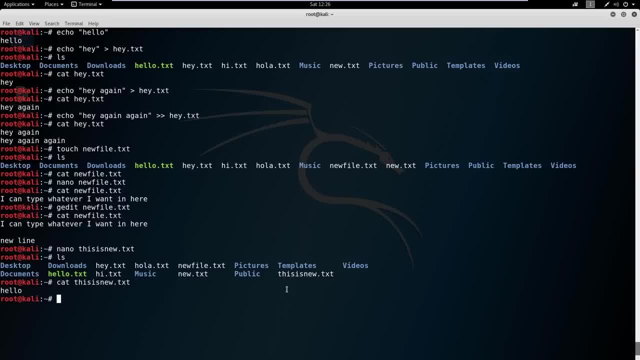 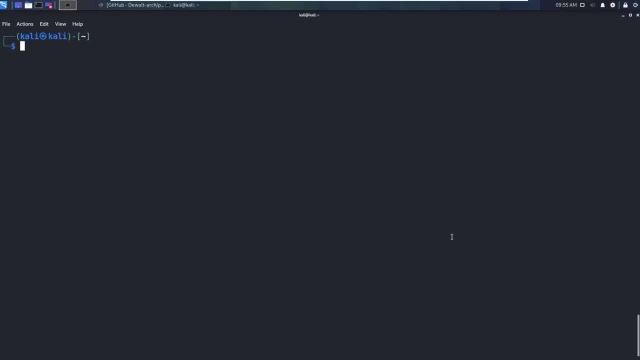 just gonna briefly talk about what services you need running on boot and how to do that Last video in the section, and this is going to be one of my favorites. So what we're going to be talking about is scripting with bash. I'm going to show you some cool tricks that we can do to kind of narrow down some of the 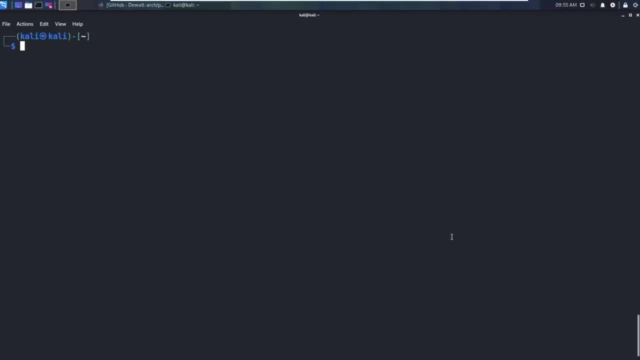 results that we get, And then I'm going to show you how you can automate some of that process and we'll take that and even write out some for loops and one line loops, which this might not make any sense right now, And that's absolutely okay. 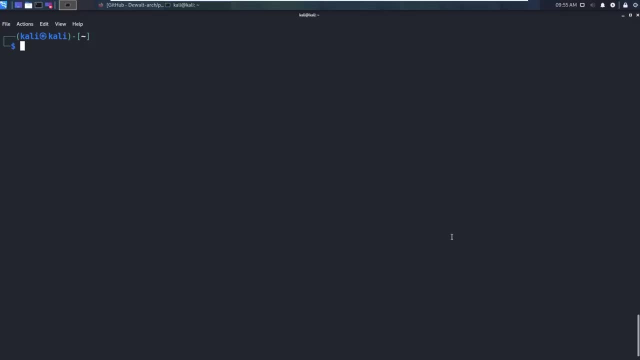 But by the time the video is done- hopefully it does. So the first thing I want to show you is: I want to show you how we're going to write a ping sweep. So we're going to write a ping sweeper. Basically, we're going to go out and say: I want to ping a device. 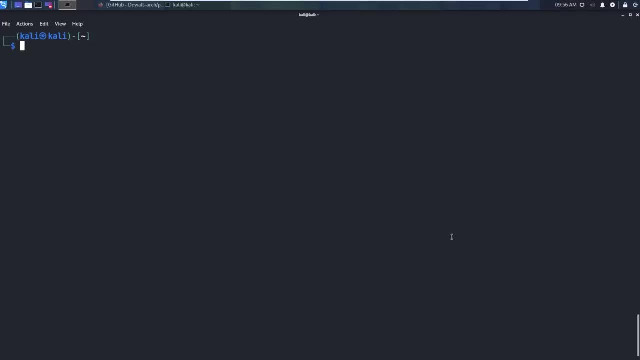 If that device is alive, go ahead and show me that result, And we're going to sweep an entire network. So what we're going to do first is we're going to identify a device that's alive, so we can test this out and then build upon that. 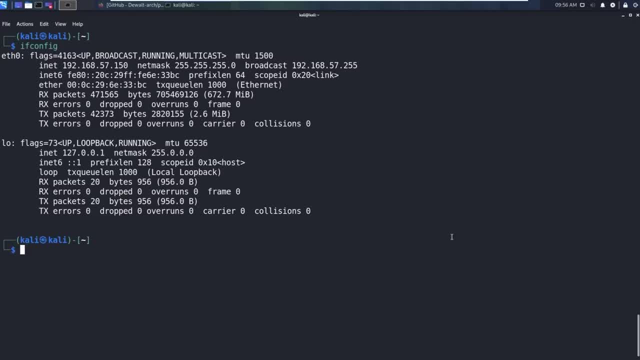 So you can go ahead and type in ifconfig And then just hit enter. Now my Ethernet here is on a NATed network, So I'm running through a different IP address subnet here, So this one is 192.168.57.150.. 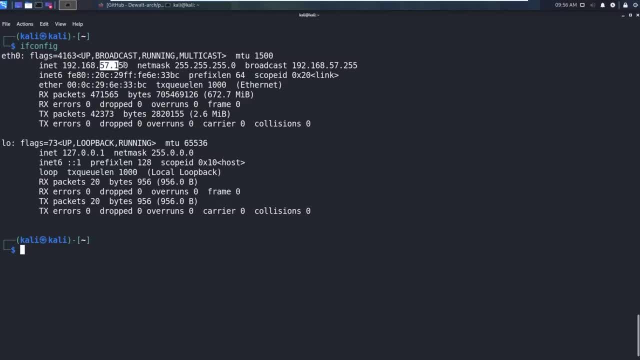 My actual IP address is on a .4.x here, So I'm going to, for this example, I'm going to be pinging 192.168.4.29,, however, and you can see I'm not going to be pinging that. we're getting back. 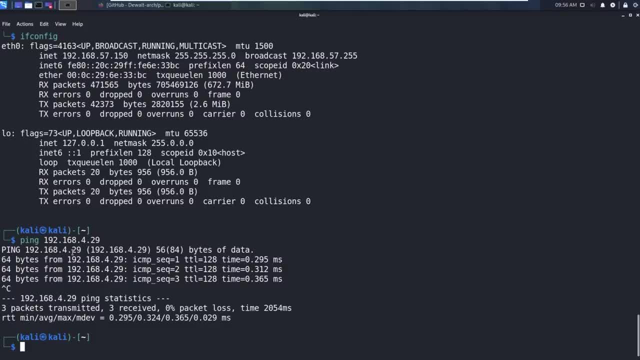 However, if you are unsure of a IP address in your house that is active or your subnet in your house, that's okay. You can just run 57.1 for this example. You might not get a lot of return results, However. you might only get one or two when we do this sweep. 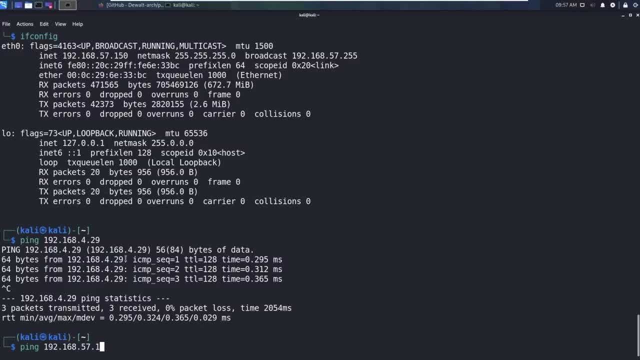 So I advise you to figure out what your IP address is. That's a good challenge anyway, And if you are familiar with networking- which you should be at this point- then you should be able to determine the IP address of your home network. 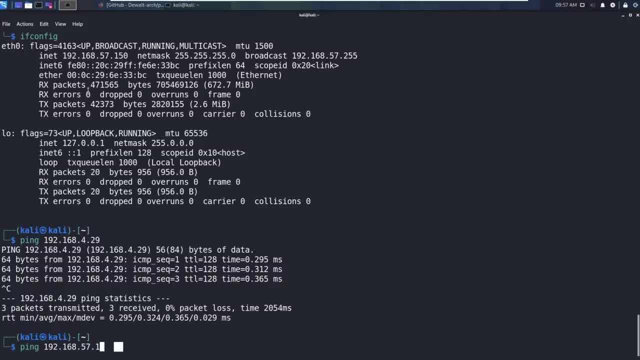 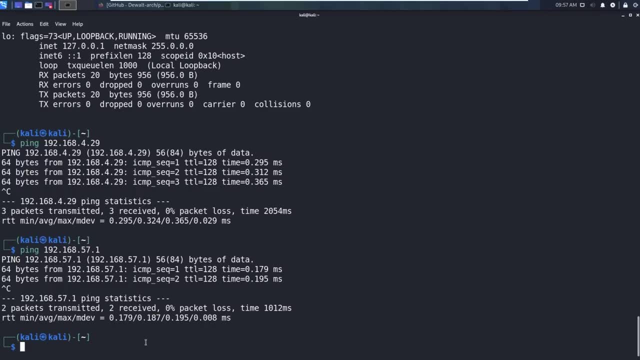 But if you do not do that, then you can use 57.1 or whatever your IP address is here on this third octet. So that will also work, if you see that. All right, so I'm going to clear this. Now, what are we noticing when we're pinging? 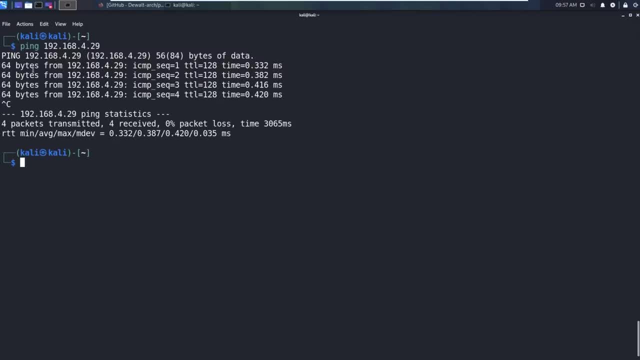 We're pinging this address and we're getting some data back. Now, if we ping an active address, you can see that we get okay, 64 bytes from 192.168.4.29.. It's saying it's active. 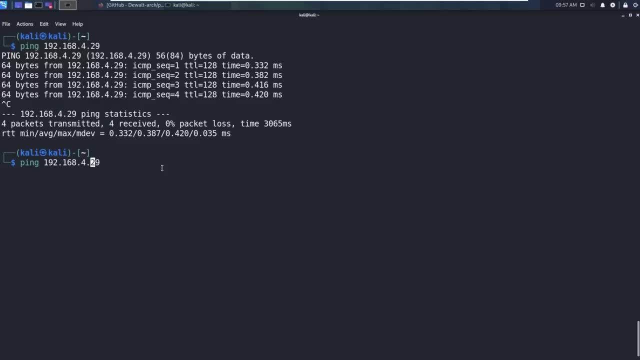 We're getting details back. If we were to ping something, Let me do that. Let's do like 41, where we just don't get any data back. Okay, And let's try this one more time. Let's try this a different way. 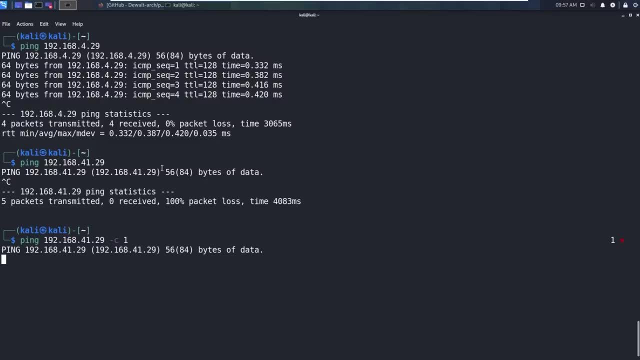 Let's do like a count of one, dash C of one. We'll do a count of one. It's going to try to send one packet over and see if it works. Nothing's happening right. It's trying to transmit that packet. 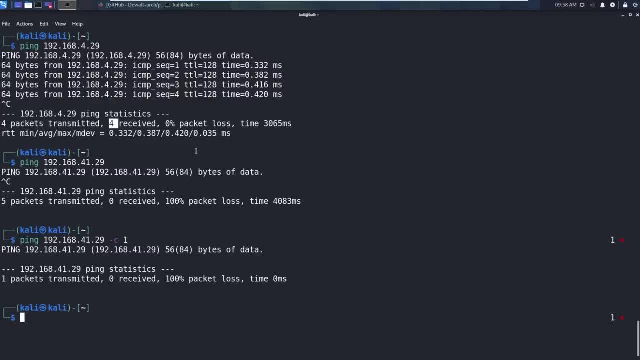 You could see that it's getting zero received here, where here is getting four received. No data is coming back. It's just not doing anything for us. So the thing that we can identify here is: what's the big difference? If we look at line one and two versus line one and two, what are we seeing when we get? 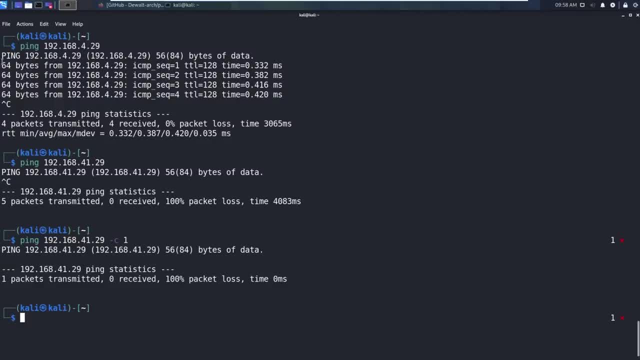 data back. Well, the big difference here is we're well two of them. I guess we see that we get this response right. That's big difference. And then down here it'll say: Hey, we received some packets, if it's not zero. 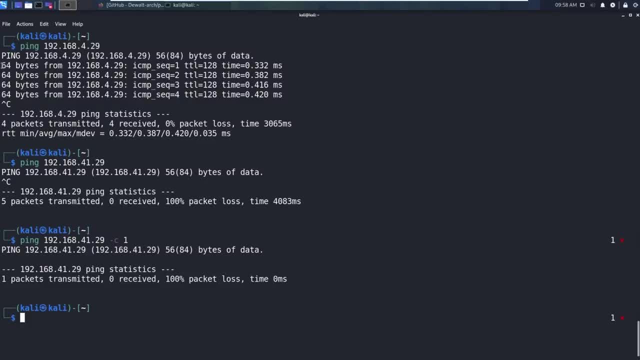 Now, the easy way to do this is to look at a line that says Hey, we received data, which is this line here. Okay, Now, what I want to do is: I want to narrow this down just a little bit. What we're going to say is: we're just going to do a ping of one time. 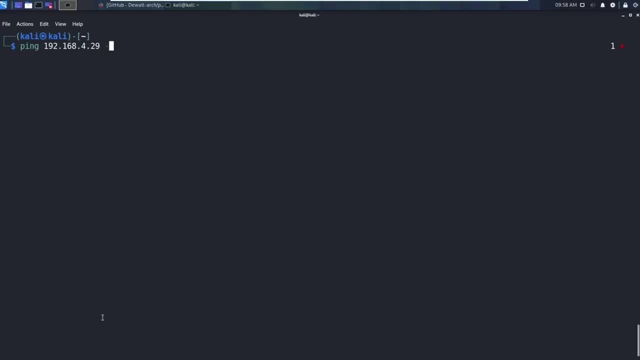 So I'm going to clear this, I'm going to bring it back to this like this: I'm going to do a count of one and that should just ping once, And that's perfect. We don't need to ping endlessly, We just want to make sure we can ping once, and then we're done. 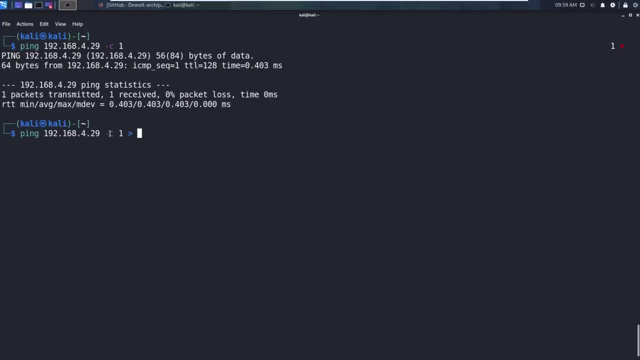 Okay, And then from here I'm going to put this into a text file. I'm just going to call this iptxt, just like that. So when I cat out iptxt now, you can see that I have this file. It's stored. 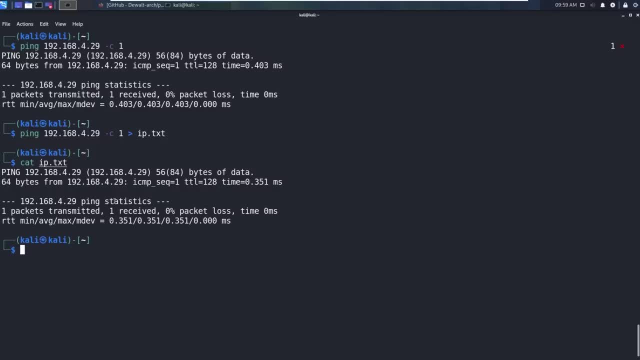 I'm going to run the command again. We're good to go. So what we're going to do now is we can take this and then we can start gathering data based off of what we see here. So what I want to do is I want to just extract this one line here, the 64 bytes from 192.168.4.29. 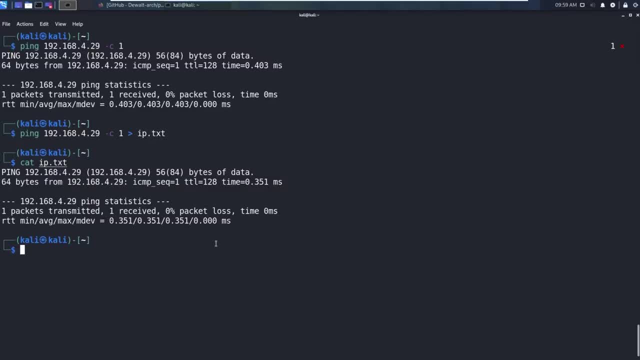 And the best way to do that is with a command called grep. So grep is going to look for a specific term or phrase, and we can do that, and it's going to pull down any line that has that term or phrase. So if I say grep here and then I just put in quotation 64 bytes like this: 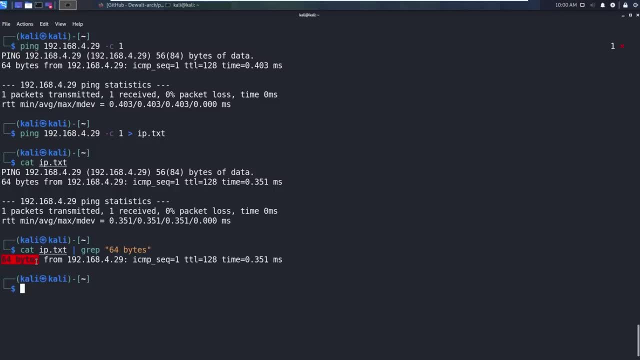 Now, when I cat out this, all I'm pulling down is this line, and it's even highlighting it for us. It's saying: here's the line that we see 64 bytes from 192.168.4.29.. Okay, So we've extracted just the one line. and why am I extracting this line? 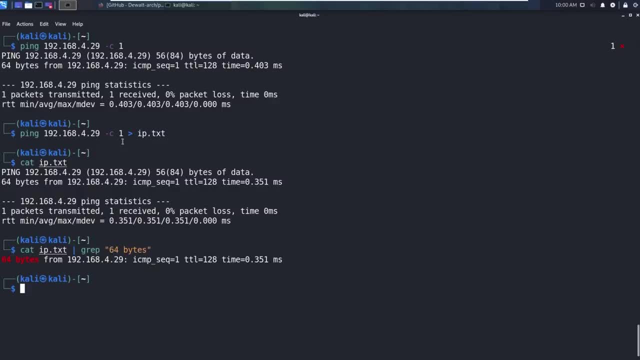 Well, for building out a ping sweeper, what I want to do is I want to sweep every single IP within a line Specific subnet. So say this: .4, right, I want to ping 4.1.2.3 all the way through 254, 255.. 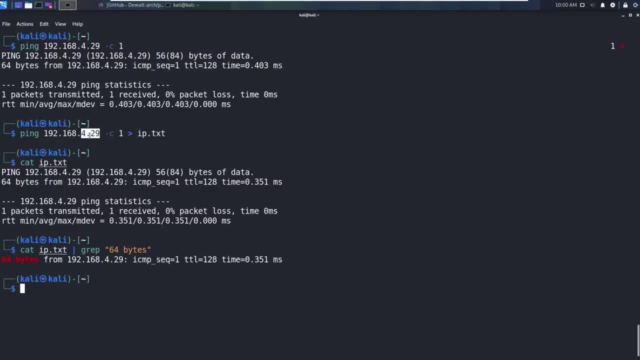 I want to see if I can get through all the IP addresses in a subnet. So what we're going to do is we're going to ping every single one of them and say: hey you up, Are you there? And we're going to do it with a count of one and we're going to say: are you there? 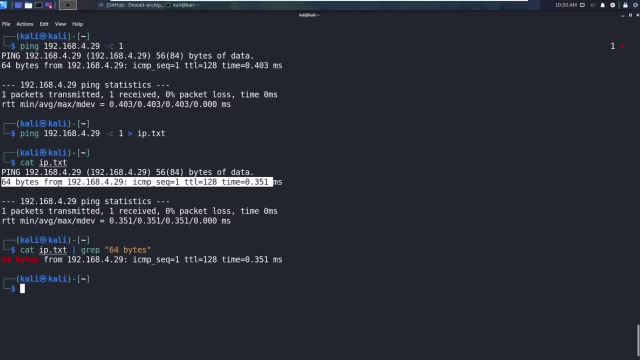 Okay, And if they're there, they're going to say: yeah, I'm here, 64 bytes- Here's my response. And it's going to say 64 bytes from 192.168.4.29.. Here's my response. 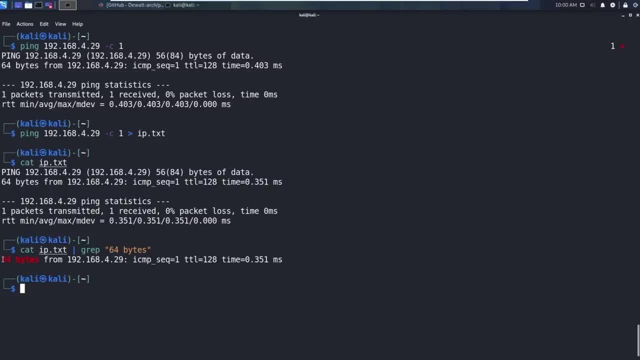 Over here. they're going to say, yeah, we're here, 4.4.2.4.4.2.. They're going to say, hey, you up, We want to extract this from this IP address. So we want to extract the IP address. 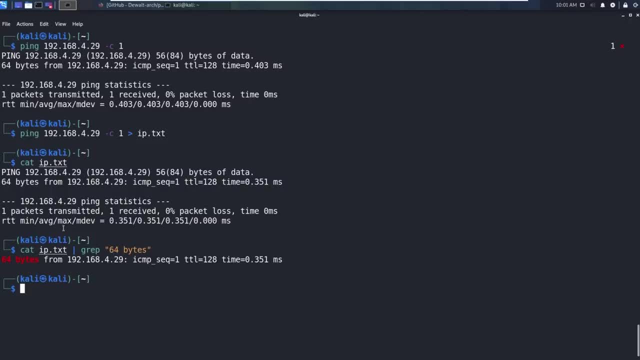 Is this a? yeah, we're alive. That's basically our goal here. So when we run this on a bigger scale- which is what we're going to do- we're going to need to get out this information and extract this information to where we only just get. 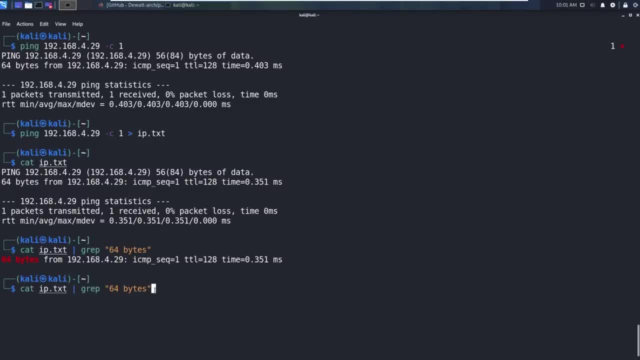 the IP address back, Okay, So what we're going to do now is we're going to start narrowing down and grabbing this IP address, And then I'm going to show you how we're going to take this all in one instance and run it. 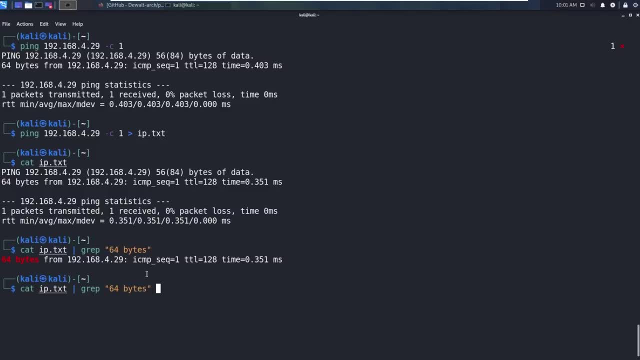 and then extract IP addresses. So from here what I want to do is I want to do another command. So every time we pipe, we're saying, hey, run this command, then with that command, run this command, then also run this command too. 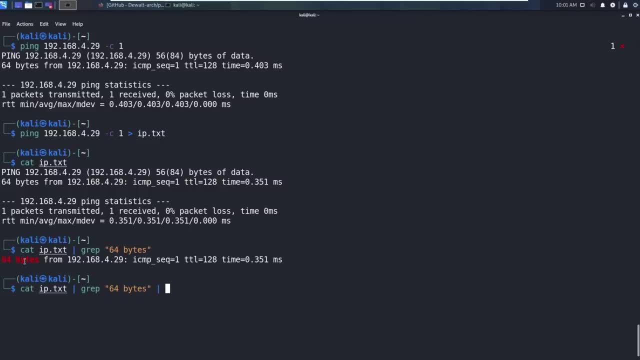 So we're going to keep running this command on top of this to narrow things down. So here's what we're doing here: We're going to run a command called cut And with cut we're going to say: I want to cut something out of this. 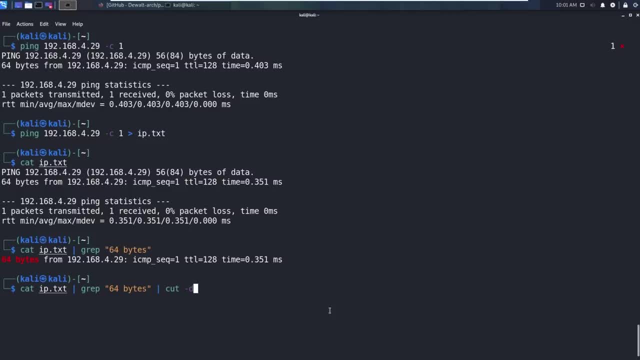 We need to provide it what is called a delimiter. So we do a dash D like this, And the delimiter I'm going to use is a space, And then I'm going to say dash F for field, And then I'm going to say four: 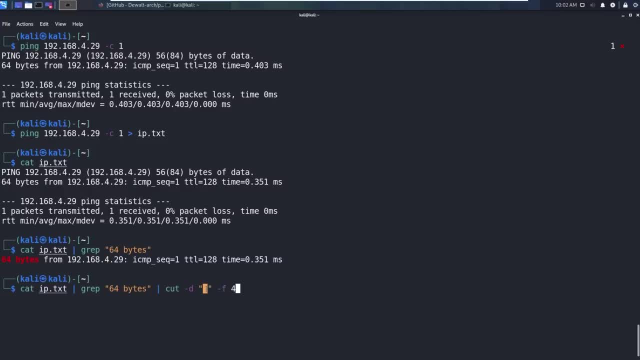 Okay, What is this doing? Well, it's saying: hey, I want to cut this line that you're getting back on a space. So the delimiter is a space. So here's a space, Here's a space, Here's a space. 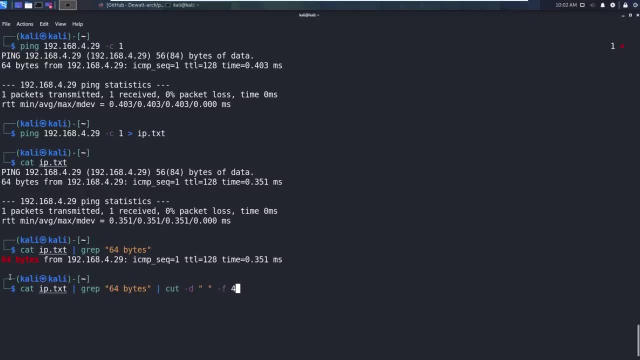 And it says: I want to count up to four to grab that data. So one, two, three, four, Right here. So if we say four here like this, we hit enter, We're grabbing that specific IP address because we're doing it by spaces. 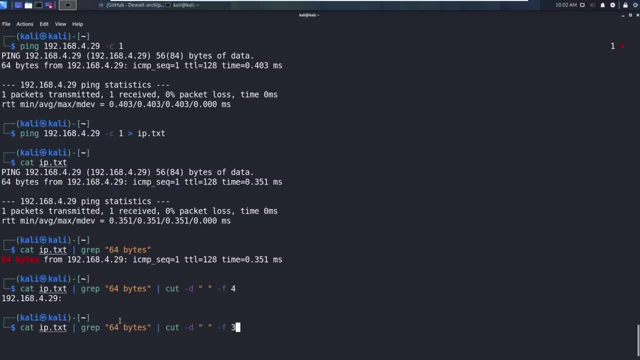 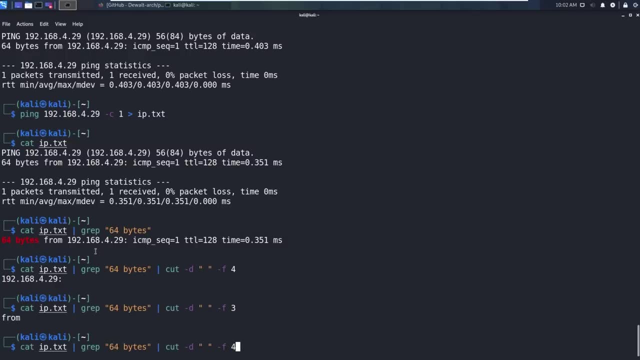 If we did it on three, what do you think we're going to grab? We're going to grab the word from, so you can see: here's from. So what I want to do is grab the IP. So we're going to use this cut just like this, use our delimiter and then get to the correct. 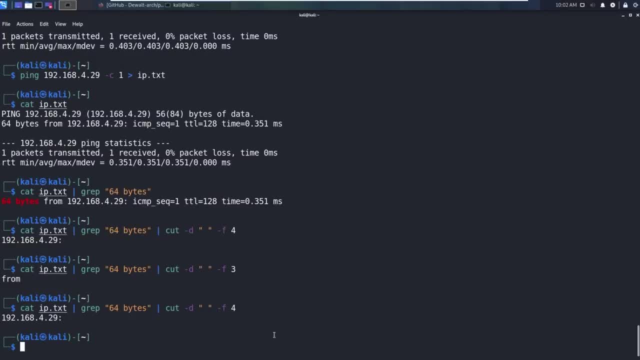 field position that we want to grab the IP address. All right, So we've got the IP address. Now, there's only one thing wrong here With this IP address is that there is a little colon on the end of it. We just want this without a colon at all. 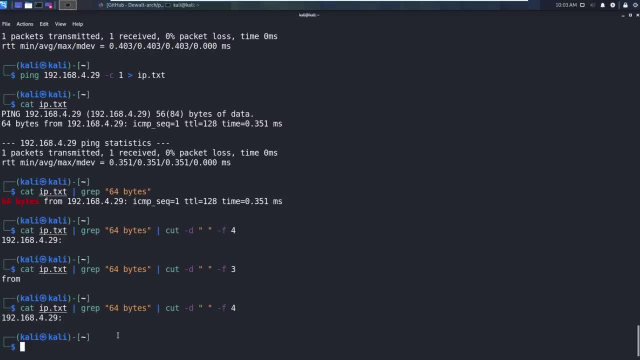 We want it just like this. Now, there's a couple of ways we can do this. We could use something called said said. it's a little bit complicated and a little bit advanced, I would say, for where we're at right now, So I'd rather teach you an easier way to do this. 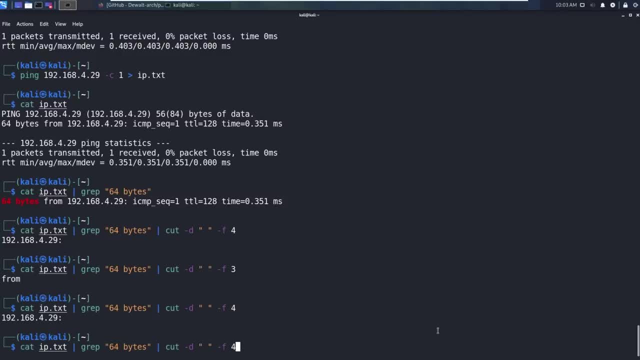 And that is called translate. So with translate, all we're going to do is we're going to do one more pipe like this And we're just going to say TR for translate, a dash D for a delimiter Again, and then we're going to say: we want to get rid of this and that's it. 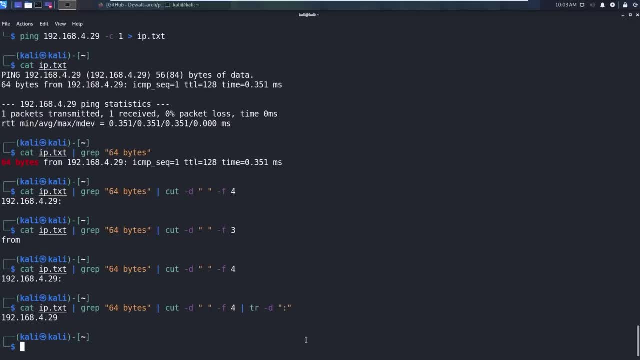 We're just getting rid of this, Okay, So we run this one more time. Now you can see that we've successfully extracted this IP address out. That's our goal. That's all we wanted to do. Now, how can we apply this to something bigger? 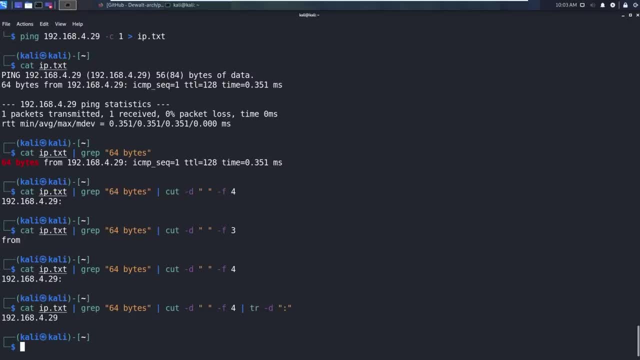 How can we make this part of a bigger script? That is the question, And we're going to do that. So what I want you to do is I just want you to copy this. Okay, Copy this entire line, And we're going to go into a mouse pad. 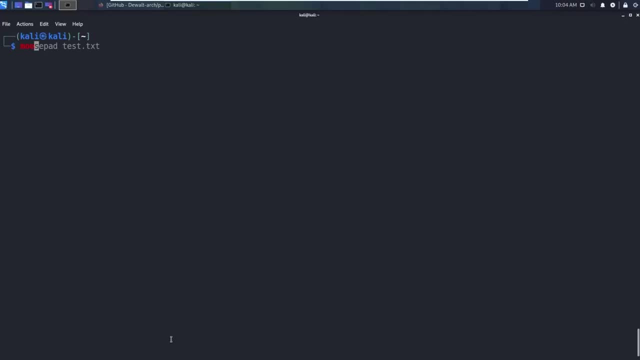 So let's copy the selection, and I'm going to clear my screen. I'm just going to say mouse pad and we're going to call this IPSuitesh. Okay, So this is going to be a bash script and I'm going to make this bigger. 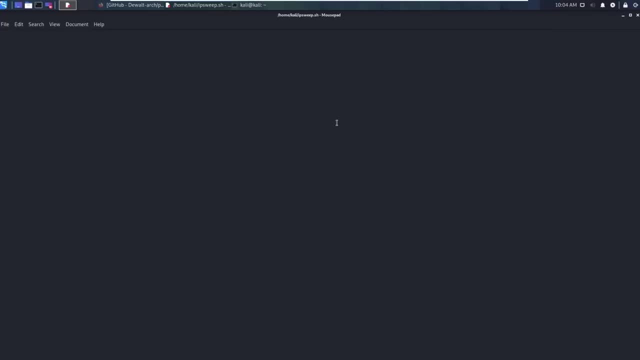 And the first thing we're going to do with our bash script is we have to declare that it's a bash script. We're going to say hash bang right here- or shebang is what we'd call this- forward slash bin, forward slash bash. 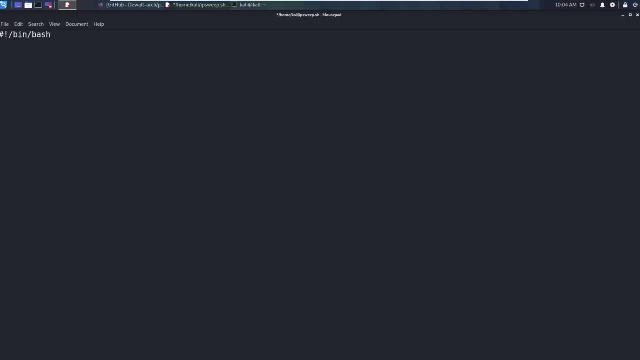 This allows the machine to know when we run this. this allows bash to know: Hey, we're calling this. Here's the location of bash. This is what we're running with the script. You're also going to see this when we use Python as well. 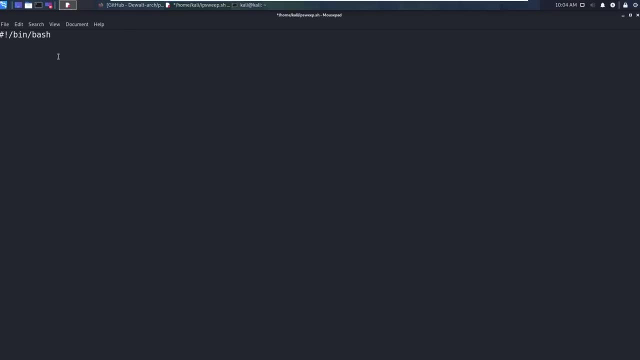 You'll see the declaration here at the top or when we're calling this out. So I'm going to go ahead and control S and save this. That'll add some nice color to this. So when we're coding this out, we get to see in color. 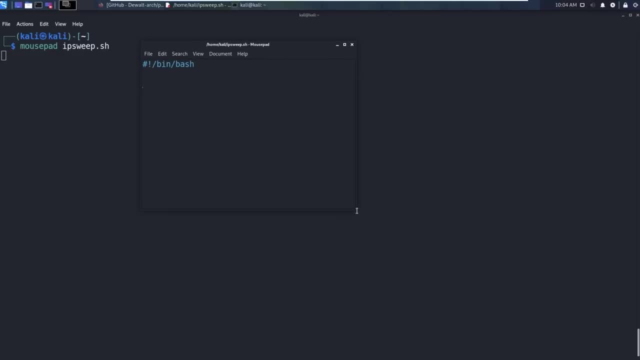 I like that a lot. I'm going to actually make this a little bit smaller and then make this like this here. Okay, Can you see the picture? Okay, So what I want to do is I want to paste in what we just wrote. 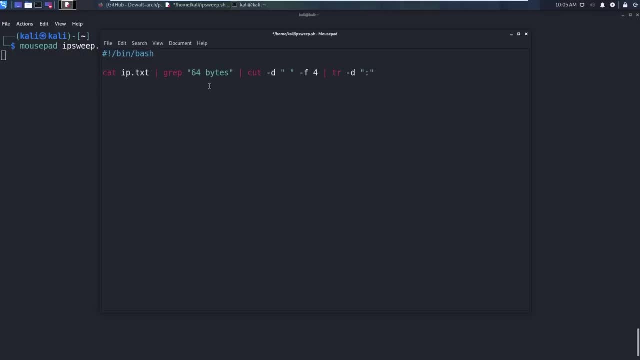 So I'm just going to control V here and paste that in, So we don't need to do a cat of an IP address here In this instance. instead, we're going to change this back. We're going to ping. Remember, we want to ping every device in the network. 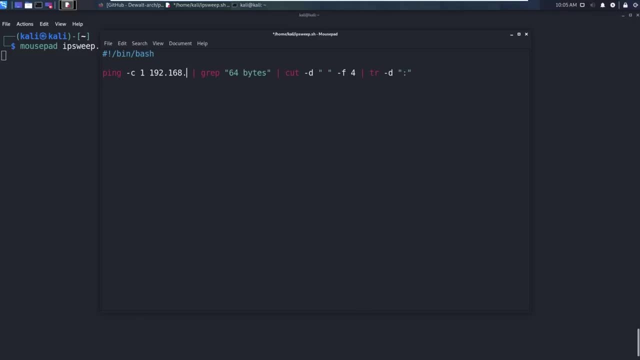 So we want to ping, say, if we're pinging 192.168.4.x, okay, We want to ping that and we can leave this like this for now. Don't worry about changing anything here. This is just going to be a placeholder. 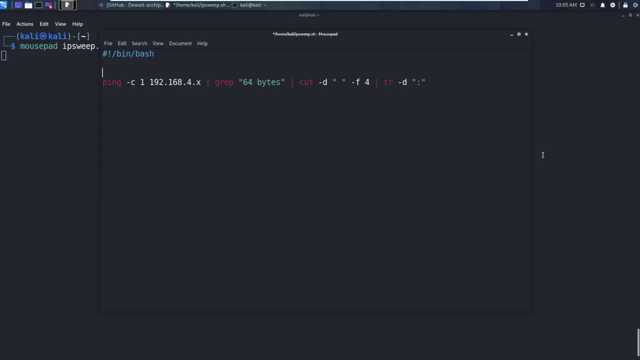 We're going to do a little bit of extra syntax here to make this work. So we're going to write what is called a for loop. So we're going to say for- and I'll explain what this does here in a second. You're also going to see this again when we get into Python and coding. 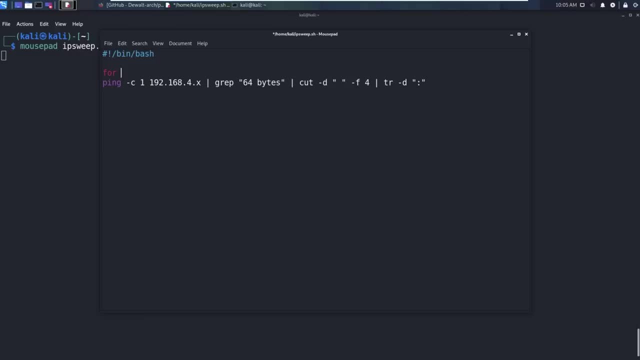 And so you'll be able to understand more and more about loops and what for loops are, while loops et cetera, They're very, very useful and very common in coding and scripting. So I'm going to say for IP in, and then I'm going to say sequence one through 254.. 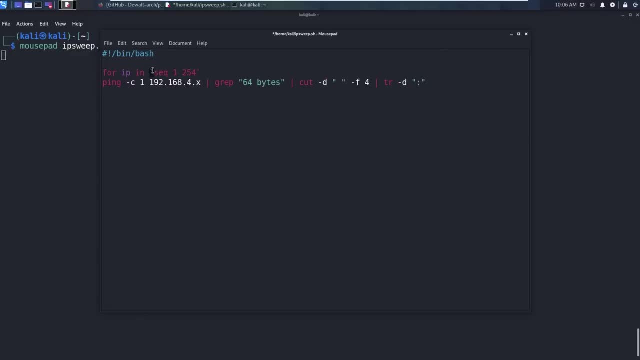 Now, very important. This character here is not an apostrophe. Okay, This is not an apostrophe. This is the little line- I don't know what it's called. It's above the tilde next to your escape button on your keyboard. 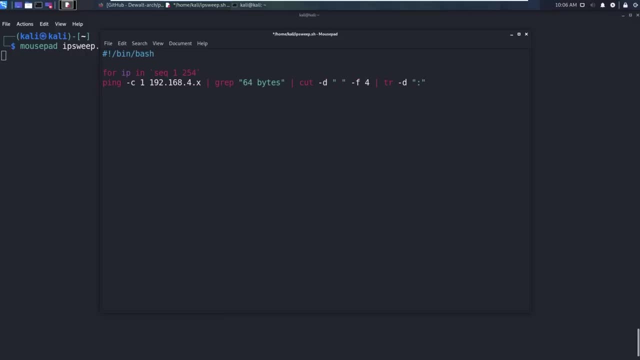 So it's this right here. Okay, It's like a backwards apostrophe almost. I'm sure there's a term for it, I just don't know it. So you come in here and you say okay For IP address, in sequence one through 254, and I'm going to explain what all this does. 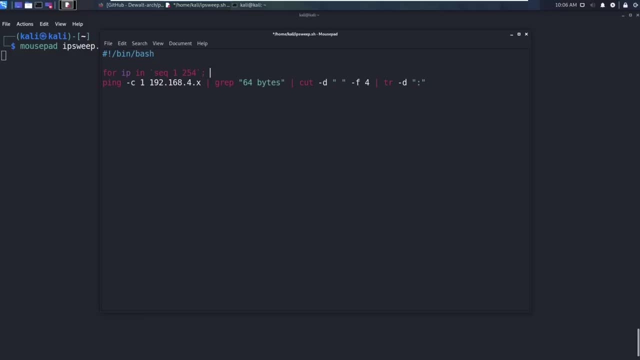 in a second. I want you just to type this out. for now, I want you to say: do all right. And then I want you to come down here and we're going to say ampersand on this line and we're going to say done. 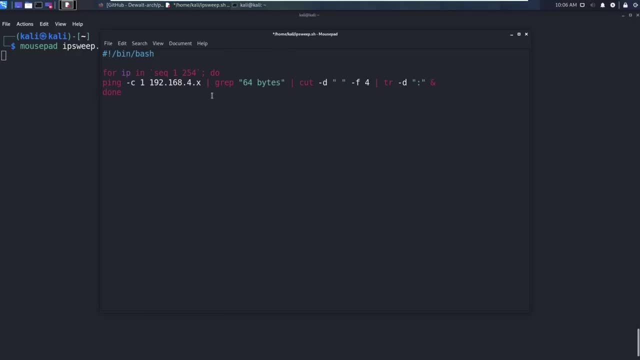 I'm gonna explain what all this means. Okay, So this is a loop that we've just created. What we're saying is for the IP address and we're just declaring this. this could be Bob, if you wanted to. I'm just making it a name or term that's easy for us to remember. 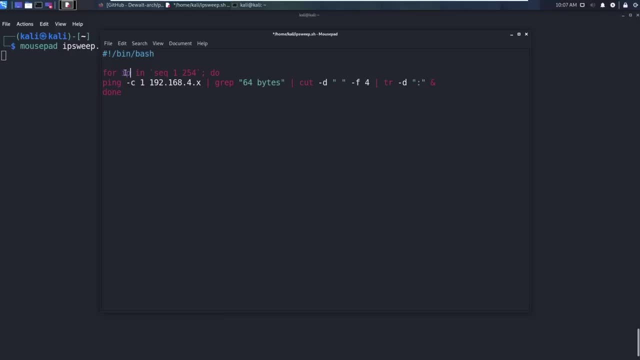 So we're going to say for IP, but if you want to call this Bob, call Bob for IP in sequence one through 254.. So what sequence is doing is it's saying: Hey, I want to count everything from one to 254.. 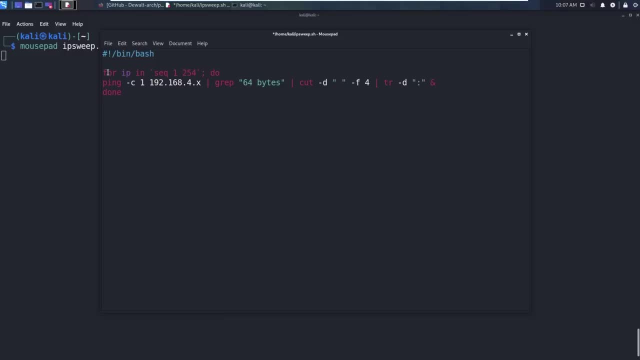 So 1,, 2,, 3,, 4,, 5,, 6,, 7,, 8,, all the way to 254.. This for loop means I'm going to do this every single time. So for IP in one for IP and two for IP and three. 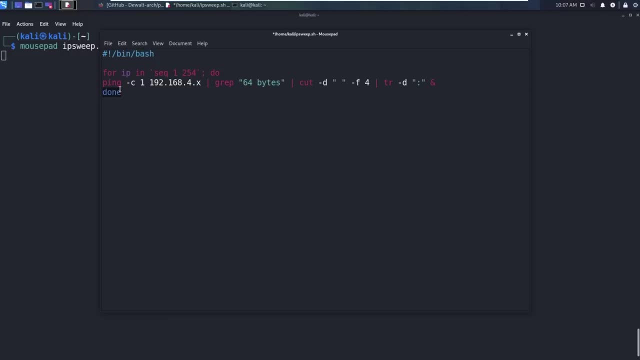 We're going to run this, We're going to run this command until we're done. So, until this sequence has run up 255 times, It's done. Okay. And now we're going to say: I want to do a count of dollar sign IP. 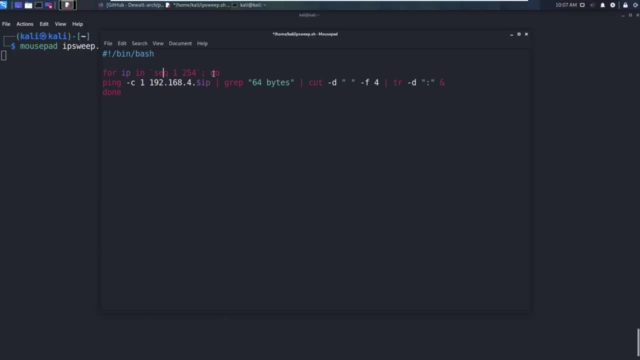 So what we're saying here is for IP, in sequence one through 254,. go ahead and do a ping dash C for a count of 1, 1, 9,, 2, 1, 6,, 8,, 4,, 254.. 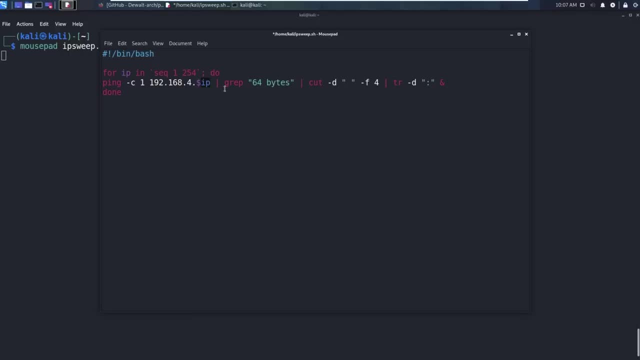 And here we're going to say dot one, dot two, dot three. Every time It's going to be over and over and over. It's going to be incrementing that number through this sequence. That's all we're doing. This is a basic loop. 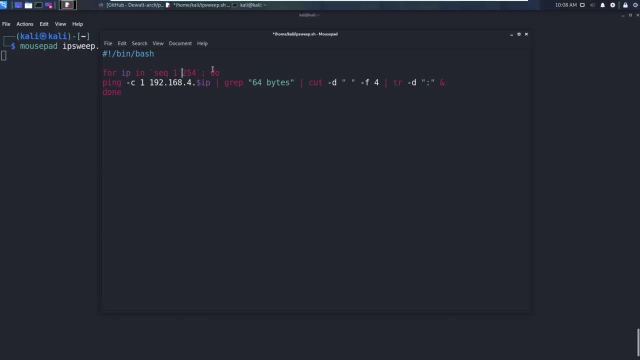 Okay, So we're going to keep going through and through and through. Now this will work. If you plugged in your hard coded IP address here, this will absolutely work. Now we can improve this just a little bit if we want to. So what's going on here is what we're going to say is, if we wanted to run this, we would. 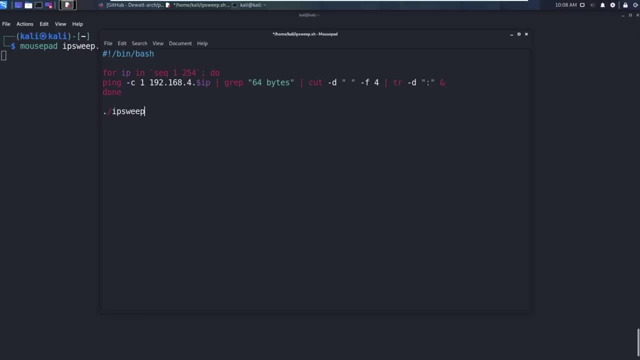 just do dot forward, slash and then IP sweep. Okay, Um, and this would work, But we can make this a little bit better from a coding perspective. We can come in here and we can give this a dollar sign one, and that means argument one. 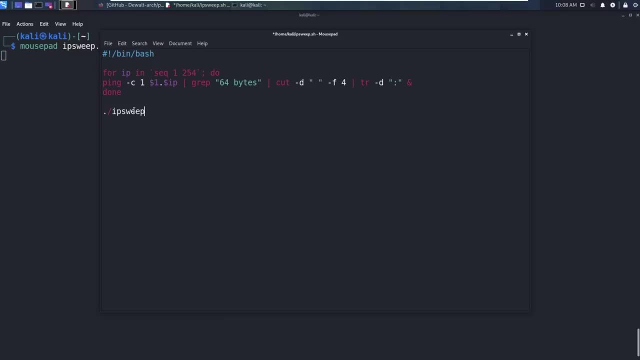 So what we're saying here is: I want to give an argument instead. So if you want to be technical, this first dot forward slash IP, sweep, dot sh, that is argument zero. So you can consider this dollar sign zero argument. one would be what you type after: 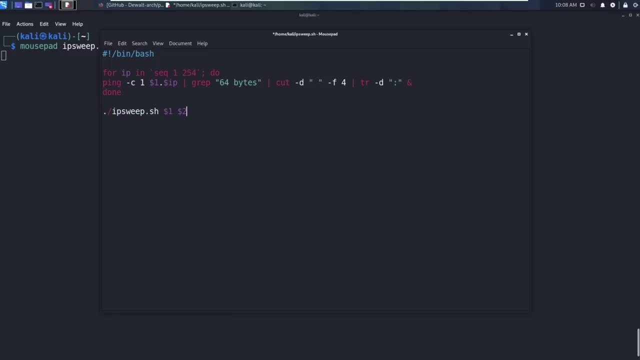 that. So this would be. So. in this case, what we can do is we could say: I want to run one nine, two, one six, eight, four, like this, And this will run the dot one, dot two, dot three after it. 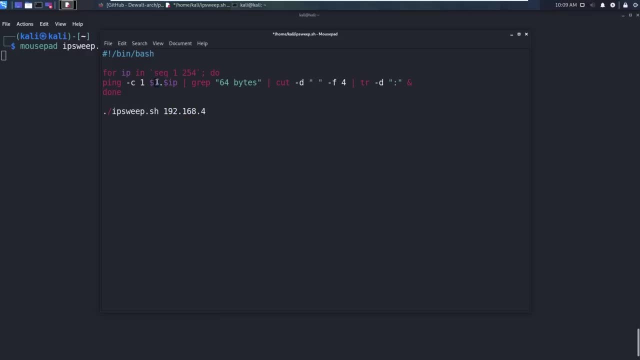 So you provide the argument, It places that here in argument one and then it does the rest for you. So this way you can specify your network And if you wanted to ping multiple networks, you don't have to come back in here and keep. 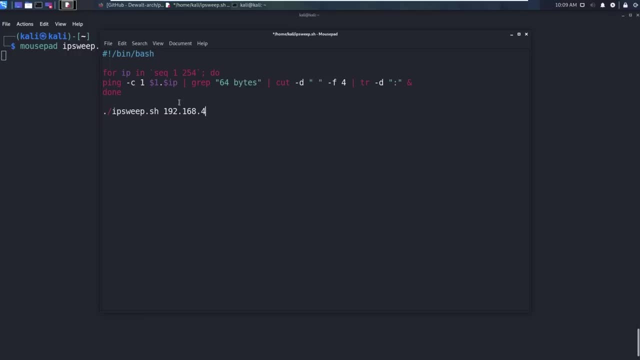 changing this. It just works So super easy. This is a great little script. You can use this for a slash 24 type subnet. Okay, Okay, So let's go ahead and try running this really quick. I'm going to just control S, save this. 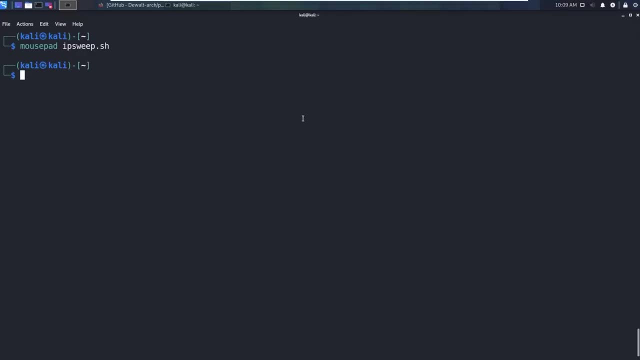 I'm going to close it. We're going to do a chmod plus X on IP sweep. If it'll allow us to, we might have to do a. okay, let's do LSLA real quick. Make sure it worked. It sure did. 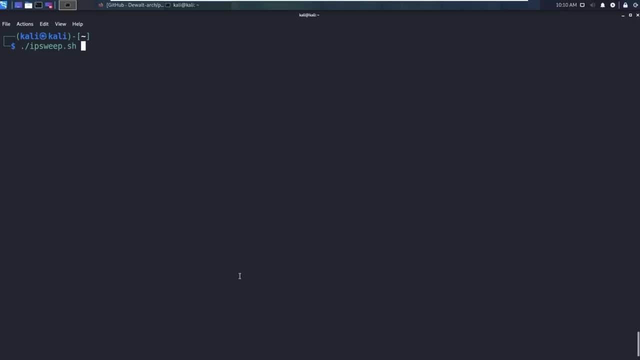 Okay. So here's what we're going to do. We're going to run the IP sweep, Okay, And we're going to say 192.168.. You just put in your IP here and I'm going to run that, All right. 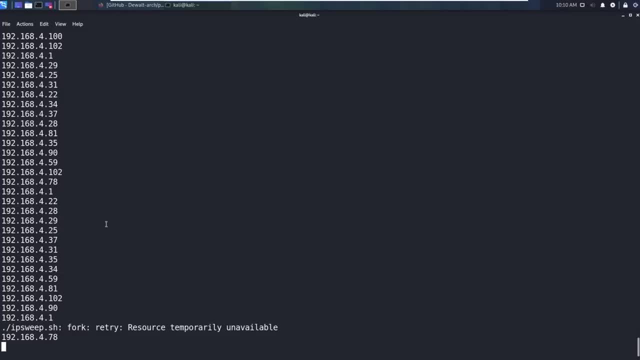 And you could see all the devices that are coming back within my network. here I'm going to go ahead and hit control C, cancel this out, And so this is grabbing all the different devices in my network. Now that's great, That works out really well. but what we can do is improve this. 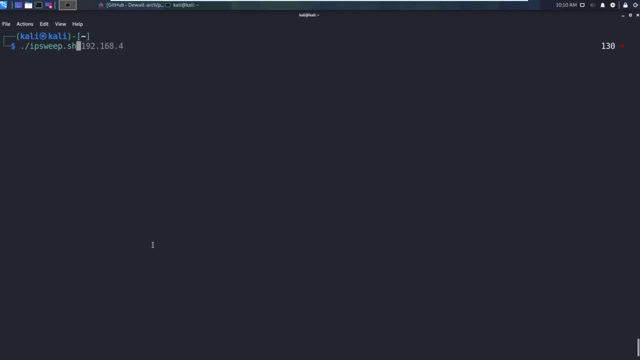 What if I typed in a? what if I didn't type anything at all? What if I just hit enter here? Now I'm just getting all kinds of pings unknown and it's going off of some of the stuff I was doing before, but it just causes all kinds of issues and errors, right? 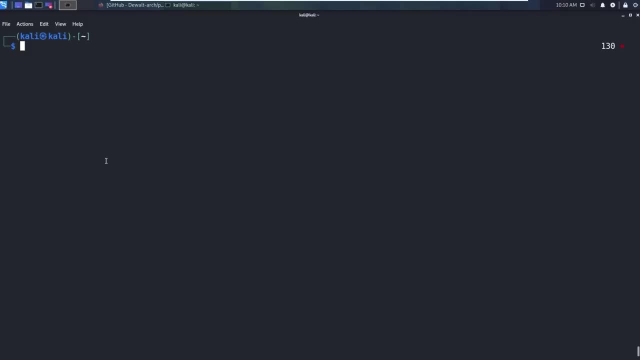 So you could see I'm trying to hit control C. it's taking its time to break. Here we get issues because we're just allowing any sort of argument here. What we need to do is we need to fix this up just a little bit. 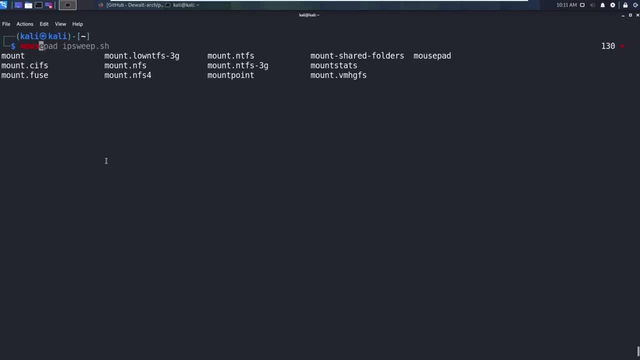 So what we can say is: we can come back in here and just go mousepad, IPSweepsh and come in here, Let's add a little bit extra. Oh, and I also left this in here: Don't leave this in here. 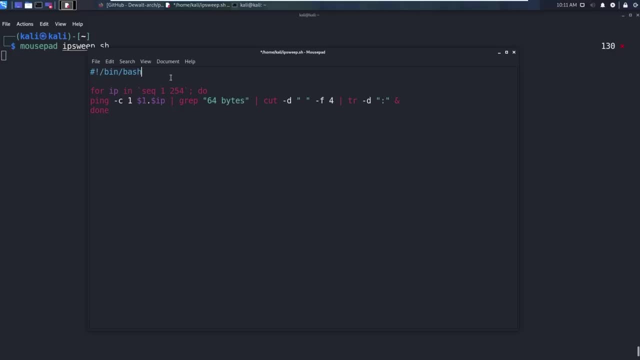 That's why that was running twice. Okay, So what we're doing here is we need to add in a statement. What we're going to do is we're going to add in a if statement. If statements are conditions, we're saying, Hey, if this condition is met, do something. 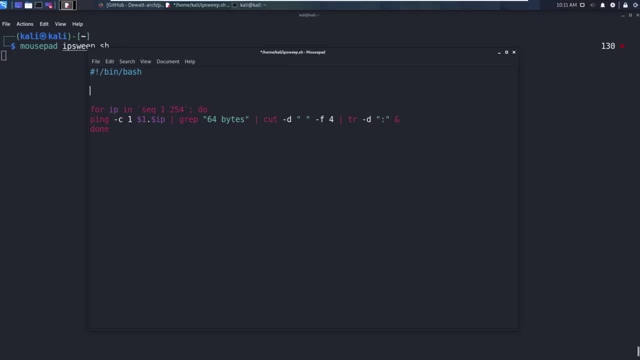 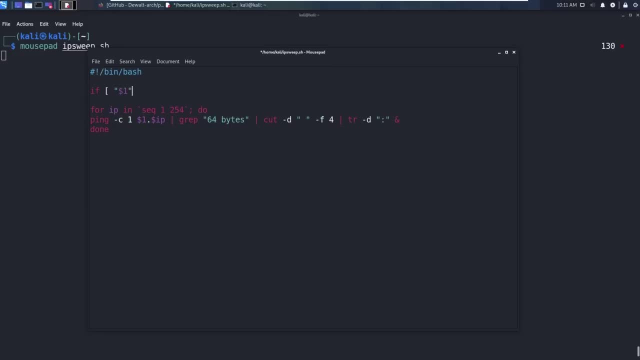 And we're going to say: if Okay, So let's just put in here: dollar sign one is equal to nothing. Then we're going to go ahead and just say then, echo, you forgot an IP address. Echo syntax, something like this: 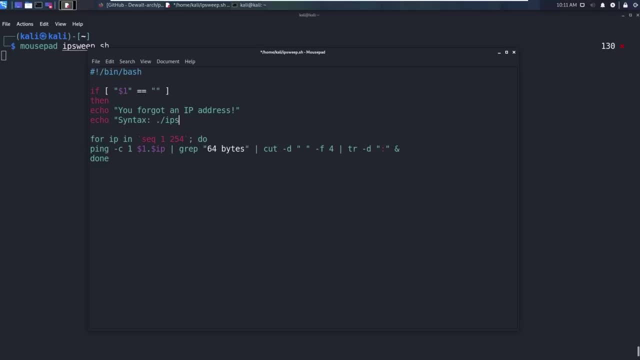 We'll just say IPSweepsh And we'll go 192.168.4, like that. Okay, okay, and then if we did do this correctly, if we do have an argument inside of argument one, then we're gonna say else, do all of this here and be done. 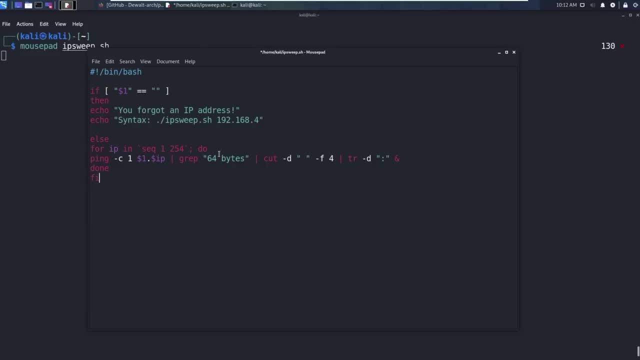 and then we're gonna end our if statement with fi. now, this script, or this resemblance of this script, is not one of my own. by the way, this is goes credit to something I've modified over time, but the original credit definitely goes to Georgia Weidman. I remember seeing this in her course a long long. 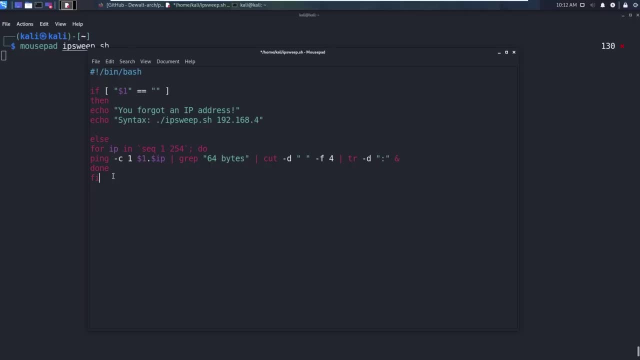 time ago when I was first getting started, and she did a great job of teaching this. this is just a modification of this script, so I just want to make sure that all credit goes to her. but looking at this, let's break this down really quick before we run this again. we've got an if statement. we 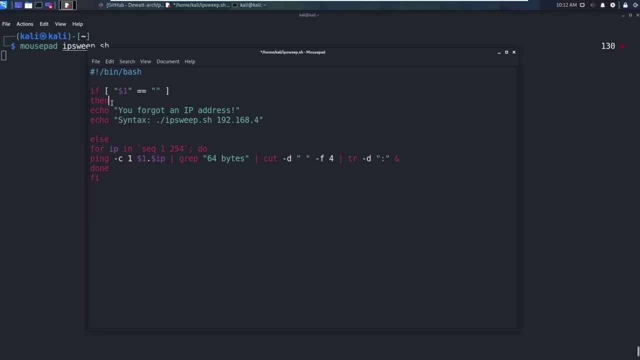 said, if argument 1 doesn't equal anything, then you're gonna echo back out and say, hey, you forgot an IP address. here's the syntax. if it does include something, then we're going to go ahead and come in here and say: let's run our for statement, our for loop, and 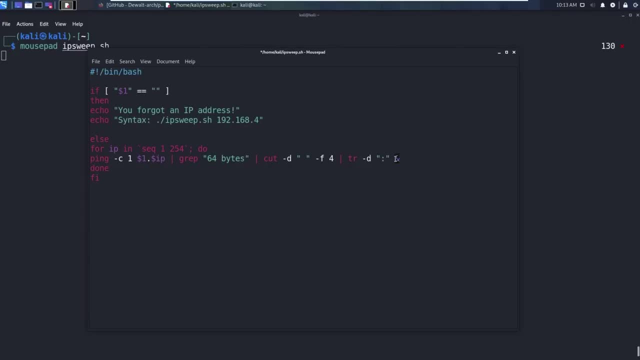 run through it and then we're going to end our if here. the only thing that i'm doing uniquely here is i'm including this ampersand, which is going to run this command multiple times at once. this is a good way to explain it. basically, we have a couple ways of doing this. we 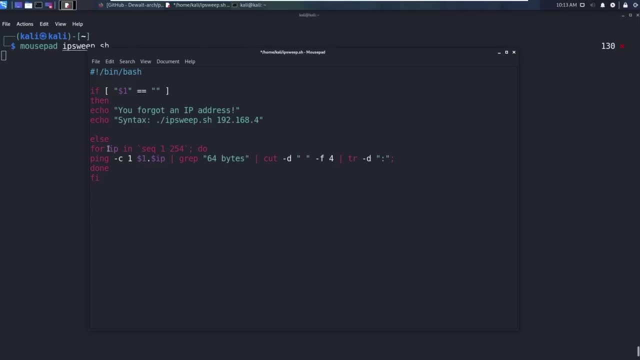 could say like this: we could put a command here and this will run one at a time. it'll say: okay, four one, four, two, four, three. this allows multiple instances of this loop to run at once and just speeds things up. i can show you the difference between that, so i'm going to go ahead and just 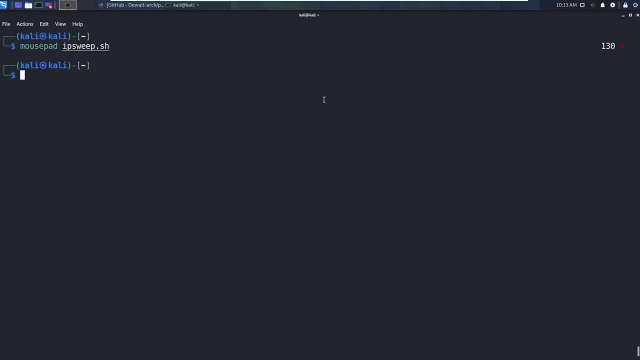 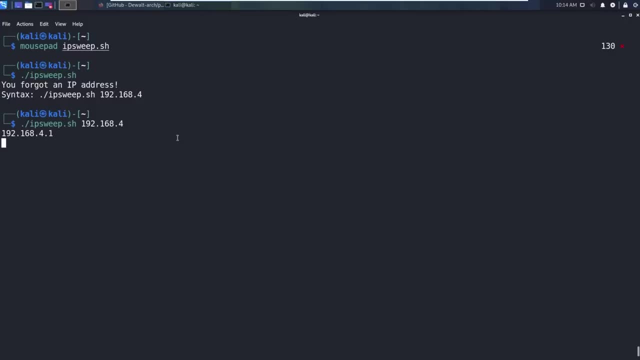 especially for the ip addresses that are going to hang, like. like, if i don't have a dot 2 or dot 3, it's going to take a while. so i'm going to ctrl c and get out of this, if it'll let me, and it looks like it's actually going to hang. so what we can do is we can come back in. i'm going 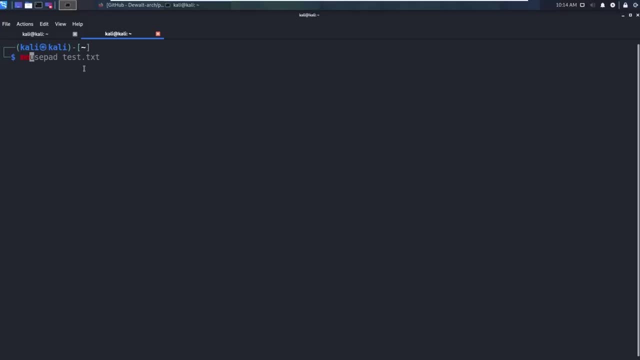 to open a new tab real quick, just while that's waiting. and i'm just going to say mousepad and we're just going to go back into ipsuitesh. it's in this folder. there we go, okay. so from here i'm going to change this back to the ampersand and i'm going to save it. i just want you to see the. 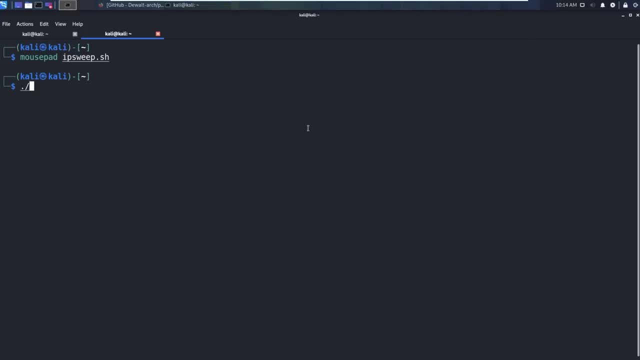 difference really quick and why i run it like this. so, ipsuitesh 192.168.4. you can see it's picking everything up really fast, all right, um, what i can do now is i can run this and then store this into like ipstxt, something like that, just like found ip addresses. okay, so now if i cat ips dot txt. 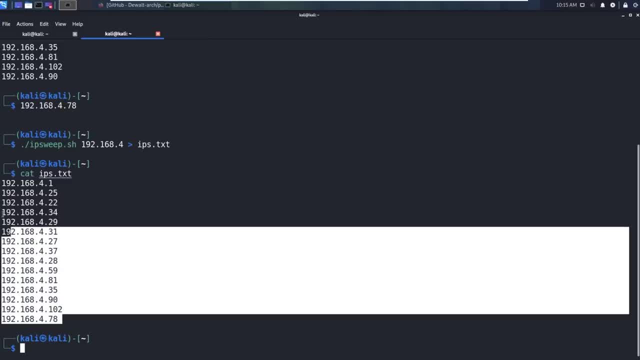 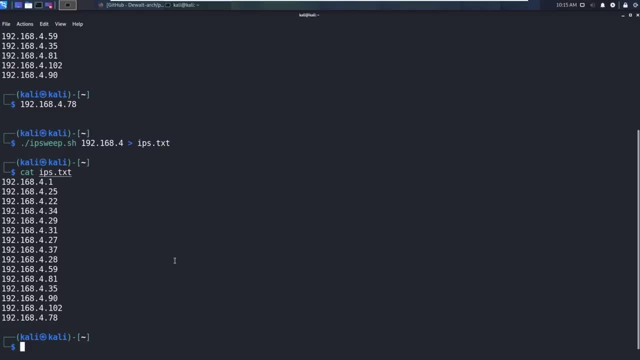 xt. i have all the ip addresses i just found- and i found them that fast- versus this, which may still be going, and it is, and i can't even kill. i'm just going to close this out, okay. so this is the big difference there, with that ampersand and the speed of what it's capable of doing. so with all that, 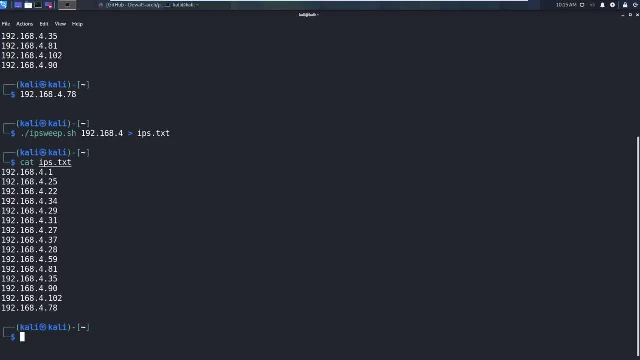 being said, we could take this and do one more thing. so i want to show you how we can utilize a one-liner. these are called one-line statements in um in bash, and we can do similar to what we just did and accomplish that in this command line. so now we have an. 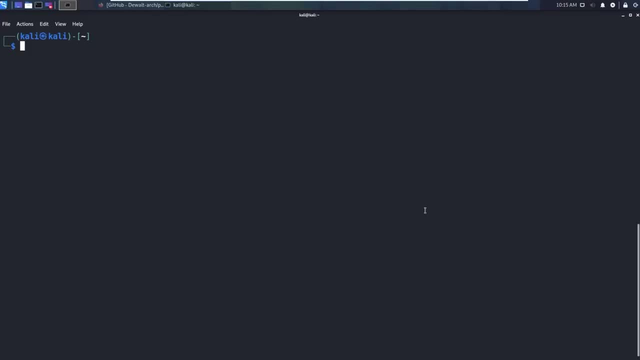 ip address. we have a list of ip addresses. let's say that we want to run and map. now we haven't gotten to mmap yet. you don't need to really know about it, just know that it is a tool that allows us to go out and do port scanning. okay, so typically we would just say something. 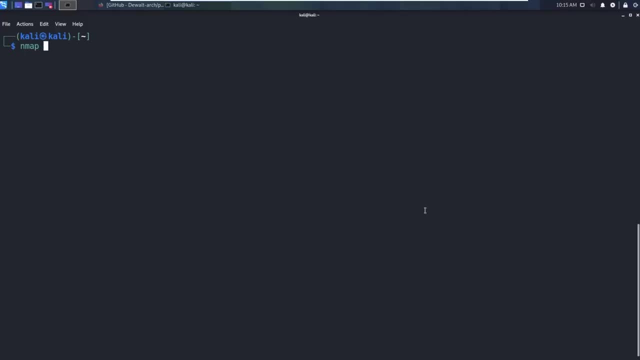 like nmap and we might do something like uh dash t4 dash a dash p dash, like this. this is just saying to run uh mmap scan. i want to look at everything and i want to scan all ports. this is just an example. you can just run mmap ip address like this, and that would be fine too, like we could. 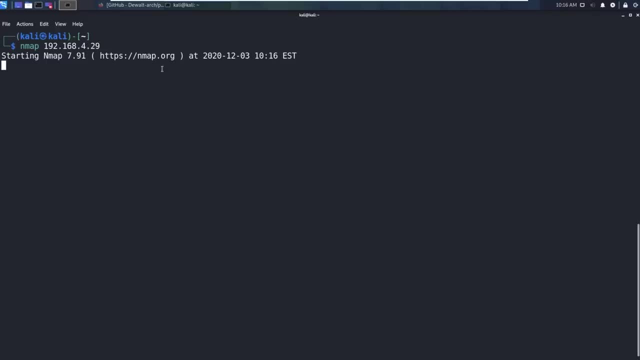 just go 192, 168, 4.29, and we'll do a quick mmap scan. okay. but what we can't do here is we can't just say: hey, i want to run. uh, well, we could. we could say: i want to run mmap for everything in. 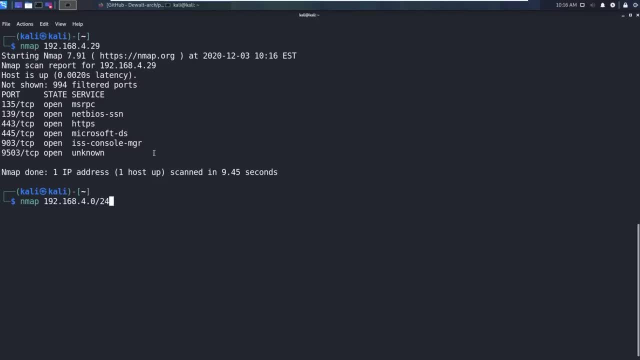 dot zero, slash 24.. the issue is it's going to take time looking and finding what ip addresses are valid here. if we have a list, we can automate this process quite a bit. we can just come in here and we can say something a little bit different. we can. 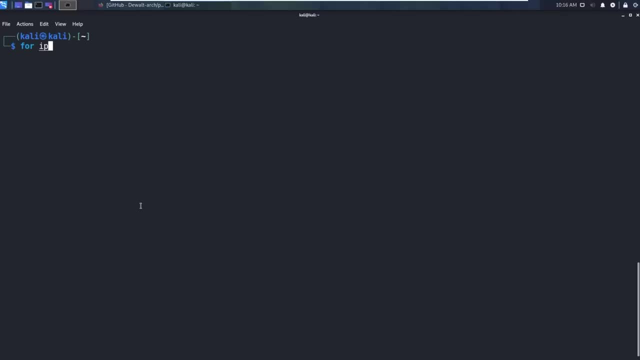 say hey for ip. we're using the same kind of syntax in dollar sign and we're going to put parentheses here. we're going to say cat, and then we're going to say ipstxt, and then we're just going to do this. we're going to say do and map. 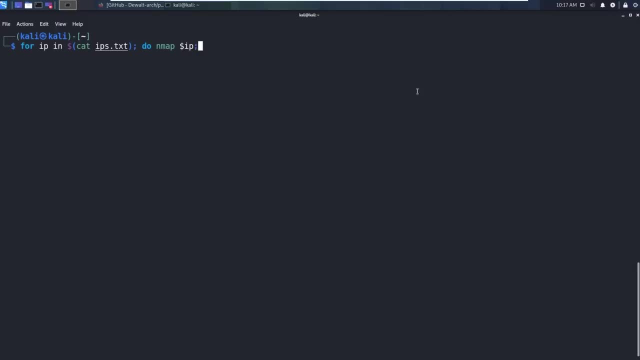 dollar sign ip, and then again we have the option of doing done, or we can do ampersand done, just like this. okay, i'm just going to do done here as an example and just show you so. this is really easy. we're saying hey for every ip address in this list and all we're doing is 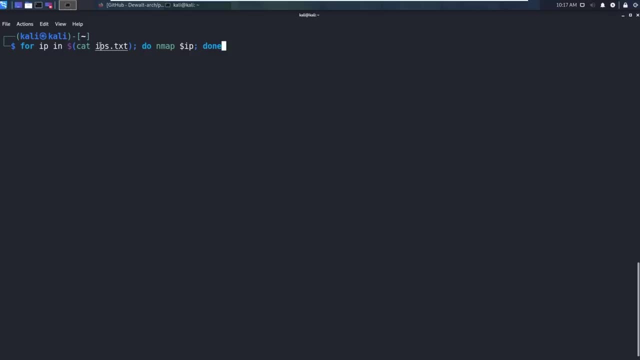 we're catting out this ip list that we just had, so it's going to take the first ip, then run the mmap scan. it's going to come back, run the next one. so until this list is completely done, it's going to run the next one and then we're going to do a simple loop. that's all. it is a simple loop. then. 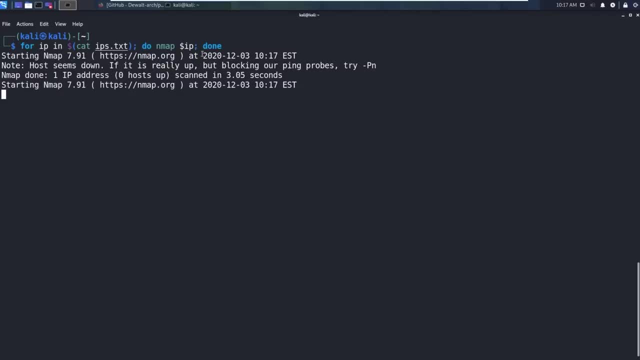 we're going to say done. it's going to take that ip address, it's going to start scanning it, it's going to go through and hopefully find information and go in a loop. so this is a quick way to automate some of this process. i actually do this with a lot of my scripts where i will do some probing. 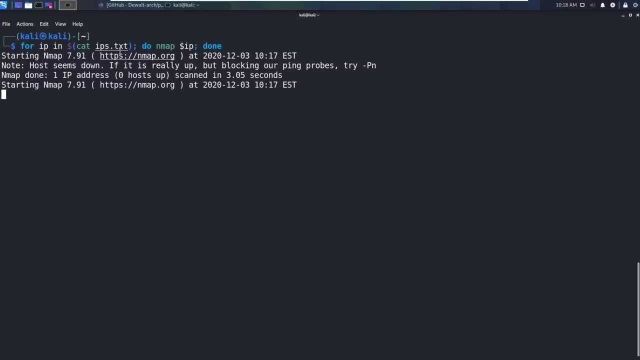 see if anything is out there that's alive, put it into an ip file- and you're going to see this later in the course- and then end map scan that. so think about this. hopefully this gets your wheels spinning and you're going to be able to do a lot of the things that you can do to really start scripting. 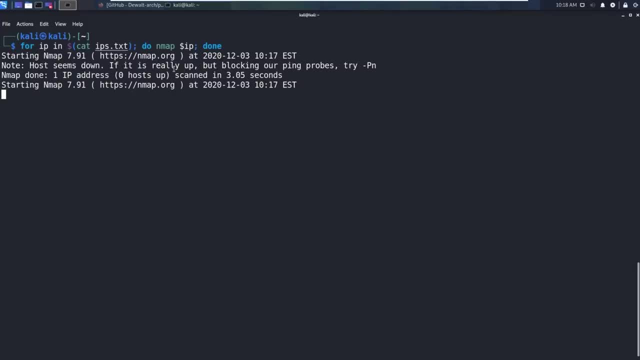 some of this stuff out, and this is going to be the first time you get your hands dirty with scripting. we're going to go on again with this and we're going to get more advanced as we go, but this should be a good introductory lesson to you on how we can build a simple tool and automate a lot of. 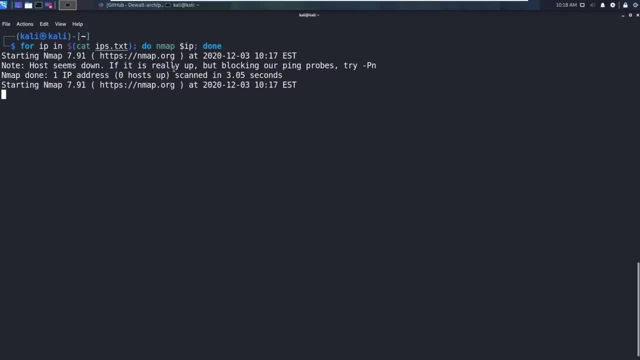 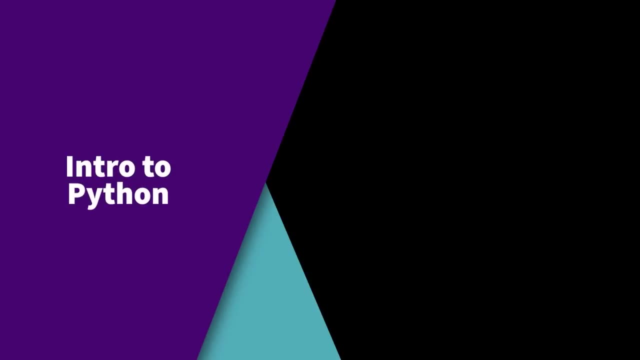 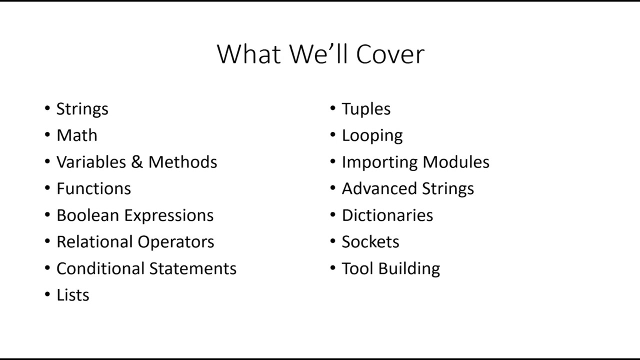 this process fairly easily with just a little bit of command line syntax. so we're going to go ahead and move on to the next section and i will see you over there. welcome to this module on python. so if you've never used python before, or even heard of python, 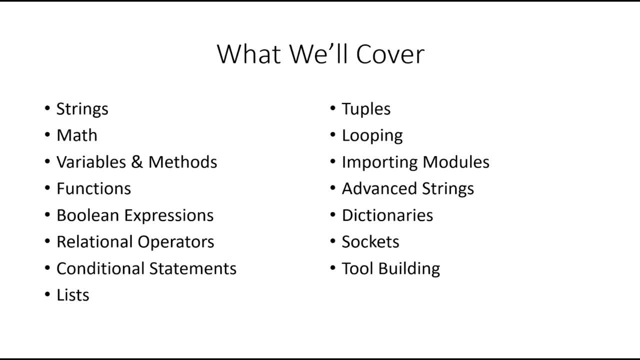 before. python is a coding and scripting language. it is commonly used in ethical hacking and it's commonly used all around the world. it is actually considered one of the best beginner languages to start with if you've never learned coding before. so that's exactly what we're going to do. we're 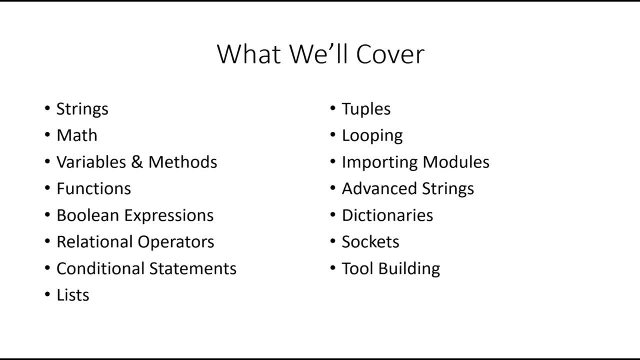 going to cover some of the basics of python, so we'll cover everything you see in this video, on this screen here: strings, math functions, we're going to get into conditional statements and looping, we'll get into some more advanced items and eventually we're going to build our own tools. 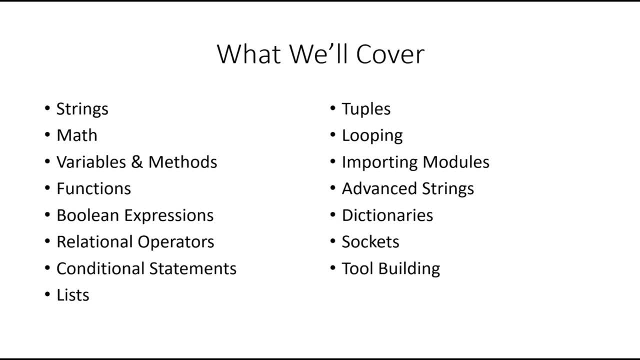 so we're going to be building a port scanner at the end of the lesson and then, when we get into the exploit development section of this course, we're going to use python again to write our own exploits. so it's going to be used throughout the course. you're going to see it again. 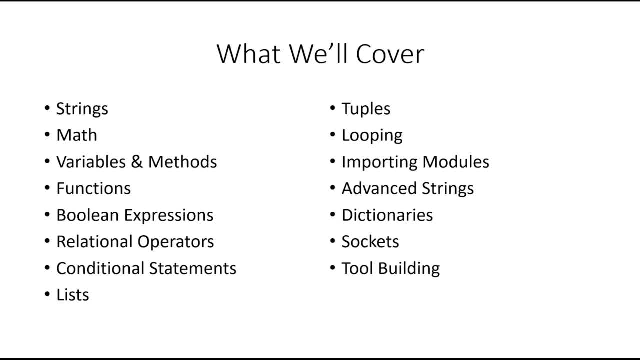 in the next section. so if you're a technical hacker as well, you're going to go on to websites and you might need to download python code or something to utilize against a host or a client, and it's just going to be frequently seen for you. so very important topic to cover, especially for 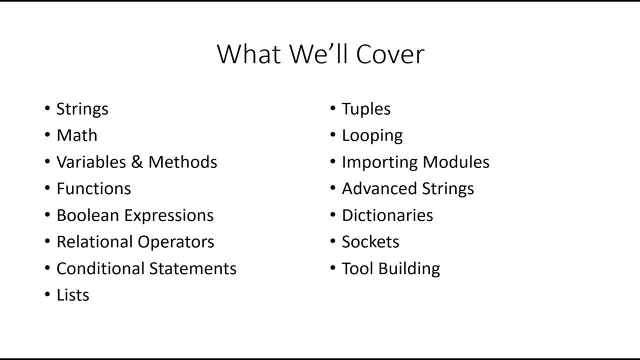 the foundations. one very big thing to point out: you do not have to be a developer to be successful in penetration testing. the important thing is that you understand what you're seeing and understand how to read code. if, when you come away from this module, you have a better understanding on how to 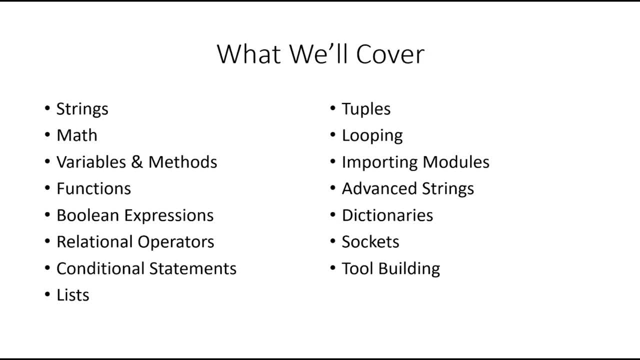 read what you are seeing in code, you'll be much better off. by no means do you have to be a developer. i am still, to this day, nowhere near a developer level and i'm very, very successful in what i do. you don't have to be a developer. so the big takeaway here is to take very good notes. 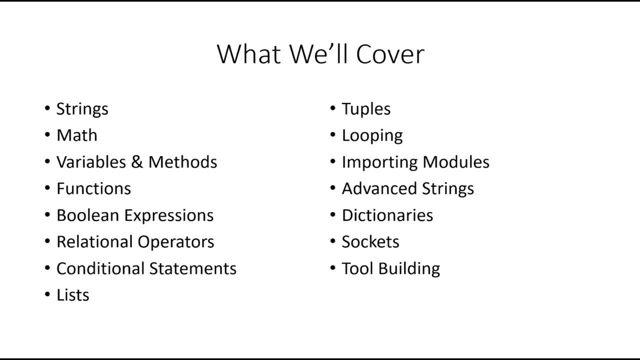 understand what you're seeing. if you need to watch a video multiple times in this section, absolutely okay. just make sure you understand everything in front of you and understand that the lessons are going to build upon each other and it should all come together in the end and you're going to. 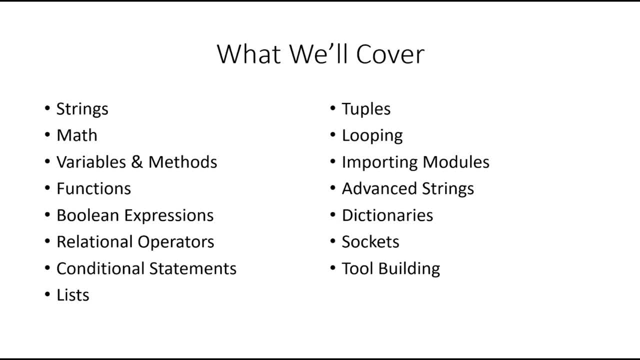 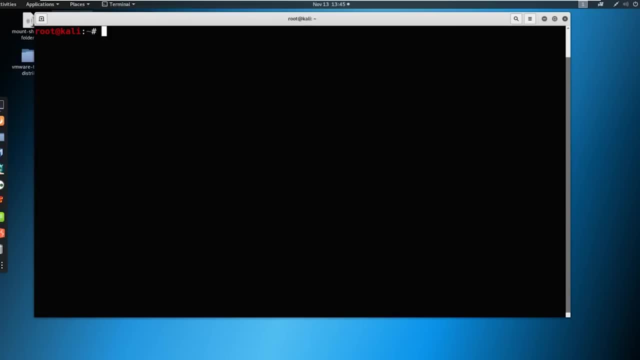 get to see it over and over through the course, especially in the exploit development section, where we write our own python script. so i look forward to teaching you this module on python and look forward to seeing you in the next video. welcome to your first video on python. so. 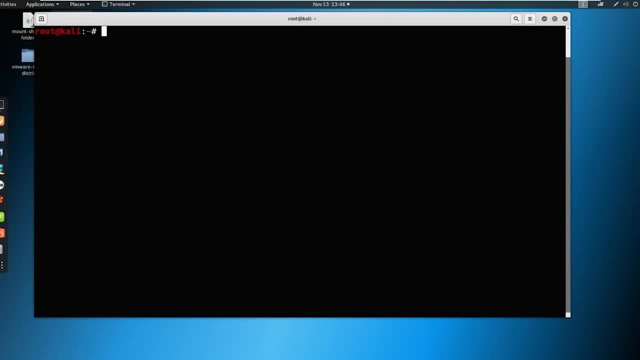 we're going to talk about a lot of a lot of what we're going to talk about in this lesson series. we're going to cover a lot of different topics and we're just going to build upon them slowly so that everything builds kind of upon the last lesson. so in this first lesson we're 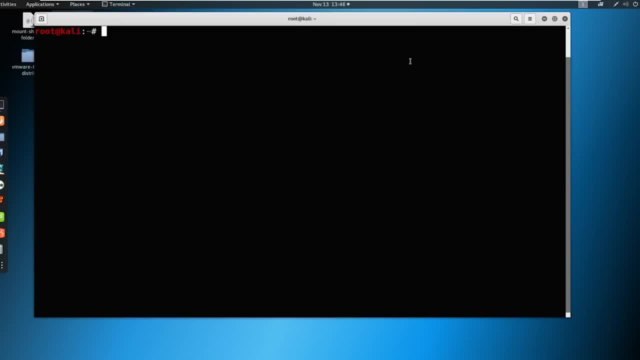 going to be talking about strings and we're going to be working primarily in python 3.. so quick thing to note is that my kali interface might look a little bit different. i'm on my personal pen test machine here. the only reason i'm doing that is because when we get into the text, 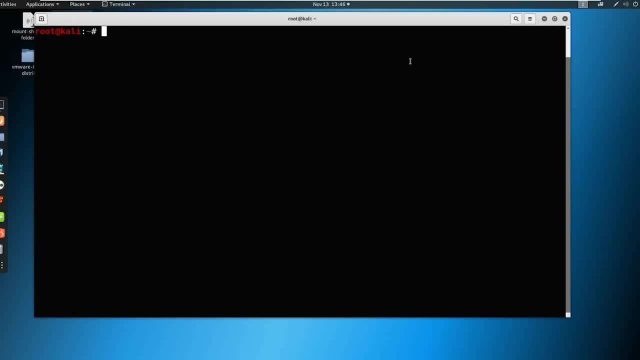 version of Kali would not let me edit my preferences very easily, So I went ahead and just went back to my machine that has an older text editor on it So you can follow along completely step by step in your, your Kali and should be fine. I just wanted to make sure that. 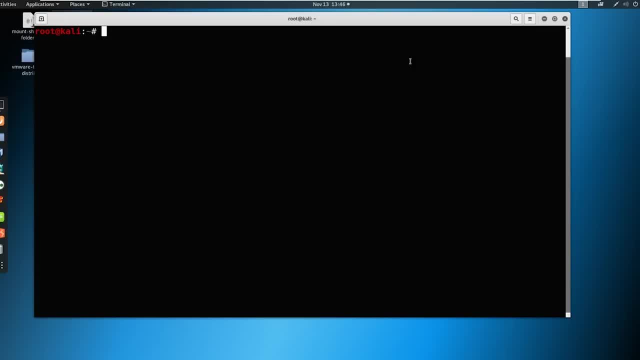 the font size is good enough for the recording. So from here, let's go ahead and make a new directory And I'm just going to call this directory Python, And then we're going to change directory into Python And the first thing we're going to do is we're going to g, edit And 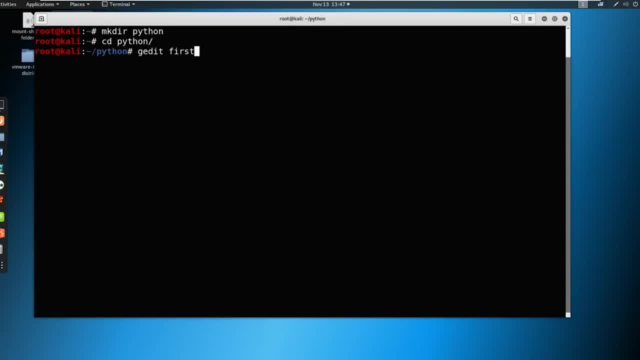 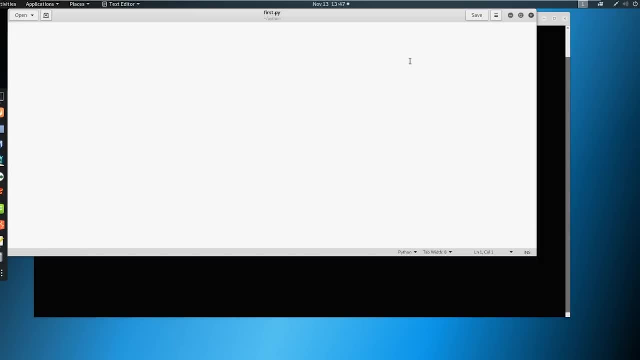 I'm just going to call this first dot pi. this will be our first Python script And we're going to build on it, So the first thing we need to do is declare what it's called a she bang. So that is a hash bang like this, And we're just going to declare bin Python three here at the top. 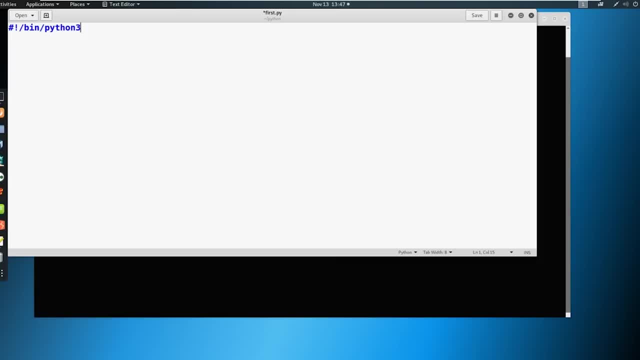 Now, what does this do? This allows us to know, or the Linux to know, when we run this, say we run this to run this like Python three, and then we just say: first, stop pi. if we run it like this, then Python interprets the hash here, which you're going to learn a little bit as a comment. So all. 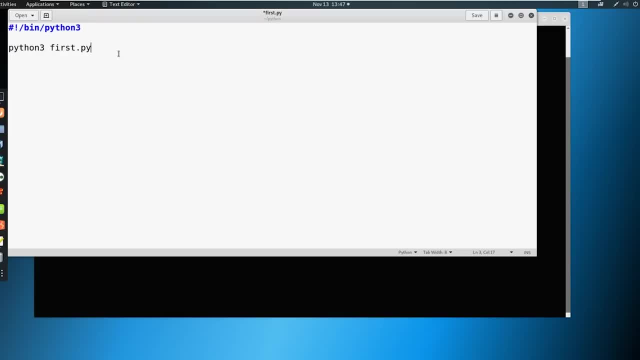 this is commented out, we don't have to worry about it. But let's say we wanted to run this a different way. we want to say: dot forward, slash first, dot pi. then it would actually be interpreted here at the top, So legs would go in here and read this. it would say, hey, this, I'm going to go. 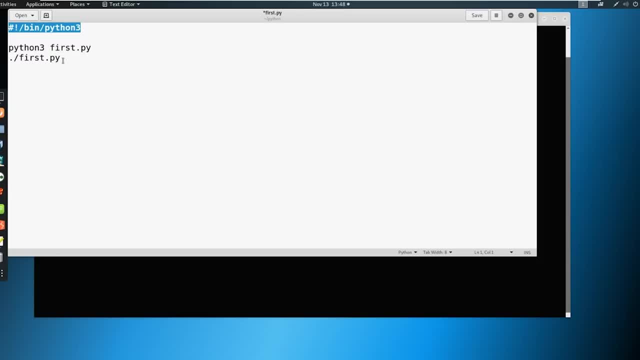 ahead and look for bin Python three. it's going to find Python three in bin because that's where it's stored, And then it's going to use that to execute Python or this Python script here. So we have two ways of running it. we can either run it- Python three first up pi- or we can run 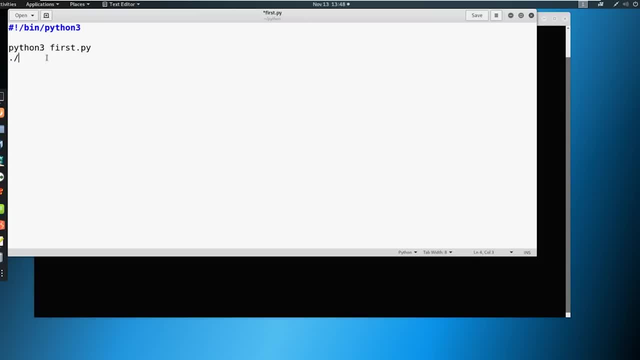 it as you've seen it with some of our other scripts with the dot slash like this. So I always like to declare at the top: it's not necessary if you're just going to type in Python three, but I always like to do it, So I'm going to give you some. 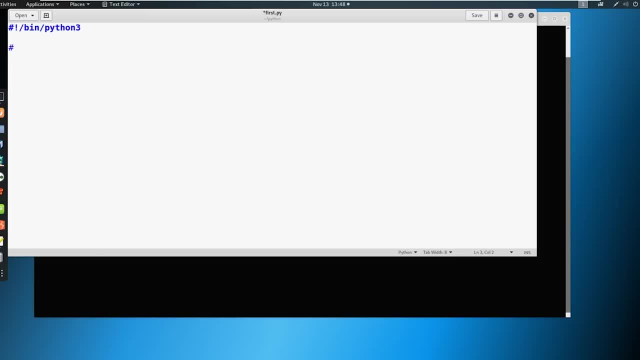 handouts, headers here. So I'm just going to put a comment in and we're just going to say: print string. And so the first thing we're going to do is print a string. Now in the very stereotypical lesson, the 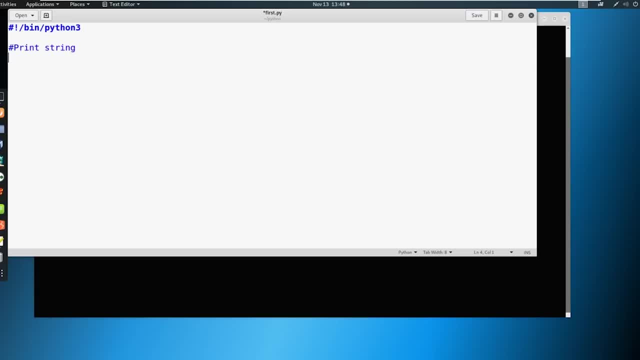 very first string that most people print is the Hello world. So we're going to go ahead and just do that. So let's go ahead and print Hello world, And we're going to do that by just typing in print And then, in parentheses with quotation, we're going to say Hello. 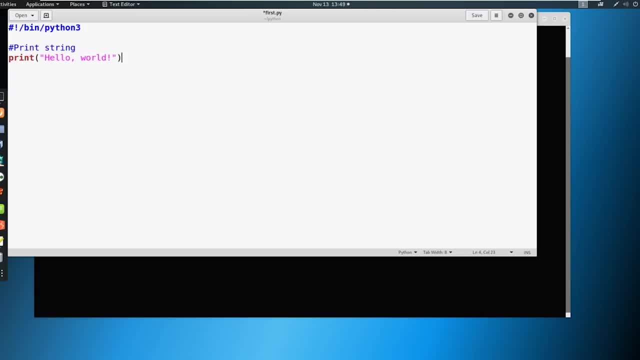 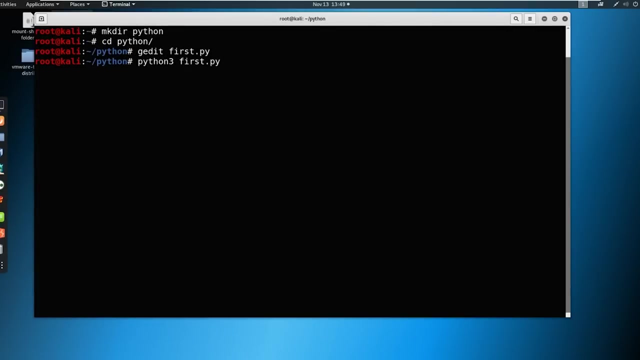 world, something like this: Okay, And that's it. So what we can do here is we can just save this And we can go ahead and give this a go. So what we'll do is we'll say Python three, and then we could say first, and it'll auto tab out to first up pi. 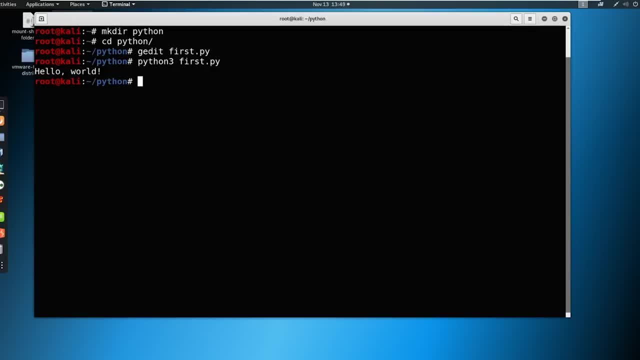 And you can see now that it wrote out Hello world. So if we go tab up twice and go back to our g edit, we can see here that it ignores the Hello world. So we're going to go ahead and give this a go. 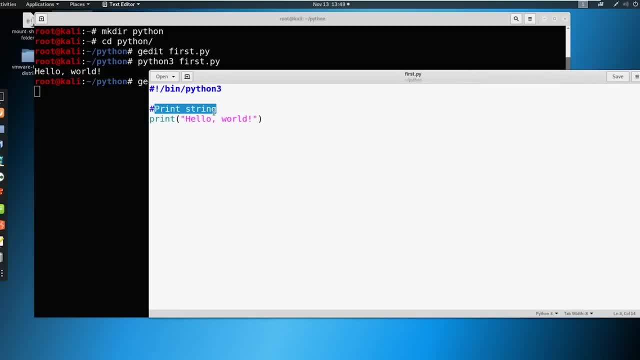 First I'm going to run this module And then I'm going to open up our SpeedC principals thing in this class. If you open this up and go up, you'll see that it now says hello world And you can see that it's clocked previously. So it's going to say: 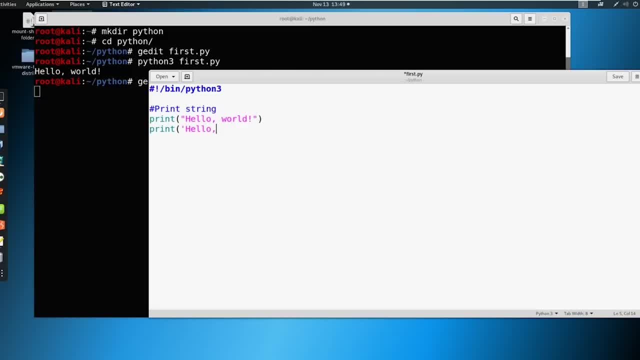 hello world, Imperial wordfm. Just go ahead and give it thatzeichn. You can say nope Also. enter my name here. This is me. How many other letters is it going to make out? It will say Hello world. 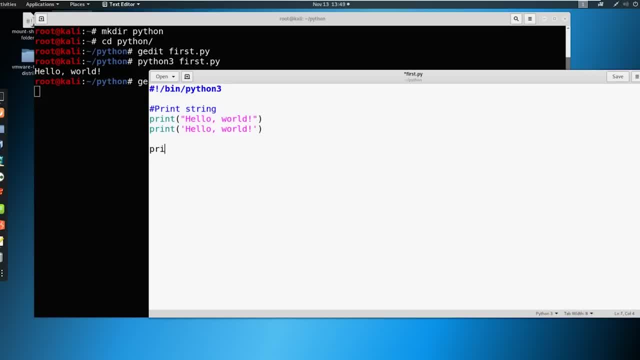 a tab or hit enter twice here, And we could say something along the lines of print: And what if we have, like, a long quote? we could say something like this string runs. And then we could say multiple lines like this: And we just put that with triple quotations, like this: 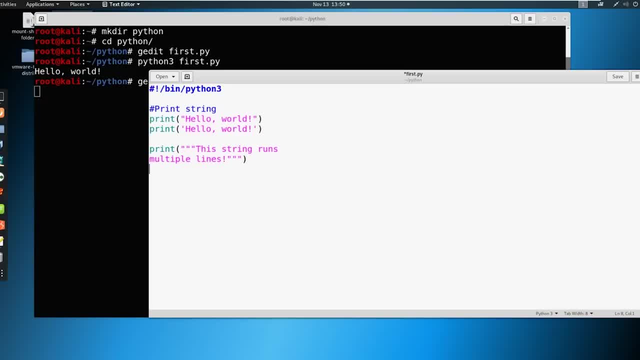 And lastly, we can do a little bit of what is called concatenation. we could say something like print this string is, and then we'll want to put a space at the end here and end the quotation. then we can put a plus sign in here And we could say something like awesome. 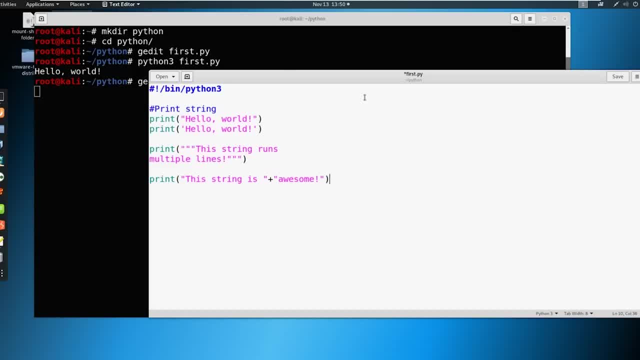 And and that parentheses. So with all this, you're going to see that, okay, we can print Hello world. it should print Hello world, Hello world. this string runs multiple lines And this string is awesome And it should be space awesome here, because we included 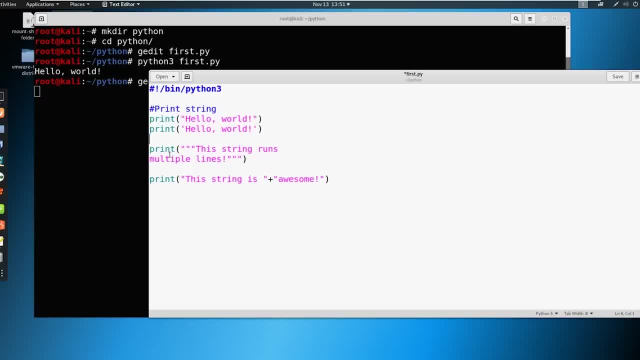 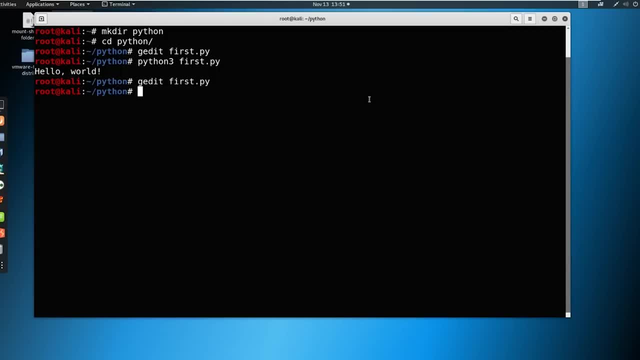 the space. Now you're going to notice, even though we put line breaks in, for us, no line breaks are going to be printed. We'll talk about that here in one second. So let's save this And let's just run it. So we're going to go ahead and run Python three, first dot pi, And everything looks as. 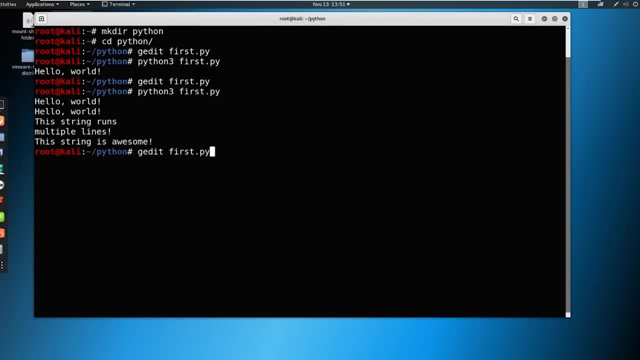 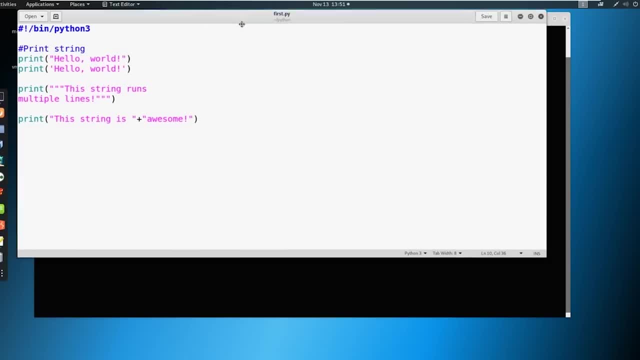 anticipated, Right? So I want to show you one thing. let's tab up twice And let's put an ampersand at the end of this. watch what this does. Now we have access not only to our script here, but we can. 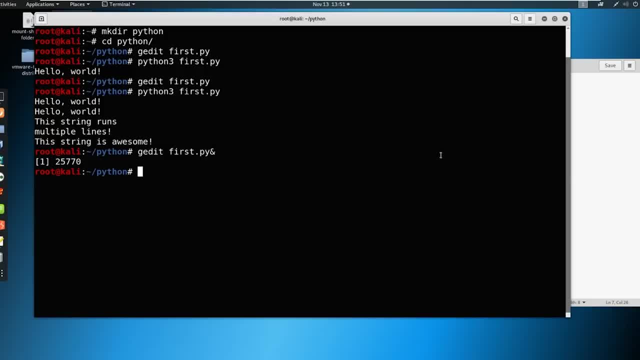 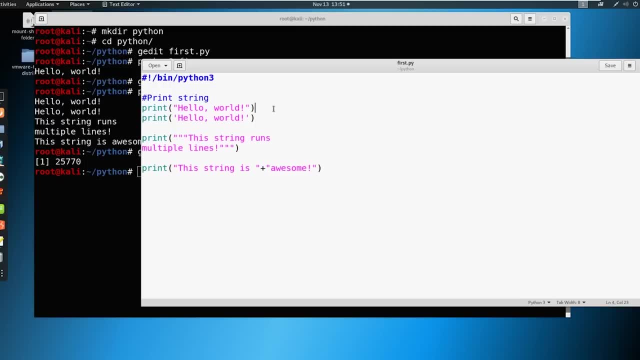 also run code as well. So as long as we save this, we can run the code and we don't have to keep exiting out back and forth. So let's say that we did want to put a line in between these two Hello worlds. we've got this here. what we can do is we can print. 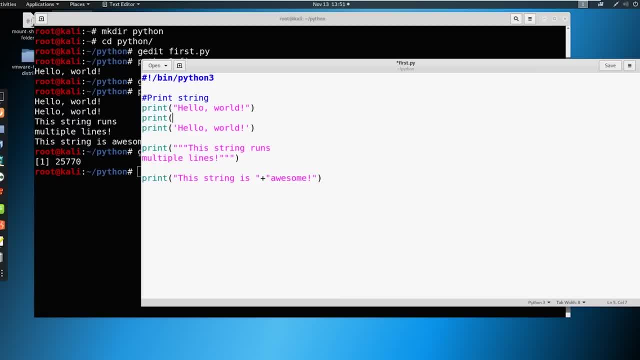 this can say something like a n, like this: I could type today And we close this off And you can put a little note next to it So you remember and just say: new line. So when you have that backslash n, that prints out a new line. So let's say that and just take a look at that. 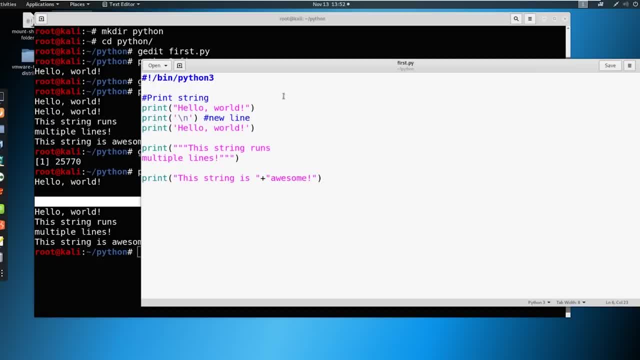 And there you go, you have a new line put in there. So quick and easy way to add a line in Or line break, And yeah. so here, very simple, very simple lesson, right? All we're doing is just learning how to print things And we're dealing with strings. So even if you want to, 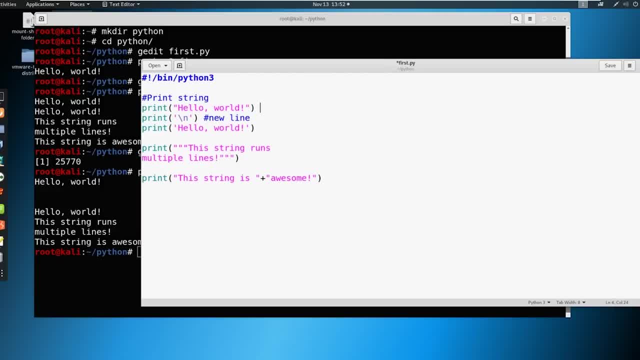 go in and build upon this. you can add comments in for yourself to make this easier. So you can come in here and say double quotes, you could say single quotes And then you can come in here and say triple quote for multi line. 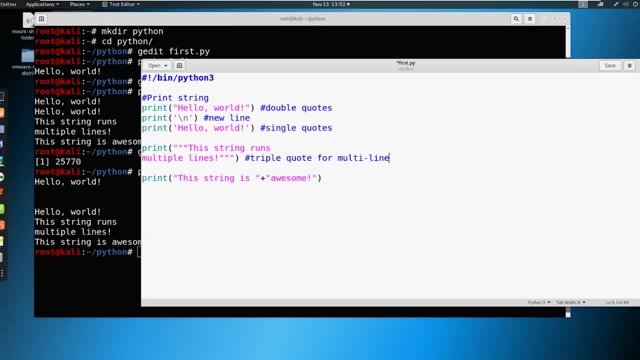 Right, And this way you know kind of what everything is doing. This one you can say: here you could say we can also concat in Nate. I don't know if he spelled that correctly, but I'm hoping I did. So that's really it for this lesson. just want to cover the basics. 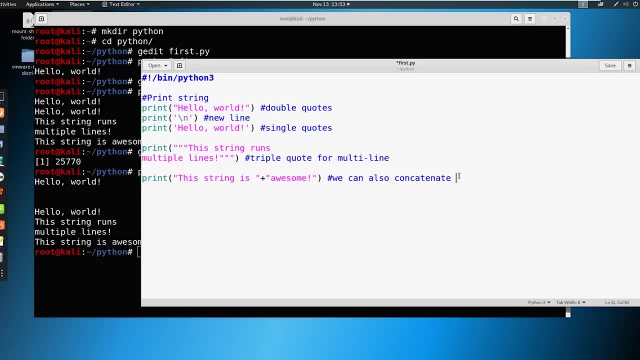 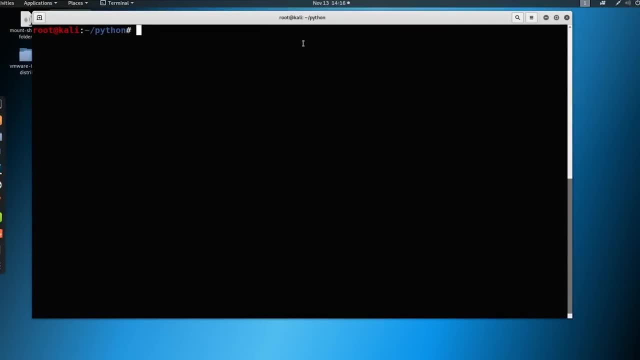 So in the next lesson we're going to start talking about math and the math that Python can do, And again, we're just gonna continue to build upon this. So I'll catch you over in the next lesson. All right, let's talk math. So the nice thing about Python is that right off the bat it has 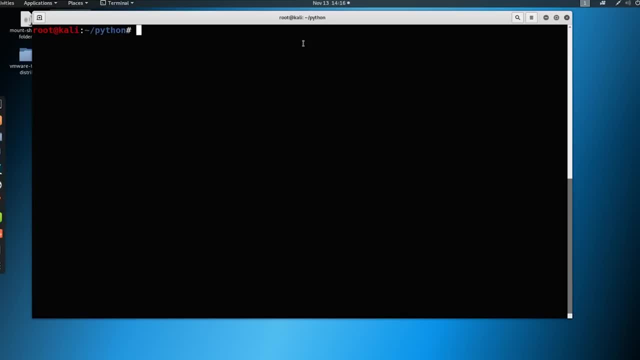 a built in math interpreter. So what we can use it for his addition, subtraction, multiplication, division, etc. we can. we can throw numbers at it and it'll do calculations for us. So let's take a look at what that actually looks like. 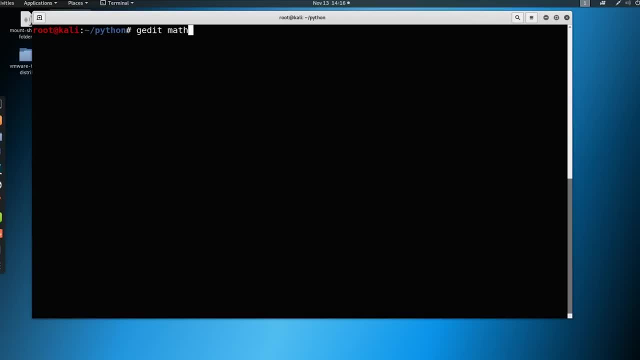 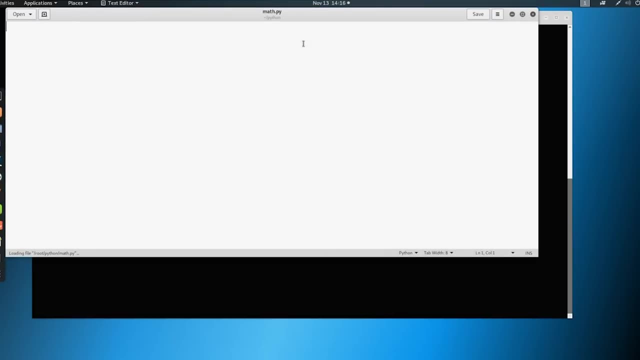 So I'm going to go ahead and G edit. we'll call this mathpy. you can call this whatever you'd like. by the way, I'm going to put the ampersand at the end again And we'll just declare our. 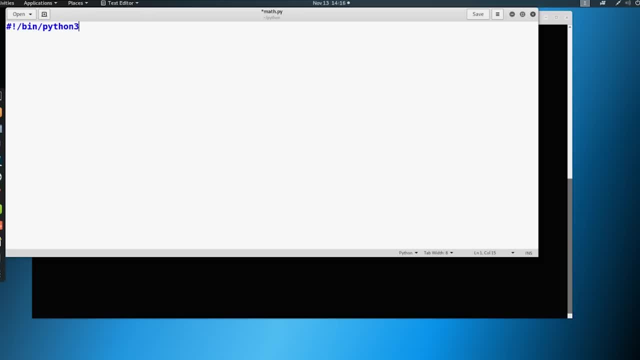 been Python three here, And then let's just call this math. So the nice thing about math is we can do a lot of different things. We're very flexible. So, for example, we can print 50 plus 50. And here we're just adding right. So let's take a look at what this looks like. 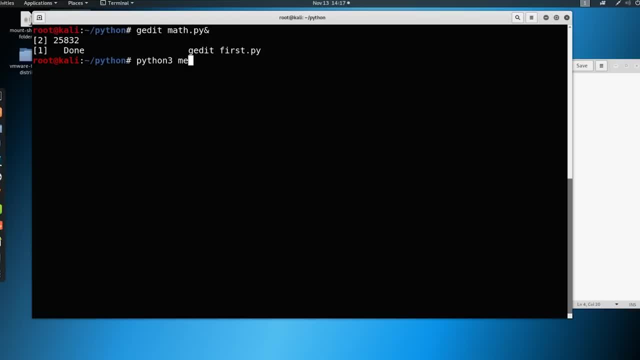 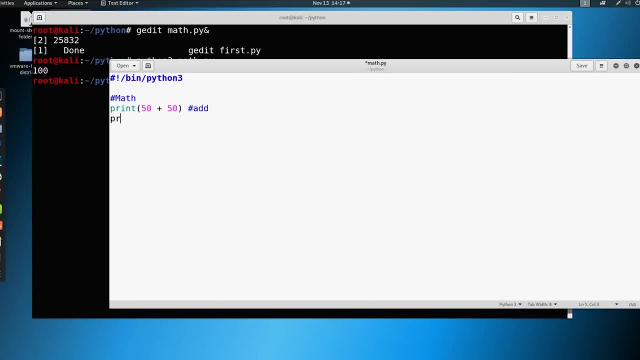 We go here and we just say: Python, three, math, dot, pi. you can see that it prints out 100.. Now we can keep doing this for all sorts of different things. right, We can do 50 minus 50, we would expect zero here. right, And we can do print 50 times 50. 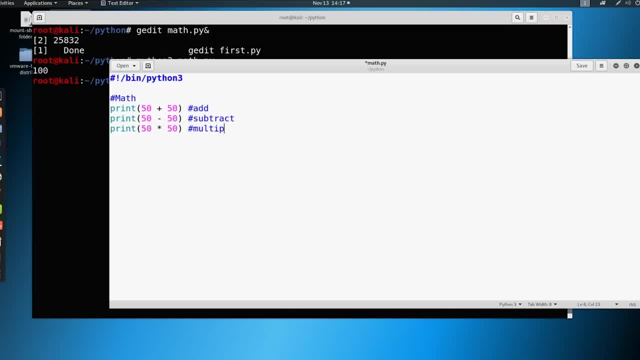 and we can also do print 50 divided by 50 and divide. so I'm going to give you a chance to catch up here. I typed that very fast. I also have notes that I'm looking at. so a little bit of unfair advantage. but so when we see these and we save this and we run it, we're expecting everything. 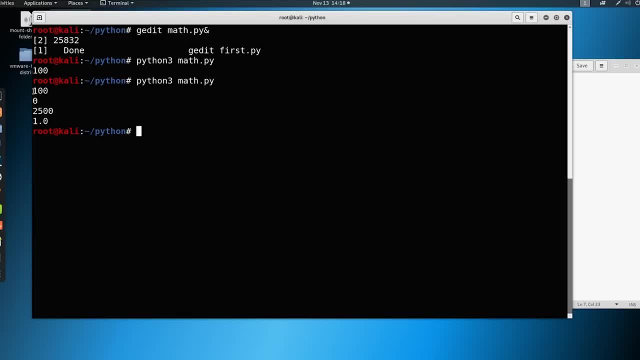 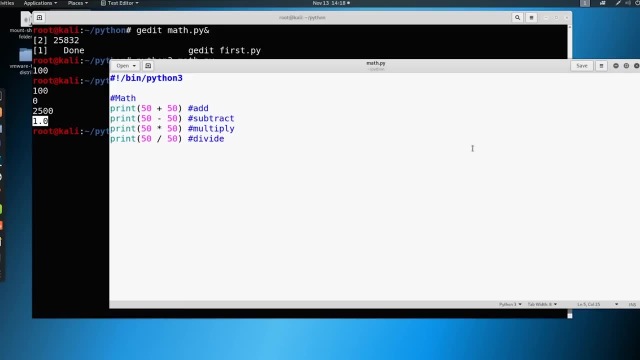 to interpret just the way it did. so you see 100, 0, 2500, and then this 1.0, which we'll get into in just a little bit as to why it's coming out in a 1.0 format. but so we, we have this here and we can. 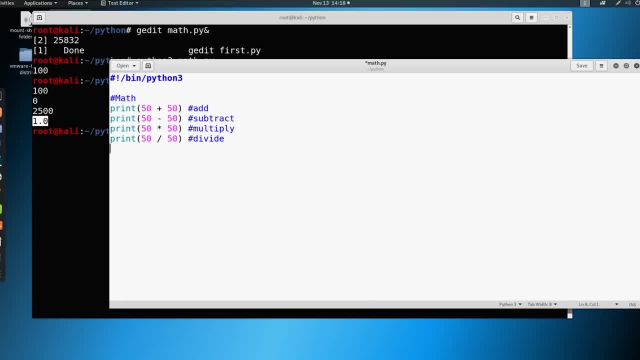 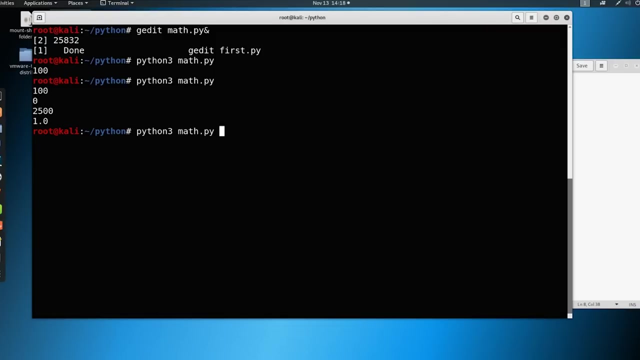 also do some interesting things like: let's do something fun, let's do print 50 plus 50 minus 50 times 50 and divide by 50, and what do you think this is going to do? our good old friend of PEMDAS, if you remember that from math class, so try it one more time. 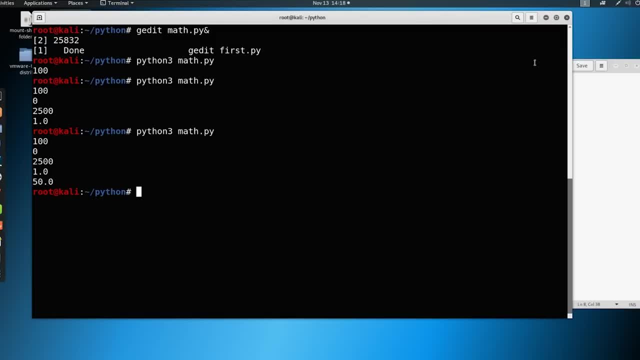 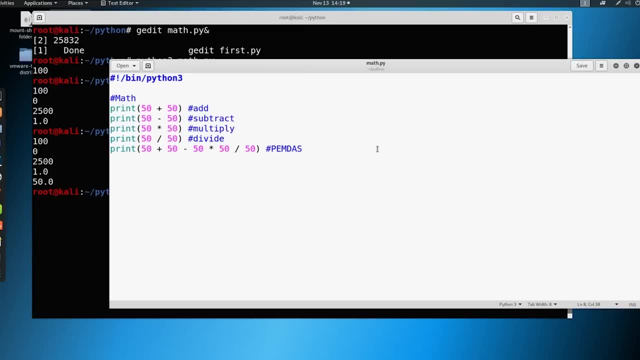 see what number it pops out. pops out 50, so it also does more complex equations as well. so there's a few other things that I want to show you in the math section. and another thing to note. I know I've already stressed this before and I'm going to keep it short, but I'm going to 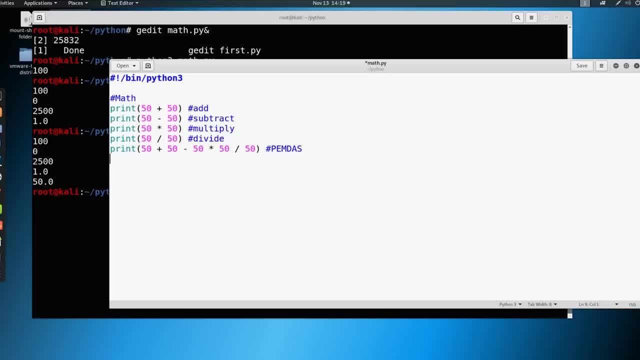 keep stressing it is to make sure you take good notes. this is absolutely going to feel overwhelming. I'm going to throw a lot of things at you, especially with all the stuff that you're learning. take good notes, have a good notebook and make sure you're writing this all down. so 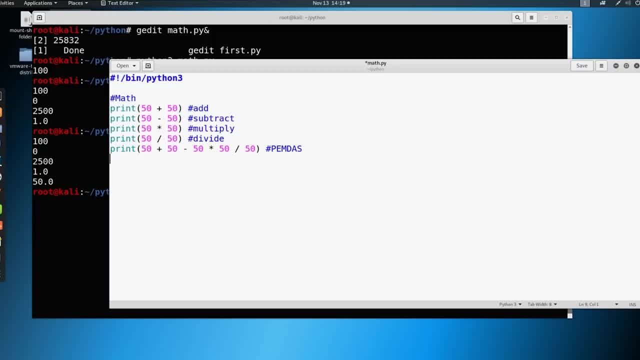 then you can just go back and you can reference it, and from here on out I'm the next video. what we're going to do is we're going to make a script and we're just going to build upon it and I'll just leave everything in that script, so that way you kind of have a place for all of your notes as. 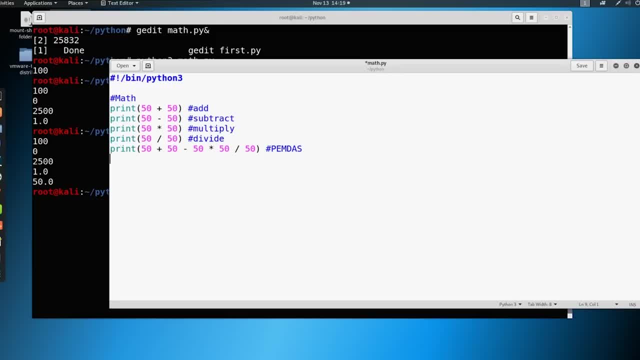 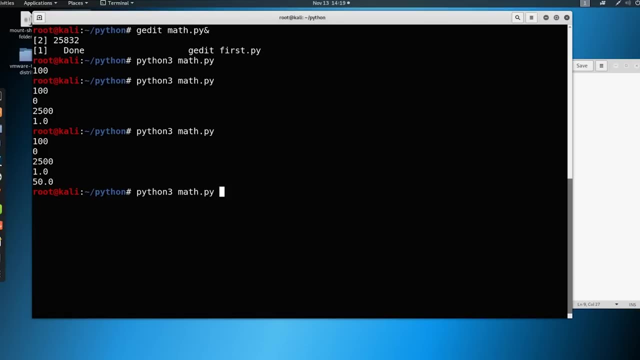 well. so here let's talk a couple more things. so we can also do exponents. so let's say, we want to do 50 to the 50th power. well, we just write it like this, and now we have exponents here, save it, run it really quick and we get this very 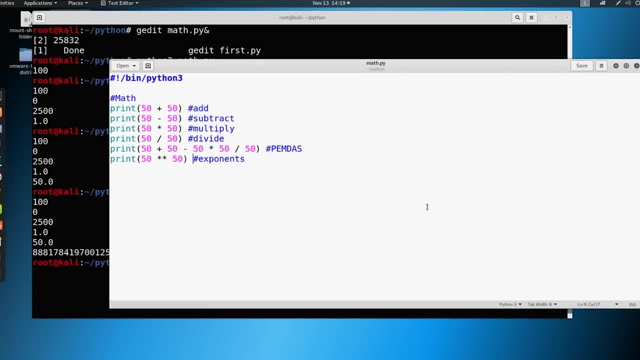 very, very large number, right? we could just make this to the second power and make a little bit simpler. we could also do this. so we do print and we do 50 percent six. now this is called a modulo. let's take a look at what it does. 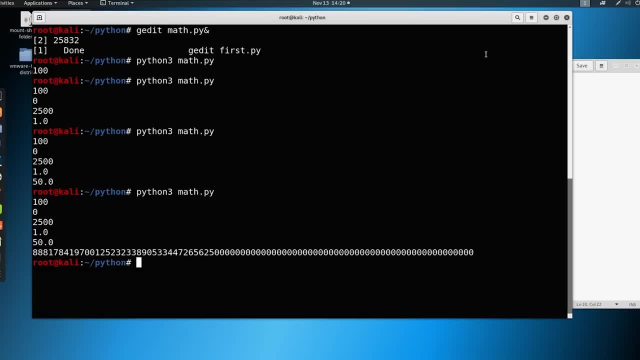 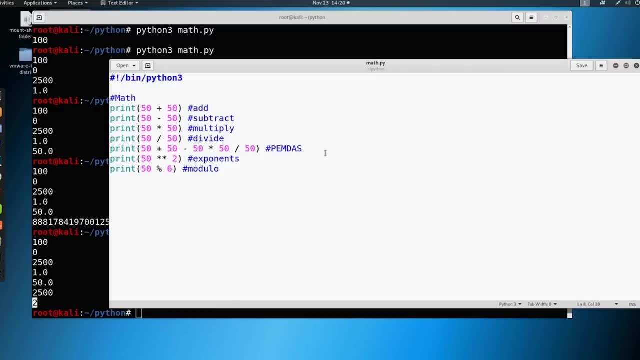 so 50 is not divisible by six, right? so what it does is it takes the number that is left over, so we do 50 divisible by six. okay, six goes into it eight times, and then it has a leftover number of two, right. six times eight is 48.. 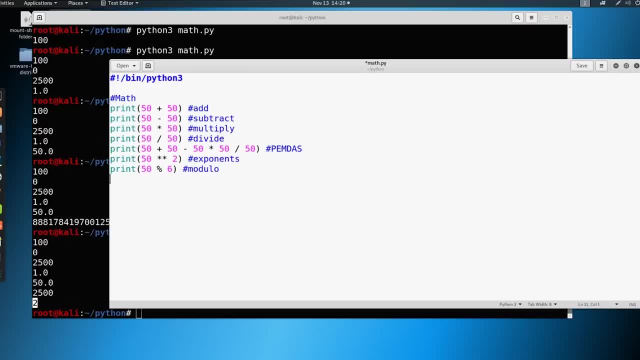 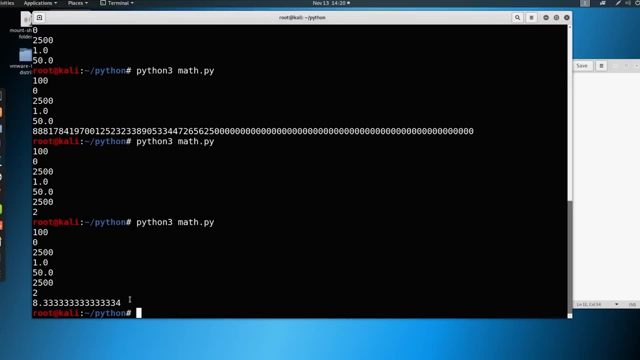 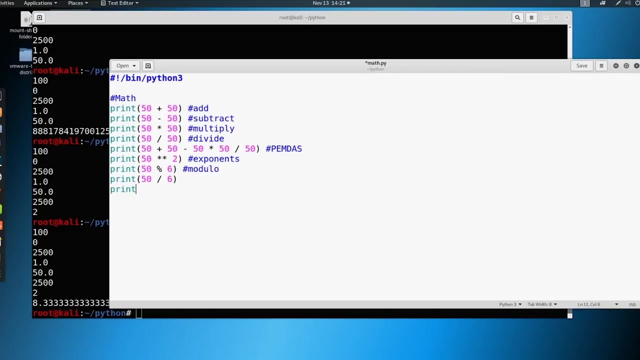 over number two. so that's the modulo. what if we were to divide by a number here, and we said 50 divided by six? what is that going to do to us? well, we print that out and you see it gives 8.33334. perfect, that's fine. what if we just want a number without any leftovers? well, we can do something. 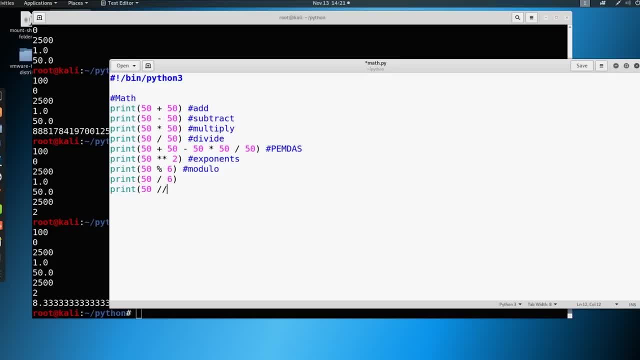 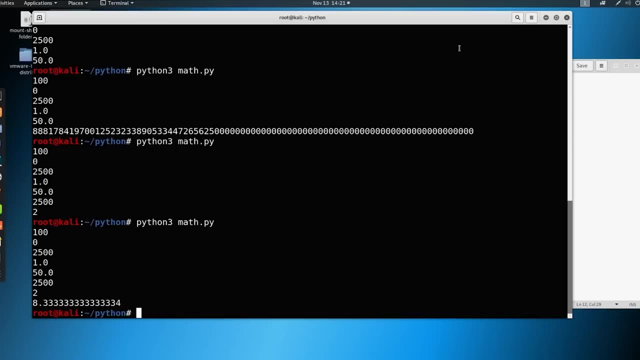 like this: you can do 50 divided by six, and then we'll just say: no leftovers here, okay, so i'm going to give you a second to catch up, we'll hit save on this and we're going to go ahead and run it, and you can see that it just 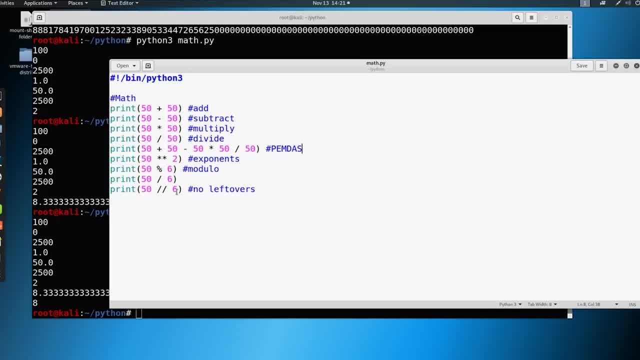 gives us, gives us the eight, doesn't give us that leftover of two that we had and put it into fraction form here or decimal form here. so we have different ways that we can manipulate this numbers and we can do math on it. so we're going to go ahead and run it and we're going to run it. 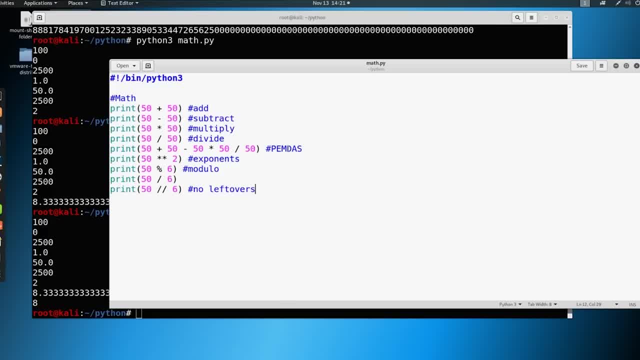 on the fly. there's also math modules which we haven't gotten to the modules yet, but there are additional math items that we can pull into this, like bringing in random numbers, for example, and other things that we can do, more advanced calculations in python, but as a base it does. 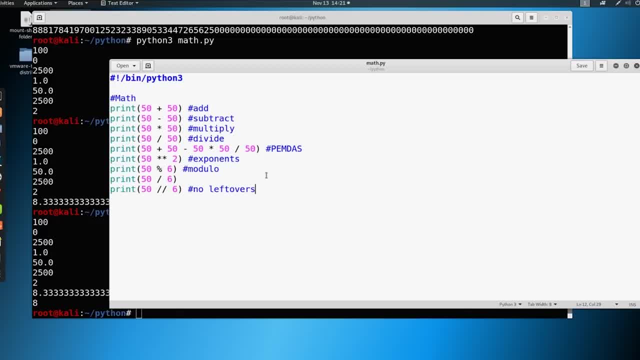 quite a bit of items for us, and it is a essentially a built-in calculator, so we can do quick math on the fly if we need to. so let's go ahead, and from here we're going to move on to the video where we're going to start talking about variables and methods. 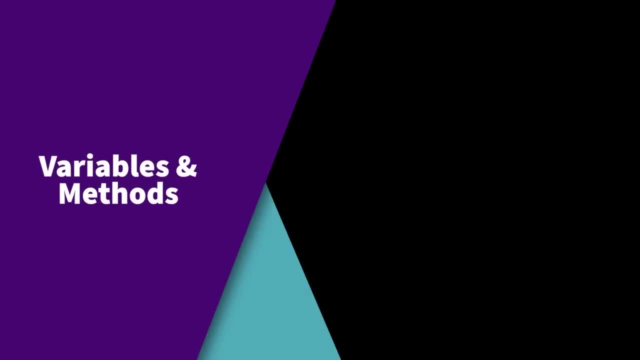 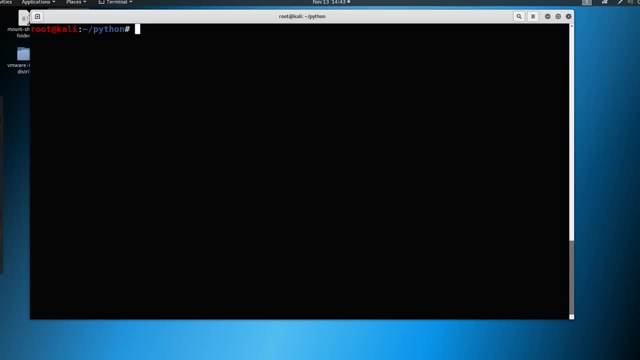 all right. so let's talk about variables and methods. so to do this, we're going to make a new file. so let's do gedit, and we're going to call this one scriptpy, because in the last video i told you we're just going to start building off of these scripts and we're just going to keep it. 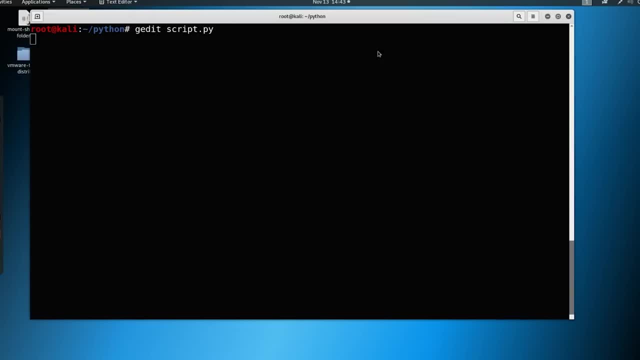 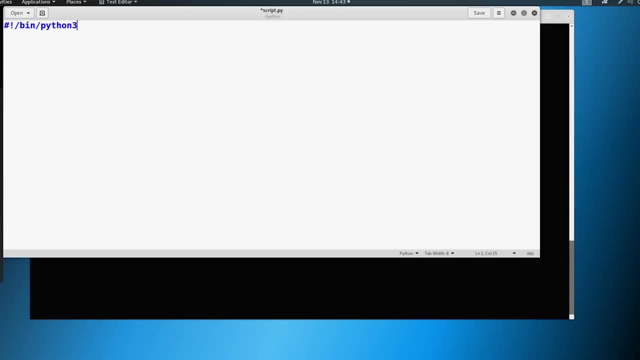 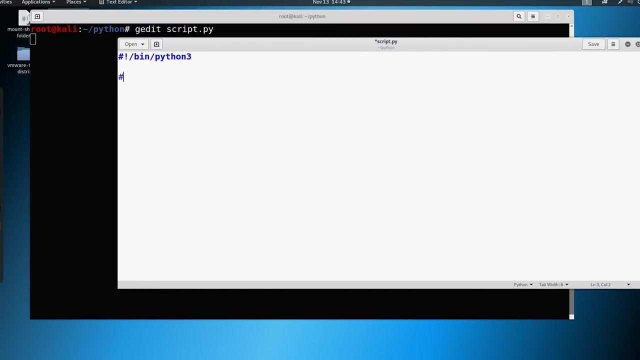 in one script and keep it going. so let's gedit scriptpy. we'll do one more shebang here of bin python 3, and then we're going to go ahead and just build this out. i'm going to drag this over just a little bit, so let's put a another comment up here. 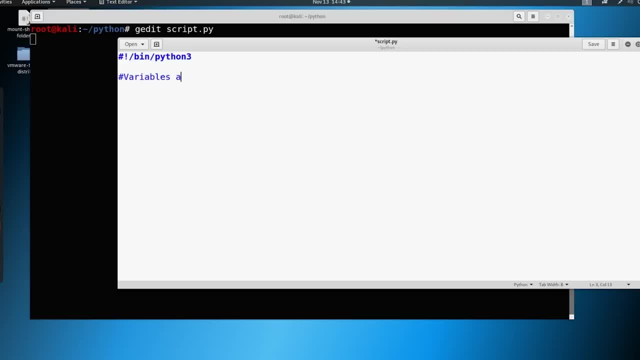 and we'll just call this variables and methods, and let's define a variable. so let me show you what a variable looks like and then we'll define what a variable really is. so let's start with a variable and we're just going to pick your favorite quote here and we're just going to say: 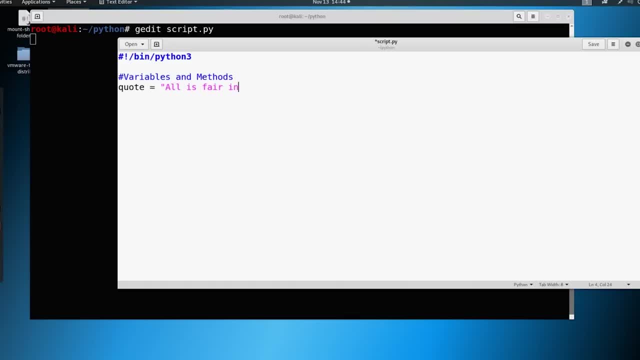 something like: all is fair and love and war. okay, so what's happening here is we are creating a variable of quote, now a variable. all you can think of a variable is as a placeholder. so instead of typing out all is fair and love and war, we can just call this placeholder at a later time and 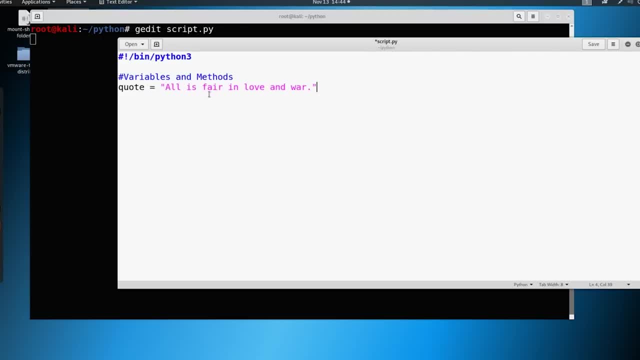 it knows, hey, i'm going to call this information and it's going to call this information and it's going to store this information inside of quote and then later we just call quote and it'll print it out, so we can do something like print quote and save this. and i forgot to ampersand, so excuse. 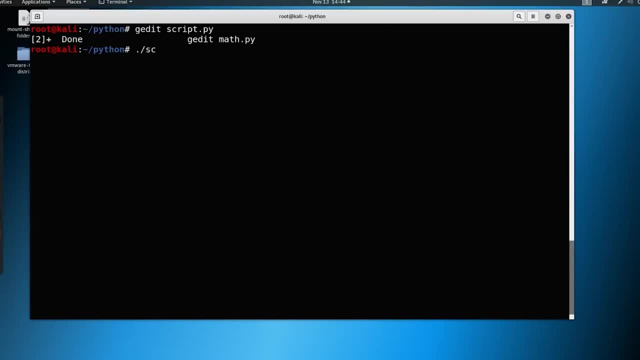 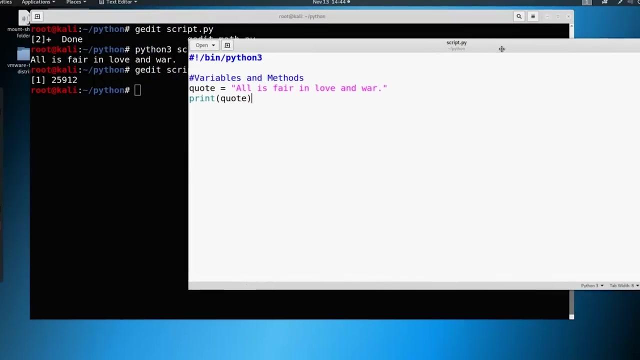 me, we're going to close it and let's just run scriptpy. sorry, python 3, scriptpy. you can see it says all is fair and love and war. so if we gedit this and add the appersand now, so we defined what was in our variable here, which was this, this string: right, we've talked. 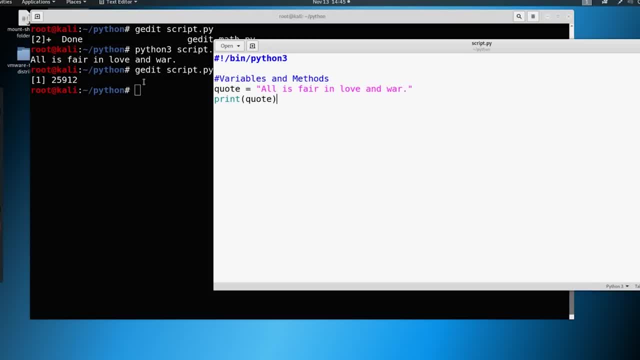 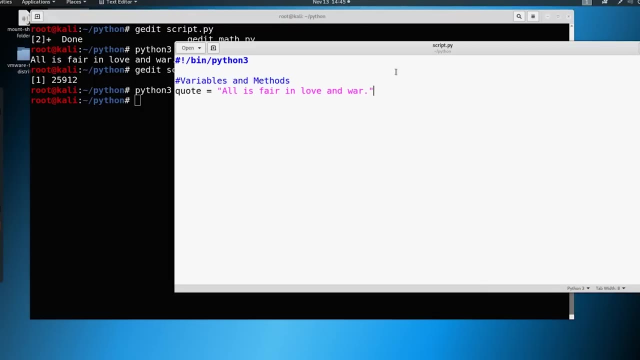 about strings. we put a string here as our quote and we printed the quote. so if we didn't put the print in here, we just we can copy this and just delete it. if we save this and we go to print this now, there's nothing telling this to print. so we have quote and we have a 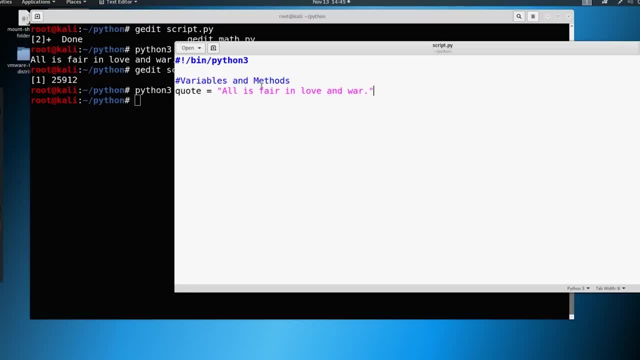 quote stored in our quote variable, but nothing instructing it to print. So we can, we can leave the print back in there, just copy and paste it back, And now it'll print that quote. Now we also have what are called methods. Okay, so methods are basically functions that are available for a given. 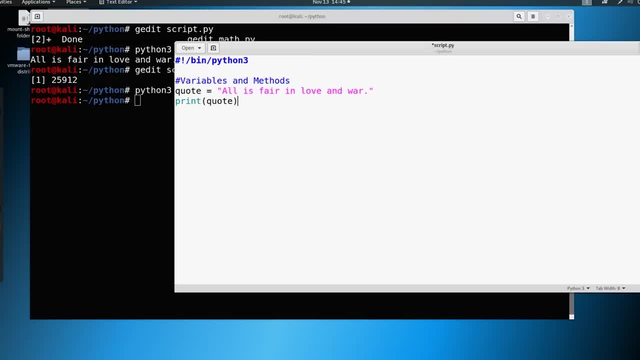 object Okay, so don't worry too much about that description. That's very dictionary based description. Just think about what a method does. So I'll show you these methods here. So a method might look something like print quote And then let's say we want to make quote upper, So in order. 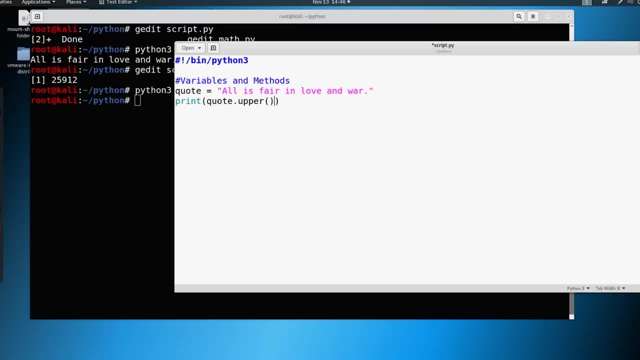 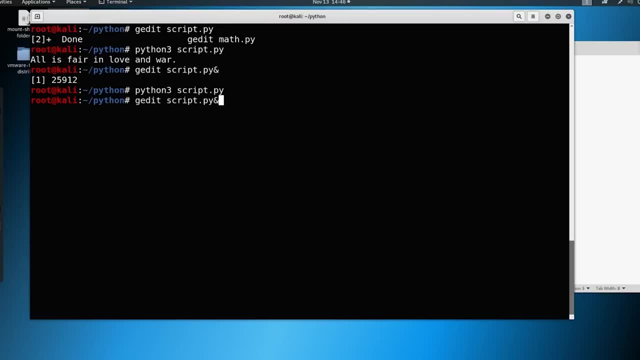 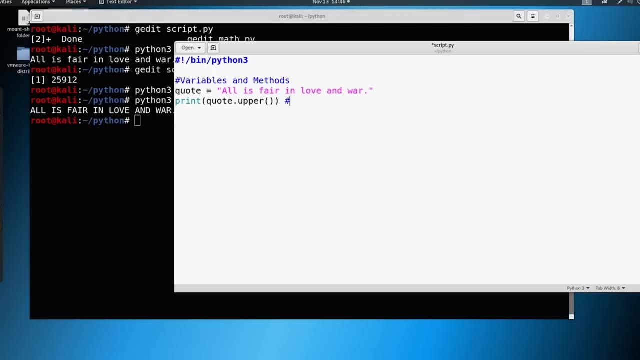 to make it uppercase, all uppercase. we're just going to throw in this method of upper so we just say dot, upper. And if we were to save that and print it? Look, now the text is all uppercase And you can make a note in here if you want and just say: makes it uppercase, And we can copy this, Let's. 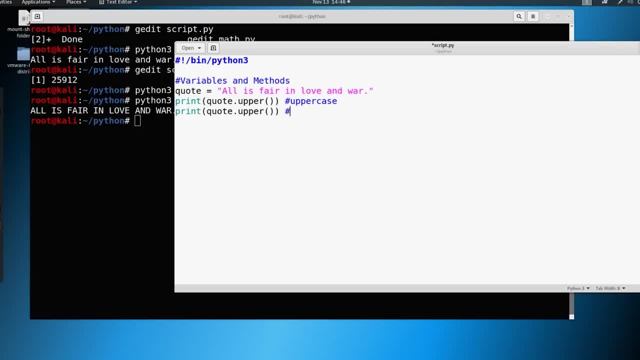 just copy this whole line like this And let's paste a couple here, So we could also do something like lower for lowercase, Or we can do something like title for title case, And we can make notes here of lowercase and title case. Okay, and we save that. And when you print it, what do you? 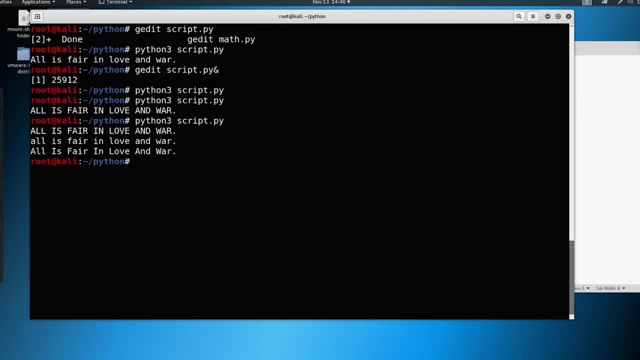 think is going to happen here. So we're going to say: all is fair in love and war. all is fair in love and war. And you can see in title case: not perfect, it's capitalizing the and here and the and the is, but it does capitalize every first letter as it's instructed to do here. So these 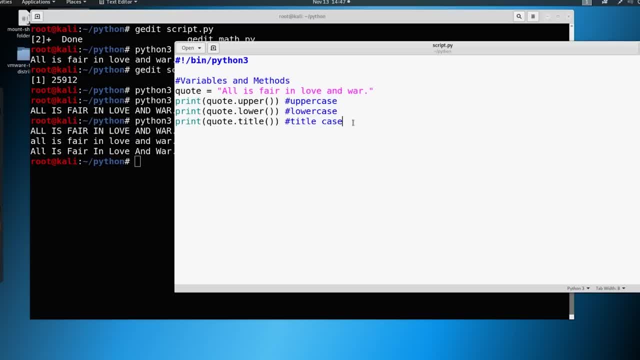 are methods. There's also other things that we can do. we can do something like say we want to get the length of this quote, we want to know how many characters are in there, And we can do something inside the quote. we can do something like print length of quote. Okay, we can just say save and. 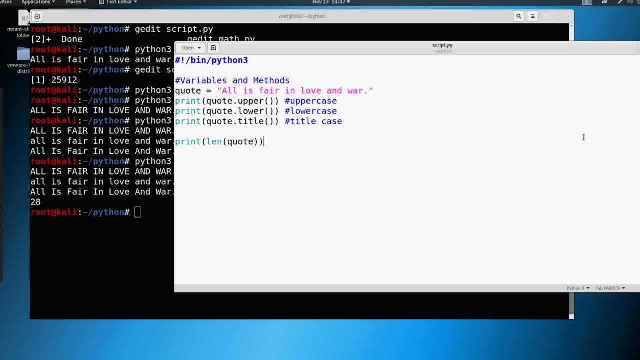 let's see what it prints out. Okay, so 28.. Now it's 28 characters completely. we were to count this all up including the spaces. there's 28 characters there. So let's make this a little bit more interesting And let's talk a little bit more more about math and bring that into it and try to tie. 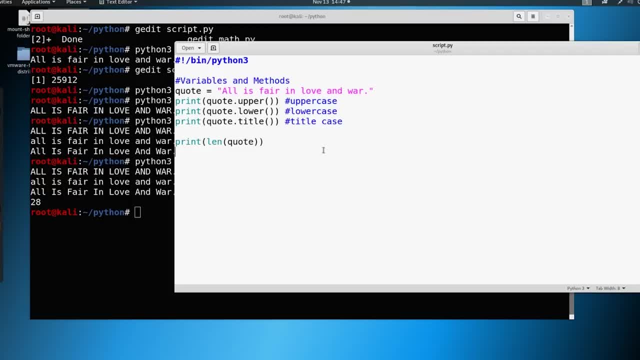 this all together with what we've learned so far. So let's use your name, let's define a variable of your name, And we're going to set it as a string. So my name is Heath, So we'll just say this is a string, right? And let's also define your age. 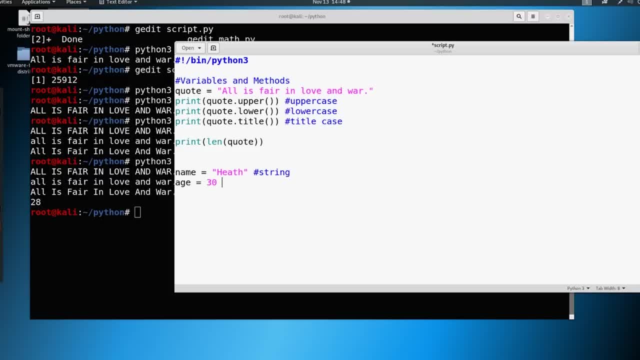 Now I'm 30. And we'll say this is what is called an int or an integer. Okay, and let's say: what's your grade point average? And my grade point average was 3.7.. And this is what is called a float. Now, what is the difference between an integer and a float? 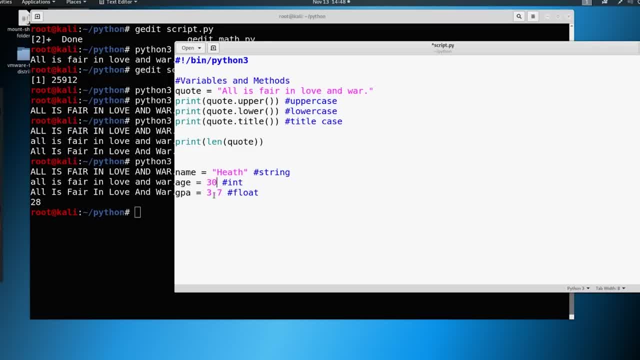 Well, an integer has no decimal point, a float does So. if I was 30 day or 30 years and 27 days, I might be 30.1 years old, right, But if I only define as an integer, if I say int 30,, 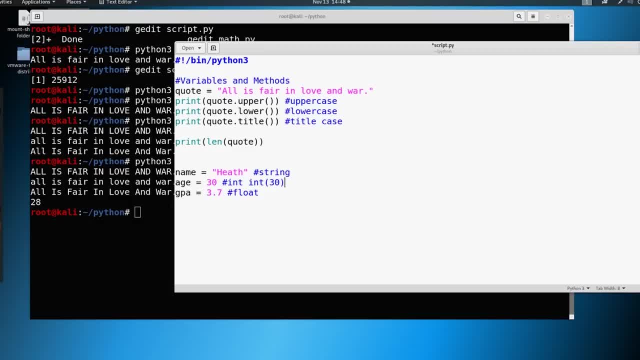 then that's going to define that this number is the integer. And if I say int 30, then that's going to define that this number is the integer. an integer and nothing else. Same thing with float, if we want to have the decimal point there. 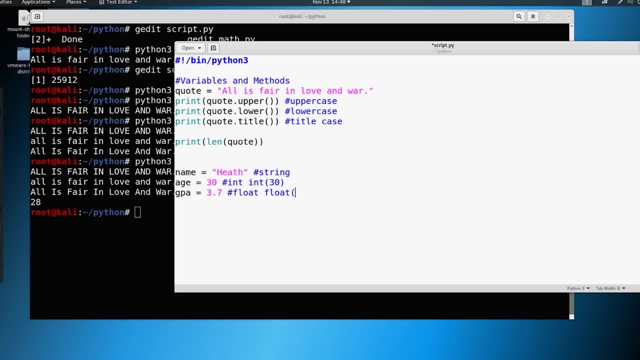 we can float a number and define it as like 3.7.. So let's make more sense of this: we can print out the integer of my age And we can also print out the integer of my, or we could say 30.1.. 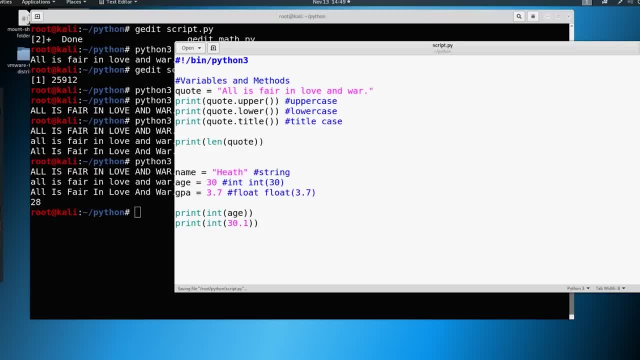 And let's see what happens, as we discussed here. So let's save this And let's just print out those two And look, it takes 30.1, and makes it 30. And it takes integer- integer of age- and makes it 30 as. 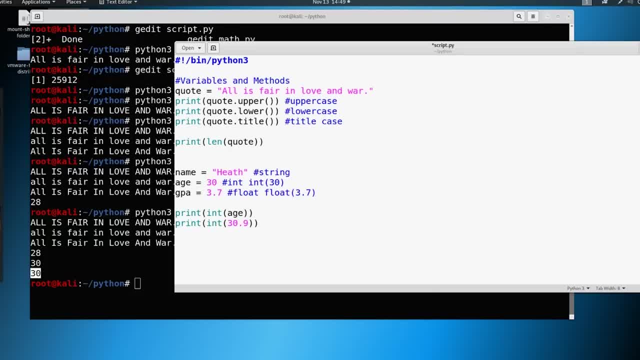 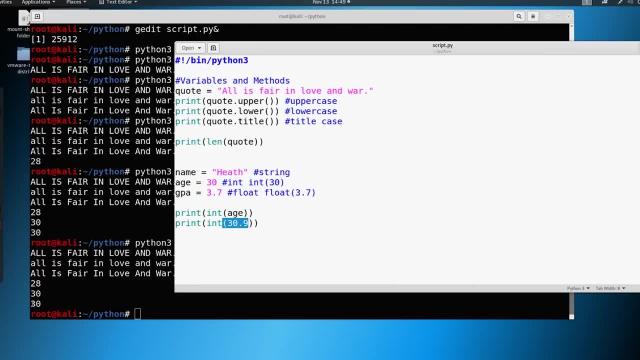 well, Now what if this is 30.9?? What do you think is going to happen? You think it's going to round. It in fact does not round. So you can see, 30.9 still came out to 30 down here. It doesn't matter. 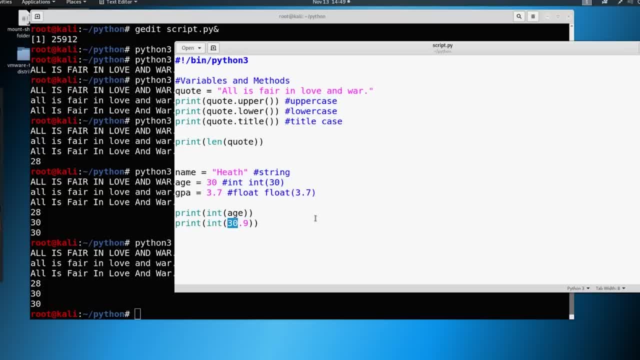 it just takes this first number when we call an integer. So make sure that if you ever use integer, you know that it does not round. So let's build upon this again. we could take a string now And let's print out a string. we could say something like my name is, And then you could say plus. 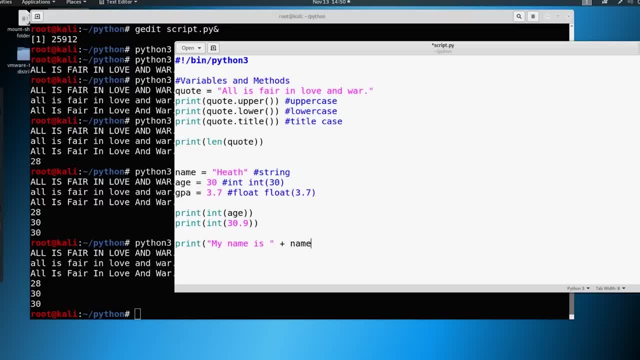 name. make sure you add the space in there, right? And you can also say space and I am space, And then let's define an age. So if we try to put age in here, watch what happens. So we're going to. 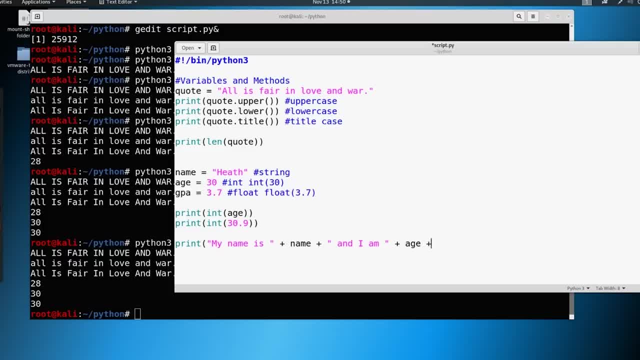 say age and we'll say space Years old, And let's save this here like this And I'll give you a second to catch up. So again, we're adding a space: space in the beginning, space at the end, space at the. 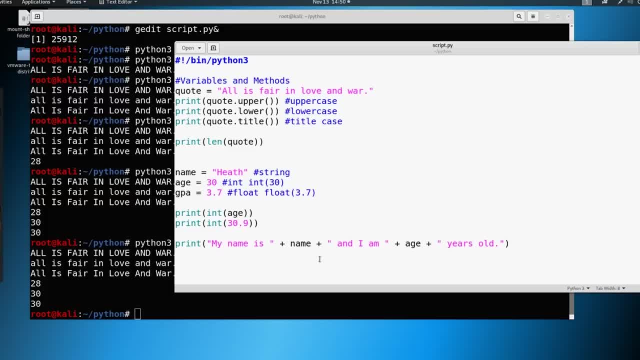 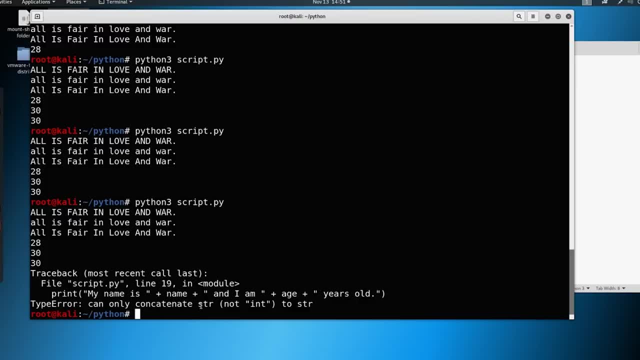 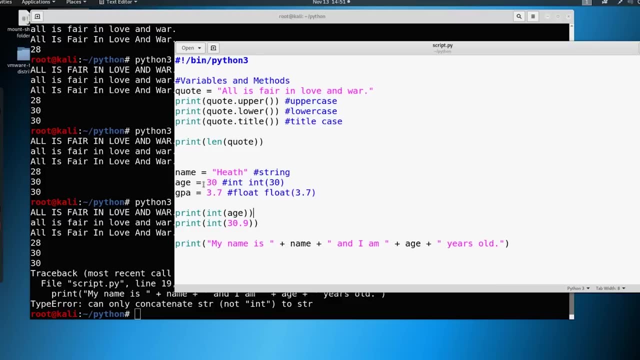 end here, just so that we have the syntax right, or else it's going to all bunch up together. So let's try to print this out And you could see, cannot concatenate a string, not integer to string. So this age here is sitting here as an integer. you can't concatenate a string with an. 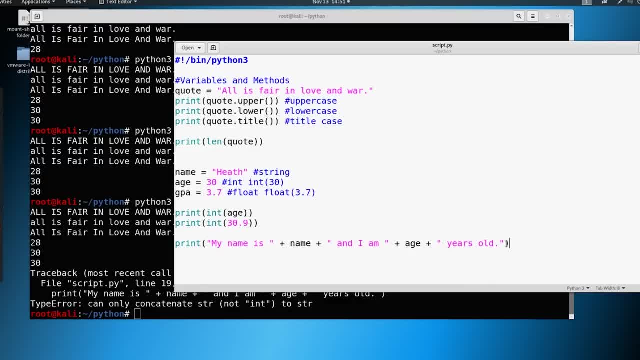 integer. So how do we fix that? Well, what we can do here is we can actually put this into an integer And we can also make this into a string format. So we'll just say string of age, something like this, and save it, and now it makes it to a string So similar as we made something into an integer. 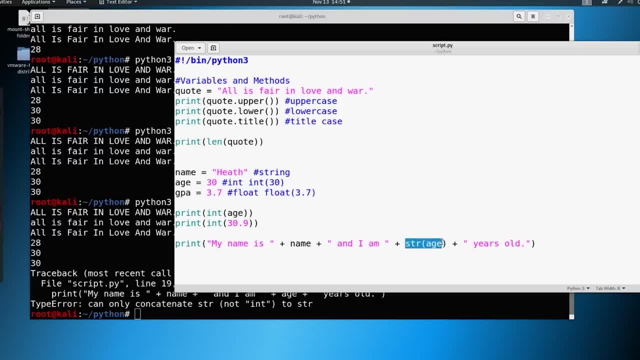 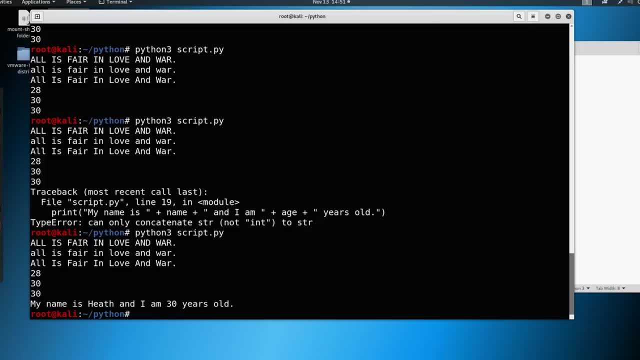 and how we can make something into a float. we can also make something into a string. So if we come through here and we hit enter, you can see now that it works. My name is Heath and I am 30 years old. 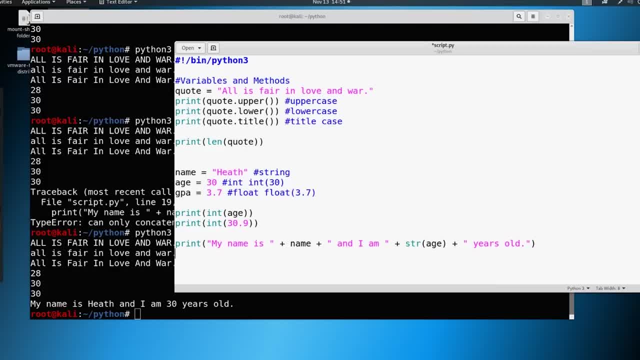 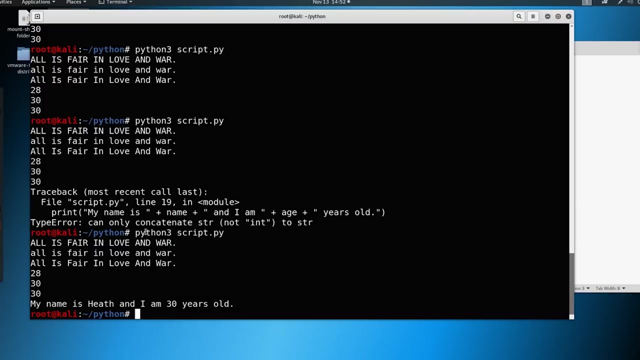 So a couple more things to know: What if we had something like our age and you know we got a year older? well, we can just say something like age plus equals one, And we could say: print our age. Now watch what happens. Age is. 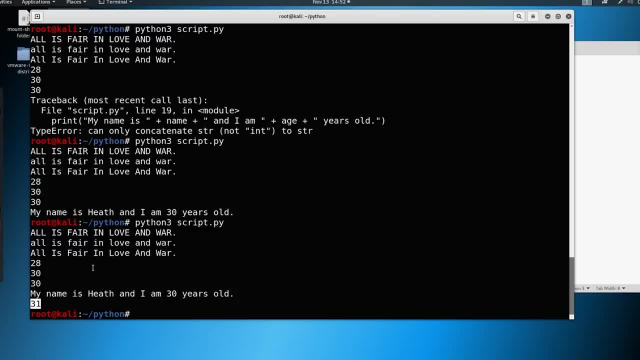 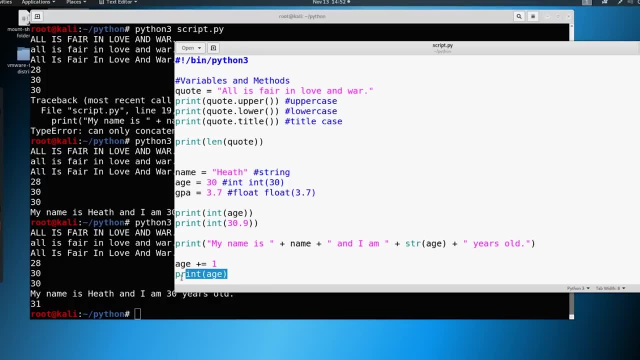 now 31.. Even up until that point, age has been 30. Right, you see age coming through here. we're utilizing it in all of our data, All three places. Now we print age down here and it's 31, because we have changed what is stored in. 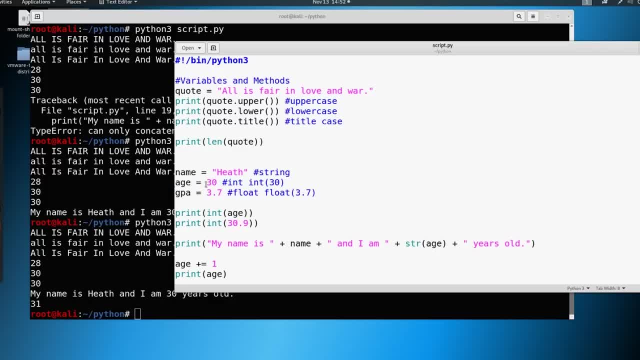 the variable. So again the variable here: of age. we had 30 stored in it up until the instruction is called to add. one plus equals one. So we're just adding one to this age variable here. then it stays 30. Now it is 31 until we change it again. So we can also do something along the lines of: 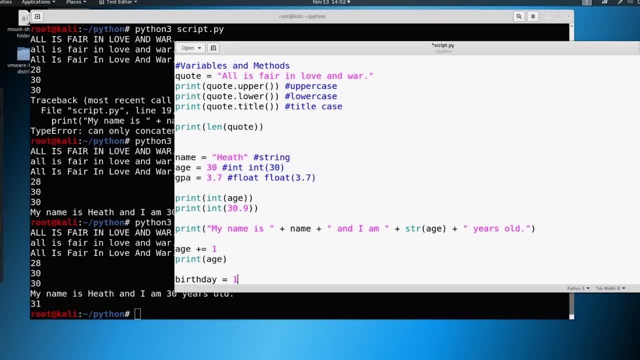 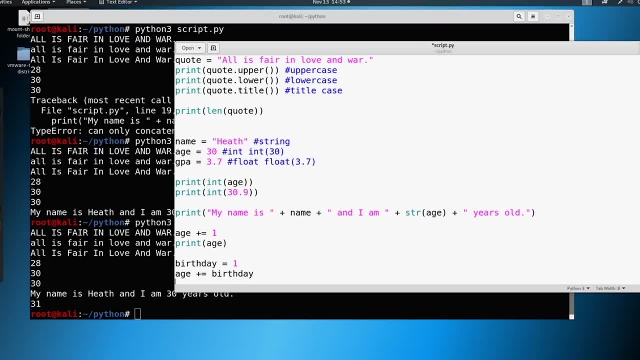 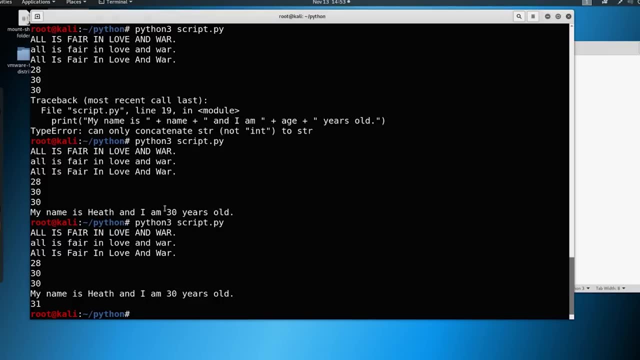 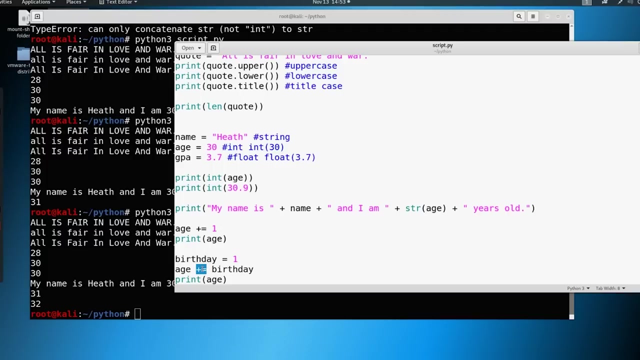 birthday equals one, so we have a value of birthday. And then we could say age plus equals birthday, And then you're going to print your age again And guess how old we're going to be? we are going to be 32.. So it doesn't matter how you store it. you can do the plus equals here or minus equals if. 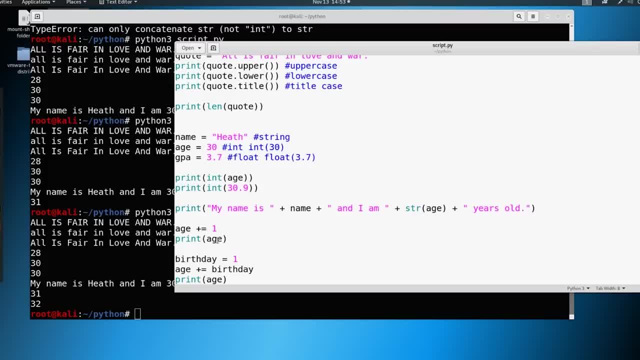 you want it to take away And you can start incorporating your math into your variables. you can incorporate your variables into your strings And you can start tying this all together. So if you need to rewatch this and to make more sense of it, that's absolutely fine. I'm going to harp one more. 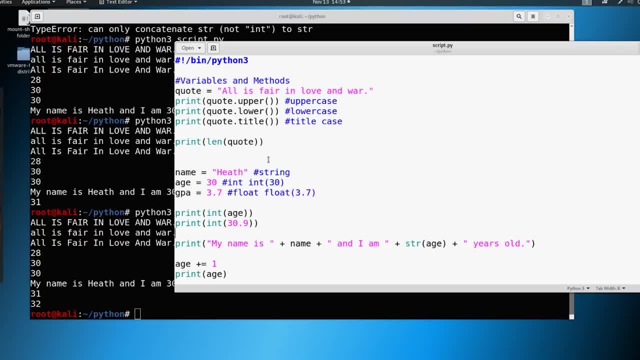 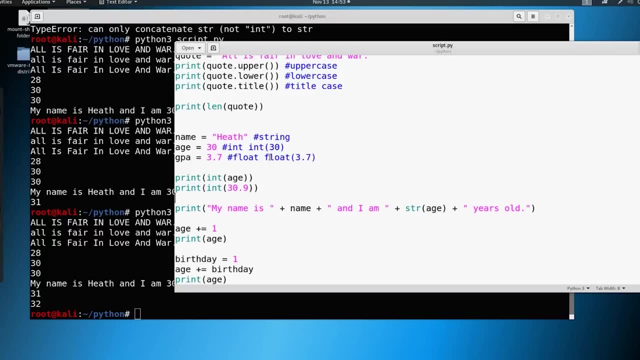 time on this. Take good notes, Practice, practice, practice. This is stuff that can get overwhelming very quick, But hopefully I'm explaining it slow enough and you're you're getting it. If you're not getting it, please do rewatch the video, please take notes And please utilize outside resources. 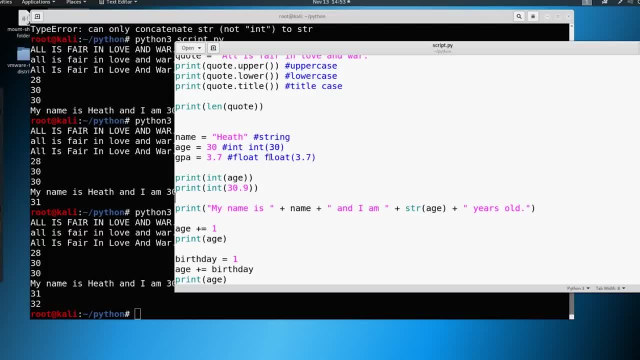 as well. I understand that I might not always be the best at teaching a particular subject, or sometimes it takes another person hearing it again from somebody else to see this. Coding is not necessarily easy, But once it clicks, it clicks, And a lot of it is just repetition. So that is it for this video. We've 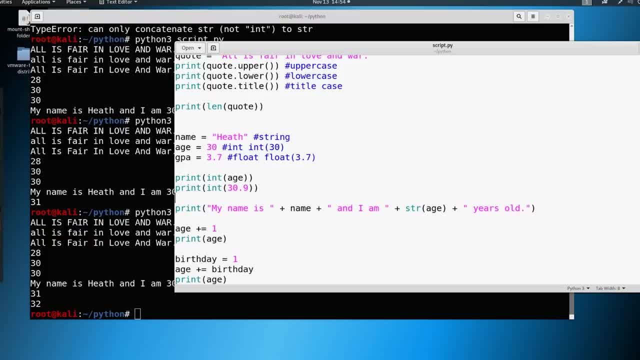 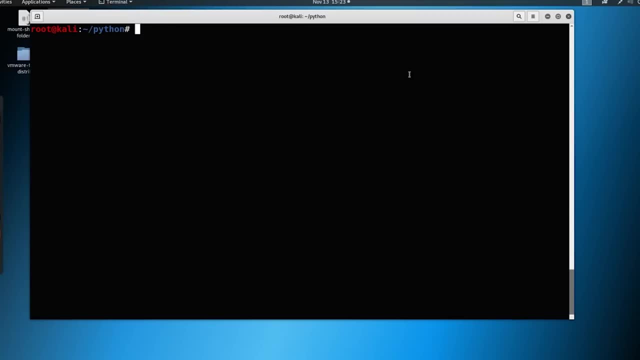 started to tie everything together. Now, from here, we're going to move into what are called functions and build upon all of this, So I'll catch you over in the next video on functions. All right, let's talk about functions Now. functions are what I like to think of as mini. 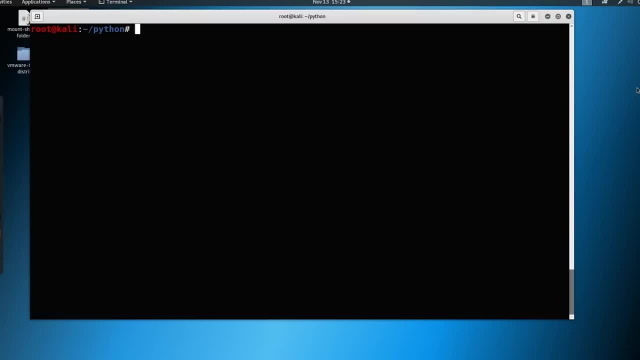 programs. It's like this organized block of code that you, you define and then you can call it later, and it makes it a lot simpler than typing everything out. So it's a lot easier to visualize this than me to just talk the theory of it. So let's go ahead and let's get our our script again. 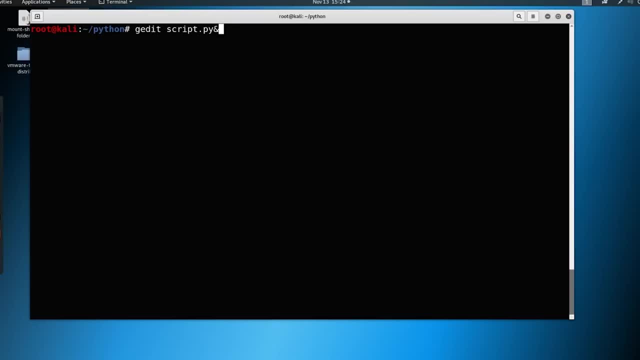 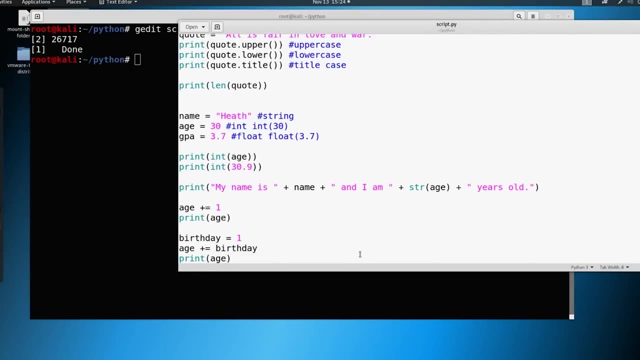 our script dot pi, and then we're going to ampersand this one this time And we should have our Python script from before. I'm just a scroll down to the bottom And I'm going to add in a new section here And that section is just going to be. 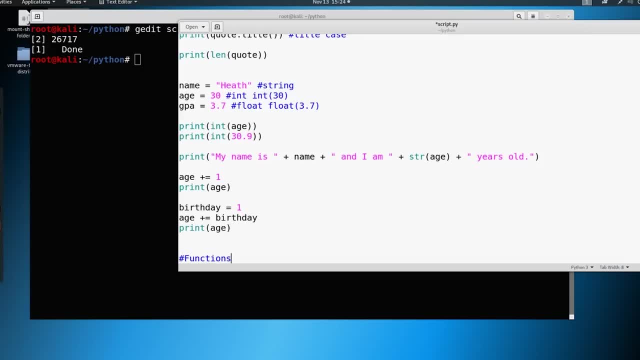 called functions. So if we want to print out, we can print out a new line to kind of put this together, And then maybe, when it's all said and done, we can print a function or make a function that just prints, and make it. 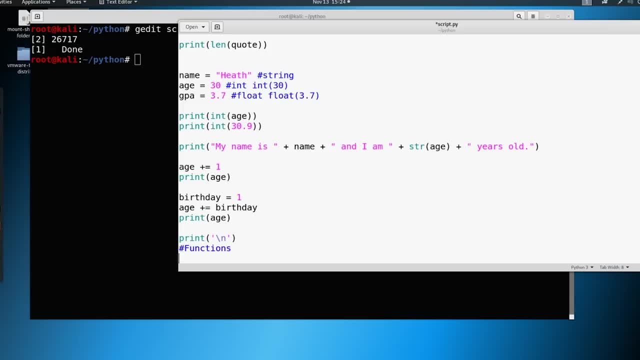 a little bit easier for us. So we're going to print a line here to find functions, And maybe we'll just print out something that says: here is an example function. So this is really just going to define the area. if we save it While you're typing yours, I'm just going to print mine. 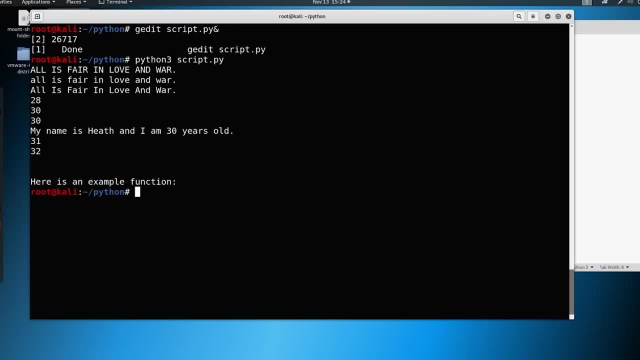 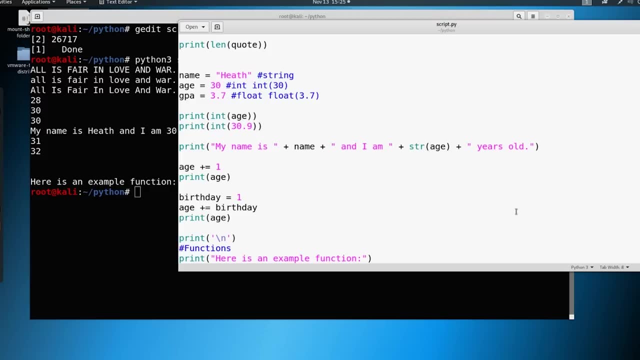 So we'll Python three, script, dot, pi And you see we've got the new line here And we see here is an example function And we just start from here. So let's take a look at a function using something that we've already done before. 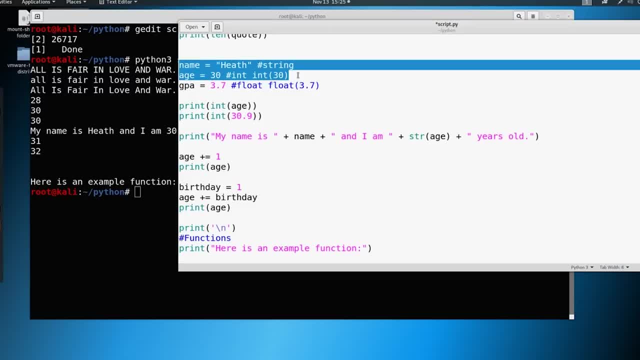 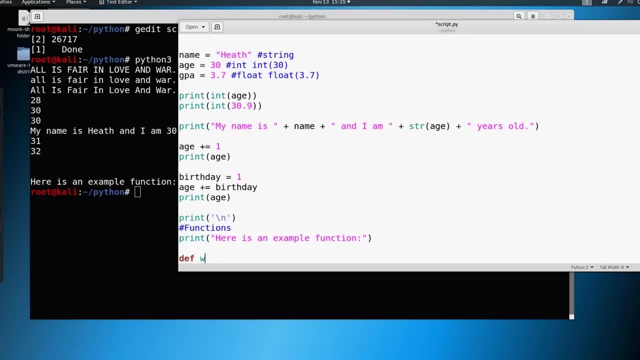 So we've got this section here and we've got name, age, GPA. we're going to kind of reuse this in this print: my name is, So let's go ahead and reuse this. we're going to say function here, right? So we're going to define kind of a Who am I? So we're going to define this And then we're. 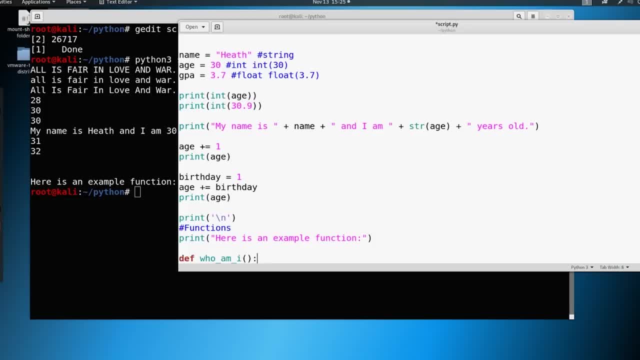 going to do two parentheses and then a colon here, So it's going to look like this, And what's important now is that we use indentation. Now, we haven't had to talk about indentation to this point, But Python is very, very critical on utilizing indentation, If you. 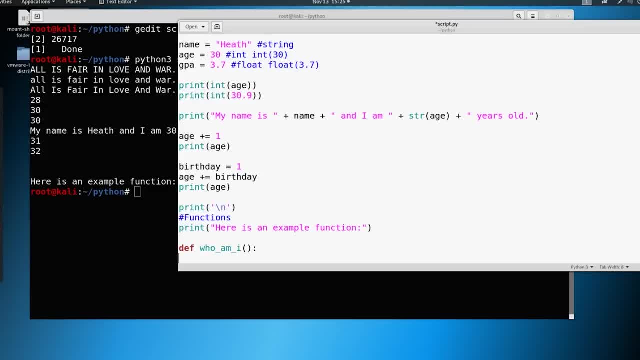 don't use it in the right places, then your program will not function. So it's very important to know when to use indentation and to indent properly. So to indent, I'm just going to tab here and I'm going to redefine everything again So we can just say: name equals heat. 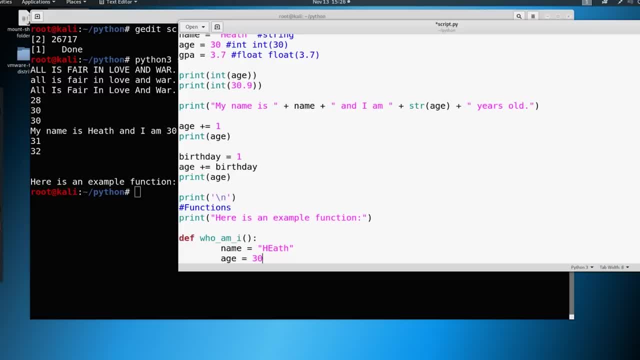 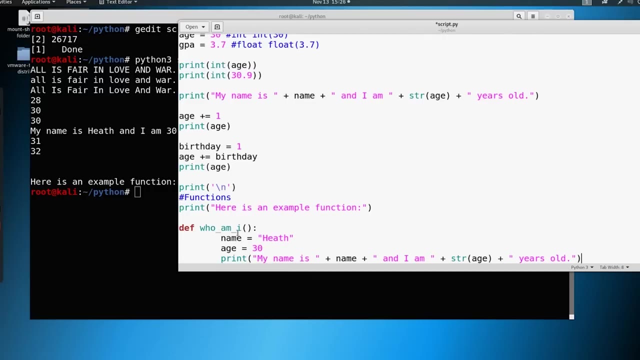 And we can just say: age equals 30.. type that wrong there and then we can just copy this print right here, So we don't have to type it all out again. just copy and paste it And you can see. define Who am I. And we're going to define in this function a name variable and a. 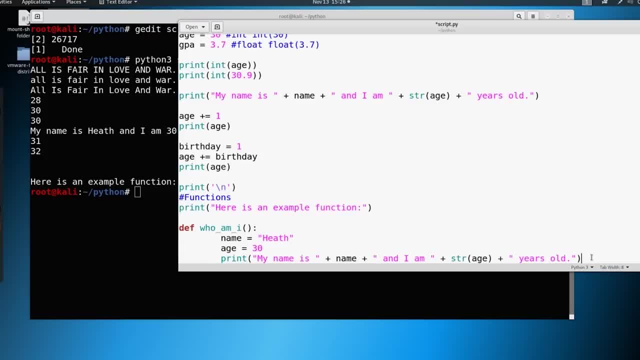 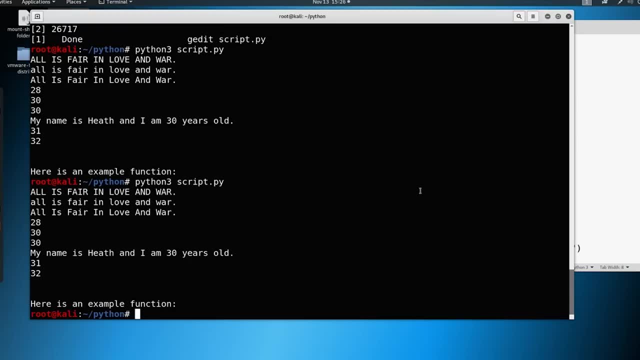 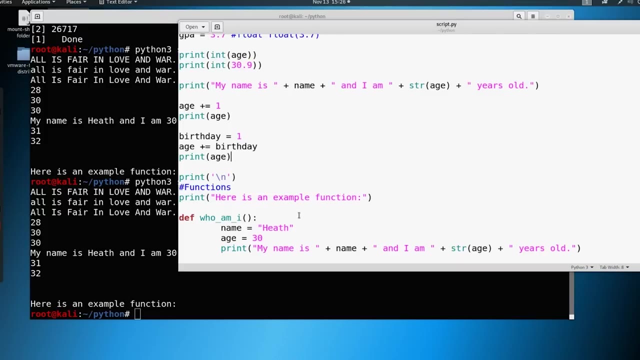 age variable, And then we're going to print this out. So if we were to just go ahead and save this and print this, nothing, nothing's here. All we've done so far is just define this function. we have done nothing to actually call it or or do anything. And let's make a note here that 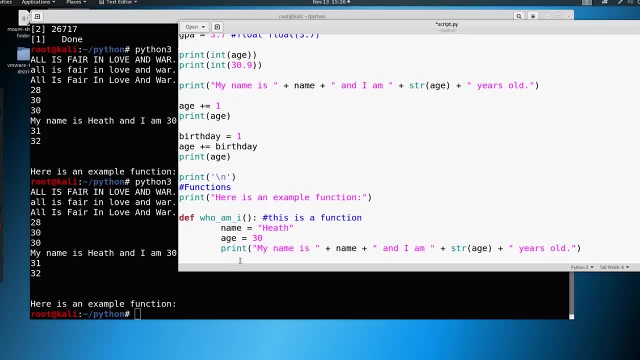 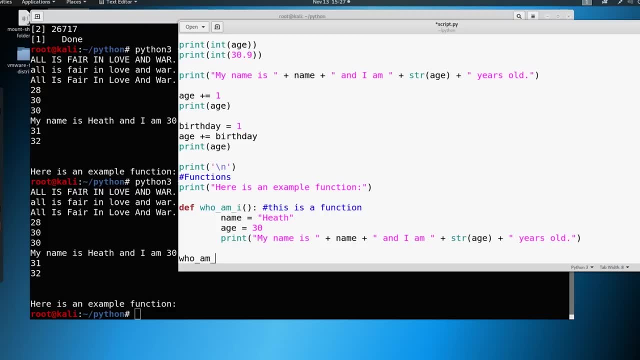 this is a function, right? So when we get down towards the bottom, let's go ahead and just try to call this function. So to call function. all we got to say is: Who am I? Let's go ahead and save this, run it again. 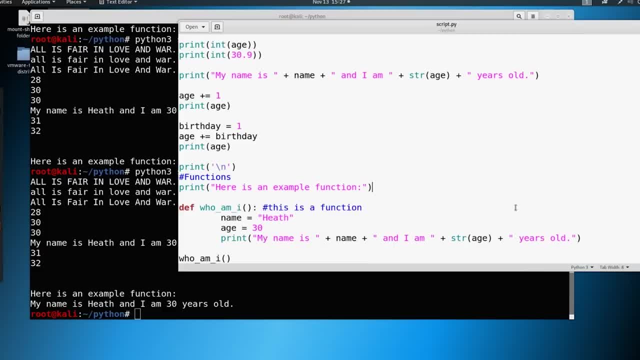 And look, it says my name is Heath and I am 30 years old. Well, what's happening here? Okay, so we're defining a set of things to do, right? This is a mini program And inside this mini program, we've defined our variables And we define an action here to take, which is printing. 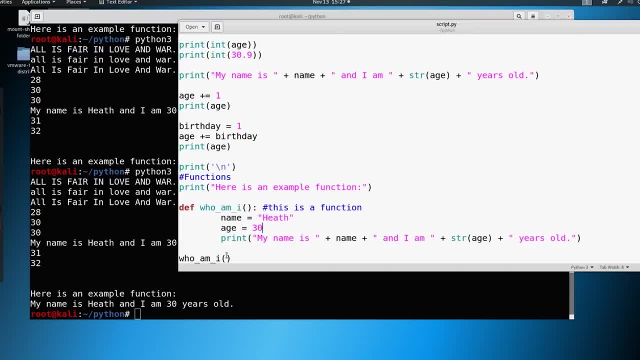 out this string. So what it's doing is, when we call this, it's saying: hey, I'm going to go ahead and take all this and I'm going to run this program and give you the result. Now what's important to know is: 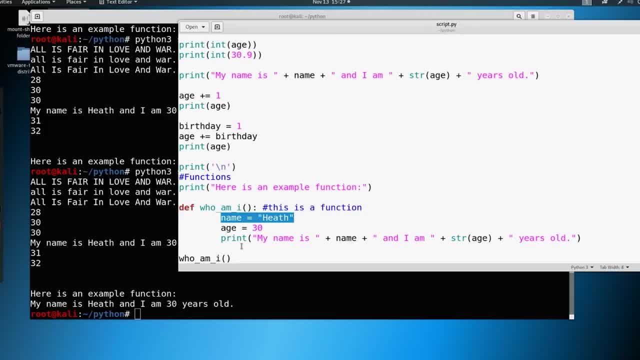 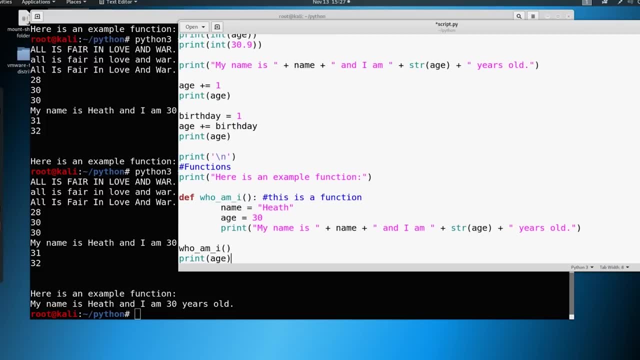 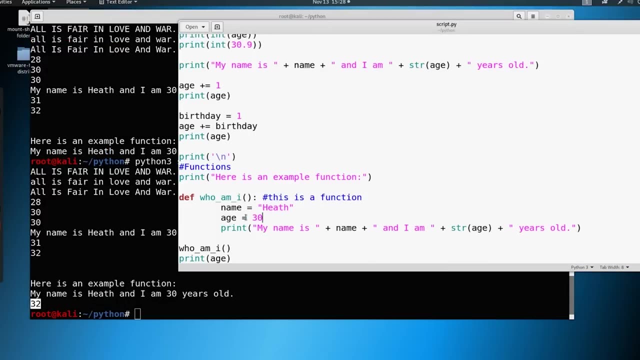 whatever is stored in these variables here is only stored there inside the function. If we were to print age from the last video, it should still be 32, I do believe So. print and you'll see: it's 32. Even though we declared age up here as 30. That only lives in the 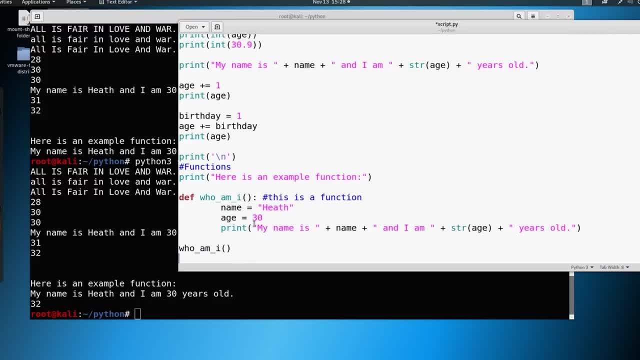 function. So I'm going to go ahead and delete this. So again, everything is living inside this function And it's a mini little program that we have here And we just call it at a later time. So let's go ahead and build out another function And we can kind of start to make sense of this. 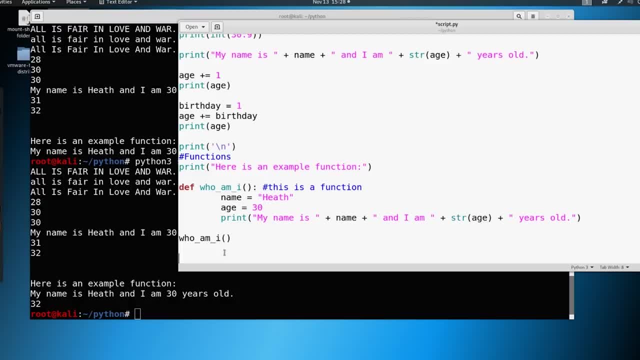 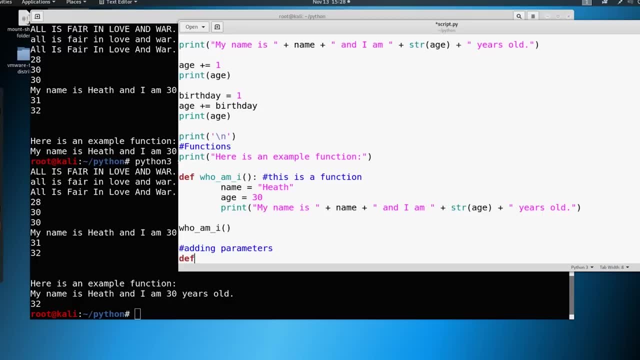 So let's start with adding what are called parameters, And we'll just do adding parameters here. So let's make a function, And this function is called add one hundred, like this: Okay, and then the parameter I'm going to actually add inside instead of giving. 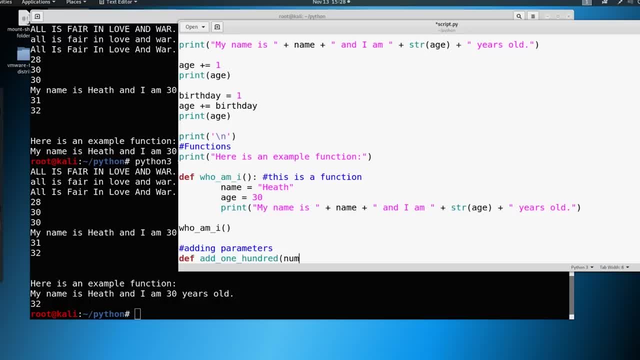 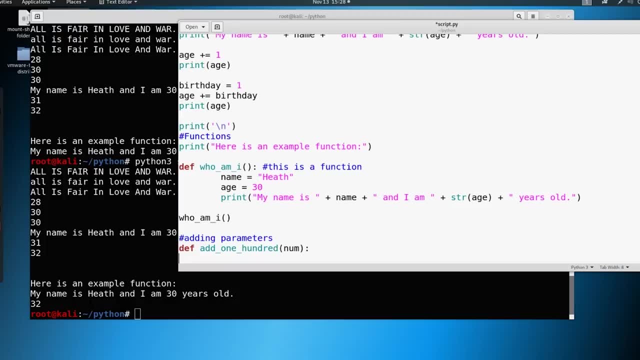 empty parentheses. I'm going to add in something called num- it's just going to be for number- And then we're going to go ahead and use our colon: hit enter, do a tab, And then what I want to do is I want to print number plus 100. So what am I doing here? I'm taking a number and 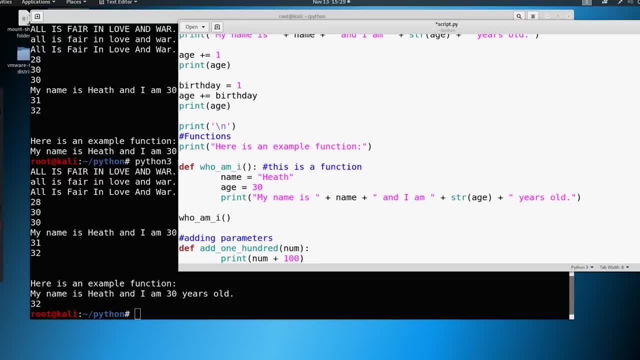 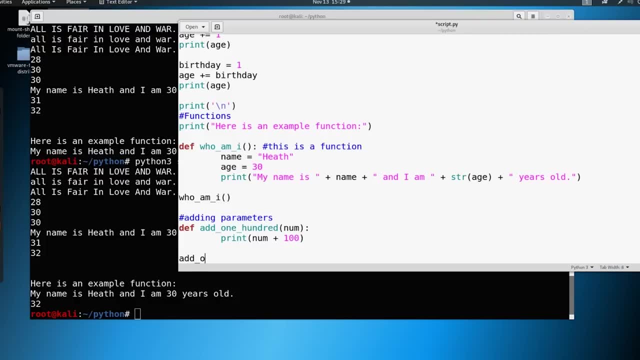 I'm adding 100 to it. So my function of adding 100 makes logical sense. Okay, so what's going to happen then if I say add 100? And then I specify a number in the parameter? Well, I'm going to say: 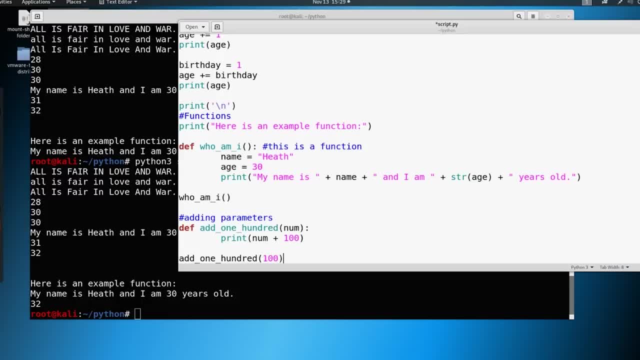 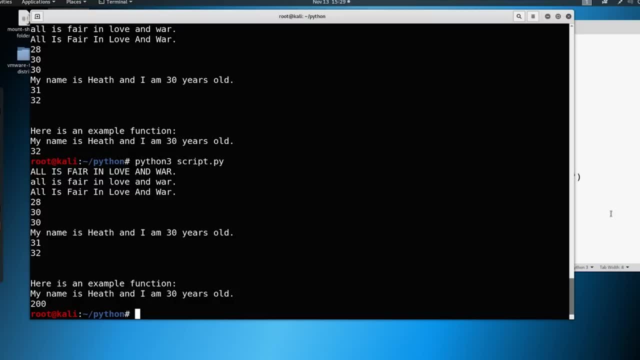 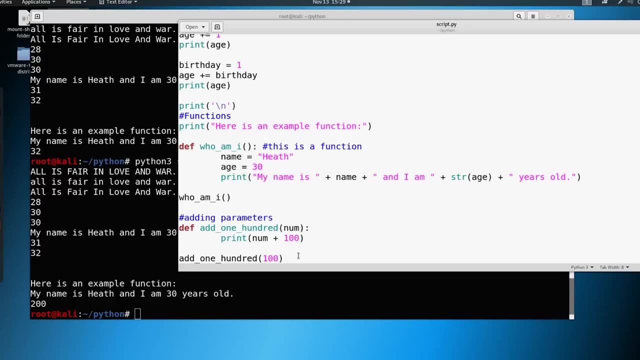 what if I want to add 100 to 100?? Well then, I should, in theory, print out 200, right? And there you go: we have successfully printed out 200.. So we can build upon this even more. So what if we want to use multiple parameters? Okay, 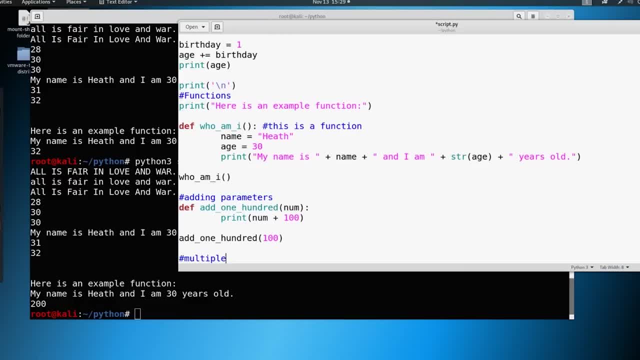 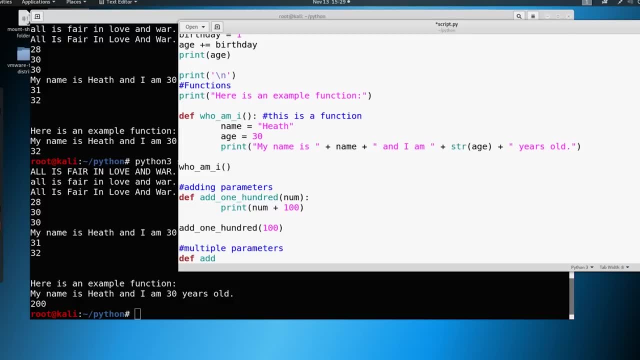 let's say we want to do multiple parameters And we want to define an add function. we're just going to make an add, even though it's built into Python, we're going to make our own. So we're just going to say: add x and y. So now we have two parameters here. Okay, we're going to add our colon. 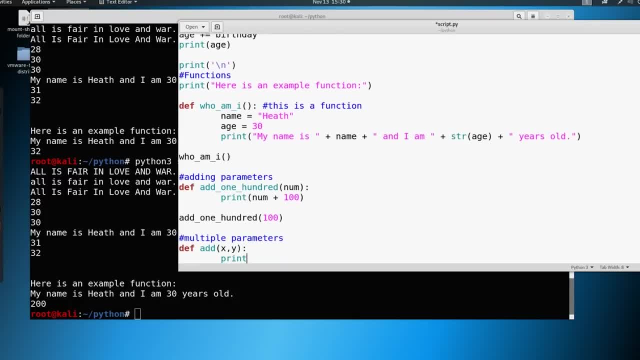 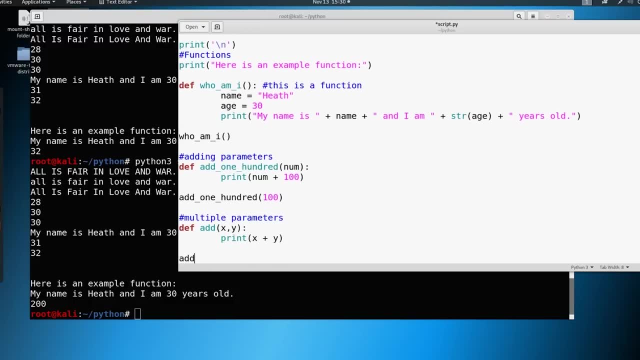 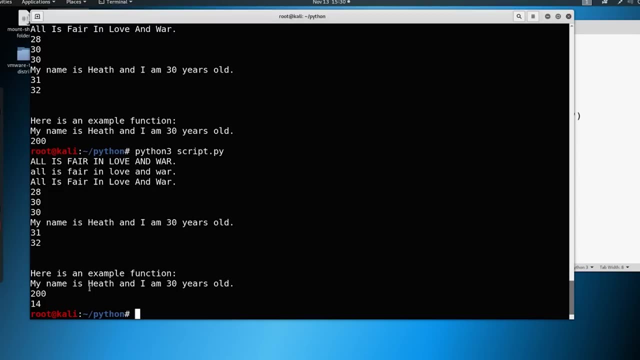 make sure we indent and then we're just going to say print x plus y. Now if we go in and we add seven and seven, we should get 14. And there's 14.. So hopefully this is starting to make sense. All we're doing is building these mini. 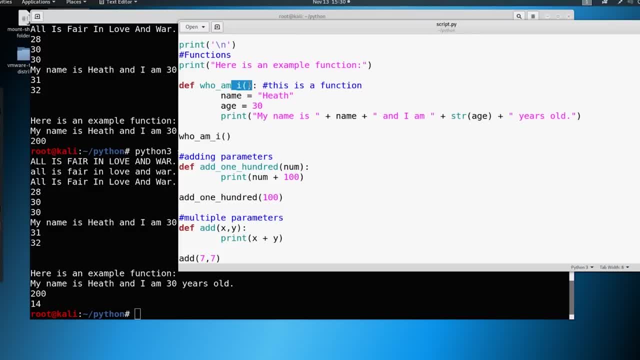 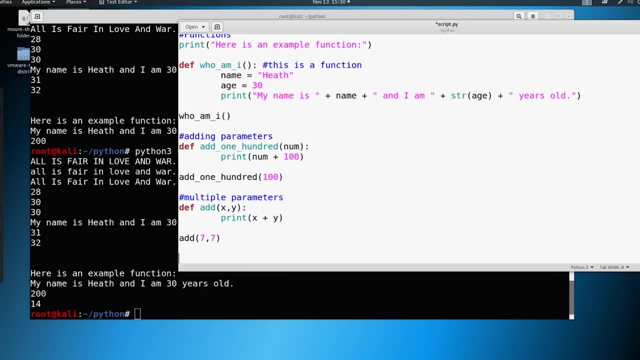 programs And we can have no parameters, as we saw up here. we can have single parameters or multiple parameters, depending on what we need. So let's go ahead and build a couple more out, just to make sense of it. So what if we wanted to define multiply And we'll just say x, y again, what do? 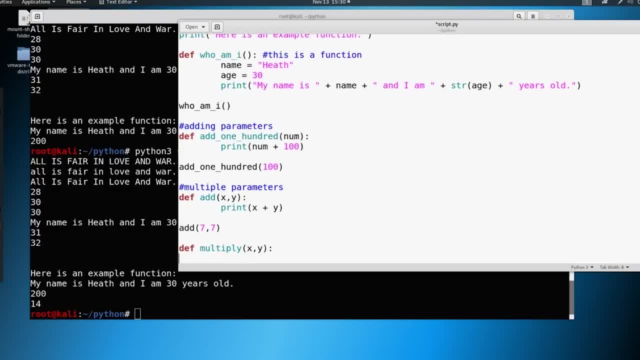 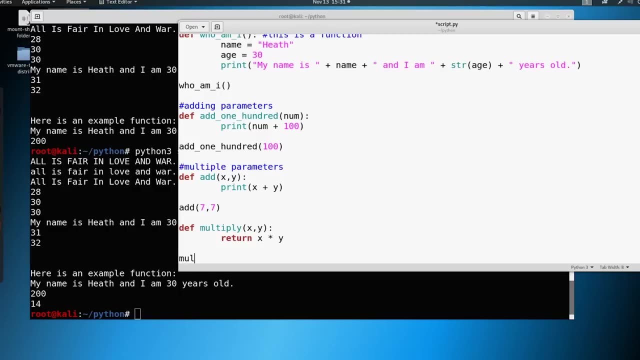 you think that's going to look like. Well, instead of saying print, what if we say return? I'm going to throw something new at you. I'm going to say return x and y. Okay, Now what happens if I call multiply And I say seven, seven again. what happens here? 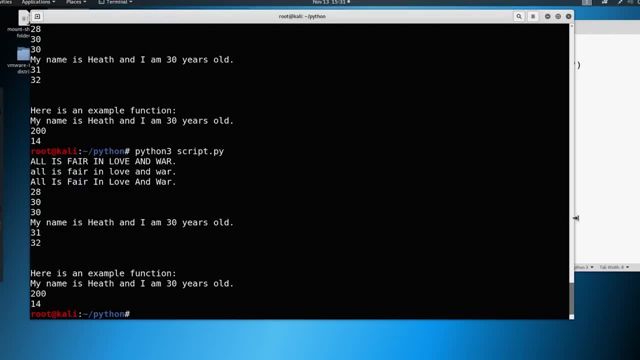 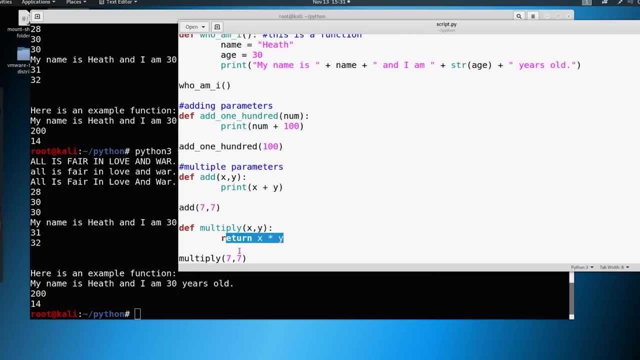 Let's go ahead and save it. Well, nothing happened. We're not printing out to the screen, all we're doing is returning. So when I'm pulling this multiply in, it's returning a certain number. So I'm calling it here And it's saying: hey, seven times seven, that's 49.. 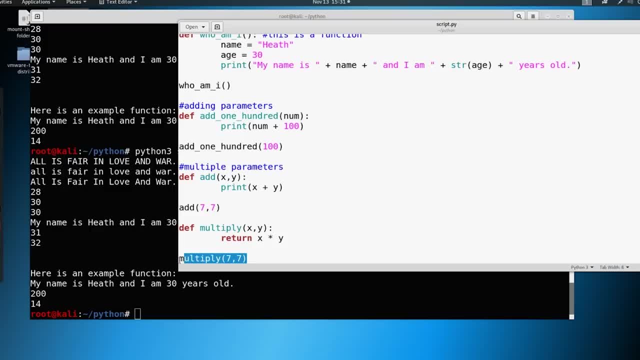 But I have no idea what you want me to do with it. Now I can say: print multiply here And then we can see what happens. And now you see it's 49. So the return feature just allows us to return the number that is back to us, right? We don't have to always print it out If we don't want to. 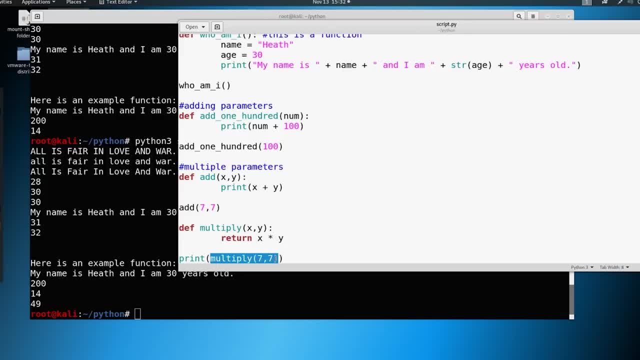 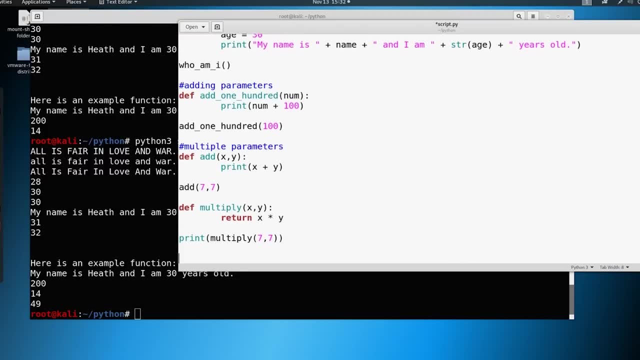 we can store it for later. So that's what we can do here, So we don't always have to print it. we can. we can return the number and then call it later. So that's one way of looking at it. Let's do one. 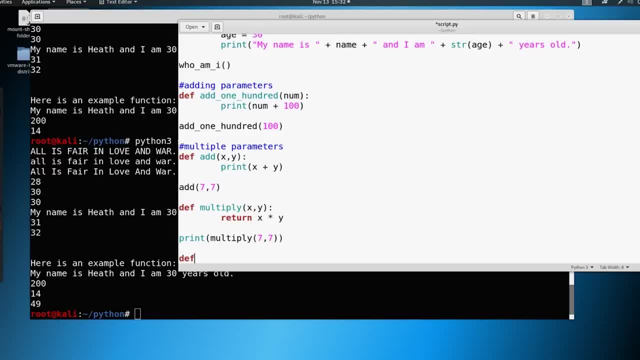 more. How about we define square root? And we only take one number here. So how would we do the square root of something? Well, let's go ahead and just print out x And then we're going to do by point five- remember the exponent with two multiplications here. 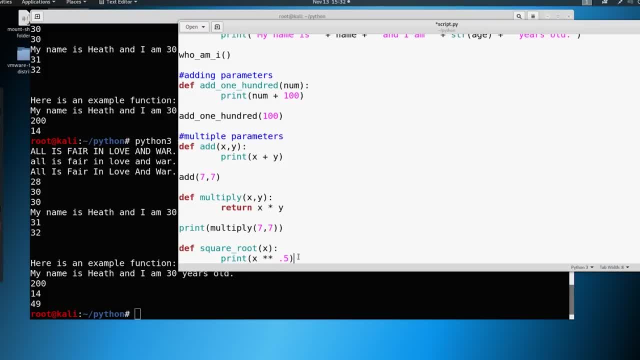 And then we're doing the square root. So we're going to take point five instead of squared, which would be two, right? so we're taking the square root, do point five. And let's take an easy one: let's return the square root of 64. So let's say square root of 64. And see what happens. And a return. 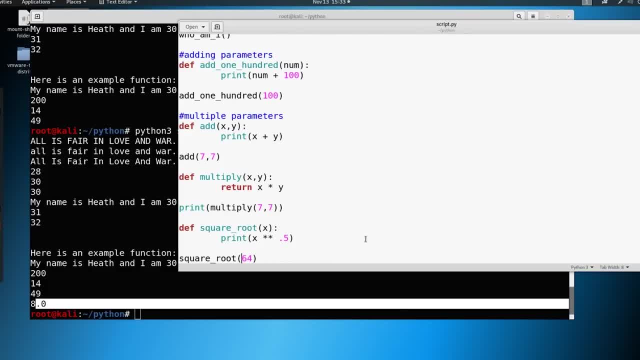 And then we're going to take the square root of 64.. And this returns eight for us. Now we can make that integer if we want to and go from there, But that's just a nice base example. So, lastly, I mentioned that we can make a function for a new line because we've been sitting in here. 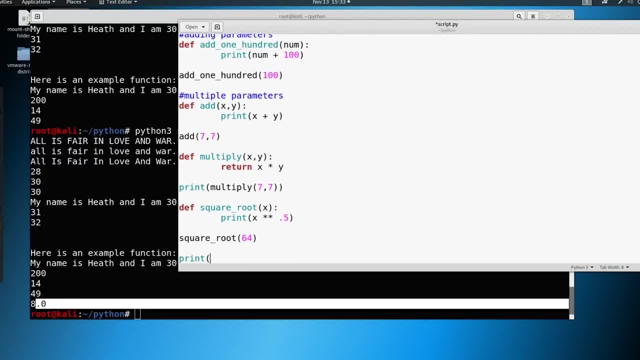 And we've been just typing print And I am slow at it. I have to sit here and think about it, And then I find the correct letters And this is how you print new line. Okay, I'm not the best at it, but what if, instead, we just did something like define new line and then we just put this here? 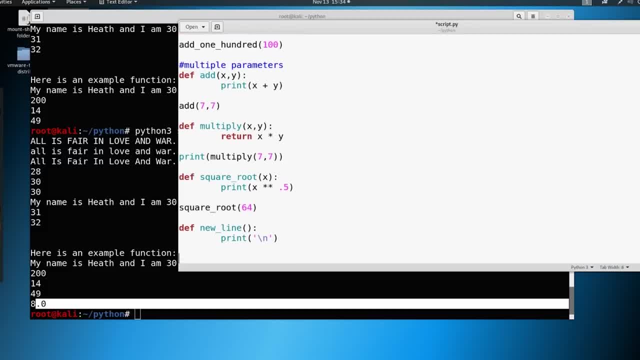 so then we can just call a new line from here on out. we could say a new line and then when this prints, it'll print out a new line, and while it's the same kind of length ish of this, we don't have to type in these special characters. look for them. we could even shorten this to like nl. 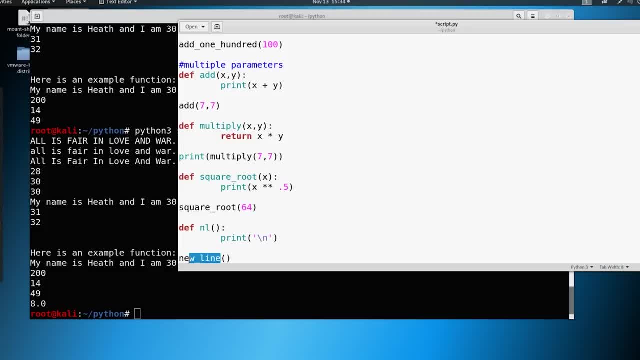 something like nl and then make it really simple, and then we save time, and this is where these programs come in and they save time. so good example of a use of a function. so i'm going to save this if you want to use this for moving forward and going on in the next videos, absolutely. 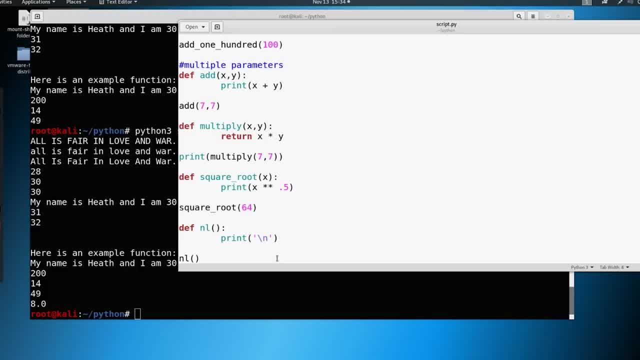 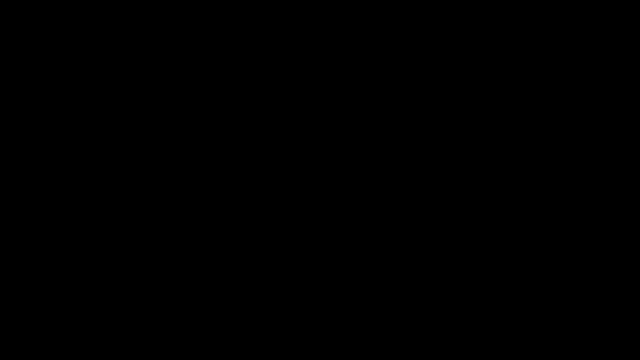 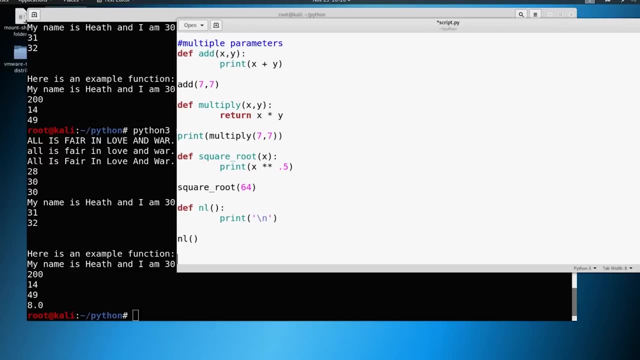 welcome to. so if you're following along, go ahead and just leave your text editor open and i will catch you in the next video. bye, bye, you over in the next video. as we start to talk about boolean expressions, welcome back. so now we're going to discuss what are called boolean expressions and we can go ahead. 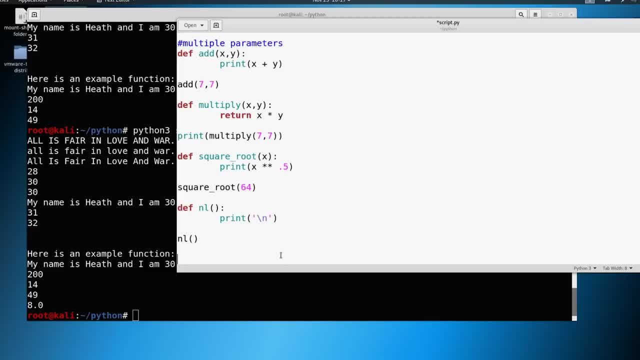 and just type this right into our text file. if you don't have your file open with gedit, go ahead and get your scriptpy open, and what we're going to do is we're going to just put in here boolean expressions, and now when we say boolean expressions, we can just think of this as true or false. 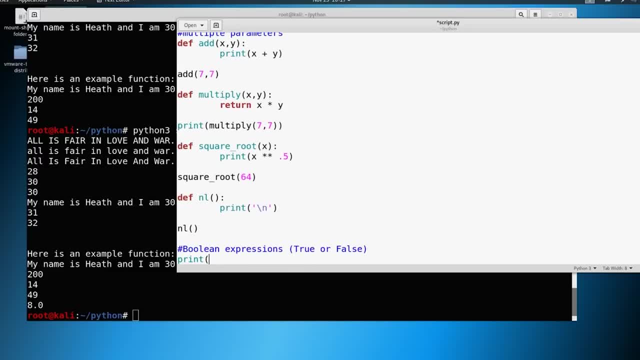 so let's go ahead and print our new subject line. we're just going to call these boolean expressions and from here let's start defining those. so let's say we have boolean expression one, we'll just call the variable bool one. now let's just set that equal to boolea expression one and we're just going to go ahead and print that one and we're going to 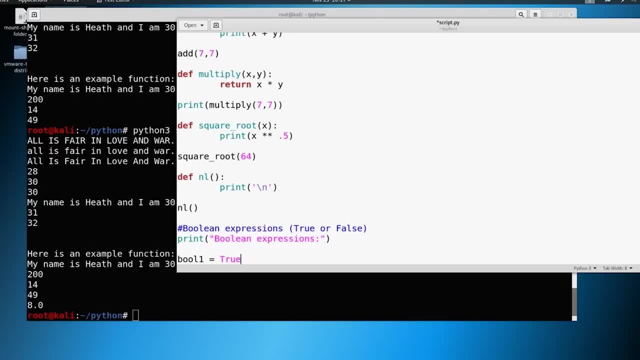 to true. Okay, And let's give an example of that as well. Let's just say Boolean, two equals. let's say three times three. Now, what does three times three equals? Well, that equals nine. So we can say: equals equals to mean something equals something, And so this number 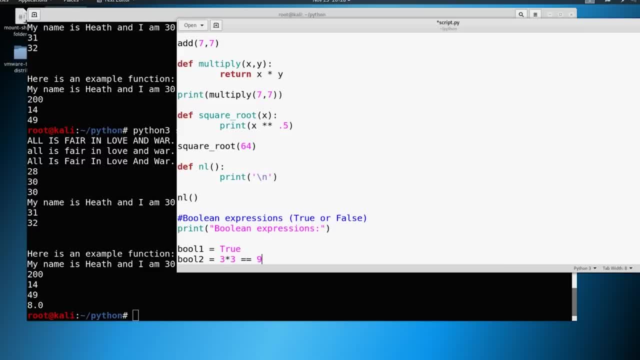 equals this number. So three times three is nine, which equals nine. So if we take this expression and we say nine equals nine, it's going to return true. Let's do a couple more So we could say: Boolean three equals false And Boolean four equals three times three. 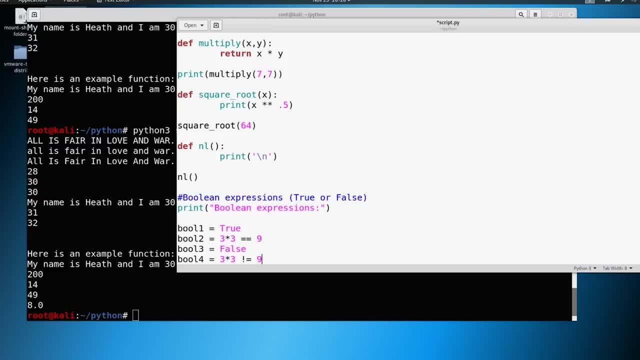 And then we can say: does not equal nine. Well, that's not true, right? So that's false. So if we were to print these all out, we could say: print Boolean one, Boolean two, Boolean three and Boolean four. Okay, and let's also print the type. So we know. 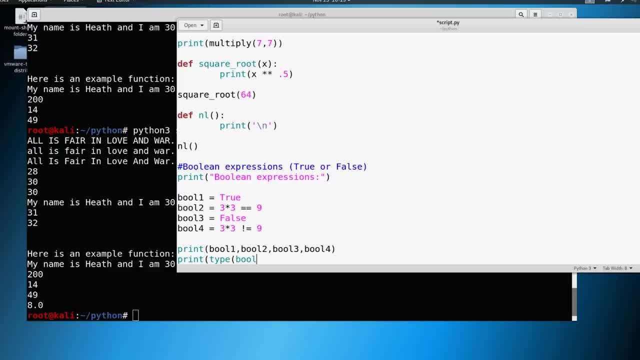 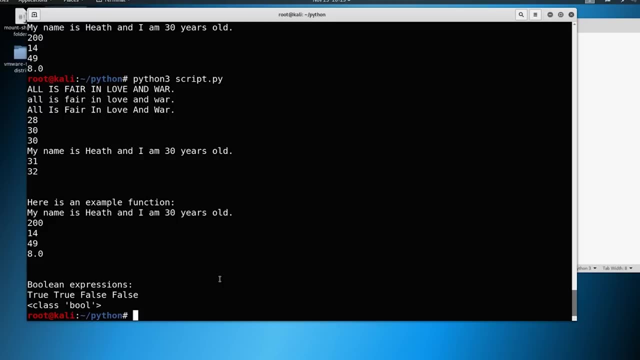 about this. So it's a print type And let's take a look at what this looks like. So once you have that all written out, go ahead and just save this And go ahead and run your file And you can see that it came out exactly how we thought. 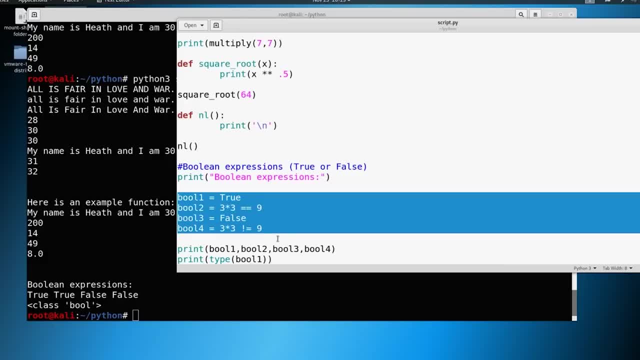 it would. So we've got four variables and they're all Boolean expressions, right. So we've got true, this equals to true, this is false And this is equal to false. So we see true, true, false, false. we print those all out And then, when we want to look at: 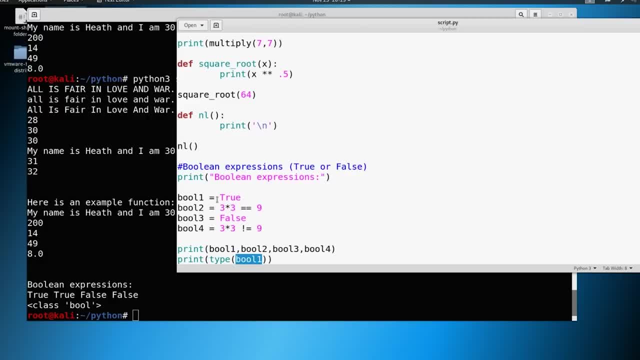 the type of the variable. So we say, hey, what's stored in here, inside this variable, what's stored is a Boolean. Now, please do note that there is a difference between true and true. One is a string and one is a Boolean. So if you were to set Boolean five, for example, to true, and then you printed: 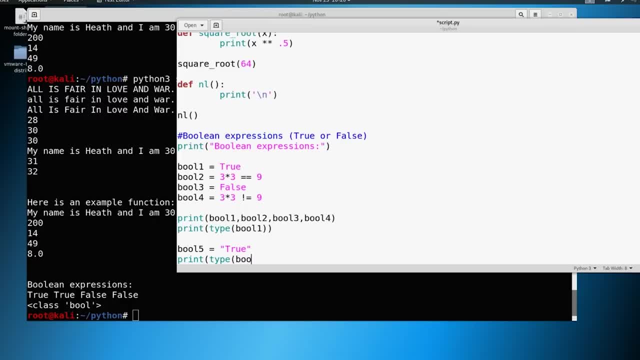 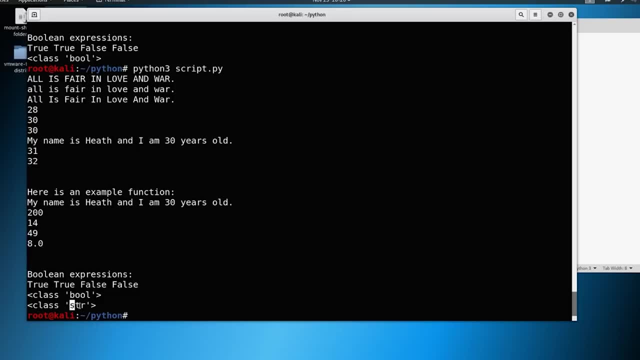 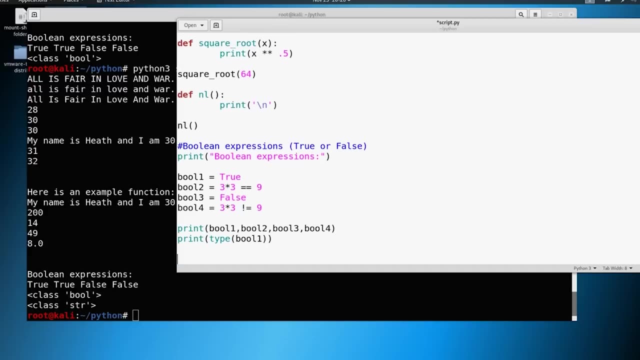 the type of Boolean five, then you're going to get a different result here. You're gonna see now that the type is a class of string. So big difference here. I'm going to go ahead and just delete this. So this is just an overview of Boolean expressions. We're going to use this later on And you 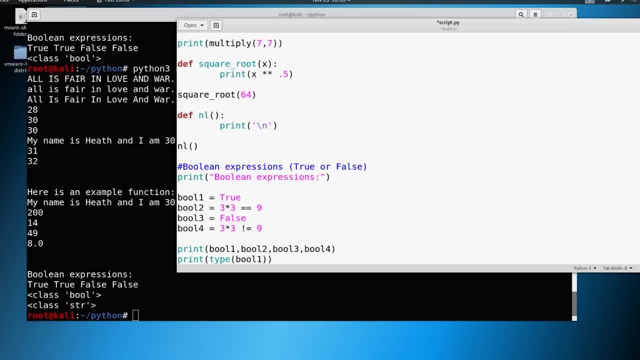 will see it again when we get into exploit development. But you're going to see certain things especially when we get into loops as well. So once we start getting into looping and we talk about that, it'll make a little bit more sense. 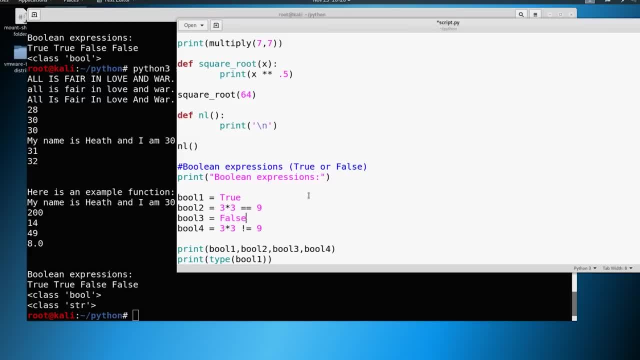 sense, But you want to know sometimes if something is true or something is false, Or when we get into conditional statements: if something is true, then do this, Or if something is false, do this. we haven't gotten quite that far yet, But we need to introduce the concepts before we can. 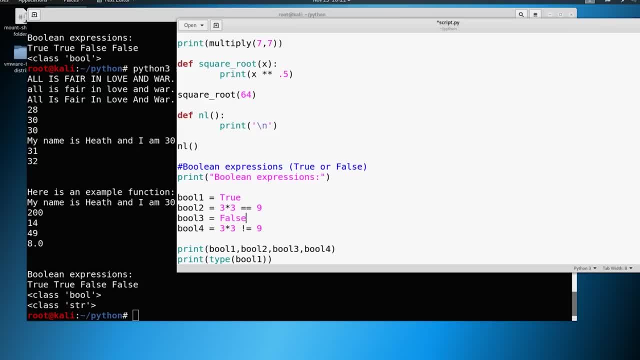 build upon it. So we're going to do in the next video is we're going to build upon these even more. we're going to take relational operators and these Boolean expressions and kind of combine them and start building upon it And then, once we get this all put together, it'll all start making. 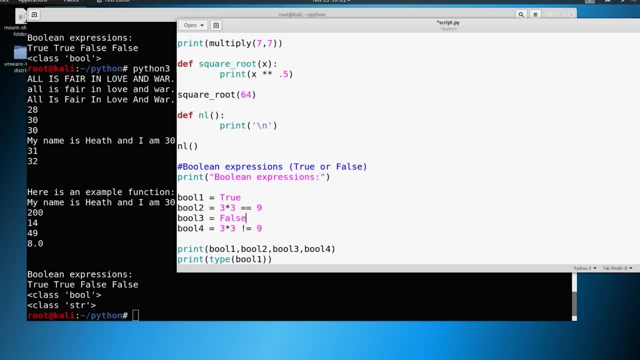 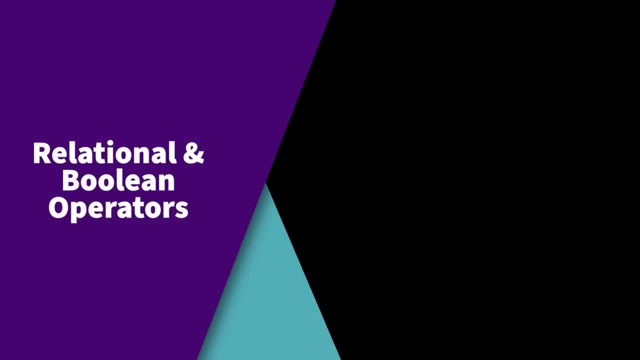 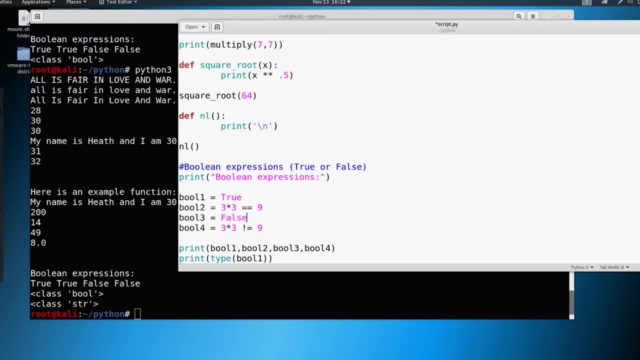 sense. So for now, all you need to know is when I say Boolean expression, all I'm thinking about is true or false, So we'll build upon that in later videos. Okay, let's build upon where we just left off with the Boolean expressions. So now let's talk about relational operators and Boolean. 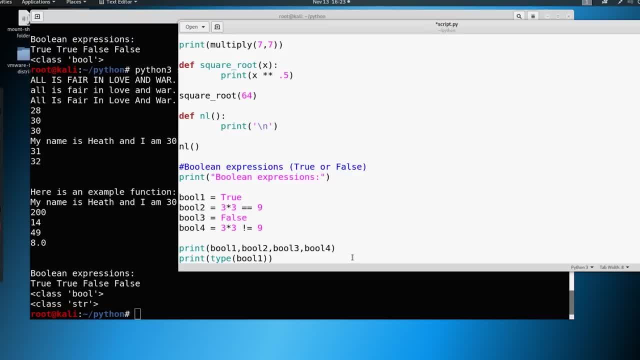 operators. So what do we mean when we say operator? let's go ahead and just add a new section here And we'll just say relational and Boolean operators. if you want, you can go ahead and just put a new line here. So remember, we specify a new line and a function And let's say greater than let's define. 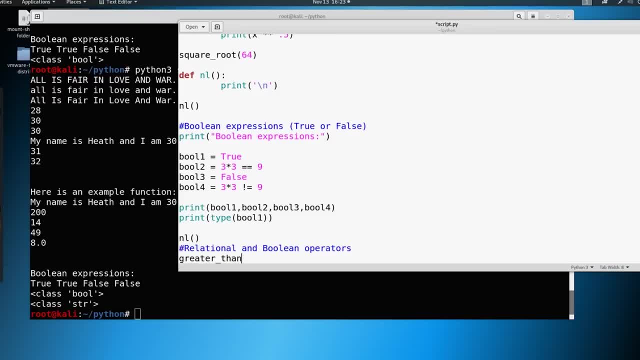 a variable called greater than, And let's just make that equal to seven is greater than five. Okay, so we're using a operator here with the greater than symbol right And we're also using a Boolean expression, because when we say seven is greater than five. well, that's going to come back. 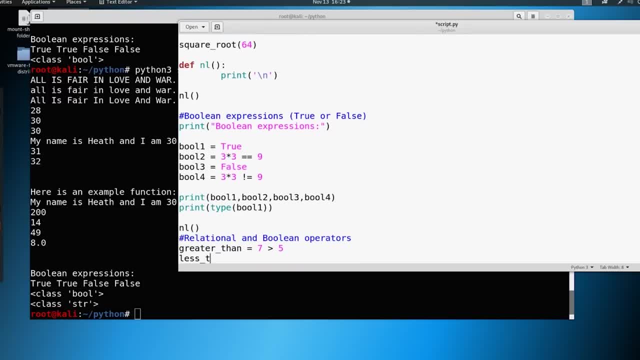 with true And we could say less than. we could say five is less than seven, And that's also going to return true. What about greater than or equal to? we can say seven is greater than or equal to seven, And that's going. 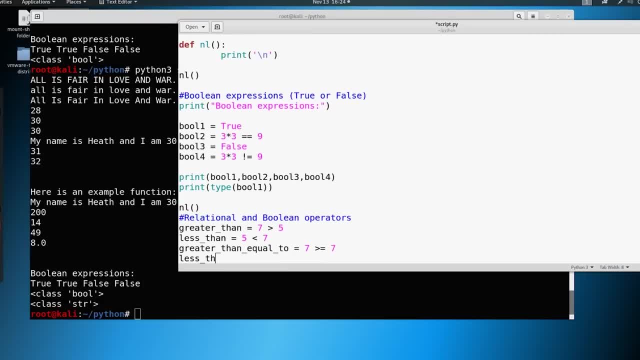 to return true as well. And then, if you can think of less than or equal to, it's going to be very similar. we say seven, less than or equal to seven, And that's also going to be true. So if we were to print all of these out, which we don't have to, they're all going to be true, So we're. 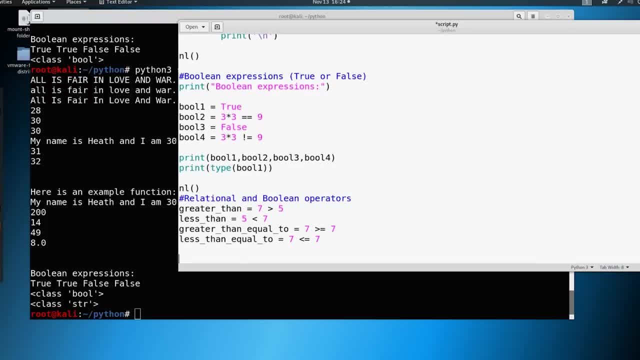 all going to return back, true? So there's other things that we can add in here. So what if we bring in multiple operators? For example, we could say test, and you can call this whatever you want. So what if we say seven is greater than five and five is less than seven? So we see here: 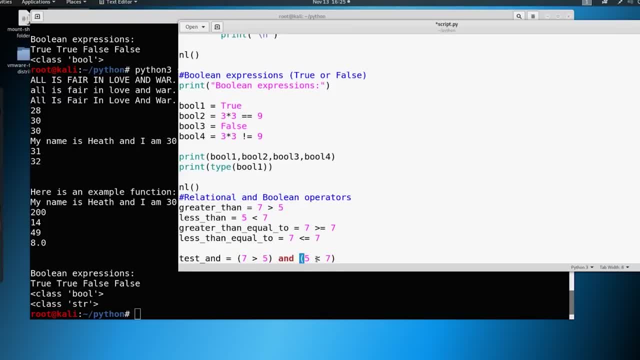 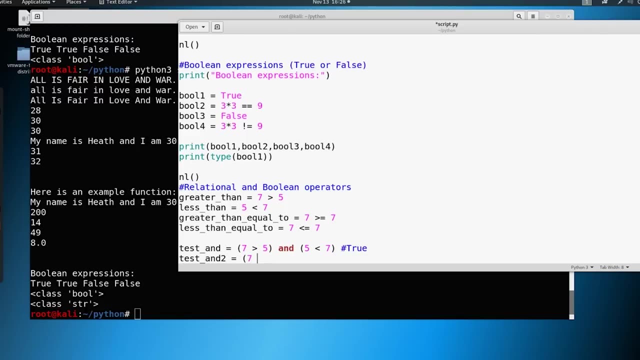 that this is true And this is true. that would make this entire statement true. So we could say true here If we were to say: let's just call this test And two. we were to say seven is greater than five, which is true, And five is greater than seven. Well, that's not true. So this whole 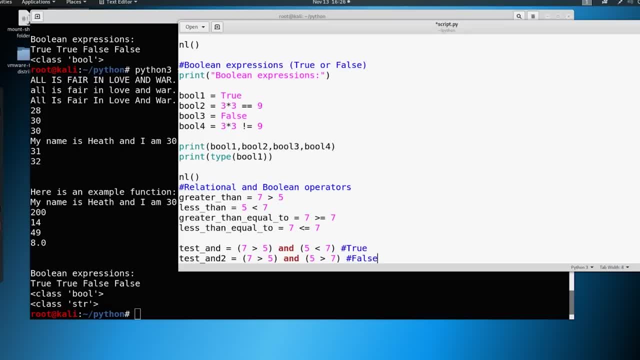 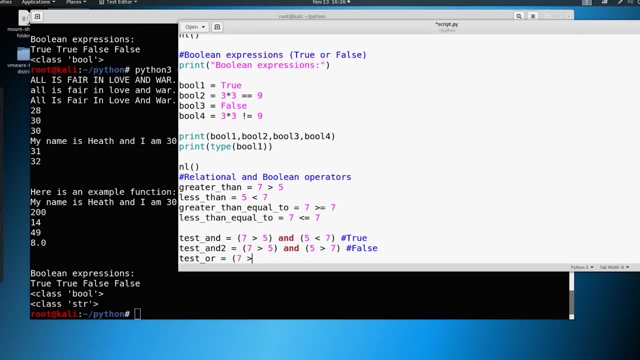 statement is going to be false Because we're going to say and and is very important here, right? What if we were to say something like, or, though, if we were to say: let's test out. or we could say: seven is greater than. 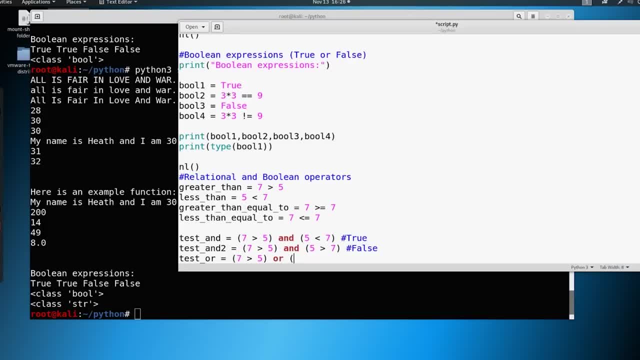 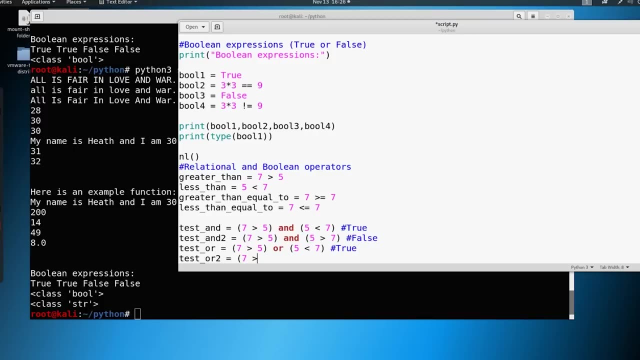 five or five is less than seven. Well, this is going to return true. And if we were to do the same thing as we did above, where we say test or two and we say seven is greater than five or five is greater than seven? 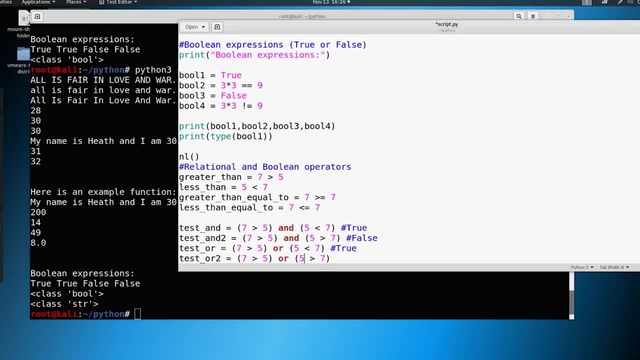 I forgot my parentheses here And this is also going to return true. Why? Because only one statement has to be true here for these both to be true In the instance of, and both statements here have to be true in order for it to be true. If one of them becomes false, the whole thing. 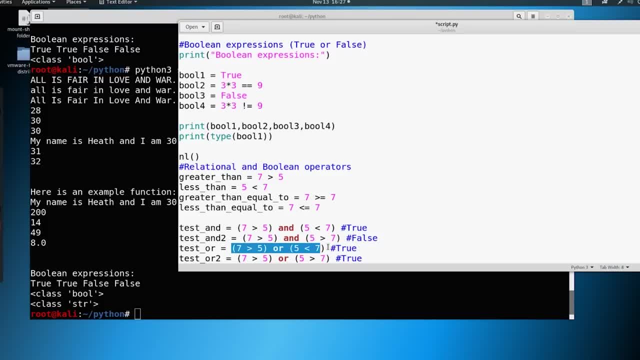 becomes false In the sense of: or or the case of or. if both are true, it's true. If one or the other is true, then it's true. Both have to be false for it to actually return false. Okay, So you can print. 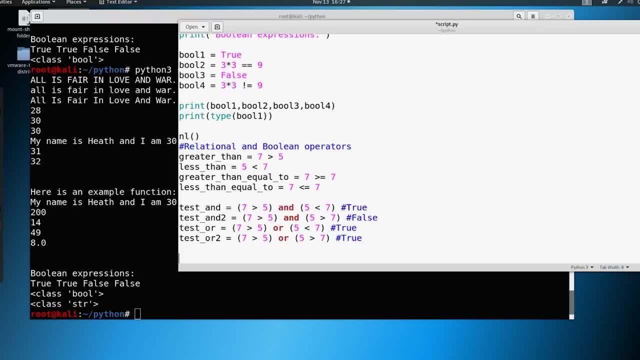 these out as well, to test this out. The other thing that we can say is we could say something like: test not. we can say something like not true. And guess what? not true is going to be false, And if we said not false, then that'll be true. So 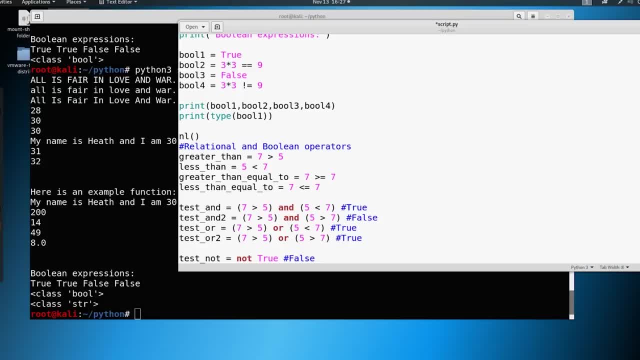 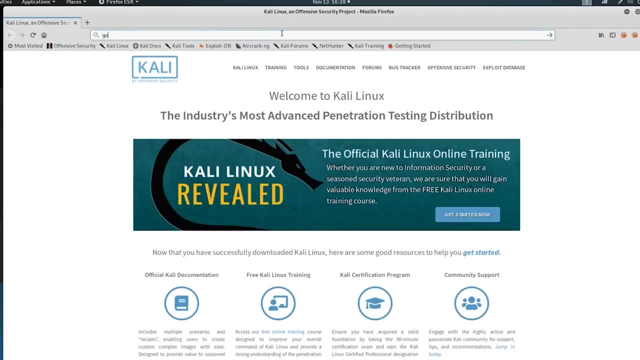 these are the ones that can start to kind of get confusing. So again, my recommendation is to make good notes on this and then go out and study it. And there are true false charts. Let's just see if we can Google one quickly. There are true false charts online. we could say: true, false chart. 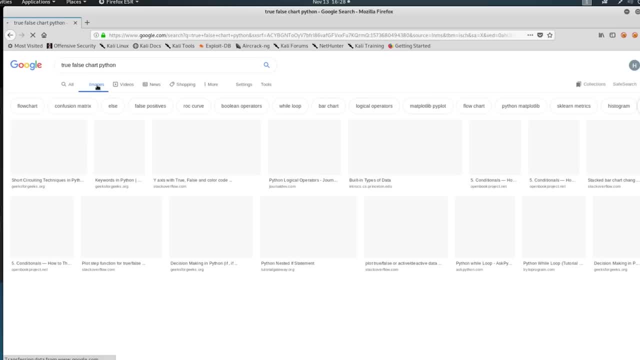 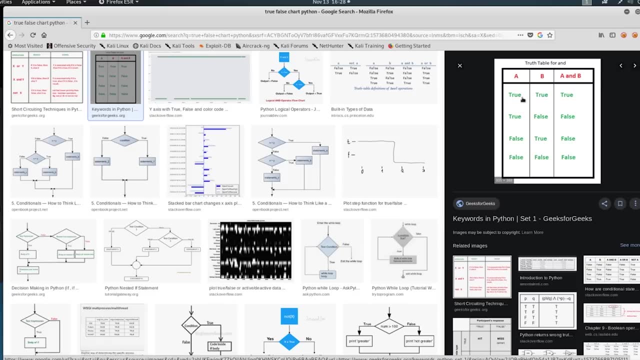 and go to images And we can see truth. tables is what they're called. So if A is true and B is true, the A and B are true. If A is false or true and B is false, then they're both false. False, true is. 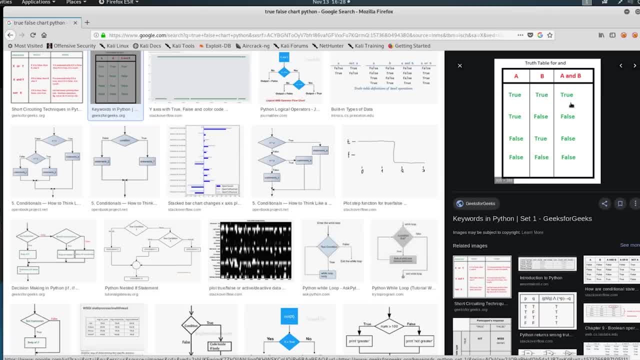 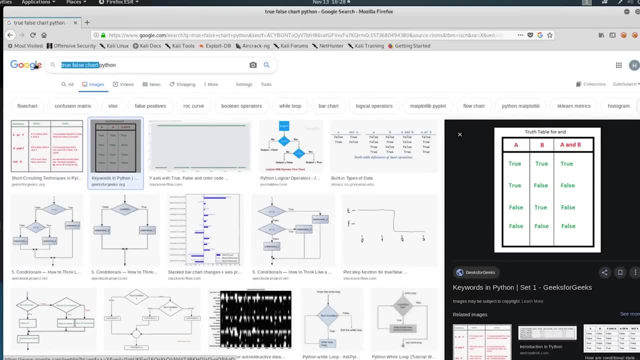 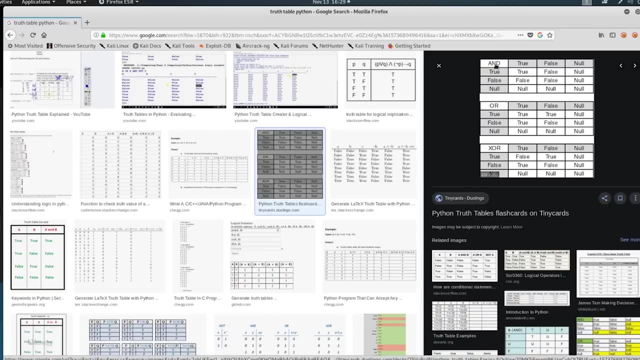 false and false. false is false. So, in order to have a truth table for- and everything has to be true. So if we search truth tables, that might give us a better chart here, And then you get something sort of like this: where you have and where you see a true, true is. 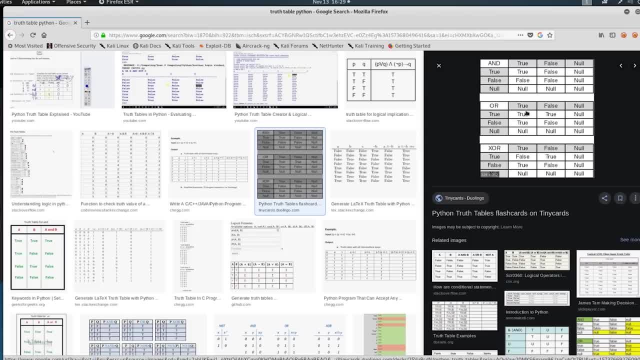 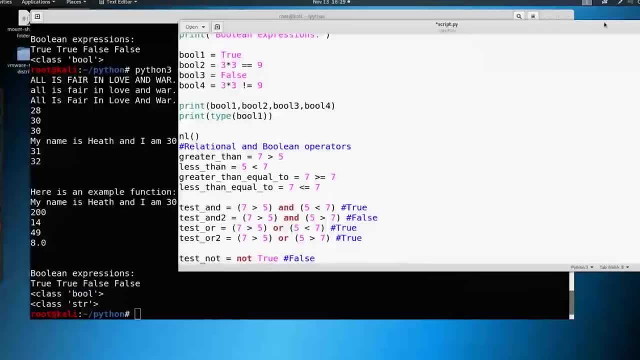 true You have, or where true false is still true, And then XOR we don't have to worry about right now. So take good notes on these, make sure you understand them. we're going to continue to build upon them over time. Really, all you have to think about, though, is you have to think about 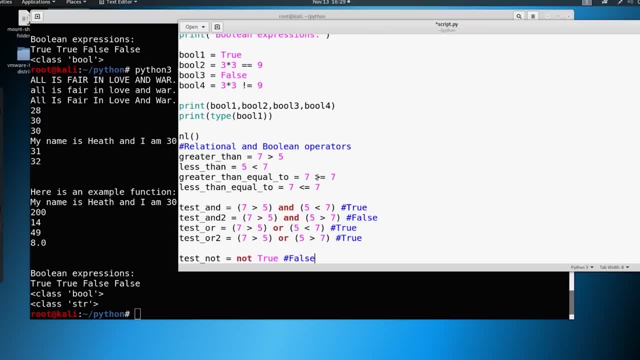 so you have to think about the definition of a truth table If you want to avoid the use of Myth. it's going to also be difficult to just say that you don't have a truth table. Let's go on, Let's take a look at some of the different definitions of truth tables, and I'm going to 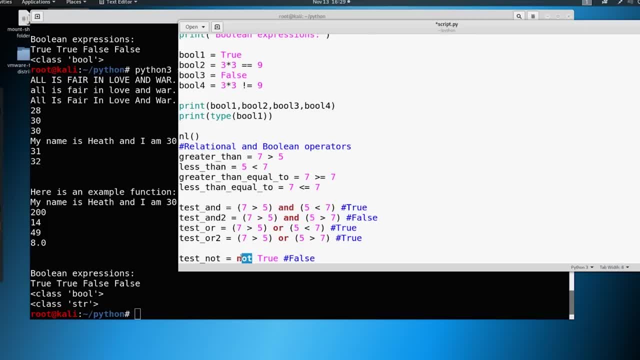 talk a little bit about them. So if I were to look up just one of the great ones about Boolean operators and these expressions And the most important things to take away from this are not just the true and false, But the greater than symbols, the less than symbols, all these different. 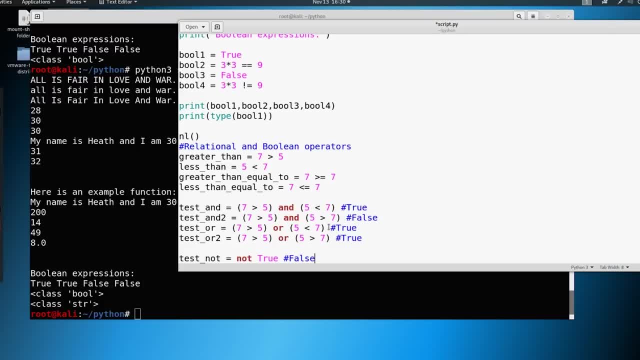 being able to develop- And I've said this before, I'm going to say it again: being able to read and understand what is going on is super important, being a developer not as important. So as long as you see these things and you see a true or you see a statement like this when you're reading, 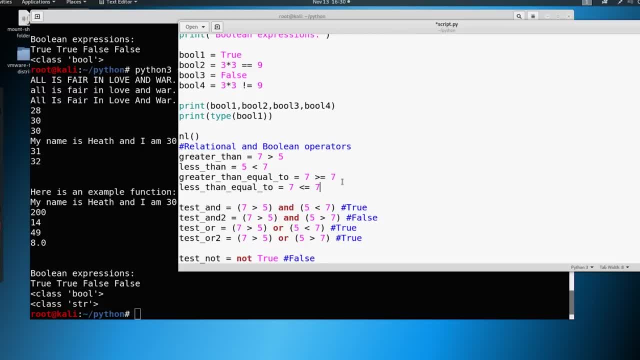 code and you say, Hey, I know that's a Boolean operator, I know it's true or false, And I kind of understand the truth tables Right. So that's really what we're after here. So, as long as you start getting this understanding and this comprehension, that's really what we're after. 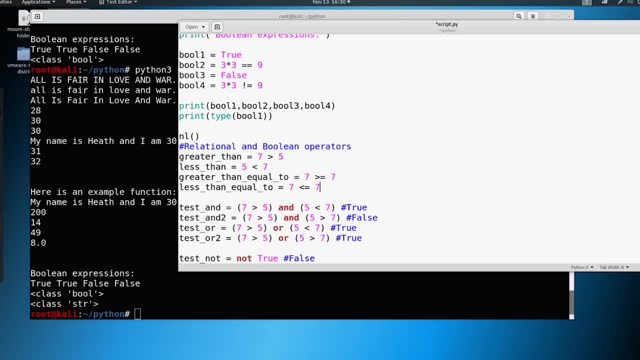 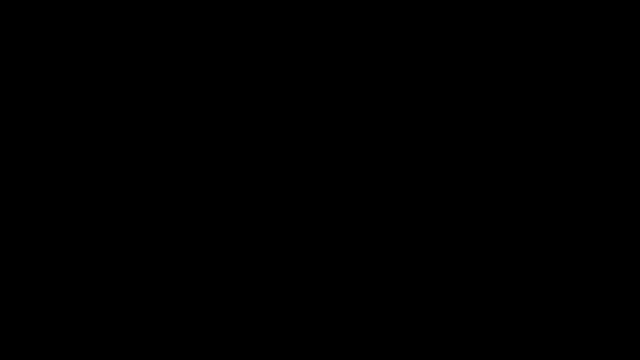 So from here we're going to move on And we're going to go into conditional statements, And that is where we get into something called if, then else, and we'll have a little bit of fun with those. So I will catch you over in the next video. Now we're moving on to conditional statements. 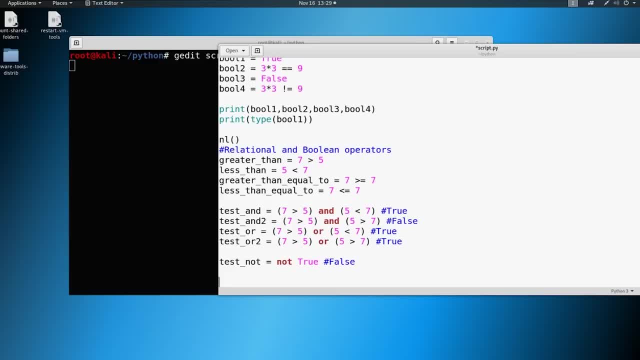 Now you can think of conditional statements as an if else scenario. but you can also think of conditional statements as an if else scenario, For example, if you go to the store and you want to purchase a drink and the drink cost $2.. 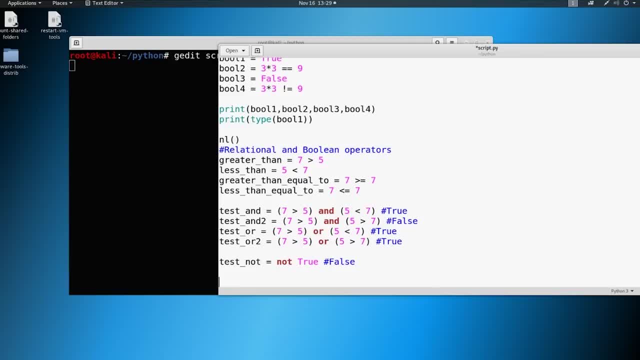 Well, if you have $2, you're going to be able to purchase that drink. If you don't have $2, then you won't be able to purchase that drink. That is a condition. So the condition there is based on the amount of money you have. We can take these conditional statements. 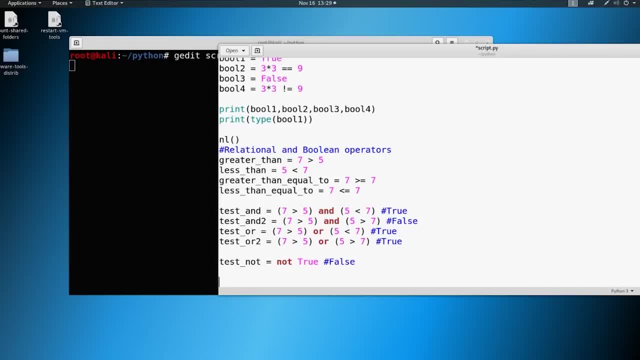 and we can run if else. we could also run if else, if else, and build upon these. Now it all makes sense when we start putting it together in our script here. So let's go ahead and just do that, Let's make a new line And let's make a comment. 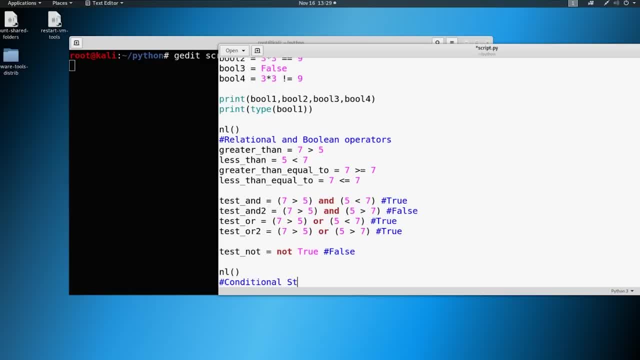 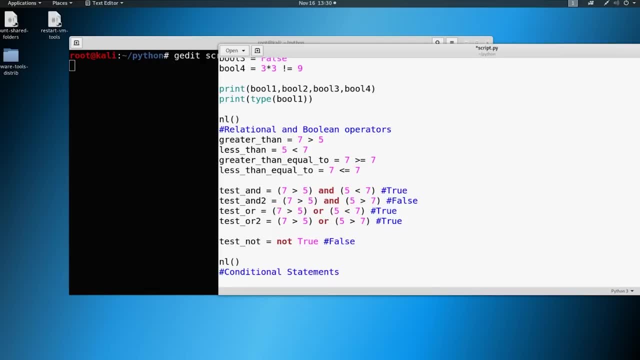 here that says conditional statements. And let's start with a conditional statement. So conditional statements. going to start off looking like a function, So we'll say define. And here let's make the same scenario. So we're going to start off looking like a function, So we'll say define. 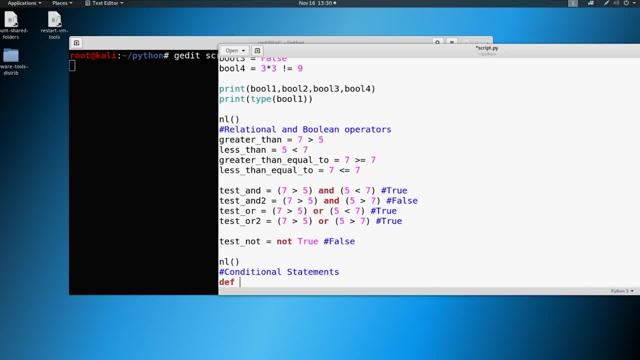 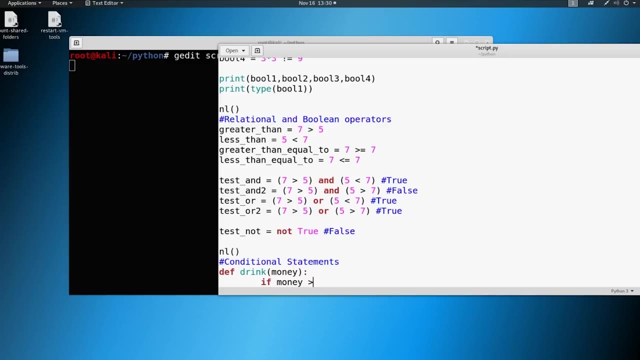 And here let's make the same scenario where we talked about the money and buying a drink. So we'll define drink And we'll just say a parameter here of money, Okay, and then let's indent and let's say if money is greater than or equal to two. remember we talked about $2 for this. 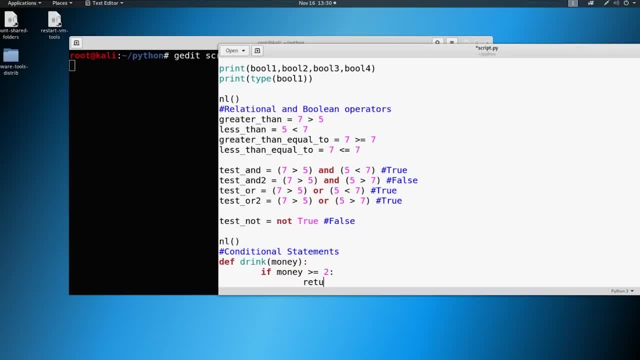 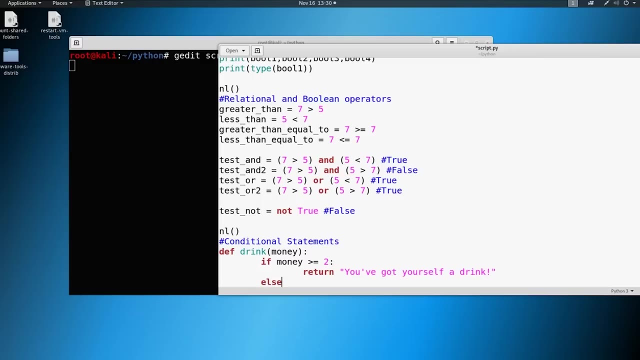 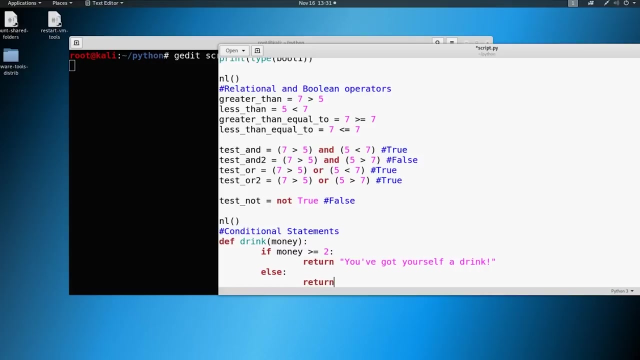 drink, then we're going to return. you've got yourself a drink, Now what if we don't have the money? So we could say else? if our money is not greater than or equal to two, then we're just going to return. no drink for you, Didn't mean to capitalize. 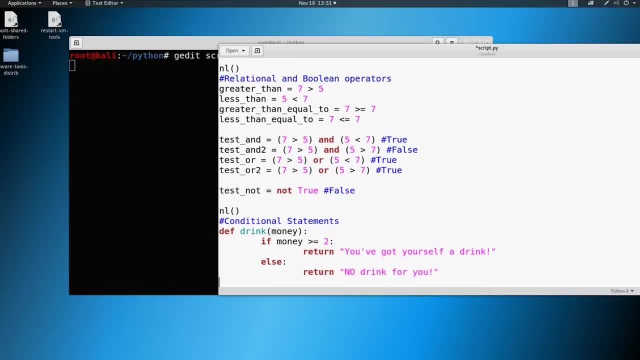 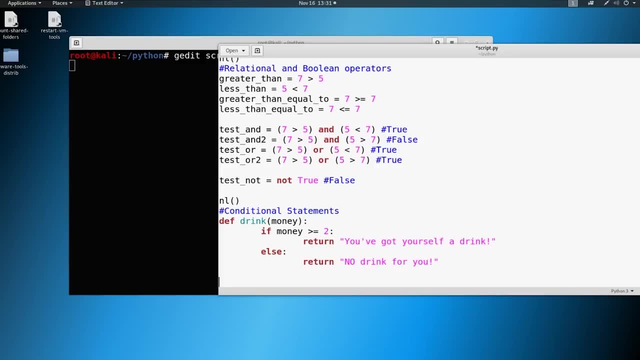 the O there, but I'm leaving it because I like it. So in this situation, we have our conditional statement already set. Now again, if our money equals or is equal to or greater than two, we're going to get a drink, And if not, we're not going to get a drink. So it could be anything else. 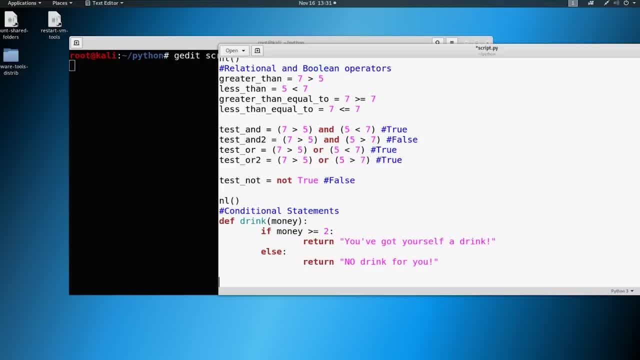 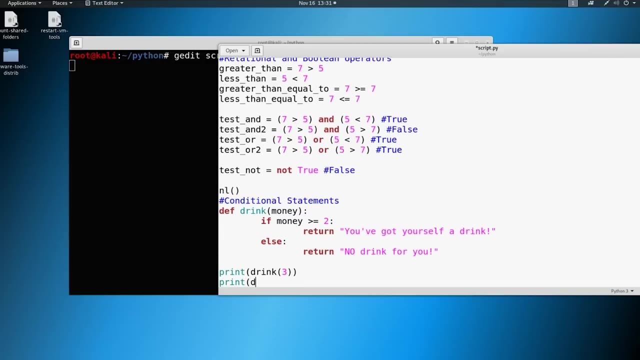 right. So what we can do now is, since this is just returning and not printing anything, we can print out something like a drink, And then we specified the amount. So if we have three, we should return one thing, And if we print drink here, 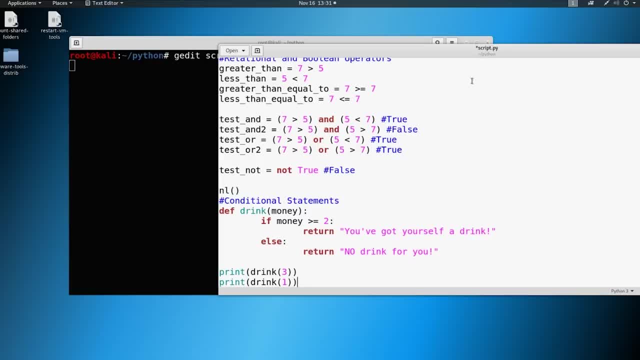 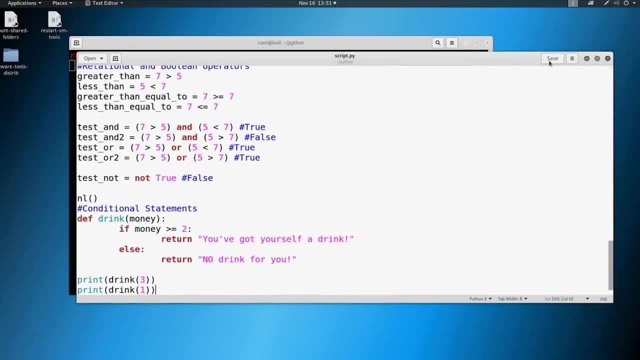 with only $1, we should return another. let's go ahead and save the script, And I didn't put this with an ampersand, So I'm going to close out and make sure I do that next time. And we're going to. 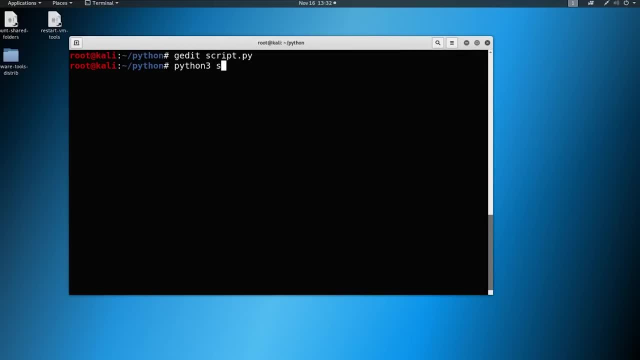 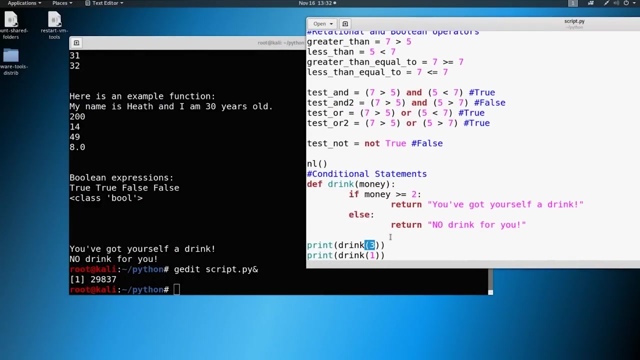 do is: we're just going to go ahead and Python three script dot, pi And you can see down here. we go back and let me run the script with the ampersand And you can see that we did a drink of three, which we were expecting to return. 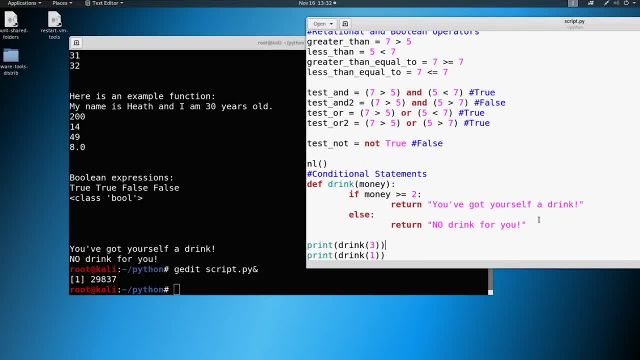 you've got yourself a drink And we did a drink of one which we're expecting to return. no drink for you. This happened just the way we thought it would, So we can build upon these conditional statements. Let's talk about a different scenario with multiple parameters. Let's say that you are an adult And here in the United States, if you're an adult and you want to have a drink of alcohol, you want to have a drink of alcohol that requires you to be of age at 21.. So, in order to purchase alcohol, you have to be one of age. 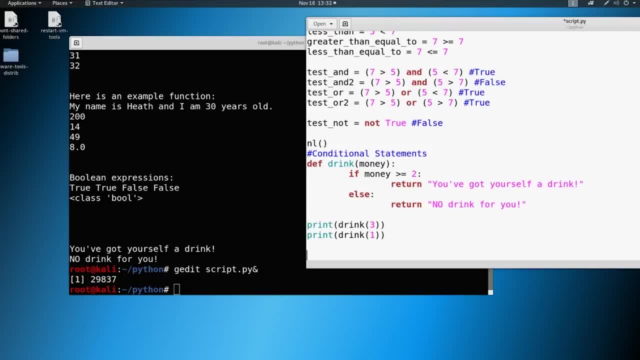 and to have money. Now, if you don't drink, that's perfectly okay. This is just a example scenario. So here let's say we wanted to buy alcohol, we have to meet that age requirement of 21. And we have to meet the requirement of money. Now we could be in a situation where we 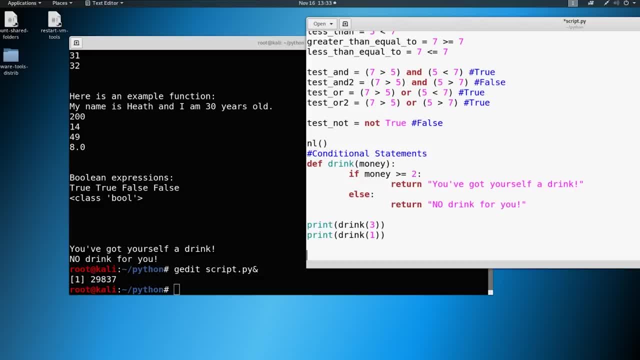 meet the age requirement but we don't meet the money. Or we could meet the money requirement but we don't meet the age requirement. Or we could be in a situation where we don't meet the age requirement and we don't meet the money requirement. So let's set this up to think. 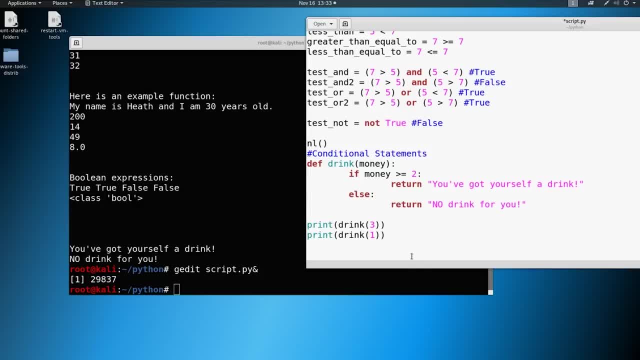 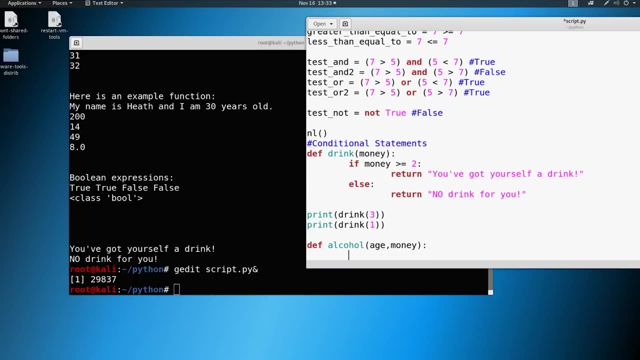 through this and how these scenarios could play out. So let's define alcohol here And we need two parameters. we're going to say age and money. So first statement here is going to be our leading if, and we're going to say if age is greater than or equal to 21,, because we need that condition to be true. And our money. 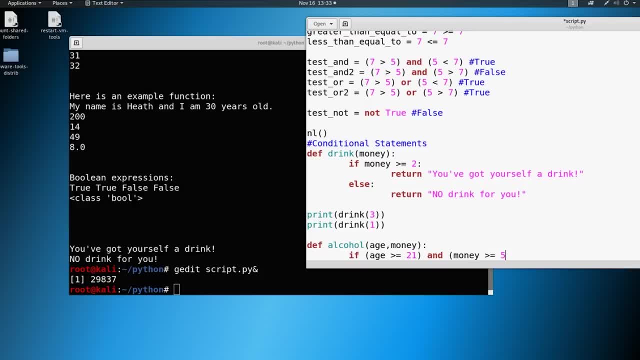 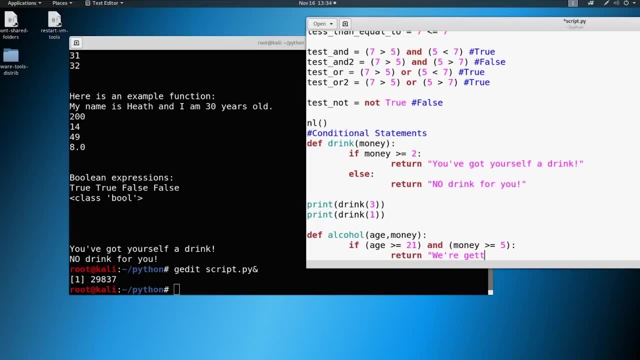 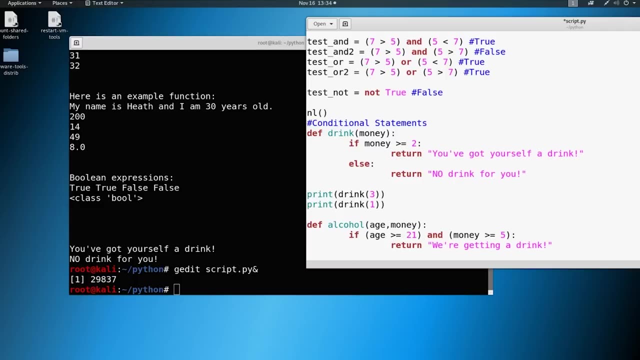 is greater than or equal to five. So we'll say a drink costs $5.. We're going to return. we're getting a drink. Okay, now, since we're going to have multiple conditions here, we're going to introduce something called else if 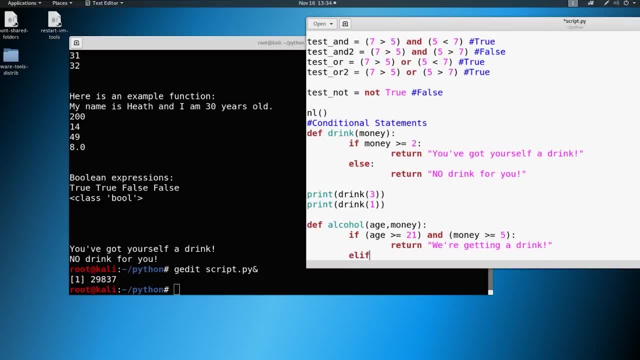 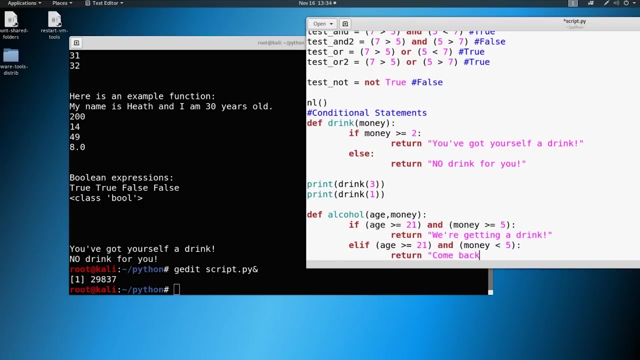 Else, if here is written like this: e l i f, So else if our age is greater than or equal to 21. And our money is less than $5. Then let's return, Come back with more money. We need another. 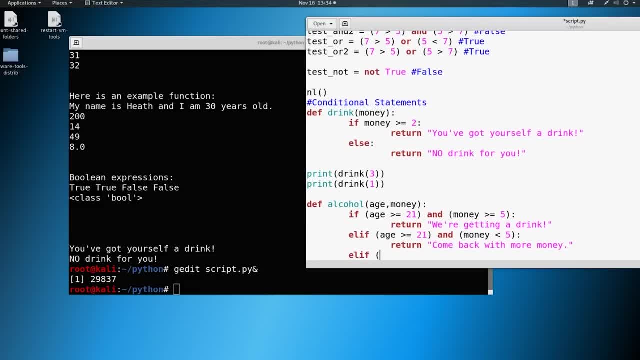 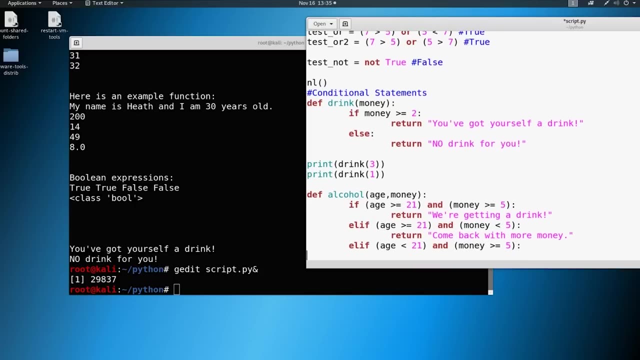 Else here, Because we have another condition, right. So we're going to say: what if our age is less than 21? And our money is greater than or equal to five? Well, we're going to return Nice try, kid, because we're not old enough to purchase this drink. And then, lastly, in our else, 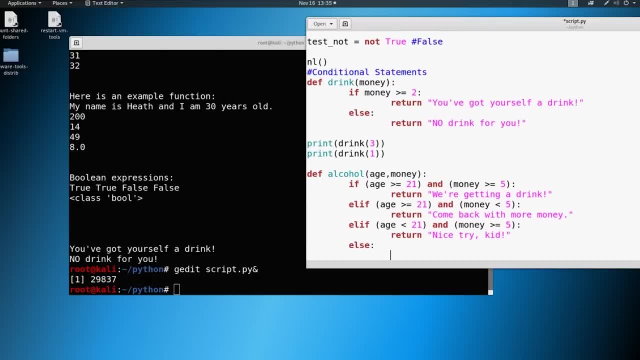 scenario: if we are, we're going to return $5.. And then, lastly, in our else scenario, if we are, we're not meeting any of the conditions above, which means we won't have the age, we won't have the money, then we're just going to return. 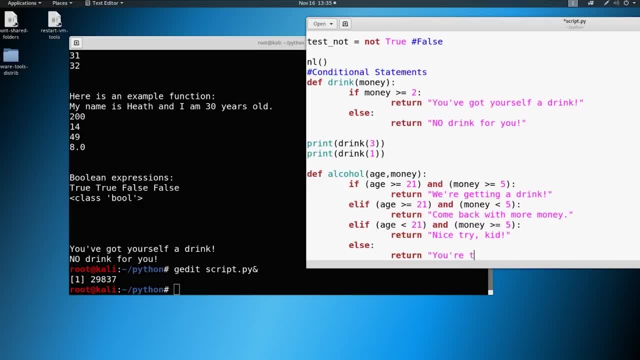 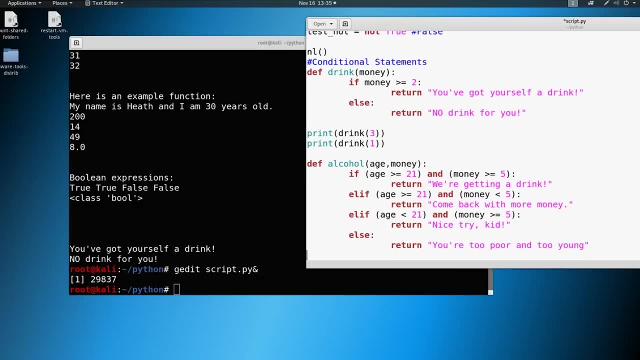 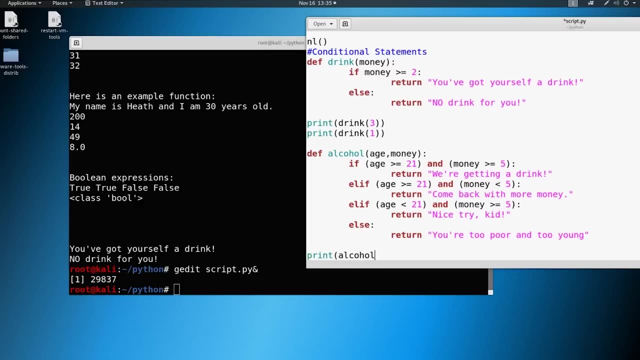 two by the type: Sorry, you're too poor and too young, So let's go ahead and run this a couple different times. So let's go ahead and print out alcohol, And we're going to give our two parameters, So let's say $2.5.. winners in this scenario, So let's. 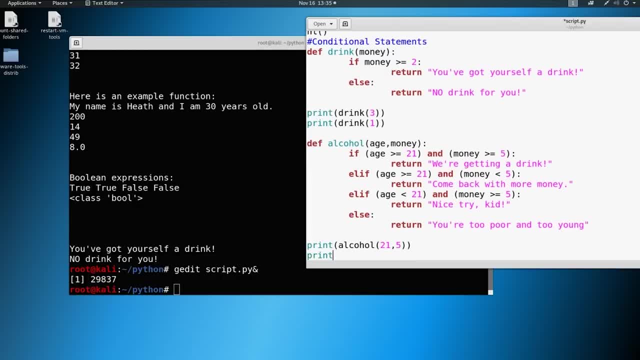 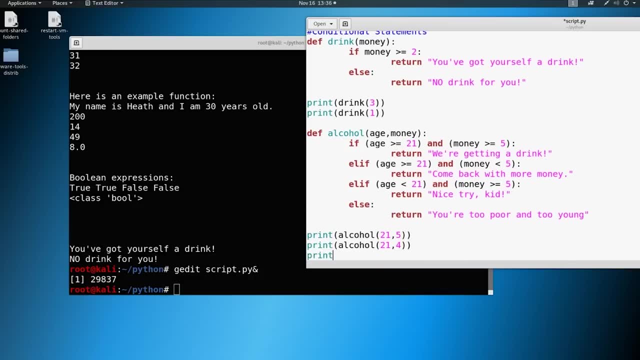 21 and 5. let's print out again alcohol and let's give a parameter of 21 and 4 and then let's print out one last time of alcohol and we'll say that we are 20 and 4, so we should meet a few different. 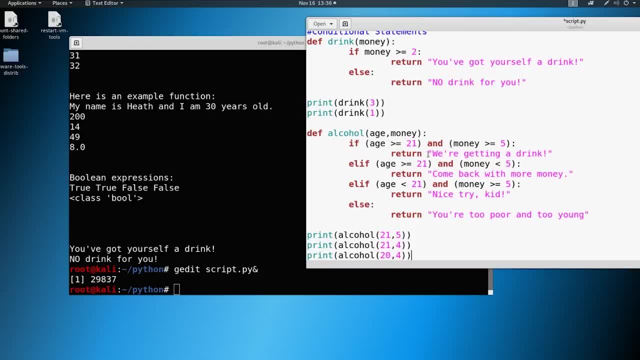 conditions here. right. so at 21 and 5 we should return- we're getting a drink. at 21 and 4 we should return- come back with more money. and at 20 and 4 we should return. you're too poor and too young now. if you want to add in a fourth condition here or a fourth print statement and you want to. 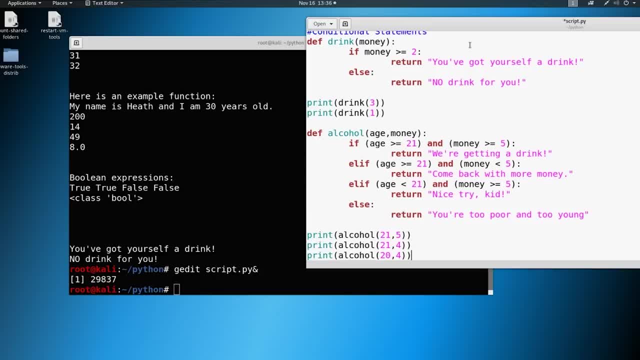 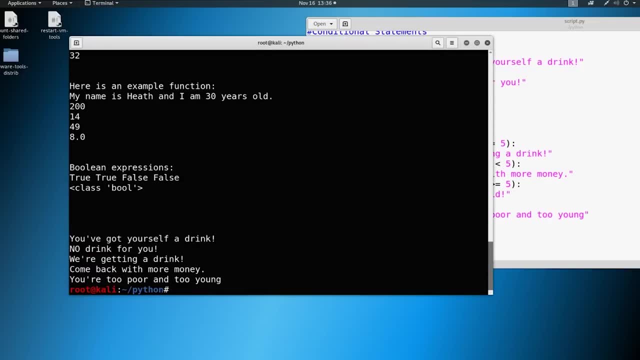 return the nice try, kid. you're more than welcome to do that as well. so go ahead, hit ctrl s or save your script out, and then let's go ahead and run it and you can see we return exactly where we thought we were going to. we're getting a drink. 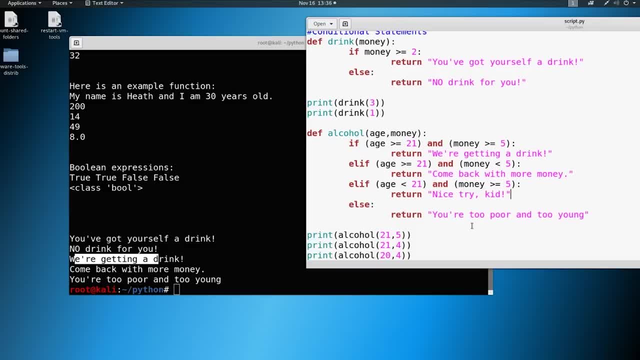 come back with more money and at 21 and 4 we should return. you're too poor and too young. come back with more money and you're too poor and too young. so this is it for conditional statements. hopefully this makes sense again. our conditions are based on certain items, right? so money here. 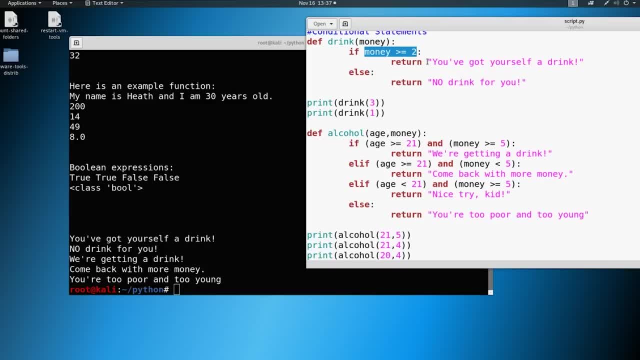 for an example: if we have the money, we're getting a drink, if we don't have the money, we're not getting a drink, and then we can build upon that. we can have multiple parameters here. so if we're not old enough to buy a drink, or we don't have enough money to buy a drink, or we don't meet. 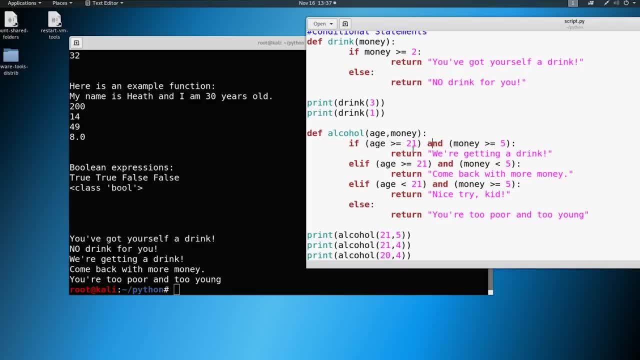 any of these scenarios, different things can happen. what you need to be thinking about as a developer program, or even writing these scripts, is all the scenarios that could happen in these situations. you got to think of the logic behind it. so when you're building out a script, you're building out your first program. you need to think logically. 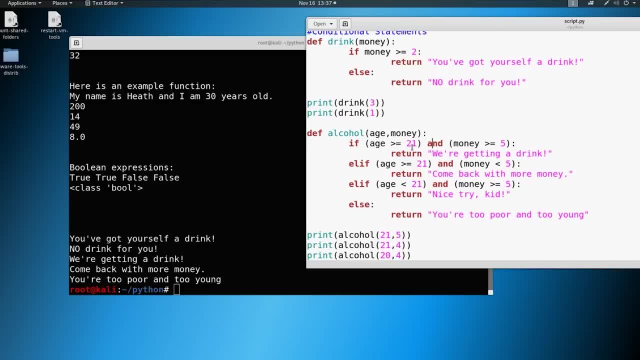 if i make an if statement or a conditional statement, what's the logic behind it? so a lot of times, for example in this scenario, we might have thought, okay, well, if i don't have the, the age or the money, okay, but you got to think about the logic behind it and you got to think about the 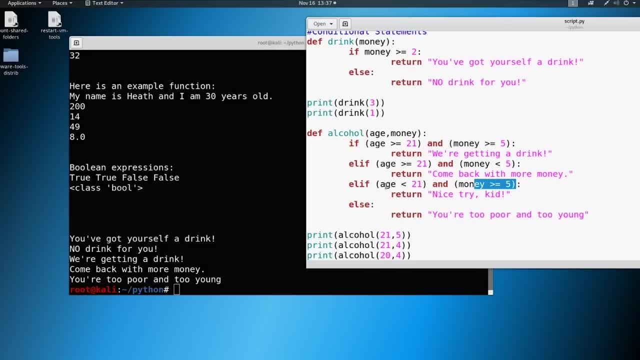 what if i do have the age but not the money? or i do have the money but not the age? so you have to think through everything in your head and make sure that it's all clicking, and this just takes repetition and just sitting down. the best way is sitting down with the pen and paper and not 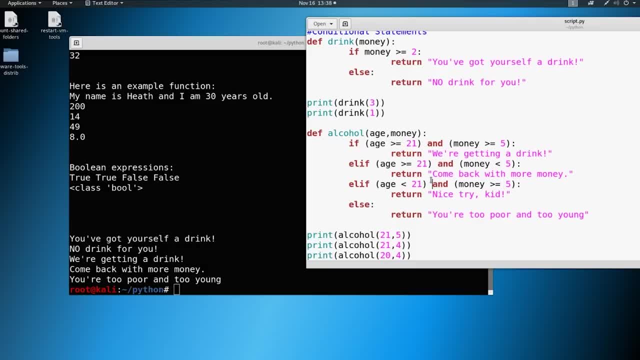 writing this in code form, but just writing this in a sense that makes sense to you, thinking through it logically and then writing it out in code. so from here we're going to go ahead and move on to list in the next video. so once you're all caught up here, let's go ahead and move right over there. 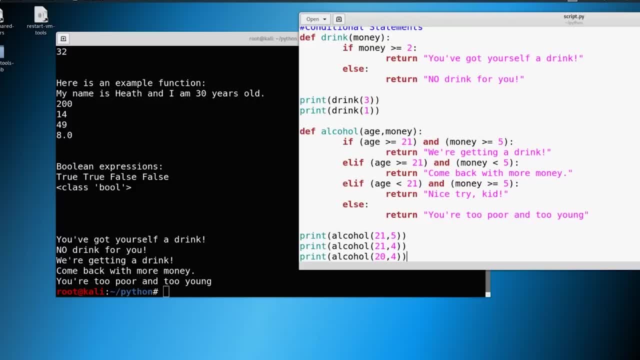 okay, now let's talk about lists. so lists are data structures. now, these data structures are changeable. we can reorder them, put them in a list, right, so they're just a group of elements and when you, when you have this list, everything inside that list is called an item and the best. 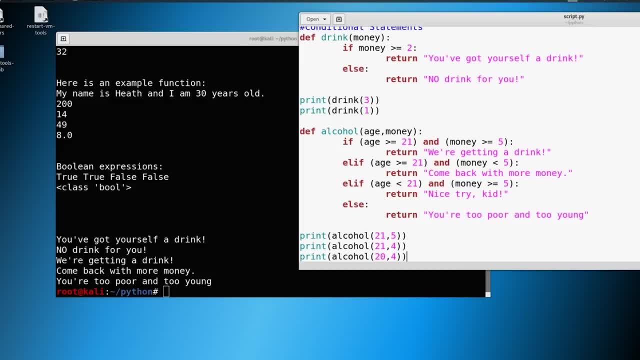 way to think of a list is to think that it lives in between brackets. you're going to see other things later on that look like a list, but it's not because it's not a list. it's because it's a list, but it's not really a list because of how it's defined and how we're going to define lists. 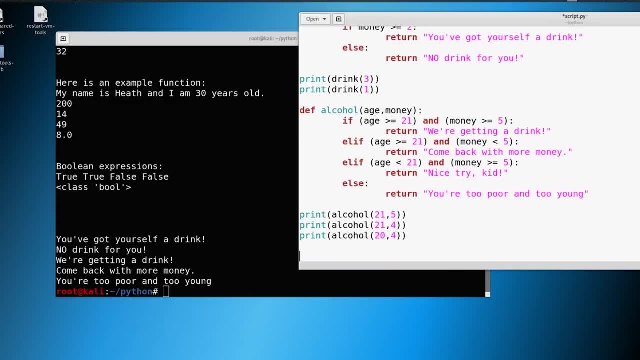 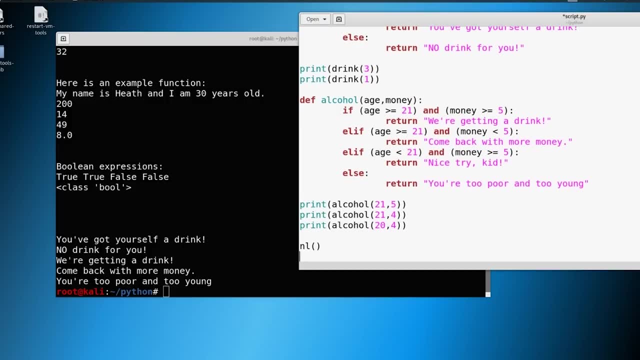 is because they live in brackets. just like a string might have quotes around it, a list is going to have these brackets around it, so let's make a new line and let's go ahead and just do something along the lines of lists and we could just say something like: have brackets like this: 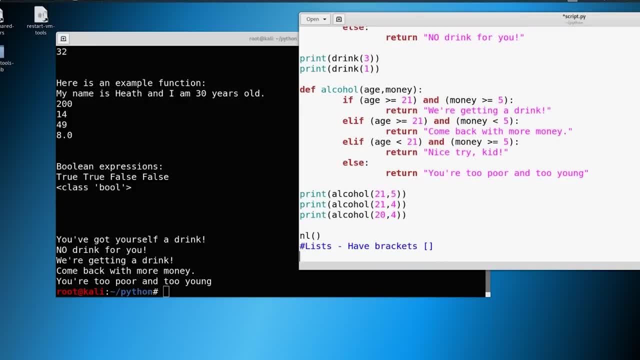 okay, so let's go ahead and make a list and then we can kind of go from there. so let's define a list of your favorite movies now. you could put in whatever favorite movies you like in here, and i'm going to put in something like when harry met sally. 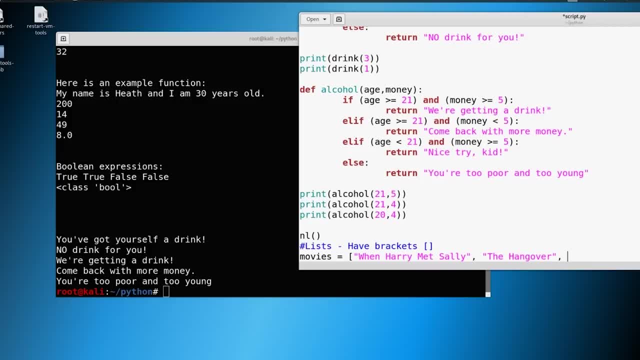 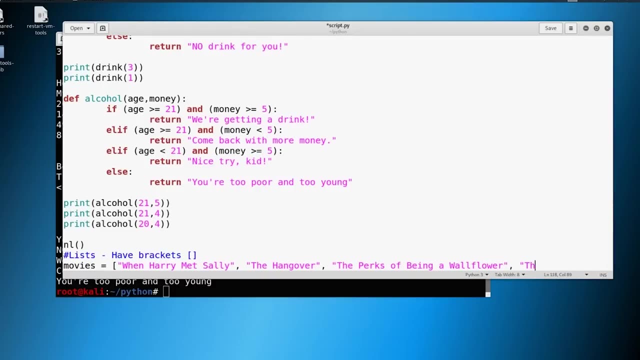 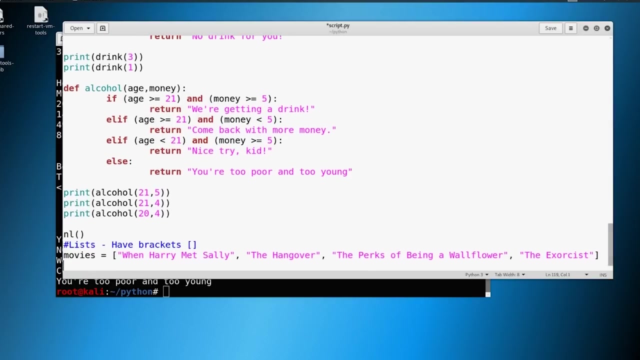 the hangover, the perks of being a wallflower. this is getting kind of long, so i'm actually going to move this over a little bit for us and we'll say one more: let's pick four movies, we'll do the exorcist, okay, and now we have this, this list. again, lists just live in brackets, so 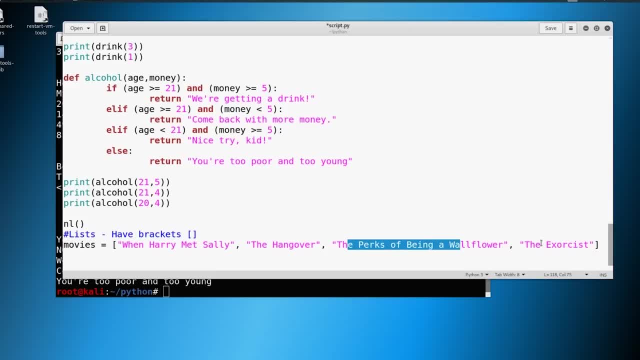 we've got list item one, item two, item three and item four. okay, so let's go ahead and print these. so if we were to print out something like movies and we said we wanted to print out movies, and so we print out gips and we've got three items, but we can print out movies and also have the boxes. as if others do that we just need to let go, or some of those folders fell in as well, so let's see if that's the the other best way to do list list item 3 and item 1. let's print the list and item 4, okay. 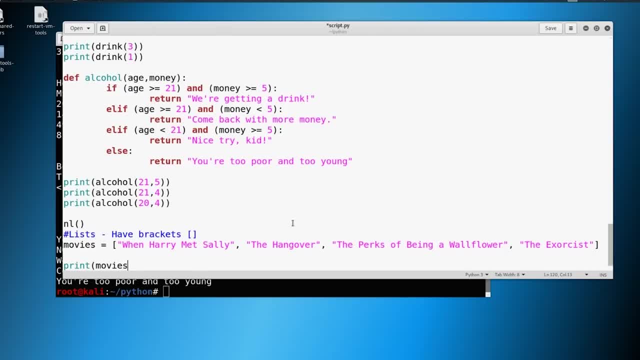 And we said we wanted to print the first item out of movies. Let's go ahead and try to print when Harry but Sally, so print the first item. So put a bracket around it, just like this. We'll print it out and we'll see what happens. So let's save it. And what's it going to return for us? 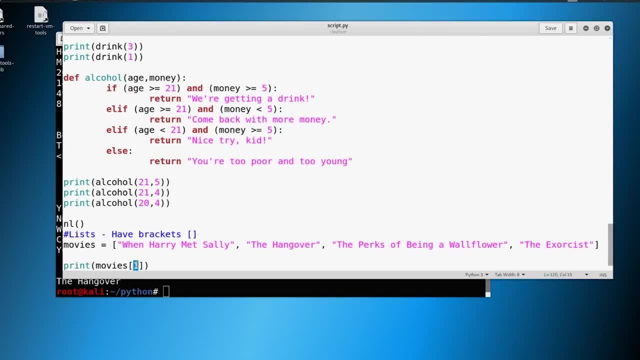 It's returning the hangover, So item one is not item one as you see it. So when we talk about items, when we talk about numerical order here in Python, item one is actually going to be referred to as zero. So make a note here for yourself that this will return the second item. So if we wanted 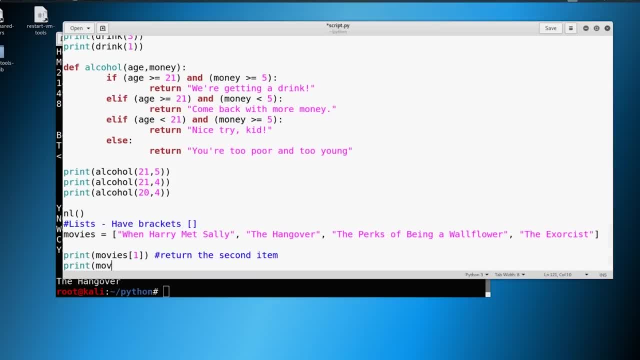 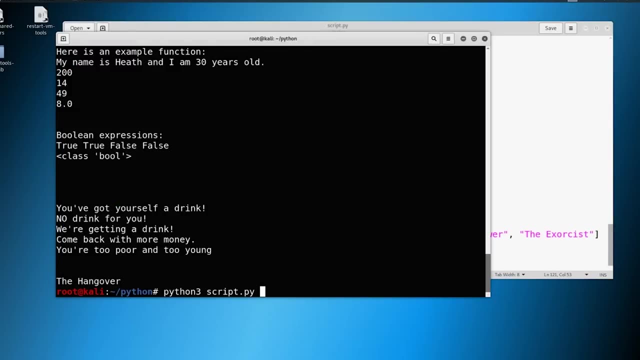 to return just when Harry met Sally. we would actually put in movies zero like this And we could say: returns the first item in the list. Okay, and we can save that And let's go ahead and give it a go, just to do proof of concept. And 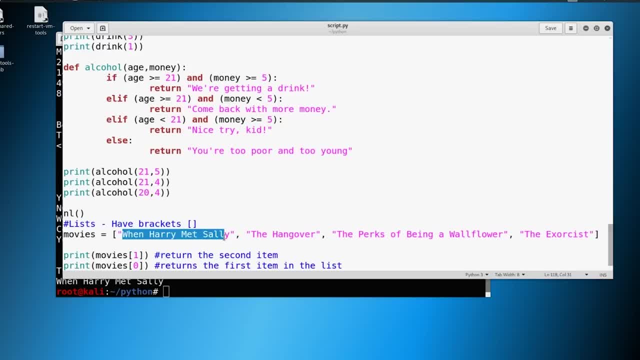 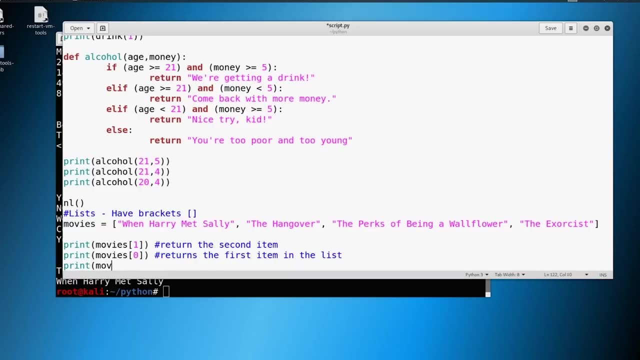 there you go. Remember that everything starts with zero and not once. when you're thinking about things, Let's think about them with zero as the beginning number. So let's go ahead and do a few more different prints. What's going to happen when we print out something like this? we'll say movies. 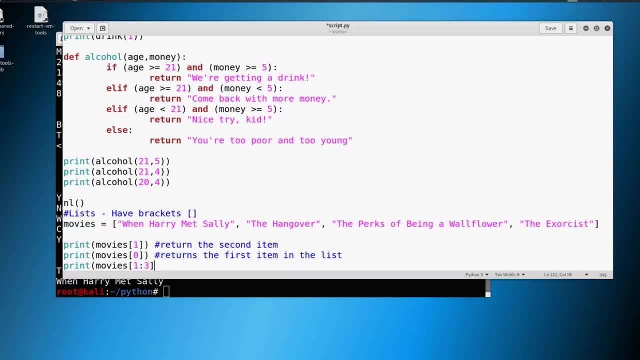 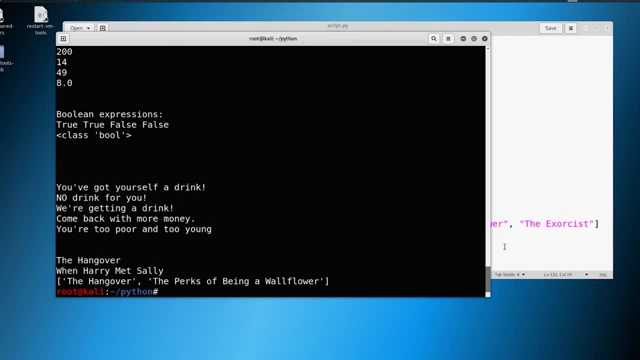 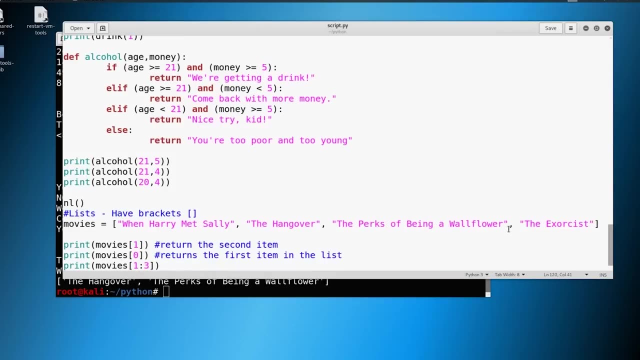 and we'll do one through three. Do you have a hunch? Let's go ahead and save it, Print it out here And it will take the list here of starting at one and it'll end before three. So let's say we want to pull a couple items out. 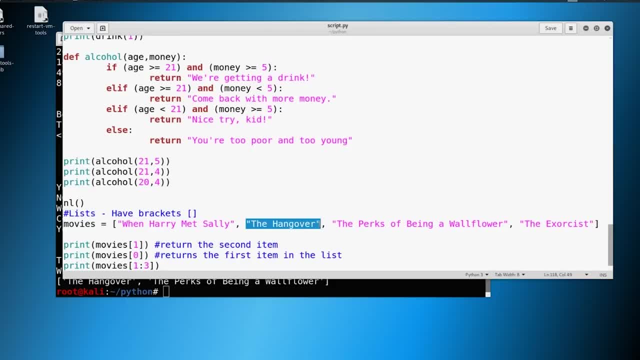 The first number that we're going to pull out is going to be the one that we want to start with, And the last number that we're going to pull out is going to be the number where we're going to stop. So the exorcist is three. But if we wanted to actually pull down the exorcist, 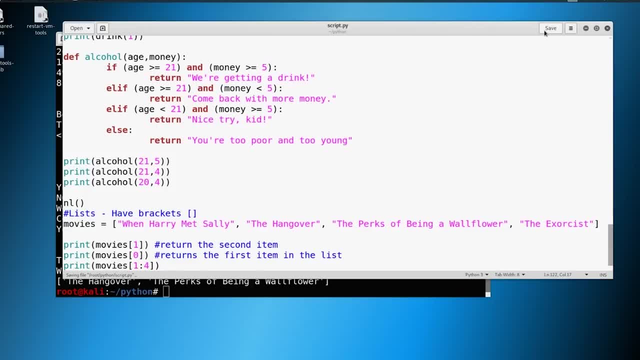 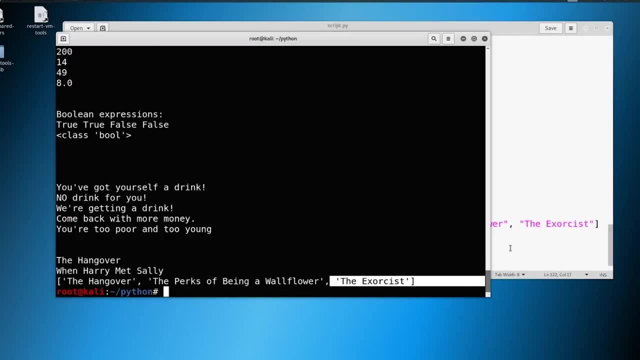 we would have to pull down four here. So if we want to try to grab more than one thing on the list, we can absolutely do that. We have to know where to stop. So now we incorporate the exorcist here. Let's say we wanted to grab everything in a list And we wanted to grab everything. 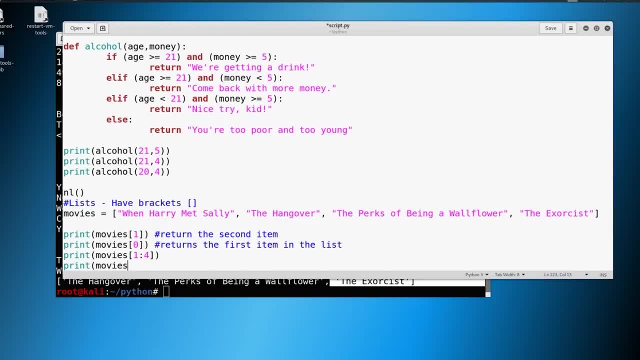 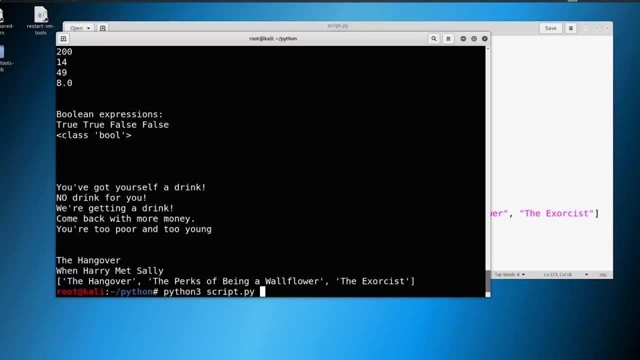 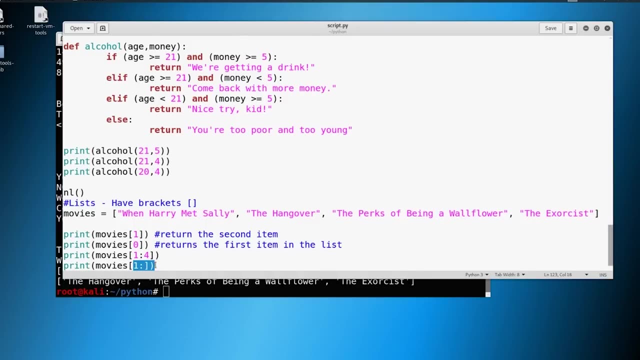 after a certain point. right, we could say something like movies, one like this, And then we should be able to grab every single thing, And that does pretty much the same thing here. So if we had 30 items here, it would grab all 30 items in this list. 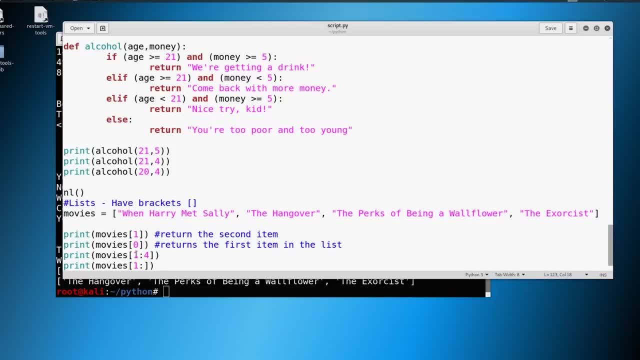 If we wanted to grab three items, as we did before, we would do one. then you just add three to that, to four, and it would stop. So a little bit confusing. This takes a little bit to wrap your mind around, But the good thing here is that you take notes. you can make notes, however. 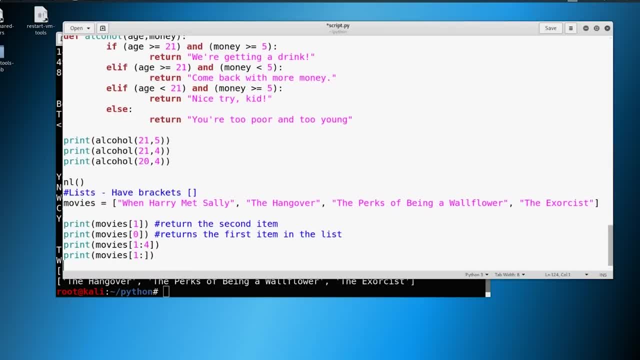 you feel comfortable with, And these tricks should be useful for you. So let's try another thing. What if we said something like movies and we did this one in reverse? we just did something like this And we did save. Let's print it out. What do you think is going to happen? 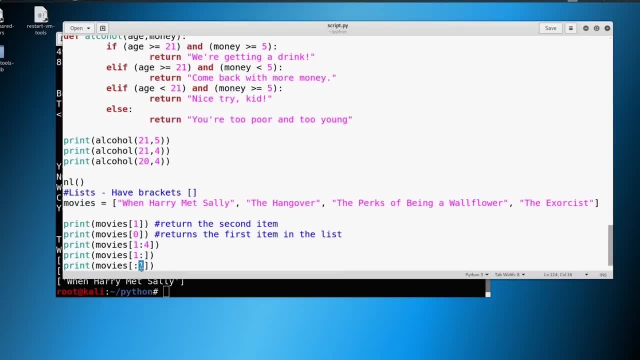 It's going to print when Harry met Sally, because it's going to stop at the one. we never get to one. here again, similar situation when we have this set to three. we never get to one, we stop at one. So we're going to grab everything before one, which is going to be just be when Harry met Sally. we can. 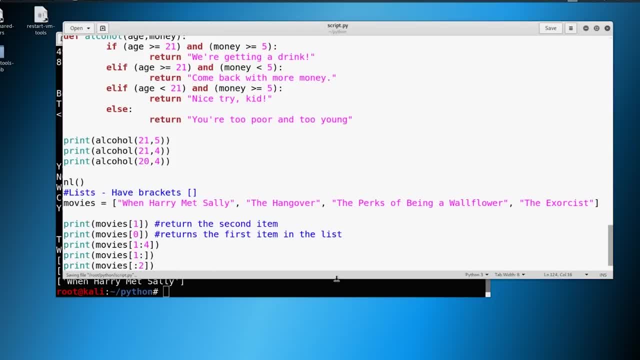 set this to two and we would grab the hangover in this as well. And just to prove concept here, so that I'm not crazy, You can see, here the hangover gets added in because we get zero and we grab one. You could also think of this, if you don't confuse yourself as grabbing two items out. 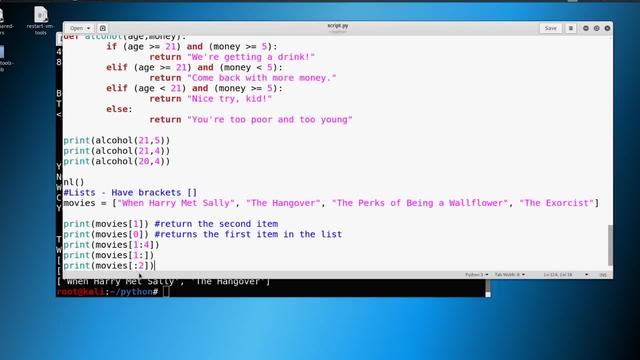 of the list, But make sure you don't confuse yourself, because if this number were to be like two through four, then it would be something completely different, right? So you need to make sure that you understand where from the list that you're actually. 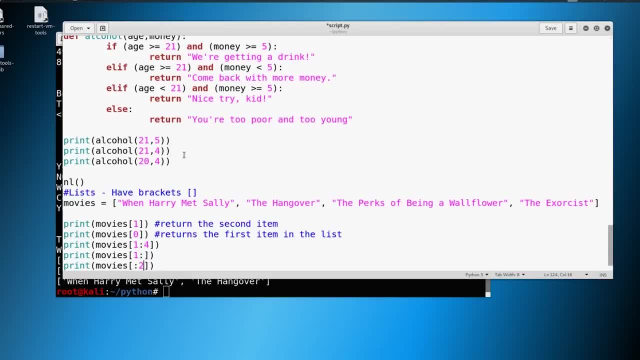 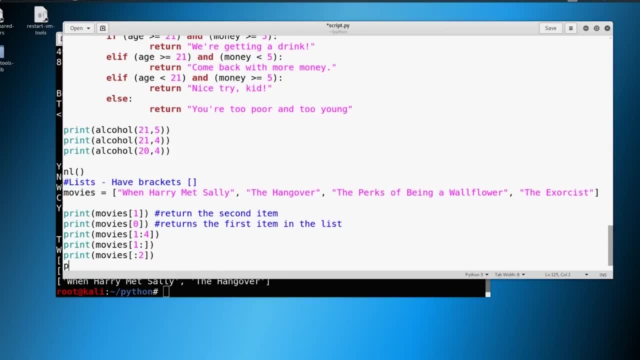 grabbing. I'm just going to Ctrl Z these back. So from here let's do two more tricks. Actually we'll do one more trick and then we'll move into some other items related to lists. So if we say movies like this and we want to grab the very last item, we can just put in a negative. 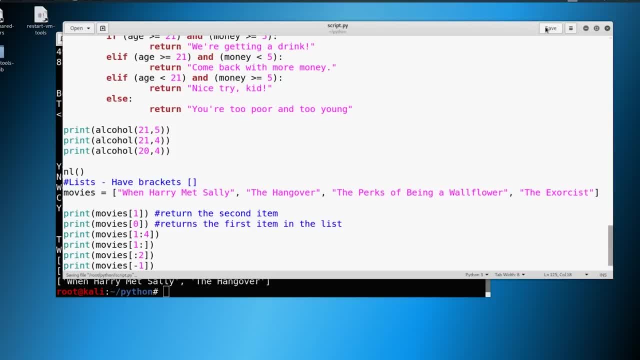 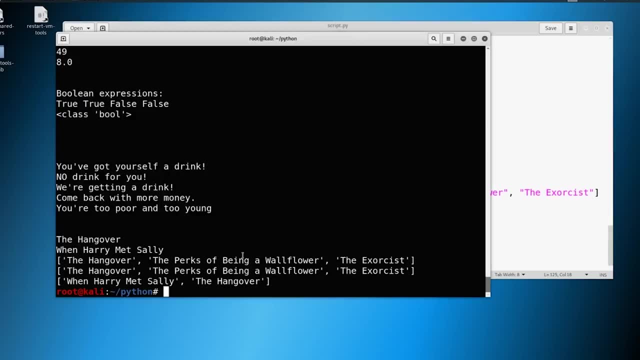 one And so grab the absolute last item off the list. That way, like if you have a list that's items long and you don't know where it ends, you could just do negative one. it's going to grab the last item for you And then you can see there it grabs down the exorcist. 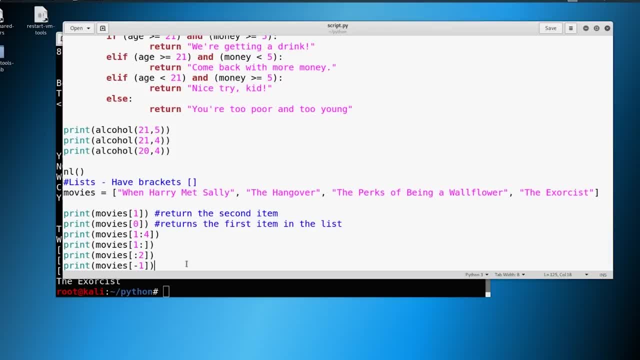 So cool little tricks. you might not use these for a while And you probably won't see these come through, at least in anything we're going to really do in the course, But they're still incredibly useful to know about because they're- they are- included in the basics of Python, So 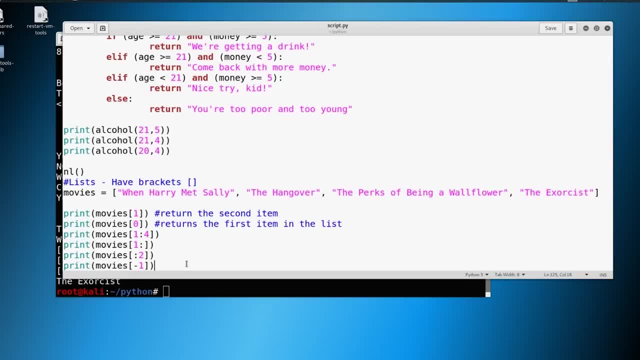 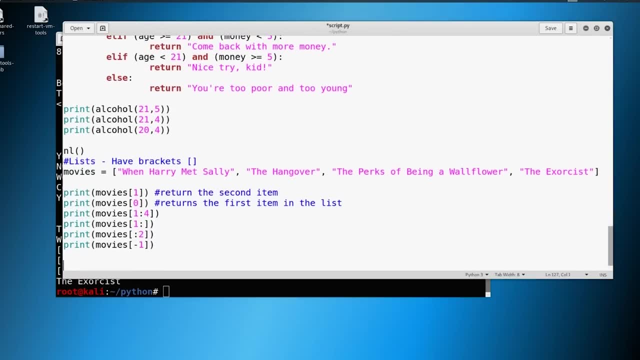 you're going to know the basics of Python And you will use these sometime in your lifetime. It's useful to know this kind of stuff So we can also do some things with lists as well. we can print out the length of our list, So we could say length of movies. 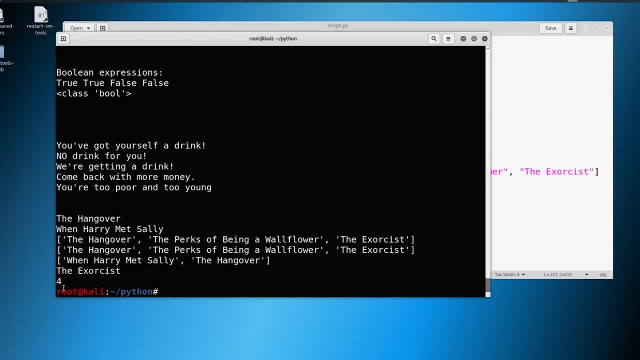 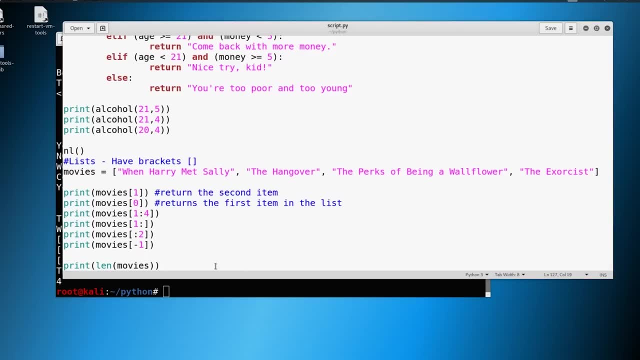 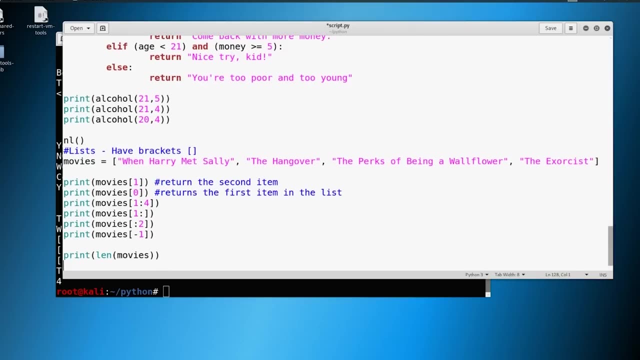 something like this and give that a go And you can see that there's four items in that list. So we've seen length before with strings and it took every single character inside that string. Here it's taking every single amount of item inside a list and printing that out. We could also. 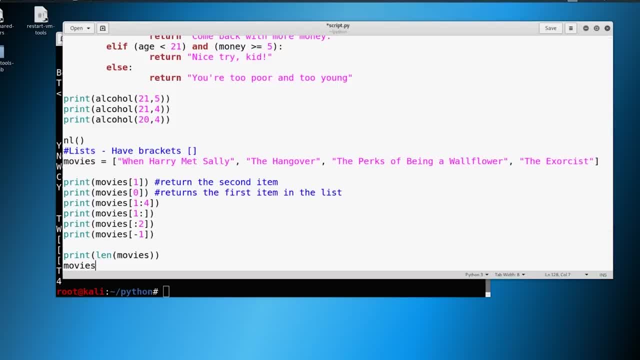 append items to the list, So we can say something like movies dot append. And what if we really like Jaws and we add that into our favorite movies? you can have too many favorite movies, come on. So let's go ahead and try printing that out. And well, we'd have to actually print it. 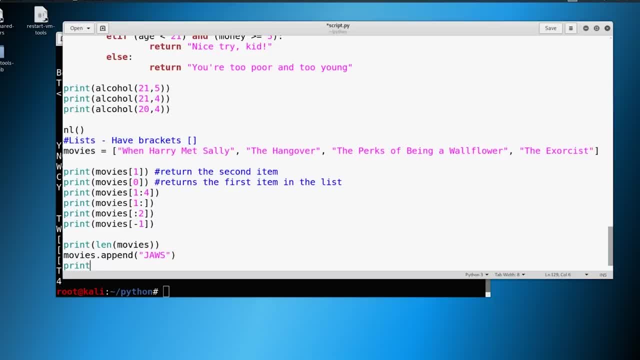 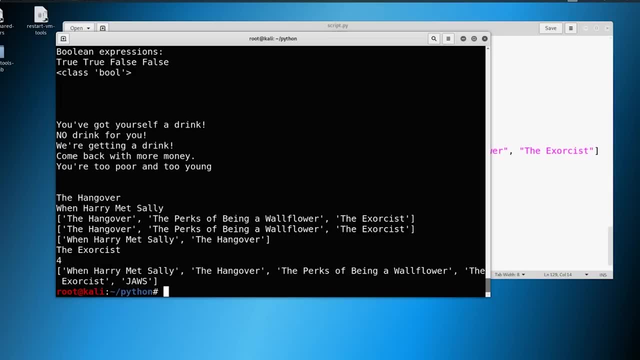 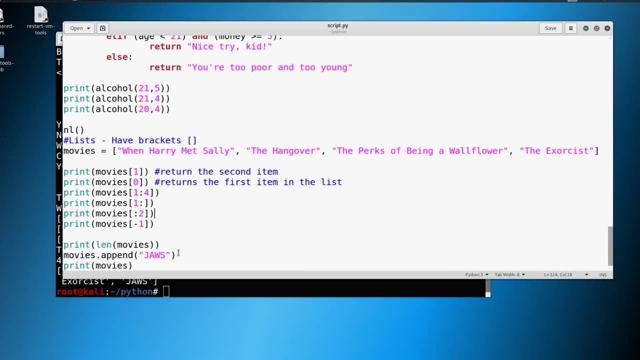 sorry, movies that append. And then we say, print movies now, And it should print out with Jaws added in. where do we think Jaws is going to actually add itself into? Well, if you said, oh, you said the end of the list, you are correct. So when we append something, we append it to the 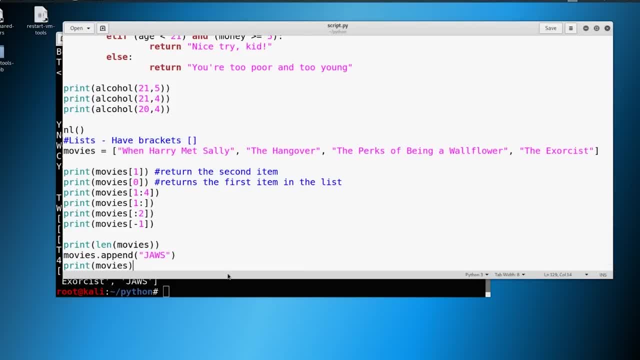 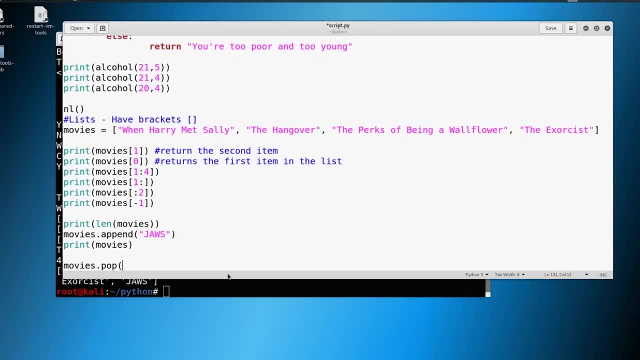 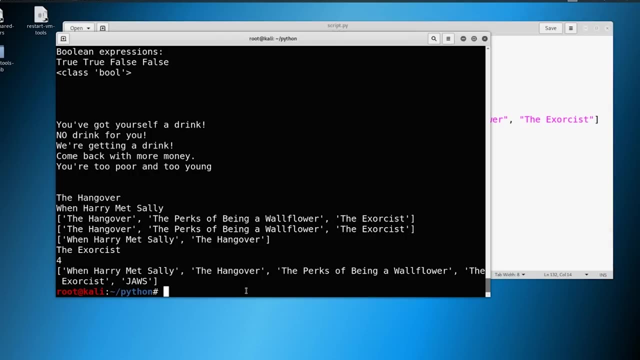 very end of the list. What if we wanted to delete something from the list? We could say something like this: movies dot, pop and print movies. Let's see what happens here And now we got rid of Jaws. So when we append, we append to the. 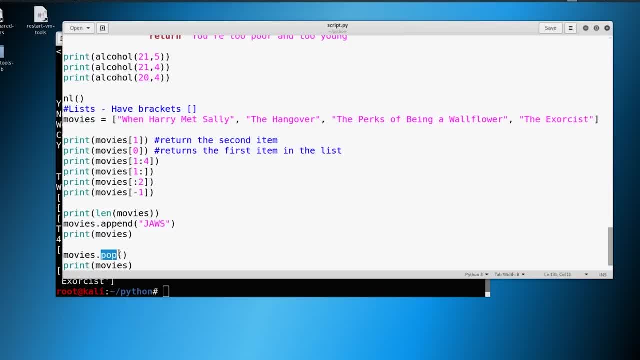 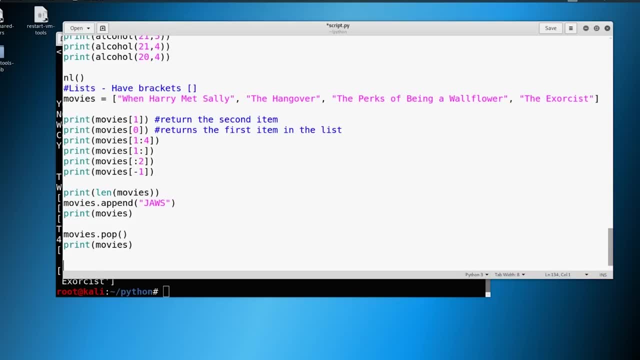 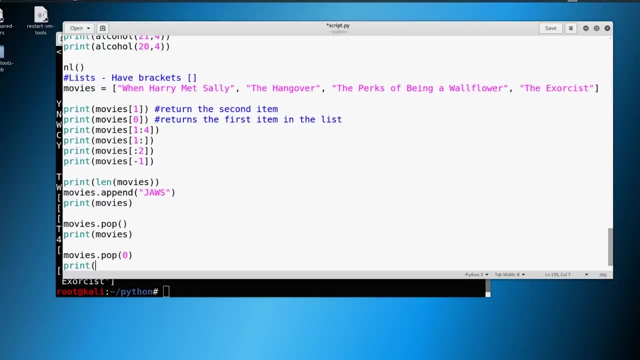 end of the list. If we want to delete the very last item in the list, we just use pop. Now, if we wanted to delete something like the first item or the second item, we could do movies that pop and, let's say, zero print movies. This will remove the very 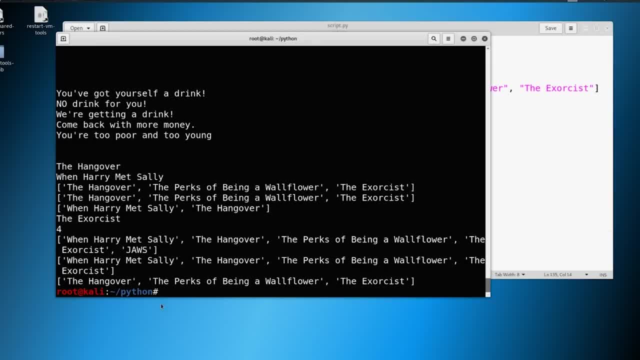 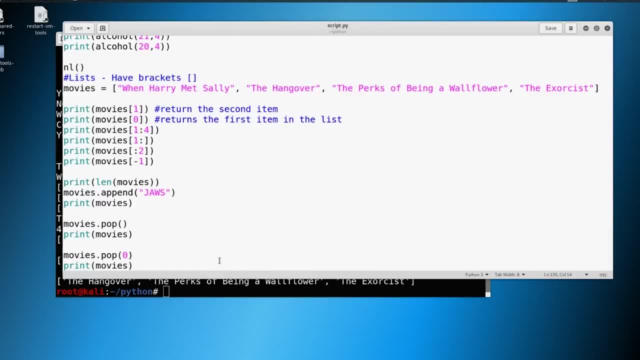 very first item in the list We should see when Harry Met Sally disappear. And there you go. No longer is when Harry Met Sally in our list, So this is a quick way that we can remove these items and on the fly, if we need to, to get rid of this. So the high level. 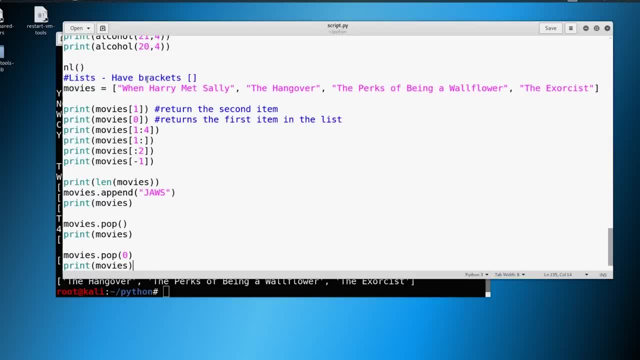 overview here, and the thing that you really need to take away is that lists have brackets. We're going to see something called dictionaries later, We might see something called tuples later, and they all look very, very similar, But here lists have brackets. inside Those brackets are 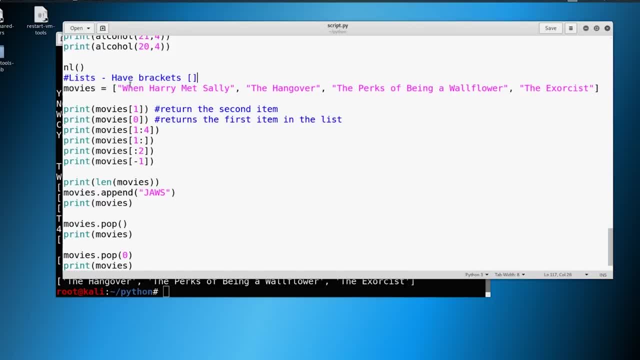 what we have that are called items Okay, And there are many different ways to return. The reason that I'm showing you these different ways is so that you can get familiar with the syntax, that we start our list or our items with zero and not one, and that we can grab. 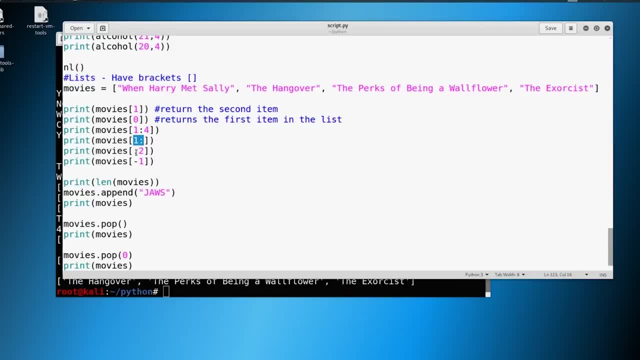 from these lists in different ways. Okay, And this will come back into play later with how we can utilize the same kind of syntax with other items as well, or other things in Python, So we can also utilize, you know, printing out length, or we can do a dot append. 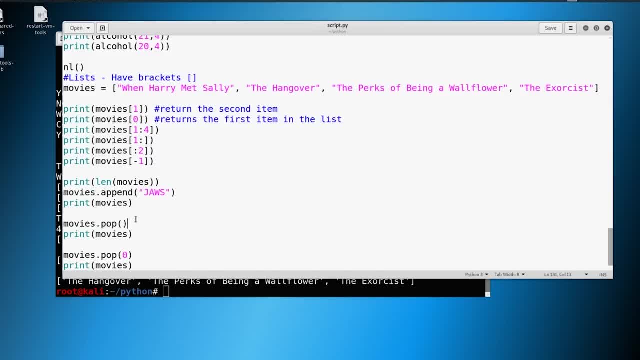 and add to the list or dot pop, And there's a lot of different things we can do here to you know, to append to these lists or remove from these lists, etc. So this is just the basics, But hopefully what you take away from this is that lists have brackets And you know the items. 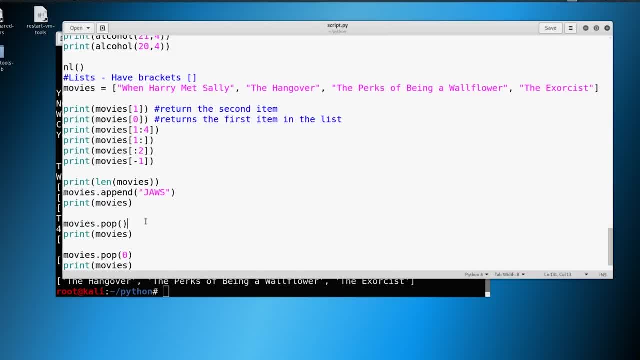 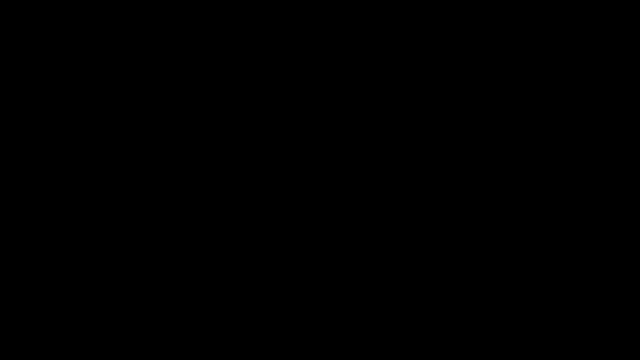 there are items in a list and they start with zero. Those are the key takeaways. So in the next video we're going to briefly talk about tuples And then we're going to move on into looping, So let's go ahead and do that. Okay, let's briefly talk about tuples Now. tuples are like lists. 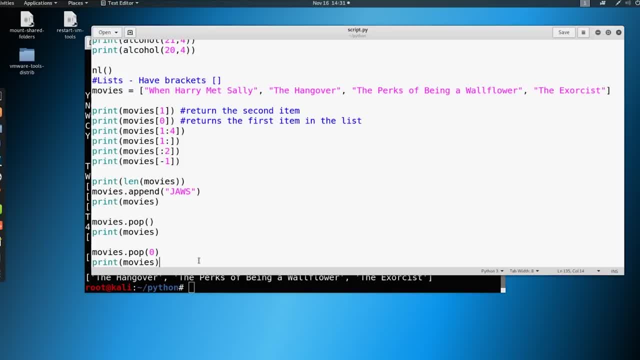 but they're not like lists. So lists are what we call mutable, meaning that they can be changed. Now tuples? tuples are immutable. they cannot be changed Now for this course, this is the last time you're going to be seeing tuples, but it's important to define what they are so that you know. 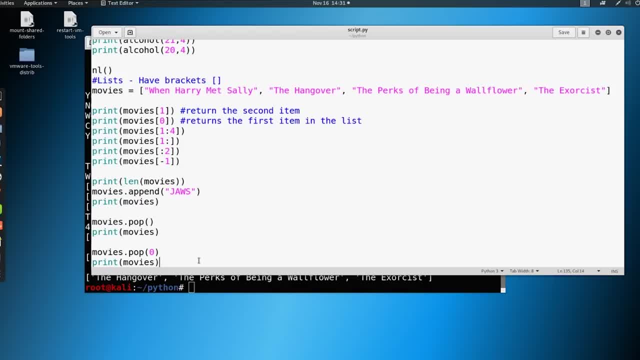 them, identify them, And they're just in the back of your mind as, Hey, I know what a tuple is And that thing is immutable. I can't change it once I have it. So let's take a look at a tuple, Okay. 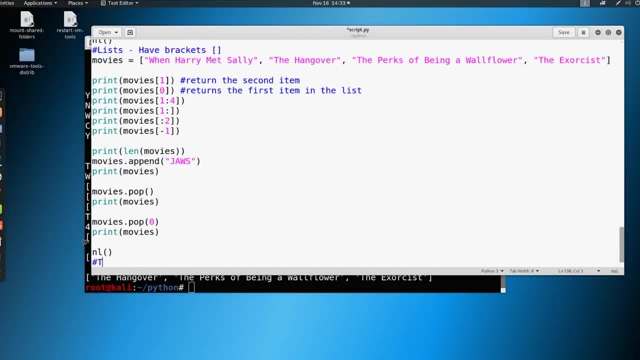 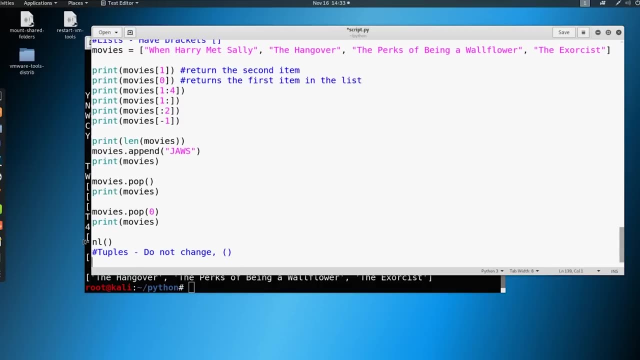 let's make a new line here and start a comment. We get to say: tuples do not change. And also we can put parentheses like this, Because remember, lists had brackets- tuples have parentheses. So we're going to say something like grades. Now we're gonna have an item that won't change. So 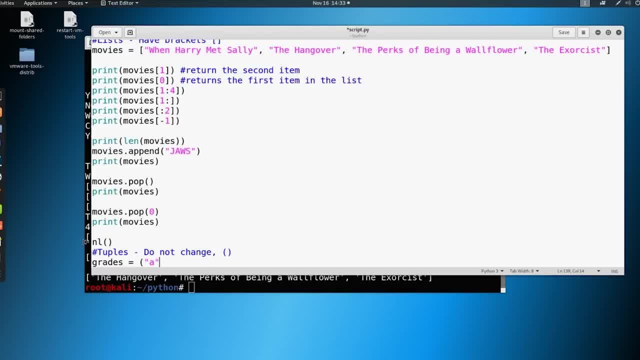 we're going to define grades here as just a, b, c, d and f, which is common for the US grading system, And this is an example of a tuple. So again, we have parentheses instead of brackets. Now, if we were to go in here and we were to try to do a grades dot pop, 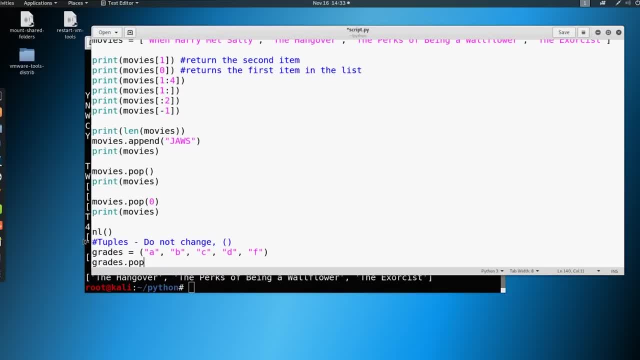 for example, and try to remove one of these- not going to be possible- or a grades dot append, we're not gonna be able to put something else in here. This is immutable. we cannot change this. once we have it defined, So we can go ahead and print out our grades And we could say printout. 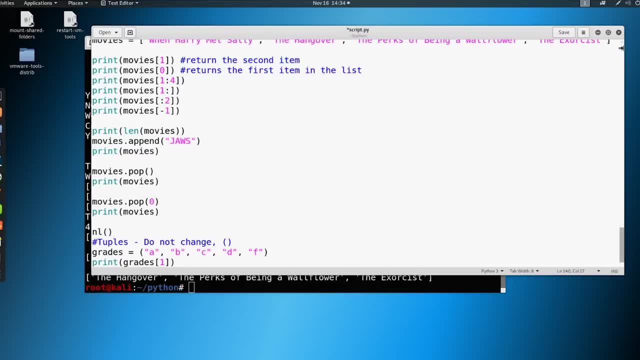 grades. let's print out a, b And that will work, And you can see. now we've printed a- B, So we have similar features, but we need to print out a render and you can see we have different results here. So. 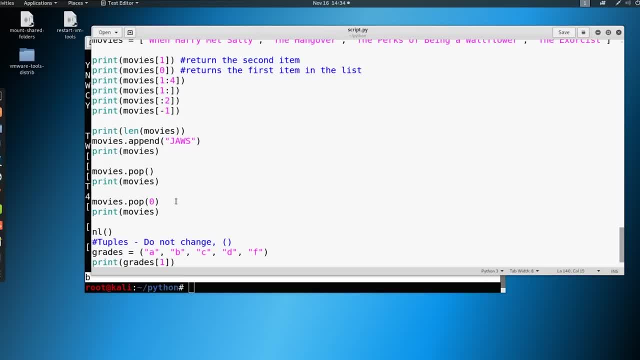 features or abilities that we did here, but we cannot change it in any way. so once we have this defined and set, that's it for us. so this is it. i just want to quickly show you what a tuple is again. we're not going to get into it at all in this course, but it should be defined and we should. 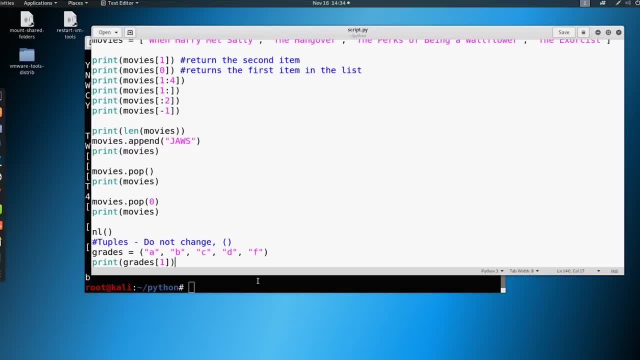 know the difference between a list, which is mutable, versus a tuple which is immutable. so in the next video we're going to get into looping. so we've already covered looping in the bash scripting section of the course, but we're going to go ahead and get into the python version of. 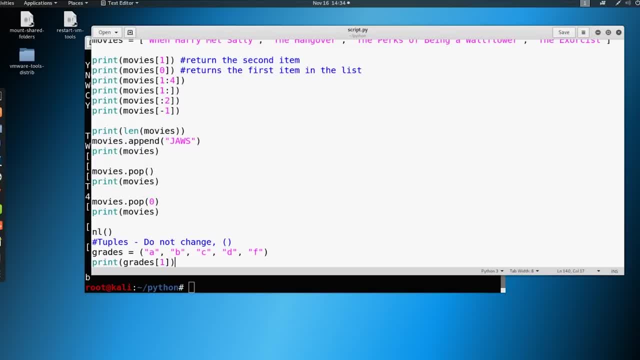 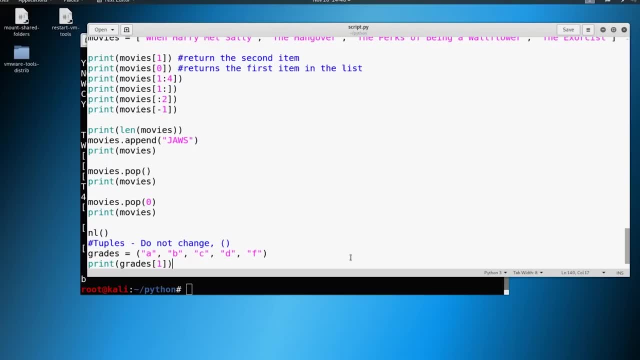 looping as well and make some more sense of it. so i will catch you over in the next video. now, moving on to looping. so we introduced looping in our bash scripting video and we took the four loops and we made one line, four loops, and those should be familiar to you. so for loop is just a. 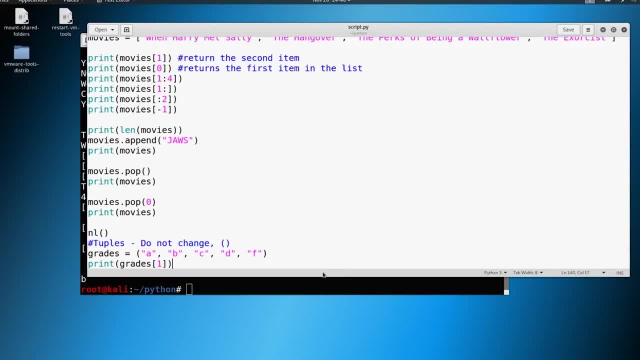 start to finish event, an iterate right. we wanted to run that ping scanner, for example, and we started at the one and we ended at 256 on our ip sweep. now we're going to introduce that in python form and we're also going to introduce a wall loop. now the wall loop is going to come back into play later on in. 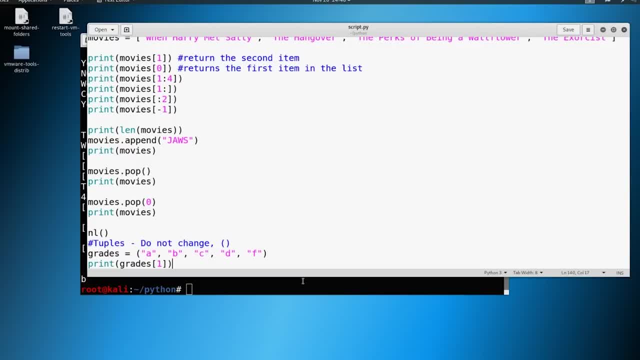 this course, especially when we get into the exploit development part of the course. so a wall loop, just think of it that it executes as long as something is true. so let's make a new section here. we're going to do a new line, as usual, and we're just going to go ahead. just say something. 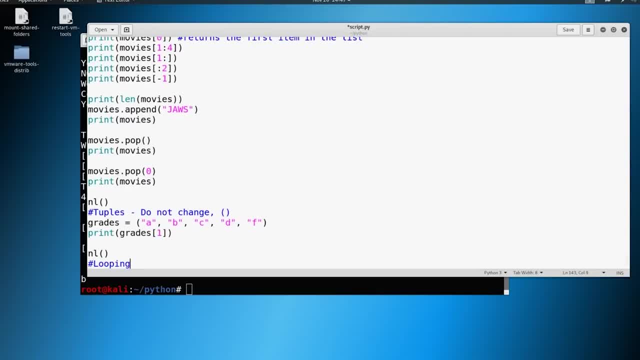 like looping and let's go ahead and start with four loops. so we'll do four loops and let's note that this is just the start to finish of an iterate. okay, so let's say, for example, that we have a list. okay, let's go back to list. 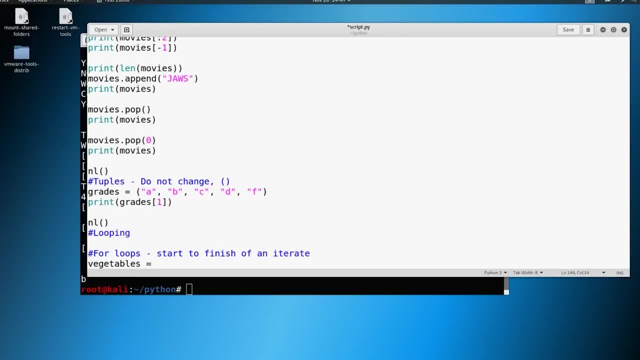 and we'll say vegetables, And let's just throw some vegetables in there. you can pick whatever you want. I'm going to do cucumber, I'm going to do spinach, And how about cabbage? Okay, And again, your list can look however you want it to look. Now for this, for loop, we're going to say for. 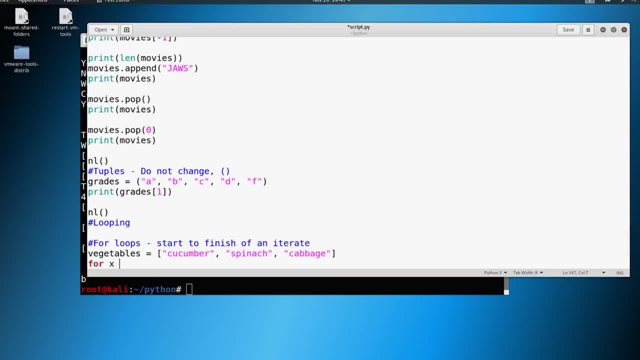 x. And remember same thing with bash: x can be whatever you want to call it. you can call this for veggies, you can call it whatever you want. I just like to use a letter because it's simple to type out. we're going to say for x in vegetables, we're just going to print x. 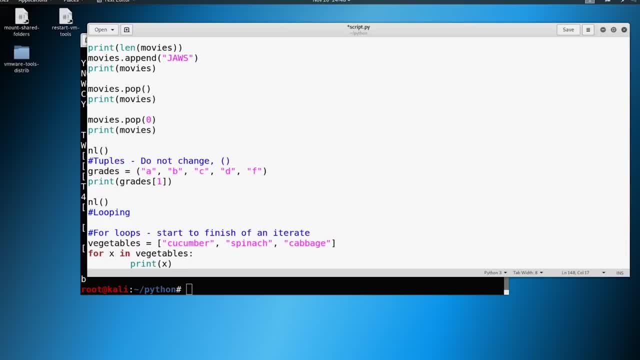 And what do we think this is going to do? This is going to go through this list, right? It's going to say: for every item in vegetables, I want you to print that out. So we're going to grab cucumber, we're going to grab spinach, we're going to grab cabbage. it's going to print, print. 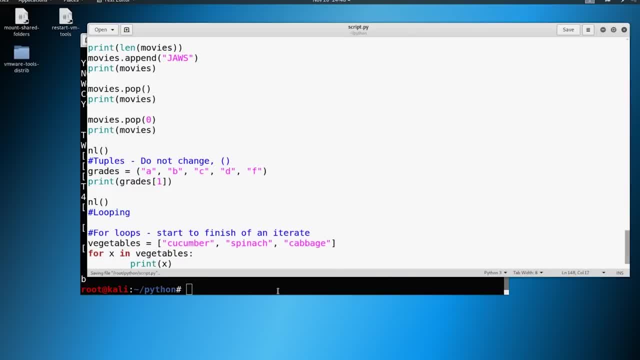 print. So let's take a look at that, Let's go And save it. We'll run our script here. You can see that it printed cucumber, spinach and cabbage. So again, you've seen this before. just a classic example of a for loop. As long as we 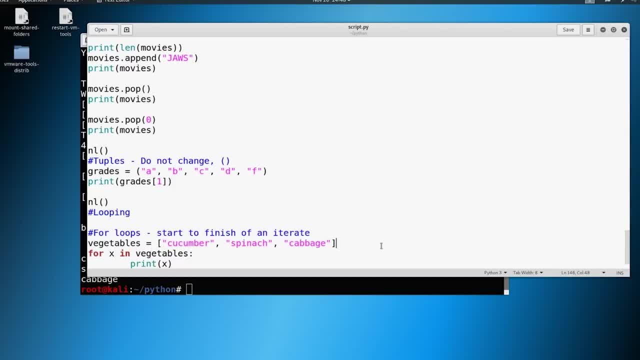 have something to iterate through. we're iterating through a list here And remember, before again we were like sequence one through 255, we iterated through that to do our ping sweep. So we're just iterating through something. That's it really basic Now. 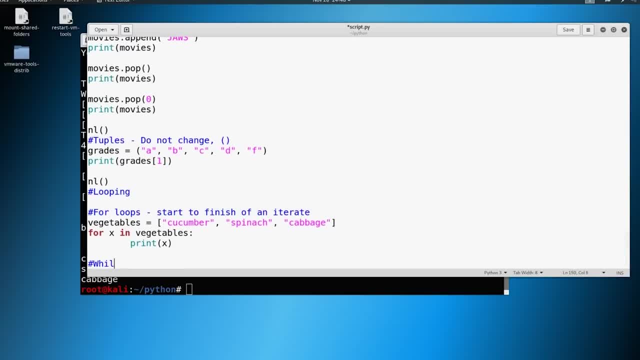 we also have a list here, So we're going to go ahead and save it. We'll run our script here. We also have while loops, So we'll say while loops and these execute as long as true. So later on you're going to see something that says: while true, the capital, while true, we're going to do. 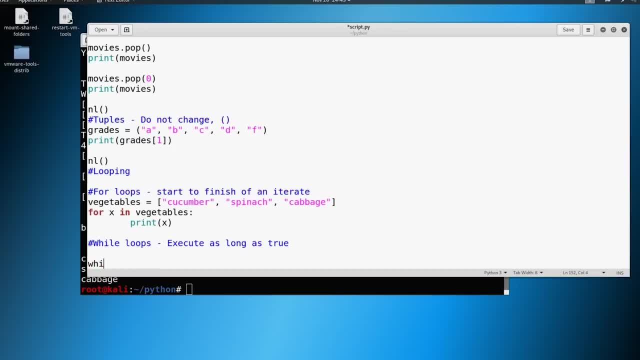 something. Don't worry about that right now. For this example, what we're going to do is we're going to say I equals one. Okay, And so we say I equals one. And then we're going to do something: set a variable- I that's equal to one. Now, let's do a while loop. we're going to say: well, I, 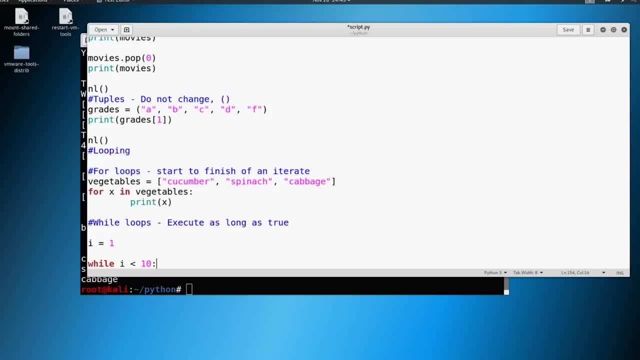 is less than 10.. I want you to go ahead and print out I, And then we're going to iterate: I plus equals one, So this should all start tying together. from what you saw earlier, Remember that we have the plus equals and we're adding one to something. So what we're doing here is we're. 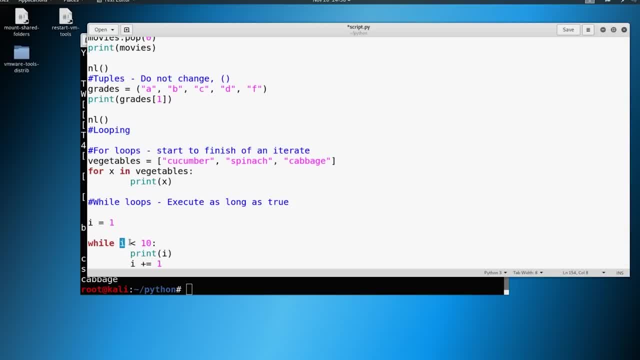 saying: hey, I equals one. And you know what, while I is less than 10, I want you to go ahead and print out I. then we're going to say, hey, I is plus or equal to one, So that means I is now going to be two. 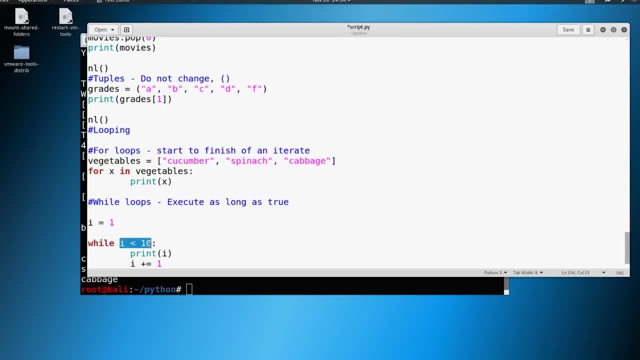 Then we're going to go back through this loop again. Now, while two is less than 10,, go ahead and print out that it's to make it three. three is less than 10,, over, and, over, and over and over, until this condition is no longer true. The second that this I becomes 10,. this loop is now no longer. 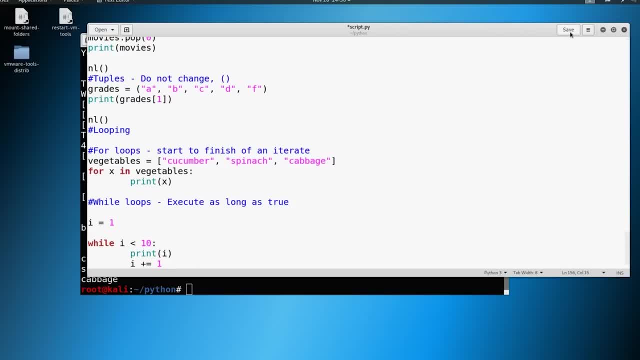 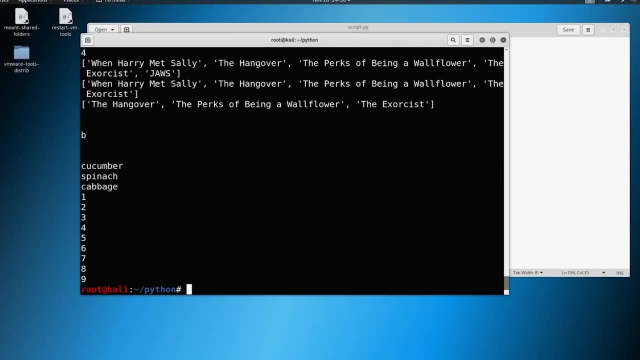 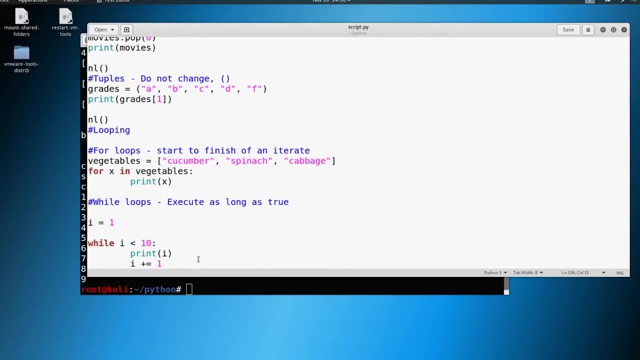 true, and it's going to stop. So we're going to go ahead and save this here. Let's go ahead and print this out, And you can see that we just printed one through nine, as expected. So you're going to get to see these again. you're going to get examples of them again, as of right. 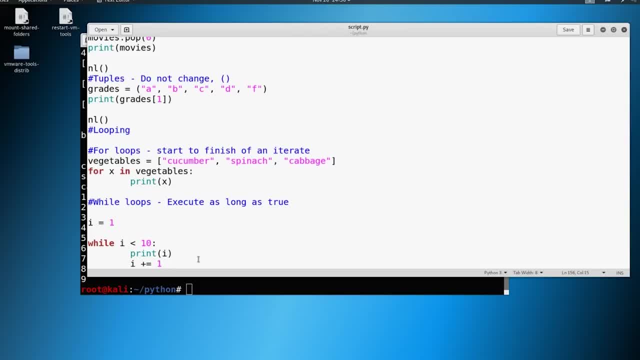 now I just want you to understand that a for loop isn't it, And a while loop executes as long as true. Okay, So don't worry about it for now how they're used quite yet. Just understand what they are, what they mean, And then you're going. 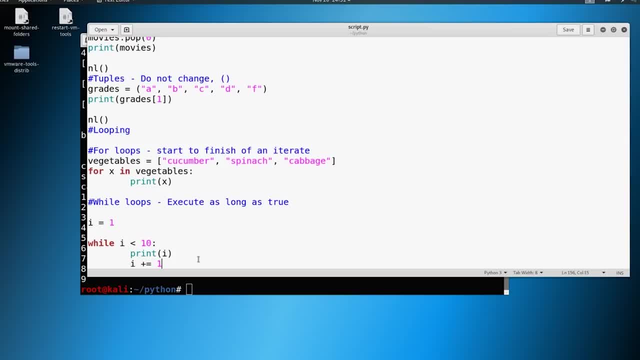 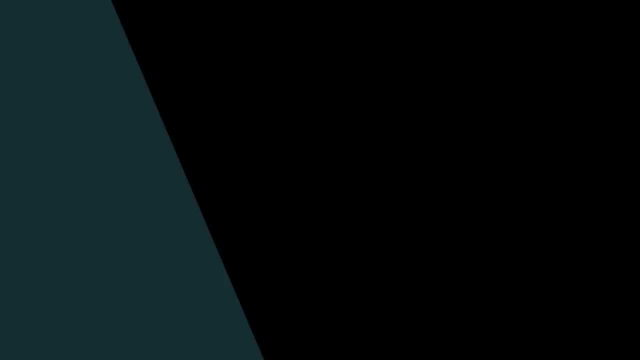 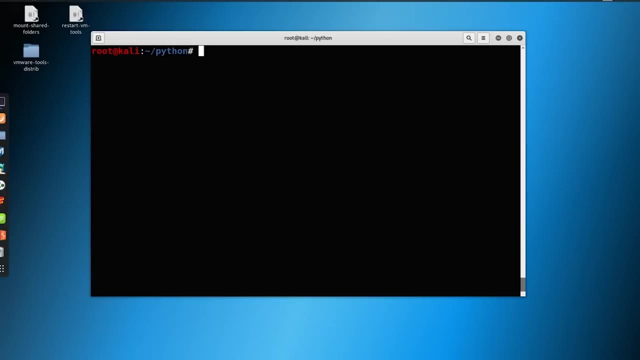 to see them come up in practical examples Later on. it'll make a lot more sense as we go through it. So we're going to move on to the next video. I'm going to go ahead and catch you over there. Okay, we are moving into. I don't want to call it advanced Python, I just want to say more advanced. 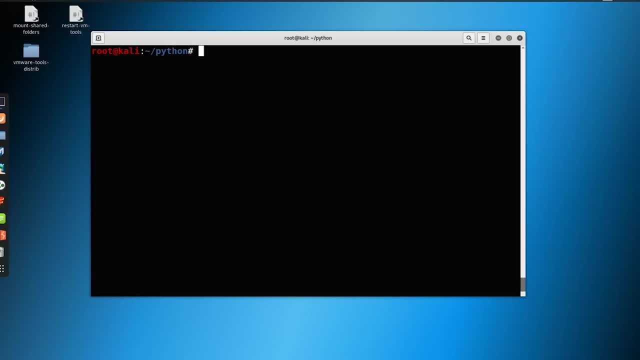 than where we were before. If previously we were in a one on one class, we're moving kind of into some 102 material. I wouldn't even call it to a one material. This is just more advanced beginner stuff. How about that? So what we're going to do is we're going to go ahead and start a new script. 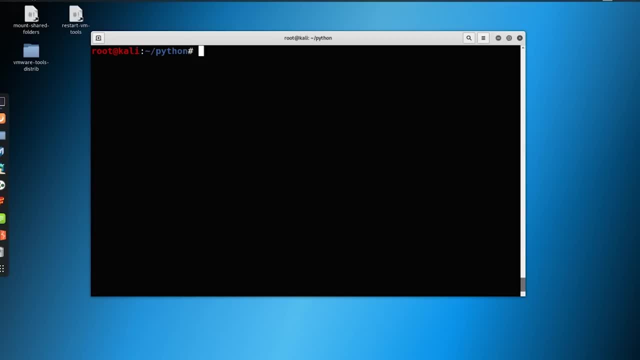 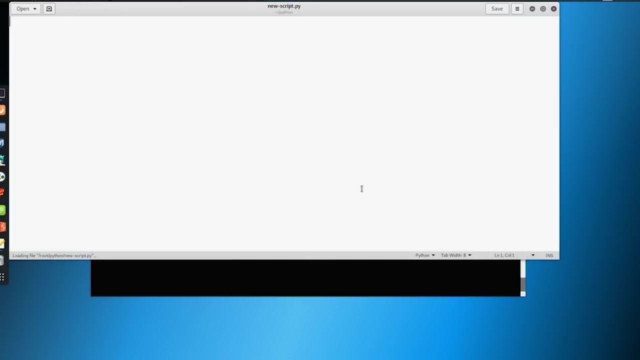 That way we can kind of have our new 102 section here and kind of improve upon what we've been doing a little bit. So what I want you to do is I just want you to g edit And we'll just call this new script dot pi. put a little ampersand at the end as usual, And we're just 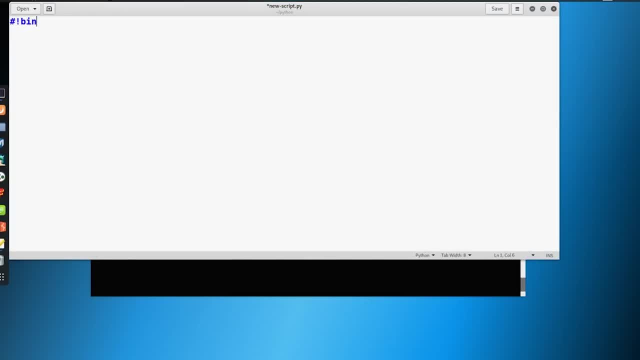 going to declare our bin bin Python three here. I can type it out: bin Python three. And we're going to go ahead and talk about our first concept, which is going to be importing. So importing is important. When we say importing, 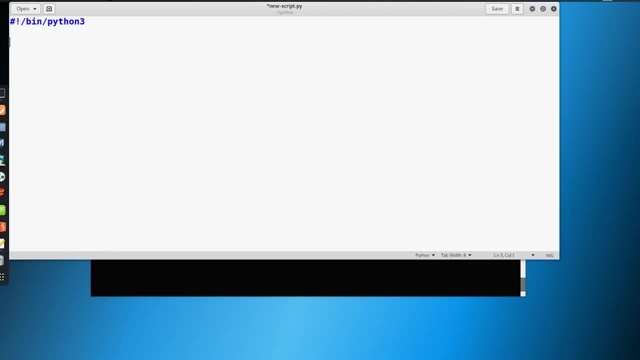 modules are existent in Python, right, And we have a lot of them built in, But there are these modules that are not built in but available to us, For example, a module called SIS. Now, SIS does a lot of important things. SIS has to deal with anything related to system functions and parameters One. 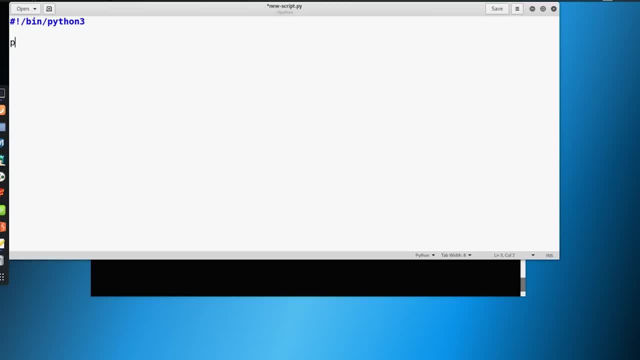 system function and parameter. that we can do is something like printing out the version of Python that we're running, So you could say: print SIS dot version version. Okay, now, if we go to do that and we say save and we just go ahead and say Python three. 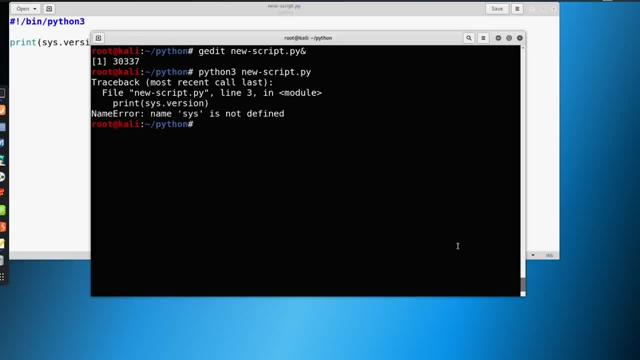 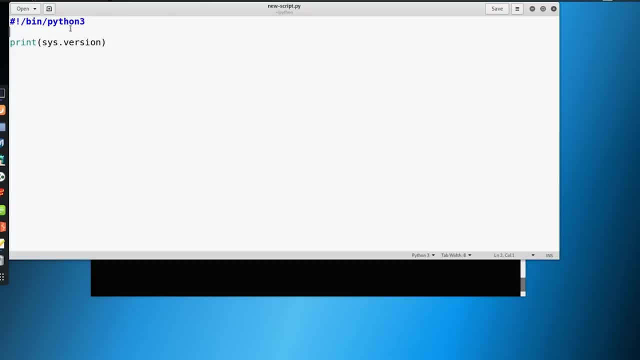 new script up high you can see the name of sys is not defined, So we're getting an error here. Well, that's because we haven't imported it. So we can do is we can say import sys And up here we can go ahead and just give this a nice comment next to it And we can just say: 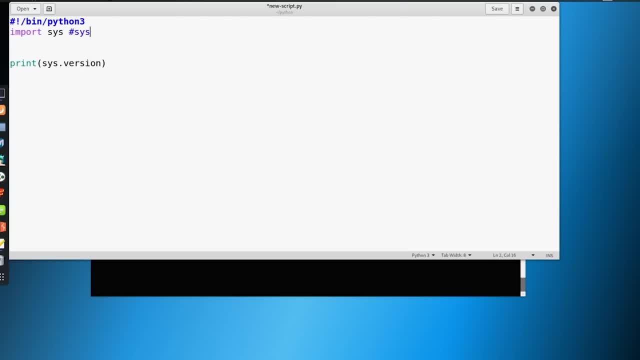 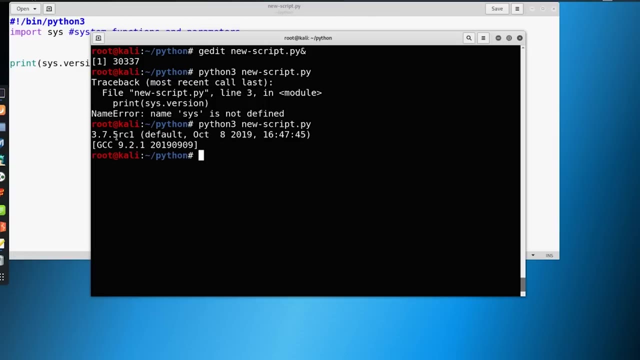 that sys is a system, a function and parameters. Okay, and then let's go ahead and save this. And now let's go and run it again. Now you can see that we are running Python 3.7.5 RC one. 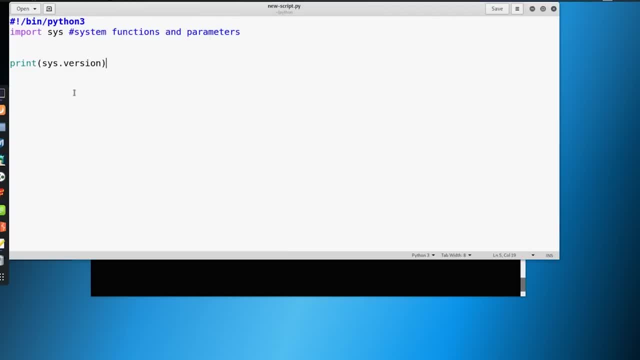 And we have now successfully printed this out. Why did this work? this work because sys does not by default come imported. Some items already built in by default. sys is not one of them, But sys is very important And we're going to use it over and over again, So you're going to see it a lot. one of the most frequent, if not the 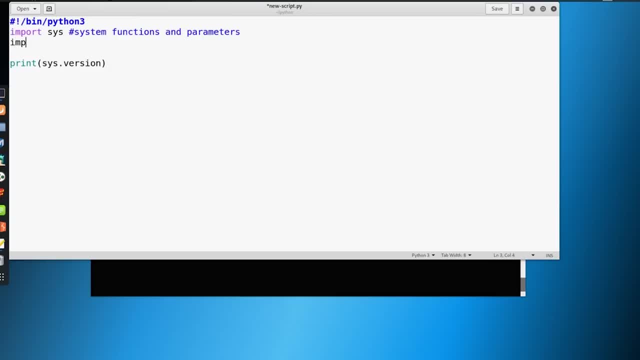 most frequent along with OS is another one: import OS. you're going to see a lot of that over and over. So why are we going to see this? Well, we have things like arg v. So arg v is arguments. So when you think about from the bash the lesson like dollar sign one. 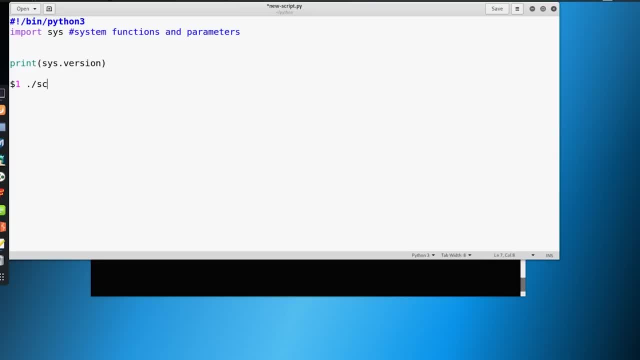 you know, when we had an argument, we were doing our ping like our script dot sh, And we had our IP address here as dollar sign one, something along those lines. Well, those are the same thing. We just call it arg v in Python. That's something. Another thing is if we want to say: 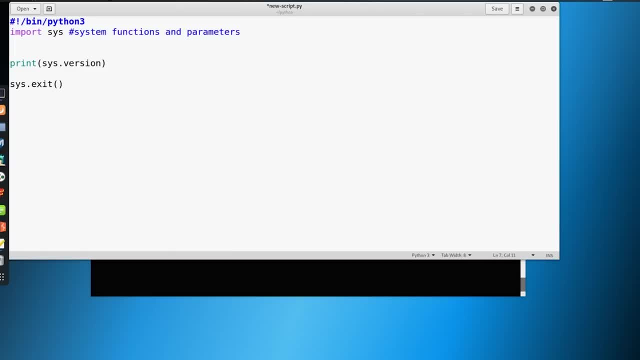 sysexit, which you're going to see again later in this course. we do a sysexit that exits Python cleanly. we need a sysexit, So you're going to see sys quite repeatedly. On top of this, there's more things that we can do with modules. let's go ahead and delete this And let's say that. 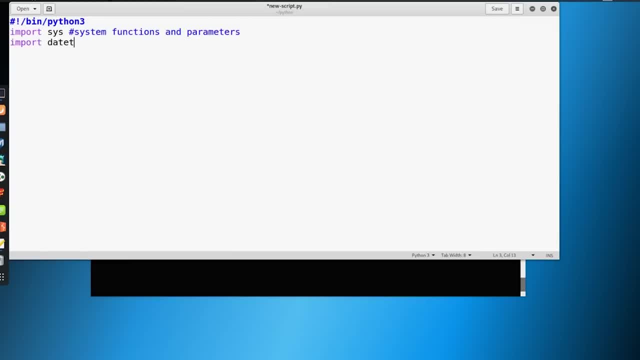 we wanted to import another module called date time. Now this does exactly what you think it does. But what if we wanted to import a specific part of date time? we didn't want to import the whole thing, we just want to import one module. we can say: from date time, import date time. So we can. 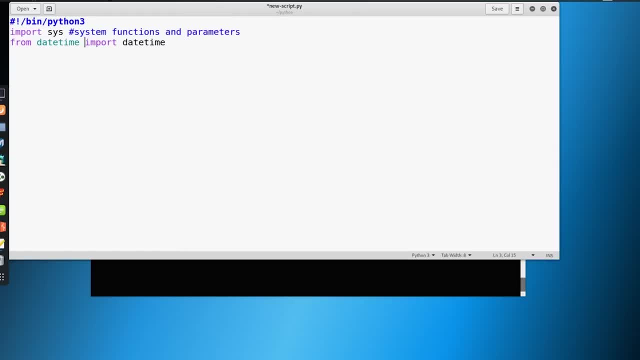 do the same thing with sys. we can import a specific part of sys, we can import a specific part of sys or we can import all of sys. So with date time we're importing a specific part of it, right, And we can do something like print date time- dot now something like that, And it should print us the. 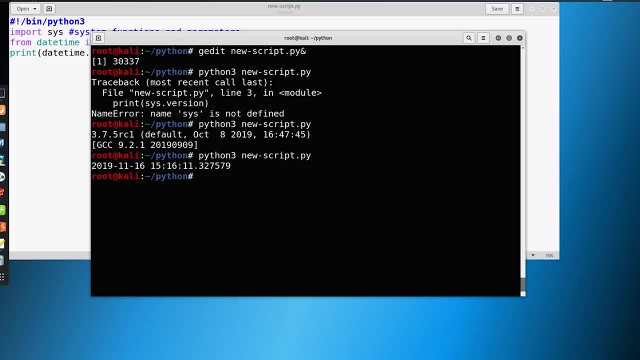 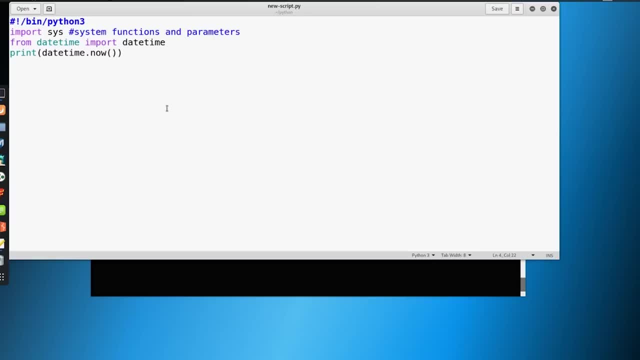 date time. So do this. You can see now, today's date is 1116 2019.. And what time we're recording. So we can also do. another nifty feature: when it comes to importing, we can import with aliases. So, instead of from date time, import date time, we can say: 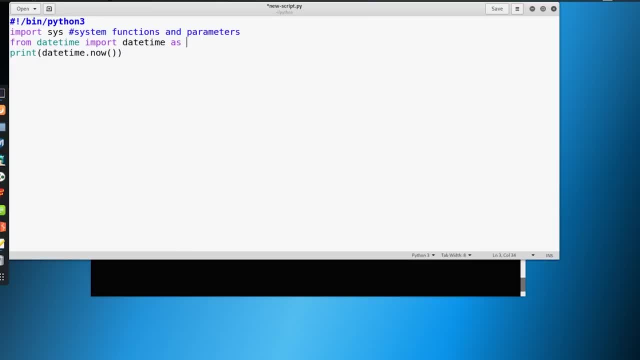 import date time as something like DT. you could say import with alias And instead of having to write date time dot now over and over and over, something like that, we can just write: DT is shorter, we know what it means And we don't have to write out date time, which is kind of lengthy. 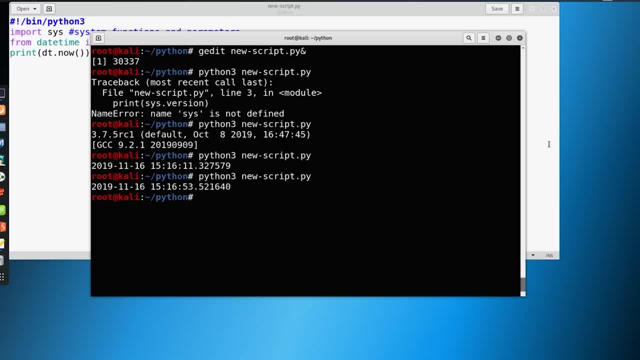 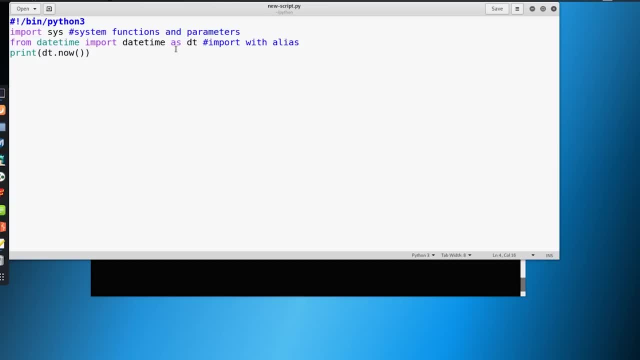 So print it again. you can see it still works. So importing is important. I'm going to say it again. you need to know that we're going to be importing certain modules out of Python. most of these are built in. there are occasional times you're gonna have to go out and download something and put it. 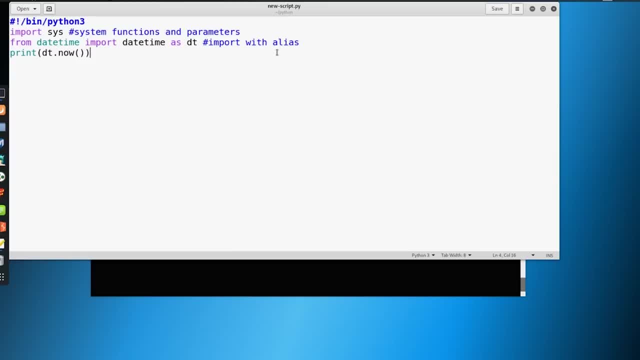 in your library and import it that way. But for the this course that we're doing, you're only going to be importing from things that are pre existing with Python, So not everything is automatically ready to go. So we're going to be importing from things that are pre existing with 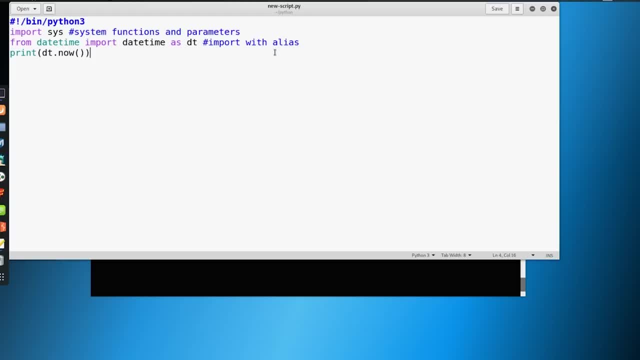 Python. So sometimes you have to import things in order to improve upon your script or do make it do what you want to do. So we're going to build off of this when we start writing our scripts, And you're going to see this repeatedly. you're going to also see this again when we do our 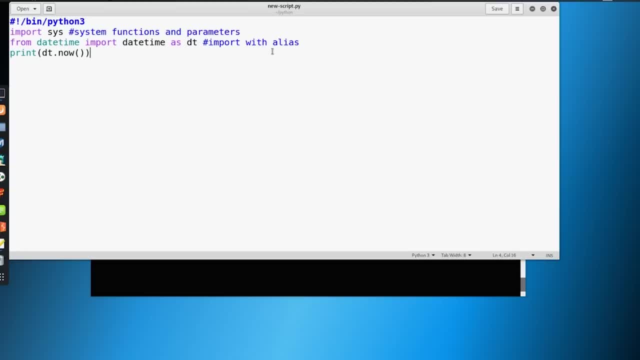 exploit development part of the course. So let's go ahead and move on. we're going to move on to some advanced strings And we're going to get close to wrapping up here and start building out some cool little Python scripts. So I'll see you over in the next video. 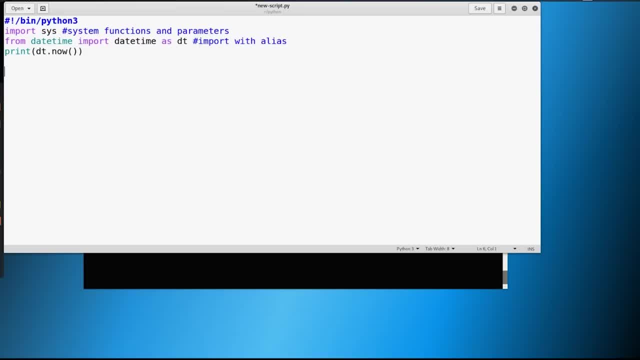 Okay, let's talk about advanced strings. So everything I'm going to show you is not going to be used in this course, But I still think it's important to know- And there's some important syntax in here to know as well, and just different ways to handle the information that is in front of. 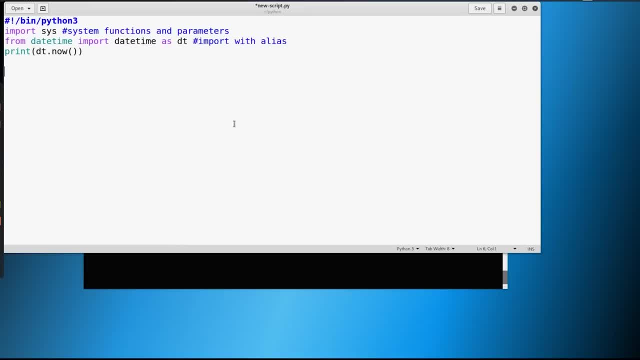 you. So let's go ahead and just print out a string, or let's make a string first. let's do a string of my name And we'll just say my name is Heath, And so, similar to before, if we printed out our name, we could say: print my name And then, if I wanted to, 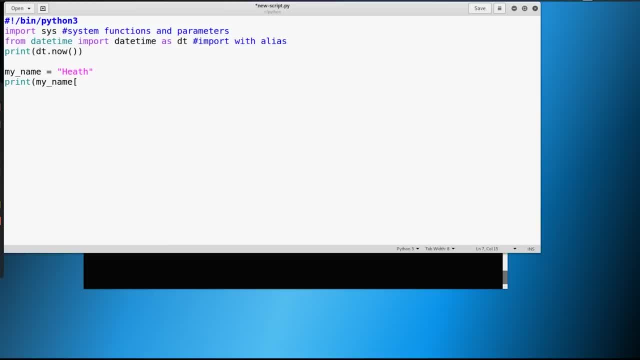 print the first initial of my name or first letter in my name. I would just do something like this, right? So this should be familiar. And if we wanted to print out the last letter, we could say negative one. this should be familiar to you from the list lesson. So we go ahead and we print this. 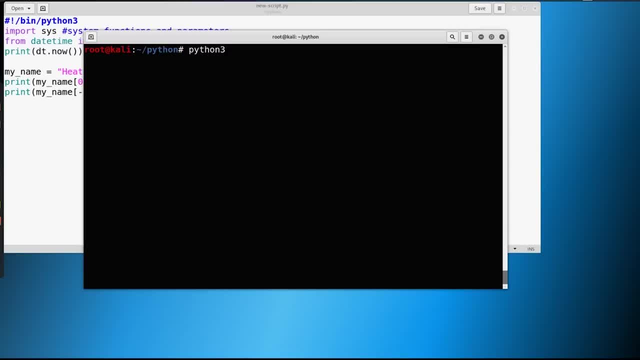 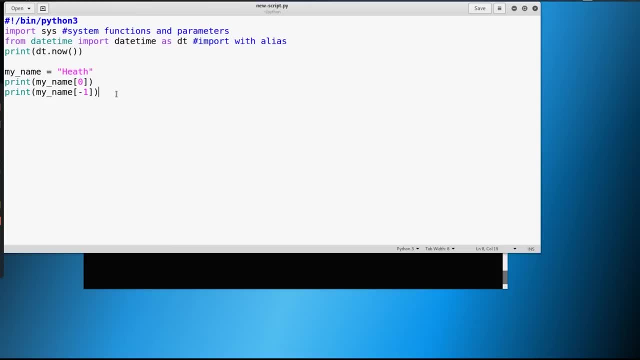 we just say Python three And we do our new script again. you could see that we have big H and a little h, because my name ends in both starts and ends in both. So we could also do something like: take a sentence And we could say: sentence, this is a sentence. 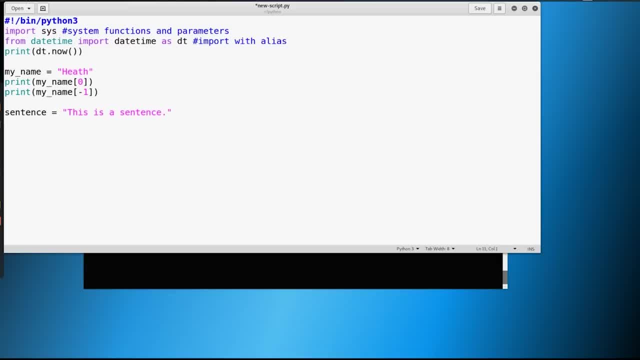 And if we wanted to print out the first word of the sentence, we would have to to know the amount of letters in it. so we know here that there is one, two, three, four. so this would be zero through three. so let's say, if we wanted to print out sentence here and we knew, 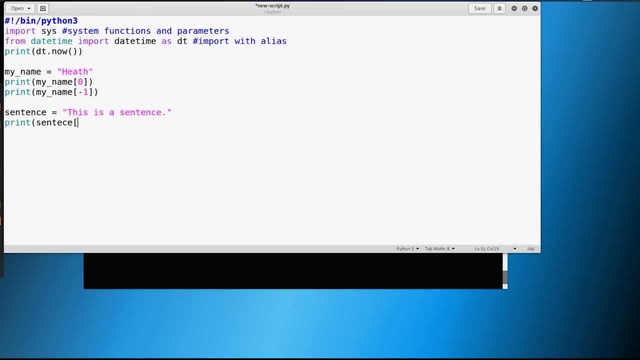 zero through three. so remember, we don't have to put zero. we could just put something like this: and then if we did through three, it would only cut off at the. i remember we have to go one further from our list lesson and we'll be able to print out the word this. we can do the same with sentence. 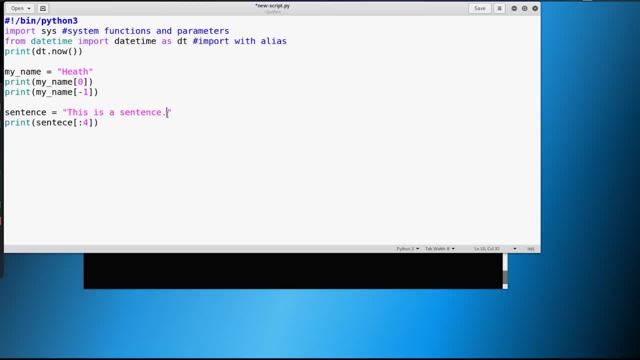 we could go forward a bunch if we want to. or we could do a negative nine, because this is nine characters long. through something like a negative nine through negative one would pull out that whole sentence or the word sentence i should say. so we can manipulate data this way. we can also. 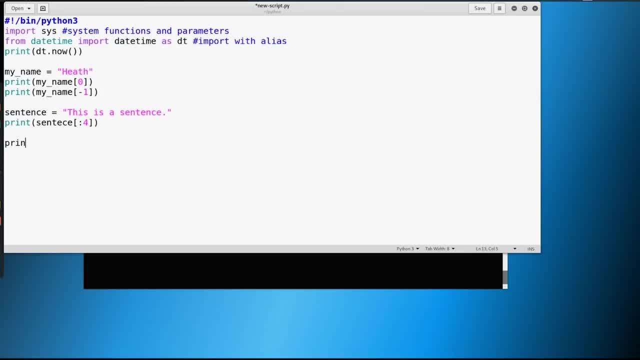 split data. so we could say something like: and do sentence dot split and this will split based on a delimiter. now the delimiter here is by default a space, and we cover delimiters in bash scripting and we're just going to say: hey, every time there's a space, i want you to split out this sentence. let's take a look at. 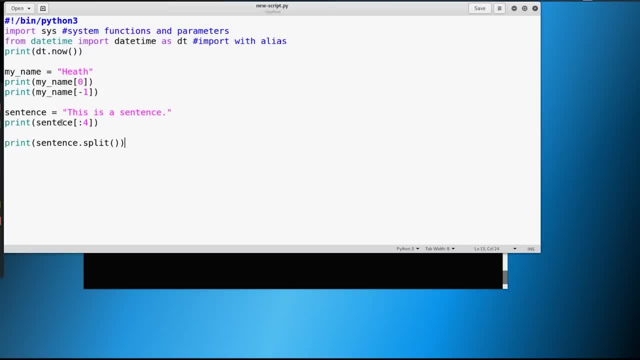 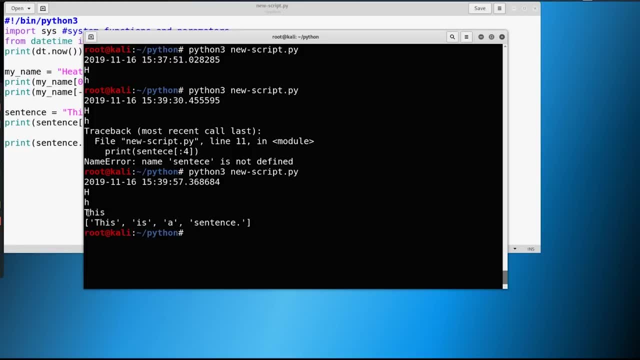 what that looks like. i made a mistake in my script. i didn't spell sentence correctly, which caused an error in the initial script, so let's try that again. so you see, here it says this: that's what we're expecting from this one. and here we have. this is a sentence. 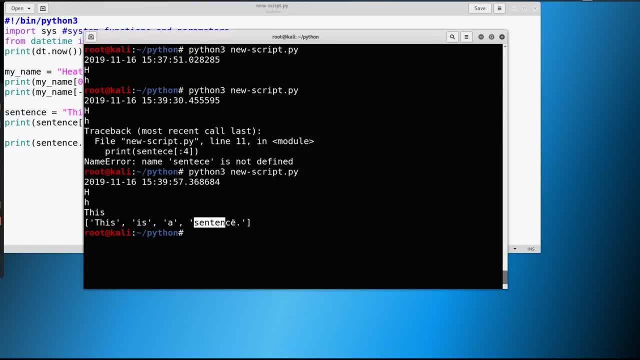 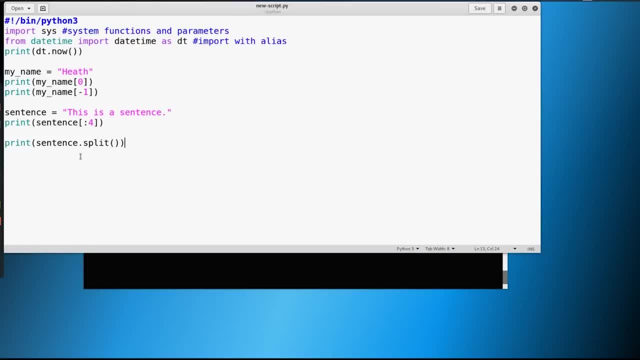 it now breaks these out into individual words based on a delimiter. so let's go a little bit further. we can join a sentence as well. so let's have a scenario here. let's say we want to split a sentence out. we'll say: sentence split is equal to sentence dot split. 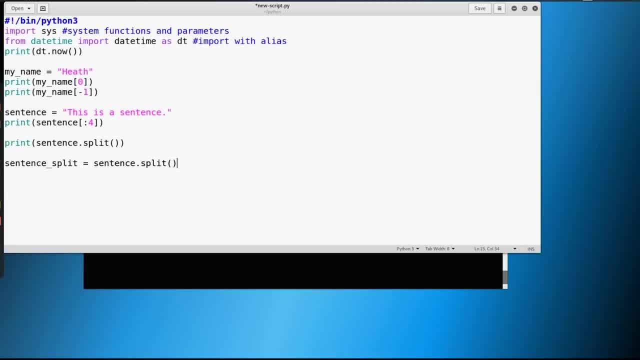 and now we just split out the sentence, right, and we're putting in this variable of sentence underscore split. now we could also join a sentence. so let's make a new variable and we'll call it sentence join, and here we can just say: based on a delimiter. i want you to. 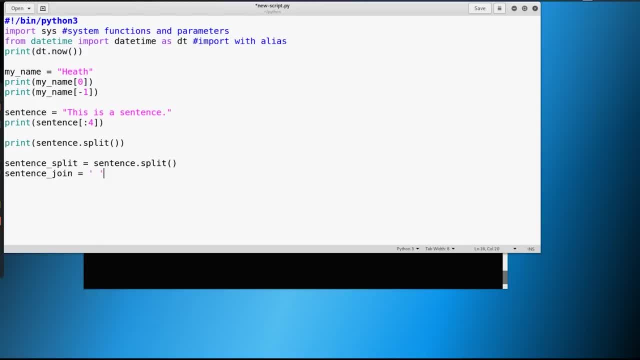 put a space in between everything here. so every, every time you see a word in this sentence split, so let's go ahead and join. anytime you see sentence split here and there's a new word in it, i want you to go ahead and join those with a space and then we can go ahead and print out. 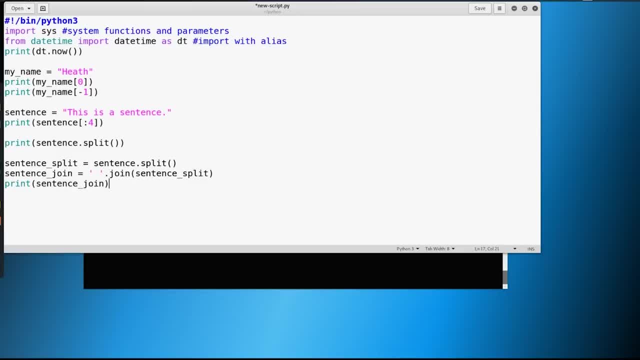 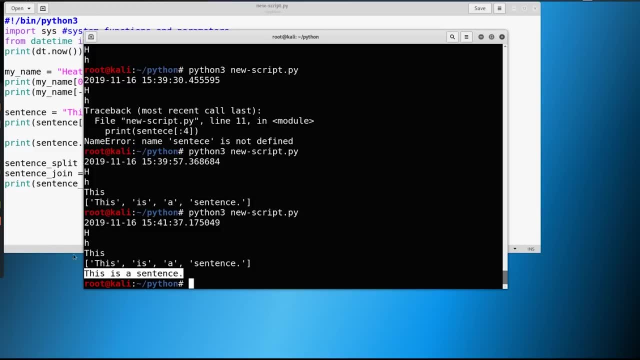 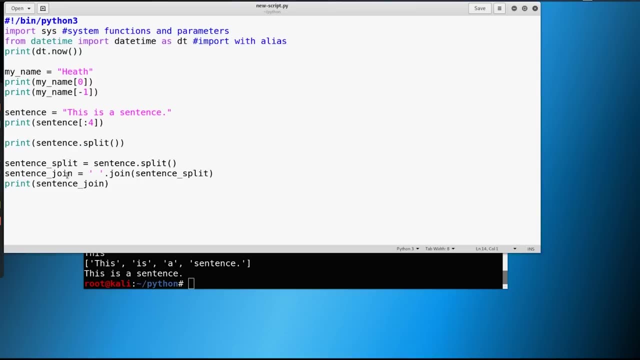 sentence join, and let's see what happens here. this is a sentence, so it brought it all back for us. so not only can we take away and delimit a sentence by splitting, we can also join a sentence and add our own delimiter in there as well. so one of the most important things that we need to talk about is what happens if we have a quote. 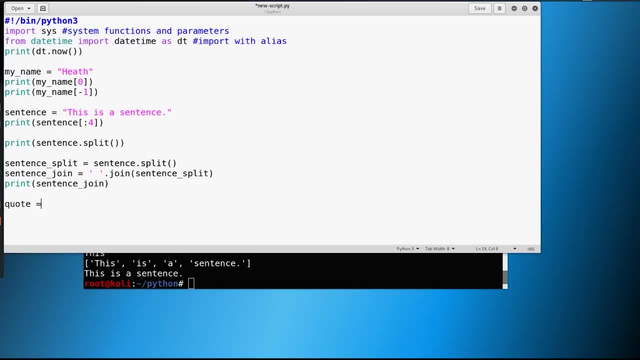 and we say something like he said: give me all your money. well, we need to add quotations in here. but if we do quotations like this, well that's just making things really weird. right, look at the color of the script. you can already tell we're going to use. 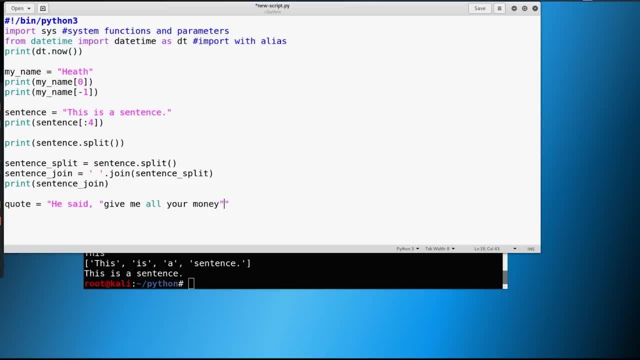 this as well. it's going weird. that's going to throw an error, But we can use single quotes and double quotes and it'll work. We could also use single quotes here, double quotes inside, double quotes on the outside, single quotes on the inside, And that's a way to have quotes inside of a string. So let's. 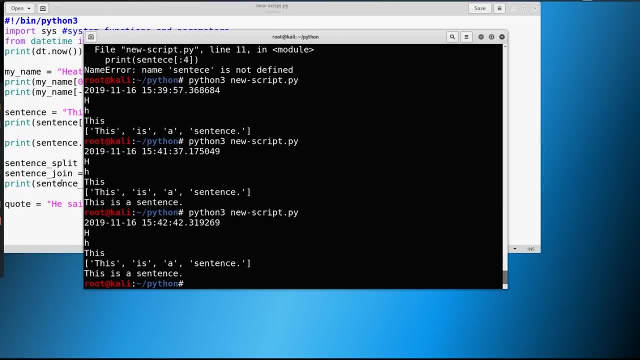 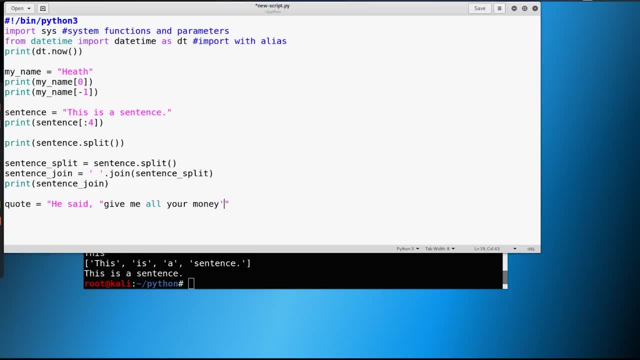 go ahead and print that out. But let's say that you were insistent and you wanted to have double quotes and then double quotes here. Well, we could do a little bit of character escaping, So we could utilize this backslash here and say, Hey, we're going to keep this string a string. And then I'm 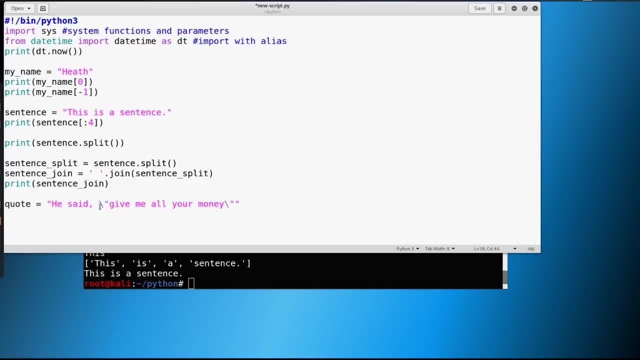 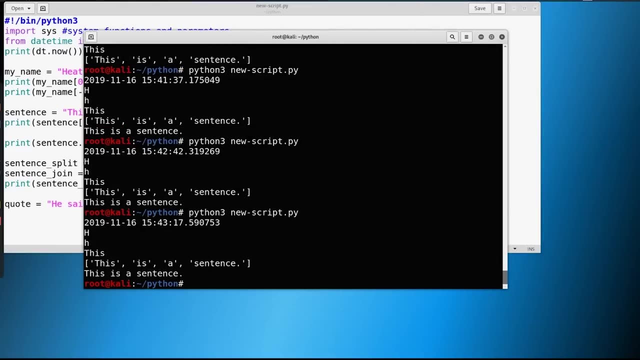 going to end it right here. So this will tell me that, from here to here, ignore these characters, right? So we're going to treat it as a string, Don't treat it as a quotation, and end up straight. So let's run it again And you can see that quote once we print it. 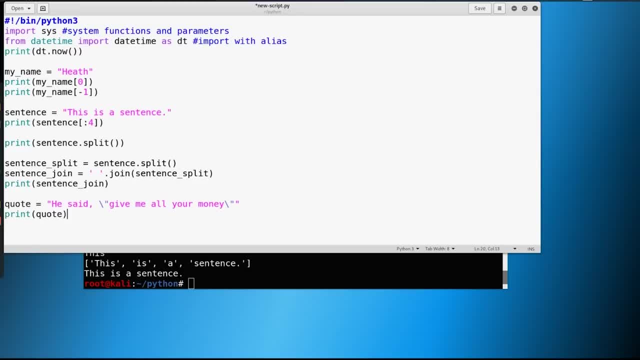 we can say: print quote And we'll actually run it here. He said: Give me all your money. And I realized that I tried to print earlier and probably did not print those quotes and never had the print in there. So I'm sorry for that, But we could do it either way. Again, we can put the single quotation. 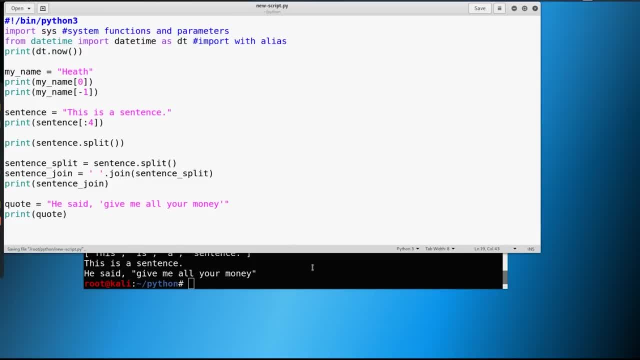 in here And you'll see the single quote works, But if we were to put in a double quotation it would break it. So I'm going to control Z a couple times And this is what the syntax should look like. This is very, very important. If there's one thing, 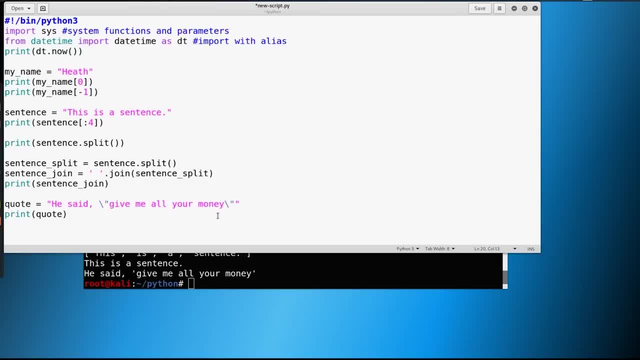 you're going to take away from advanced strings, please, please, take this away from it, Because you need to know how to do some character escaping and that you will encounter that again in your career. So a couple more things. Let's say that we want to have a string here. Let's say we'll 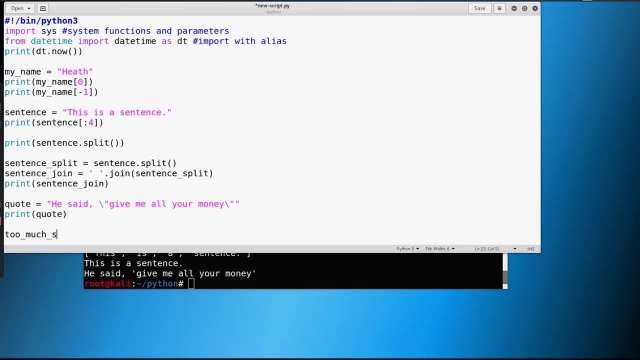 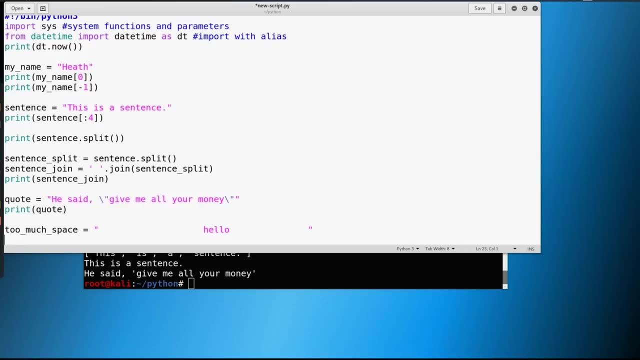 call the string too much space And we have something like: Hello, and we just, you know, copy data put into this and somehow too much space in here. we can strip out the space, So we can just print too much space here And we can do the same thing. 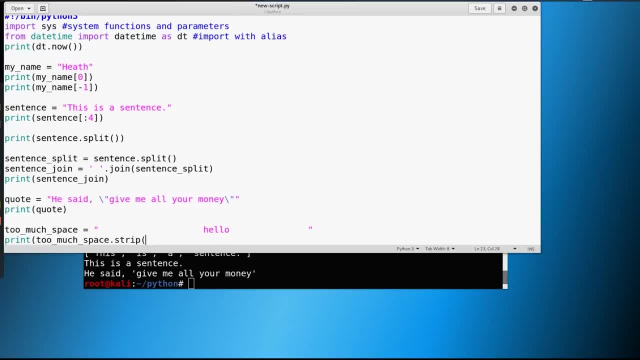 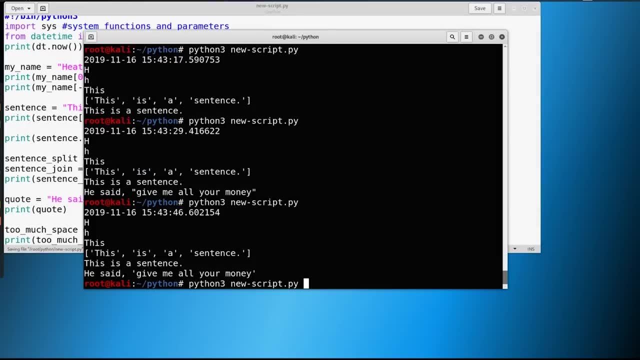 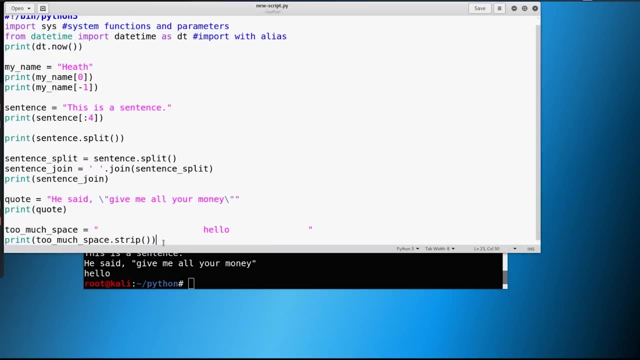 as we did before, And do something like a strip like this, Save it And look what happens. Now it's just going to print: Hello, there's no space around it, we're good to go. So that's a nice little feature, Another feature that we should. 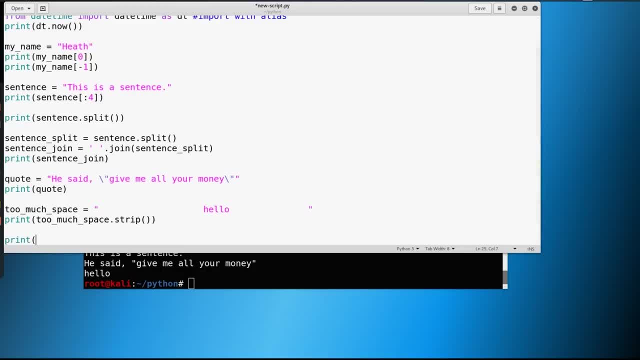 know is: let's say we had something like print a an apple. What's this going to return? True, What it's looking for is: does a exist an apple? Well, what if we did a lowercase here? Try it again And you're gonna see that it's false. 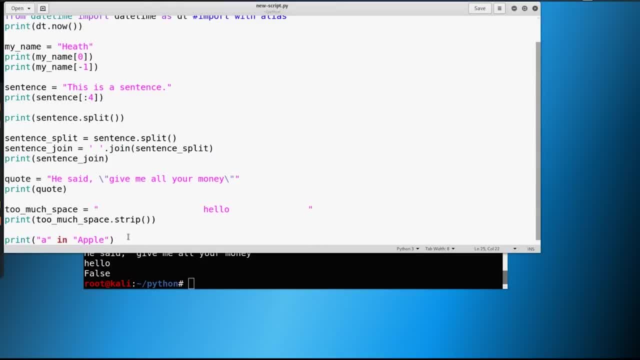 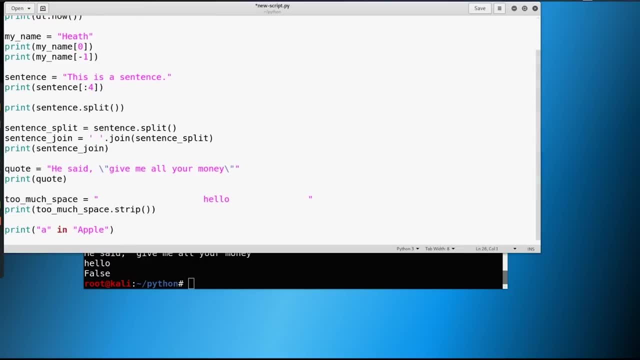 So it's very case sensitive. Well, what about? we wanted to say: hey, is there an a in the word Apple, And we don't know if it's capitalized, not capitalized? Well, we might say something instead like: hey, we're looking for a letter of a. 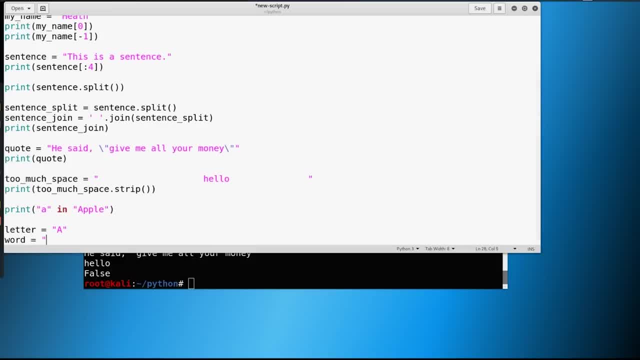 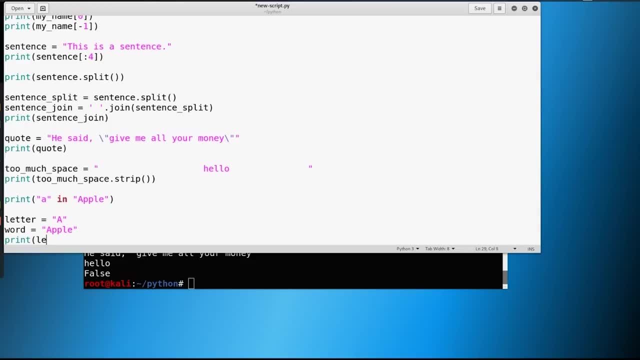 and we're looking for the word of apple- Right. But what about we say print letter- dot lower- Right. then we say in word, dot lower, like this: Now this becomes improved because we're looking for a specific letter inside of specific word, And when we lowercase everything, we lowercase this letter. 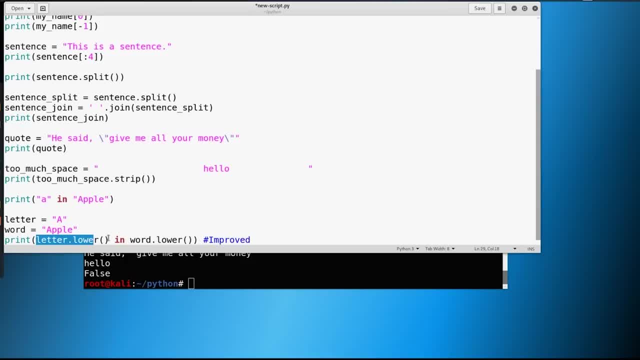 lowercase all these letters, then we're looking for a specific letter. in a word, we don't have to worry about case sensitivity, And you will see this logic come into play when you're thinking about looking for specific items or specific key phrases or matching anything specific you might. 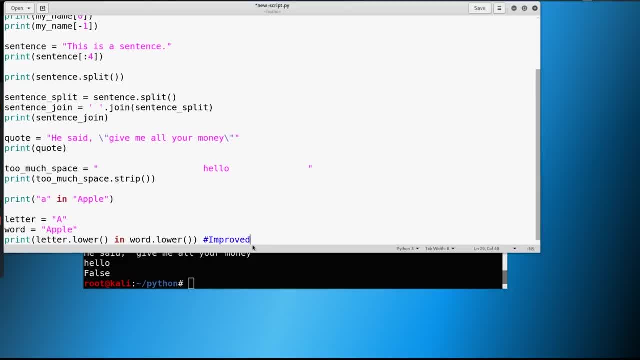 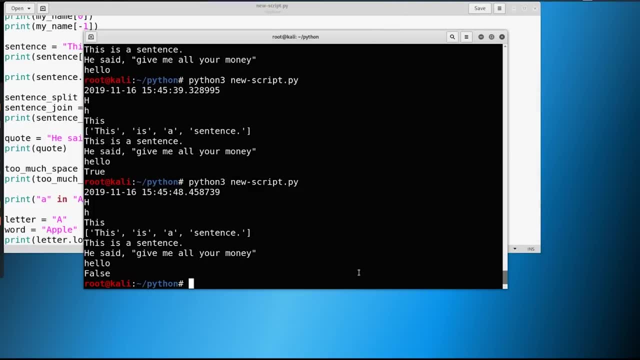 want to consider putting everything in the lowercase and then trying to find it that way, unless you are critical on case sensitivity. So this will probably come up again in your career as you look at code. So if we run that again now, you can see that it returns back, true? So one more. 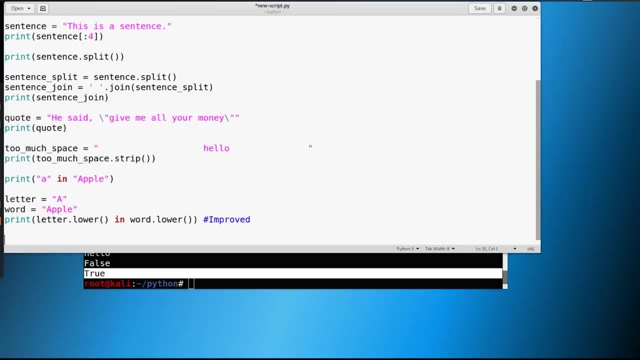 thing I'm going to show you, and there's a lot of things that we can do with advanced strings. I don't want to be too much into it, but I want to show you how to do that. So I'm going to show you how to do that. So I'm going. So one more thing I'm going to show you, and there's a lot of things that we can do with advanced strings. I don't want to be too much into it, but I want to show you how to do that. So I'm going to show you how to do that. So I'm going to show you how to do that. So, because I really 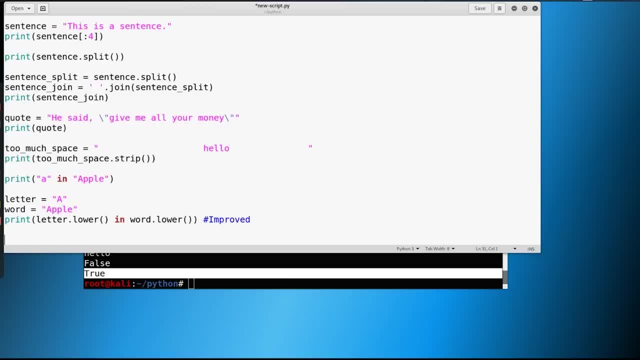 feel that this can get into overkill, because there's so many things and tips and tricks that I can show you, But I really feel like some of this can be out of scope for the course. But I do think that, as long as you're taking good notes and it's valuable now, you're going to have that. 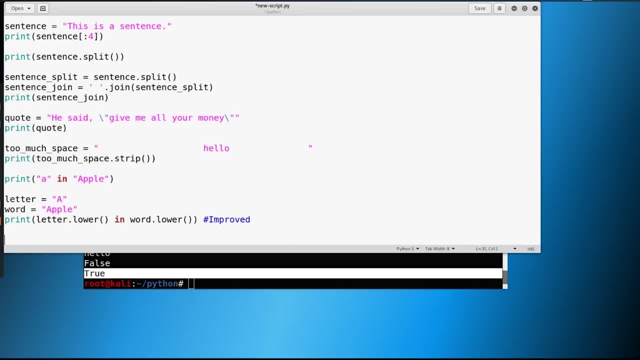 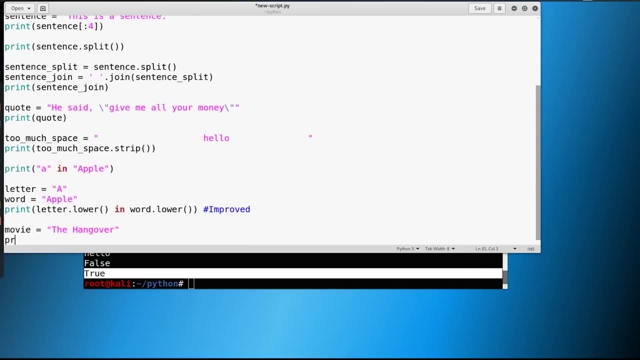 as something to remember and look back upon as you do more Python development. So one more thing is a format. So let's say that your favorite movie is The Hangover And we'll just keep that as a string. And let's just say something like print: 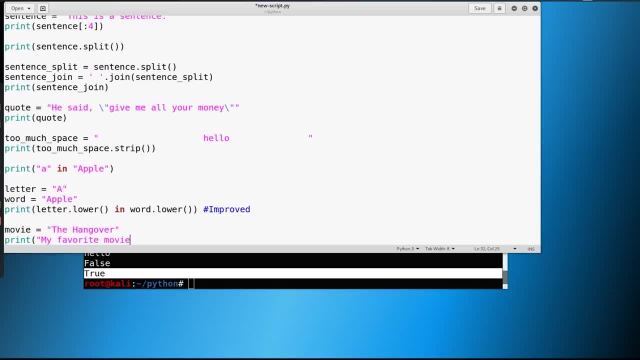 My favorite movie now we have done in the past is: and we could just say something like this: plus, you know string. if it's not a string, or we just say movie right, And then we'd have to add a period in here, something along those lines: we can improve upon this. 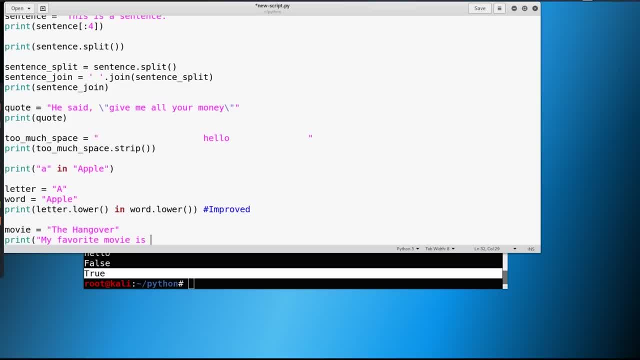 We could say: my favorite movie is, and then we can just add a little placeholder here and then put a period. Now, what we do after this is we just say dot format, And then we say movie, And now it knows to put in the movie that we have here For the variable that we have stored in. 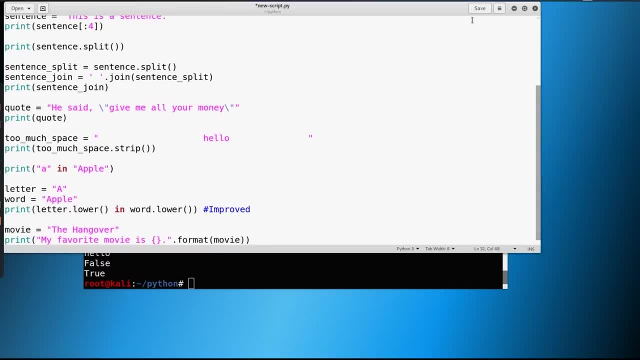 movie, it knows to put it into these brackets. here we save this and watch what happens. My favorite movie is The Hangover, So you don't have to do a bunch of spacing And if things get weird, you know with with your, your string, or you know how to write out your sentence. 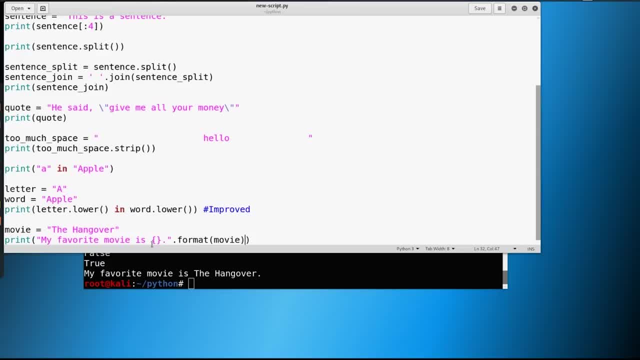 it's very easy to just have these placeholders And then if things change, you know it just updates easily. So this is a very nice way to hold things in a placeholder without making these weird formatting changes. So I like this method, opposed to the concatenation method that I showed you in. 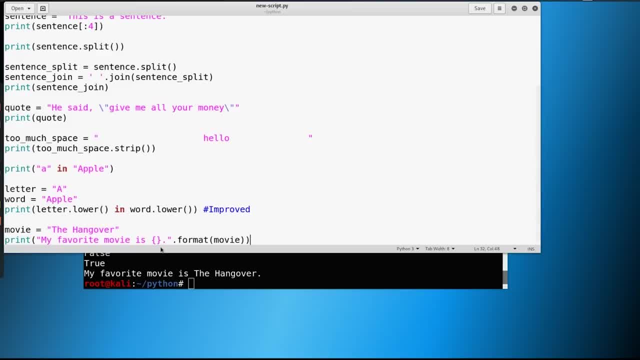 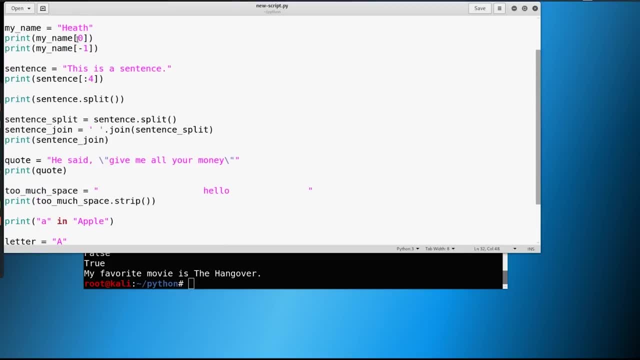 our first video on strings. So if you're going to take away some things today, just take away that. you know we have different ways of doing things. we've shown you with the list before the zero and the negative one I told you was going to come up again. just know that again, zero is the first item, or first. 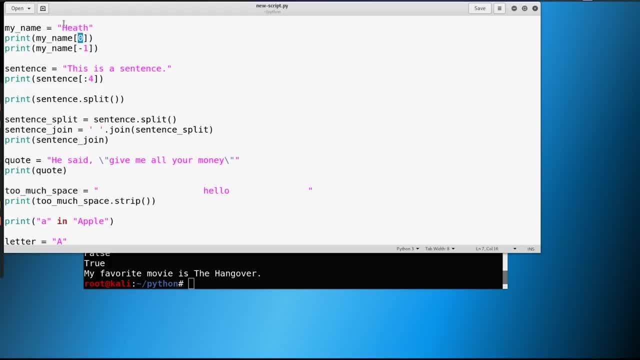 letter or first whatever. when we're talking about Python and we're talking about our variables, lists, strings, always start with a zero. there's different ways to do the same thing and apply them across other items, right? So I've shown you this with lists, I've shown you this with strings. So get those wheels spinning. 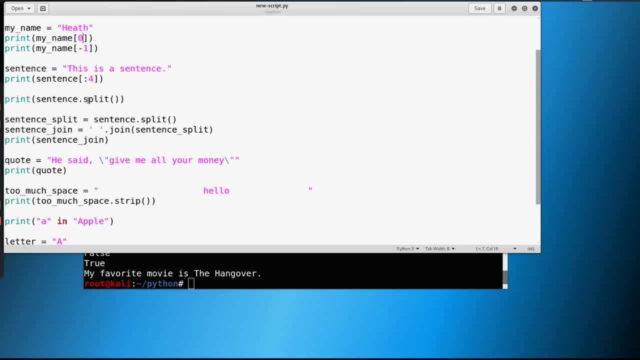 and think about how you can utilize some things. Now, sentence has all different kinds of methods that we can use with it And again we're just touching back on methods and making it a little bit more advanced. But we you see that we can split a sentence, we can join a sentence. 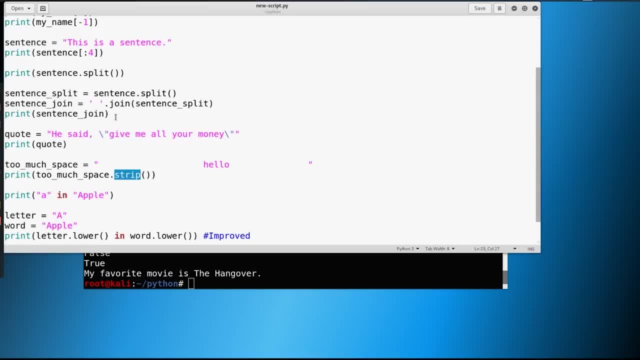 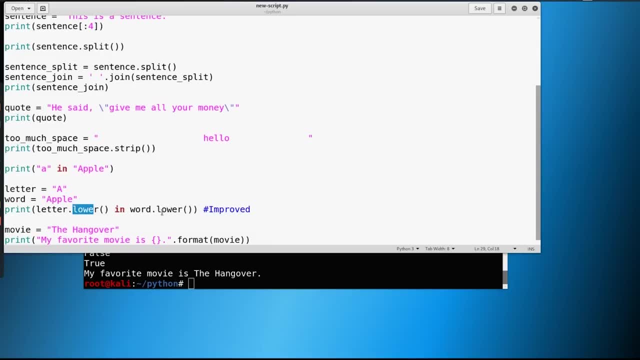 we can strip a sentence or we can strip a string. So, understanding that there are a lot of cool methods- Lower method, we could do an upper method. we talked about those as well. knowing the different types of methods per, say, like a string, or per class, or however you want to combine it together. 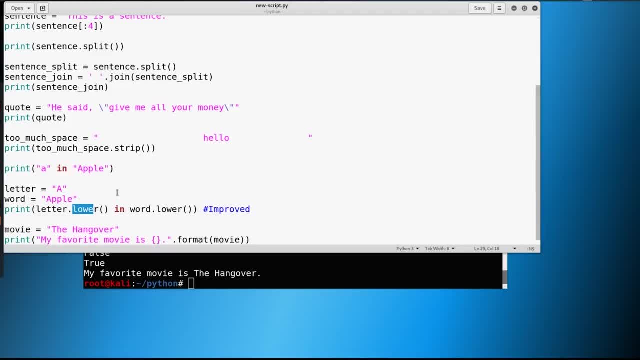 is important as well. So always do your research when you are looking into you know how can I improve it. So if you're saying like, Hey, is there a way to make something uppercase, just go to Google and say, Hey, how do I make a string all uppercase And of course it's dot upper. But if 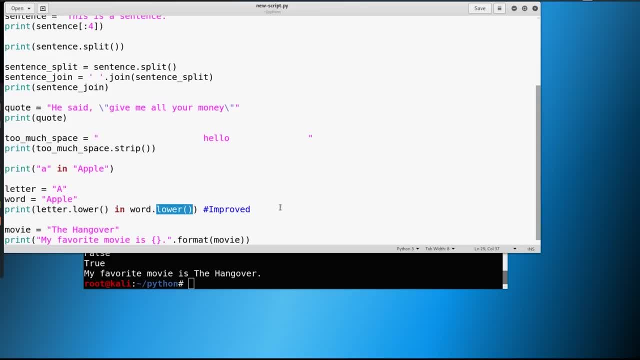 you didn't know that, then you know the Google machine would know that for you And a lot of your code is going to be found on Stack Exchange or on Google etc. So just be aware that these things exist And be aware that there are better. 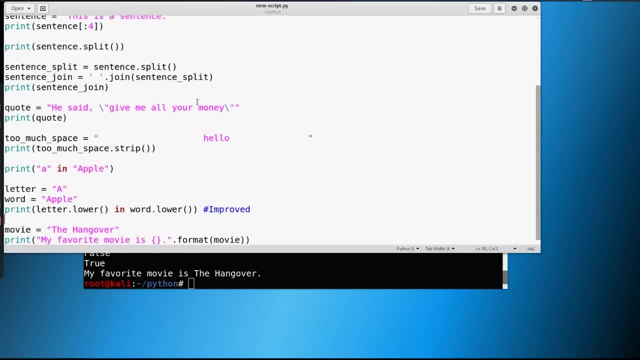 ways to format your strings, And there are important syntax when it comes to escaping your quotations as well. So that's it for this lesson. we're going to have a couple more little lessons here, And then we're going to move into script building, And then we'll be. 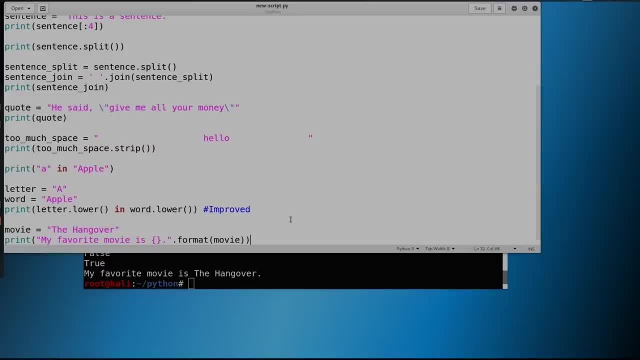 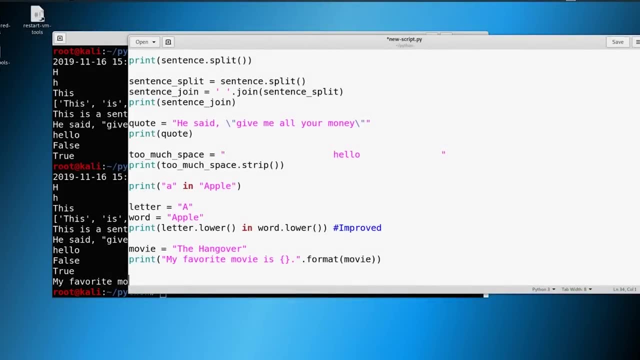 starting our hacking journey, So I'll catch you over in the next video. All right, we're in the homestretch, everybody, So we're going to cover dictionaries now, And when we think of dictionaries, we need to think of key value pairs, So let's go ahead and make a new. 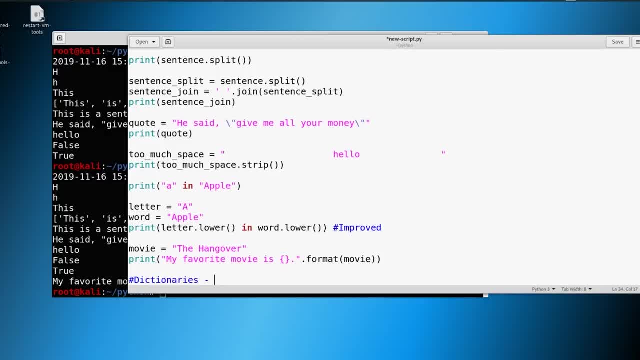 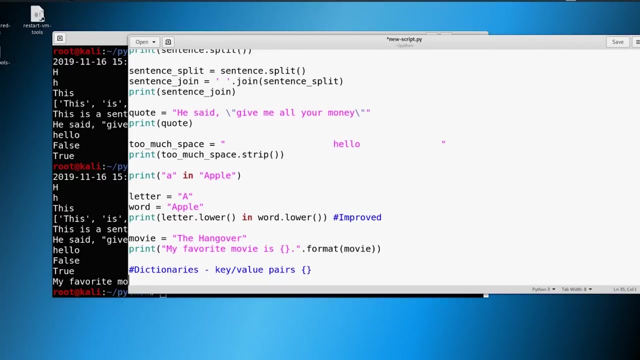 section called dictionaries And we'll just note key value pairs, probably put a slash here, key slash value pairs, And we'll also put a little note of curly braces like this. So let's talk dictionaries. So let's say we have a dictionary and we want to have a menu. 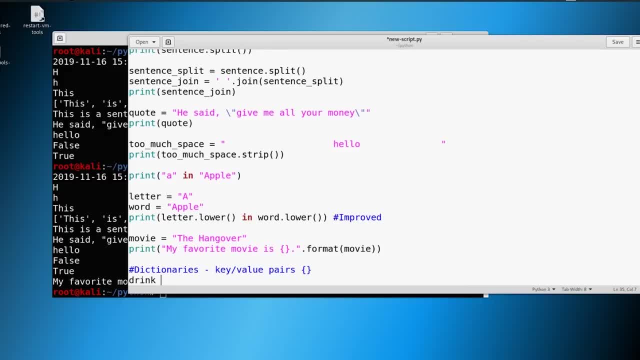 let's make a drink menu Again. make this however you want. I'm going to make this based on some alcoholic beverages. you can absolutely make this more you know: PG or PG 13,, or however you want to do it. But let's say a white Russian. we go to a bar, there's a white Russian on the menu And 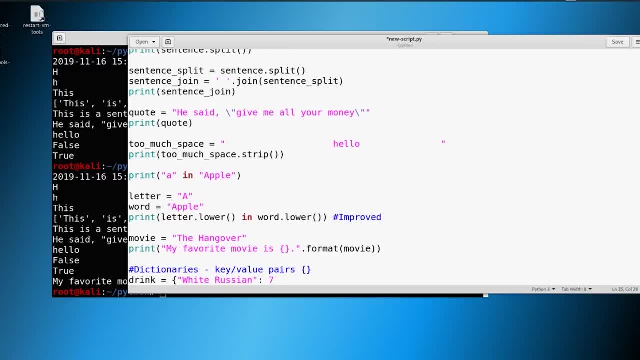 that white Russian costs $7. And there's also an old fashioned And we just say that's 10 bucks. And then we have a lemon drop which is $8.. So we've got these and we'll close off this with a curly bracket. And this is what a dictionary looks like. So if you were to print out drinks, 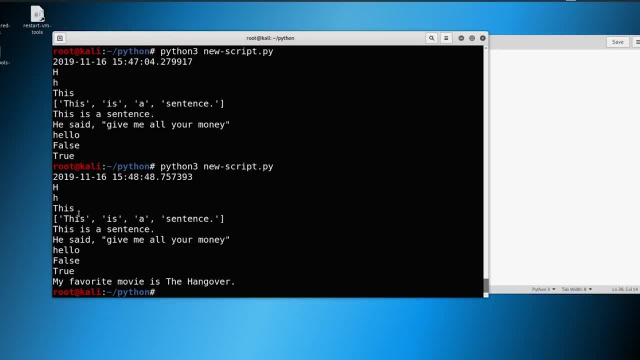 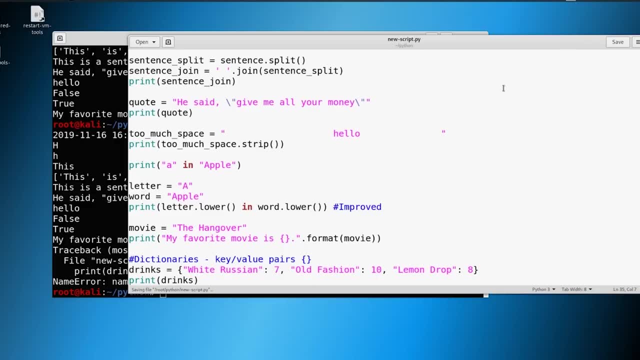 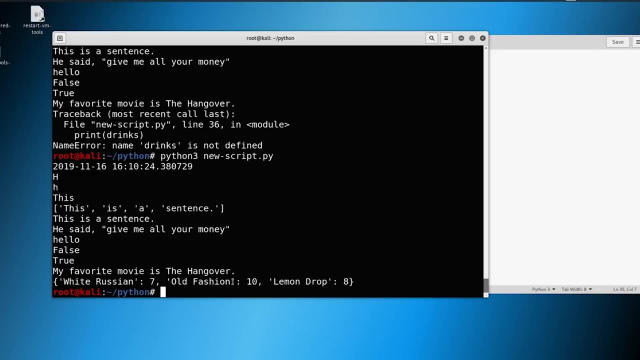 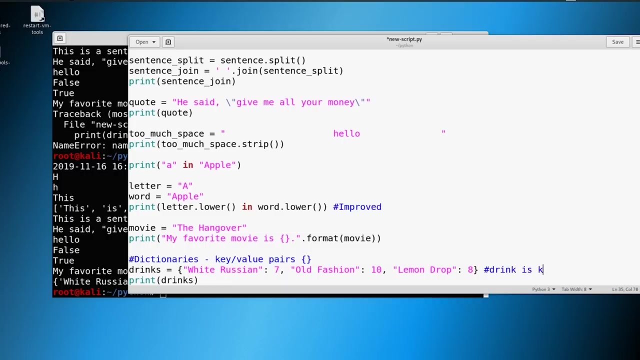 we would return our dictionary. So let's do that. If I would make this the correct syntax, this would work very well for me. I am human after all. So you see here: white Russian seven, old fashioned 10, lemon drop eight. So what you can note here is that the drink is your key and your 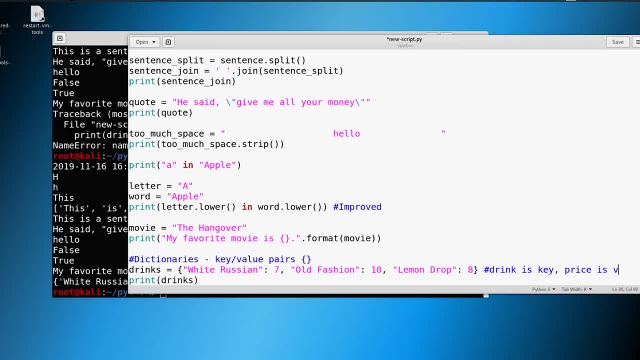 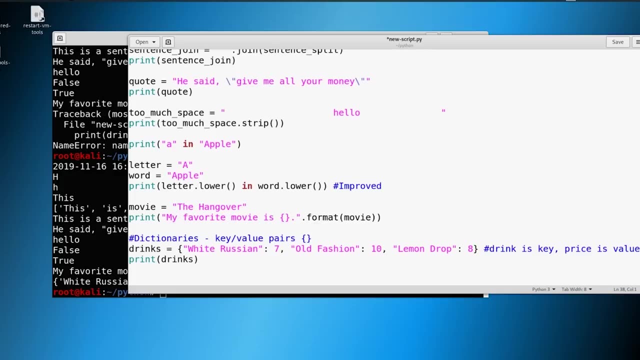 price is your, is your value. So you have your key value pair here. So key value, key value, key value. Let's think of it as another way. we don't have to just have one parameter or one value, we have to have a key. 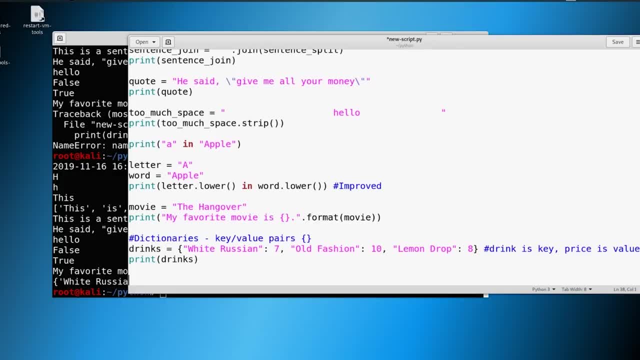 we can have multiple values to a key. So let's talk about employees, And I'm going to use one of my favorite TV show, which is Bob's Burgers, to do this. So let's say we have employees and we have different departments. So let's say we have a finance. 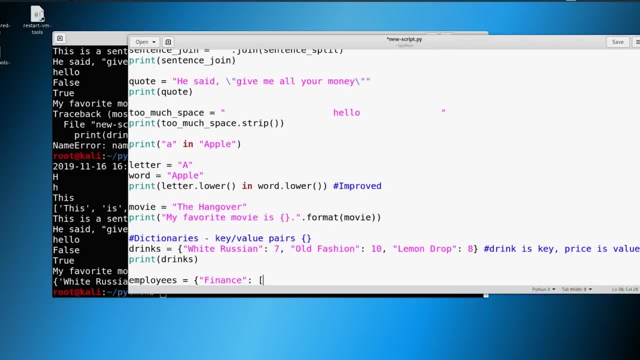 department, Okay, and inside the finance department we've got Bob, we've got Linda and we've got Tina, So we got three employees in the finance department. then we've got an IT department, And inside of it there might be Jean and Louise. We'll add Teddy to this too. 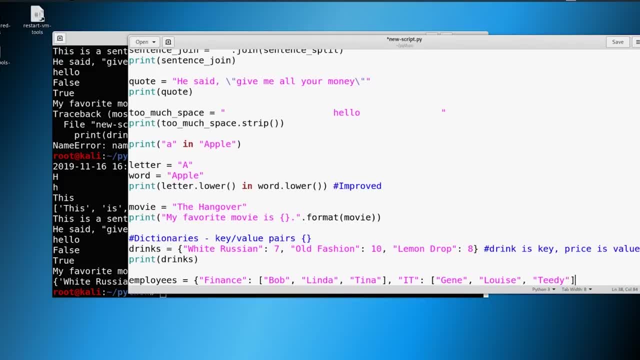 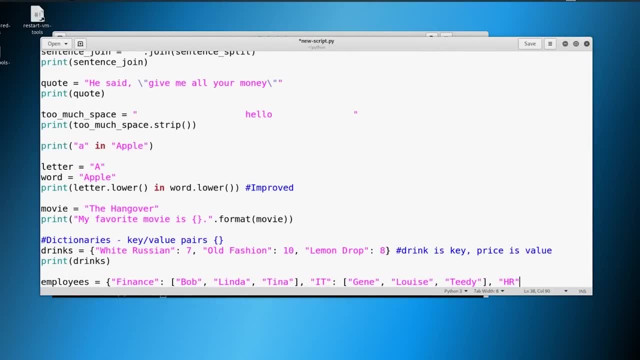 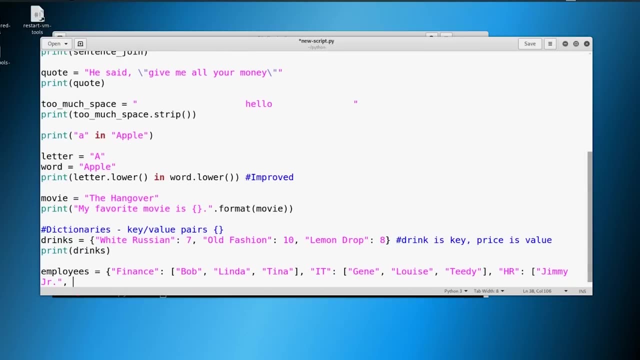 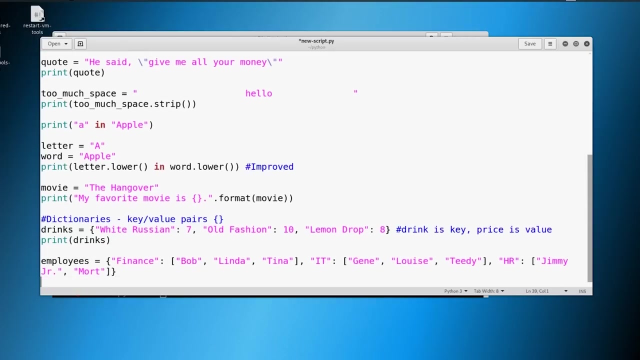 why not? I'm gonna have to move this over, it's a little bit long. and then let's do one more department. let's say that there's a department of hr, our favorite department, and we'll say: there's jimmy jr and mort. all right, so this is our dictionary. now again, we can print out employees. 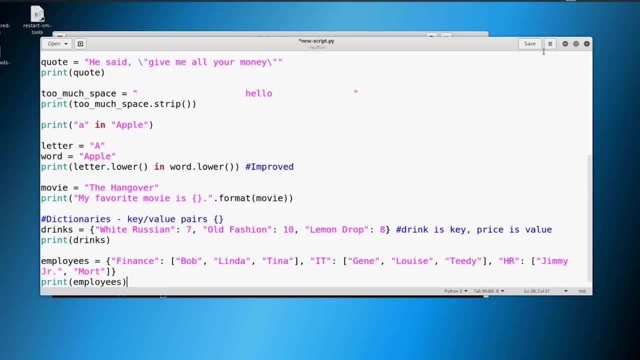 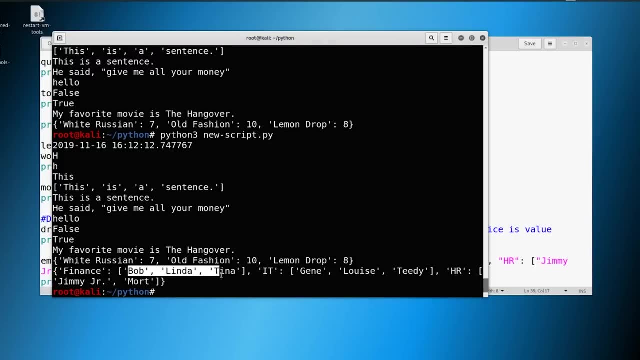 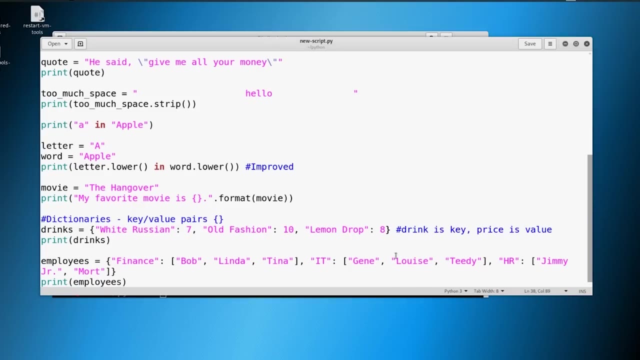 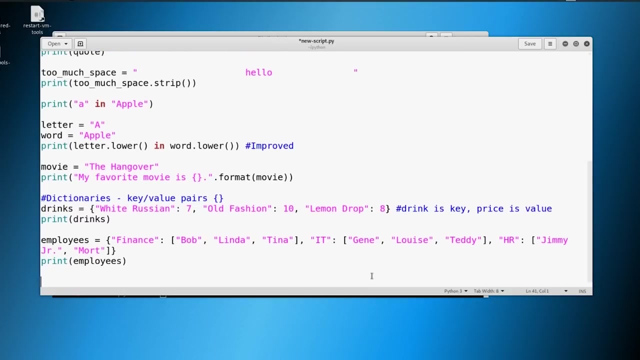 and we should be able to see our dictionary here. save this, give it a print. okay, you can see. finance has bob, linda, tina, it has gene, louise and td and jimmy jr and mort are in hr. i'm gonna fix this typo and all right, so let's say that we want to add a new key value pair. 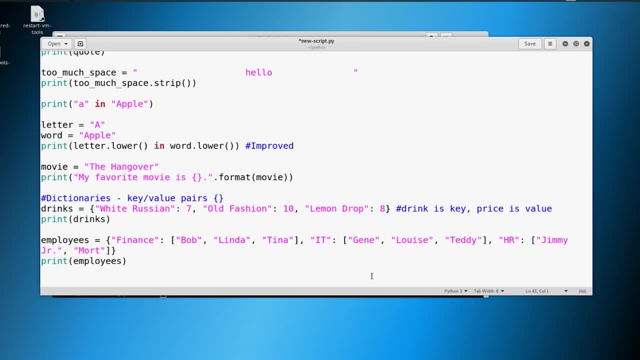 well, we can say: let's say there's a new department, and we could say there's a new department called legal, so employees, and let's add in legal, and then we'll say: in legal there is mr frond, all right, and this will add a new key value pair, something like this: all right, so we'll save this, go ahead and just print it. 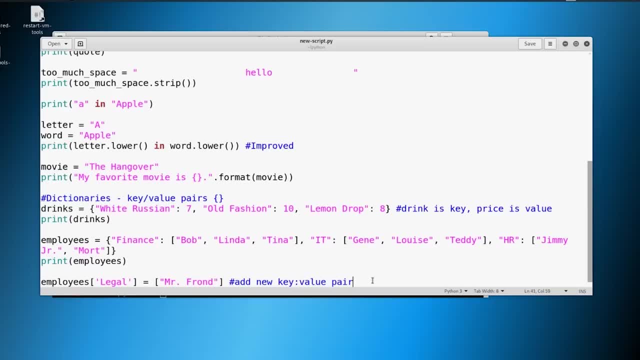 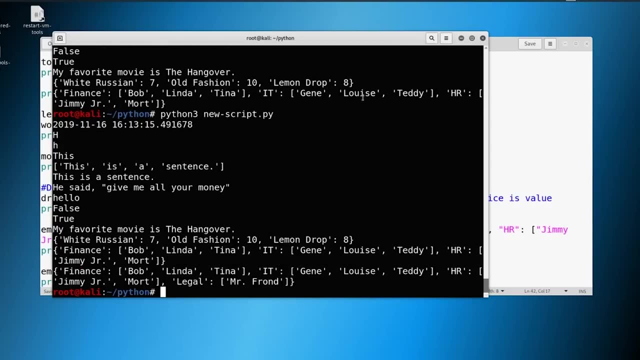 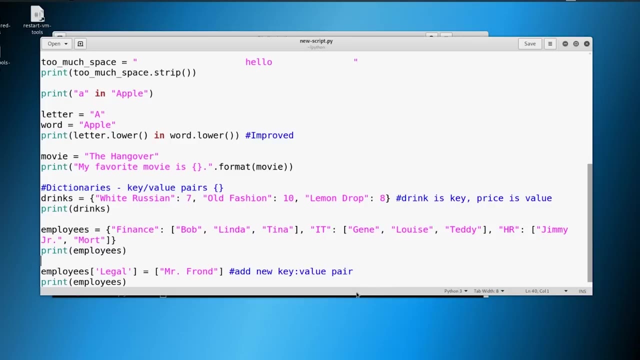 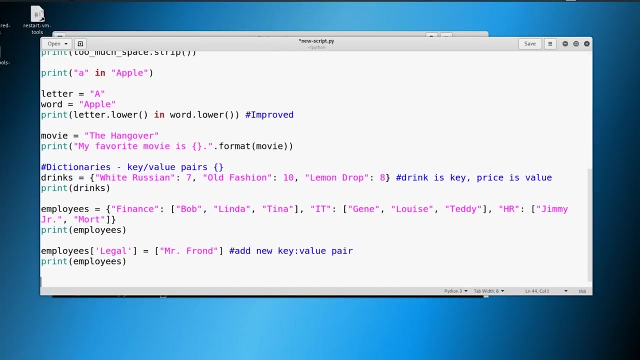 and if i were to write print afterwards, print employees and we'll save it. let's print it one more time. now. you see that legal has been added, with mr frond working in legal. okay, let's do another. let's say that we've added somebody to the sales team, and let's do it this way. we didn't have a sales team before. 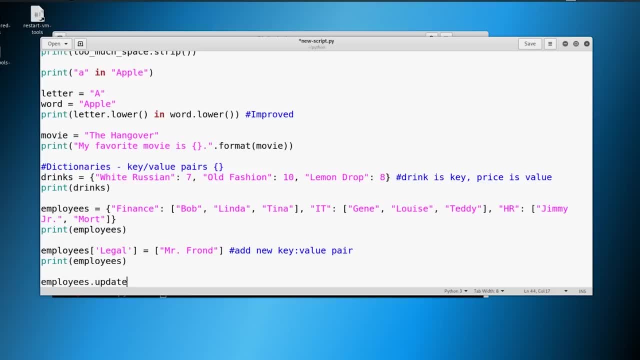 before, but we do now, so we can also do an update. something like this: we can say update and then we can add in sales and we can say: hey, we've got a nice new sales team of andy and ollie, and it'll look something like this: so now, when we print out employees, 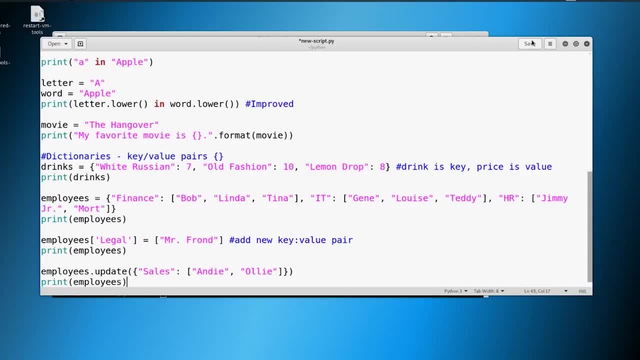 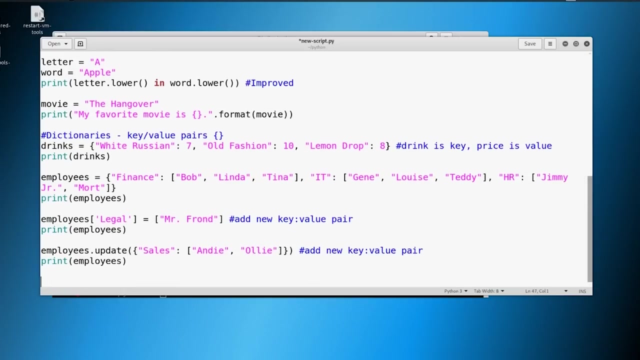 we should have andy and ollie on the sales team as well. so there's multiple ways to add in new key value pairs. so we can copy this and paste it over here as a key value as well, so we can also update things. this is last thing i'm going to show you. we can also update things. so we could say: let's. 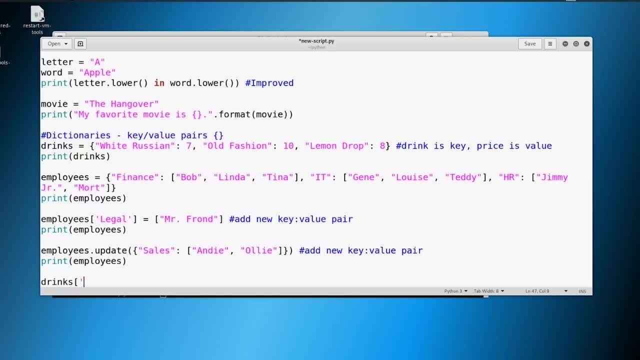 go back to our drinks and let's say that we've got the white russian. let's say the white russian is no longer seven dollars, our menu has changed and it's now eight dollars, so we're gonna make eight dollars. then we'll just print out drinks and we can save that. 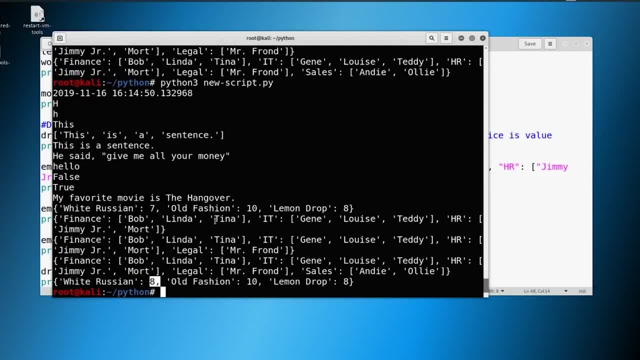 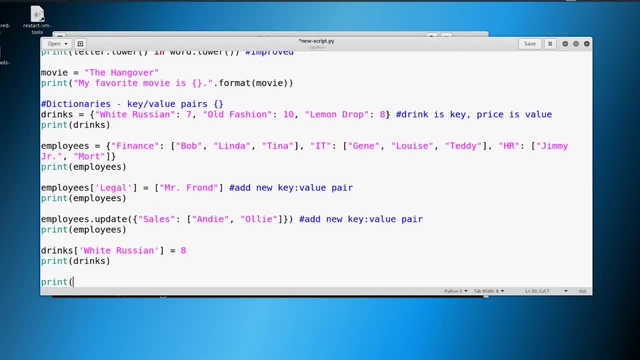 print it, and now you can see, the white russian is now eight dollars instead of seven from before. we can also get some items out of a dictionary. so we say: print drinks dot get, and we'll just get the white russian and let's see what that returns. 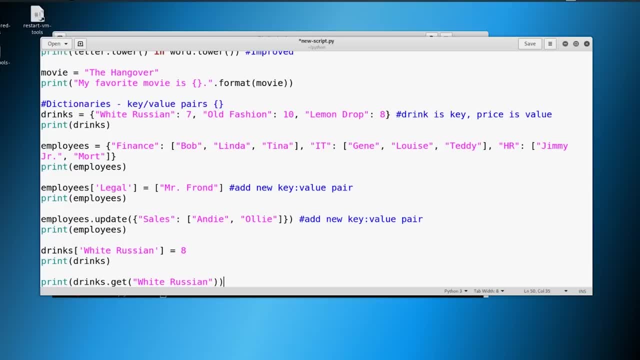 or print drinks dot get. so you can pull specifically from a dictionary here and you see that the white russian has a value of eight. so this is it for dictionaries. you're not going to really see it come up in this course, but again, this is another valuable. 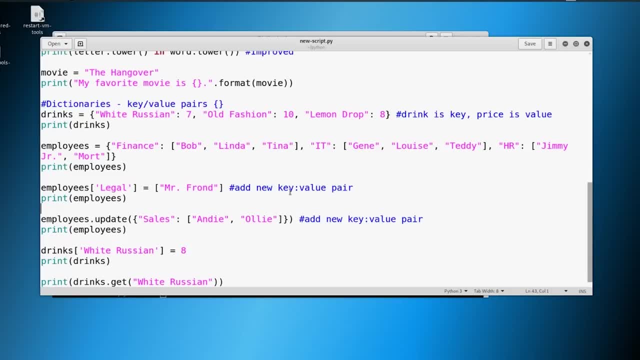 thing with python to know. so we have covered lists which have brackets like this, we've covered tuples which have parentheses, and then now we have covered dictionaries which have the curly braces, and now when you're reading code, you should be able to identify all of them differently. this 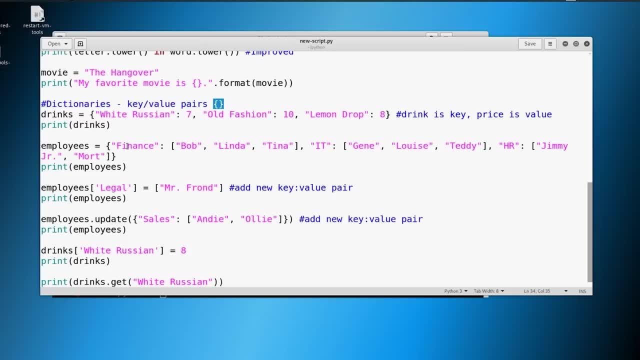 is why this was important. everything has been building upon up until this point, right, so now you should identify. okay, i see those curly braces- you know that's going to be a dictionary. or i see these, these brackets here. that's going to be a list. so keep that in mind and moving forward you. 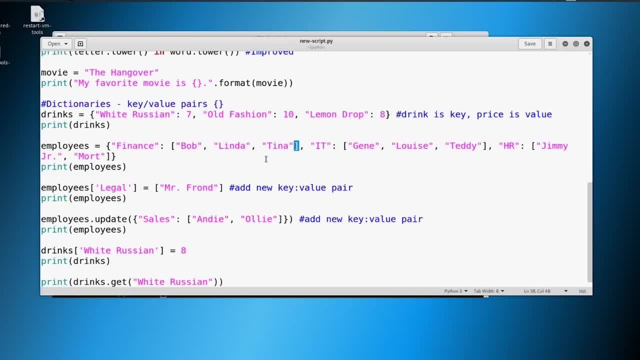 should be able to now start reading this code and understanding this code. and from the beginning i told you we don't have to be developers, but we do have to be able to read code. so the more i show you, the better off that you're going to be. so we're going to wrap up this lesson. we've got a. 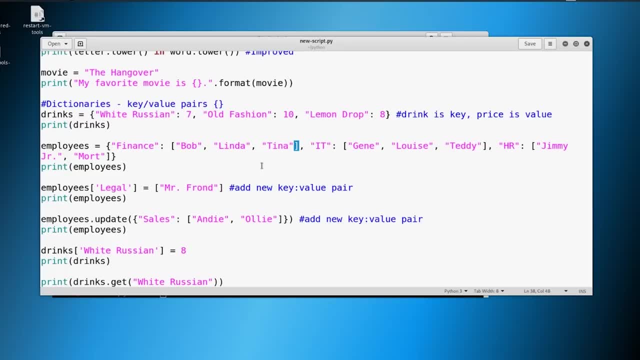 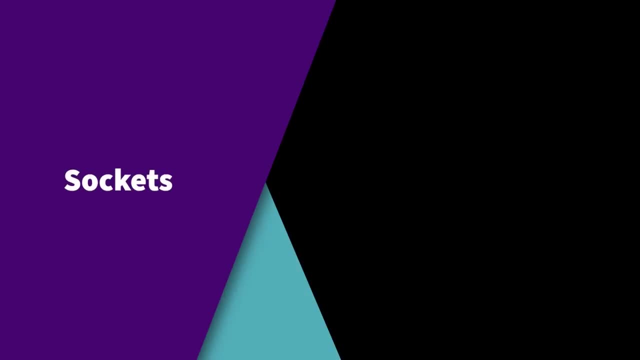 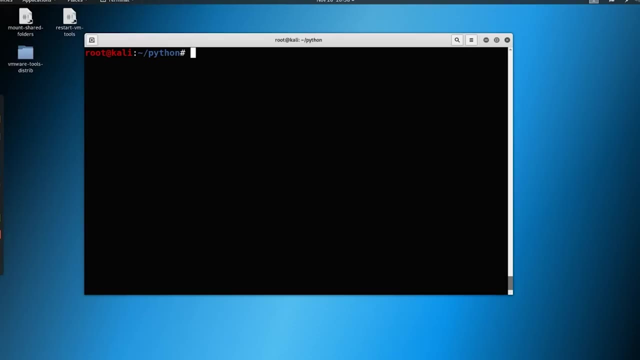 couple more before we start building our scripts and we'll be be good to go and move into hacking, so i will catch you over in the next lesson. welcome to your final module before we start working on scripts. so this last module is a very important one because we have to define what 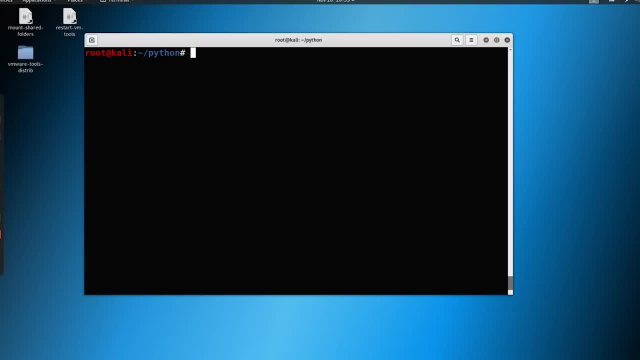 sockets are. so we're going to be using sockets to connect two nodes together. really, that's it and more layman's terms we're doing is we're going to use sockets to connect to an open port and ip address. so you're going to see this when we build a port scanner, you're also going to see 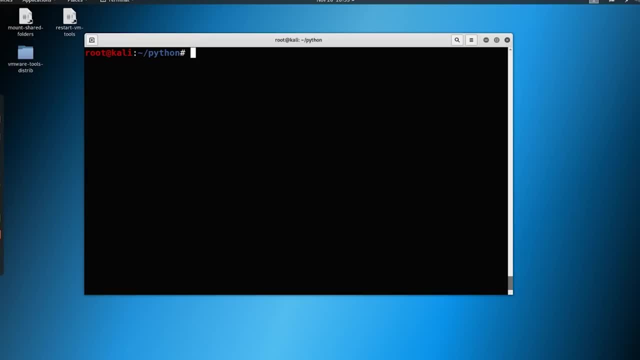 this later on in the exploit development portion of the course, where we have to reach out to a specific port and ip address, establish a connection and send malicious data. so what we're going to do here is we're going to just build out a simple socket script and 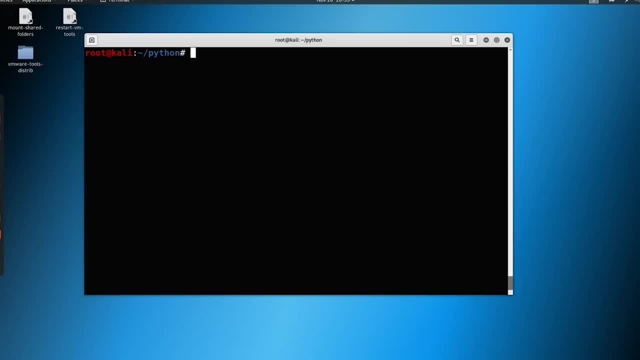 we're going to connect to an open port with that script and it'll start to make sense. and then, when you see it in the next video, when we build out the port scanner, make a little bit more sense and you see it again in the course, you're going to say: hey, i remember that we use sockets for. 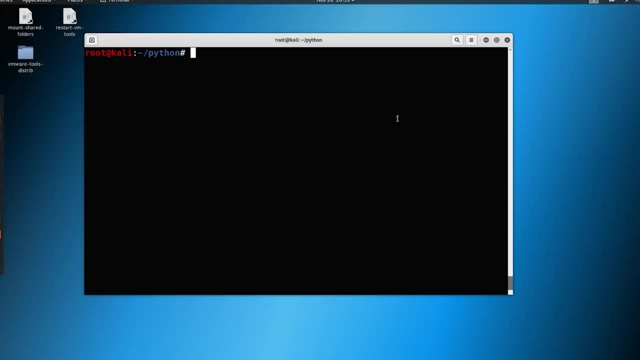 connecting two ports. so here's what we're going to do. we're going to make a file and call the file spi. you can call it whatever you want, just do not call it socketpi. if you call it socketpi, you're going to run into issues because it's going to think it. 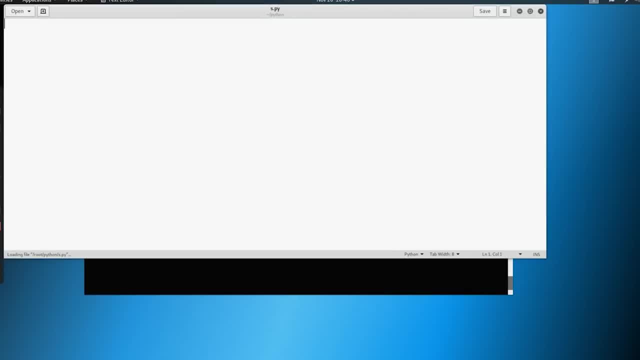 is a socket. so we need to define a couple of things first. so what we're going to do is we're going to, of course, shebang up top, do our bin python 3 and we're going to import socket. so we're going to import socketpi. so we're going to import socketpi. so we're going to import socketpi. 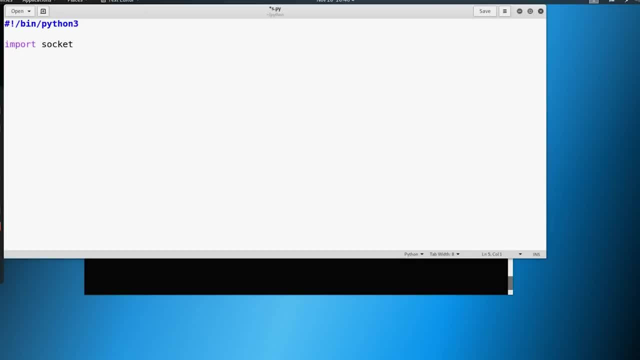 up here at the top. now let's define a couple of variables. so the first variable we're going to say is host, and we're just going to give that our local address here of one, two, seven, zero, zero, one. this is our local host. and we're going to define port, and i'm just going to give mine all sevens. 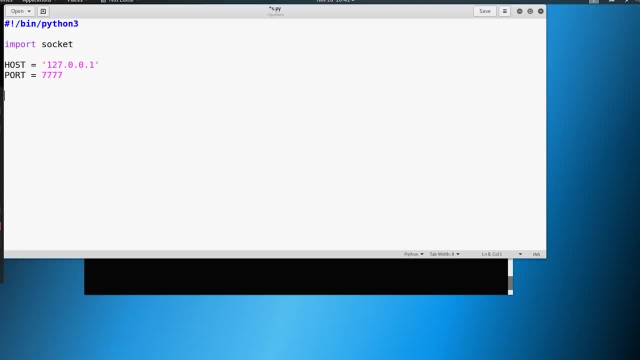 you can give it whatever you'd like here, and i'm going to define another variable, so i'm going to give it like this: s equals socket, dot, socket, socket, dot. af. init. socket, dot, sock. underscore stream. now this looks long and intimidating. please do not be intimidated by this. we are just making our life easier on ourselves, so we're. 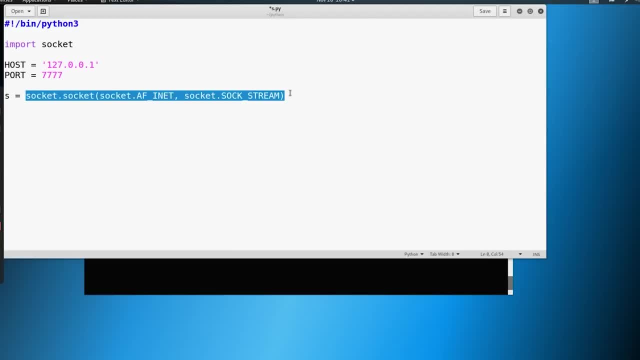 defining a variable that stores all this into one, and this is very, very common when it comes to sockets. This syntax here is very common. So what we're saying is: hey, we want S2 equal socket, dot socket and this socket, AFInet, socket, SockStream So AFInet. just think about that as 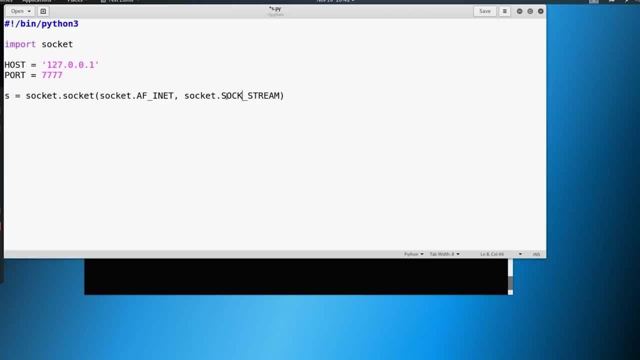 IPv4.. We're connecting over an IPv4 connection: Socket, dot, SockStream. you could just think of this as a port. So AFInet, IPv4, SockStream, it's a port. So let's say we want to make a connection. 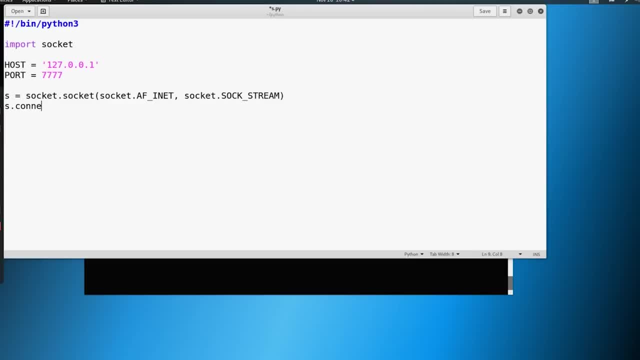 We're going to say S, dot connect. Now, connect is just another part of the socket module, So we're going to make a connection here And so, if you think about this, we're using all this and then dot connect, right, So we're declaring this and then we have these two parameters here: socket. 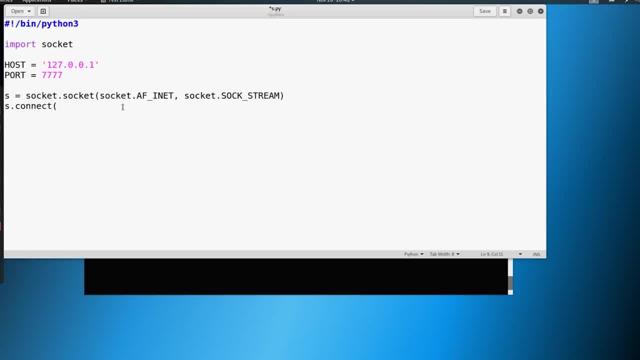 AFInet, socket, SockStream. So the AFInet. we need to say, hey, let's make this our host variable and then this one our port variable, And we could in theory just put in 7777 and 127001.. But it's just easier to find those in. 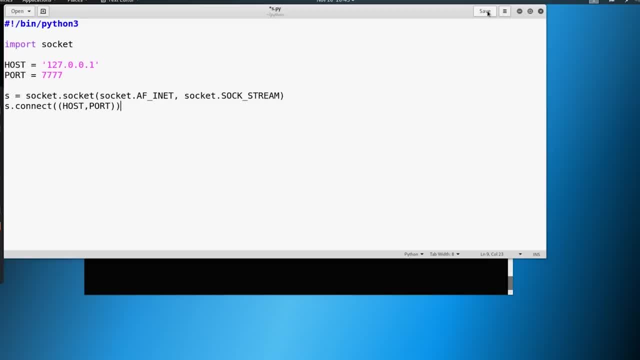 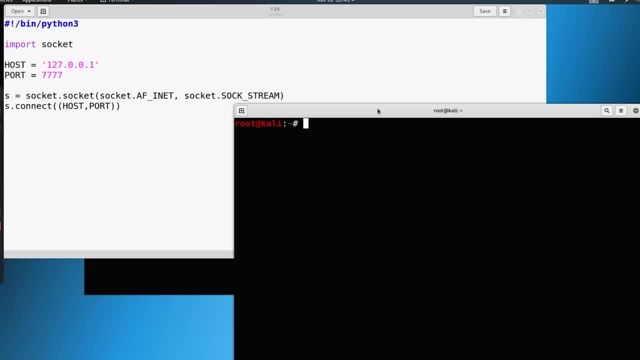 a variable up top and then use them later to connect. So I'm going to go ahead and save this And then I'm going to open up a new terminal in a new window here And I'm going to utilize a tool that we have not used before, And this tool is called Netcat, And we'll use this later on in. 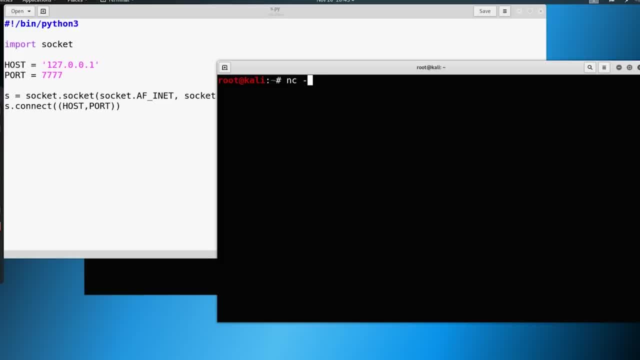 the course quite a bit. So we'll say Netcat And I'm just going to say NDLP. This means I'm going to establish a network And I'm going to say, hey, let's make this our host variable. And then 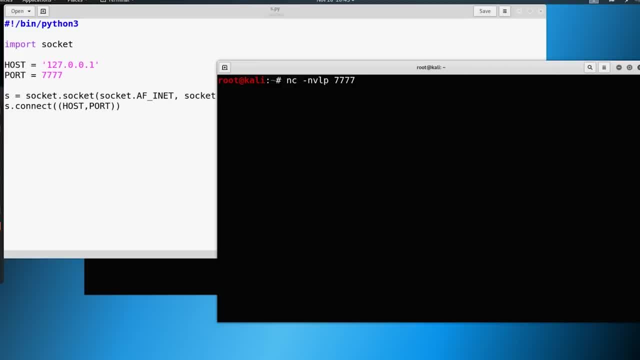 I'm going to establish a listening port. I'm going to listen on port 7777 for connection. So you see, here it says: hey, we're listening on any interface for all sevens. You don't have to worry too much about this right now. We're going to go into detail on Netcat at a later time, But 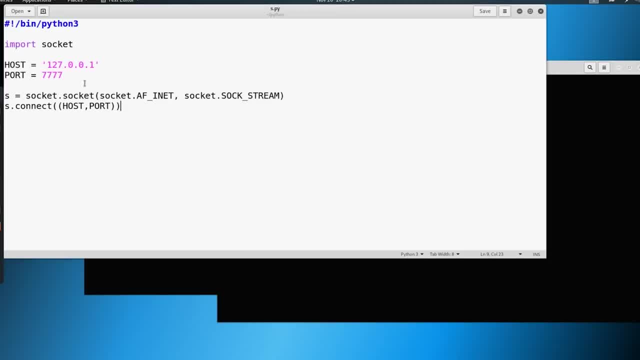 all we're doing right now is we're waiting for anybody to connect to us. Now, here we're sitting at our local host of 127001.. So we need to establish that connection, which is what we're going to do with this script. Now, the script does nothing. We're going to say, hey, let's make this. 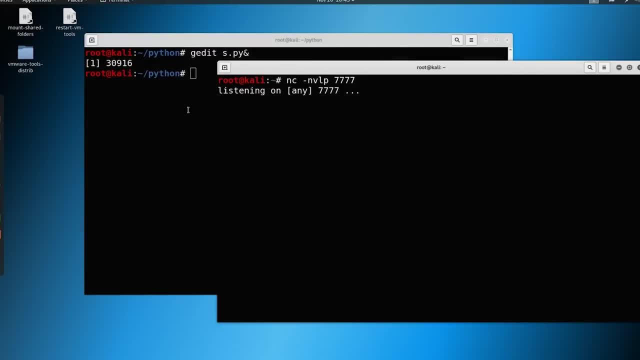 a connection, It establishes a connection And that is it. So let's go ahead and take a quick look. We're just going to say Python 3, spy. Do that, Come over here And you see that we had an. 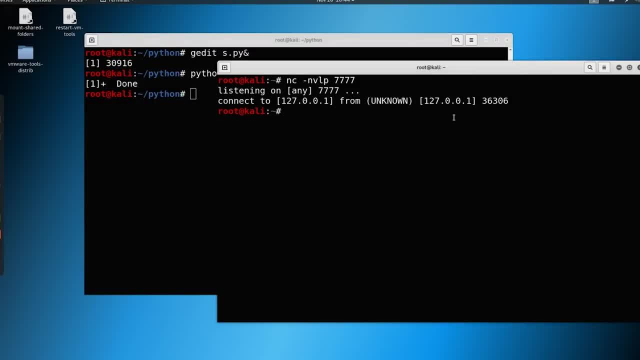 established, connection made And then the connection closed. We didn't tell it to do anything. There's nothing here to say, hey, keep this connection open, send over some data, do anything at all. We just said, hey, make a connection really quick, And it did. It made. 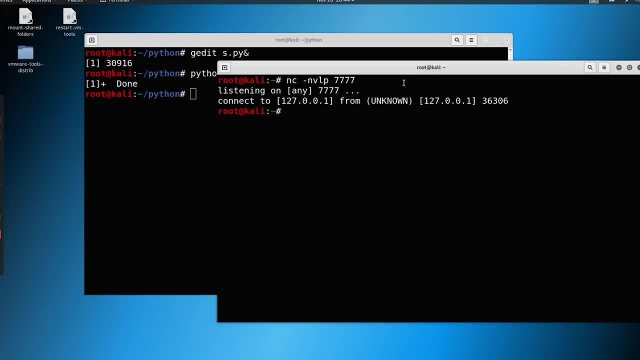 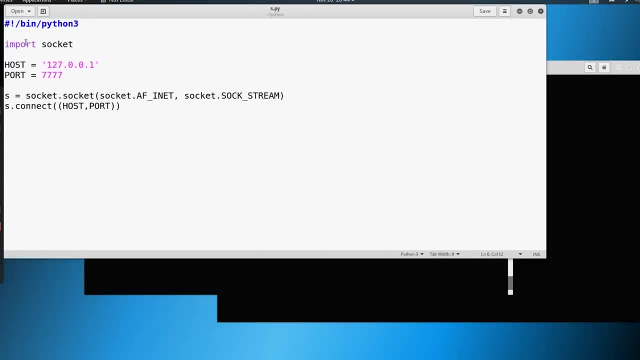 a connection from 127001 to 127001.. We connected To ourselves, But with this script we have successfully achieved what we wanted to, which was to utilize sockets to connect one node to another node. That's it, So we're going to build. 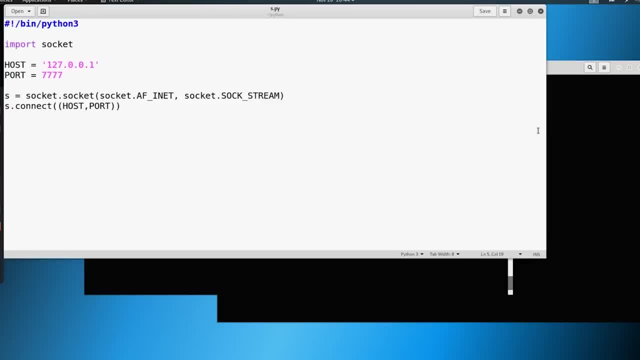 upon this whole thing here. In the next lesson we're going to build a port scanner. It's going to be a bad port scanner, but it's still going to be a great lesson. So let's go ahead and just take a look at that port scanner and I'll catch you in the next video. 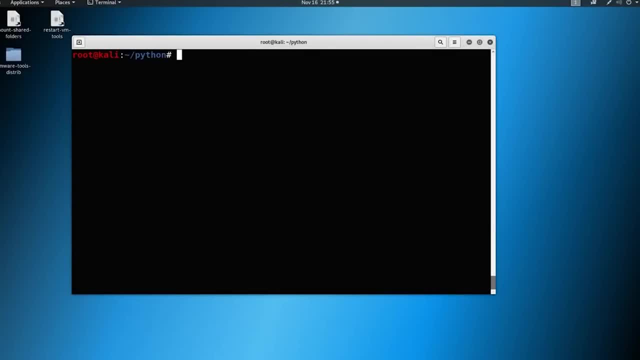 All right, welcome to the last video in our Python module. So now we're going to be making a port scanner, And you heard me say in the last video that it's going to be a terrible port scanner, And it is. but it's going to be a functional port scanner as well, And we'll talk. 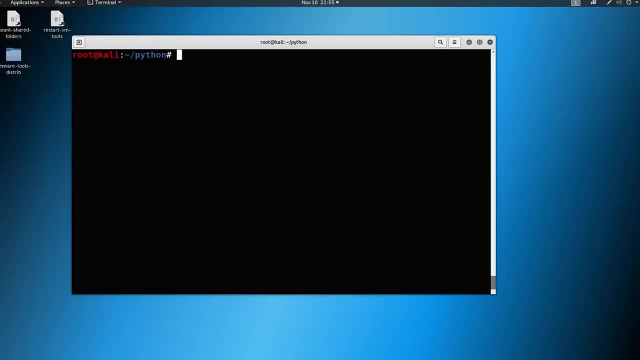 about what we can do to improve it and how we can think this through. So what we're going to do is we're going to go ahead and open up a g edit here. So I'm going to say g edit And we'll just go. 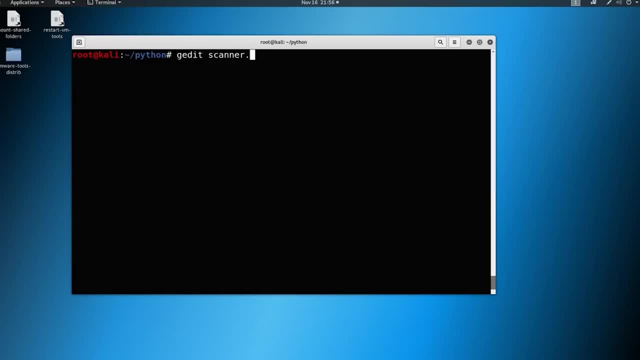 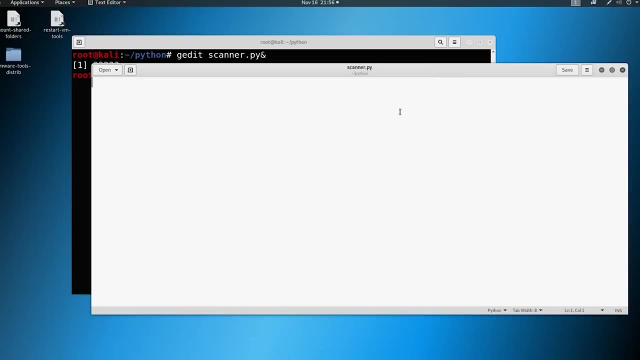 ahead and call this scanner. And we're going to go ahead and call this scanner And we're going to enter dot pi And we'll do the ampersand at the end And let's go ahead and declare that this is going to be Python three. And now let's talk through some things. So there's going to be a. 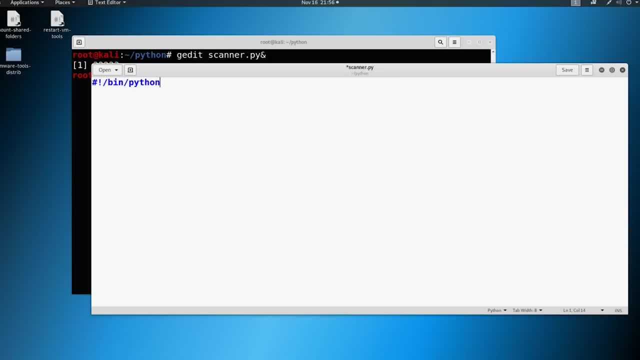 lot of familiarity. everything I've done up until this point has been for a reason, And you're going to start to see it all tied together. So the end goal of this project is going to be that we run something along the lines of Python three scanner, dot, pi, And we provide an IP address here. 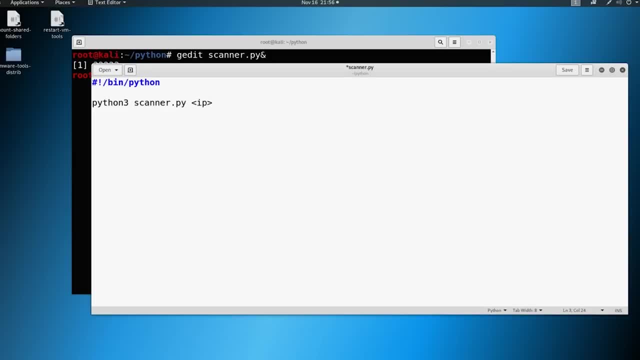 Now, with that IP address, it's going to go ahead and scan through a selected port range for us and try to return back results whether or not the port is open. So we're just checking if a port is open on a machine. So to do that we're going to need a few things. So first of all, 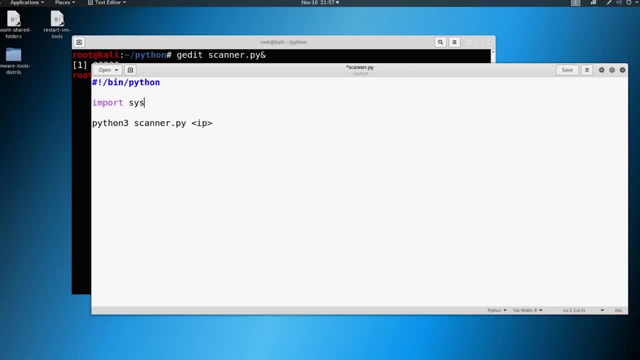 we're going to import sys. we're going to import socket, as we are going to make a node to node connection, And we're going to import date time from date time, as we're going to make a pretty little banner as well. So why was this important? I told you this would come back into play, So we 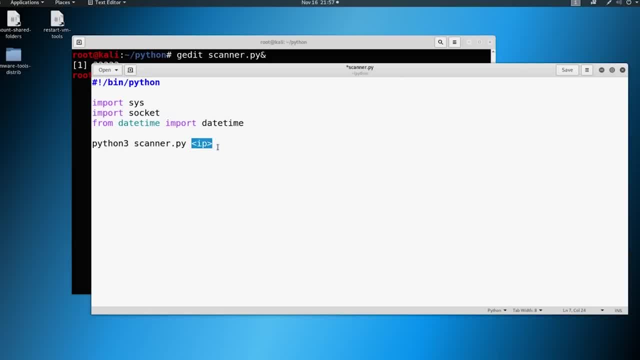 have here an argument, So they're actually going to be a little bit more complicated And we're going to actually two arguments in theory. argument zero is that we're running scanner dot pi. Argument one is that we are running against an IP address Now, since we're building this script out. 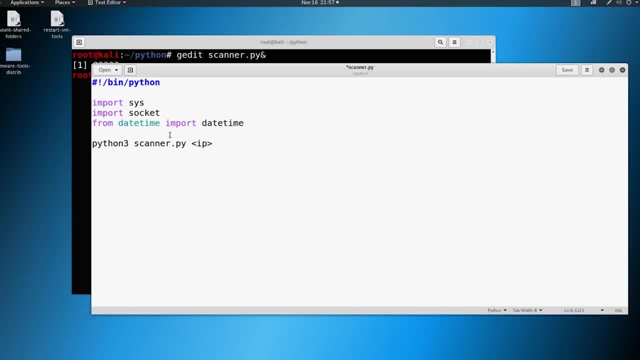 we want it to take two arguments and only two arguments. So we're going to build that into our script from the get go. So let's go ahead and just define our target. And it's always good, when you're building out a script, to have good results. So let's go ahead and just define our target. 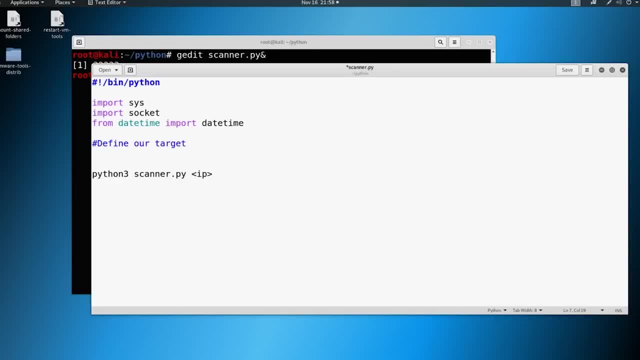 So let's go ahead and just define our target, And it's always good when you're building out a script to notes in there as well, So not only that you can go back and read it, but if you send this to somebody else, they could also read through it as well. So put good comments in here, good notes saying what. 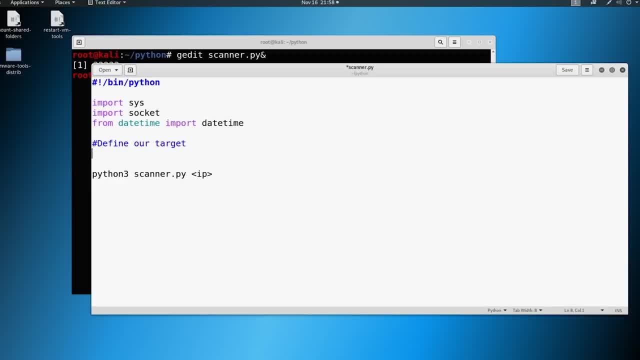 you're doing So in this instance we're going to put an if statement- again conditional argument here. we're going to say, if the length of sys dot arg v- remember, this is the same thing as, like a dollar sign, one in bash, we're going to take that. we're going to say, if it's equal to two, we're. 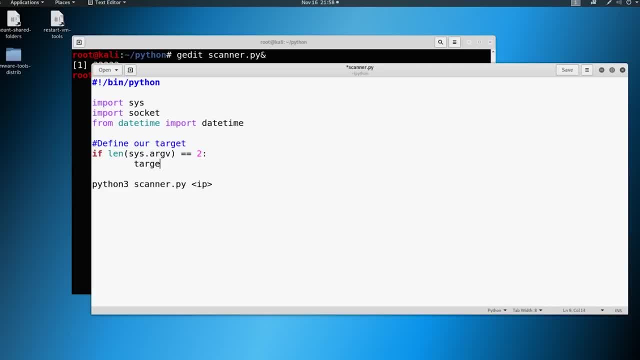 going to say: if the length of sys dot arg v- remember this is equal to two. we're going to say: if the length of sys dot arg v, we're going to declare a variable of target and we're going to say socket. 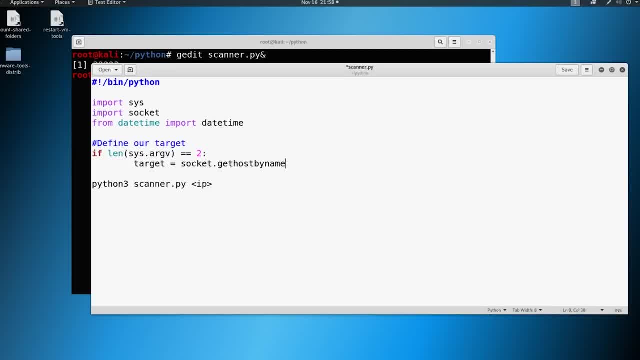 get host by name, And then we're going to get sys arg v one. so we're taking the first argument Again. this is same thing as dollar sign one like this in Bash. Why are we doing this? Well, we're just translating a host name here to ipv4.. Now this: 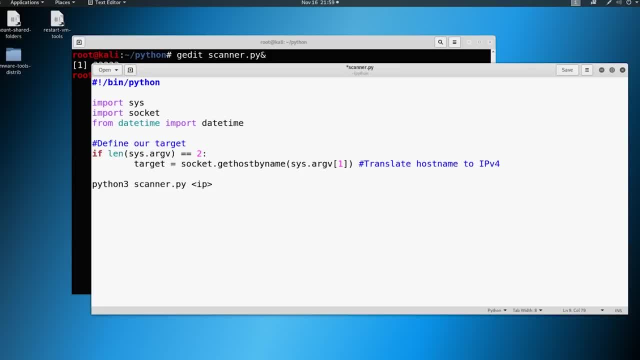 This is not inherently necessary. We could just declare the target by input. it could just be: target equals sysarg v1.. But we're just taking an extra step here In case, instead of somebody putting in an IP address, they could just put in like a host name, say we. 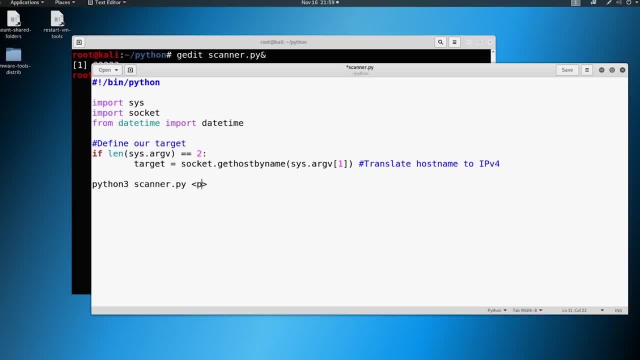 have a host here And it's, you know, like a one of mine is called the Punisher. You know what, if it we they put in Punisher? Well, that Punisher name does DNS and it resolves to an IP address. it's going to go ahead and do that with this argument here. So we're 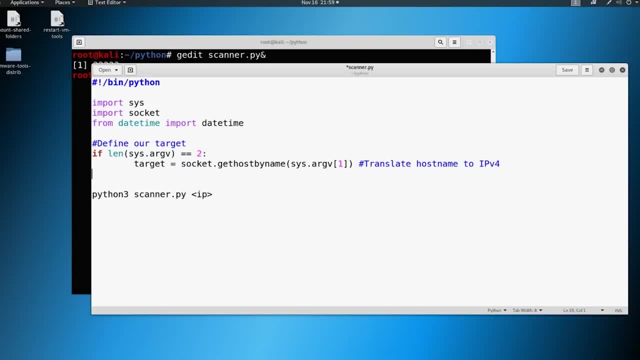 just putting in an extra step, thinking ahead, We also need an else to this. So if it doesn't equal to, if it's three, if it's one, it's none, then we're going to go ahead and just print out and say invalid amount of arguments And then we can actually take this here And 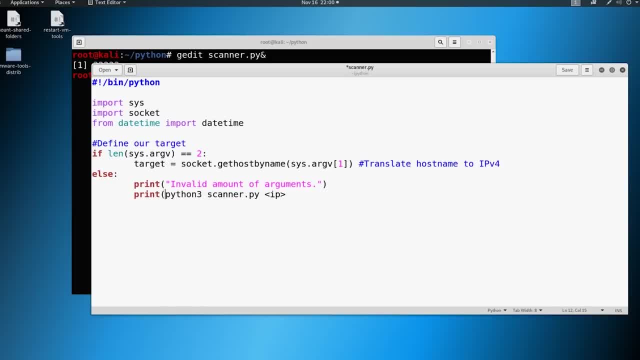 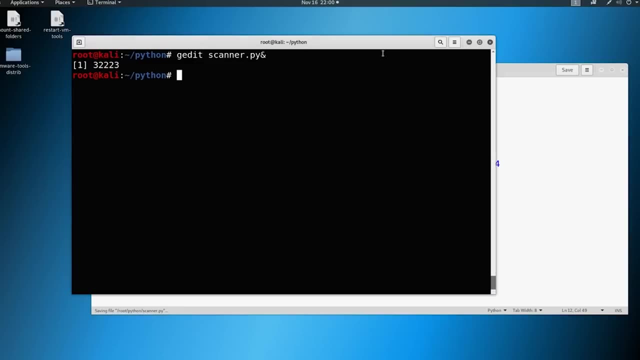 we can put this into a print statement as well. Just print, Just say something like syntax: Python three scanner, IP address, something along those lines. Okay, so I always like to save it and then just run it and make sure everything works fine. So let's go ahead. 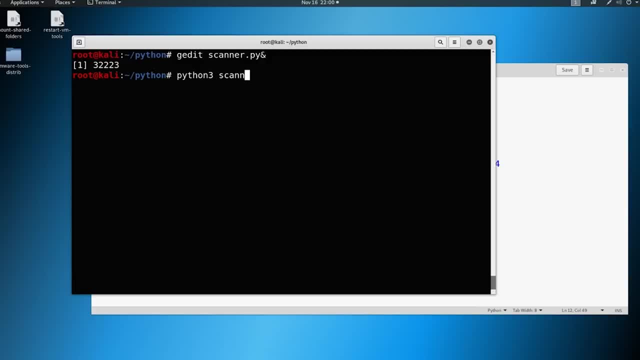 and give it Python three, we'll say scanner, dot, pi, And we'll give it no argument And it's going to say, okay, invalid amount arguments. Say no argument, And then you're going to say it's valid. And then you're going to say, okay, invalid. And then you're going to say 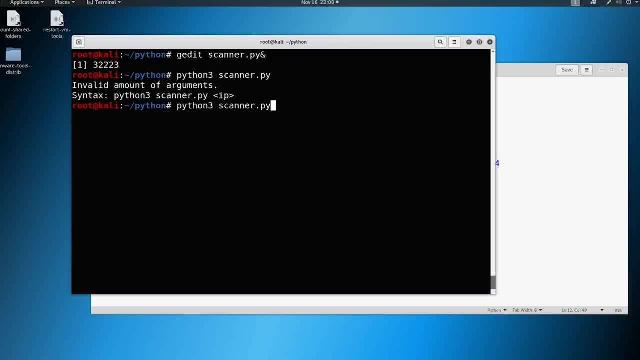 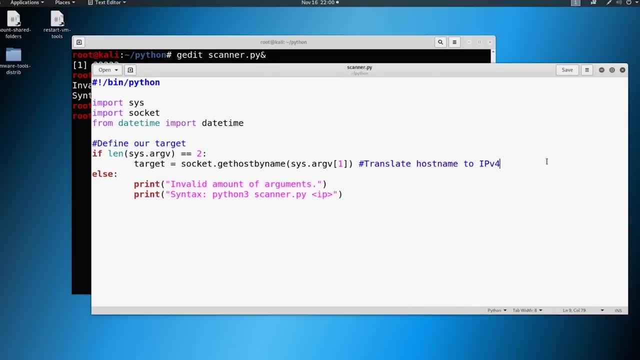 no argument. And then you're going to say, okay, invalid. And then you're going to say no argument. syntax is Python three scannerpy IP, So we'll just give it an argument here. Okay, so it runs. didn't get the. we met the conditions And we set the target variable to well to this right. So 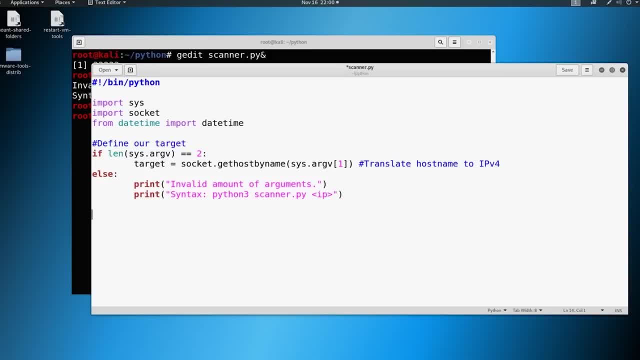 that's okay for now. So let's go ahead, And I like to always put in a pretty little banner or something you know. so let's add a pretty banner And I'm just gonna do something like this: I'm going to say print And we're going to do dashes, we'll do 50 dashes And then we'll go. 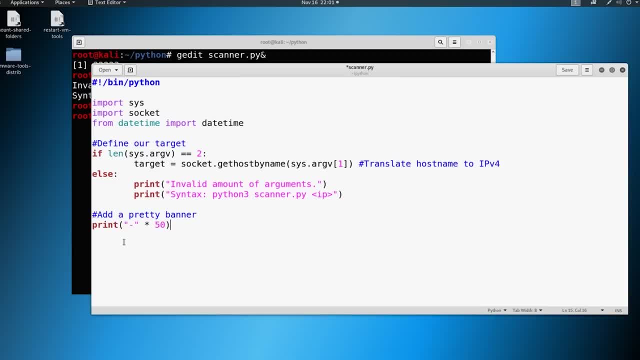 ahead. I'm going to copy this just to be easier, And let's go ahead and print a couple things. we'll say print, we'll say scanning target, And then we'll add a space and we'll just do plus target And then we'll say print time started, And then we can just do a space there. 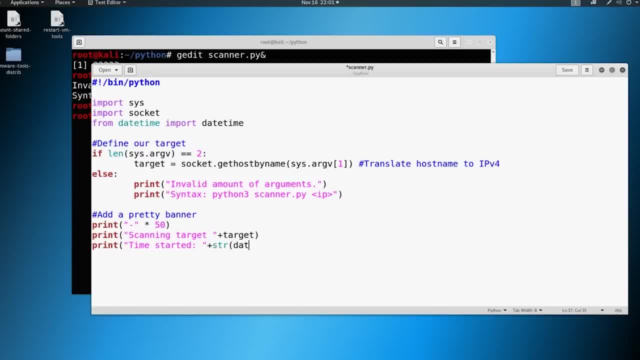 plus the string of date time dot. now, now that came back into play as well, So make sure you have three closing parentheses. So we've now utilized sys, socket and date time, all of which we have seen in the past, And then that last copy paste here for the banner. So let's go ahead and save. 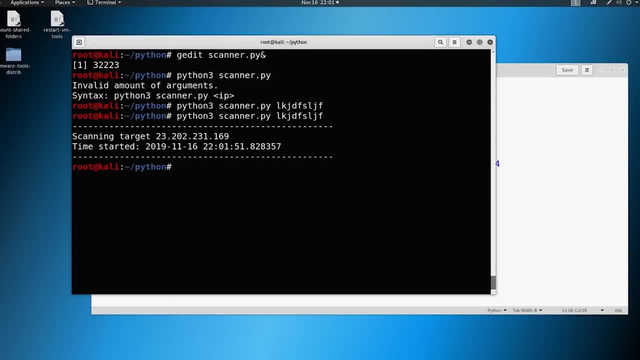 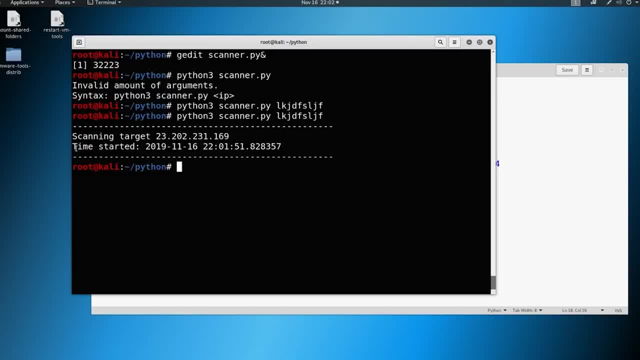 this is not accurate, but you know, just let it do its thing And then it's got the time started of the scan here. So you can see, here I'm putting in a host name and it's trying to resolve to DNS to. 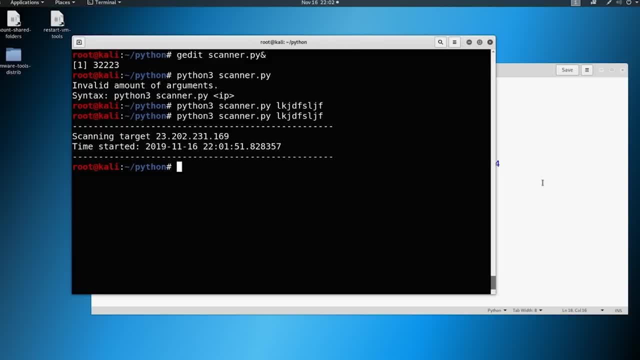 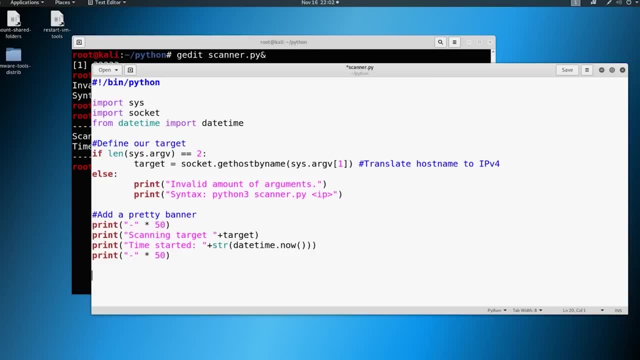 this. Maybe this is how what it resolves to. I don't know, But we'll move on. So the next thing we're going to do is what is called a try statement. So we're going to try to do something, And if we can't do it, we have exceptions. So you'll see what this looks like when it's all. 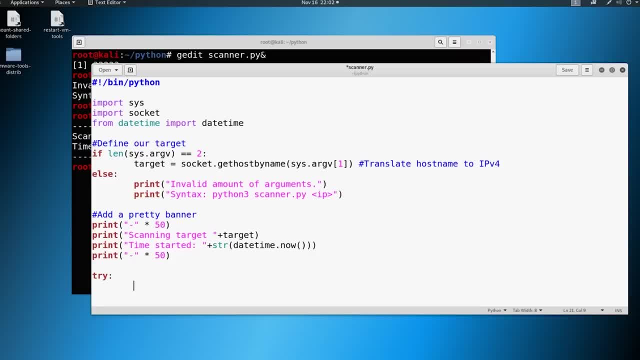 built out. So go ahead and type, try And you're going to see try later as well when we get into the exploit development. So we're going to do a for statement. So for port in range, Now we need to specify the range. If we were going to do a full on port scanner, we would do for port one. 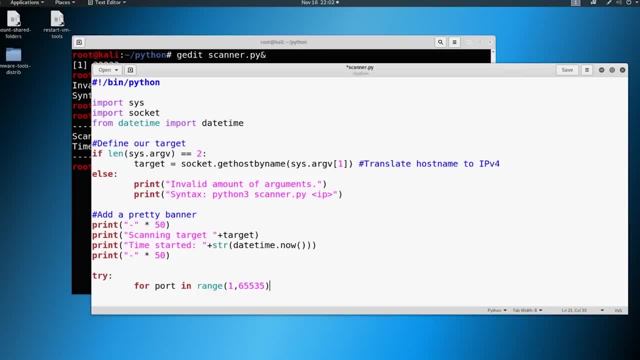 through 65 535.. Okay, that will take forever. We'll talk about why I told you this was a bad port scanner. We'll talk about why we're going to do this And then we're going to do a full on port scanner. We're not going to do this in a little bit, So let's go ahead and delete these. 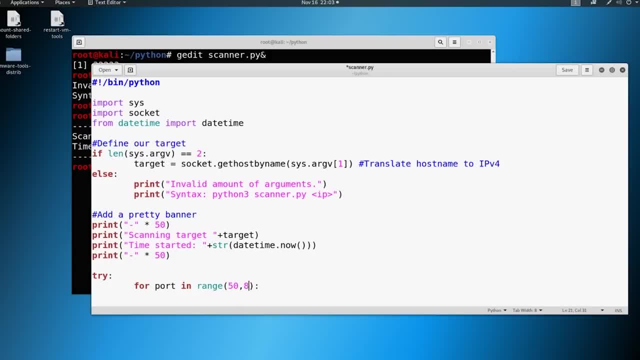 And we're just going to put something like 50 to 85.. And I'll clarify why we're doing that in just a second. So on top of this, let's add: in some familiar language we're going to say: s equals socket, dot, socket, and then socket, dot, af, underscore, inet comma. socket, dot, sock stream. 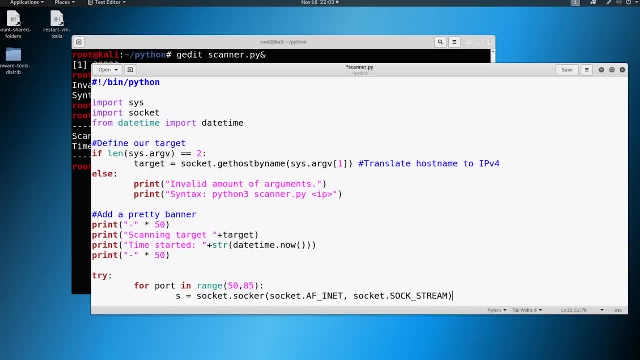 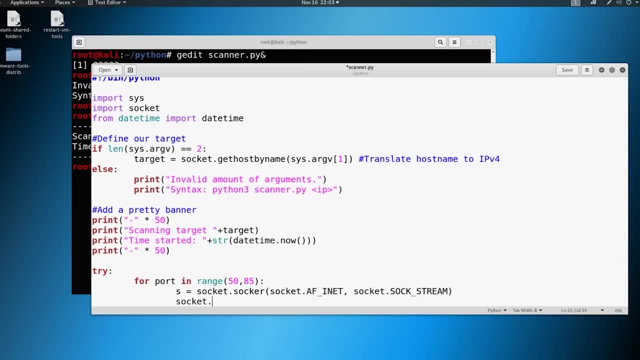 Remember, af inet is the same as socket dot socket. So we're going to say s equals socket dot socket. So we're going to say socket dot. set default timeout to one. Why are we doing this? this is going to attempt to connect to a port. If that port is not connectable, it's going to wait one. 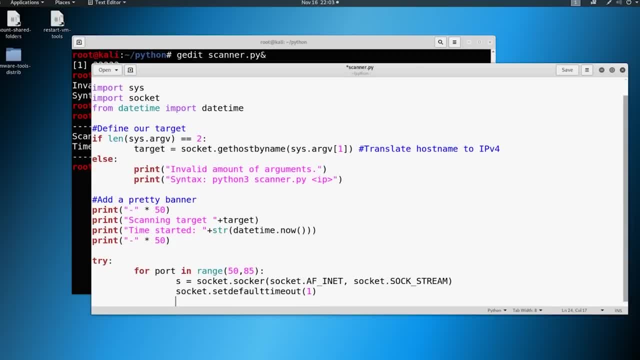 second and then it's going to move on. That way. we're not sitting there forever trying to make a connection to a port. we set the timeout ourselves, So we're also going to do a full on port scanner. We're also going to store a result, So the result is going to be s dot connect, underscore ex And. 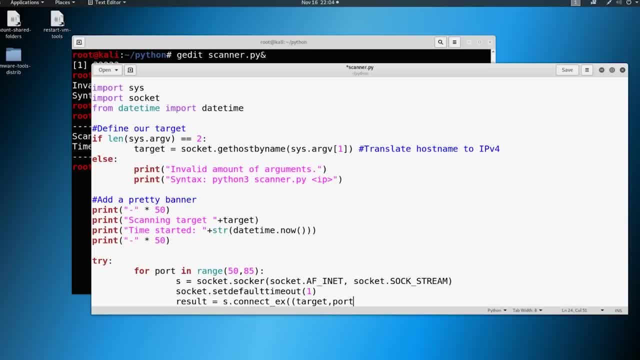 it's going to be target comma port. So why are we doing this? Well, when we do this connect, underscore ex right, it returns an error indicator. So I'm gonna put returns an error indicator. If a port is open. the result back is going to be s dot connect underscore ex And it's going to be s dot connect. 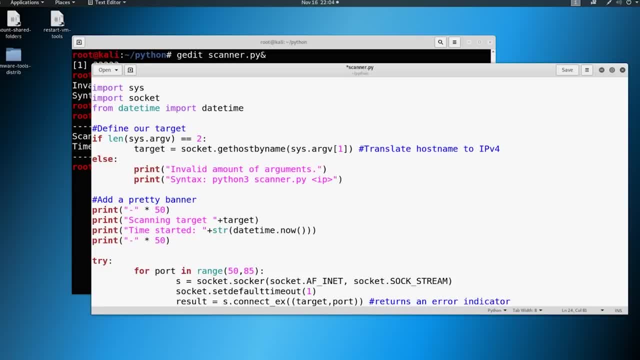 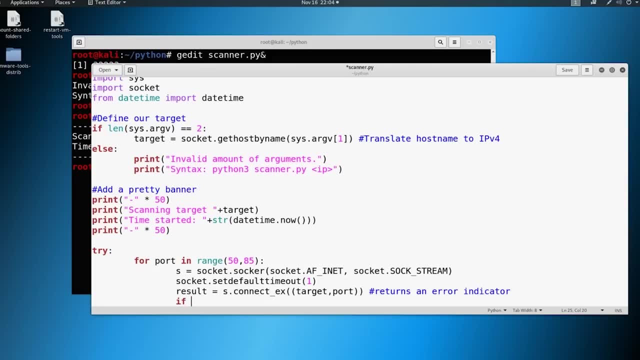 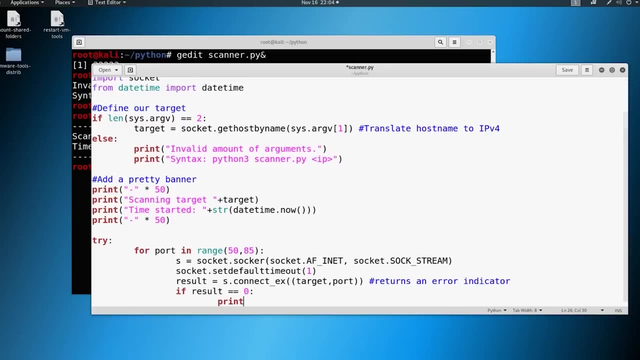 zero. If a port is not open, it's going to throw an error which is going to trigger a one. So let's think that through. If result is equal to zero, then we're going to go ahead and just print out that this port is open. We'll throw this in here this time for a placeholder Instead. 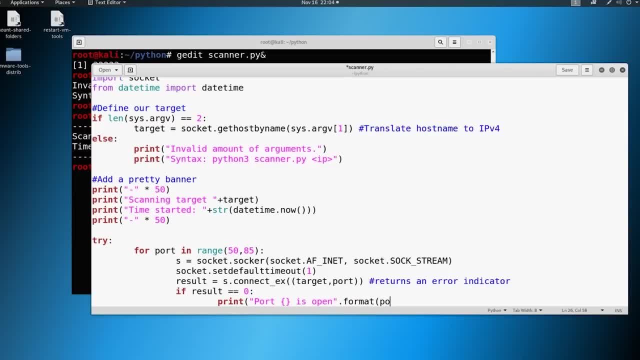 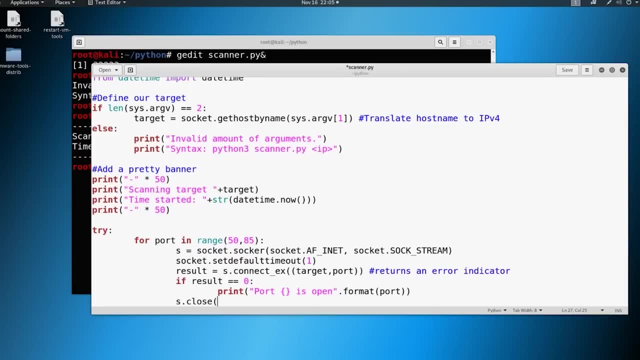 we'll say: is open, and we'll do format port. And then one more thing: I'll close it out And we'll walk through this one more time so that it all makes sense. Okay, so then we're closing the connection. Okay, so we've got this try statement, Let's walk. 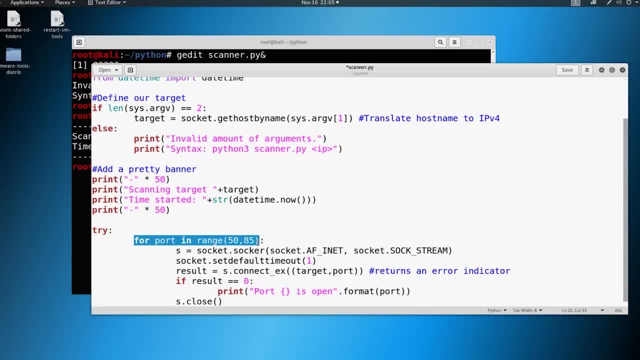 through it one more time. We've got a for loop here. Remember, for is just an iterate. we're going through an iterate, we're going through 450.. In so we're defining a port right in this range, So 5051, 52, all the way up to 85.. We're going to repeat this whole process. we're going to establish. 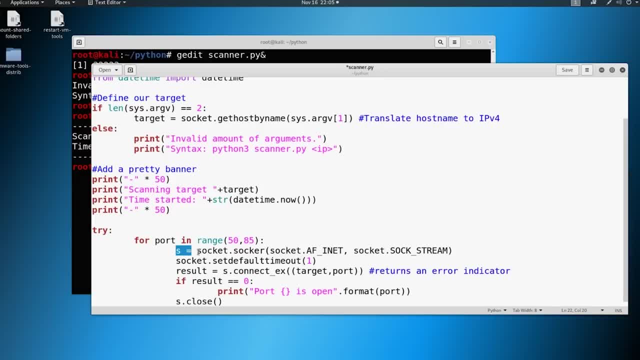 our variable of s, which we did in the socket video, the previous video. right, we're just declaring: hey, I know I'm going to want to connect to IP before and a port When I do make that connection. I want that default timeout to be one second. Okay, so then I'm going to store. 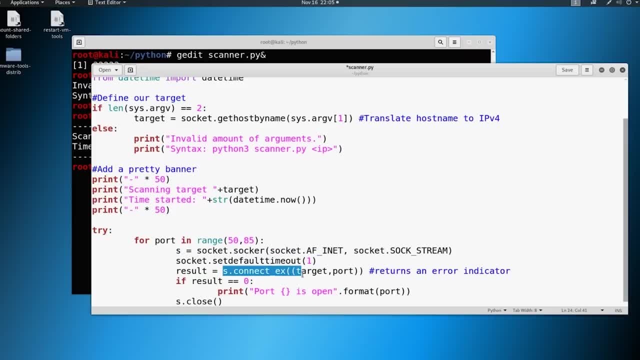 inside of a variable of result. I'm going to say let's connect to the target which we've already established as sys arg v one And the port which is our iterate here in our loop, and if that port is open it's going to return zero. if it's not open, it's going to return one. 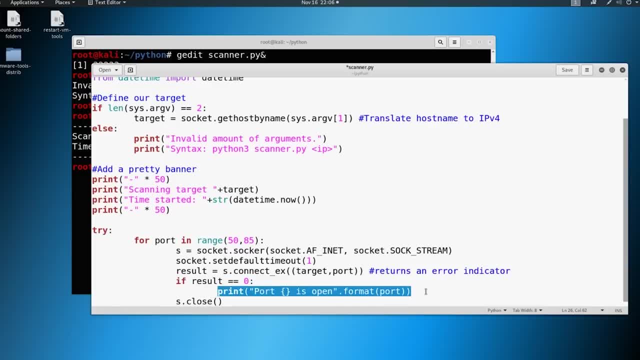 So if that result is zero, go ahead and print out that that port is open, close the connection, And then we're going to go back and try to establish another connection with port, or with port number 5152, 53,. we'll loop through all this until we make it all the way through 85.. Okay, so it's. 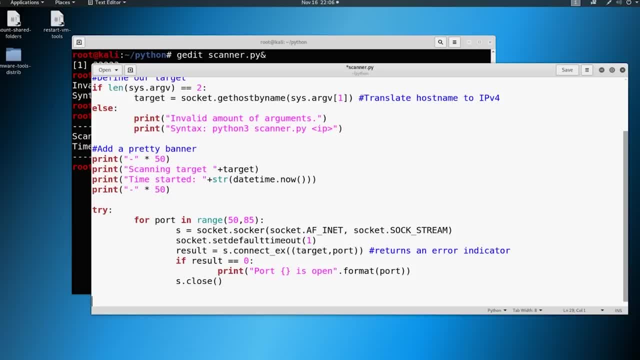 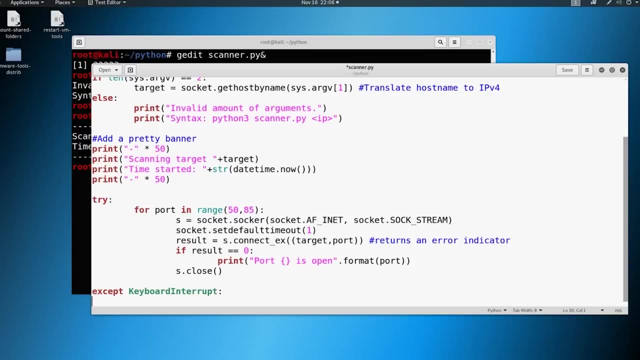 just one big loop that we're doing. Now we need to throw in a few exceptions to make this code really work. So here's an exception: exception- keyboard interrupt. So if you've been using Linux for a little bit now, you should know something like Ctrl C is a keyboard interrupt. So if we want to, 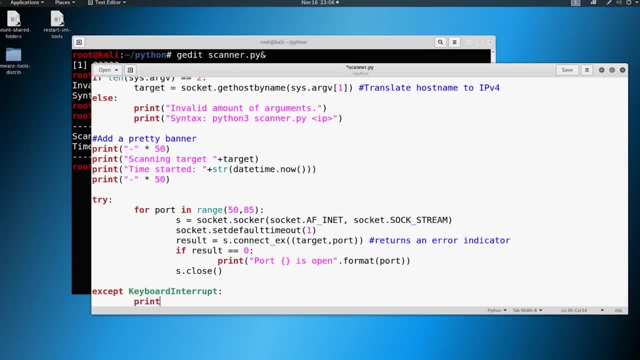 interrupt the scan. we need to define that there is an interruption here. So I'm just going to put in something like exiting program, Okay, And we're going to say when that happens, when there is a keyboard interrupt, we're going to say sys exit. 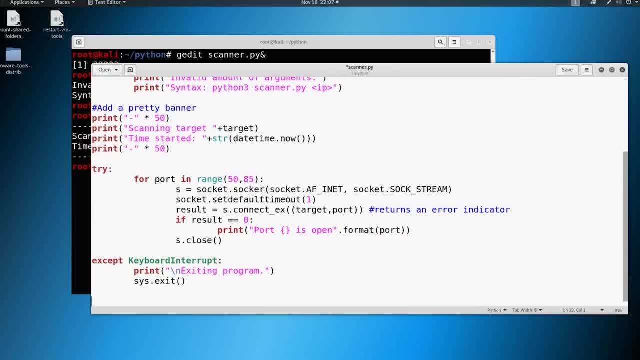 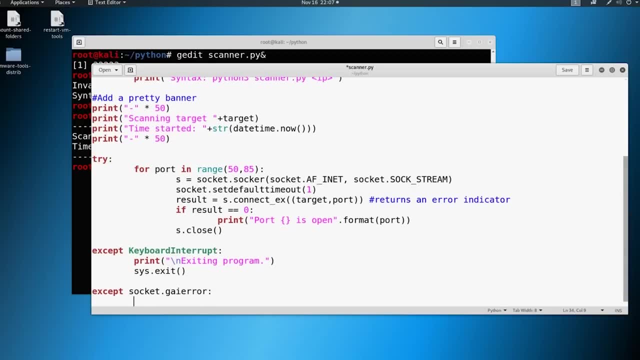 That allows for that clean exit. Okay, there's another exception that could be occurred here, right? So we're going to say socket that ga I air And we're going to say print: hostname could not be resolved. So if we can't resolve the hostname, DNS is failing us. 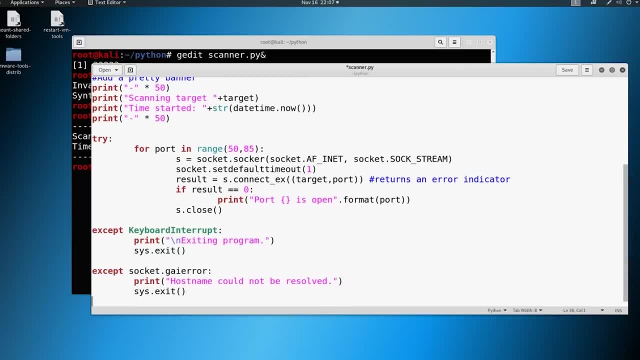 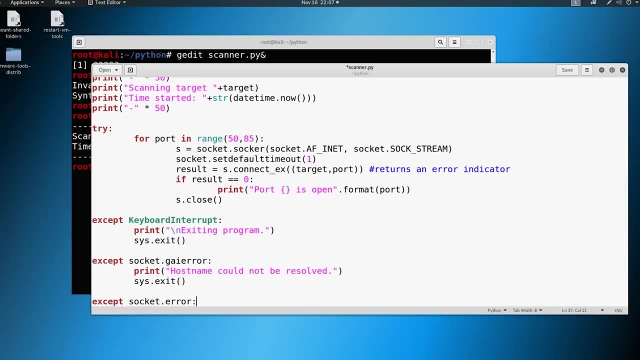 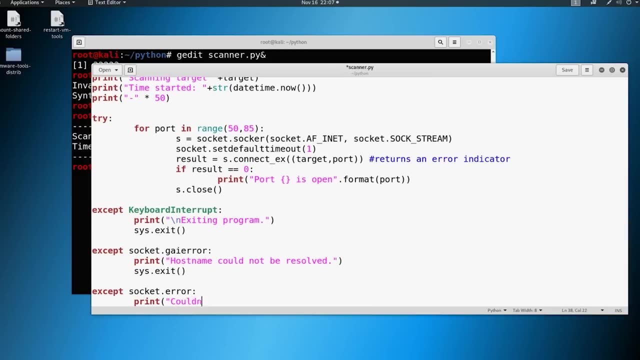 we're just going to go ahead and exit out. And then one more: What if we can't make the connection to the address in general? Well, that's what's called a socket error. So we're going to say socket dot error And we're going to print out: couldn't get like a type I couldn't. 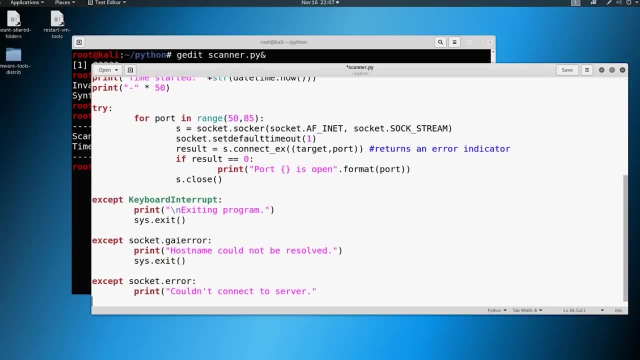 connect to server And then we're also going to exit this. So we'll say sys dot exit. So I'll give you a little bit of time to catch up on this script If you're behind. I was typing fast and talking as well. So one more walkthrough. we're going to do our for loop through these. 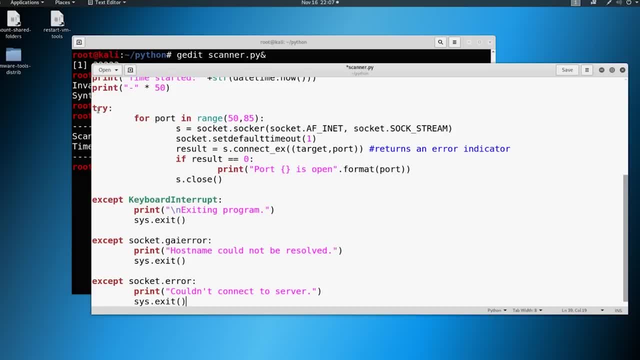 specific ports, We're going to go ahead and have some exceptions, So we're going to try these with exceptions here. if we hit Ctrl C, we want to exit the program. If there's no hostname resolution, we want to exit the program If we can't connect to the. 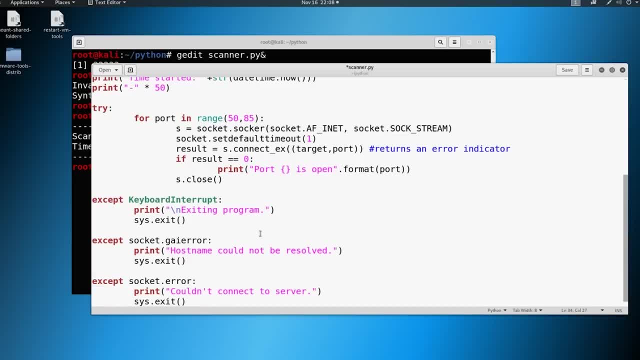 IP address that we specify. we want to exit the program, So we need to build in these exits And these are those that. this is that thinking logically that I talked about earlier in earlier videos- right, that we wouldn't hurt to build this out, and then just think logically- and I will be- 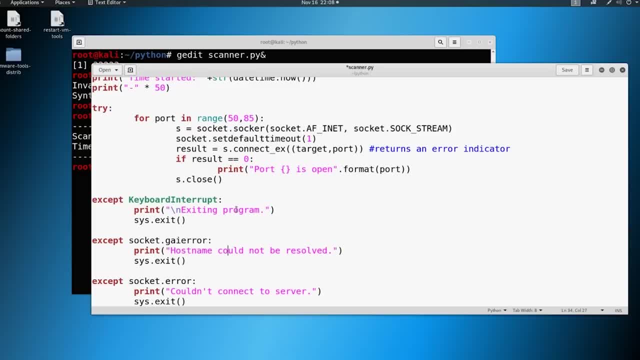 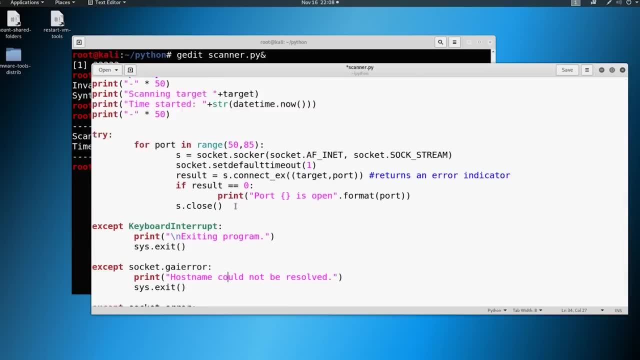 able to tell you that when I build the script out and I write it, it's always terrible. First time is always terrible, 10th time still probably pretty terrible. You have to start thinking of things logically. Like you might not define an if statement at the beginning, right, You might. 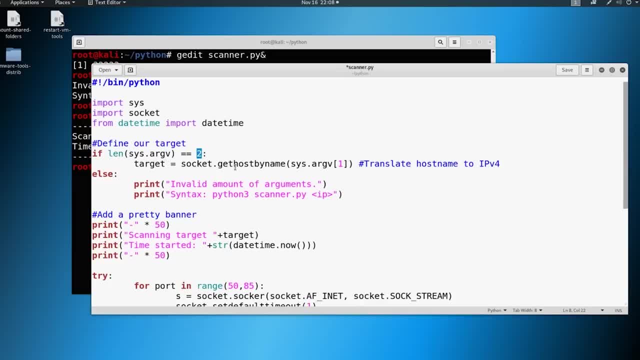 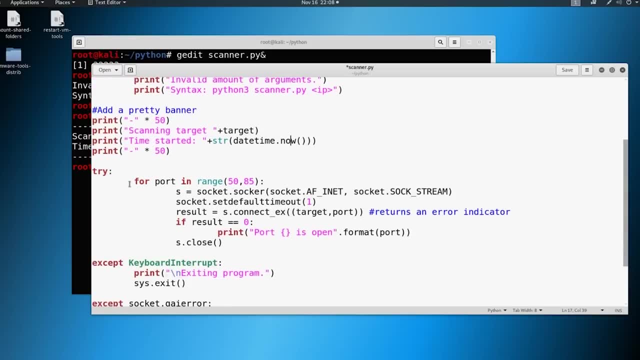 have to think through that, Because you might need one argument, or two arguments, or three arguments and you don't know. So maybe this doesn't look like this And it doesn't look like the pretty banner in here either, And you just start with this for loop And then you realize, well, maybe I should. 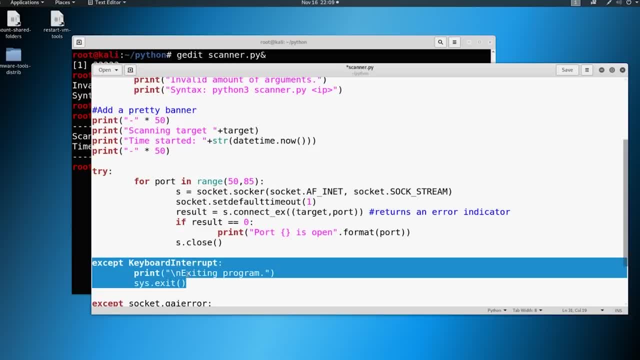 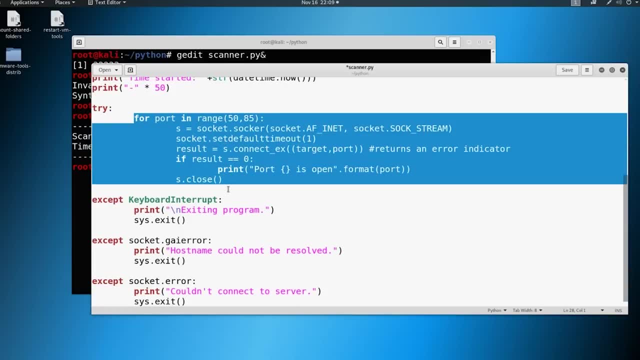 make that a try statement, Because what if the user wants to exit? Or there's no connection for a host name, Or there's no connection to the server? How do we get out of that? Or else we're just going to be stuck in this for loop until it's done. But if we get into one of these air, 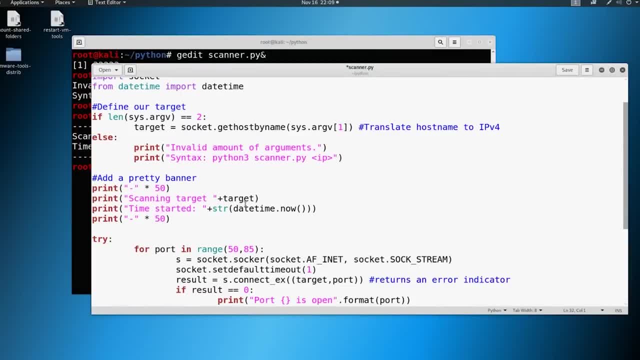 situations, it's going to get weird, Right? So, and then you start thinking through: okay, well, I know my arguments, So let me go add in a statement at the top So the user knows how to use it. And then 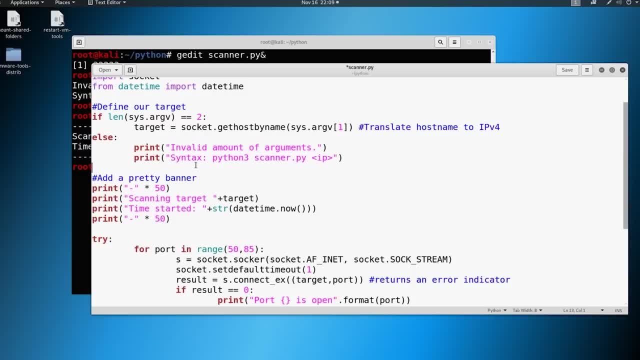 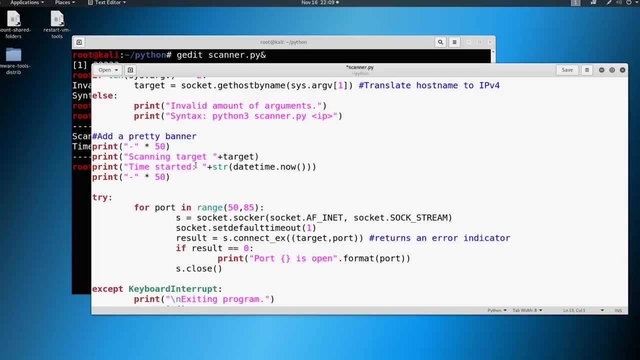 maybe I'll put a pretty banner in there when it's all said and done And it starts to really- you know- design itself. Now, before we run this, let's talk about why this isn't great. This is going to sit here and 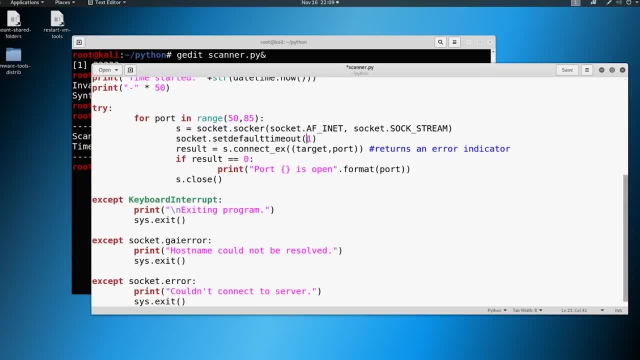 run through one port at a time for a second of a timeout and then reiterate: this is going to take a little bit to run through these little ports. Now, when we get into scanning, you're going to see that there are tools out there designed that do it much better, much more efficiently and much 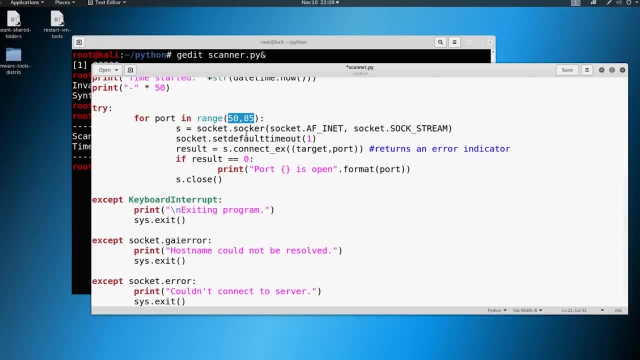 faster. This is not the best way. there's something that we could do, called threading. Now, threading is going to be a little bit more complicated, But if we run it, it's going to run multiple processes at once for us and allow us to scan a lot of ports at once. That would be a potential. 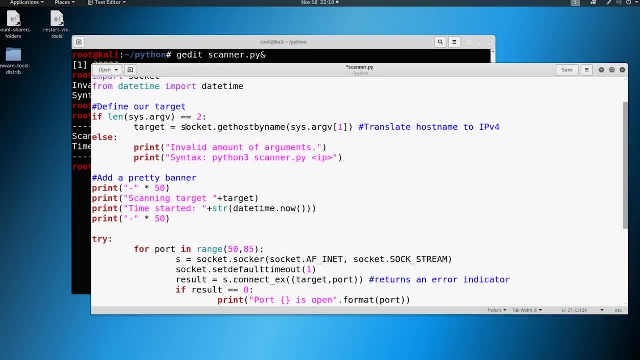 idea here And there's just improvements that we can do. You know, some of the things that we thought about already, like the, the socket get host by hostname. you might not have thought about that in your first iteration. you might just say: Hey, I want to just put it to IP before. 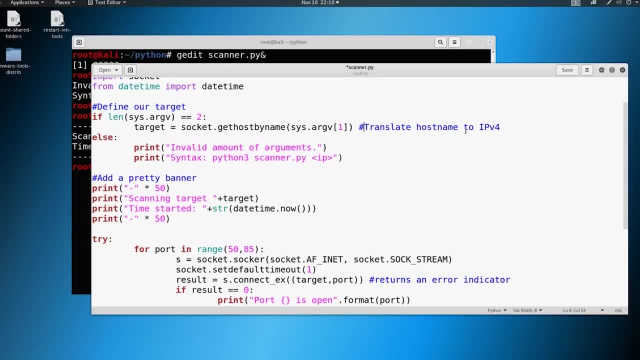 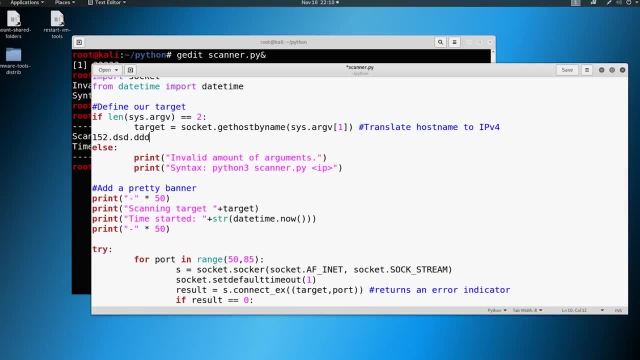 And what happens if you know we supply an argument and the argument is a bunch of numbers. you know it'd be like 152. And then you got letters and somebody mistyped, or or what if you give you know an IP address that doesn't exist, something like this: 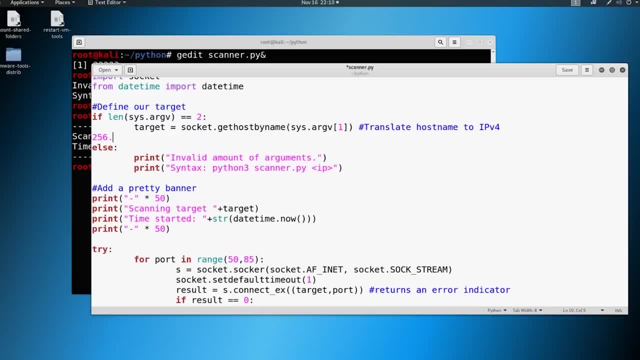 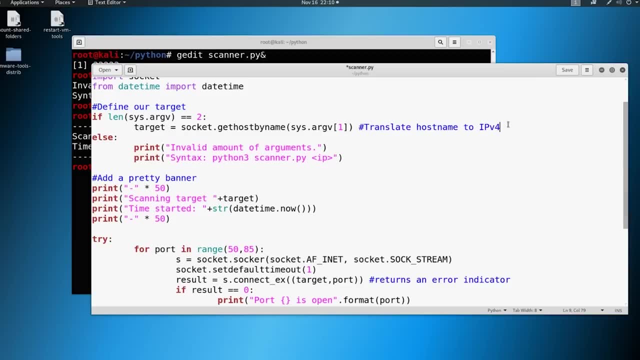 or you know, maybe like 256 dot or 257, or something. you know that that isn't possible. how is that built in? How are we going to prevent that in our script? Right now, not that big of a deal. We're writing this for ourselves, So you know it's not, doesn't? 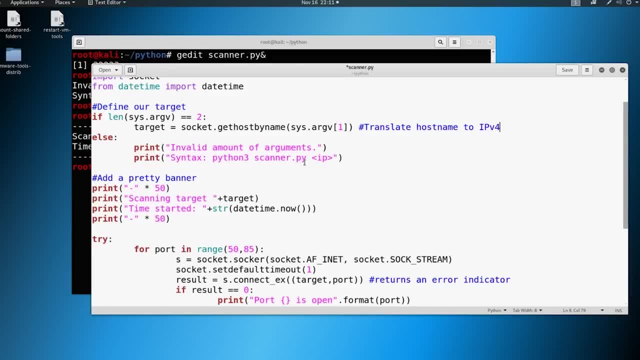 be perfect, But if we write this for somebody else, we go put this on GitHub. we kind of want all those errors to be handled, And that's where these exceptions come into play And these if statements at the beginning come into play as well, So we can handle those errors and those. 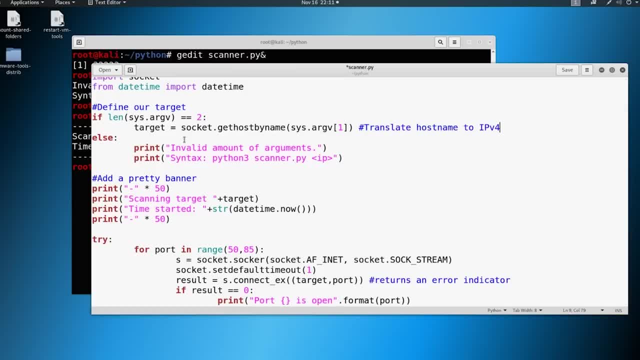 exceptions And we can really start thinking logically on how an end user might fat, finger something or break a program or do something, even maliciously possibly. So there are ways around this, And we'll talk about it as well when we get into a bash script that I wrote later on in. 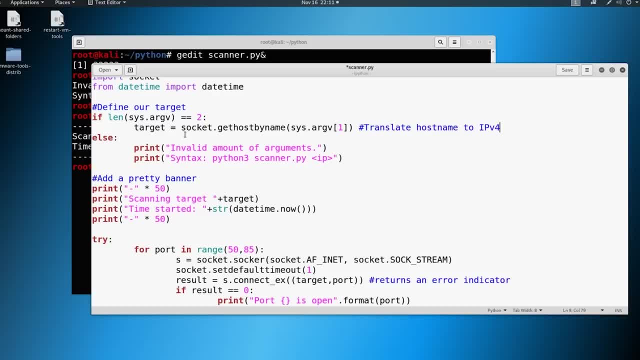 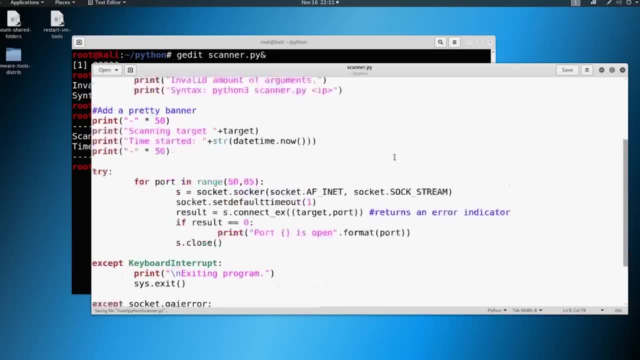 the course And we can kind of look at how that was written and how it strips out some arguments and prevent some human error. But we'll get to that later, So let's go ahead and actually save this Now. we've got our scanners scanner script and we're going to go ahead and run it, So I'm 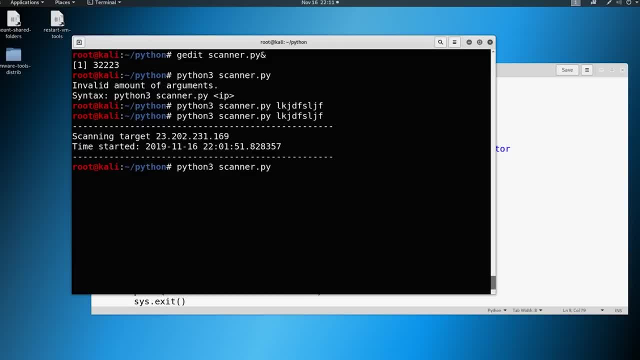 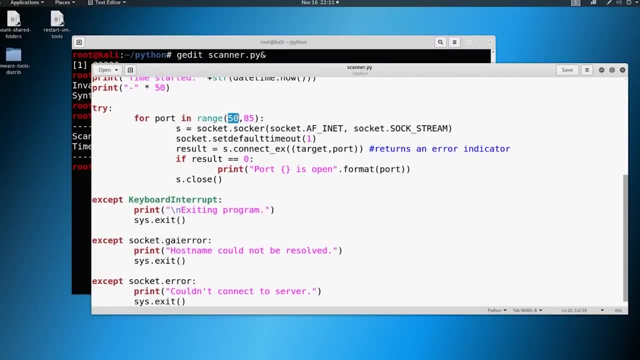 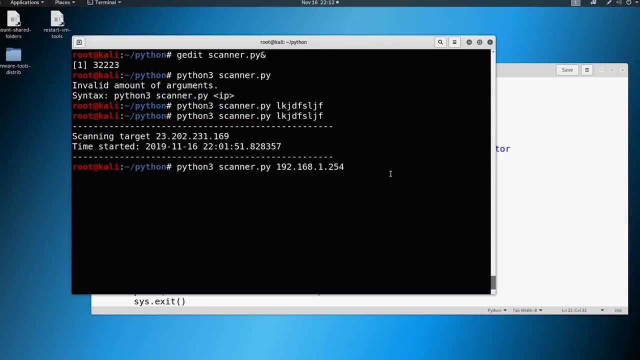 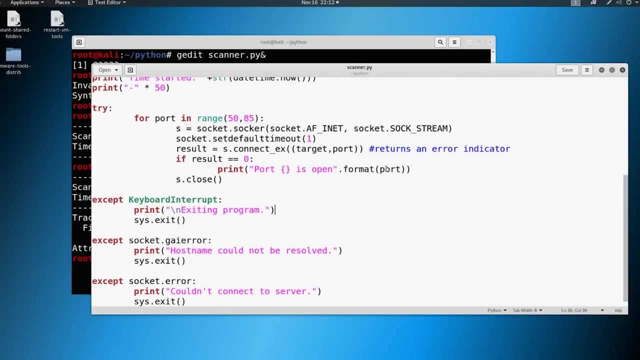 going to run this, And I'm going to run this against my router. So my suggestion to you is to do the same, or do it to a machine that you know is in your network and has a port open. So I'm going to go ahead and run this And I have a typo, So I have something called soccer here. I. 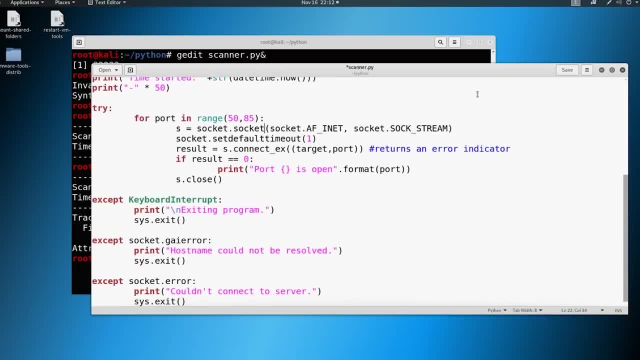 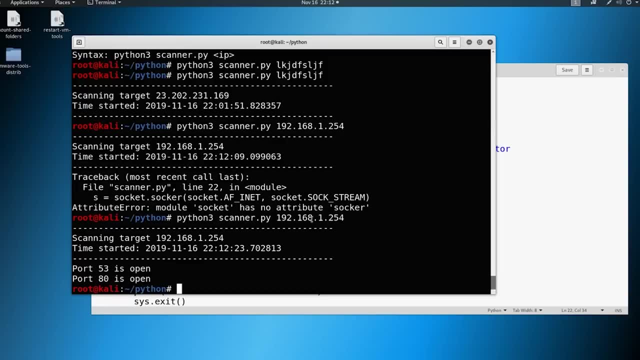 sure do. If you caught that originally good job, You knew I was gonna mess up. Let's try it one more time. And there you go. So it just ran through it really fast, said: port 53 is open, port 80 is open, And immediately. 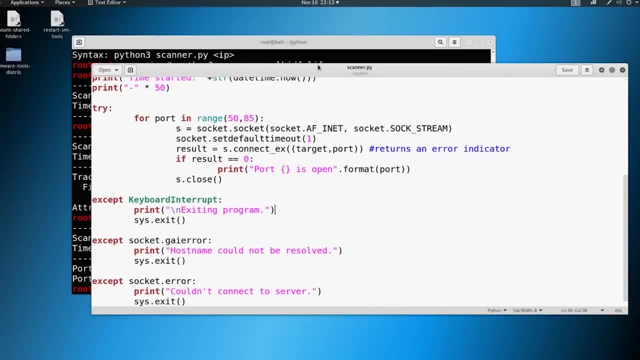 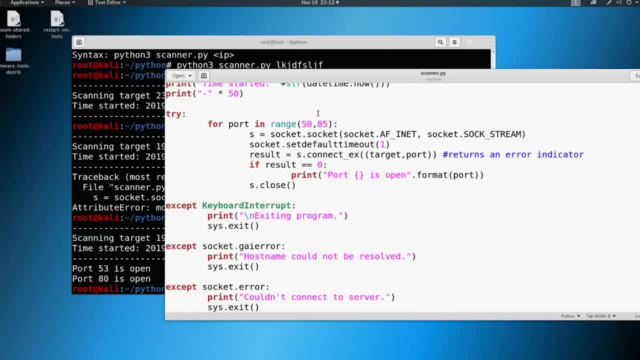 you know, it knew, it knew, So it did its job. it went out there And it found port 53 and port 80, which is what I was expecting. Hopefully yours did the same. Now I could back this off to one through. 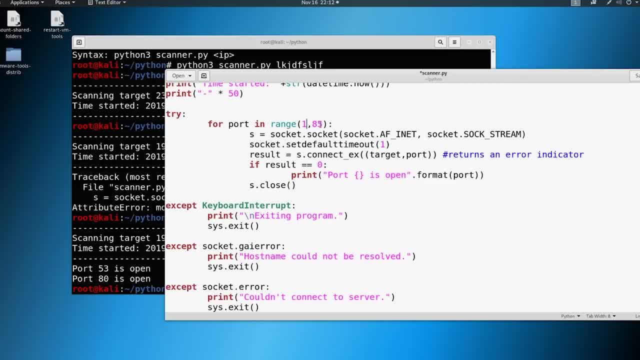 you know 65,535.. And another thing we can do: if you want to see the speed, let's say 65, 535,. I'm going to keyboard interrupt this, but we can print out something along the lines of checking port and then we'll do something like this: Okay, and then we say dot format. 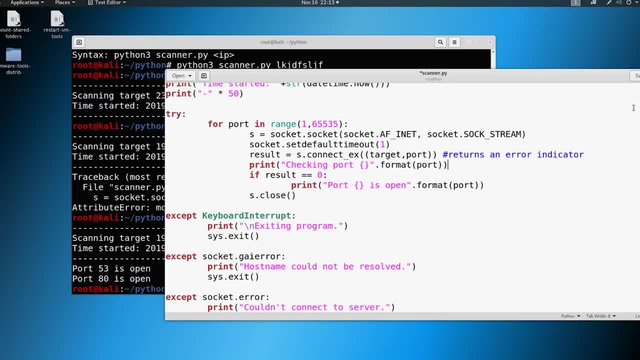 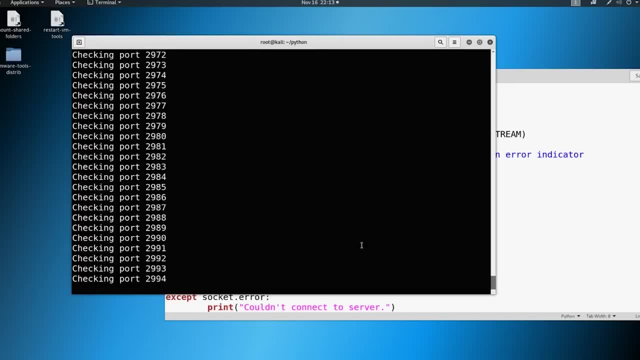 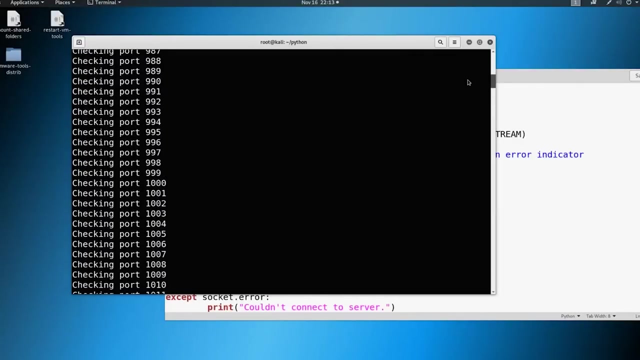 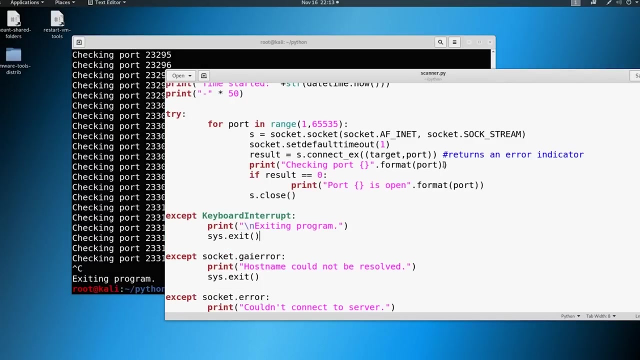 and then part. So when we save this and we run it, take a look now. So it's checking through all these ports. It's going kind of fast. Look it's, it's finding ports. But this isn't pretty right. We wouldn't want this. we only want it to say: when the ports open, But it's taking some time, We're on port 20,000 of 65,000.. So, on top of you know, just being being a little bit annoying, it's, it's really, you know, throwing our screen into 20,000 lines now. So the only reason I would put a statement in here like this is if I was doing a couple numbers and I wanted to see, like, if we go back to 50, and to 80,. 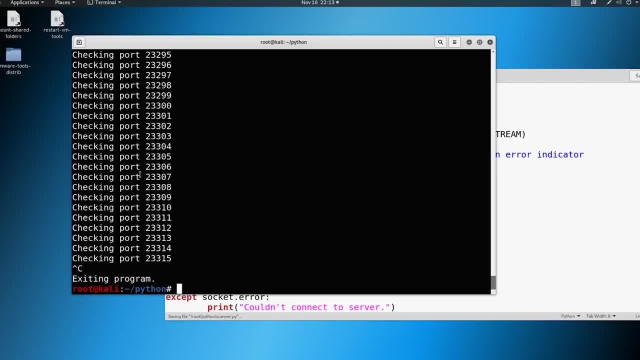 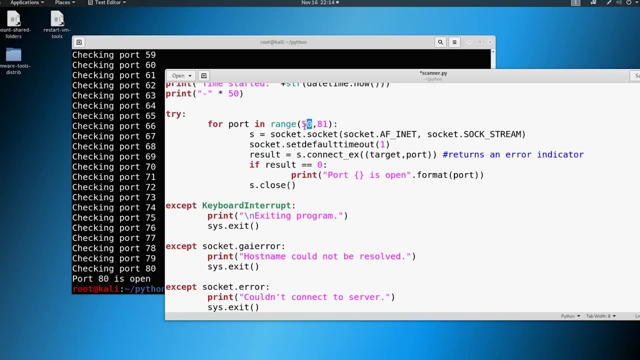 we'll do 81.. We do this. it's good way to see how fast your scanners running. if it's running, It's a good way to have print statements in there if you might see any errors, And you can see. it ran through 80 pretty fast and found 53 and 80 open, So I would delete this. if you want to do a full port scan Again, you could do one through 65 535.. Go ahead and save that. Sorry if you heard my dog barking. It's really windy tonight, So we're gonna go ahead and do it one more time. And now. 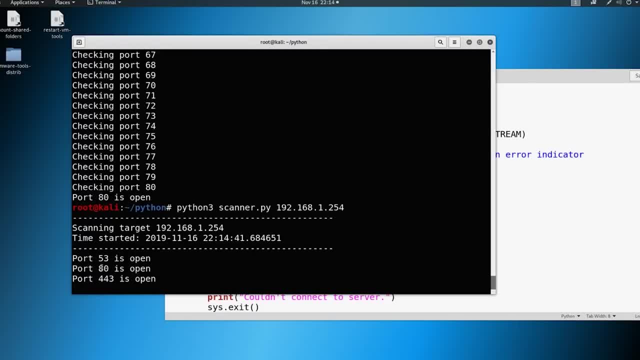 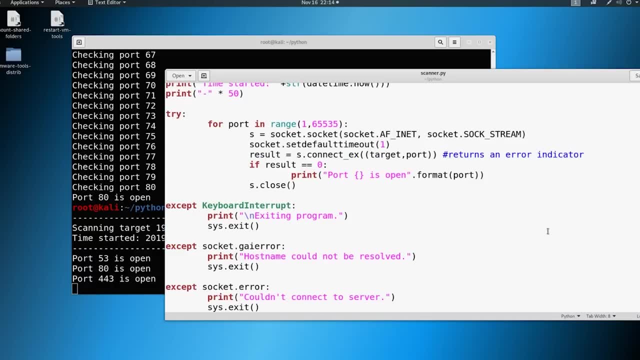 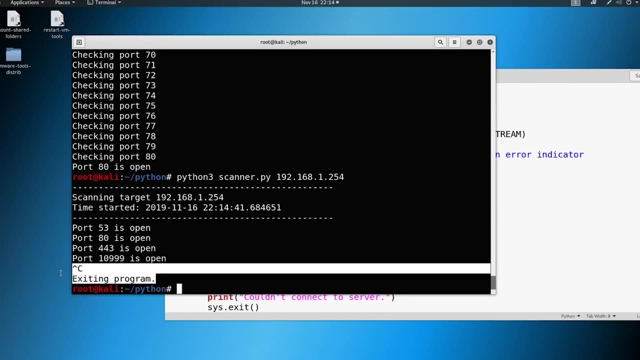 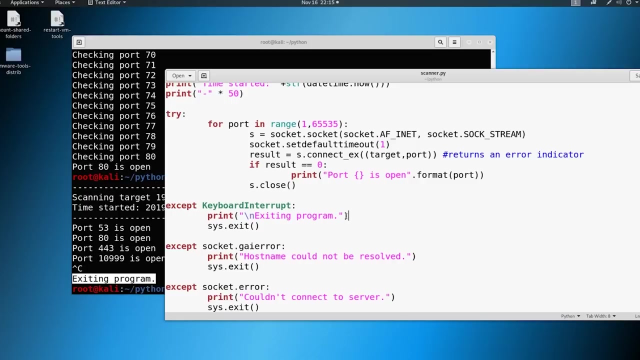 it should be a little prettier. And then, as the ports are open, it'll print out And if you want to get fancier, you can have a little thing at the bottom that says: Hey, this took this long to scan. here's how many ports are open, etc. So this is finding all the ports. So I'm going to go ahead and Ctrl C and you can see now exiting program. our keyboard interrupt worked. So everything is working really, really well And that is it. So that's it for the Python series And hopefully this all made sense, This all built upon it. 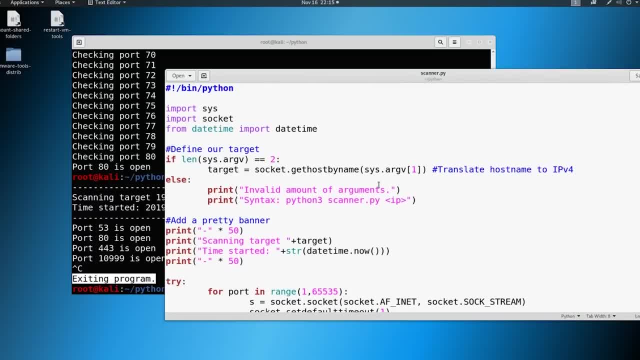 You know we could take this, and the goal here again is not to be an expert in Python. The goal here is to get you interested in Python, to get you seeing that it's really not that bad. And in about an hour and a half to two hours time we started with nothing and built out a nice script that all you know just built lesson upon lesson till we got here. So we're going to move on and actually get into the hacking. you have successfully completed all of your foundational courses. we've got the Linux down, we've got the networking, 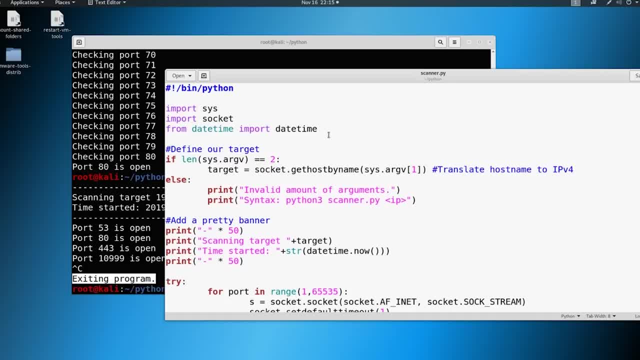 down. we've got the Python down and now we're ready to get into the good stuff. So I'm very excited to do the hacking. This is our strong suit, This is our bread and butter And we're really going to knock it out of the park. So I will catch you over in the next video when we start learning about hacking. 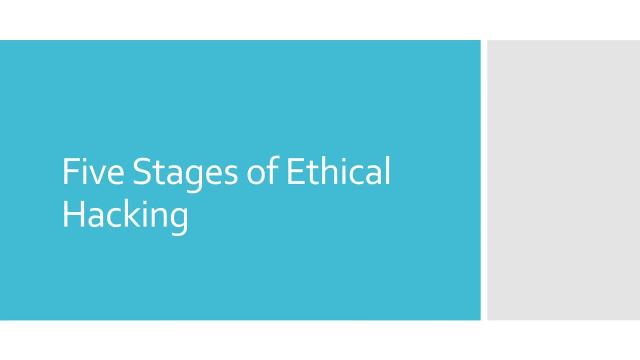 Okay, before we get hands on, I have to give you a little bit of death by a PowerPoint, but it's for good reason. So we need to introduce the five stages of ethical hacking. These are the five stages that you will go through on every assessment. So before we do that, let's first make a big note: From here on, we are moving into the ethical hacking. 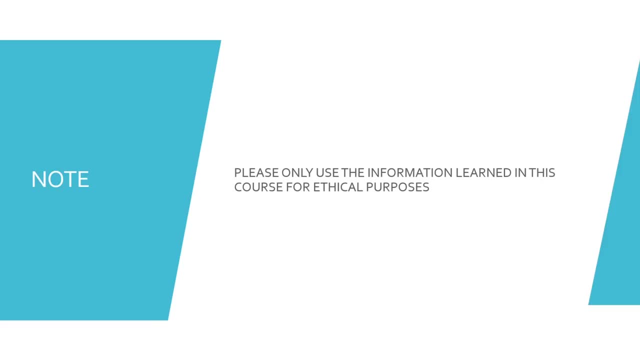 portion of our course, we're going to learn malicious things. Please only use the information learned in this course for ethical purposes. Do not attack your neighbors. do not attack anybody that you do not have explicit permission to do so. You can and will get into trouble for doing that. So with that out of the way, let's talk briefly about. 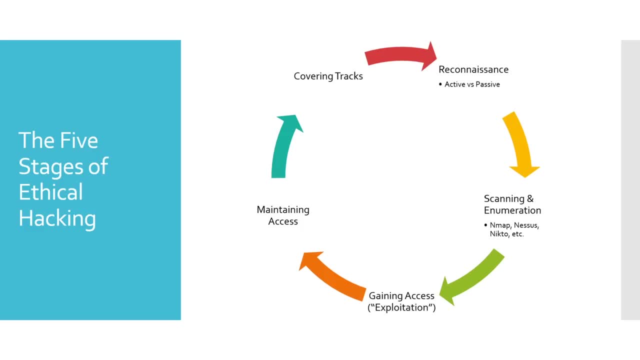 the five stages of ethical hacking. So we start up at the top And we actually start with what is called reconnaissance. The stage is also known as information gathering, And there are two different types. There's active and passive. Now, passive is saying like going out to Google and 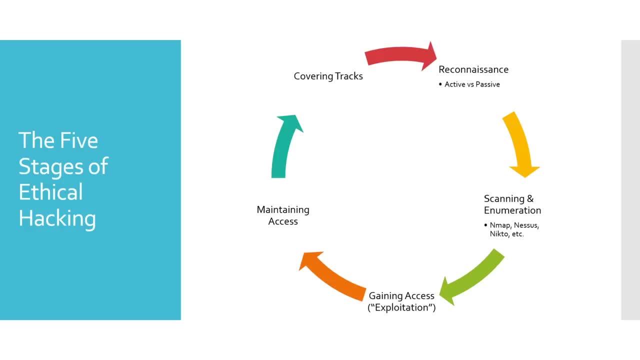 searching for somebody. say, you're given a client and you want to look at their Google. you want to look at LinkedIn. you might be looking for I don't know a picture of their badge or an employee's name or maybe an employee's Twitter page. That's all passive. you're not actually going out to the 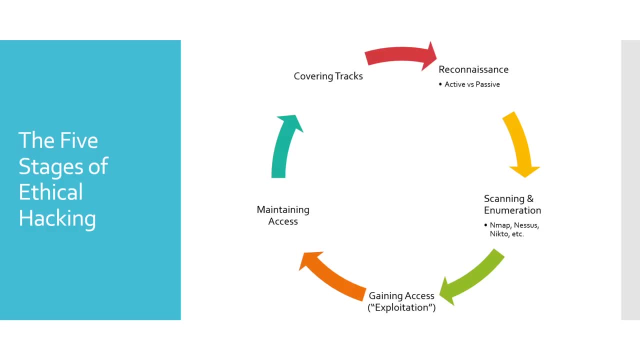 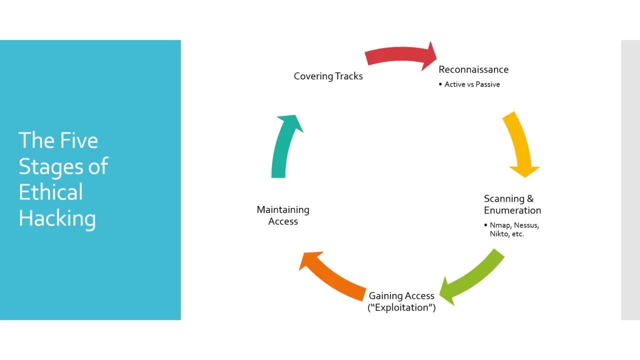 tools such as NMAP and Nessus and Nikto, and you've never heard of any of those. that's fine, But we take those and we scan actively against a client. Now what we're looking for are open ports, vulnerabilities, different items And with what returns on these results when we do this scanning. 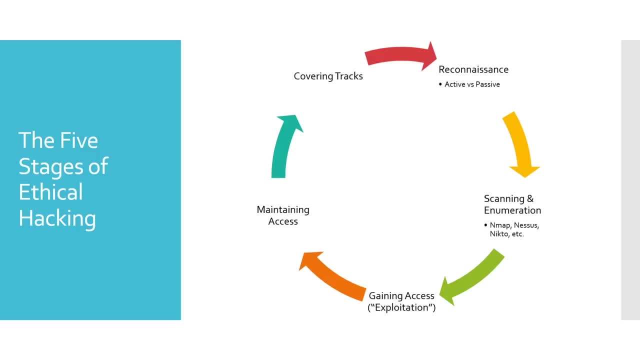 we also perform what is called enumeration. Enumeration is just looking at items and digging into them to see if we can find anything of value. Say that there is a web server running on port 80. We see port 80 is open and it's running something like Apache 1.2,. 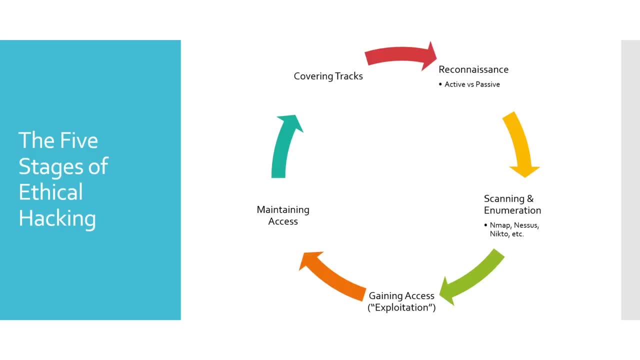 which would be really, really outdated. We would go out to Google and we would say, Google, do you know if Apache 1.2 has any exploits for it? And we would do research. That's the enumeration portion of it. So once we do our information gathering, we do our scanning enumeration, then we move into 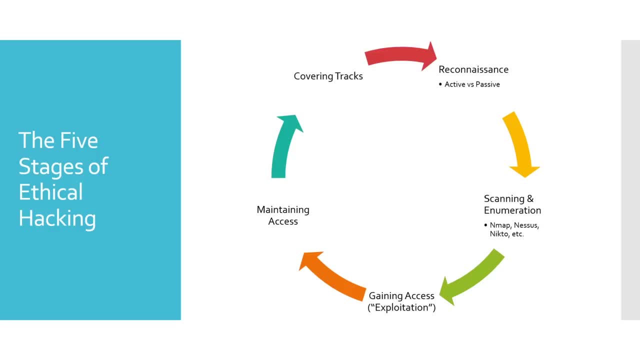 the gaining access portion. This is also known as exploitation. We will run an exploit against the client or against the vulnerable service, or whatever it may be, to try to gain access into a machine or into a network, into an environment, etc. Once we have. 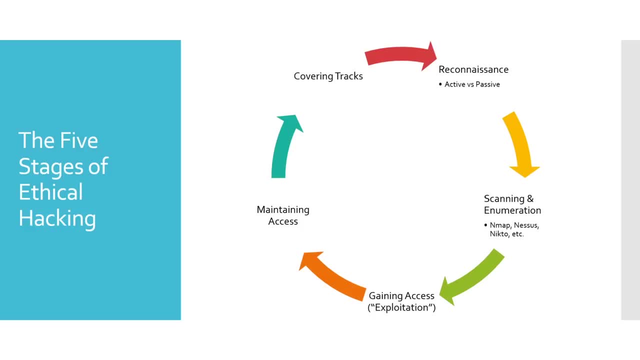 that access, the process starts to repeat. We do scanning and enumeration again and we also want to maintain that access right. So if we were to get kicked out, okay, or a user shuts down their computer, how do we maintain that access? So when they do that, we're going to have to do a 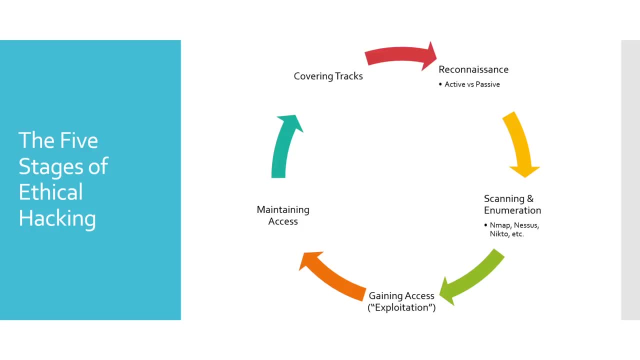 lot of things. We're going to have to do a lot of things. We're going to have to do a lot of things back on. we still have access to it. And then, lastly, there is the covering tracks. you want to. 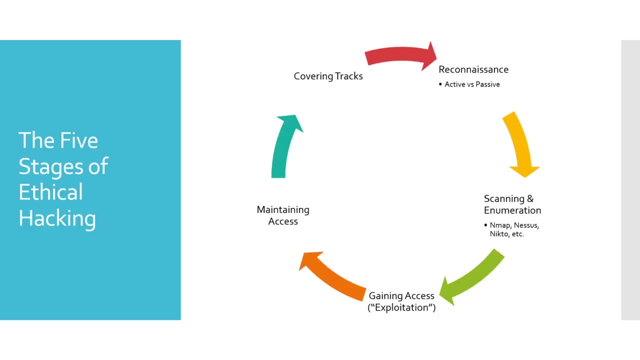 delete any logs that you may leave behind. you want to delete any kind of malware that you upload, which is more important as a pen tester- any accounts that you create for any reason. you want to delete those as well. you really just want to clean up is a good way of putting it. covering. 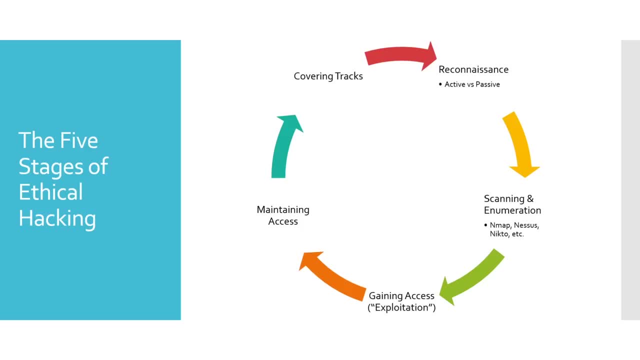 tracks is the more hacker way of putting it. But as a penetration tester, you really just want to clean up. So we're going to go heavily through steps one through three In this course. we'll also cover four and five briefly, But the process and methodology never changes regardless. if you're 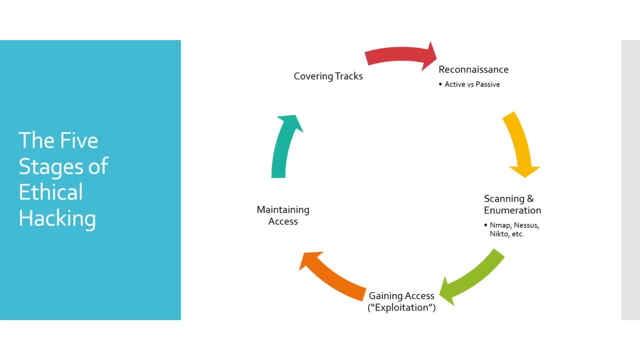 doing network, if you're doing web app or if you're doing a different type of assessment, it's all similar In this five stages of hacking. the tools might change, the attack methods might change, But the overall methodology is always the same. So we're going to go heavily through steps. 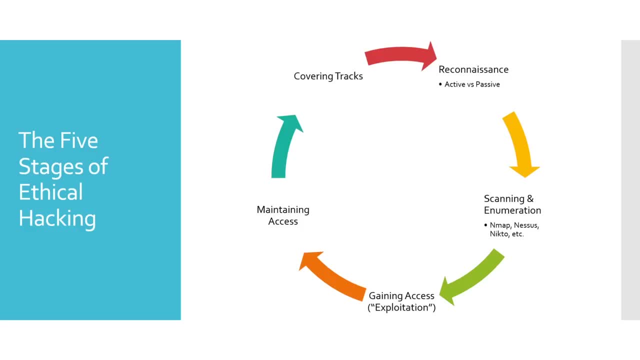 one through three, and then we'll go into scanning and enumeration And then we'll start with exploitation and do that repeatedly till we get it inside of our heads And it feels almost second nature, right. Once we have all that done, we'll do some practice boxes. you know, give it a go. 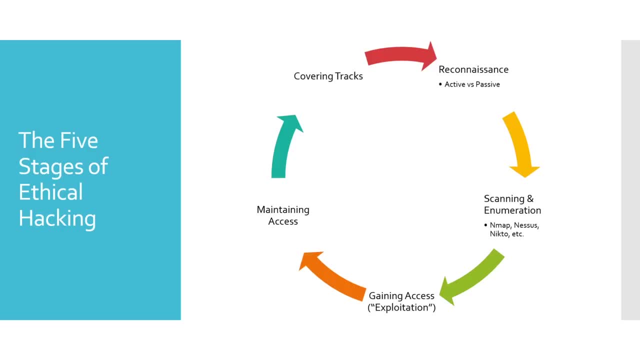 see how we do. we'll move into the internal side of things with active directory. we'll start working with our web applications and our wireless and we will touch on the maintaining access and covering tracks. But you're going to see this methodology over and over And you might also get this question on an interview, you know. 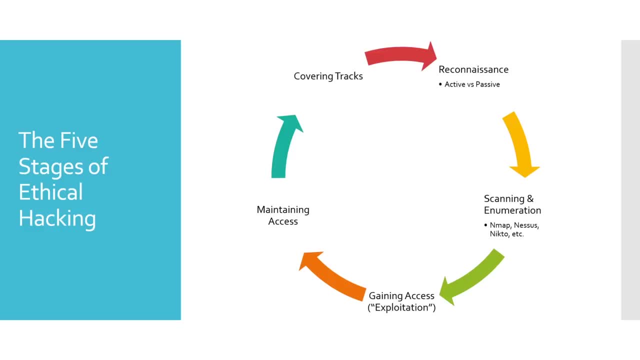 to describe the five stages, So it's important to know these. it's just something that every ethical hacker can rattle off pretty quickly. So have this written down, think about it, keep your wheel spinning And let's go ahead and move on to our first section, which is going to be about how you 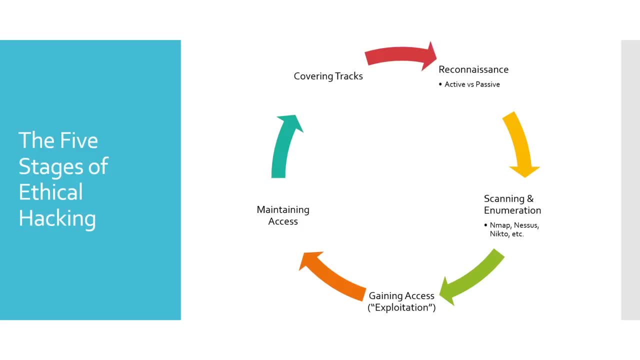 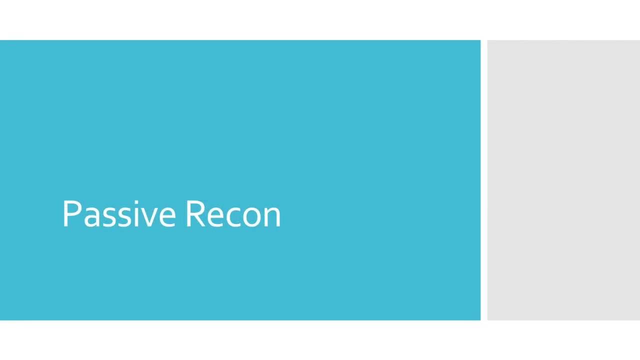 can use a client, which is going to be information gathering, slash reconnaissance, sorting, some cool tools, some Google foo and just what kind of information we can actually gather on a potential client. So in this section we're going to be talking about information gathering and all the 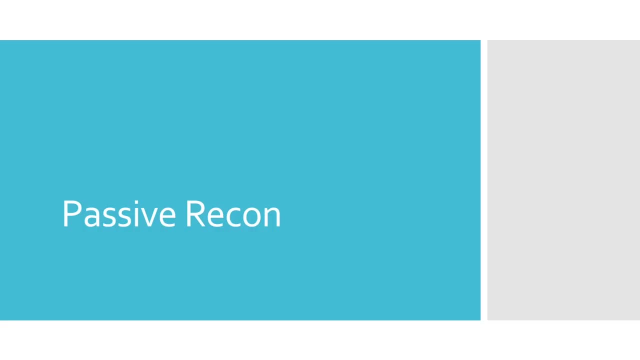 information gathering we're going to do in this section is going to be passive, So I'm calling this passive recon or passive reconnaissance. I wanted to give a brief overview of what we're going, review of what we're going to be covering, and talk about some high level topics before we get. 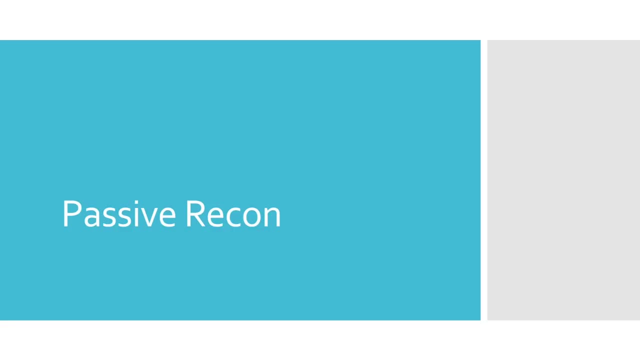 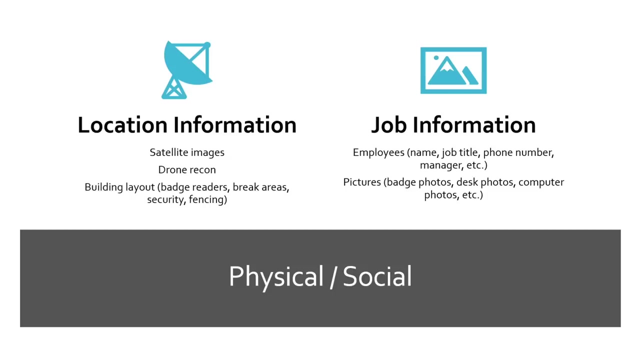 into the weeds and really dive into our target. So let's talk about the different types of passive recon. So on the physical or social sides. physical meaning actually going on site and maybe doing a physical engagement, or the social engineering aspect of maybe doing a phishing assessment or 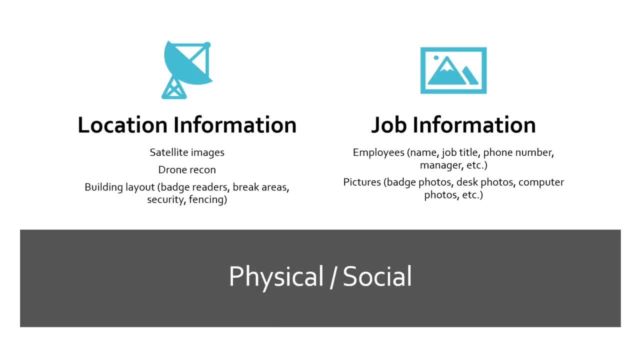 even including it in a physical engagement or a phishing assessment. just gathering this information from the physical social aspect is incredibly useful. So we have location information, So we might utilize something like satellite images, or often we'll go on site and do drone. 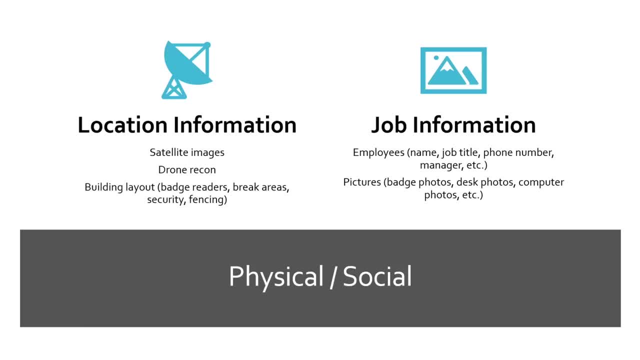 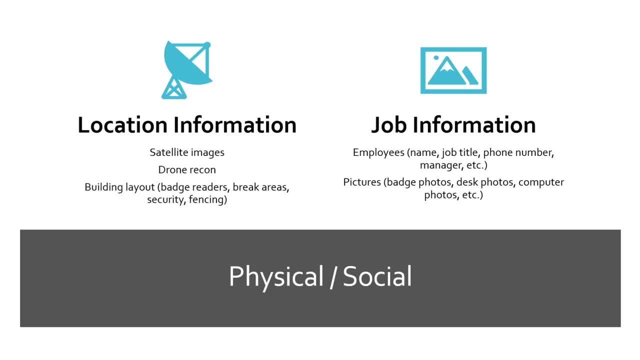 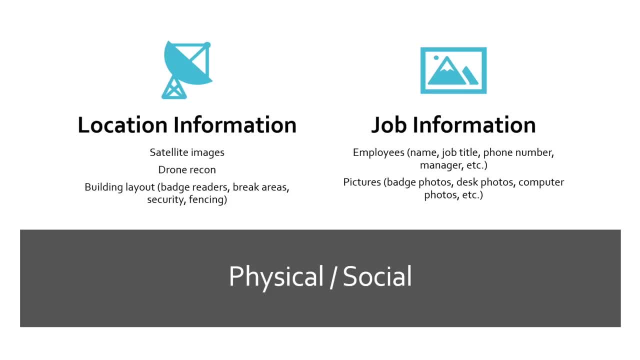 like: Are there areas where they're just leaving the doors propped open? Where do people go out and smoke? in these break areas? Because those are good place to just walk up to somebody, light up a cigarette, even if you don't smoke, and just start a conversation and then tailgate right in with. 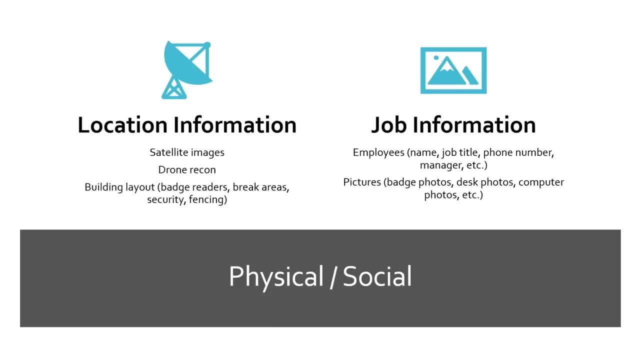 them into the building. Now, the other aspect of this is the job information, So we might be looking for employees online. I might want to know somebody's name, job title, phone number, who their manager is. I try to get a good. 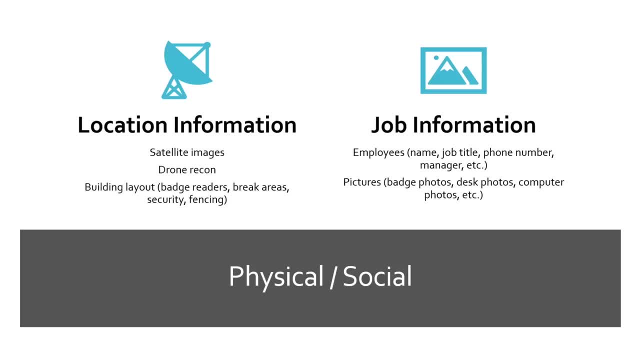 idea of what people look like, So if I see them on site I have a good idea who they are. I also look for pictures, So I cannot tell you how many times a badge photo is posted on LinkedIn or somebody posted on Twitter. you can see all the memes out there about the badge photo, So I can 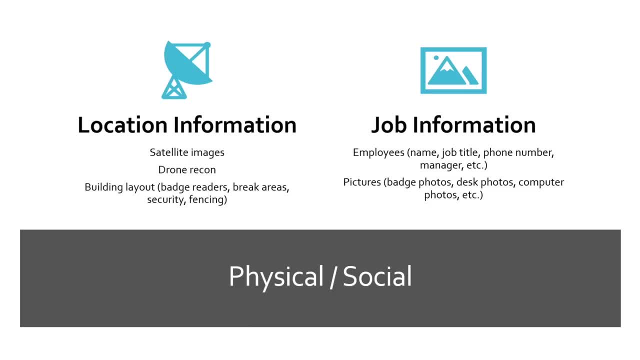 see all the memes out there about people posting their photos at work And it's bad. It happens all the time. I see it to this day. So we're looking for badge photos. I'm looking for desk photos, computer photos. I had a situation once where somebody took a picture of her watching a game at 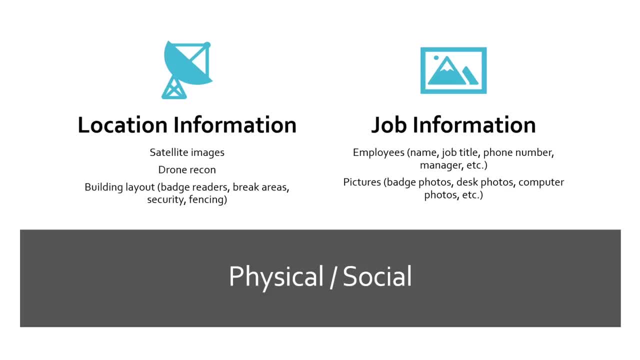 work. She was watching a basketball game at work And the basketball game was on her computer And on her screen there is showed all the different tools that they utilize that work. She had a work. in this photo there was a desk in the background. you can see different things And it just gives us. 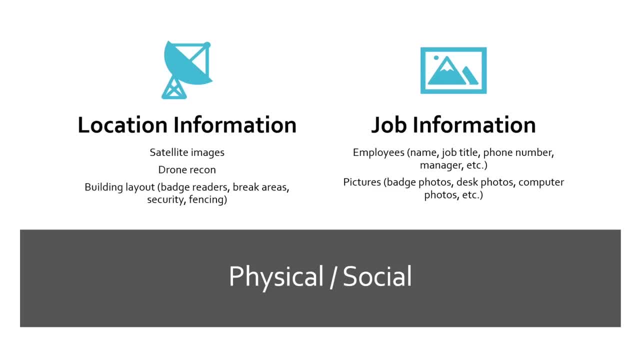 information, And that's really what we're after. What kind of information can we gather? Now, this course is not a course on physical or social, So I kind of wanted to give a high level of what to expect. We won't really be doing a whole lot of this in this course, with this type of information. 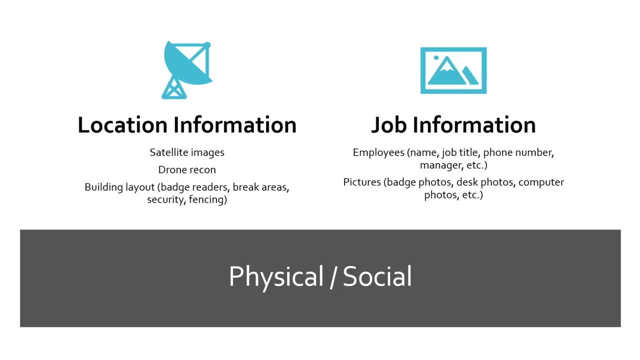 gathering, But these are the things that you should be looking for. So if you are tasked with a physical assessment, do go out there and look for the information that you're looking for, And if you're looking for satellite images, try to get a good feel of the building layout And also try 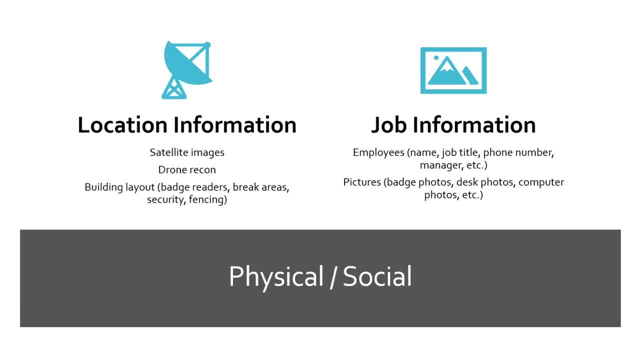 to get a feel for who the employees are, who maybe the IT manager is. in case you're going to say: you know I work for it, they might ask you who your manager is. you might need to know those names. And, of course, look for pictures. you can find a good badge photo and what that looks like. you can 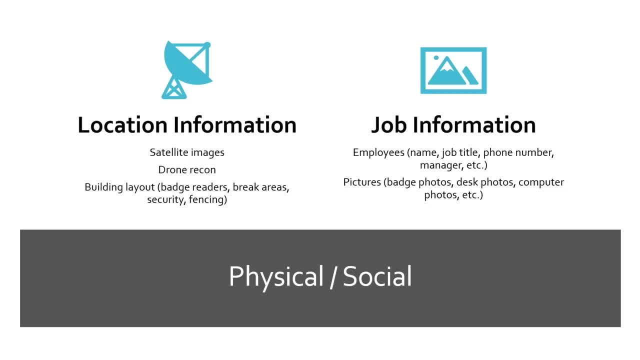 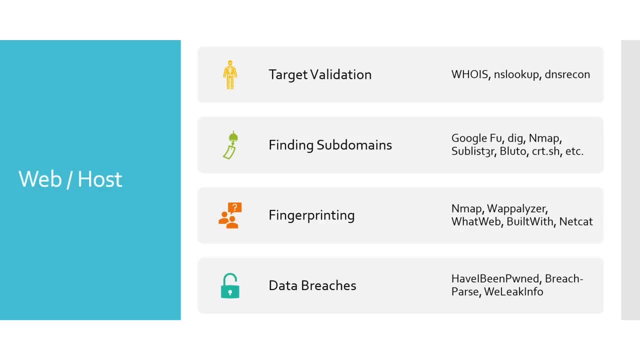 make a fake badge. go on site and you'll be way more passable with that badge, But sometimes they don't even look. it can be drawn in crayon. So there, let's go ahead and talk about what we will be doing, a lot of which is the web and host. So 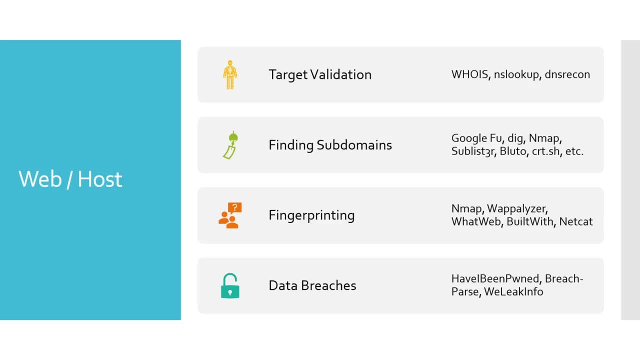 when you get a web or a host assessment, the first thing you really should do is what is called target validation. So we're going to be targeting something on bug crowds. we're not really going to focus on this, But what we're going to do in the real world is we would validate the target Now. 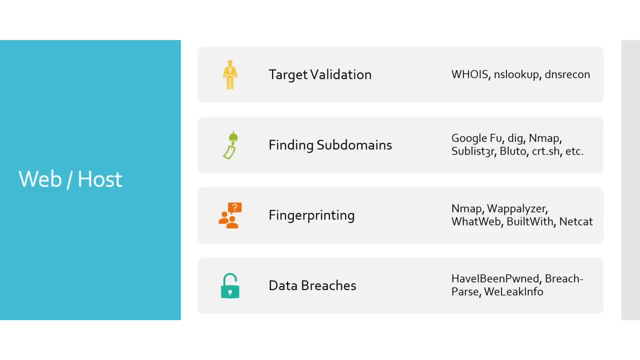 there are situations where a client will give you an IP address or a website and they might- they might- fudge it right, they might accidentally fat finger it, put the wrong number, put the wrong letter on the website And then, guess what? you're off attacking somebody else's website And there, if you're a podcast listener, there's a good 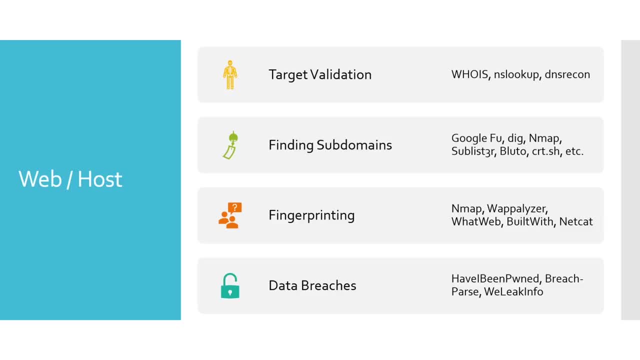 Darknet Diaries episode on this. If you don't listen to Darknet Diaries, go check it out. There's a great episode with a guy named Rob Fuller, aka Mubix, And he talks about getting the wrong IP address on an assessment and attacking the wrong people and actually gaining access to the. 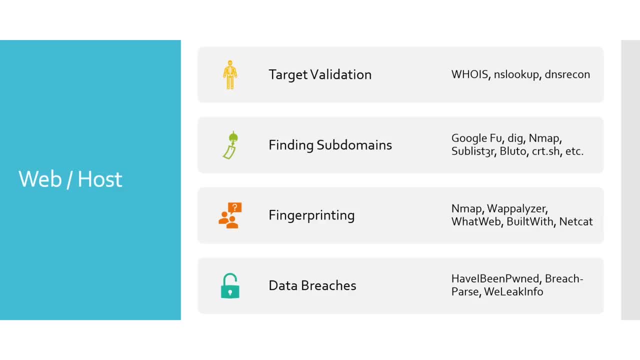 machine, which is a really, really big, big screw up on both parts right, So you should always validate your targets. On top of this, we're doing our web and our host on the website. we're going to look for subdomains And we'll talk more about that as we get into it, But we can do that with 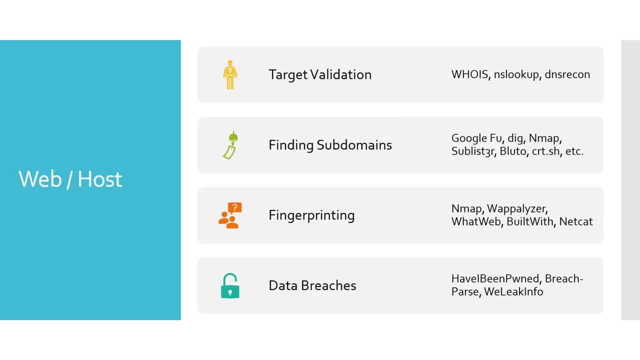 Google. we can do that with nmap sublister. there's so many different tools that we can use And we'll cover some of the tools and how to do it. get a little deep into that as well, especially as we get into the website of things. 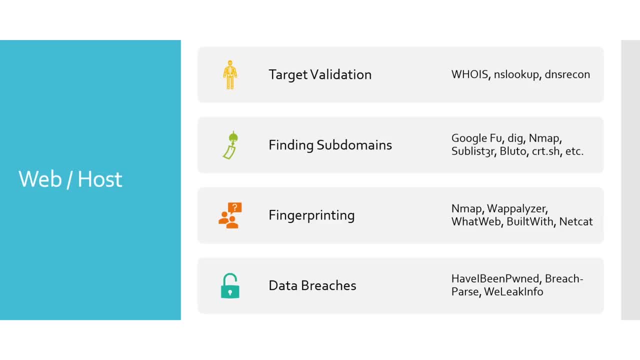 There's fingerprinting. we need to know what's running on a website or what's running on a host. what kind of services are out there? Are they running a web server? What's that web service? IAS, Is it Apache? What version is it Right? Are they running? what ports are open on their? 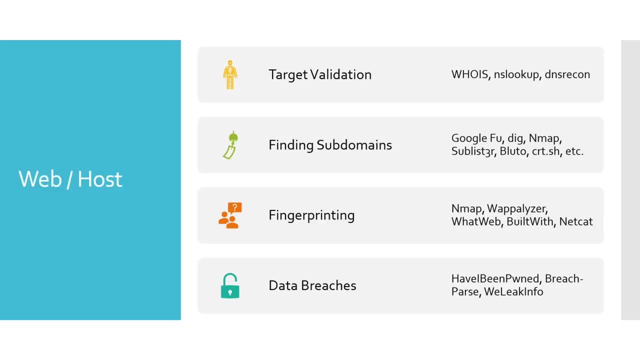 machines. Oh, they have FTP open. what version of FTP is open? So we need to fingerprint machines and kind of understand. But on the passive side we're not touching any machine right? So we're not gonna be doing much scanning against a host, we just have to utilize what kind of information. 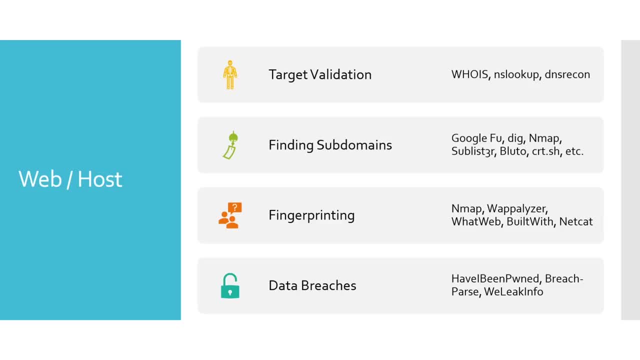 might already be out There. So if we go out to a website it's on the border of active, but as long as we're not scanning it in my book it's still passive. So we'll do. we will cover some of the passive slash active side. 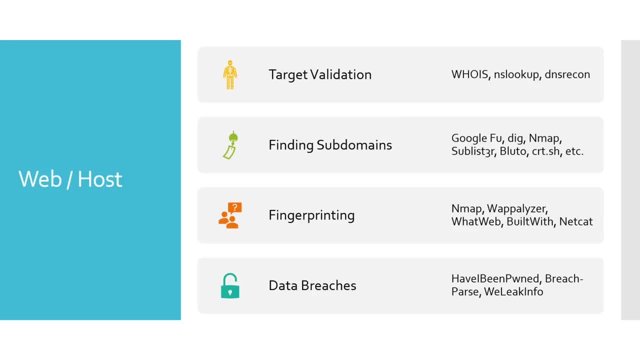 in this section And then when we get into scanning, we'll get way more active with it. Lastly, we're going to hit heavy, especially in the beginning, on data breaches. Data breaches are the most common way, when we're doing an external assessment, that we get into networks, Absolutely. 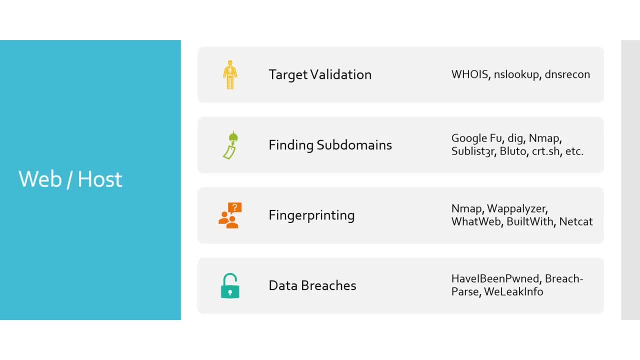 by far. when we talk about data breaches, we're talking about breached incidents from the past that have leaked data. Again, these are like Home Depot, Equifax, LinkedIn- all kinds of breaches that are out there that have had credentials dumped And then those credentials become 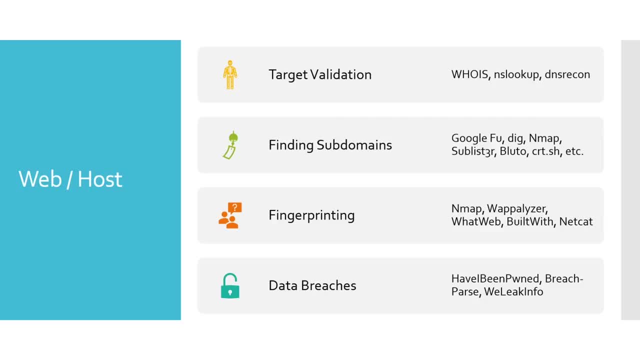 available to us eventually, And we try to utilize those to gain access, or at least utilize the usernames to gain access. Nowadays, most of the time, there's not going to be an easy just scan, find something, respond to an Instagram post or a text message, but at least we're going to be able to do it. 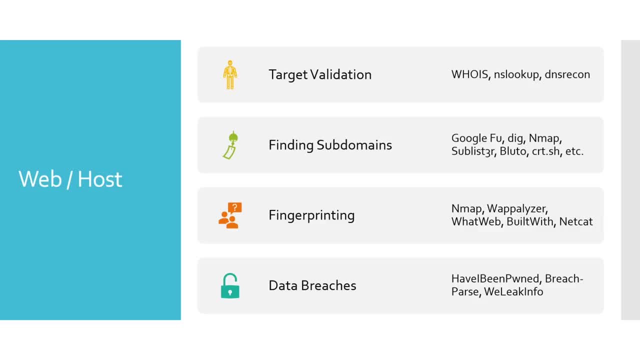 And we're going to be able to legally be able to use the information that we're not gathering now to mine it, to take advantage of those vulnerabilities and consider through the analysis- because it's way easier to learn them and no wonder they're so vulnerable- and exploit it on the 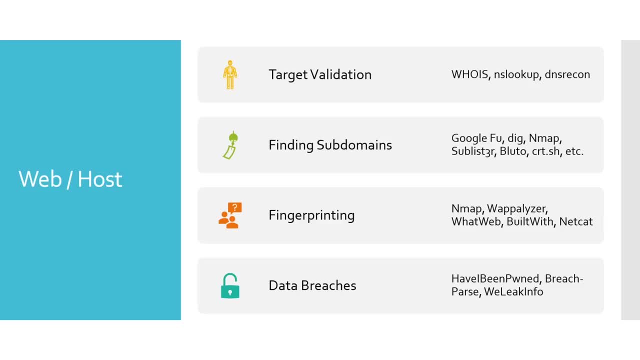 external side of the house. So we're looking for these data breaches and this information that we. So we're gonna start in with identifying what our target's going to be for this part of the section And then we're gonna go ahead and start talking about data breaches. 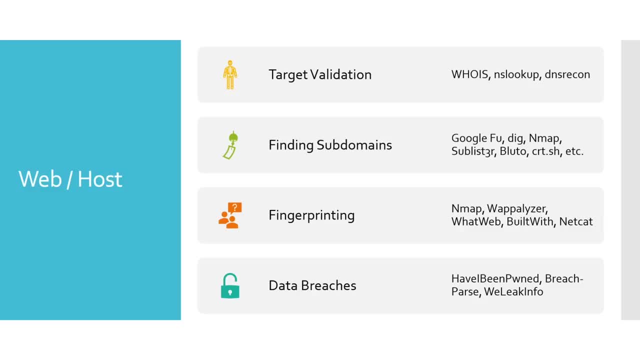 and why they're important and go deeper into that, And then we'll go off some of these tools that you see here on this list and really dive into those. So I will look forward to seeing you in the next video when we identify our target. 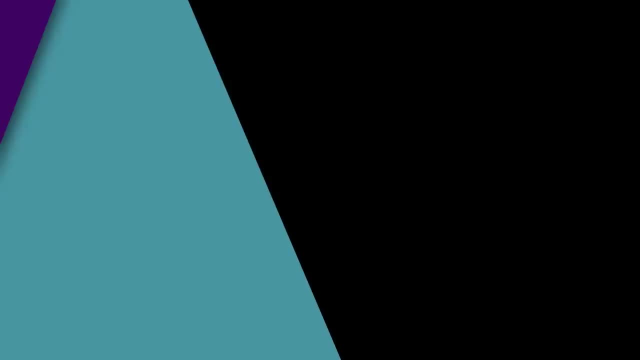 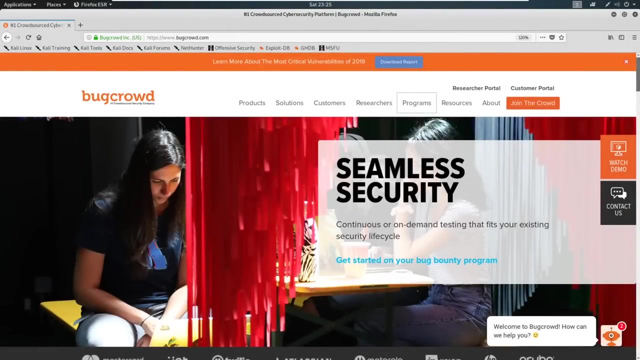 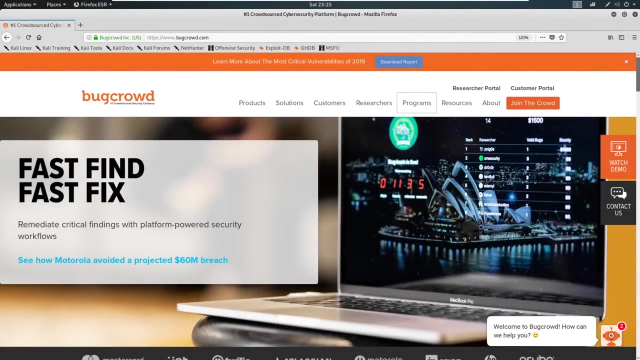 and get some information gathering started. All right, before we begin doing our reconnaissance, we have to establish a client to attack. So for this course we're going to be utilizing a client out of Bug Crowd. If you've never heard of Bug Crowd, 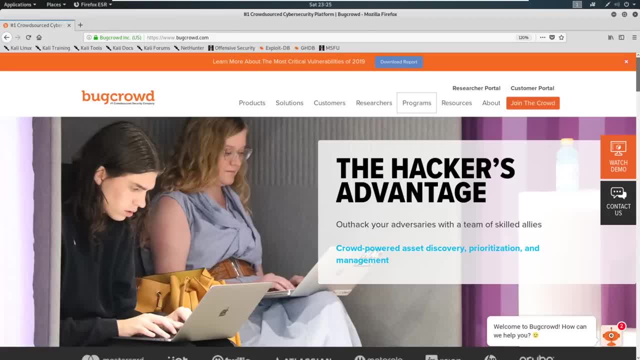 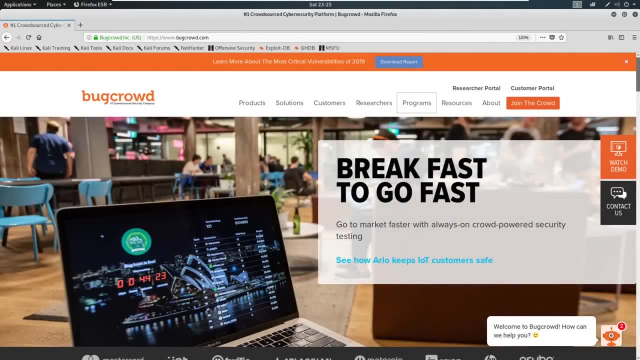 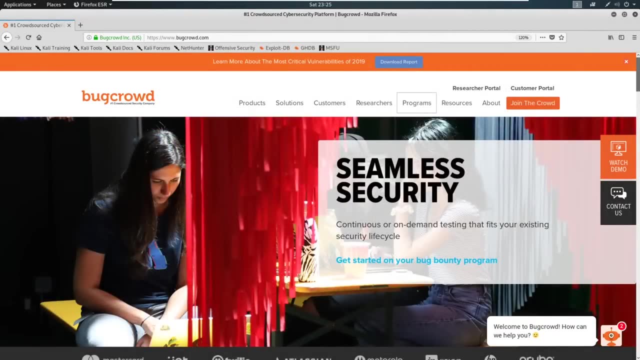 Bug Crowd is a public bug bounty program. What that means is there are programs on the website that will allow you to attack them, And if you find a bug against the program, you're able to submit it and potentially get money for it. So you are able to hack these programs publicly. 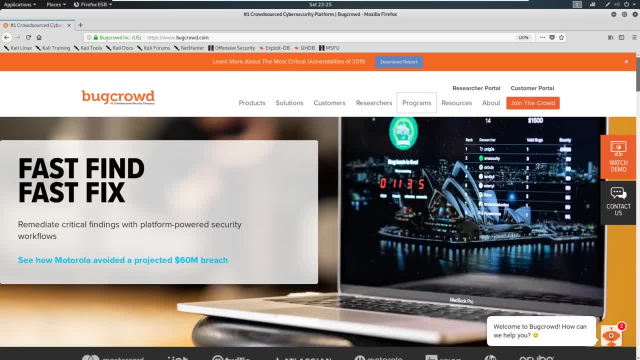 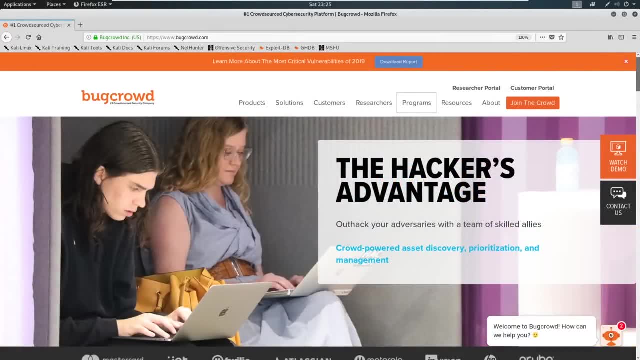 as they are part of this program. Now, the program we're going to be attacking is Tesla, So Tesla is part of Bug Crowd. Now please do note, please double check when you're watching this course, as some time may have passed. 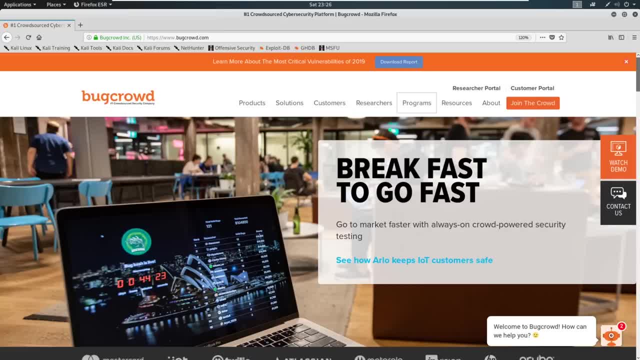 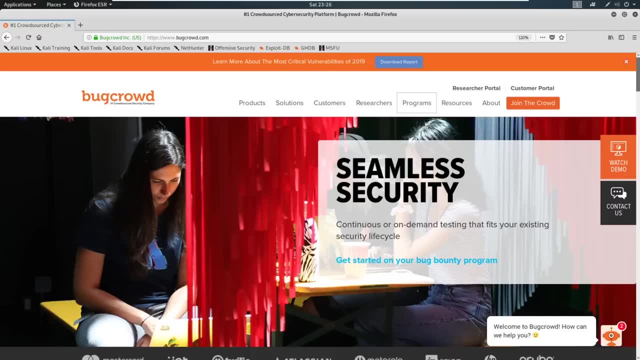 Tesla might no longer be part of this bug bounty program, So it's very critical to make sure that you are still within scope before you attack. If, for some reason, Tesla is no longer in scope, just go ahead and pick a new client and do information gathering on them. 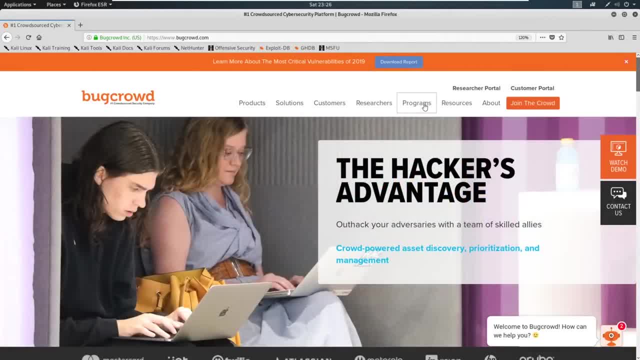 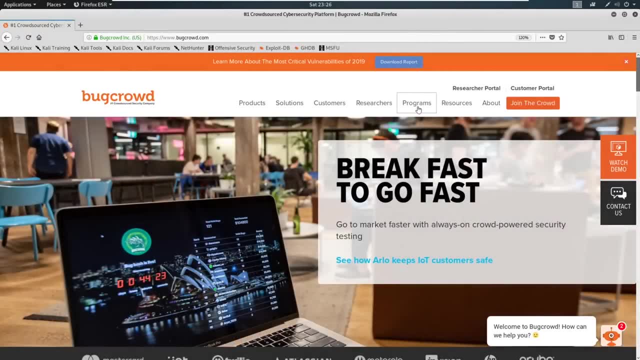 You don't have to pick Tesla when we're doing this. You can just do it to follow along with me. but you're also welcome to pick any program you want. So if you go to bugcrowdcom and we go to programs, 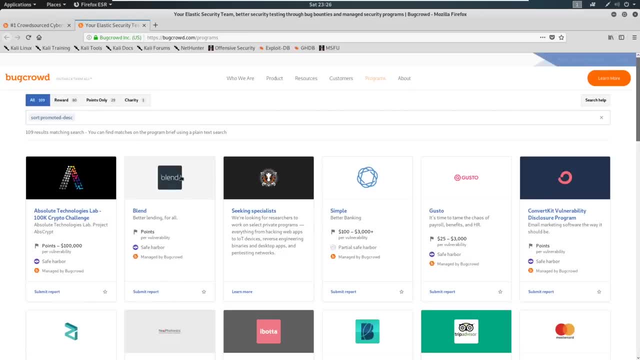 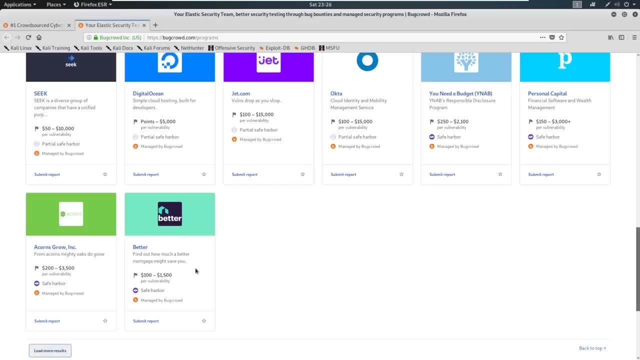 I will show you where Tesla exists. Now you can see here that they have all different types of programs in here, And if I were to scroll down and continuously, I could find more and more and more. There are hundreds of programs involved, all kinds of names: DigitalOcean, Okta. 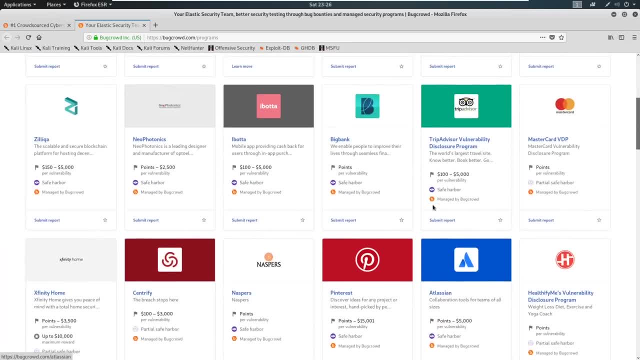 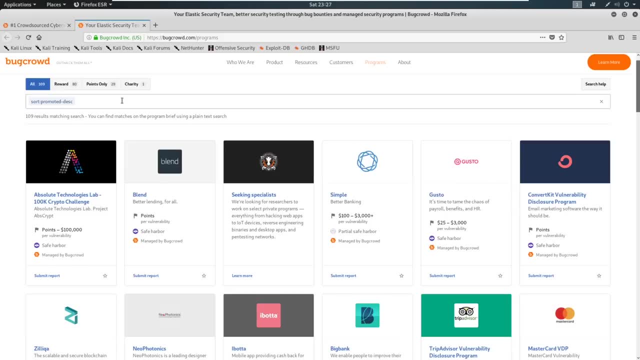 really big names: Pinterest, Altassian- Anything that you can imagine- probably has a bug program. if it's reputable, okay, Any of the big names most likely have a bug program, especially if they're reputable. So here you could see what's based on reward. 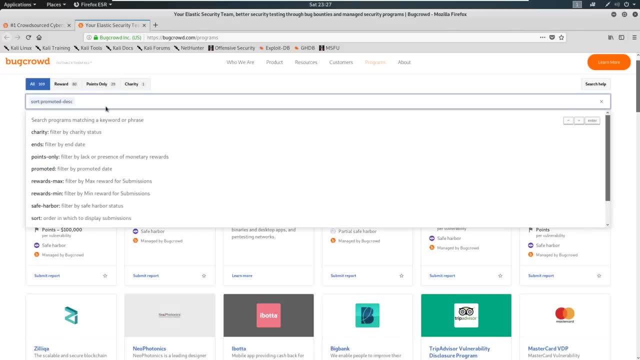 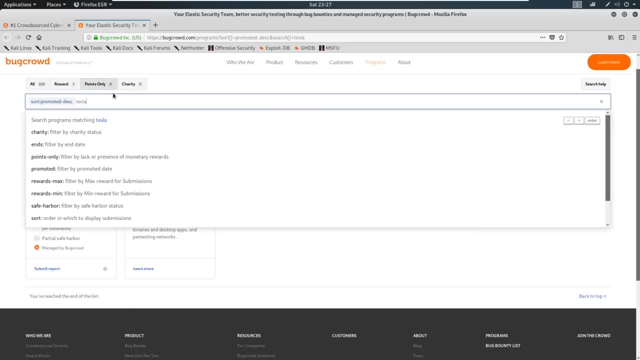 what's based on charity and what's based on points only. That's how the bug bounties are rewarded. Some of them are not all cash, Some of them are just for points and for kudos, And the other ones are for charity. 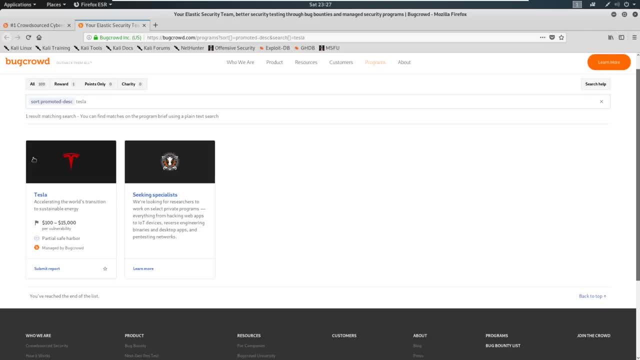 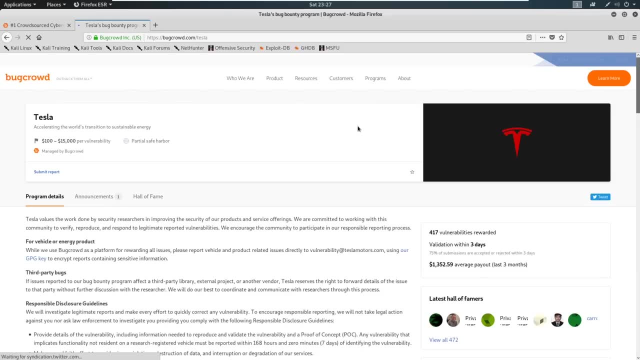 I'm gonna go ahead and just search Tesla, And when I do that, you could see here that Tesla comes up Now. this is your first lesson into rules of engagement, And we're gonna talk about rules of engagement later, but it's super important to read the program details. 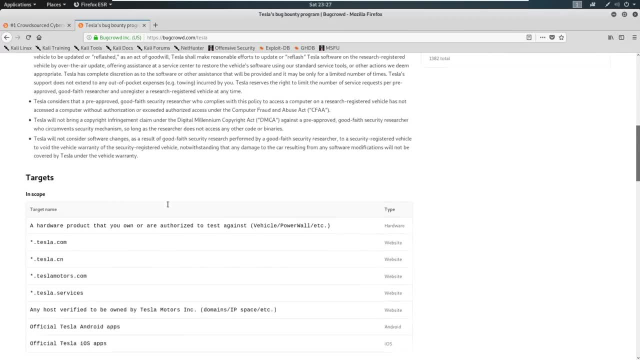 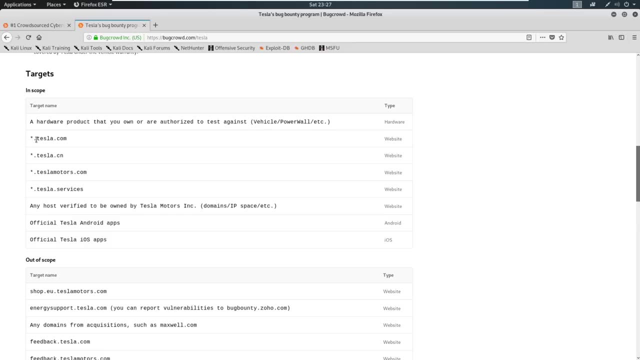 that you see here, And what we really need to do is we need to scroll through and make sure that we stay in scope when we're doing this. So we have a while. We have a wildcard here, So this means that any subdomain inside of teslacom. 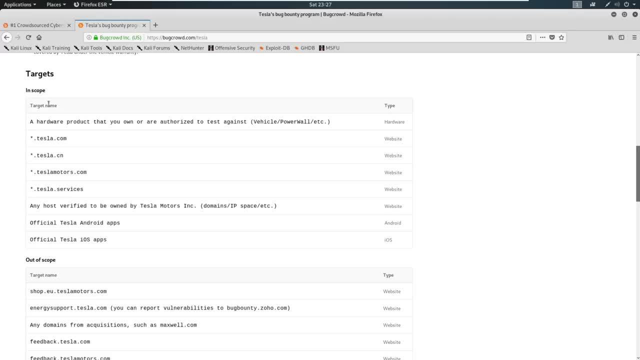 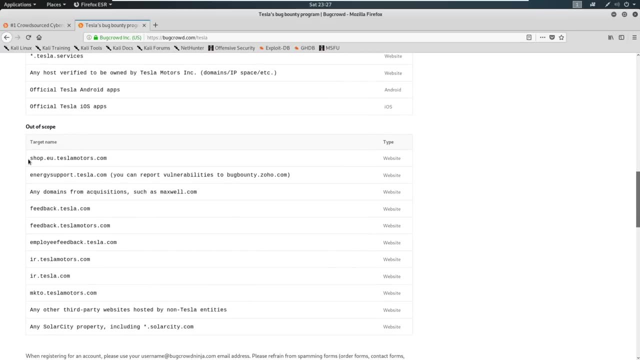 is fair game: teslacn, teslamotors, et cetera. What is more important is that we stay within this, out of scope, So we don't want to attack shopeuteslamotorscom or energiesupportteslacom. 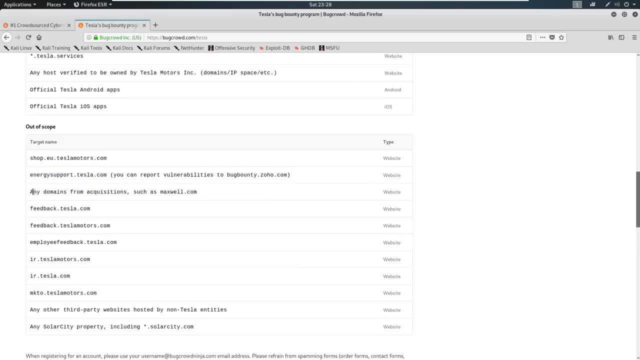 It says you can report vulnerabilities to bug bounty for this one, any domains from acquisitions such as Maxwell. So we have to stay within Tesla And there's a few more sites. We're not gonna worry too much about that When we get into the web app portion of the course. 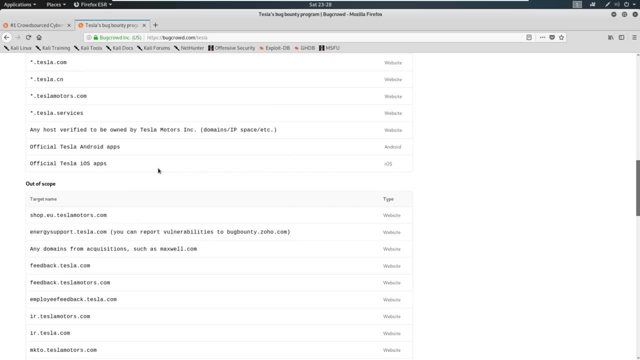 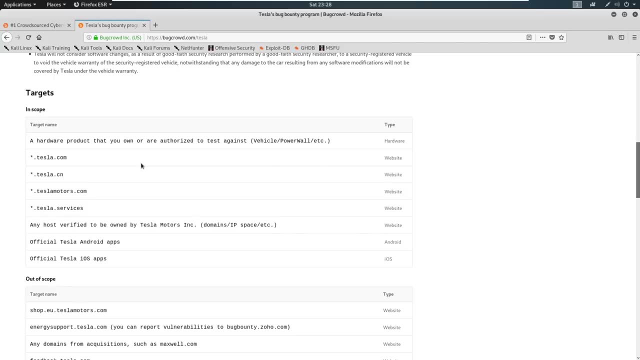 we're gonna talk about way more detail on enumerating web applications and go into that. So for now, what we're gonna do is we're just gonna focus on information gathering. What kind of information can we gather from this client? So again, I'm setting my target to Tesla. 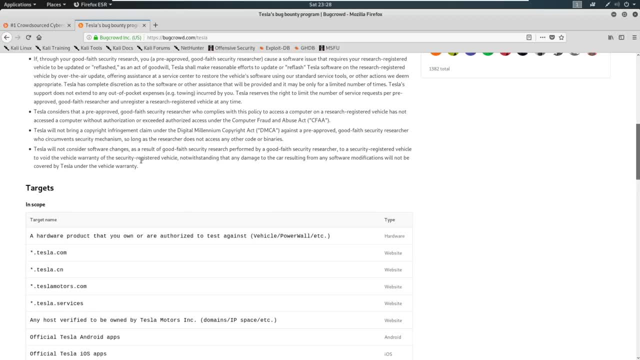 If you pick another Tesla or another client, just make sure you stay in scope of that client. So from here we're gonna move on to our first client, Tesla. So we're gonna go back to our first video and get our information gathering started. 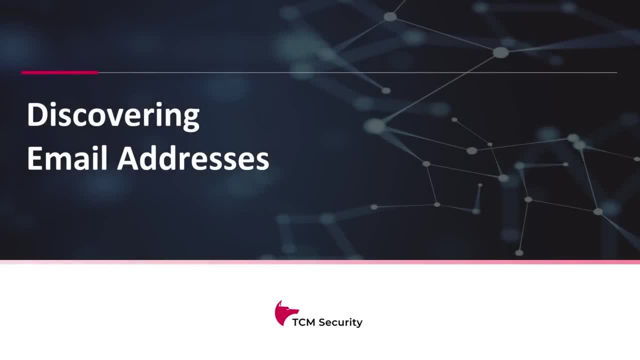 Welcome to the email OSINT section. We're going to talk about discovering email addresses, And this is something that I do on a weekly basis, So I'm gonna show you the most common tools that I use to actually look up email addresses and try to find people. 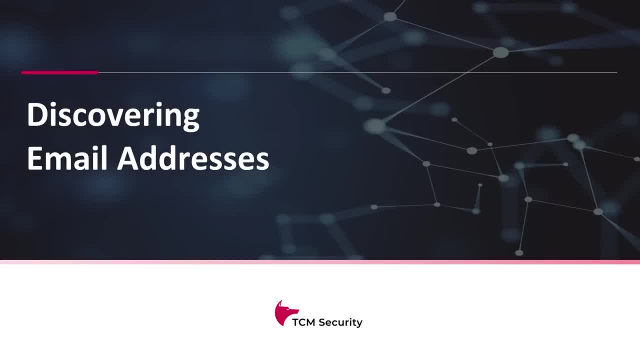 What you can do to kind of verify email addresses. So I'll show you some of my favorite tools and concepts. And this is something that I do because not only for OSINT and doing it for investigative type work, but think about sales If I'm trying to find a lead. 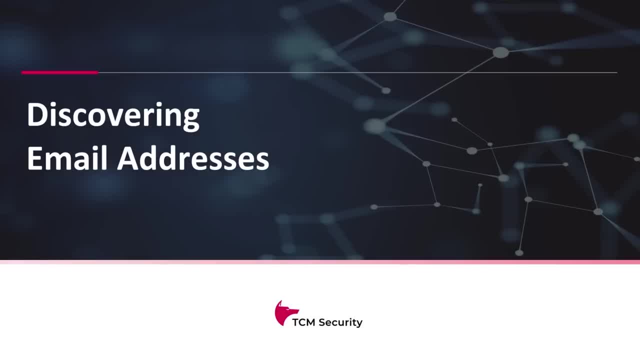 or I'm trying to find multiple leads within an organization. I have to figure out where the emails are, who the people I'm trying to email are, So maybe I'll Google them and say who is the CISO- Okay, CISO or chief information security officer for this company. 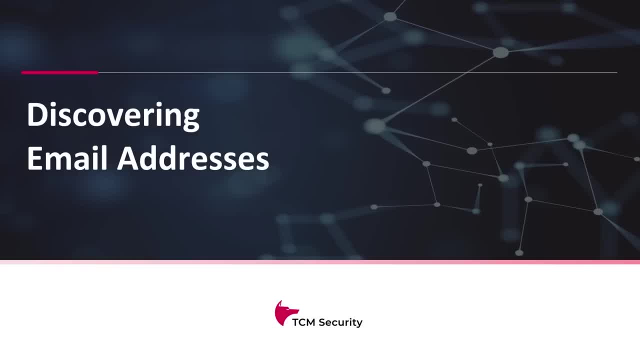 And I might find that it's Bob Jones. And we go look up Bob Jones and we say, okay, well, how do I get Bob Jones' contact information? Can I find it via Google, Maybe? maybe it's out there in the public. 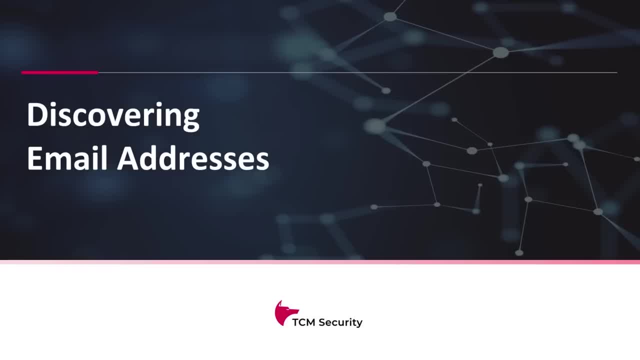 but maybe we have to dig a little deeper, Maybe we have to kind of do some guesstimation and see if we can figure it out. So that's what we're gonna do today is look at the email addresses, formats and try to determine. 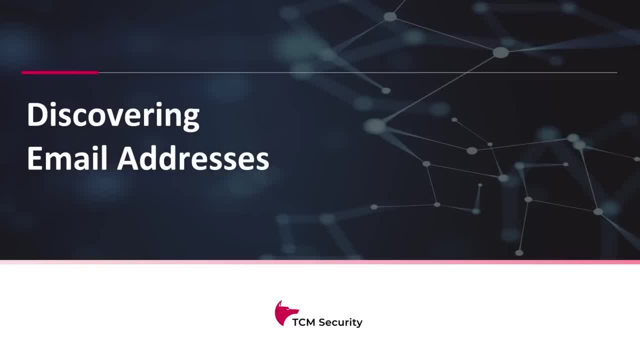 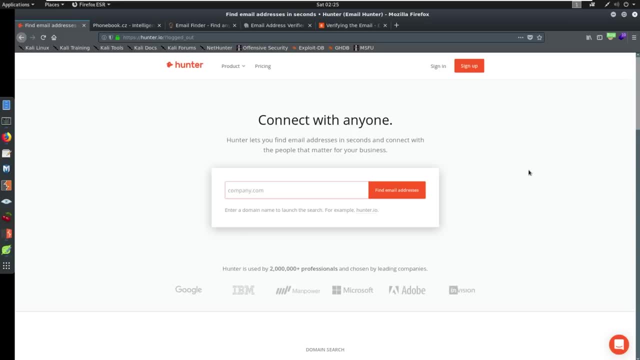 if we can find some emails. So let's go ahead and move over to the Kali Linux machine that I've got, And the first website is one of my favorites. So hunterio. you just come to hunterio, you get like 50 or a hundred free searches a month. 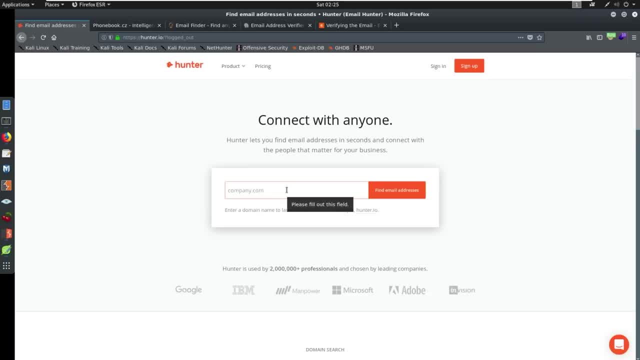 I don't remember what it is. It's a fair amount. You can come here and basically just type in a company name. So, like say, I wanna type in TCM security, TCM dash sec, and you can see TCM security here. 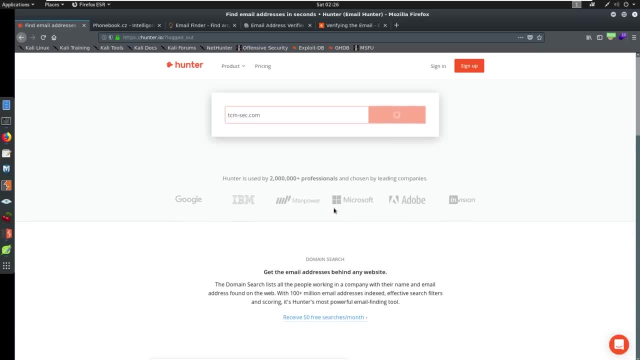 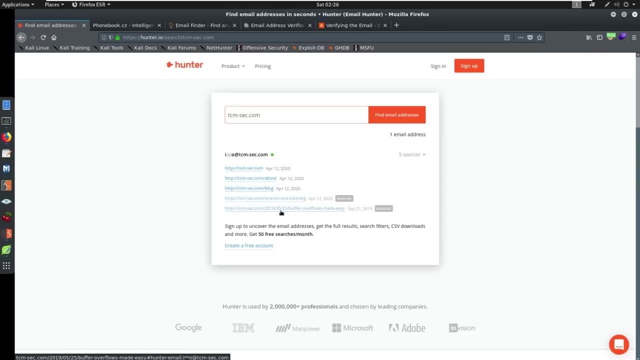 We get one result on the email address, So we'll click it and see what happens here And it looks like we have like an info at tcm-seccom. It tells us: hey, there's five sources that identify this, So we see tcm-seccom. there's an about blogs. 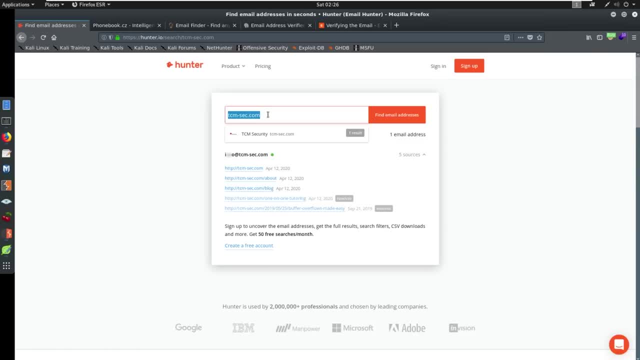 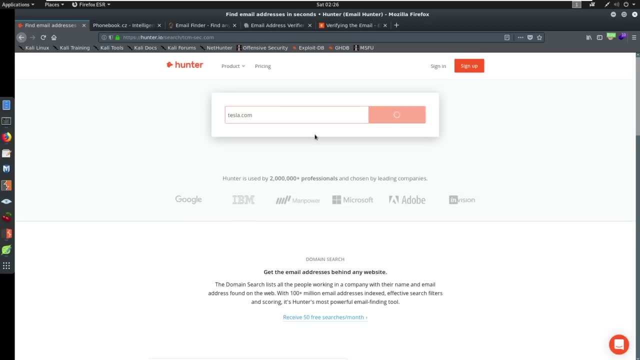 This is where they're finding it. okay. A better example maybe something that has more users, like Tesla? Tesla has 468 users. If we come in here and we look well, we can see that they have a pattern identified here. 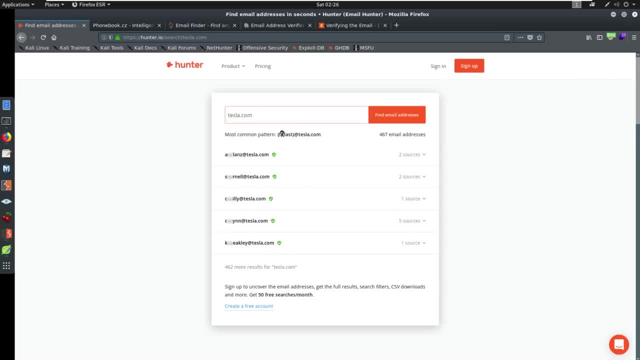 So their pattern they're identifying is first initial last name at teslacom, And that's really what we wanna see. And then we can gather email addresses here if we want, But say like we knew Bob Jones. again going back to that example, Bob Jones, 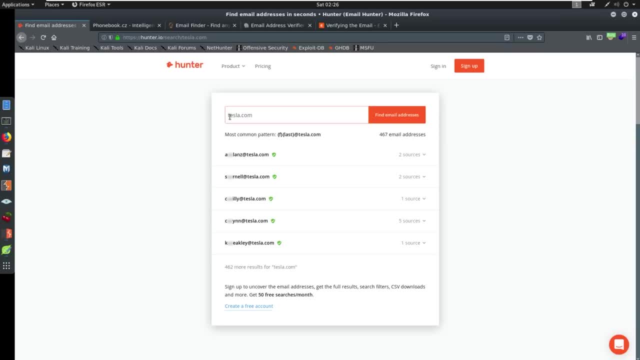 So maybe Bob Jones works at Tesla. Maybe his email would be bjones at teslacom. So it's something to think about. Now we can sign up and get actual information here. You should be able to sign up with a Gmail account. 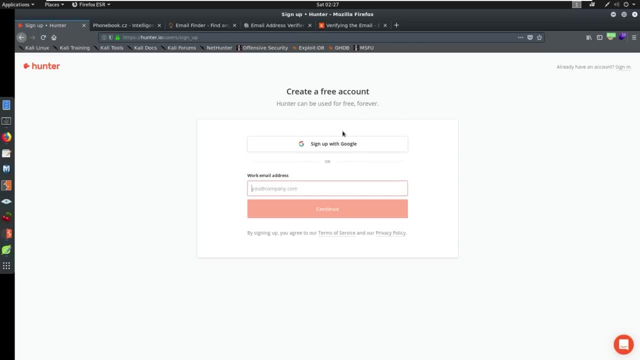 Sometimes this does not work, depending on the country that you are in, So be cognizant. you might have to use a different email address, but I just tried signing up with a Gmail account that I have on here and it worked just fine. 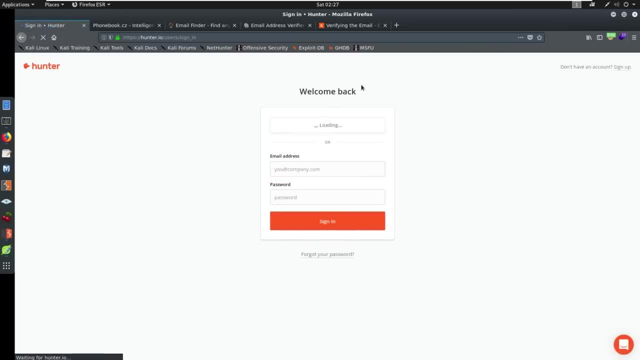 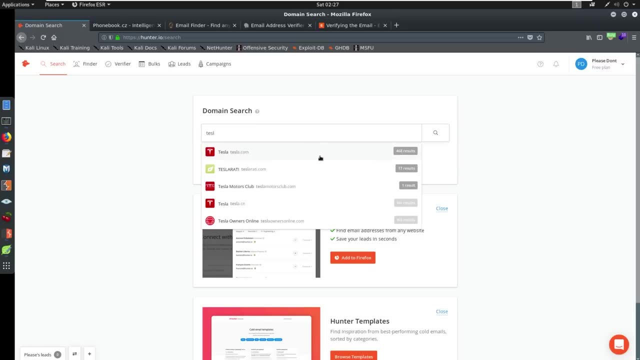 So I'm gonna go ahead and try to log in. I'm gonna sign in with Google with what's already here And just now I'm logged in, So we can go back now and try searching Tesla again And you'll see that the results actually come back. 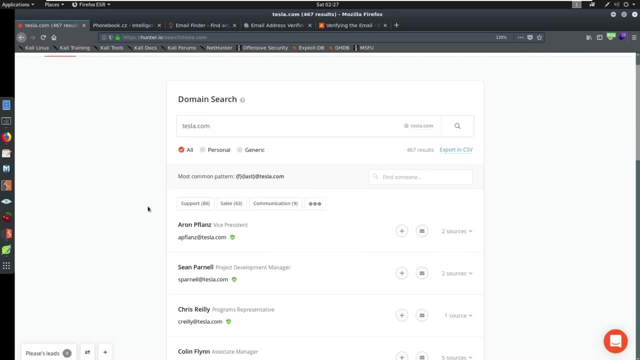 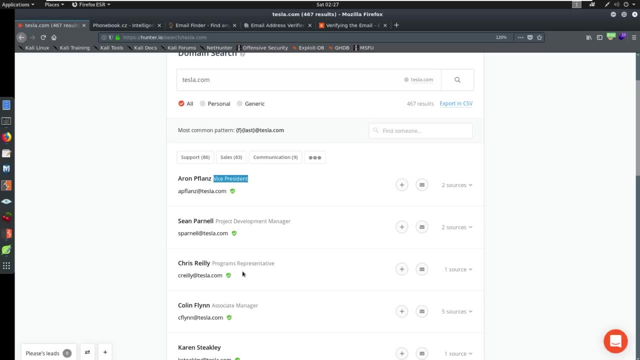 So we get information here. now We get- let me make this a little bit bigger- We get information as to: okay, here's the vice president. This is the vice president's email address: Project development manager. Maybe you want to talk to somebody in human resources. 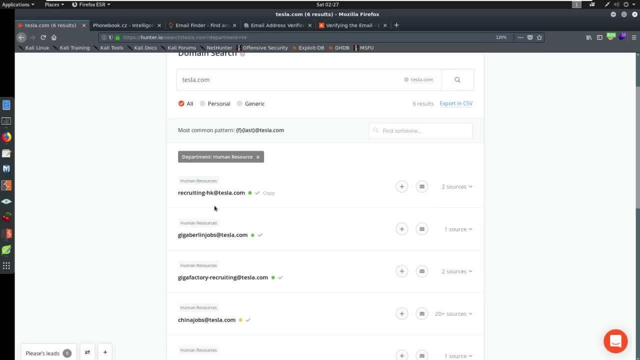 So you can click here and go to human resources, And then here are the different human resources emails that are here. So, and then the sources that they found On these email addresses. So this isn't a particular person in HR, but it's still human resources email addresses. 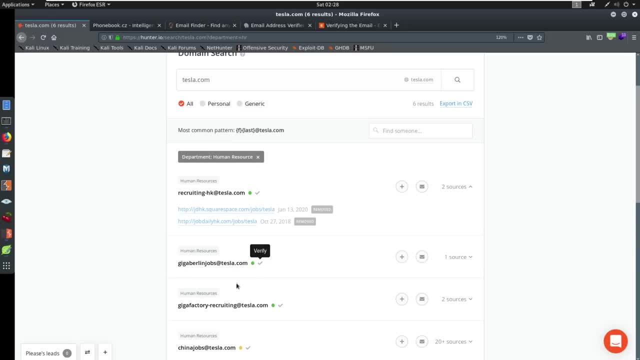 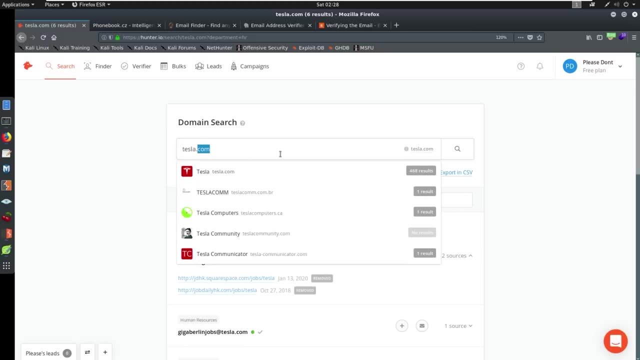 So this looks like it's probably for Hong Kong. This is for Berlin. This is gigafactory, So they have different email addresses based on where they are. Now, if you looked up TCM security here, you're really not going to find much on us, because 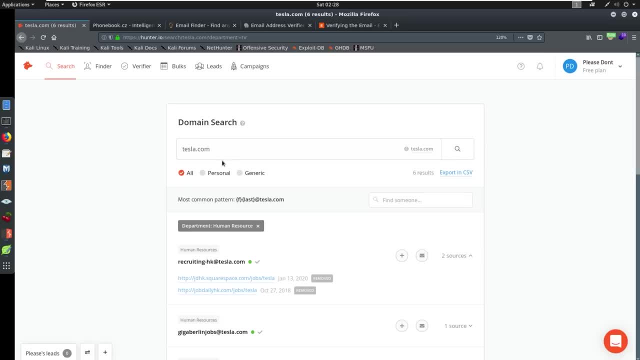 we don't have a ton of email addresses out there, but I think that we can find more in other ways now, So we only get so many users here. We'll just keep thinking about this as we move forward. So a hundredio great, great resource. 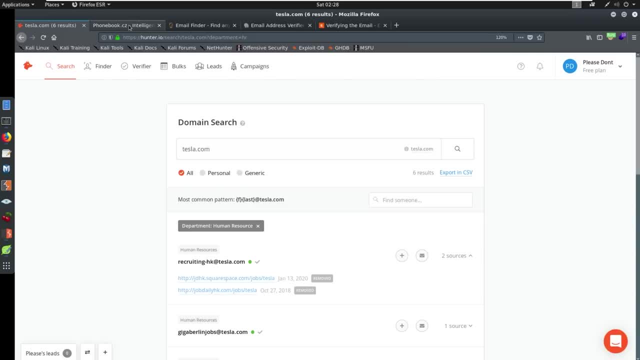 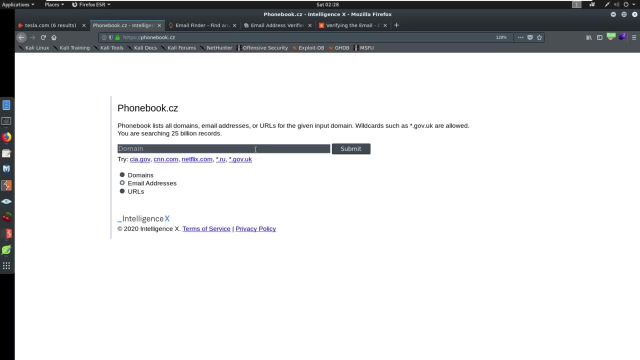 They have plugins If you want them. I think it's fantastic place to look. phonebookcz is the next resource I want to show you. This one is fantastic. Let's start with tcm-seccom and see. so we're going to tcm-seccom and we're going to search. 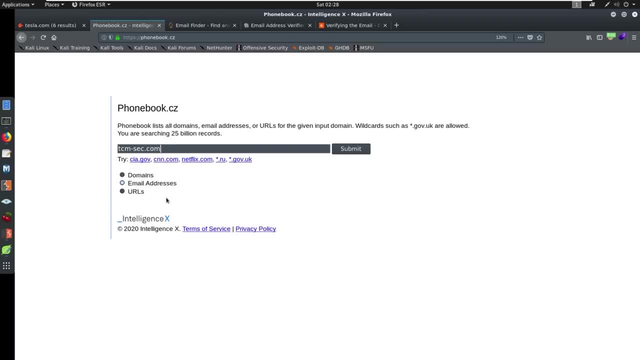 email addresses here, So they do domains and URLs as well, which I think is awesome. but let's just search for email address, See if anything comes back. No, no results. Okay, Let's try Tesla and see what comes back there. 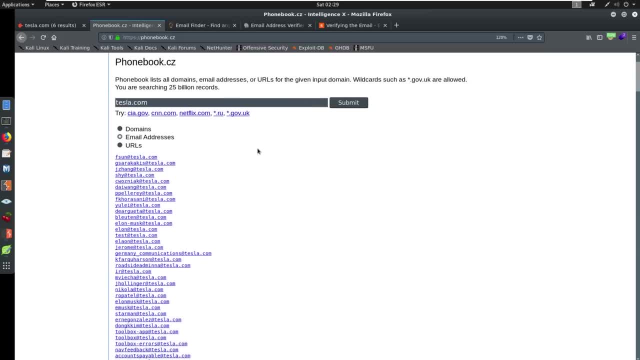 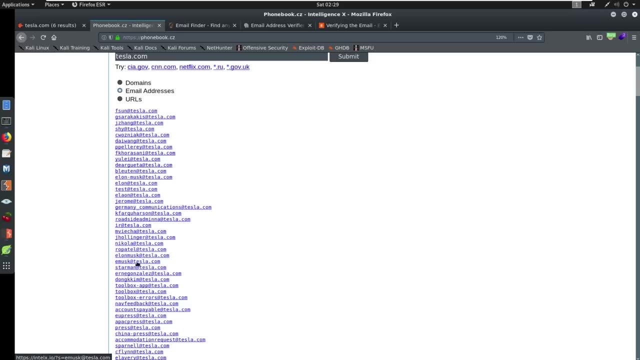 Okay, A lot more. So we get quite a few email addresses. We could see Elon Musk all over the place. We've got Elon Musk, Elon, we've got Elon Musk over here and we get a ton of emails. Look at this. 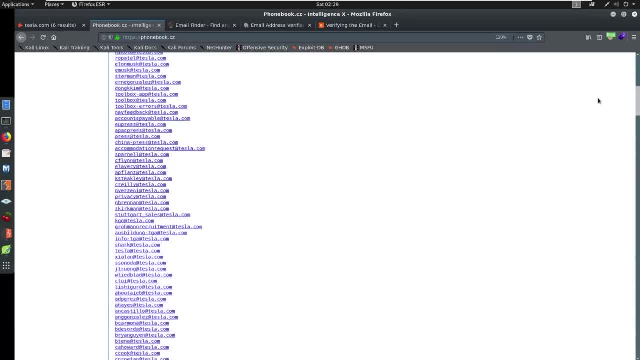 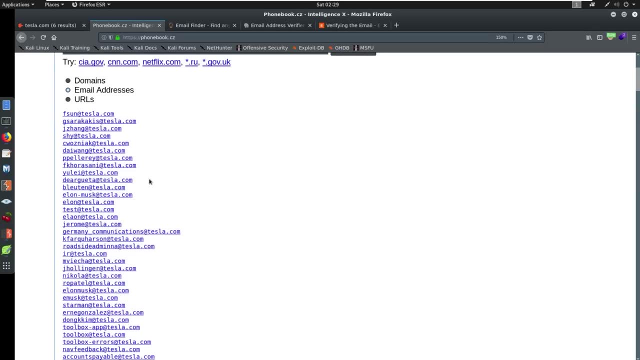 So what's nice about this is we can sit here and try to identify what the possible email addresses are. So again, first initial last name: looks like it's showing up quite a bit outside of, maybe like the Elon musks of the world. 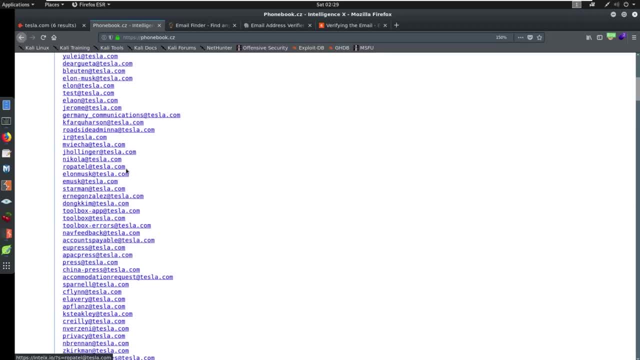 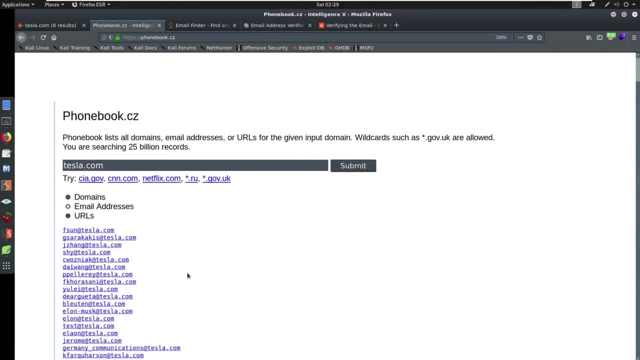 We're getting a bunch of mostly first, initial, last names in here, So I think that's pretty spot on with this. The other thing that we can do is we could utilize this list, Say we're we're trying to do something called credential stuffing, which we'll talk about. 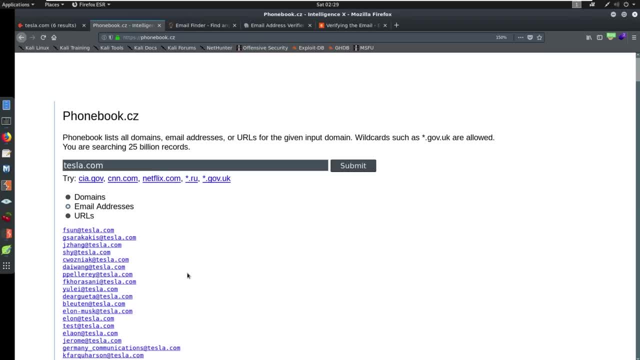 in the next section. actually, when we talk about breach credentials but say we're trying to gather a bunch of usernames and test, See, See if we can log in with those usernames anywhere, Or maybe password spraying- not so much the credential stuffing but password spraying- 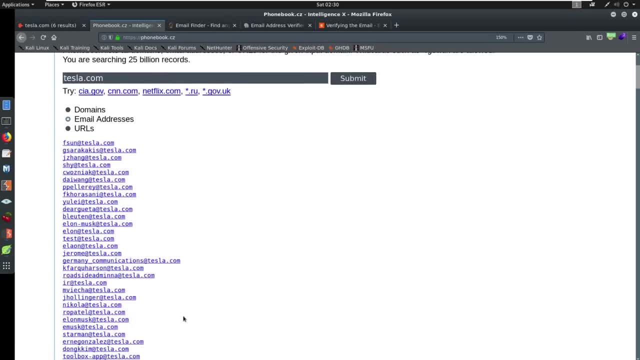 where we take all these usernames and we just throw it at a login form and say, Hey, summer 2020, exclamation point. you know, see if that logs into any of these accounts and you would be surprised that it happens quite a bit. 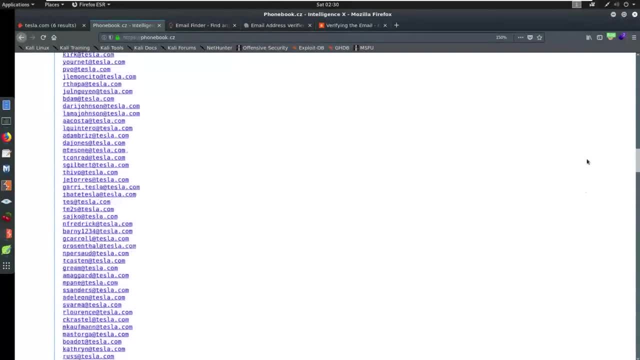 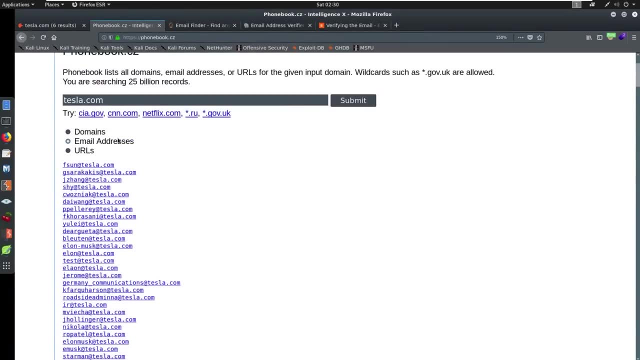 So you know these are. this is valuable information, Even if we don't know exactly. maybe we're not just hunting for one email, maybe we're hunting for an entire domain. This is a great way to get free entire domains with a quick copy and paste capability. 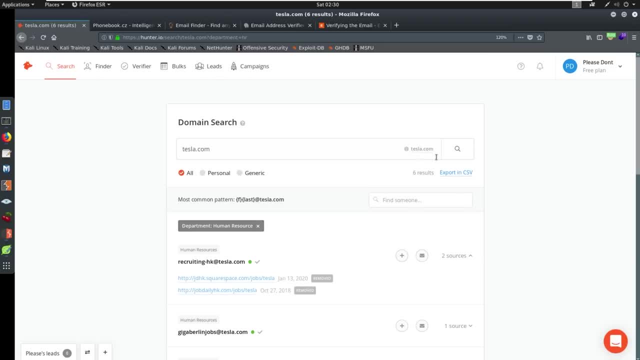 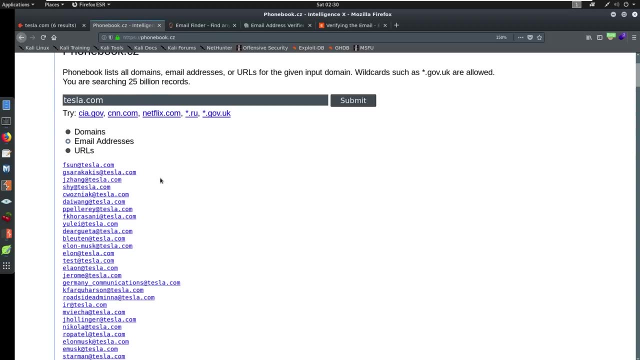 Like we have the Tesla here We can export the CSV from hunterio, but you only get so many results that you can export into a CSV. here You get a bunch. There's no guarantee These are all valid, but there's still. it's still information. 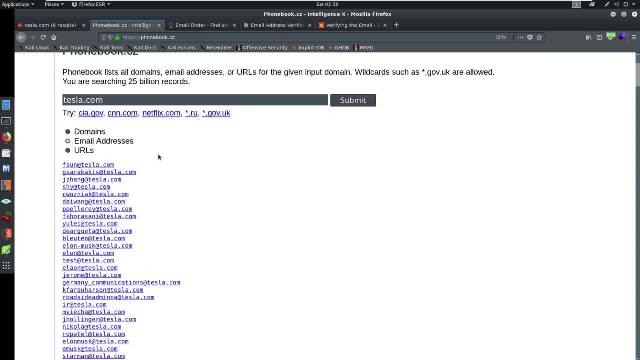 Information is what we want. This is all we're trying to gather is as much information as possible. So these are all potential email addresses For teslacom. I think it's a great, great resource. Now we could also use something like a voila no bear. 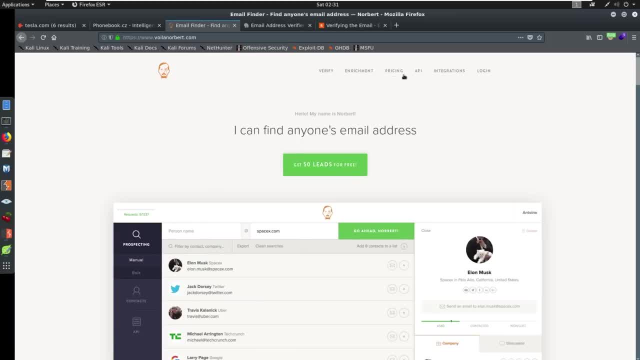 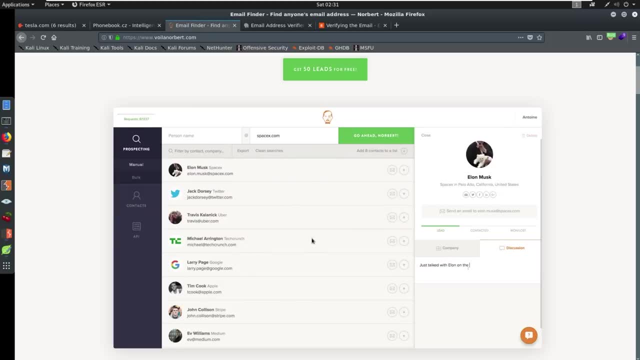 Now this one. you can get 50 more leads for free. I'm not going to show you. it's the same kind of deal as a hunterio. They're showing you how to utilize it here. Basically, you can just search for people and see to try to find their email addresses. 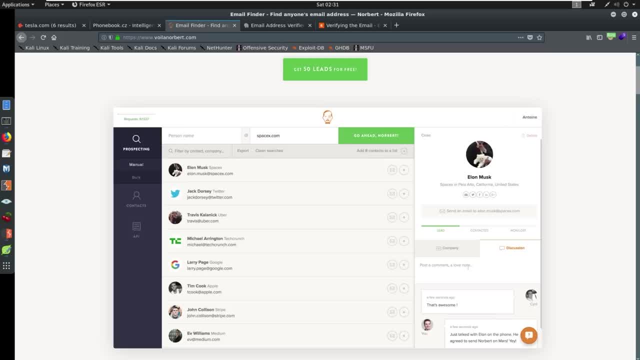 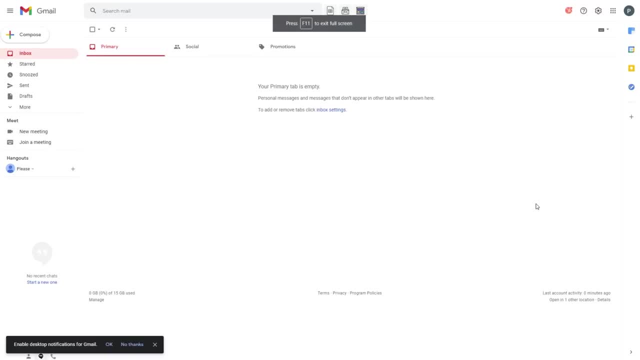 There is one I want to show you that I do use and I have quite a bit of success with, and that is called clear bit, and clear Bit has to be used in Chrome, So I'm going to bring up this here: Clear bit has to be used in Chrome so you can download the Chrome extension for clear. 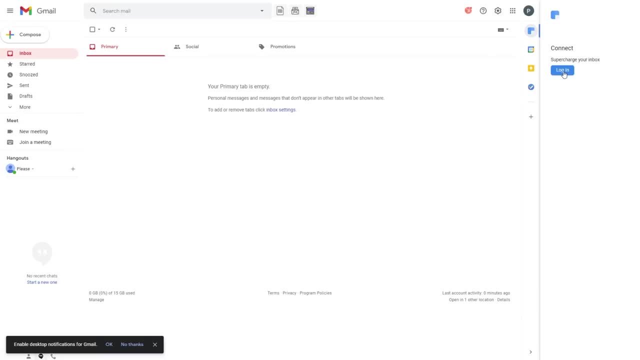 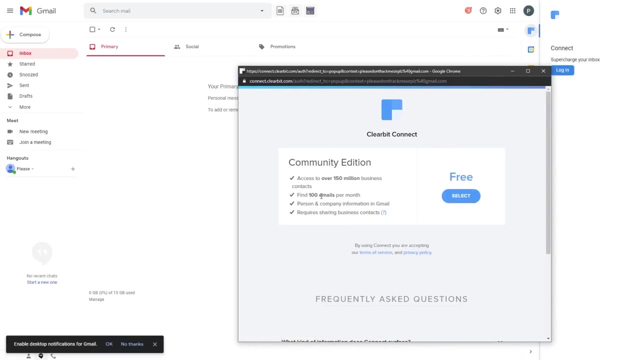 bit And all you have to do is go to Google, Let me log in really quick, And then I'm going to just select the free account. We get so many searches, a hundred emails a month, So basically you're going to search for clear bit connect and you would just say, Hey, clear. 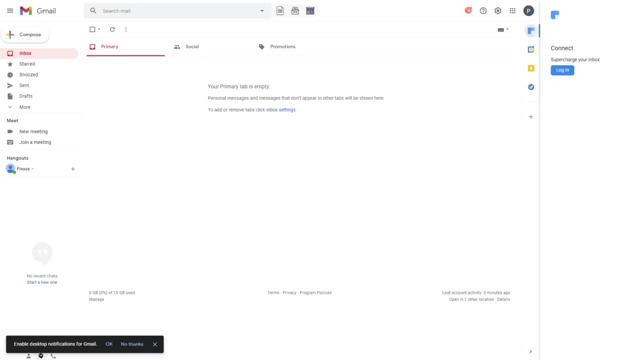 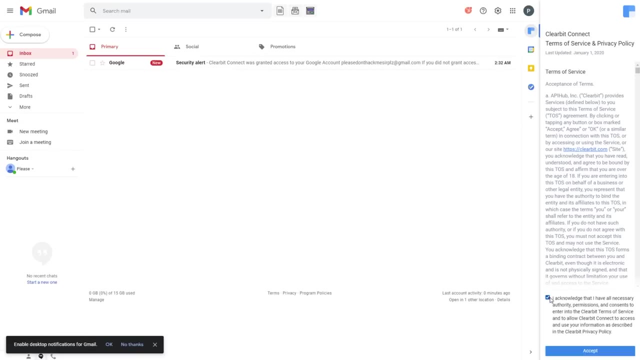 bit connect. I'll put a link down below, by the way, But clear bit connect is awesome, You'll. you'll see why here in a second, once I authorize this. okay, we're going to come down here acknowledge, probably give out, our first born. 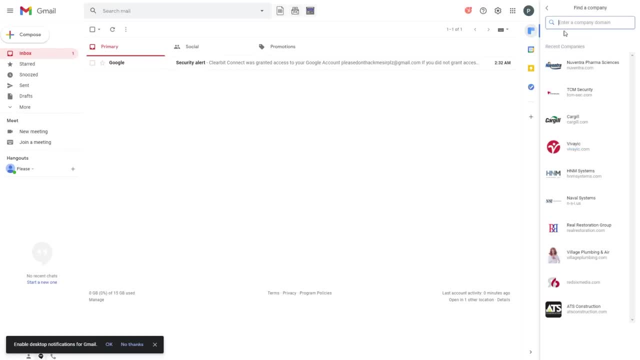 And then now we're going to say, Hey, I want to find emails And here's all different kinds of things that we can sit here and search for. You can see TCM securities in here. These are some searches that I've done. 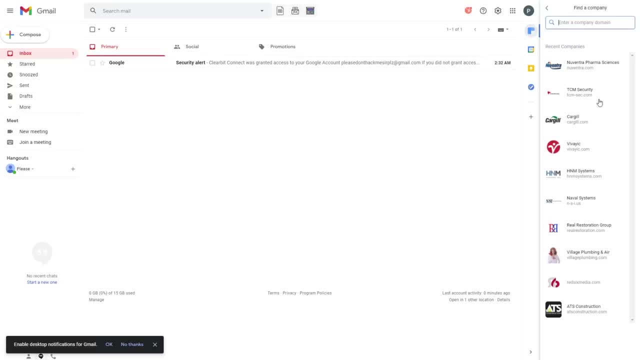 These aren't any clients of mine. These are just searches that I've done in the past, maybe looking for information or looking for possible leads or anything. So, Uh, if I come in here and I say, Hey, I want to look for TCM security, 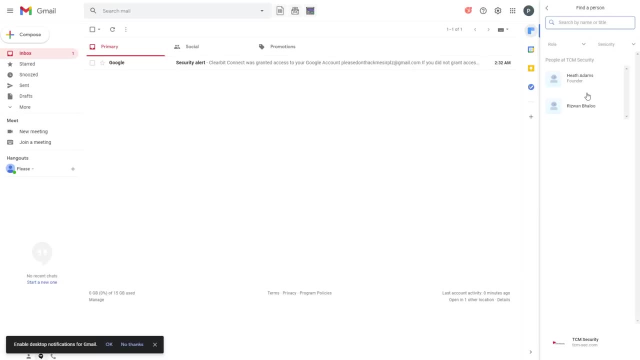 You could type that in. I'm going to just click on TCM security and look what it discovered that the others didn't. It discovered me, Okay, And if I click on me, look, it says heat that TCM dash seccom. where, where did that come? 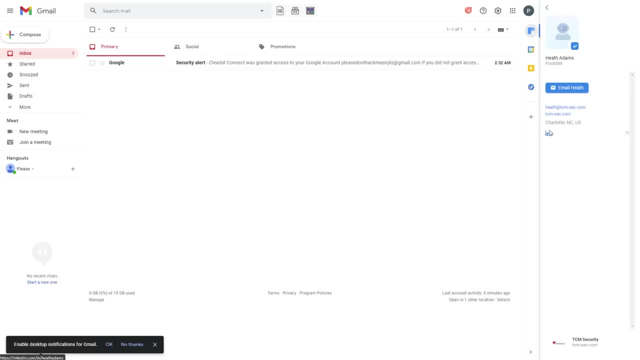 from. And then look, it has my LinkedIn right here as well. That's amazing. That's awesome. And it says: here you can email heat, just click this button. And then it's also got Rizwan Rizwan's on my sales team. 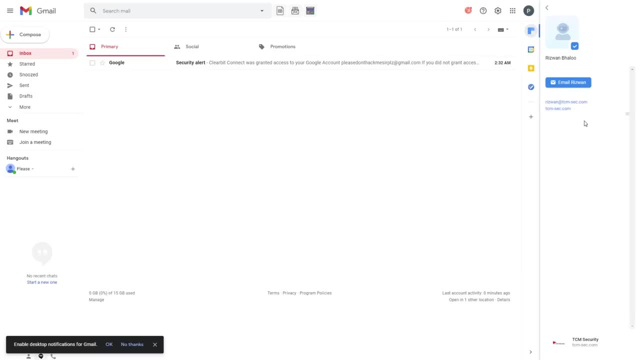 Look, it's got Rizwan at TCM dash seccom. What does that tell you? That tells you that we're using a first name basis for our email addresses. It's awesome. Now let's come in here and maybe we want to look at Tesla. 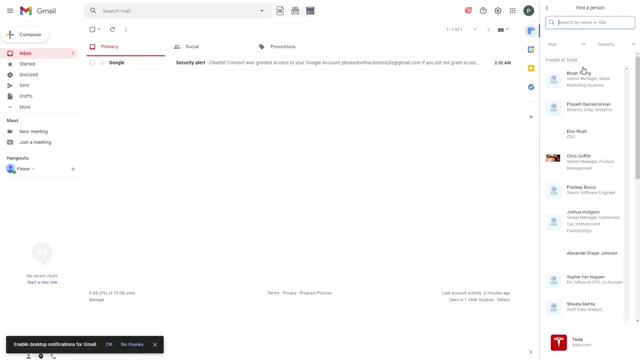 Maybe let's try Tesla one more time. Maybe we're looking for the CISO of Tesla. Tesla has a CISO. You can come in here and look like Elon Musk is right here, obviously CEO. but you could come in here and maybe go by role and they have different roles in here. 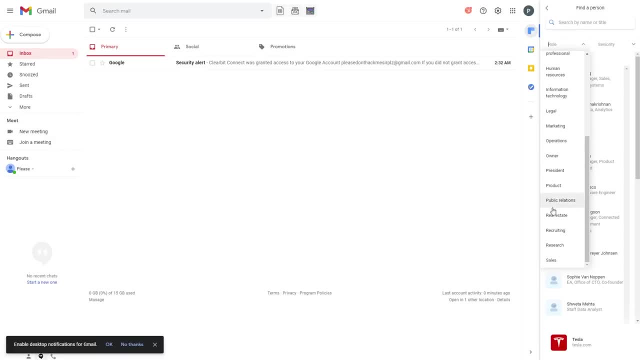 CEO. Let's see if we can find any sort of CISO. I don't see one, but I do see information technology. So maybe we can find somebody in the information technology department or IT department, And then here we go. We've got quite a few IT people. 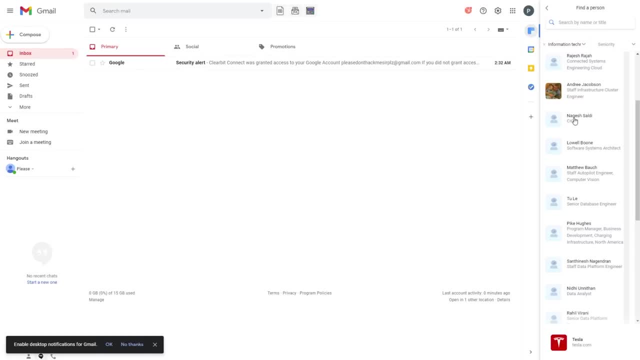 Here's a CIO. This could be somebody of interest that we might want to reach out to, And we could just scroll through this list and find people So say we want to reach out to the CIO. just click on this. We get first initial, last name, just like we thought we would. 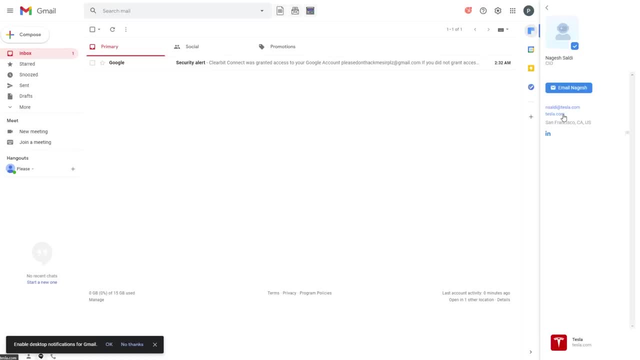 We get this person's LinkedIn, We get their LinkedIn page, We get their location website. This is awesome, Awesome, Awesome. So I typically will start with a Google search. If I'm trying to hunt something down, I will start with a Google search. 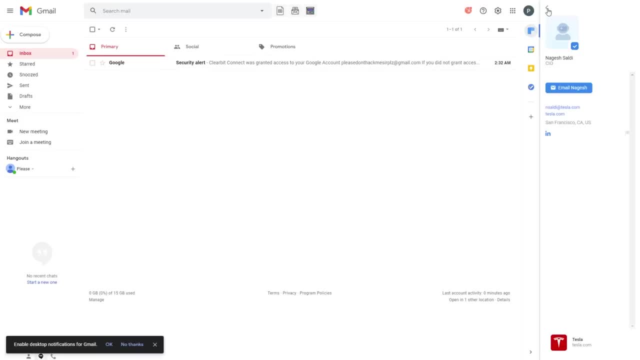 I will say who is in this role at this company. If I'm looking for a specific person at a company, then I will go to phonebookcz or hunterio, try to identify the formatting of the email and then try to find that person. 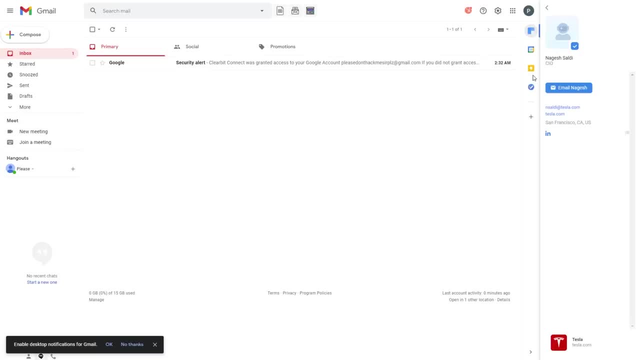 or guesstimate that Once we get to that point. I try not to burn through these clear bits unless I need to, but clear bit is very good at identifying this. Once we get to that point, we can take this email, say like this email or we'll even. 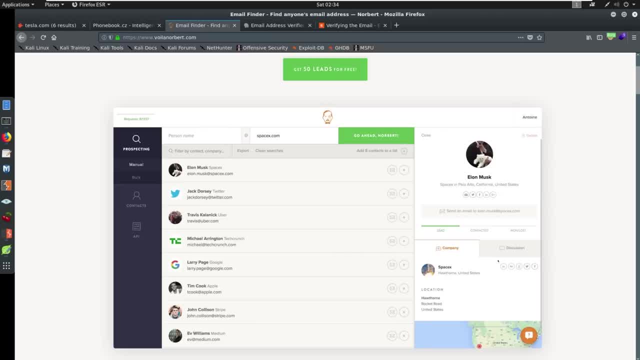 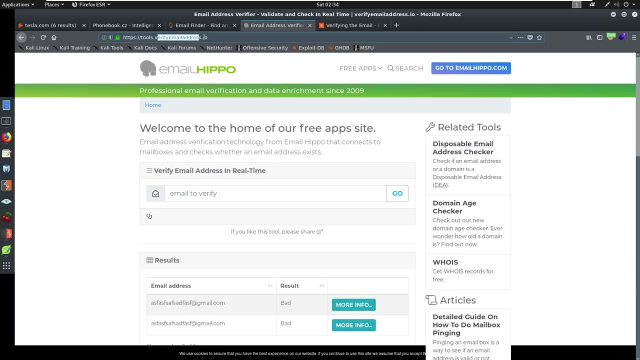 try a different email. I'll show you a couple, but we could take this and we can go try to verify this. So there is a website called email hippo. You can go to toolsverifyemailaddressio and all you have to do is type in an email. 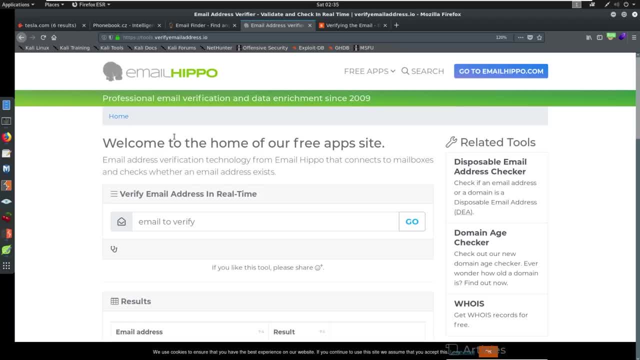 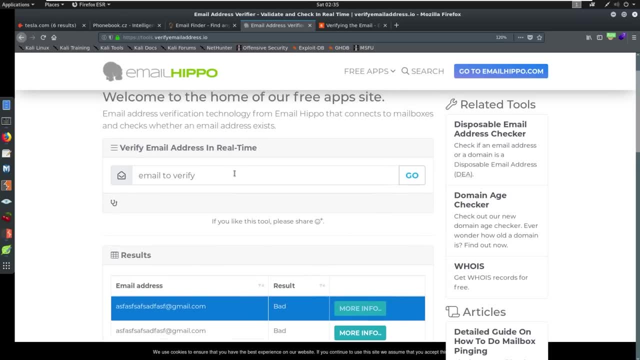 address here. Sometimes you can get false positives If they're good or bad. here I typed in this email address a couple of times and just got a bad result. This is an email address that does not exist. Now let's try an email address that we saw info at: tcm-seccom. 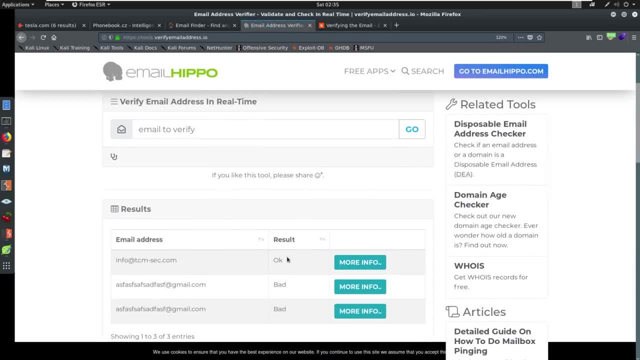 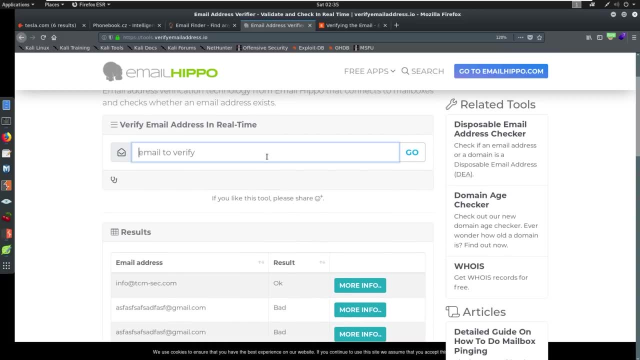 See if it works. Result is okay. So it says, yeah, this email address works, So we're verifying that this is up. So say that you get somebody and you see that they have a potential email address. You can come here and try to verify it first. 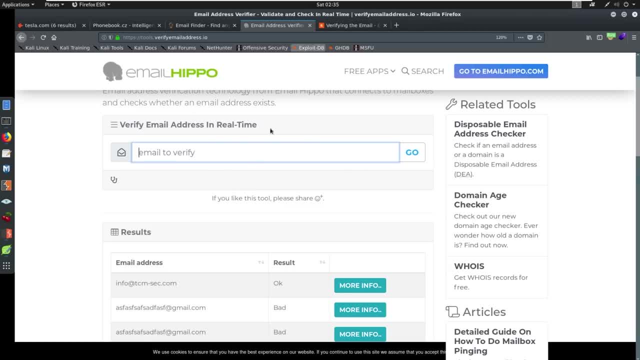 And see if it works before you go fire off an email or don't. you don't even have to fire off an email, You don't have to do anything or interact. So this is the benefit, Like if you're from a sales perspective and you're doing OSINT here, the this is the 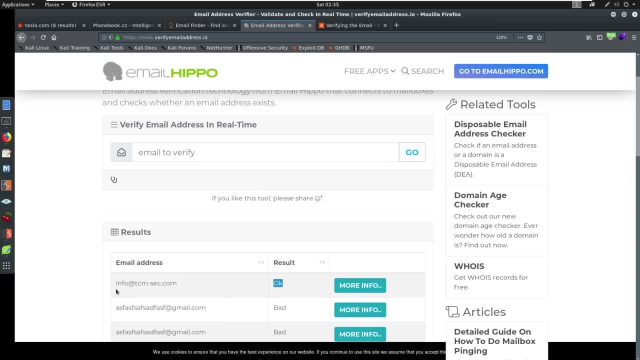 benefit of not having to email, get waste your time, get it rejected. You can come in here and just validate If you're doing an investigation. you don't want to interact with the person or company that you're investigating. You want to come in here and just verify, without any interaction. 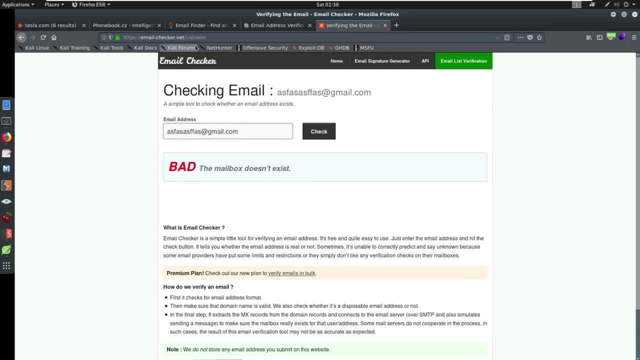 This is the way to do it. Same thing with this website here. Email checkernet slash- validate. email-checkernet slash- validate- say: Hey, checking the email. I put the same email address here. You could see it says bad. We could try again with info at TCM dash seccom and see if that works. 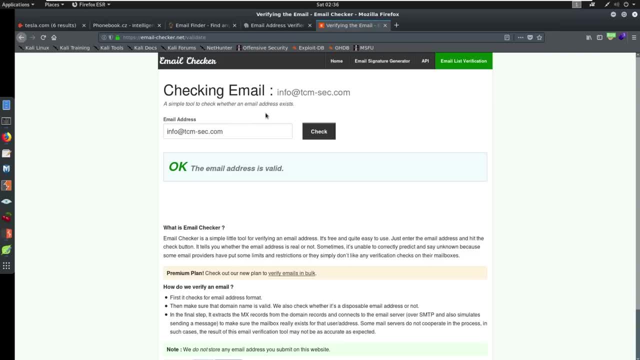 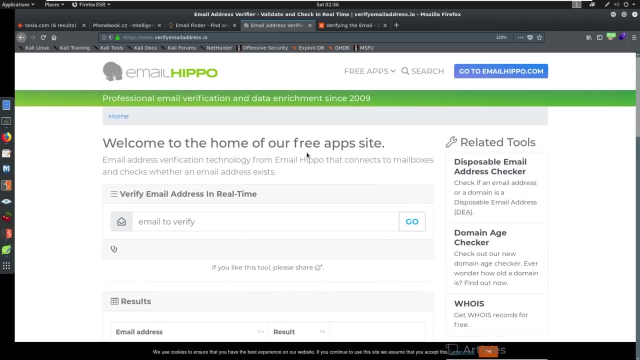 And it says: okay, So again, this is doing a great job. There are possibilities of false positives. There are so many searches that you can do per month on these. I do believe they have APIs, which is nice If you want to automate this or script this out, but I think this is. this is fantastic. 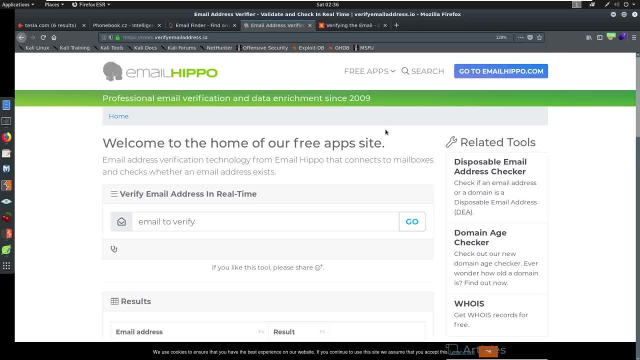 This is great stuff. Now there are plenty of other ways to verify email addresses. in the next section We'll talk about that even more as we talk about breach data, because if somebody shows up in a data breach, guess what That email address has been used in the past. 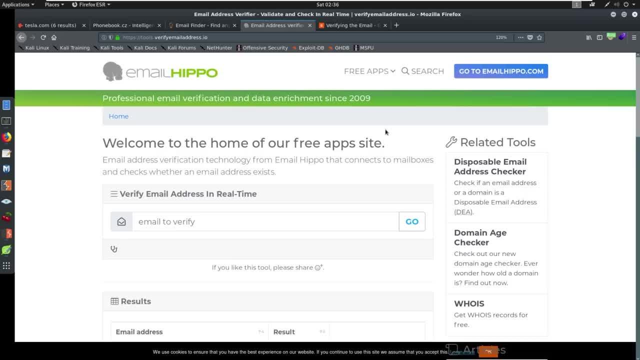 If you look at something like a have I been pwned, which we'll talk about in the next section, and they show up- guess what? That person's email address has existed. So we're trying to verify, if an email address exists, who that address might belong to. 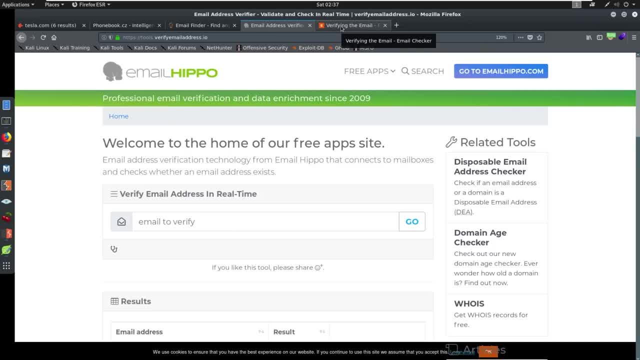 et cetera. Now this is more- has been from a business perspective. Some of this hunting down of emails may be more difficult to do if you're trying to find a specific individual. that's where breach data comes into play in a lot of this research. 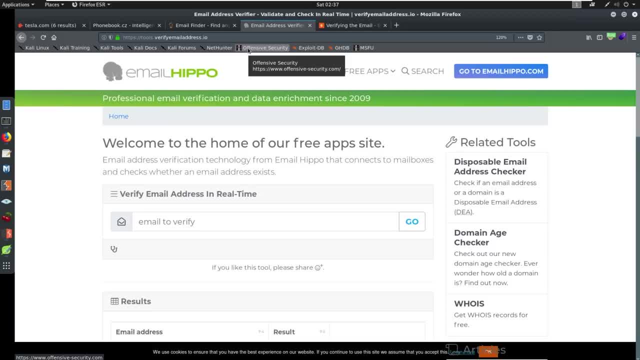 And what I'm going to show you in the next section. we'll try to hunt down individuals with maybe having loose pieces of information like a name or a username or something along those lines. Breach Data can come in handy. It can come in handy very well. 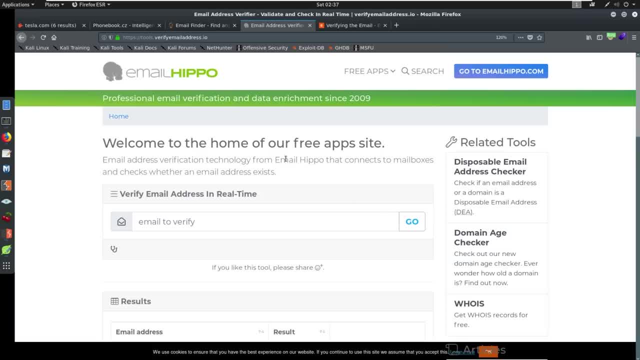 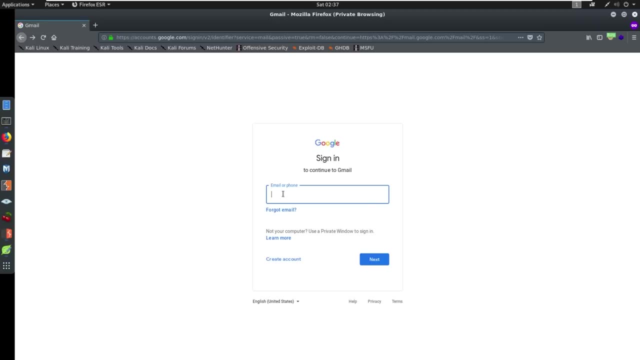 So this is kind of scratching the surface. Now there's one last thing I want to show you, One last little tip and trick: Do not underestimate forgot passwords. Do not underestimate them. Let's go to Google, for example. Right now I am logging in under an account that is: please don't hack me, sir, please. 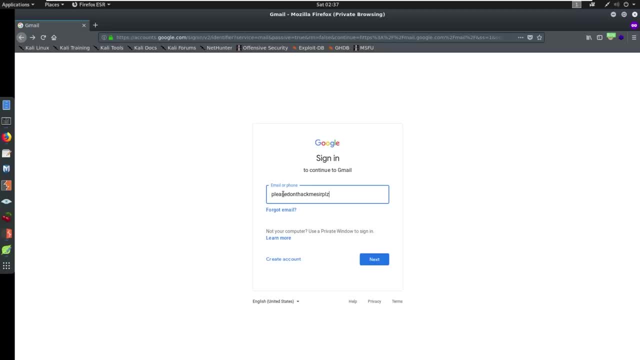 So it's: please don't hack me, sir PLZ. I do believe I'm going to go ahead and try hitting next on that. Okay, So It said: Hey, welcome, Hey, what does this mean? This means that we have a valid account here. 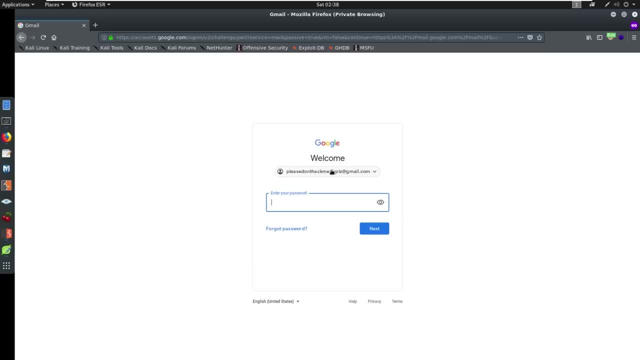 That's great. This is validating that this Gmail account exists. Here's something else: We can use this to tie to potentially another account or help validate. Say, we know that this email belongs to somebody that's harassing somebody else. We don't know who this person is. 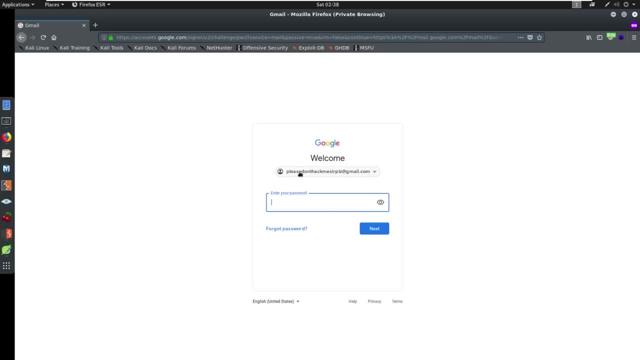 They're using this spoofed email, but maybe we have a hunch, or maybe we don't. Maybe we just want to try to get more data. You can come to forgot passwords. You can come to forgot password And it's going to say what's the last password you remember using. 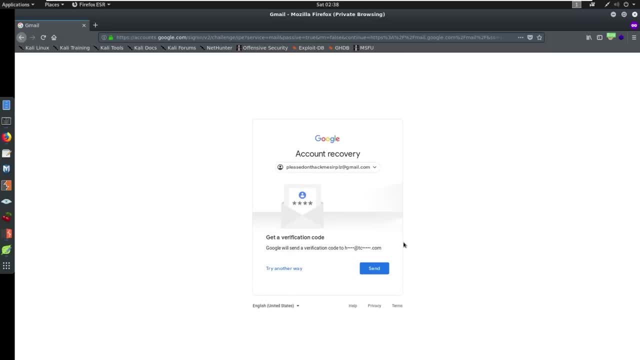 I don't know, Let's try another way. You come down here and it says: Hey, let me make this bigger. Google will send a verification code to H and it says: look, it shows you the rest of the, the digits here. 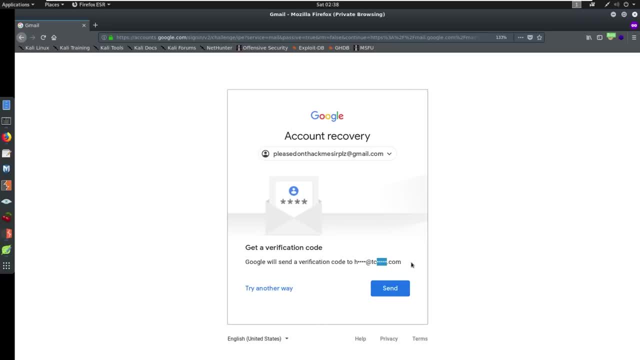 And then at TC: da da, da da here. that would give you a pretty good indication, If you're tracking who your subject is, that this email could tie to somebody else like this: is heat that TCM dash seccom? Okay. 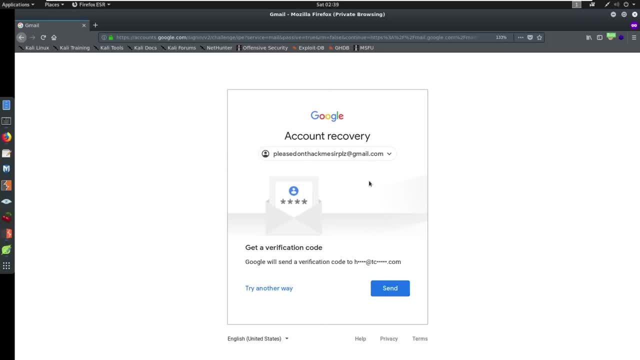 So this email belongs to me, This is tying back to me. Now you have another point here. So if you knew about this email address and now you have the link, the connection to guarantee that this person- this is evidence right here- Say you were doing something which we'll learn about again in the next section, where you're 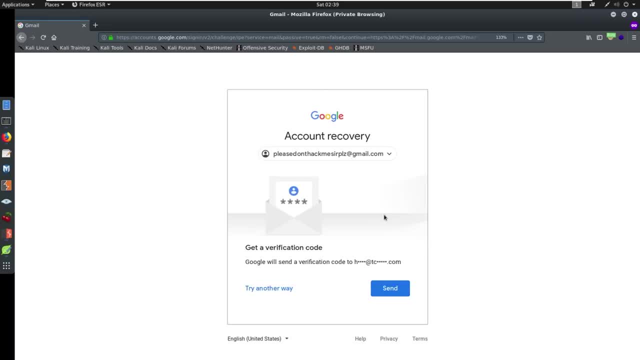 looking through breach data you find a username that matches this email address and also matches this email address. but people can reuse usernames. There could be multiple people who use the same username So you need to verify or some link. This would be a proof of a link between. those are pretty strong proof. 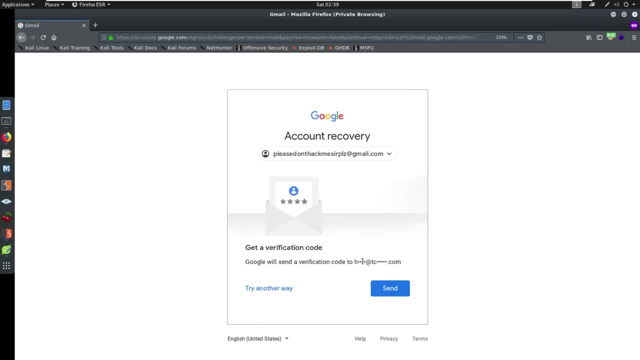 If you ask me if you can say Hey, I identified two email addresses with the same username. I did an account recovery, came in here and saw that this had this same first character and first domain name. I think that's a pretty strong correlation. 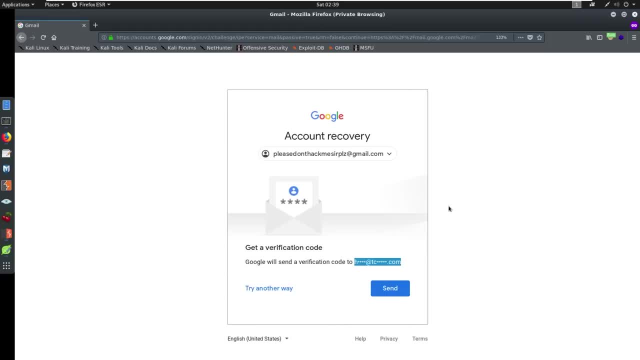 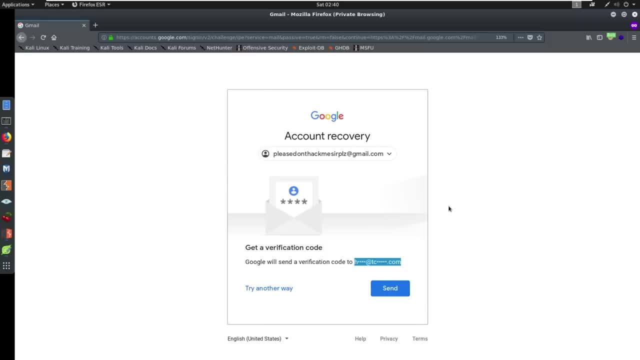 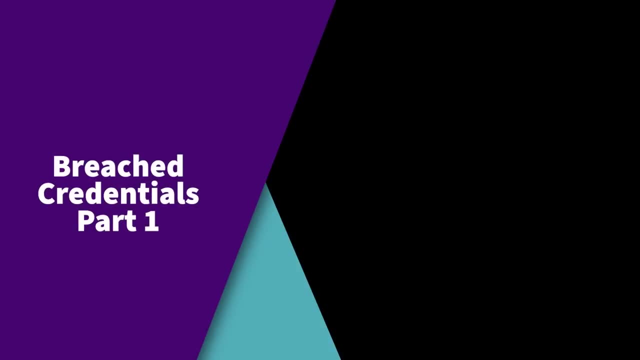 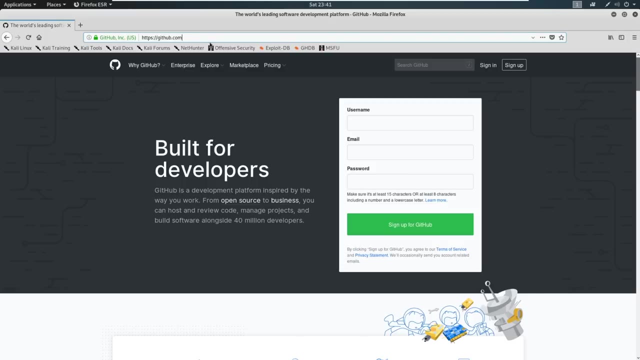 I'm really excited because password hunting is one of my favorite things, So let's go ahead and move on to the next section when we talk about password OSINT. Okay, So I would like you to go out to githubcom and then, once you're there, go ahead and just 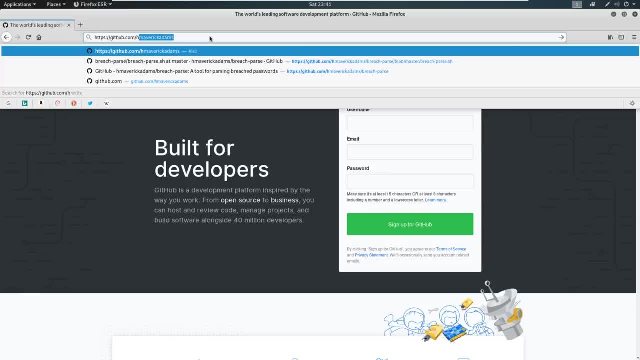 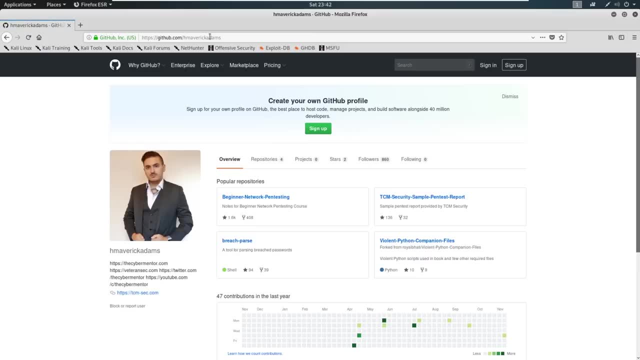 do a forward slash H Maverick Adams, H M A V E R I C K Adams and hit enter And you can see me in my snazzy photo here. But what we're after is, I want to show you a tool that I wrote called breach, parse and 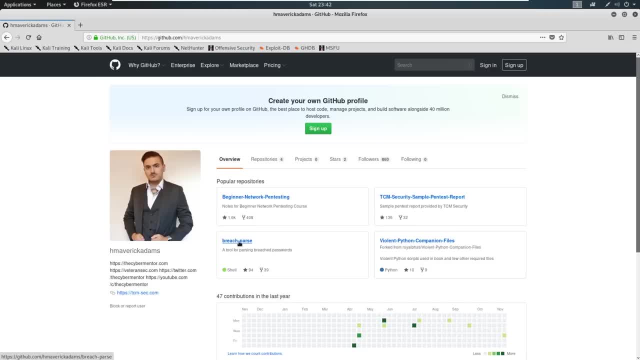 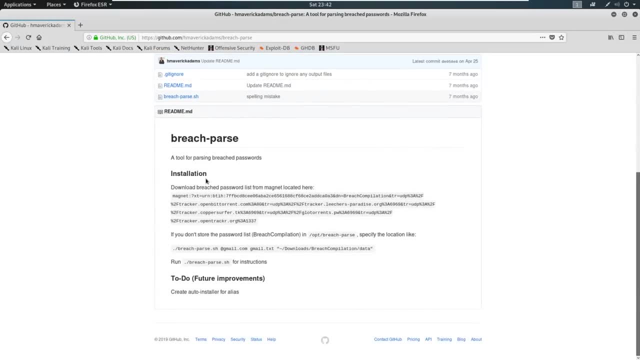 we're going to walk through what it does. Now go ahead and click on breach parse And you're going to see a bash script here and a little bit of a description, So you do not need to download this. Let me preface with what we're doing here. 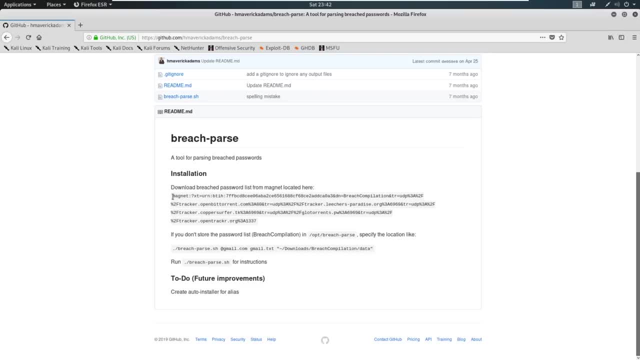 This magnet link. You're going to need one, A torrent, some sort of U torrent or bit torrent, and you'll need to download this, And it's also something along the lines of 44 gigabytes extracted. It's a huge file, so you don't have to do this. 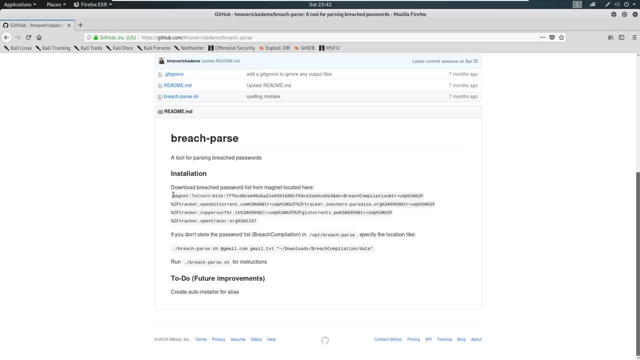 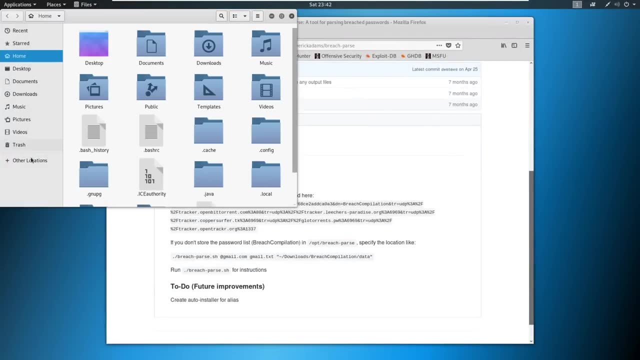 You can just watch and follow along. You are more than welcome to install this on your machine. I'm going to show you what it looks like, So I'm going to go out to my applications and my files here And then I have put this into my opt folder. 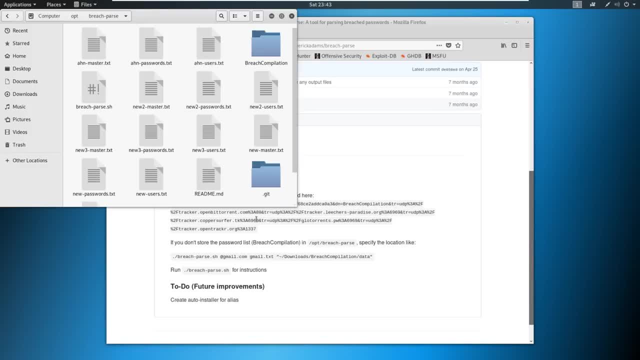 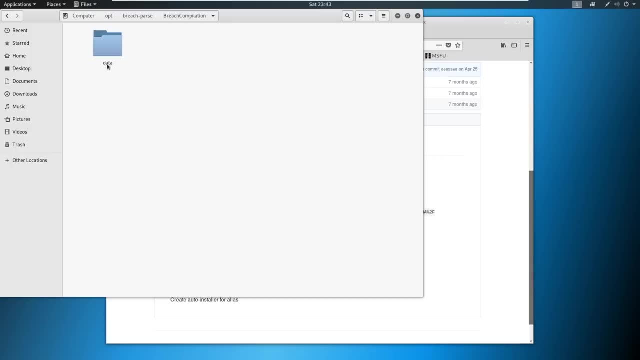 So if you come into opt here- and I've got breach parse- If you come into this breach compilation folder, which is what we'll download, you're going to see that we have data here. Okay, So this data has a bunch of different data. 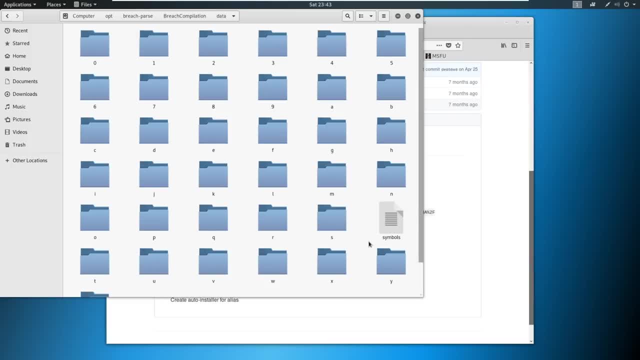 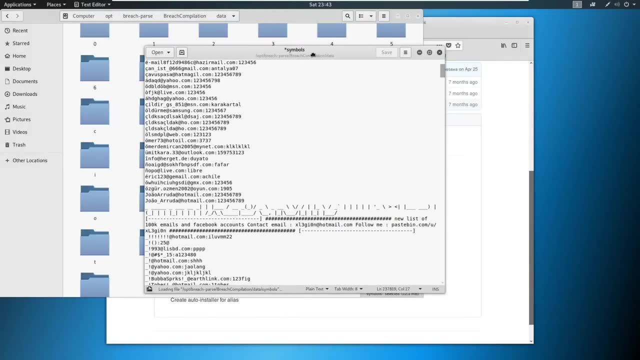 It's got emails starting with zero: one, two, three, four, all these different ones. What's living inside of this is, if we can display, it is emails and passwords. Now you see, these ones have weird symbols inside the emails. Okay, 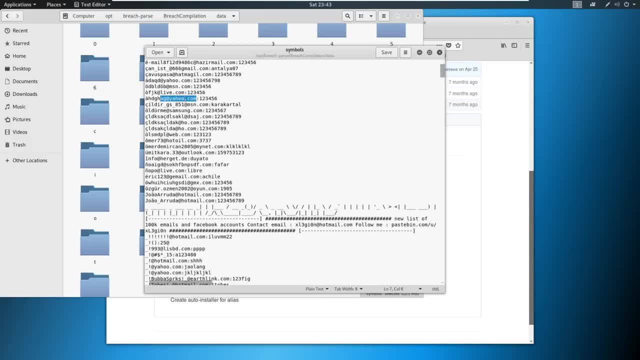 There's a bunch of emails and passwords in here, like somebody at yahoocom, and their password is one, two, three, four, five, six. Well, these passwords are coming from credential dumps, So we talked about it earlier, about thinking about the, you know, Equifax or the LinkedIn. 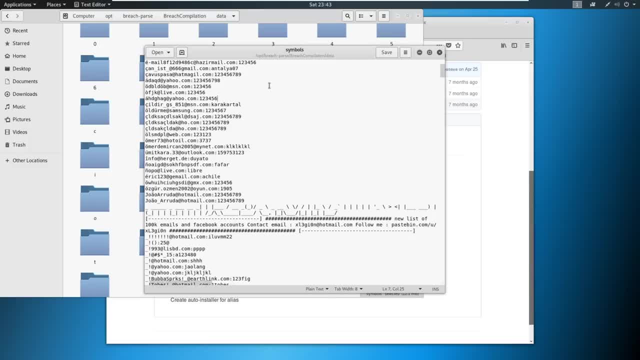 breach or home Depot, all these big breaches that happen. credentials get dumped out and guess what? They show up on the dark web and eventually they show up in these lists. So we utilize these lists and we've got you click into this just hundreds of files. 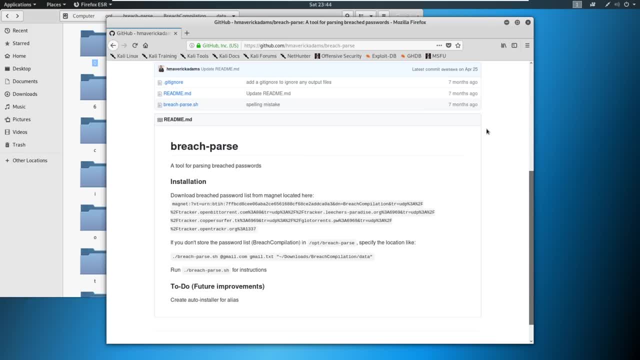 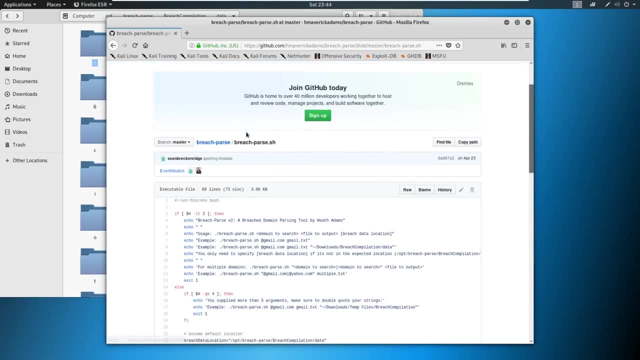 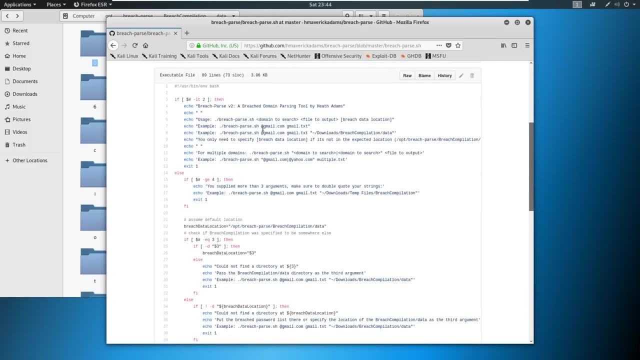 here And again 44 gigabytes. So I did was I built a little tool that can search through this data and pull down names So we can take a quick look at the tool and what it does. But basically what it does is you just put in the syntax, you search for something like: 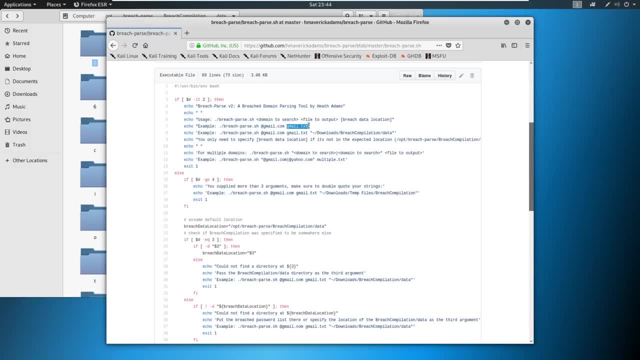 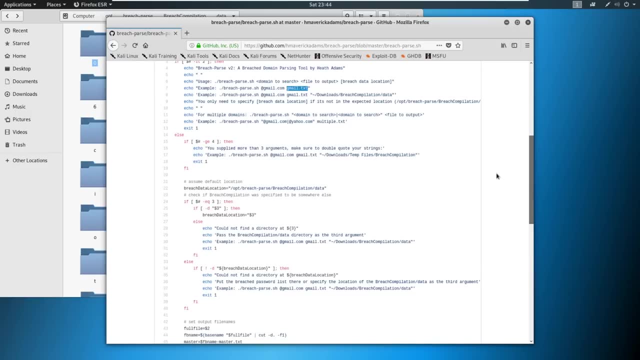 at teslacom and then you specify: you know teslatxt And it's going to search through All of these files for at teslacom. If you're more interested in the code behind it, you're more than welcome to read the code. 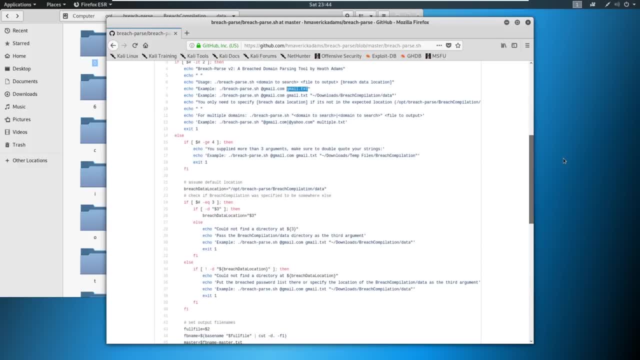 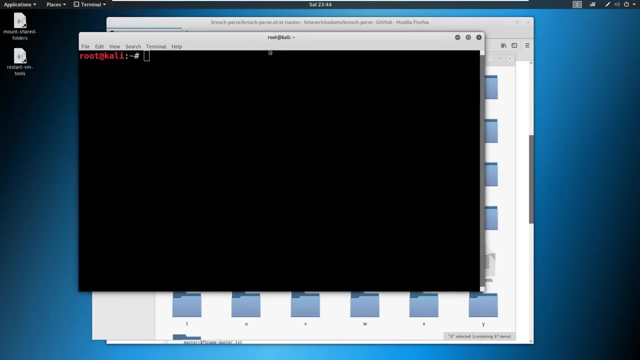 in here and see if some of the items that we've covered already with the batch scripting and the Python scripting kind of ring a bell. So what we're going to do is I'm going to come ahead and go into the terminal and make it a little bigger. 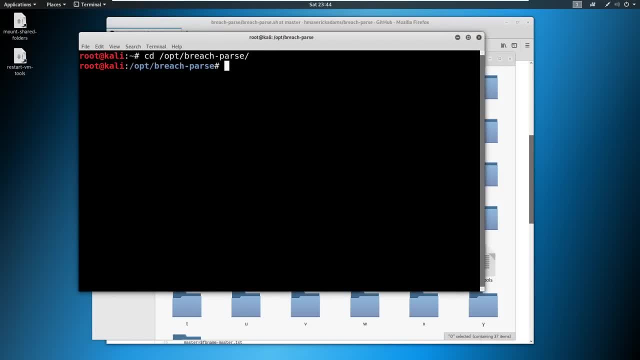 And then I'm just going to change into that app folder breach parse and I'm going to run breach parse, So breach parse here. And what we're going to do is I'm just going to say at teslacom and then teslatxt. 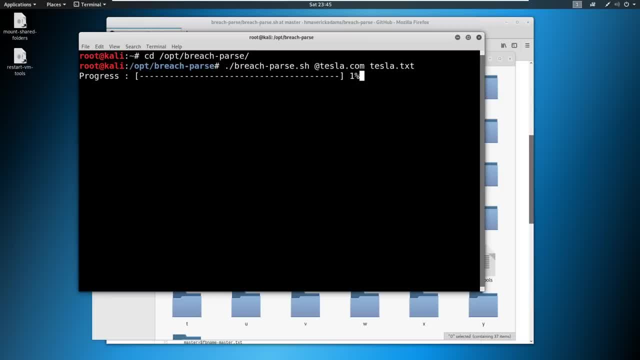 And that's going to run. So, again, you do not have to install this. This is only for visual purposes. I'm going to show you in the next video another way to do this. So this is going to run through. it's going to take a minute here and it's going to grab. 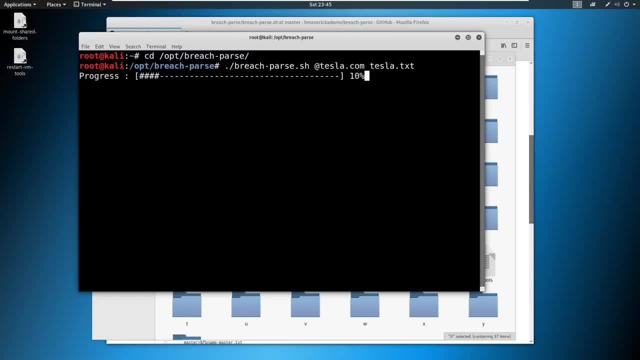 everybody's username and password. that says teslacom And the username, And then it's going to have all the passwords and we're going to be able to decipher things from this. So I'm going to let this run and as soon as it's done I'll come back and we'll talk about. 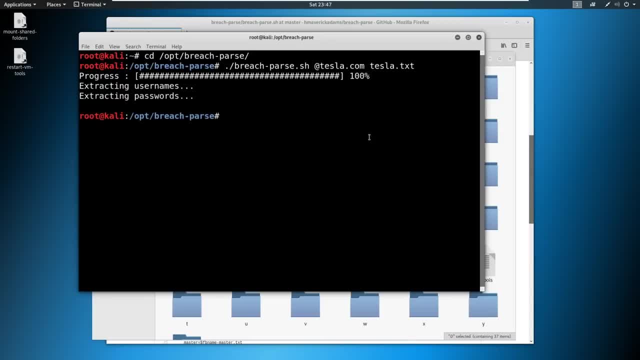 the results. Okay, The results are back. So this breaks it down into three files. There is a it's cat, Tesla. There is a master, passwords and users. So the master has the username and password And then the user's file has the users password. 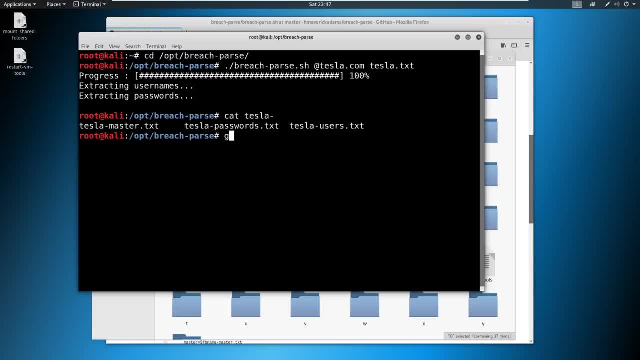 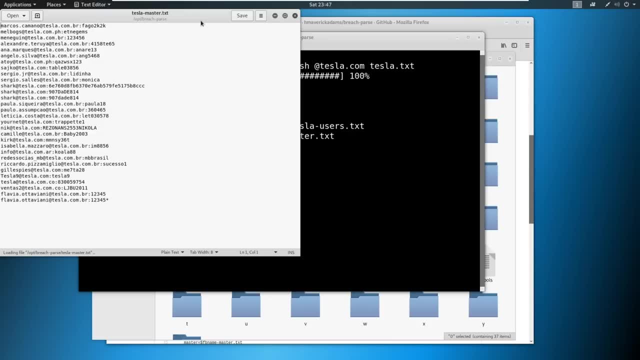 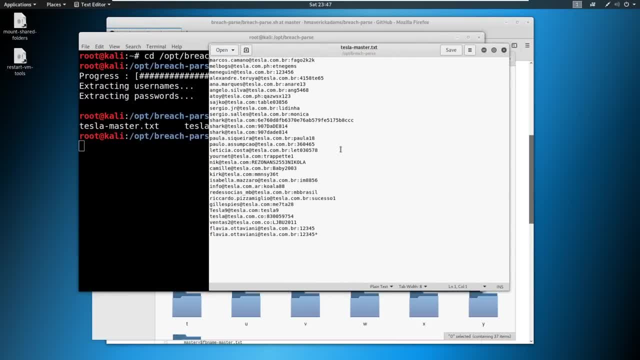 So from here, we don't have a big list, surprisingly for a company the size of Tesla. So what happens is people utilize their work credentials or their work emails and they log into websites and probably shouldn't be using their work emails for, and we just use 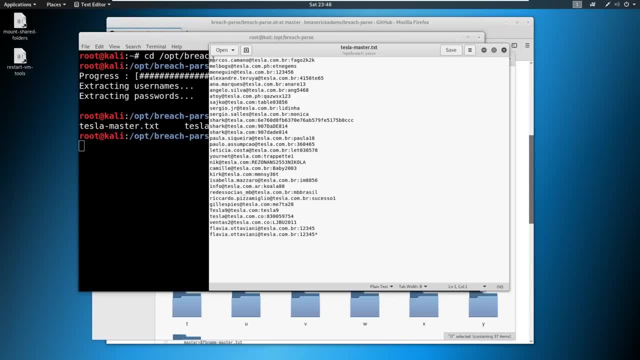 it to our advantage, Okay, So what we're after is we're after not only these usernames, but we're after these passwords as well. So we see these usernames and we see these passwords, and I like to look for repeat offenders. I like to look for the syntax as well. 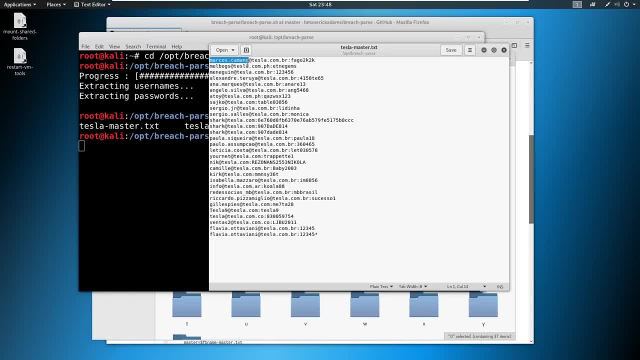 Remember we had first initial last name, but we see first name dot last name here. We see, possibly you know just a single name. There are different types of things in here, So a nick at teslacom as well. So you know if you're looking for a password, you're looking for a password. 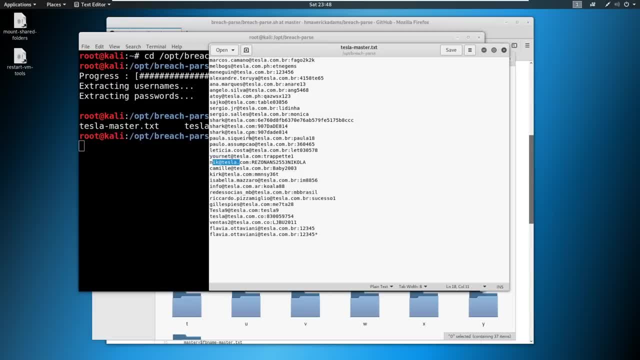 It's changed up. I think nowadays it is first initial last name, but maybe in the past they use first name, dot last name, then move to an easier format or vice versa. They started first initial last name. They got too big, Then they had to do first name, dot last name. 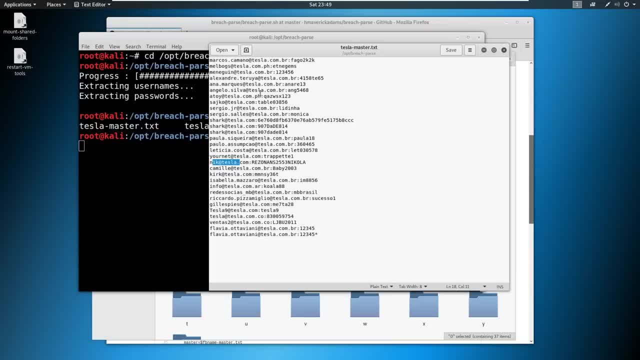 But again, what we're after here is potential repeat offenders. So look at this shark at teslacom. It got popped twice and the password is very, very, very similar. So if I were to attack teslacom through a login interface, I might spray this username. 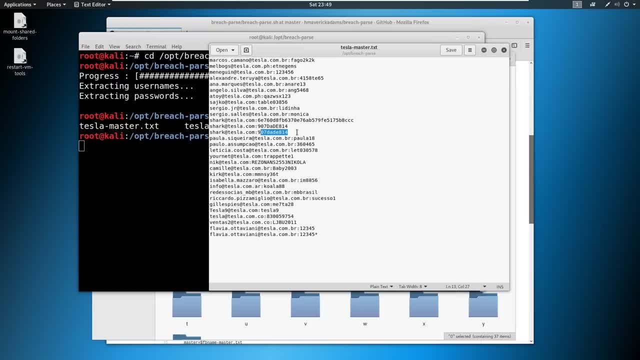 with this password and this password. That's what we call credential stuffing, because we already know the passwords. And then I might make some modification of capitalized letters and non-capitalized letters with DADE, because 907 and 814 appear to be consistent, You know. so I would alternate capitals and non-capitals here in lowercase and just see. 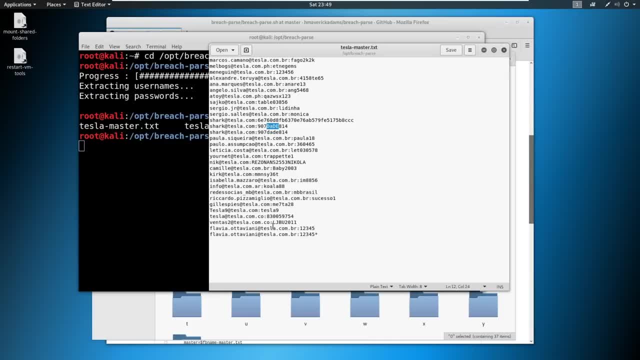 maybe if something sticks. So this is something that's interesting. This user down here- one, two, three, four, five. one, two, three, four, five star- probably not going to get in with that on a company like Tesla, but you never know. 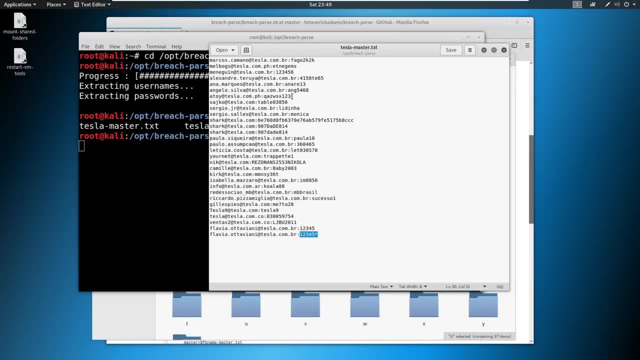 But this is what we would do: We would take the usernames and we would throw these passwords at it, and that's called credential stuffing. And then we would take these usernames and all the known usernames and we would spray passwords at them, like fall 2019, like we talked about in the last video. 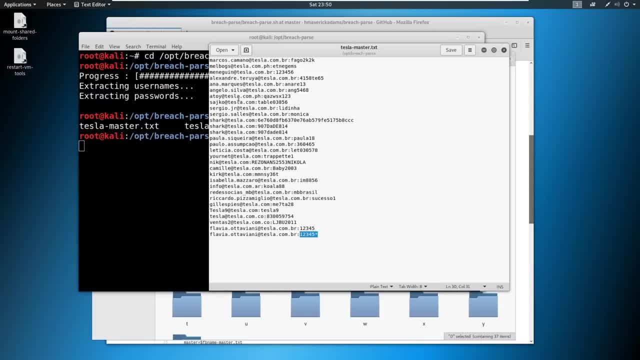 That's password spraying. So this is a important and very, very critical Okay. The next critical part of information gathering is gathering these usernames and these credentials right off the bat. You want to identify those with your targets. So this is kind of what it looks like. 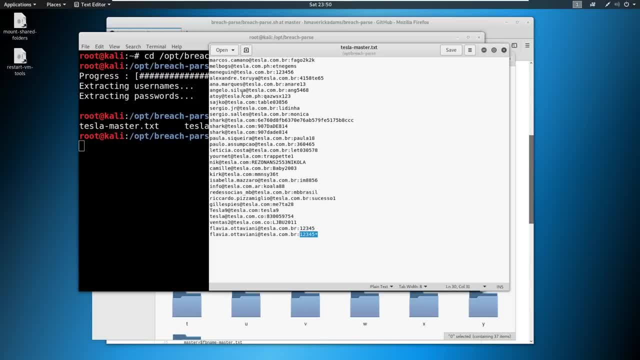 This is what I do during every assessment and hopefully that makes sense and that works into it. In the next video we're going to go ahead and just show another method and start thinking again about these credentials and how they can be utilized, And then we'll do some other information gathering as we move on and learn some techniques and 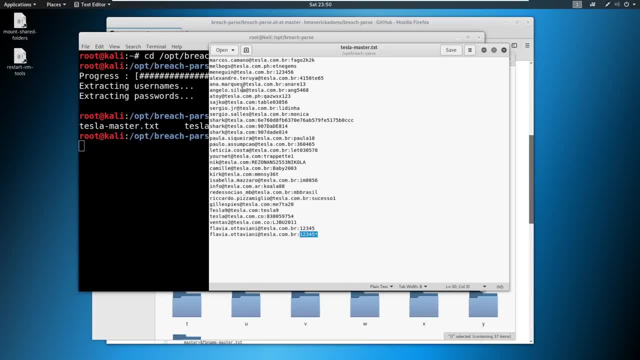 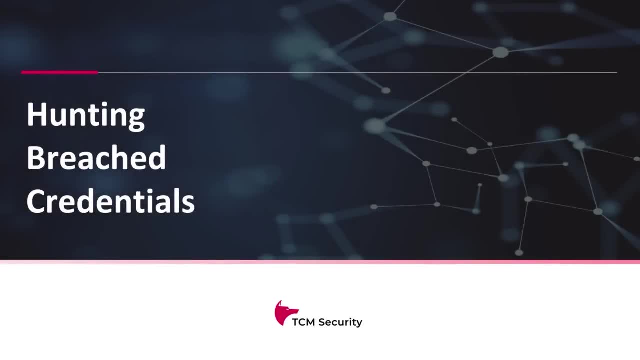 how we can get information on a client. So I'll see you over in the next video. Okay, Let's talk about hunting breach credentials and let's get hands on Now before we get started. I know I stressed this in the beginning of the course. 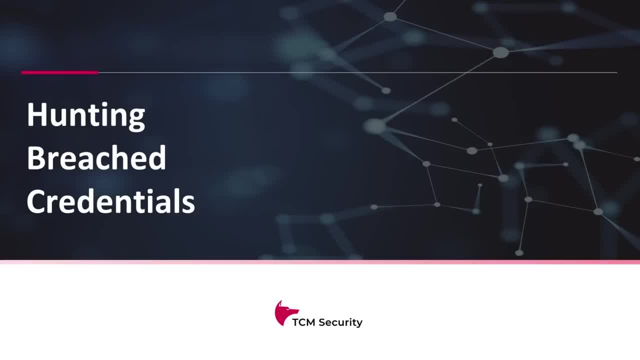 I'm going to stress this again. What I'm going to show you here could change Now. I released a course about a year ago which was on ethical hacking. We talked about breach credentials, And I Utilize a website called we leak info. 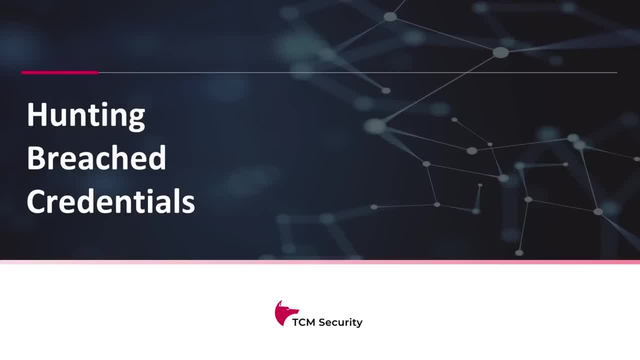 We leak info was then eventually shut down, and I got all kinds of emails saying, Hey, this is shut down, I don't know what to do. There's more out there. Okay, There's always more out there. What I'm showing you is the methodology I could show you on a specific website, which 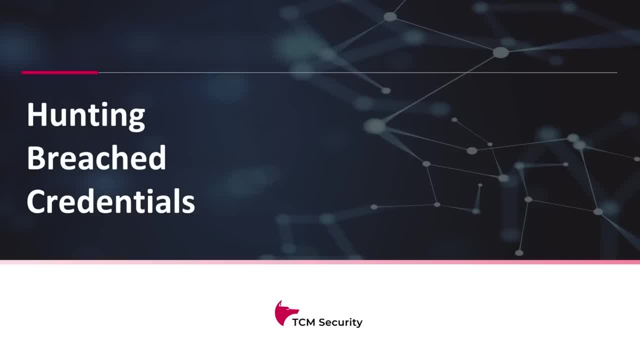 I'm going to do. That website could go down tomorrow- We never know- but what you need to retain is the thought process and the methodology behind what's about to happen. from there You could take that, You could utilize it elsewhere. So if a website does go down, you still have the same thoughts why you're doing it and 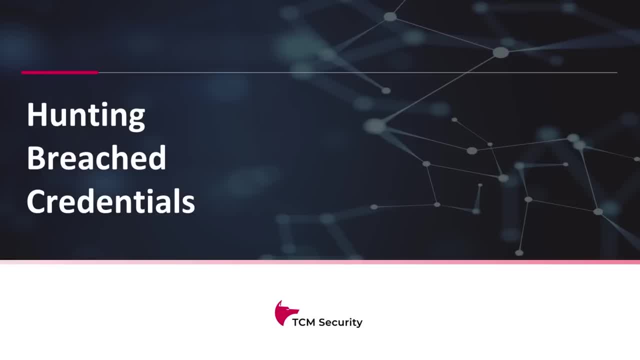 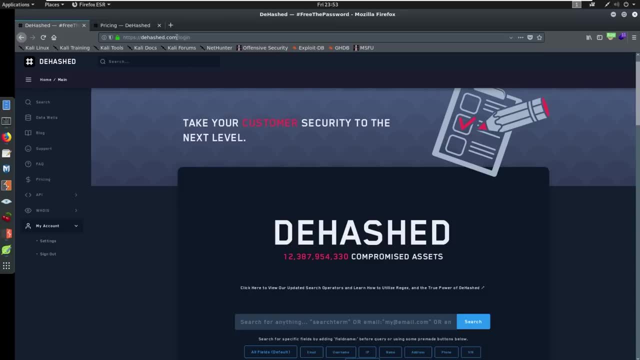 why you're thinking about it. So let's go ahead and move over to a website now. So I want to take you to a website called de hash. Now, this is de hashcom. I do not expect you to be able to follow along at this point, because this costs money. Okay, It's five bucks for a week, So $150 for a year. This is only. it used to take credit card. They only now take Bitcoin, I do believe, or some sort of cryptocurrency. Absolutely worth it, In my opinion. even get a week. get a week see if you like it. 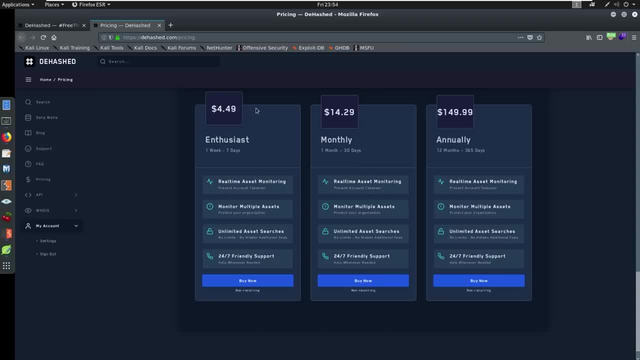 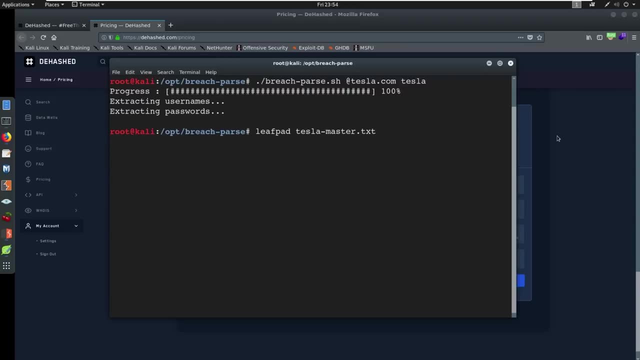 It's amazing. There's going to be tools I show you later on the course that will go through and we can do it locally, Like the one I just ran. in the last video I ran breach parse, right. This is something that I put together and set up, but- and it's free- but the database. 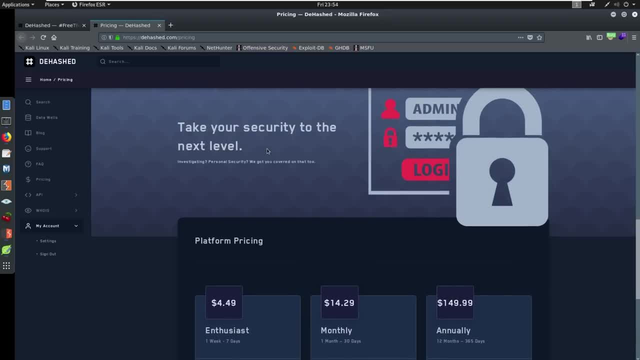 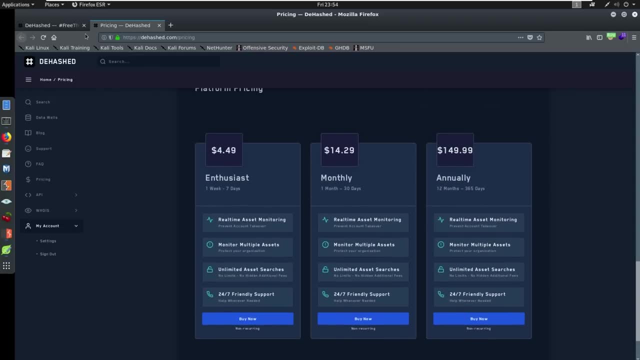 isn't maintained. It's a slow search. I don't get the results back as instantly. Okay, You can buy it to as many data points as a website like this can. I think this website's great. Now let's talk about what de hash can do. 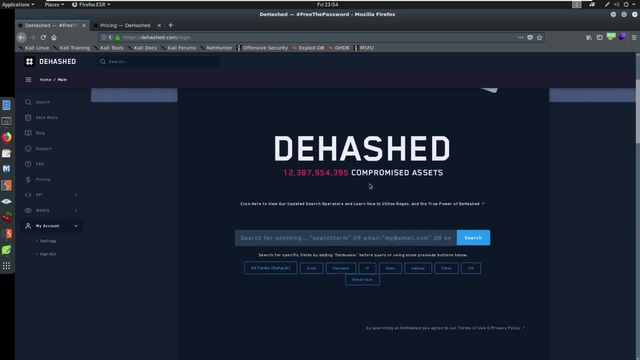 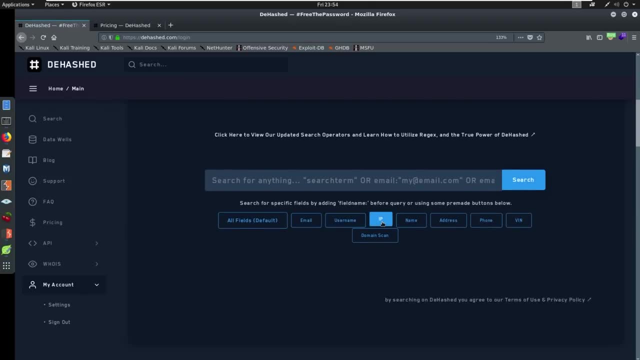 Now that I'm logged in, we have the ability to search by. let me make this a little bit bigger. We have the ability to search by email, username, IP address, name address, phone number, VIN. Okay, Think about this. 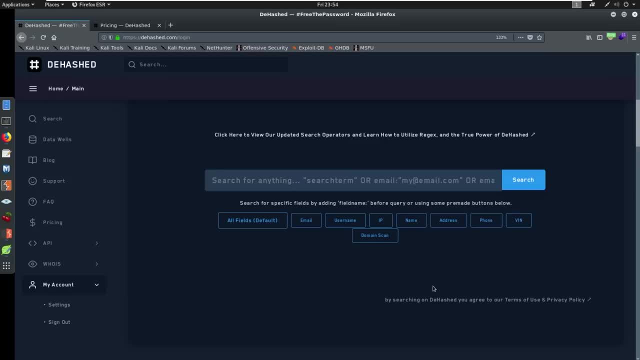 Say we know a email address, Okay, We know an email address. Say it's Bob, Bob at teslacom, We're not going to search this yet We take Bob and we know Bob has an account and we're looking for him. 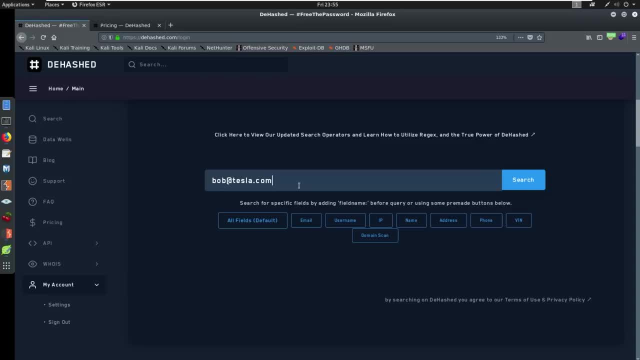 We search him. Bob shows up and we see Bob shows up and we see maybe his name, like Bob Jones or something like that, shows up. Maybe something that he's been leaked in has his address, or maybe there was an IP address tied to the client you're looking for, the person you're looking for. 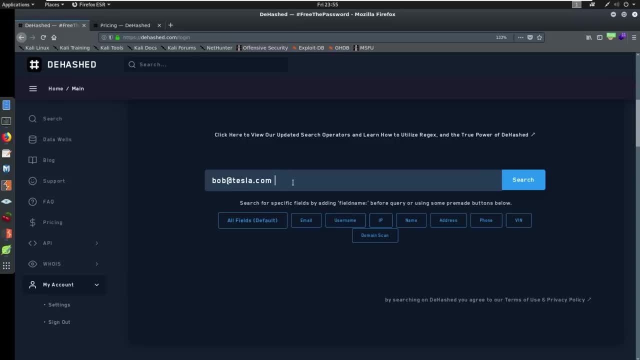 This can all be identified. What if Bob has a username? It's like Bob, Bob rocks one, two, three. Okay, Well, we can search that username in here and see if that username has repeated itself at all, which is great. 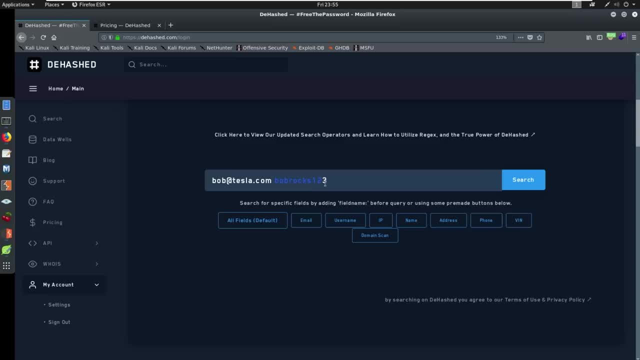 We could search by password. So say, Bob's password was Bob rocks one, two, three. We could search that password and if it's unique enough, then maybe we can actually do some advanced searching. Like if we go back to the example from last time, like this last video, we saw this nine. 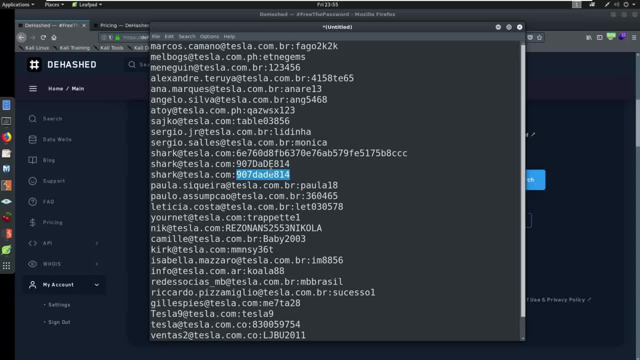 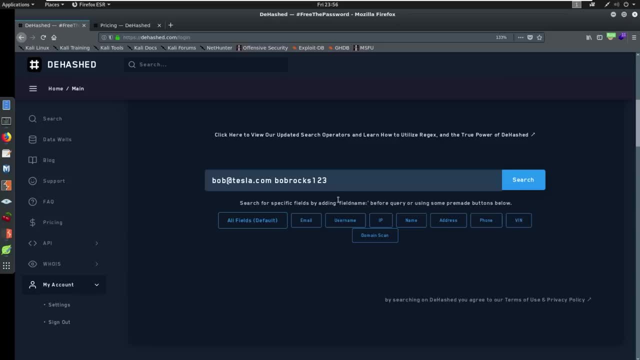 zero seven D a, D E, eight one four. Okay, We could put that into a search engine and see if that comes back to something else. Maybe that comes back to a user that is not at a teslacom, but maybe it's like Bob at. 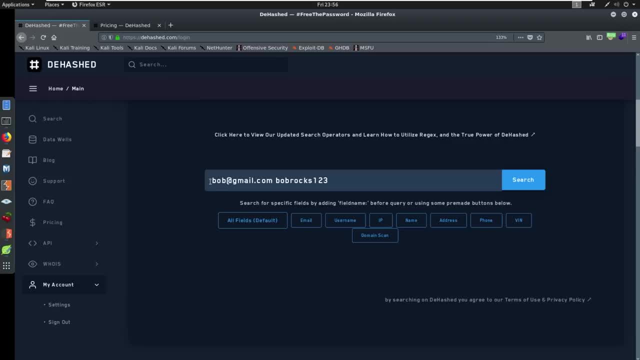 gmailcom. And then guess what? Now we have Bob's personal account, or now we have Bob tied to another email account, especially if we search by name or something that we can tie them together. We need to start being able to relate other accounts to each other. 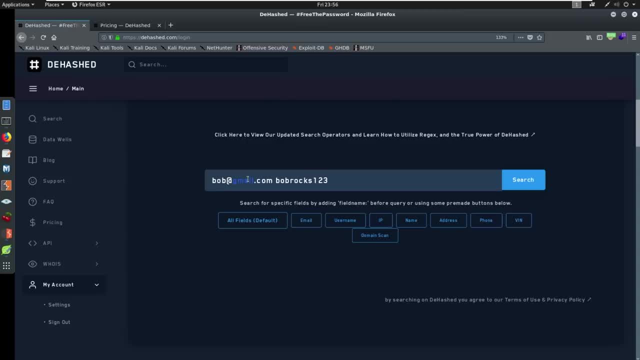 We can do that with hashing. We could do that with passwords. There's a lot of things. There's a lot of things that we can do and we want to start tying this together. as a real world example, When I am looking at an organization and I'm doing research on on hashing, or I'm doing 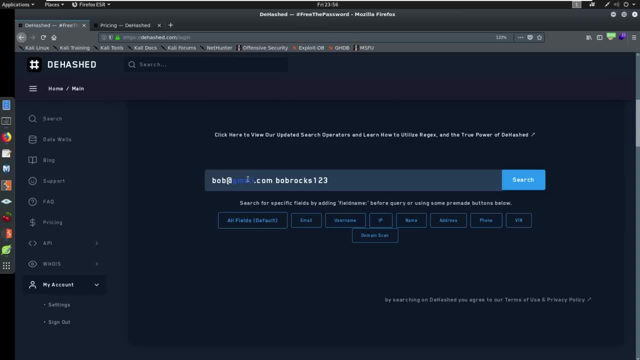 research on breach credentials. I'm trying to think: okay, first if my client, if my client is teslacom, I might come in here and search at teslacom and I might come see how many results are in here. Let's see what happens. 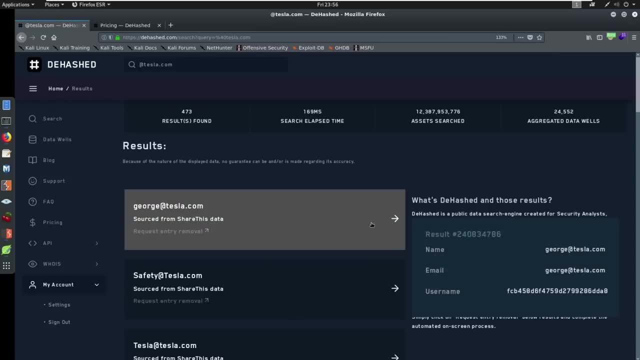 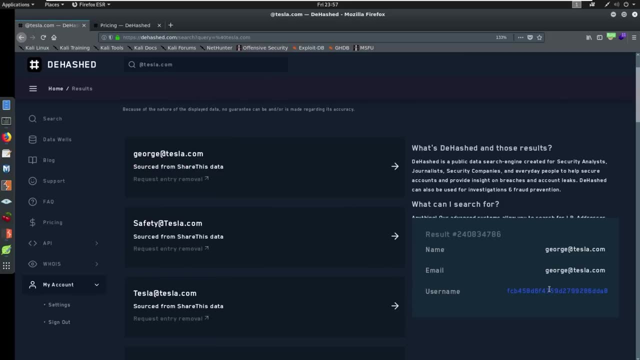 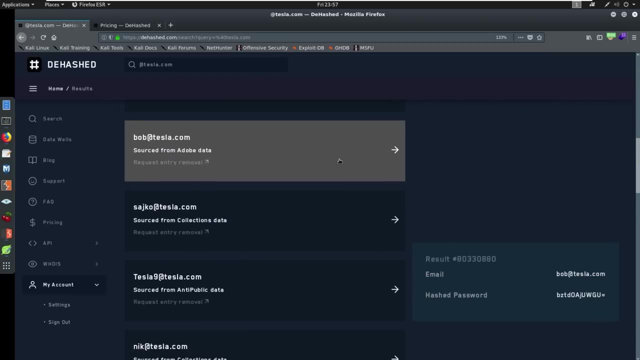 Okay, Here's George at teslacom. George has been in a shared data, So there's no actual um any data details here besides a potential username, a name, email. Okay, Same thing with safety. We'd have to scroll down and see if we can find something that okay, here's Adobe. 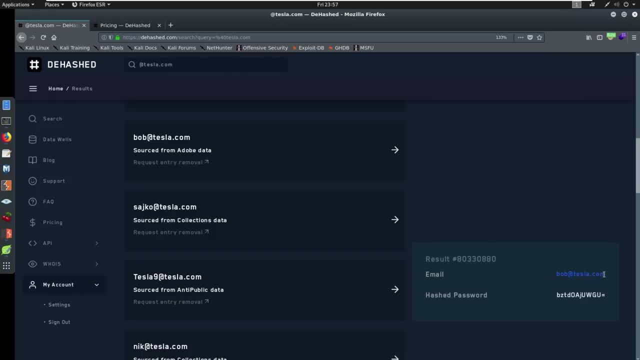 Now Adobe will have a. there's actually a Bob at Tesla. um, Bob at Tesla has a hash password here. Okay, So now we can say: well, first of all, we can go see if we can figure out what this hash is, which we'll talk about in a second. 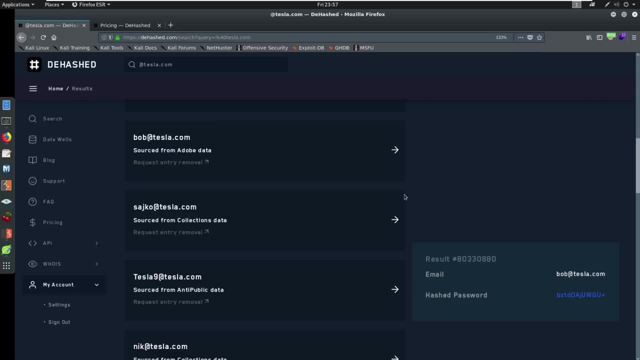 We can also go and say: okay, Bob, uh, does Bob exist Anywhere else? Does this hash exist anywhere else on this website? Can we tie it to another account that maybe, even if we don't crack the password, then we can say: okay, this Bob. this ties to Bob at gmailcom. 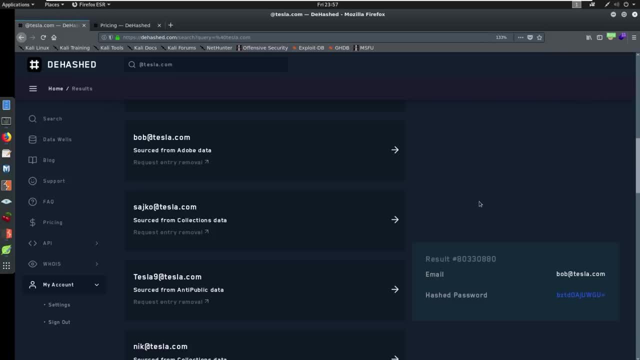 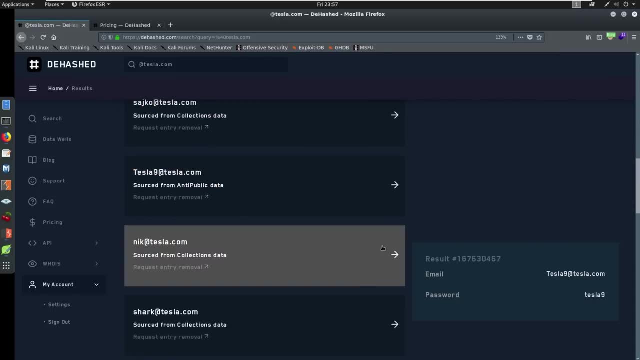 So, like I would note this down and I would take this and copy it. So for me, real world example, I would take all the data that I see on this website. I would collect all of the passwords, all of the usernames, everything. 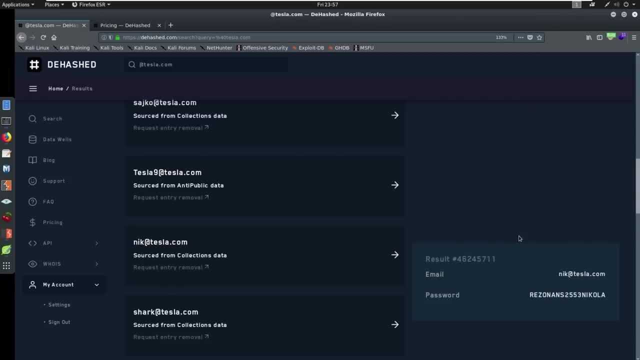 So, like Tesla nine, all of this, I want to know what the passwords are. I want to know, I want to know who the people are. I want to know all the data because if I could start finding patterns, if I could start putting 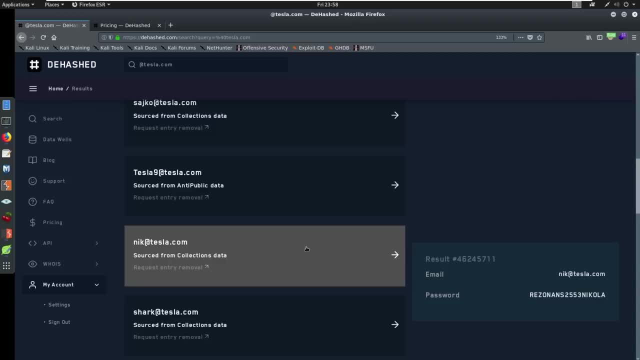 things together. maybe I can even relate these back to their personal email accounts, like we're talking about, And then I could see password patterns there or other passwords and just start tying this down, because my goal is to break into an organization. If I'm doing a pen test, my goal is to break into an organization. 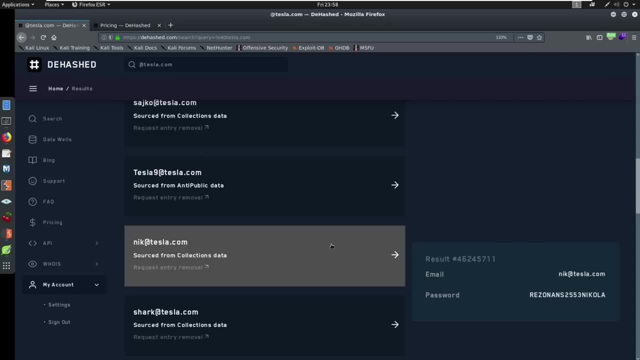 So I'm going to take that data And if I can find other passwords related to a personal account, I'm not going to go attempt to break into a personal account, But I will take that data and I will put it together and maybe try to break into their. 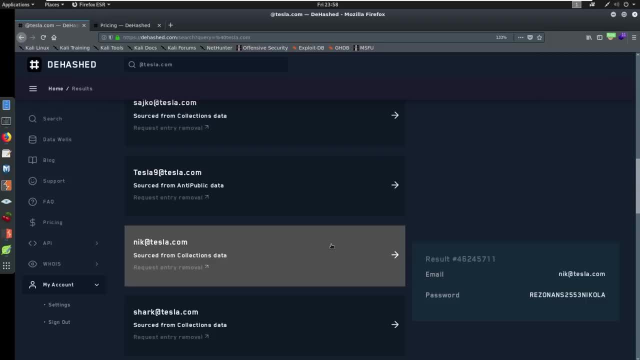 work email account with those passwords, that information. This can tie to an investigation as well. If you're hunting down an individual, you're trying to tie them to other accounts. This is incredibly useful if you can find their data in a breach database and have a. 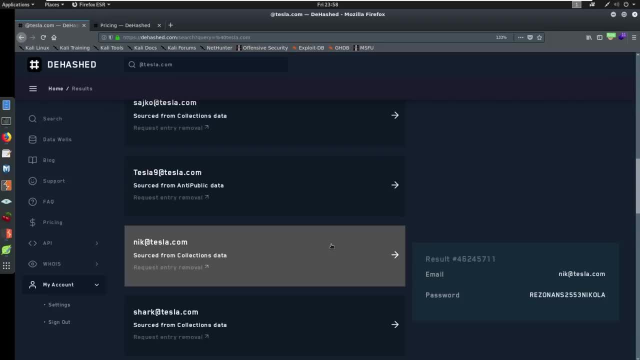 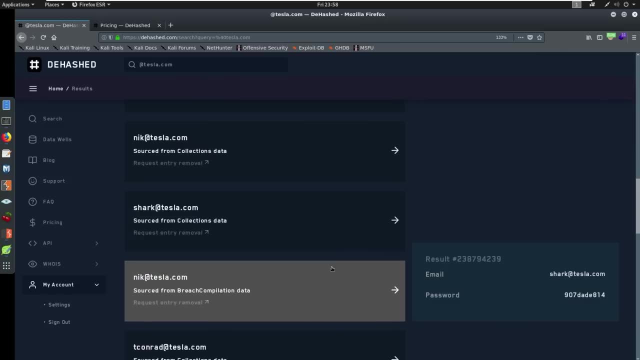 password and that passwords unique. you can search it, maybe find them somewhere else. You find an IP address, you find a name. There are often IP addresses in here which we can tie. Let's say this is a key to a location, possibly. 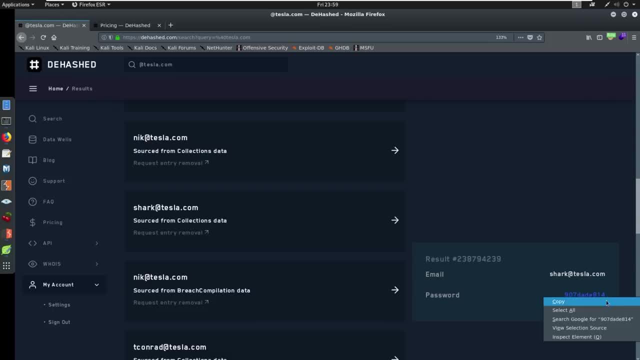 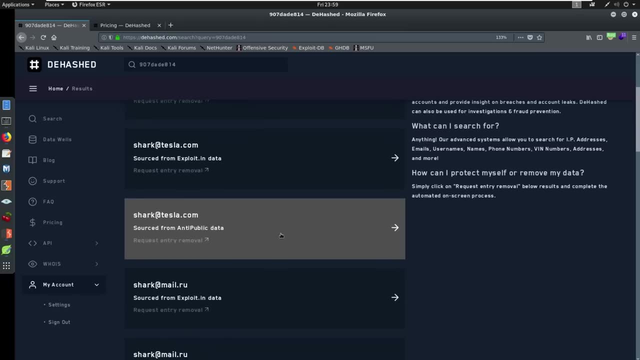 And see, here's that: 9078 or D a, D, E, 8, 1, 4.. We could take this and maybe search it and see if it comes back. Anything. Who knows? shark at Tesla. shark at Tesla, Okay, Shark at mailru. 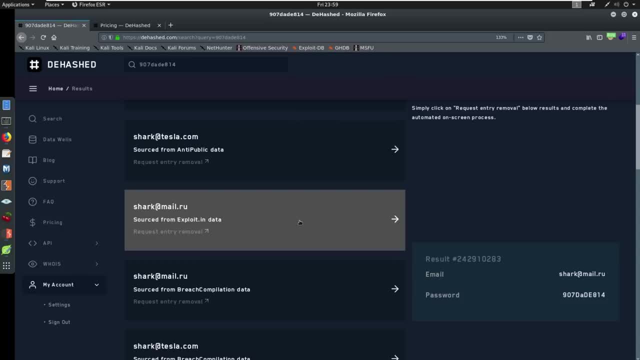 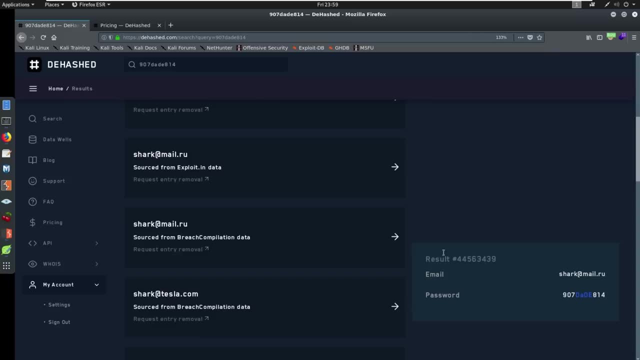 Look, this is a new new email address. We didn't know about this one before And look, it does us a favor. We searched D a, D, E, but here's the capitalize. We didn't search for capitalize. We're not searching specific. 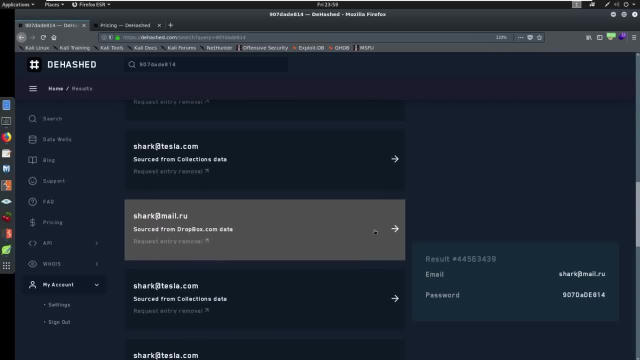 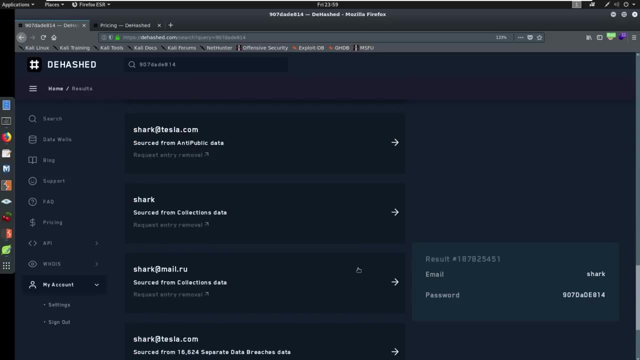 Okay, information. Look here's one for Dropbox. Okay, so it tells you where this is coming from and how you can tie it in. If we can get any sort of name out of this, any sort of anything that would be. 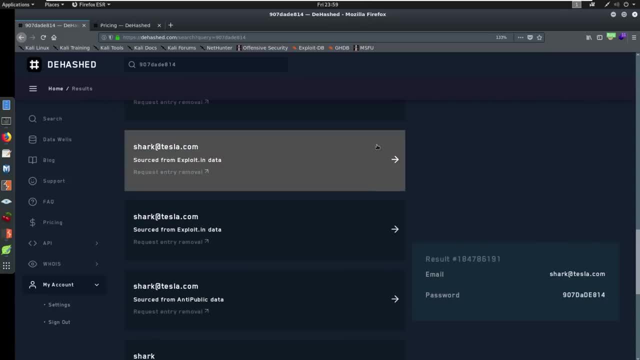 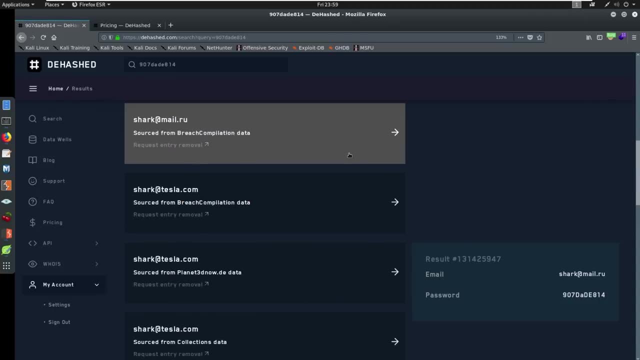 amazing. We can get a person's name or IP address and we can start tying them down. But when you're doing different searches like this, you need to start almost, you know, like in the investigations where they have like the the red yarn and it's going from one pinpoint to another. you kind of 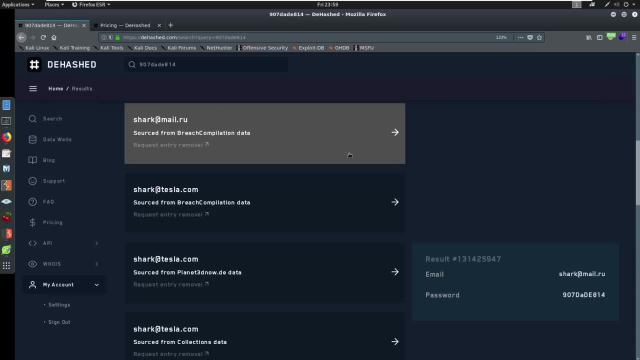 have to zigzag that back and forth and really try to tie this down. And you'll see that when we get into reporting, how you might take one individual and really just see like a password tied to an account tied to this, And this was the exact methodology that we took to get to that point. 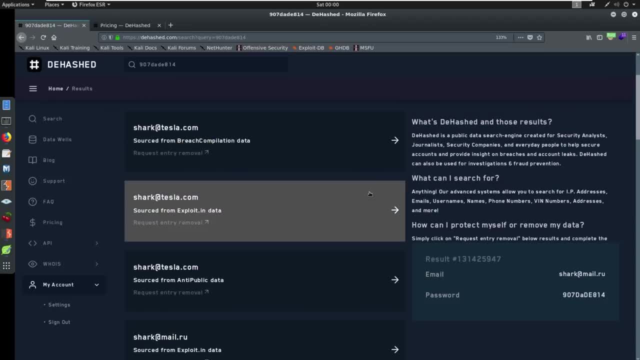 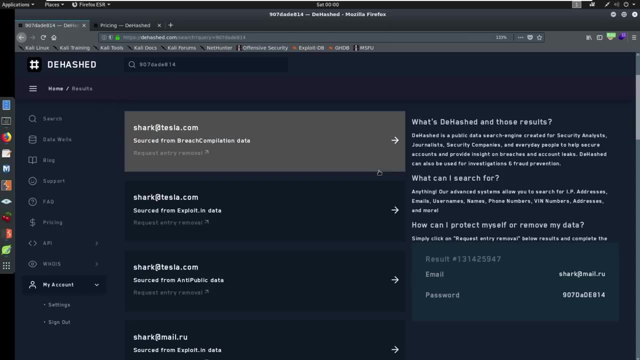 Because when you write a report, you want to make sure that the investigative person or the say you're handing off to the police or whatever. you want to make sure that the person that is doing what, what you did, or they can replicate what you did with ease. And there's. 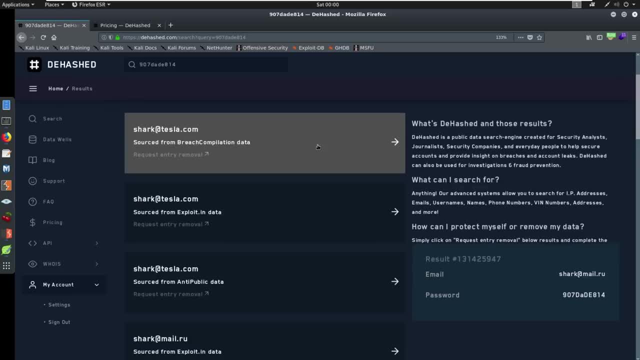 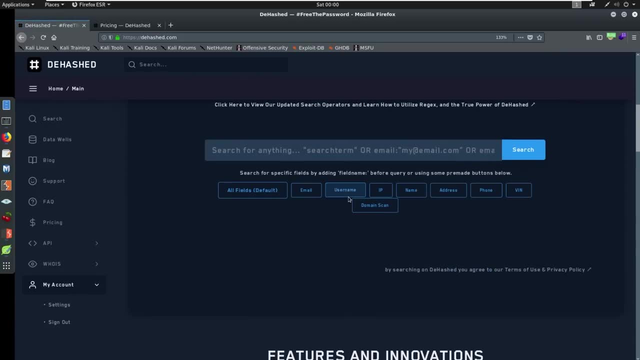 no, no question about it. So this is some of the searching that we can do Now. if we come to the hash again, we can come here and we can search by email, username, name, anything, So you can put your name in here. I mean, if you want to search on here, I think it's great, You can come through. 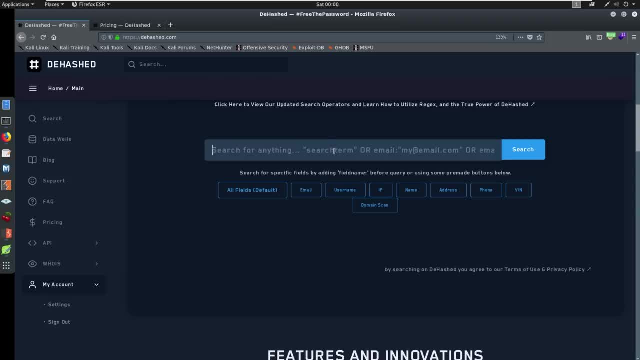 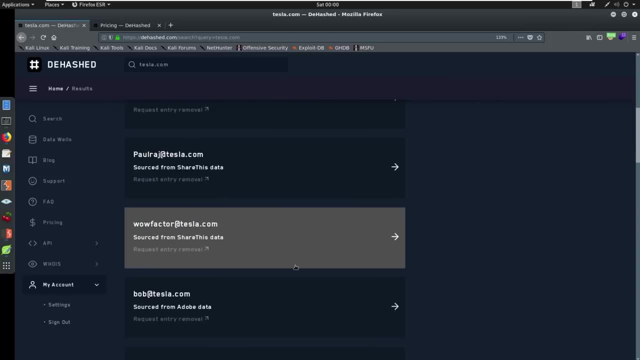 here and just search for your name. Let's go back. let's search Tesla again. I saw a hash in there. The Adobe hashes are kind of interesting. They're not the easiest to pick up, But let's see. let's find this Adobe hash. 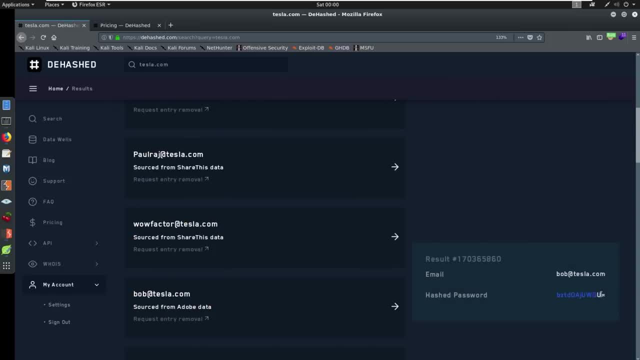 So let's say we get a hash like this. We could try to identify what this hash is. we can try to crack this hash. we can see if it's been cracked somewhere else. This hash- as of right now we have no idea, But we know. Bob at teslacom, We can maybe paste this in here first of all and see if. 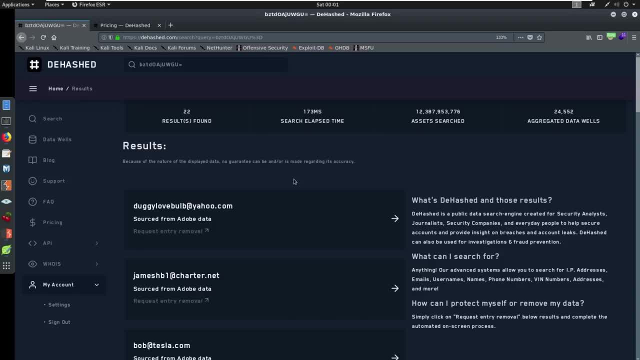 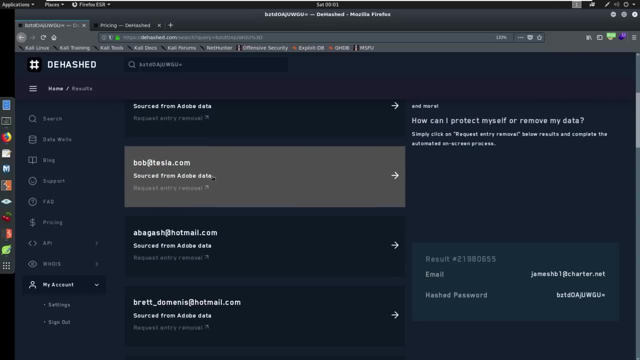 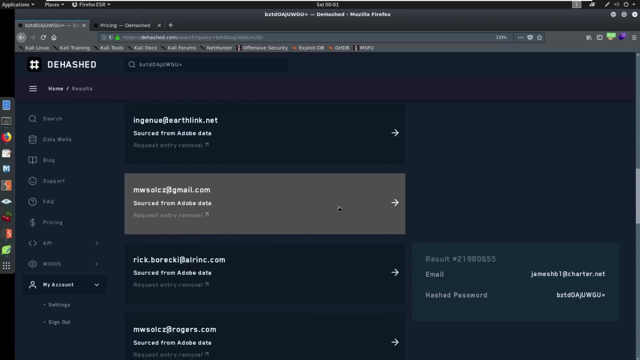 it ties back to anything And there's 22 results back. You know I would probably be looking for somebody that has this password With the name of Bob. it's probably not going to be like a Brett or Michael. you know, we might want to see if we can find another account somewhere else. 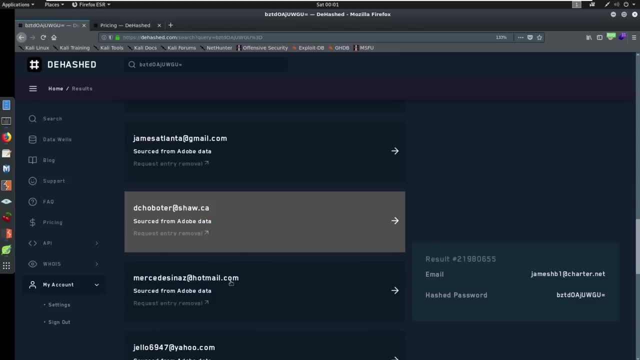 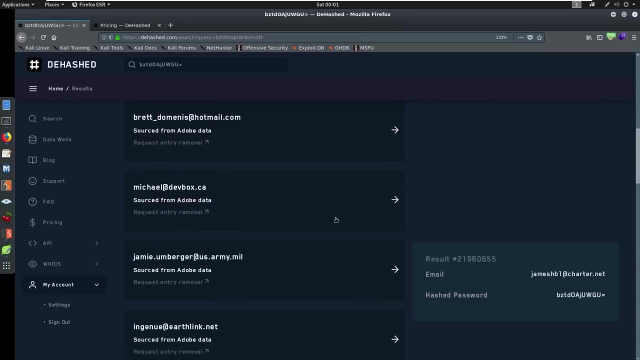 But these are all tying down to a hash from Adobe, So depending on how they were hashing this data, we might not find anything else of interest. But you can see all the things here, all the different opportunities that are here for us to just do research and tie down information. Now we can. 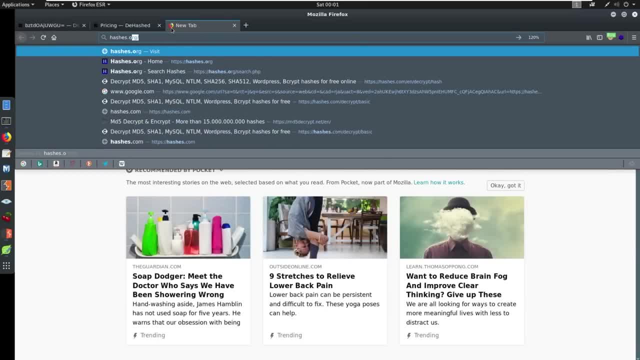 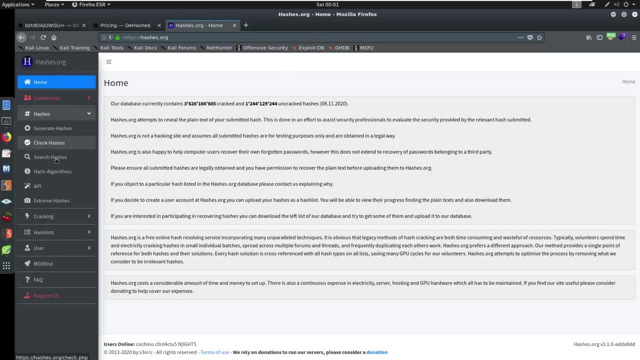 go to a website called hashesorg And if we come here we have the capability to actually try to search for this hash. So we could search hashes and see if we can find it. So you can come in here and just paste it. 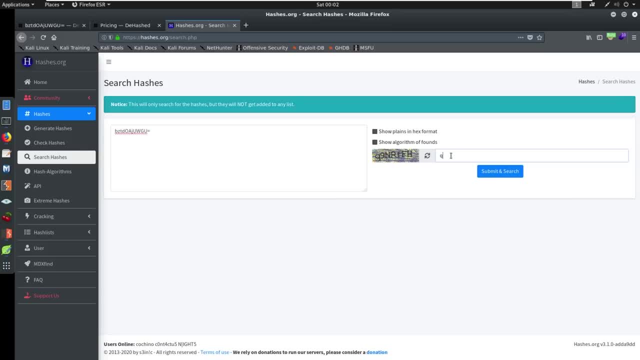 And again, it doesn't do a great job, in my opinion, with the Adobe hashes. sometimes they crack, but a lot of times it says it can't find them. Oops, there we go. Let's try hitting a search here. Okay, so it says not a valid hash. Now 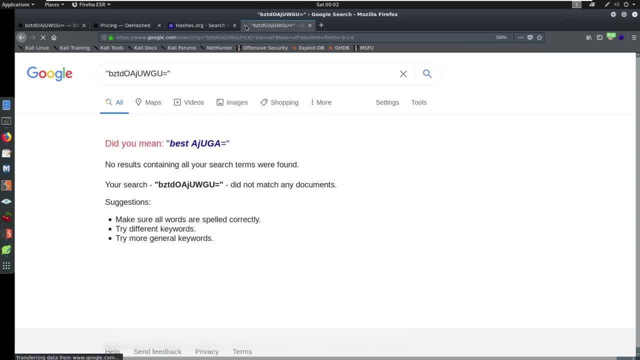 if you put this into Google as a search, you can see it didn't come back with anything either. We want to make sure that when we're searching this, you know we we try all options. there is an Adobe database that if you do put in a hash and it does show up. 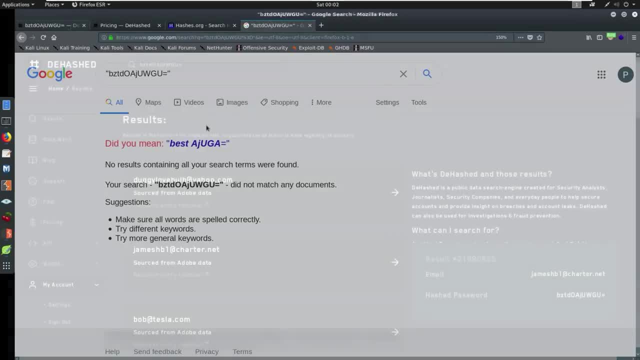 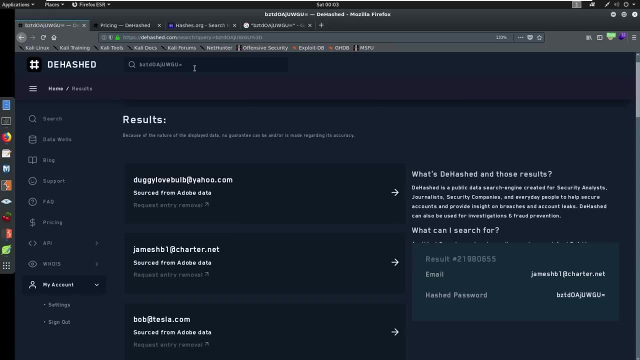 there's a GitHub Adobe database that will actually show up here. So, with that being said, this is kind of what I want you to start thinking about when we're hunting down breach credentials. How can I take a person or company that I'm looking into? So, if you have a company, 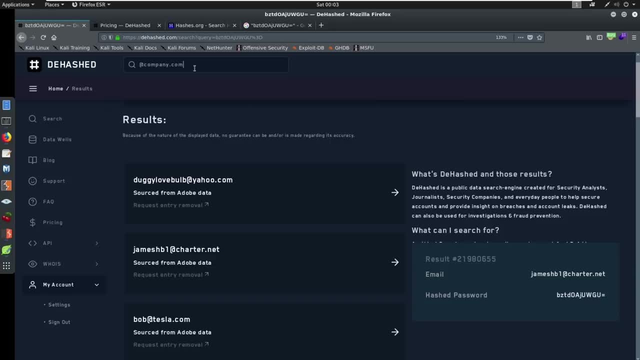 you can just go at company namecom or dotnet or whatever it is, search in here, see how they show up. If you have a person, maybe a personal email account, if you can find that person, if you know their email account, you come in here and say Bob at gmailcom. 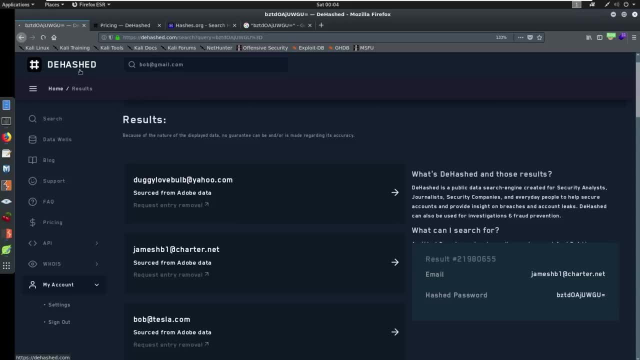 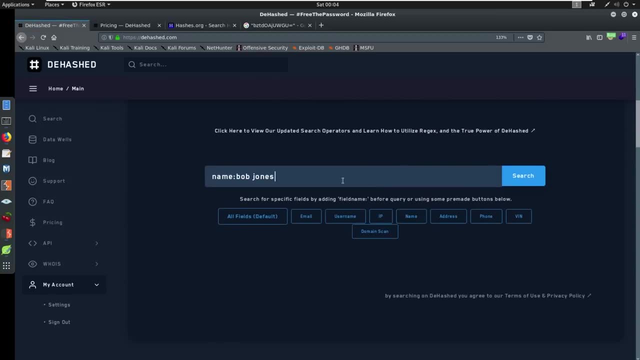 Maybe you don't know what their, their email addresses. then maybe you come here to the main page. you go: Okay, I'm gonna look for a name, I'm gonna look for Bob Jones and search for that, And then you start taking this and trying to find the patterns. If you know, Bob lives somewhere. 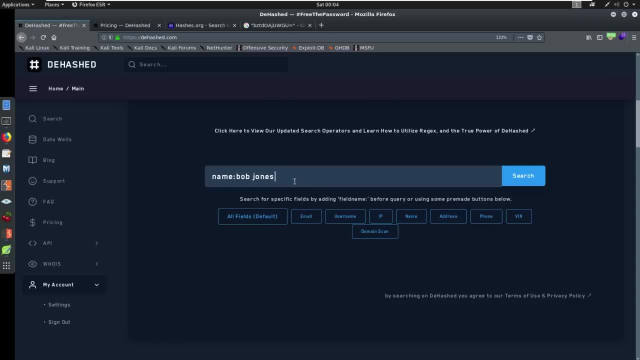 maybe you could find an address for Bob or maybe you know Bob lives in like Arizona. You could search Bob Jones and see if Bob shows up and then kind of take it from there, And there is some search operators that you can utilize. you can see Bob Jones is taking forever. you can put. 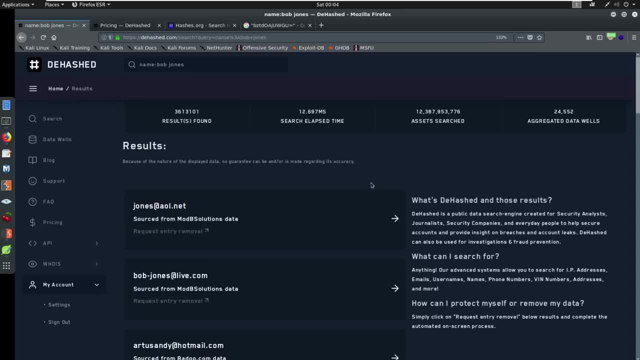 this in quotations and search it again and kind of narrow down your results here. So if we click on this, you can see like here's a name of we got a lot of results, but here's the name Bob Jones. This is a very common name So, but you could see like, if we're trying to look this down, 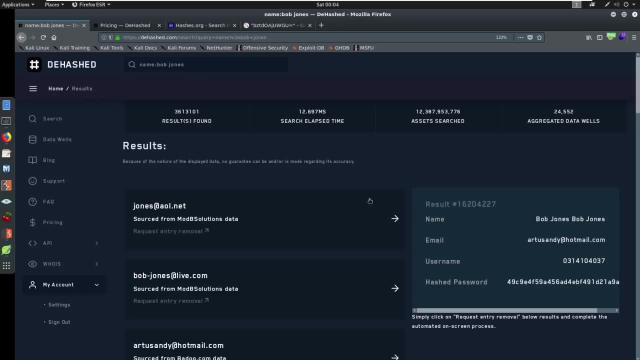 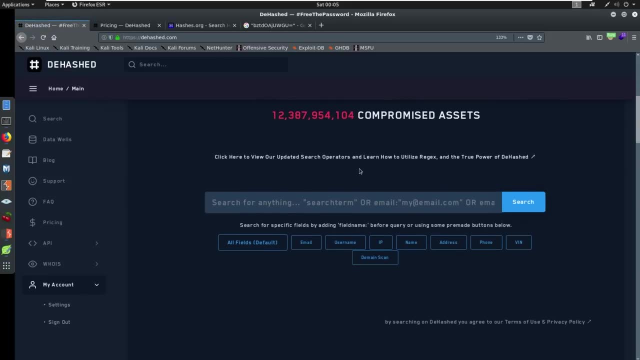 we can start searching and adding operators in here And trying to see if we can figure out to tie a username or something to them. So again, get your wheel spinning. Don't rely on just de hashed, But just rely on thinking about this. 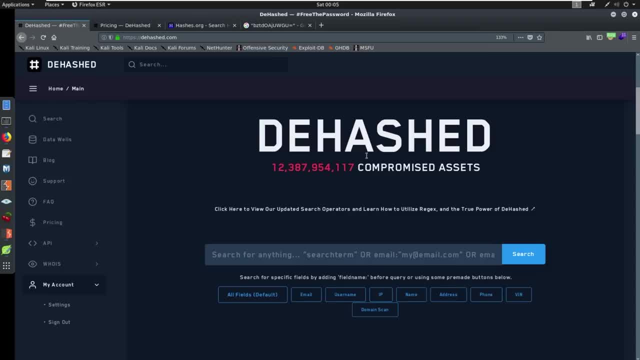 this is the thing you should be thinking about Again. the hash could go down tomorrow, But if you're thinking about it in the way that the credentials and the information can be interwoven, remember that red yarn again. that's really what I want you to take away from this. 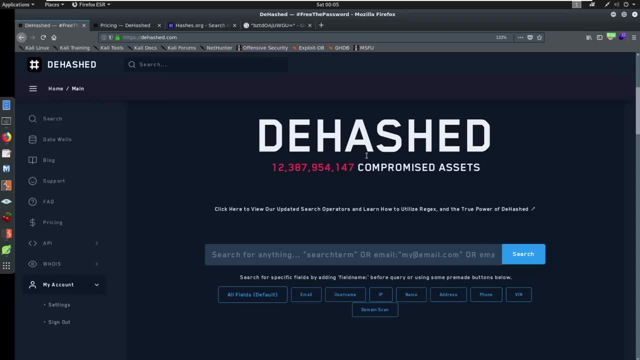 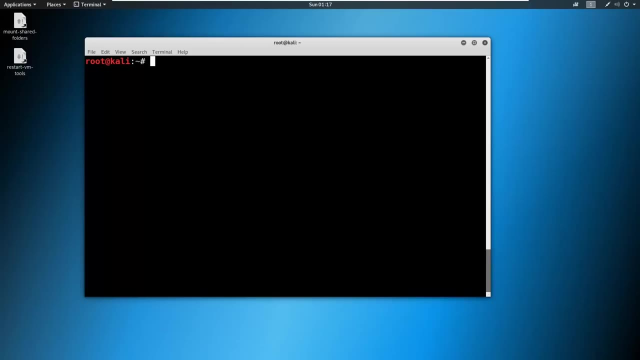 So we're going to do another video on this. I'm going to show you some more. I guess tools that are out there and some other things that you can do offer alternatives to this, And then we'll wrap up this section. So I'll catch you over in the next video. The next several videos are: 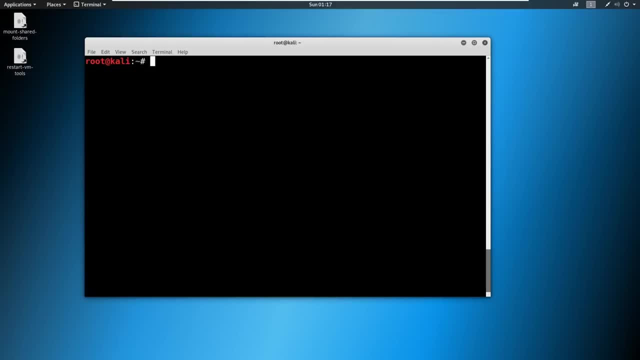 going to talk about web information gathering. So this is going to be important because a lot of the times we're going to be tasked with a web penetration test or we might encounter a website on an extra, etc. So we are going to be working on a web penetration test. we might encounter an. 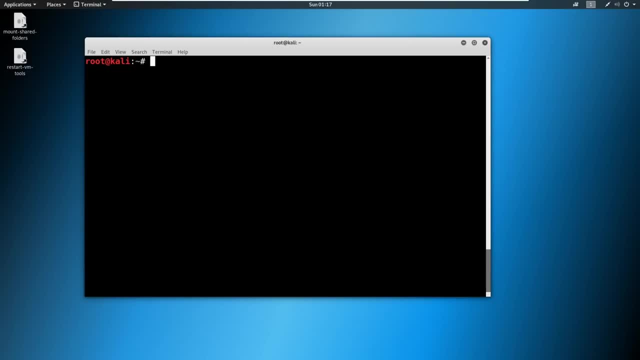 external or internal penetration test, And being able to gather information and perform enumeration on those websites is super important. So what I'm going to show you throughout is how to gather some of the information passively that is out there, And then we'll talk about active methods that 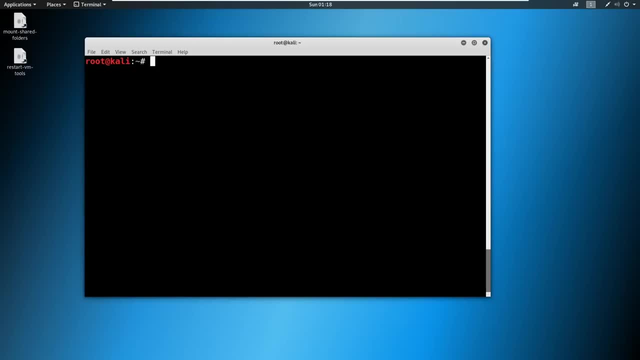 actually involve going out to the website and gathering information that way as well. So the first and most important thing, especially when it comes to websites or bug bounty hunting etc. is that we need to identify what subdomains are out there, And you saw earlier when we were looking. 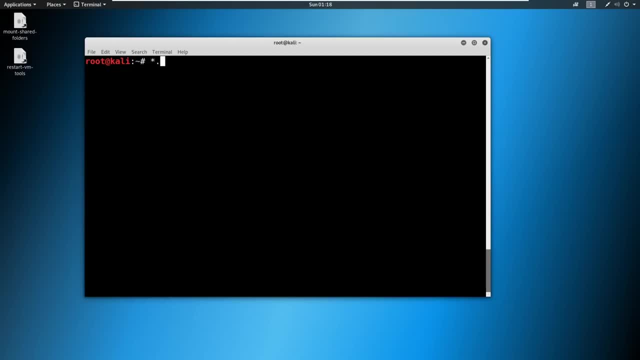 at Tesla. it had a scope of something like asterix teslacom. This asterix is a wild card. This means that anything and everything is open to us in the scope, except it was out of scope in the subdomain range. Now we can utilize tools to our advantage to discover these subdomains. Why are subdomains? 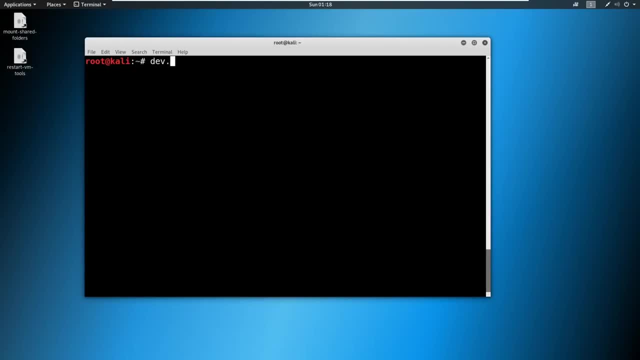 important. Well, we might run into something that is like a devteslacom, Or we might run into a website that should have never been out there, right like the dev or like test siteteslacom, for example, or you might find login forms. Another reason that it's so important is because 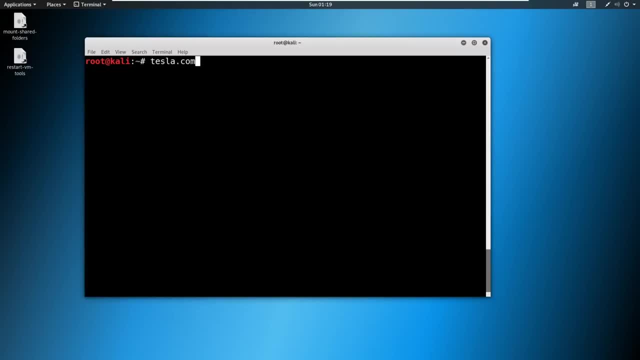 if you just look at the website, you're going to see that there's a lot of information out there. If you just look at teslacom, you're limiting yourself to one website, where there could be potentially tons of websites on these subdomains. So we really really need to hunt these and be 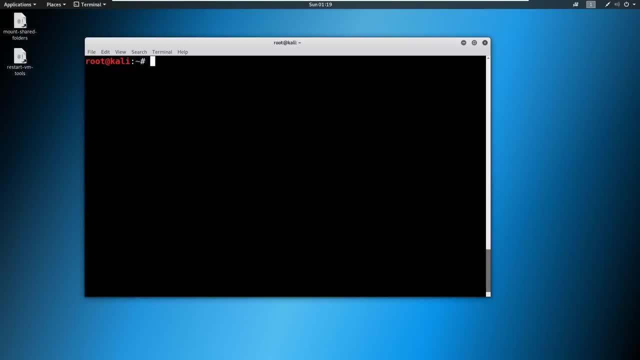 certain that we're incorporating everything that we can when we're doing our assessments. So one great tool that I want to point out is a tool called sublister. Now we need to install that. So let's type in apt- install sublister, like this: 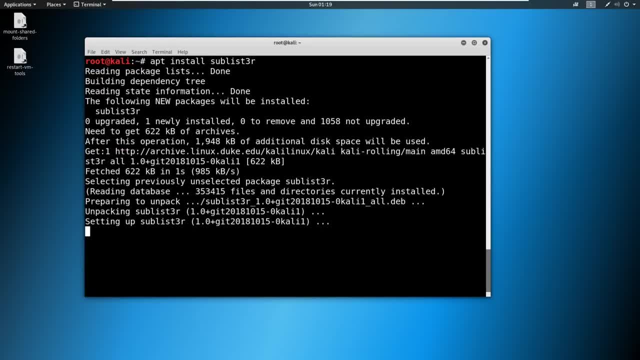 Okay, and this will just take a second to get it all set up, And we will utilize this tool to get these subdomains Okay. now that it's set up, all we have to do is type in sublister hit tab for. 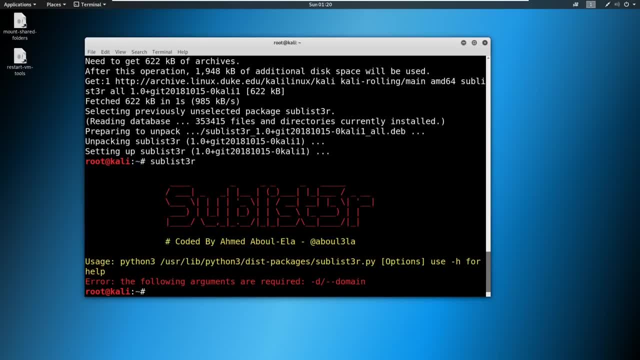 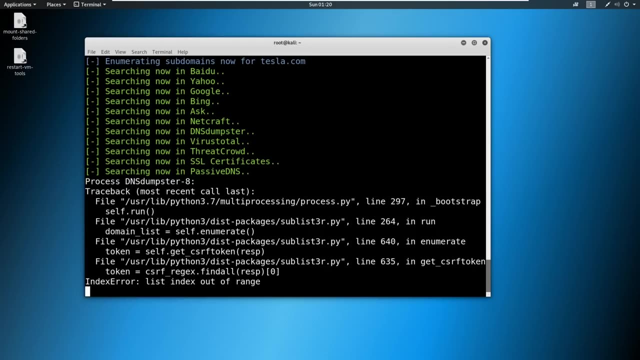 autocomplete. hit enter and it gives you the syntax. we can do a dash- dash h for help or dash h for help, And all we really need here is a domain. So we can say dash D for teslacom And it's going to start searching for teslacom And don't worry about this error if you get the 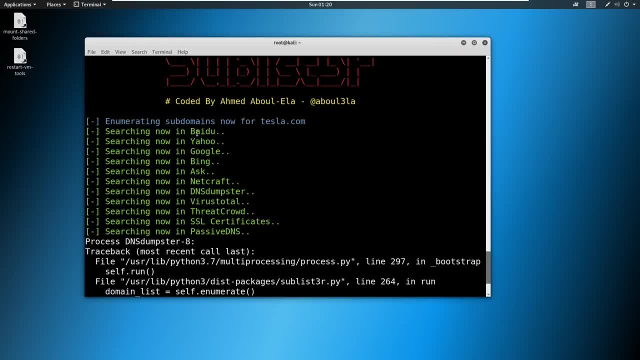 error. So it's looking through all these different search engines, similar to what the harvester was doing, But you're going to see that it's going to return quite a bit more. So we see Baidu, Yahoo, Google. it's going to go through all these and try to search Now while this is going on. 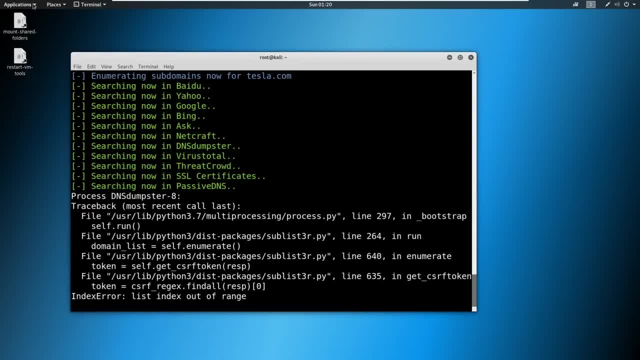 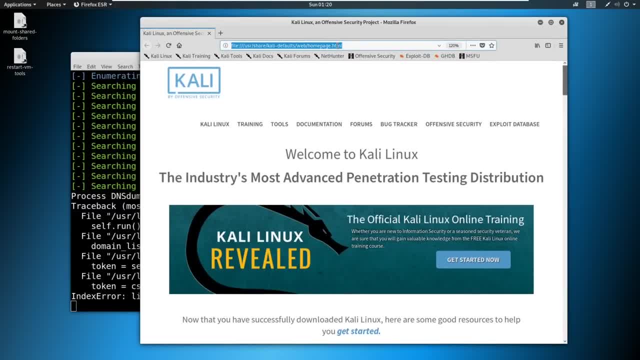 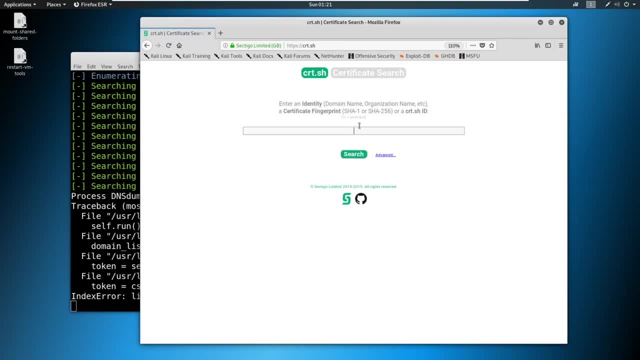 load up another site called crtsh. So we say crtsh like this. it'll load up a website like so: let me make this a little bigger for you, And we can do the wildcard ourselves. So you see, the percentage is a wildcard. So we're just going to say percentteslacom. Now what we're doing is: 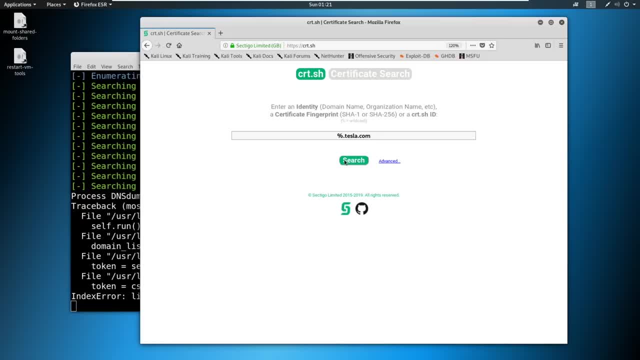 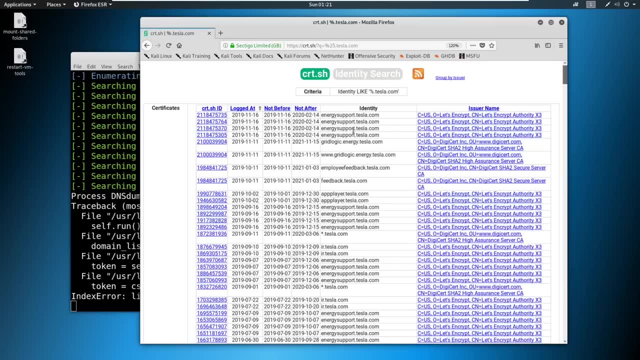 we're using certificate fingerprinting. Now we're going to go out and look for certificates that have been registered And it's going to attempt to find those and tell us what's out there. So you can see that we can find energy supportteslacom, grid logicenergyteslacom, And we would scroll through these and try to. 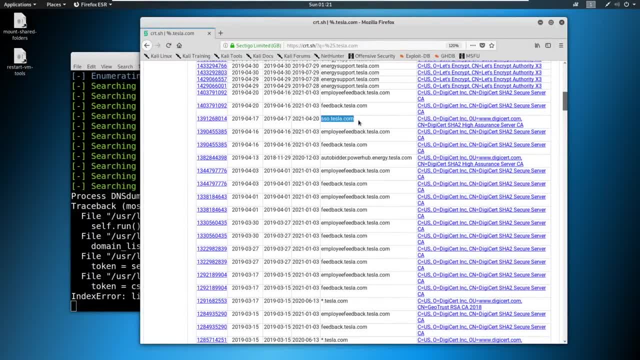 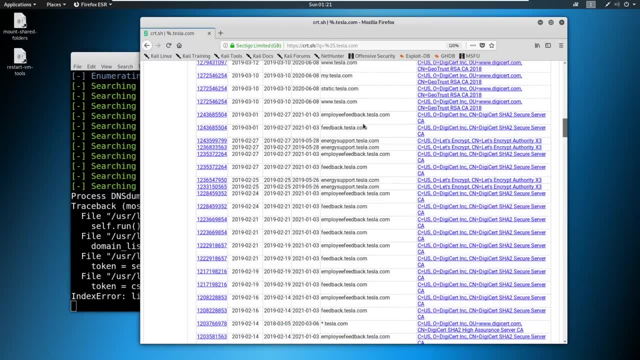 identify all the different ones, like SSO single sign on. That might be interesting If I could find anything in here that's like vpnteslacom or devteslacom, Any sort of thing like that. I'm also interested in it API tool. 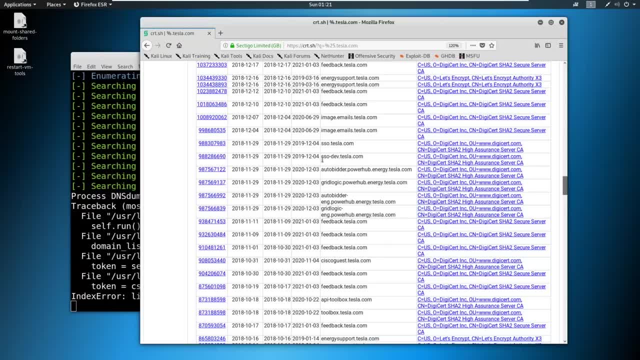 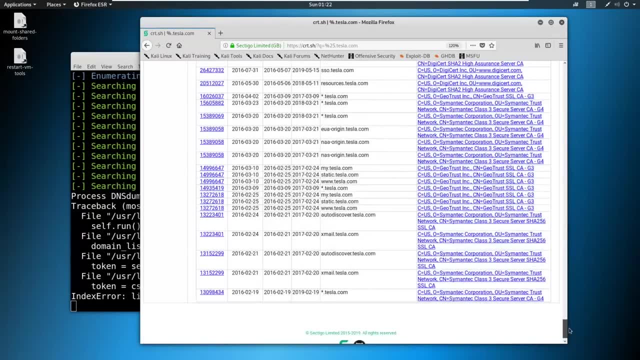 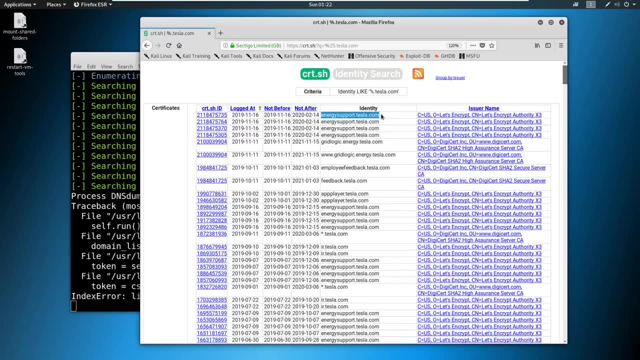 The blocks could very well be interesting: SSO, dash, devteslacom. So these are the sort of things that we're after And you see right now that we have different levels to domains, like here. you see that we have our sub domain, but what about a sub sub domain, like a fourth level of a domain? You? 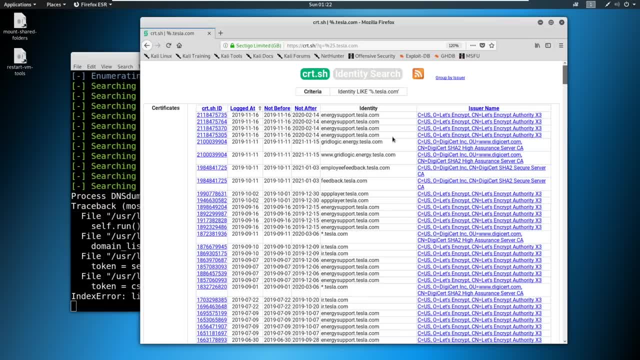 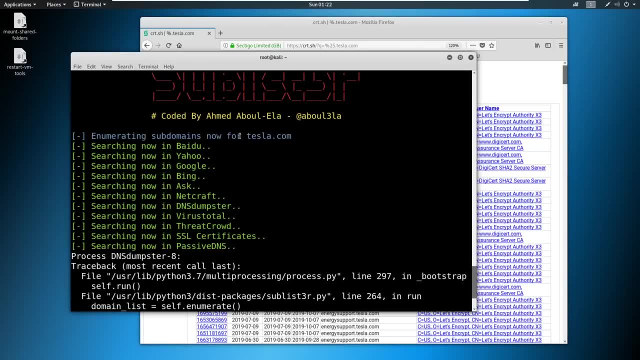 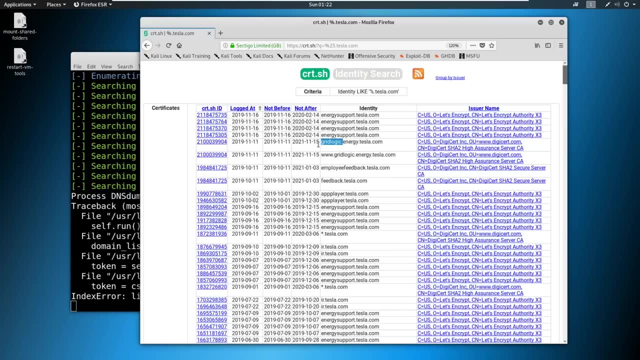 see grid logic, that energy, that teslacom, So we can go deeper and deeper when it comes to these domains. what sublister is going to be doing right now is it's going to try to find just the sub sub domain, so it's going to look for third levels. it would not discover this grid logic, dot energy at tesla. 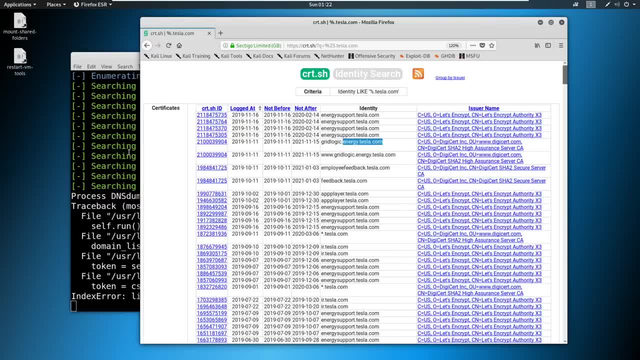 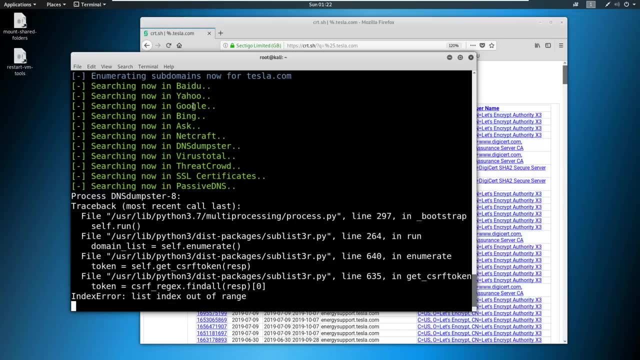 dot com without a little bit of finagling and looking through the help to figure out how to do that, so we can come to a site like crtsh to see if we could find any additional subdomains within this, and we can utilize tools like sublister as well. so i'm going to let this finish, but in the 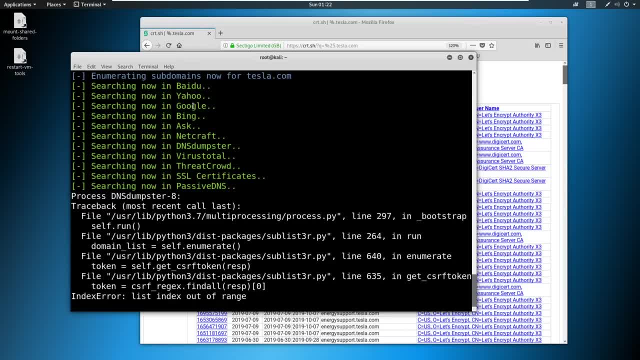 next video. what i'm going to show you is i'm going to show you how to improve upon this process with some tools that have been written in go that i think are fantastic. so i'm going to let this run. we're going to have part two of this video, where we actually review the results. 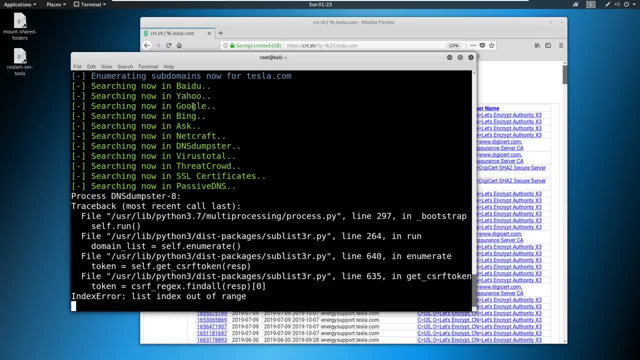 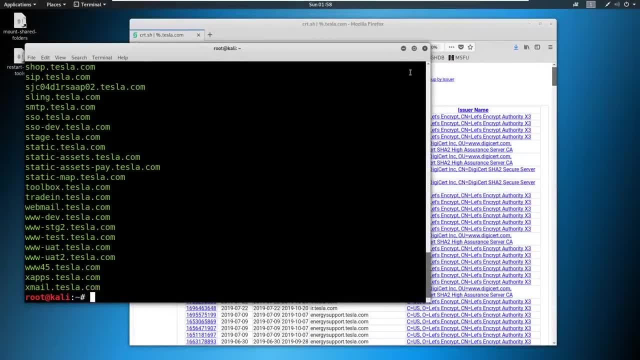 and then we'll go from there, so i will see you over in the next video. okay, so we have our results back in part one. we went pretty quick. part two: i want to talk about the results, what might be interesting here, and then identify some other tools that you can. 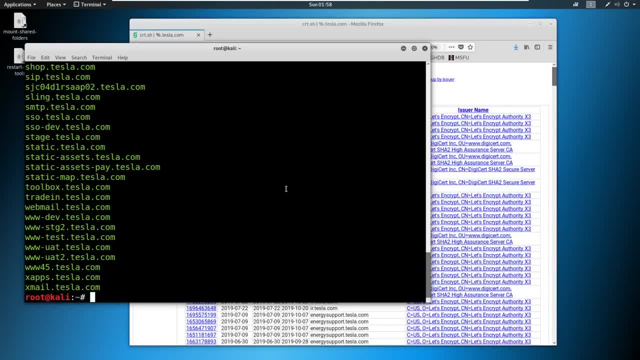 download and use and go play with on your own. so this has identified quite a few things. i mean, there's a big list here: 87 subdomains, and i lied to you when i said that it didn't get fourth levels. i thought there there used to be a recursive feature where you'd have to do a dash r to get those. now you don't. 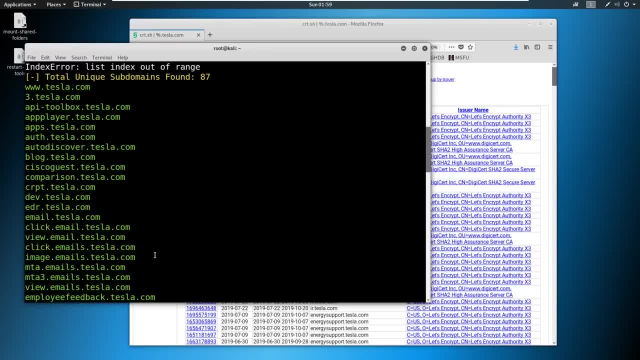 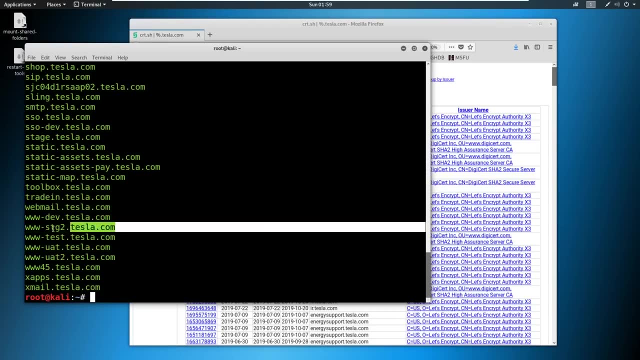 have to do that. it just picks up fourth levels for you now. sublister is great at finding some of these things, like, if we come through here, there is a devteslacom and i saw down towards the end that there was some staging staging two here a dev, here a test. these all look juicy sso. 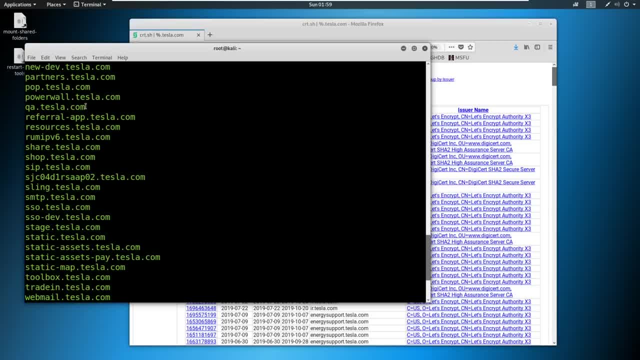 dash dev looks juicy. you might be after something like qa as well, or something like vpnteslacom. i want to know where your mail is at, so here's webmail, xmail, anything here. you could also look through these lists and possibly identify what kind of tools they're using. you might see something like linkteslacom. 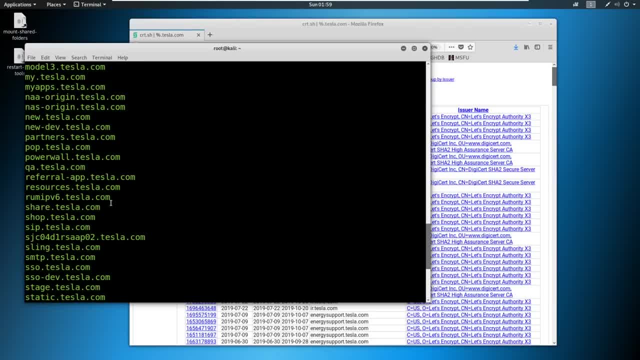 or zoomteslacom, and this really just kind of drives home what they're running on their back end for a lot of things. now, this isn't going to be a lot of work, but it's going to be a lot of work, but it's going to be a lot of work. but this isn't. the all-inclusive sublister is a great tool. 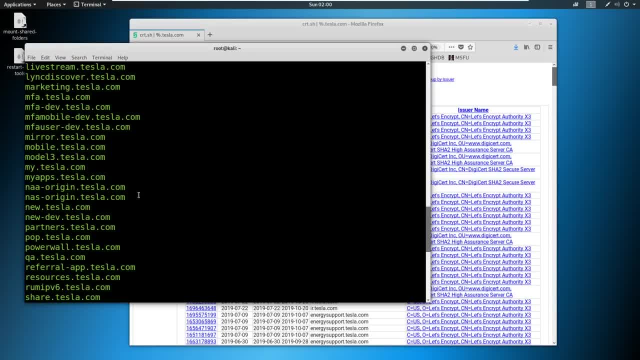 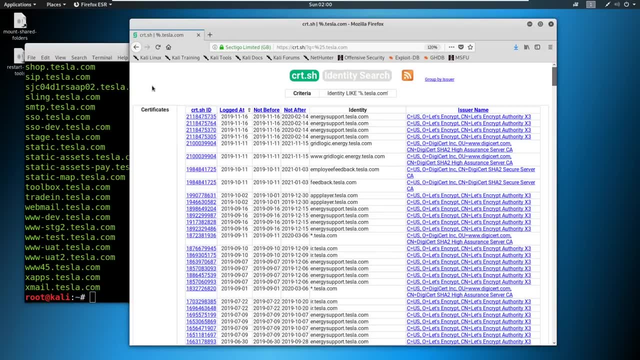 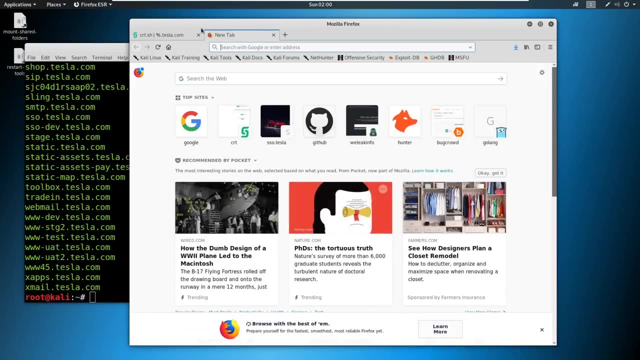 sublister was ahead of its time when it came out, but there are better tools out there. there are tools that incorporate pretty much everything in one go. so you might have certsh like this, you might have sublister included and the one tool that is really popular if you go out to google. 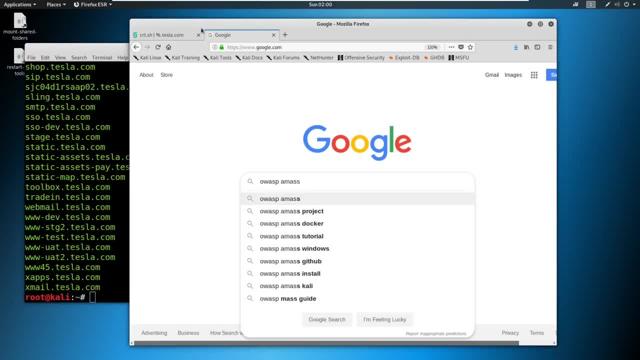 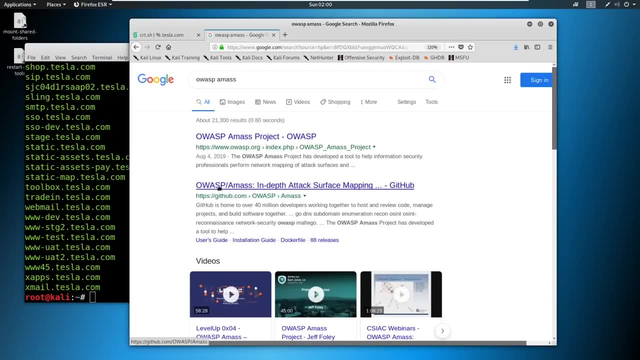 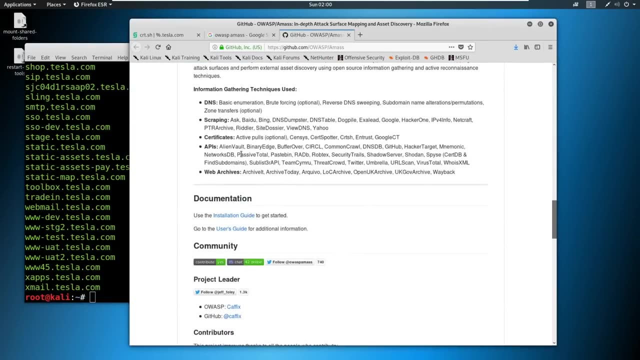 type in owasp amass, and this is the go-to tool for a lot of people doing bug bounty hunting. so if we click on the amass project here in github, you can download the project and install it per the installation instructions here. so you have an. 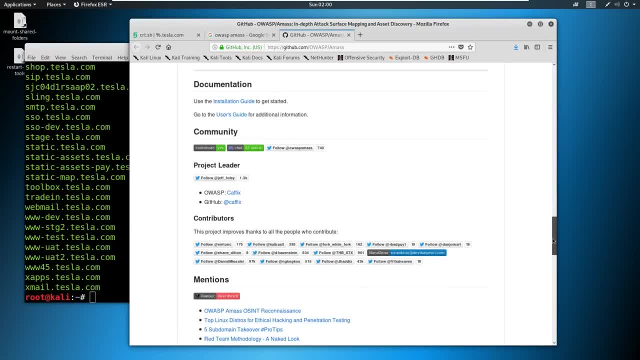 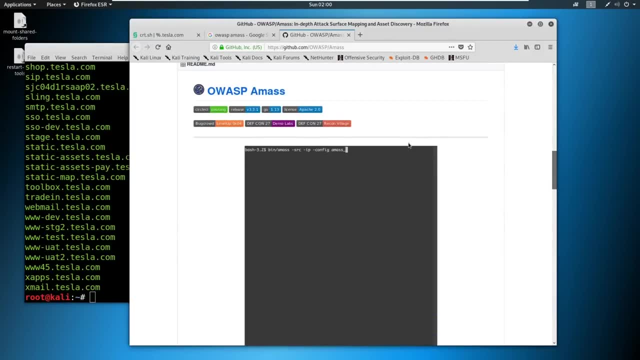 installation guide down the documentation. the reason i have chose not to show it in this series is because actually running amass takes a long time. but you can configure amass to do a lot of things and find a lot more subdomains. so my challenge to you is to get amass installed and 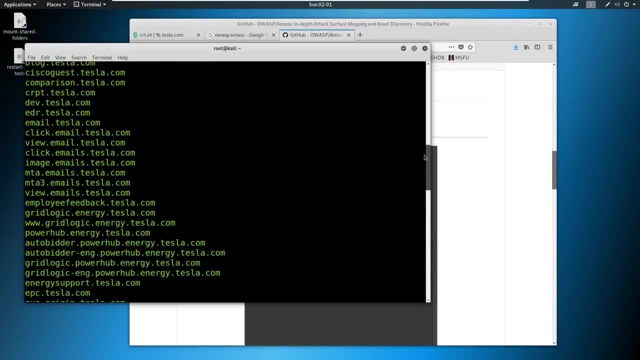 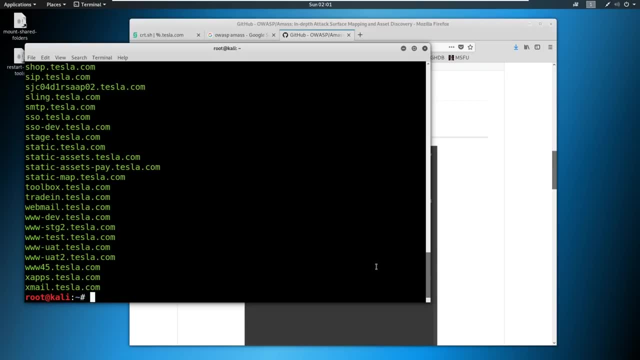 on top of that, see how many more subdomains than 87 can you find when you actually run it. so another last thing to point out is if you want to use sublister- and you were- you used it. it was really, really slow. it's always helpful to check the dash h on the help and you can see in here that there. 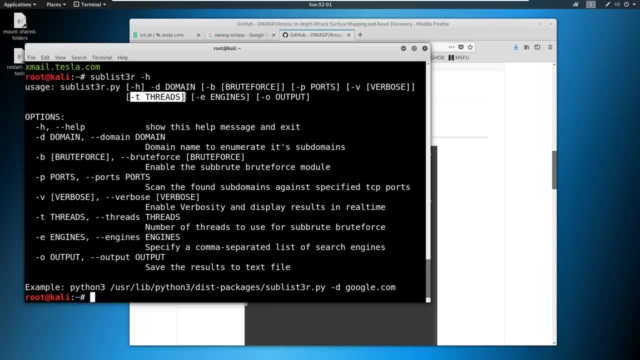 is a dash t for sub threads. always check the help So we can specify a domain like we did before. do something like dash D of teslacom, And then you can specify threads of like 100, as opposed to maybe one thread or 10 threads that was running originally. we give it 100 threads. it's going to go a lot. 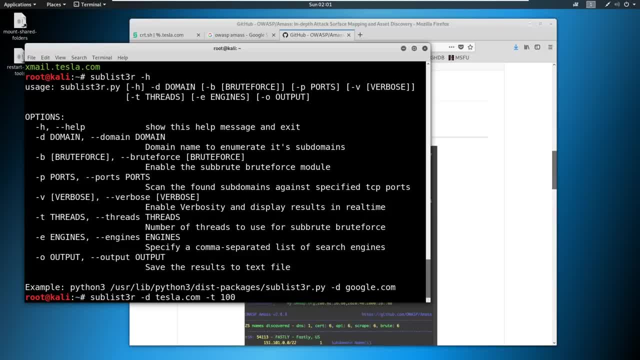 faster, we're going to get a lot more results. You could also do a dash V for verbosity here and get your results in real time if you're impatient or you're trying to go out to the web. So there are great tools out there for doing subdomain hunting And again subdomain hunting. 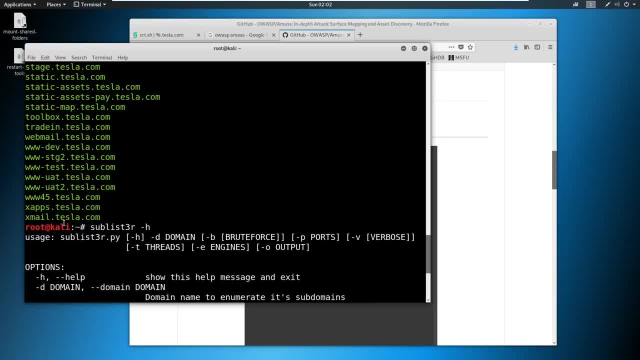 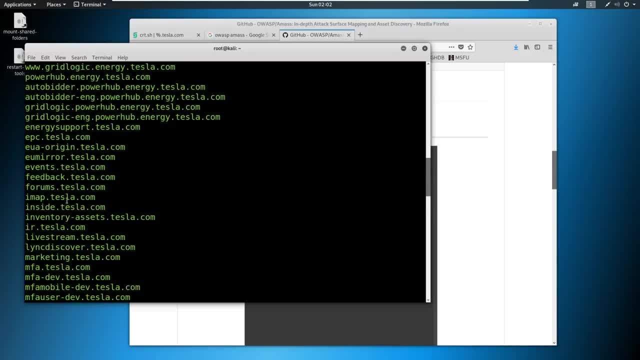 is very, very critical, Because if we just limited ourself to teslacom, look at all the things that we would miss. So we can find out a lot here. Now, not all of these pages are going to be alive. Also, there's a good possibility that we can go to something like this mfadev or dash dev. 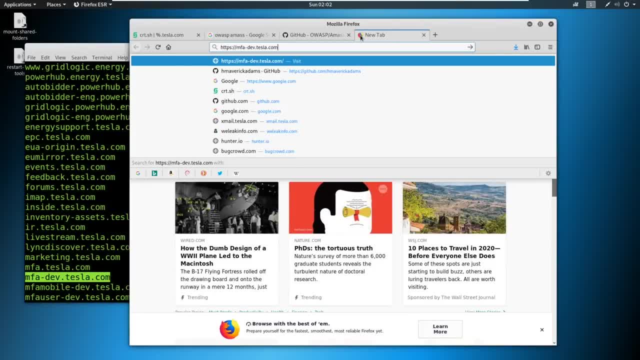 dot teslacom, And then it won't work. we can give it a go, And so we're going to go to this mfadev or dash dev dot teslacom, And then it won't work. we can see, like, not always do these work. These are what show up in search engines, But it's worth. 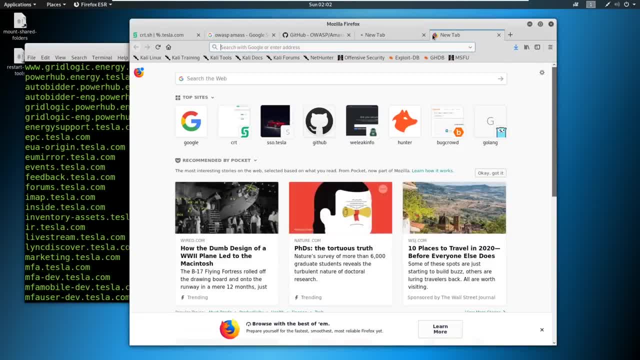 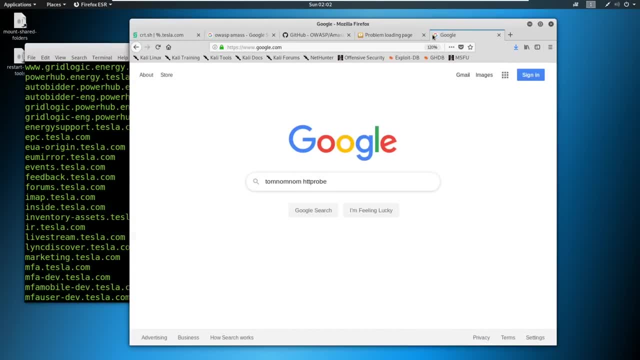 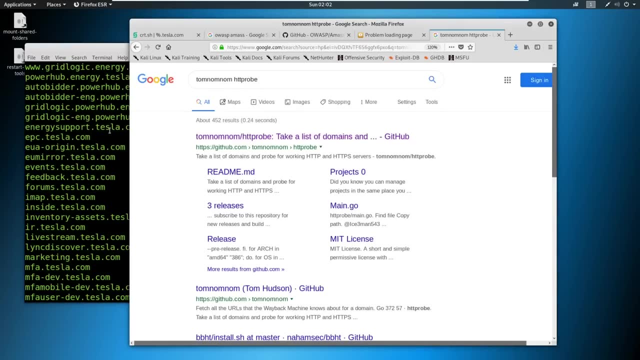 knowing about them. And there are other tools out there, such as like: go to Google, such as Tom nom noms HTTP probe like this, tools like that out there that will probe the list that you give it and give it this list into the probe. it'll say, hey, this website's alive or this website's. 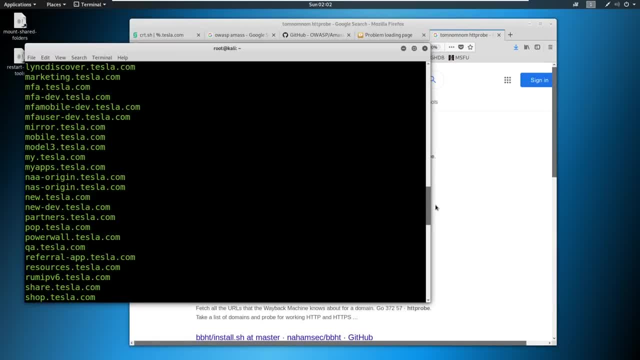 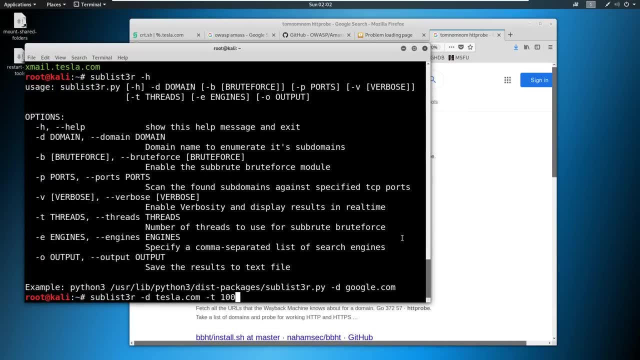 not alive, And then you can start narrowing down these lists as well. So that is something to think about when you get your wheels spinning. But for now, for information gathering and for the scope of this course, we don't have to worry about it too much, But I do. 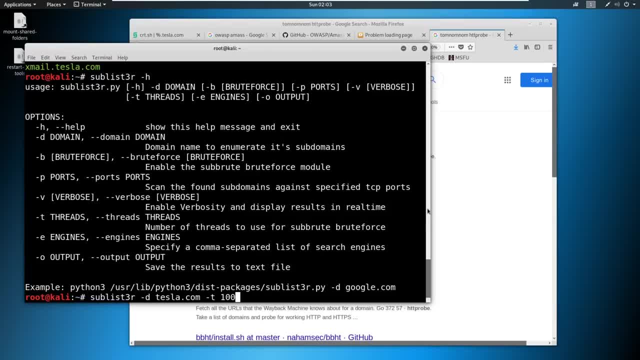 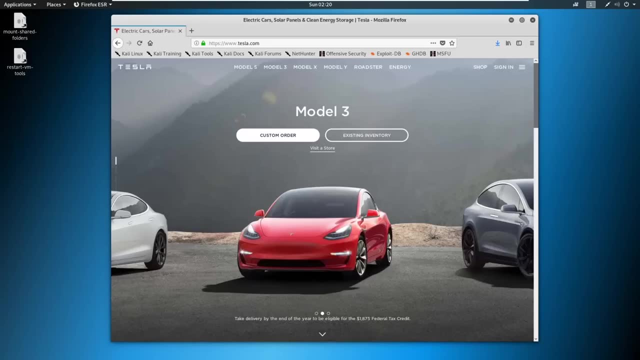 want to point out some other alternatives and ways to do subdomain hunting and then what to look for in subdomain hunting. So that is it for this video. I'm going to catch you over in the next one. Now, the next few videos have to deal with the subdomain hunting, So I'm going to catch you over. 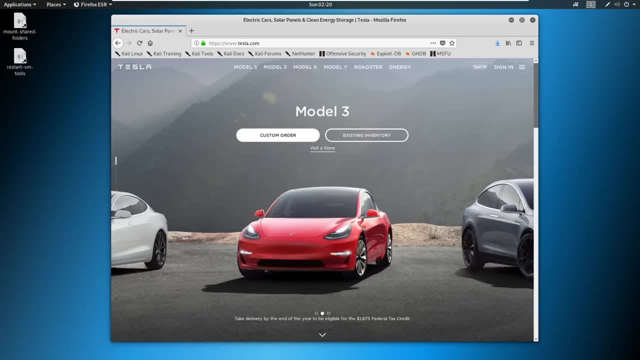 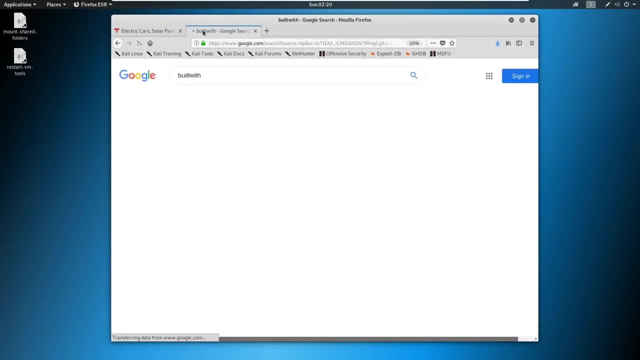 with web apps as well. But instead of looking at subdomains, we're going to look at what a website is built with, And that's a good indicator here of built with. so let's go out to Google And we're going to just search built with And we're going to go right to built withcom And let's take a 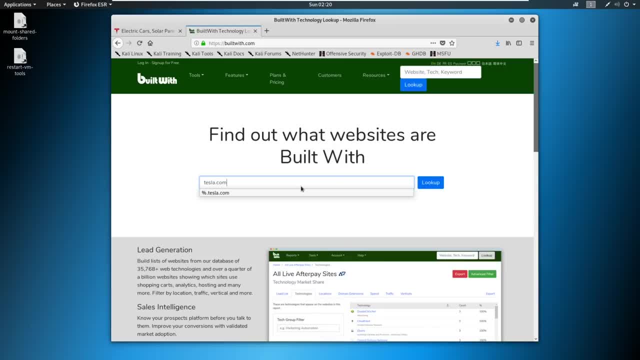 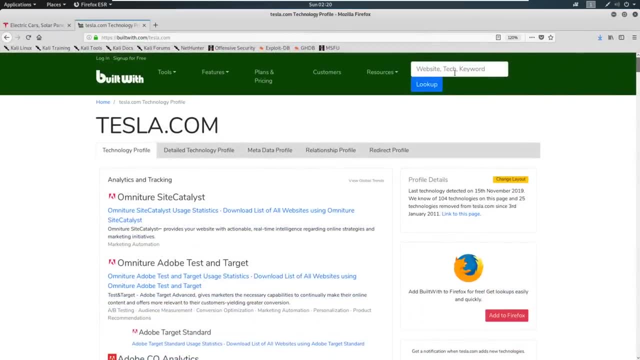 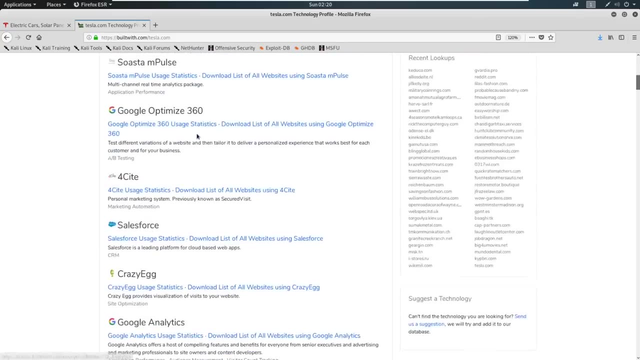 look at what this does. So let's just search teslacom, For example. we'll do a lookup And I'm going to make this a little bit bigger so you can read it. And what this does is: this goes out and it looks at what type of tech Tesla is running. Now it gives all this stuff that it can. 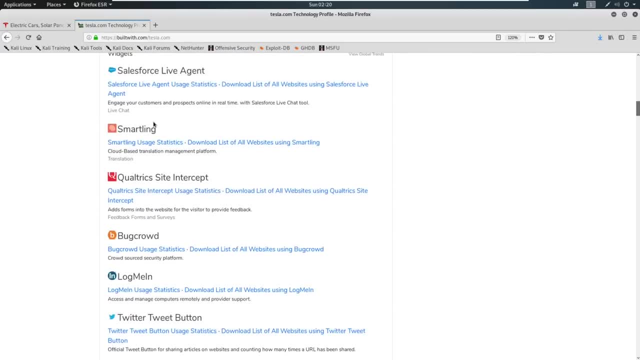 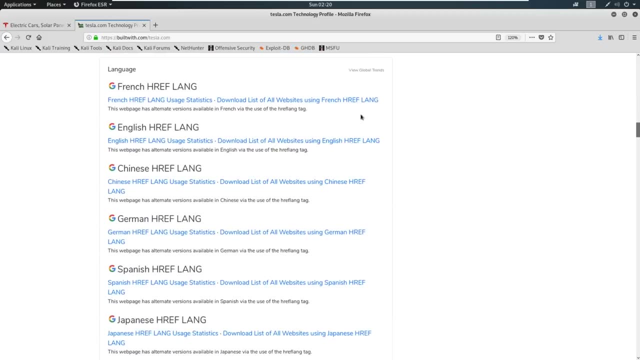 see Google Analytics Salesforce. that's great, But it also tells us the widgets that are running. you can see it is part of bug crowd log me in Twitter. Okay, it's got these language things here, But what we're really after is what kind of frameworks it might be running on. So 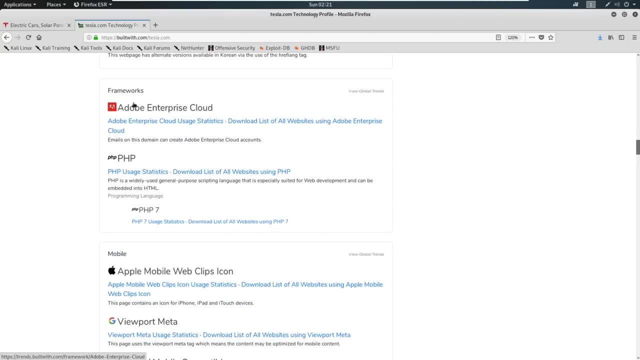 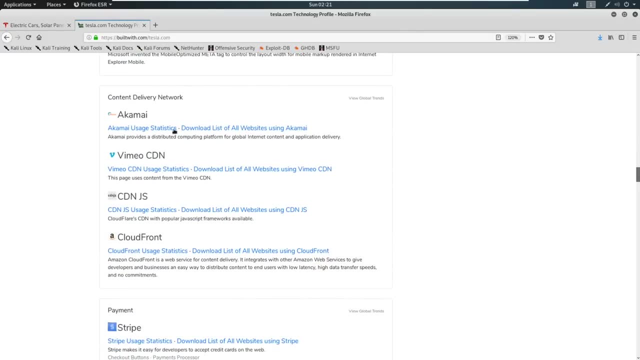 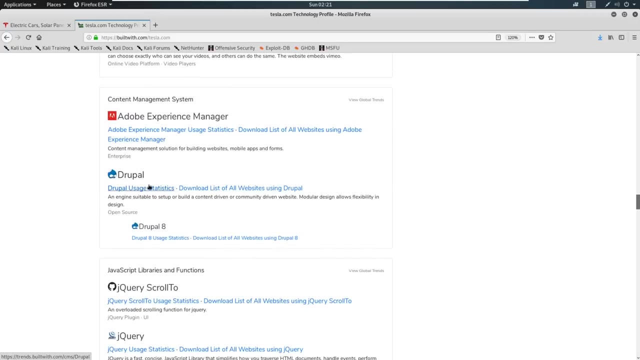 it says here that it's running on PHP. It has Adobe Enterprise Cloud- Okay, that's interesting. It's got CDN, the content delivery network, Interesting. It utilizes Stripe. Okay, we can scroll through. this looks like it might be written in Drupal. That's an indicator there. 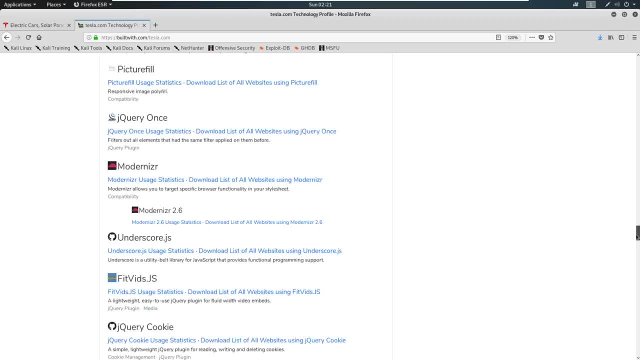 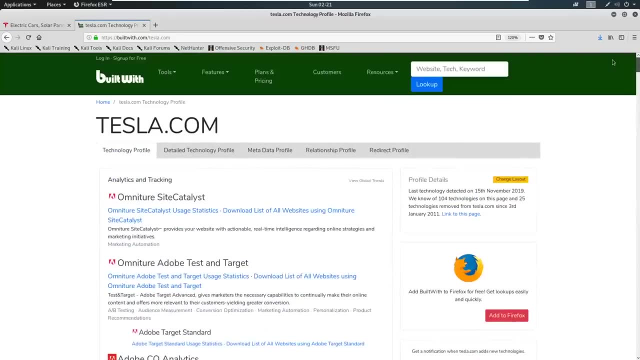 And this is a big website, So it's got a lot. look at all the information here And it might be a lot to track down. So with this, with a big website like this, there's a better way. I think now built with is a great. 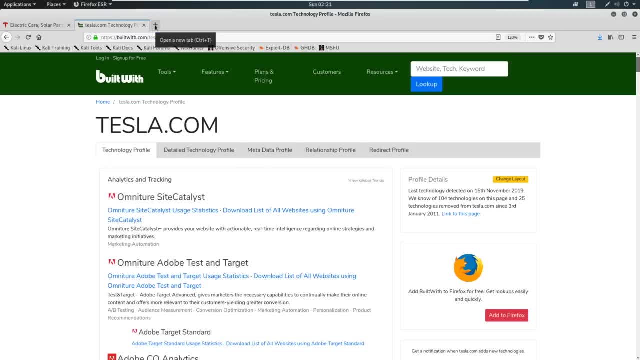 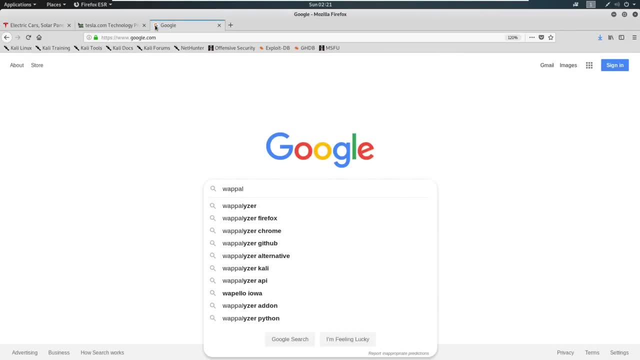 great resource, But I think there's some other stuff out there that might help us a little bit better. So let's go out to Google as well And let's search for a tool called WAP Elisir, just like this, And we're going to use it for Firefox, So it should pull this up here. 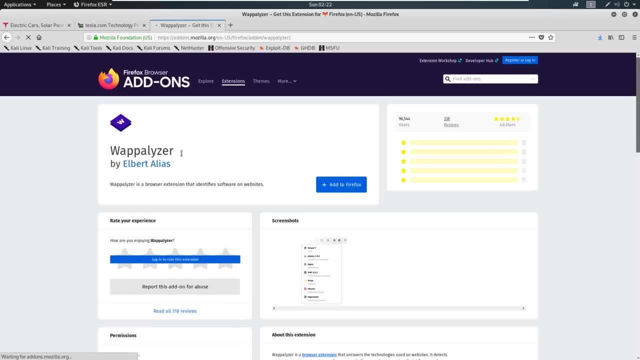 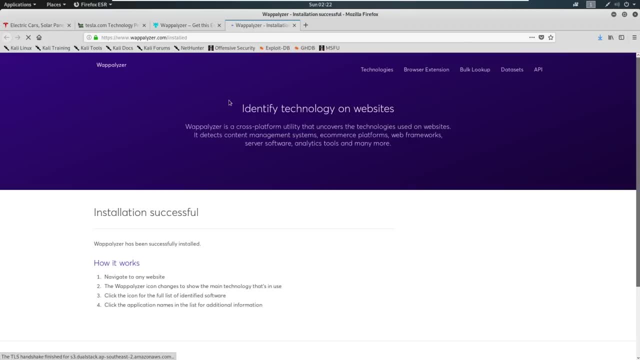 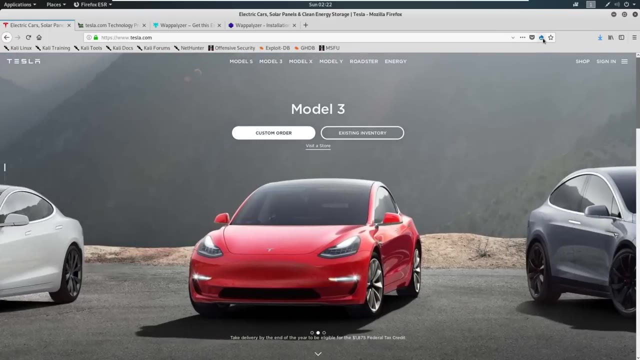 And we'll click on the first one And go ahead and just select Add to Firefox, Select Add, And now it will appear. So now we have WAP Elisir, Let's go back to Tesla. And you see this little guy here in the corner. we're going to click on this. 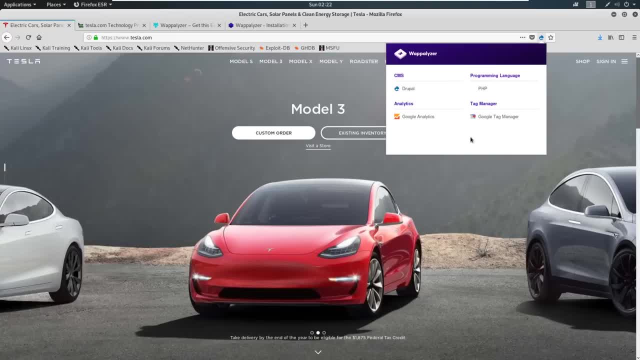 we're going to accept it, And now we get a little bit of information as to what's going on. Not as much information as built with, but I actually like WAP Elisir a lot more, because it kind of just gives you an indication right away with what's going on. Now WAP Elisir is more of an 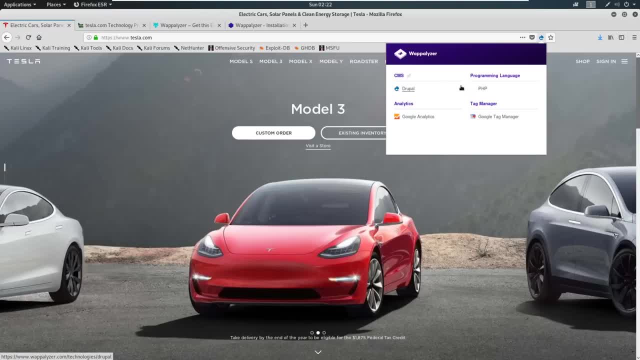 active type of reconnaissance. I only say that and I don't necessarily believe it, But it's because we do have to interact with the website Now. we're not doing any type of scanning, we're just going out to the website like a normal user would, And to me it's still kind of passive because we're 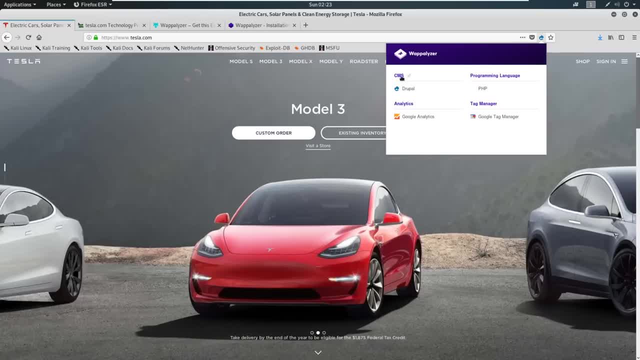 not doing anything that would be out of the norm. So here we can see the content management system is running on Drupal. we can see the programming language is running PHP. those are both identified with built with as well. So we can see that we have a lot of content management system running on. 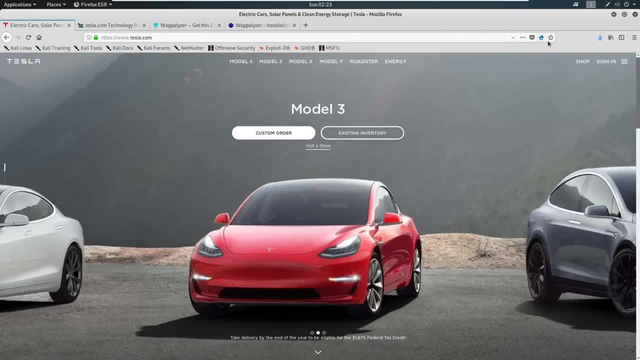 Drupal. Now why is this important to, you're telling me? Well, it's important because if we know that's running with PHP or Drupal, there might be a vulnerability within those. A lot of times when we have this, let's see. if we go to this website, you can see PHP is running. we get 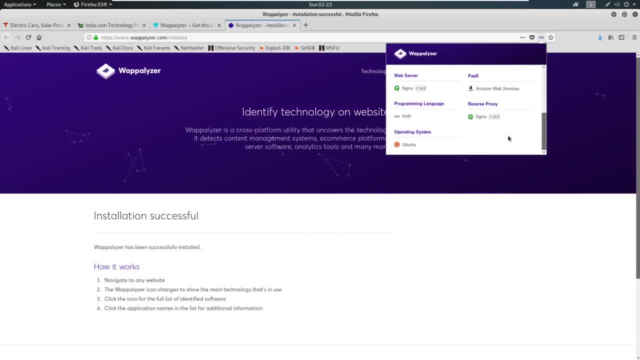 a lot of things and we get version numbers. So look at the WAP Elisir website. you see that it's running on an operating system, Ubuntu. it's got a programming language of PHP. the web server is Nginx with 1.14.0 version number. Okay, it can tell that it's running on Amazon Web Services. 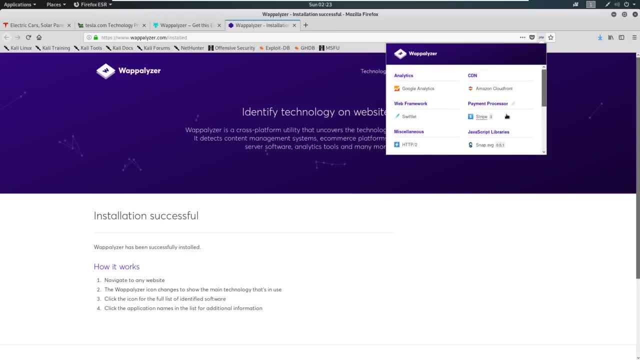 as a platform. It's got all kinds of information here. It's got the payment processing, it's running Google Analytics, So see the type of information that can come through A lot of times. you'll see things like jQuery and other type of libraries here, and the version numbers as well. Now you 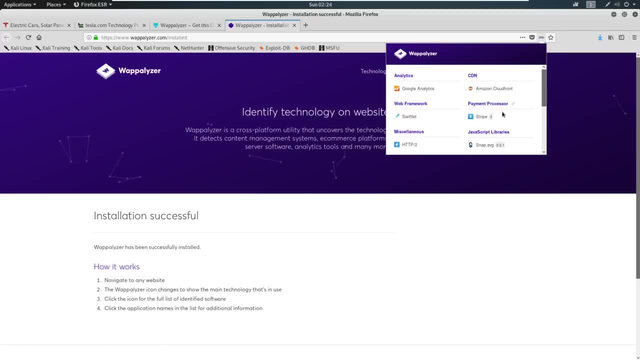 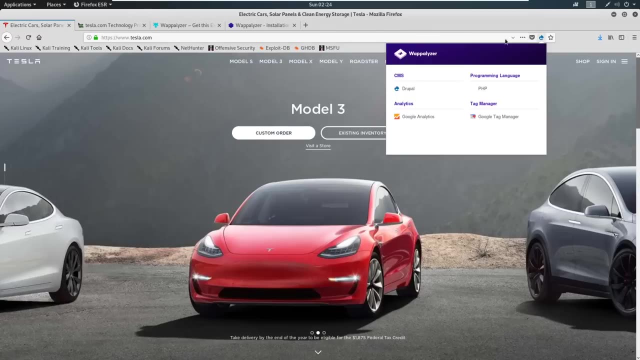 take those version numbers and you do enumeration on them And you try to find any type of vulnerabilities that might happen there. And the more information that we can gather on a client on a website, whatever it is, the better off we are. So when we're gathering information on Tesla, 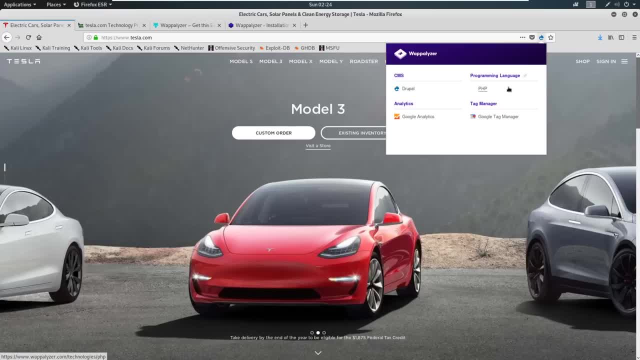 okay, now we know the content management system is written in Drupal, the programming language PHP. is that going to lead to an exploit? Maybe, but you don't know where it's going to come up in the future. So this type of information gathering is great. Now one more thing that we can use. we've 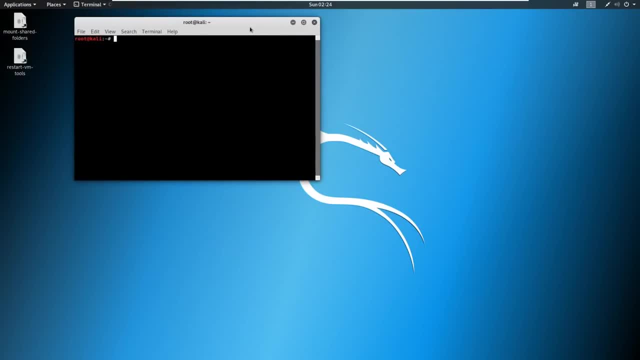 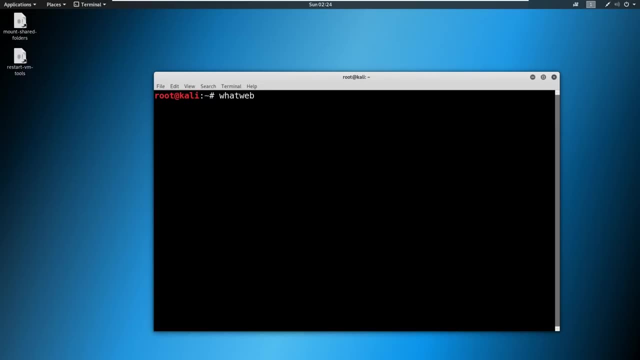 got something built into our machine. Let's go out to the terminal And we can take a look at it. So we've got a tool called what web, just like this, and hit enter on it And if we look at the syntax, all we need is to specify a. 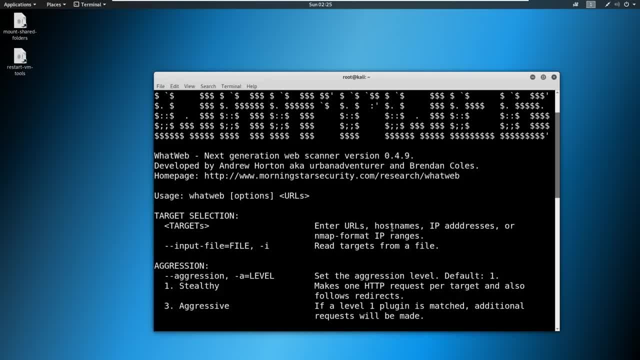 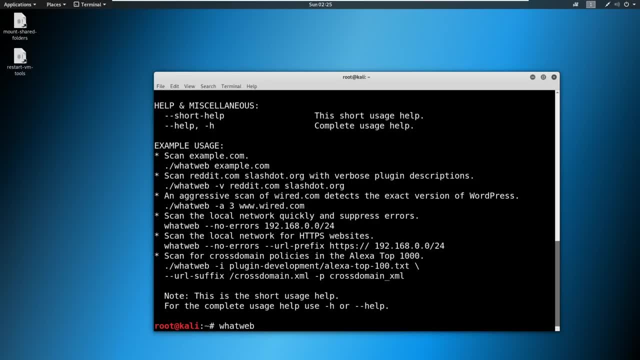 target. So we enter the URL, hostname, IP address or nmap format, So we just say what web URL. So let's give it a go. We'll say what web And we'll just say HTTPS- Tesla dot com. 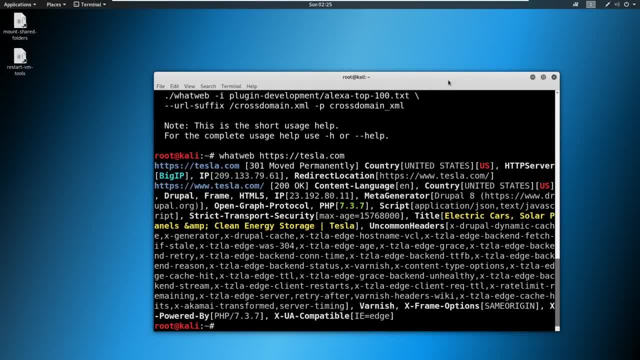 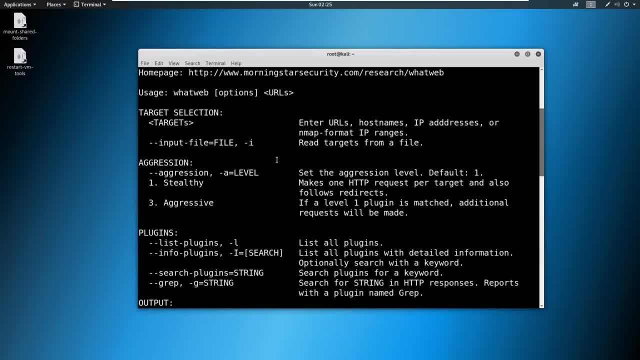 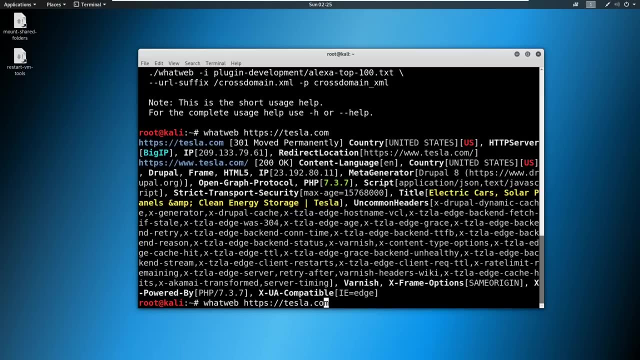 And it is a redirect, So it might not pull down everything for us here. So it did pull down an IP address. it gave us a redirect. I don't know if there is a follow redirection option here, But what we'll do is we will just say something instead. we'll say, like teslacom instead of 443 and see if. 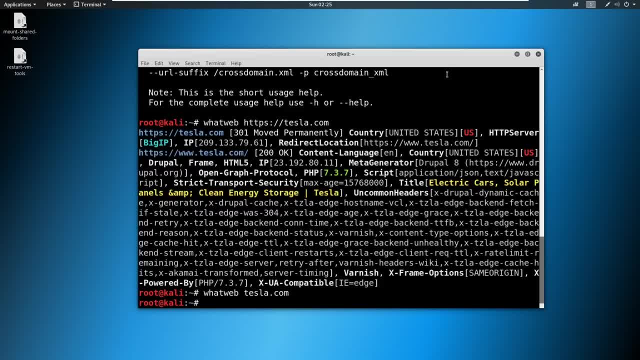 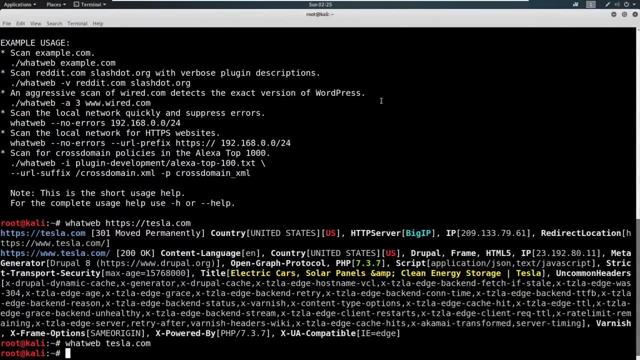 that does anything different, And it didn't. So it does give us some information in here. It's not as pretty of a layout, but it is a tool that is built in to Kali Linux for us. So, look, we can pull down Drupal eight. we didn't know. 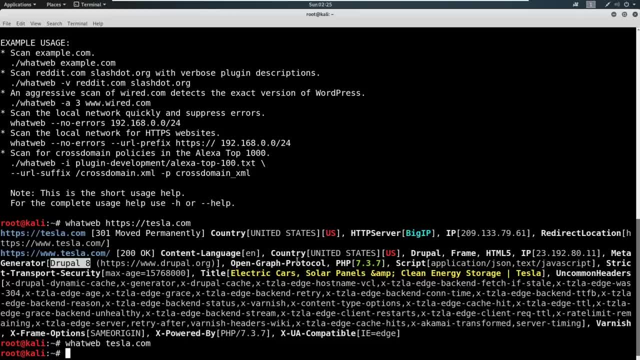 what kind of Drupal was running on. Now we know it's Drupal eight. we see that it's running PHP 7.3.7.. That's identification two that we didn't have previously. So using more tools to our advantage gives us more information. 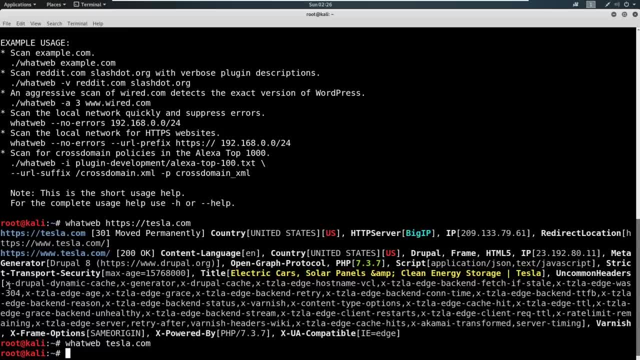 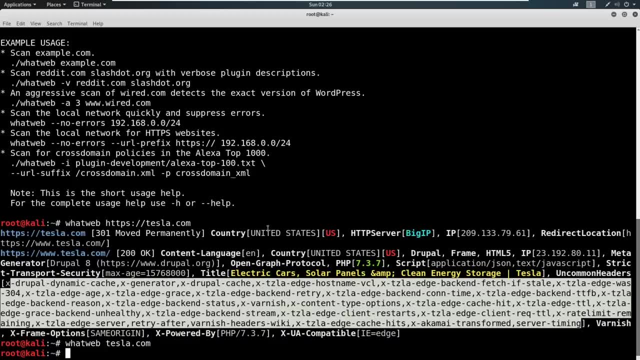 And we can pull down the headers that it has here, And you see, they have different types of headers, which we're not going to get into this quite yet. When we get into the web app portion of this, we'll talk more about headers, But this is just yet another thing that we need to look at And we 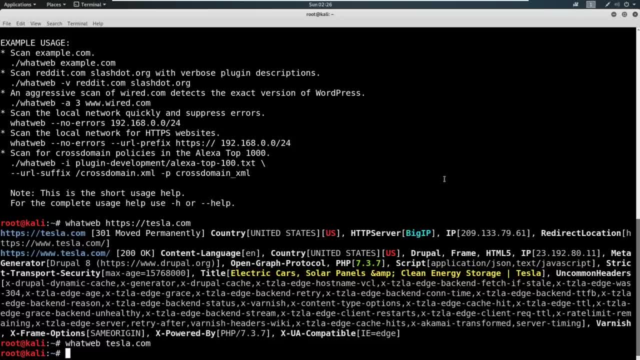 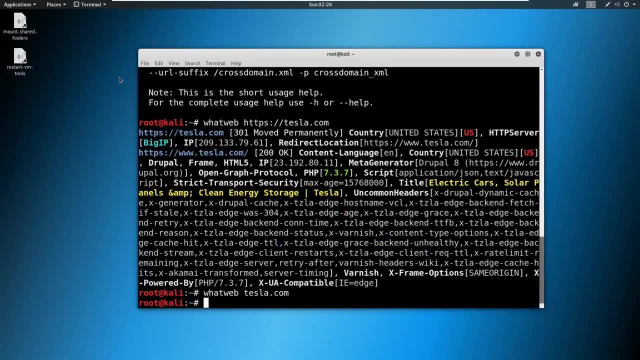 pull down the IP address as well. So a little bit more information that we can gather here and just keep going from this. So that is it: utilize the resources around you to gather information. we could utilize Resources that go out and scan a specific web page. like this: we can go and utilize a resource such as: 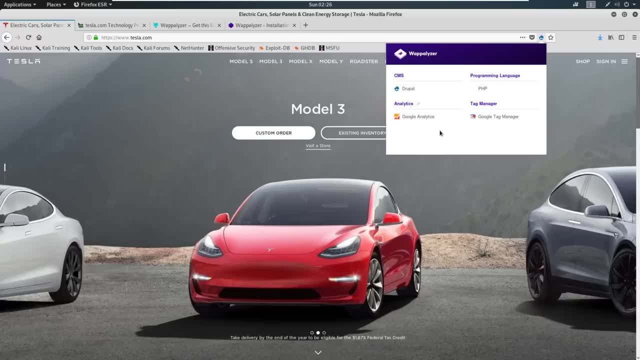 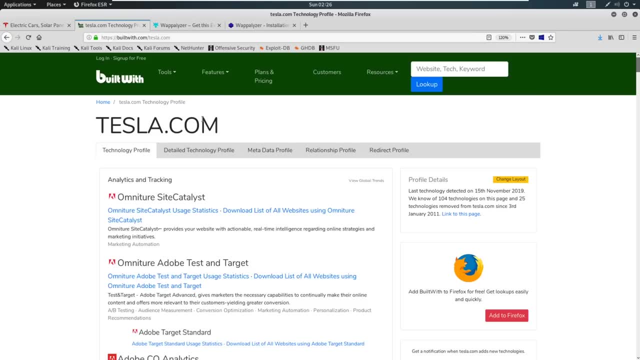 wapalizer that you just visit the web page and you can see what's running on there, or a website like builtwithcom, where we just don't even navigate to the website, we just type it in and it does all the. 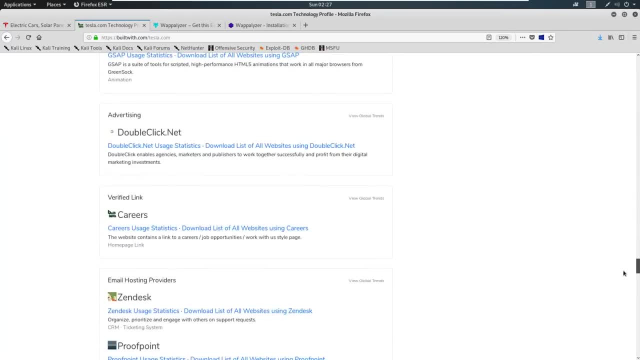 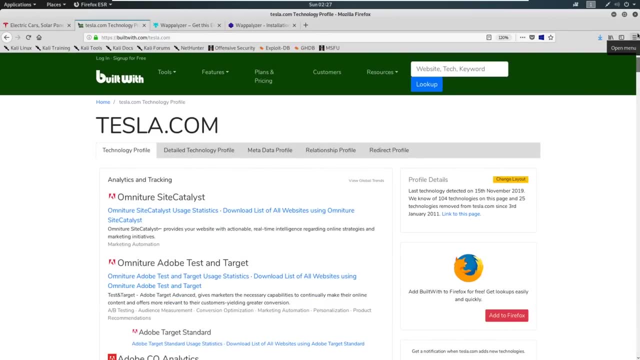 work for us And we can pull down all this information, which is by far the most information out of these three tools. So utilize all the resources available to you And you will have much advantages when it comes to pen testing and your enumeration skills. So that's it for this video. 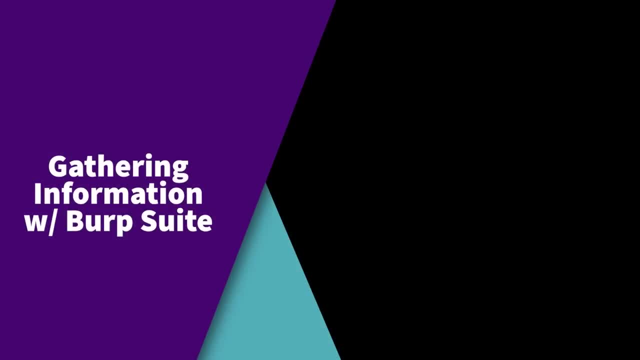 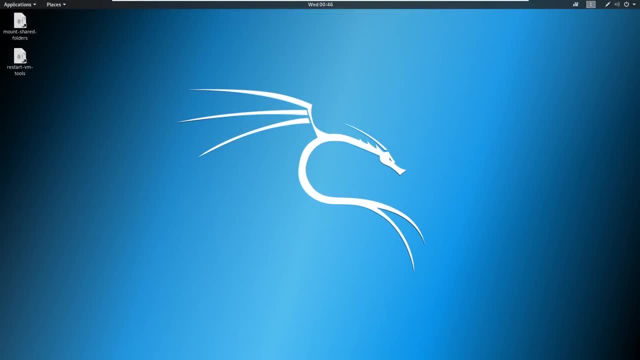 I'll catch you over in the next one. Another useful tool when it comes to web applications is a tool called burp suite. Now, let's go ahead and open up burp suite. So we're going to go up to the applications. 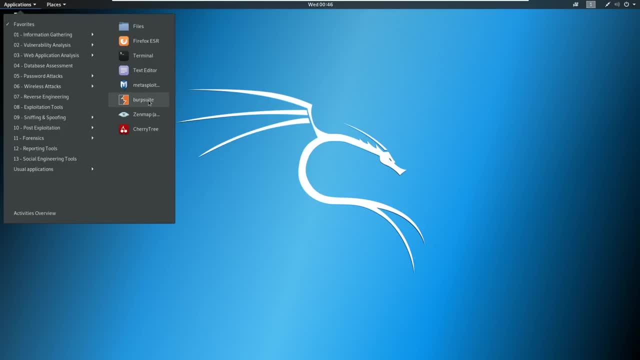 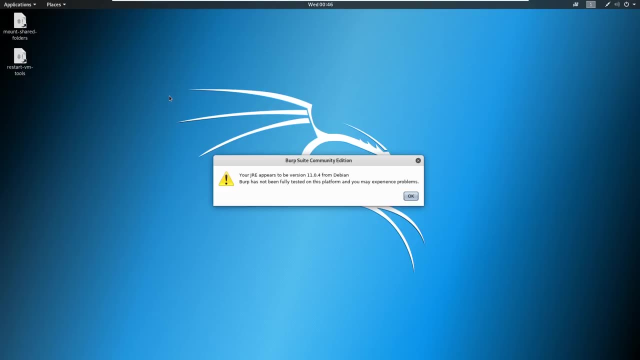 and in your favorites should exist burp suite here Now, burp suite is what we call a web proxy. Now, web proxy means that it has the capability of intercepting traffic for us, and we're going to see what that looks like. So you're probably going to get this error about this. 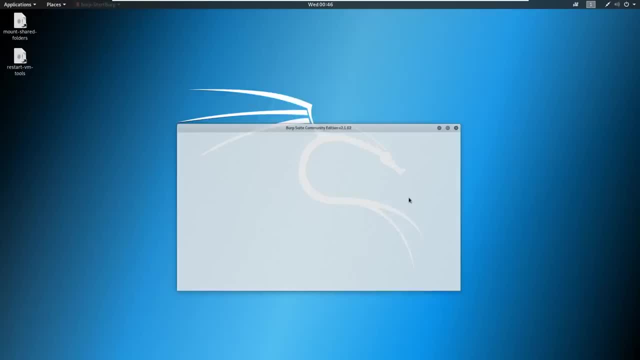 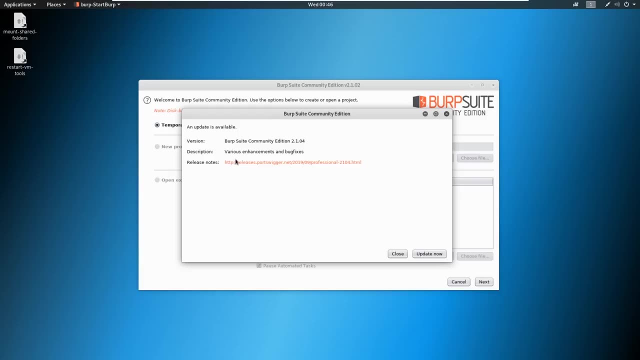 Jerry, don't worry about it. We're just going to say, Okay, you might get a. you need to accept this license agreement. when you first start, go ahead and accept that as well, And if you see an update screen, go ahead and just close. So we are on the community edition, So we will have a limited 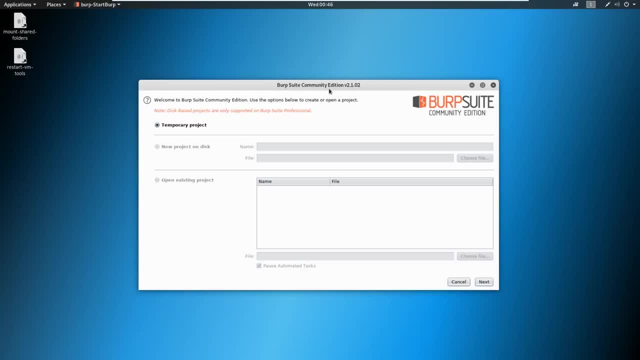 features. We'll talk more about those when we get to the web application section, but I just want to introduce you to what Burp Suite can do in a very basic form and how we can actually gather some information out of a website from Burp Suite pretty easily. So let's go ahead and just select. 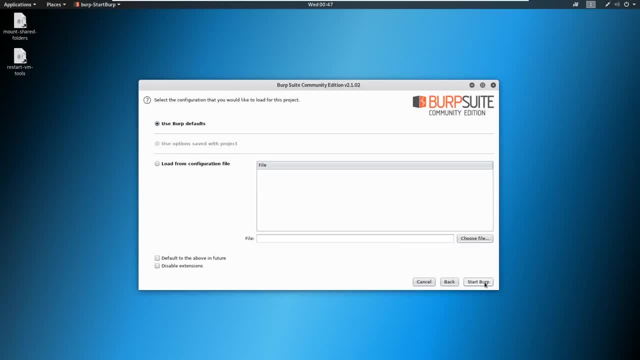 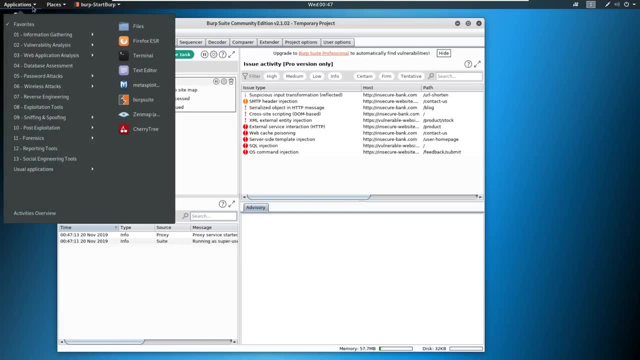 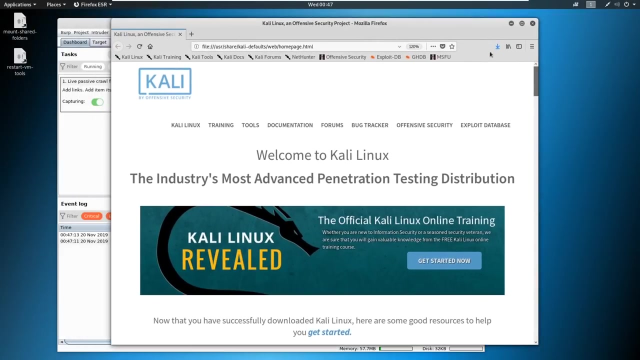 temporary project and click next and then select: start Burp. Now the first thing that we're going to do is we're going to set up our Firefox for utilizing Burp Suite. So go ahead and go to favorites in Firefox, and I want you to go over to the right hand, little hamburger here. 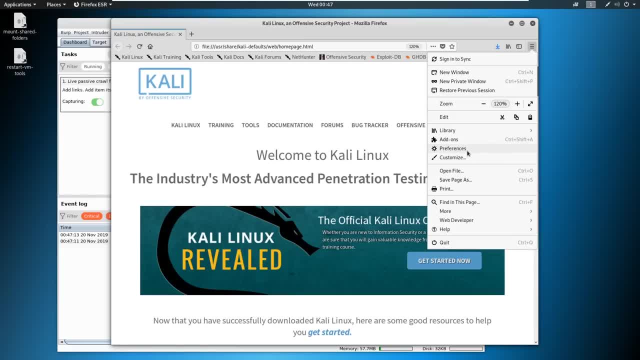 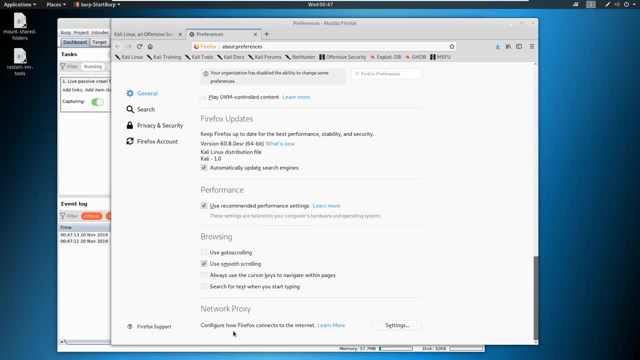 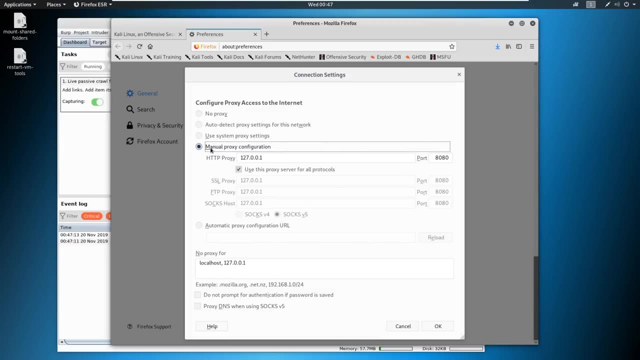 and you're going to go and select preferences. From preferences. we're going to scroll down all the way to the bottom and we're going to select settings. Now we're going to select this manual proxy configuration here and we're going to say 127.0.0.1.. 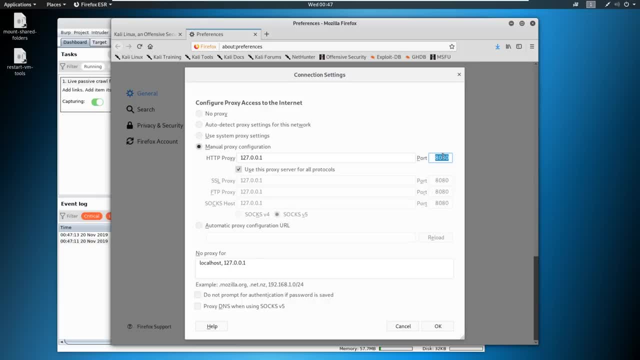 On port 8080.. Later, when we get to the web application section, I'll show you a much easier way of doing this with a tool called Foxy Proxy, But for right now this is a very high level overview. So go ahead and use this proxy server for all protocols, and that should fill in the 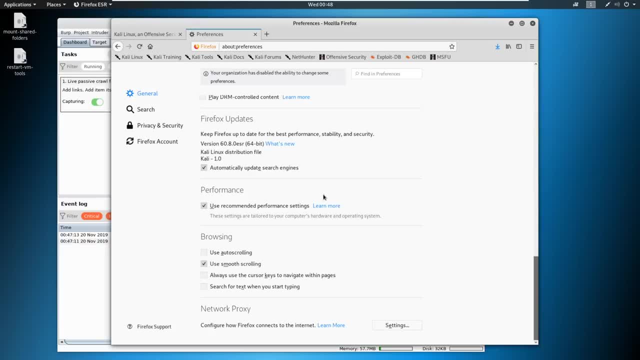 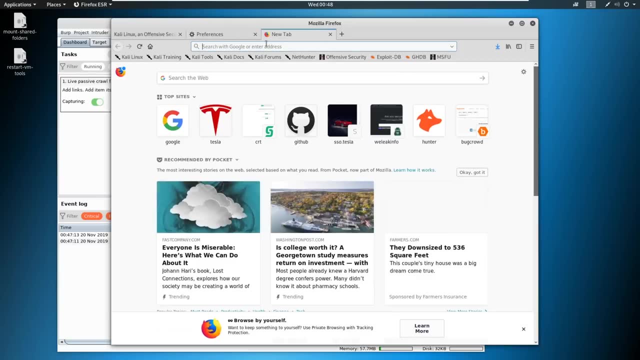 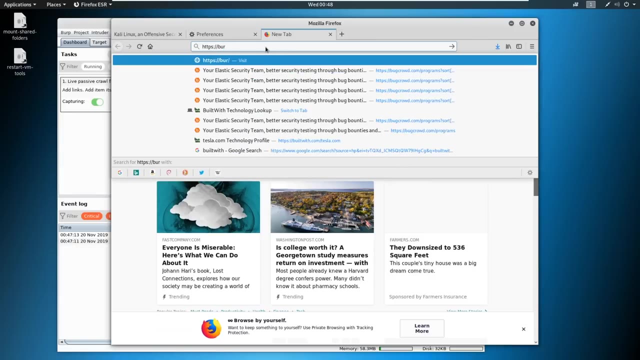 rest down here. We're going to go ahead and hit OK And we're going to leave this open. I'll show you why in a second. So I also want you to go to a new tab and I want you to go To HTTPS double dot, slash, slash, burp like this. Now, your first page might not show up like this. 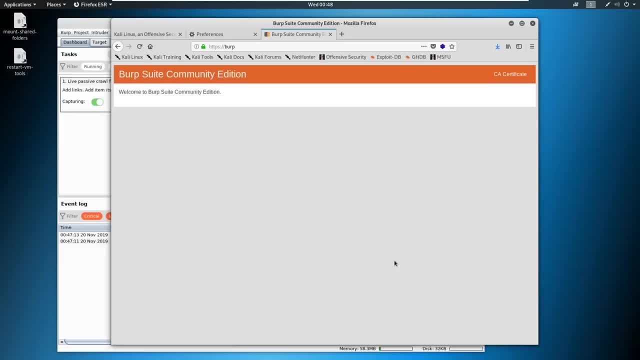 It might show up with a: you need to accept this certificate. You're just going to say allow. down at the bottom and say yes, permanently, store this exception. And then you'll be brought to a screen somewhat like this: So what you're going to do is you're going to go ahead and just click on. 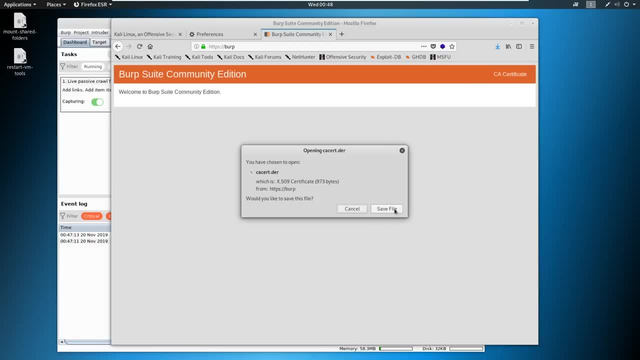 CA certificate here and then save the file. Mine is already saved, as you can see in my downloads right here. So what I'm going to do is we're going to go back into preferences once we have that saved And we're going to go to privacy. 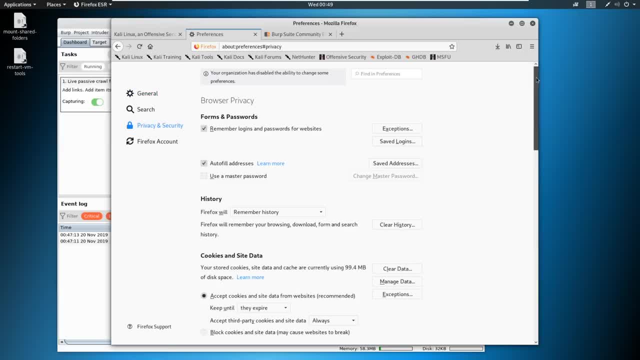 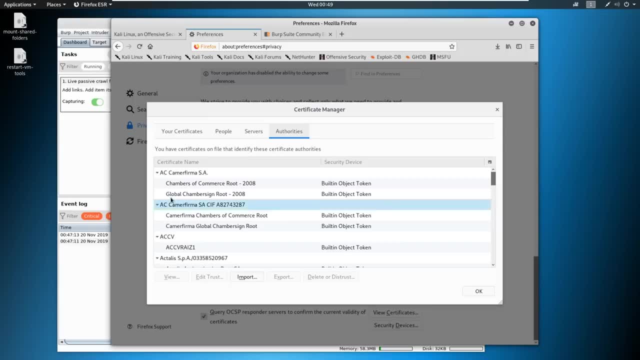 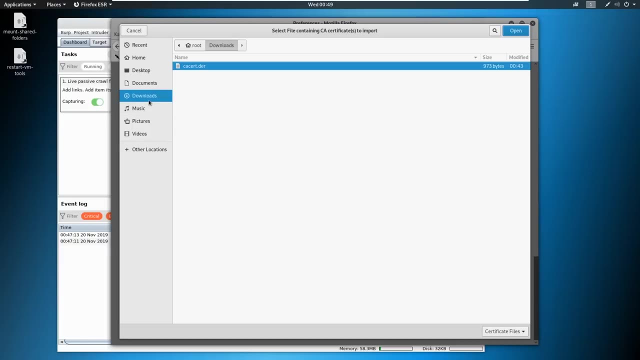 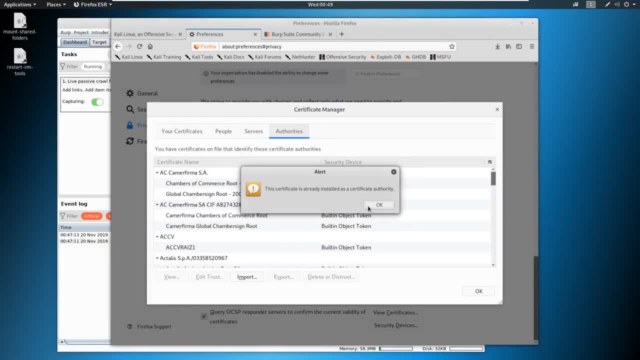 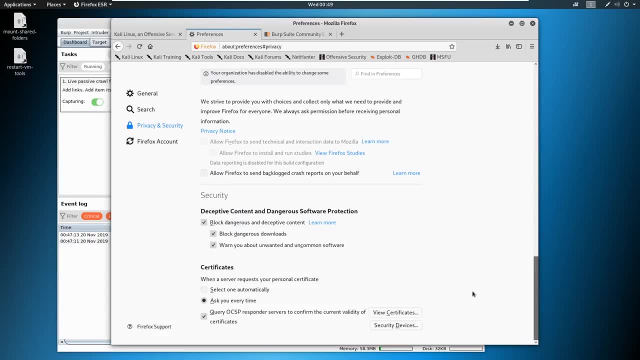 the are hit open And then it's already installed for me. but you will have to check boxes, check both of those boxes and select OK, And then it should now be imported for you. So a couple things to note. Firefox sometimes changes things around. I'm recording this video in 2019.. If you watch it at a 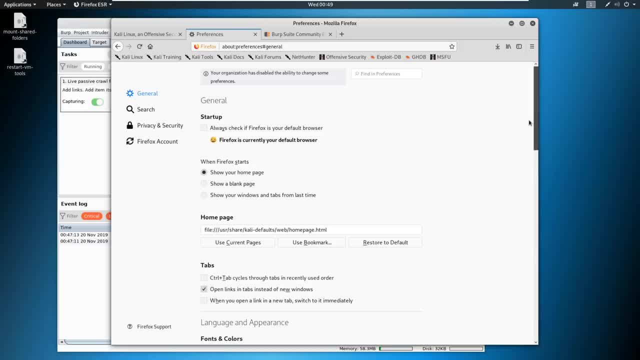 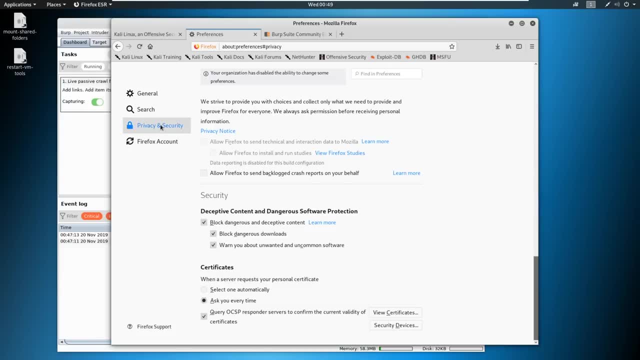 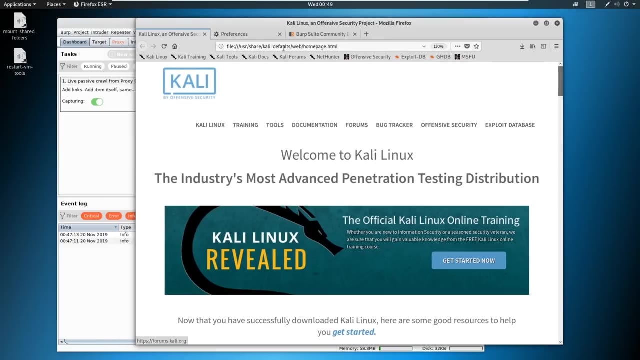 later time. just be cognizant that in the General tab, usually towards the bottom, is the network settings, and the privacy and security settings Usually contain the certificates, So look around for those. sometimes these move. So from here let's go ahead and just see what we set up. So I want you to go ahead and try to go to a website we can try to. 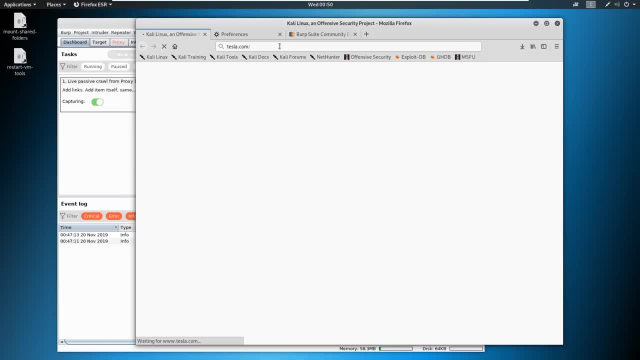 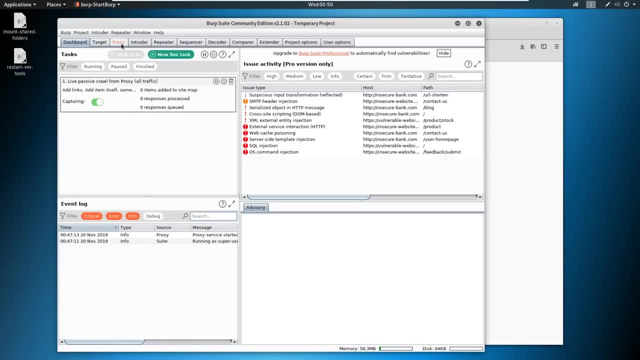 say teslacom, And it is going to stall out what is going on here. So if we go over here we see this proxy tab is lit up in orange. we're going to go ahead and click on that And you can see that it's. 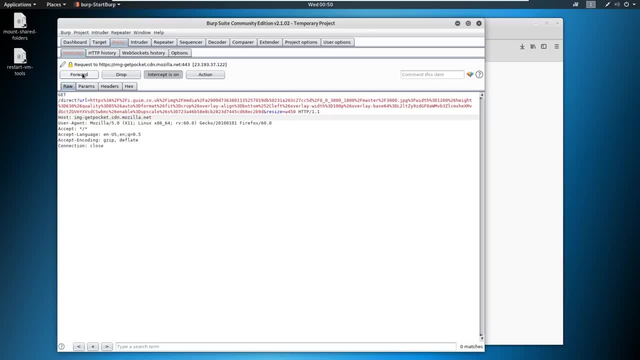 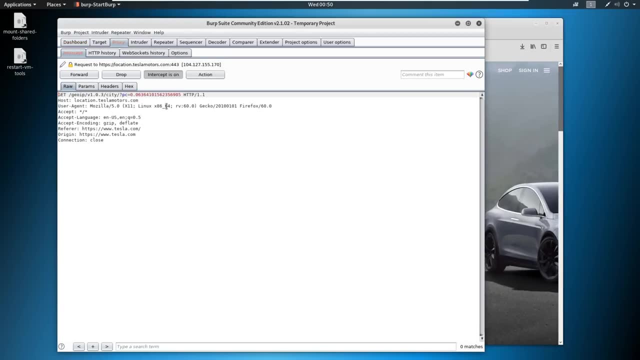 gathering some data here. it's captured some stuff from Firefox. We've got more Firefox. we can just click forward through this if we want, And now we can see Tesla starting to load. And we're what we're doing is we're intercepting requests that Tesla is making. 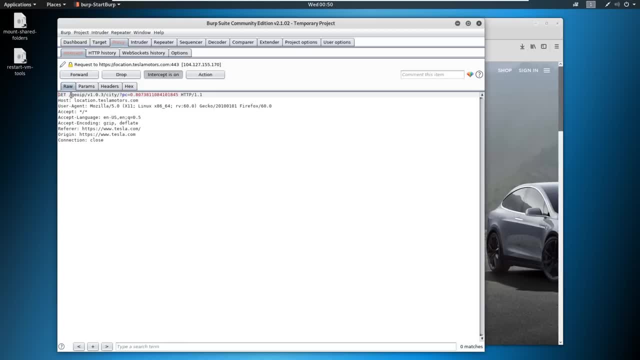 out. This to me looks like a API request or a geo IP request. So this might be geolocation looking for a city. So we're just clicking through. clicking through, all we're doing is capturing all different kinds of traffic And we can modify this traffic. Say, we have this request here, you don't have to know. 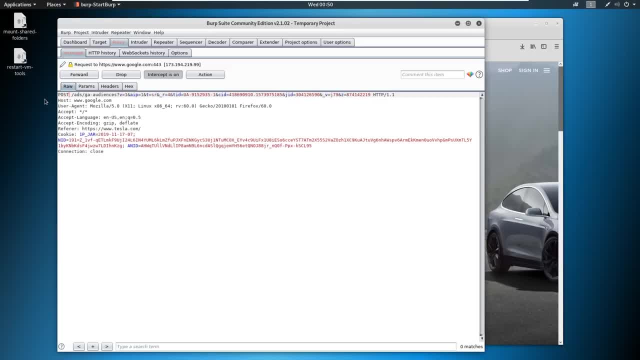 what this is right now. But we have got this get request. we can make this a post request and forward that and see what happens. I'm just going to turn the intercept off. I'm going to show you what's going on here So we can go. 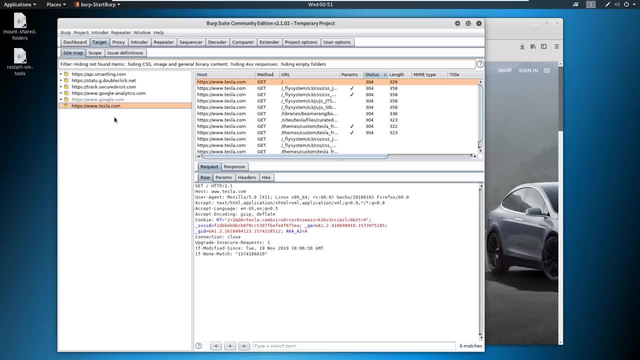 over to the target And you can see all the pages that have loaded in here. This is all the traffic that has been intercepted so far since we ran Tesla. So not only is Tesla running, but you can see that it pulls Google Analytics. it pulls this secured visit, which looks like tracking as well. It pulls double click, which looks 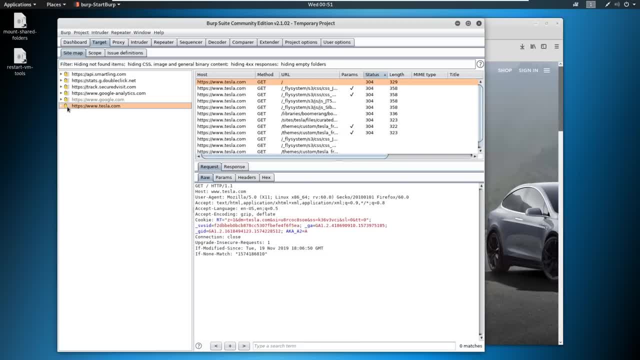 like maybe ads, And then it has an API running here as well, So it's gathering all this traffic through. but we're going to dig into this Tesla here And I just want to click on the first forward slash and see if there's a response to our request. There isn't, let's go ahead and just look at maybe. 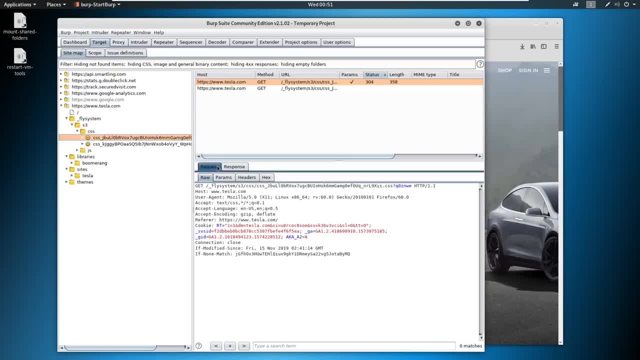 the let's see if we click into one of these. if we get a good response, We don't let's refresh one more time on the page And you might even need to hit enter Okay, and sometimes it doesn't come through right away, So let's go ahead and just click around. 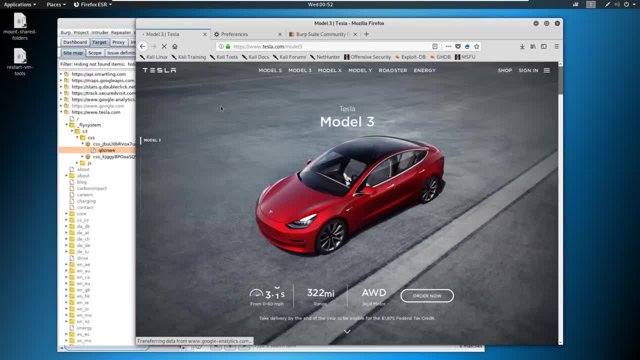 There we go. Do you see all this stuff coming through now? That's more like it. It wasn't picking everything up right away, So what we can do is we can look at some of the things that just came through like we just went. 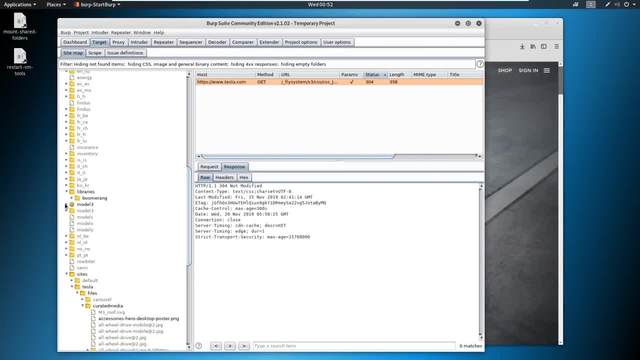 to the model three page. So let's go ahead and click on this model three and see what it's got for us. So you can see that if we look at the request for this get model three, we made a get request to model three And 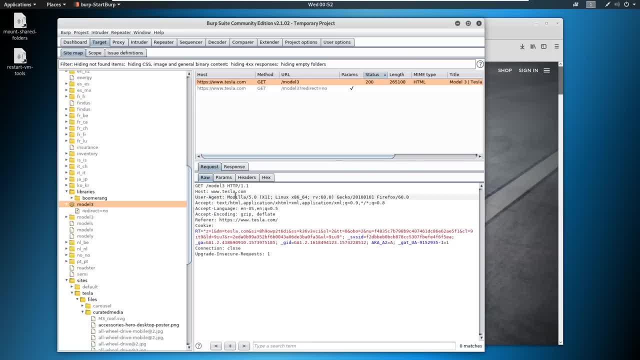 what's happened is we say: hey, I want to go out to this page, go ahead and take me there, and then we can view the response as well. Now in the response we can get so much information. Look at this. We're seeing here that PHP 7.3, point seven is. 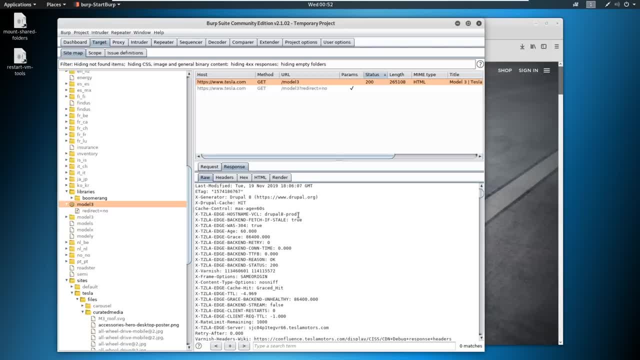 running on the back end. We can see a bunch of information here as well. Like Drew, Paul eight is running. We identified that earlier, but we're identifying it again. We could see a lot of other stuff. There's weird things here going on, to like there's a server name sitting in here. Typically on an assessment, this would actually be a. 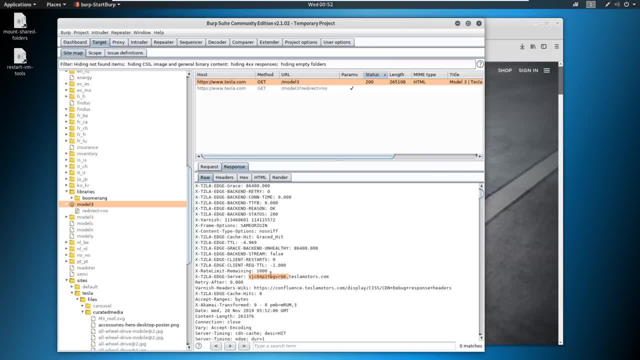 finding a low finding, but it's informational, As this is giving us information on possibly naming structure inside the network. But they also have their own Tesla type header here, So this is very unique for a client. But what the point of the matter is here is that we can. 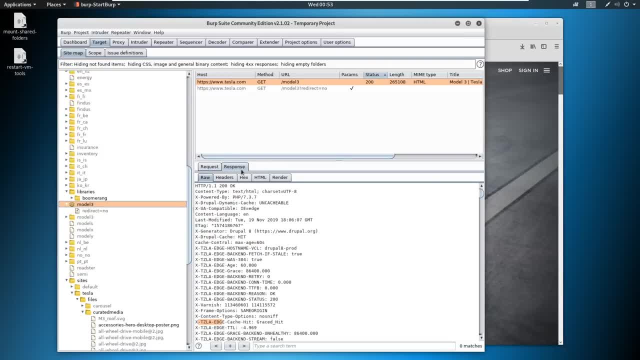 intercept a basic request and response and get a lot of information through burp suite. we're going to hit home on this really hard when it comes into the scanning and enumeration section And when we get into the web section as well. But for now I just want you to take away that we've installed burp suite and we can go out to a website, And I still 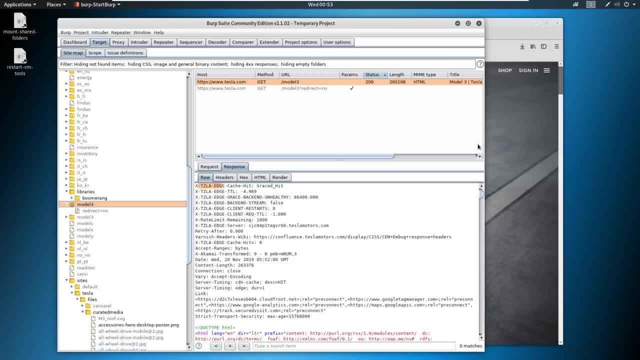 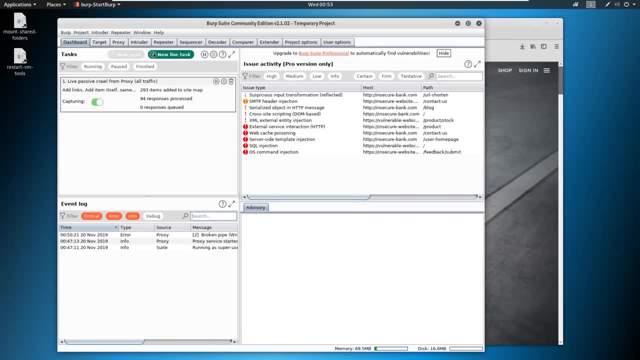 define this as not active scanning. There is a feature in burp suite that has active scanning that we could actually run, but that is a burp suite pro, so it has a vulnerability scanner built in. you can see see up here. upgrade to burp suite. professional automatically find vulnerabilities. I have burp suite pro. it's $400 a year is absolutely fantastic worth the money. I'm going to limit it to one of the few applications that I would recommend anybody buy, But for the course I'm going to. 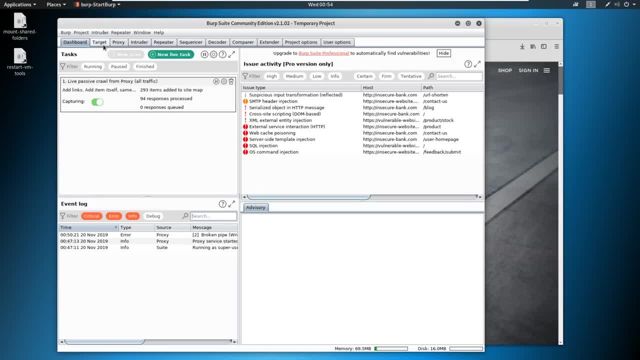 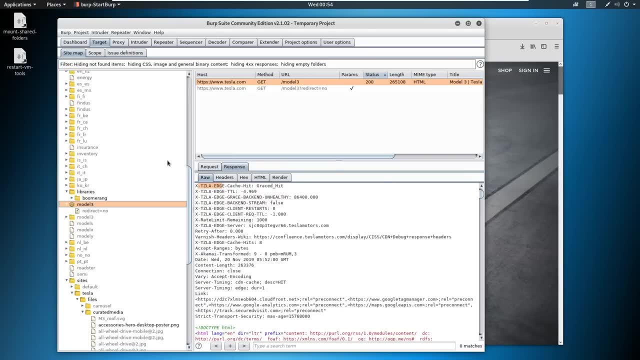 limit it to utilizing community edition. I will bring in pro sometimes just to show you some features, But we're not going to worry about that. So long spiel short. I still feel that we are in step one here, even though we are accessing the. 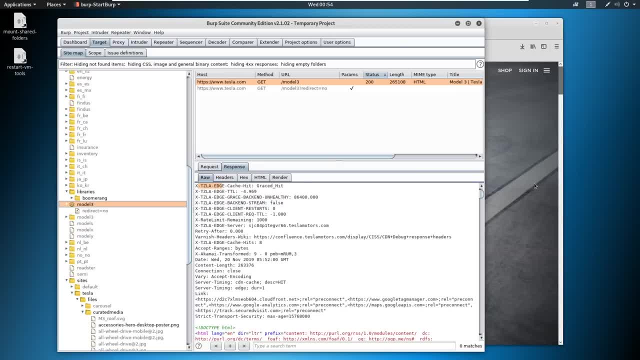 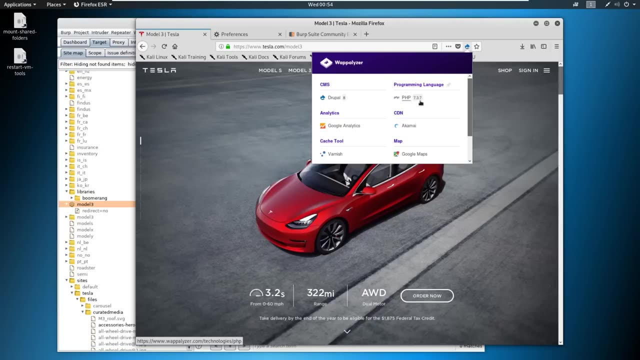 website. we're not doing anything very actively with scanning. this is all very passive. we're using traffic like a normal user would. So you can see that we can intercept traffic and get a lot of information. Again, tools like wap, Eliza- look, it pulls down the headers for us and it says: Hey, it's running, PHP 7.3.7.. It's running. 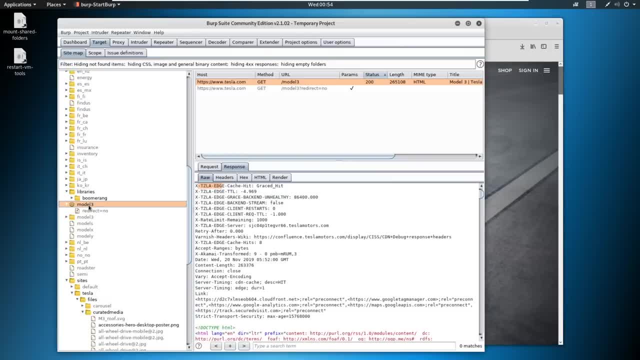 Drupal eight. where is it getting that from? Well, it's getting it from these responses, So it's pulling a lot of that down for us automatically. But there's a lot of things that we can do when we get into burp suite as well, So consider this just a mini. 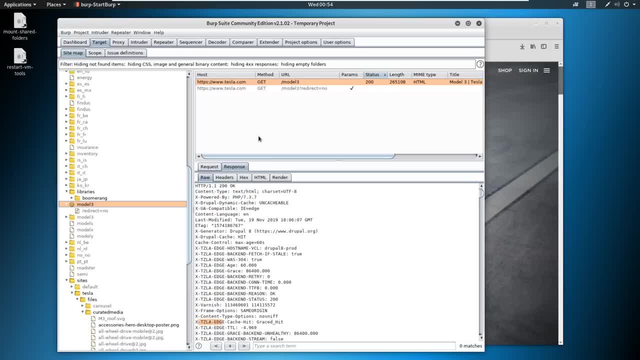 introduction into the tool, And then we'll touch back on it over and over again as we go. So this is it for this video. we're going to get into some Google foo in the next video and talk about social media as well, So I'll see you in the next one. 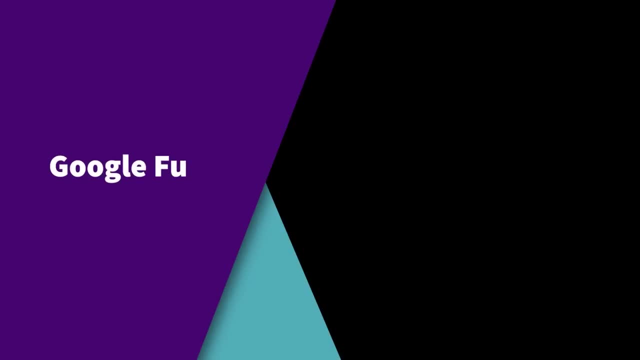 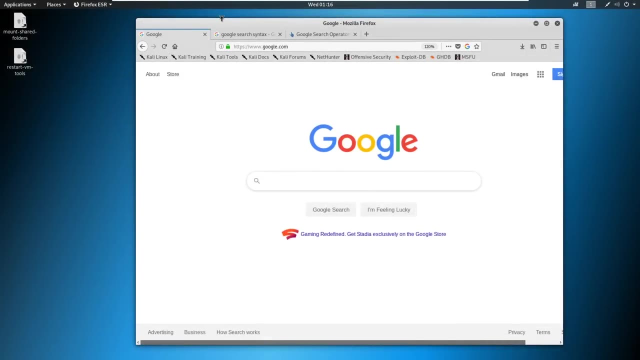 Okay, now on to what is going to be your absolute best friend in your entire life and in your career: Google, Google, everybody. I cannot stress how important it is to be good at googling, And you don't have to be amazing at it, But there are so many things that 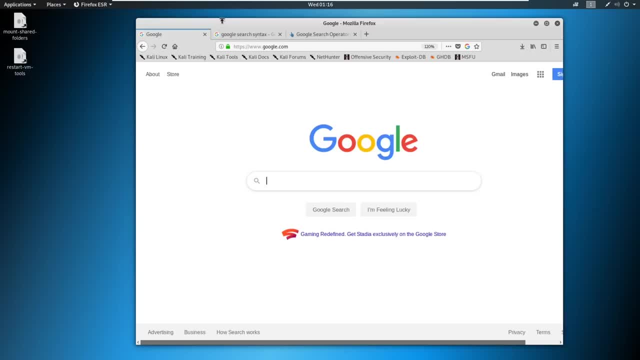 people approach me with that you can find on Google in a second And if you've never seen the, let me Google that for you. that's a. that's a lot of my life when it comes to the questions I get asked And what makes a really good pen tester or really good anything. 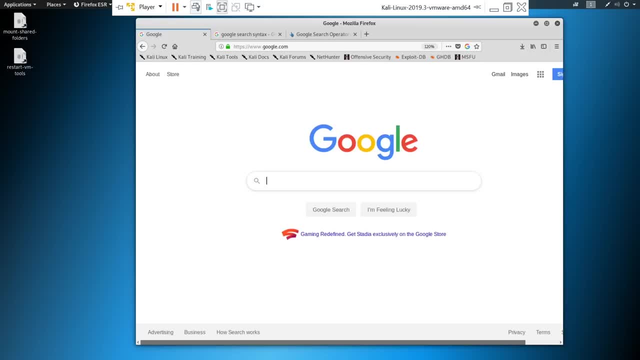 especially in it is the ability to Google. So being able to look this stuff up on your own and being able to find your own resources and find solutions to your problems are going to make you a way better teacher, pen tester and just way better at your career with troubleshooting and everything else. So I'm done harping. I just wanted to stress how. 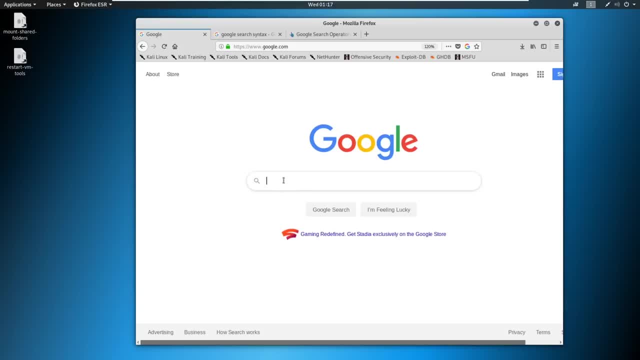 important I think Google is. So I'm going to show you today what's called a little bit of Google foo. So I'm already out on the interwebs, I'm out to Google And here we've got Google up. But I want to show you that I just searched for Google search syntax, And the first one, Google. 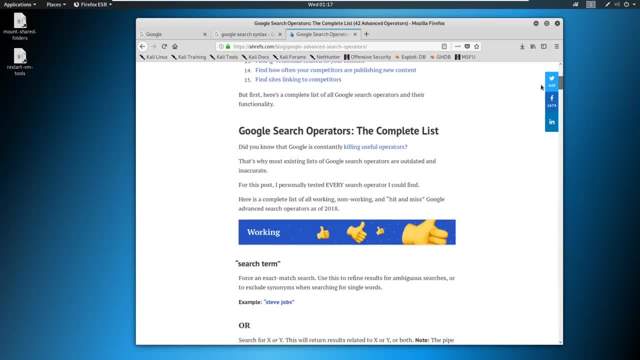 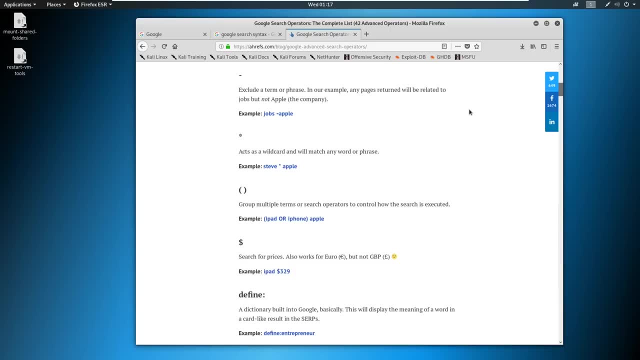 search operators came up. If you go look at this page, this is a really nice list of some things that you can find on Google, So I'm going to show you a list of some things that you can run on Google And we'll help you out. I'm going to show you just a few things that we can use to search. 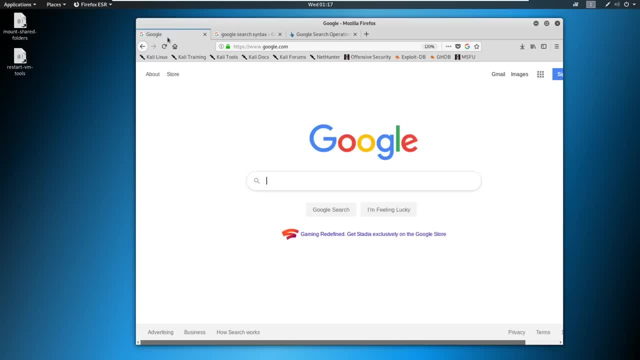 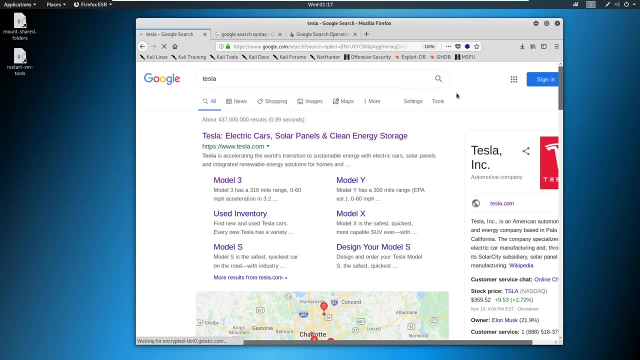 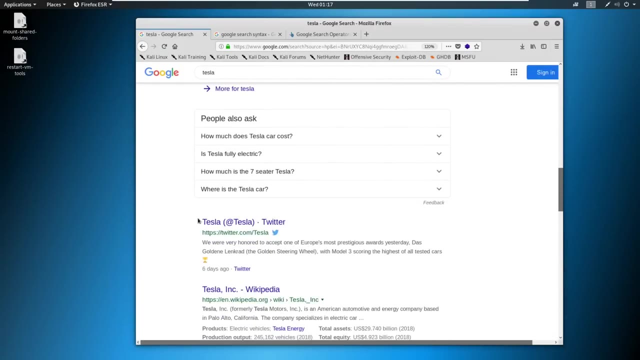 for and how we can start narrowing down some results. So if we go to Google and we just type in something like Tesla, that's going to bring up Tesla here- Okay, we found the main Tesla site. But we're going to get news articles and we're going to get all kinds of stuff- Okay, we get the. 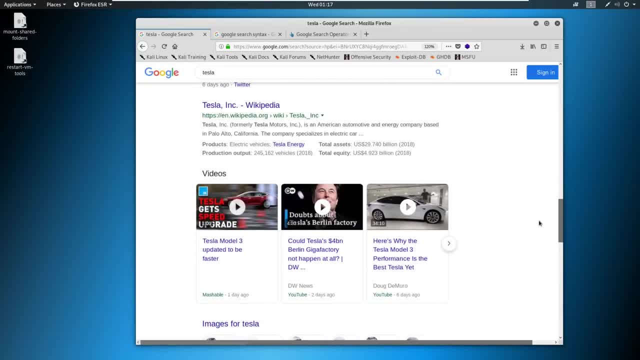 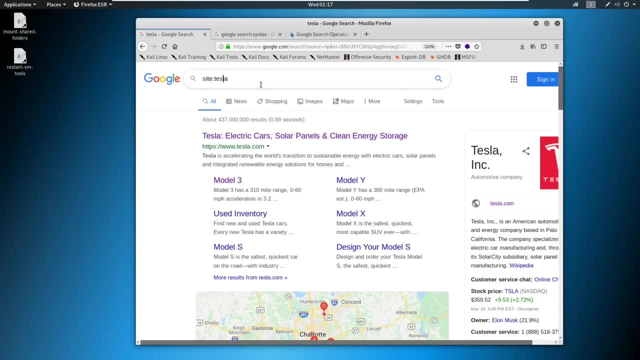 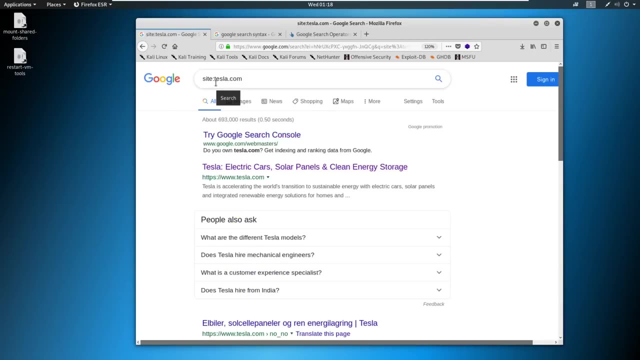 Twitter, and maybe we want this, Maybe we do, Maybe we don't, Maybe we don't want all this mess, Maybe we only want items from Tesla. So we could just say something like site teslacom, which we've discovered here, And notice, I'm not putting in the WWW because that will limit us to that specific domain. So we have 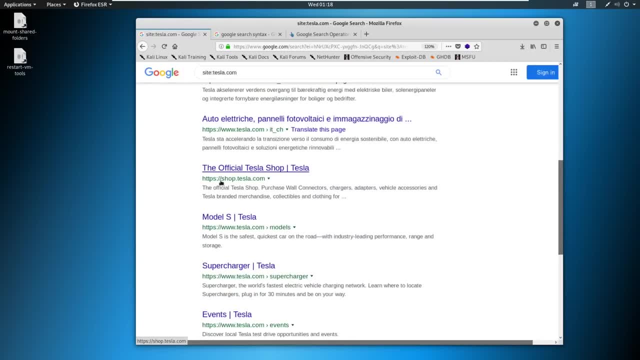 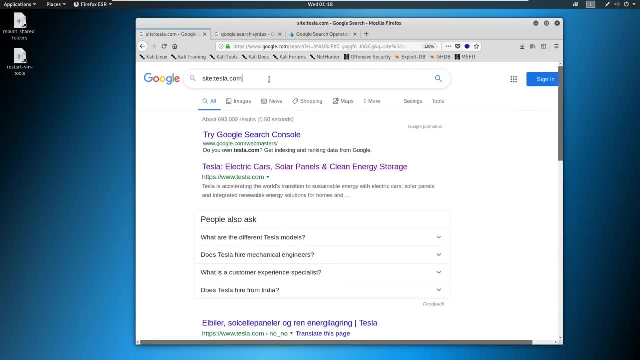 the WWW is in here, But you could see that it's starting to pull in something like shop and other items. right, So we can search for teslacom And maybe, maybe we don't want teslacom WWW, maybe we take out with the subtract here, maybe we just take out WWW And we're going from. 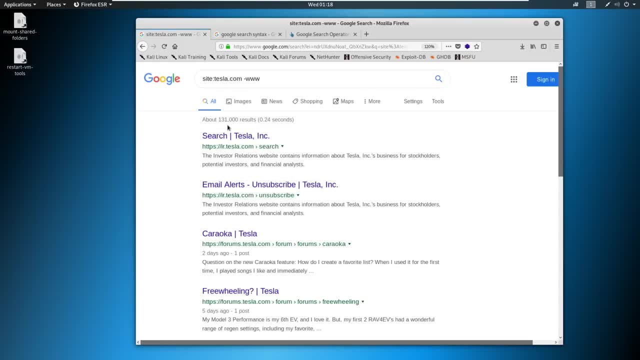 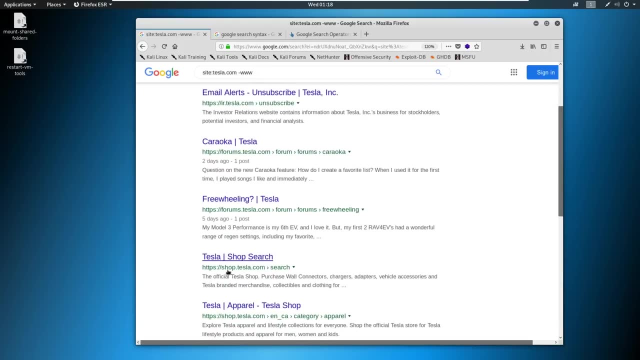 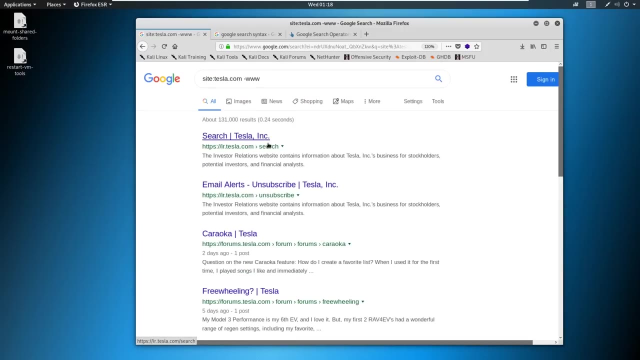 600 and almost 700,000 results to 131,000 results, And you can see, now we're pulling in IR, we're pulling in forms and we're pulling in shop And we're getting all these different unique subdomains. So I've showed you sublister and I've showed you other ways to find subdomains, including 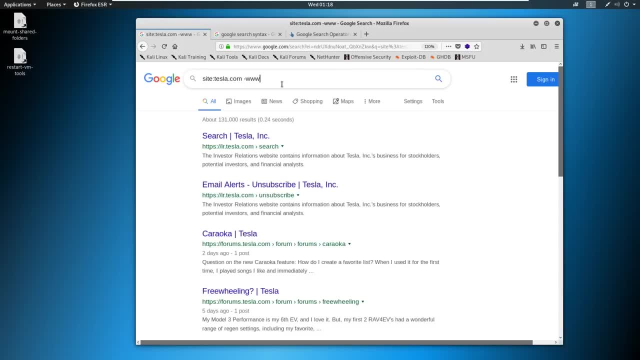 subdomains. But you can find subdomains like this as well, And let's say, you only want to find things like you know IR. then we can just come in and we can say: IR, dot, or maybe you don't want WWW And you don't want IR. you can take those both out And you start finding more like partners. that Tesla shop again is. 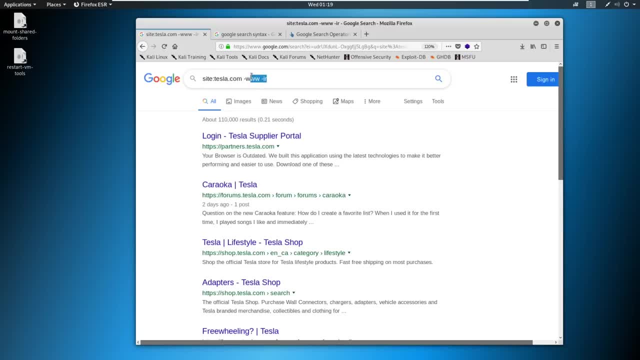 coming up, So you can start finding different subdomains this way, Pretty good. A couple other things that we could look for. Okay, What about file type? We could say file type like this, And we could search for something like I don't know, doc x. maybe there's a doc x out there. 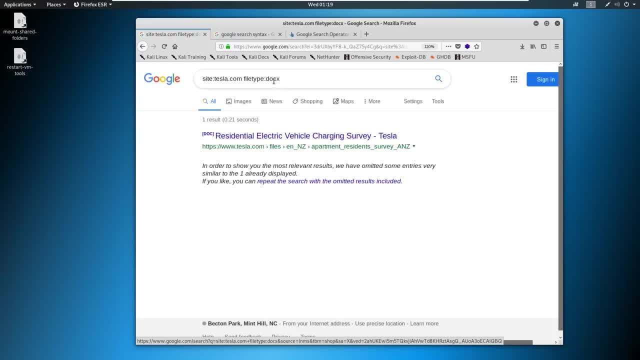 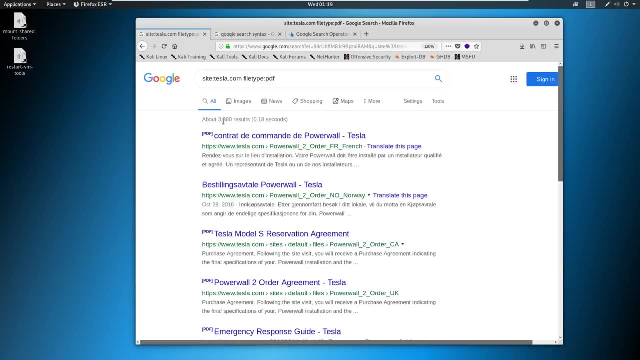 And there's one, doc x. Okay, it's a survey, probably not useful to us. Maybe we can search for PDFs. With a company as big as Tesla, it's probably going to be a lot to search through, but there are 3,300 of these, almost 3,400 of these. 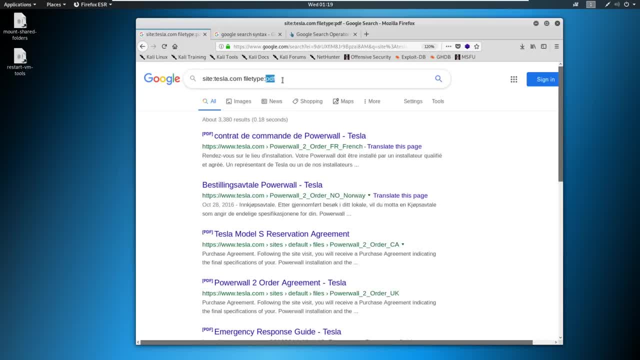 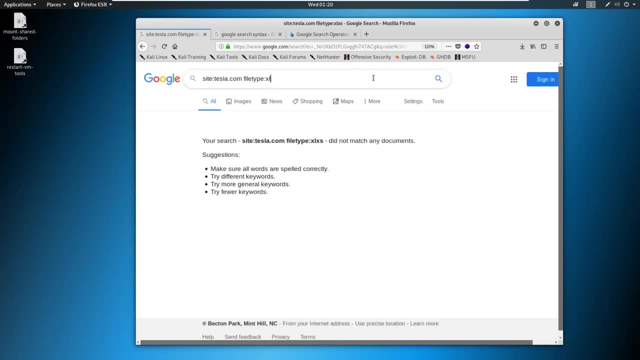 So they've got different items here that we can look through, Okay. Okay, So that's what we're going to be looking through. You know, maybe Excel, XS, Excel, right, Actually that's SX. You can see if there's any Excel and CSV. 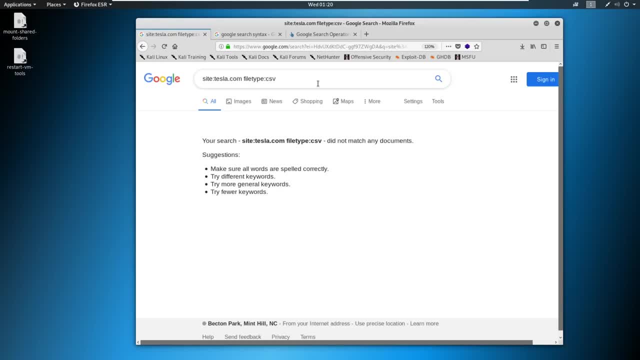 So what we're doing here? what's the point of me doing this? Well, the point of me doing this is me looking for potentially sensitive files out there or information. you would be surprised what a little bit of hunting on a domain now give. granted here that Tesla is a big company, big domain. 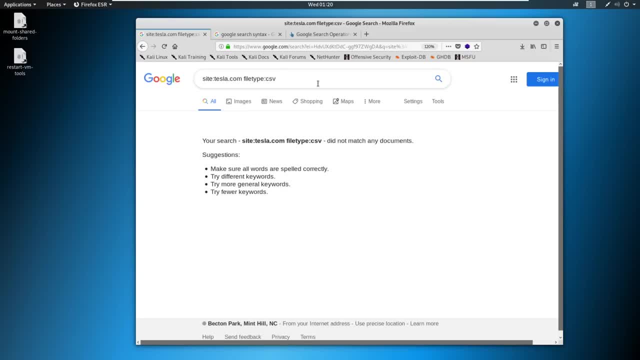 Okay, And it's going to be hard to find some of this information, But you'd be very surprised with a little bit of prodding, a little bit of Google foo and narrowing down the type of results that you can get off of a company. 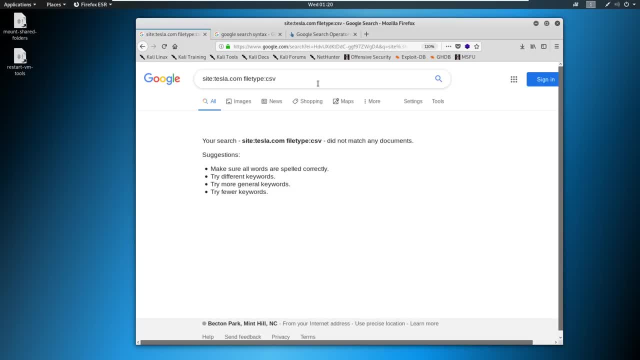 I mean, we can find all kinds of interesting stuff. For an example, just the other day I found a backup page of an entire website just by doing something like this entire website: credentials, source code, everything Okay- And just through a little bit of Google food. So again, Google is your absolute best friend. Before you ask anybody a question, no matter how complex, I challenge you to Google it. first make sure you have done your research and then ask somebody you know. it's just good to get in that habit. 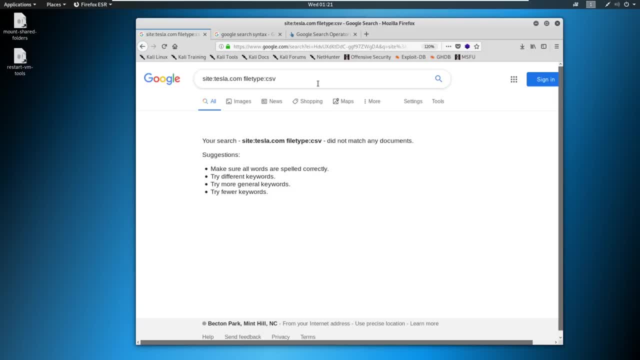 But first make sure you have done your research and then ask somebody. you know, it's just good to get in that habit, And this is what is going to make or break you. I believe in your career, So please, please, do not ignore the Google machine. It is out there to help you And it will be there for you. 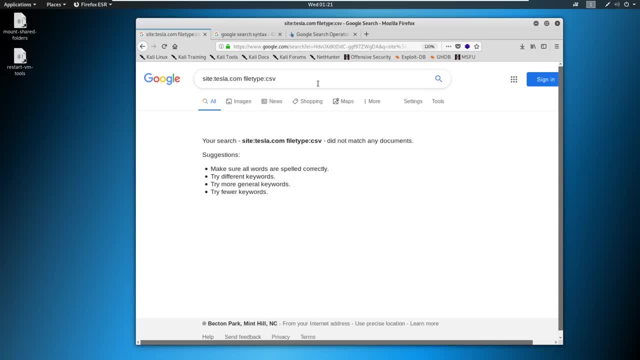 Okay, will pay your salary over and over again. So that's it for this video. We've got one more video left in this series, or the subset. We're going to talk about a little bit about social media and how we can target that, so I will catch you over in the 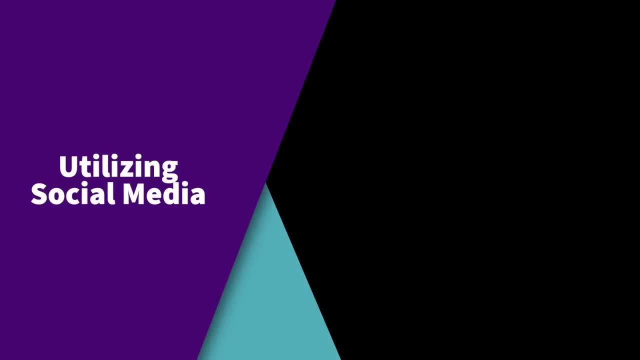 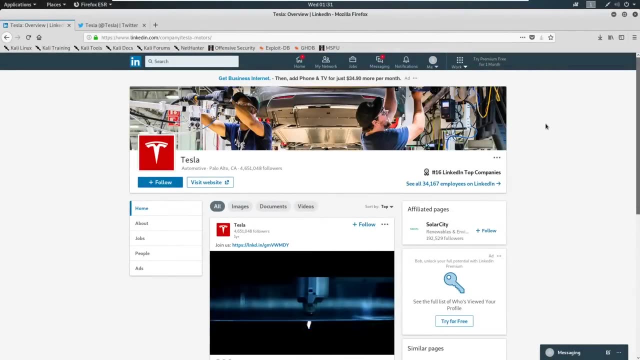 next video. Okay, so you don't have to follow along this video. I just kind of want you to start getting the wheels spinning and thinking about other items that we could be looking for when it comes to OSINT. Now we could look on a website like LinkedIn. 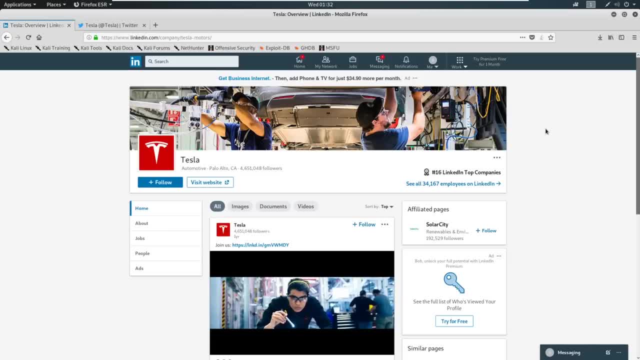 or like Twitter and find useful information. I was on this website for literally one minute. I've logged in, I went to Tesla and I've already kind of found something and I want to show you how fast this is. So you come in here and you go to Tesla- the 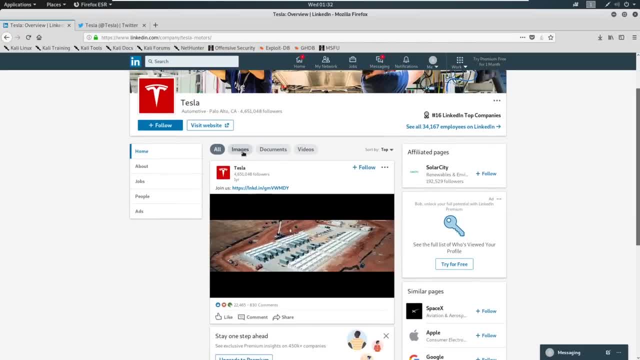 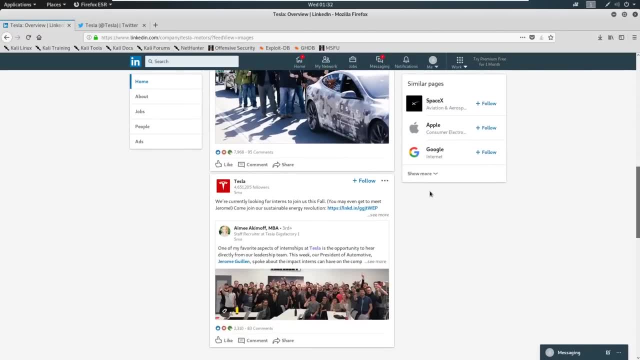 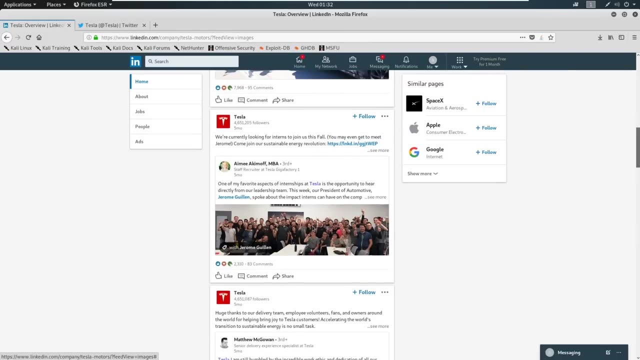 company, the company, the company page here, And I love to click on images. There's always employee photos on images. Now you scroll down a little bit and you can see somebody has recently posted a picture of their internship at Tesla. And what we can do is 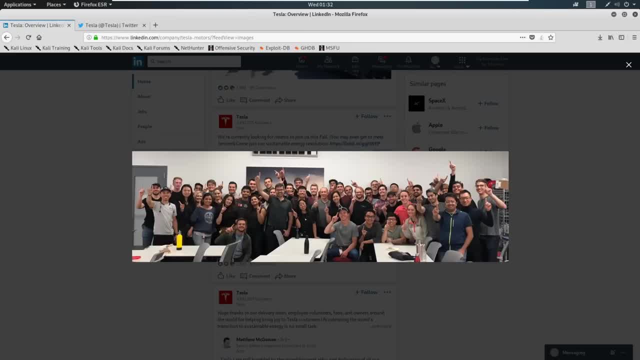 click on the picture and look for things like badge photos or desk pictures or anything of the sorts. Now, good employees are told to hide their badges from pictures and you could see that they've done a pretty good job. But if you look down here, right. 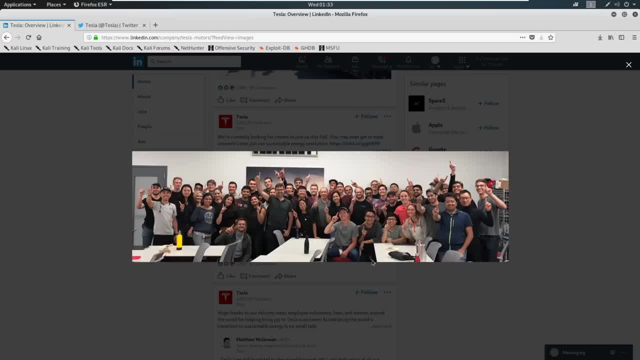 down here. it's hard to zoom in, but there is 100% a badge there. Is this a great picture? No, but this is a good example of an easy way to find a badge is utilizing social media, And you can find a. 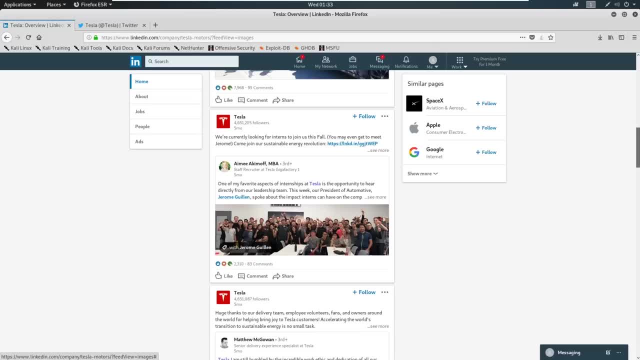 lot of stuff very, very, very quickly. So another thing to point out, too, is that Twitter is a goldmine for these kinds of things, So if you're looking for a badge, you can find a lot of these kinds of things. I have found badge pictures desk. 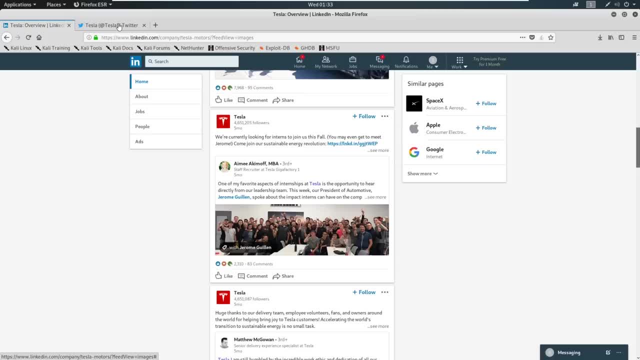 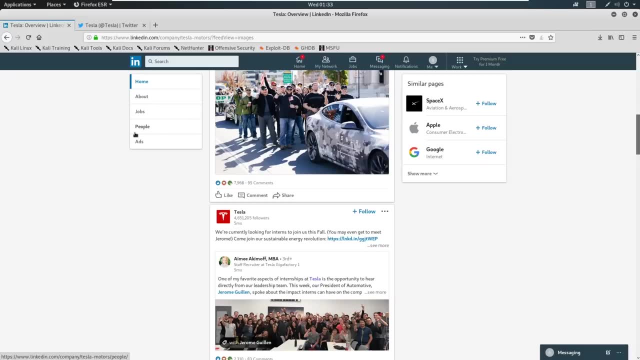 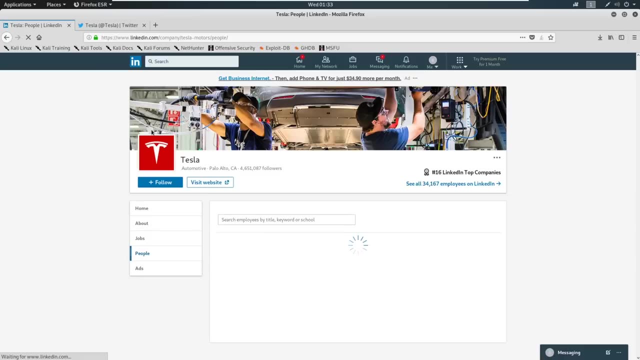 pictures, software, all kinds of stuff via Twitter and via LinkedIn, Now from the non physical perspective or information gathering perspective for what seems like physical assessments. The other thing to point out is that it's really good to find the people like. LinkedIn is great, So we. 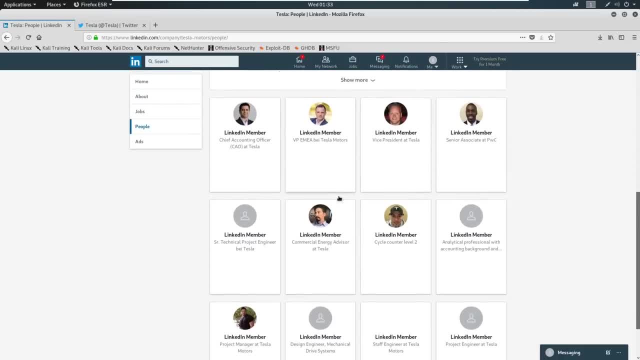 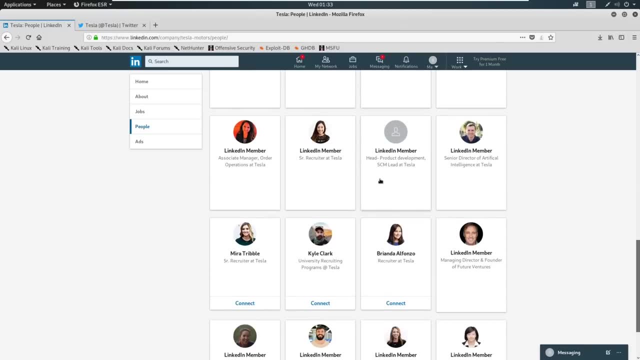 can come in here and we can find members right, and these are all going to say LinkedIn members. I don't have. this account is just kind of my, my peeping account that I just utilize when I want to look in, not trigger anything weird when 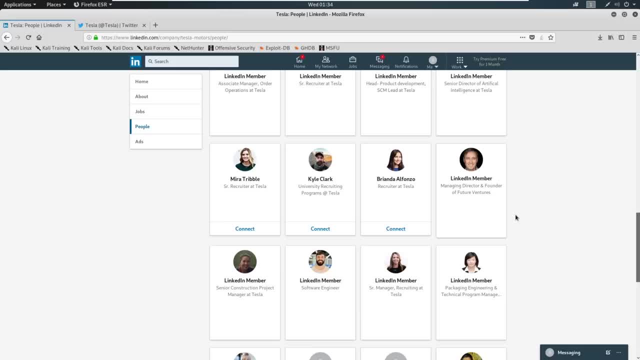 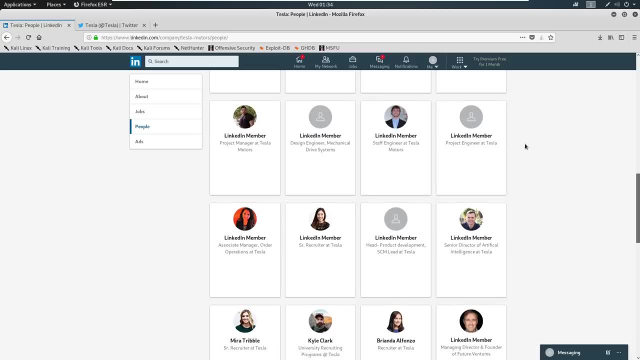 I'm looking at a company, because if somebody sees me as a person looking at a company might say: why is this guy looking at my profile? So we might not get names. if you don't have the premium on some of these, you might see LinkedIn member. But 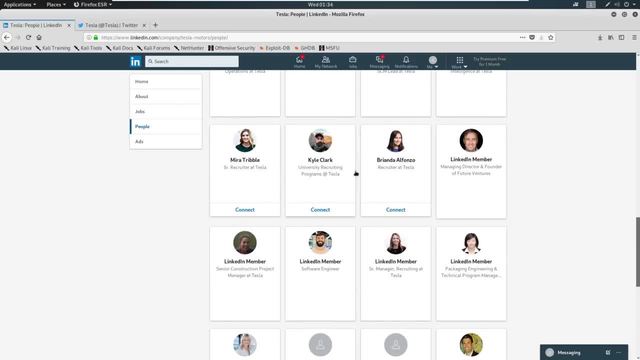 you can also dig some names like here's a name, here's a name, here's a name, And you take those names and you remember the formatting from before, right, The formatting when we looked at hunterio And we said: Okay, 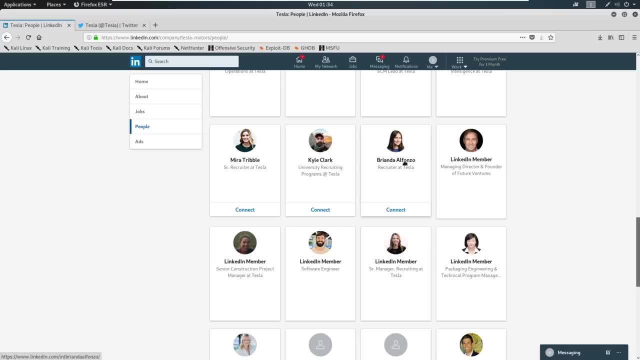 first initial last name. well, I might take a first initial last name here And I'll add that to my list. Now we could utilize scrapers out there to look through the employee list and pull down all the names and then transfer those names into first. 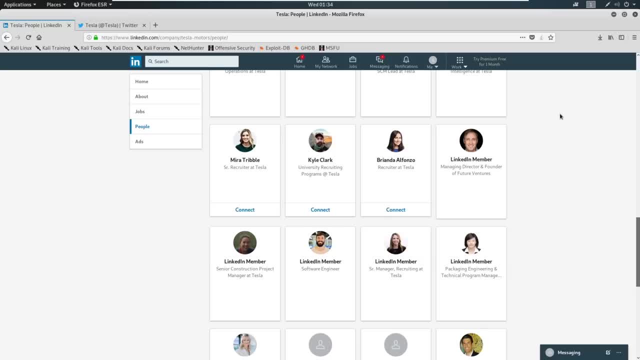 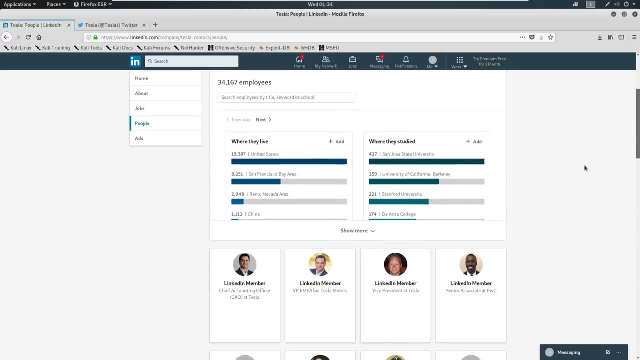 initial last name. you could write a script to do that with Python. if you want to challenge yourself to do that, I guarantee you there are tools out there to do this. But this is the kind of information we're after. We're after what kind of credentials can we? 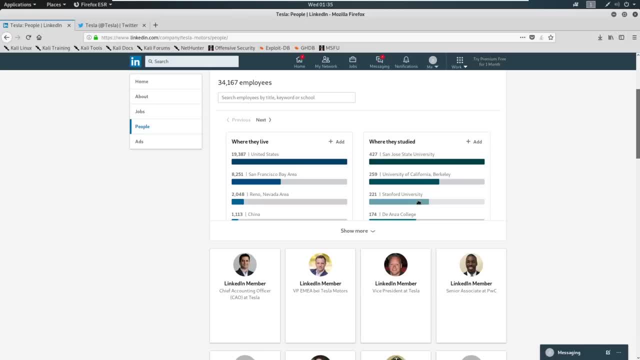 gather and this loops all back. this is the the wheel spinning here, right? You want email addresses. we're talking network and we're talking what you're going to be doing with these kinds of assessments. you want these email addresses. you want anything that's been a part of a breach: current credential. 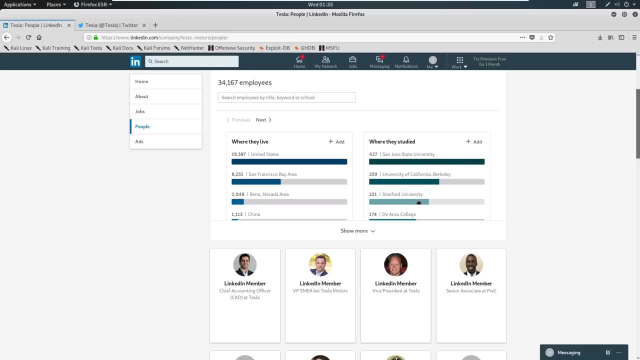 leak right And you just want as much information on the employees as you can gather. When you take all these email addresses and it says something, it says 34,000 employees. when you take 34,000 employees, I would almost. 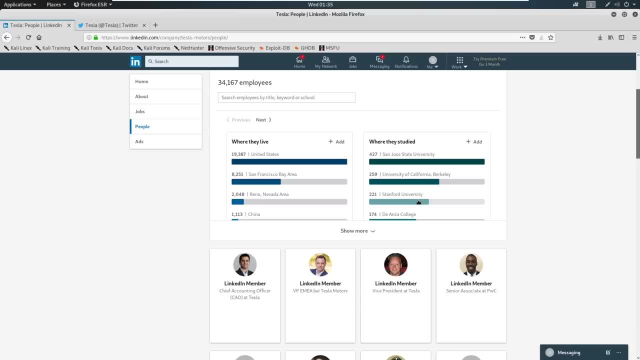 bet money on it that one of these employees has a password or something like fall 2019 or winter 2019 exclamation. or something like Tesla 1234 exclamation. People are always the weakest point of an organization And people will be. 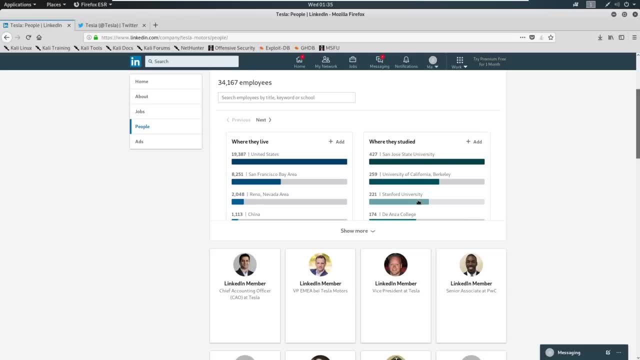 lazy with their passwords, unless you absolutely force them to use long passwords. I do not know Tesla's password policy, but in almost every external assessment with a weak password like fall 2019, or winter 2019.. So I want you to think about. 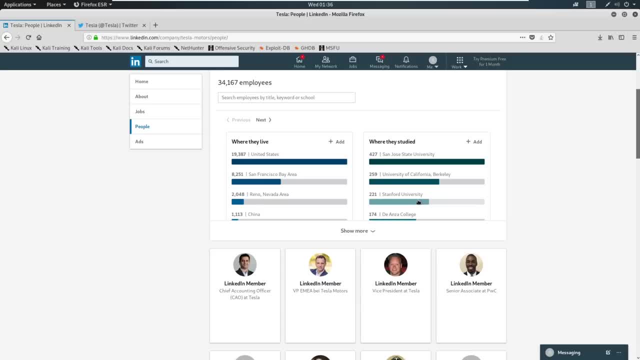 these things. we're not going to go too depth into social media, but have that in your wheelhouse as well. We're just trying to utilize as much resources that are out there in order to use them for our advantage. So there's a lot of tools that I've. 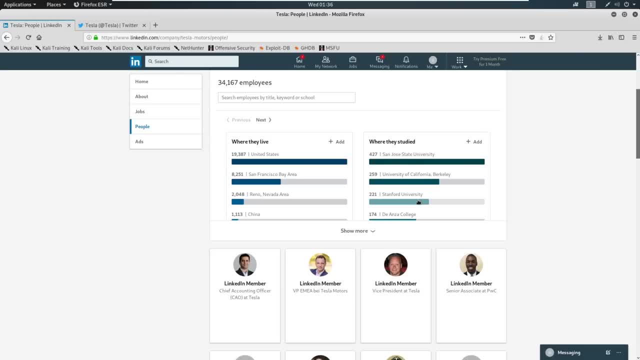 shown you And I've given you a lot of the basics, And really that's all you need for information gathering. Google is your best friend. utilize Google to your full advantage. utilize social media- people post things all the time that they shouldn't be posting And just dig deep. 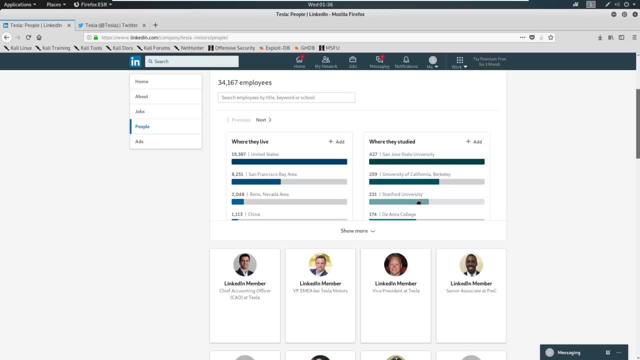 Information gathering is one of the most important steps, along with scanning, enumeration. Keep repeating that to yourself and you'll be very, very successful as a penetration tester. So that is it for this section. I kind of just wanted to give a brief overview of this and then give you some ideas to get your your. 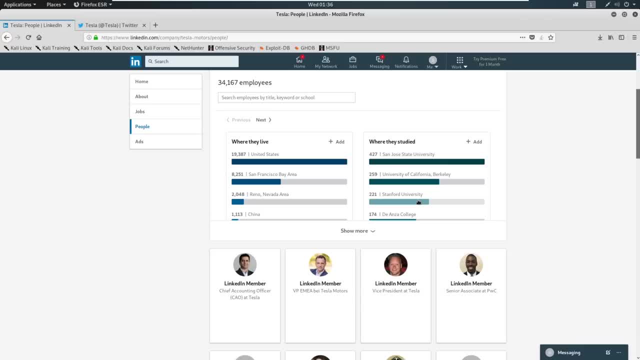 wheels spinning and really think about it. Again. we're harping on breach credentials mainly, So from here we're going to move into scanning and enumeration. we're going to start doing our hacking, getting into the real weeds of hacking. 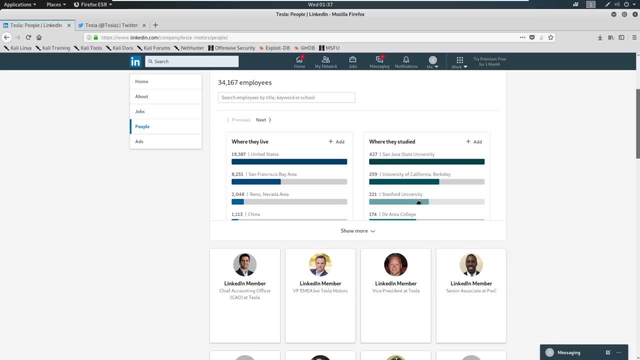 And I'm very, very excited about that, And you're going to see some of the stuff that you've seen before when it comes to reconnaissance pop back up. So I'm excited to see this play out through the course and how we're going to utilize it. So that's. 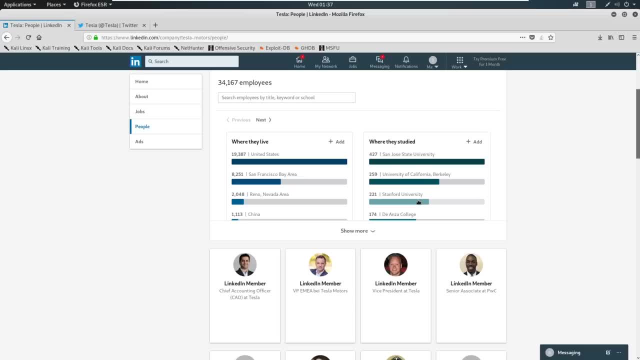 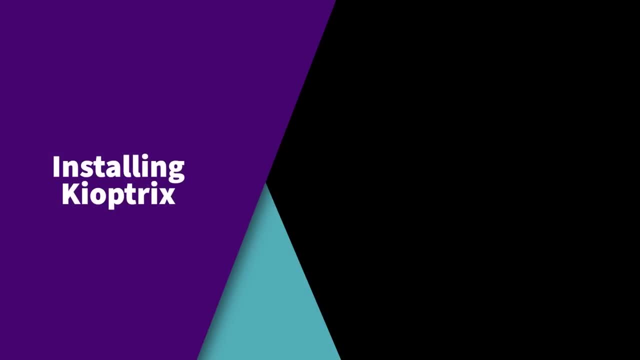 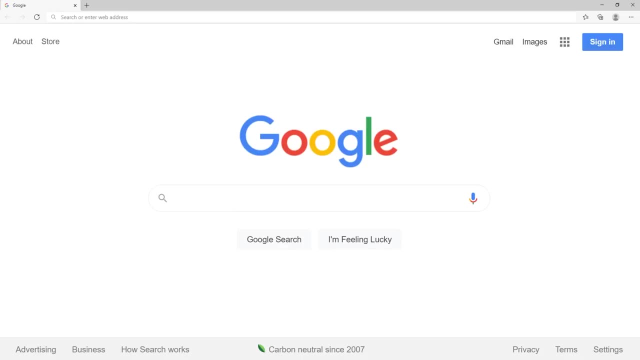 it for this section. I look forward to seeing you in the scanning enumeration section. Catch you over there. Welcome to the scanning and enumeration section of this course. It is actually now 2021.. When we're recording this and we're doing some light updating on how we go about starting off. 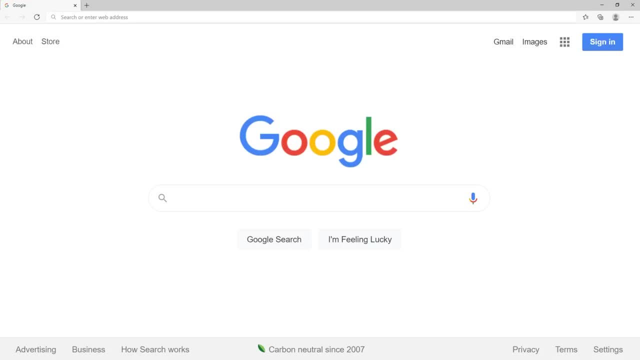 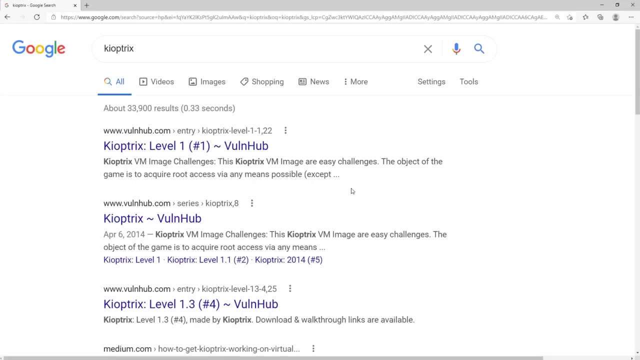 this lab in this section. So we're going to be using a vulnerable machine called key optics. If you go to Google you can type in optics and find it fairly easy. So you go to key optics like this: k, i, o, p, t, r, i, x- And we're going to be using level one. I'm 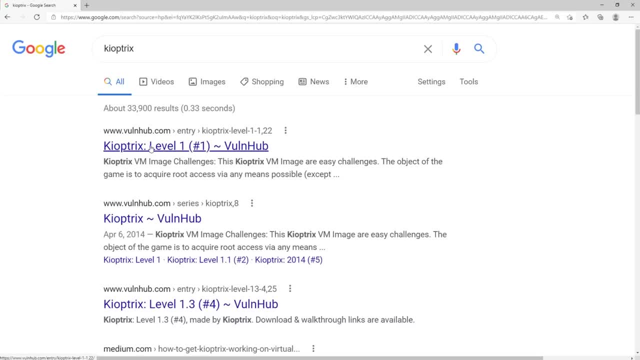 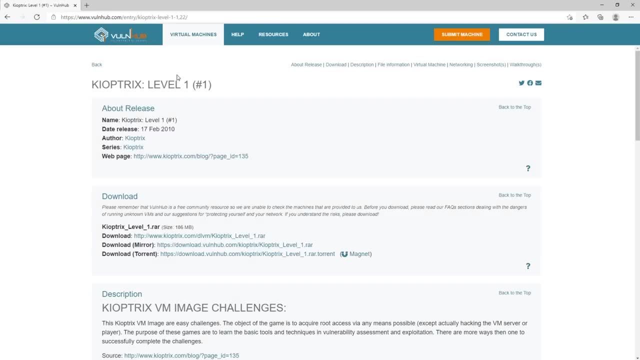 showing you the source of where it's coming from. But we're actually going to provide this VM just to avoid any sort of confusion. So key objects, level one here comes from a website called bone hub. let me make this a little bit bigger, So you 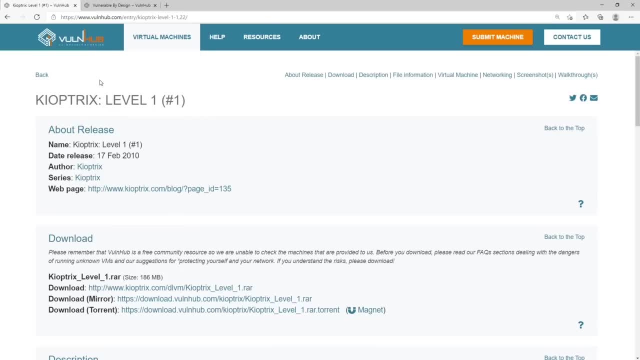 see bone hub here. bone hub is a great website and great resource. Once you kind of get into hacking and learning a lot of stuff, you're going to be able to get a lot of information in there. So you're going to be able to get a lot of information. 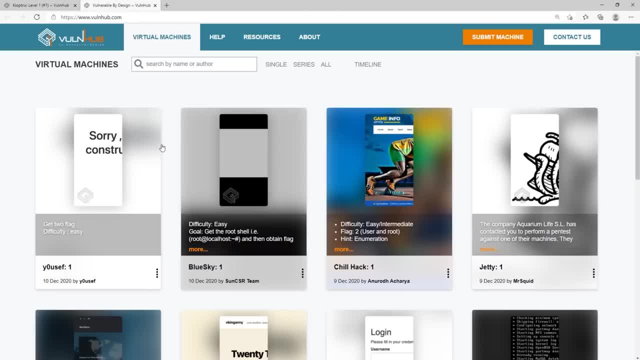 in there, So you're going to be able to get a lot of information in there. So you're going to be able to get a lot of information learning about this, where you could come to bone hub and just download a vulnerable machine, run it on VMware or VirtualBox. 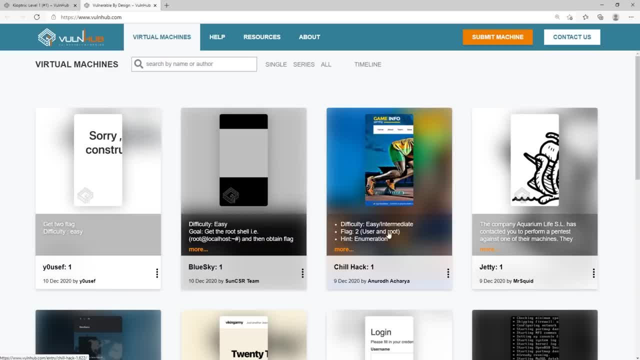 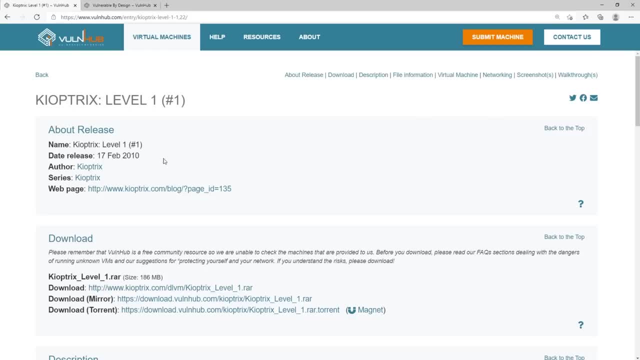 or however you want, and try to attack it And you can see they have difficulty. easy intermediate: you can come through here and just have fun playing with vulnerable machines And that's all captures is. it's a beginner level vulnerable machine that you can download, install and 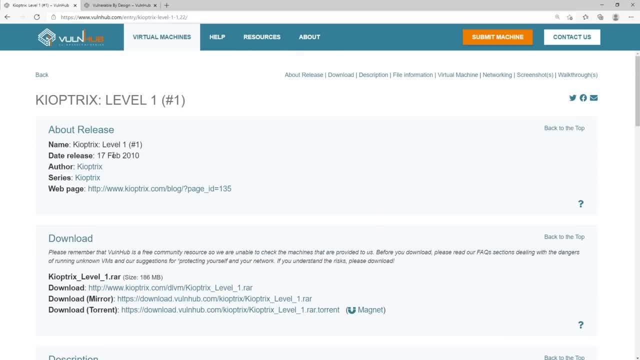 run Now the download and the install. you can see this is from 2010.. Some of the stuff was broken, sometimes a little bit difficult to get running in the original lab, So we're just modifying this a bit to make it easier What we've done on our 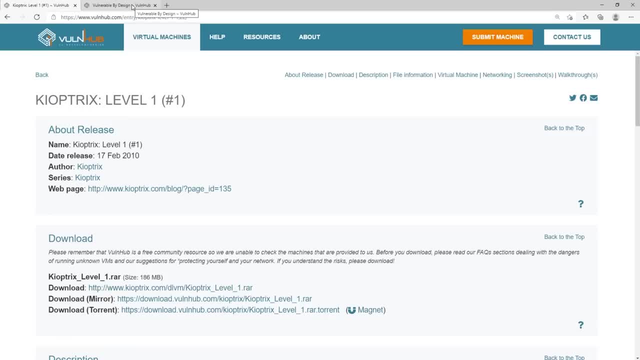 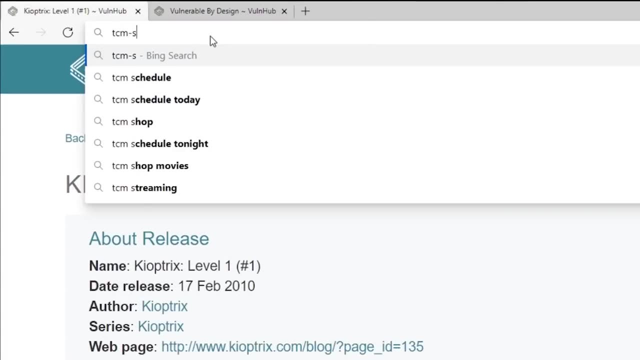 end is just hosted a file that will work, that will should by default install and run. So if you go to your browser and you just go to TCM, dash seccom, like this and you type in forward slash key optics K, O, P, T, r, i x. 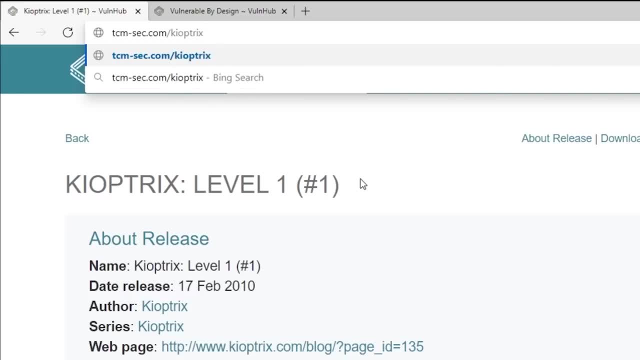 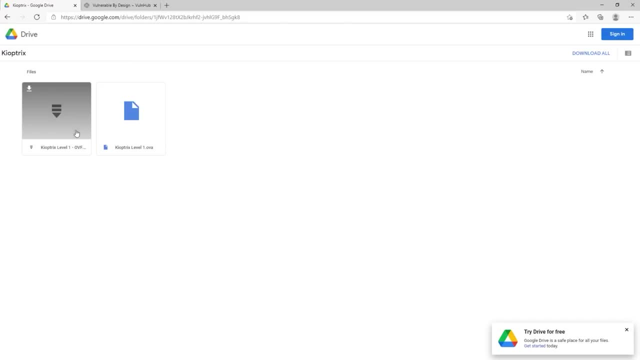 pause for a second, make sure you see this, and then you just hit enter. you'll be brought to a Google Drive. Okay, and this Google Drive here should say key optics. you should have an OVF and OVA file. all you need here is the OVA And all you'll have. 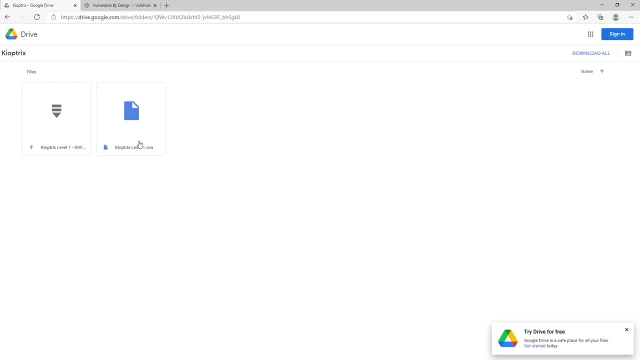 to do is just hit download right here, get the download going. I believe this is around 250 megabytes, So it might take a minute. go ahead, download it, pause and then come back when you're ready to continue. Okay, so moving on, I'm going to show you how to install this on. 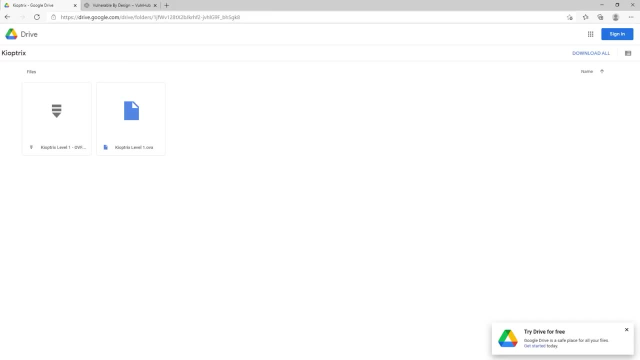 VMware and on VirtualBox. These are the only two supported methods that we're going to utilize in the course. If you're going in, you're using something like VMware horizon or you're using a different type of virtualization software. that's. 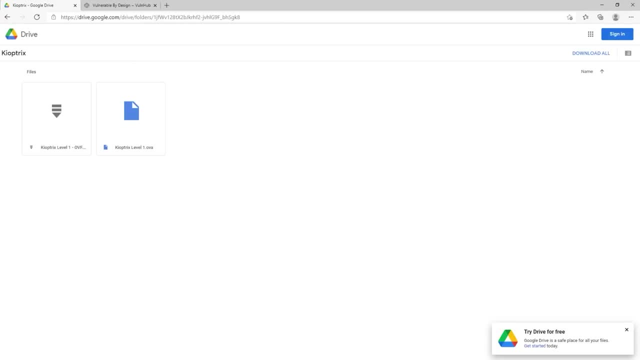 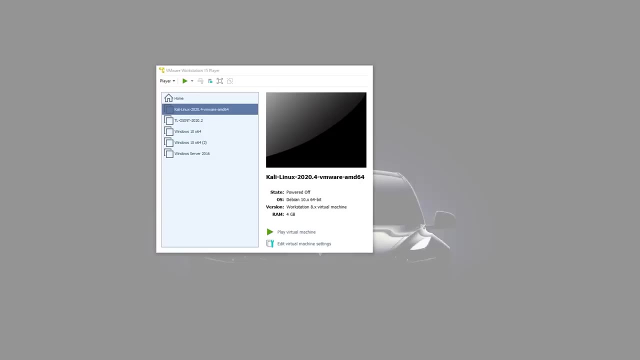 fine, but we can't support it if you run into any issues. So we strongly, strongly recommend using VMware. If you're using VirtualBox, that's fine as well, But we're going to be doing most of the course in VMware, though it should not matter too much. So. 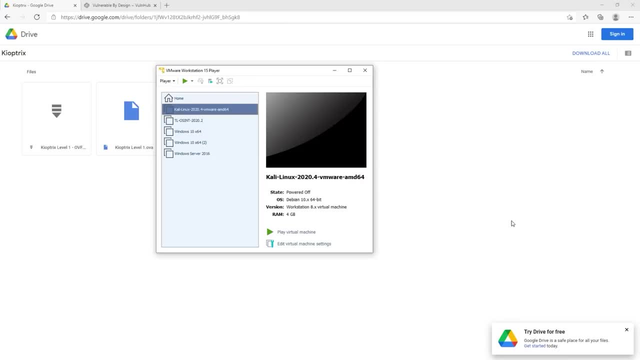 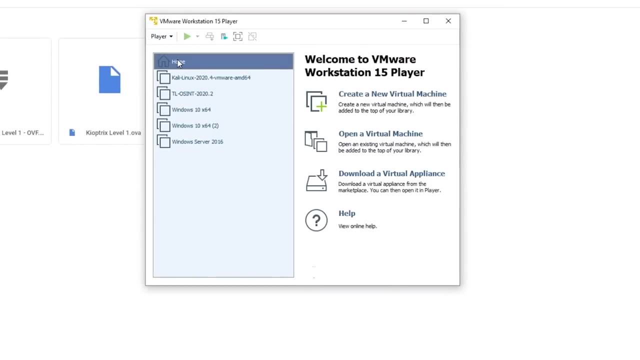 here is VMware. I'm going to show you first how to install it here, And then we're going to go ahead and do the same thing in VirtualBox. So all we're going to do is we're going to go to player up here, or we can go to home, actually, And we can just. 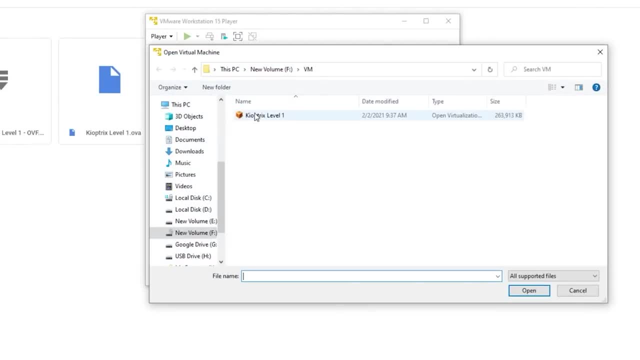 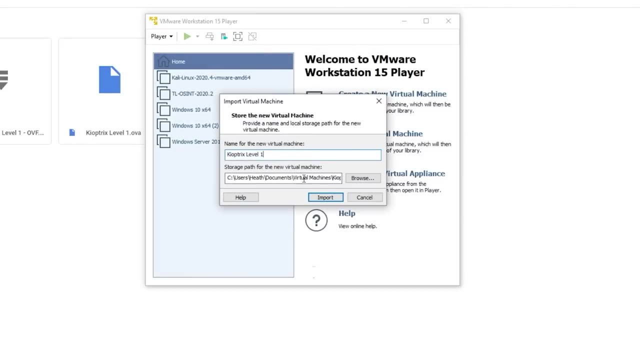 say: open a virtual machine And then just go ahead and navigate to the area where you downloaded it. Okay, so here's my file, key optics, level one. I'm going to say open. I'm going to go ahead and just save it here. So I'm going to say: this is where do you want to? 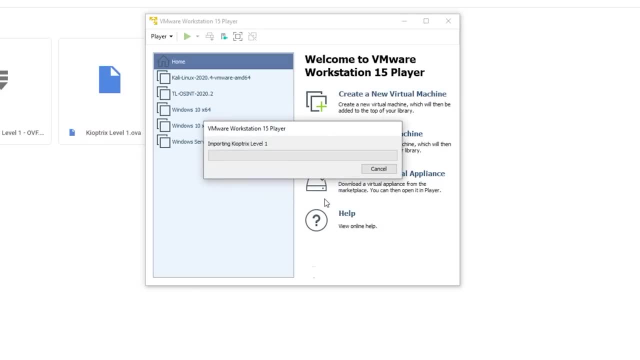 save your storage path. I'm saving it here. call it captures. level one: import. the defaults are fine. you might get an error right here. that's okay to just hit retry and it should work fine. It's going to take a second to import While we're 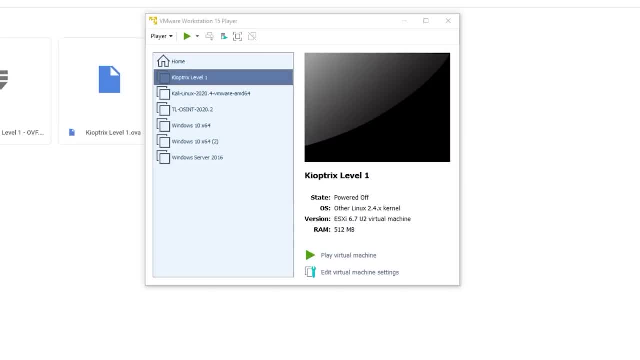 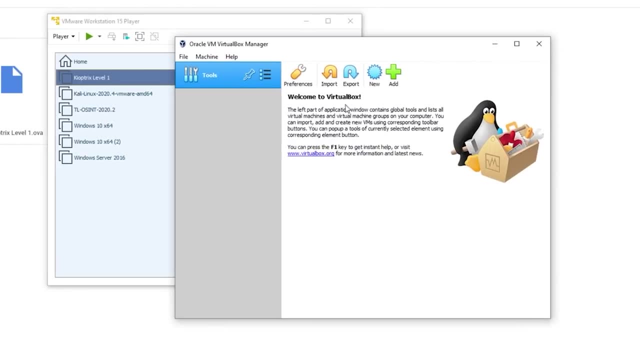 waiting. I'm going to go ahead and also do the same thing with VirtualBox. So I'm going to get VirtualBox going, And what we'll do here is a similar process. So we'll go to import and then we'll just select the area for our file. 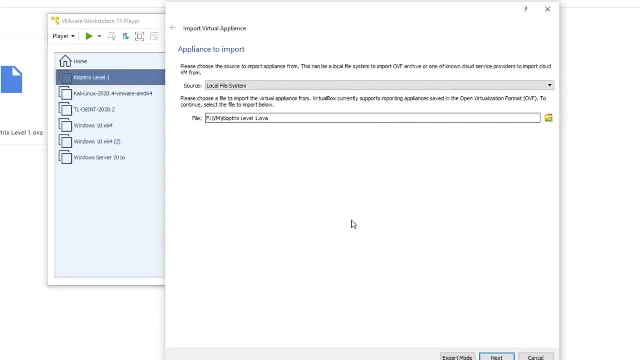 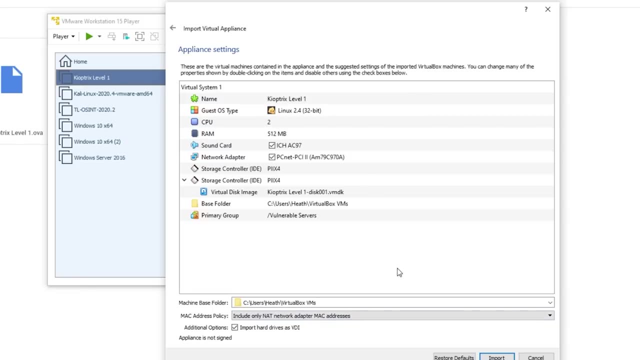 And I'm going to go ahead and select the area for our file. And we'll go ahead and select the area for our file and then we'll go ahead and select import And I'll hit next. And then it's going to ask me some questions here. We're just going. 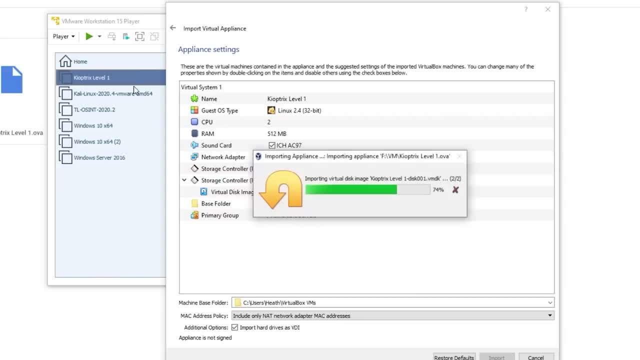 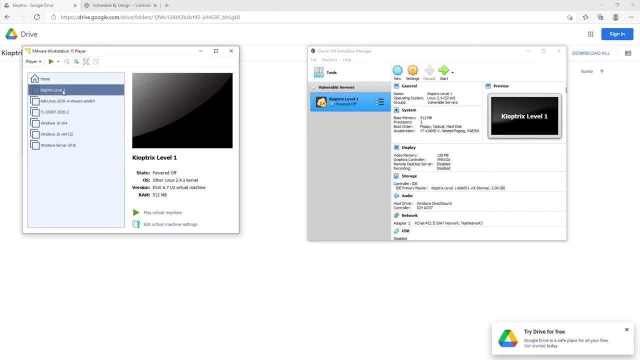 to hit next on this. we'll go ahead and set these up in a second. So I'm just going to say import And that'll be fine, Alright. so looking at the settings for both of these machines, I'm going to go ahead and drag this over here we can. 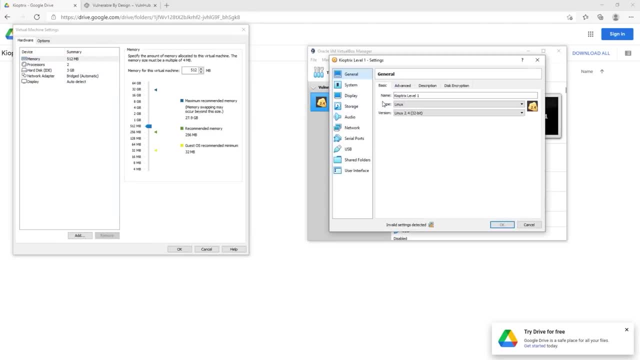 just right click and go to settings. Same thing here. you can right click and go to settings And we're going to set these up the same. So, either way. on 512 megabytes, this is fine. Honestly, if you wanted to kick. 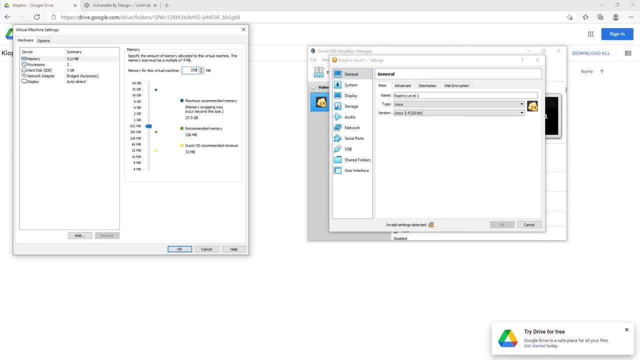 this down to 256, you could. I would not recommend going any lower than 256. Though- Oops, I did not mean to exit that, Though I will say that, if you have, I wouldn't go lower than 256, we're just gonna be running this in the background, But you. 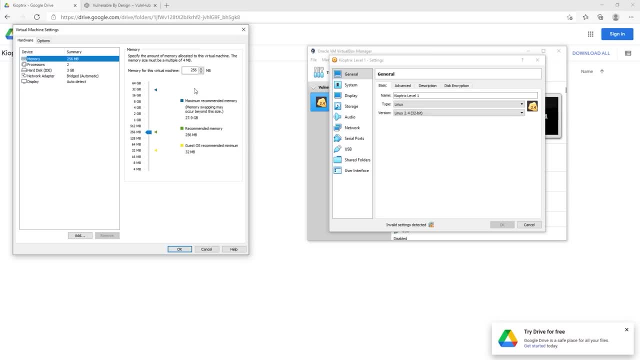 don't need to go higher either. So 256, I think is fine. If you want to give a 512, that's fine too, depending on the amount of RAM that you have on your actual machine. So 256 is good. And then here in the network adapter we're going to. 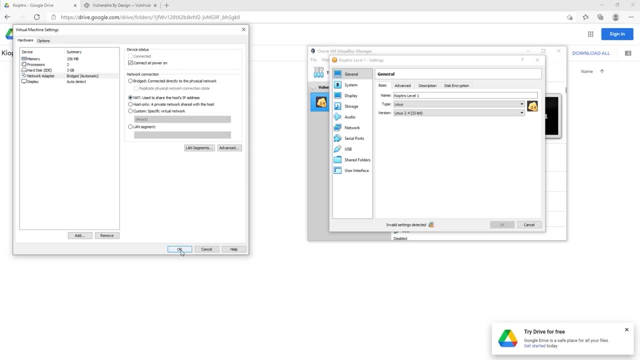 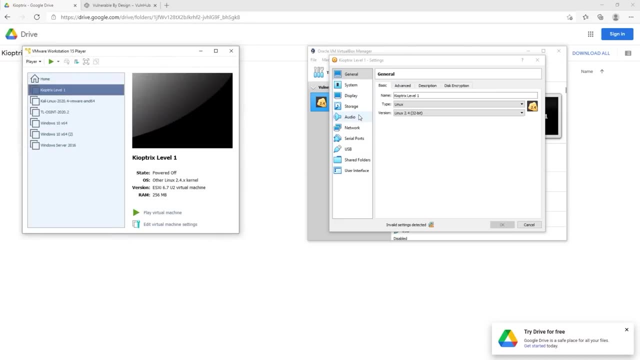 switch to NAT. Okay, so make sure you're good there and just hit OK, And that should be it. Same thing here. So if you want to switch the storage, you can, or the the amount of RAM allocated, you can. only big thing here is just going into the network And 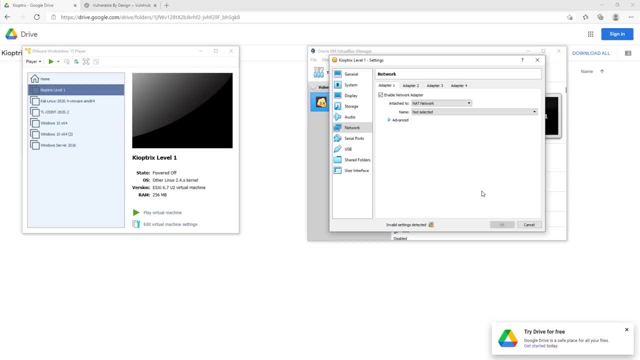 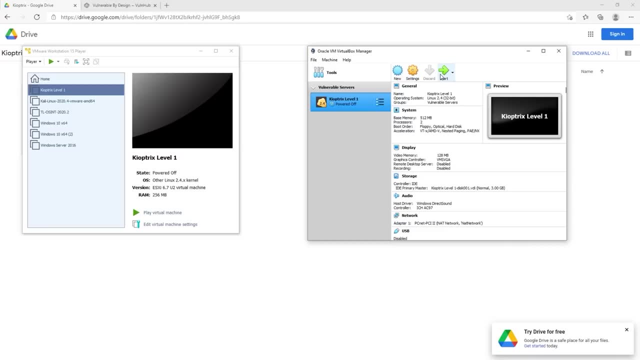 you can see that it says NAT network, And that's exactly what we want. Okay, so this box is set up, just fine, And then all you have to do on these is just hit play. Okay, all you got to do is power it on. you could just say: start here. 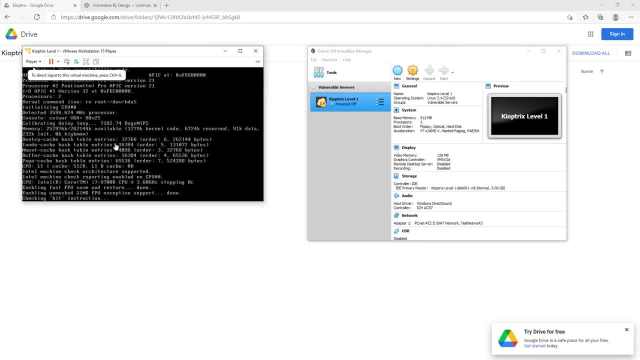 And I could just hit play here and both will start. All we're going to do is just let this run. So that's all you want to do at this point. you're just going to let it run. You can see, I've got. 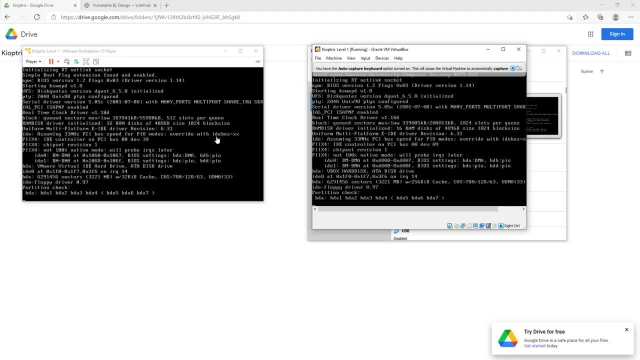 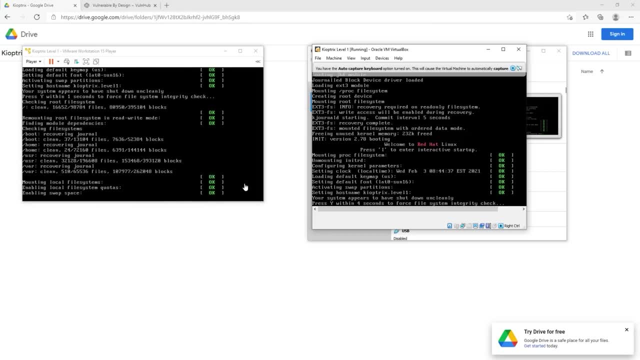 both machines booting, you will come to a login screen And that's when you know that this is ready, Okay, So when you're at the login screen it'll say, hey, key optics, blah, blah, blah, And then we're going to take it from there And we're going to figure. 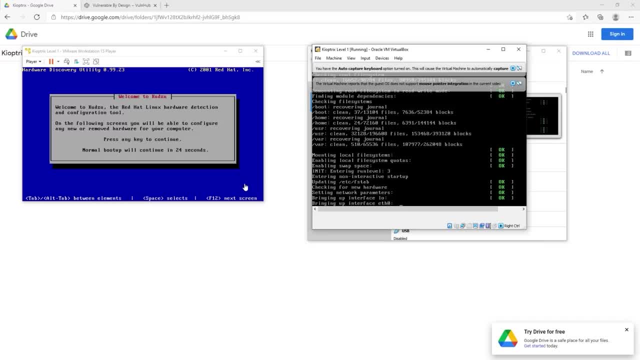 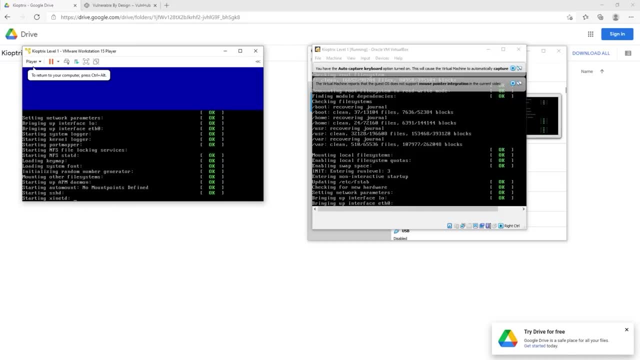 out how we can get into this machine. Okay, so if you get a screen like this, you can just say do nothing And just let this keep booting. But other than that, once this runs to a login, we're going to go ahead and move on to the next video. So you see this. 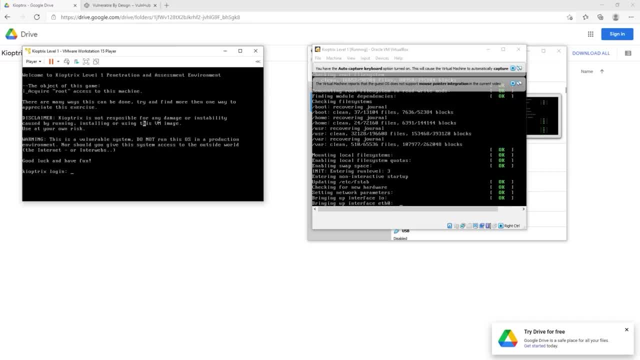 once you're at the login screen, you are good to go. Alright, and that is it. So I will catch you over in the next video as we walk through how to find this machine, And then we're going to start scanning it and tacking it and hopefully rooting it. So 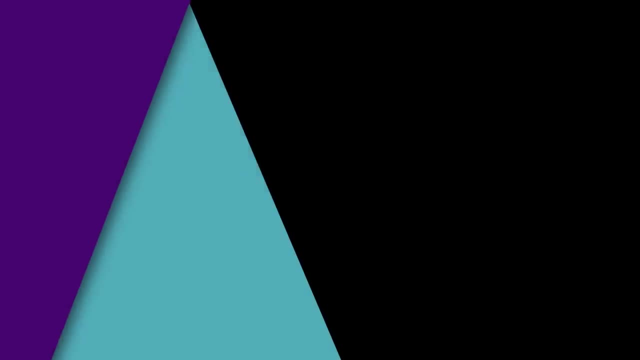 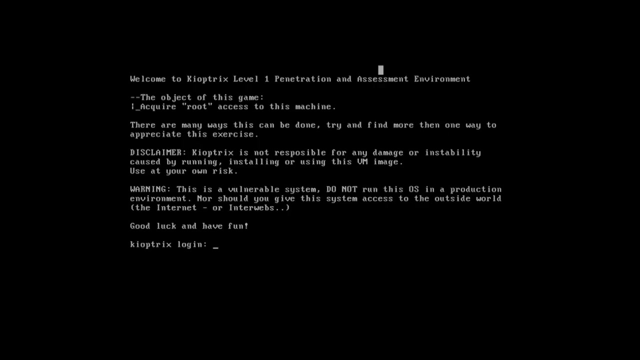 I'll catch you over in the next video. Hello everybody, and welcome to this section on Nmap. I'm actually recording this in 2020.. So the video you're going to see here shortly is from 2019.. We've had a little bit of issues with the command that. 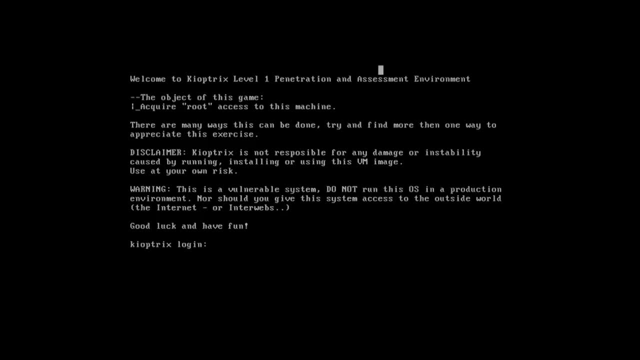 I show, which is net discover, on how to find your IP address of the key optics machine to actually be, begins scanning this machine. So I'm going to show you a couple of alternatives And then I'm going to let the video play as it was before And you'll have several. 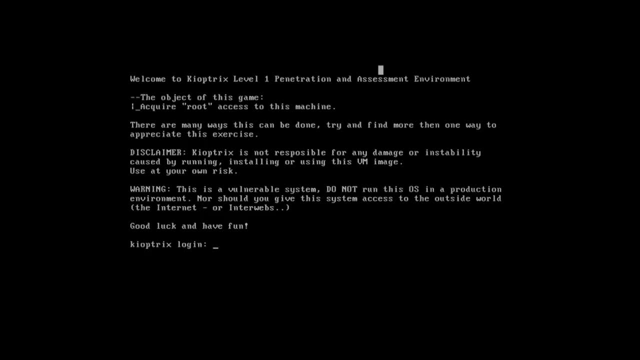 options on how to find your key optics machine and hopefully find IP address. So at this captures login page we can cheat just a little bit. So what I'm going to do is I'm actually going to give you a login here And just go ahead and type john as a login And 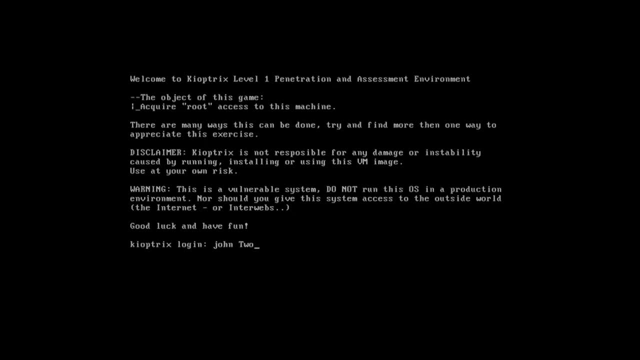 I'm going to show you the password before I delete it. The password is going to be two cows, to just like that t w o c o w s, two with the T and a C capitalized. So go ahead and type in john, and then two cows, two, And you can see. we are now logged in as john at key optics. Now this machine is. 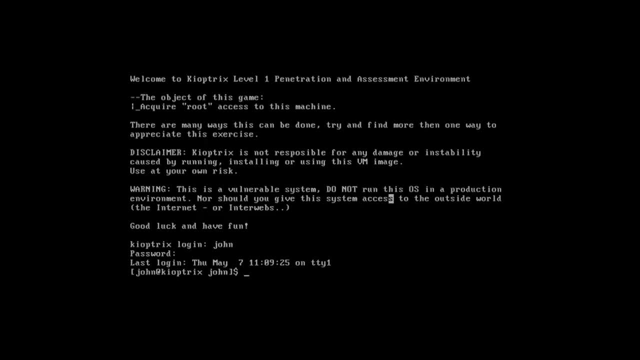 very, very old. So the typical if config or IPA or any of those do not work on this machine. However, we can do a quick ping, for example, to anything we want. we could say 8.8.8.8.. 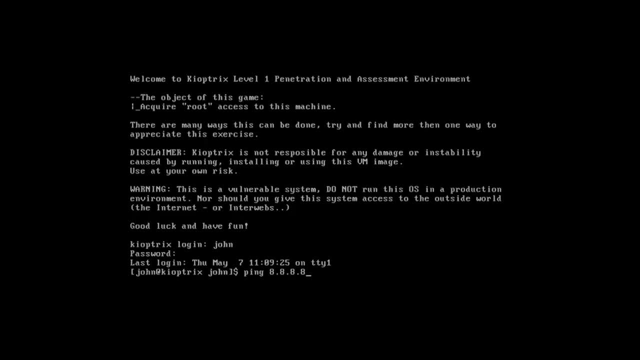 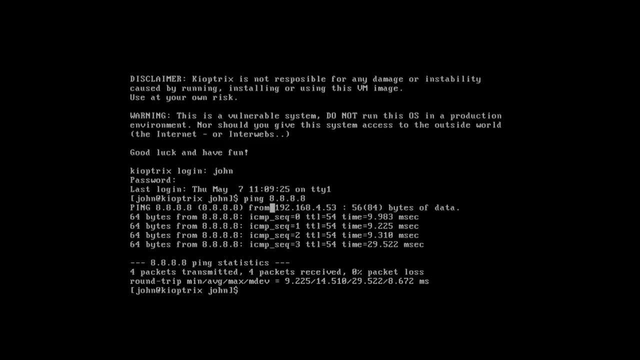 It could be an internal IP address. it doesn't even have to be an IP address. that resolves. But we could say ping, And as we ping I'm going to hit Ctrl C. here you can see that we see ping from 192.168.4.53.. That's my IP address. Now, the IP address you're going to see here in the 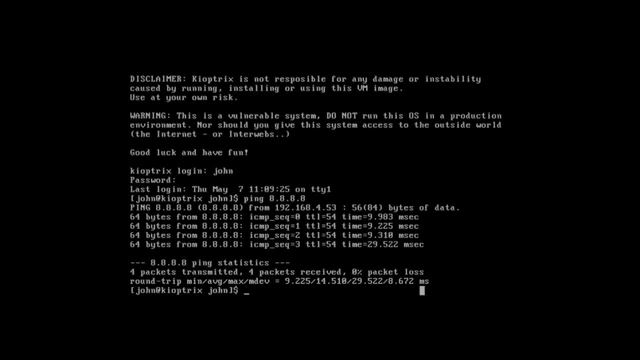 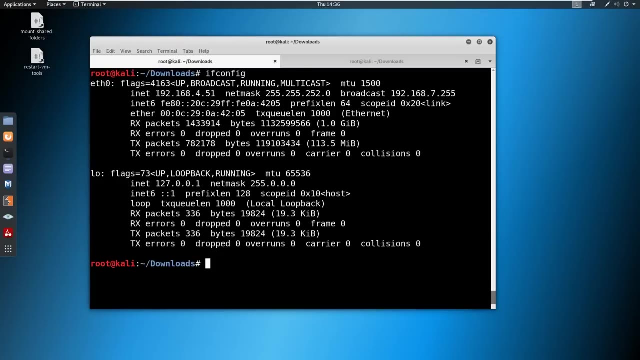 video shortly is going to change. However, as of right now, the IP address I'm seeing for captrix is 4.53.. Now we also use net discover, but there's actually a cool tool we can utilize as well. Now, if we come into the network, you can see that I have a IP address of 192.168.4.51 for. 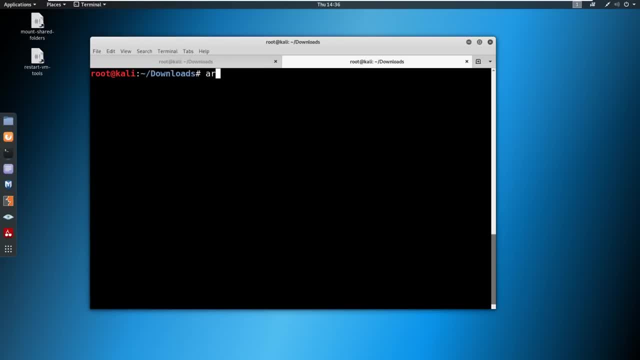 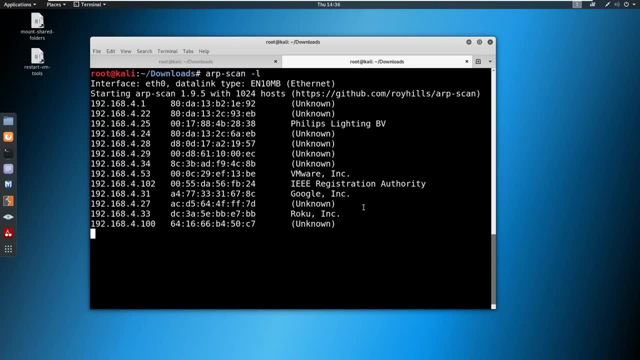 myself. Now there is a tool built into Kali Linux that is called ARP scan, And you could do a syntax of a dash L with that. hit enter and it's going to pull off an ARP scan as well, which is what net discover is doing. 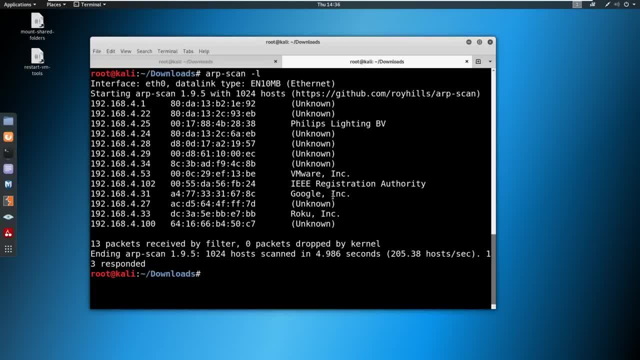 What we need to be looking for- and you could see this is kind of my home network. What we need to be looking for is VMware. you could see VMware is sitting here at 192.168.4.53.. The only one to be on the lookout for is possibly yourself, which were at 51.. I don't see in this. 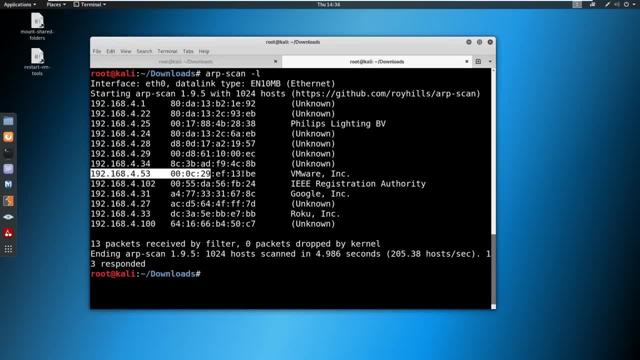 list. it didn't pick us up, So I could see 192.168.4.53.. So if you're using a virtual box or something like that, it should show up here, So kind of identify. either this way or you can come in and identify it through the key object login itself. 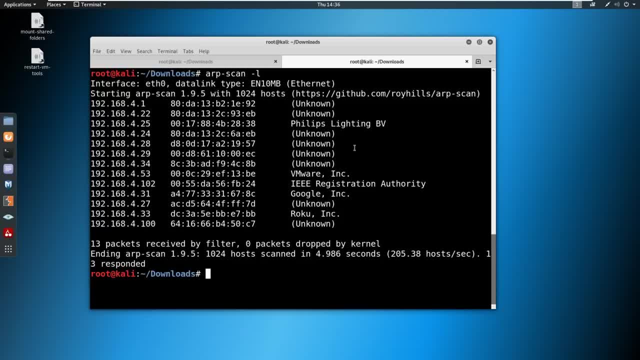 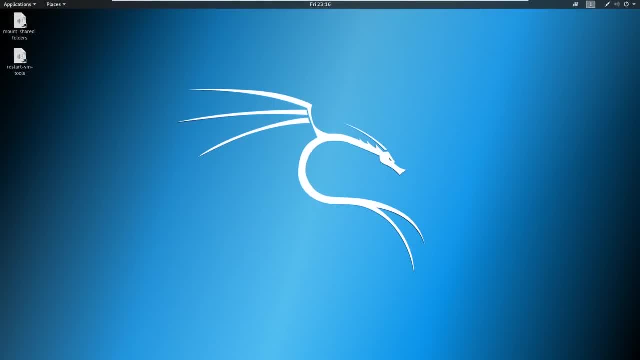 Of course, you can use net discover, as shown in the video. So, without further ado, let's go ahead and go into the video on scanning with Nmap. Okay, so now we have key objects up and running. we need to determine where it actually is, And then we can do a little bit of scanning. 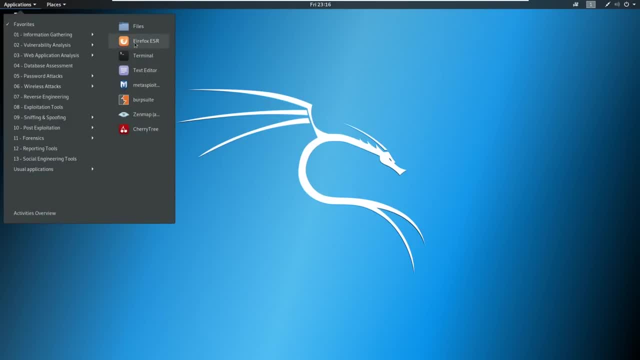 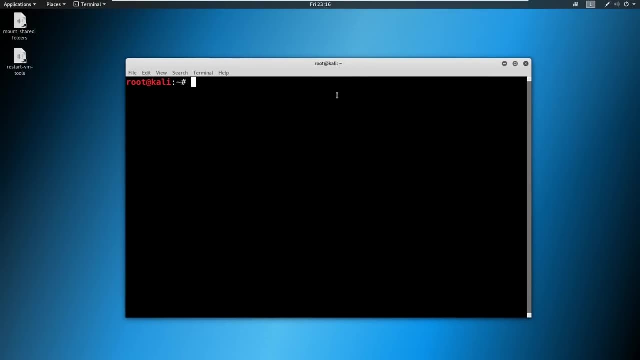 So what we're going to do is we're going to go up and down the network And we're going to go up and up into our applications and open our terminal- I'm just gonna make this a little bit bigger- And we're going to run a tool called net discover. So before we can do that, we need to type in if. 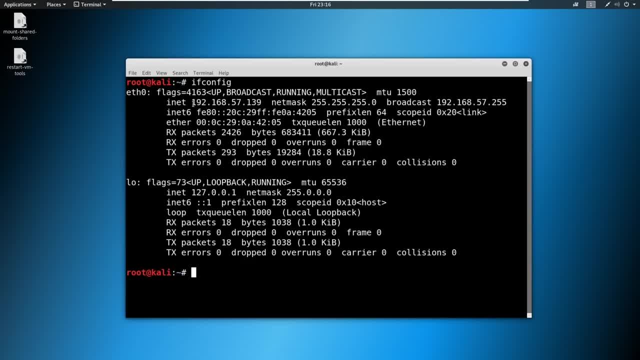 config and identify your IP address. So I'm just going to go ahead and copy this first three octets here And we're going to run net discover. So net discover is going to look like this: we're going to say net discover, we're going to do a dash R for range. 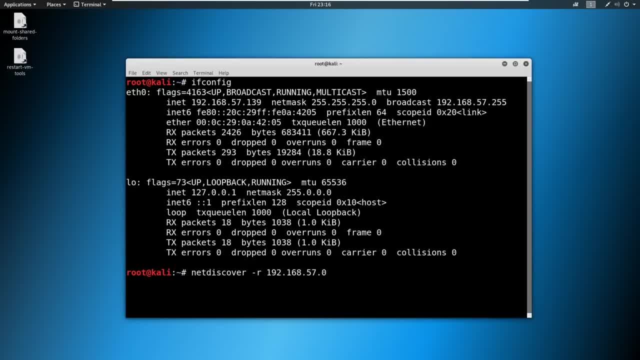 we're going to paste in this and do a dot zero, slash 24.. So what are we doing? we are going to be using ARP to detect all the machines on the network. So you should be familiar with ARP from the Linux lessons and from the networking lessons. So we're going to attempt to use ARP to address 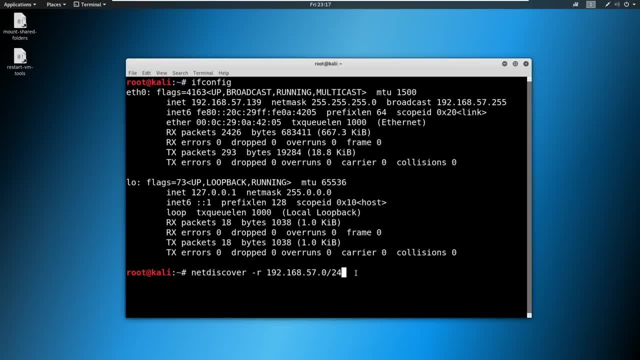 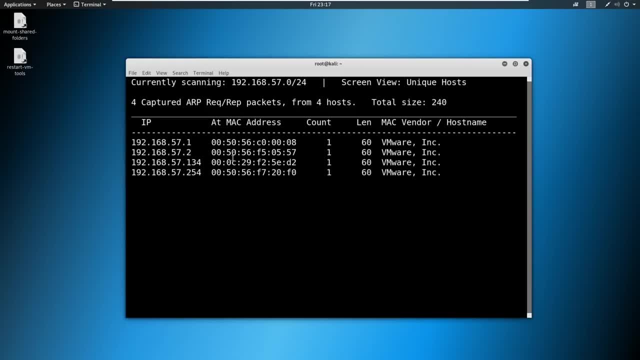 anything on the network And we're sweeping the entire subnet of slash 24.. So I'm gonna go ahead and hit enter And in a second here our machine should start popping up and it does So. remember our host was at 139.. This host here. 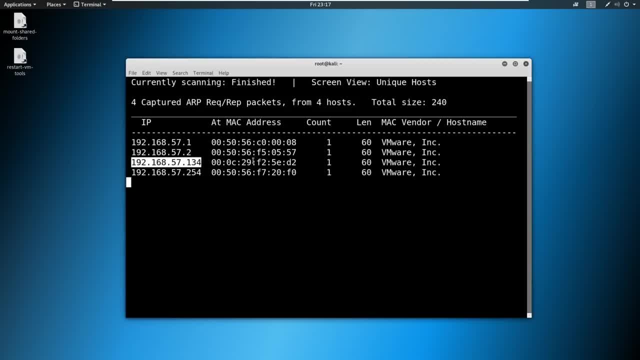 at 134 is likely our culprit. So you should only have two machines in network. because we're only running two, you can ignore dot one, dot two and dot 254.. We are only focusing on the one that looks similar to ours, which is 192.168.57.134.. So now we know our machine address, we can start attacking. 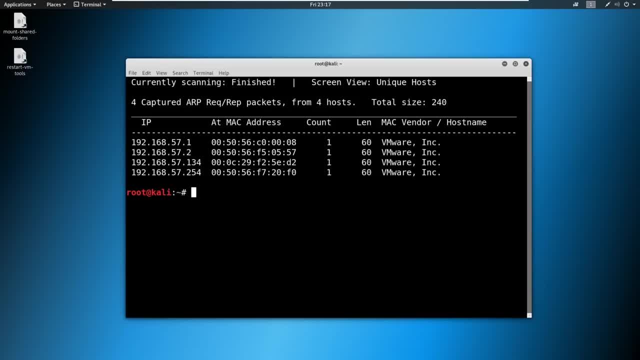 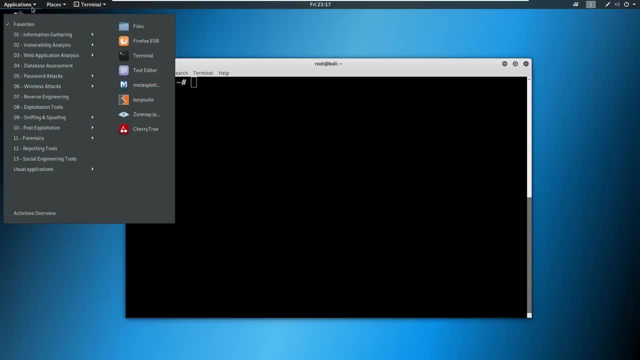 it. So I'm going to go ahead and hit enter And I'm gonna hit CTRL c, which is going to kill this session here, And I'm gonna hit CTRL l to clear my screen. Alright, so I'm going to open up a notepad and we'll just store this away. for a rainy day we need to. 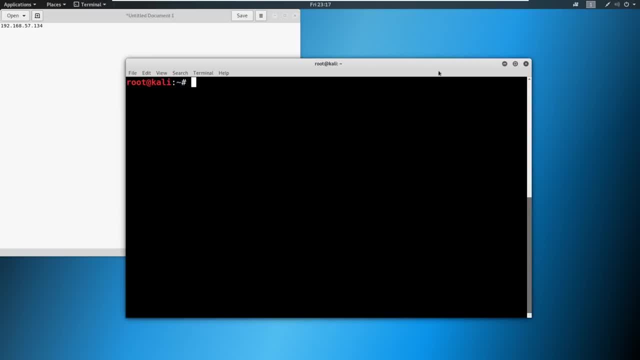 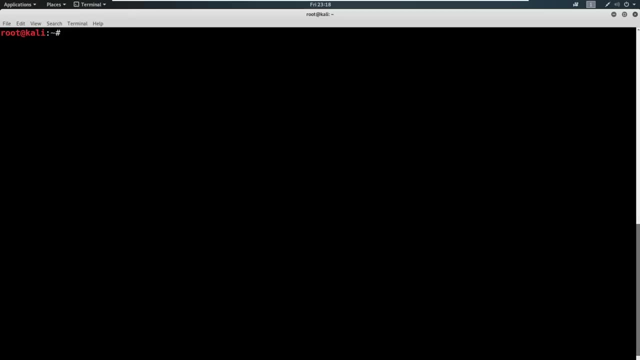 first talk about what we're going to be doing here. So remember before when we ran our TCP three way handshake, we had something like sin, SYNACK and AK Right, And we can just say SYNACKX and we will then run the. 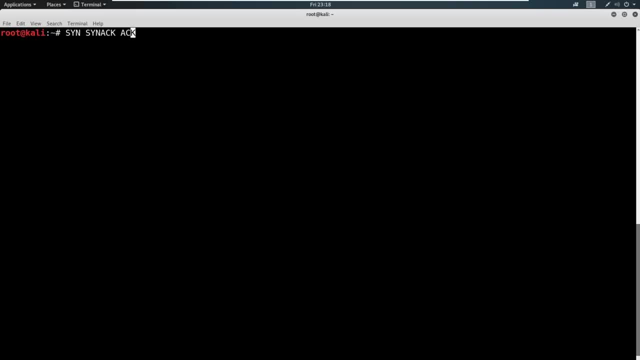 of like this, to combine it. So we've got three parts. We've got the part where we reach out to a port and we say, Hey, port, are you open? And the port says, Yeah, I'm open, Let's go ahead. and 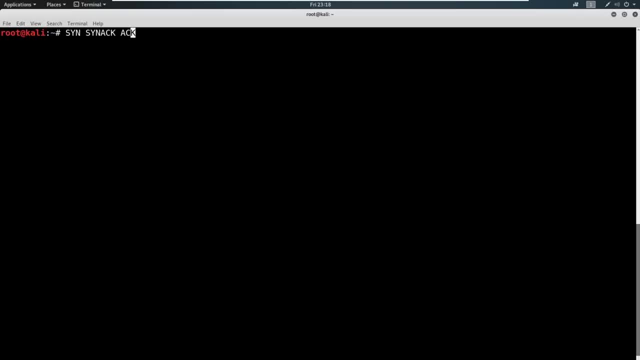 make that connection And then we go ahead and connect to it. So what we're going to be doing is we're going to be using a tool called n map, And n map stands for network mapper. Now, what network mapper is going to go out and do is is going to scan for open ports and services. Now, 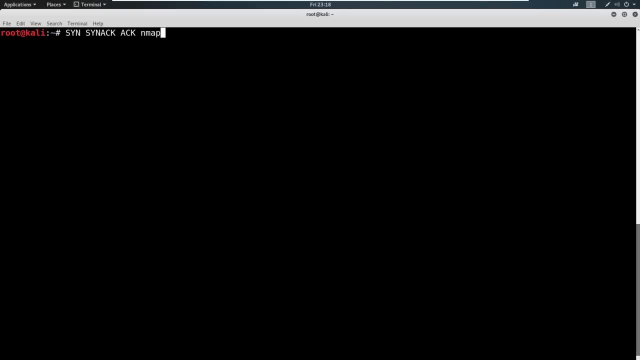 this scanning is going to take place And it's going to identify these open ports with something similar to this three way handshake, So we're just going to modify it a little bit. Now, what the process that we're doing is called stealth scanning, And it used to be written out like this: 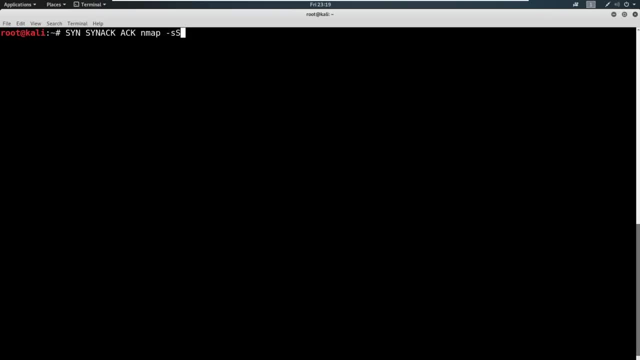 Now it's just done by default And we'll get to the switches here in a second, Don't worry about that. just we're going to be running stealth scanning, And now the stealth scanning used to be stealthy, right. That's why they called it stealth scanning, because it used to be. 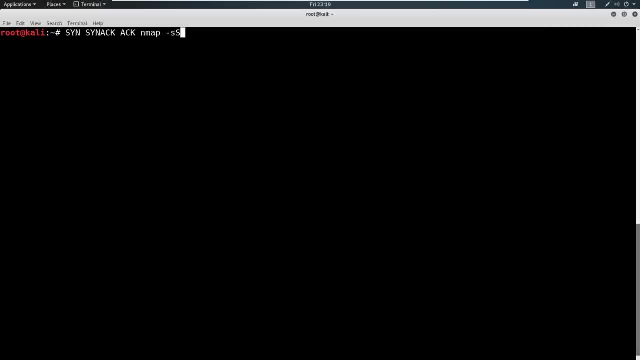 undetectable Nowadays very detectable. If you run n map in a network that has good security, you're going to get picked up, Although, being a pen tester, I would say n map probably doesn't get picked up in 80% of the assessments that I run, So don't expect clients to be running good. 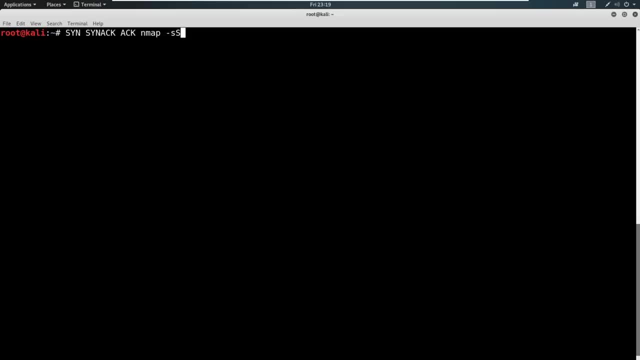 security. But just know that even though it says stealth, it's not stealthy at all. So the stealth scanning, why was it stealthy? Why was it called this? Well, if we go back to the three way handshake, what the stealth scan does is it does the sin, says: Hey, I want to connect to you And the open. 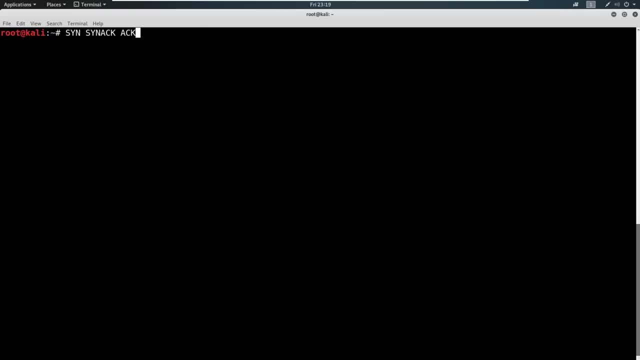 port if it's open. we'll say, yeah, I want to make that connection back with your friend. And what's going to happen is we're just going to say- you know what? I'm just kidding, I'm going to send over this reset flag. So this RST, Why? Well, that means we don't actually establish a connection. So 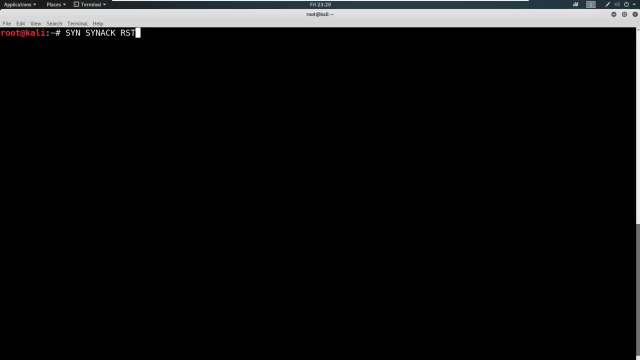 like when you go out to a website and you go to Google and Google loads. well, guess what? you establish that connection. you establish that three way handshake. what we're doing is we're going out and we're saying, Hey, I want to establish connection. 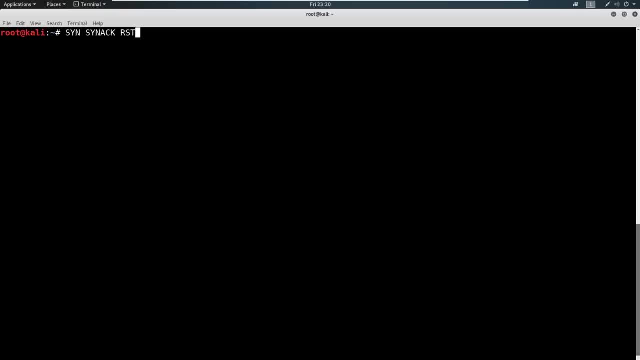 the port reveals to us that, yes, I am open for connection, And then we're going to say, just kidding, let's not make that connection Because we never established that connection, then it was technically stealthy. So that's what we're going out, we're doing, We're never making. 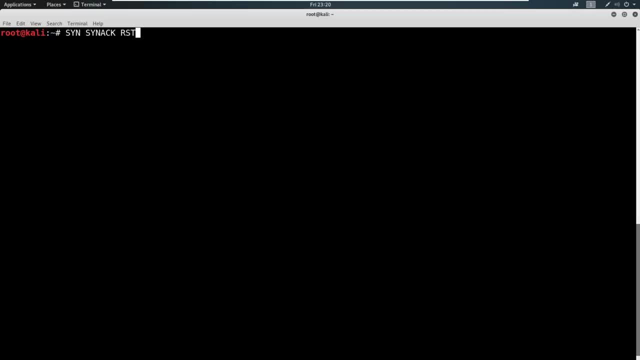 connections, these ports, but this is how we're identifying them as open. So we're going to use a tool, and we're going to use a tool like this. we're going to say and map and we're going to say something along the lines of dash t four, dash P, dash dash a. Now 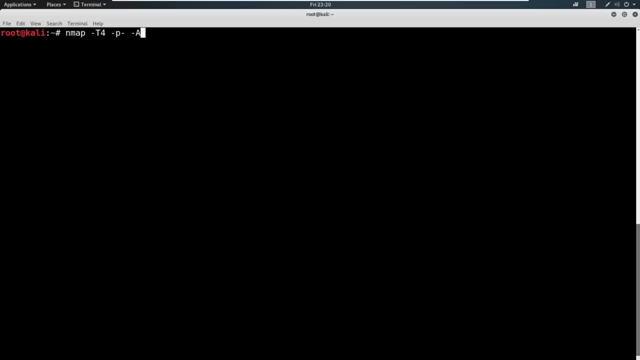 you have no idea what this means And I don't expect you to, but I'm going to walk you through these. And what we're doing here is we're saying, hey and map, I have a choice and speed, and that choice and speed can be between a one and a five. one's really slow and fives really fast. 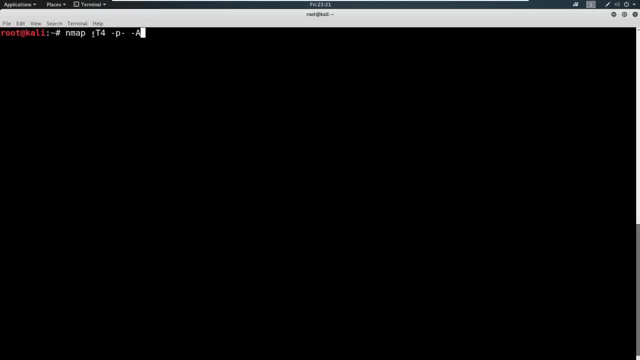 Now the default for me has always been- for now I'm teaching you my preference- it's always been four Okay, And we utilize this in I think five. five is okay, but five kind of fast. maybe you're going to miss something, maybe it gets caught. the slower the better in terms. 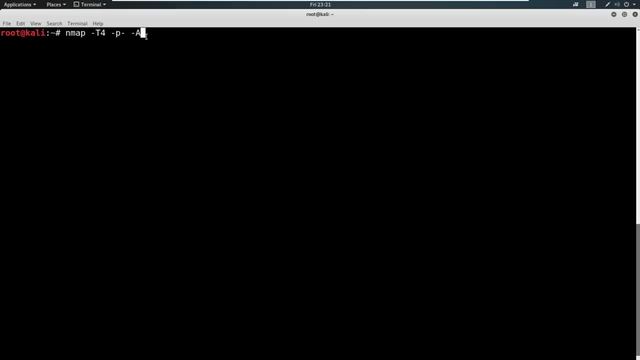 of detection. But in the instance that we're going to be running it through, this course we're going to use, for anytime you do like a bone hub or something like a hack the box which you're going to see here in a few videos. you're going to run t four just because you're. 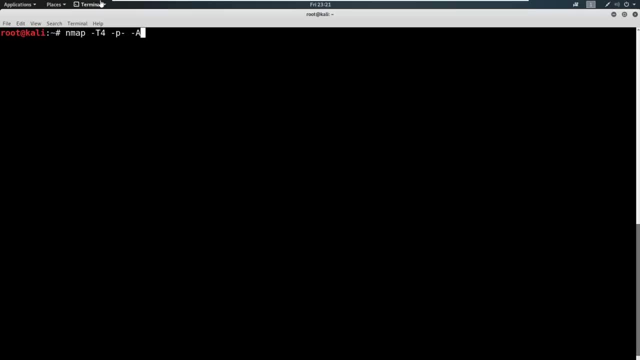 not worried about this detection. you're not worried about anything. So t four is speed purpose. Now dash p, dash- well, this stands for I want to scan all ports. Okay, we could say something like dash p, or we could just have dash p left off completely. Now, if we leave off, 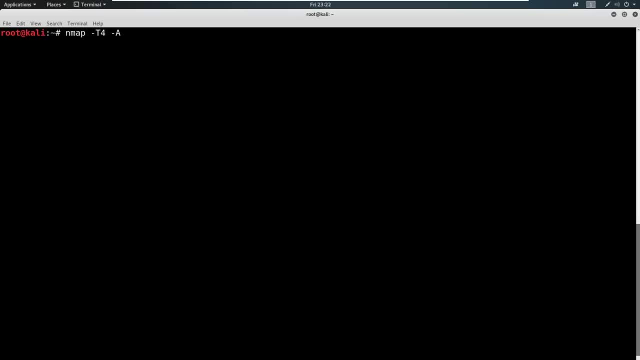 dash p completely. it's going to scan what are known as the top 1000 ports. The top 1000 ports are your most common ports, So think of, like port 80, port 443, 139, 445, all the ports that we covered in the networking section. 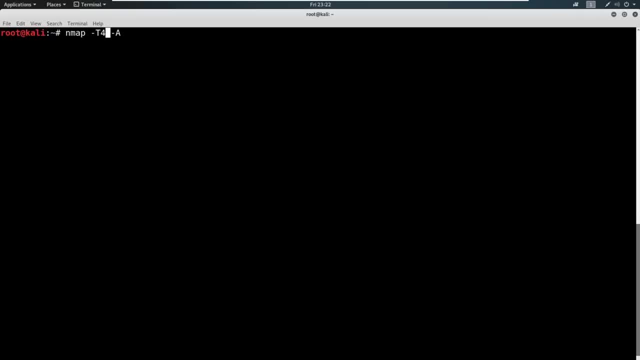 going to show up again here, But there are 65,535 ports out there. we want to scan every single one of those, because what if, for example, there is a service running on port 47,700? Well, that's not. 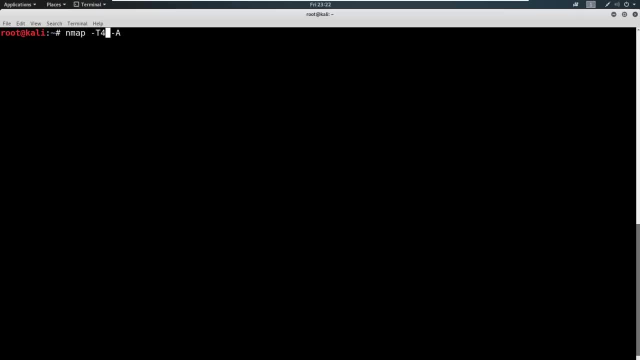 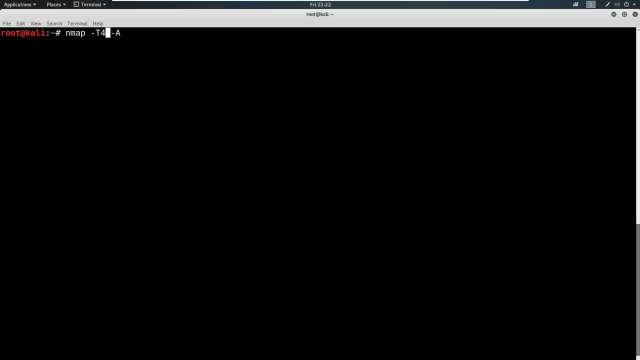 miss that port And that could be something incredibly valuable to us, right? So I always scan like this: dash p dash. you can also do things like scan specific ports. you could say like 443.. Or say you wanted to scan just for web servers. you could do 80, 443, something like that. 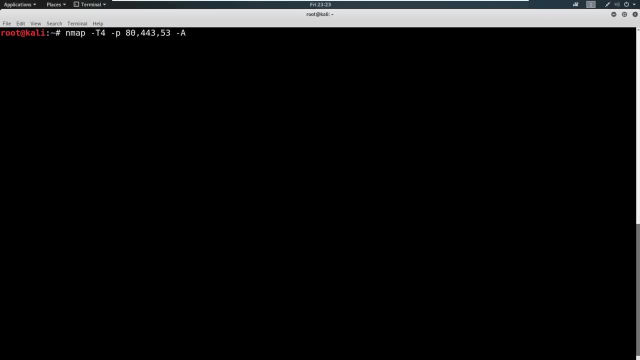 Or you can mix in, say you want to scan for DNS as well. you can add in 53, etc. you can scan for specifics And we're going to get into that in a little bit of a later video on why we might do. 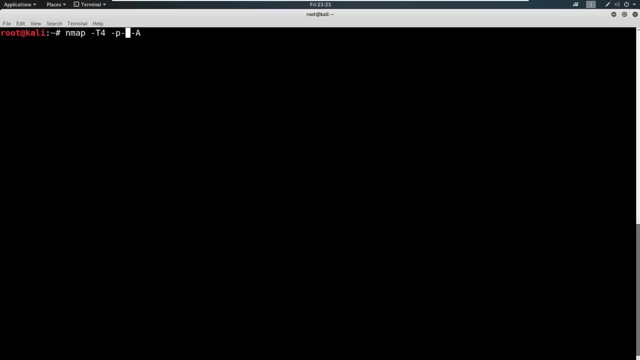 it this way, But for now, for the beginner lesson, dash p, dash. we're going to scan everything And lastly, we've got this dash a in here, So dash a stands for everything. I want to scan all of it. 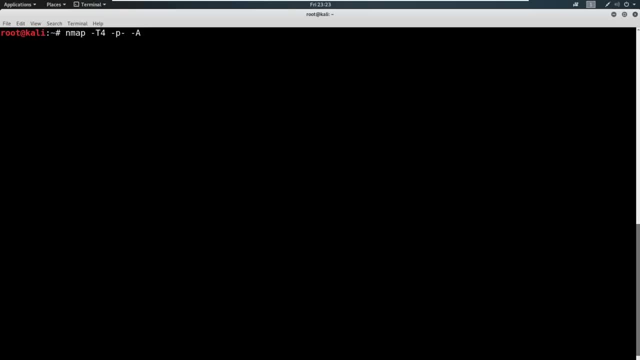 I want you to tell me. I want you to tell me the version information, the operating system information, anything you can tell me, fingerprinting, etc. Now, this may all be confusing. it's going to make a lot more sense when you see a scan. 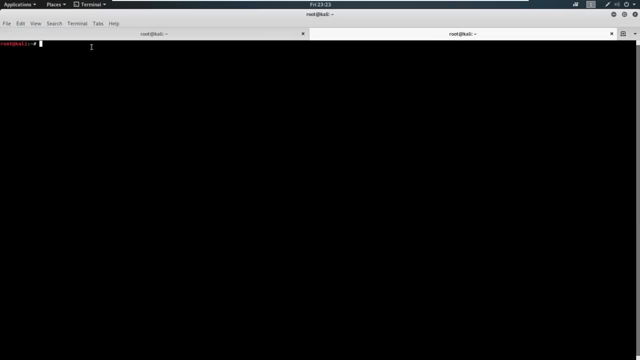 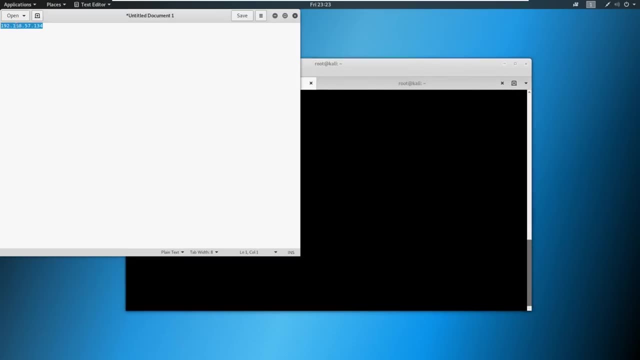 I'm going to go ahead and open up a new tab, And what I want you to do- let's go ahead, and I'm going to blow this up for us- And what I want you to do is I want you to go ahead and start running the scan while we wait. So go ahead and copy this here. And the last thing: 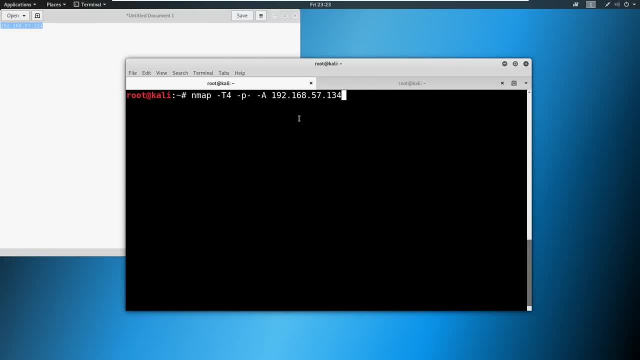 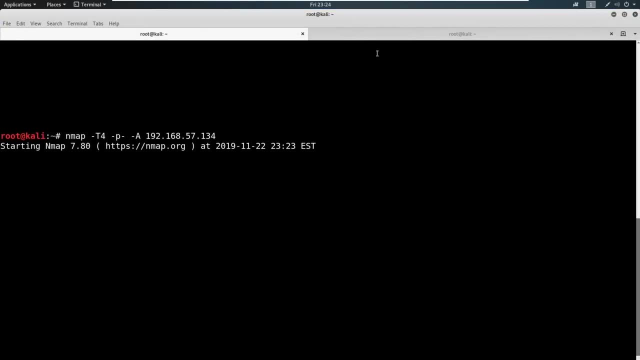 we're going to do is we're going to put in our IP address And that's how it knows what to scan. We're just going to hit enter on that And now we're scanning. So from here, what we're going to do is we're going to take this and I want to run m app again. 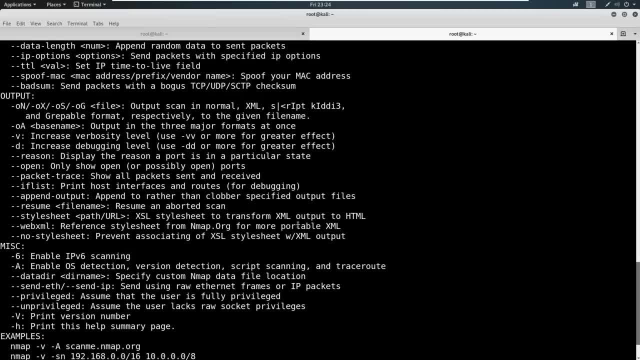 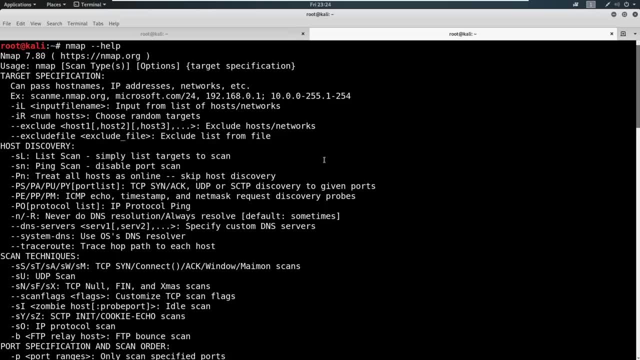 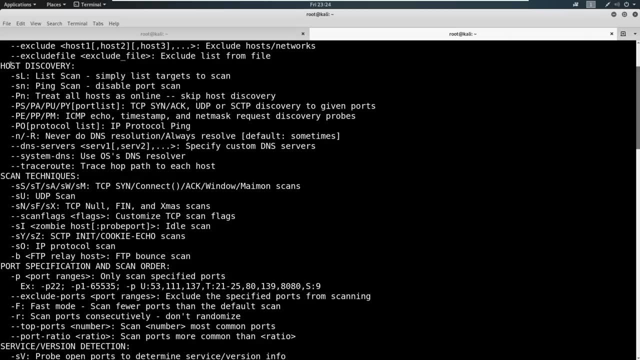 dash dash help, And I want to talk through some of these settings in here so that you understand fully what we're doing Now. dash dash help is always great. As I said before, man pages are good as well, But let's talk about some things here. So we've got this host. discovery section. 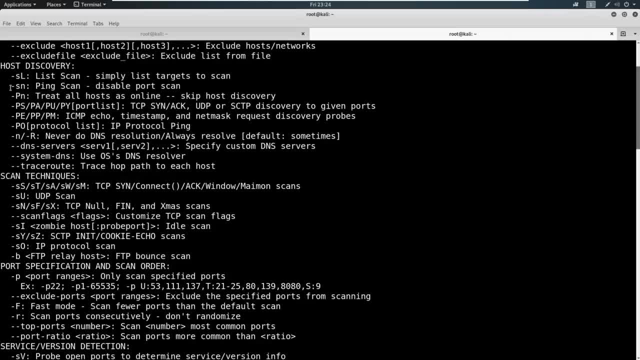 which we're really not going to use in this course. But this is good for say dash and say you want to do a ping sweep of the network. Well, you can do a ping scan right where you're going to just sweep an entire subnet- slash 24,, for example- and see what's up. very quick, a dash PN. 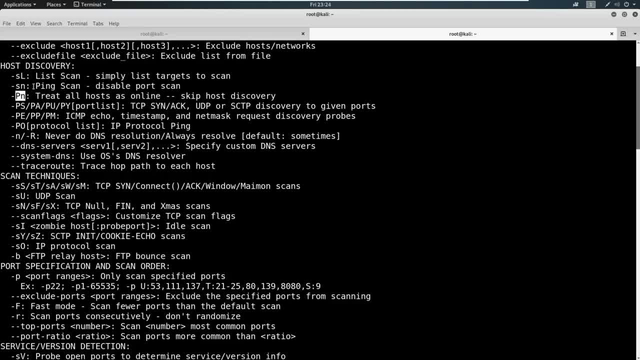 maybe the host isn't acting like it's online, but you know it's there for sure. You can say dash PN. and you can say Hey, I want to leave all the hosts. or treat all the hosts as if they're online. 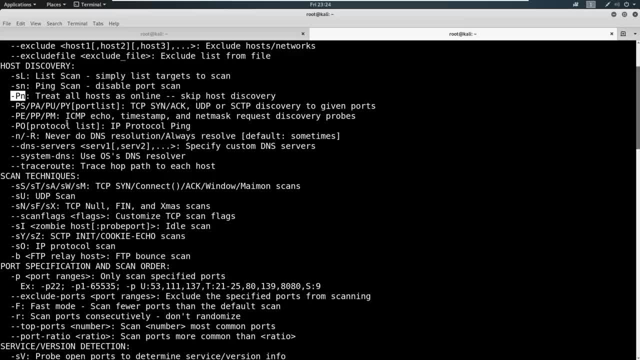 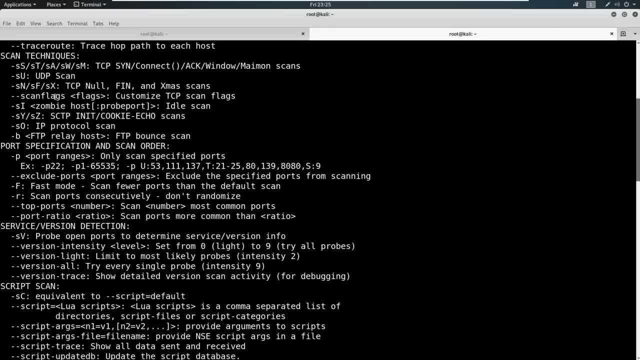 even if they're not responding to my ping request or anything. So make yourself familiar with this kind of stuff. This is interesting And we'll cover a lot of this as we go in the course, But just for the first time, we're going to go ahead and do a ping sweep of the network, So we're going. 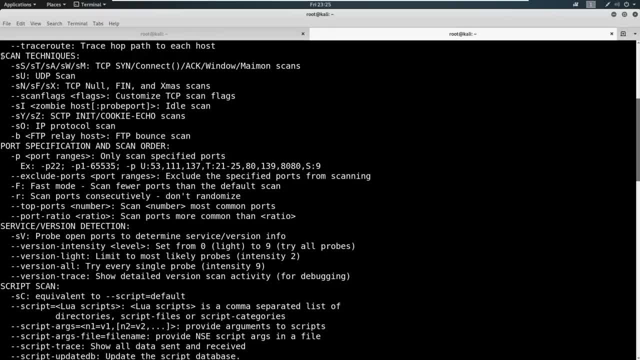 to just walk through while we're scanning. I think this is super important. Now scan techniques, this dash SS- this comes back into play. TCP sin is what it's called, but it's also known as the stealth scan. There's all these other types of scans. you're not going to need them. I there's. 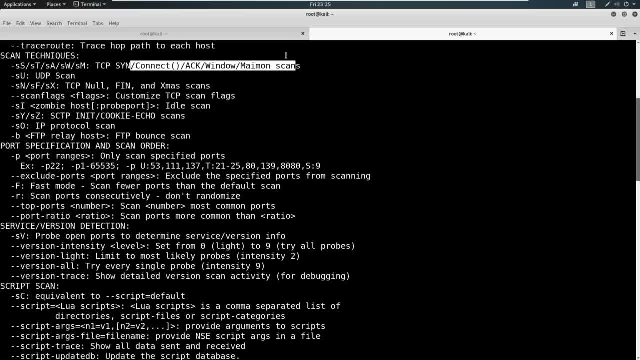 only maybe one scan out of all these. that may be useful, but you're not going to need them through this course And you're probably never use anything but the SS and the su 99% of the time. So for the scope of this course, we're going to go ahead and do a ping sweep of the network And we're going 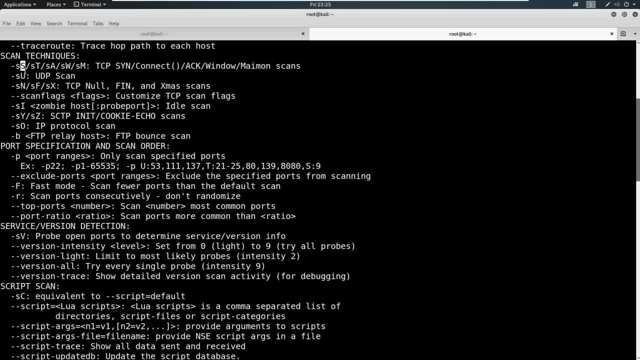 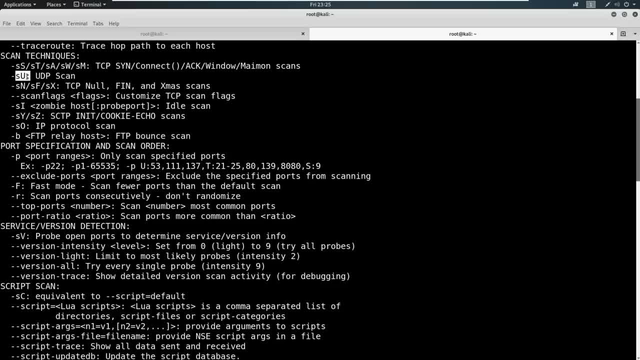 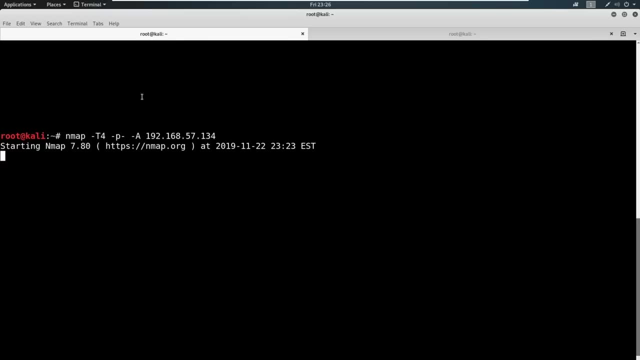 we talked about TCP. Well, guess what? there's also UDP, And there's 65,535 ports over there as well that we have to scan. Now, UDP is a connection less protocol. So what we're going to do when we scan it? let's go back to this scan. what we're going to do when we scan it is: we're going to 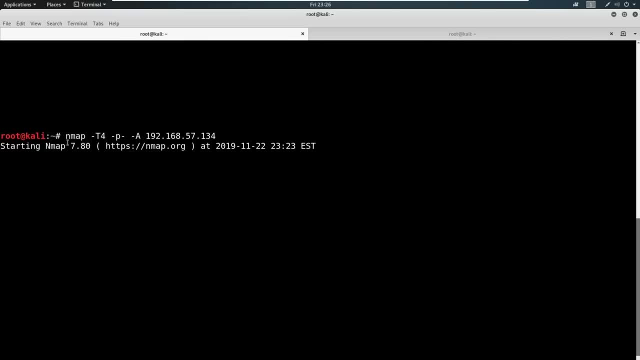 actually do that su in here and I'll copy the syntax and just move it to the next one. So we're going to do it over So it looks a little cleaner. We're going to say something like we can put it anywhere we want, the order doesn't matter. But we can say something like dash su to. 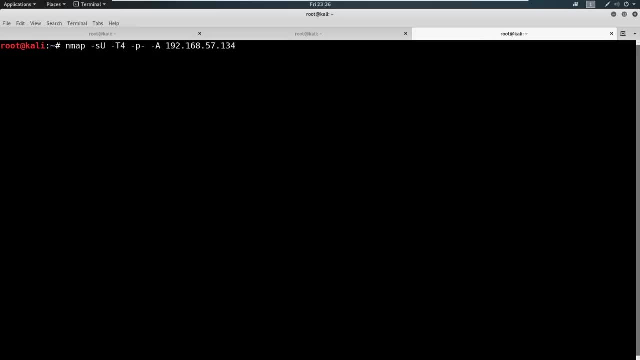 scan for UDP And the one little change that I make here, two changes actually. I take off the dash a and I do a dash p, dash. why do I do a dash p? I should say, why do I do this? I do this. 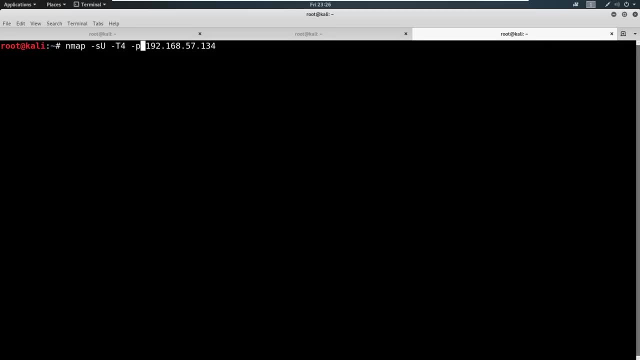 because UDP takes for ever to scan, absolutely forever to scan, Because it is a connectionless protocol. it does not have that instant response time. So when we scan UDP, typically we scan the top 1000.. That is my recommendation to you, or else you will be. 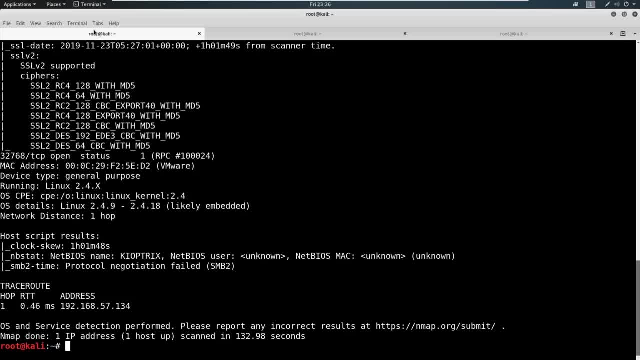 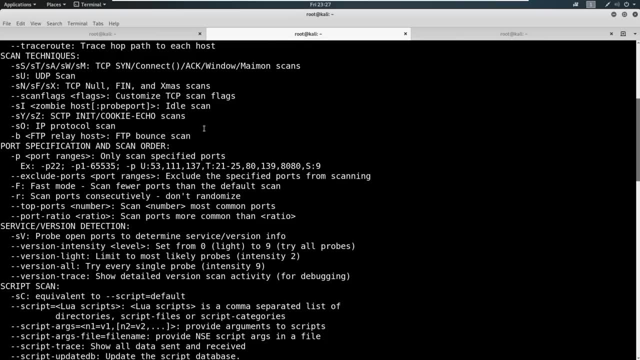 sitting here waiting for hours upon hours for a scan to finish. See now, our scan over here is already finished. If I were to run this UDP with the same thing, it will take forever Going back into this before we get into the scan. You can see here that we can specify dash p of port. 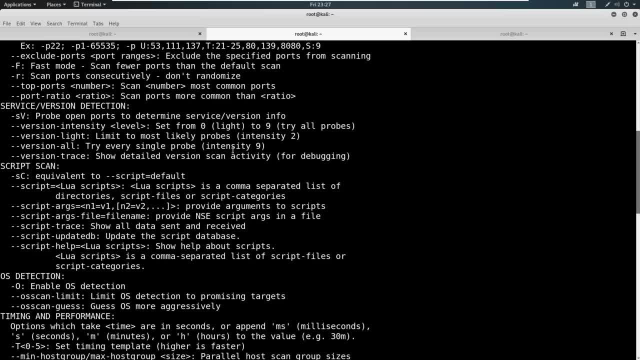 that's going to be very common for us. But here's where I really want to get into. We're doing a dash SV, a dash SC, a dash O here, all with the dash a, okay. so we're probing open ports for service information. we could say dash. 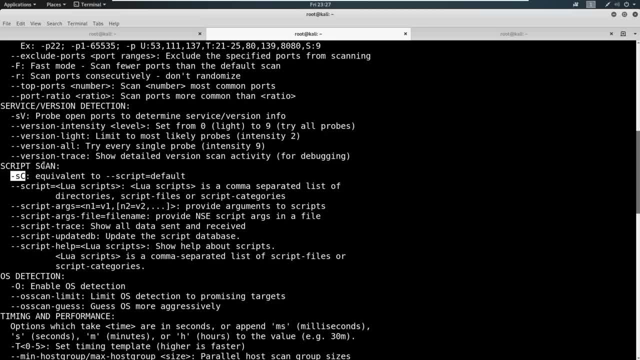 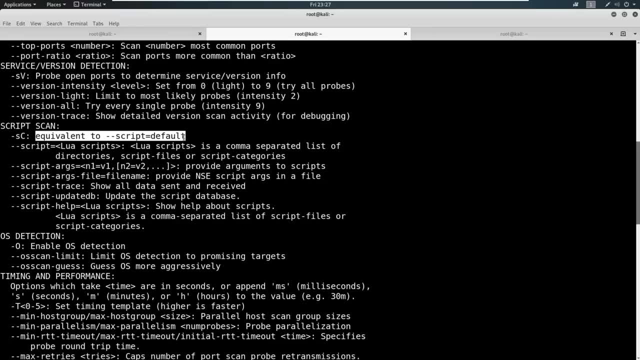 SV and we can say dash SC or we could pick these. you know one or the other, a mixture of some of these. But we can also do script scanning, which we'll get into script scanning here in a little bit as well. But we can do OS detection, where it goes out and it tries to define an operation. 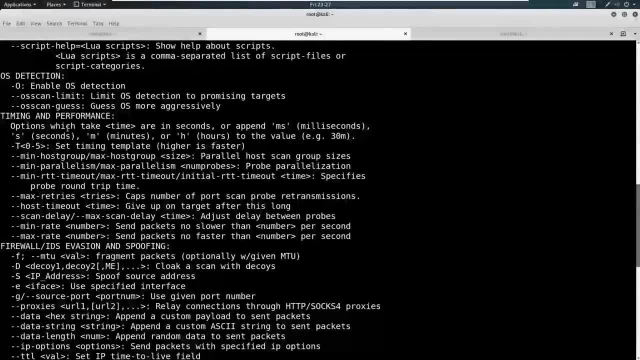 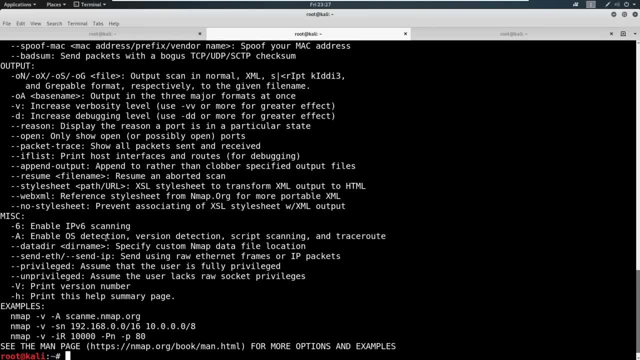 So we're going to use the operating system And you're going to see all this with our scan. But when we use dash a, it does it all for us. So why- why not use dash a? So you can see it does OS. 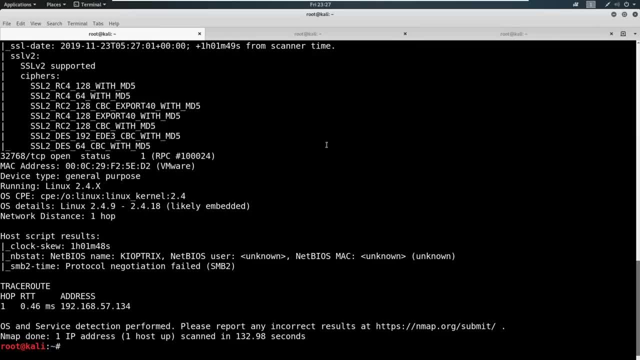 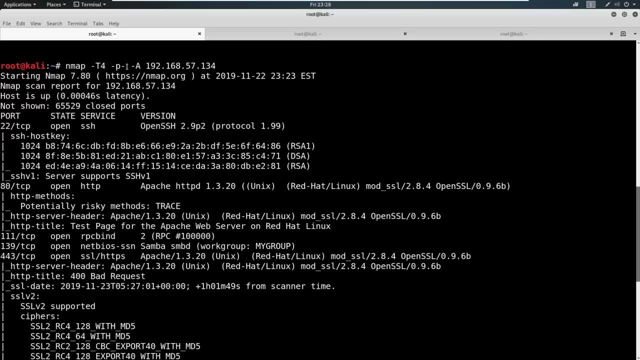 detection version, detection script, scanning and traceroute. Now there's one caveat to dash a and we're going to talk about this in another video. in a thought process, It is much faster to remove the dash a and scan a dash p dash. Typically that'll come back much, much, much faster. 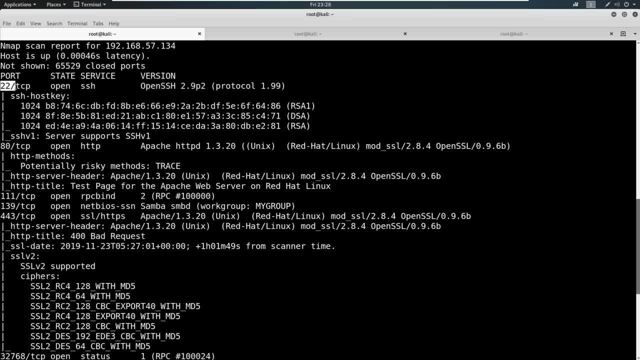 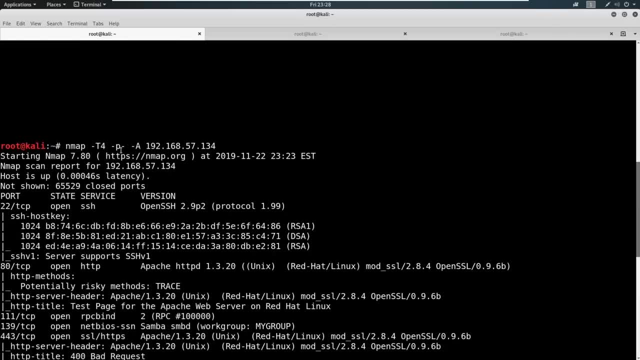 You can do is you can define the open port So say there's port 22,, port 80. Okay, just go through this. you can specify those ports specifically. you could say dash p, like we did an example earlier with 80 and 443. And then do a dash a on those. Now that will just scan only the specific. 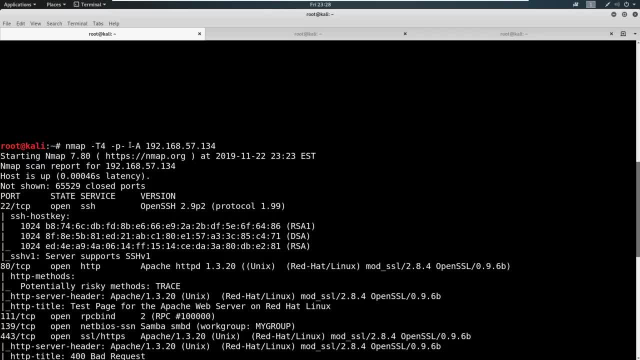 ports with all, instead of going out to every single port and attempting to do all on every single port. It's just a little bit faster Now if your wheels are spinning and you're thinking about it. maybe even you can script this. right, you can script something to say: hey n map, I want to. 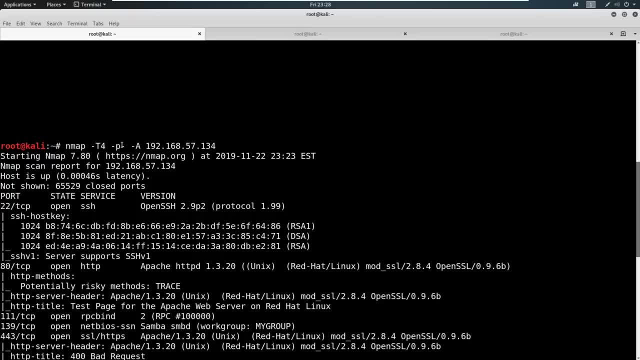 take. I want to take these ports from a basic scan. anything that you pull back, and I'm going to go ahead and I'm going to run a new scan on it with the dash a only specifying the ports that we found. That gets your wheels spinning. This is where scripting becomes important. If you want an. improvement on speed For me personally. I've never, ever done that. I don't think for me personally, that it's made much of a difference. I just let my scans run as they run And I work on other things. while scans are running, there's plenty of time to do other. 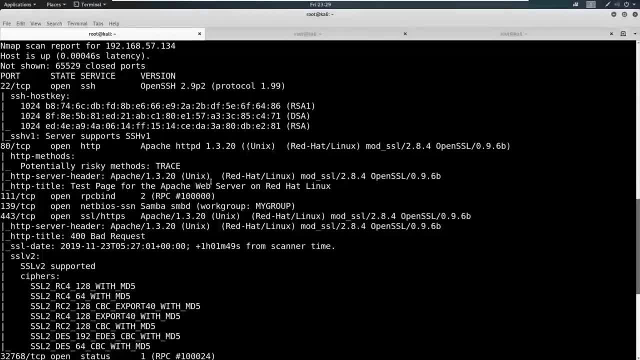 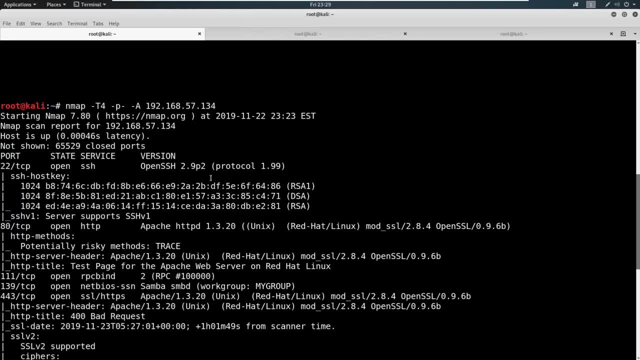 things while you're doing your scanning. So, and typically another thing to note is typically we're doing scanning when we're doing our OSINT as well. So if we start up a client assessment, one of the first things I'm going to do is probably kick off a NASA scan or an n map scan. 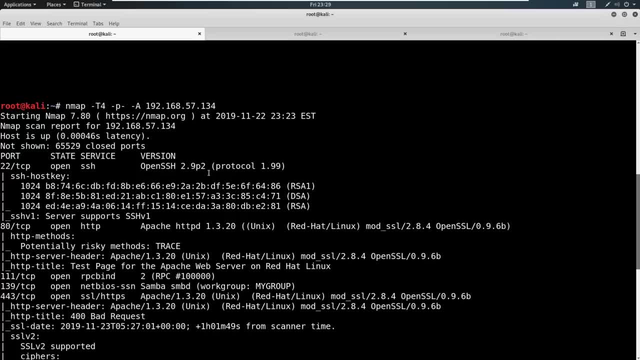 And while I'm doing that, I'm going to go look for those breach credentials, or I'm going to look for that juicy information on Google or social media or where I can find it and utilize that time while this is scanning, or else I'll just be sitting on my hands doing. 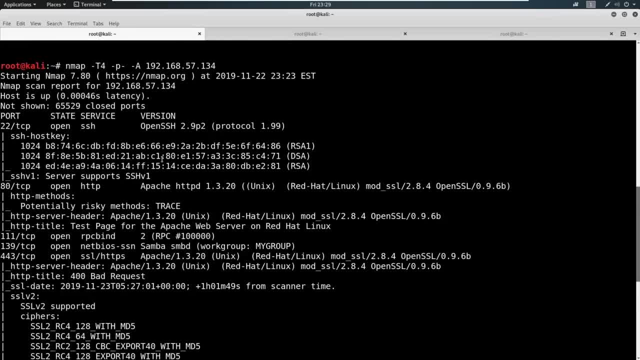 nothing while these wait. So we're going to take this information now and we're going to start reviewing it. So we have here our scan results And you can see the scan results come back And the first thing we notice are open ports. That's what we're want to look at. we want to look at 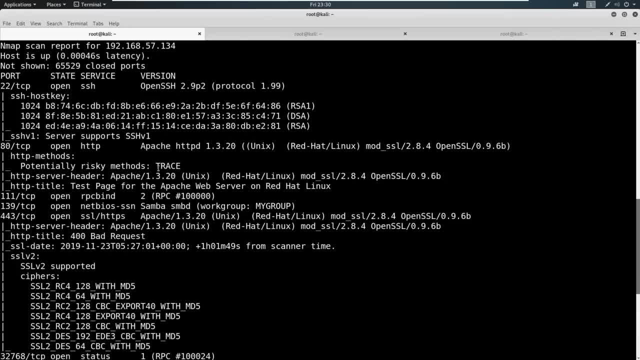 these open ports, And then we're going to go ahead and we're going to go ahead and we're going to look at this And we want to look at what's running on these open ports. So we see here that what's running on port 22 is SSH. Okay, on top of that, it's got a version here for us. So 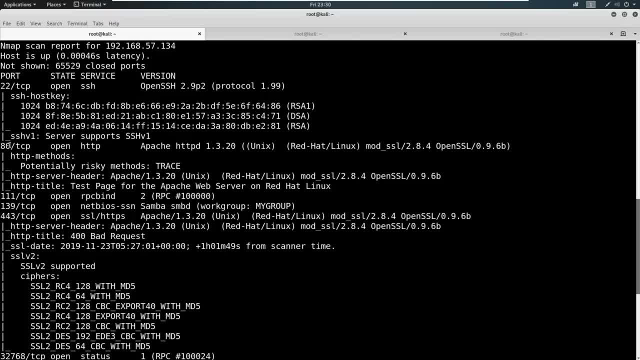 open SSH 2.9, p, two p, and then we see apache is running on 480. we've also got Apache running on port 443.. And we've got this RPC bind in 139.. Now remember from the networking lesson these kind of. 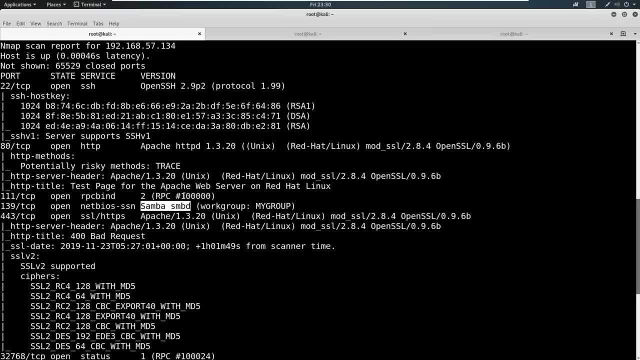 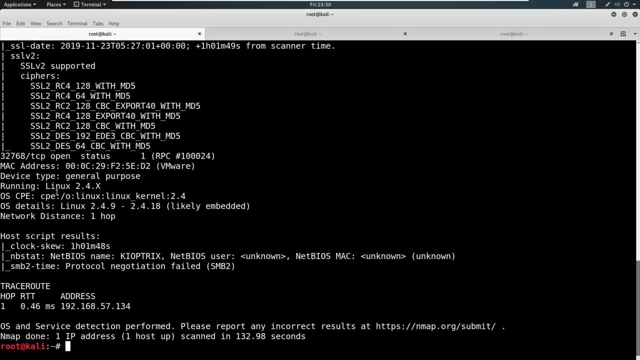 always play together So and be open. basically, Samba shares And what we can do is first step is usually enumeration. Once we see this, we take the scan and we scroll down a little bit as well And we can look at some things and see: okay, there's no OS information. I found Linux here, 2.4, point x, And it's most. 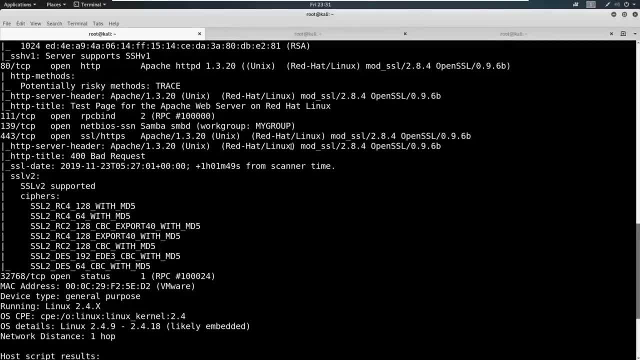 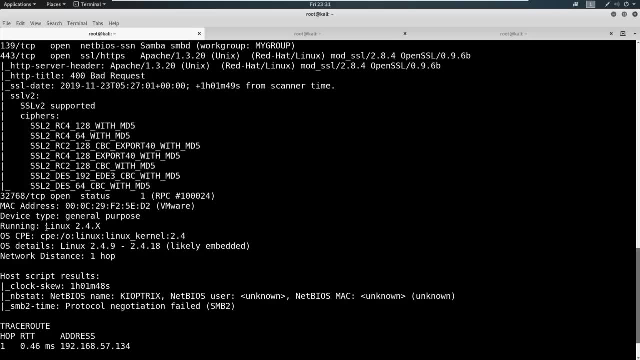 likely pulling that down from from the, the Apache. it's probably a best guess because it's running Red Hat, that it's running Linux and taking a stab out of here, or may have actually determined that from sort of header or some other location. A lot of times this isn't so sure as it's saying. 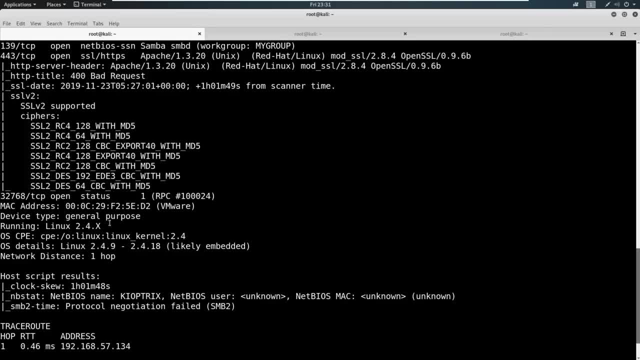 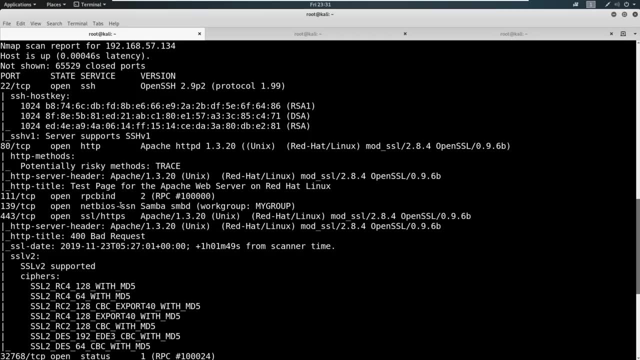 it is here A lot of times. it'll give you a percentage, So the OS is not always definitive as it is here. So we've got the OS, which could be useful for us later when we do enumeration, And you'll see how that comes into play. What I want you to take in right now is that so far, 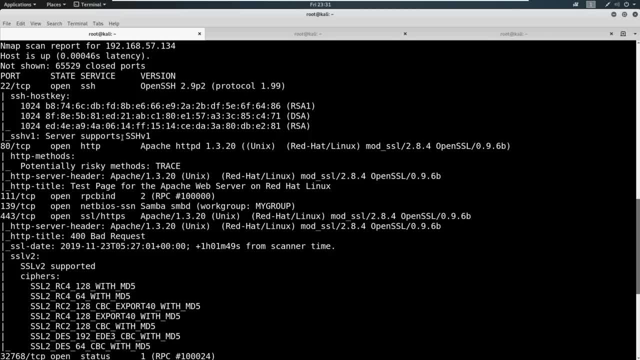 we've got a scan result back And that scan has gone out And it has looked for open ports. doing that modified stealth handshake So it says sin, SINAC, reset RST. Doing that it's found a few open ports. Now it is our job to look up the information that we are seeing on these open ports and try. 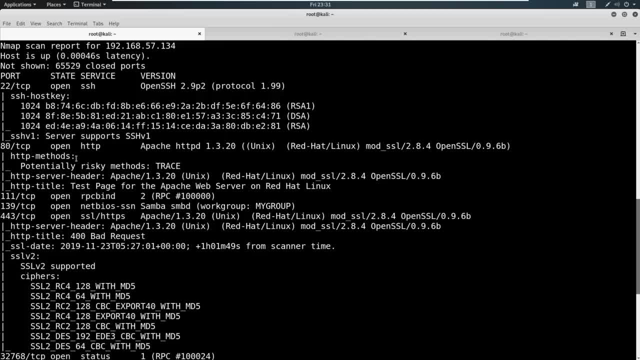 to find exploits on them. So that's what we're going to do And I'm going to cover in the next video. we're going to go kind of step by step And I'll talk through the methodology and the steps that we're going to take to make sure that we're doing the right thing. 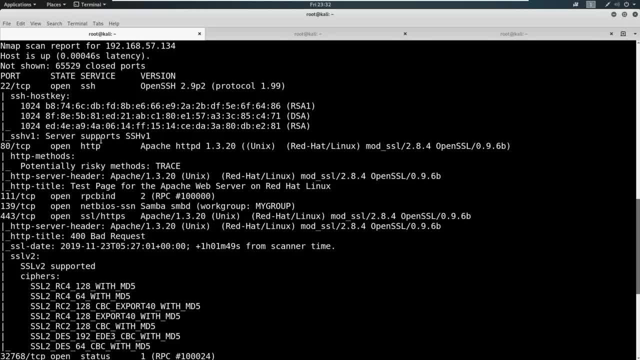 So that's what we're going to do And I'm going to cover in the next video we're going to go and why I attack certain ports. first, what ports those are, how we can enumerate those ports, And then we'll enumerate everything. get all the details down. Once we have all. 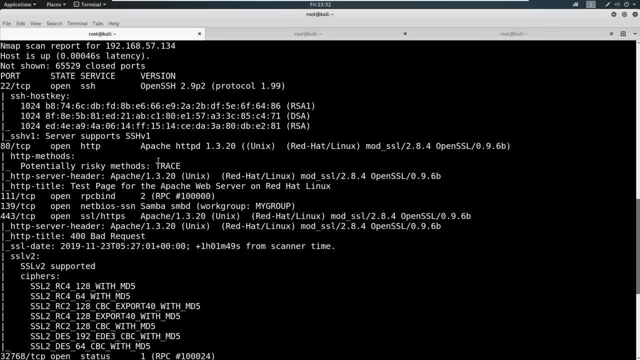 the details down, we're going to move into the section of exploitation. it's going to get really fun And we'll exploit this machine in multiple ways. So from here, just take apart or take that away from the lesson that you officially successfully scan this machine. 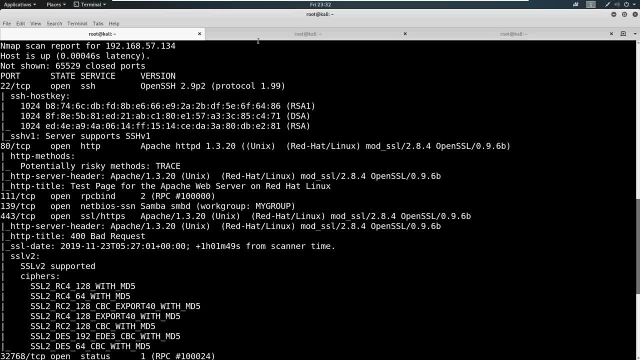 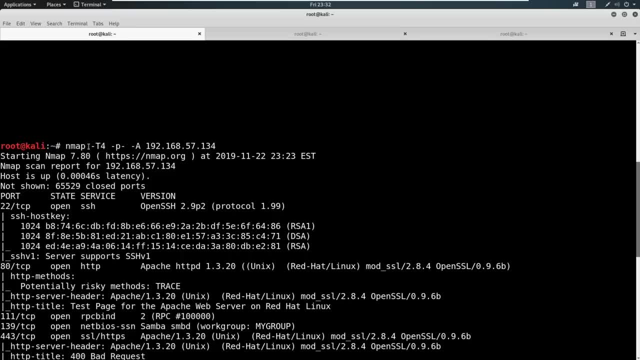 I encourage you to maybe go back and take notes, Or to go back and scan it again. get the syntax down in your head, keep typing this out. remember it. this is the one thing you're probably gonna type out more than anything else. And then also: 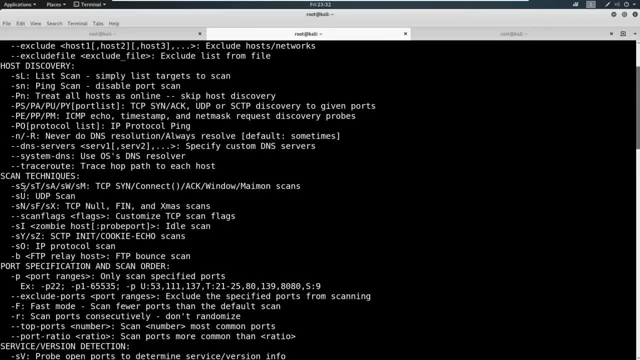 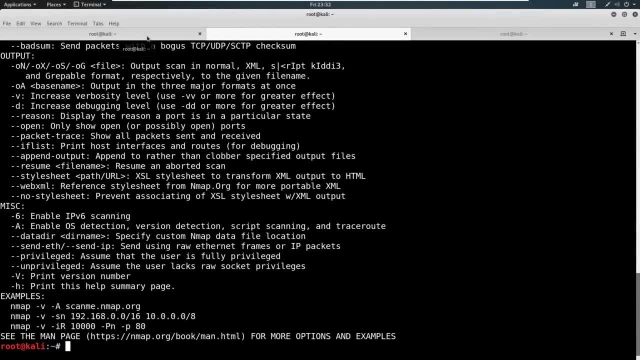 go through and look at the different types of options you have there. If there's one that interests you, just run it against the machine. play around with it. this is your lab time. make the most of it. So for now that's it. In the next video we're going to start enumerating. 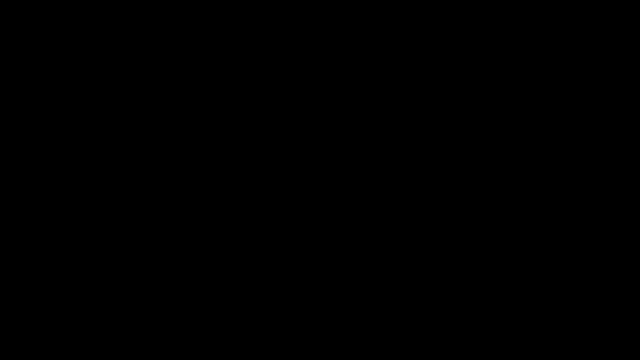 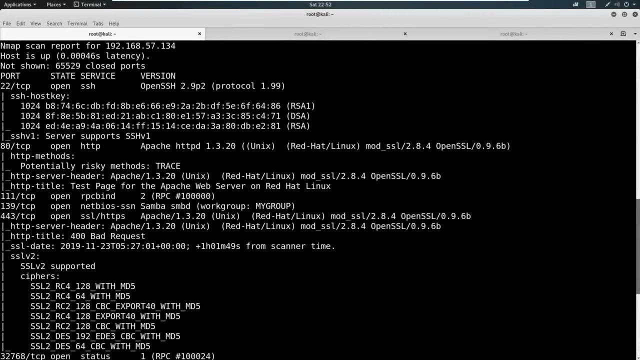 these ports, So I will catch you over in the next video. Let's talk about the scan before we dive into any enumeration. So the scan here: we've got these open ports, we've got 22 with SSH and we've got 80 and 443, which are hosting. 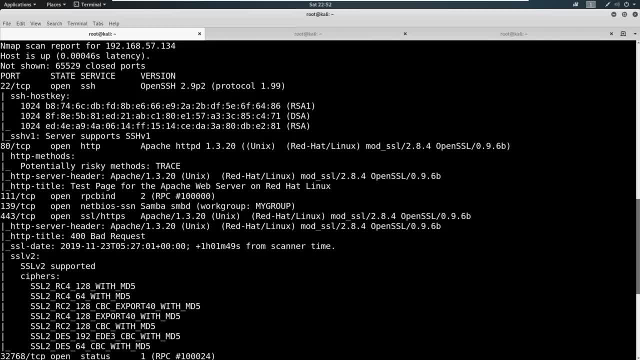 websites. And then we've got 139,, which has got a file share with Samba on it. And then you've got the 111 and 32768, which are RPC and related to the SMB. So we need to think about point of attack as an attacker. Now, when I see this scan, I light up with 80 and 443.. And 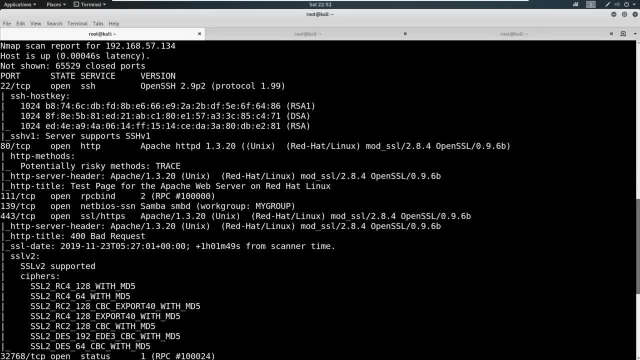 I light up with 139.. And sometimes you'll see 445 with it as well. I light up from those because those are commonly found with exploits. If we think back about all of the exploits that have been out there for a website, for example, or if we think to Samba or SMB related exploits. 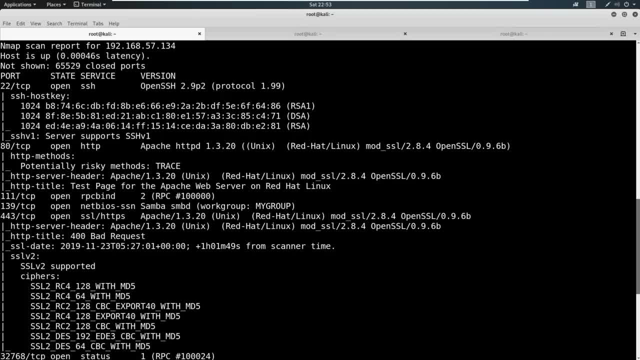 just recently. right now it's recording in 2019.. In 2017, there was malware that went around called WannaCry And that was based off of something called EternalBlue, also known as MS-17010.. It was a. 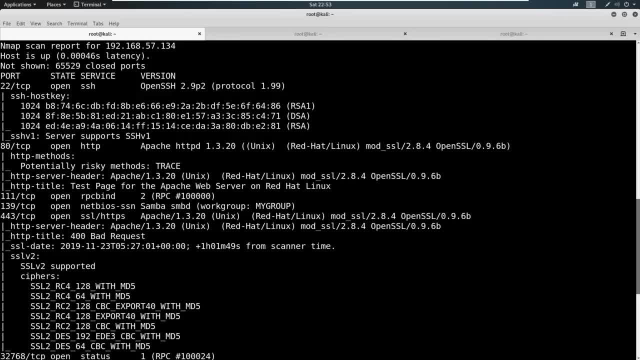 pretty wicked exploit that utilized a flaw in SMB. SMB has been historically bad and websites have been historically bad. Now, when we see something like port 22,. port 22 is a lot of SSH And historically it hasn't really been that bad. Now we can try attacks against it. 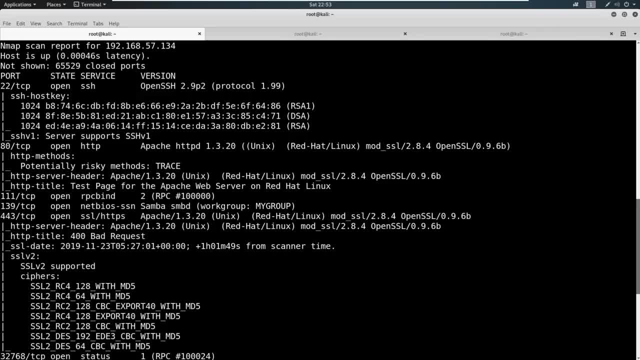 like brute force attacks. we can try something like default credentials or root tour on it, for example, But when we look at it we can maybe enumerate the version, but there's not usually what we call remote code execution on SSH, remote code execution being that we can run an exploit. 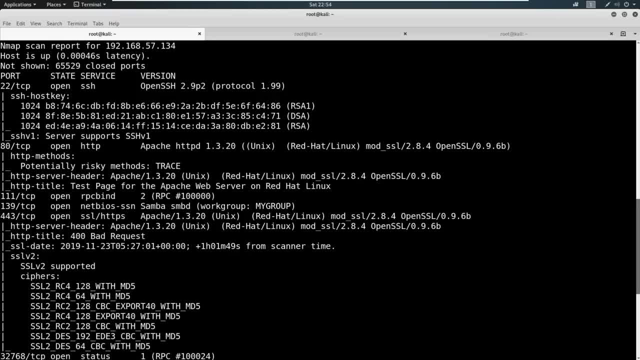 against it and get something called a shell back, And we'll talk more about that when we get into the exploitation section. But for now just know that it's not really common to attack SSH. So when I see SSH open we can do some things at it. But when we talk about low hanging fruit and that's really what- 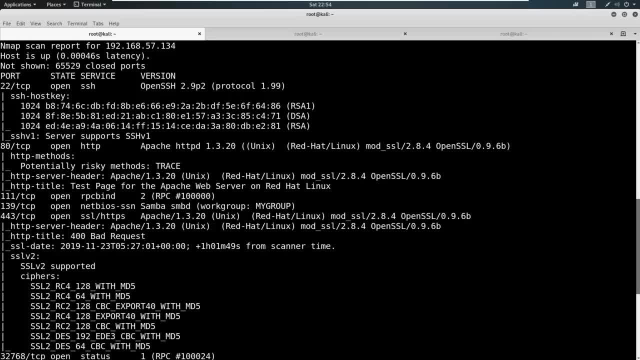 we're after as an attacker. we're going to see what's juiciest first and kind of go from there. So you'll develop your own methodology over time. But I'm going to drill into your head at least my methodology, why I do things, And there will be several videos of walkthrough. 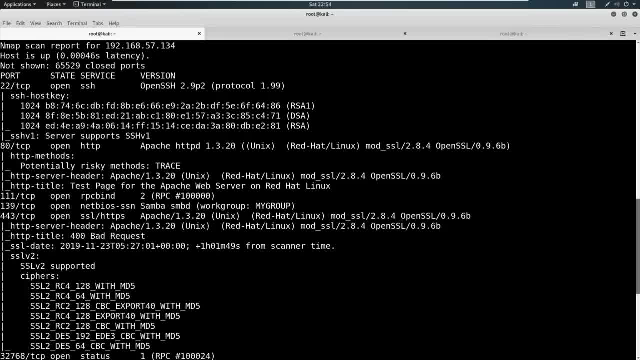 machines in this course. So you're going to get to see this over and over and over And I'm just going to explain my methodology repeatedly so that you can get introduced to new tools and new ideas and ways of thinking. So from here, I do want to dive into my first thought process, which 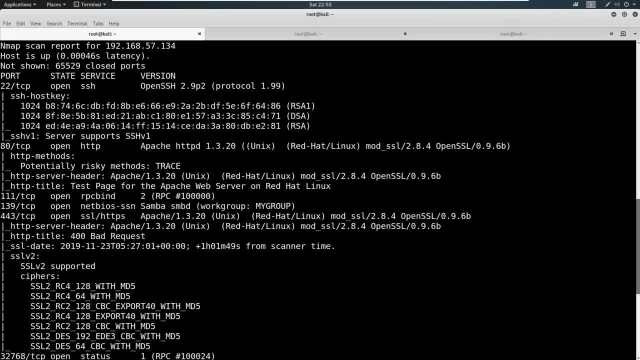 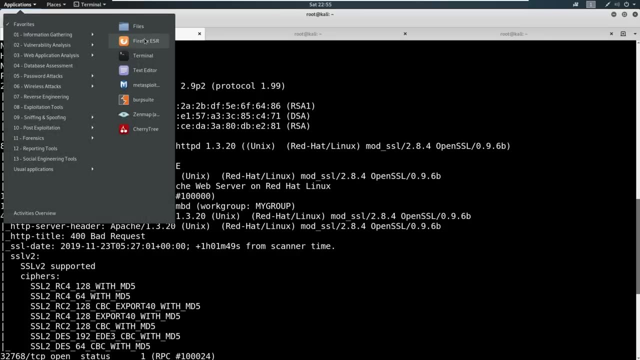 is. I want to investigate port 80 and 443.. I would either here I would do 80 443, or I'd go right after 139.. So we'll do 80 443 and start working towards those. Now let's go ahead and just do the first step. This is always my first step If I see a website. 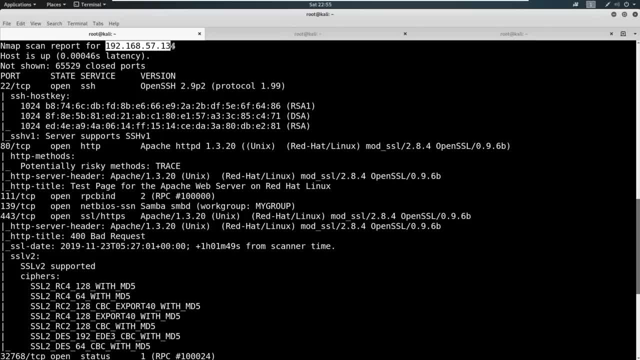 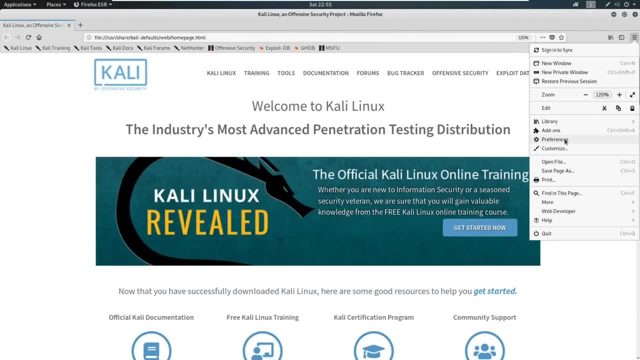 I'm just going to go out to the website, So I'm going to go ahead and just copy this here And I'm also going to go into the little hamburger and go to my preferences. And I have not turned off my burp suite settings And it's possible that if you're just following along you haven't turned. 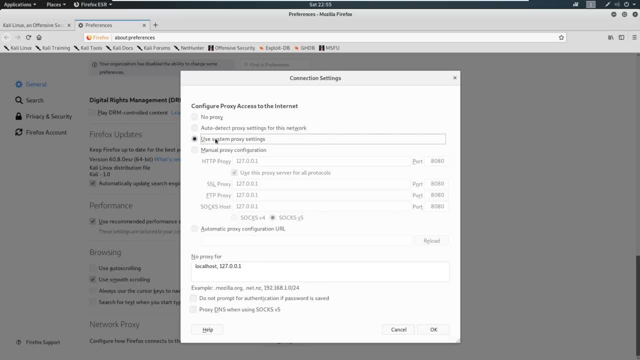 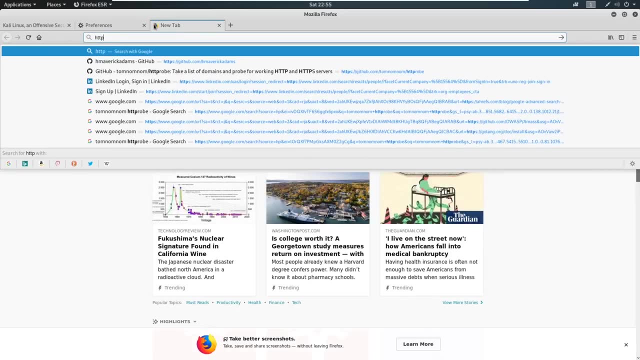 it off either. So go ahead and just select use system proxy settings And we'll just say okay. So now we're going to go to our website and you should be able to navigate to our website. I'll just open up a new tab just in case We'll do something like this. Good, That worked, And then 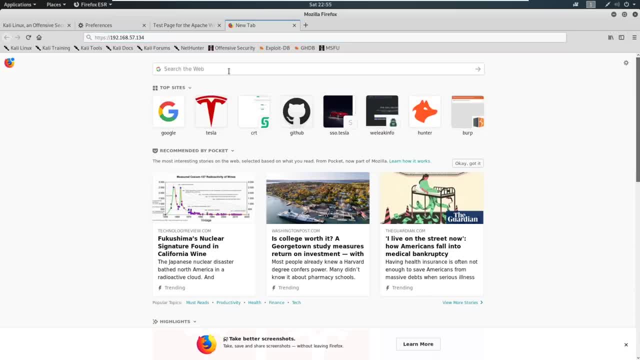 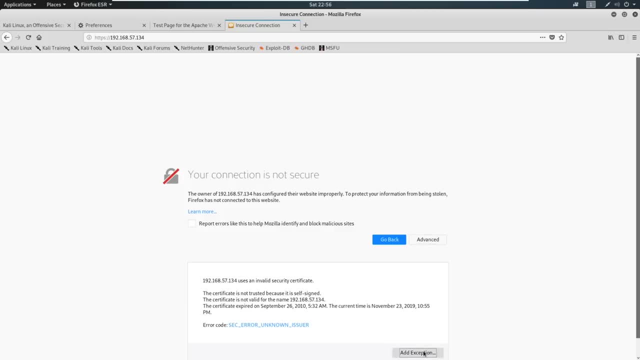 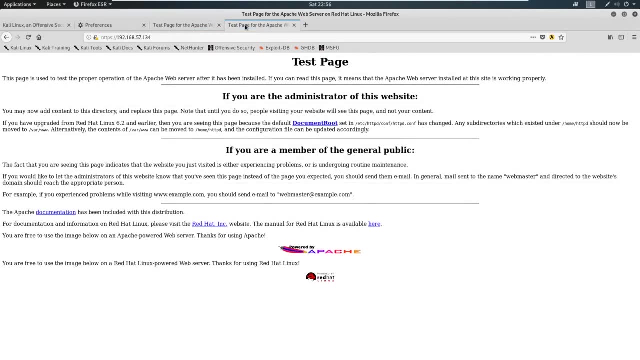 we'll do the HTTPS version, because there's also 443.. You might get something saying your connections aren't secure. just go ahead and say advanced and add an exception here, Confirm it And you'll see this. Okay, so what we have here on both of these is we have a default webpage Now. 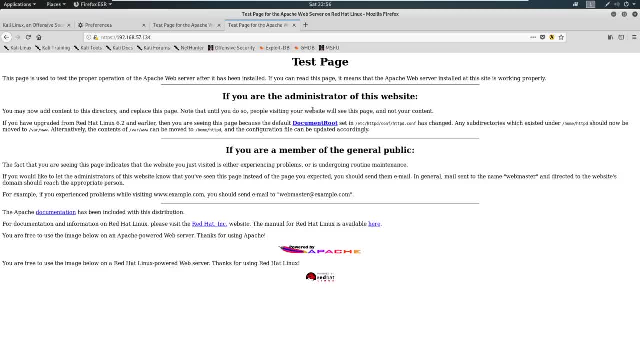 we talk about performing a network penetration test, or even a web application penetration test. if we see a default web page like this, this is an automatic finding. Now, why is this a finding? Is it exploitable? No, not really, But it tells us a little bit of something about the architecture. 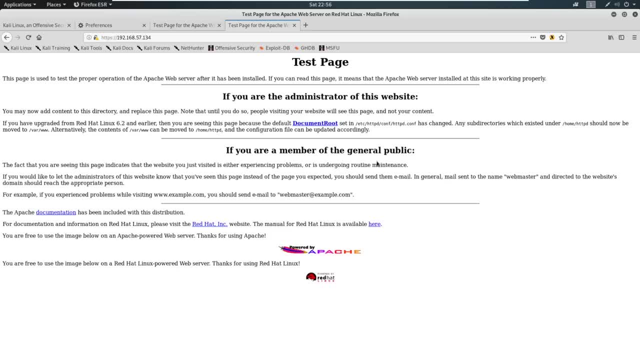 that's running behind the scenes And it tells us a little bit about the client's potential hygiene. So if we see this, well, we know that it's running Apache, we know that potentially the box is running Red Hat Linux And we're just getting ideas of what's going on behind the scenes. 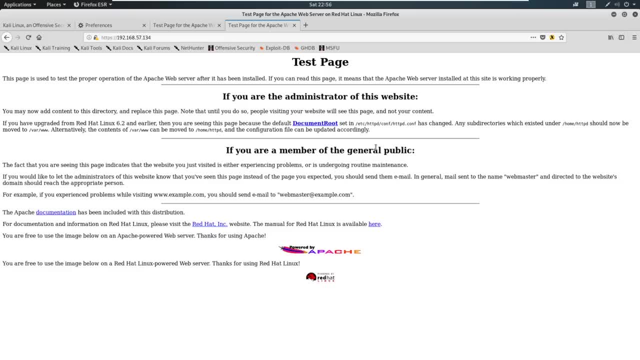 More so if a client is running a default web page. it brings up two questions. One: are there other web directories behind this? So we'll show you something here in a second where we do directory busting and attempt to find a directory. 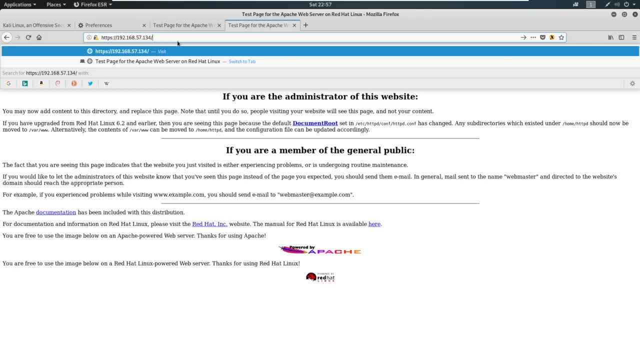 Like say: we're looking at this and we don't have anything to click on, but we say: you know, slash admin, maybe that directory is there. Okay, are they hosting a website somewhere else? that's just not at this IP address on this base, Or maybe they aren't hosting any website. 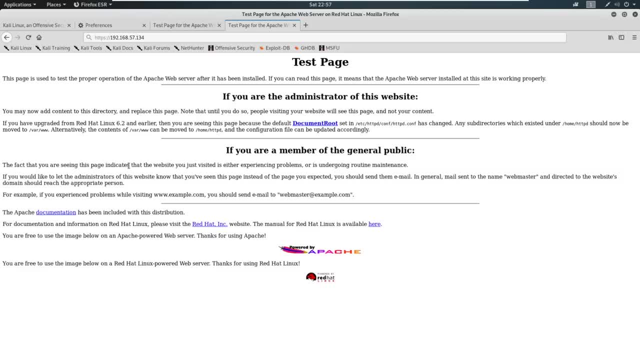 and they just left 443 and 80 open for no reason and put this default web page out there. Now, when you think about that, that signals to an attacker poor hygiene, And I'm going to think to myself as an attacker if I'm going to do this, I'm going to do this, I'm going to do this. 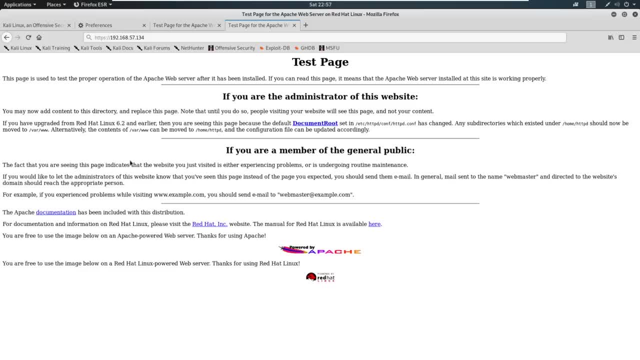 if a company or client is willing to just put this out there willy nilly, what else are they doing? What potential vulnerabilities might they have If they're doing this? so this immediately signals poor hygiene. we would write this up on a test And I'm going to show you guys my notes. 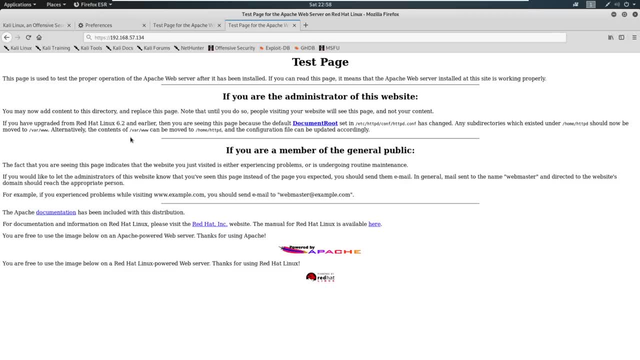 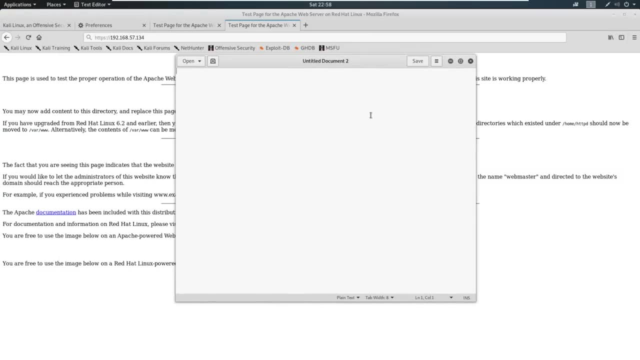 once we kind of get towards the end of the enumeration. So make sure you're taking good notes And we can do that and like a little notepad here and kind of what we're doing. I think this is useful. I'll make a nice little keep note or you you can make a cherry tree and make your own notes out of. 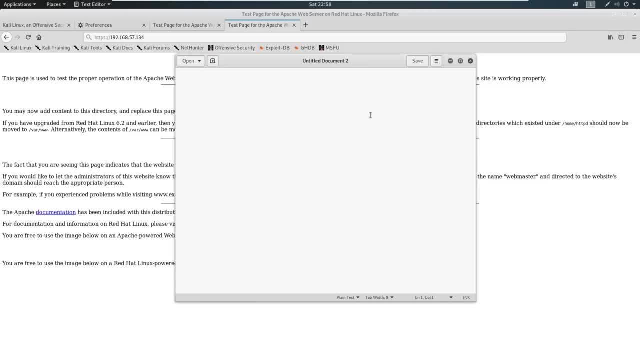 this And I'll show you what it looks like toward the end of the enumeration. But we can say something like 80: 443.. And then you can put the IP address, And sometimes people like to put notes at like what time they did this. So you could see up here: it's 2258 or 1058pm my time And we could. 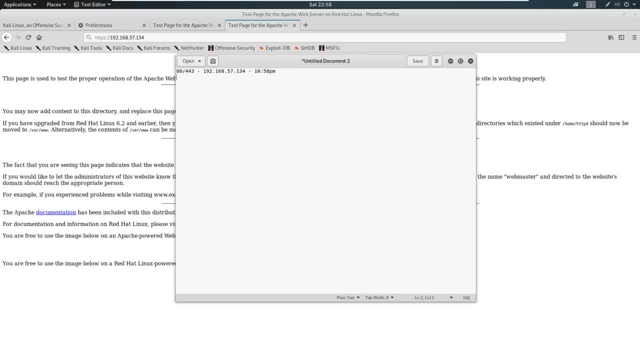 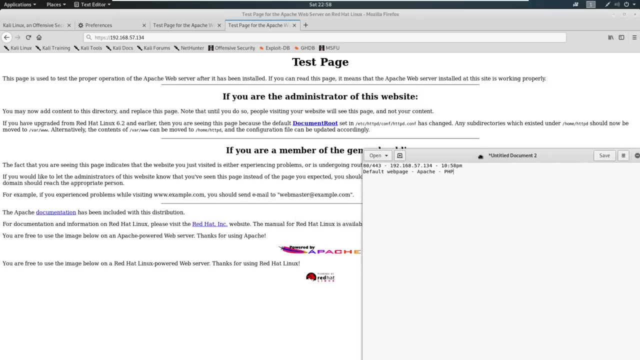 take that and we can just say default web page And we can say Apache And we could tell that it's running potentially PHP And we'll get behind this as well, And we just have these little notes. So we know that we navigated to it right. At least this is part of the enumeration here And you don't have to timestamp everything. I'm just giving you that for an example. But we can see that it's running this default web page. So we have a default web page. there's nothing really for us to click on. I mean, we've got, like, the documentation, we've got the 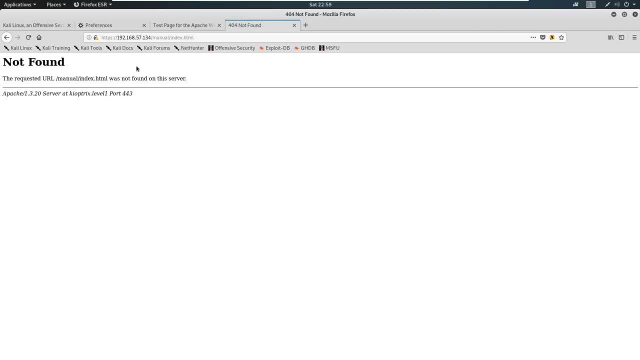 we can go to, like it looks like the manual might be here And this here. we just clicked on a link and it was a bad link. Now, this is also what's called information disclosure, So this will be another one to bring up. But we see here that we have an error page And this error page is saying: hey, it's not found. Now, this is typical of what's called a 404.. And when you see a 404, you think, okay, it usually redirects you to a page it's like: hey, we can't find this. 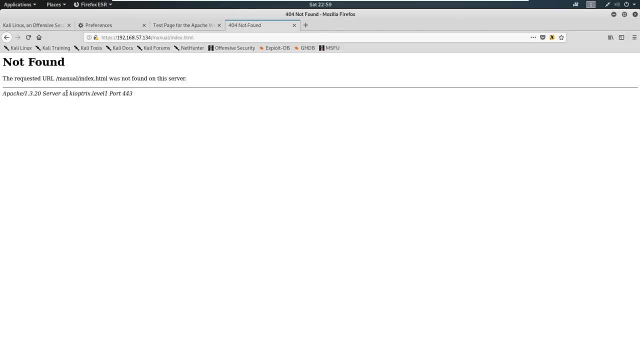 This is giving us a little bit more information than we should be getting. We're seeing here that we're getting Apache version 1.3.20.. So now, if we didn't know already, we do know that we're running Apache 1.3.20.. And we got a host name here: kioptrixlevel1.. That is a internal information host name. right, So we can get naming convention out of a client we could potentially know how they are utilizing. 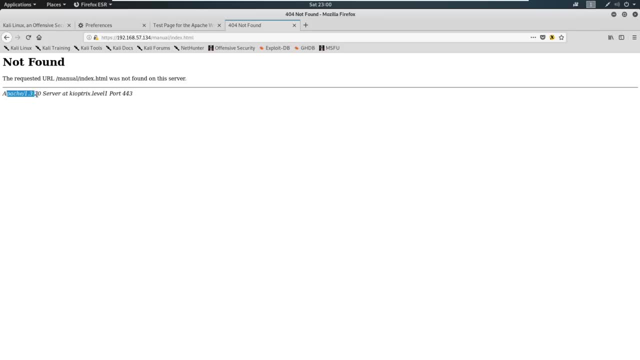 naming conventions on their internal networks And we've got some version- enumeration or information disclosure. So this would be a screenshot as well, that we would take a picture of And you can also notate that in your notes and say something like you'd say: information disclosure. 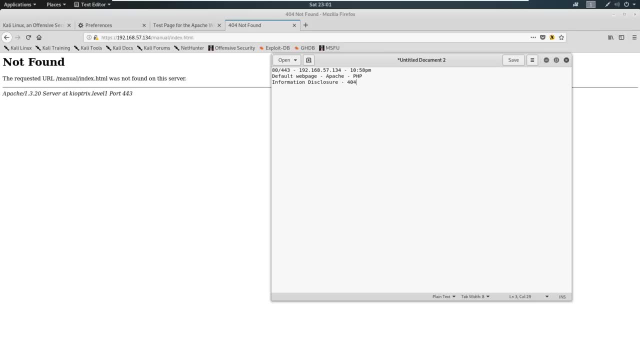 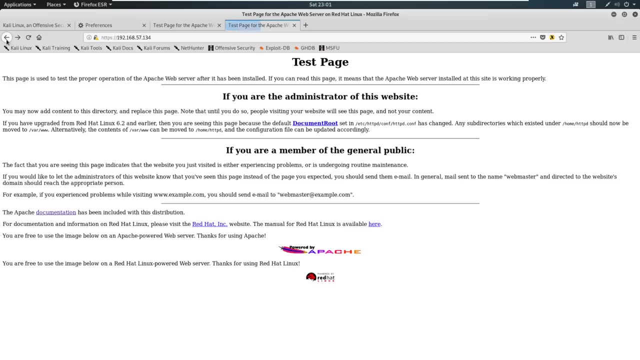 And then you could say something like 404 page and then you would just have your, your notes or a screenshot of this, And then that would indicate to you what you can write up on the report and kind of where you found it. So we can click around on this page Or we can do a little bit of what I like to do, which is: 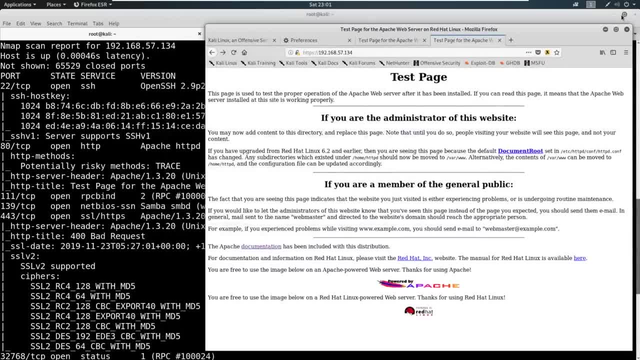 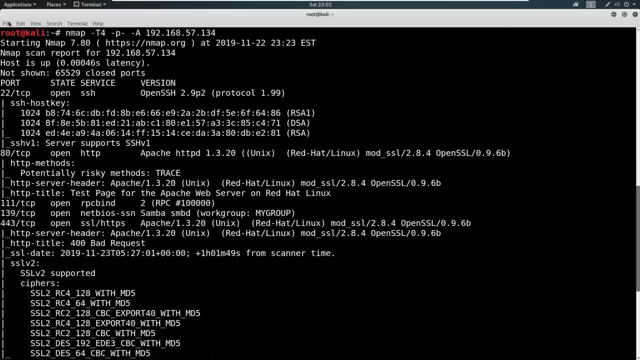 vulnerability scanning. So I'm going to introduce you to a another tool which is called nicto. So let's open this up, up a new tab. we can close these two tabs out if you've got extra tabs, like I do, And 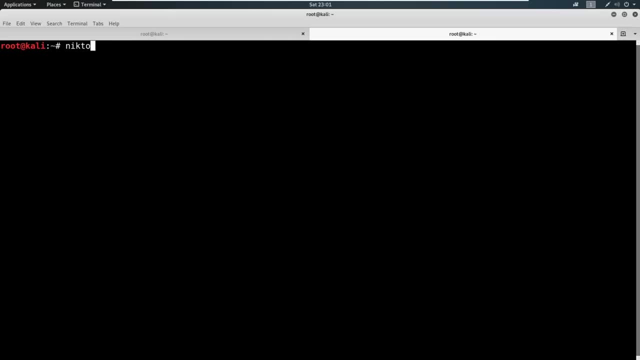 this tool is called Nick doe- it's just like this. So Nick doe is what is known as a web vulnerability scanner. This is a great tool When you're learning the beginning stuff, when you're practicing against phone hub or you're practicing on a CTF or something like a hack the box, which. 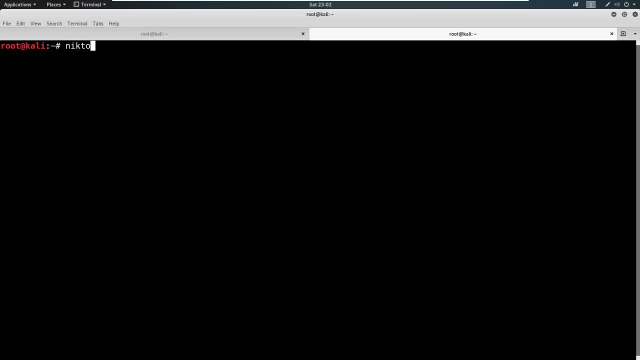 I haven't introduced to you yet, But it will help you do vulnerability scanning against the website. The issue is that if the website is running good security, you might run into some issues with that and it might actually auto block it if it detects. Nick doe scans- Not always very commonly, that's. 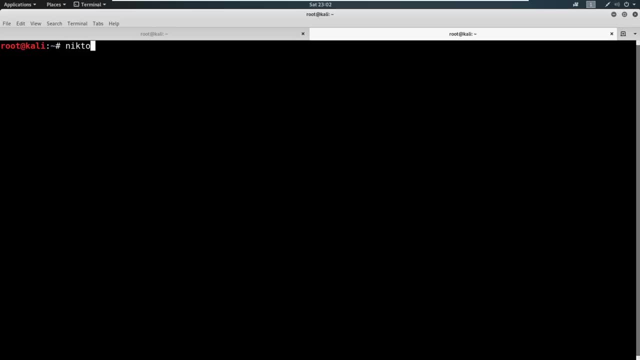 not the case. But if they've got good security or a good web application firewall, it might actually block these scans. So you have to kind of be wary when you use it And really use your hunch if you think that this client is using a web application firewall or not. 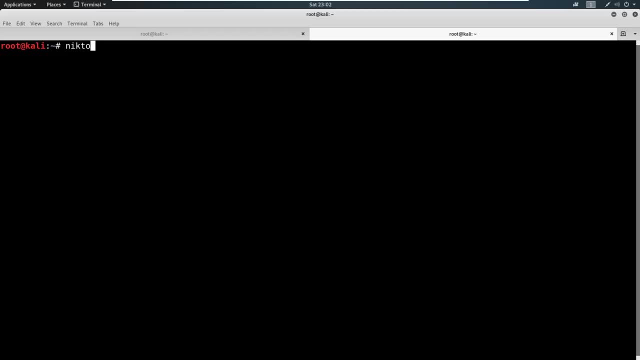 And you'll really get a feel for the client just as you gain more practice. And once you're getting in there and you're starting to notice vulnerabilities or not, you'll kind of understand whether or not they're running something like that. So from here we're just 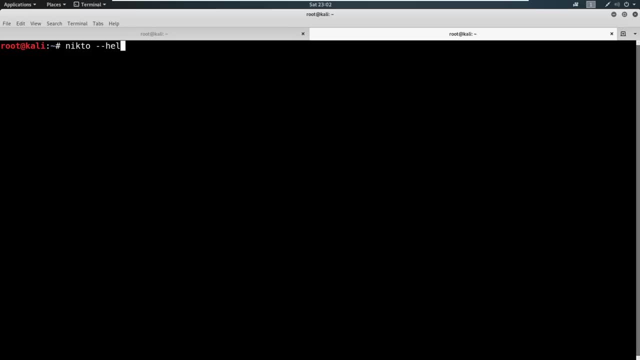 going to say: Nick doe, and you can always do dash, dash, help. But it's pretty straightforward. All we're going to do is say a dash h for host, And then we're just going to say something like HTTPS, And then we'll just paste our 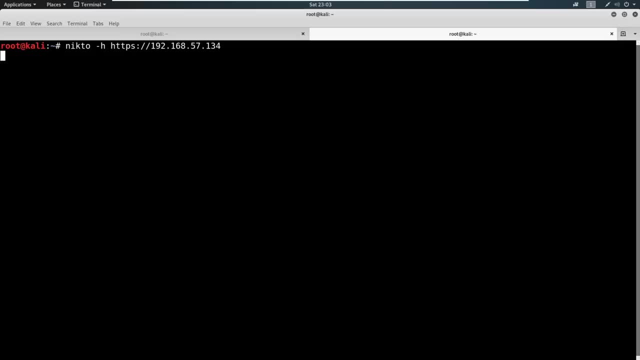 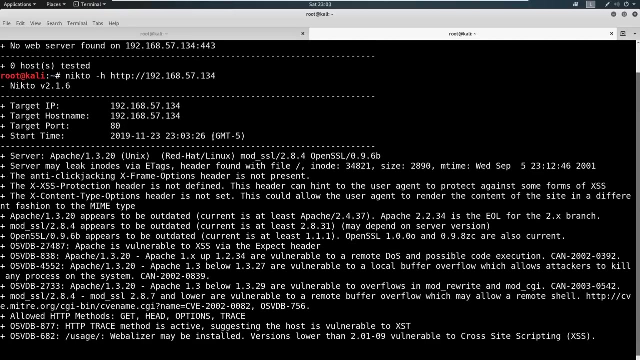 our address, something like this, And that one did not work. So let's go ahead and try HTTP and see. there we go. For some reason, it's not picking up the SSL on this, So I'm not sure why it's not discovering. But now we can see our scans. 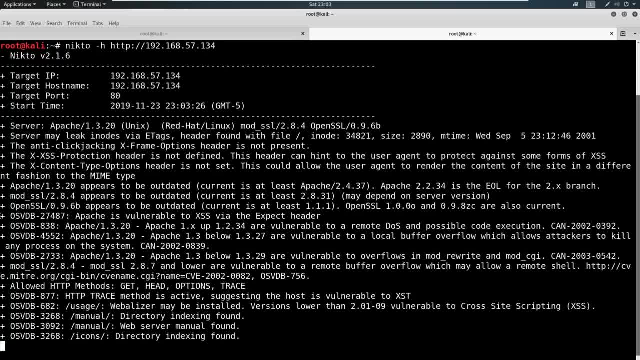 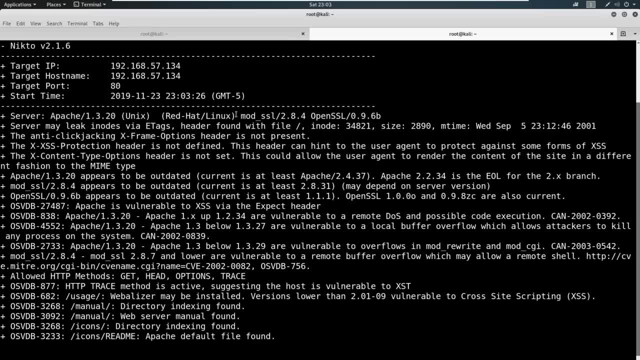 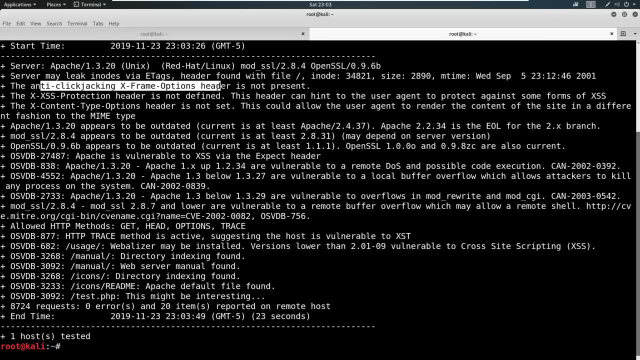 kicking back And immediately we can see that it's doing some detections here. It's detecting that the server Apache 1.3, point 20, is running. It sees this mod: SSL, SSL with open SSL. It's giving us some vulnerabilities back. It's telling us what. 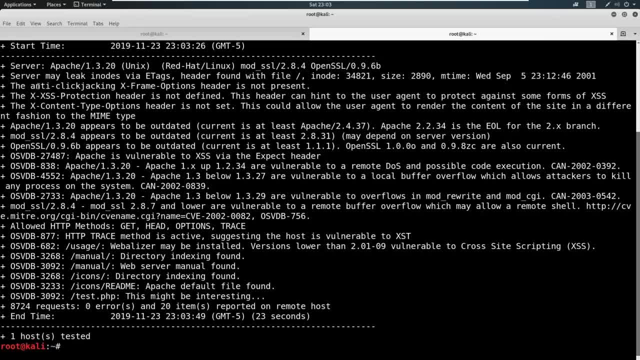 is missing in terms of protections. Now, these protection headers: if we're doing an external penetration test, not really that important. If we're doing a web app penetration test, these become more important, But we don't have to worry about them right now. So when we come, 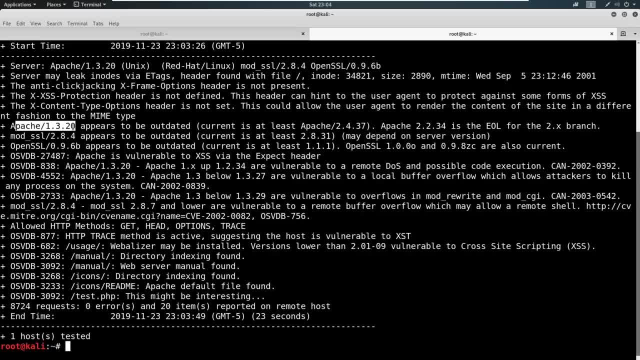 through. we keep looking and we see Apache 1.3.20 appears to be outdated. Okay, mod SSL appears to be outdated. Open SSL appears to be outdated. These are all findings. Depending on how outdated it is, a 1.3.20 to a 2.4.37 is pretty outdated. So these would be findings that we would notate on. 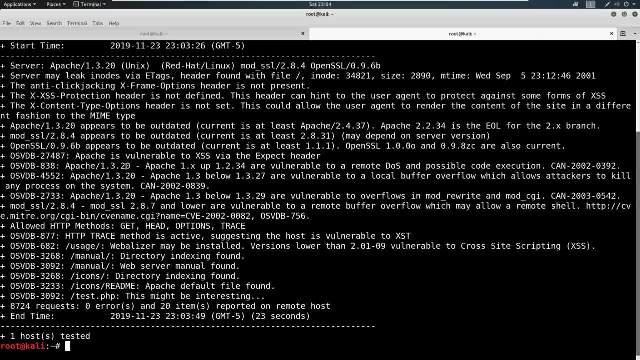 a report as well We can look through and you can see what types of attacks this might be vulnerable to. So one, if you're looking through, there's this Apache here that says remote denial of service. Well, typically denial of service is out of service. So if you're looking through, 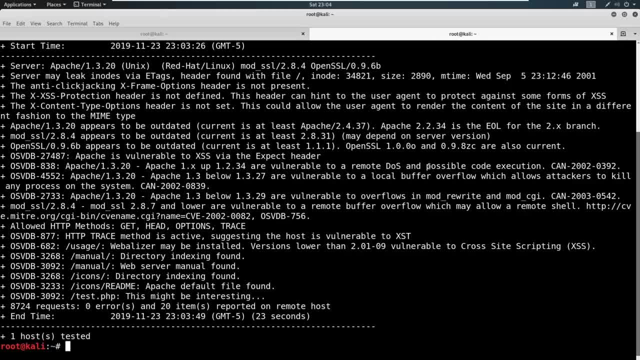 scope when we're doing a pen test, so we're not interested in that Possible code execution, so maybe interested in that. We are also potentially interested in a overflow and rewrite, And this one says this is vulnerable to a remote buffer overflow, remote being important. 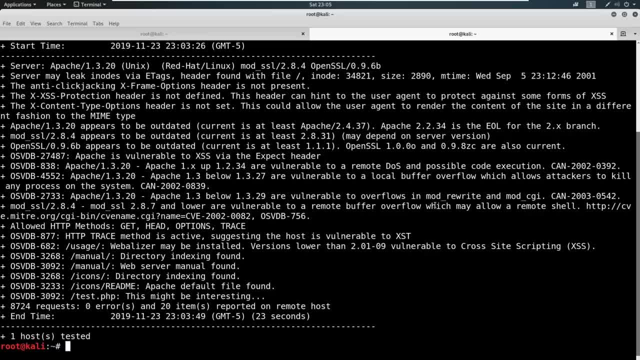 which may allow a remote shell. So remote meaning we do not have to be local, So I skipped over this one. where you see local. This one is remote meaning we can run the remote shell, So we can run that against a site sitting in our pajamas in our house and that site's running somewhere else. 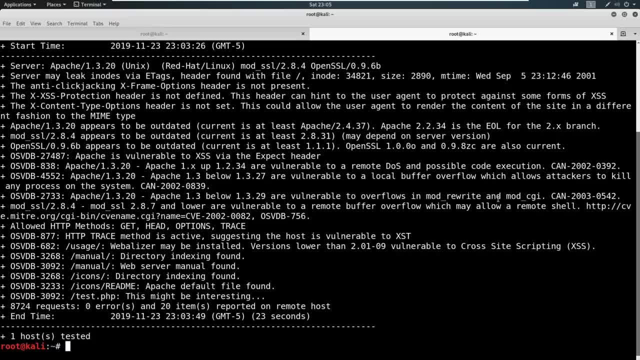 And we can do this all remotely. So immediately it's found potential vulnerabilities. So we've got this potential mod SSL vulnerability And it's come down here and it's looking at some other things. You could see that this trace method is active and we're still haven't gotten into web. 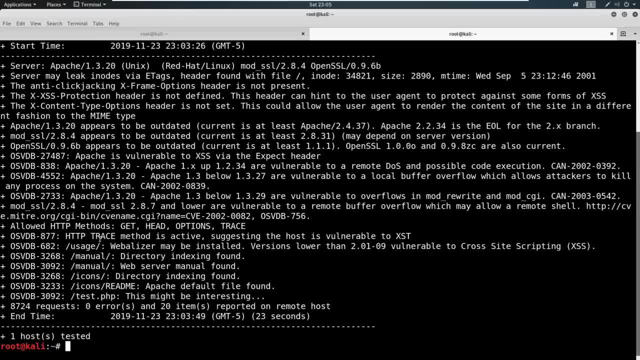 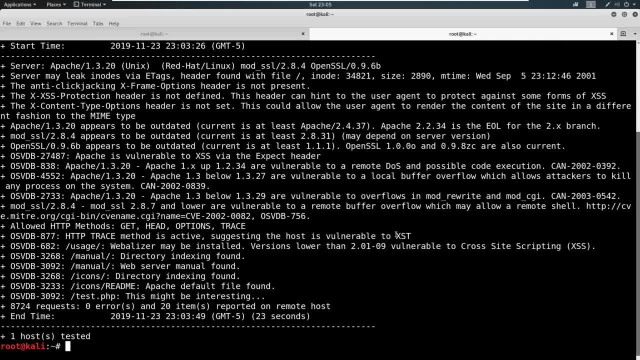 scripting which you see up here And that could lead to something called cross site tracing. but you kind of need both of those. But again, that's just informational At this point, you don't have to really be taking notes on that. So we're coming through. it does a little bit of directory busting. 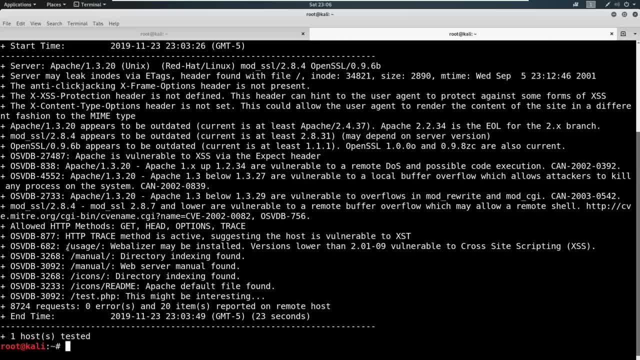 for us. So what that means is it's just going to come through here and it's going to run like a word list And that word list might have, like admin usage manual, right, test, dot, PHP. it's got all these different items that it found doing this word list. Now we're going to do a 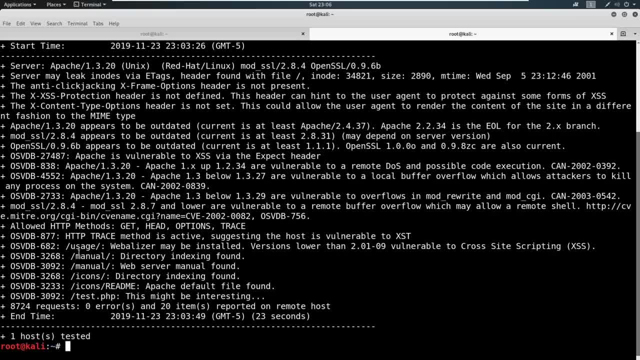 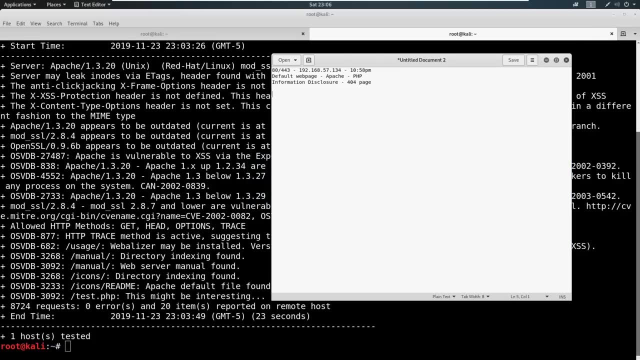 little bit of directory busting here in a second. So we'll save this scan And we'll keep this in our notes And we'll refer back to it here in a little bit. But what we need to know is we can alt tab and we can get our text editor And we could say something about: let's just copy and. 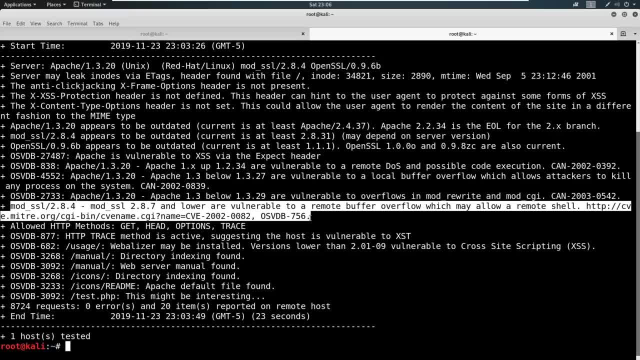 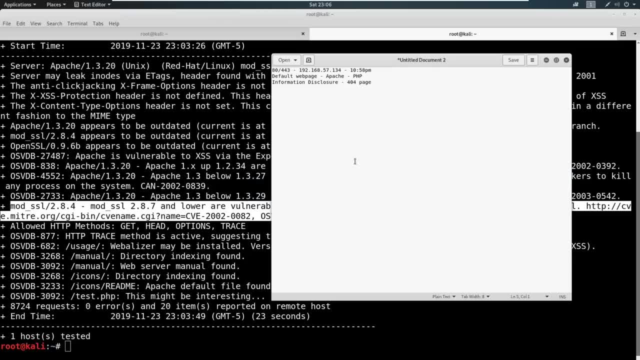 paste this line here that potentially, this mod SSL is vulnerable. So let's copy that And we'll, we'll put that into our text editor And we'll make that as a note. So we're still doing enumeration. we're not going to, we're not going to do any exploitation until we get to the 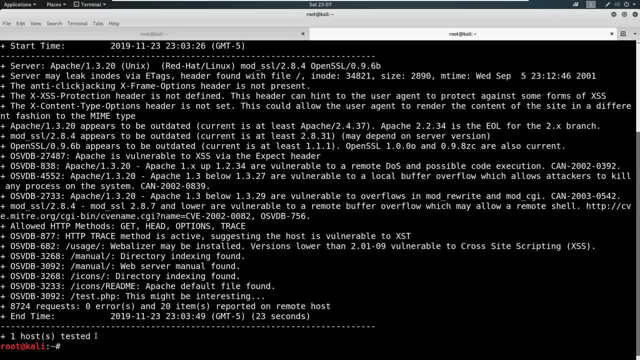 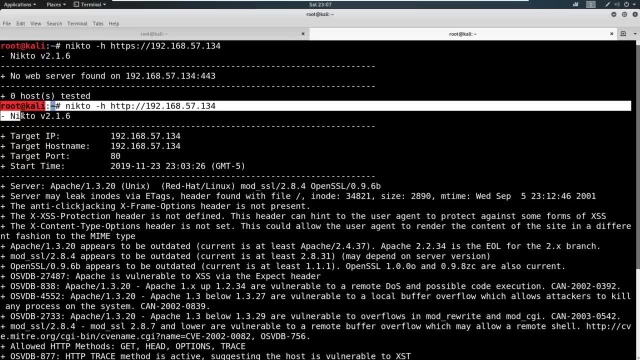 exploitation stage. So what we would do typically is we'll save this out to a file. So you might want to like copy this, all this right here to show what you ran, And if I could copy, that would be really useful. So you copy this and you would just make maybe a directory and you can call this. 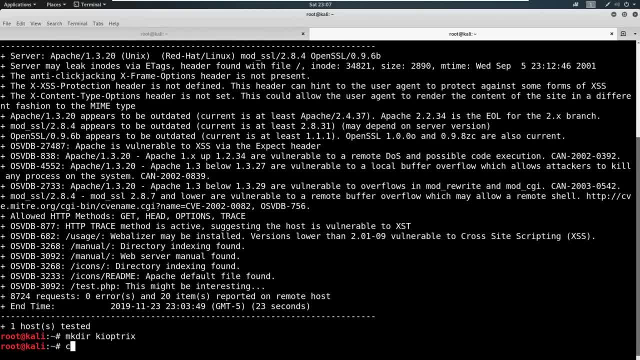 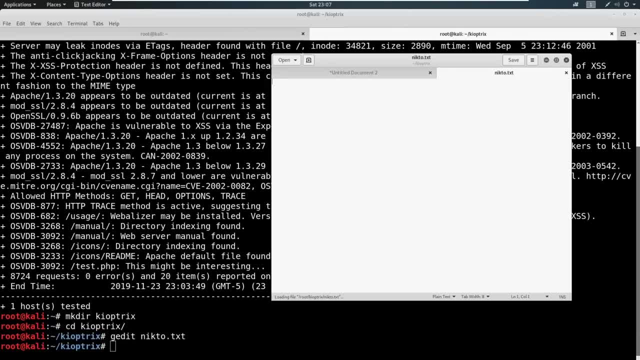 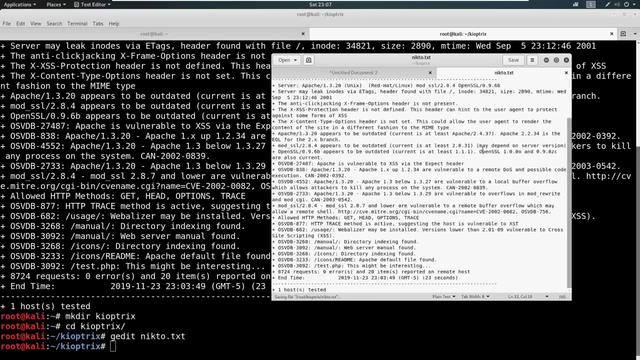 some like key optics and then we could see the into key objects And then you could say Gedit, Nikdo, that text And then you have your Nikdo scan saved. So this is part of being good pen tester is saving all of your scans and having them available in case you need to go back for notes. So we'll save that. 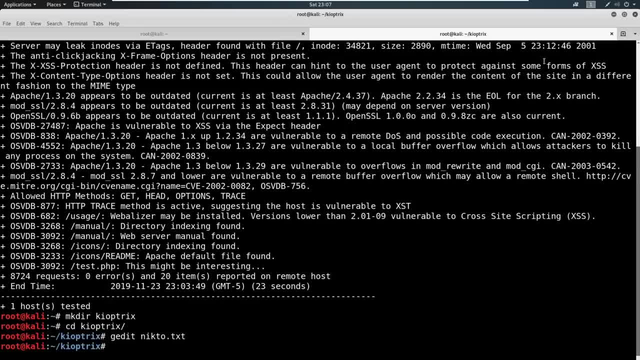 And then what we're going to do is we're going to pause here, we're going to call this part one and then we'll go into part two and talk a little bit more about directory busting and look at some other enumeration features. I'll just kind of show you this in one more minute, But what we need to 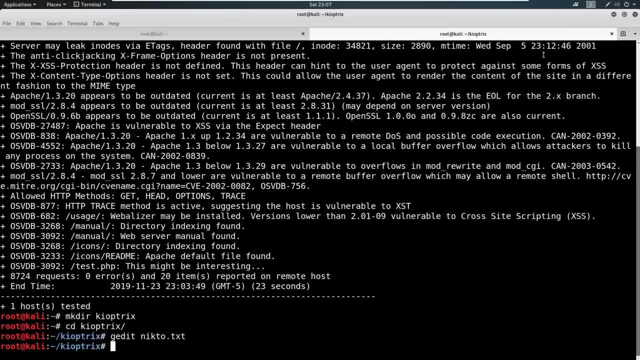 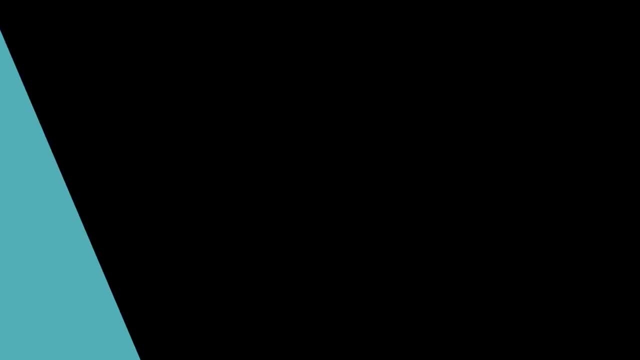 that we have for this, And then we'll start focusing on other ports and really enumerate this box thoroughly before we work on exploitation. So I will catch you over in part two of this video And I'll see you when you get over there. So now we're going to use a tool called 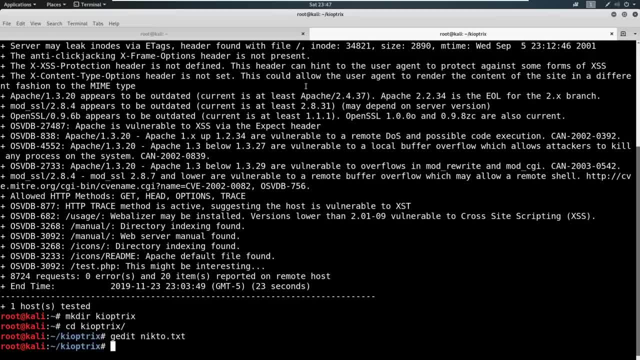 der buster to do a little bit of directory busting. There are other tools out there that are similar or do the same thing. There are two built in tools, In fact: there's dirt buster And there's also a tool called derb, And then there is a tool called go buster. 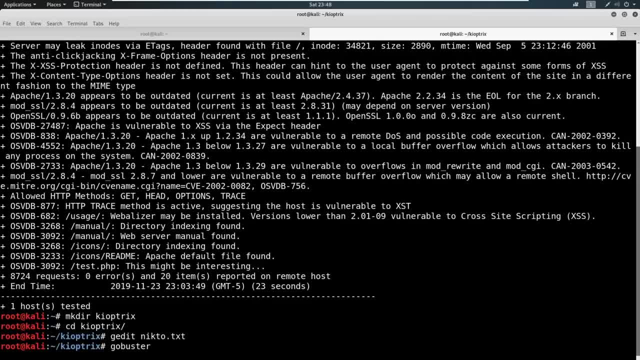 And you have a lot of options. My option of choice is dirt buster, But I do recommend that you write these down and just explore them for yourself and see which one you like the best. So I'm going to go ahead and run dirt buster and I'm going to run it like this. 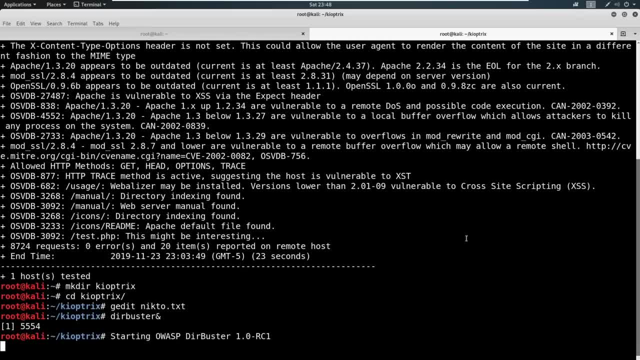 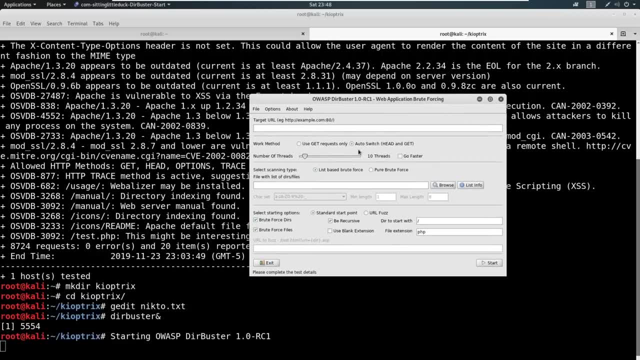 with the ampersand at the end, And it's going to load up this nice little interface, And what we're going to do is we're going to say: Hey, I want to run against this target URL, I'm going to go ahead, just copy. 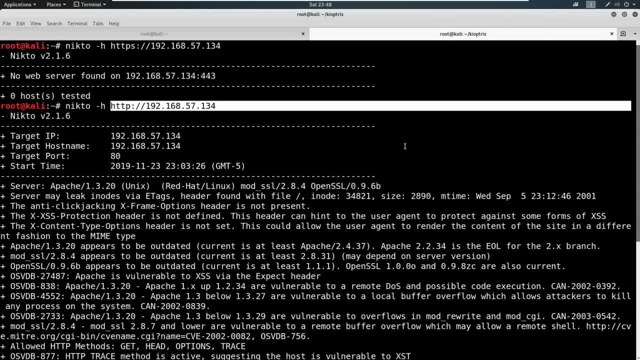 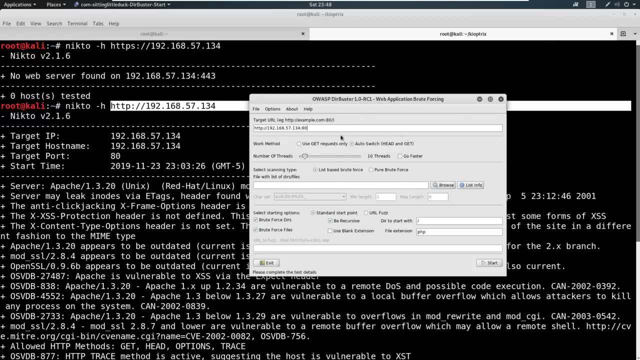 this right here And I'll tab back into it. And syntax is important. It's going to want the port at the end- you see the port at here with a slash, And we're going to say go ahead and go faster on these threads. 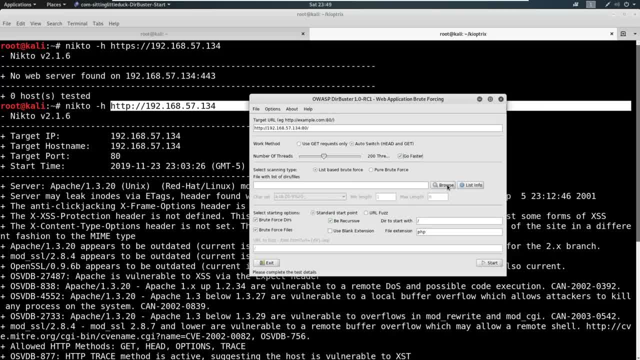 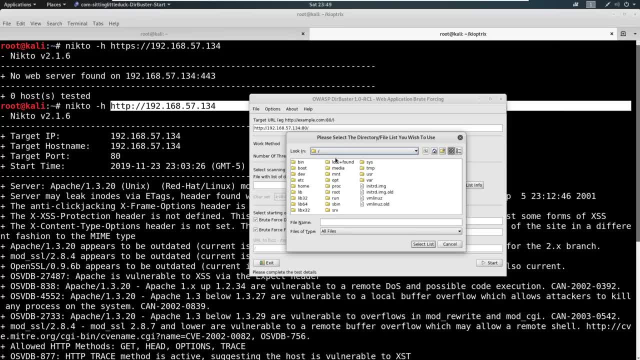 And then we're going to go ahead and pick a list. So go ahead and go to browse, And let's go ahead and go to your base folder here, Go into your user, your USR folder, your share, which is right here, And then if you start typing word lists, it'll bring up word. 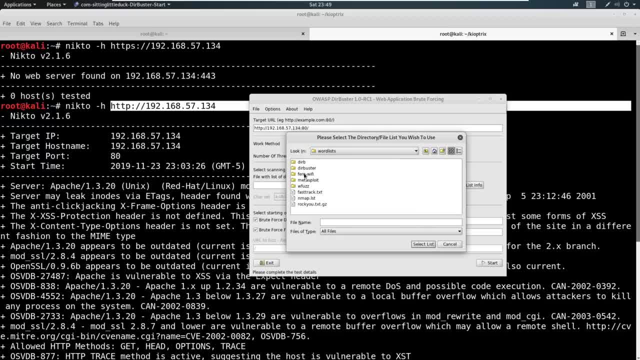 lists right here. And then you see dirt buster has its own folder right here. So we're going to select dirt buster And from here we can pick a variety of different lists. I like to just use the small list If I'm not finding anything at all. maybe I'll move up to the 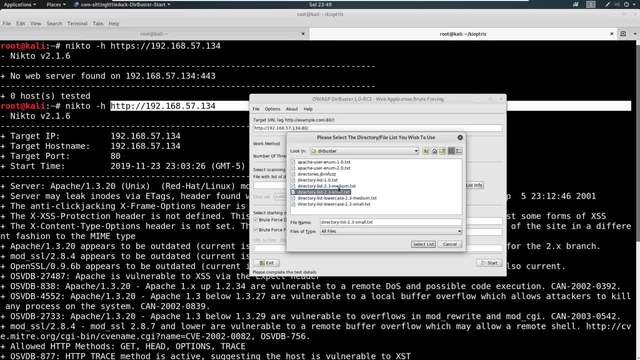 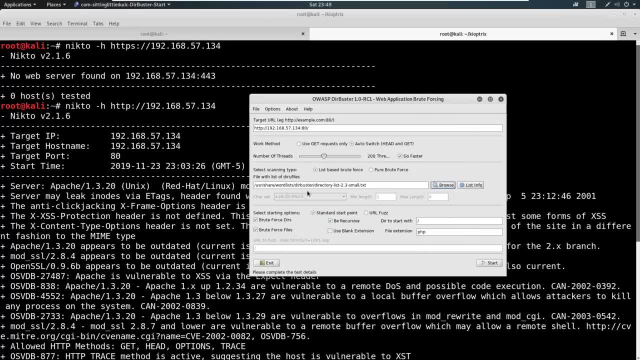 medium and out on the interweb is a large list as well. Let's just go ahead and start with small for proof of concept. And so now let's break it down. We've kind of talked about in the last video, But let's just do a quick reminder. what we're doing is we're 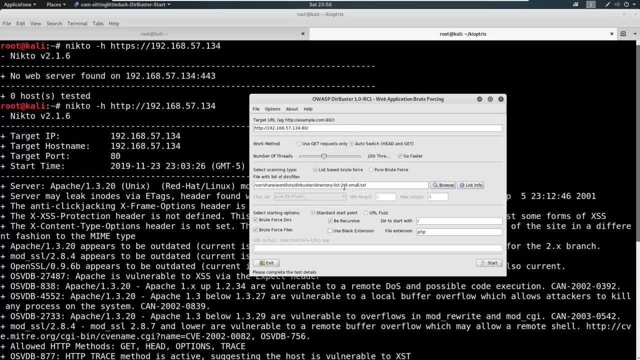 going out to web directories and we're using these word lists, And these word lists have hundreds, if not 1000s, of different well known directories, So it could be something like admin or like CGI bin, etc. And it's going to go out and try to navigate to these. It's 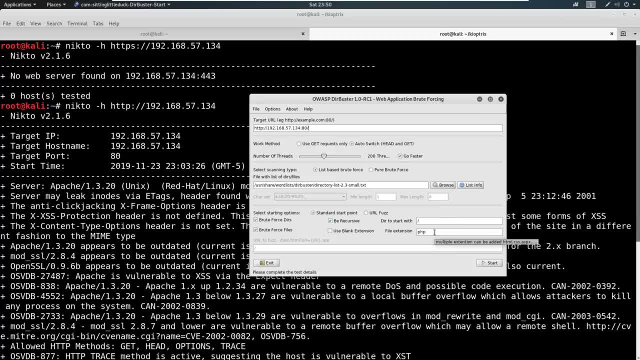 also going to look for specific file extensions. So we know that we're up against an Apache website. Well, Apache runs PHP. Up against something like a Microsoft website which is is. well, those tend to run something called ASP or ASP X, And so this is why enumeration is important as well, because we need to know. 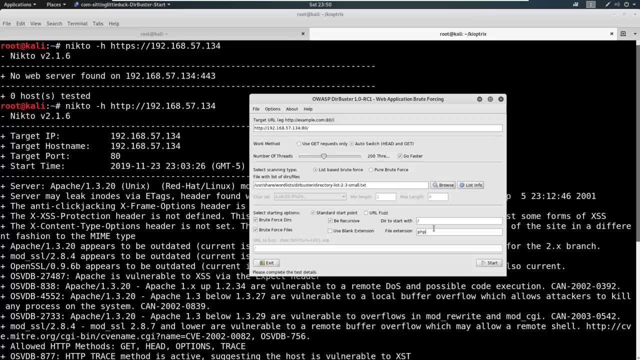 what's running on the back end, to find or make the most use out of it. Now, what we can do with these file extensions, and what I like to do is like to run it against PHP or whatever the base of the server is, But I also do like to run something like a text. 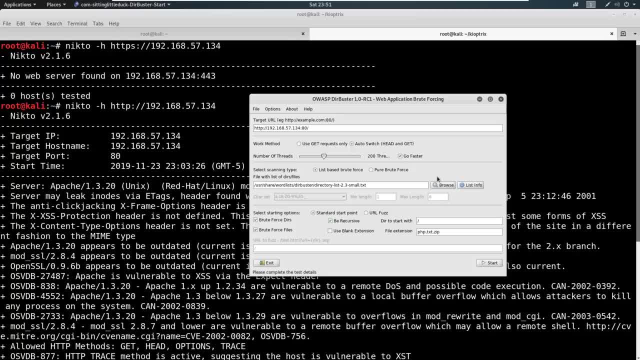 file, something like a zip file, And you can make this as long as- or, Yeah, as many as you want. you could say raw PDF, doc x, But the more of these that you put in there, the more times it's going to search. 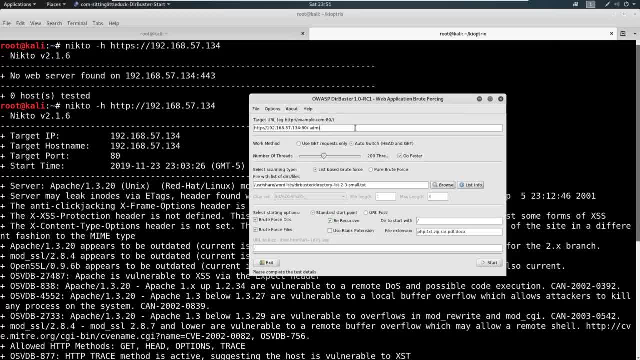 because it's going to search through the word list and say the word list has admin in it. it's going to try admin PDF or admin dot zip. So it's important to limit these to what you need For our sake. I'm just going to go ahead and just use PHP And we're going to just scan. 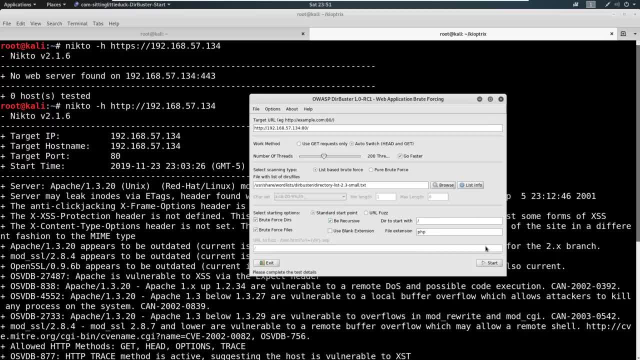 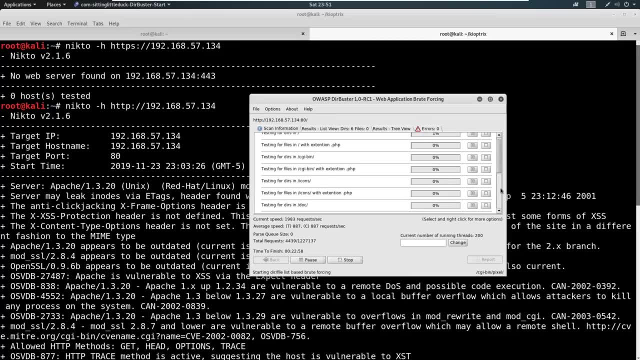 with the default results here and just kind of see what happens. so we'll go ahead and start that and this will kick off and start scanning and it's already finding right away it's finding some stuff. you can see the list getting big and you can go to this results view where you can see 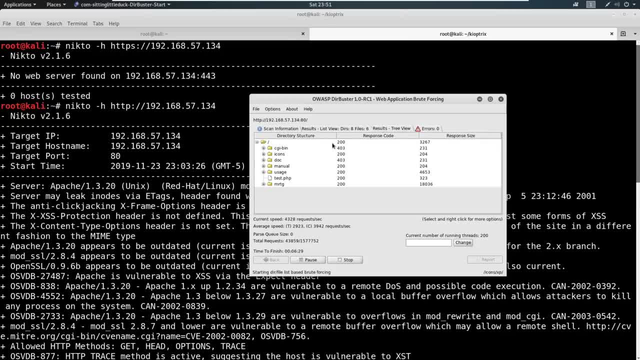 what it's found. and you can also go to this tree view here and see what it's found. you can kind of click in. you can see it's found some potentially interesting files. we can go enumerate these as well. and it's found testphp page. you can right click on these and open in browser. 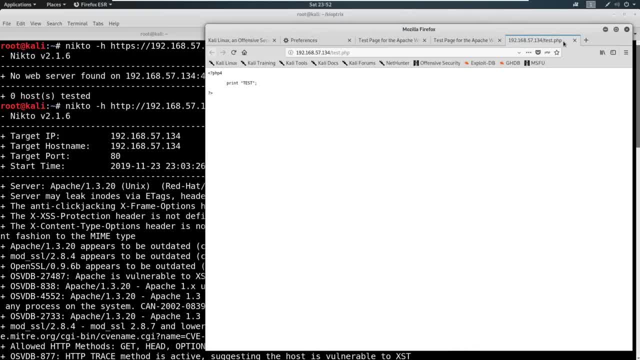 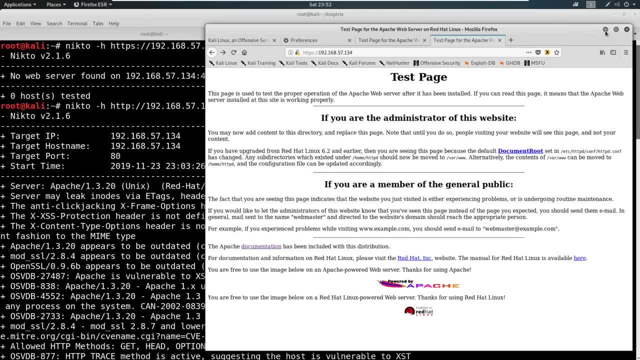 and you can see that it's found this print test here in php4 so we can look through some of these pages. we're going to go ahead and just let that go for now. it's going to take a minute. it could take up to a while to scan, depending on how big your word list is. how many options. 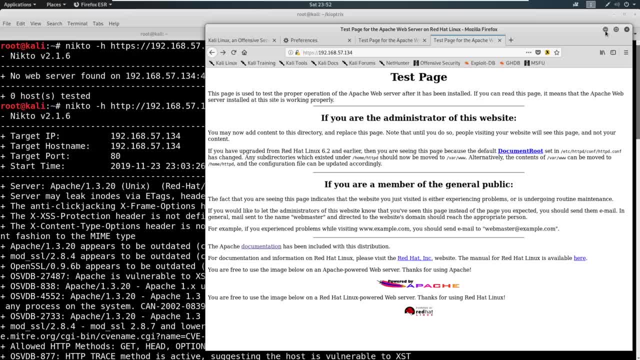 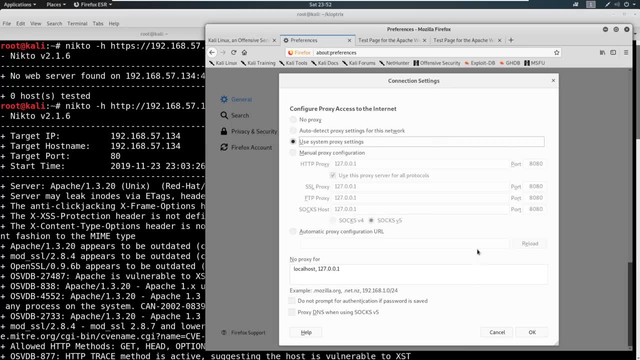 you choose and how well your website is cooperating with your scan as well. so from here, i'm going to show you a few more things. so let's go back to our preferences. if you still have that open, go ahead and go back. and let's go ahead and just go to the settings and we'll go to. 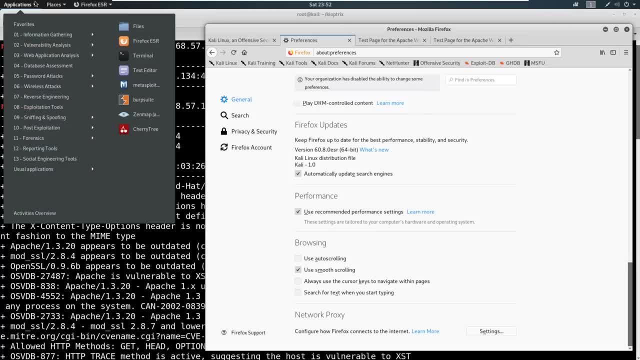 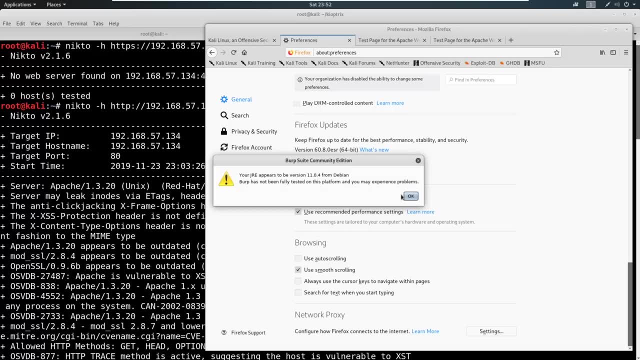 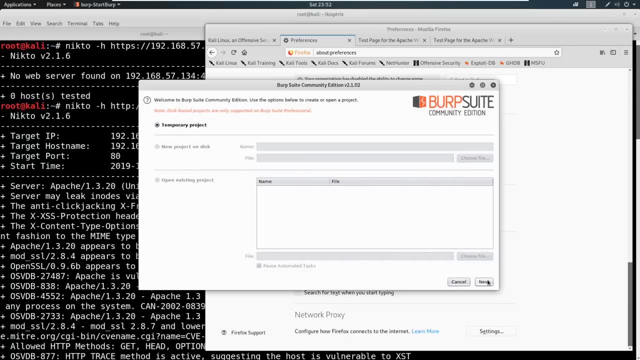 our manual configuration and let's boot up burp suite- and this is just another proof of concept that burp suite is your friend, especially when you're looking at websites, so we're going to utilize it just to take a peek. i just want to see what's out there, so we'll go ahead and just hit. 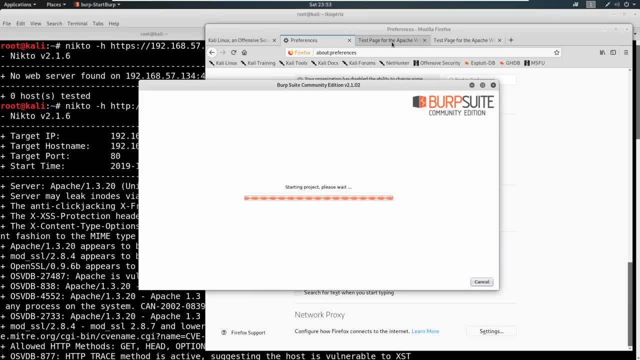 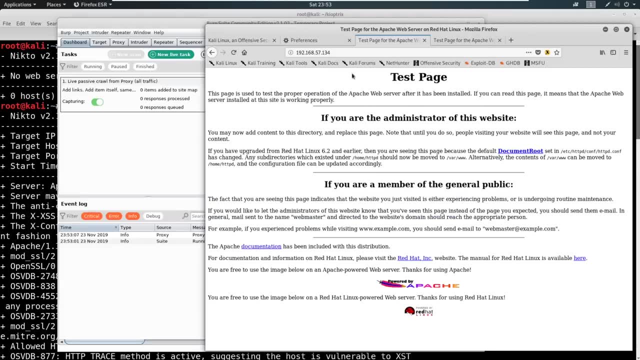 and start burp suite here on this, and while we wait, another thing that i need to point out is if this were a website like a real website instead of a test page, and a very important thing to do is view the source code, so we can right click in here and we could say: view page. 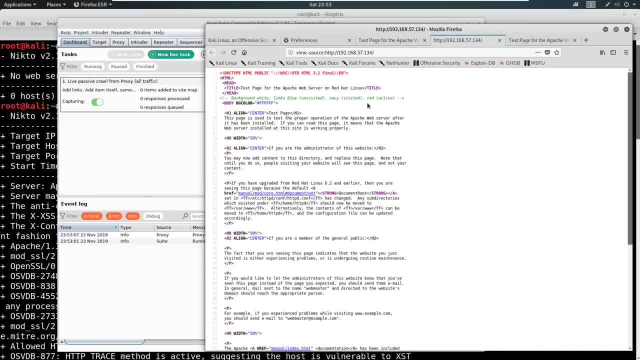 source and we can view the source code now. what we're looking for in source code are any kind of comments, potentially any kind of information disclosures. we might be looking for any sort of keys or password or user accounts or anything that might be disclosed in a source. 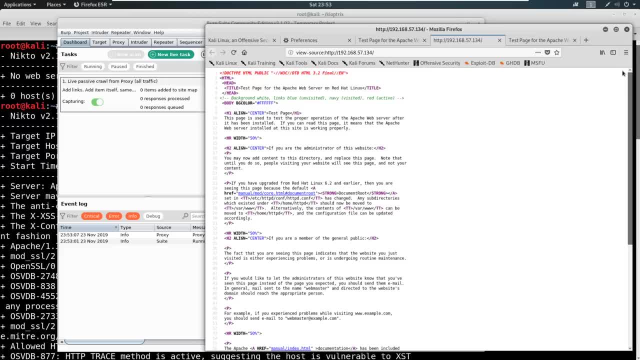 code that should not be disclosed. a lot of times when you do ctfs or you do hack the box or vol and hubs, they hide little comments in source code. but in a pentester point of view we're looking for more important things like the passwords or keys etc. so we've got burp suite open. 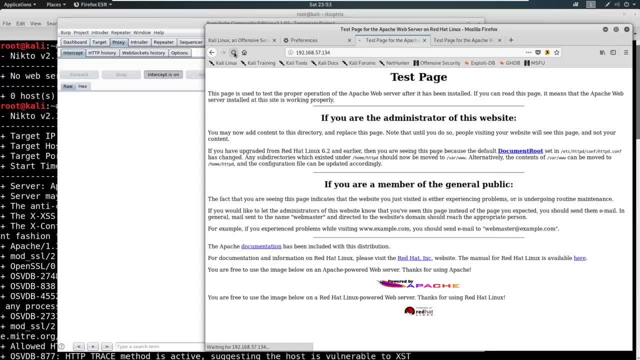 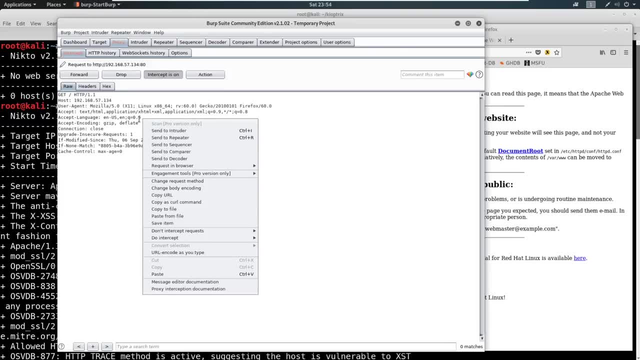 and we're just going to go ahead and intercept one request here and we're going to go ahead and just let this forward. actually, we'll send this to repeater. i'm going to show you a little trick. go ahead and send this to repeater, so you right click send a repeater and you'll see your repeater tab. 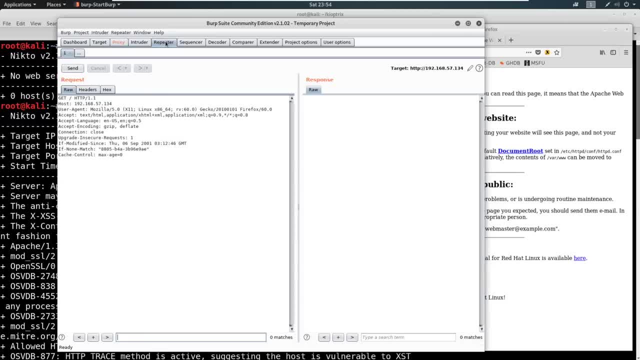 opens up here. now the neat thing about repeater is that repeater will show you your response in real time and you can modify these. so you could say, hey, i want to send this here. or you could say something about, like, i want to send a post request, maybe, and let that run and you could. 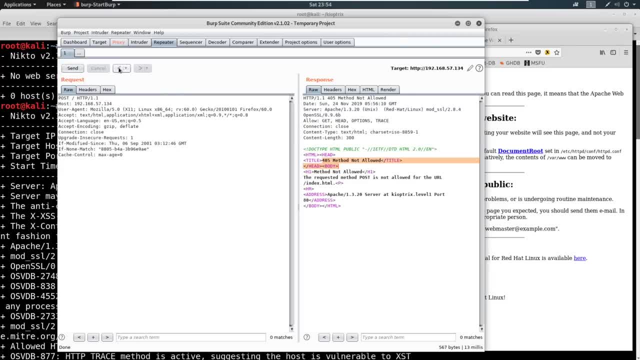 see. well, it says okay, method not allowed, so it doesn't like that. but you can send different results, modify what you see here and see how that works for us. now this is not taking this exactly, so let's forward and see, maybe, if we're missing anything, and we're not. so another thing: 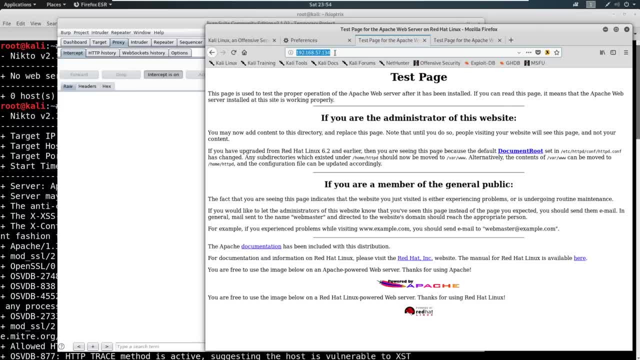 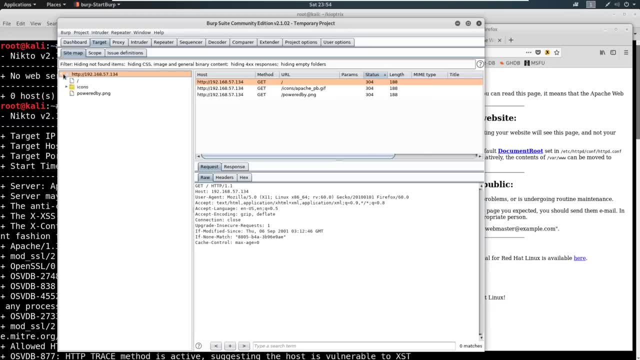 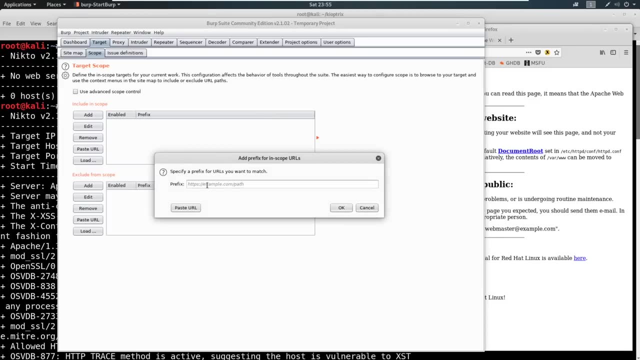 that we can do is we can actually copy this. and what we can do is we go into the target here and we've got the target showing we could set the scope if we need to. so we can just we can go to scope here and we can just say add and then paste this in here for http and we could. 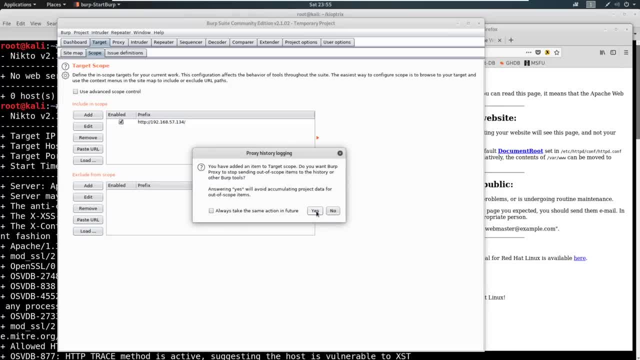 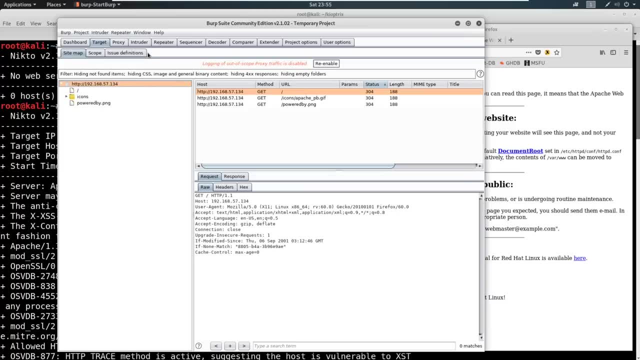 do https for both. let's just do http and we'll just say yes, and what this does for us is this: limits only searching for in scope items. so we're going to just limit now and then we're going to go ahead and look at the response that came back and you see there's no response here. 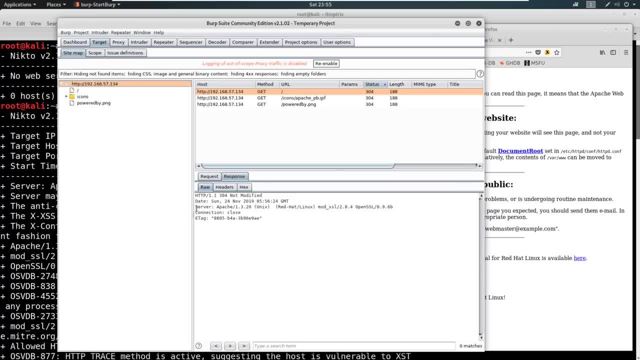 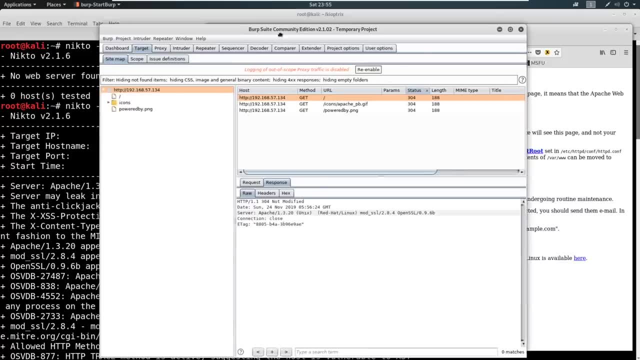 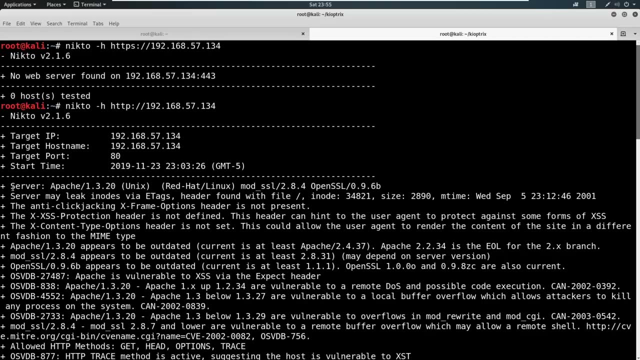 but there is a 304 not modified. and the interesting thing is, look at the server header. the server header is disclosing information to us as well and we saw this in the nycto scan. it's all coming back around, right. we saw the nycto scan say apache 1.3.20 and it pulled down this server. 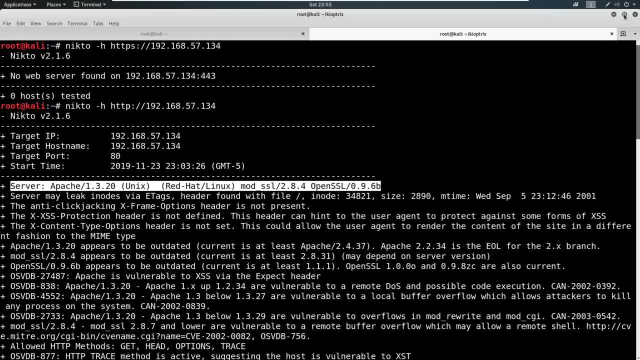 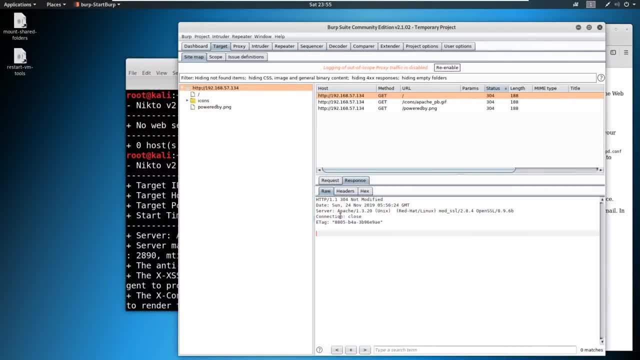 header. this is why it's so useful, and this in itself a screenshot of this. right here is information disclosure as well. so this client that we're working on has a little bit of information disclosure problems, and we can just say information disclosure problem and we can just say: 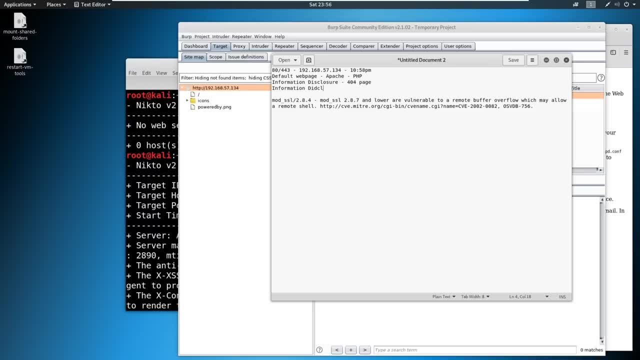 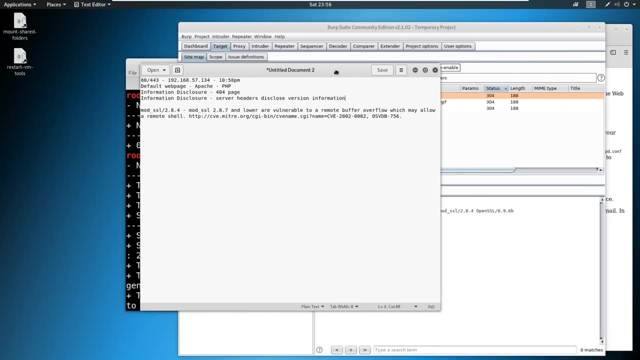 information disclosure here. and we'll do something, if i can type disclosure here, and we'll say something like server headers disclose version information, and we'll take a screenshot of that and we'll put that in our notes as well. so we're going to get really deep into burp suite. 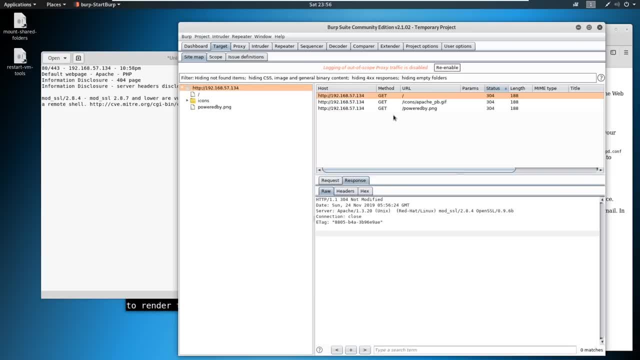 once we get to the web app section. i just like to get you utilizing it and familiar with it and just so you're comfortable by the time we get there. we're going to use it a few more times when we talk through network items and then, once we get to the 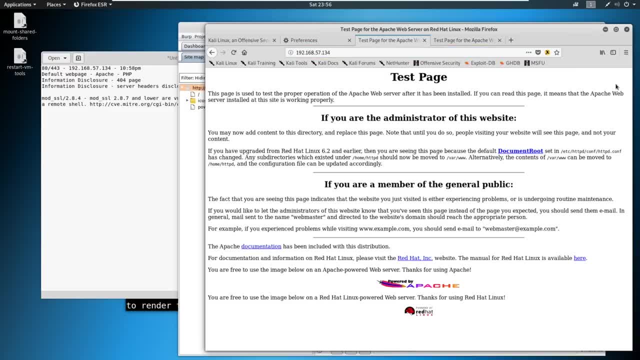 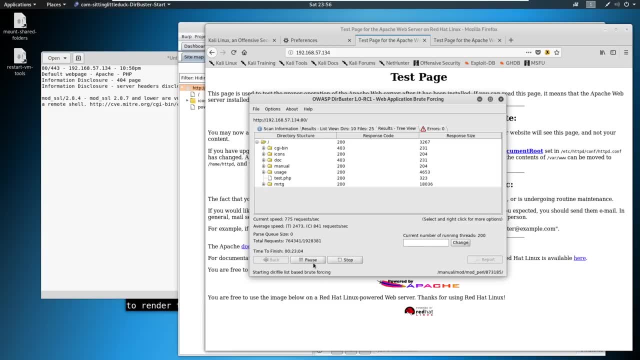 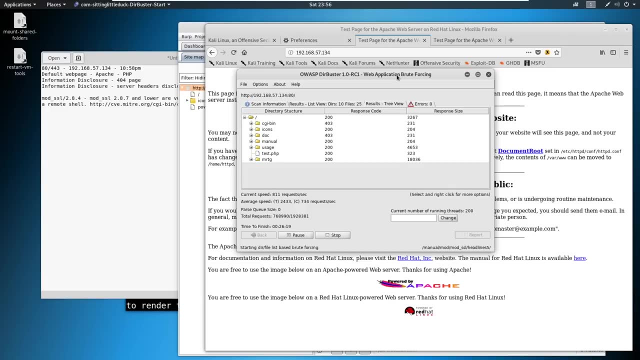 the web app. it's going to be a lot of burp suite so we'll get very comfortable with it very quick. so let's take another peek at our dir buster and see how that's working and you can see that it still has 23 minutes. but i really just want to put you through the concept of it. the concept of it. 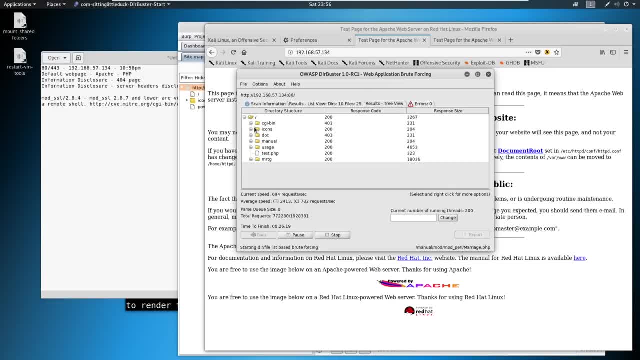 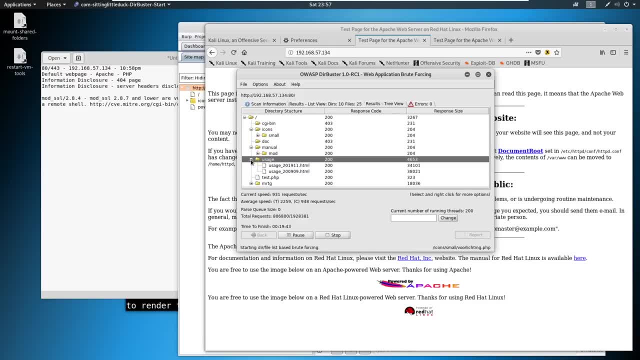 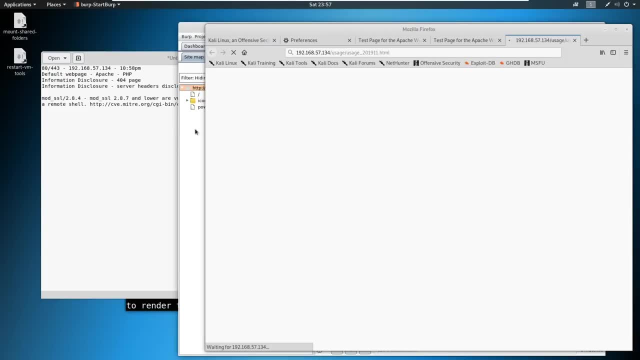 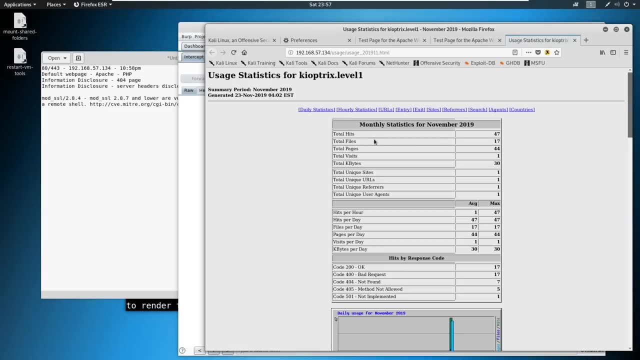 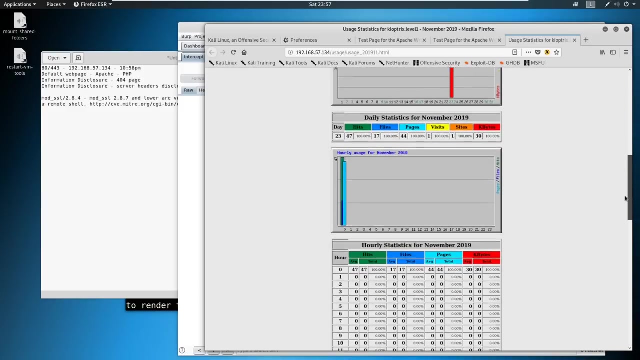 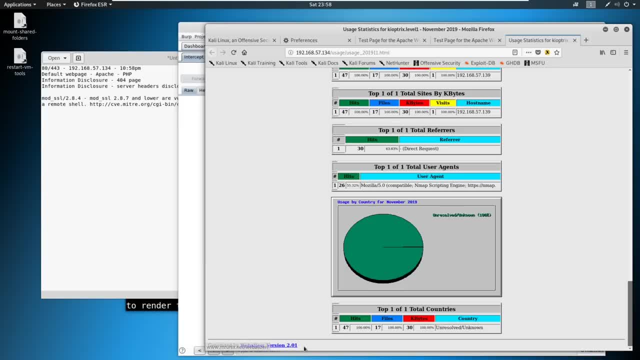 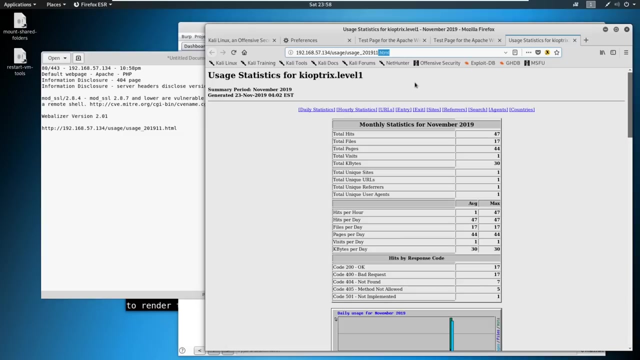 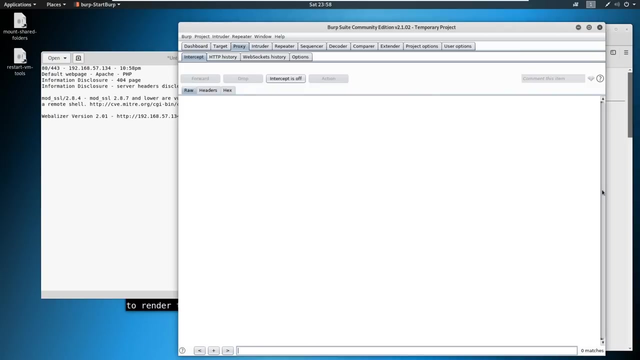 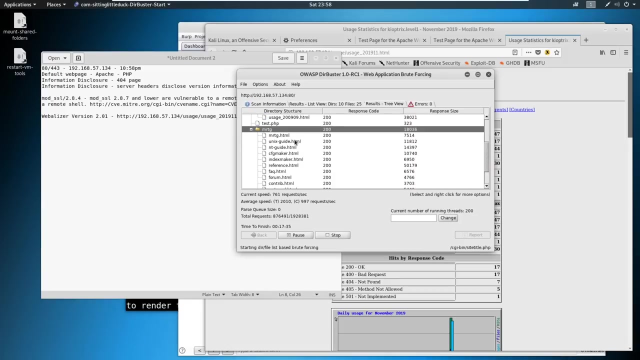 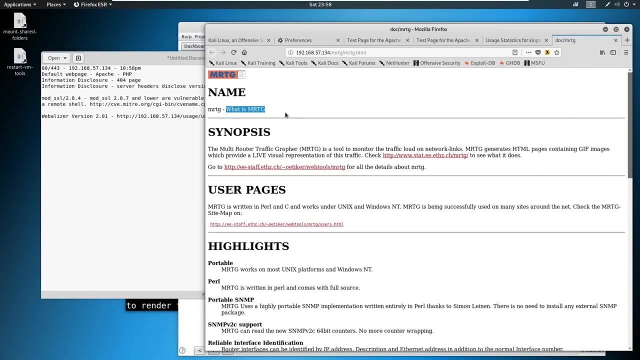 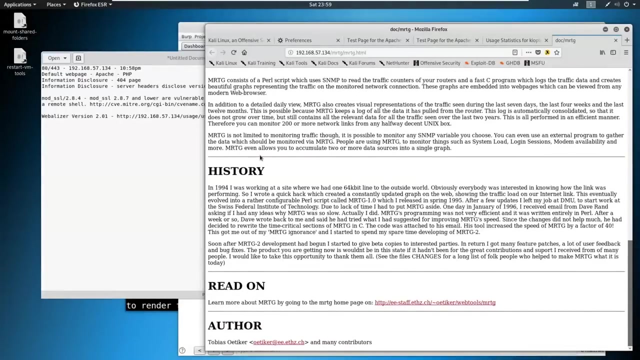 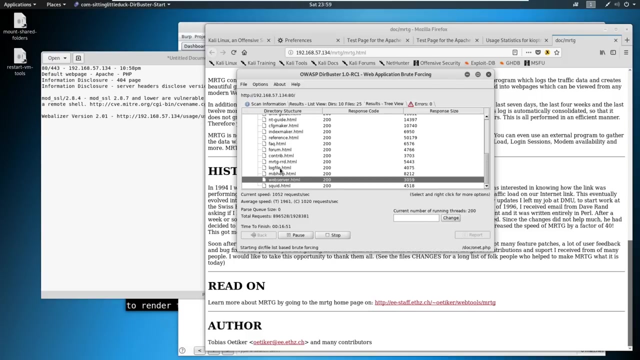 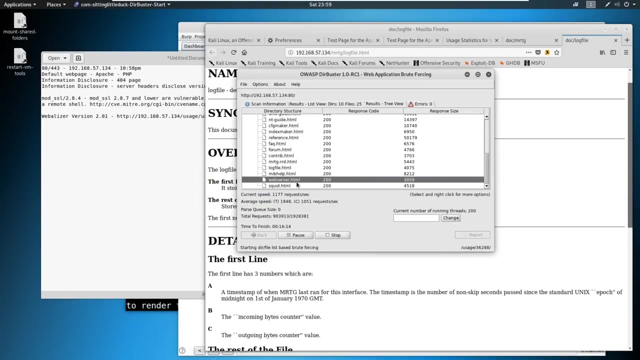 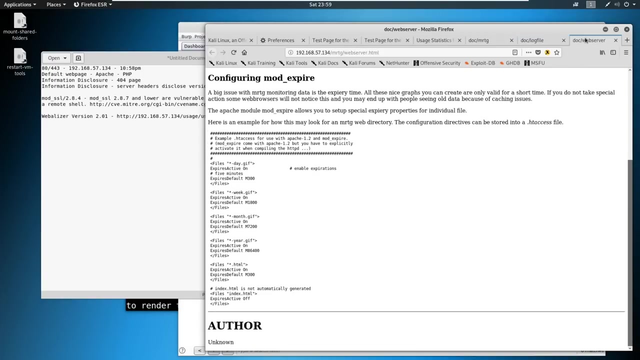 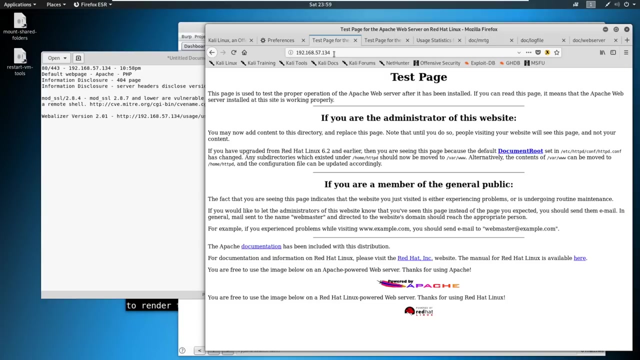 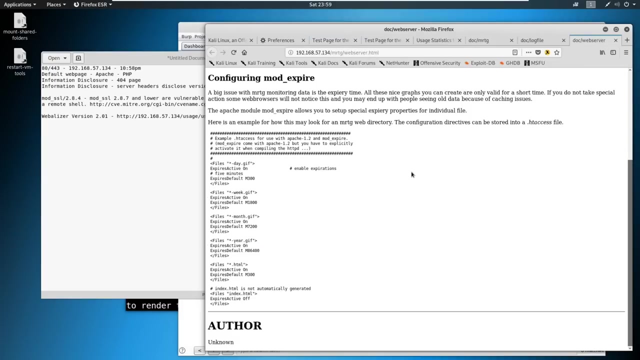 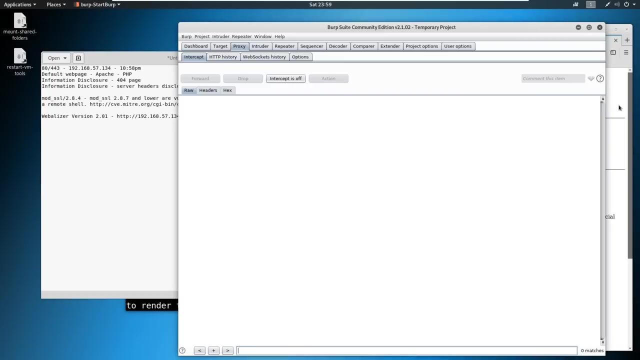 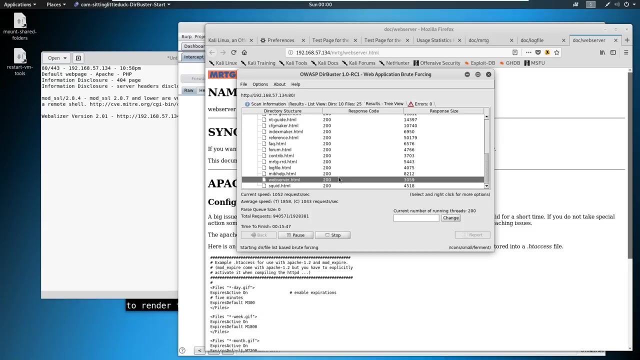 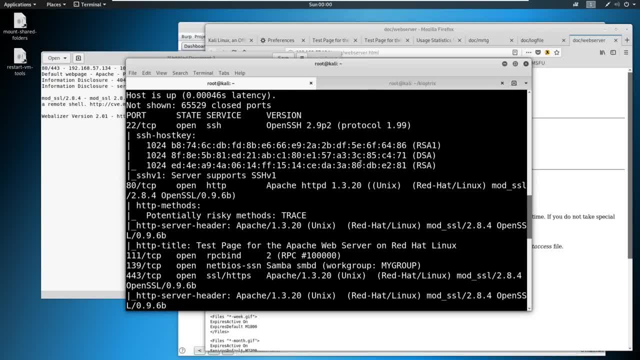 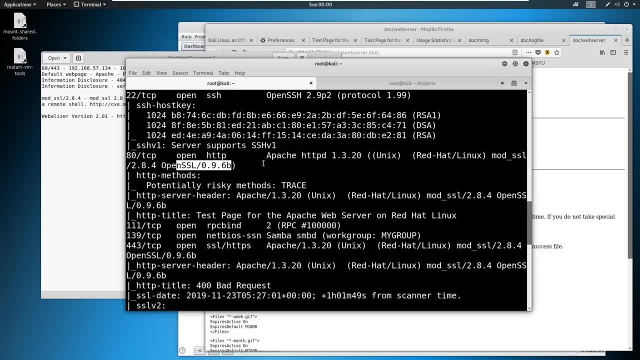 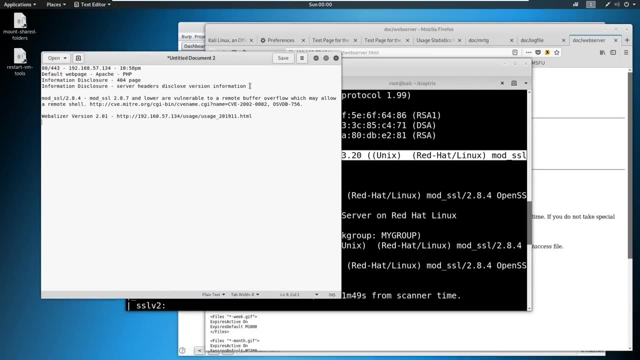 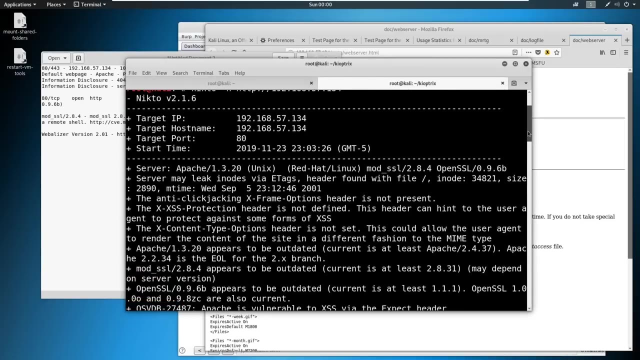 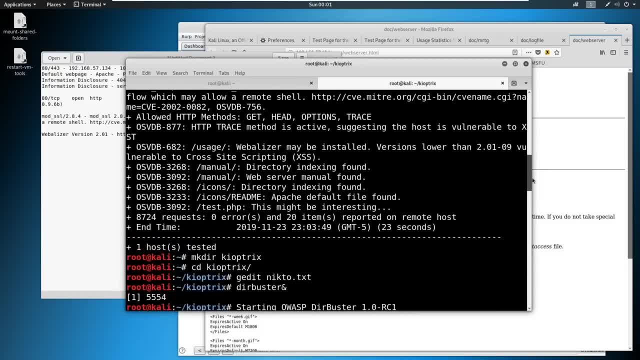 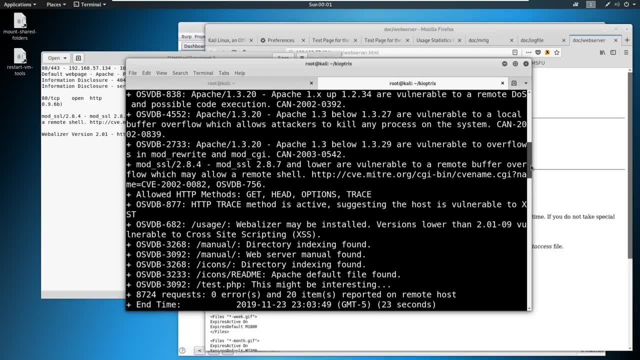 that we've written down as well. So it appears that there are some potential vulnerabilities here, But we won't know until we start digging into Google. Okay, and that will be very, very important, But we're going to get to that when we start getting into the end of. 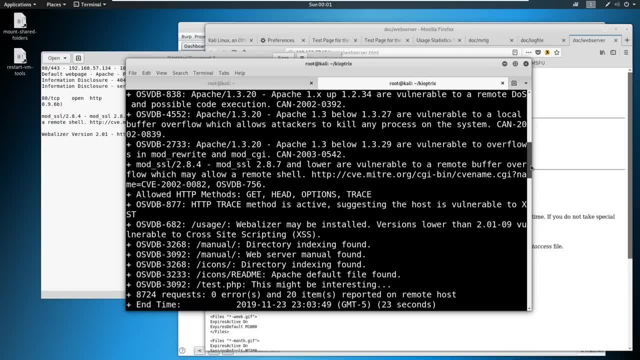 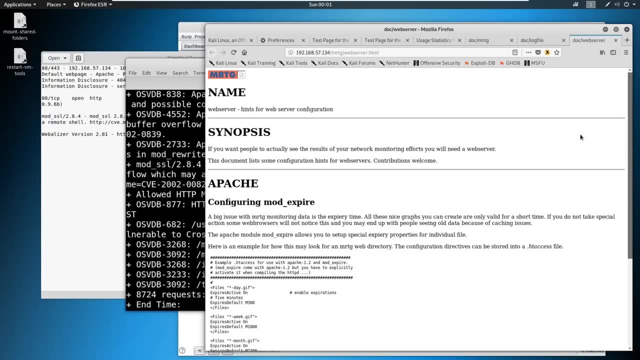 this little series here And then we get in transition into the exploitation part of the series. we'll work on exploiting these. So this is just a few tricks on how you can enumerate websites And when we're coming through and showing you these ports and we go over all. 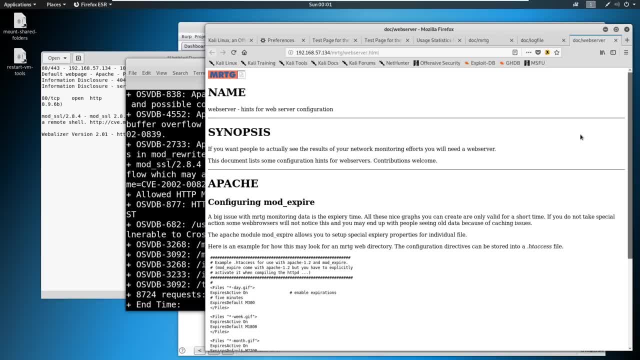 these ports that we see. we're going to come across new ports when we do pen tests And what. what it comes down to is just having a methodology. you might discover a new port And as long as you have a methodology, that's all you need. So we're going to work on building that methodology And 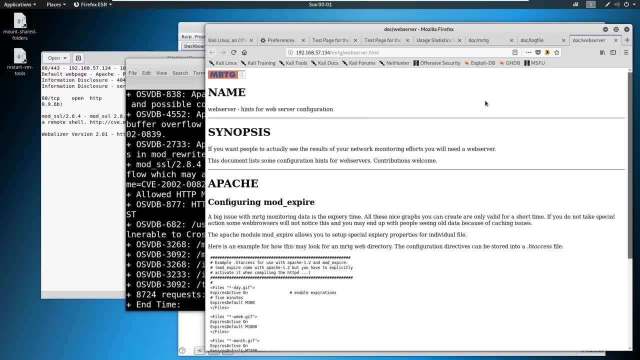 you might find other tools for for searching websites that you like. you might say, Hey, I hate your methods, or you know, these tools just work better for me, And that's absolutely fine, as long as you're developing your own methodology. So just start thinking about, when you see a website, what are? 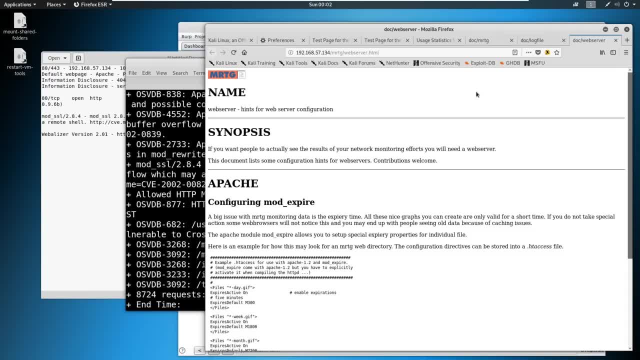 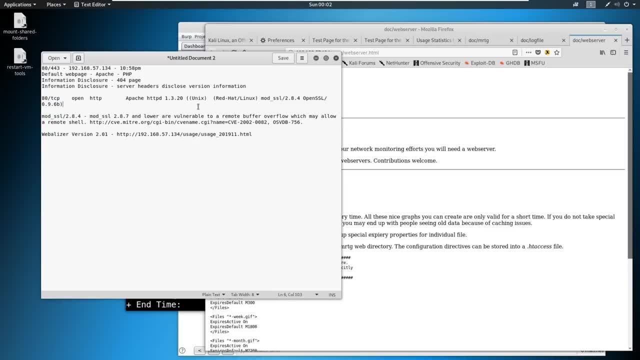 the basics that you're looking for When you come across the website. you're looking for service version information, which we have here. you're looking for any sort of- maybe back end- directories. you're looking for source code. you're looking for potential vulnerability scanning with Nikto. 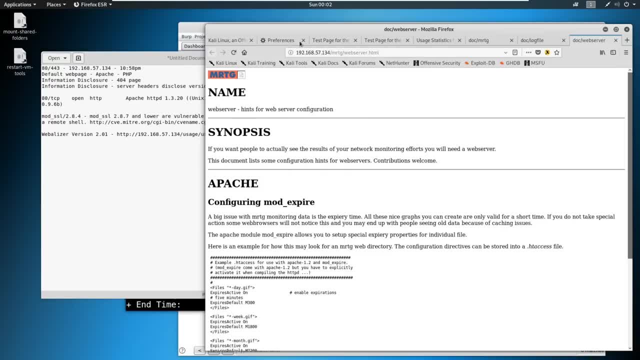 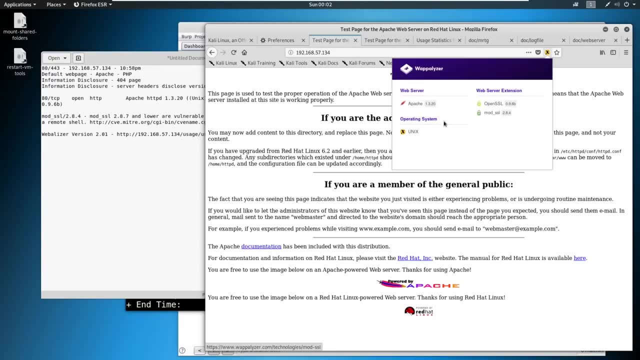 and any sort of information that you can divulge. Same thing. we can come back here- we talked about it before- with wappalizer. you can click on wappalizer and see a lot of the same things that we saw. it knows the operating system, it knows the web server extensions and it knows what's. 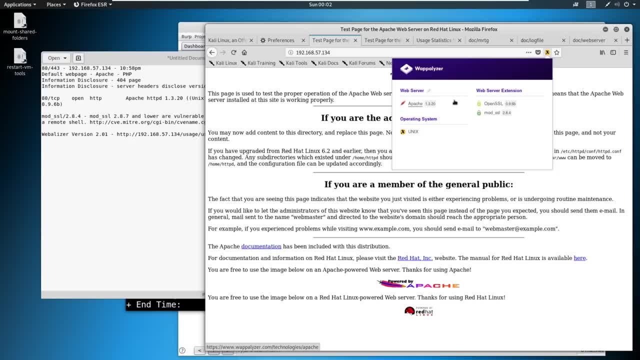 running on the back end. So there's a lot of useful information here And this is all we are after at this point. we just want to scan and enumerate And then we're going to dig deep and exploit. So that is it for this. we're going to move on to the next part of the video. So if you're 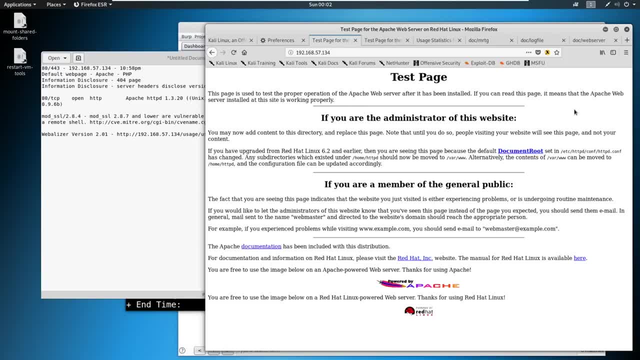 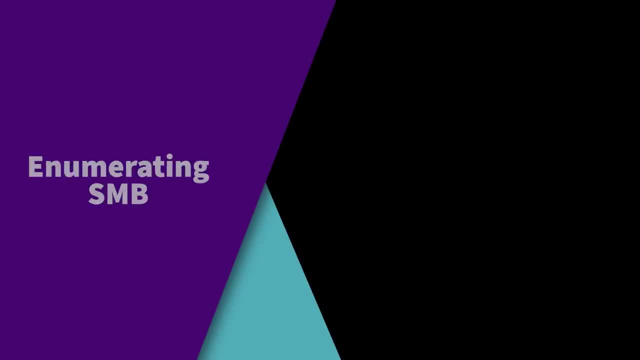 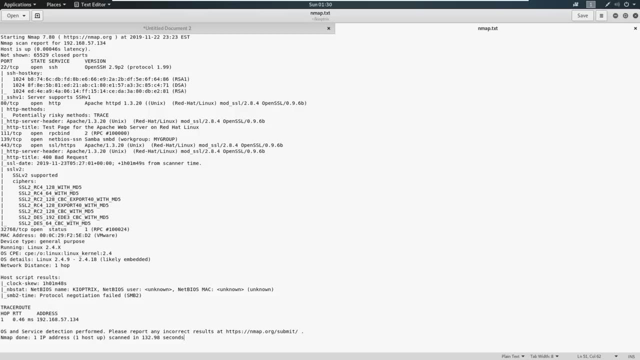 new to this section. we're going to do a little bit more enumerations, see what else we can uncover. So I will catch you over in the next video. Now that we've taken some time to enumerate web pages on port 80. And 443,, we're going to go ahead and shift our focus over to SMB on port 139.. 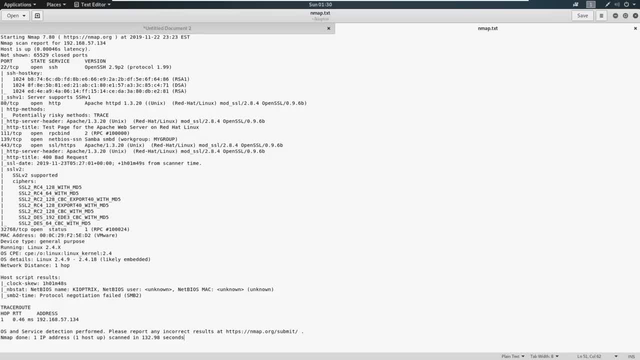 So if you are unfamiliar with what SMB is, SMB is a file share. So think about your work environment. if you go to work and let's say that you have a drive you access, that's not like your common drive, like a C drive, maybe it's like a Z drive or a G drive. 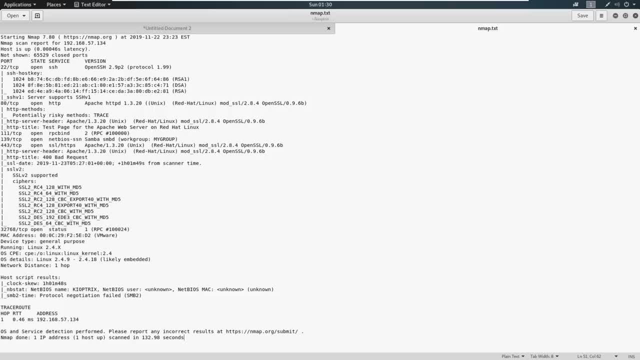 And you access that, that drive to get files and you can upload the files, download the files And then maybe some of your co workers can also see that file share And that's why it's called a file share. Another example is say you have a scans folder and you go to your printer. 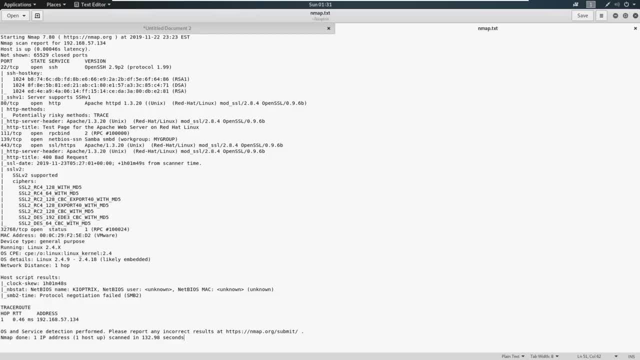 you scan something and magically it appears in your scans folder on your computer. That's another example of SMB. So SMB is commonly used in work environments and internal environments. So when we see it we think internal and we think about all these exploits that I have mentioned in the 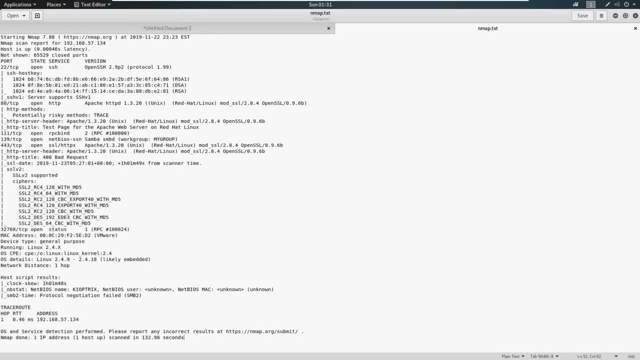 past with, especially with latest and greatest being MS 17 010.. And even though it's two years old, it still shows up, And it's going to show up again in this course later on. So we're going to do is we're just going to take a quick look at our scan and see what we have. 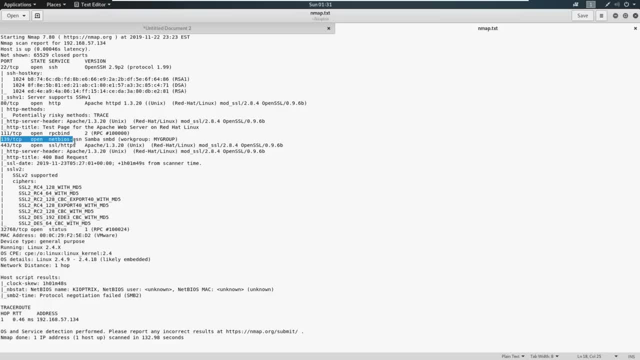 available to us. So on port 139. Here we see that. okay, NetBios SMB workgroup- my group- not really a lot of information we could scroll down And the great thing about the dash capital A that I had you run with this scan is that it does run script for us. So these scripts that 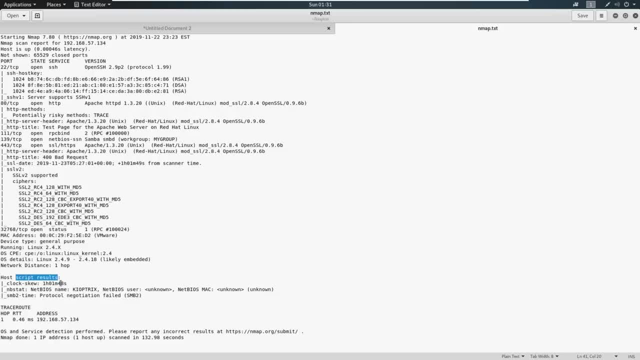 we're running, go out and do a little bit of enumeration or additional enumeration, And here it came through and it's pulling down some information. we could see that, okay, the NetBios name of this is called captrix. Well, we kind of already knew that. But 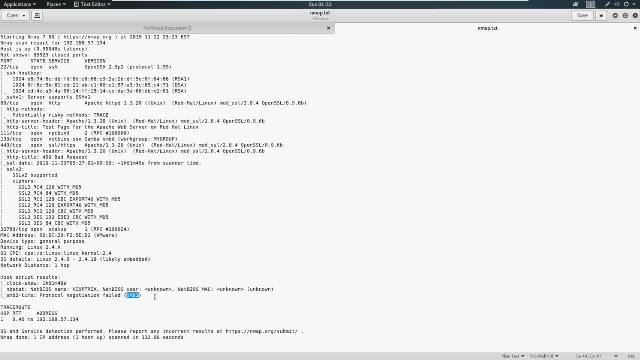 and we can see here that it's running SMB version two. we really don't know that for sure or what SMB version it's running exactly. So that's really important because the type of SMB version that's running could potentially lead to an exploit And we need to know. 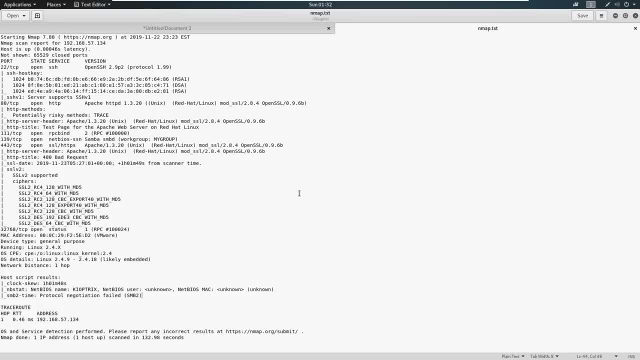 that And we need to know that the type of SMB version that's running could potentially lead to an exploit And we need to know that kind of information. So we're going to look for version information. The other thing is we're going to try to connect to this machine. we're going to see if there's any connections available. 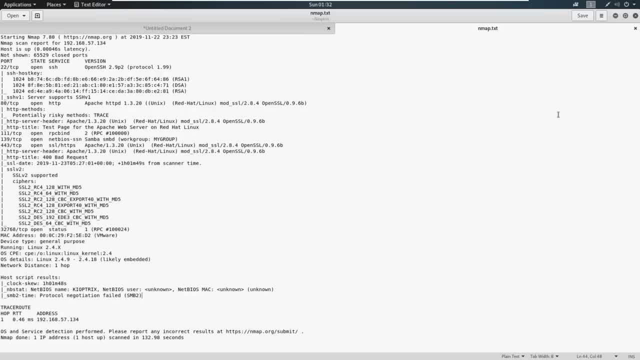 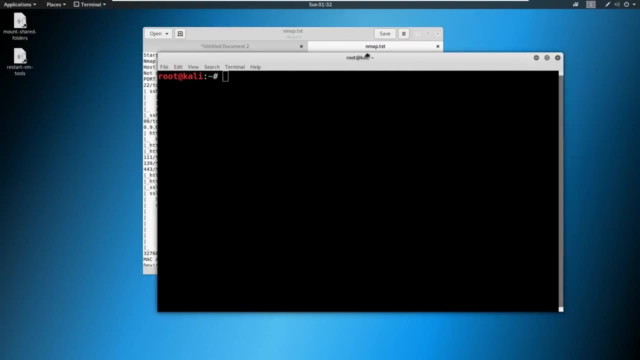 to us And if we can make that connection, if we can get to the files on the share and see if there's anything potentially malicious or that we could do potentially malicious. So let's go ahead and let's get into a terminal And we're going to load up a tool that you're going to be intimately. 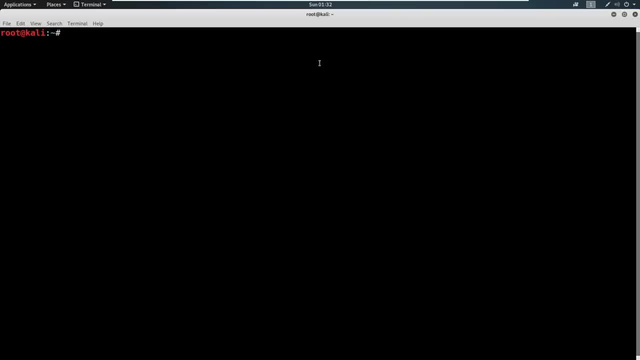 familiar with by the time this course is over, And that tool is called a terminal And we're going to run that tool called Metasploit. So to run that tool, just go ahead and type in MSF console like this And hit enter Now. 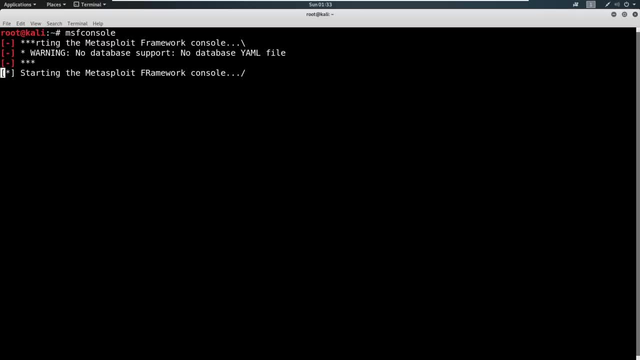 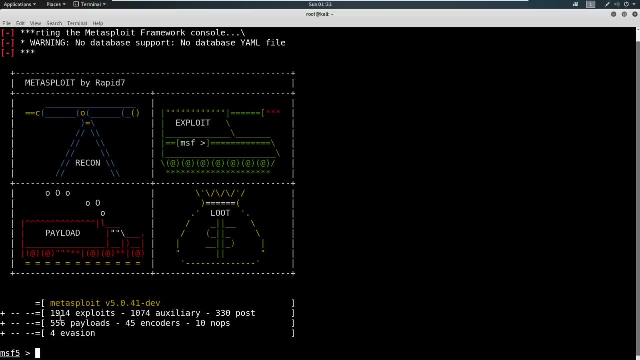 Metasploit is a exploitation framework And it does a lot more than exploitation, As you can see down here. you can see that it does exploits what are called auxiliary modules. Now, auxiliary modules is like scanning and enumeration, So we can actually do port scanning. we 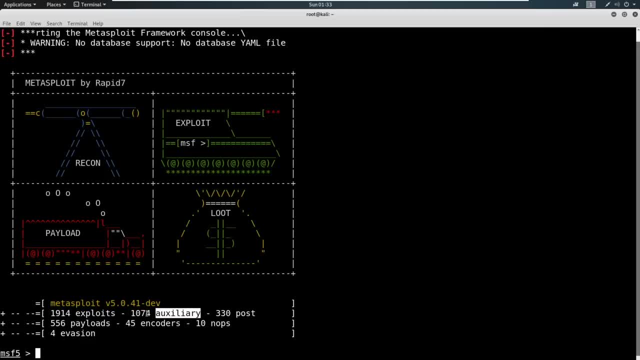 can do all kinds of information gathering With these auxiliary modules. they're awesome. We're going to go through one right now. There's also these post modules which do post exploitation. So say, we get a shell on a machine, which means we've exploited a machine. 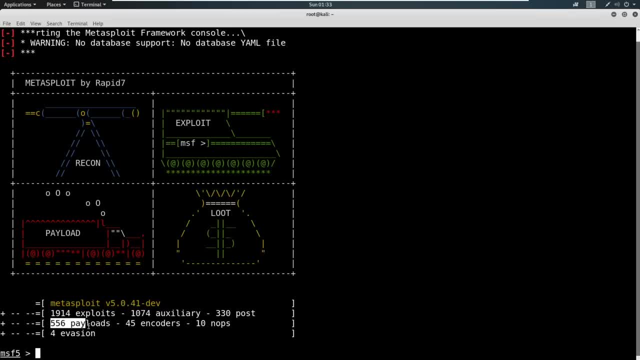 we can do some things in post. there's all different types of payloads which we're going to cover when we get into the exploit section And then the rest of this. you don't have to worry about that for the scope of this course. But we will be seeing another tool by Metasploit, which is MSF venom. 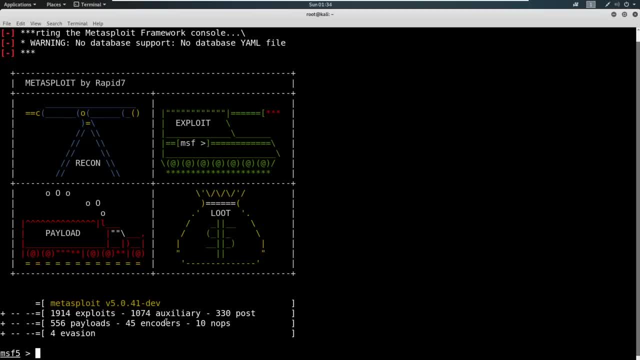 later in the exploit development section of the course, because we're going to utilize that to build payloads out for our own shells. So what we're going to do for now is we're just going to introduce this slowly. don't feel overwhelmed. It's just a little bit of a learning curve when 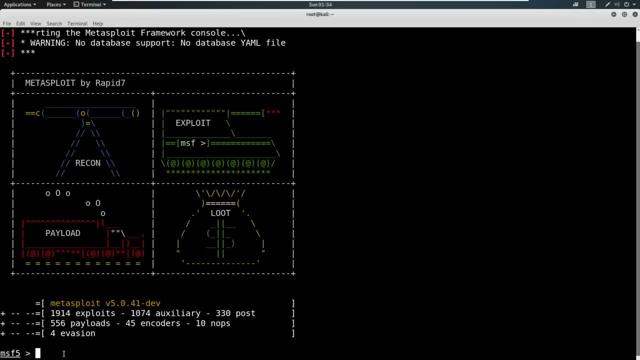 it comes to learning all the features that it has available. But it's second nature once you learn it and it's going to be one of the most commonly used tools that you use as a tester in the field. So we're going to go ahead and just search for SMB here, And I'm going to do this. the 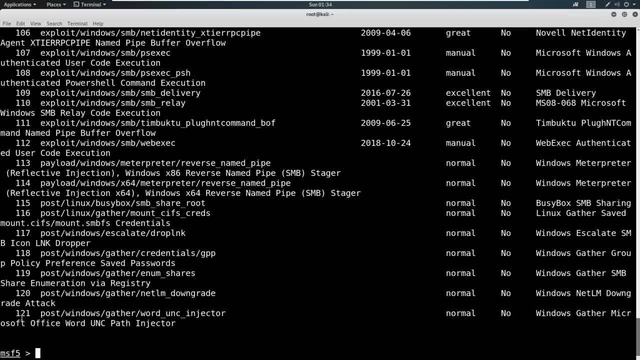 terrible way. we're just going to search SMB And you can see that there's 121 results. Now that's going to be quite a pain to sift through. But what we're after and say we didn't know much. but we were trying to see if, Hey, maybe does medical eat have any kind of modules? I don't know. 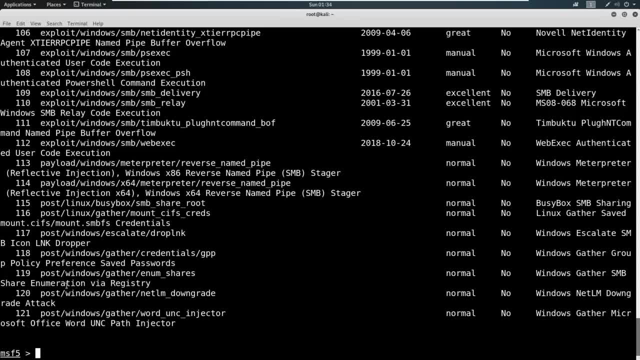 for SMB enumeration. Well, we know auxiliary modules are enumeration And we're going to go ahead and just search for SMB. And we're going to go ahead and search for SMB. And we're going to do this the terrible way. We're just going to search SMB And we're going 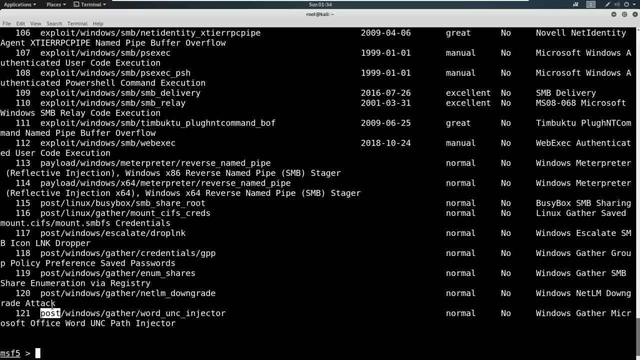 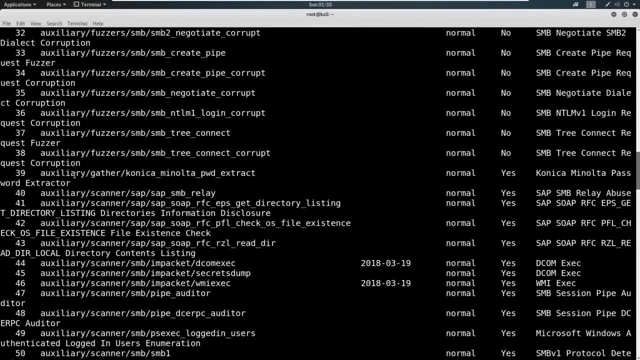 can look right here in the front and see what type of module it is. So you see this is a post module And you see we could scroll up. we're going through exploits and then we're going to go up into auxiliary. Now, the second part of this is the type of of action it's doing. So you can. 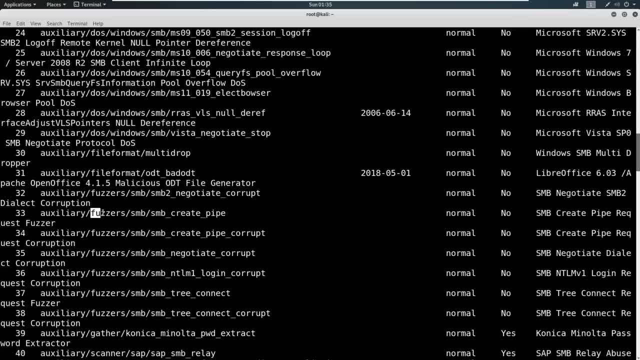 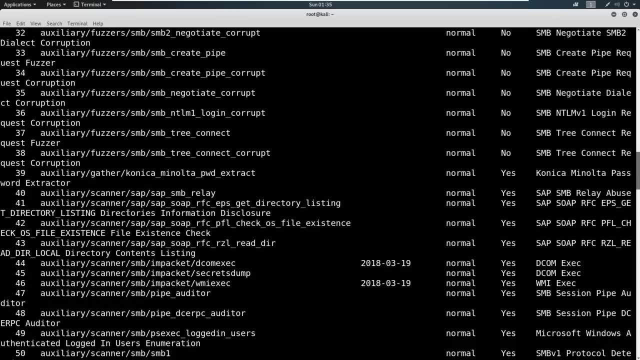 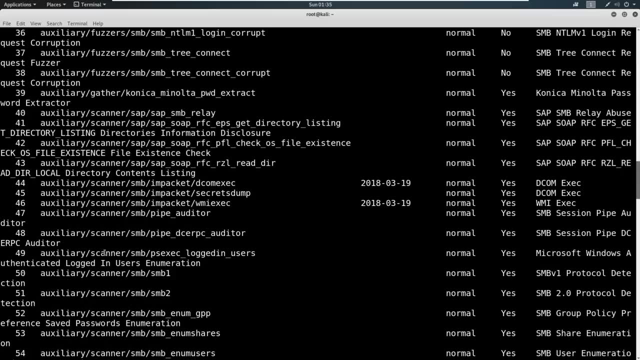 see auxiliary denial of service, auxiliary fuzzing, auxiliary scanning, gathering- and we're going to utilize this to our advantage. So we're going to take a look at the syntax Now. what we are after is SMB version information, And if we look kind of through this, we can come down to scanner here. 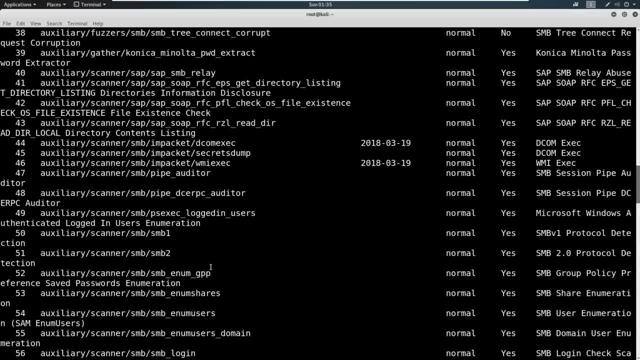 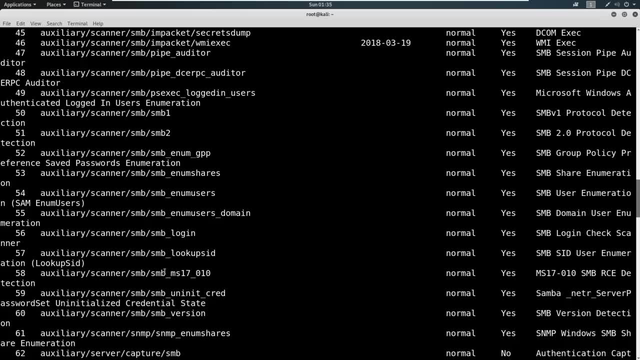 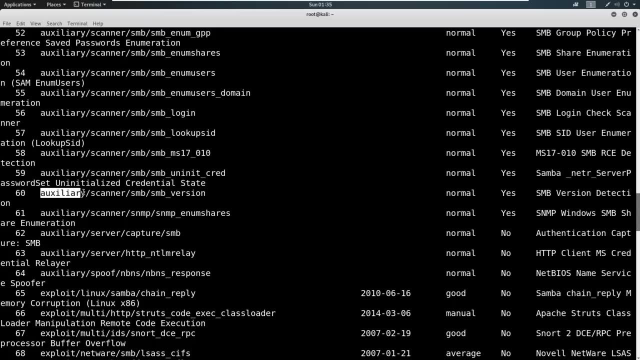 And you can see it's looking at some B one to GPP, which we're going to talk about, ms 17 010, which we've talked about. you have an auxiliary scanner to see if there's anything out there with that vulnerability And if we look right here on number 60,. auxiliary scanner. 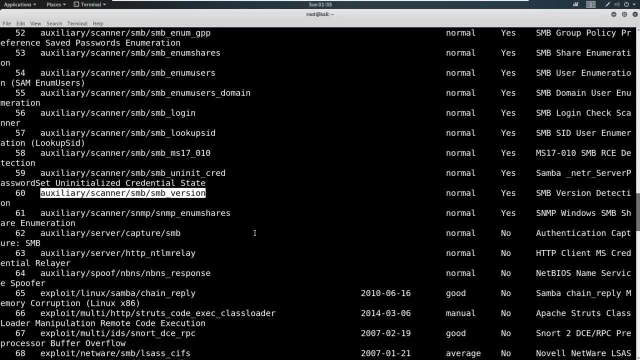 SMB version information. And if we look right here on number 60, auxiliary scanner, SMB version, SMB, SMB version. Now, this is a bit of a long, convoluted way to do this. go ahead and copy this, by the way, or memorize your number. I'll give you two options. This is a long way to do it, But I. 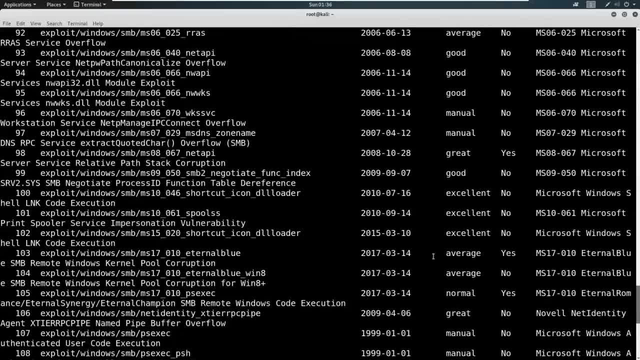 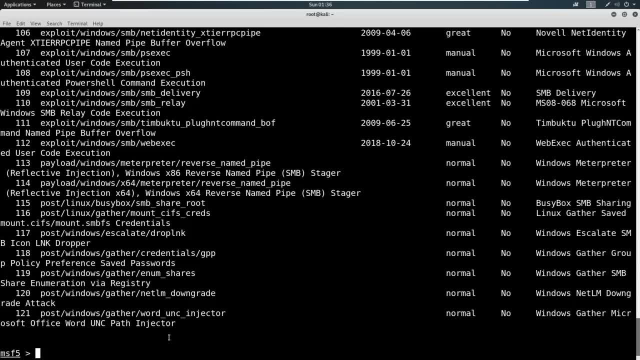 wanted to show you this way of doing it because you're going to get better at it. But you know, when you see something on a scan result and you don't know a lot about the tool, the best thing that you can do is just say: Hey, you know, I know Metasploit does things like this. Let me see if. 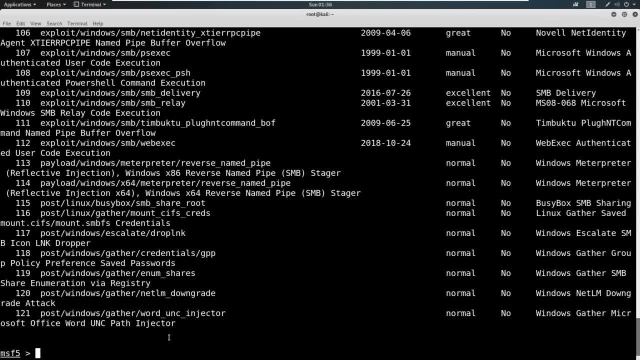 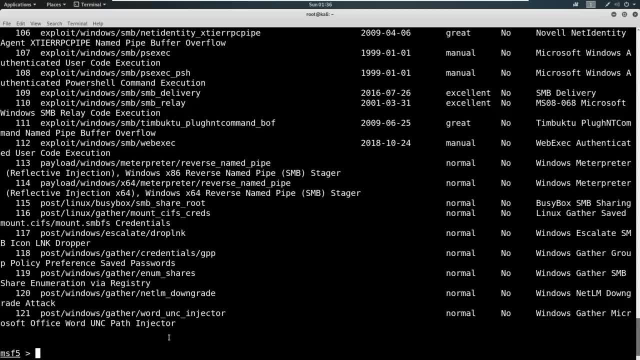 to use search feature to try to look up items and learn about them. So let's say we've never used this before. we're going to go ahead and just say use and then we're going to paste this module in here. Your other option is, instead of pasting this module, you can put the number that 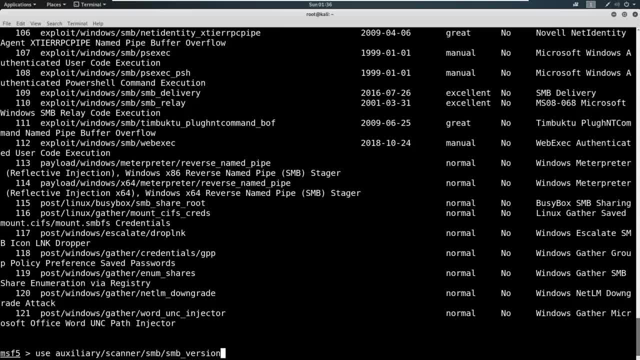 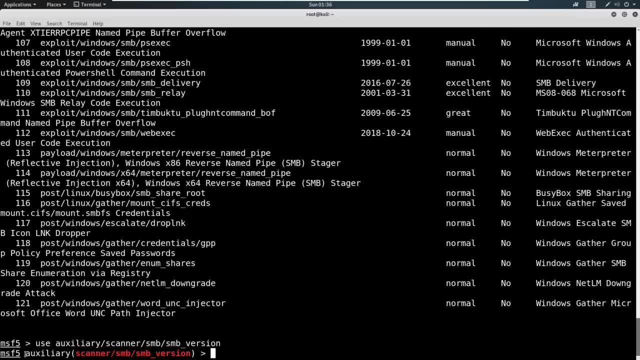 you had, So like, for example, 60,, you could say use 60. And it will also load this model. So go ahead and hit enter for that And you can see here that it says: now we're in an auxiliary module. 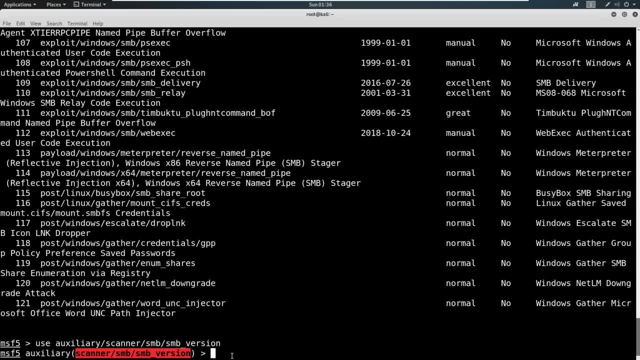 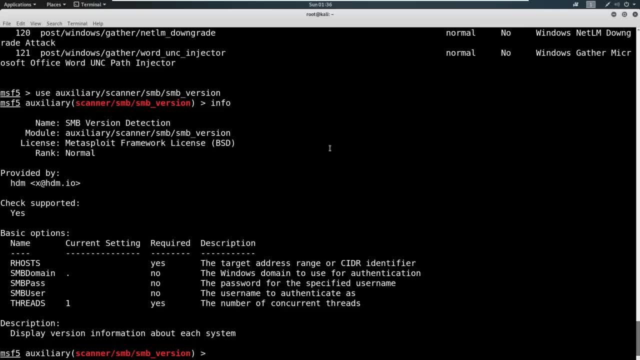 of scanner SMB, SMB, underscore version. So from here it's always good to type out info and see what info is available- And just tells you a little bit about the module that you're running. So here you see that this is going to display version information about each system. Perfect, 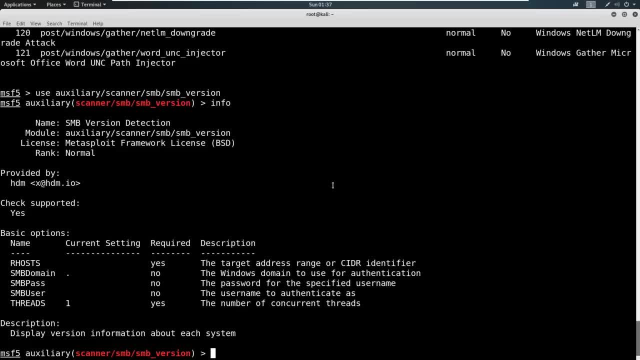 it's an SMB version detection. That's really what we're after right now. So this is great, And we have options here, these basic options. Now, you're going to see me do this a lot. you can go right into options by just typing options and just see that instead of printing. 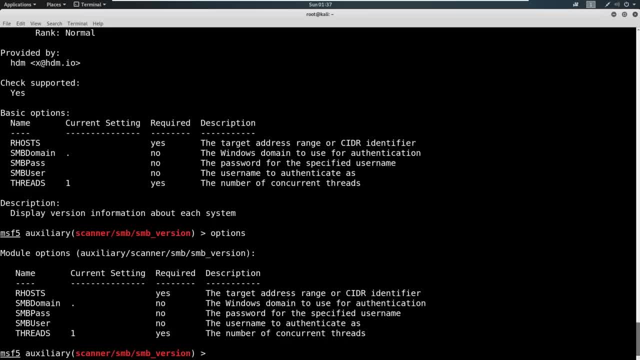 out all the long stuff if you don't want to. So in our options we're presented with some items. we've got something called our host. Now, our host is what stands for remote host. you're also going to see an L host later on, which stands for local host. Our host is always. 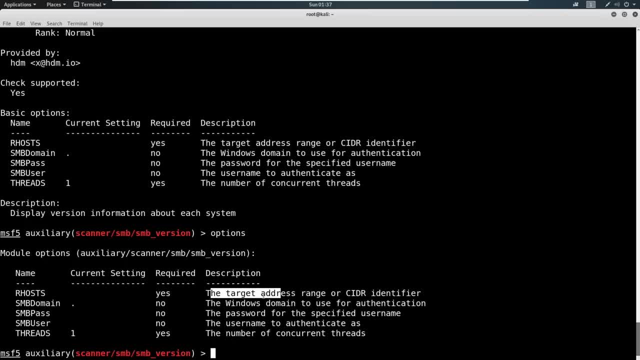 the victim. That's who we are attacking. This is the target address. you might see our host or our host. plural Our host means you can only implement the same thing over and over again, So you can see the same thing over and over again. 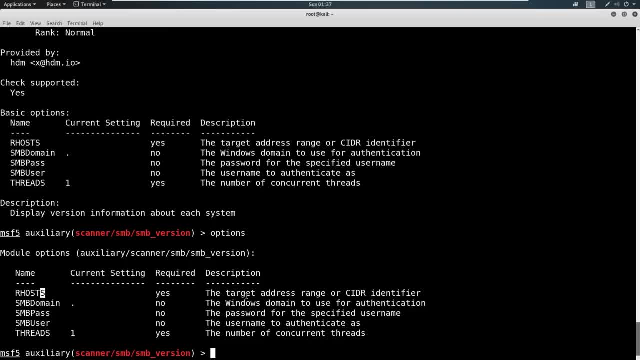 One host. if we have our host plural, we can use cider notation, meaning that we could put slash 24 and try to sweep a range, for example. But in this instance we're only attacking one machine anyway. The rest of these SMB, domain password and user. if we knew the domain password. 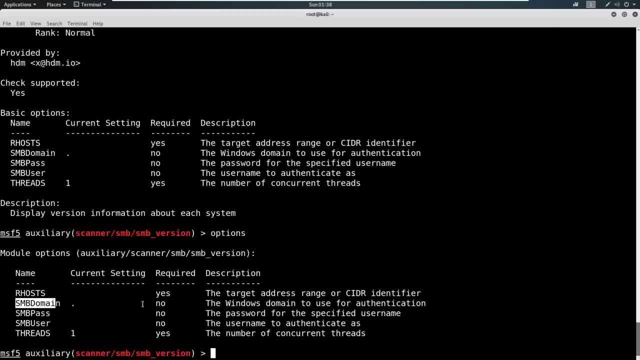 and user. In this instance, we could fill it out and try to get a little bit more information, But we are unauthenticated. We have no credentials at this point, So we're just going to go ahead and just put in our host, which is required, and not fill out any of the non required fields here. And 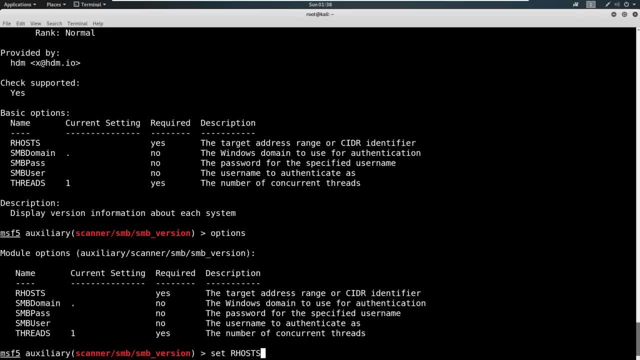 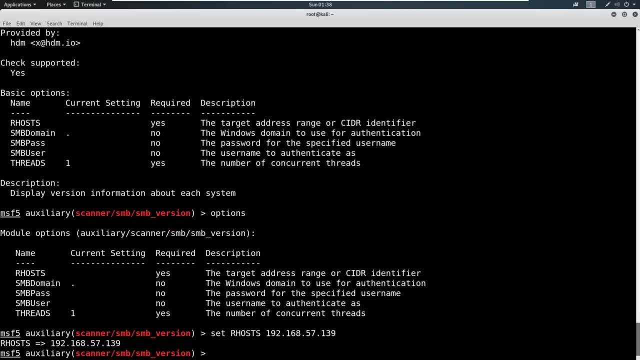 what we're going to do is we're just going to say: set our hosts, And this isn't case sensitive. I just like to type it out, case sensitive. And then the IP address of the machine that you're going to scan. So we're going to say 192, 168 minus 57.139.. And then I'm just going to type in: run. 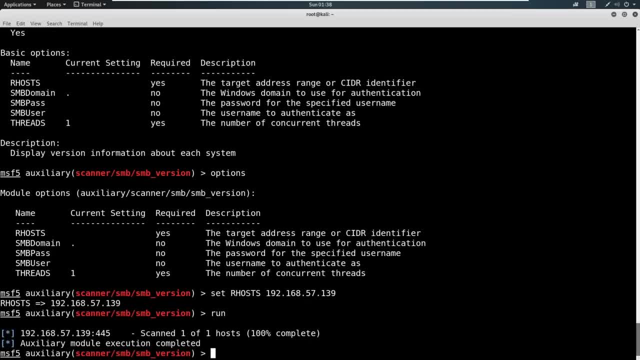 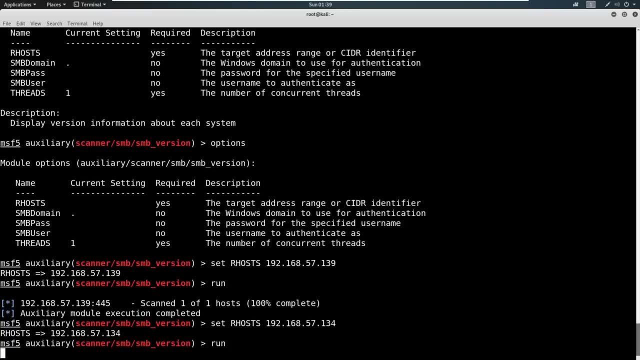 give you a second to catch up And run. Okay, I totally lied. My IP address is 139.. The machine I'm after is 134.. And run. your screen should look something like this: I'm over here, instead of copying and pasting, trying to memorize. 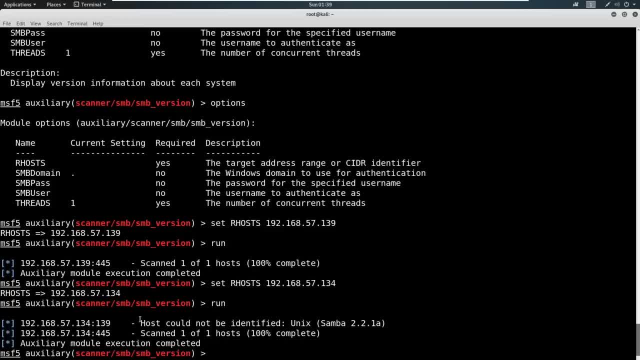 So hopefully you can see that I make mistakes too. So here we are. we see a little bit more information, and it might not look like a lot right now, But knowing the Samba 2.2.1 A is very specific and this is going to help you. 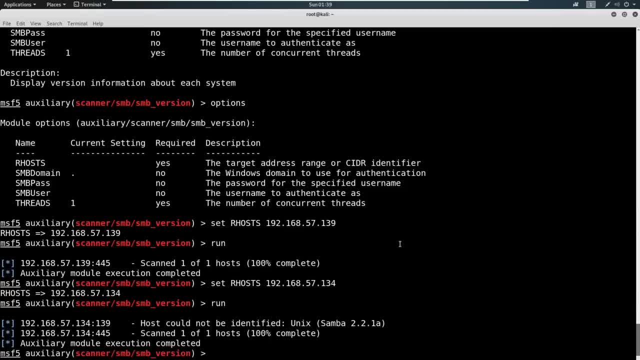 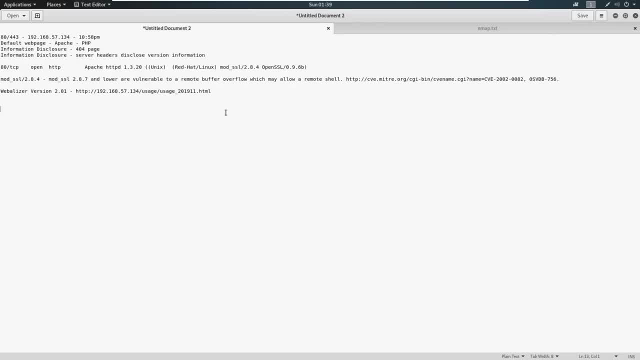 out quite a bit. So let's just copy this guy And let's open up that text editor we've had going And let's just come in here and maybe make some notes or just put it in here and say something like SMB, And then we can just put, paste, that we know the version now And this is going to become. 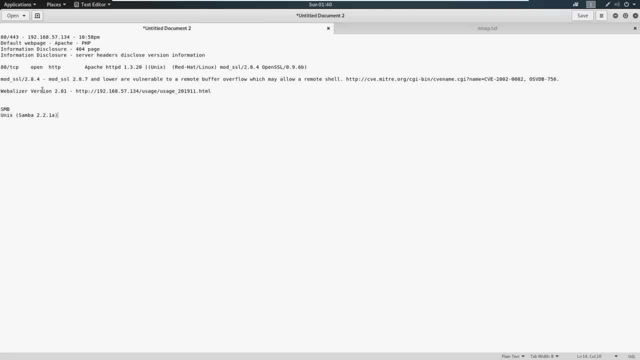 important when we start doing research on what we've found. So we found all these different types of versions running up here And we're going to do research on exploitations against them. But we're also going to do research on this and exploitations against this. So as much detail as we can get, that's what's. 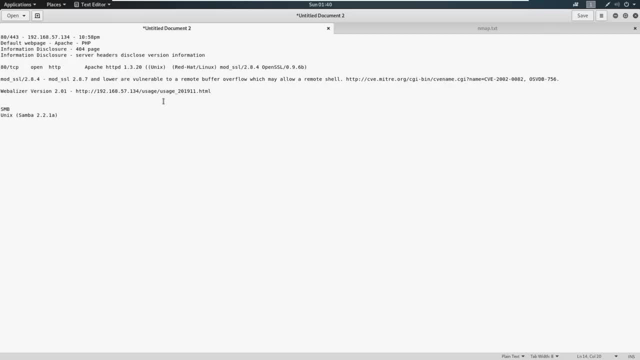 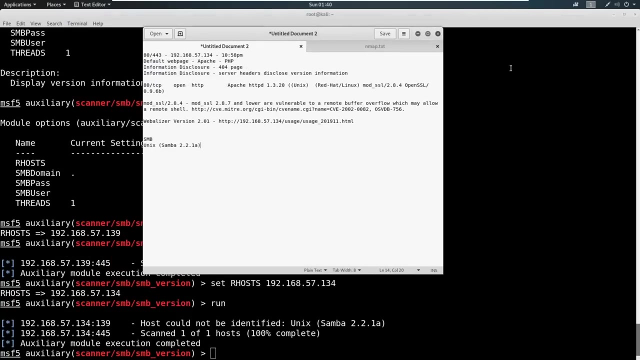 important And what's going to set you apart from other hackers or other people even trying to break into the field is your ability to information gather and your ability to enumerate. if you can do both of those, The exploitation is actually the easy part, in my opinion. So we've got the 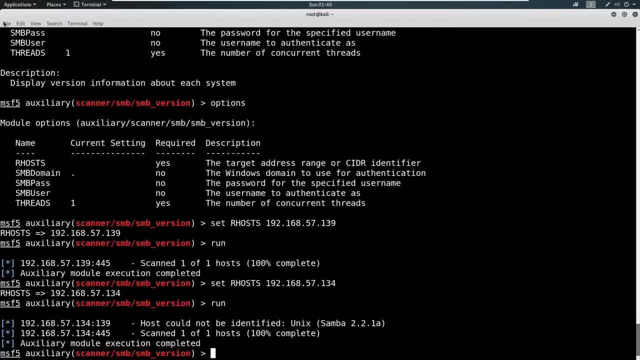 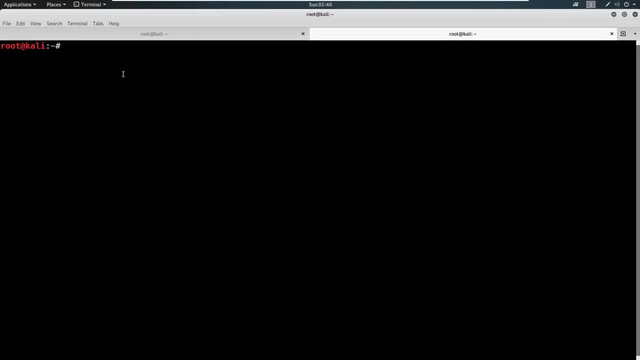 version information. That's great. We're going to use a new tool now, So go ahead and go file new tab And I'm going to go ahead and show you a tool called SMB client. Now SMB client is going to attempt to connect to the file share that's out there. Now, if we have the ability to connect to 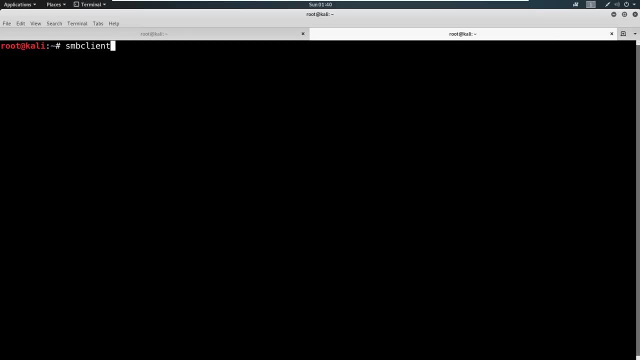 the file share with anonymous access. what that'll do is we can get in there and we could potentially see files. Now, these files might give us an inkling of what's going on the network, or they may even be, you know, valuable to us. they may be something like a backup file, or they might even you knowert an link to an online marketplace- ligo, PX, etc. And we could also put a zing or zine in there. Now, preload is perhaps going to provide us that data in here, but I guess we don't have a pause here. We're doing this because we couldn't find it in quite due to the 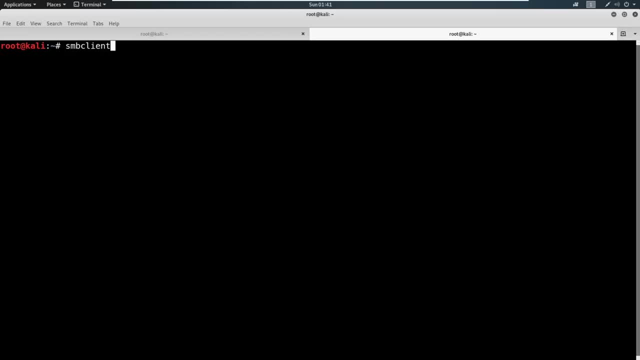 something like a backup file or password stored in a text file. you never know what you're going to find until you actually look. So what I'm going to go ahead and do is do a dash L, and that's going to be to list out the files, And then the syntax looks something like this: you can do two. 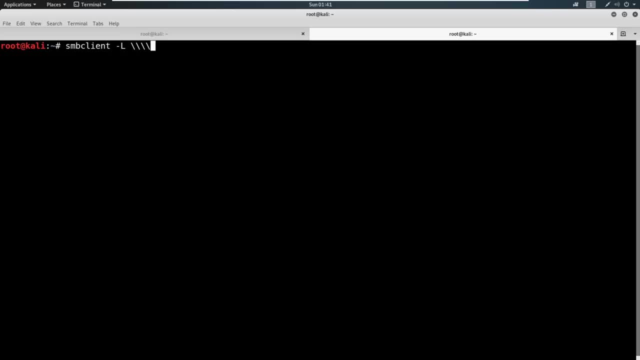 backslashes. I like to do four, it really doesn't matter- And then you just type in the IP address of the machine that you want to try to connect to. So 192, 168, 57, 134 for me, and then two more. 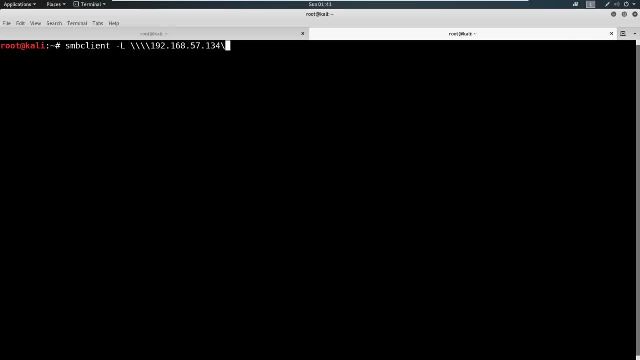 slashes like that. If you're running it with just two slashes, you don't have to put any there. So this is just character escaping because we're in Linux. So go ahead and hit enter And you see that the server does not support extended security. Okay, don't worry about that. anonymous login. 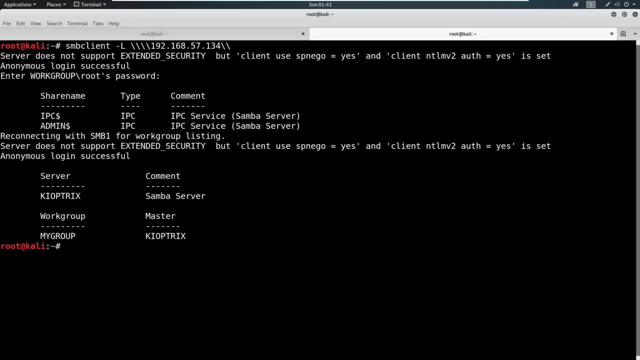 successful. go ahead and hit enter on root password, because we don't know it And you can see that we did list out a file share, So let's go ahead and try to connect a different way. Let's tab up and let's delete this dash L And we see that there's two file shares. 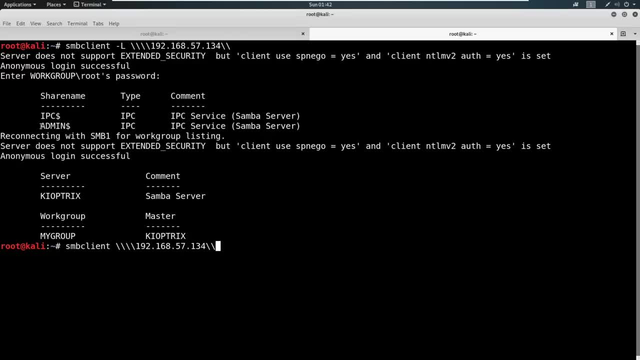 there is an IPC dollar sign and an admin dollar sign. The IPC is not really usually valuable to us, But the admin would be really valuable if we could connect to that. So let's go ahead and just paste that in here And see if we can get that connection. Okay, let's try this. hit enter And you can see we have. 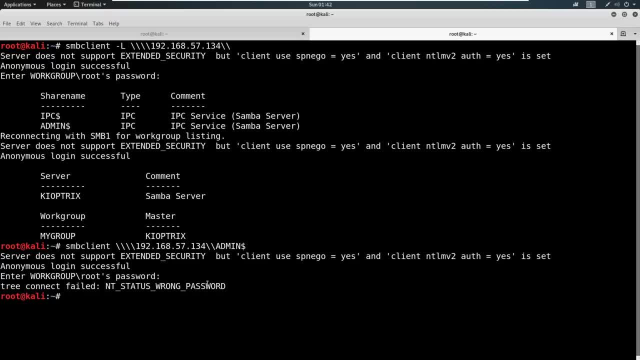 wrong password, So it's not going to let us connect to this share with anonymous access. So that's unfortunate. We could also try proof of concept to see if IPC works. Hit enter on that And you can see. now we're actually in this And this is interesting, So we could say help to see. 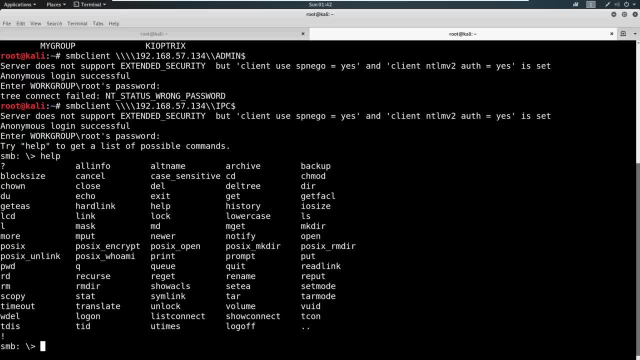 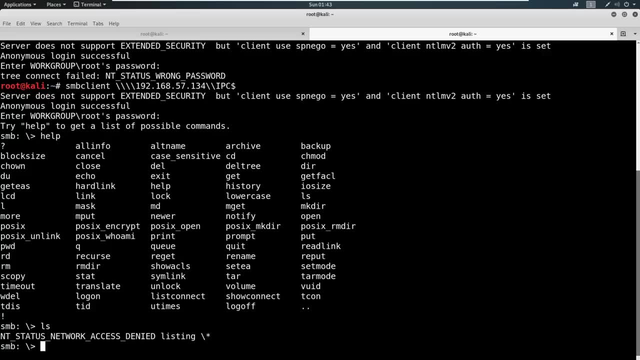 the list of commands, And it's very similar to being inside of a Linux server. So let's go ahead and click on the next machine. Now we can do something like LS to list the files, And we're actually access denied here. So this is what we call a dead end. We can't really access this. So 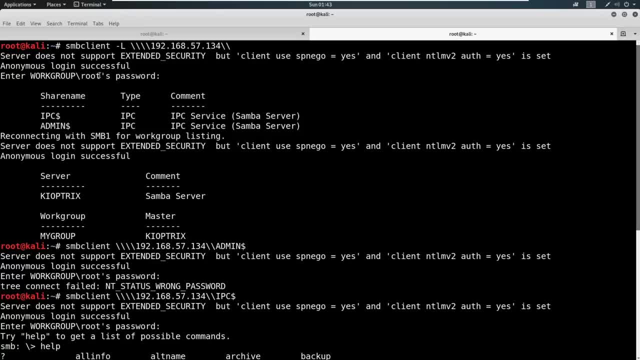 we don't have any information extra gathered. we're going to come back to this time and time again with SMB client. this isn't the last time you're going to see it in the course, But I want you to know that it exists in the reason behind what we're doing here, And this is some of where the 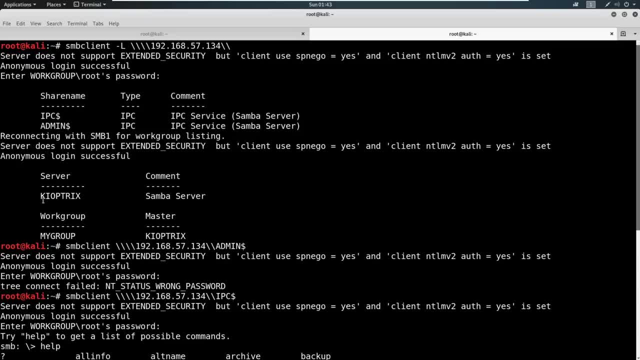 information is coming from. in our scan We're trying to connect out. we see the server names. there's a comment that it's a Samba server And we're going to try to come in here and connect to a file and maybe get lucky. But this time we didn't get lucky, So we're just going to go ahead. 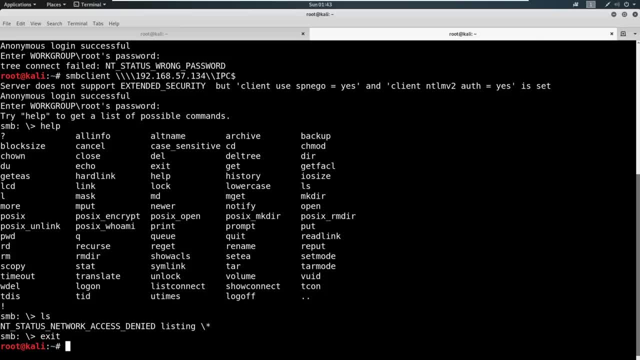 and exit out. So that's all you need to know right now for SMB. SMB is an amazing protocol. When I see SMB I get very happy, But we're going to focus on that very heavily when we get into the internal part, the Active Directory portion, of this course, because that's when things get really difficult. 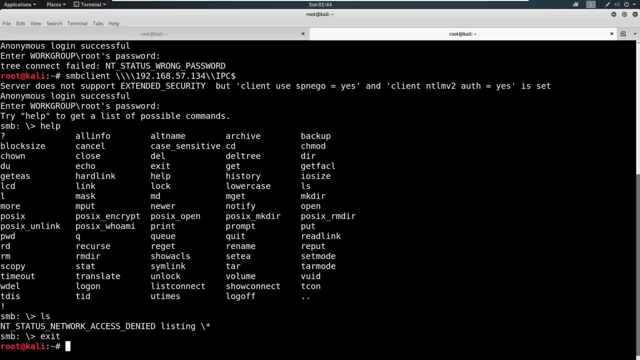 Right now we're just going to do: keep it simple, stupid. on a lot of this stuff it might feel really easy or very, very straightforward, depending, But I promise this is just going to keep building, and building, and building until we have a pretty big understanding on this And 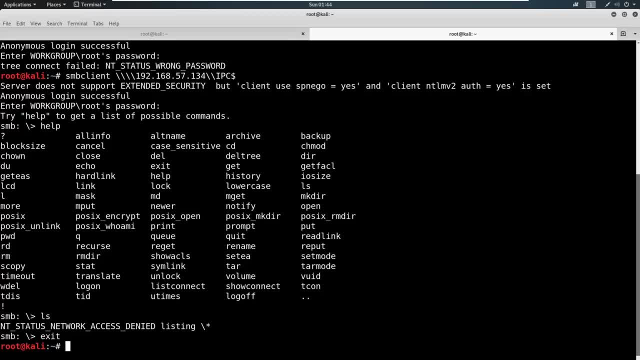 there's going to be a lot of repetition and a lot of practice, And I think that's the best way to learn. So from here I'm going to do a brief enumeration on SSH- how we can do enumeration with SSH- And then we're going to talk other items of enumeration and 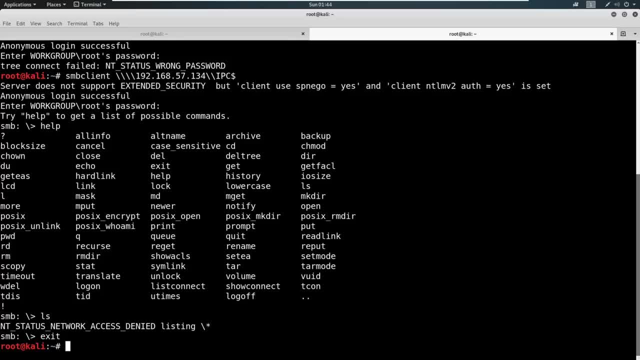 talk research, what are we doing? we've been collecting all this information and putting it into a text document and you're probably like: so what? what can we do with it? And that's where things get exciting And that's how we start to lead into exploitation. But we got to do a little. 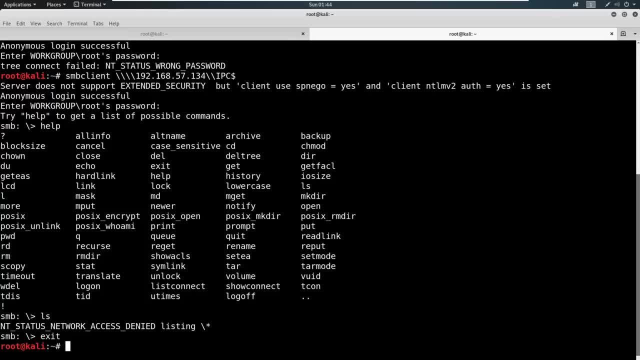 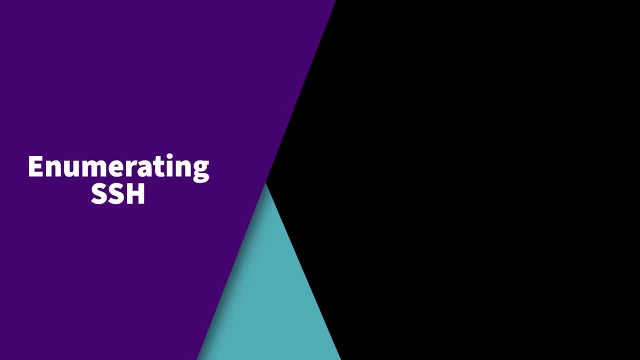 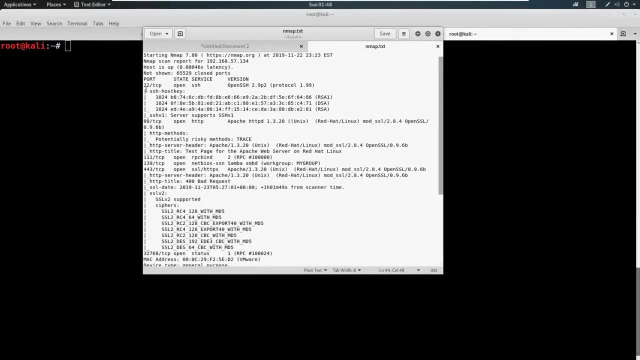 bit more research first before we can get there. So that's it for this video. I'll catch you over in the next video when we are enumerating SSH. So now let's take a look at SSH. So from the original scan we saw that it was open and we saw open SSH 2.9 P two. So we're going to. 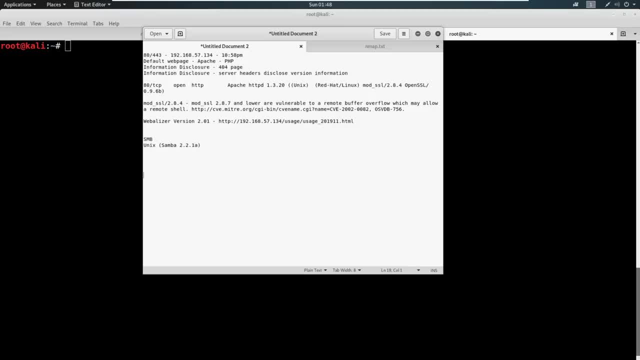 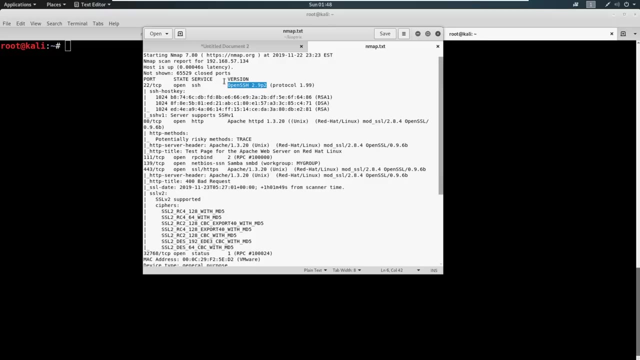 copy this and just make a note of that in our notes as well. I think that's important. So we'll just say SSH, we've got the version there. So let's take this and let's do a little bit of enumeration and talk through it. So sometimes you're going to get a scan back and your scans. 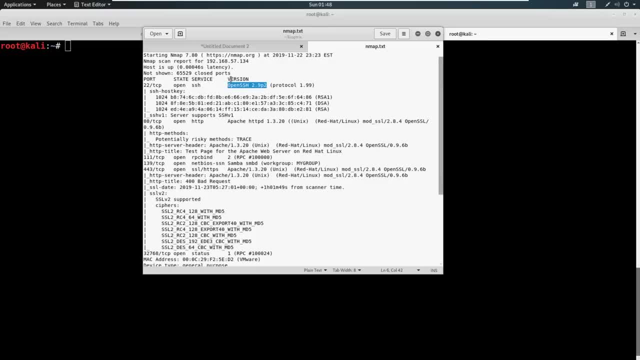 not going to have really a version here. it's just going to say SSH And we can go and try to find that out ourselves And it's always good to attempt that. what we're going to do is we're going to attempt to connect to SSH to this specific port. 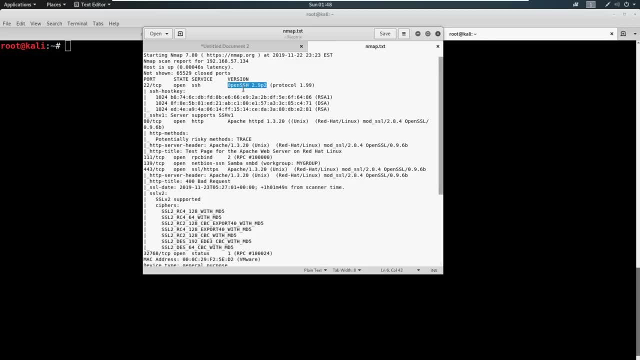 and see if it gives us any information about what's running. And that's really it At this point. it's that's most of the enumeration- that we can do anything with SSH. the second that we attempt to make a login attempt is going to be exploitation, Even if we just try. 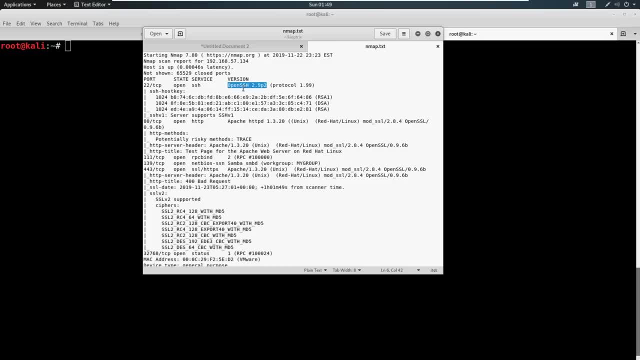 one password. guess that's exploitation. So we're not going to do that right now. we're going to save that for the exploitation part of the course. But I do want to show you a connection and just something funky with this anyway. So let's go ahead and just go to our 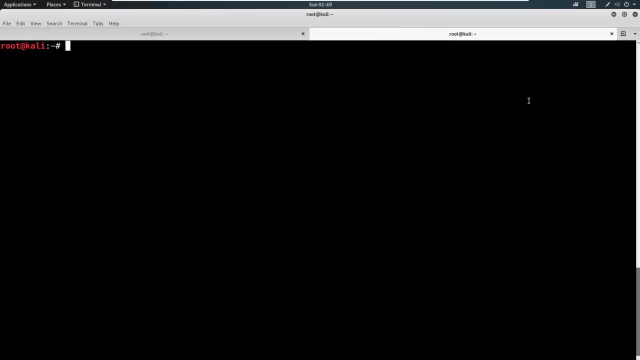 terminal And the typical way to SSH- if you've never done it before- is you just say SSH and I want to SSH to a specific IP address. So this is the IP address I want to. I want to SSH to the IP address And what we're going to do with this box is: this box is old, So when we go to try to 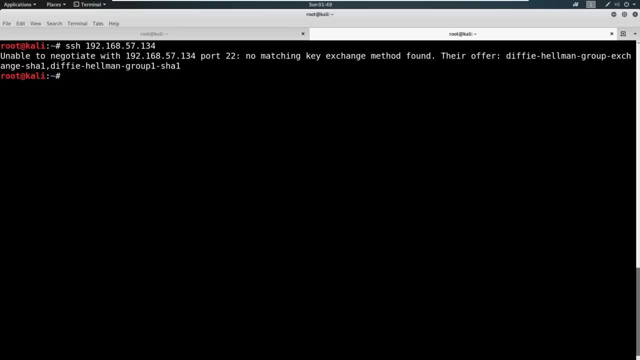 SSH to it. it's going to say this: hey, we haven't found a matching key exchange, So they they're giving us a few different offers here. we're going to have to type in a little bit of syntax. this is not common, But this is also useful to have in your notes, because this does come up. 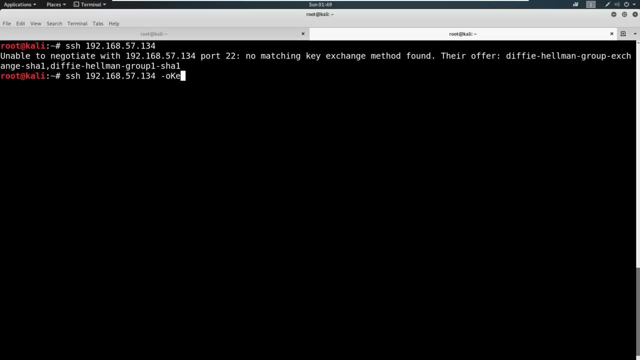 occasionally. So we can just say a dash O and we're going to type ke X like this, and then algorithms plus sign, And I'll stall for just a second so you can catch up, And then I'm going to copy this: 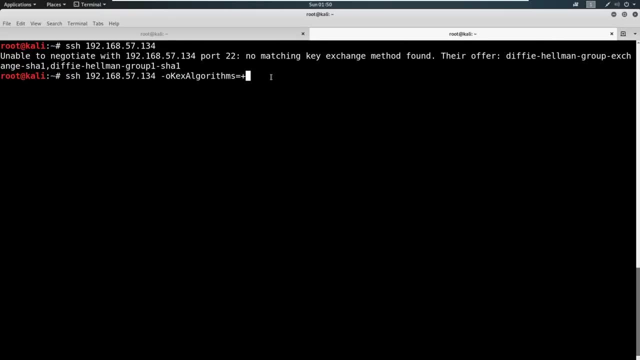 one here And then I'm going to paste it And you're going to see, we're going to get one more error And this is going to ask about a cipher. So it says there's no cipher found. we're going to do a dash C for cipher, We're just going to copy this And we're going to paste it And this should. 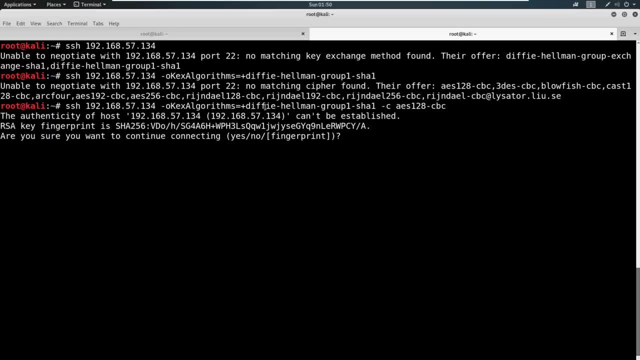 now provide the opportunity to paste it, And this should now provide the opportunity to paste it. to connect says the authenticity can't be established. We've got an RSA fingerprint. do you want to connect? we're going to type in Yes, Okay, and what's happening here is asking us for a. 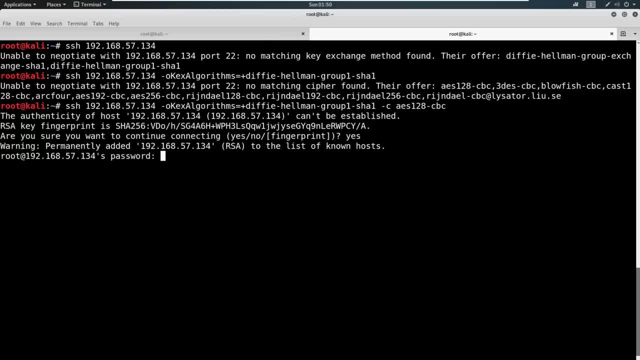 password. There's nothing here for us, So I'm going to hit Ctrl C. Why did we do this? Why do we even attempt to make this connection? Well, sometimes what happens is a banner is exposed and the banner will say: 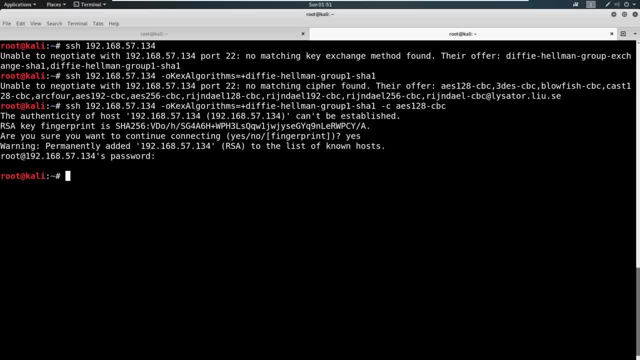 Hey, we're running. we're running SSH version x, y, z, And this is built by this person, by this company, etc. So here we're looking for a banner. Unfortunately there was no banner, So that doesn't. 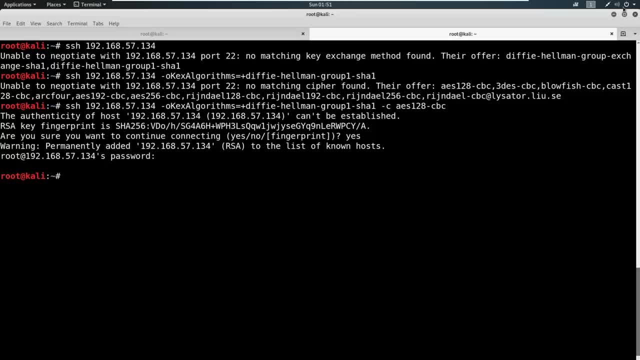 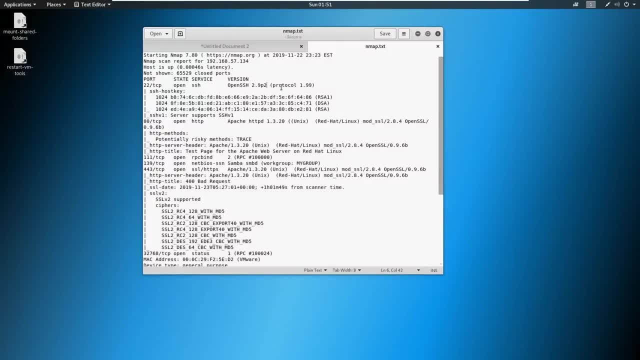 give us a lot of information. But fortunately for us, when we had our, our scan here, we were able to pull down at least the open SSH 2.9 P two. So that's it, And I told you in the beginning. 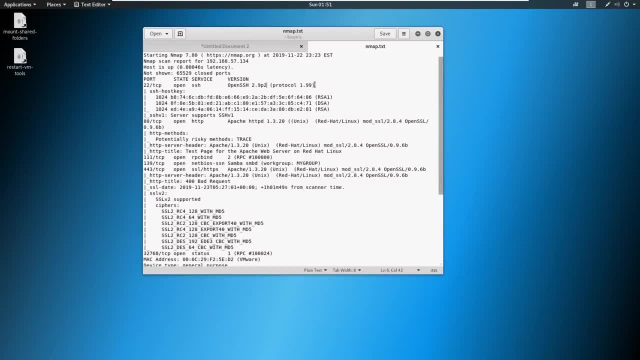 SSH isn't very exciting because there's not a lot of opportunities for, like, remote code execution. Really, the way we're going to have to do this is hammer it with brute force, And we'll talk about the reasonings why later. but we'll have to hammer with brute force and just pray. 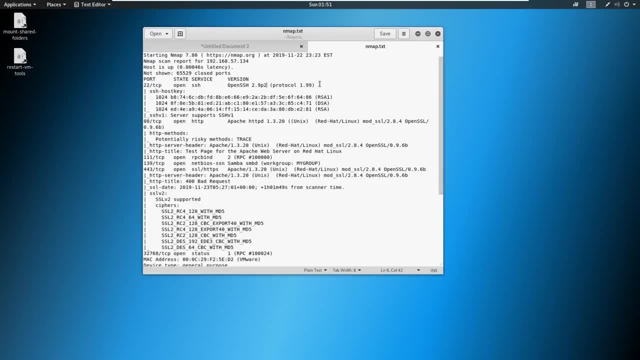 spray and pray, as we like to call it sometimes. But for now that's it for SSH. So we're gonna start moving into research- different tools we can use to research vulnerabilities and additional videos on that. So I'll catch you over in the next video when we start digging into some of what we 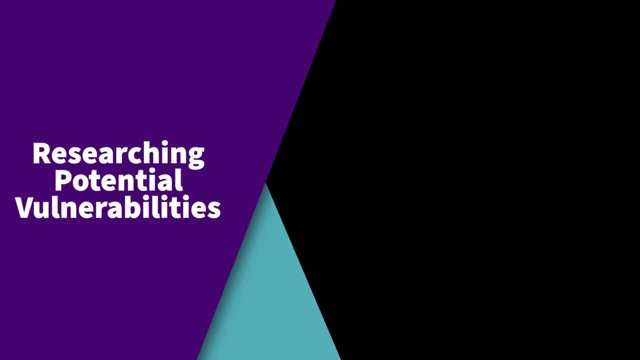 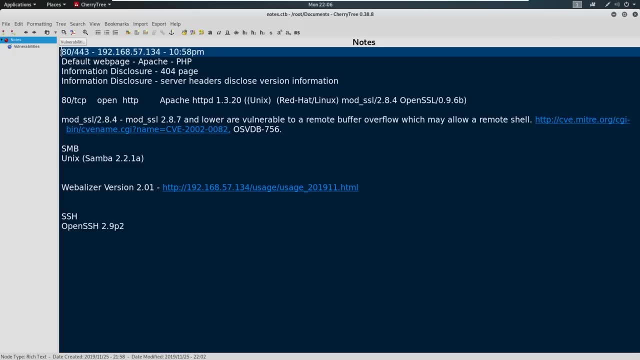 found. Let's talk now about identifying and researching potential vulnerabilities. So we have our notes here And all I've done is moved them off of notepad and into cherry tree, Because cherry tree is a bit more visual and bigger font for us on video, And I made two nodes. 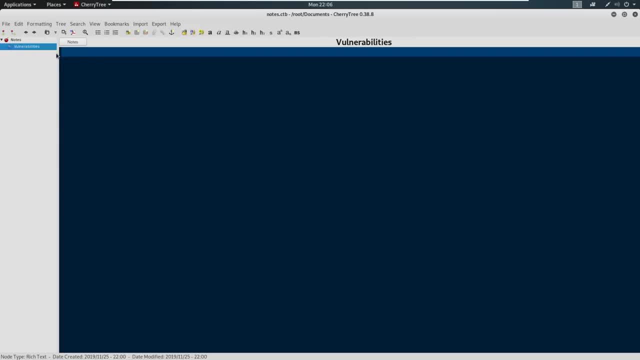 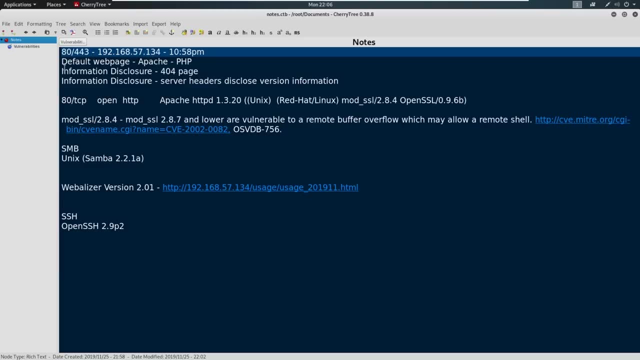 I made the main node here notes, and then I made a child node here of vulnerabilities. So if we recall from our notes we have 80 and 4043 and we've identified some findings that we're going to write up on a pen test report And those findings are, you know, a 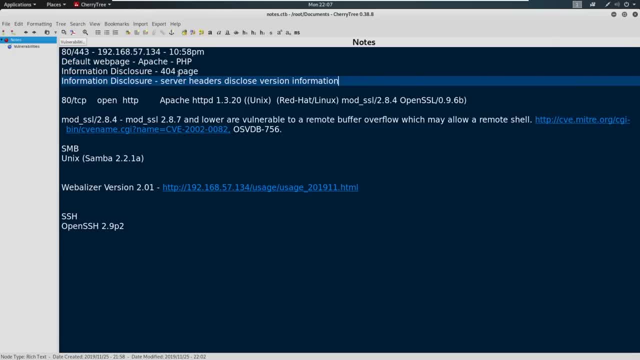 default web page, 404 page was giving a little bit of information disclosure and the server headers were disclosing some information as well. On top of that, we've identified some information that we need for research. Now we've got 80 here and on port 80 we've got this Apache, this mod SSL and this open SSL that we could. 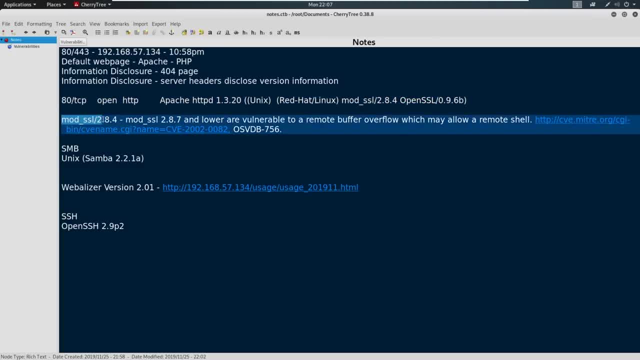 research And when we ran our NICTO scan, we identified something potentially juicy here. where mod SSL 2.8.4 falls in line with this, which is 2.8, and 7 or lower, which we are, are vulnerable to a remote buffer overflow, which may allow. a remote shell, Remote buffer overflow, meaning that we are, don't have to be local, we can be remote, which we are, and we can be remote which we are, and we can gain access via a remote shell, meaning we can gain access to that. 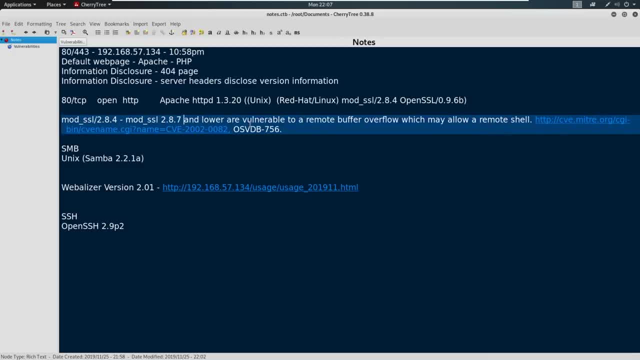 machine. So that's good, that's really good. The other one here we see is SMB, and we identified SAMBA version 2.2.1a. We also identified a web analyzer, version 2.01, and we've identified open SSH 2.9 p2.. So 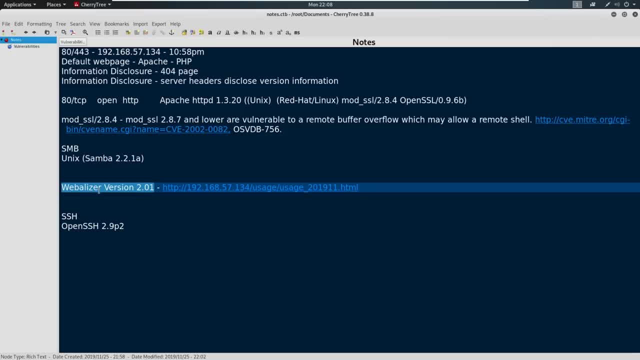 for this video. we're going to target the low hanging fruit and I put this in order of how I would attack it. And again, I always think 80, 443, and 139, 445 are the juiciest to me. This web analyzer might be juicy. 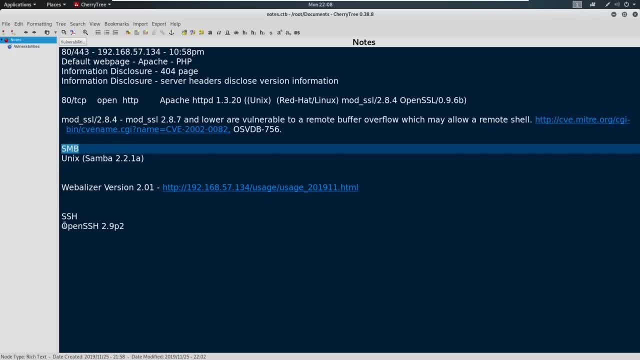 open SSH? probably not that juicy. So we're gonna do is I'm going to go ahead and research 80 and 443, and then we'll research the SMB as well, and then I'll leave you to do a little digging on these, just as practice and we can see. 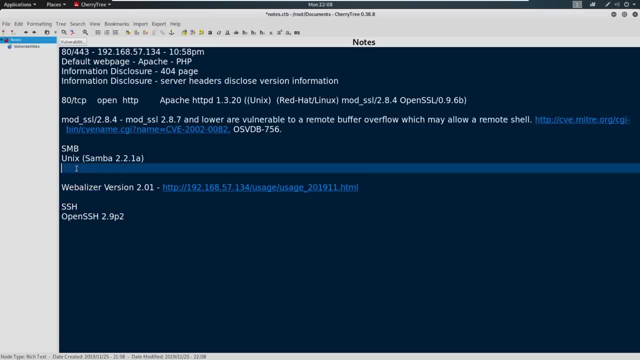 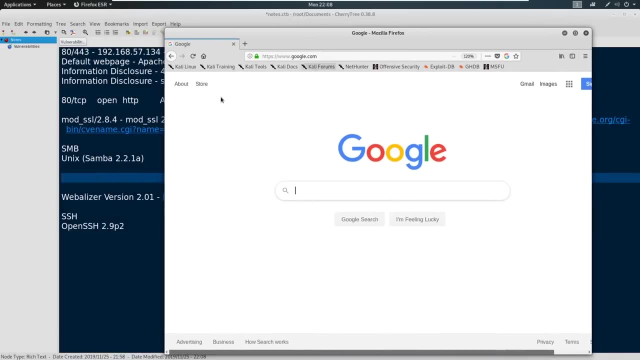 where we go. So from here we're just gonna go out and let's say we want a open up Firefox, and we'll go out to Google and on Google we can pick and choose which one we want to research here. now this mod, SSL 2.8.4, is probably. 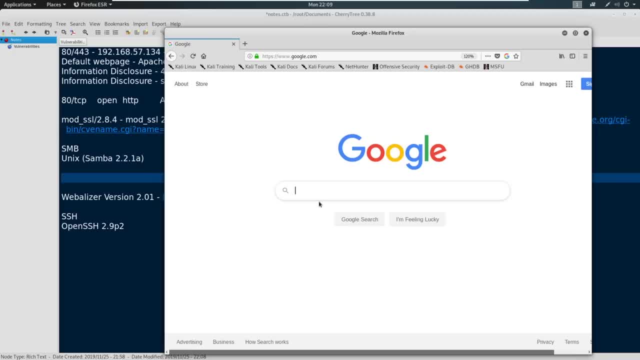 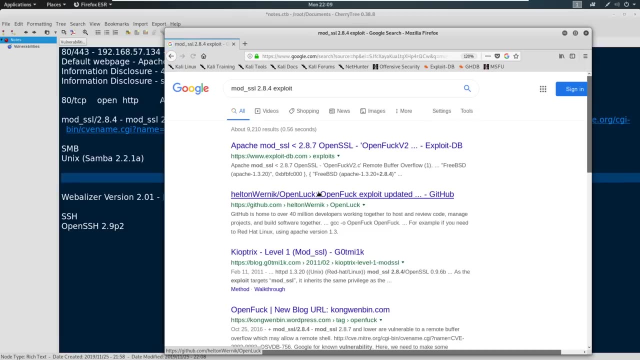 the juiciest of the items and we might want to start there. so let's just say something like: mod SSL 2.8.4. you see the 2.8.7 exploit showing up. by the way, we'll just do 2.8.4 exploit and we'll see what comes up now. 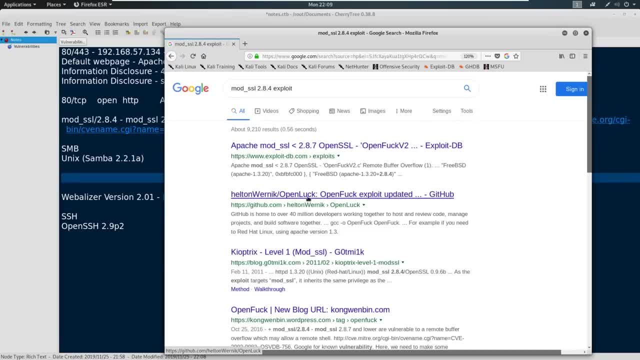 naughty words, naughty words. we'll just call it open luck. okay, and you can see, don't cheat. Keoptrix is coming up as well, but we're gonna go ahead and just open this, open this Apache mod, and then we're gonna also open this github one. 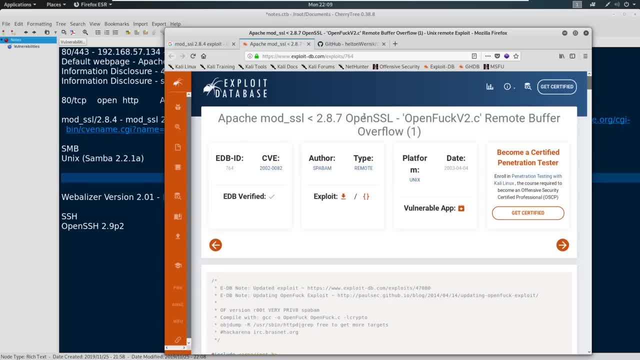 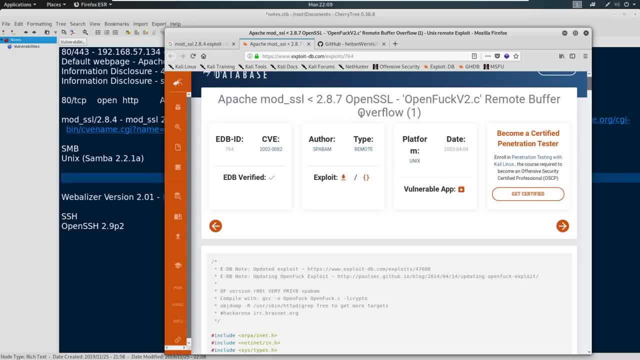 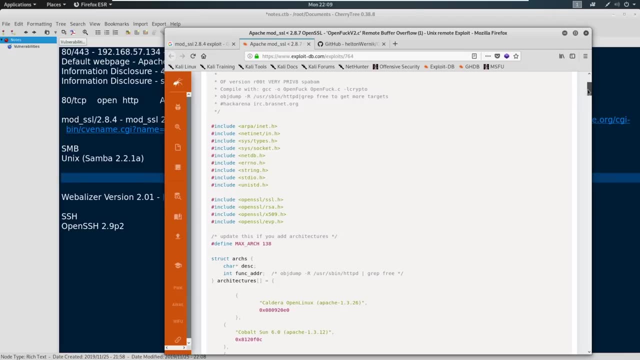 and I'll cheat a little bit and tell you why here in a minute. so Apache mod SSL 2.8.7, less than 2.8.7. scroll through here and it just has the code for us. now this is where you have a chance to come through and read the code. 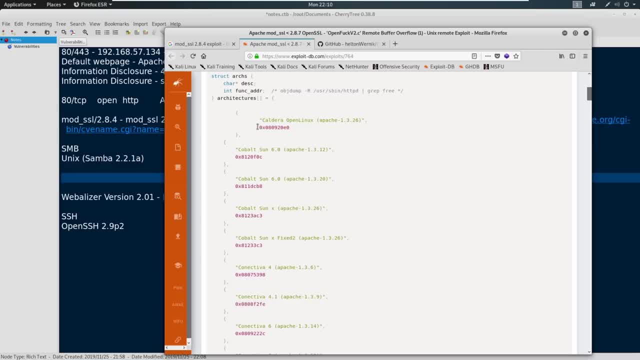 now it looks like to me that they're just identifying. if you've never seen a buffer overflow, which you probably haven't, there will be one later in the course. it's identifying where it's going to have the architecture right, so the architecture has its own identifier. so 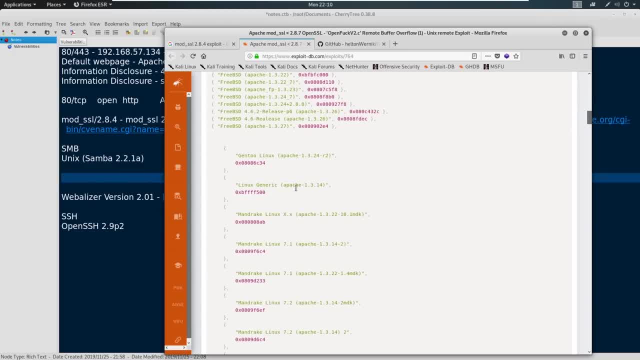 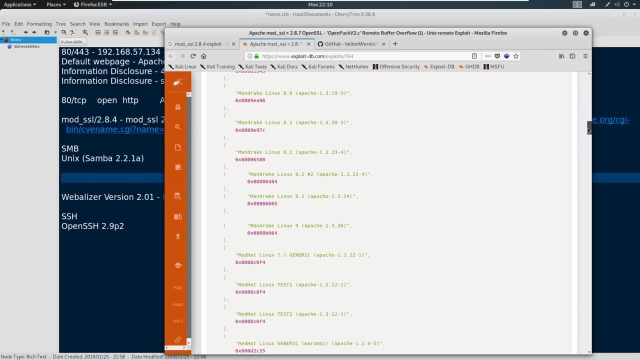 depending on which. it looks like this works for quite a bit of different architectures of Linux. depending on which Linux you're running, is this return address here? so that's all this is doing, and then there's going to be code down here, I'm guessing, for an overflow which you see a bunch of A's as you're gonna. 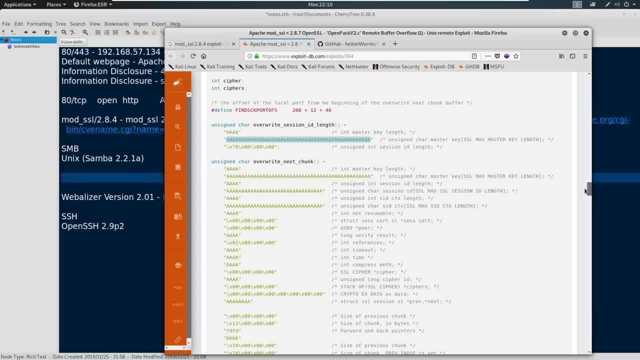 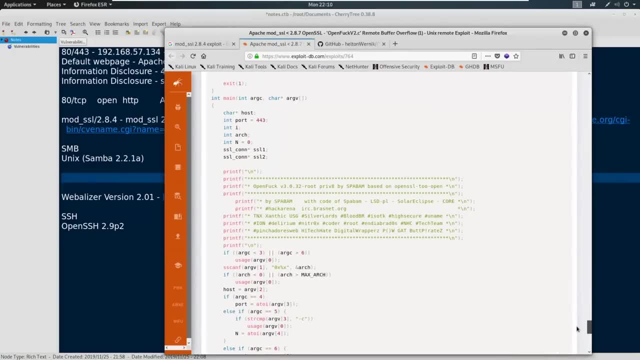 see later in the course. this is just overflows, so you'll learn to read this over time again. like you do not have to code this, you do not have to be, you know, you don't have to be super good developer, but just understanding kind of what's going on and making sure that you know the code that you download is safe. 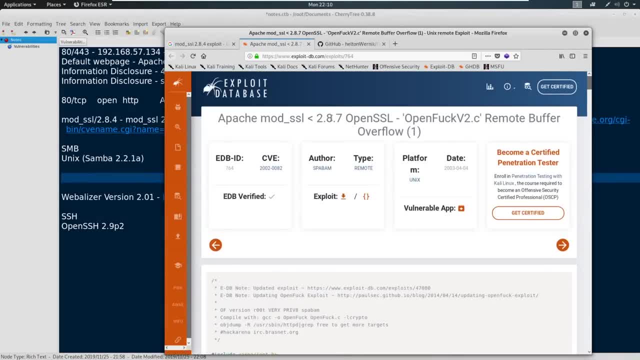 on your computer and it's good to go. now this is coming off exploit database, so you can- I wouldn't say- assume, but you can trust it for the most part- that this is safe code. you have the option here to download the exploit and you actually have the option to download the vulnerable app as well, if you ever want. 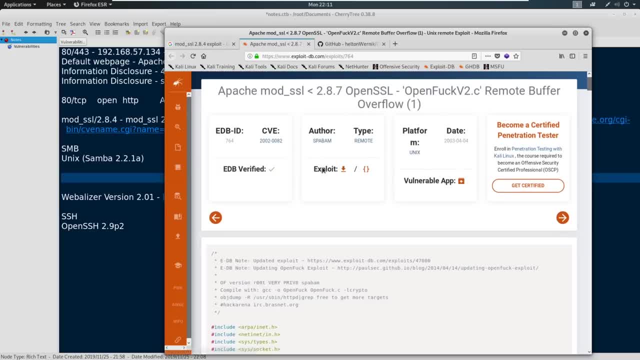 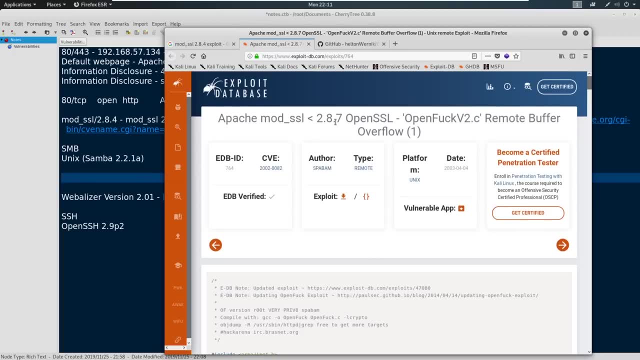 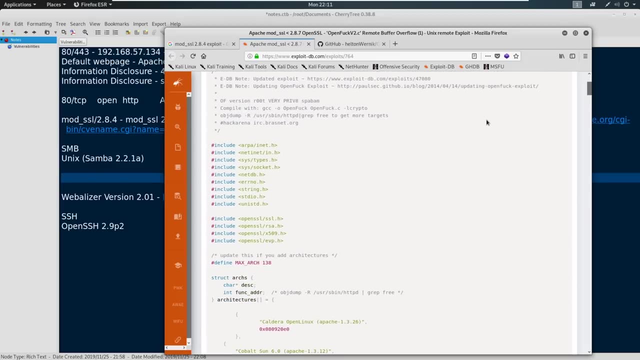 to build out a machine and play on your own. so we have a little bit information here that it just says: hey, you know, this is a less than 2.8.7 open SSL and we've got a remote buffer flow. there's nothing else here, but that's okay, that's you know, this might be good for us. this is something that 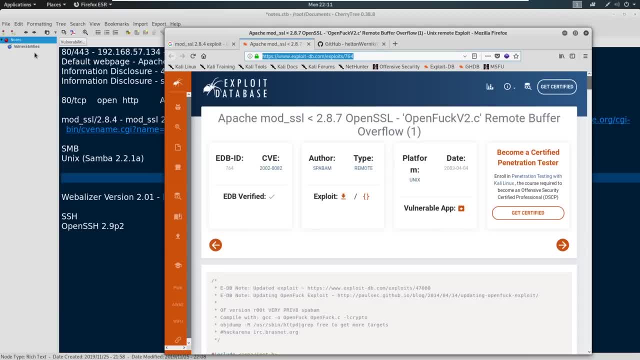 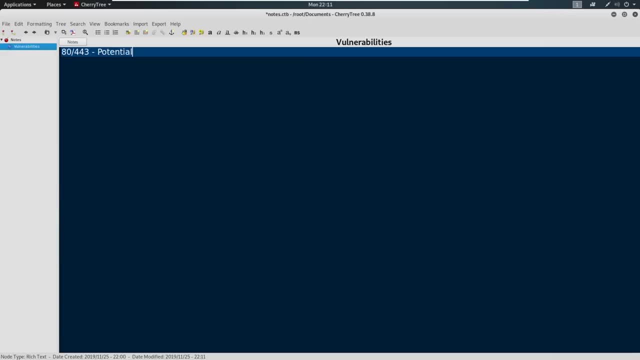 we need to note, so we can copy this and I would put it here and we could just say something like 80 443 potentially vulnerable to. we'll call it open luck, and then we'll just put it here and we'll also: we should also save this open luck and I'll cheat a little bit and tell you: 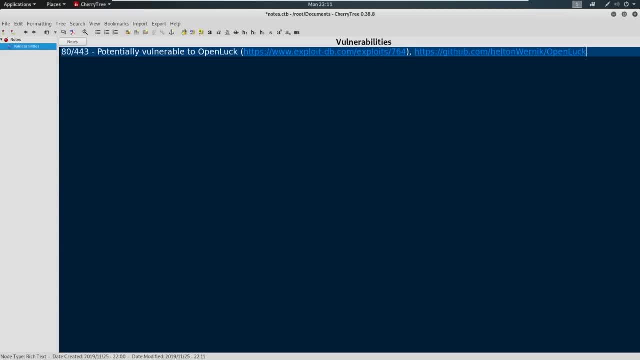 guys, why is? because this open the, the exploit database one, without saying bad words, is not going to allow us to work. it's not going to work. the the exploits a little dated and that's why there is a GitHub one out there that actually does work, so we're going to utilize the GitHub one. 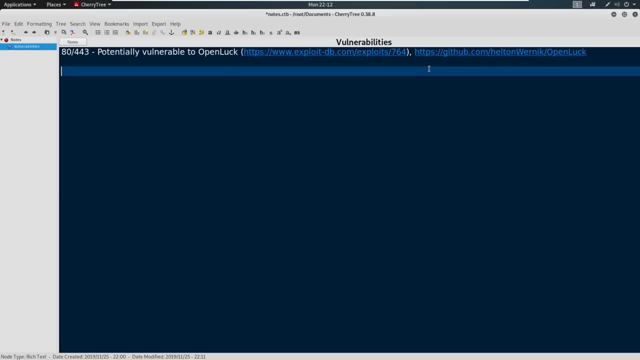 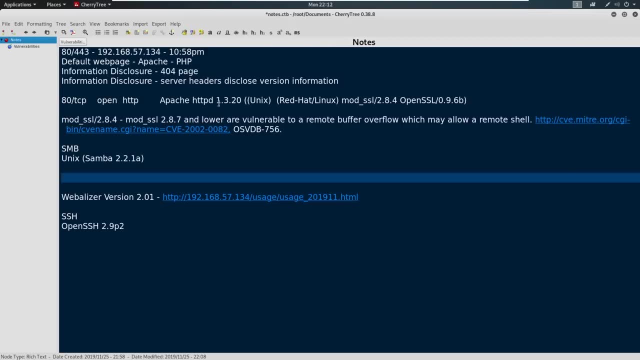 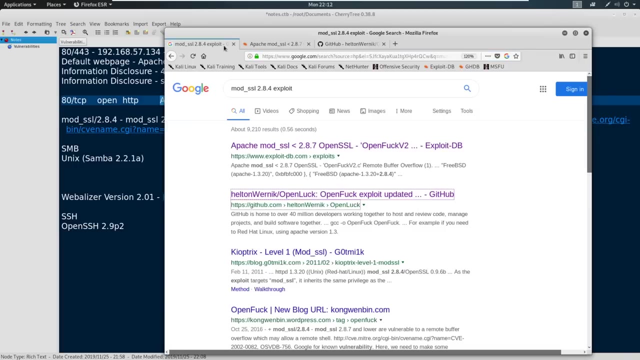 instead, when we do get to the exploitation section. so a little bit of a hint, a little bit of a foreshadowing, we are going to utilize this exploit so we could also go in and research. we could say: Apache, httpd 1.3.20, copy that and come to Google and just say, hey, I wonder if 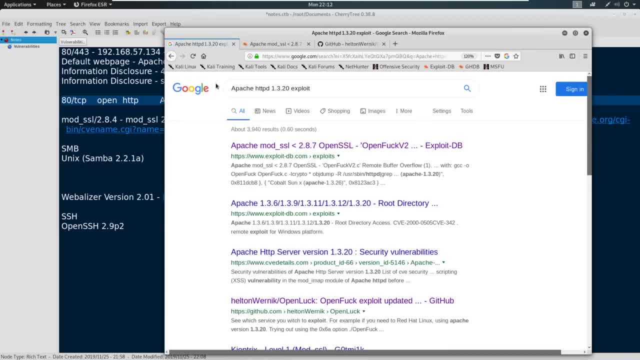 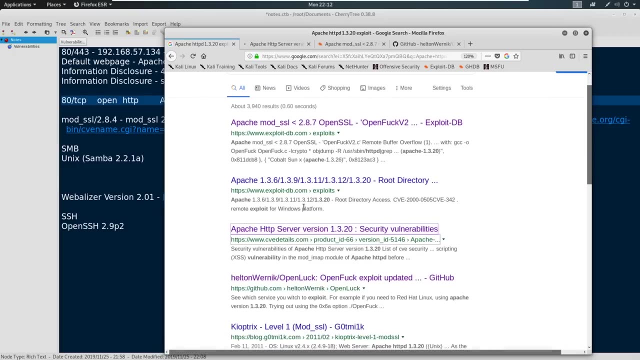 there's an exploit for that and you would just search something like this and you can see in here: Apache 1.3.20 is actually showing up in this vulnerability as well, so that's good. and then sometimes we see these websites like this: CVE details. these are okay to look at, uh. 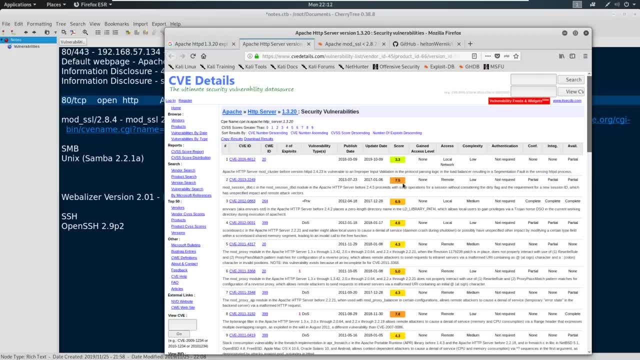 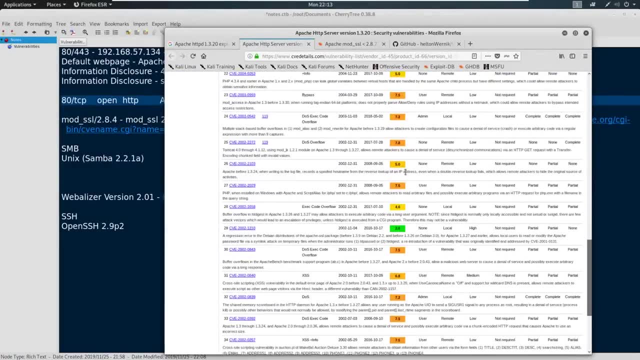 they're, they're all right. like you come in here and what you want to look for is the score, immediately my eyes shift to the score. I don't care about anything else. if I see something that's red, I get excited. um, but we see no red here, so I I don't think that necessarily. this is vulnerable to. 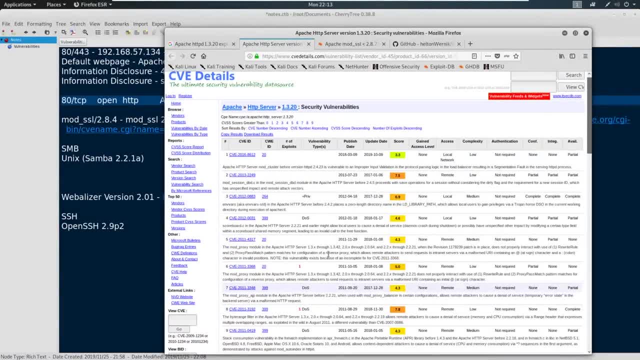 like a remote code execution. it's got a lot of denial-of-service, but I would want to see like a high score, which means a critical. that's what red is, red is critical. So we've got high, moderate and low here, but we don't have a critical one. So this doesn't look. 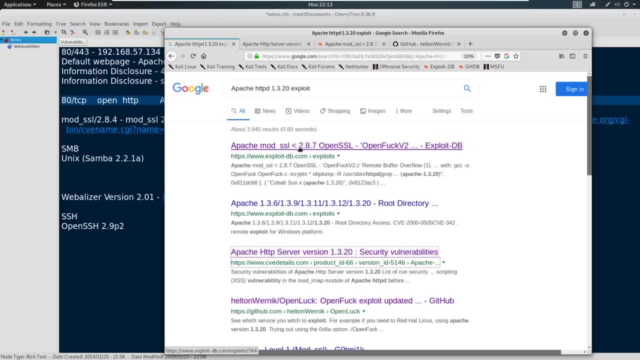 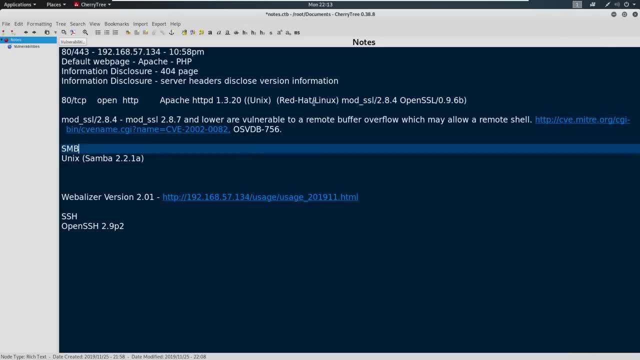 like it really probably has anything, but it is tied to this, which is another wheel spinning indicator here, that, hey, you know what? we probably got an exploit here with this thing, or at least something that we should try, And that open SSL is tied directly to this mod SSL. 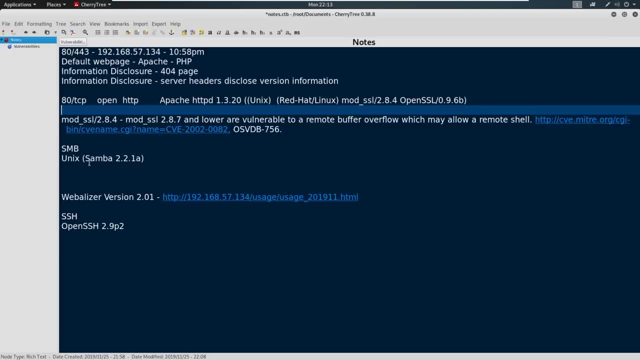 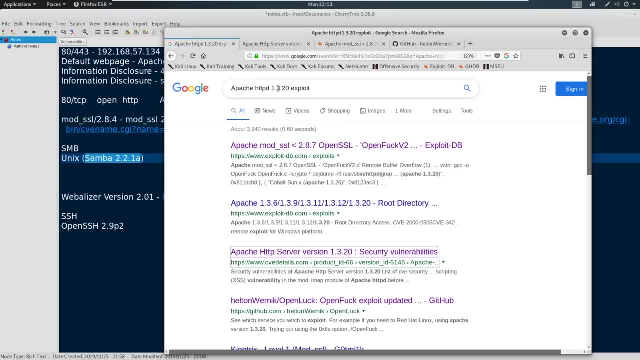 So we don't really have to research it. Now let's move on to Samba here, Samba 2.2.1a. Okay, let's copy this And let's check for an exploit. So just as simple as is doing this. 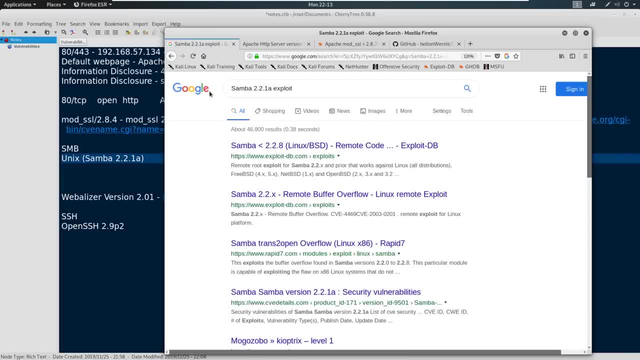 and saying exploit, And we've got a few here. We've got this Samba 2.2.8 remote code execution. We've got Samba 2.2.x remote buffer overflow And we've got one down here which I love to see. this is rapid seven. So let's go to rapid seven first. 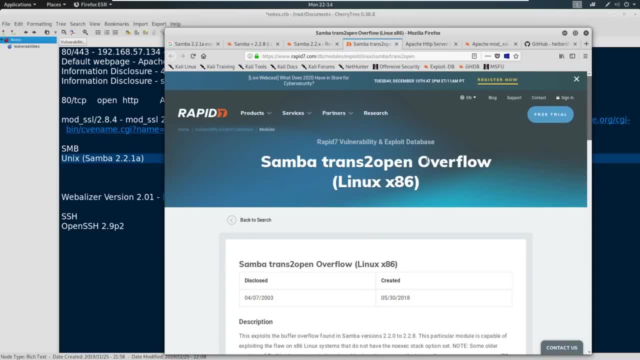 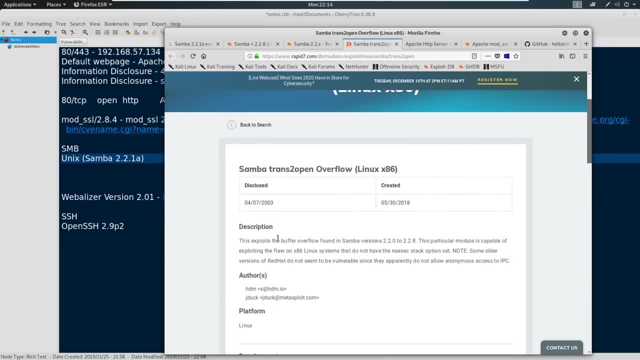 Why do I like this? Why do I like to see rapid seven? Well, rapid seven makes Metasploit, So it looks like this exploit is called Samba trans, to open, And let's read a little bit about the description. So it. 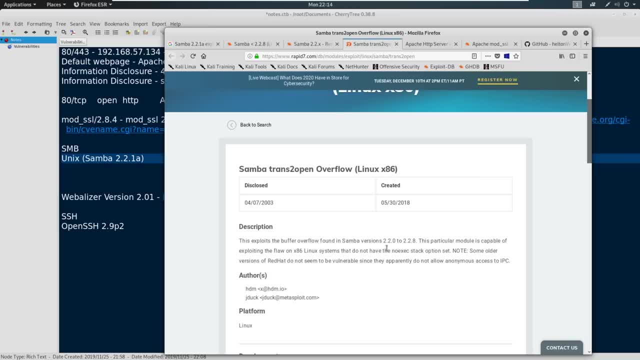 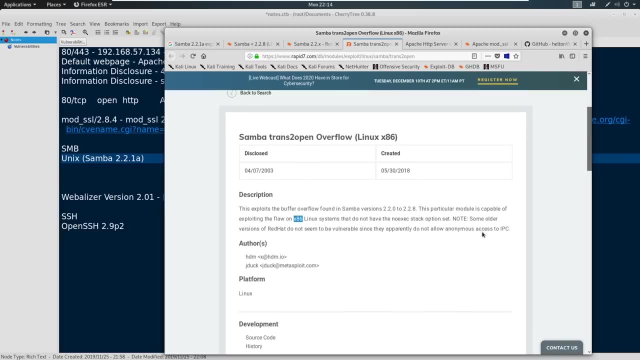 says this exploits the buffer overflow found in Samba versions 2.2.0 to 2.2.8.. That meets our criteria. This particular module is capable of exploiting the flaw in x86 Linux systems that's important to know that do not have the no exec stack option set. Note some older versions of 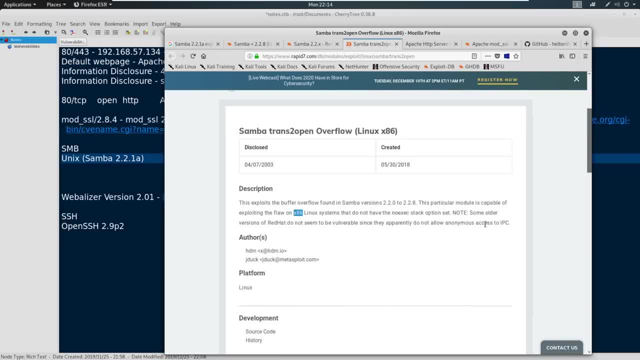 Red Hat do not seem to be vulnerable, since they apparently do not allow anonymous access to IPC. So remember, we did get anonymous access to IPC earlier when we connected to it via via our SMB client. we never got access to admin. we could never do anything in IPC. we tried to say LS. 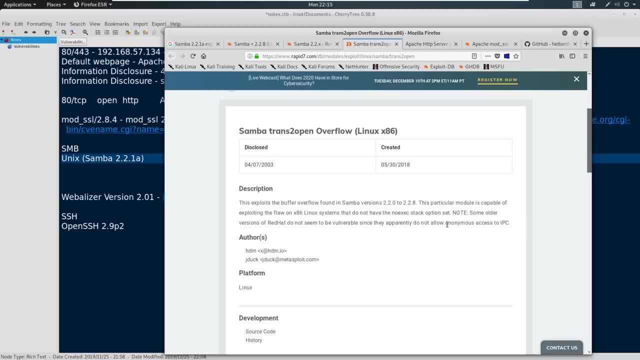 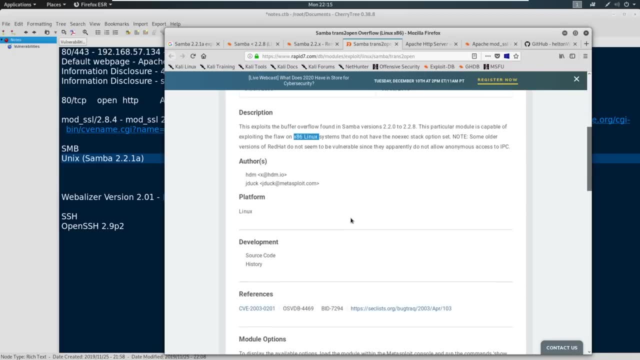 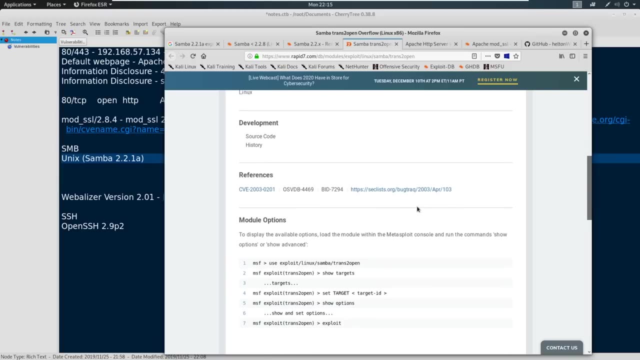 and it said denied, but we still logged in, So we do have anonymous access to IPC. That's interesting, And we are potentially running against an x86 Linux system, So that's interesting as well. We're potentially meeting some of the requirements here. Now, here is where this is great. You scroll. 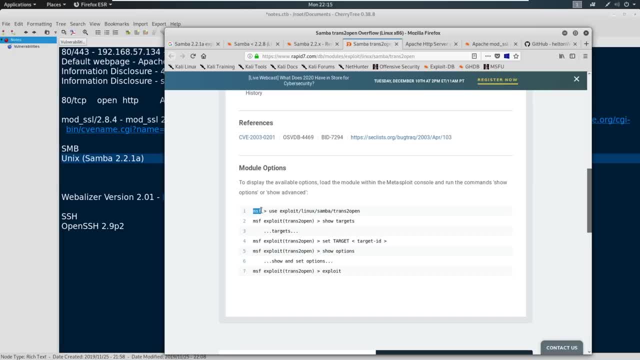 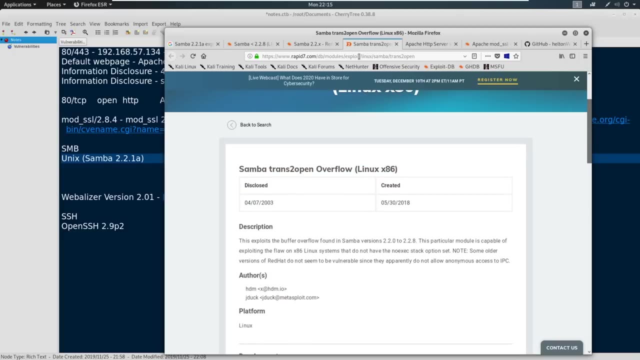 down here and you see module options And look, this is Metasploit. It gives you the module options that says, hey, use, exploit Linux Samba trans to open, And then it tells you, hey, how to do this, And then you're good to go. That's really nice. I really like that. So I'm going to copy this one. 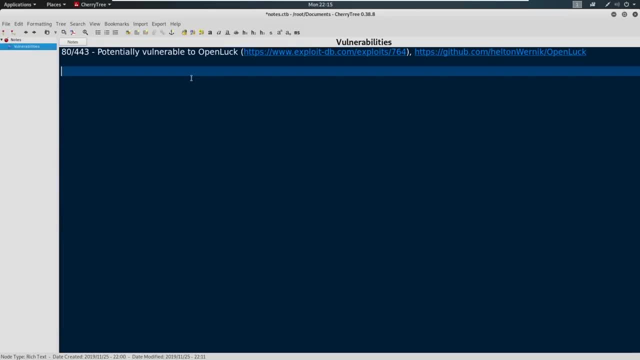 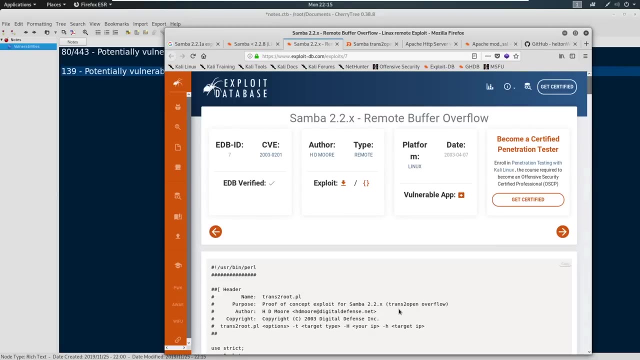 And we'll just come to our notes And we'll say something like 139.. Potentially vulnerable to trans to open, And we'll just paste the link here And we can come read these as well. So this is the trans to open overflow. here This looks like the. 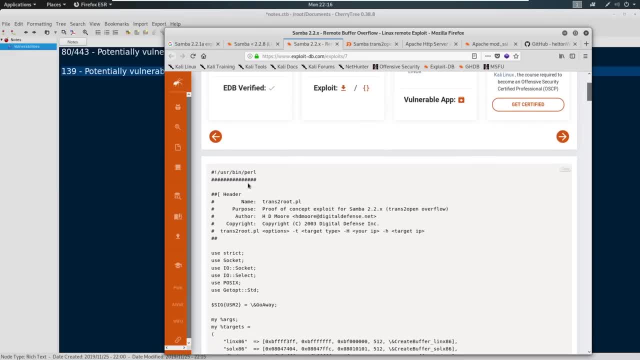 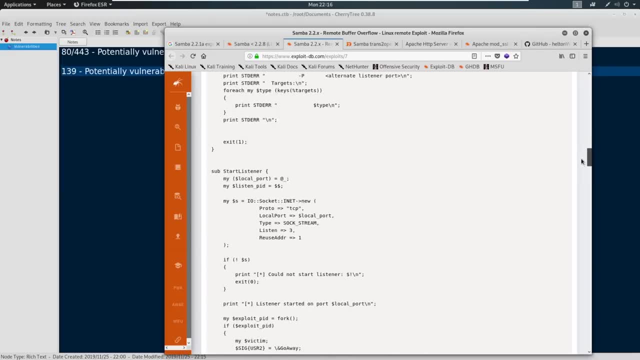 manual version of trans to open overflow. It looks like it is a Perl script And again it looks like an overflow. So you'll learn to read these and see what they look like just over time. But you know, you just want to look at the content And then you can see that it's a trans to open overflow. 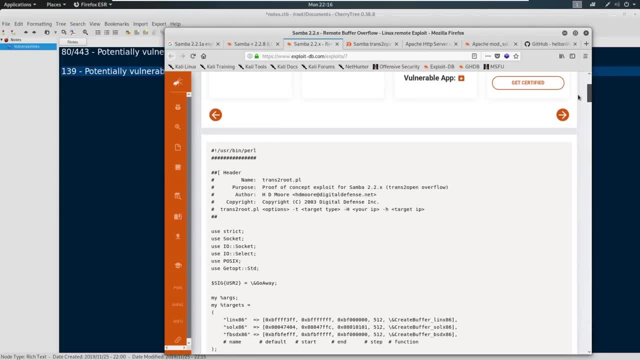 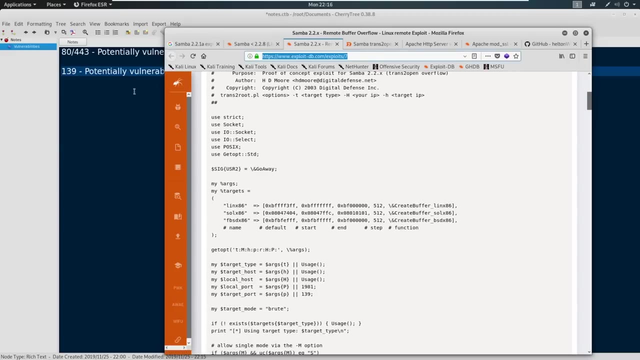 Make sure everything's good to go. You will need to run this with Perl. It gives you the options here: Trans to root Perl, What option to select, What target type to select Your IP address and your target IP address. So we'll save this one as well, Why not? And we'll take a look at the other. 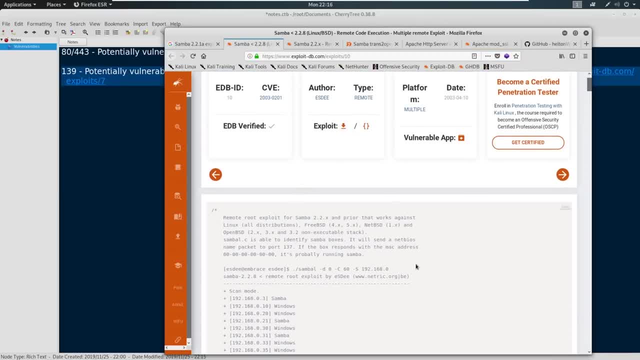 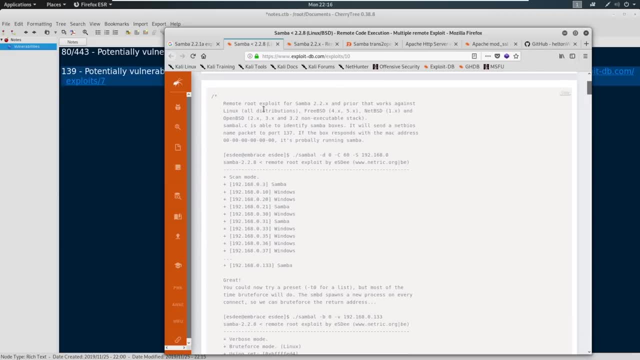 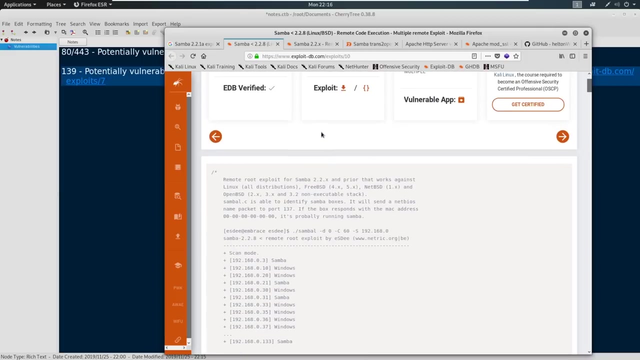 one Just see what it is And It looks like it could work for us remote root exploit for Samba 2.2.x that works against all Linux distributions- Sambac. I think this is a possibility as well. So this is C code here. 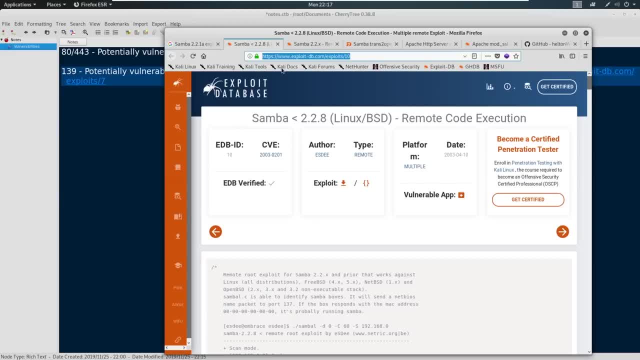 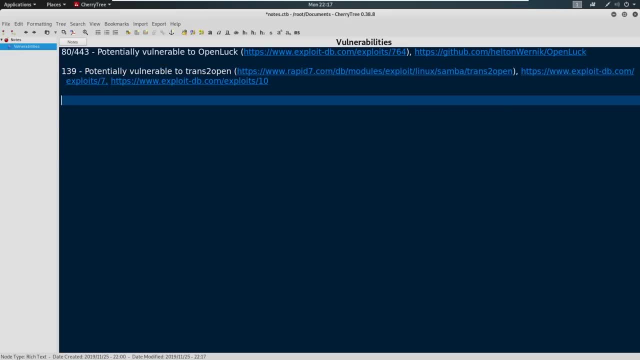 We're going to go ahead and just copy this, and we'll go ahead and add this to our list as well, and we'll figure it out. So all we're doing right now is the research. Okay, so from here, I've showed you the Google way. 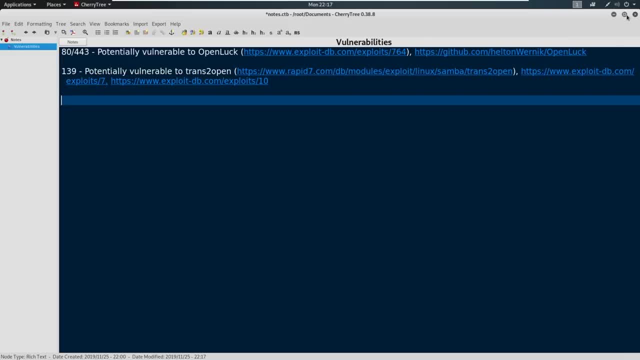 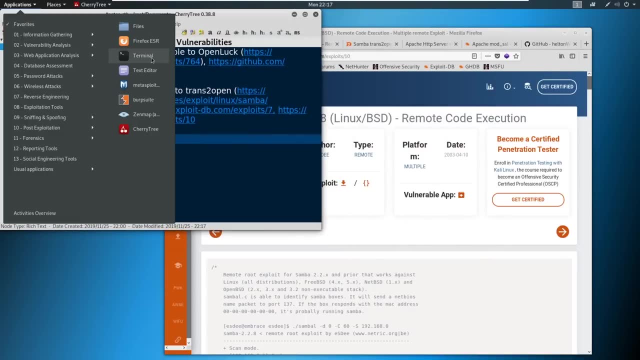 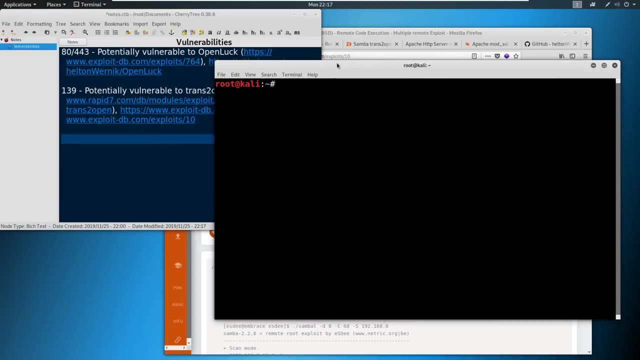 Let's say, for some reason, you want to do this on the fly, you want to use another tool, or you're in a network and the network has no access. you have no internet access out, you have no research capabilities. You can go to the terminal and there's a great way to research this as well. 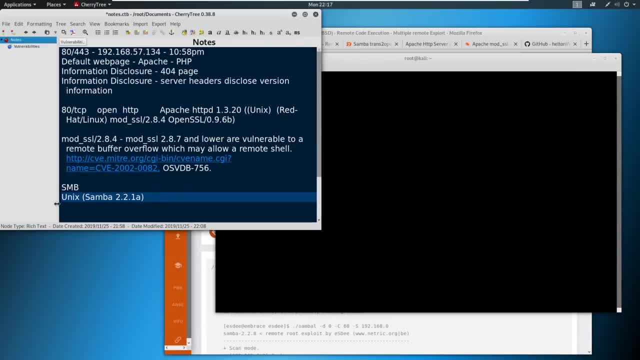 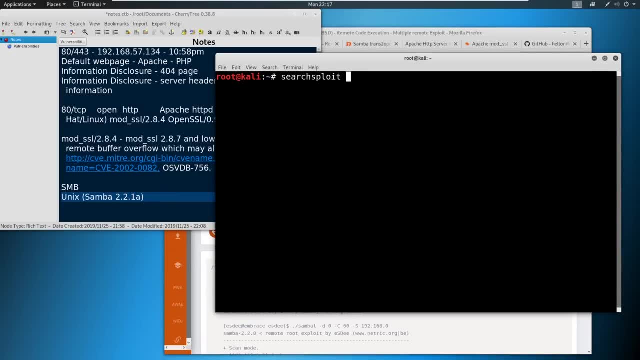 So let's go back up to our notes and take a peek Now. let's take this Unix Samba 2.2.x, Let's take this Samba 2.2.1a, for example, and let's do a tool called SearchSploit. 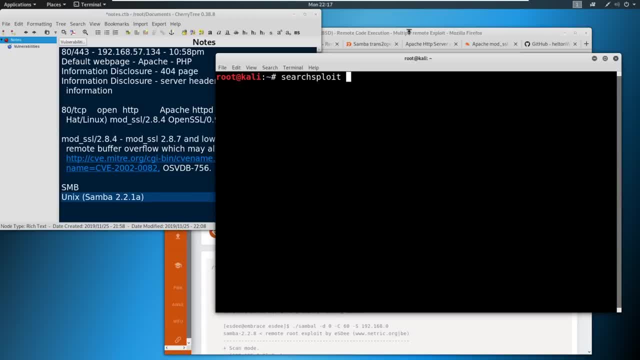 Now SearchSploit is going to search for the exploit database, this whole database here that we're looking through. It's brought down onto your machine. Every time you update your machine and the database updates, it updates down your machine and all those exploits get downloaded for you already. 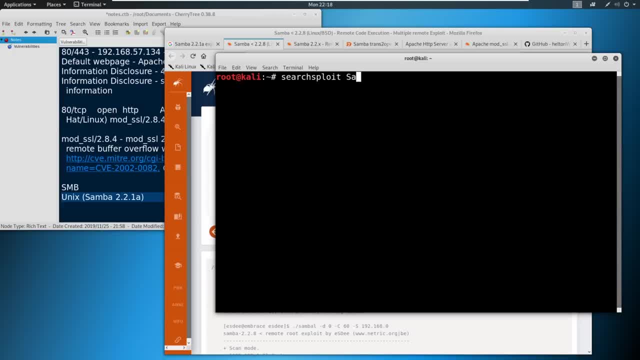 But you could say SearchSploit and maybe we search something like Samba 2.2.1a. Let's see what happens. No result? Well, okay, Why is that? Well, let's delete this Now. you cannot be too specific with SearchSploit. 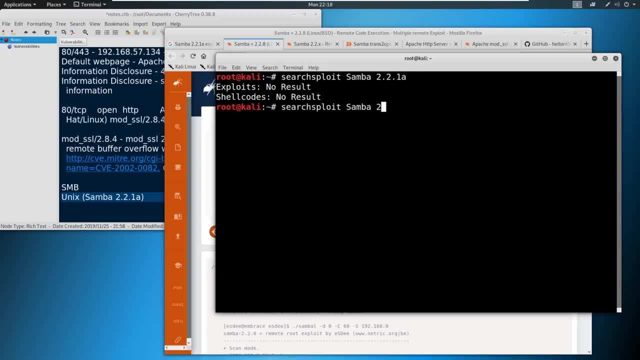 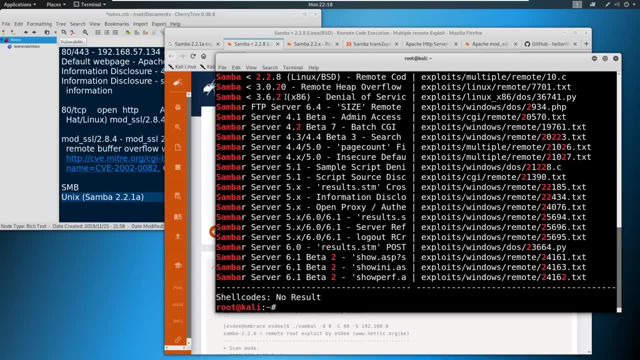 The more specific you are, the worse off you are, because SearchSploit is searching the exact string that you are using. Now you see that we search Samba and it's searching for Samba in a 2.. Okay, now we can start to see some things here. 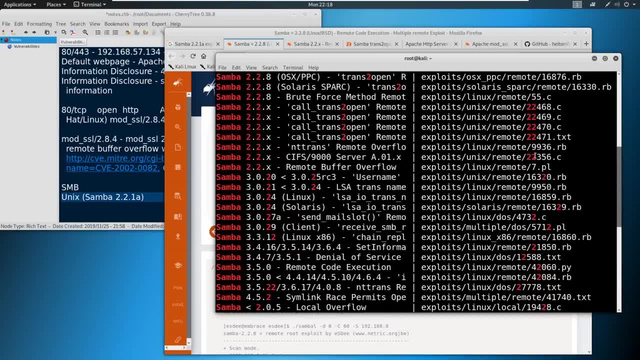 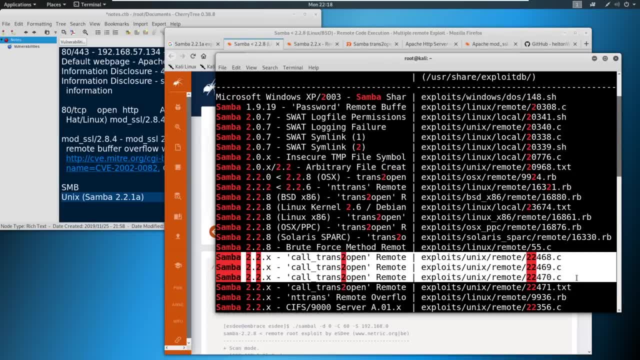 We see a Linux remote code execution right here And we're going to have to look through these Now. it's not pretty right, It's not the prettiest, But you see, the trans2open does show up Now it's not the easiest way. 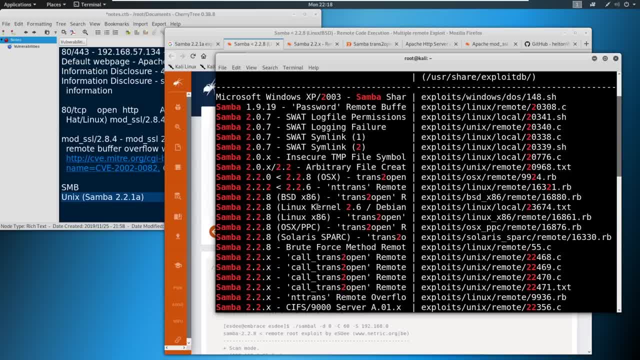 I do prefer Google, But if you're in a pinch or you want to look at all the different possibilities and see maybe- hey, is there a 2.2 in here. So like, look, Samba 2.2.0 to 2.2.8 OSX. 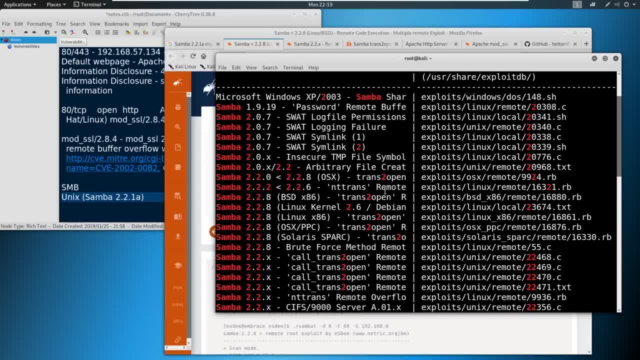 That's not our operating system, but it's called trans2open And we see that over and over and over again. So maybe the It'll spin again and it says, hey, trans2open. I think that that's potentially what we're looking for here. 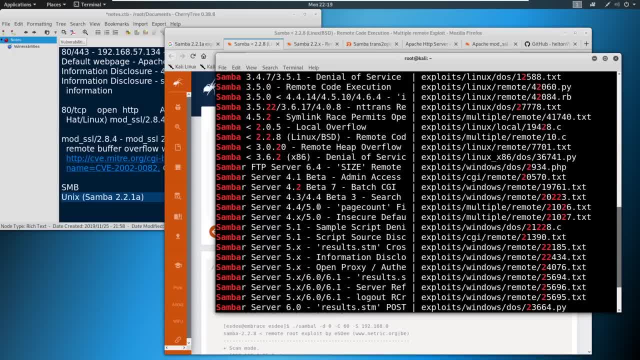 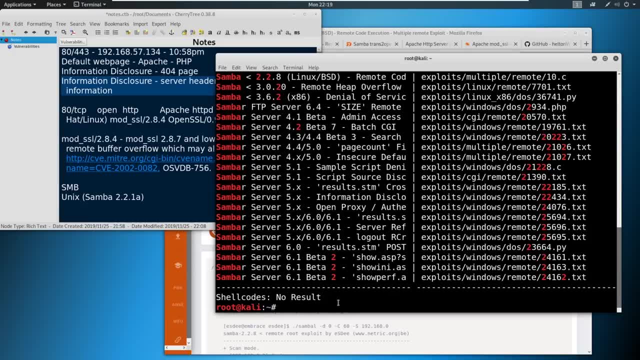 And then, once we get down to the threes, we know: hey, we've gone too far, This is not our version, etc. We could do the same thing with, let's say, the mod SSL, And we can say something like mod SSL2.. 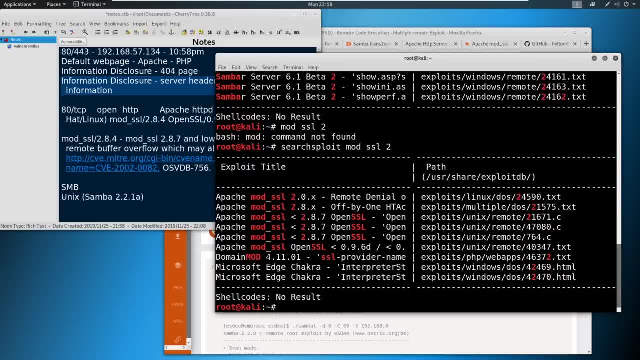 If I type search split in front of it And do some searching there And we can see: okay, there's denial of service Not it. 2.8.x. Potentially right. And then mod SSL 2.8.7.. 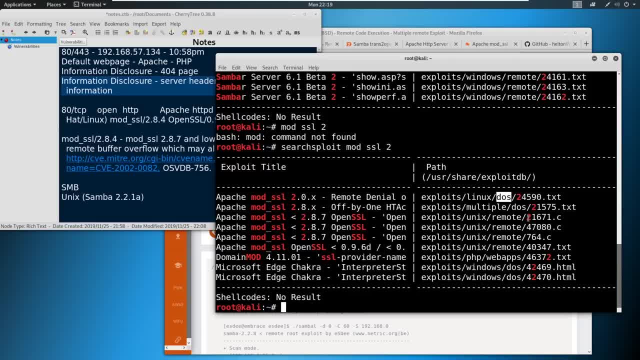 And another thing to look at over here: Denial of service. Denial of service Remote. Remote is huge. Remote means remote code execution. So learning to read these as well: Exploit Check, Unix. Okay, we're running on Linux. 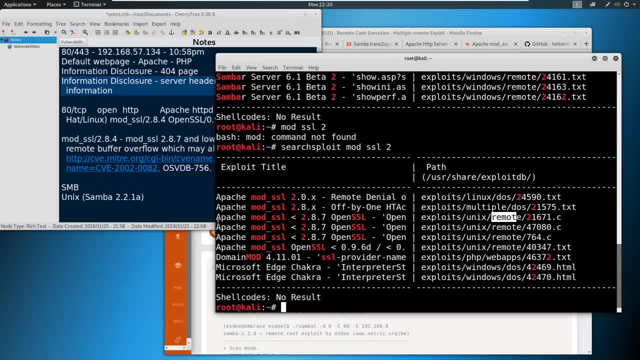 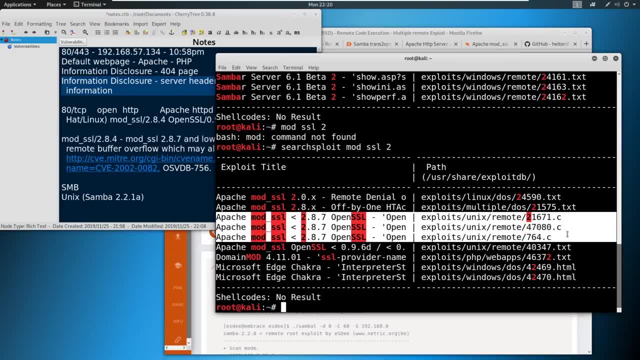 Check, Remote code execution Check And Apache mod SSL less than 2.8.7. Check. So there's three different versions of this, And this is kind of why when I said earlier that you know they don't really work. 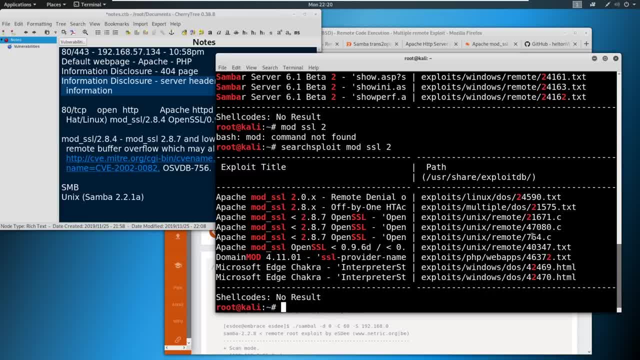 One's been broken. They've rebuilt it. I just like the one off GitHub, So we'll play around with that one in just a little bit. But this is what you're doing. You're either going out to Google with the information that you find. 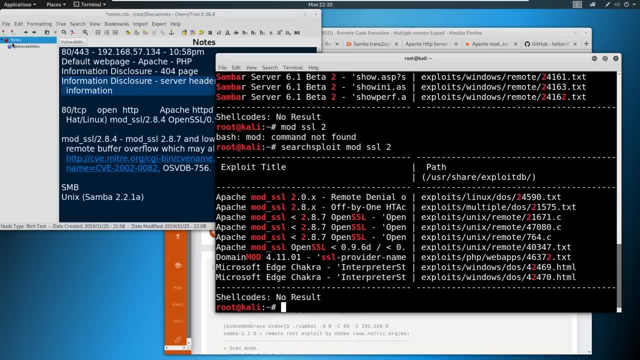 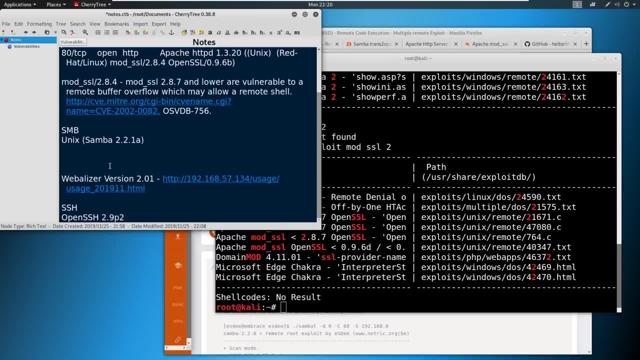 Or you're going to search exploit. You're just doing research. So now we've identified a couple of potential vulnerabilities And we can go from there. So what I encourage you to do is just do some research on this Webalyzer. 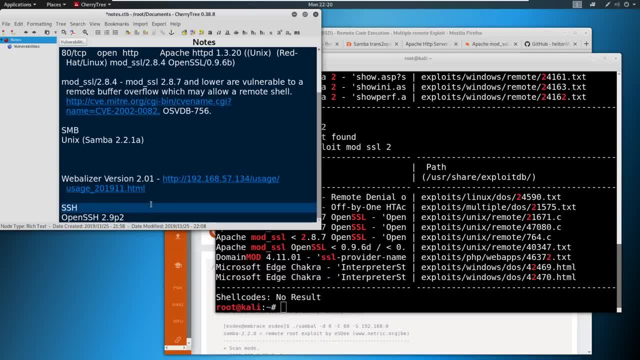 Do some research, Do some research on OpenSSH, See what you can find out Just for research sake. Practice with Search Exploit, Practice with Google, And then meet me in the next video. So what I want to do before we get into exploitation. 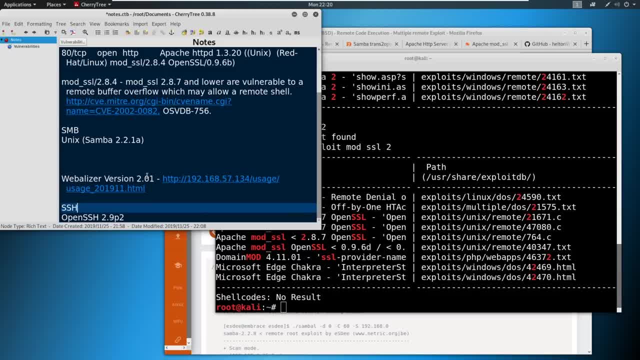 I want to give you a quick sneak peek at what your notes should look like so far, So you can see what good note keeping is. And this is in terms of an assessment. Okay, Just in terms of an assessment. And then from there we're going to practice with some other scanning tools. 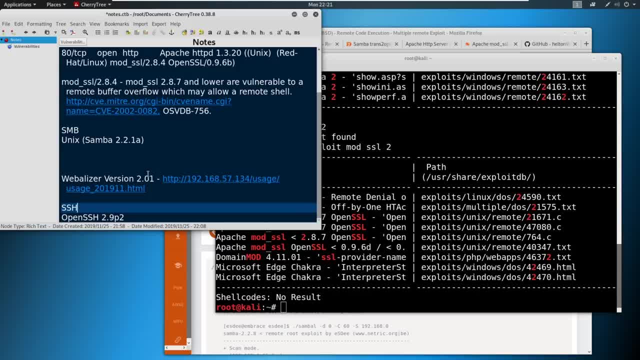 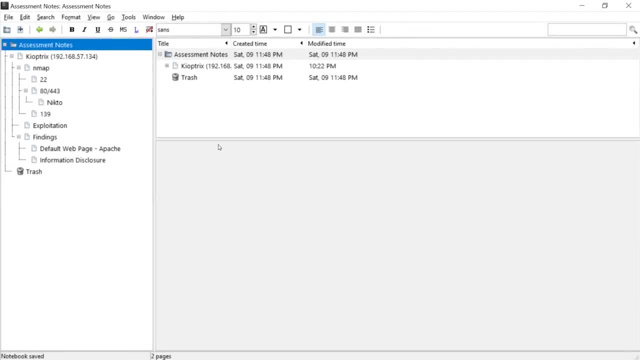 Just to get you familiar with other things, Then Using just Nmap, And then finally we'll move into our exploitation. So I will see you in the next video when we look quickly at our notes Now, looking at our assessment notes so far. 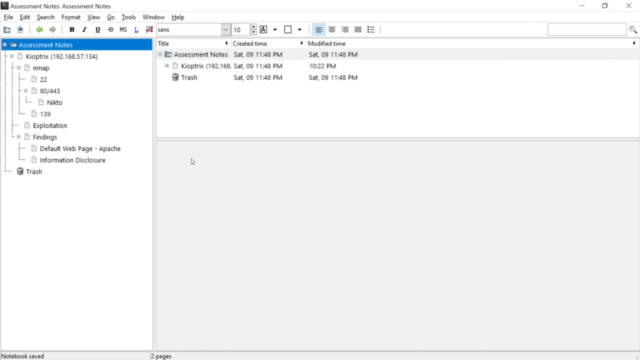 So you can make this however you want to make it. Whatever makes sense for you is how you should do this. Now, this is just a basic example of how I might take notes on an assessment. Now, this is just one machine. 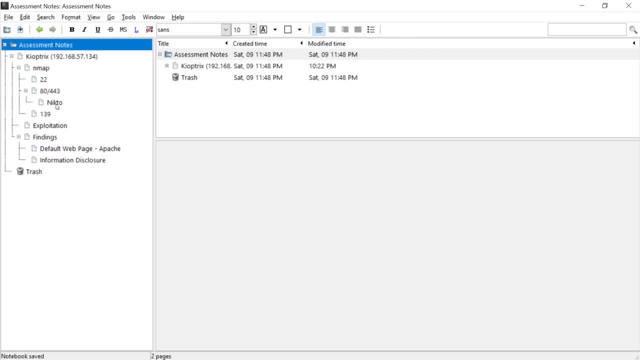 You might be scanning against hundreds of machines sometimes, And that's okay. You just make the notes against the machines and what findings you have. So, for example, here I've got this machine And it's all under this one tab. 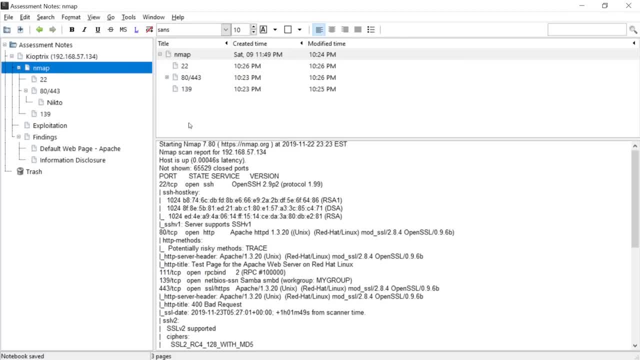 And we've got some Nmap results. And then on the Nmap results we've got the different ports that I found open. I did leave off the RPCs, But we can see our Nmap full results here We can see. 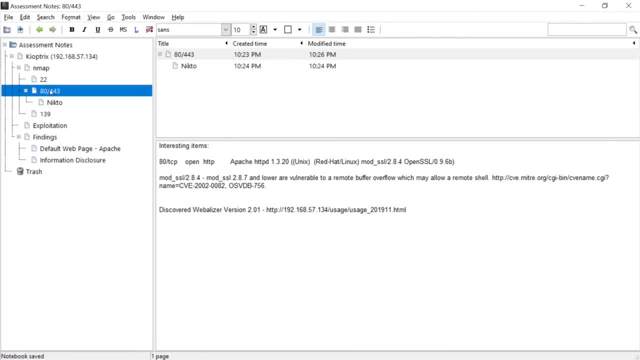 Okay, On 22, I found open SSH On 80, here's some interesting items I may have had. You know again, this is just from our notes. Looks familiar. And then I put in the Nikto scan under here. 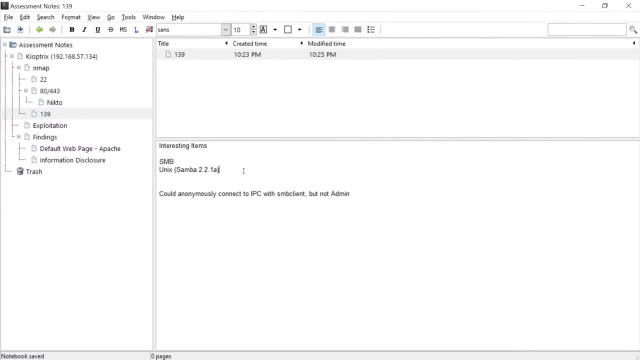 And on 139, I've got the Samba here And this is just notes for us. Again- could anonymously connect to IPC with SMB client but not admin. Your client is never going to see these, So make sure you make good notes for yourself. 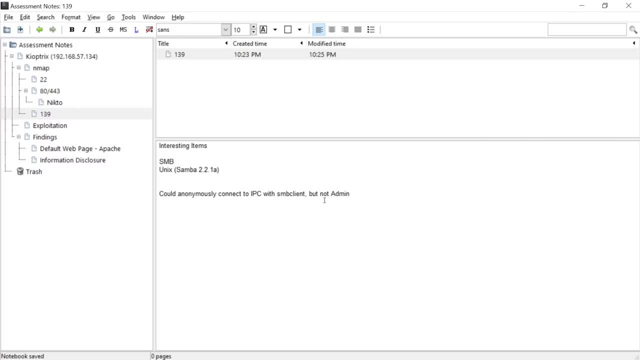 How you can understand it And, importantly, make sure that if somebody goes through here, they can also understand it, Because sometimes somebody else might need to go through your report or through your notes or somebody might be helping you write your report And it's important to be clear and concise with what you're doing. 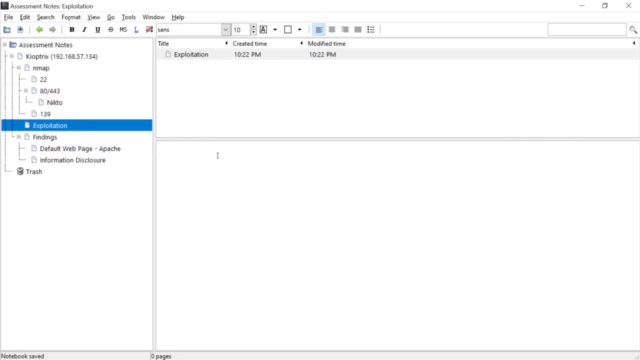 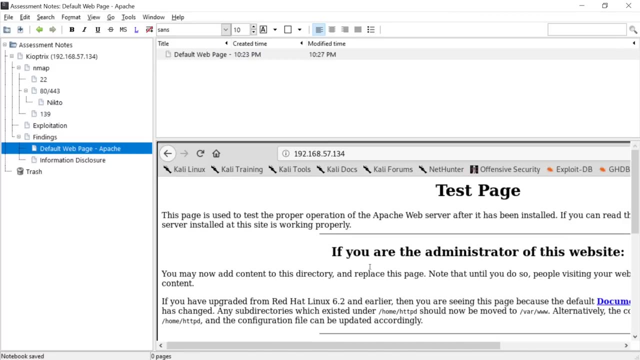 Now I've got an exploitation tab here. We have not exploited anything yet, But I do have a findings tab here as well. So we've got a couple of findings already. We've got this wonderful default test page And it's hard to see. 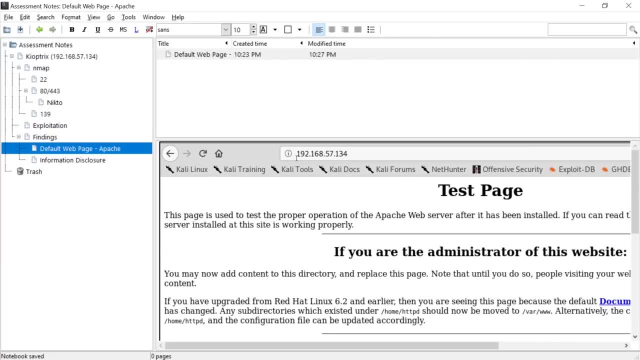 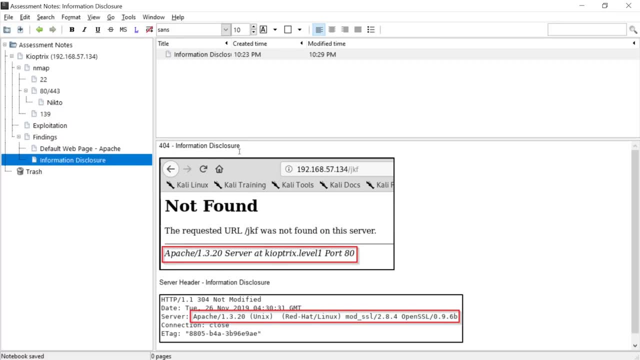 Because I've got it on my screen- that's blown up, But you saw it once- And make sure that you have the IP address or the host name in your pictures. That's important. And then information disclosure here with the 404 page. 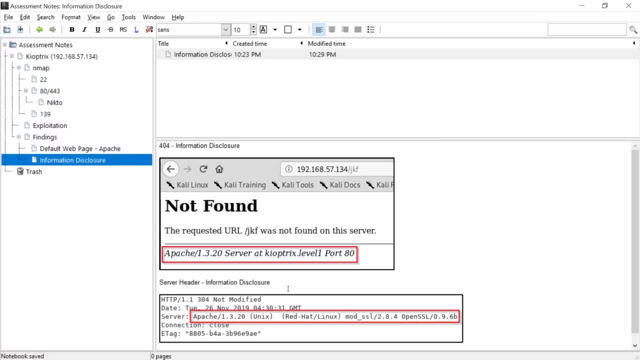 And we've got the server header information disclosure. Now these are both taken in GreenShot. And a couple of things to point out, just for details. I've got borders added around these And I've highlighted where exactly the finding is Okay. 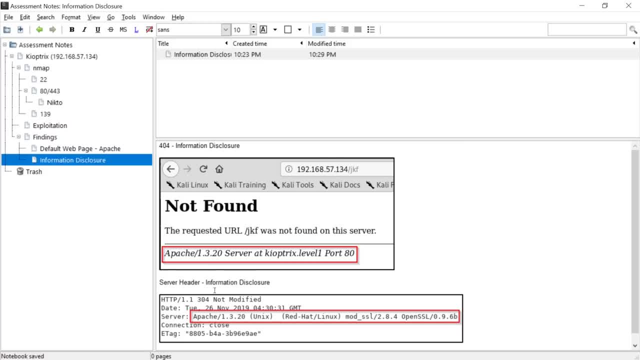 So it's best to point out, Because if these screenshots are going in a report, It's best to find out and just point out to the client Exactly where it is Where they need to be looking. And again, make sure you have your identifier here, if you can have it. 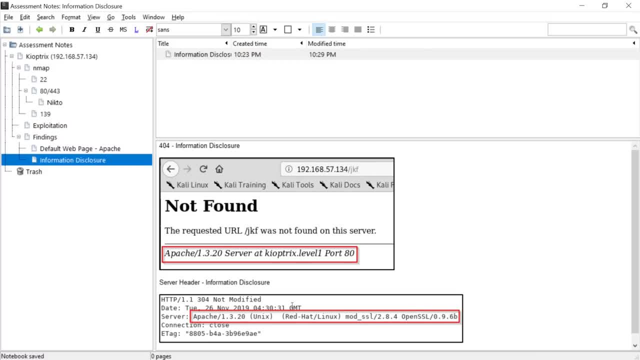 And then here is a response from the website And again with the information disclosure. So that's just a quick example of how your notes should start to form And how they should look, And then we'll do another one after the initial exploitation. 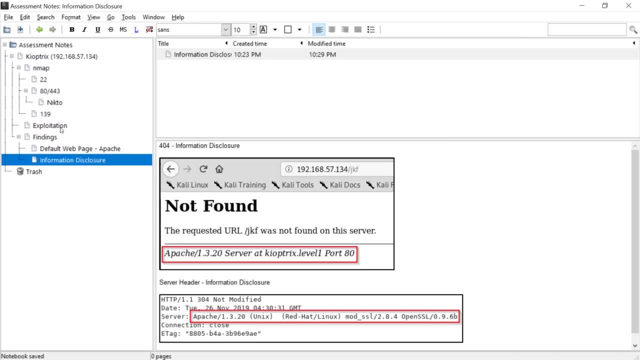 To kind of show how we exploited this machine And how we might take some notes for the client as well, And then you'll get to see this All over again in the sample report When we cover report writing towards the end of the course. 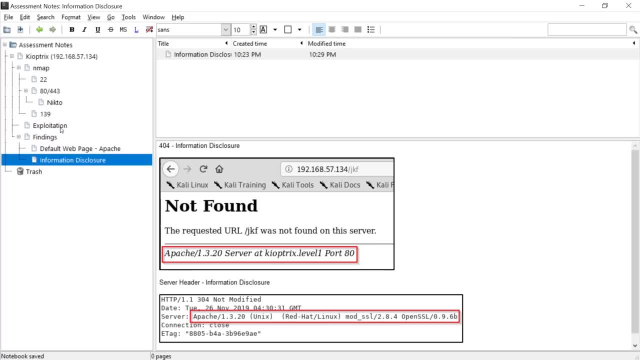 So that's it, Just a quick lesson, Just to make sure you're still keeping up with your notes. I'm going to harp on this throughout Because it's very, very important, So I will catch you in the next videos. 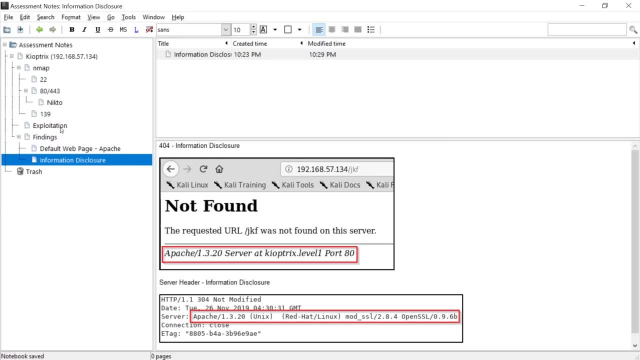 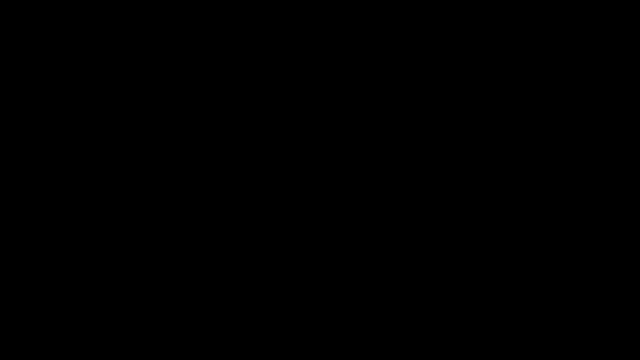 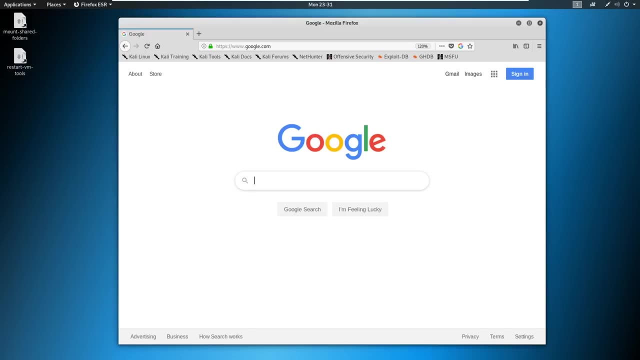 Next little mini chapter on some additional scanning tools And we'll get right into exploitation. Now it's time to play around with Nessus. So when it comes to Nessus, Nessus is what is called a vulnerability scanner. You're going to use this quite frequently when you work as a penetration tester. slash ethical hacker. 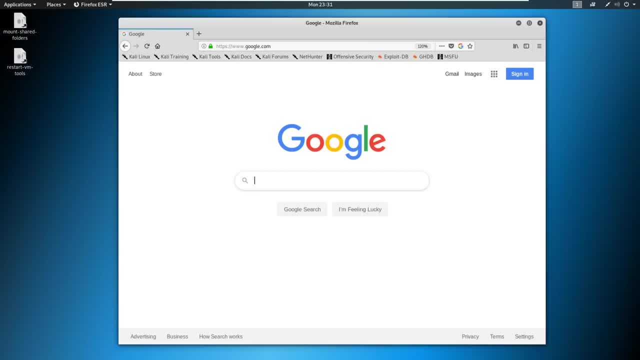 Basically, let's say you're doing an external assessment. Chances are that you're going to use Nessus in that assessment. Probably even right away you might kick off your scans. Basically, you're going to send out an email saying: hey, scans are about to start. 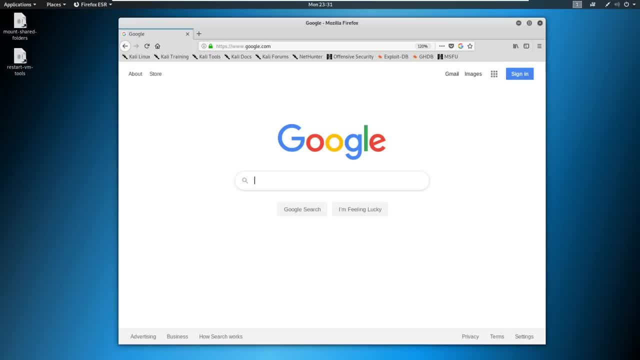 And then you're going to start your scans And then you're gonna let those scans run. And while you let those scans Run run- they take some time- you're going to go out and do your information gathering. maybe look for. 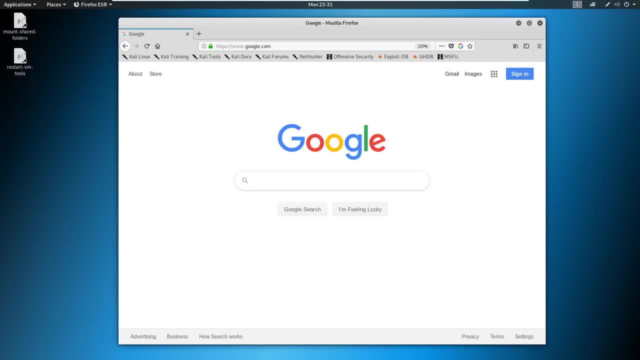 those breach credentials. try to find something juicy on the client. then you'll come back and you'll review your scan results and see if there's anything interesting there. Same thing with internal. the process really doesn't change. we use Nessus quite a bit, So we're going to use 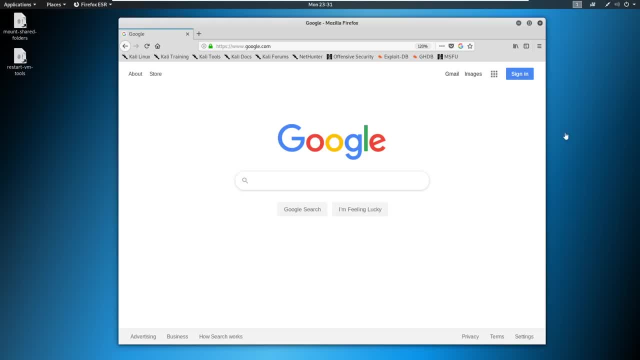 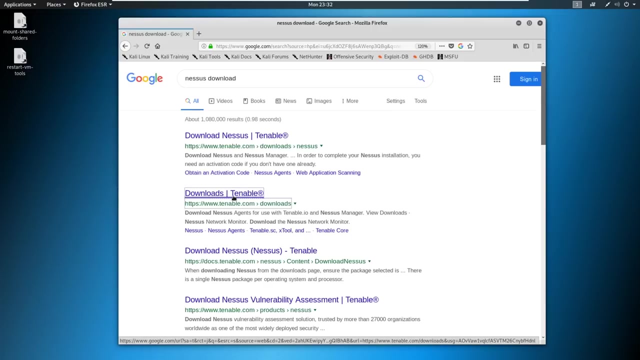 Nessus here and just see what it looks like and how we can use it to our advantage. So let's go ahead and just go out to Google and we're going to Google Nessus download And we're going to go to downloads right here from Tenable. Actually, we'll download Nessus right here, sorry, And up. 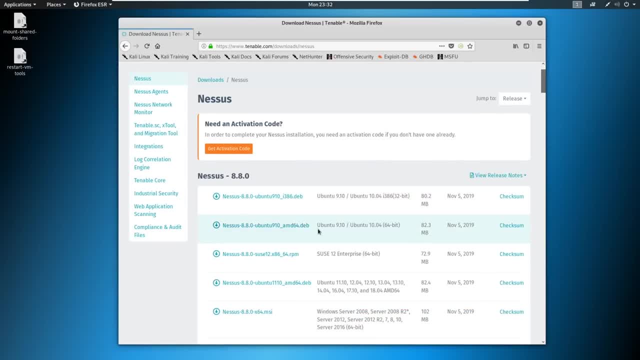 at the top. we are looking for 64 bit Debian. So it says Ubuntu. but we're just looking for the Debian, So we're gonna go ahead and just click on that and download it. We'll agree, we won't even read it. 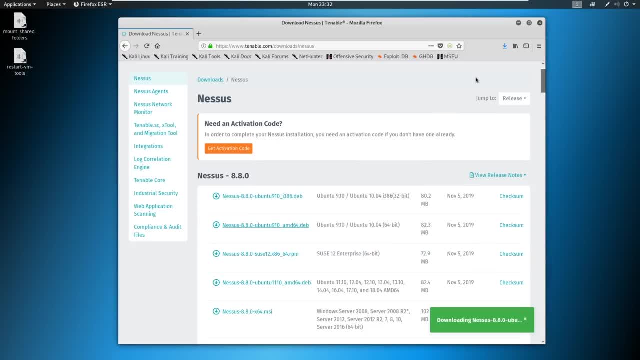 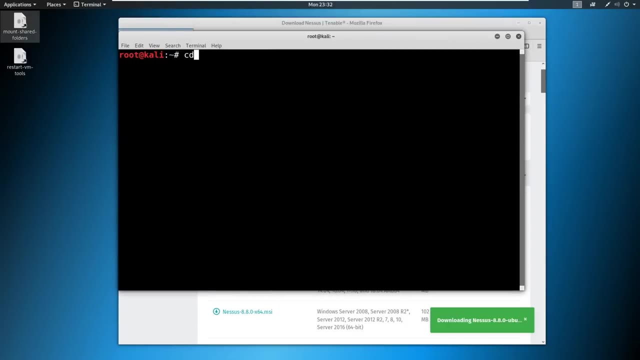 And we'll save here, And this will take a minute or so to download, depending on your connection speed. So if you need to pause, go ahead and pause. Now we're going to open up a terminal And I'll make this a little bit bigger And I'm going to CD over to my downloads folder, because that's. 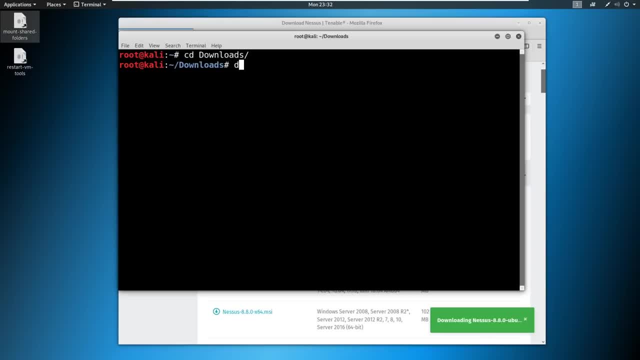 where it is. And then we're going to say dpkg, which is D package, And we're going to install with the dash I and we're just going to say Nessus, There we go, Just tab. if you have nothing in there. capital N on the Nessus, and it should. 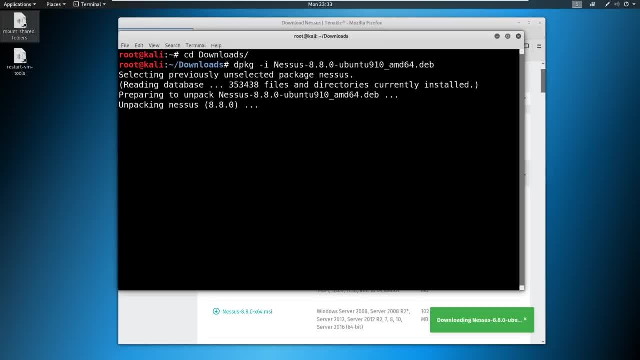 autocomplete And then we'll hit enter And it's going to grab the package and then start to download it here and install it. You can see automatically it has been installed. So it says you can start Nessus scanner by typing forward slash Etsy in it: D Nessus D start. we're just 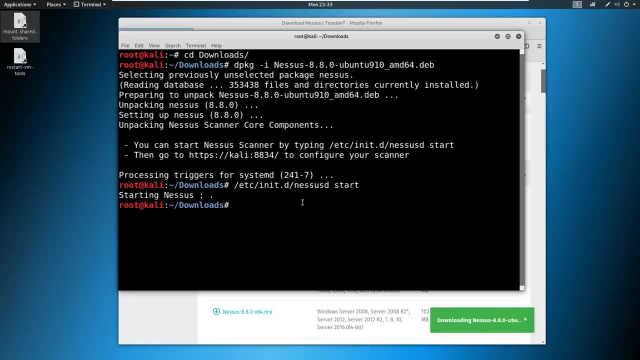 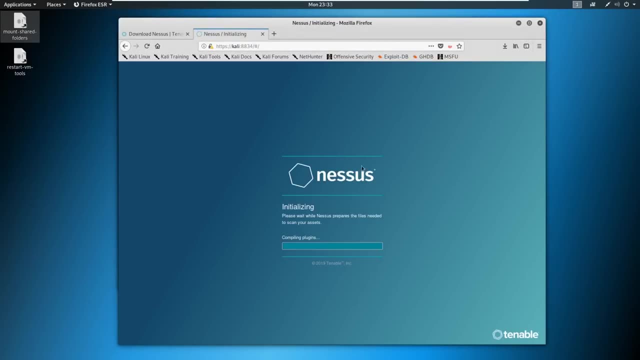 going to copy that and paste it, And then we're going to navigate to this Cali 4438 for 8834.. I cannot talk. And then you're going to see your connections not secure. we're just going to say advanced at exception, confirm. And here is 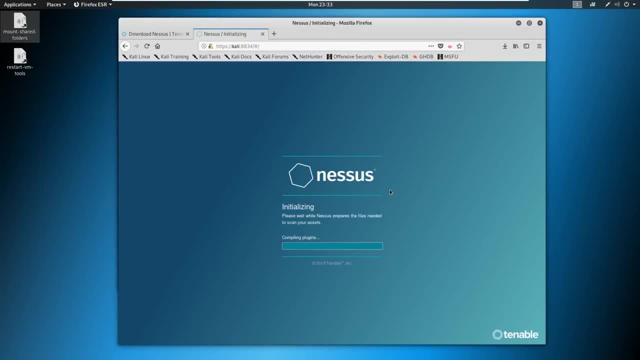 Nessus. Now, this is going to compile plugins here, So this is going to take some time. go ahead and let this finish And when it does, go ahead and say we're going to download or install Nessus essentials, Okay, and then you're going to provide it. 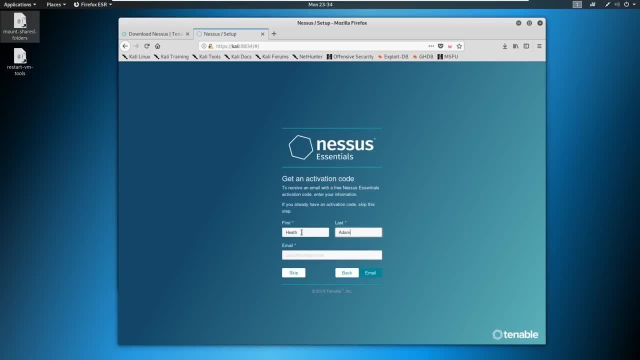 With your name and you need a valid email for an activation code. All right, Once your activation code has arrived via email, go ahead and just copy paste and then hit continue And then it's going to ask you for a username. So I'm just going to say H Adams for me, And then I'll just do password. 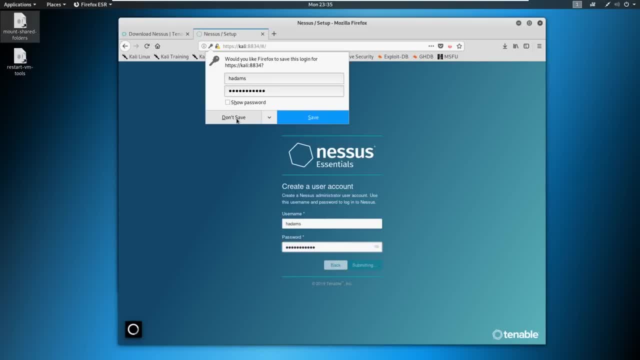 123. Because you know, I'm super secure, I'm not going to save, and then now it's going to take a minute, So just go ahead and pause your video, let this install. go get a drink. go get some coffee. 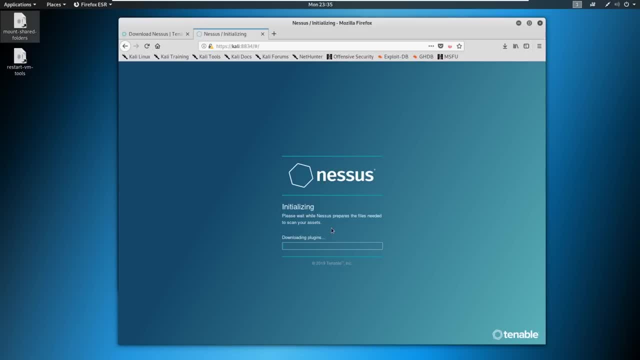 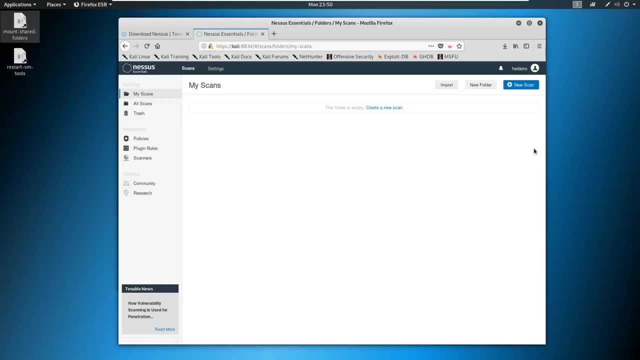 whatever it is that makes you happy, And once your Nessus is installed and you are at a login screen, go ahead and log in and then come back to the video And we'll start from there. Whoo, that took forever. All right, so we have loaded Nessus, it's installed And now we're. 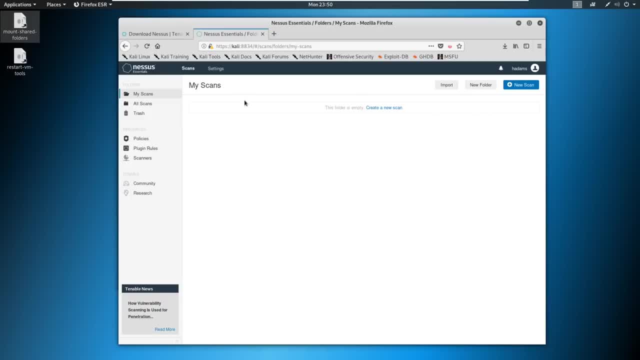 brought to this blank screen that says my scans. Why is it blank? Well, it's because we haven't made a scan yet, So let's go ahead and go up to new scan And let's quickly talk about what we're capable of doing. So this is the free edition of Nessus. 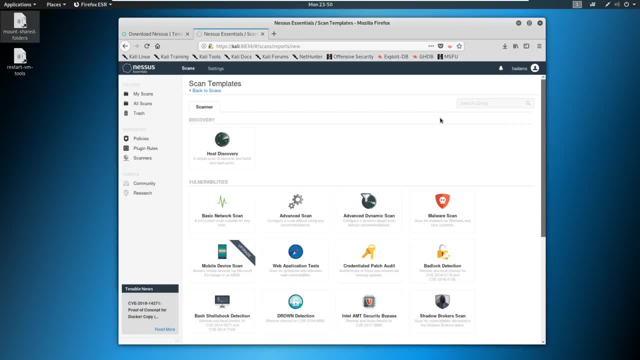 This means that we can scan against any private IP address And we can scan up to 16 of those, I do believe, at one time. So remember, back to the networking section of your class A through class C. that's what we're capable of scanning here. If you were to try to go out and scan a website or 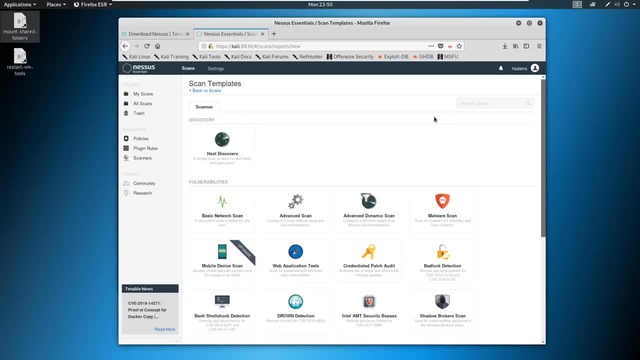 external host not going to happen. We do have a couple options here. We're going to start with this basic network scan And then we'll talk a little bit about the advanced scan. So let's go ahead and click on this basic network. 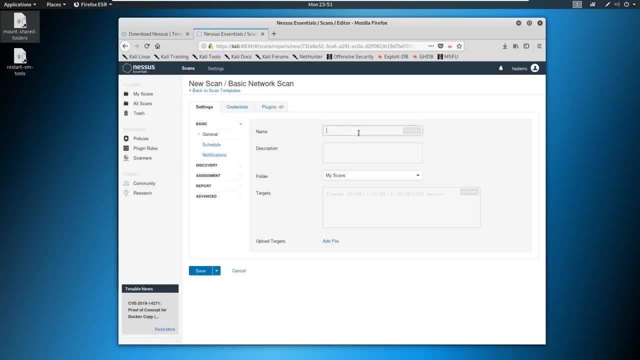 here, And what we can do is we can just type in something like key optics for the name, And then I just always copy this because you need a description. I just like to paste it in the description as well, And then down here it's going to say: hey, what targets do you want to? 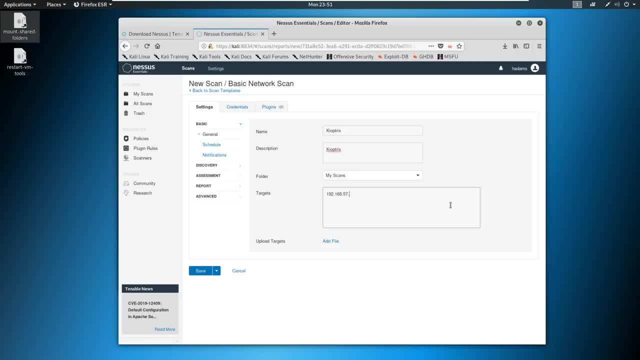 scan against. Well, we're only going to provide one IP address And that is the IP of key optics. So we're going to say the IP address of key optics And then we're going to try and do the same with the tab. We're going to go ahead and work with the tabs here on the side. we've got the 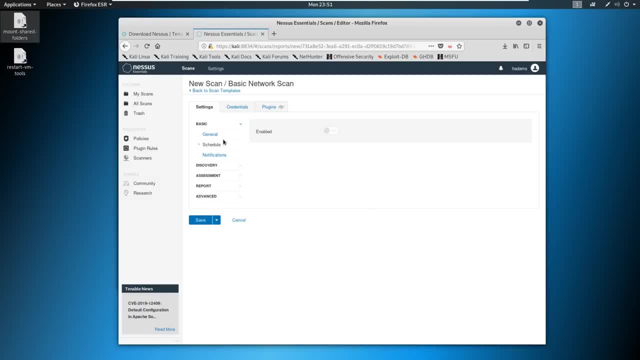 schedule. tab schedule sounds exactly what it sounds like It's: scheduling. So let's say that you are into automation and you're working as a pen tester And you, some Monday morning at eight- maybe you want to sleep in just a little bit longer- And you say: Hey, you know what I got to. 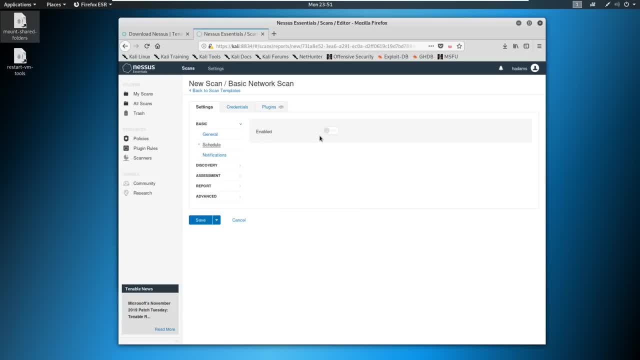 email a client, I'll schedule that email go out at eight o'clock and then email is going to say: can schedule that to happen And then you can wake up a little late. Pro tips there. Also, you can enable scanning for once daily, weekly, monthly, yearly. So if you're in a business you can do this. 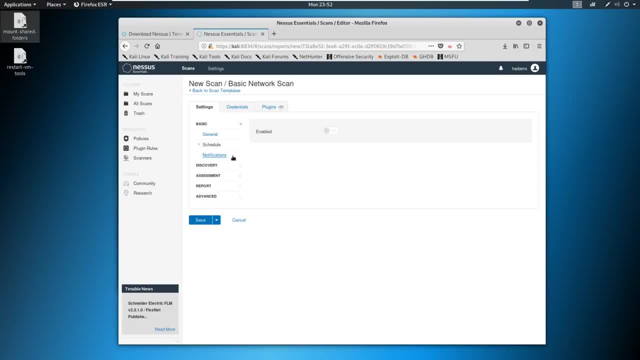 on a periodic basis and get updated scan results. There's also notifications via SMTP if you have an SMTP server. Most importantly, discovery. So it's going to do port scan of common ports here. I actually like to do port scan of all ports. Again, this is the same thing as like a dash P versus a. 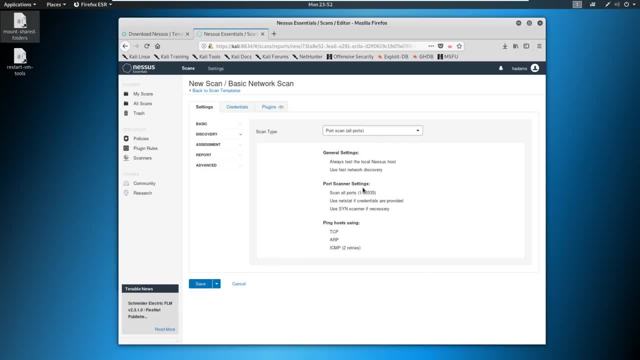 dash, P dash, You see the one through 65,535. here We come down just common ports. I'm guessing top 1000.. So let's go down into assessment and we see scan type: default. So we can scan default, We can. 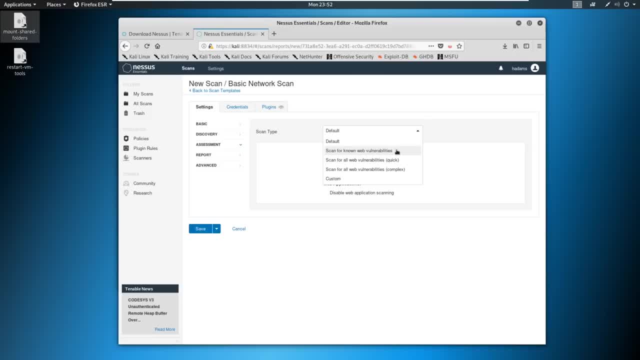 scan for web vulnerabilities. We can scan for all web and all web complex. Let's just scan for known web vulnerabilities. If we go into complex, it's going to take a while And this just depends on how deep into the scan you want to go. But we're just going to say, for now, scan for known web vulnerabilities And it'll show. 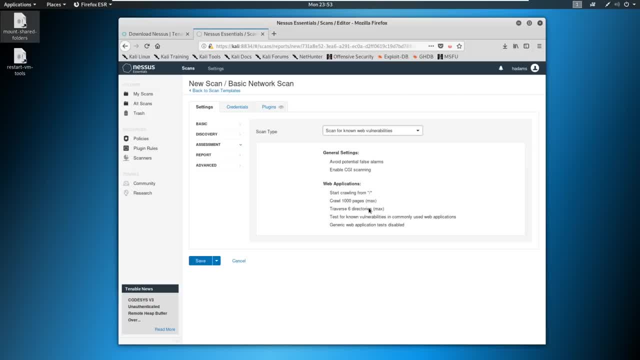 what it's going to do. It's going to do some page crawling, do some directory traversing and look for vulnerabilities. Okay, on the report, it's going to say, hey, can we edit scan results? Yes, we can. Should we display hosts that respond to ping? display unreachable hosts? I just leave this. 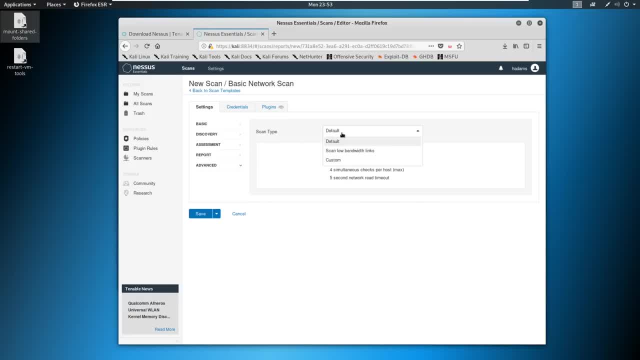 as default And then on the advanced tab we have scan type. I just like to say default here, So we'll save this And then we'll go ahead and just launch it And you'll see the wheel starts spinning, And now it means we're. 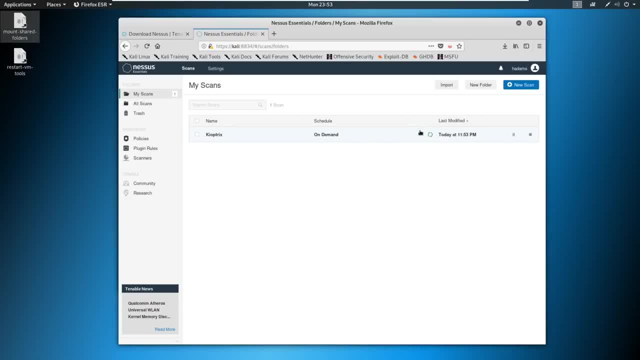 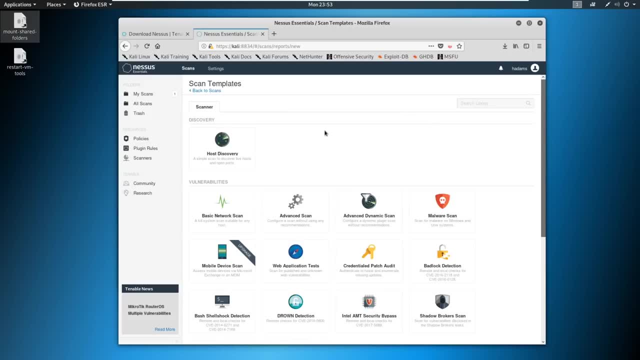 running and this is going to take some time. So while this is going on, let's go ahead and hit new scan up here And let's look at this as well. So we've got the advanced scan And they've got other scans here, which 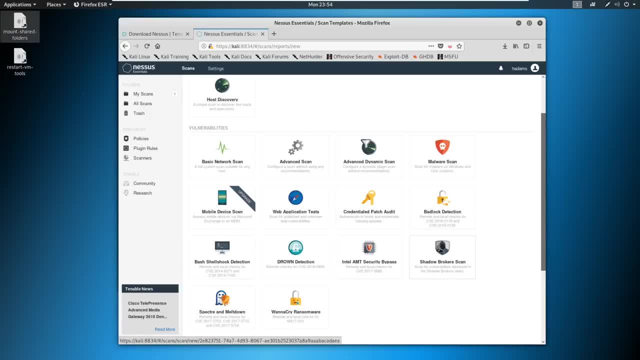 will then show up in the editor. I don't use a lot of, but you might have used them in the past if you're familiar with Nessus, or they've got little one offs, like they've got this shell shock detection And it looks like. 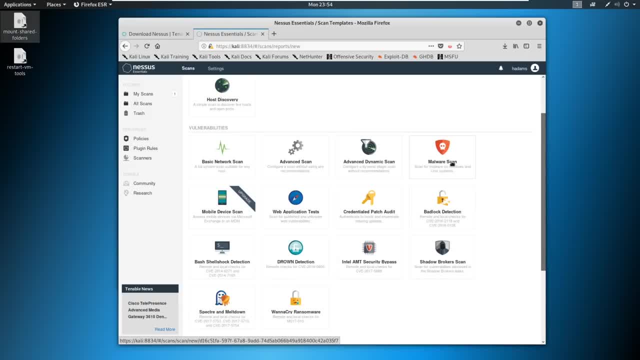 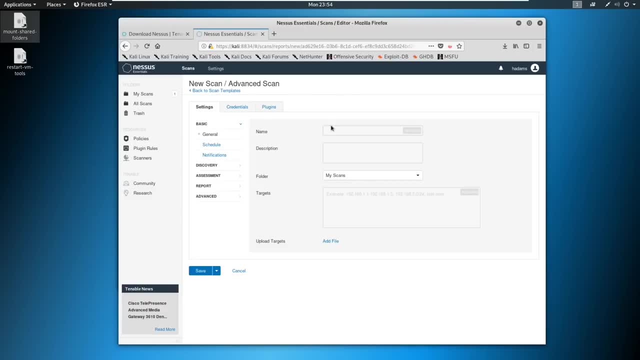 they've got the shadow brokers detection here. So they've got a couple different scans, even a malware scan. But we're going to go into advanced scan. these are the most common two. you'll be using Same deal here And when we go into discovery you see the discoveries a little. 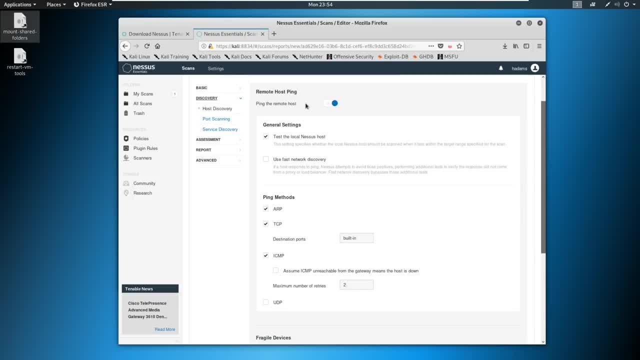 bit different. So we've got host scanning And it says, Hey, do you want to ping the host, Or maybe you don't want to ping the host? And if we do ping the host, what are we looking for? Are we looking for our TCP, ICMP or UDP? What do we want to scan? Do we want to scan network? 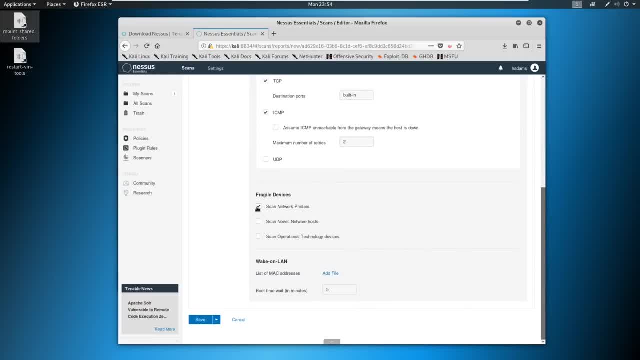 printers. If we're doing an internal network assessment, maybe we want to click that, Maybe not, you know- and we can do a different types of scanning here. There's a lot more options, which is what advanced scanning is for. We could do port. 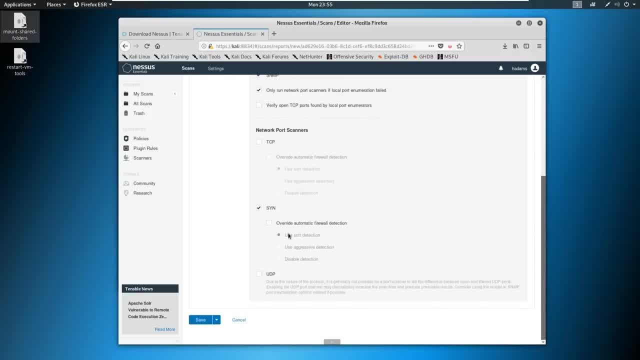 scanning. you see the SIN scan comes up again, aka stealth scanning. we could do UDP And even down here it says it's really not possible for UDP to pick up between open and filtered ports. So UDP scanning takes forever And it's not always reliable. We can do service discovery. 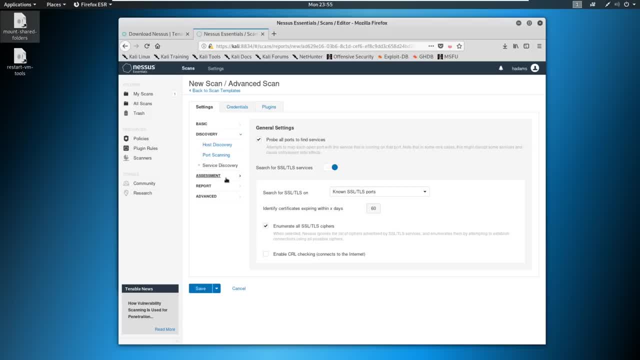 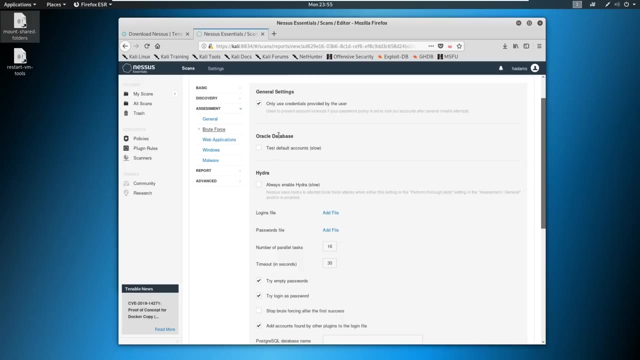 I kind of just leave these blank or leave them as default And then we come through assessment. same thing. It just gives us additional options here, So it's always good to click through these. Do we want to brute force any logins? we could use hydro to do brute forcing. if we want, we could test for default accounts on. 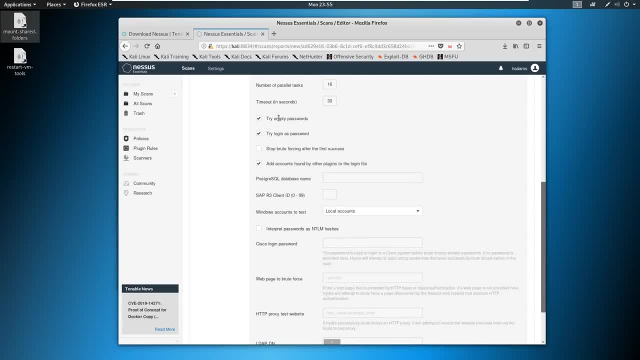 if we could discover, like an Oracle database etc. But this is going to go through and try empty passwords, try login as password, etc. So this just does a little bit more here. we can scan web applications And we can say: hey, we want to use a specific user agent or we want to crawl. 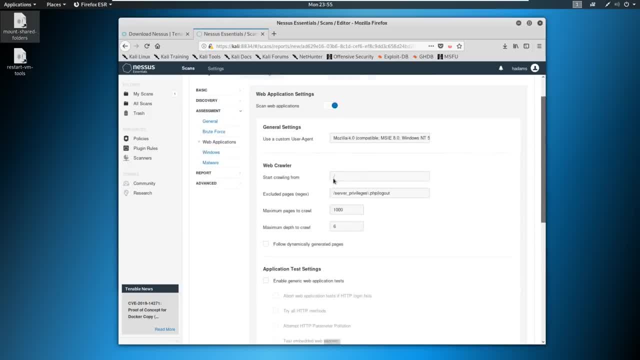 from a certain web page how many pages we're going to crawl Again. it just gives us more control. So if we come down here, reporting looks the same, And then advanced, we have a little bit of more options here as well. 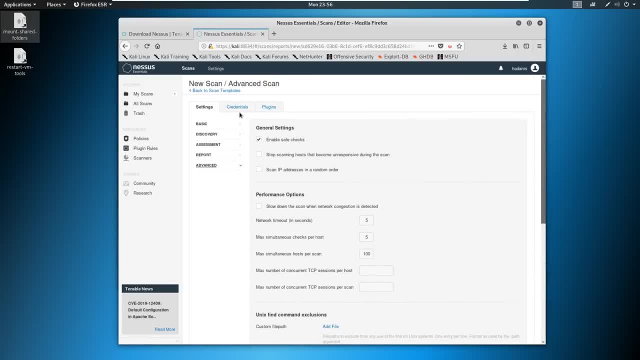 But again, either, either way, if you use advanced scan, I would start with the basic scan just as a beginner and then kind of play around with the advanced scan and see if you can scan against the same host and maybe get back more information And maybe key objects. is a good one to play with. 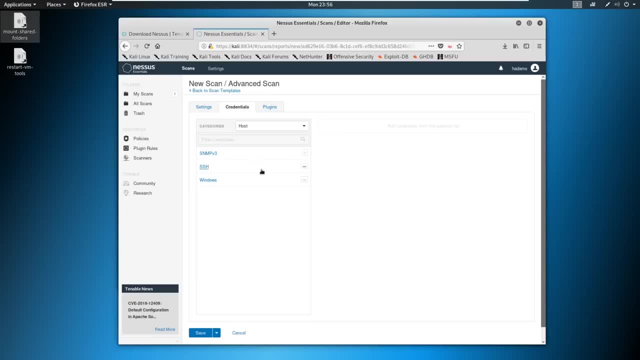 But let's go ahead and go over to credentials. And now, if you had credentials for a machine and you wanted to like log into that machine via SSH or Windows or even SNMP, you can enter in credentials And you could scan a little bit deeper on the 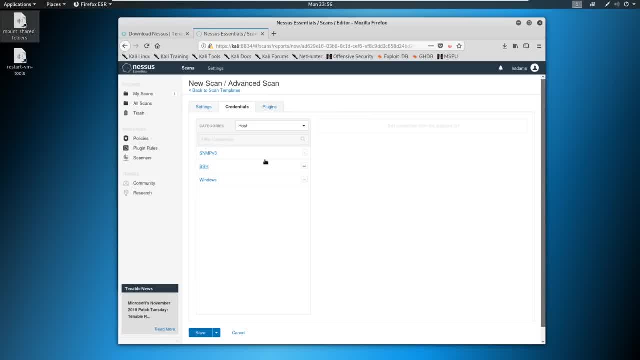 machine, but you're likely never going to get that as a pen tester, because you usually don't have any access. So let's go back to our scans And you see now that it's scanning and running. The nice thing is that it does update vulnerabilities as it finds them, and it is finding them. we're actually at 99%. 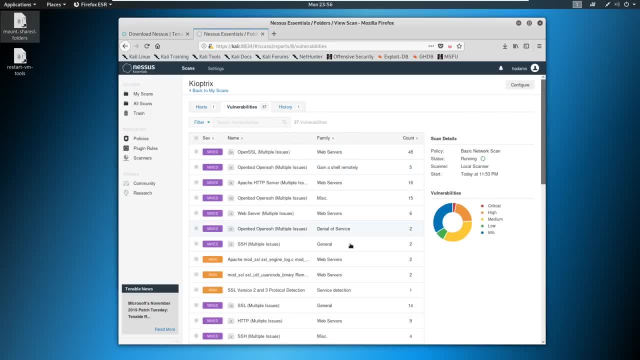 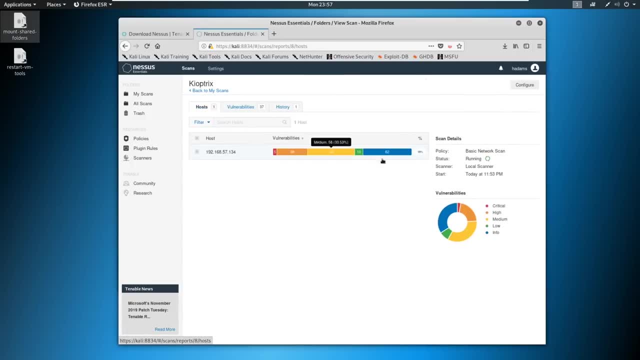 right now So you can click in it And you can see that it's got all different kinds of vulnerabilities And right now they're kind of grouped So we won't worry about them too much. we're going to ungroup this. once it's done, So I tell you what: go ahead and let your scan finish. 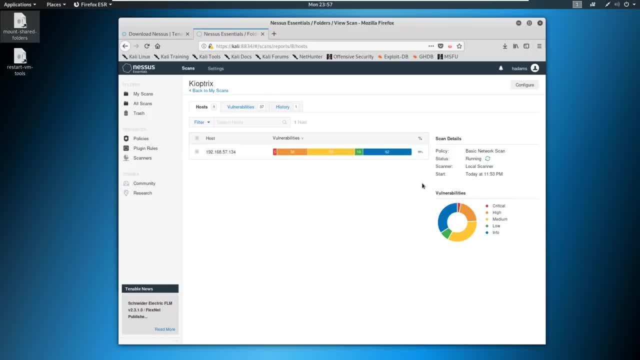 Once your scans finished, I'm going to meet you over in the next video, which is going to be part two. we're going to look at the scan results, talk about them a little bit and see what Ness's can do for us. 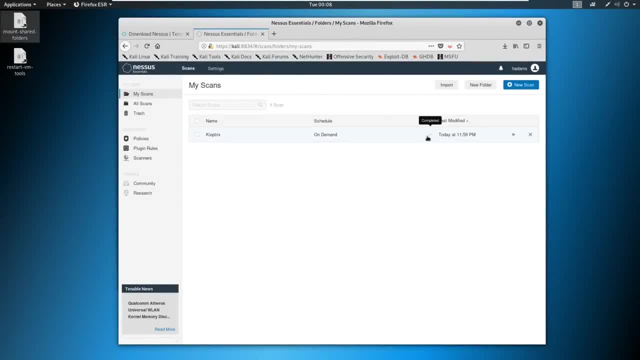 Now on to part two. our scan results are done And we can tell, because we've got a nice checkmark here that says complete. So we're just going to click into our scan results And, looking at the overview, we can see here that we've got five critical, 38 highs, 59 mediums. 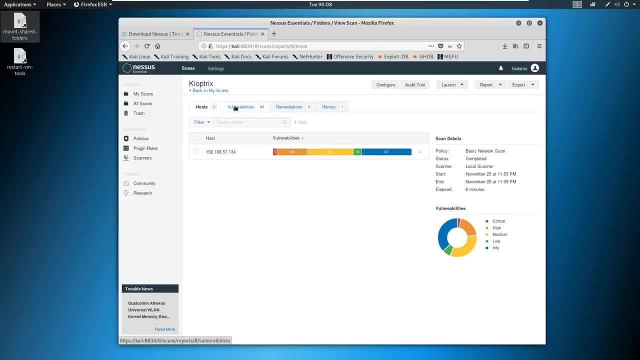 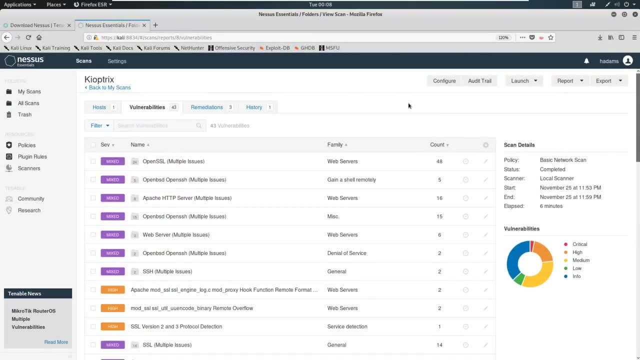 10 lows and 67 informational. So we're going to click on the vulnerabilities here And let me make this bigger. So we're going to do is we're going to just take a peek at this And this new version of Ness's actually starts grouping these together. Let's go ahead and 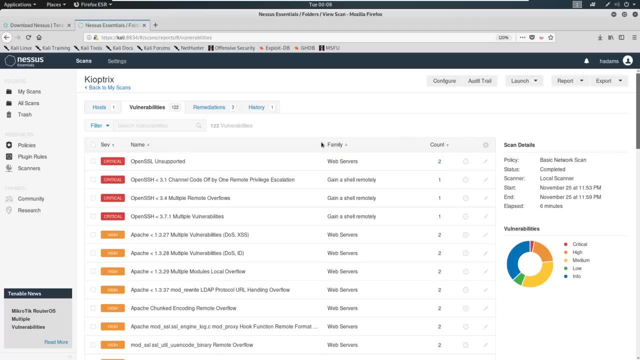 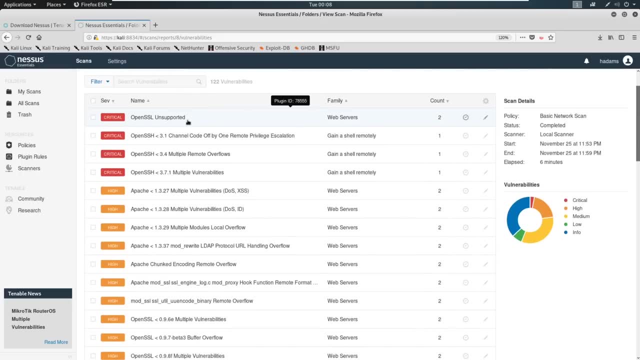 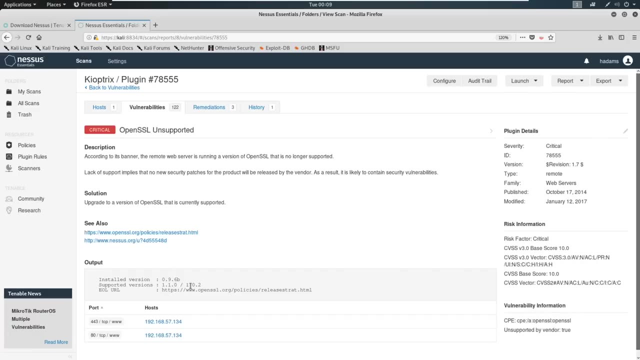 hit Settings and disable groups And that'll show us by severity coming back up: OpenSSL unsupported. Let's check it out: 0.9.6b, 1.1.0 and it's saying: according the banner, the remote server is running OpenSSL and it doesn't. 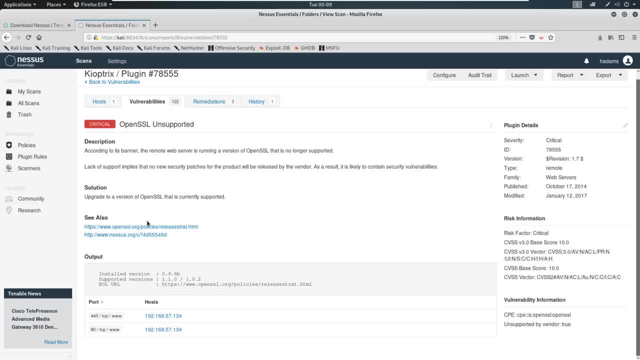 tell us much about it. We'd actually have to do a little bit of research, click into this, see why this is such a bad thing, but this is absolutely out of date. Okay, so if we're making a screenshot here, we're gonna say, hey, this is out of. 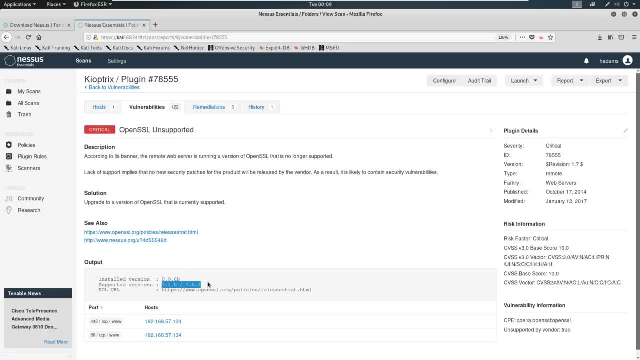 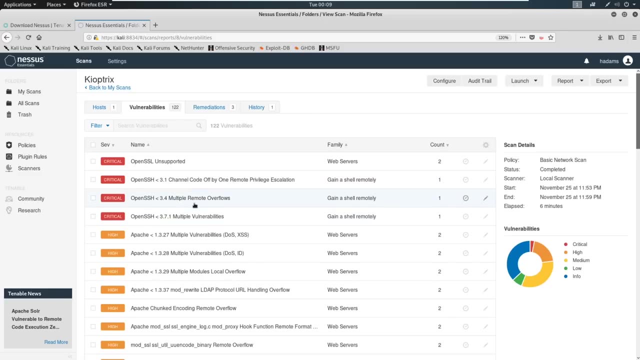 date. We see this installed version. It's recommended to patch to this version. So if you're taking notes, you can go ahead and add that into your notes for your vulnerabilities. This is insufficient patching. Come back through here. It says even OpenSSH has remote privilege escalation. It's got remote overflows, so 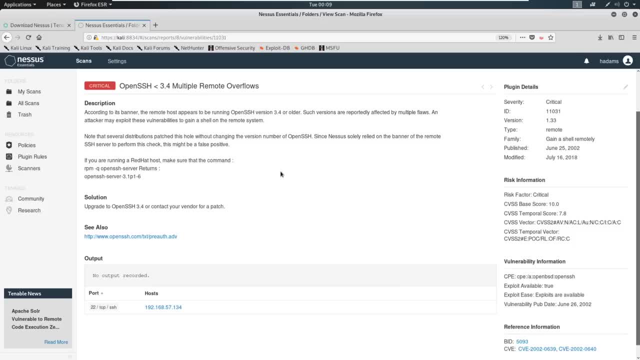 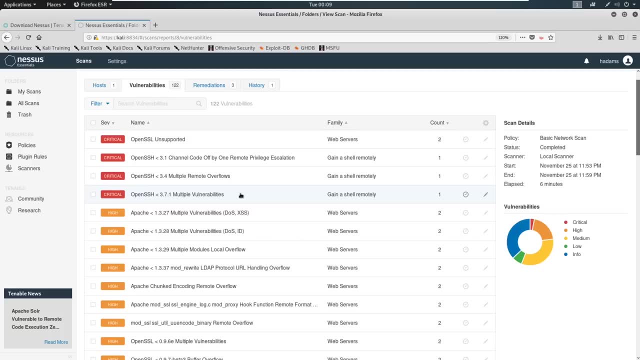 it looks like you could possibly perform an overflow. If you did that, thenut travel is not going to happen. So then, if you overflow against SSH, So if you did some research and you were able to find a vulnerability with that, that's cool. And we come through here and you see, the Apache has denial of service cross. 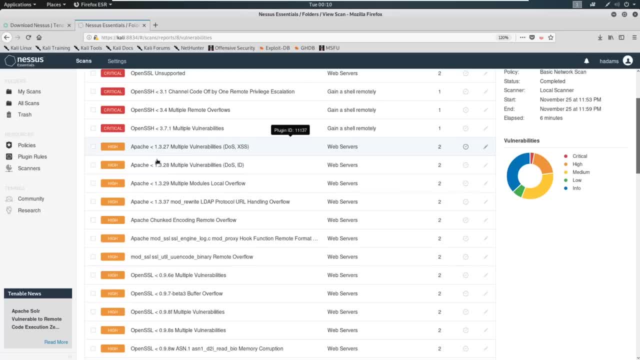 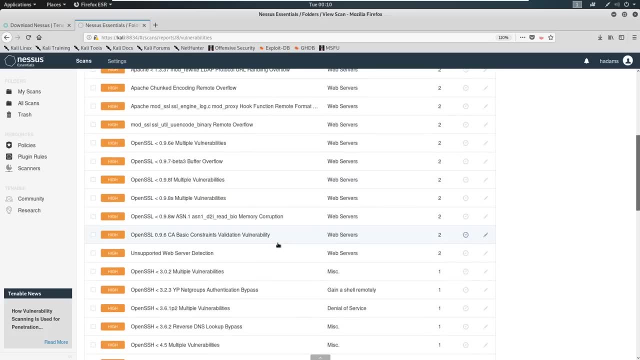 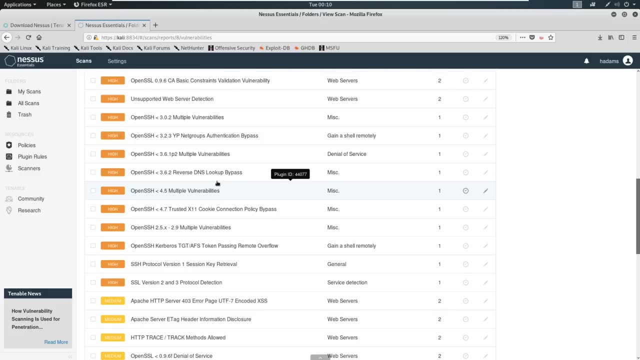 site scripting Again, Apache looks like insufficient patching and mod SSL shows up, open SSL shows up And I mean we've just got vulnerability after vulnerability. So we would write a lot of these up and, depending on the assessment and how the assessment was going, 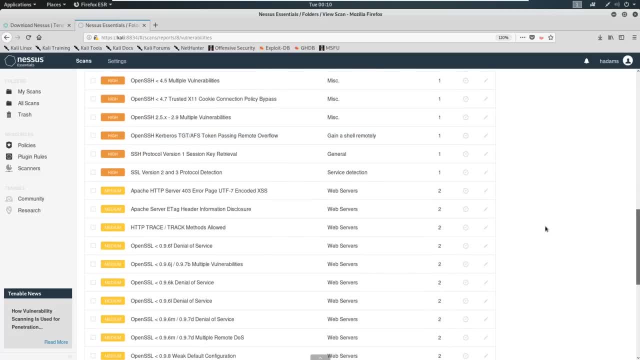 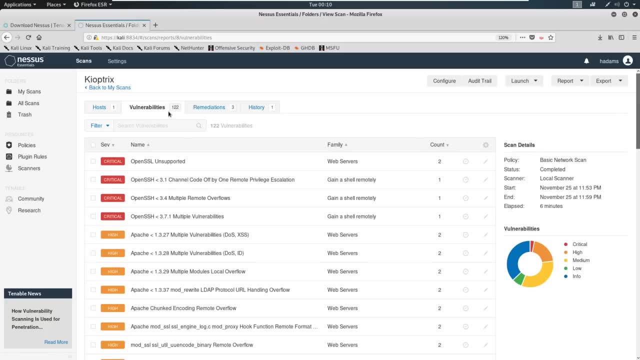 depends on the severity that we're going to write up Now. if we find remote code execution, we get a lot of access to a client and a client just lights up like a Christmas tree when it comes time to reviewing their scans. then a lot of these, you know we might report on a lot of. 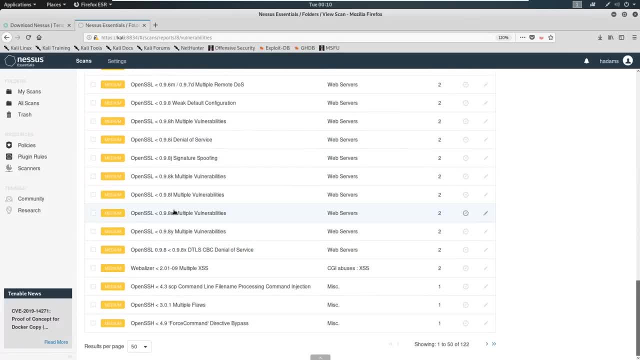 these and we might not report on a lot of lows or a lot of the mediums. But if we're in the opposite situation, where you know we aren't finding a lot but there's still stuff to report, then we might report on a lot of those. 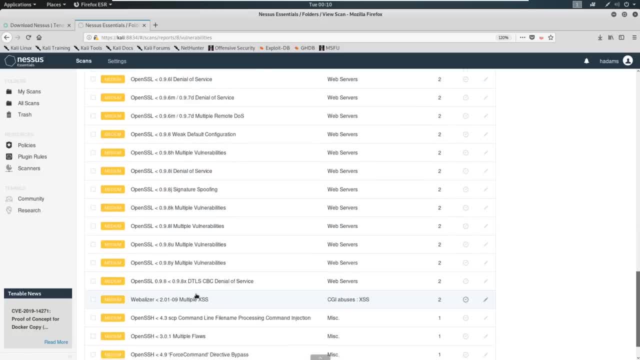 Like, hey, open SSL is. you know it's out of, you know it's out of date. And then we go to the next page and we find a low and maybe there's like okay, there's, there's something in here. 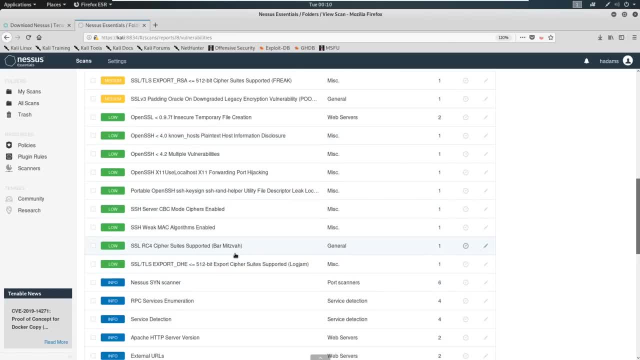 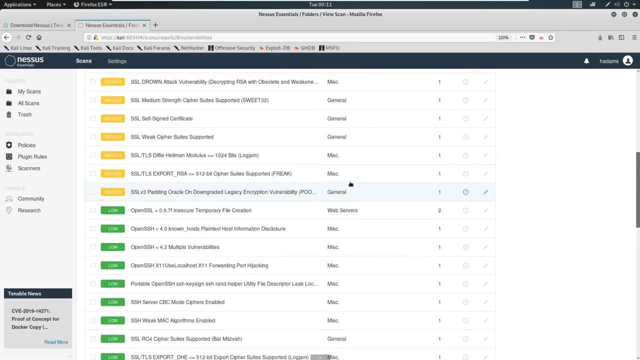 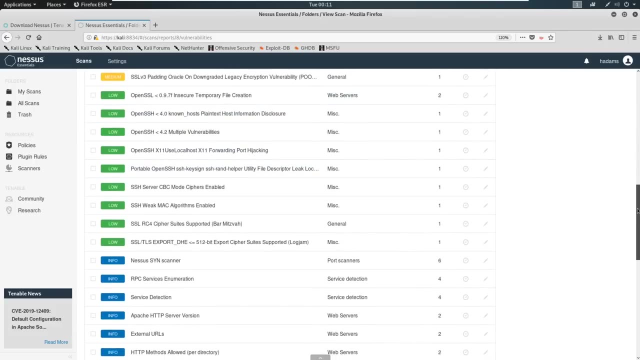 that's related to SSL TLS. This one is an unsupported cipher. we might report that as well, just depending on the potential in how many vulnerabilities that there actually are. So as of right now, it looks like this box is pretty critical. But what we also do as penetration- 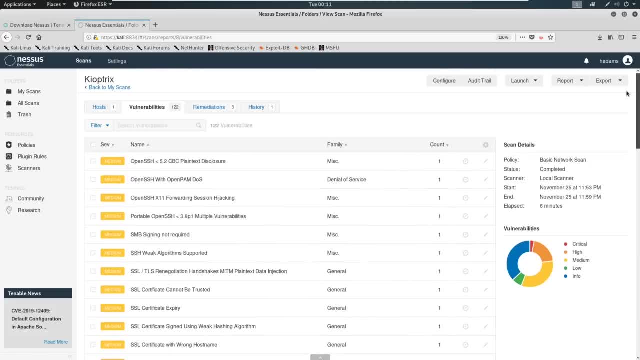 is we take all the results in front of us And what we'll do is we'll come in and we'll download this Nessus file. we'll take that Nessus file- And there's tools out there to convert a Nessus file into an Excel document And it makes it nice and pretty And we'll hand that over to the client. 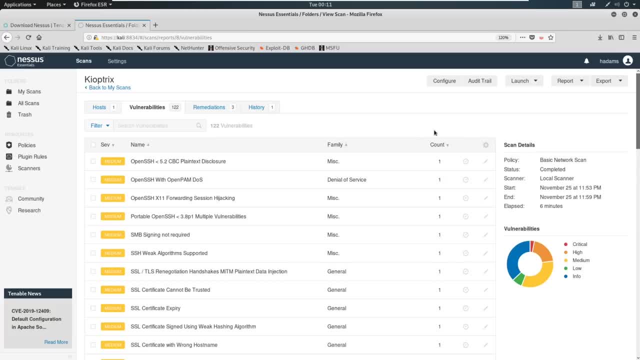 as well, And in the report it'll say: hey look, we've covered some of the vulnerabilities. there's no way for us to touch all of them, Because this is a timed assessment. we focused on the low hanging fruit, we focused on what we could. So please do go look at the 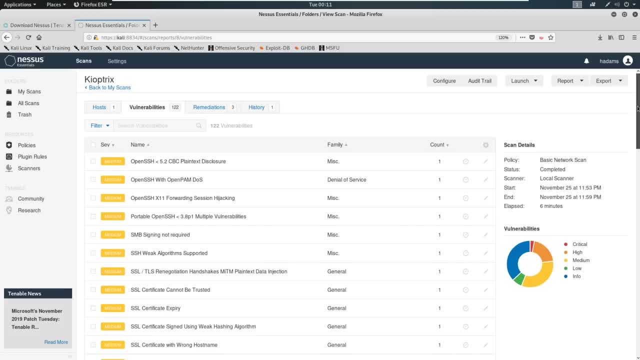 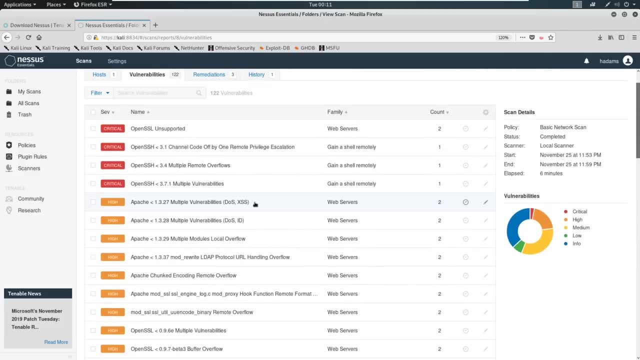 Nessus scan results and all the information that we provide you because it's super important. So, again, if we have a client like this, where we're going to have remote code execution, we're gonna have a lot of vulnerabilities. then these things just start to stack up, And this is what a Nessus 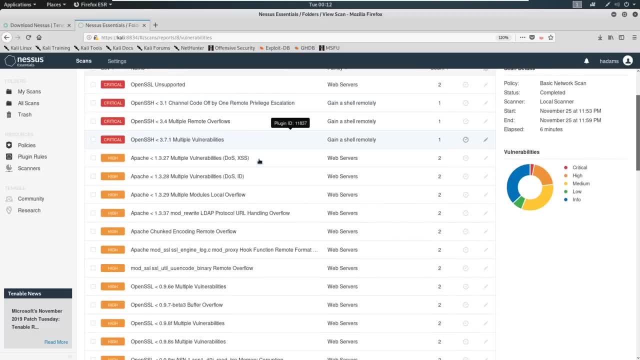 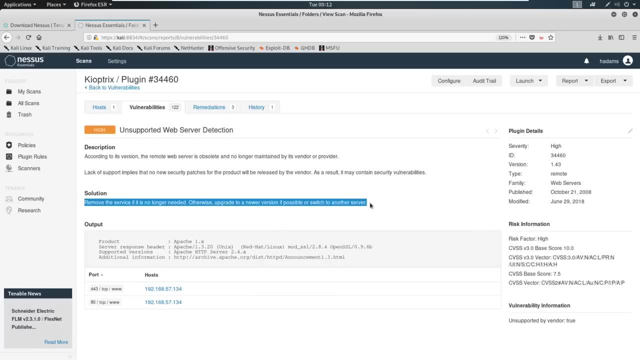 result looks like you can click into these, you can get more information and possibly even you know details on how to exploit it and how to solve it as well. So there's useful links in here a lot of the times and just 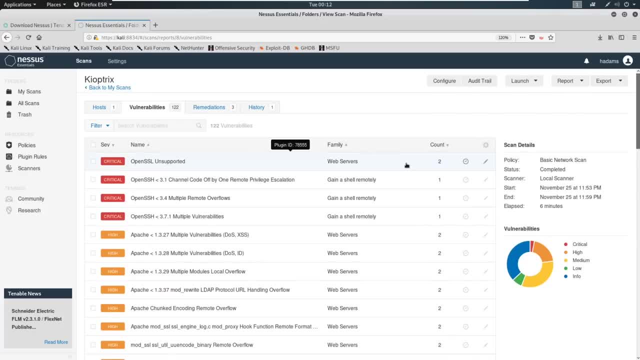 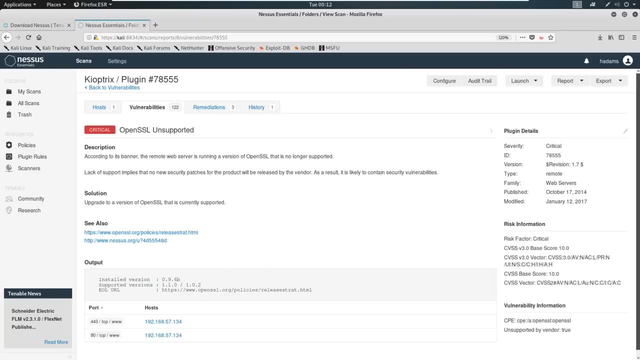 you know they give you information, but you should always go out and verify. never trust your vulnerability scanner Just because it says, hey, we detected it. you should go out and look and find it. Just like we had that screenshot from before with the Apache service version. 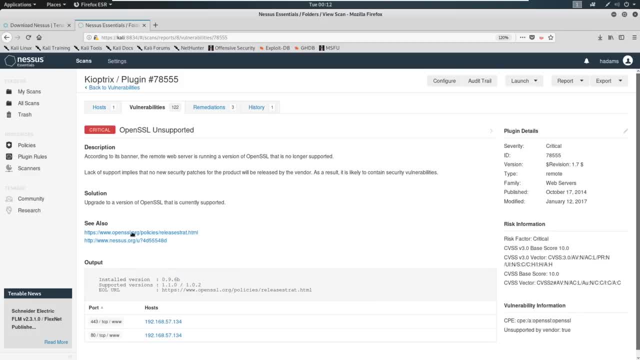 we know this exists, we wouldn't provide a screenshot of the output of Nessus. we would go provide a screenshot that says: hey, we actually proved that. we know it's there And you're out of date. So hopefully that gives you an idea of what we're doing with Nessus and why. 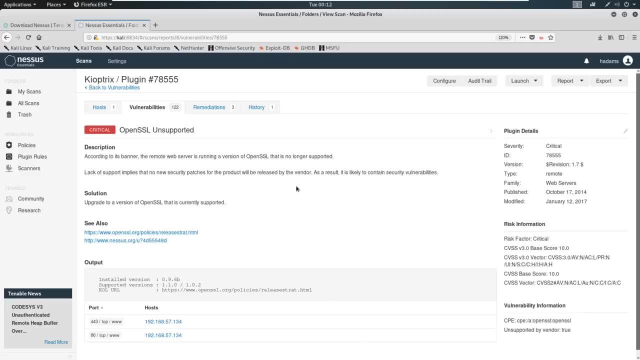 we're using it and how it could be used, And if you're interested in learning more about this, please go to the link in the description below And we'll see you in the next video. advantage to us: Sometimes we're so overwhelmed with everything around us that we might miss some. 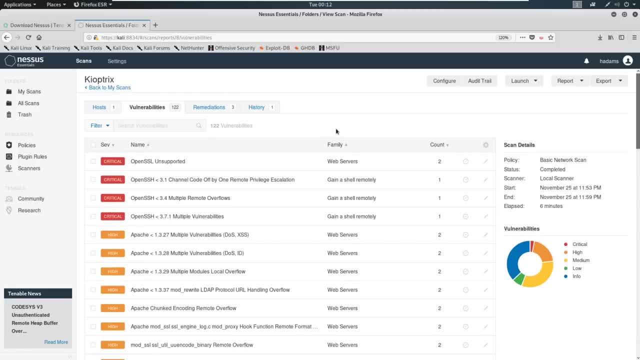 vulnerabilities And it's nice to just have a scanner detect a lot of vulnerabilities just for us And it gives us something to look through, something to verify, double check etc. It's just an extra layer of vulnerability assessment for us. It's a friend in the game. So I own two programs. 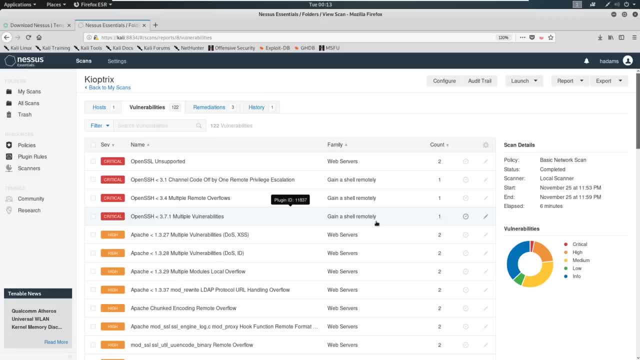 as a pen tester. two programs that I pay for: Nessus license is one, burp suite Pro is the other. So that's it for this section. Now we're going to move on to exploitation, really start to get into the fun stuff. talk about some different. 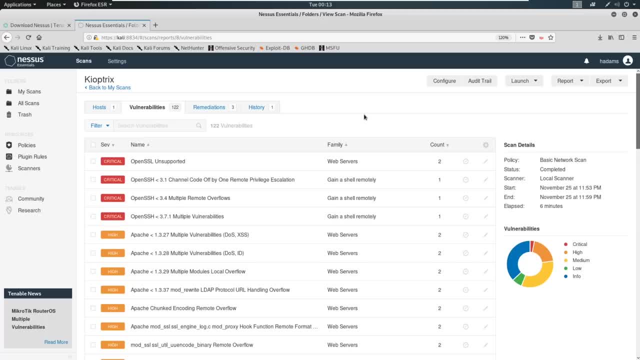 exploitation techniques you're going to see, And then we'll do a bunch of box walkthroughs and get into exploit development And it's about to get so fun. This is the fun part of the course. Up until this point it's just been scanning, enumeration, learning about the process, And it's been nine. 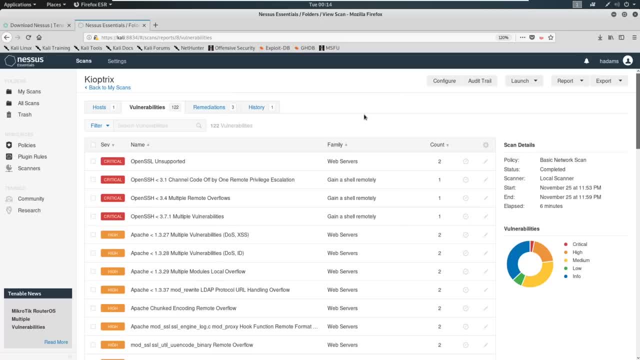 hours, of course, but it's been a lot of fun And we'll see you in the next video. Bye for now. materials so far: almost eight hours, of course, material just to get to this point. That's how important I think that information gathering and scanning, enumeration are, along with the 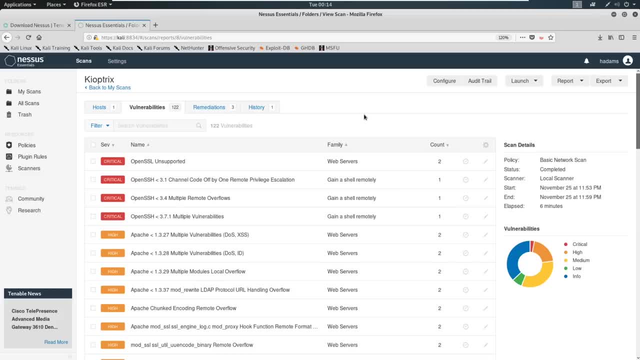 foundations and the materials. you need to know all that before you can just start exploiting machines. So now we're there. Congratulations, pat yourself on the back. We're almost halfway through the exploitation part of this course. So once we get to the middle of the course, capstone, 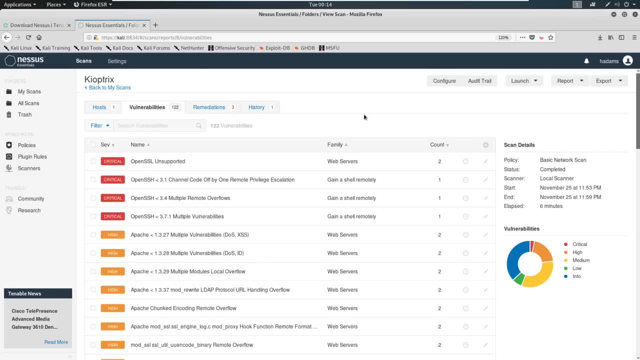 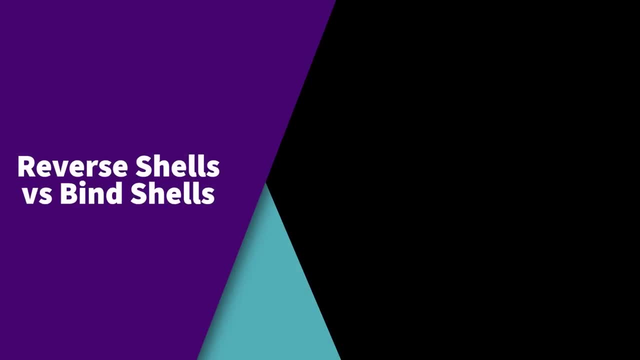 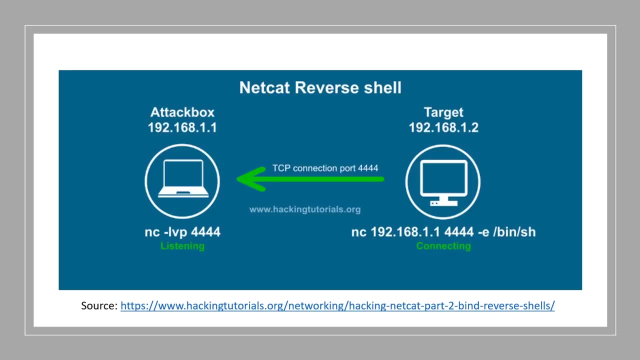 I think it's gonna be really fun and exciting. So that's it And spiel. I'll see over in the next section when we start learning exploitation. Before we could start the cool exploitation phase, we have to first define a couple things. So we're going to quickly define different shell types. 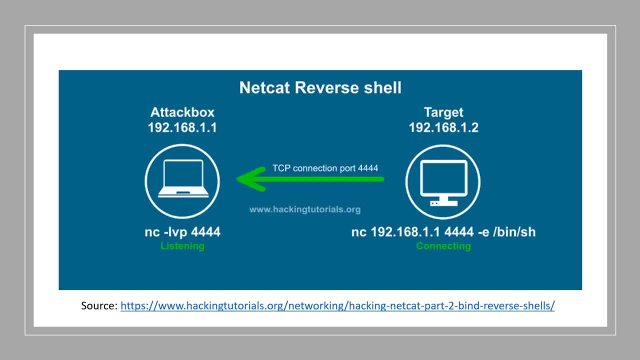 we're going to see. And then we're going to define different types of payloads we're going to see. So let's first start with the shells. The most common shell you're going to see is what is called an reverse shell. Now, in this example, it is using a tool called net cat, which you're going to see. 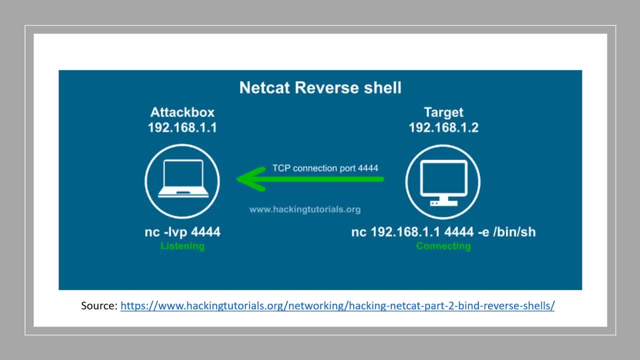 here shortly And a shell. all a shell is is access to a machine. So when we say we pop a shell, that means we get access to a machine Now, reverse shell. reverse shell means that a victim connects to us. Here you see, it says target connecting to attack box And you may get asked. 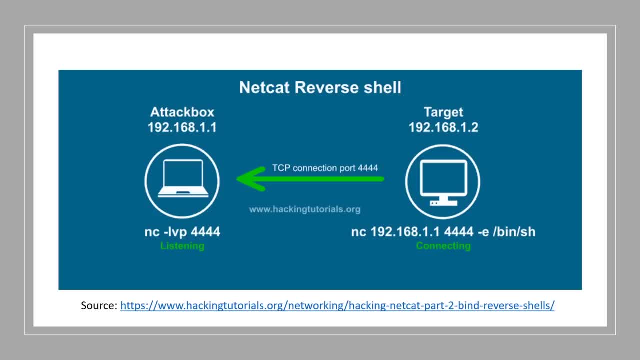 this question about shells in an interview. What is a reverse shell? What is a bind shell? So reverse shell means again, a victim connects to us. you see that it says target is connecting, attack box is listening. So what's happening here is that on the attack box you can see that we 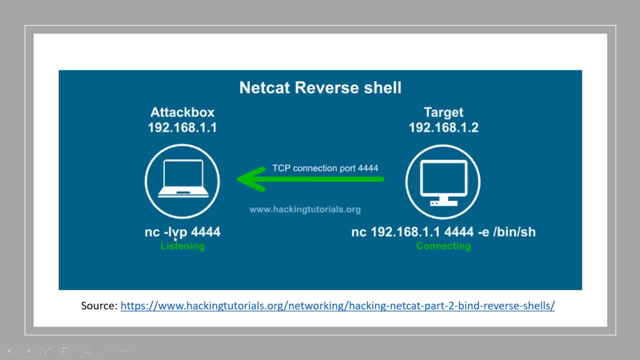 have a net cat. this is NC And we're just listening on a port here. LVP means listening, verbose port. So we're listening on port four, four, four, four. that means on our machine. we're opening up that port. when we use net cat On this machine, it's going to say Hey. 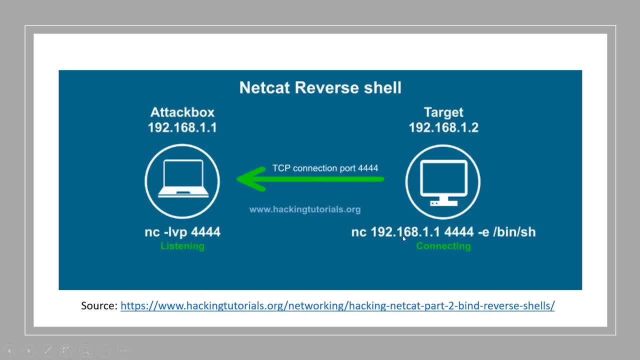 net cat. I want to connect to this IP address here. I want to connect to it on port four, four, four, four, And when I do that I'm going to establish this bin shell here. So I'm going to execute bin shell, which is a Linux machine. If this was Windows then it would be commandexe. 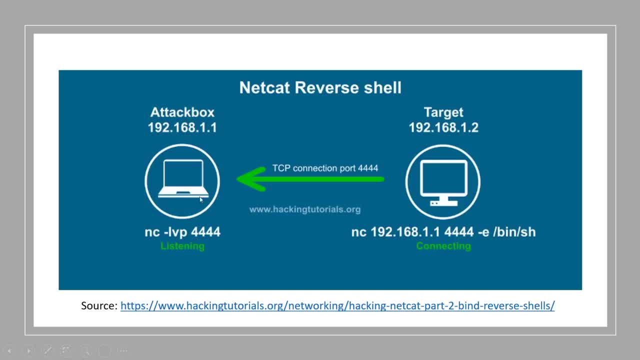 So what we're going to do is we're going to say, Hey, let's connect over here, And this is going to connect. So all we're going to do with reverse shell is we're going to listen. Now, with the bind shell, a little bit different, We have our attack box and then our target. So, with the 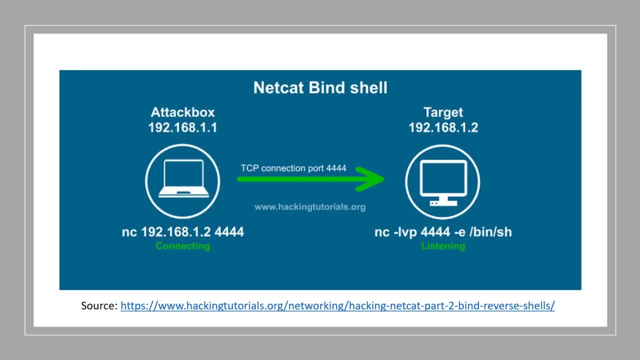 bind shell. we actually open up a port on the machine, then we connect to it. So we fire off an exploit, the exploit goes in and it opens up a port And then it's listening for us to connect when we connect on that specific port to that specific machine with net cat. 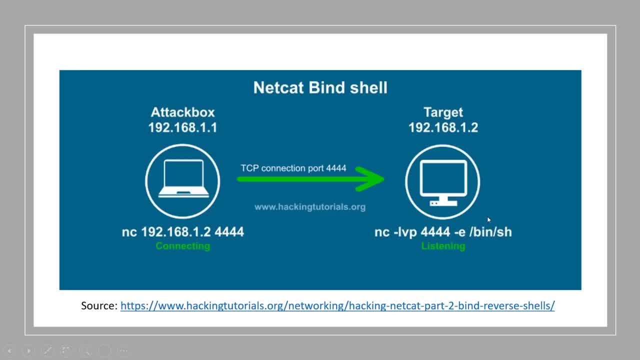 Then we're going to go ahead and get that shell And on this side it's going to execute for us that bin sh. Now, if we go back, same thing here. we're going to send some sort of exploit that's going to talk back and say: Hey, I want to. when you exploit this, go ahead and just connect to. 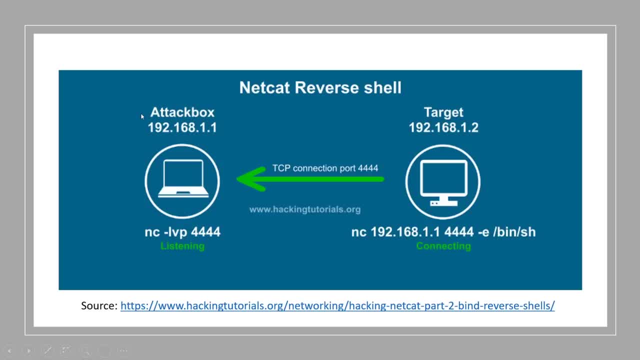 four, four, four, four on this machine. Now this is going to come together very clearly when we get into our exploit development part here in just a little bit. But all you need to know right now is that a reverse shell means the target connects back to us. A bind shell means we connect to the. 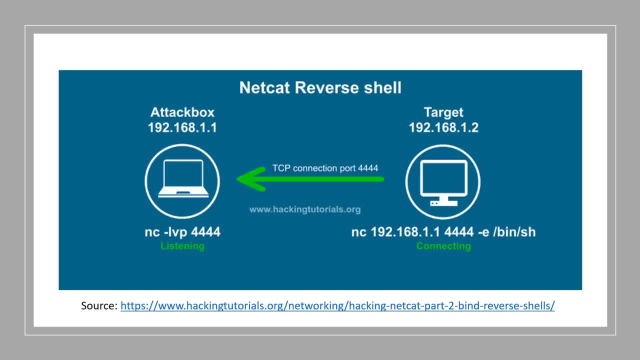 target. Now a little bit more about reverse shells. you're going to use reverse shells 95% of the time. There are instances where you're going to use bind shells. bind shells, most likely, are going to be on an external assessment, If you think about it. or reverse shell, you're sitting. 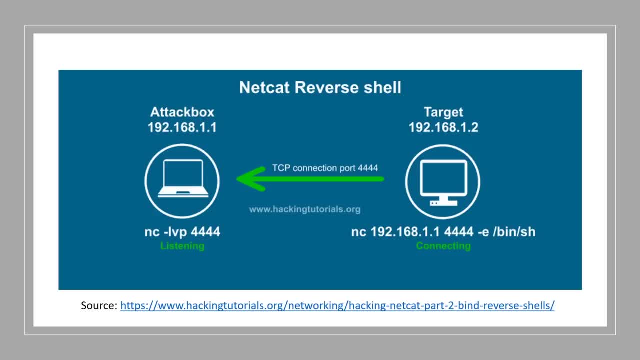 in your home network And you are sitting on a VM. in that VM is using an internal IP address, is talking out NAT, it's going through your public IP address and you're attacking a target. Well, how are you going to connect that public IP address of the target back to yourself on an internal IP? you're 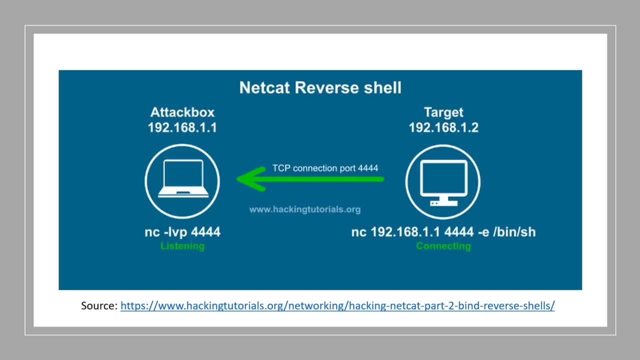 going to have to set a port forward or port trigger on your firewall to talk into that specific machine. It's a little bit of extra work. you're opening some stuff up on your side. The other idea is to say, Hey, bind shell, why don't I just go ahead and connect to that internal IP address? 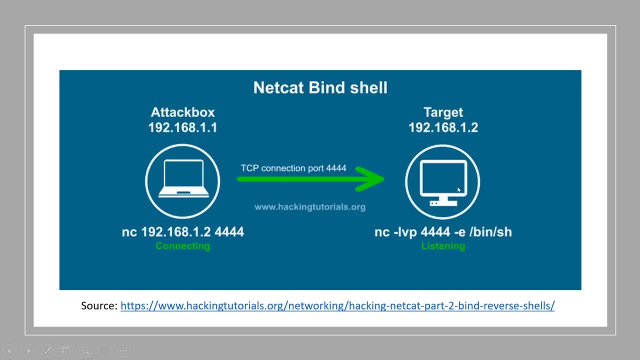 And it's just going to run a standalone server and say, Okay, I just want to open a port for you in my private IP address. You're just going to go ahead and open a port up on that target. I'll not my way through my public IP address and I'll just connect to that port. It doesn't care what. 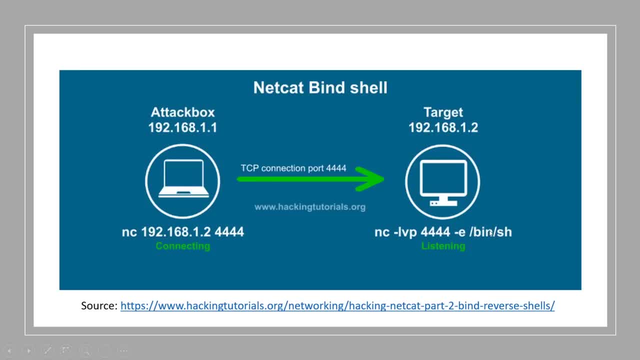 IP address you're coming from. you see, it's just listening, So we can come from any IP address and connect to that port on that machine. So this is where bind shells are useful, when we have to bypass some sort of firewall or just makes sense. Sometimes a reverse shell just doesn't work And 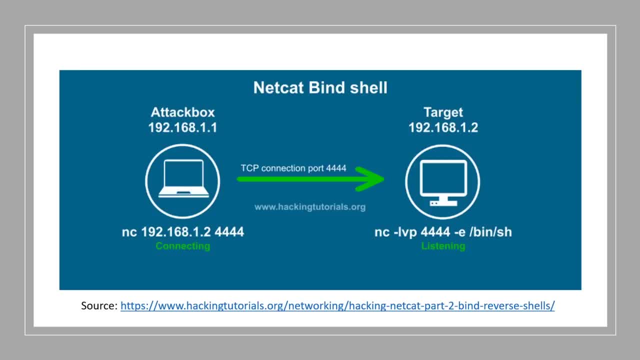 we have to use a bind shell anyway. So we have to think about the connection and how it's getting of the time, especially because you're going to practice a lot in labs and you're going to do internal assessments as well. Most of your shells are going to come in the form of reverse shell. 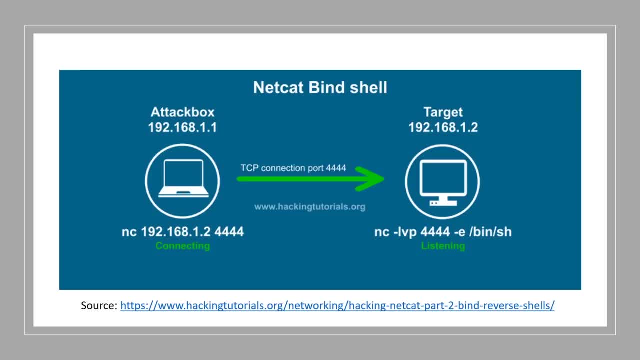 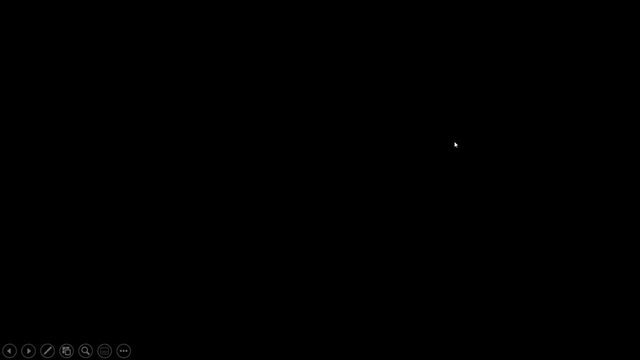 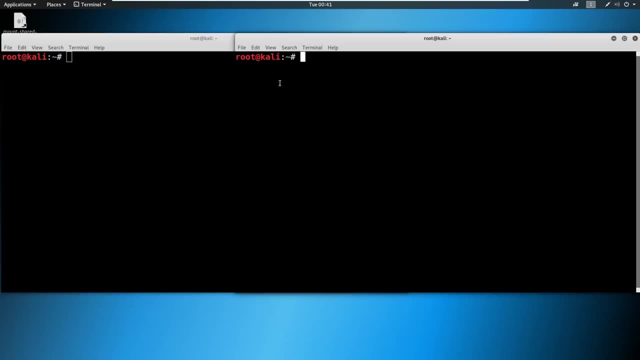 However, bind shells do exist and you should know what they are as well, And, again, for an interview, you should know the difference. So, before we finish here, let's go ahead and take a look at what these look like, And I'm going to log back into my machine And I've got two things. 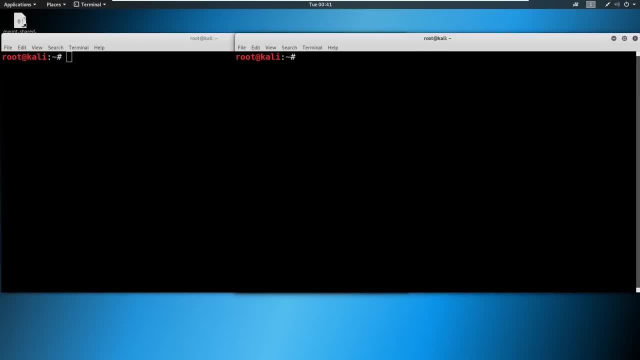 open here. I've got one into. we're going to play victim and we're going to play target right or attacker. So on the attacker, if we have a reverse shell, we're just going to say: net cat. I want to listen And I like to do NBLP, But you can do LVP as well. VLP, it doesn't matter what order, I just 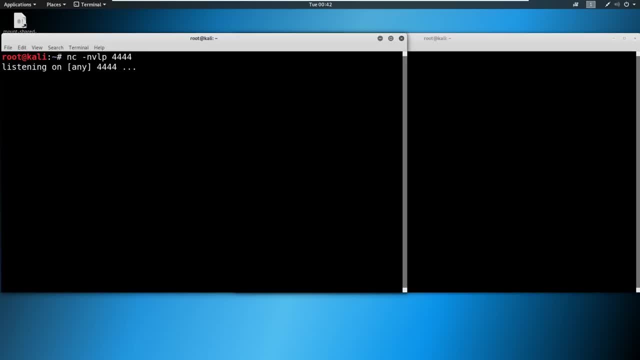 do the NBLP and all fours. So now we're listening on any, on all fours, right? So here we're going to say, on the victim screen we're going to say, hey, net cat, I want to connect and this is a self. 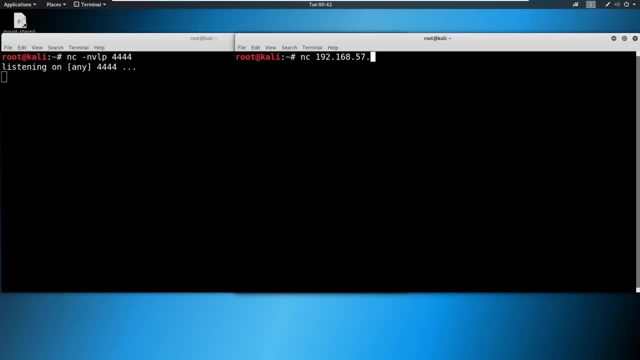 connection, But still, I want to connect to the victim machine or I want to connect to my attacker from the victim machine And our attackers IP addresses 139.. They've got 4444.. Open, let's establish that connection And we're going to offer them bin bash when we do. And here's that. 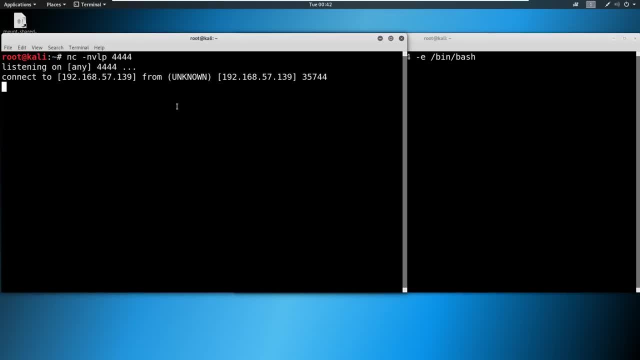 connection. So this is a reverse shell: we were listening as the attacker And then the victim connected to us And then we could say something like Who am I? and you could see root and then hostname Callie, and we have a connection And we offered up that bin bash here. So that works. 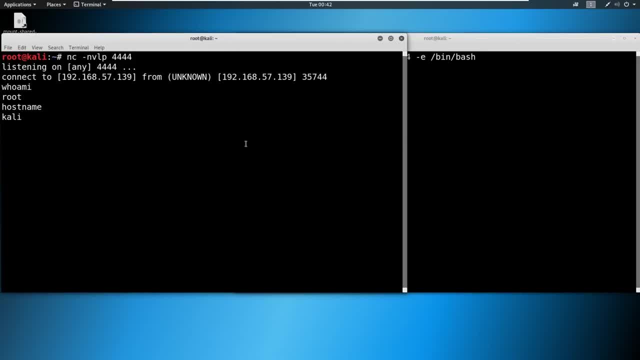 So that is an example of a reverse shell. So I'm going to Ctrl C, this connection, kill it. it dies over here. Now let's say we wanted to flip the script and we want to bind shell. Well, now, guess who needs to be listening? Now, in this instance, we're going to be listening. 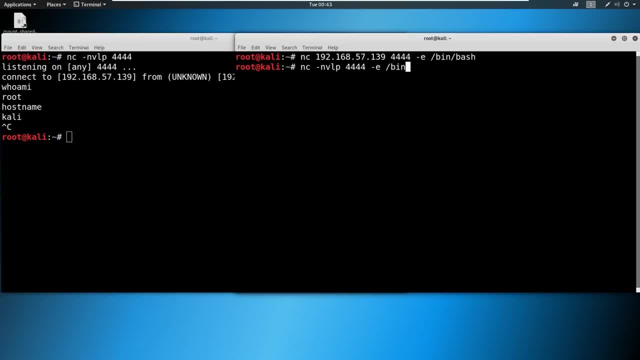 and we're going to be offering up the bin bash because we are the victim. Okay, so we still have to offer up whatever command line we are going to have here Now. all we have to do as the attacker is connect to our victim And we have the same connection. 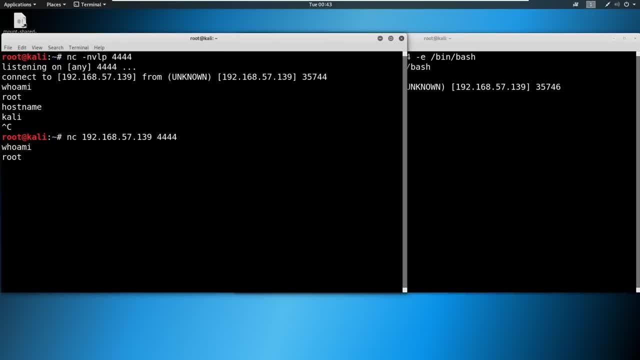 you see, the connection happens here. Who am I root hostname: Callie. So that is the difference between a bind shell and a reverse shell. Remember, reverse shells are most commonly used, but bind shells are important. Again, just a hammer at home, reverse shell means a victim. 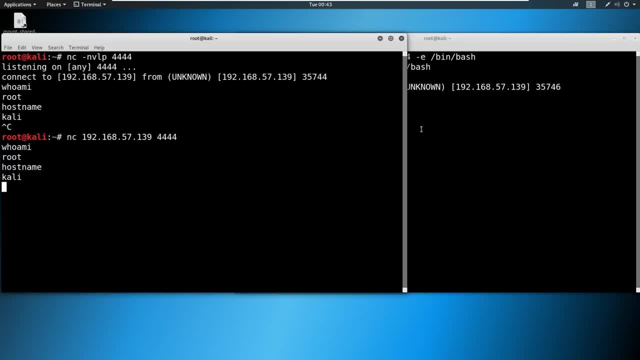 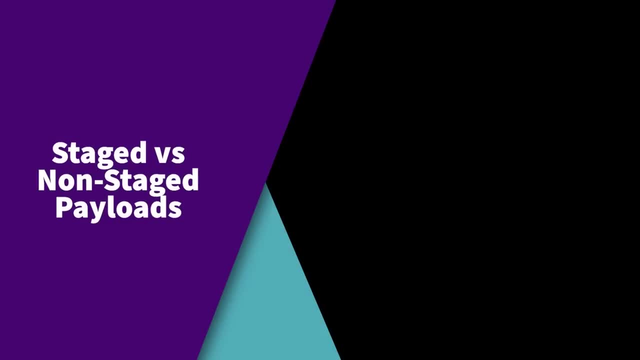 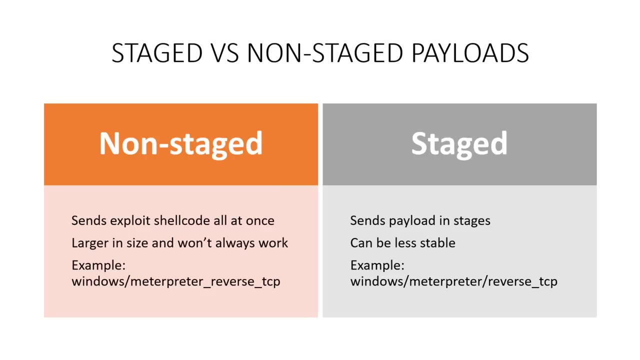 connects to us. bind shell means we connect to a victim. So I'll catch you over in the next video. when we talk about staged versus non stage payload, Now let's talk about staged versus non staged payload loads. And before we do that, we must know that when we're talking about the status of your command, 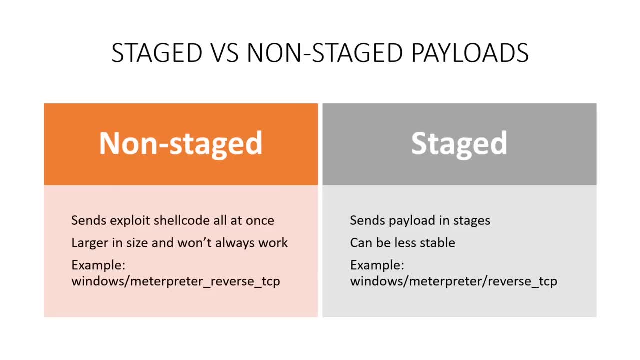 if the common comma or activates the hotkey Interpass л is in line two, this tells us the hashtag. Before we do that, we must talk about a payload. So a payload is what we're going to run as an exploit, And when we run that exploit it's called a payload. we use different types. 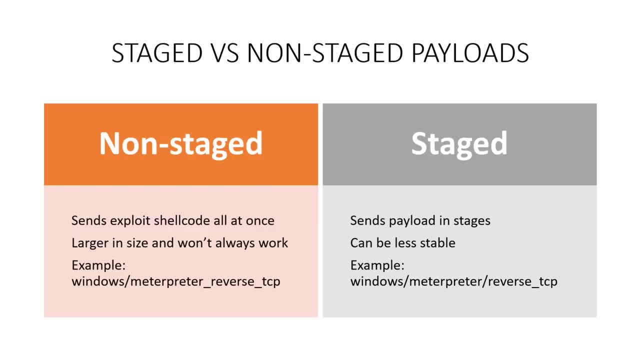 of payloads, depending on what it is. So you might see a Windows type payload or a Linux type payload or easy see on the screen. meterpreter type payload. there's Python, there's all different types. there's like 500 and something that we saw in Metasploit alone, And these 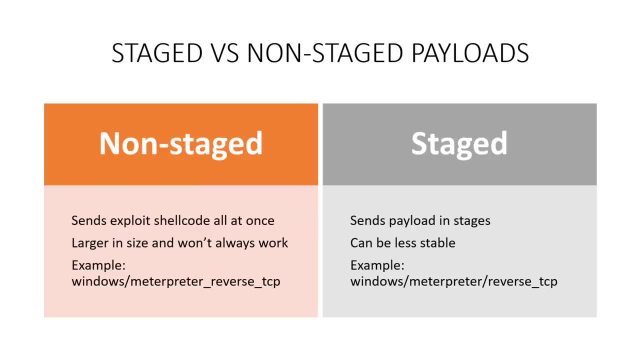 payloads are what we use to send to a victim and attempt to get a shell on the machine. Now it's going to make more sense as we go. it's okay if you're still a little bit confused on all this. There are two main types of payloads that we need to pay attention to. There is 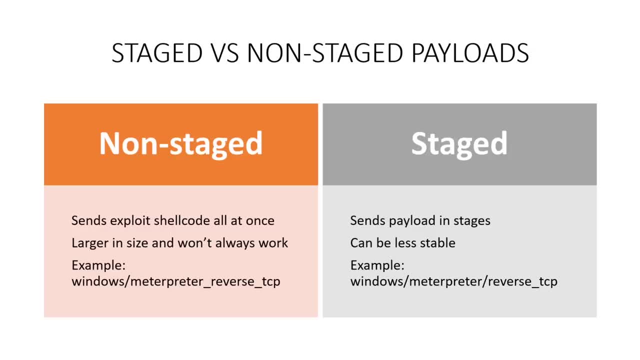 what we call non stage and what we call staged. Now a non stage payload sends the exploit should be a non stage payload. Now a non stage payload sends the exploit should be a non stage payload. Now a non stage payload sends the exploit should be a non stage payload. 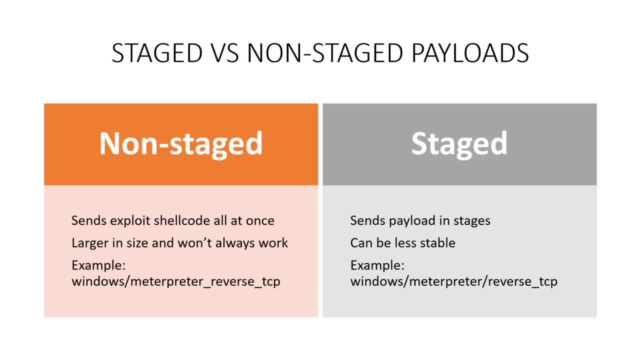 shellcode all at once. where a stage payload sends it in stages, the non stage payload is larger in size, and it doesn't always work where the stage payload can actually be less stable. So each has its con And we have an example of it, And this is really what I want. 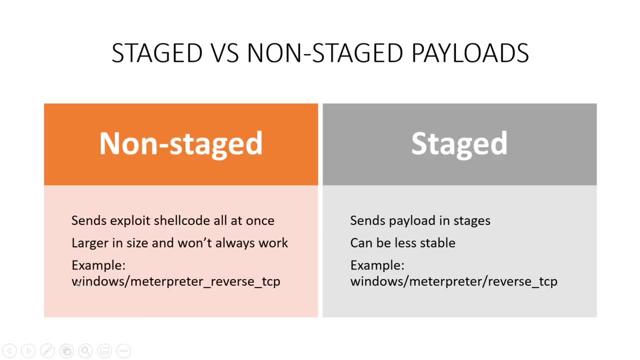 to point out is we have this non stage payload and we have a stage payload and you see the one difference between the two. All it is is a forward slash. So when we see these and we're using something like Metasploit and we have to, 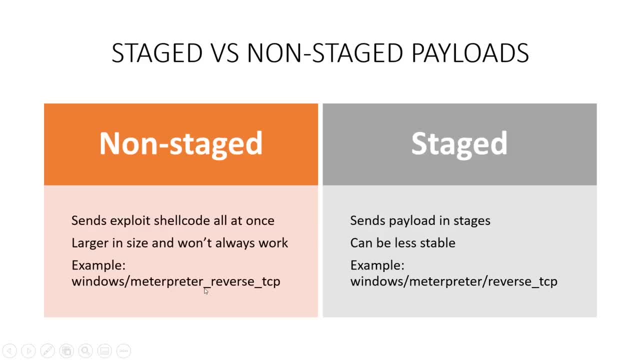 pick out a payload. If we see something like meterpreter- underscore- reverse underscore TCP, this identifies that this is a non stage payload. we can ignore the windows here, But here we see meterpreter forward slash- reverse underscore TCP. This means we have a stage. 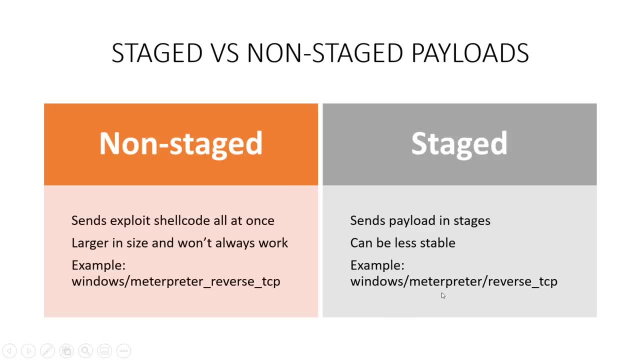 payload. what's happening? it's saying hey, stage one, stage two. What's happening here? it's saying hey, let's send this all at once. So this is going to become very important very quick, as we will attempt an exploit here very soon. and it's: 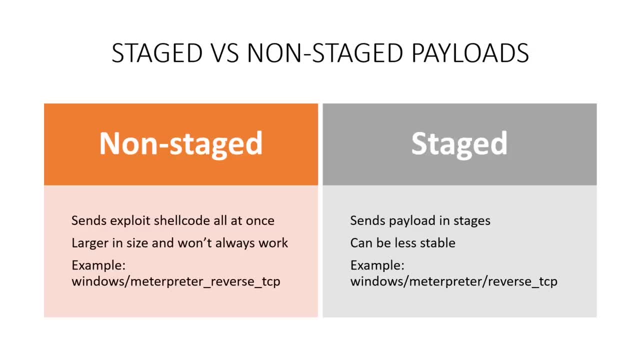 not going to work And then we're going to change the payload and it's going to work beautifully. So understand that. what the really the takeaway is: if you have a payload that does not work, maybe try the other, other type of that payload. If you see something like: 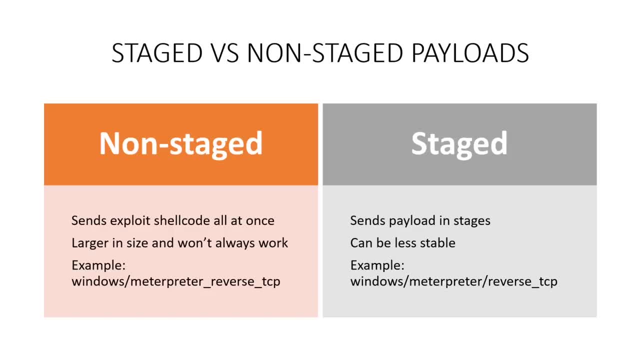 reverse TCP, which is a reverse shell, by the way, over a TCP connection. if you say, hey, I'm going to send this stage reverse TCP. it's not working, All right, let me try to send a non staged reverse TCP. Okay, that's not working, But I'm sure my exploits right, so maybe I send a. 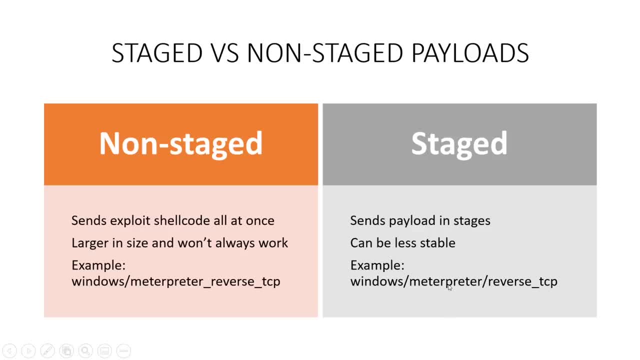 bind shell instead of reverse shell here, and I'll send a bind shell stage and then non stage And we just keep trying until we find a payload that works. Not every payload is the right payload And we have to find the one that works for us. So the takeaways: remember the forward slash. 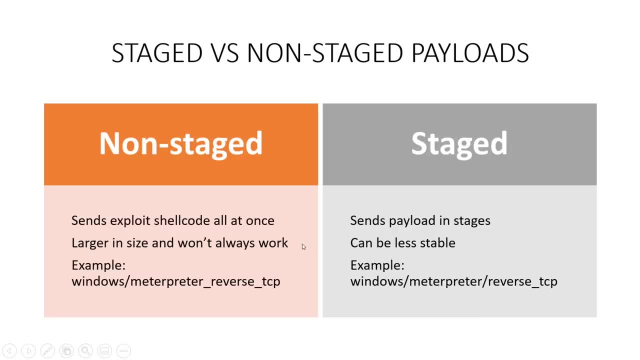 remember the slight differences between non stage and stage And remember if your payload fails but you think it's the right exploit, maybe change your payload. So we'll see that here very shortly as we start to get into exploitation in the next few videos. 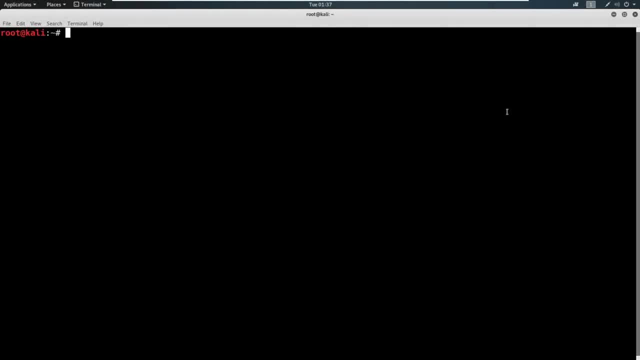 Oh, I am excited, And let me tell you how excited I am. This is not the first time I've recorded this video. This is actually the second time recording this video, because the first time I forgot to hit the record button, So now it's. 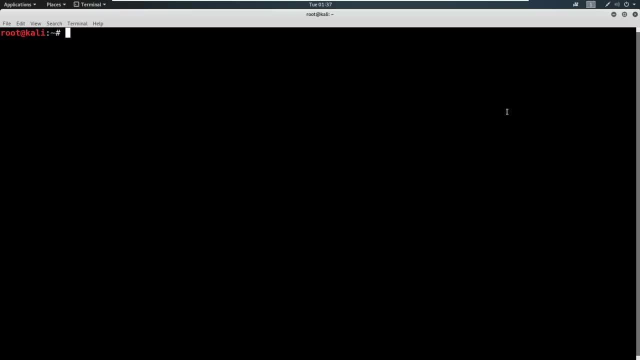 blinking red right in front of me, guaranteed recording. And I'm still as excited, even the second time walking through this. I'm so excited because this is what we've been building up for, This is everything we've been doing: the scanning, the enumeration, even the Linux and the Python. 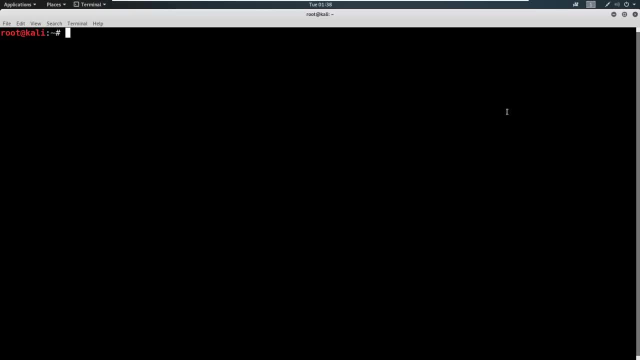 this is all building up to this, And now we're ready to exploit. we're going to get our first shell. we're going to pop our first shell today, And I'm so excited for both of us. So what we're going to do is we're going to run Metasploit for this one, And 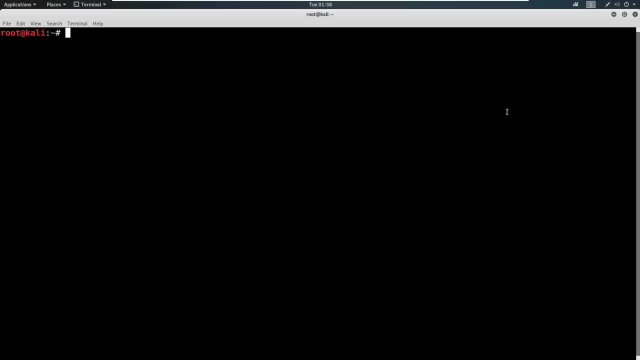 Metasploit. it's a little bit automated, but that's okay. In the next video we're going to go ahead and cover it manually. So what we're going to do is we're going to attack SMB here And with SMB. 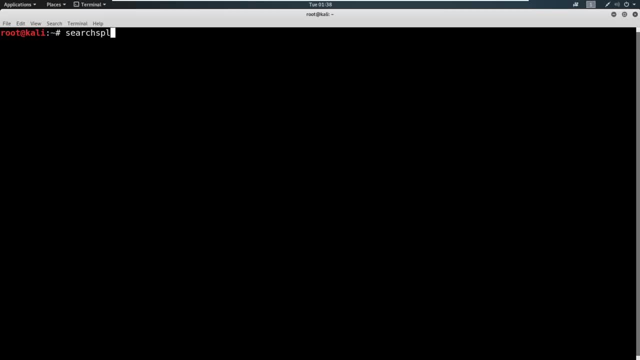 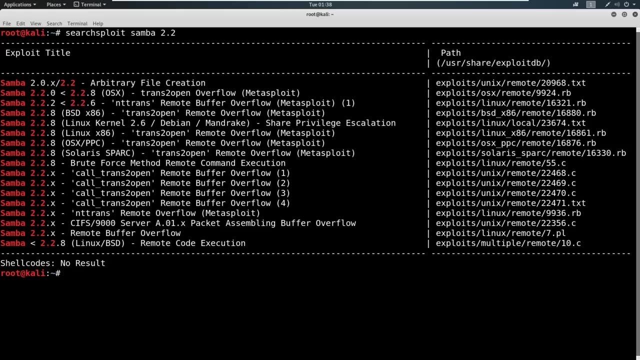 what we're going to do is, if you don't remember, search splite Samba 2.2,. we found Samba 2.2, we found Samba 2.2, point one a. We searched around, we went out through the interwebs, we did search. 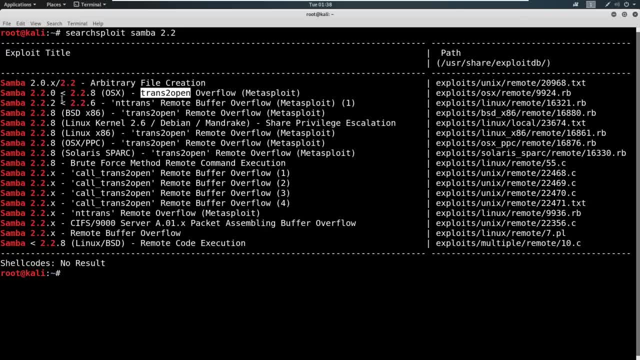 poli and we kept seeing this Trans. two open show up Like here and here, here, here, all down here right, repeatedly, and it meets the criteria. everything seems to make sense. It had that IPC anonymous connection as well. So I think, I think this is a winner And we're gonna go ahead and 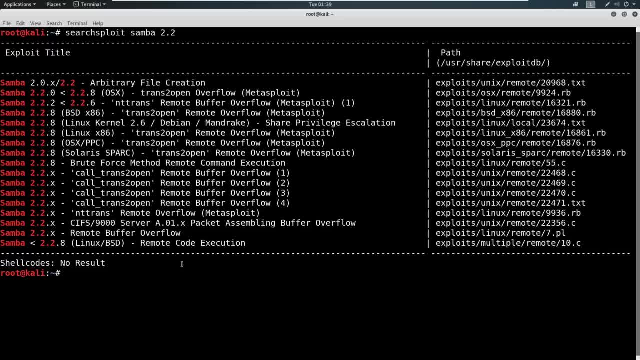 give it a try. So I'm going to copy this and we're just going to go ahead and type in MSF console and load up Metasploit. Once Metasploit loads, we're going to go ahead and just search for this guy and see if we. 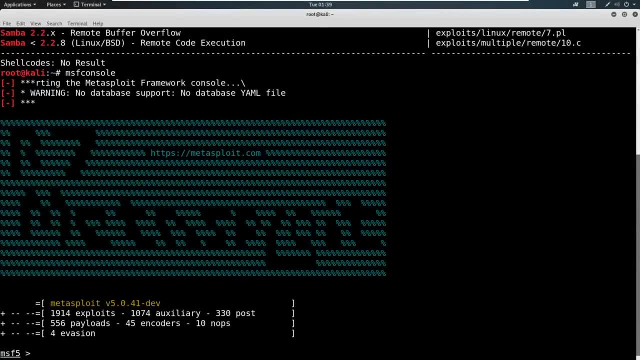 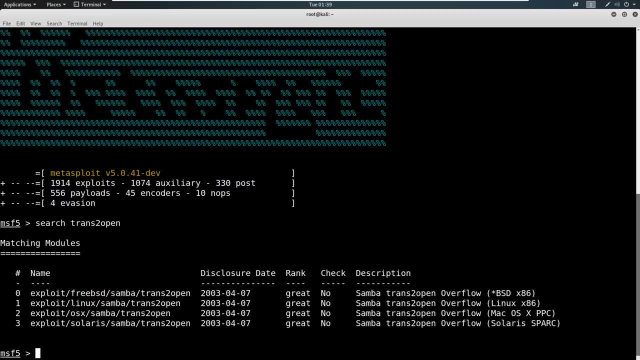 can't find it Now. we know it exists because we did find that handy dandy rapid seven website that said it did, So we're going to search it here and we're given four options. Now these are all operating systems here, but we have been good enumerators and good. 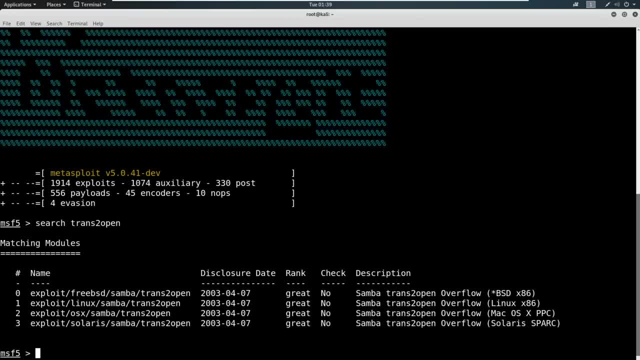 investigators, researchers, information gatherers, et cetera. We could have willy nilly. just saw one 39, said Hey, I'm going to try to find exploits against it and never looked at any other ports. but that's not us. 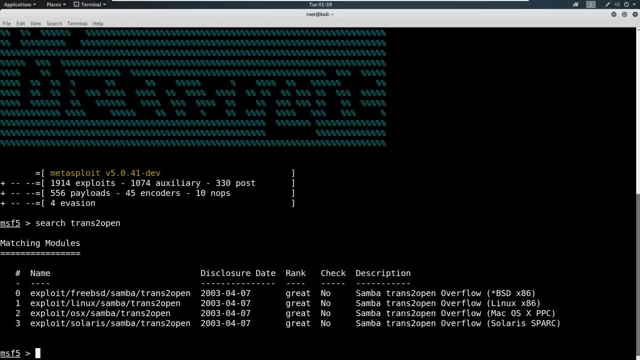 We went out to port 80. We saw that it was running red hat. We discovered Linux on the machine. So we know we're going to pick the Linux module. So we're going to say: use one as that corresponds. So we're going to say: use one as that corresponds. 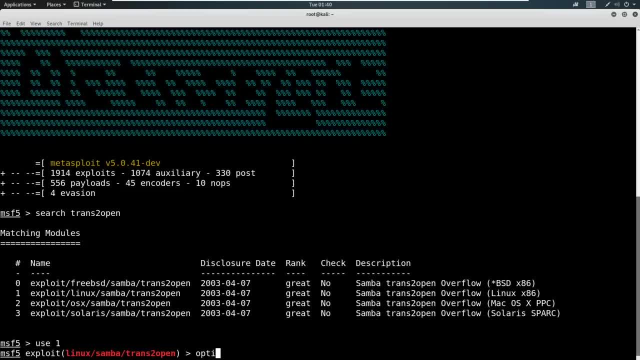 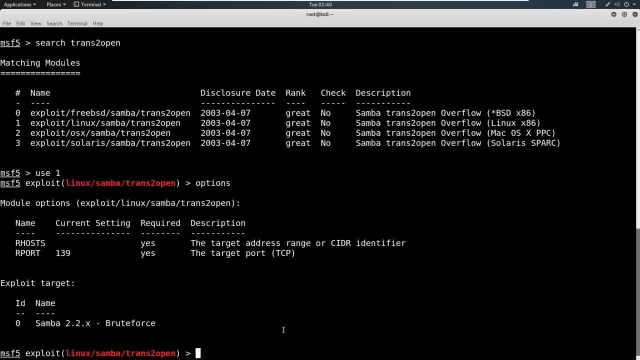 So this module here, and then we're going to type in options and all we have to do is set a our host. So remember, our host stands for remote host or the victim that we're attacking. So we're going to say: set our host and 1, 9, 2, 1, 6, 8, 5, 7, 1, 34.. 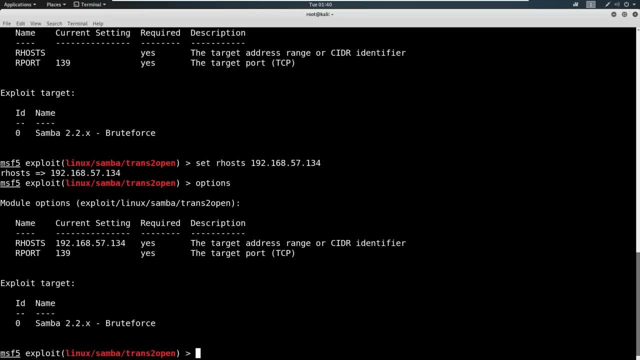 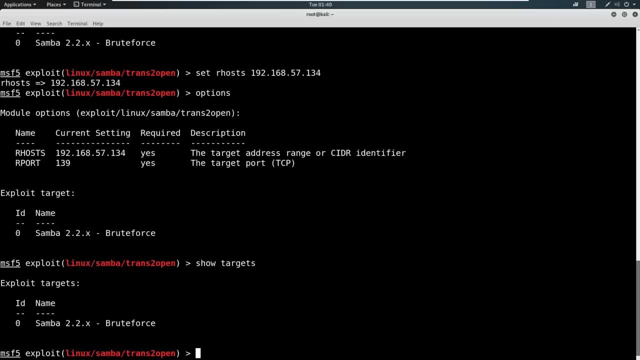 And we're going to say options one more time. Make sure that that actually sat in there, and it did. Now, one thing I like to do is type in show targets. Now, there are no targets here, but, as you're going to see later on in the course there, 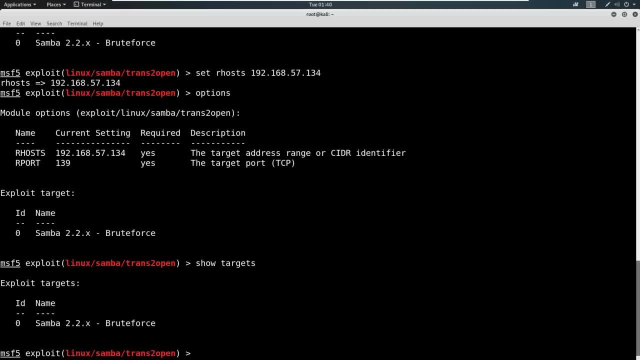 are often targets that we have to pick from. Not always is the first choice that's auto selected right for us, But in this instance there's only one choice, So it's the right choice. So now we have two options. Both are going to do the same thing for us. 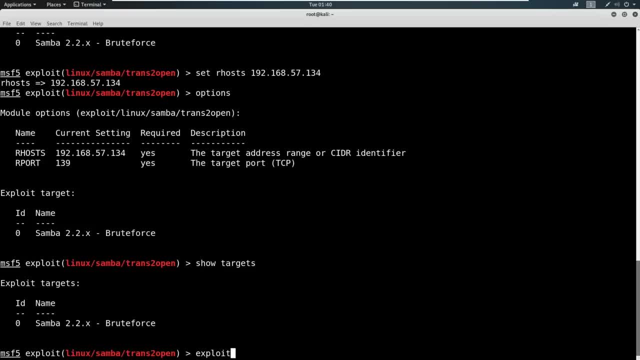 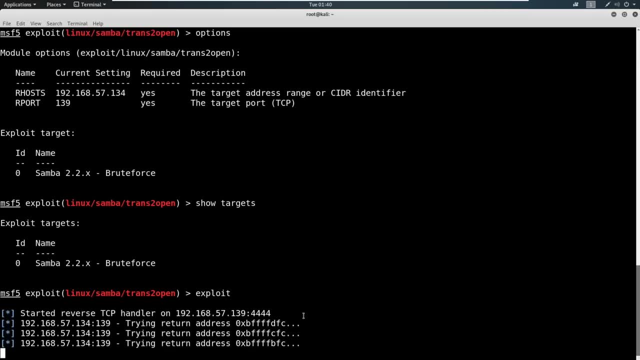 We can type in run or we can type in exploit if we want to be cool. I want to be cool, Let's type in exploit. So we're going to run this and it's going to start this brute force attack, Okay, And it's going to start opening shells and closing shells. 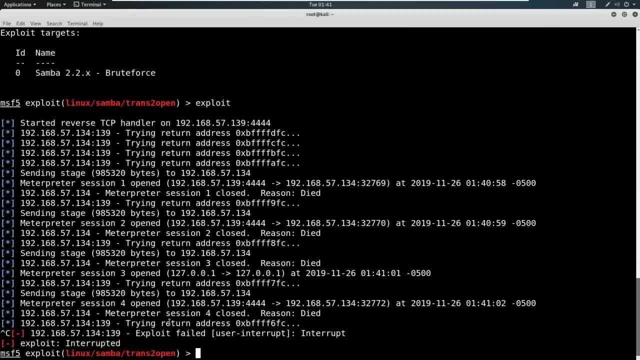 What is going on. So let's control C. if yours is doing this, go ahead and control C. interrupt this. Let's talk about what's happening. So you see, it's trying this brute force attack. It's trying different, different return addresses here. 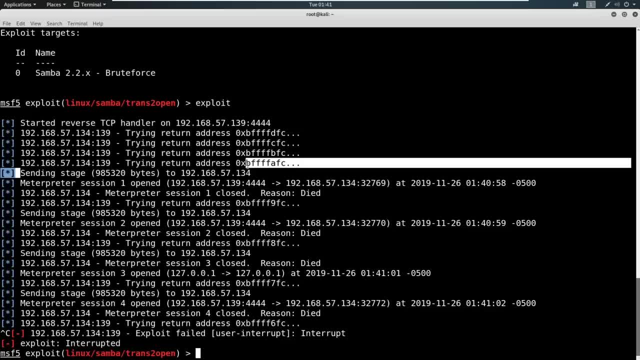 And finally it lands on one that works and it says, Hey, I'm going to send this stage. This is always a good sign, by the way, sending the stage. Then it says, Hey, I've got this meterpreter session open because our payload has worked. 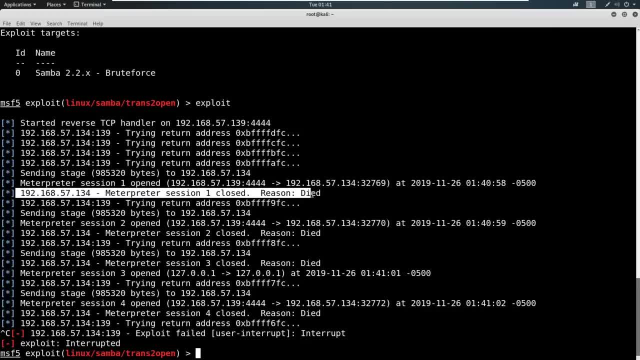 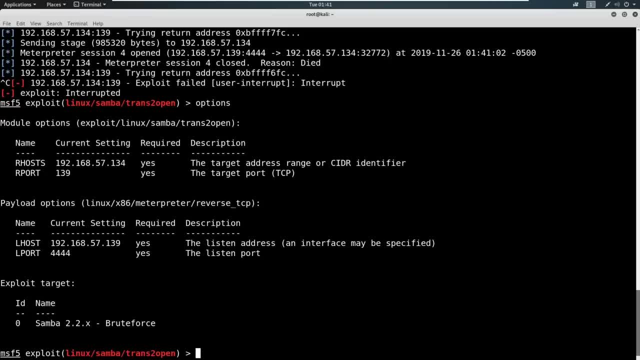 Now, you don't see this the first time you do it, but you see it the second time because Metasploit says: Hey, if your payload is not working, maybe the payload is the issue, And I'm going to give you payload options this time around. 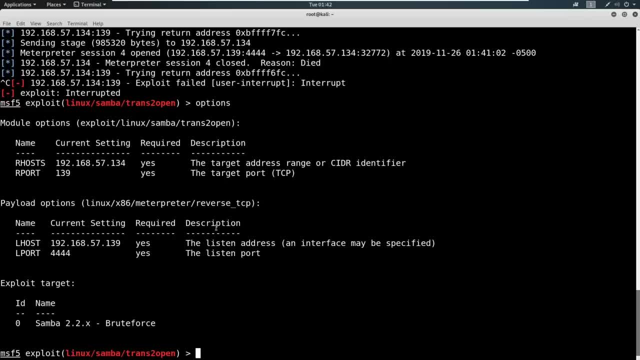 Now we see payload options here in the middle. That wasn't there before. We can see that we're running Linux x86 interpreter: forward, slash, reverse, underscore, TCP. What does that mean? Well, that means that we are running a staged payload. Couple other things to note while we're in here. 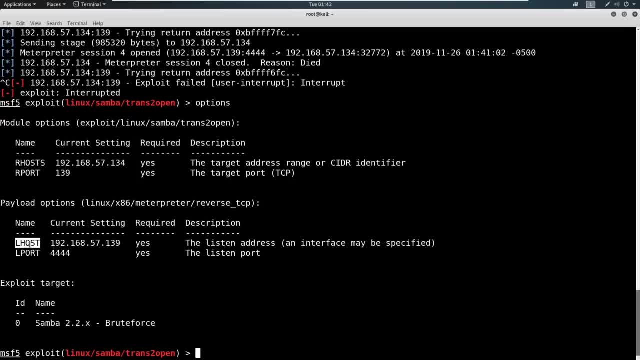 We see L host. That is the opposite of our host. L host is us. We are the listening host, So we sit here and we have our IP address. Sometimes this auto selects correctly, Sometimes it doesn't. In this case it did. 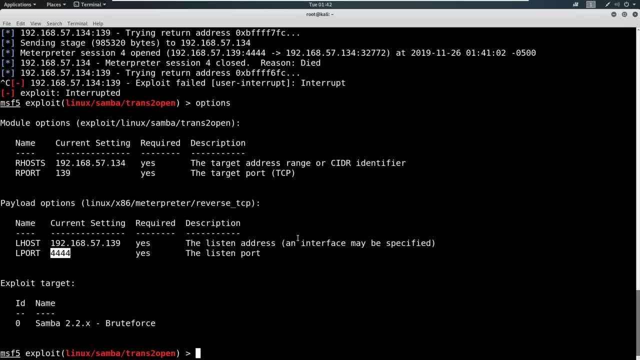 And then we have the L port, which is by default all fours. So that's fine for now, It's fine for these lessons. When you get into actually running this in the wild, all fours is probably going to get you picked up pretty quick because this is a default meterpreter port. 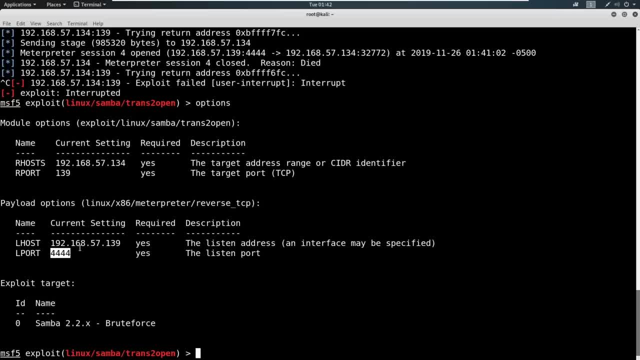 So some connection sees a or some antivirus or detection software sees four, four, four, four open up. This is going to trigger an alarm here, But anyway, for this course You're not going to need to worry about it too much. 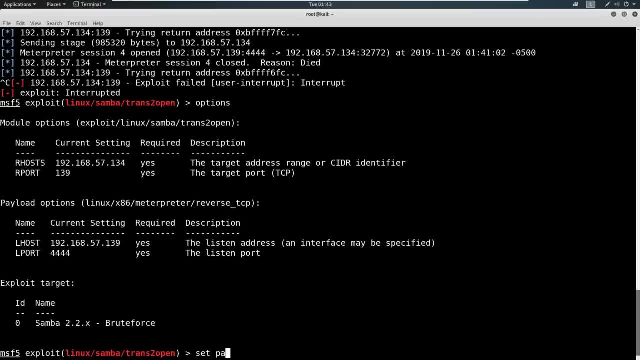 Right now we're going to go ahead and set a payload. We're going to say set payload And how do we know what payload to pick? Let's just start typing out Linux and hit tab, and it auto tabs out the x86 part for. 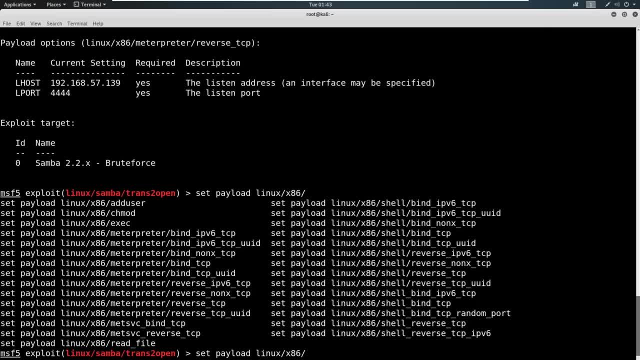 us And then let's just hit double tab. All right now with double tab, That's great. Look at the payload options we have. We've got a bunch Now. we've got a bunch of interpreters, but unfortunately they're all staged payloads. 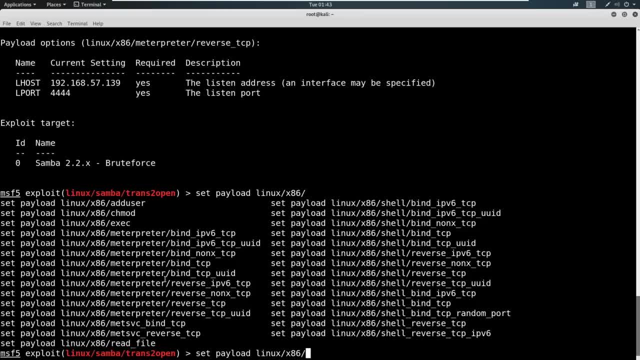 Here. I love a good meterpreter shell and you guys will understand why as we move forward- But as of right now it doesn't look like we're going to be able to use one. We come over to this right column. here You can see that we've got other shells as well. 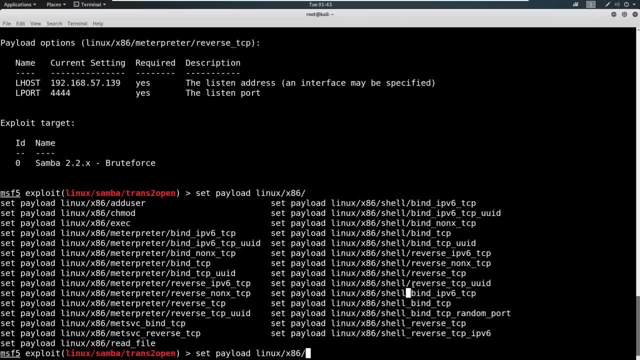 And we come down and finally, down here we've got a few options that are non-staged. So let's go ahead and try this shell reverse underscore TCP right here, And you can just start typing that out, Okay, Okay, So I'm going to go ahead and hit auto. tab complete for you. 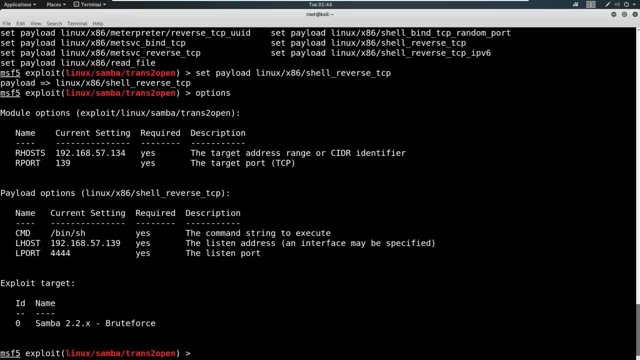 Go ahead and hit, enter, hit options one more time to make sure that this actually works. You can see here that it actually picked up, And now let's go ahead and try to run this and let's see if it happens. Fingers crossed. 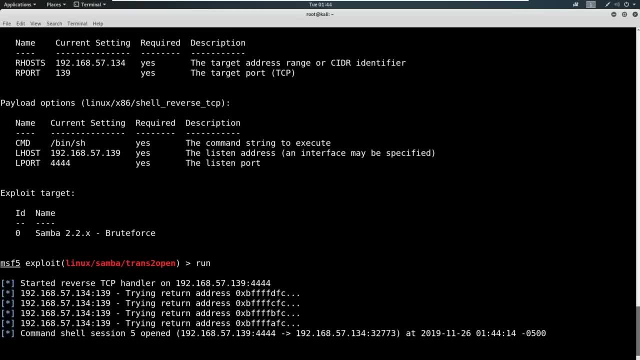 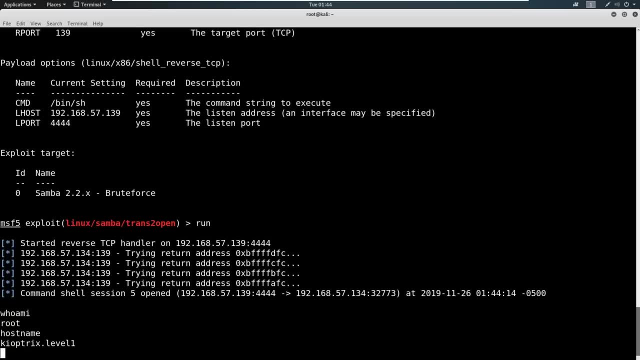 Hey, look at that. So we've got a shell now and it says: command shell session open five. Let's try. Who am I Root? Host name: We have successfully rooted this machine. Root is the commander of the system. We cannot go any deeper than this. 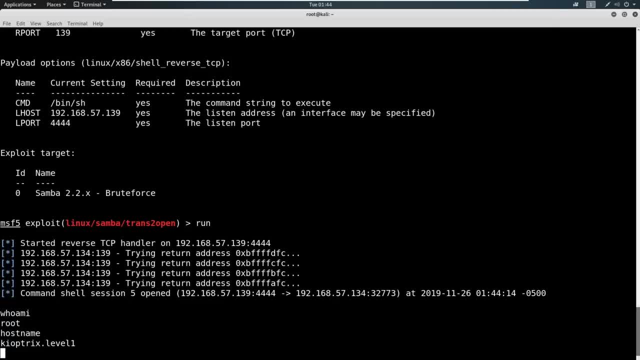 We own this machine. hands down, It's our machine. So congratulations. You have made it this far. This is your first rooted machine. You should be very proud. Pat yourself on the back. You're awesome. So from here we're going to go ahead and we're going to focus on port 80 and 443 and how we can. 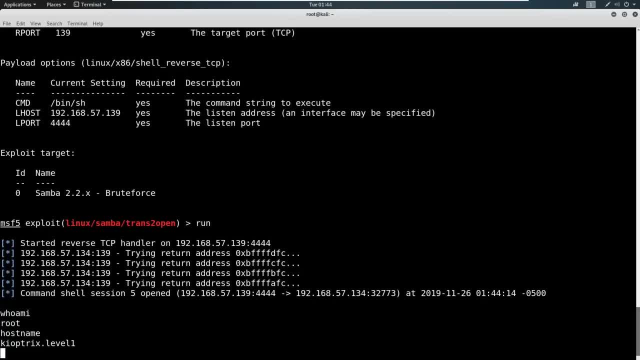 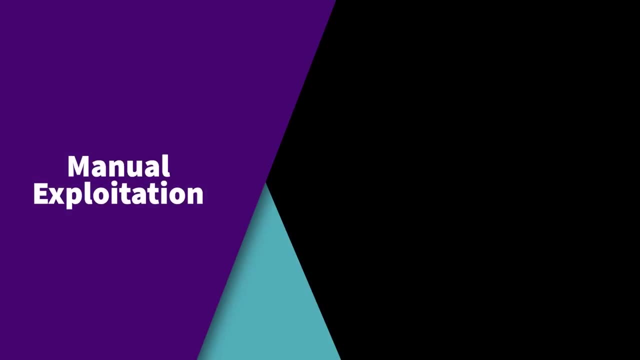 exploit those manually, And then we'll move on to some other exploitation techniques. But for now, congratulate yourself: You have your first shell. I'm very excited for you, So I'll catch you over in the next video as we start some manual exploitation. 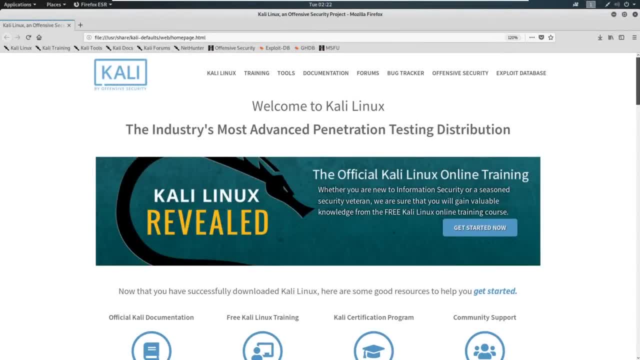 So we have gained root with Metasploit, but now we need to gain root with some manual exploitation. So remember, earlier We discovered that we had an exploit with our mod SSL And we're going to see what we could do about it. 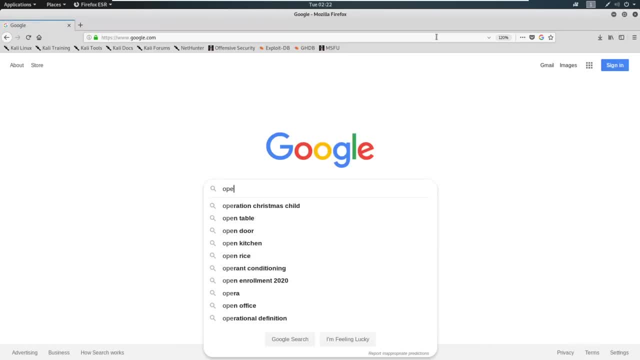 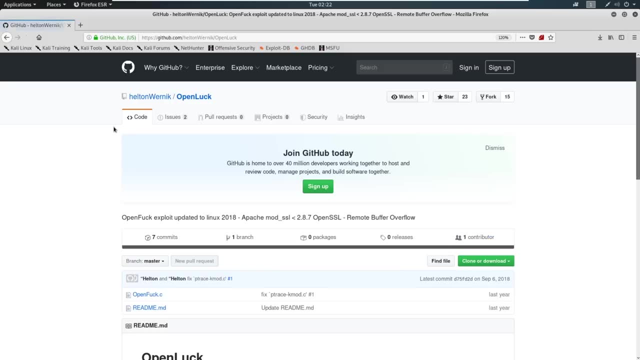 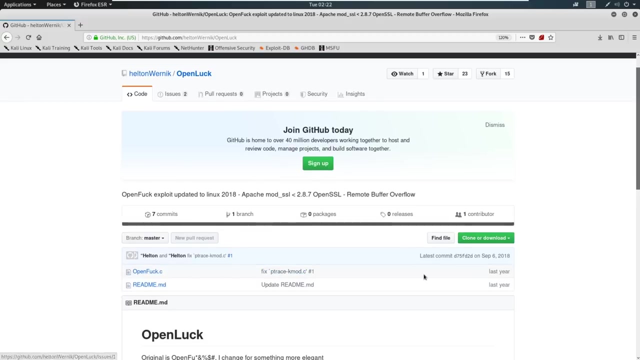 So we went to Google and we researched mod SSL and we came up with something called open luck, If you remember that. So we clicked on this open luck here And this is the same as the one that is out there on exploit database, but it is fixed. 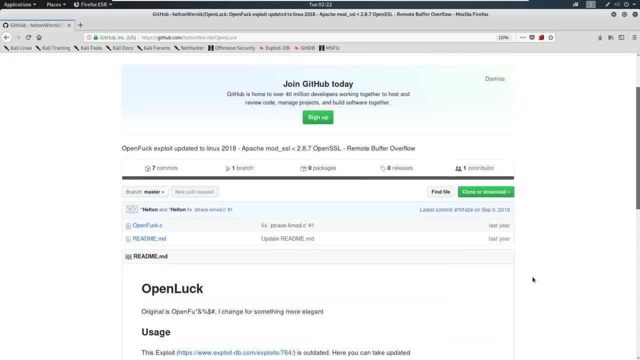 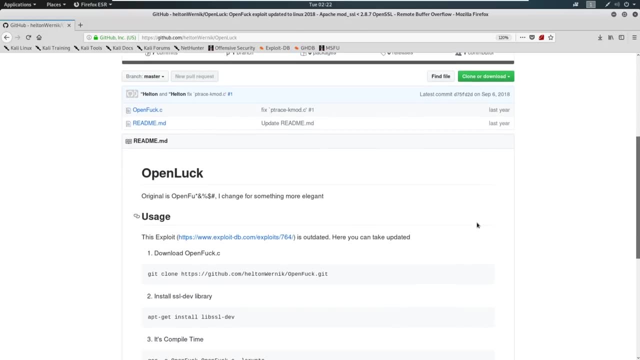 So remember the exploit database one is broken, So we'd rather use this one. That is fixed. So we're going to do is we're going to follow the instructions here And this is very well laid out. So it tells you to get clone this: we need to do an install of an SSL dev library. we 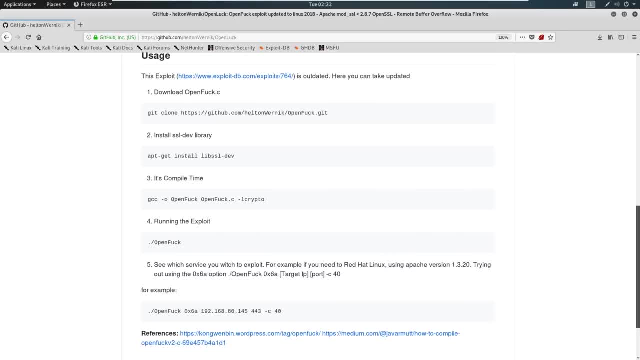 need to compile and then run the exploit. So very, very straightforward. we're going to go ahead and do exactly what it says, And let's go ahead and just copy this first line here, And I'm going to just make this a little smaller: go into a terminal. 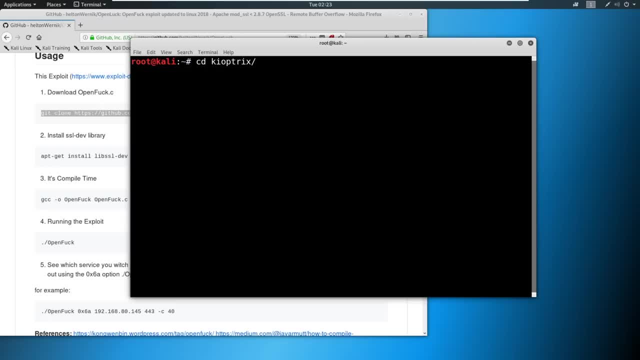 And I actually have a folder for the optics. I'm going to CD into it And then we're going to go ahead and just paste that line And it will get clone everything if we LS. now we see that it is there. So let's CD into that folder, the bad word folder, and we'll LS. 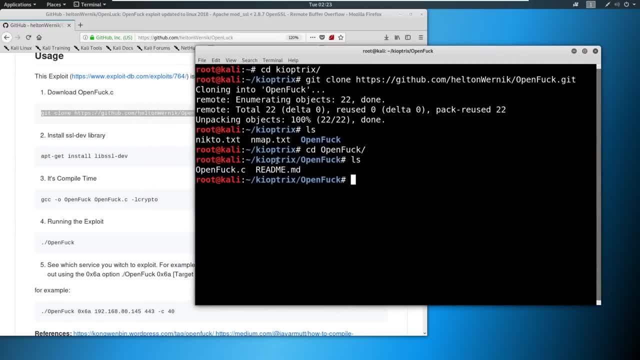 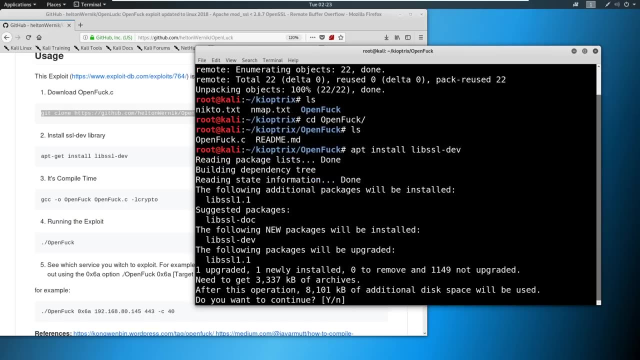 And now you can see that there is just the C file here in the readme. So what we're going to do is we need to paste this, We need to install this live SSL dev. So we're going to say app install and then live SSL dash dev like this: hit enter. 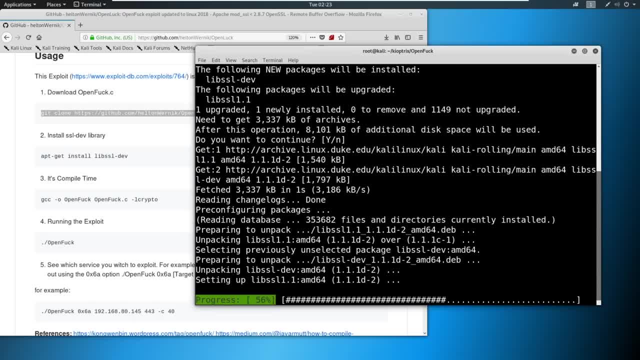 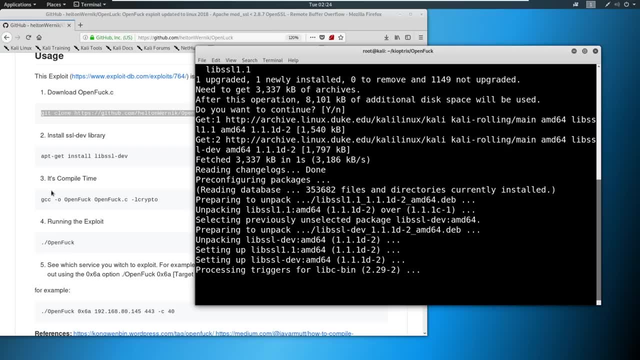 And then just hit enter because it says yes already. this will take just a second to install. And then, once it does this, we're going to use a tool, looks like, called GCC, which GCC is a compiler. So if you've never used C or are familiar with C, we have a C file, but this isn't ready. 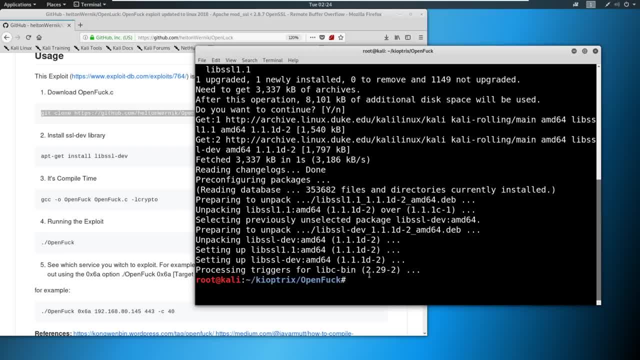 to use. we have to compile that C file in order to actually use it. So that's what we're doing here is we're downloading a little bit of stuff to actually be able to compile that. GCC is built in, and we just needed some other things additionally. 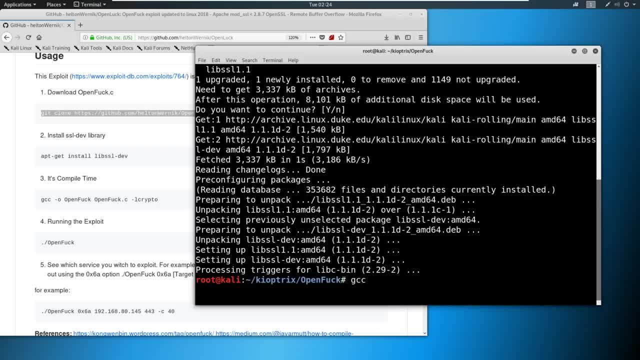 So now what we're going to do is we're going to say GCC And typically you say dash O for the output, so we can call it whatever we want. We'll just call this open And then we'll just specify the file. you can start typing it and then tab out. 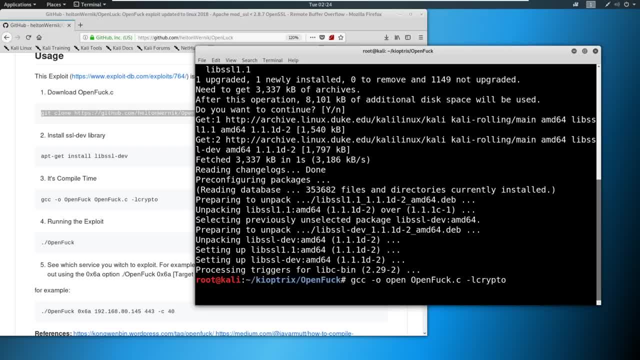 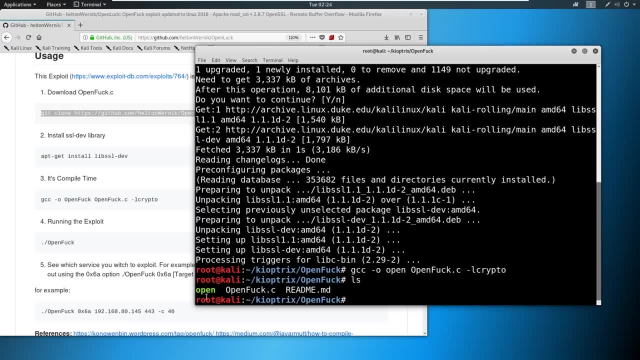 And then it says this L crypto, which is important. Hit, enter okay, and then hit LS. And you see now in pretty green green lighting up and saying, hey, we're executable, We have our our executable right, we have our script that we can run. 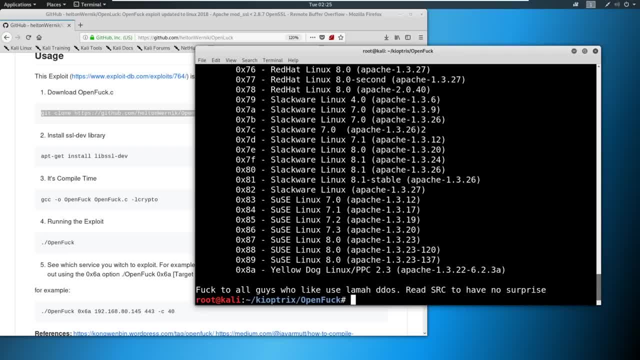 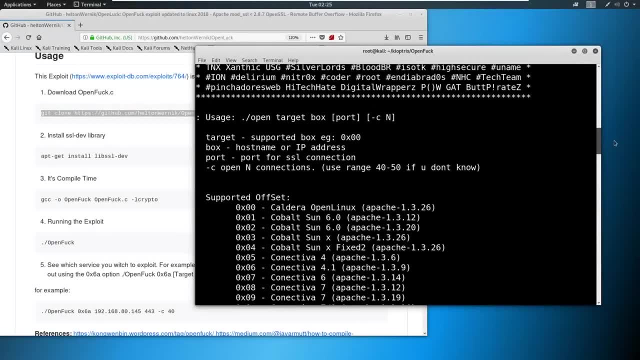 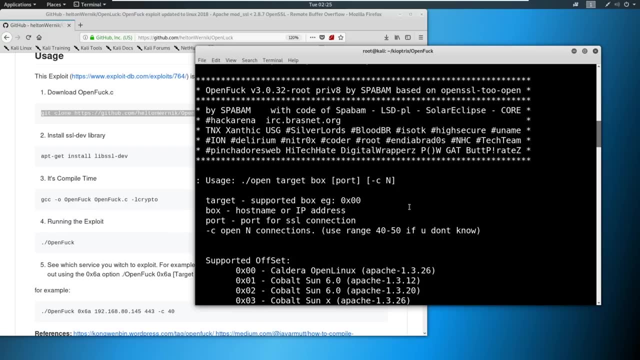 So we could say: dot forward, slash, open and run it. And you can see in here all the different options that this runs against. So you remember when it was brute forcing- The last one when we saw the, we saw the trans to open was kind of doing brute force. 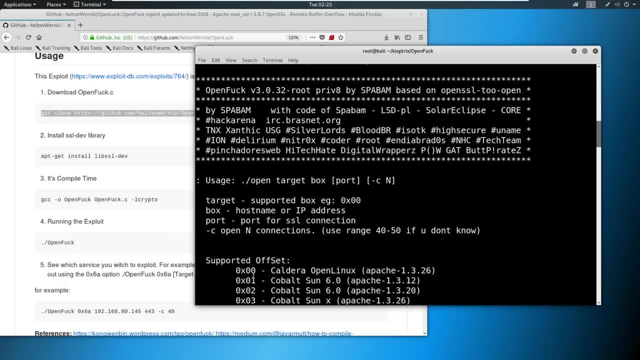 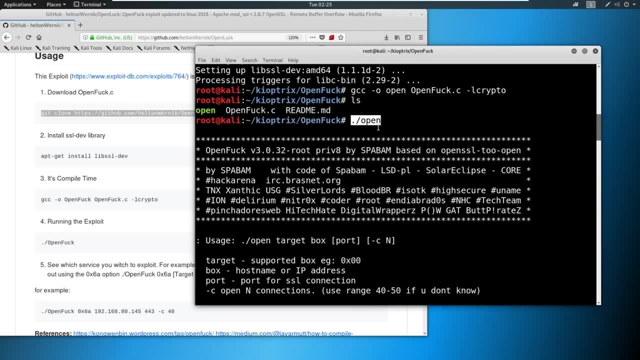 In theory, this is what it could do as well, But here we actually have to pick a return address based on our machine. So we're going to look at the usage. I always like to do the application without any usage to see what the usage is. 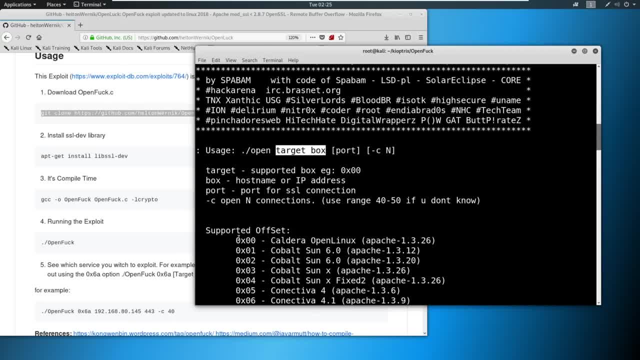 And we need to use target box, which is one of these down here. we need to select a port. maybe It says: for SSL connection. we're not going to be using an SSL connection, So don't worry about that- And then a dash C number. 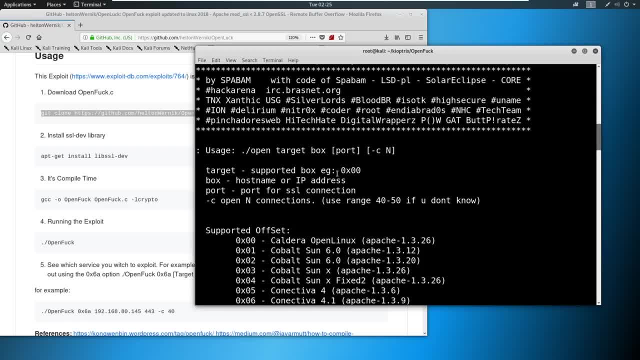 And it says use range 40 to 50.. If you don't know so, our syntax is going to look something like: dot forward, slash open one of these offsets that we're going to pick, And then it's going to be a dash C, probably 40.. 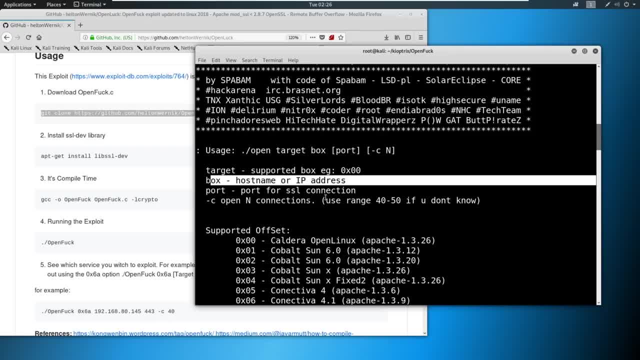 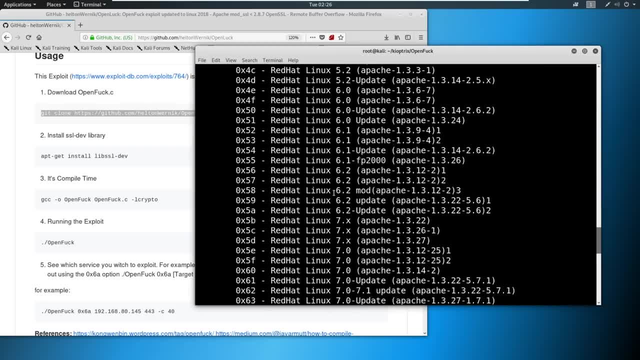 With the box IP address in between. So how do we find what we're looking for? Well, I'm going to go ahead and hit enter. Well, I'm going to cheat just a little bit and tell you guys to scroll down, down, down. 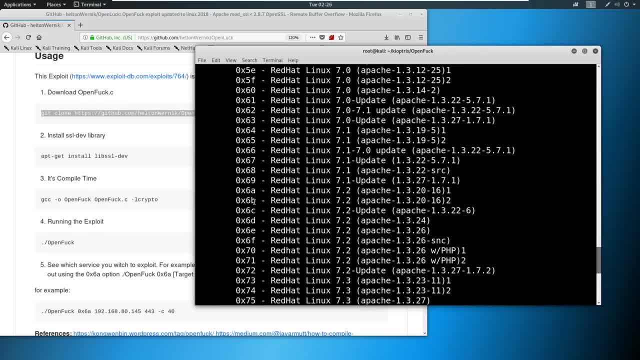 down, down. And if we look at six B here, remember we were up against Apache 1.3, point 20.. See enumeration comes into play big time. So Apache 1.3, point 20.. Now there are two we can run against. 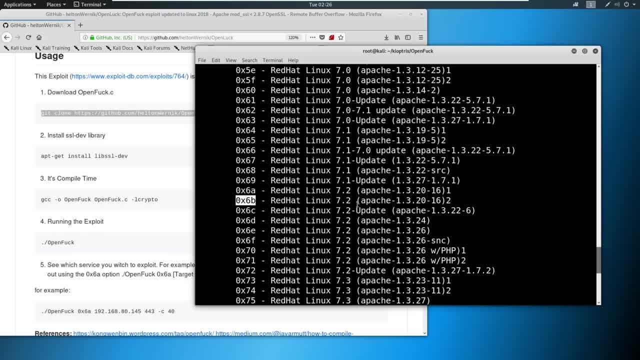 I'm picking this one. I believe it's the more stable one, So we could pick either one, But I would choose B. I think A doesn't work all the time, So let's choose B here And Apache 1.3, point 20 is the indicator. 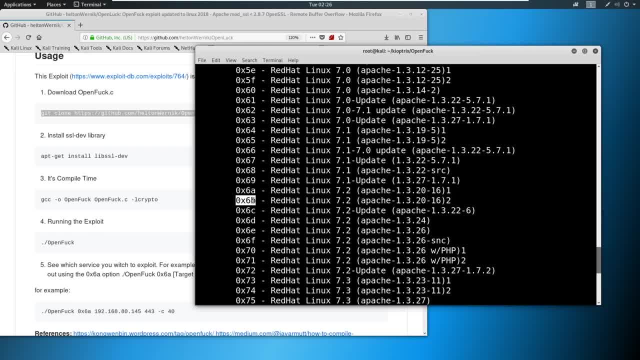 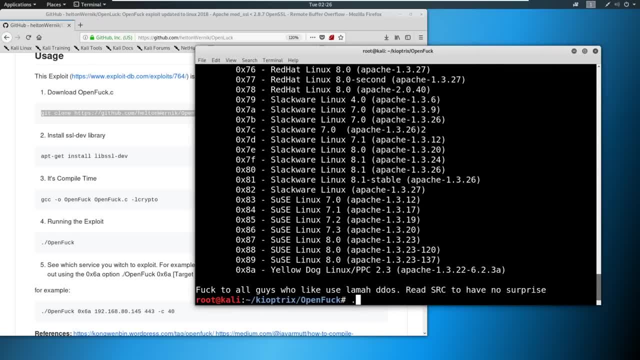 And again Red Hat Linux. That's another indicator. So let's copy this so we don't forget it, And we're just going to scroll down and we're going to say, hey, dot, forward, slash open. And we're going to paste that: 0x6B. 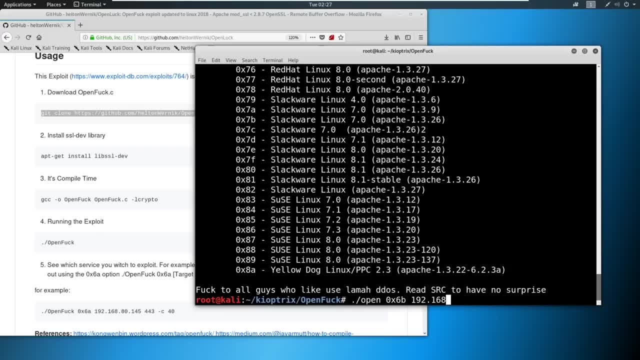 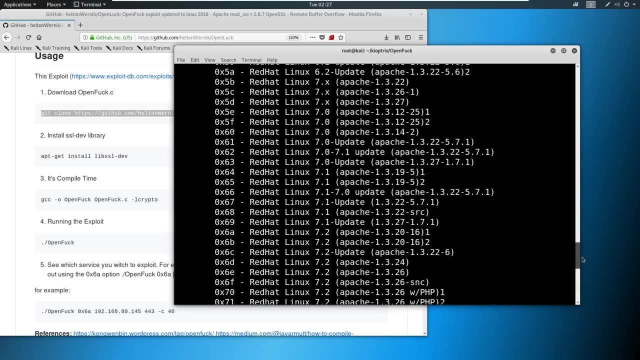 And then we're going to run this against the IP Address because it said box was next, So 134.. And then, remember, we had to give a dash C of 40. So that is the syntax. Sometimes you have to follow along and it's, I don't. I don't think most of them are as 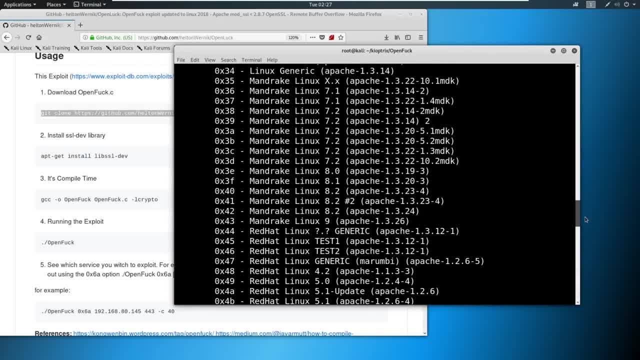 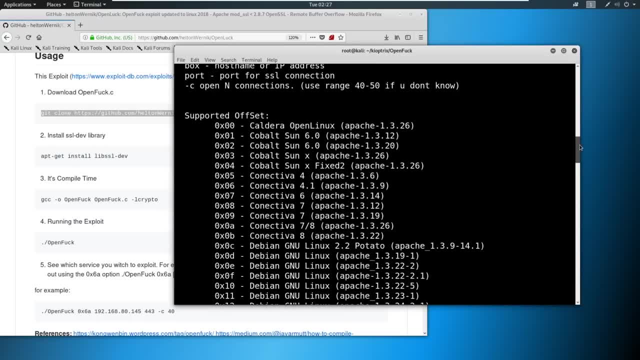 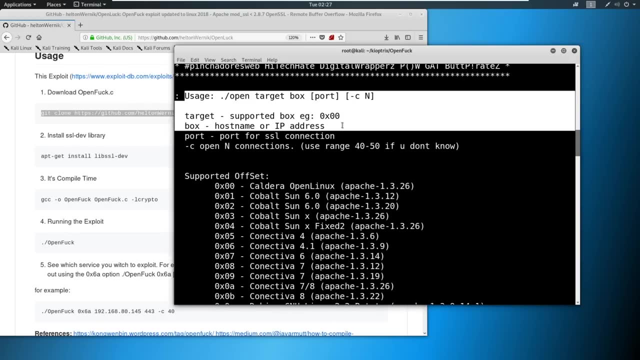 confusing as this. I don't want to say this is confusing. I would just say it's pretty lengthy for a exploit because you have to go through all the different offsets here to find the offset and actually fire this off. But You know, you have the opportunity here to actually be able to read usage and just understand. 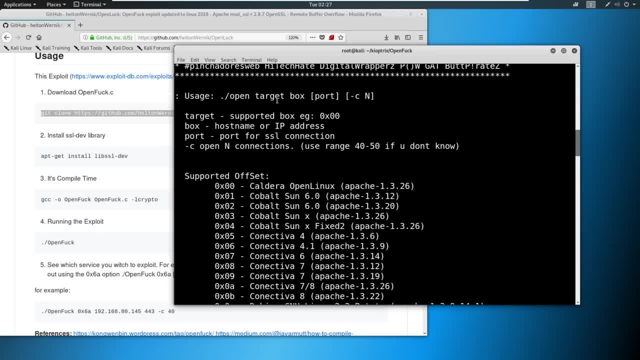 your your way through it. So once you get this little syntax and all this part down, it's really not that bad. So to check off the list, we've got the target, we've got the box IP address. We don't need the port because we're not running against SSL. 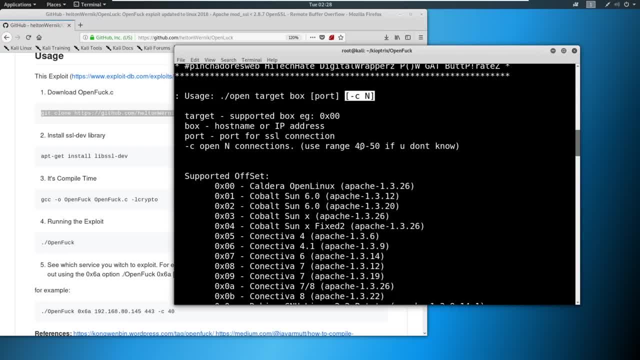 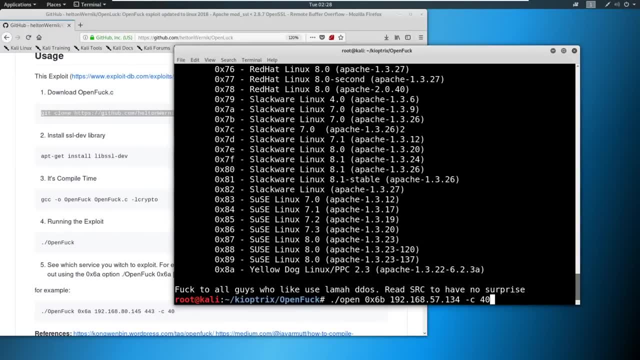 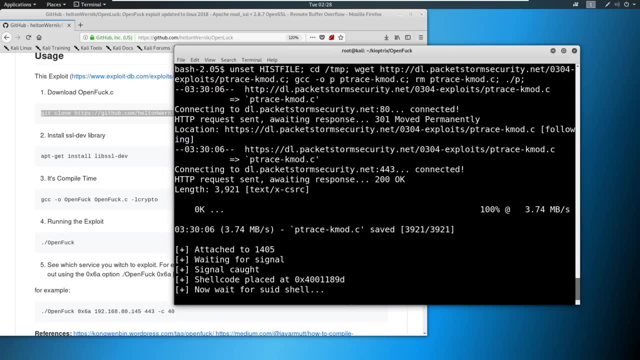 We're just going to run this against port 80 and then we're going to run dash C of 40.. So let's go ahead and try to fire that off and see what happens here, And this may just take a second. OK, it says it's spawning a shell. 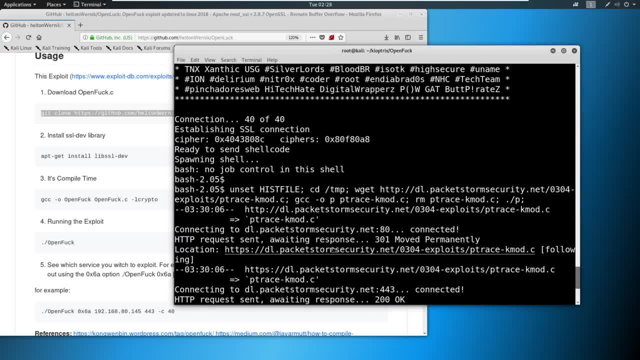 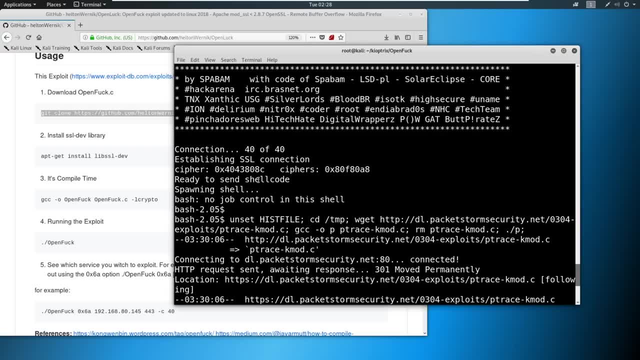 Now we wait for the SUID. Let's scroll up just a little bit while we're waiting here to see. So it looks like it sent the shellcode and it spawned a shell. It says: hey, we have no job control in this shell. 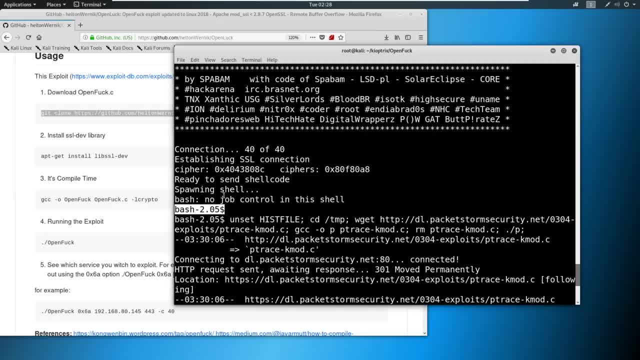 And then it has a shell here: Bash two point zero, five, That is a shell. And then it's going in and it's doing. it's doing some W gets. Now this is able to get out to the Internet, It's going to go ahead and try to do. W gets against these. 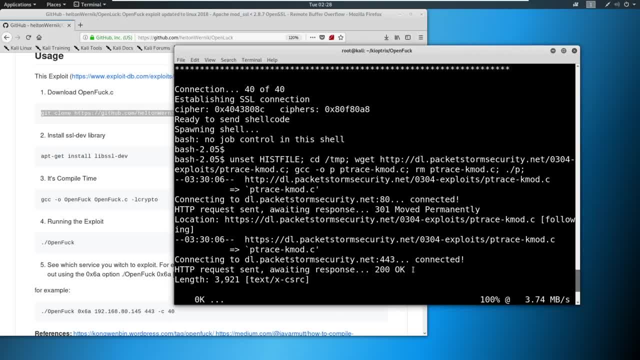 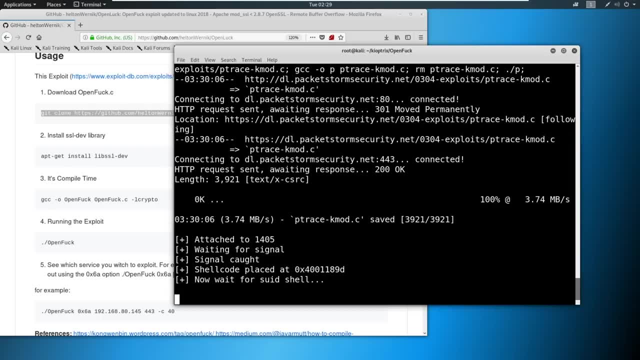 It's going to keep downloading and it's going to get the response here. OK, And now it says we wait for the shell because it saved this dot C file here And let's see if maybe we already have a shell. Who am I? 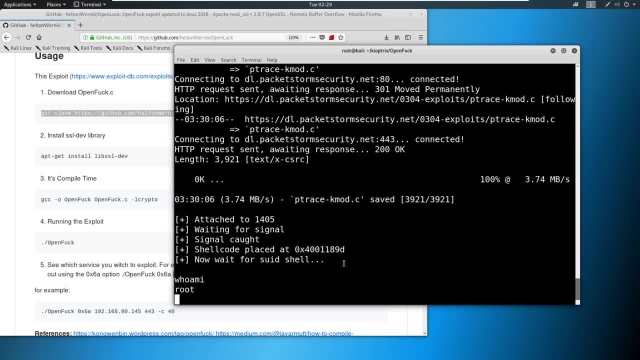 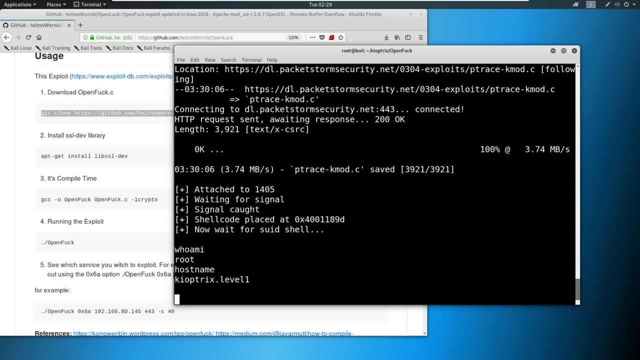 Root. OK, So it looks like it downloaded something and allowed us to maybe privilege escalate here And let's say hostname. OK, So we've gone through and we've rooted this machine with Metasploit. And now we've gone through and rooted this machine with the manually downloaded exploit. 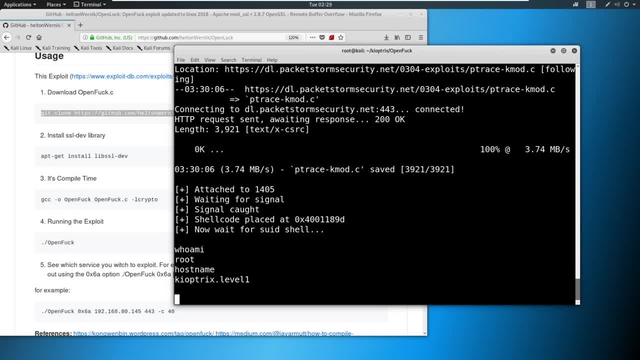 So there's two options. You're going to find out that Metasploit is a more robust and popular option, especially if you're going to be using Metasploit. OK, So you're going to use Metasploit as a penetration tester. 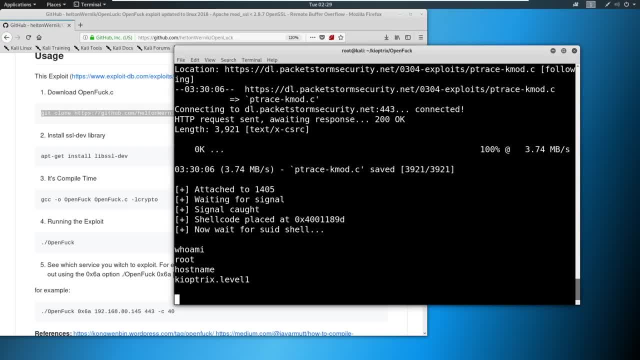 Now there is a common misconception or thought process put out there by certifications. The OSCP, for example, doesn't let you use a lot of Metasploit. only one instance of Metasploit on their exam. So everybody thinks: man, I really shouldn't use Metasploit. 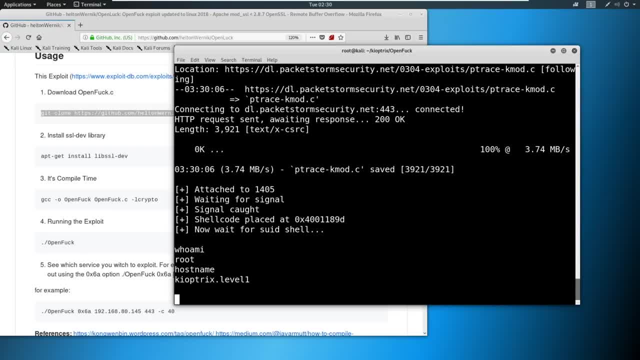 But you're going to see in this course how useful it really is and how robust it is. And if you talk to a penetration tester, they're going to use the best tools available. OK, They're going to use the best tools available to them. 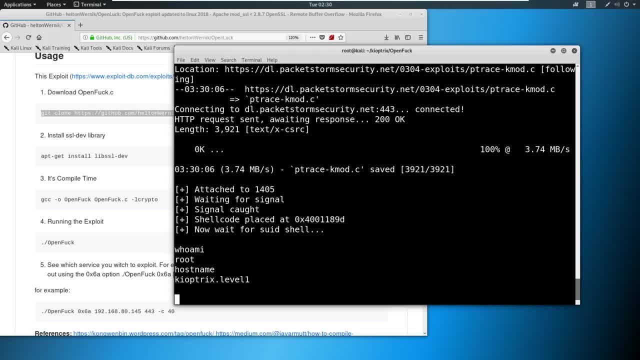 The certifications out there that do that are just making it harder to pass the exam intentionally than they are, you know, for practicality. This course is all about practicality. So from here, now that we've exploited it manually, let's talk about a couple of things. 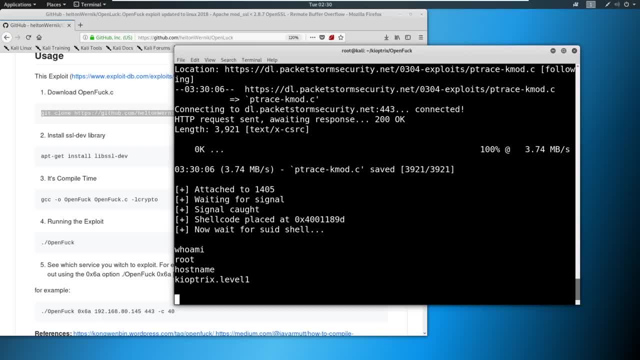 that we look for in post, So post being post exploitation, and we're going to cover this over and over and over again. We're not going to get into it fully right now. OK, We're going to get into an idea as to the thought process. 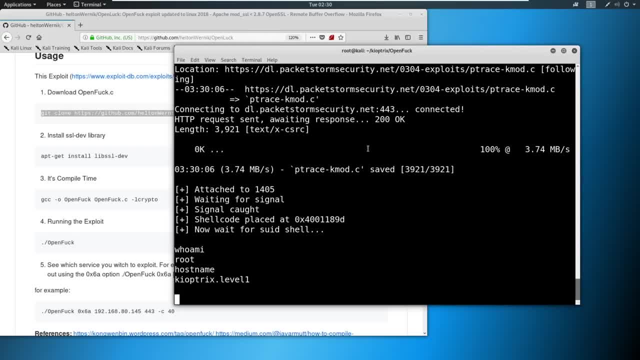 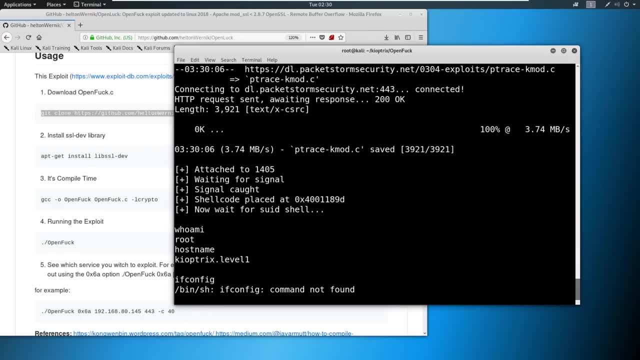 So the first thing to think about is what is our IP address? We could say ifconfig, if it'll allow us to. It depends on what kind of shell we're in. And see, this one is a weird shell. We could try IPA. 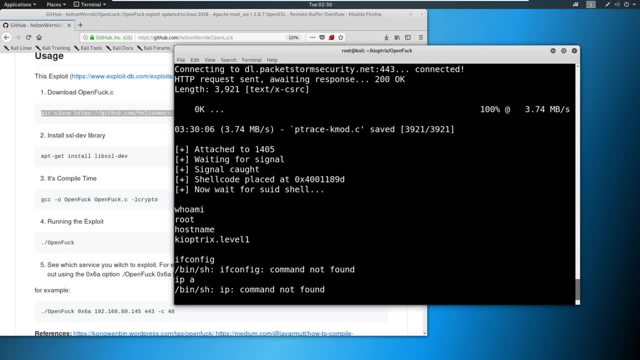 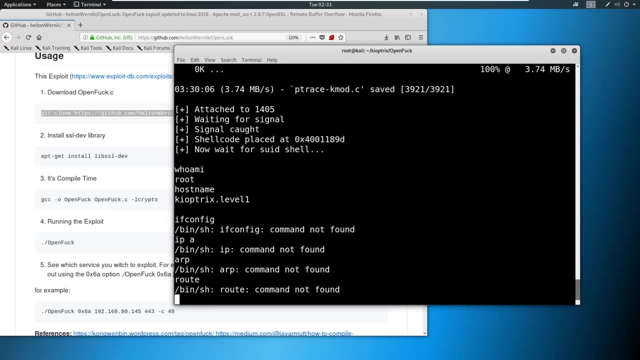 It's still not going to be found. If we try some commands like ARP or route, I doubt they're going to be found right now either. But we want to look at, like the routing table, the ARP table. We want to see if this machine is what's called dual homed. 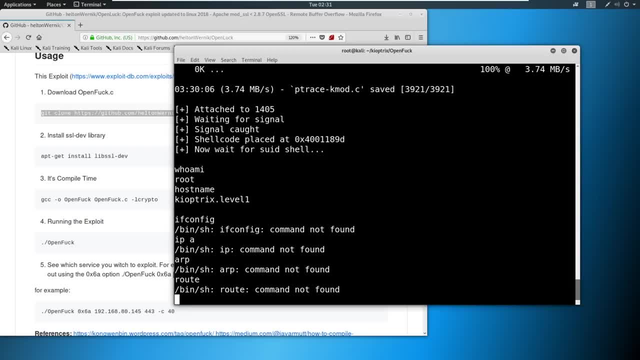 And you're going to learn more about that when we get into the pivoting. But if this is- this has like two NICs and we're on one network and the NIC is on a second network that we never saw before- then maybe we can do something called pivoting and move. 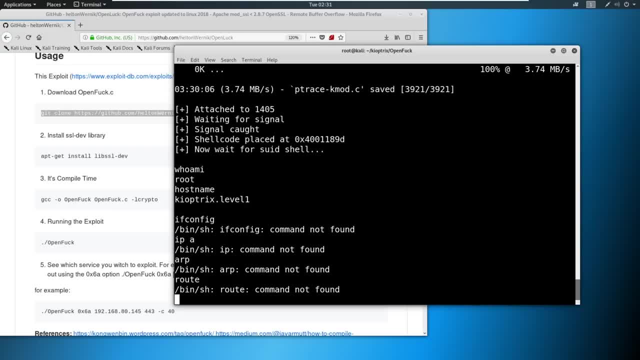 into that new network. But we would be able to identify who the machine's talking to with an ARP table or a route We could also look at like pseudo privileges. so we could say something like pseudo dash L. But we are root So we can run as everybody. 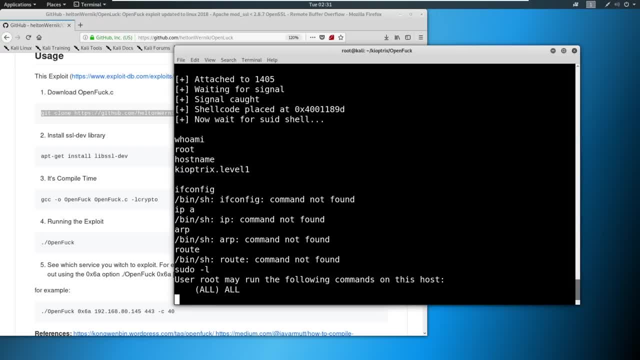 So a pseudo user, as we talked about in Linux, Linux lessons pseudo user is able to run commands as elevated, But here as root we're obviously already elevated. So other things that we can do: we can cat what's called the Etsy password file. 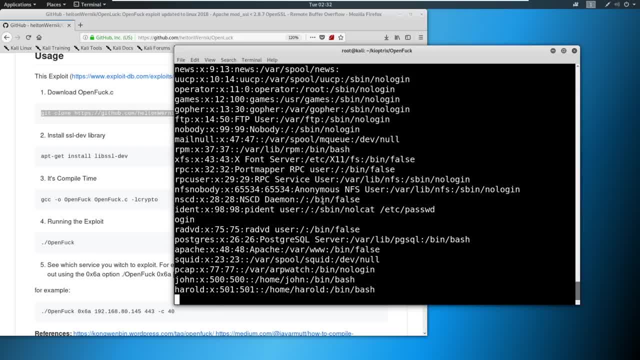 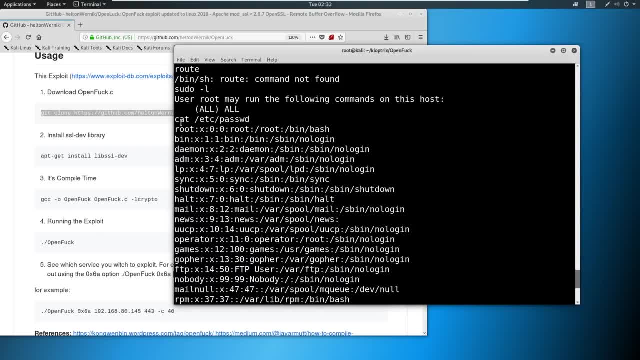 Now this is very misleading, because the Etsy password file used to be the password file. Now it just holds a placeholder, So you could see all the users that are on this computer route being this one. There's a lot of built in users here. 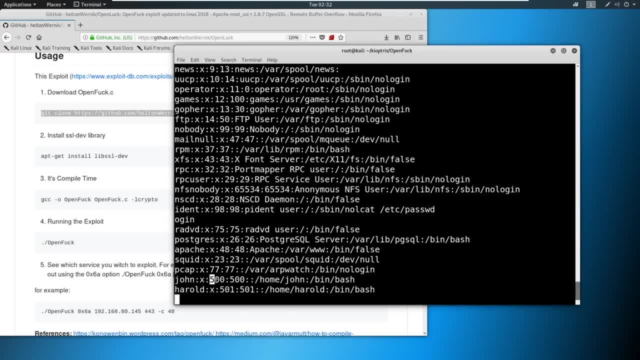 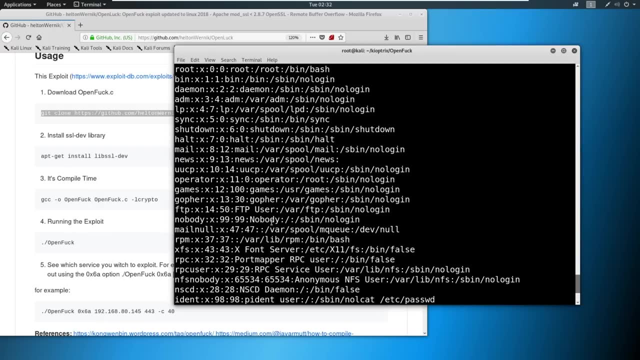 But if you always scroll down to the bottom and you start at the 500s, that's where your users start. So there's actually two users on this computer as well. One's named John, the other is named Harold. So we look at these users and we say, OK, well, there's no password in this password. 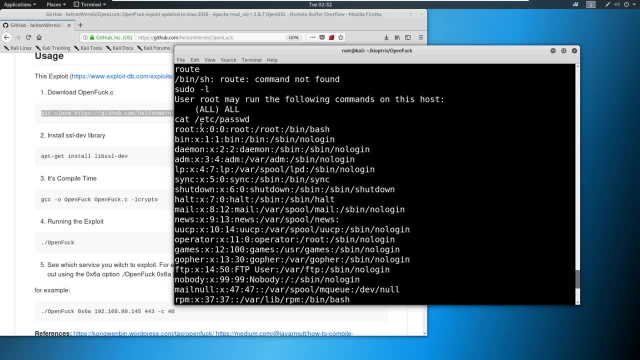 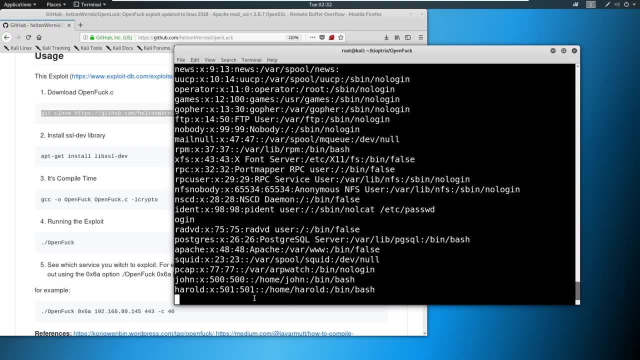 file, but there used to be Back in the day. there used to be, That's why they call it this- And now they moved it to this placeholder of an X, And what we can do is we can come in here and we can say: hey, cat, Etsy shadow. 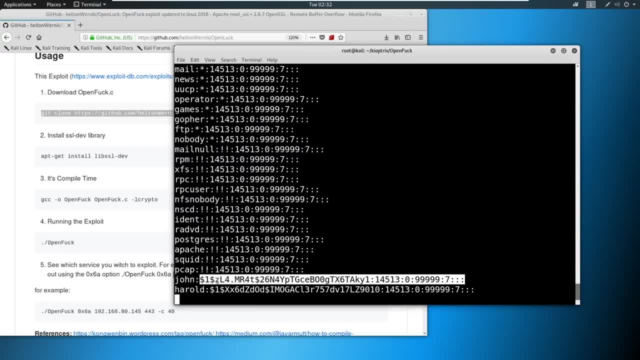 And now you see the hashes are in here. So these hashes are what the X is placeholding for. We can actually combine both of these files with the tool and go offline and try to crack these. We'll work on that later on in the course, but just for now, like getting your wheels. 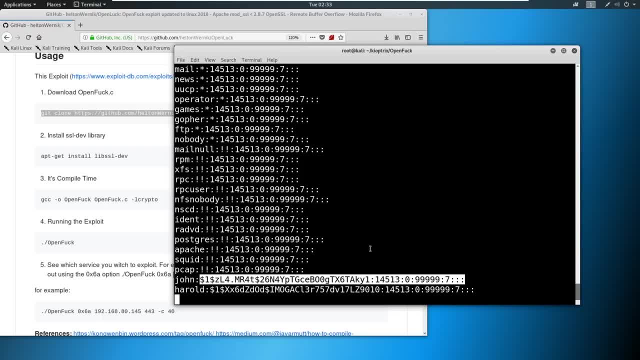 spinning on as to what we can do with root level access. We need to start enumerating again, looking at files on the computer, seeing what what's out there and what we can do with it. But we'll get into post exploitation techniques and thought process as we go through the active. 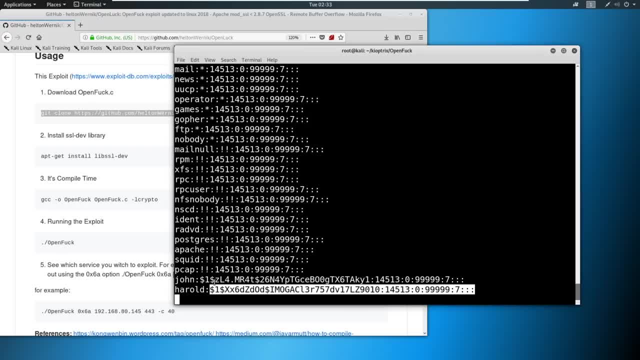 directory portion of the course because I think it plays hand in hand and we can talk about password cracking there and how to attack some of this stuff. But there will be a password cracking video on on Linux as well when we get into the post exploitation phase of this. 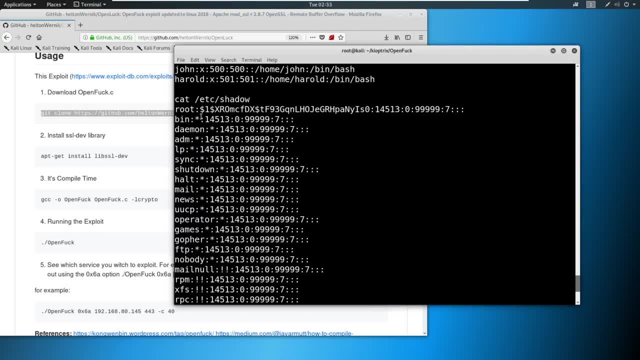 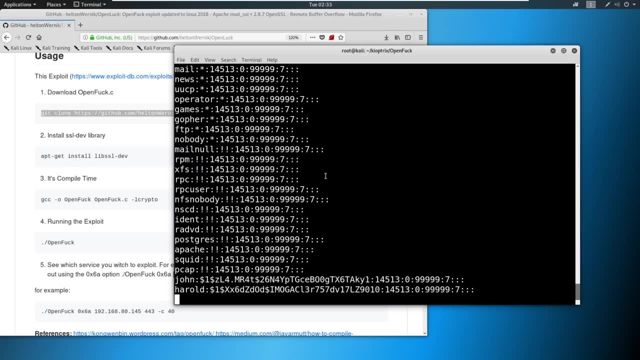 But That's really it for now. So we've got the, we've got the shadow. We could take this offline, try to crack it. We can enumerate files. We can try to, you know, break into user folders and see what they've got in there. 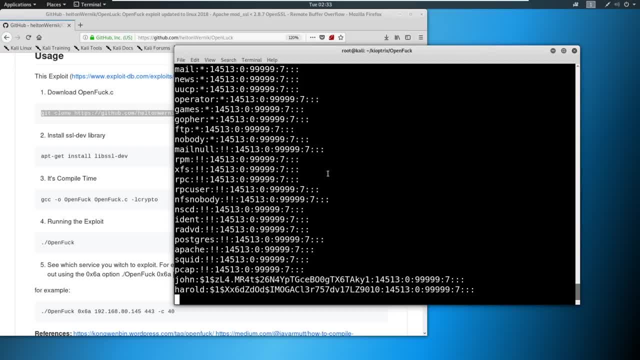 Maybe they've got password files stored in there, et cetera. So from here, we have rooted this machine twice. We rooted it with Metasploit, we rooted it manually, and now we can start moving on. I do want to show you a few more attacks. 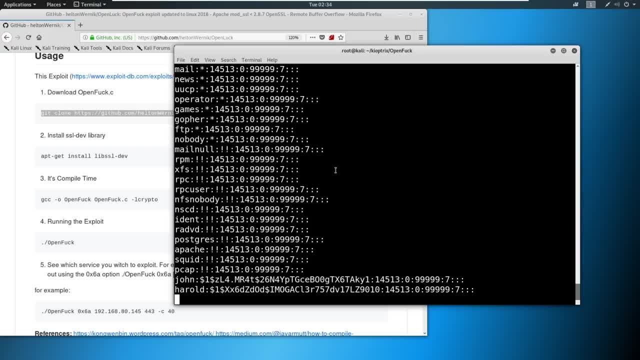 So here's what's going to happen. We're going to go over the next few videos. We're going to talk about brute force attacks- really quick on SSH. We're going to talk about credential stuffing. We're going to revisit that concept that we talked about in information gathering. 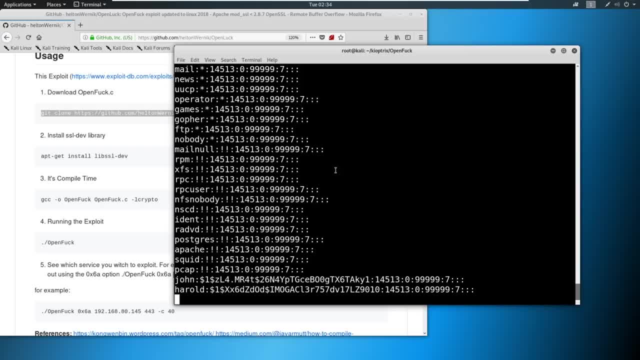 And then we're going to look at our notes and we're just going to compare notes and see where we're at with findings and everything else. After that we're going to get into what I like to call the mid course capstone, which 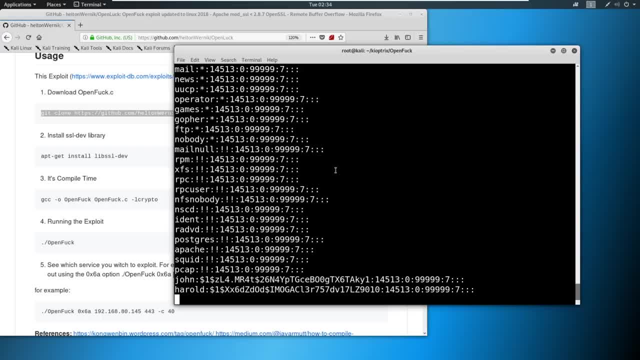 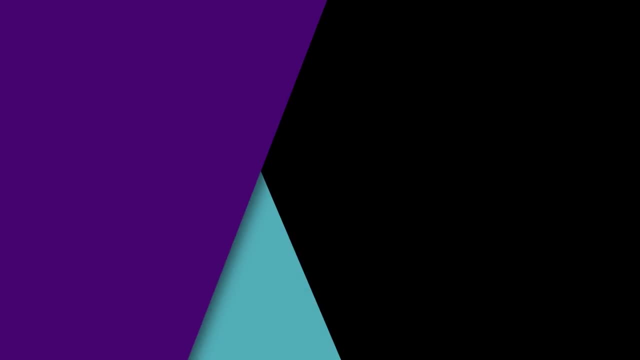 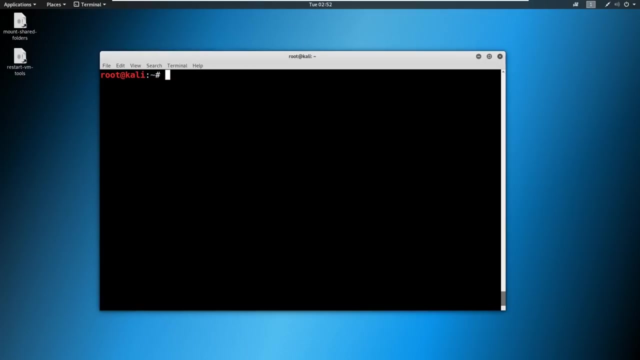 is going to allow us to do a bunch of exploitation against a bunch of machines, and it should be really fun. So End of spiel. again, I will catch you over in the next video as we talk about brute force attacks. In a previous video we discussed SSH and that it's really not always that much of a 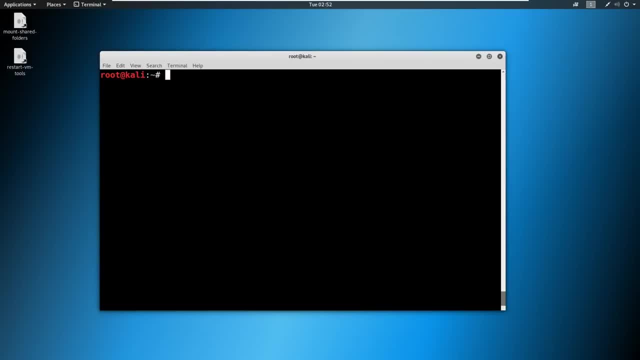 low hanging fruit. So we've got SSH here and say we want to attack it. Now there are three reasons we're going to do this, And this is from a realistic perspective. If we see SSH on an assessment, we're going to try to brute force against it or use weak 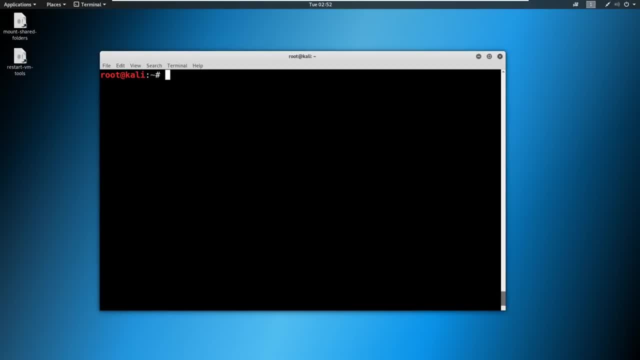 or default credentials. And we're going to do that because, one, we're going to test password strength. Two, we're going to see if we can get in with a weak password or default password, And if we can, that also attests to password strength, correct. 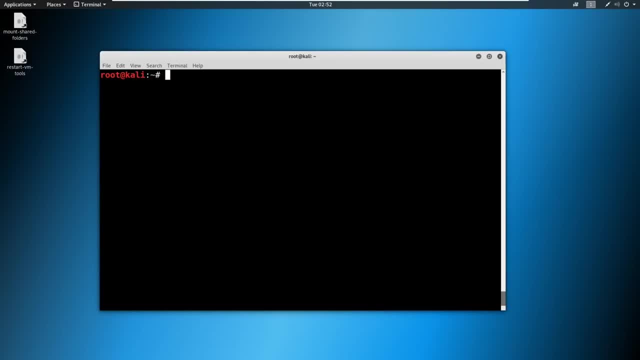 And three. we're going to see how well the Well the blue team performs. Do they catch us? Do they see us? brute forcing? This should be something that should alert when is being performed, but you would be surprised how often it does not. 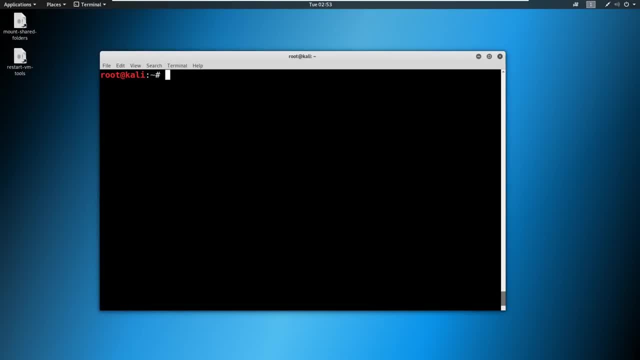 So during a pen test, I am as loud as possible. This is not a red team assessment where we're trying to be quiet. This is a pen test where we are as loud as possible and we are hoping to be caught, sometimes just as or just told to tone it down. 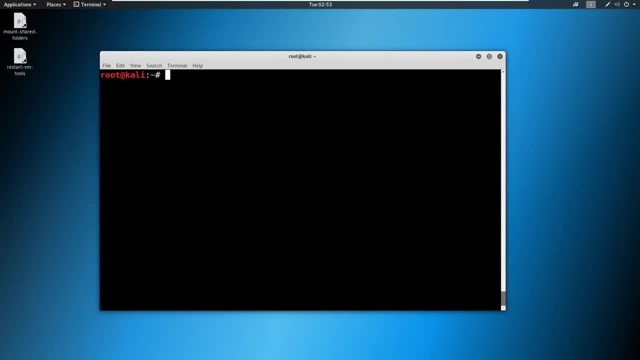 Okay, You know, Hey, we're seeing you. Can you be more quiet? And we just want to be caught sometimes so we can give kudos in a report and say, Hey, you saw a scanning here and here and kudos to you, but you didn't see a scanning here. 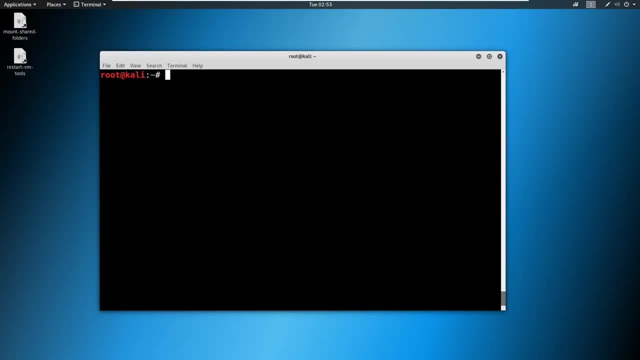 and here. So this is how we really help fine tune a blue team and help fine tune a client as well- is being loud sometimes. So we're going to practice being loud today and we're also going to practice brute force attacks, and we have the perfect opportunity to do that with an SSH port being open on. 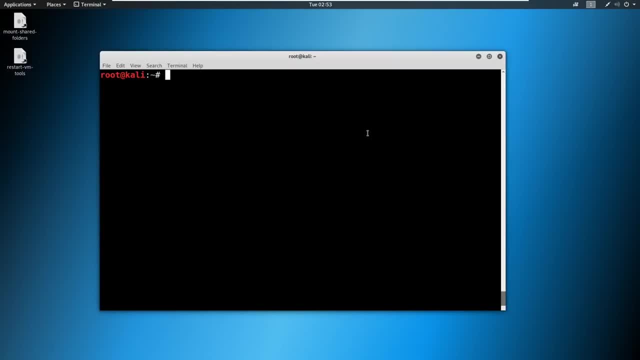 this Machine. So what we're going to do is we're going to use a tool called Hydra, and then I'll show you the Metasploit way as well. So Hydra is a brute force tool. So the syntax for Hydra is going to be this: we're going to say Hydra and then we're going. 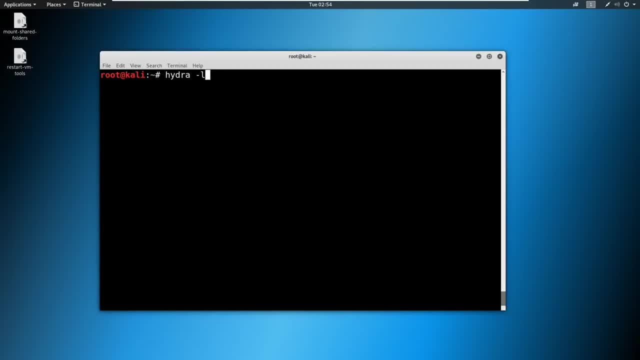 to give a dash L for the user that we're going to be utilizing. In this case I want to attack root and then we're going to give a capital P for the password list. So if we wanted to use a password list with L, we can just say capital L. but here we're. 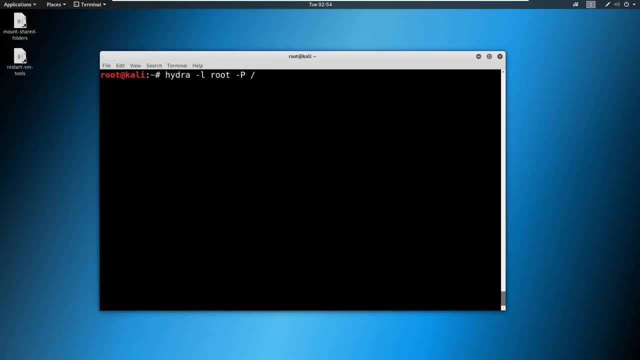 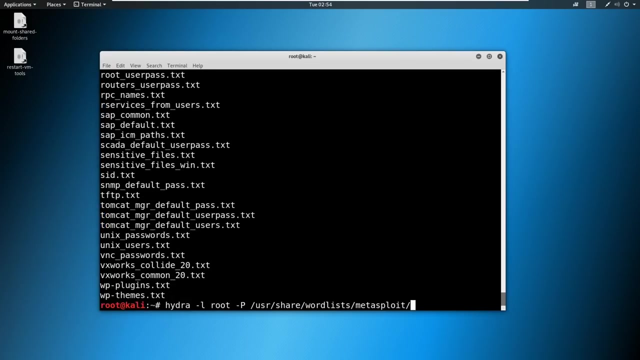 going to say capital P for the password list And then we're just going to say user share wordless Metasploit, And I'm just going to double tab in this folder so you can see how many words are actually in here. There's quite a bit of wordless and you can space, space and it has wordless for all different. 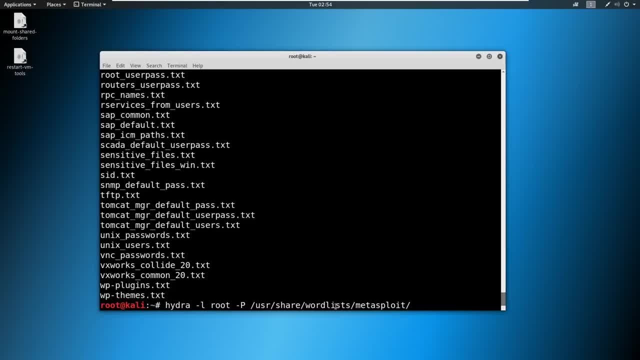 kinds of things built in, and these are all over Kali, So it's good to know You don't have to worry about your folder locations. but user share wordless is one that we'll use quite a bit, And what we're going to do is we're going to utilize an attack with these Unix passwords. 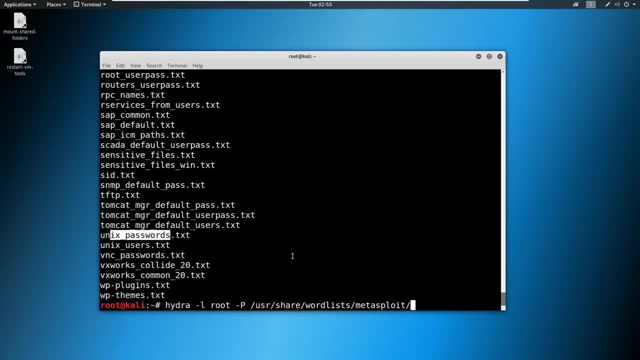 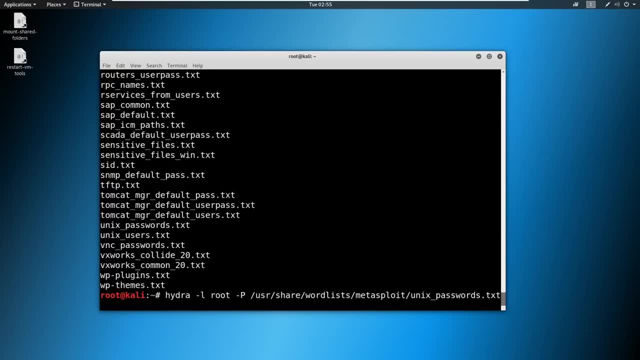 here. So we have a Unix users and Unix passwords. We're going to utilize the Unix password list and just try to brute force with that. So we'll say Unix passwords, something like that, And then we're going to need to specify what we're attacking. 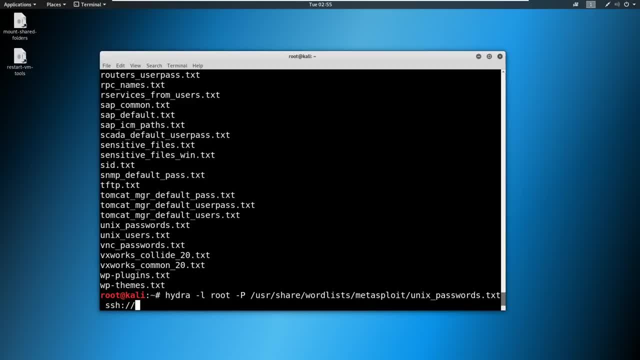 So we are attacking SSH Like this and our IP address of our machine that we're attacking on port 22.. And then we need to have a certain amount of attempts or threads at once And we're going to limit that to four, And then I'm going to do a capital V for verbosity, just because I want to see the user attempts. 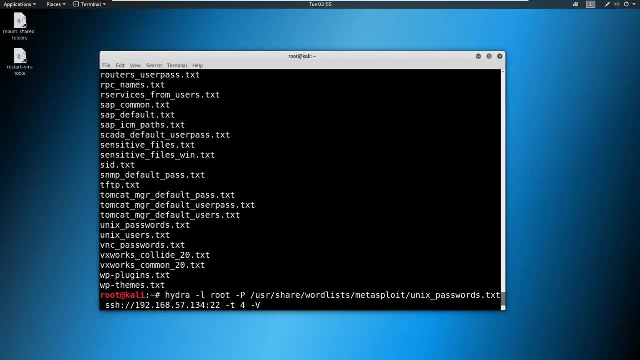 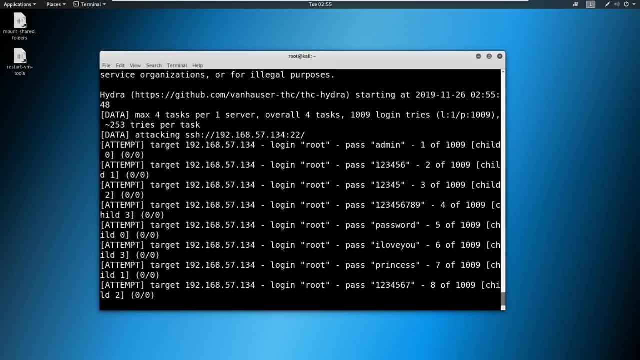 flow through so that we can actually see what's going on here. So once you've got the syntax ready to go, go ahead and hit enter Okay, And you're going to see that it's starting to attempt root login password with all these. 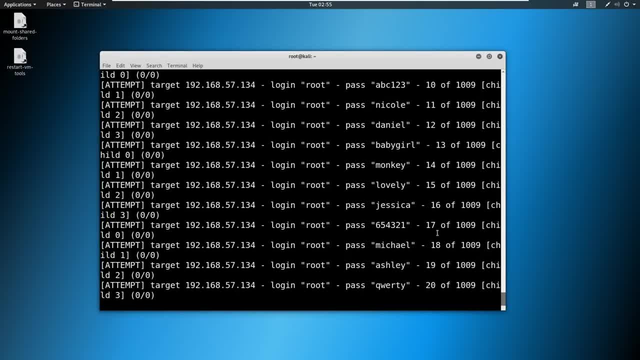 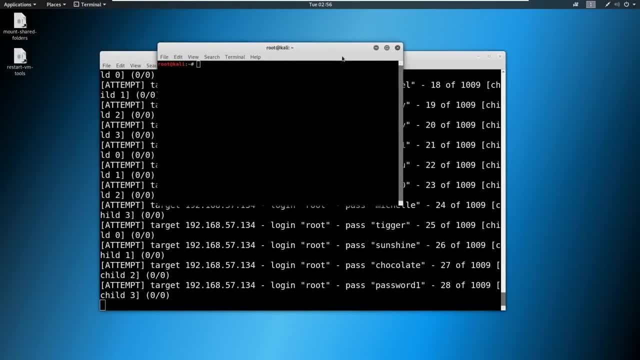 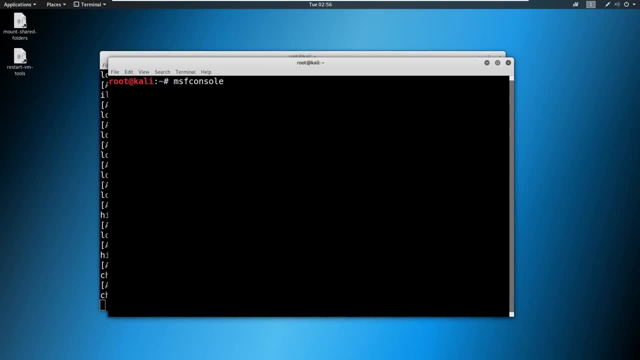 weak passwords here and hopefully it might find something. but let's go ahead and open up a a new terminal here And we're going to just make this a little bigger and I'm going to load up Metasploit as well And we're going to run the same exact thing in Metasploit. but I think it's good to know. 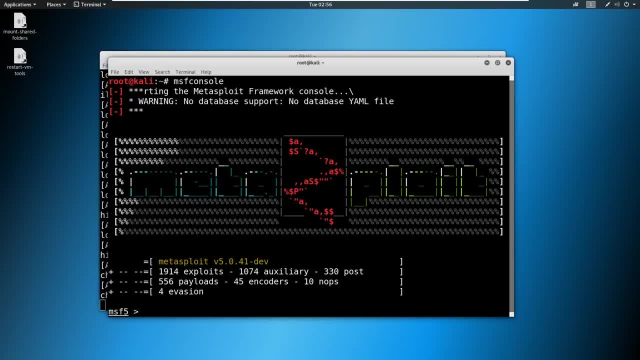 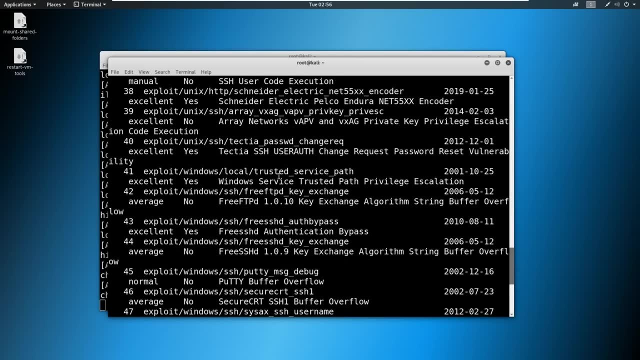 multiple frameworks and multiple tools to perform the same task. So here we're going to search for something like SSH, and this is going to be an auxiliary module, So we'll just scroll up and we're going to look for something like SSH login. 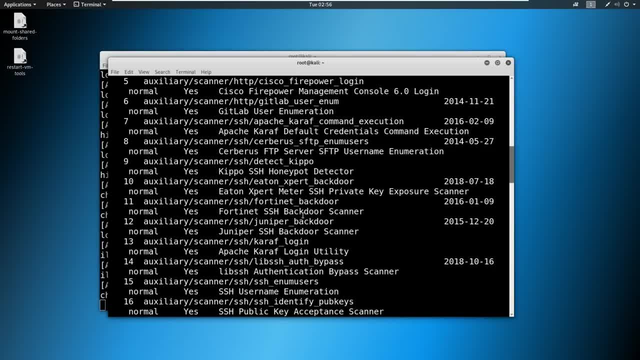 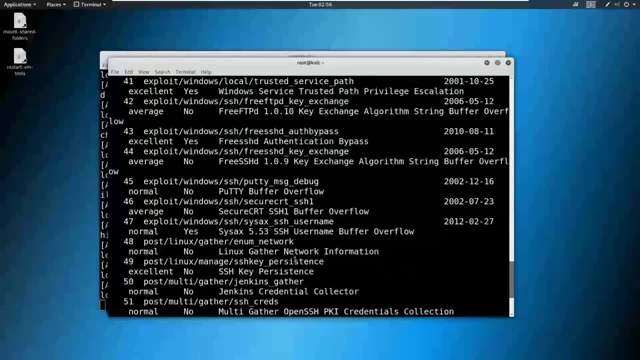 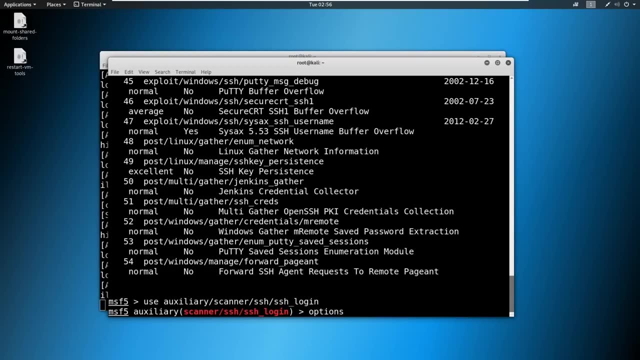 Perfect Login check scanner and make sure we don't have anything else. And it looks good to me. So let's go ahead and take this SSH login And we're going to go ahead and say, okay, Okay, Okay. So we're going to use options. 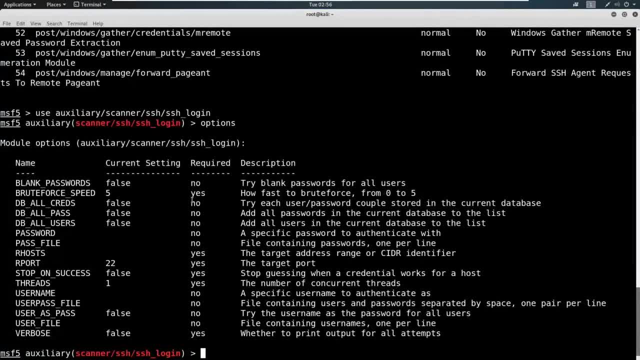 And now we have kind of our brute force options here. Let me make this a little bigger, So it's prettier. So we've got a brute force speed from zero to five, five being the fastest. Try playing passwords. No, no, no. 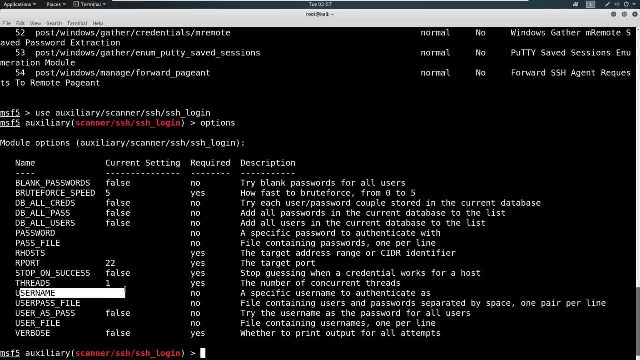 We can set a hard password and we could set a hard username. We could set a user and password file, a user pass user- as password file. Again, we can have a password file as well. So we have a lot of different options here that we can utilize, but we're going to go. 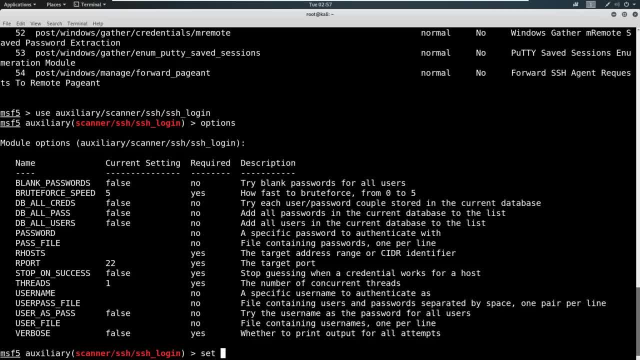 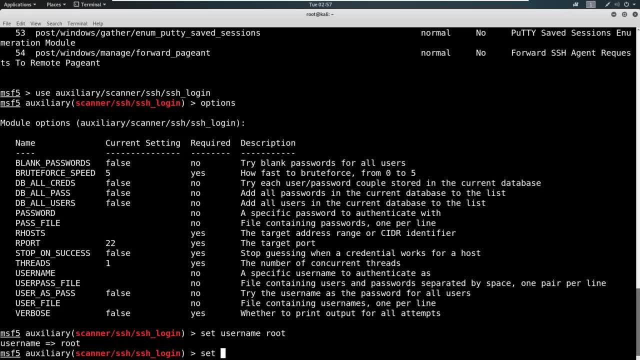 ahead and do the same kind of thing. We're going to say set username and we're just going to say root And then we're going to say set pass file and similar to what we just used. we're going to say user share- wordless. 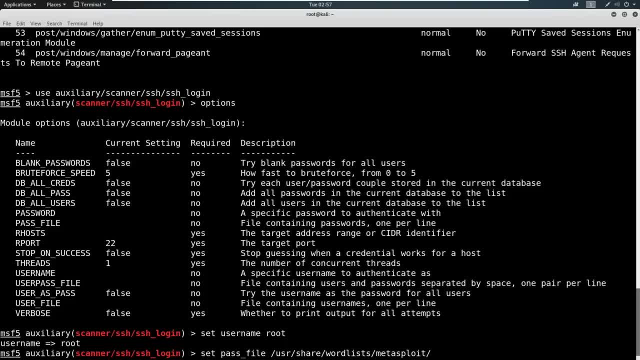 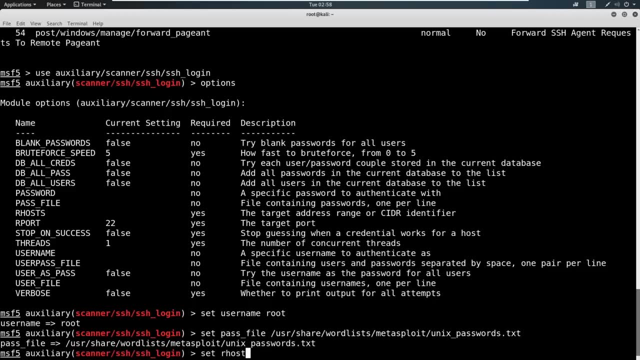 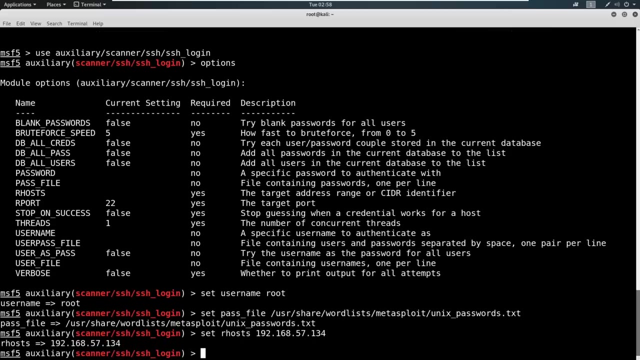 No Metasploit. And then we're going to say Linux, Unix- sorry, Unix passwords, And that should set the pass file. And then we just need our host as well. Set our host and we'll say 192.168.57.134 say options. one more time. 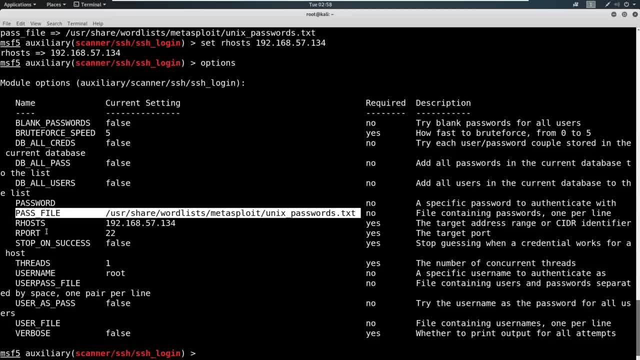 And you can see that we've got our password file set, We've got our our host set, We've got our. our port on 22 threads is one username root, and we should be good to go. Now we can set multiple threads here. 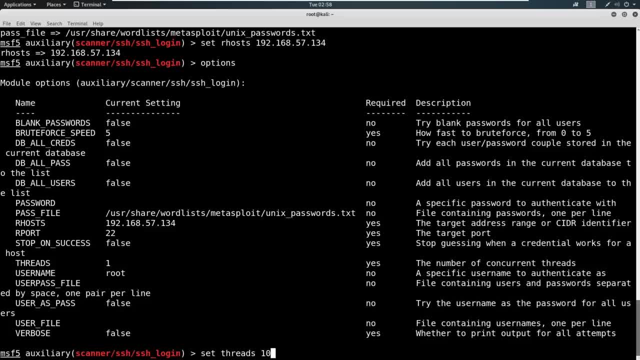 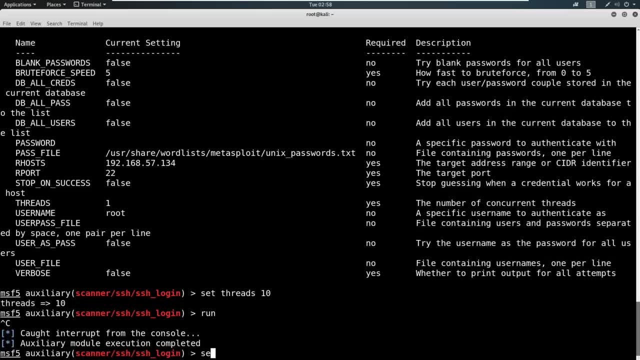 We could set threads to like 10.. This is really going to amp it up. I mean, this should be detected in a second, but we're going to try to run it and we could set actually. let me control C. let's set verbose to true as well. 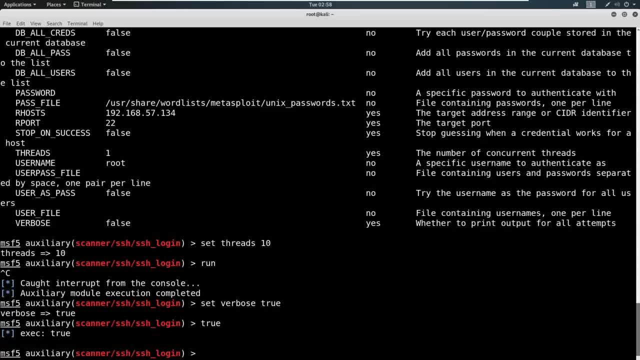 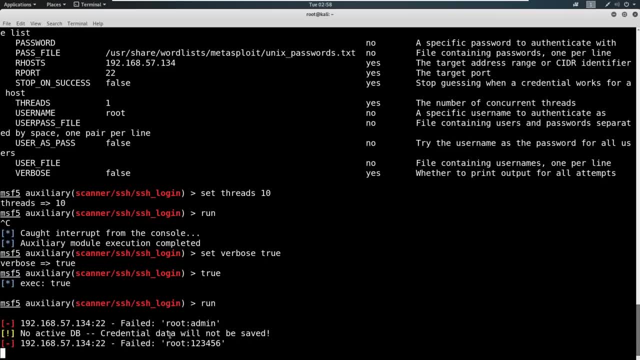 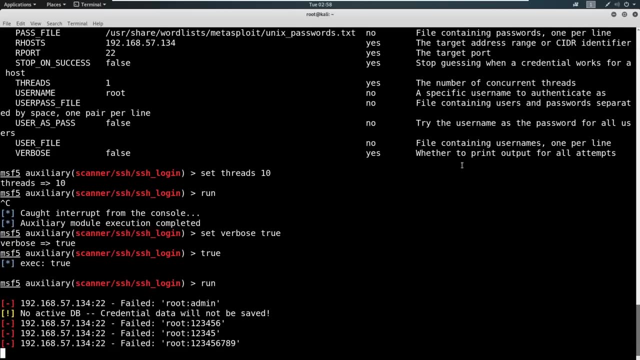 Just so you could see that it's actually working. set verbose to true. and then we're going to run this And then it's going to attempt different credentials here and it'll say, Hey, I found it. and it'll light up green and then we'll know it's good. 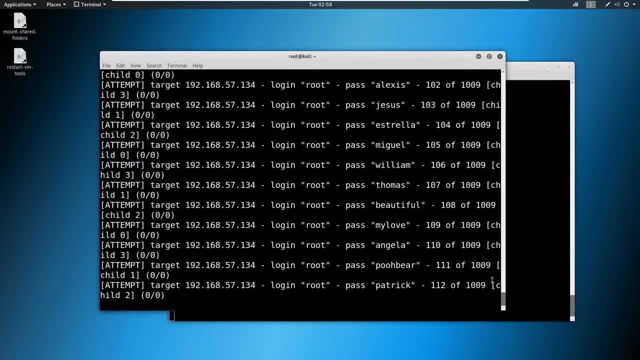 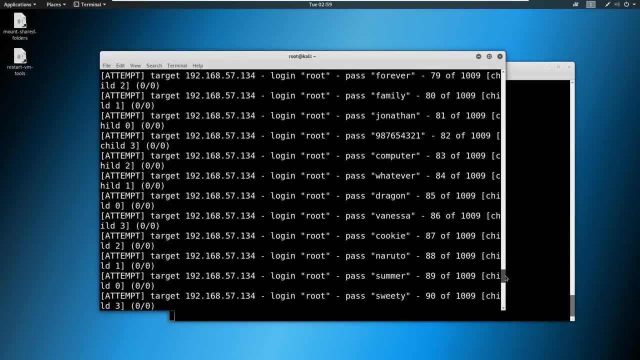 So this is actually going kind of slow, surprisingly, And you could see here that we are at attempt one 12, one 16. So this is also going slow And we do not have a successful attempt or login. I actually don't believe that there's going to be one. 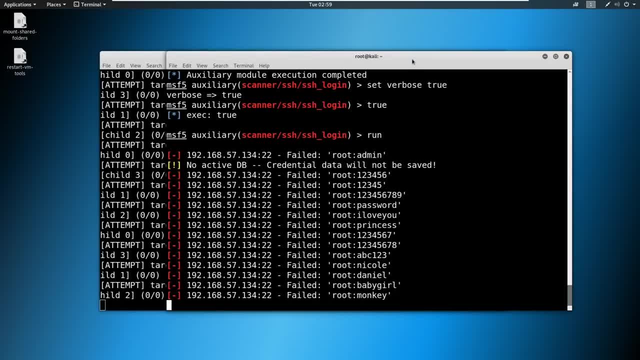 But you never know. I believe I remember taking this offline and trying to crack the password and it wasn't any kind of weak password. So you can let your Bruce brute force run if you want to go with it, but I'm going to go ahead and kill mine. 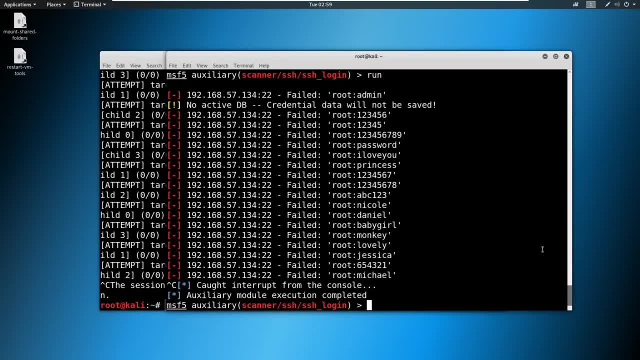 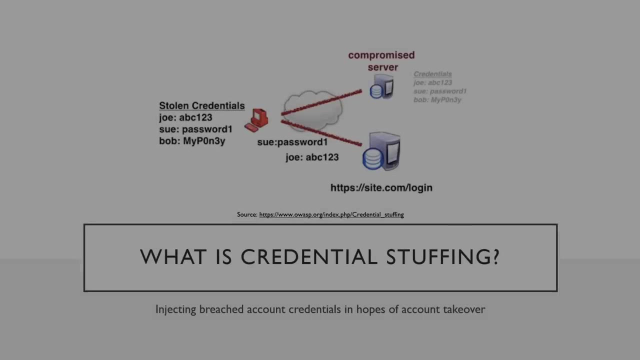 And that's it for this video. So from here we're going to talk about a similar methodology called credential stuffing, which we've already talked about before, except we're not brute forcing, but we're using common knowledge to our advantage. So we'll talk about a little bit of crash stuffing in the next video. 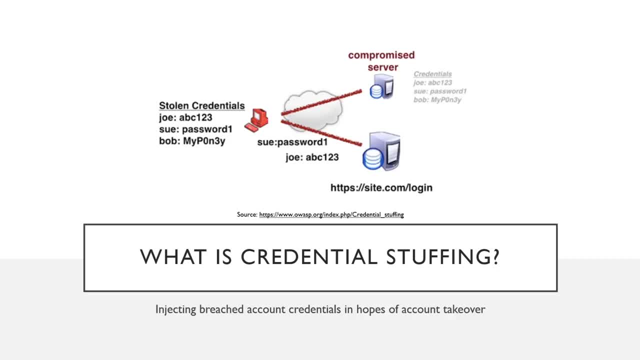 Let's talk again about credential stuffing And, while we're at it, we're going to talk about password spraying. Now I realized we talked about this earlier in the course with breach parse and we leak info. But I do think that hammering concepts over and over and how important they are does. 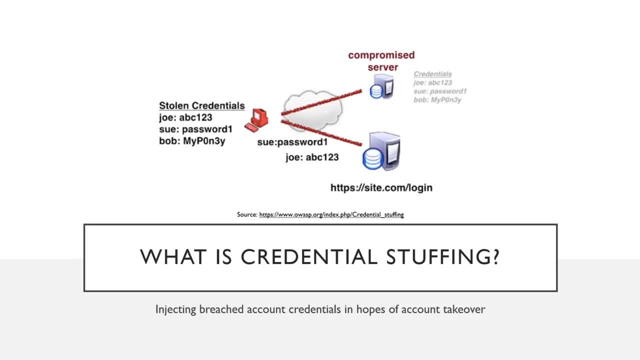 help for information retention. So again, if we look at this example here, what is credential stuffing? Well, it's just Injecting breach account credentials in hopes of account takeover. So if you look at the compromise server here in the upper right hand corner, we pull down. 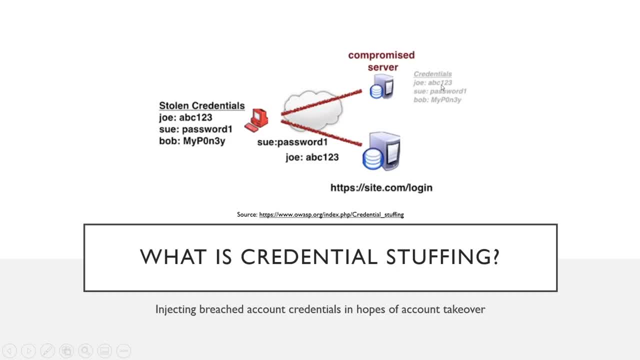 usernames and credentials and we get these from leaks like the LinkedIn link or the Equifax link or whatever those have come out recently. We get these leaked credentials and we grab these databases, We search through them, like we did with breach parse or like we can with. we leak info and 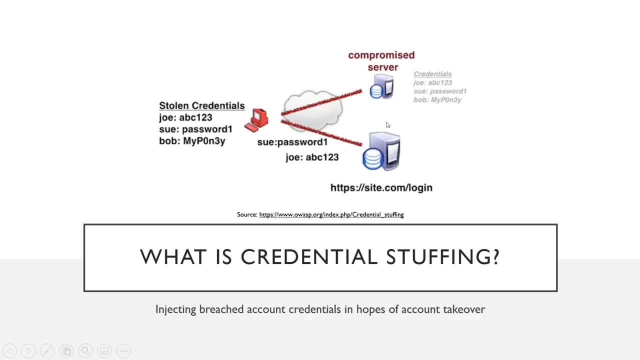 we get these stolen credentials and we take these credentials And we try to pass them to the site login. Now we can take a look at a real life example of that which I have pulled up here And again, this is just an example of the Tesla breach parse. 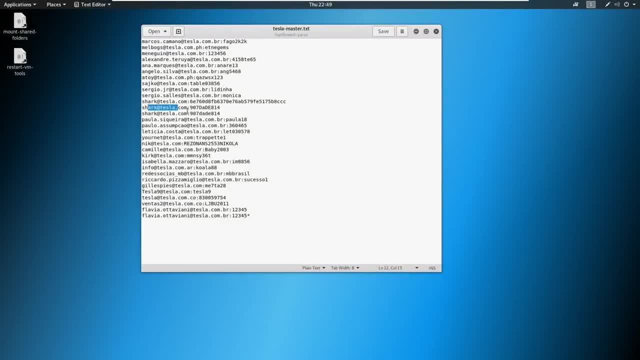 So we have some usernames and passwords, We have repeat offenders- Remember, we also have similar passwords here. but the art of credential stuffing is taking these passwords and these usernames and throwing them at a website. That's all it is. So we're going to throw them at a website and just kind of spray and pray. 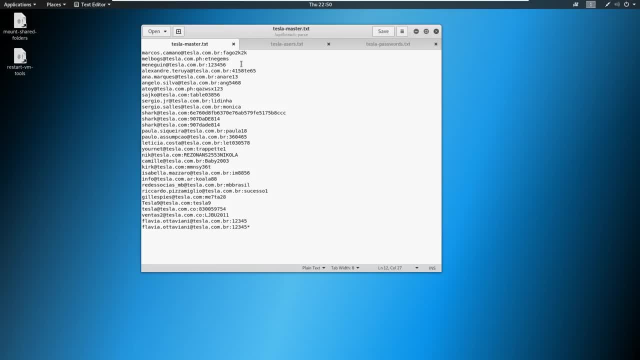 Now I just gone ahead and open up this same Tesla dash master. I've only opened up the users and the passwords, just for an example of spraying. This video is going to be in theory only. I don't want you attacking Tesla's website. 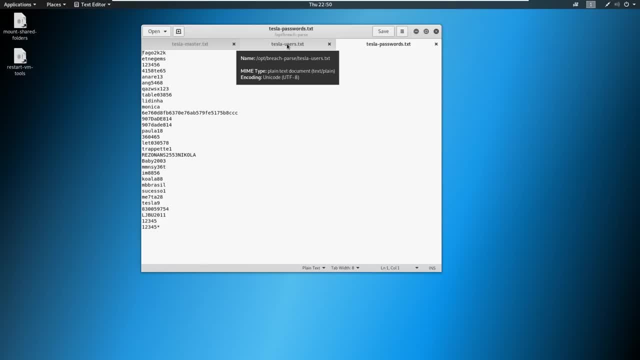 So just take this, for example. you can follow all the way up until the point that we actually hit attack, if you want to follow along, But for this, Please Don't attempt an exploit against Tesla. You do not know when the criteria is going to change. 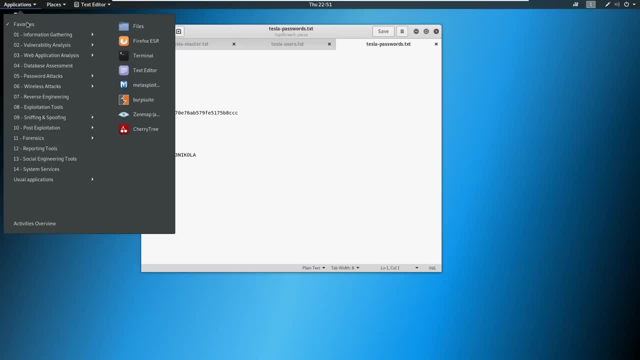 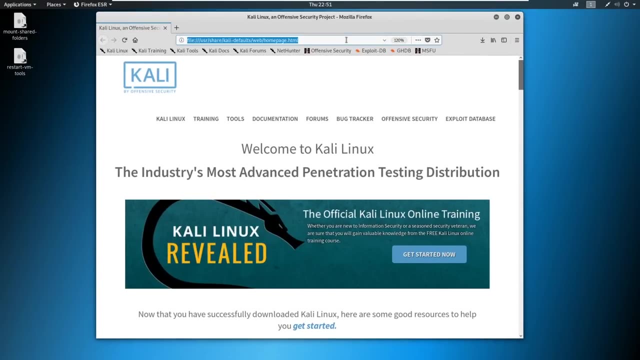 And I just don't want you getting in trouble, just in case it does. So, from here I'm going to go ahead and go to Firefox, And while we are in Firefox, what I want to do is I want to take a quick pit stop and 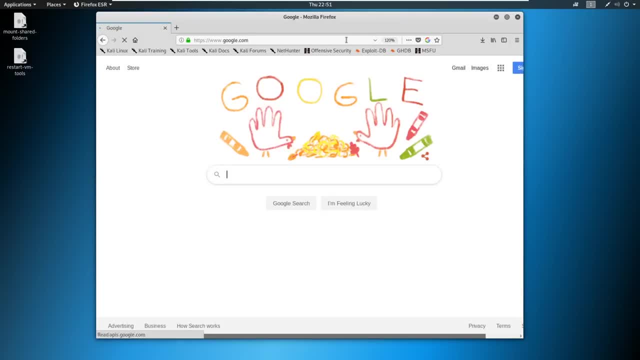 go to Google and I want to look up something called foxy proxy. So go ahead and do this. Look up foxy proxy like this, not froxy foxy proxy- And go ahead, Click on this top one here, the standard. 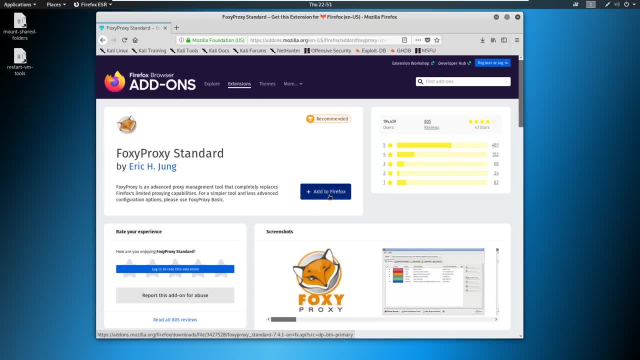 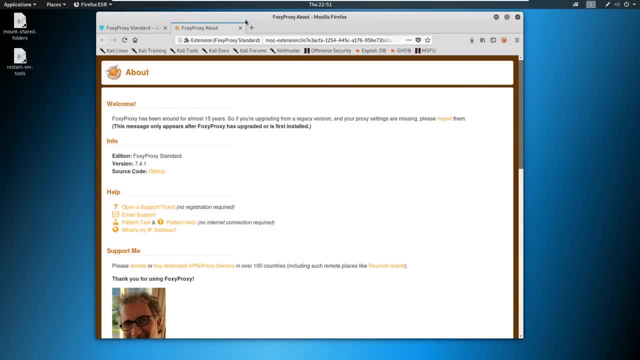 And we're just going to go ahead and install the standard to our Firefox, And this is going to be a useful tool that we'll be using throughout the course. So, okay, we've got foxy proxy installed. Now what has happened? up in the right hand corner? we've got this here. you can see foxy. 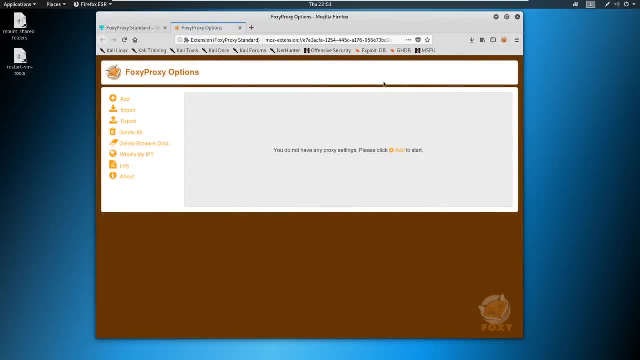 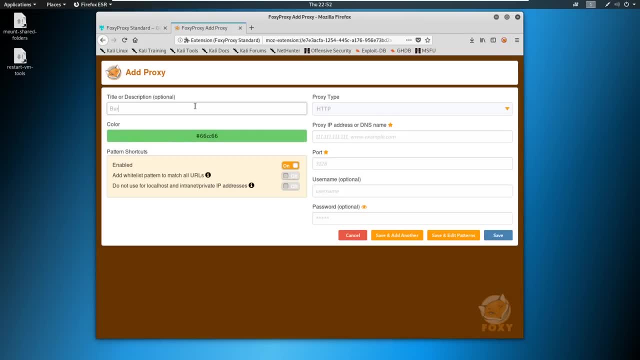 proxies here And we can just say, hey, options, And in the options we're going to add in a proxy over here on the left And we're just going to call it burp suite, And then over here we've got proxy types. we're just going to leave this at HTTP. 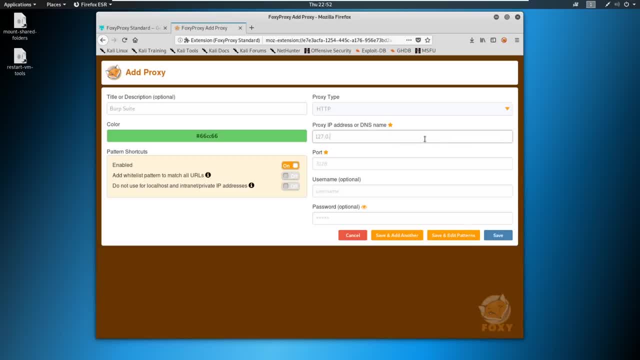 And then we're going to give it an address which is 127.0.0.1- same thing as before- And again, this is 8080.. Will this hit save? And then we're going to go ahead and close out, and then all we got to do now is click. 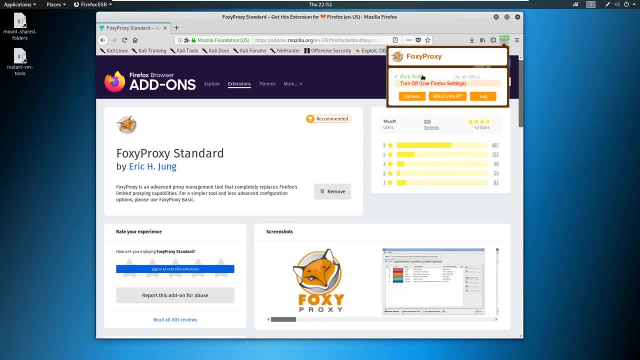 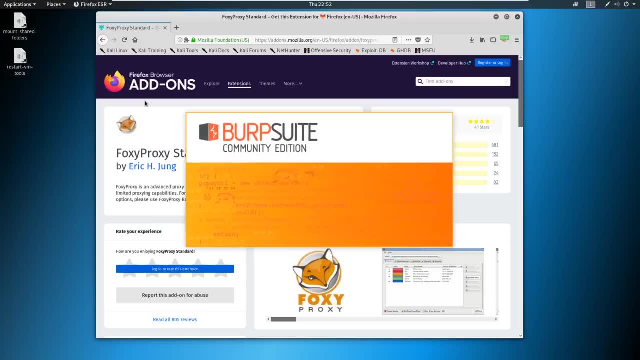 this and click this And now burp suites turned on. super simple. So But also to our applications and let's just go up here and open up burp suite And let's test out our proxy and make sure. ignore the errors. 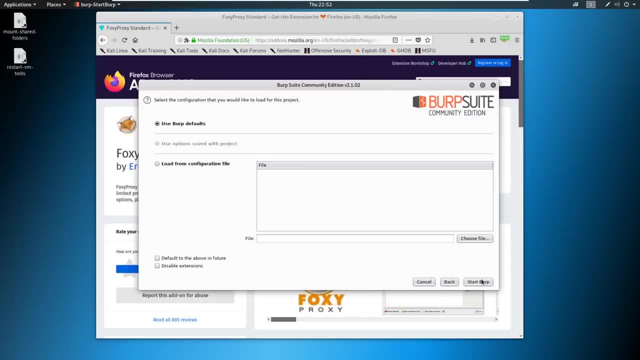 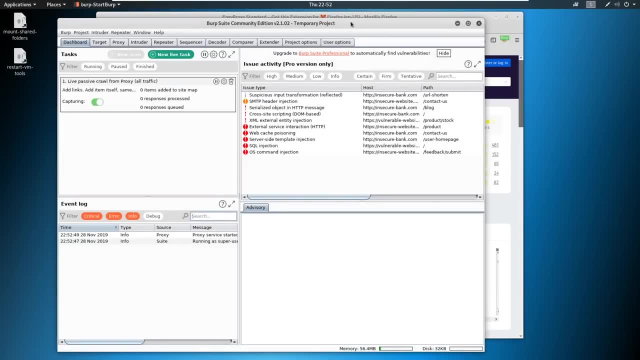 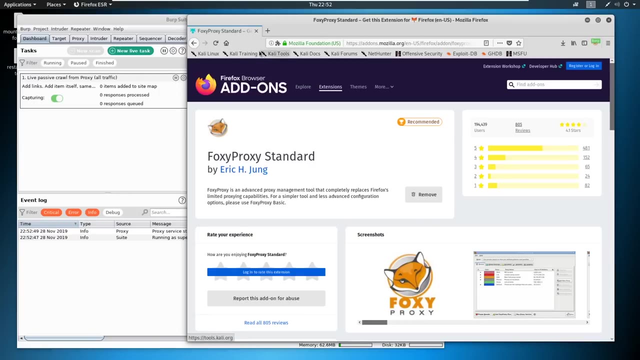 Don't worry about those- was: go ahead and hit next and use burp defaults, And I will give you a second here to catch up, because I realized that I might be clicking through a little fast. So once you have everything set up like this, what we're going to do is we're just going. 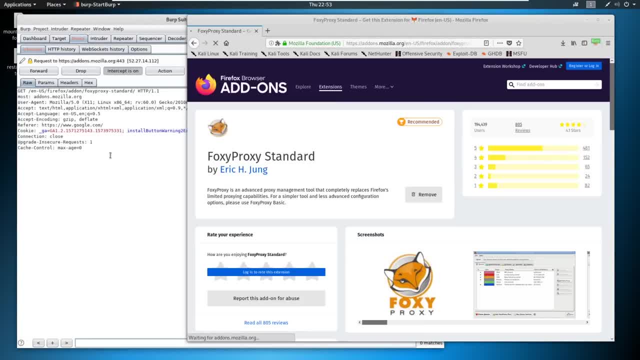 to make sure our proxy works, So I'm just going to refresh the page and you can see that it worked. So easy on, easy off. That's all we're looking for here, instead of having to go in the menu and go to preferences. 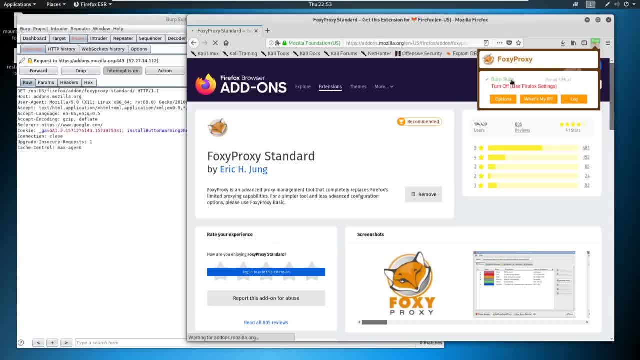 and you know, go through that whole process. All we got to do is click a little button. we can turn it on or off within a couple clicks. So from here, I'm going to turn the intercept off And we're just going to go ahead and go to teslacom. 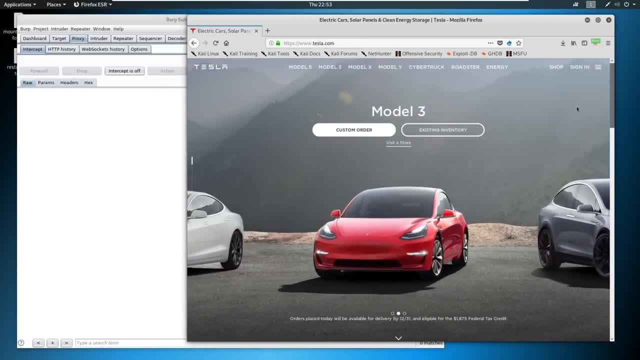 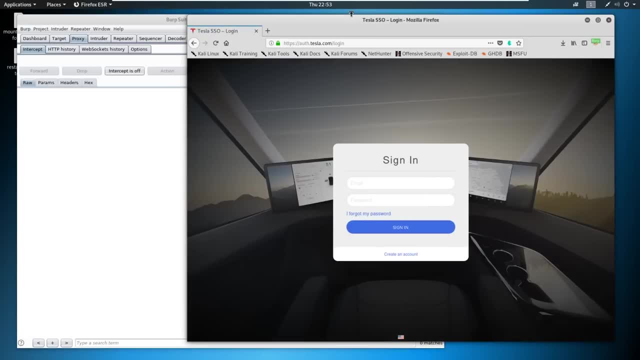 And Tesla should look like this when you go to it. In the upper right hand corner there is a sign in button. go ahead and click sign in. And again, this is just a watch and learn exercise. you can follow along up until the. 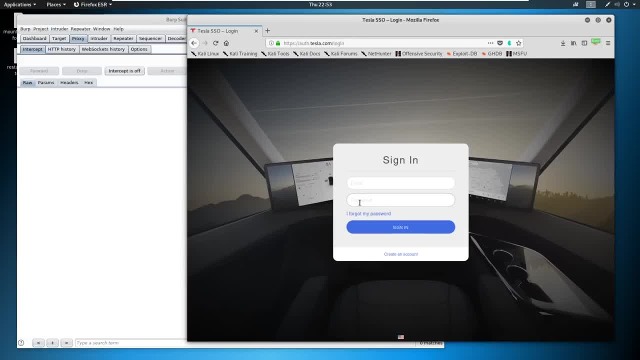 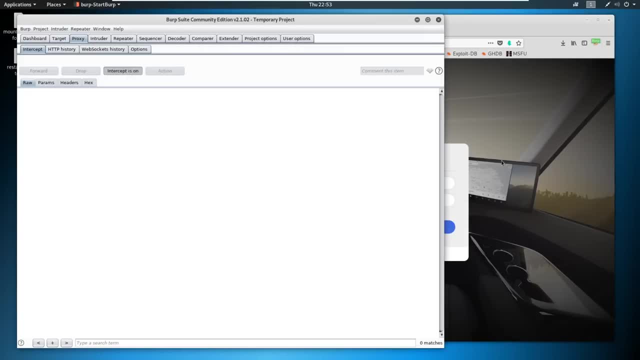 point that we fire the attack. there will be opportunities here in very, very soon, videos where you actually get to do this And you can practice along. So from here, let's turn on the intercept And let's go ahead and just put a fake email. we'll just do test at testcom. 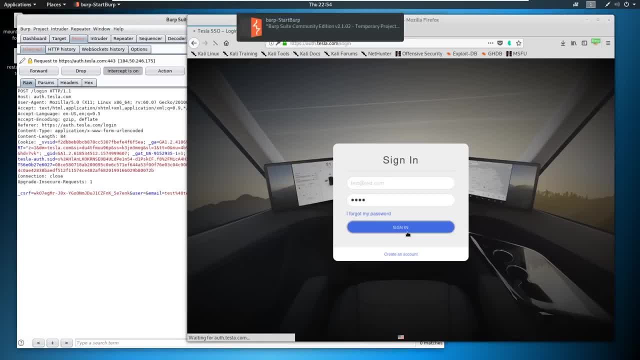 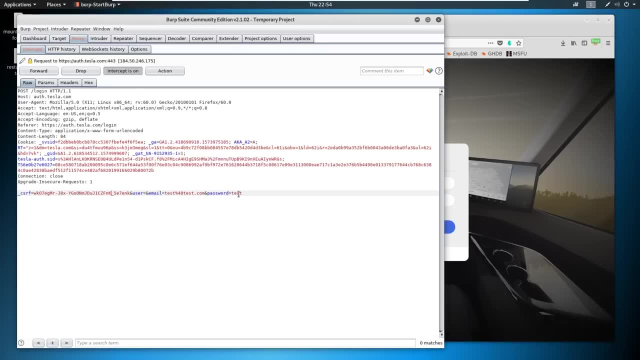 And we'll do test as the password Okay And hit sign in And that intercepts here. So you can see the user equals or email equals test at testcom and password equals test. we're going to go ahead and just right click this and say send to intruder. 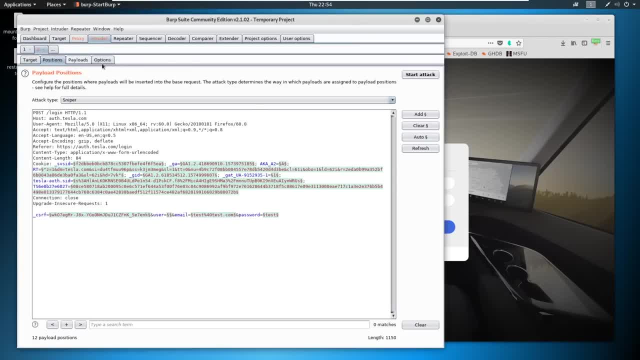 And from intruder. what we're going to do is we're going to go to positions in here And then we're going to clear it. All those green go away, because it tries to auto select positions for us. So now what we're going to do is we're just going to highlight. 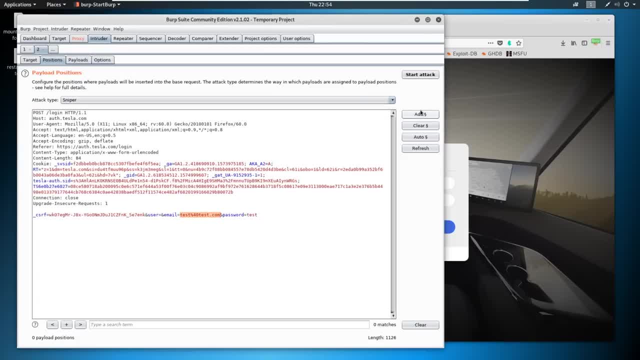 This here And we're going to say add. And then we're going to highlight this here And we're going to say add. So we're selecting two different parameters: We're selecting the email parameter and we're selecting the password parameter. 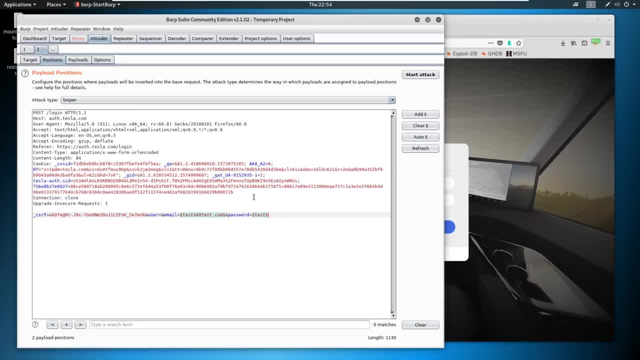 And now we have different attack types up here. the most common that we're going to use is either sniper, but sniper uses one parameter, So we're actually going to use what is called a pitchfork here And we're going to go ahead and go over to our payloads. 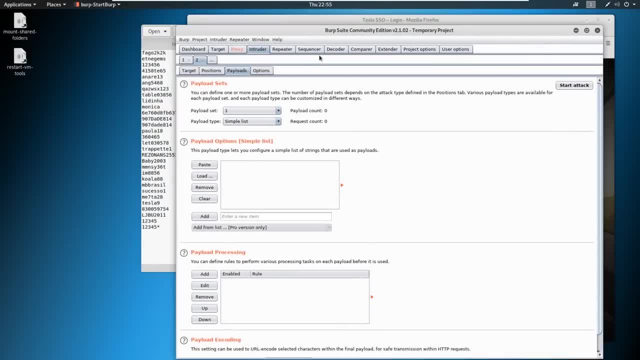 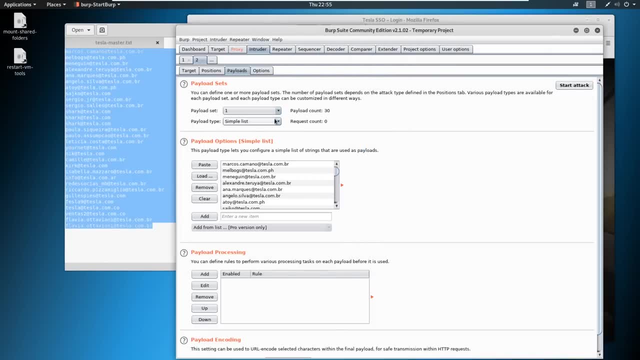 Okay, And what we're going to do, or what I'm going to do, is I'm going to take this list of users and I'm just going to copy this, I'm going to paste it, And then, on the second one, I'm going to take my list of passwords and I'm going to paste it. 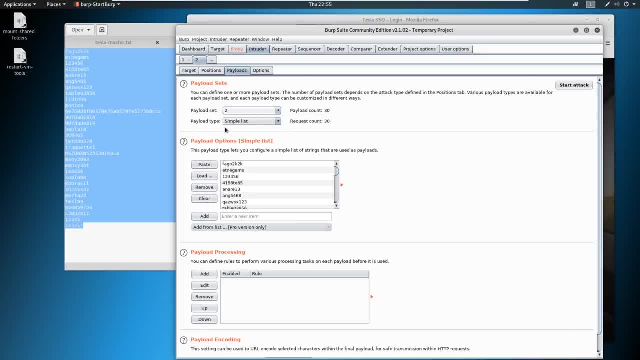 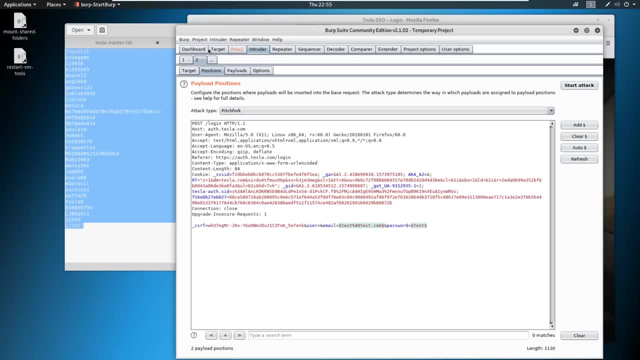 Now what this is doing. if we go back, payload set one is all the usernames. It's going into the first one we set here. Okay, payload set two: all the passwords. those are all going into here And we have 30 total counts. meaning what's happening with this? this pitchfork is payload. 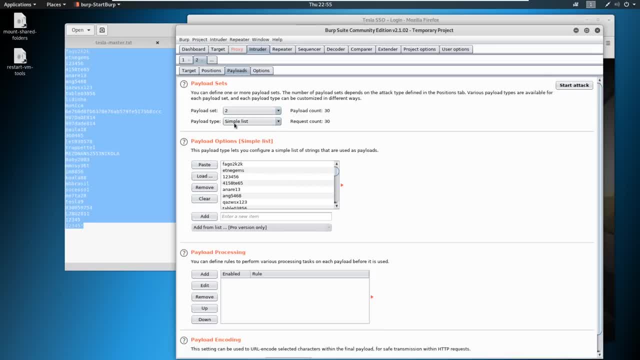 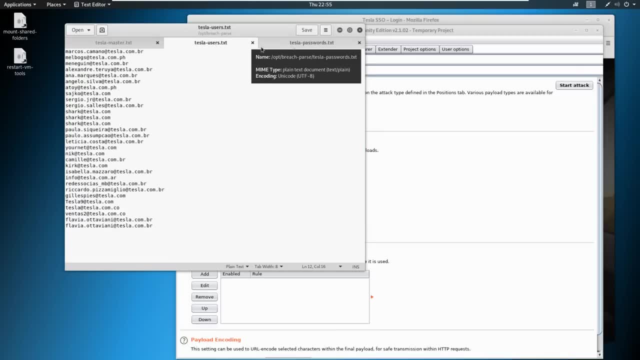 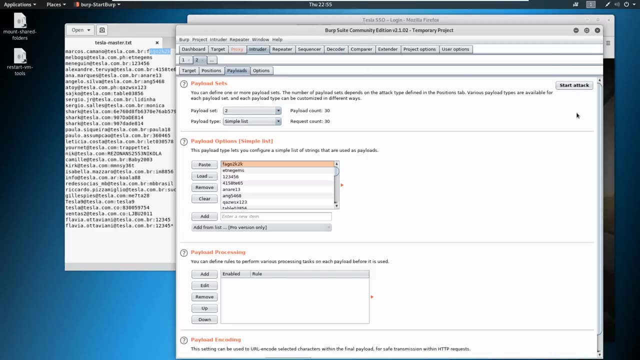 one number one is corresponding to payload two number one, So they only run together. So this will run the username and password. These are just the separated users and passwords. This will run this username against or against this password here. So what we're going to do is just we started. 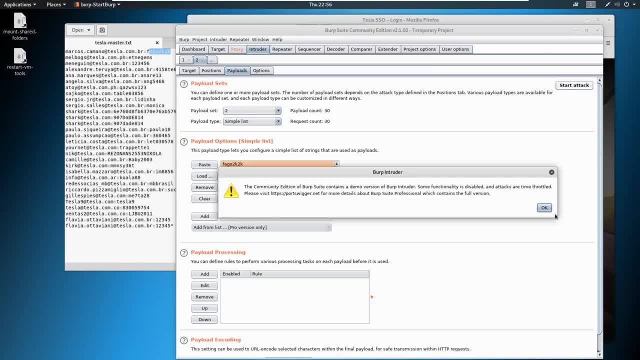 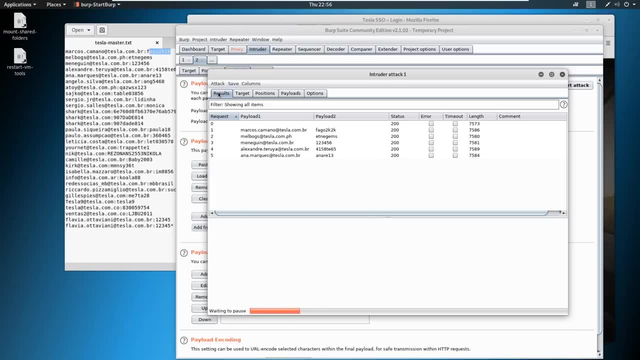 And it just says: hey, this is a demo version of intruder because you're on community, Don't worry about that. It still runs, It's just a little slower. I'm going to go ahead and hit pause on the attack. 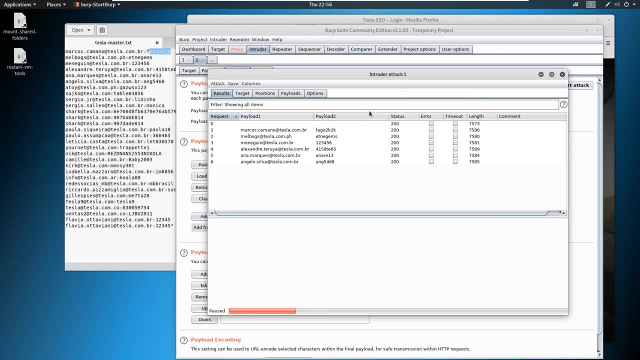 Now there are some interesting things that we can look for when we're doing this. What we're looking for is a status code change of some sort. Maybe we see 200s here and we want like a 301, which means a redirect. 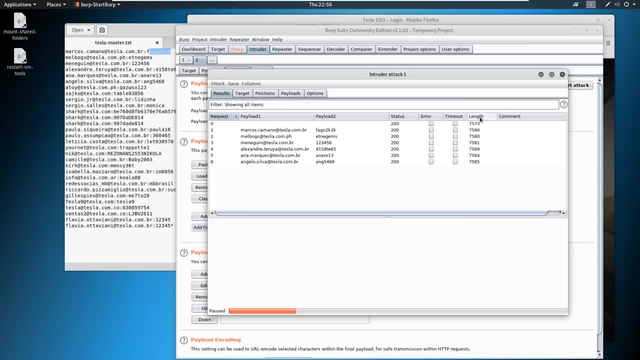 Or we see a significant change in length. That would be a good indicator that maybe we had a successful login. Other items too, is that we can click in here and look at the response and we can say, OK, what did the response say? 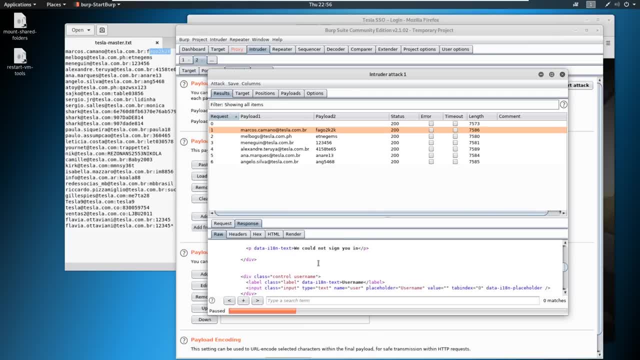 And if we scroll down, maybe it said something in here about fail login. OK, we could not sign you in And we could just take: we could not sign you in like this. Copy this And then we can come back. We'll close this attack. 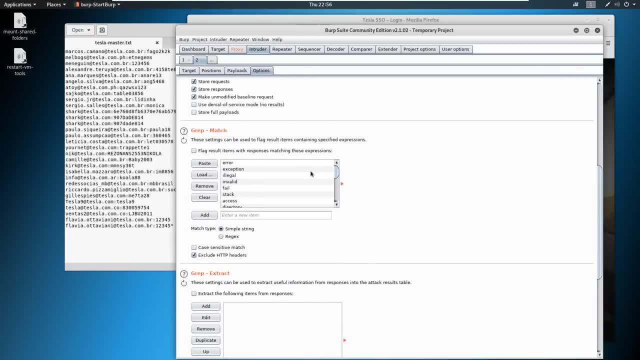 We'll come into options here And there's actually a grep feature So we can remove, We can clear all these In this little box. we can just paste this and say: yes, match, match this here. So watch what this does. 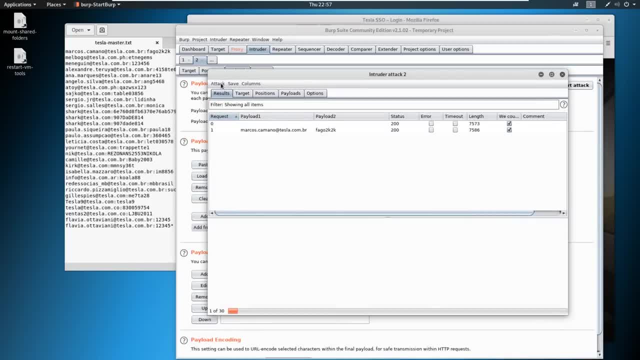 So we're going to start this attack again And then I'm going to pause it. And you can know immediately: look at the checkboxes. This means it's showing up in the response, It's grepping it out. It knows immediately that we didn't sign in successfully. 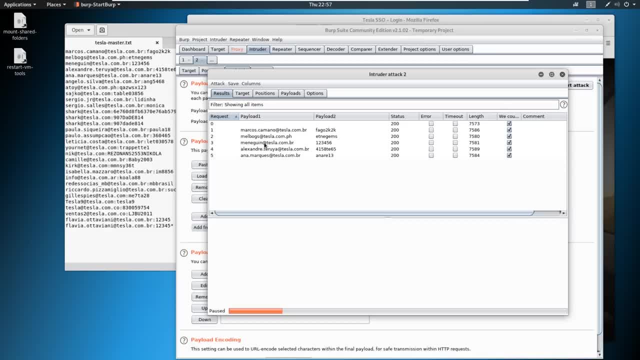 So this is an example of a credential stuffing attack. So we're looking for these few different things: A status change, A significant length, Like we're seeing all the same kind of lengths here, But what if it was like five thousand or two thousand or fifteen thousand? 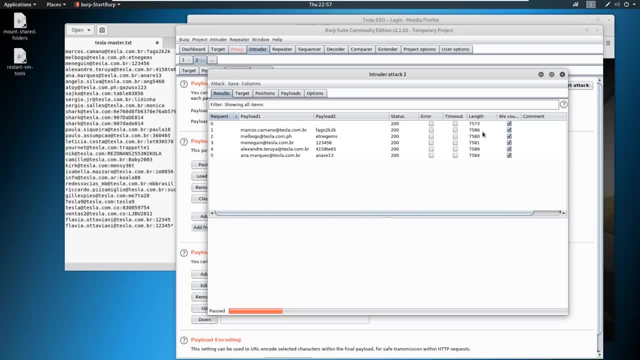 If the page length changes, there's a good chance that you signed into something and we have a successful login. Same thing here with this. If you can find your error code or what it says and then grep on that, then you can click up here and just sort by that. 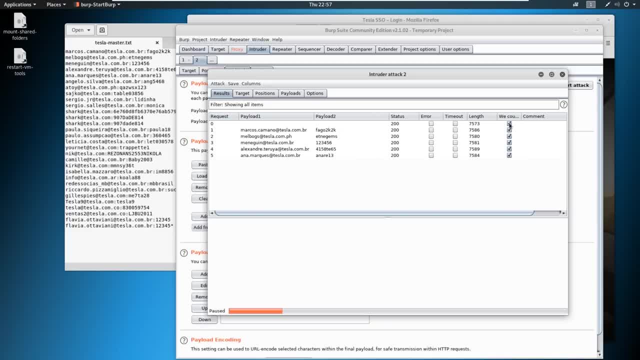 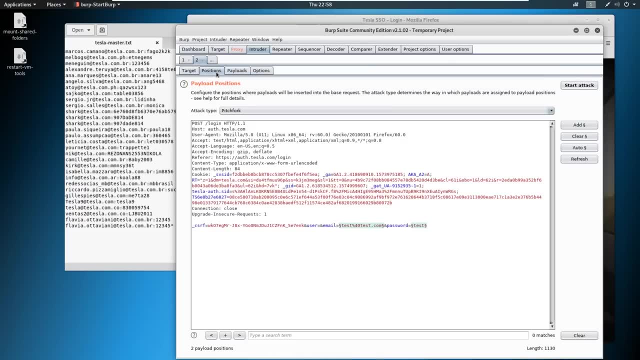 And you can search for the ones that don't return that and possibly have a login as well. So this is the art of credential stuffing. Now let's say we wanted to close this out, We want to go back and we want to do password spraying. 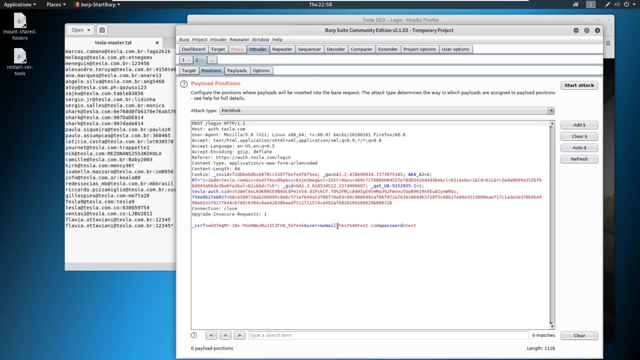 Well, we're going to go ahead and just clear this out And, if you remember, password spraying is the art of using known usernames without a known password. So we'll just say add here and we would gather a list of all the possible users that we can think of. 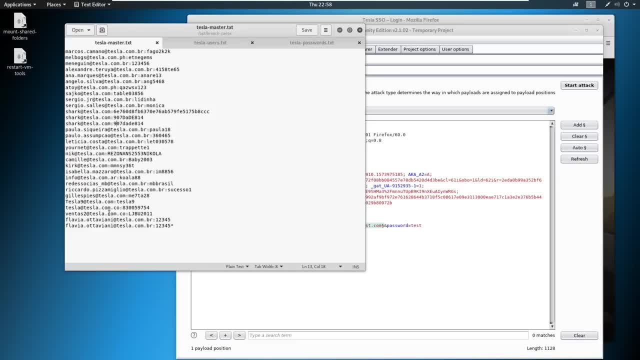 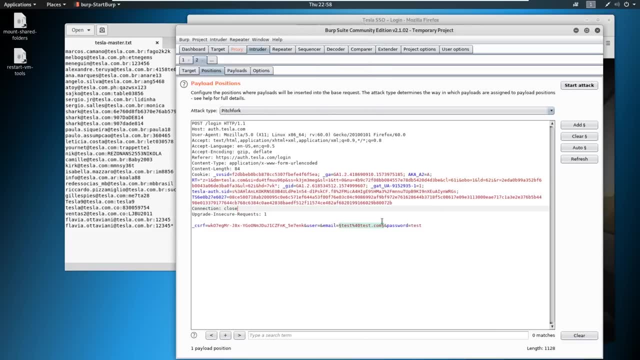 We can look at Hunterio. We can look at, you know, the breach password list. We can look at LinkedIn and gather people who work there, come up with this big list And then actually clear: Sorry, No, this is right. 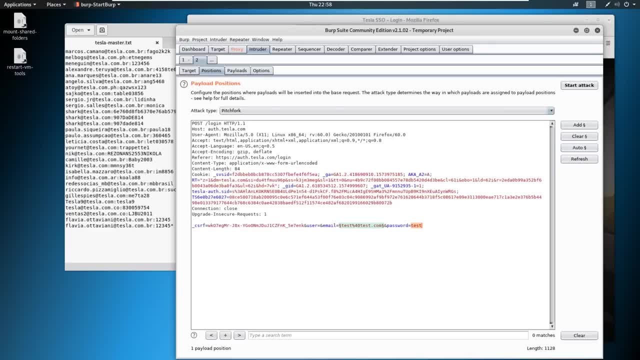 We'll add these and we'll have all the different users And then for this we'll just change the request to like fall of 2019.. Or we can set it up to: we could set this up here like fall 2019 exclamation, or whatever the time frame is, or however you want. 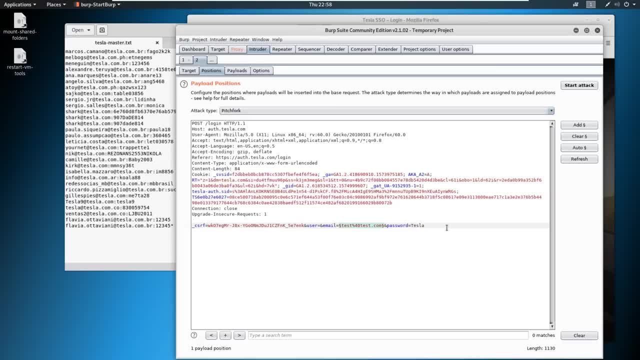 Or maybe you know they work at Tesla, So maybe we'll do Tesla one if they have a weak password policy. or one, two, three or At sign or pound, You just try a few of these. The only downside to this is you are most likely attacking active directory accounts. 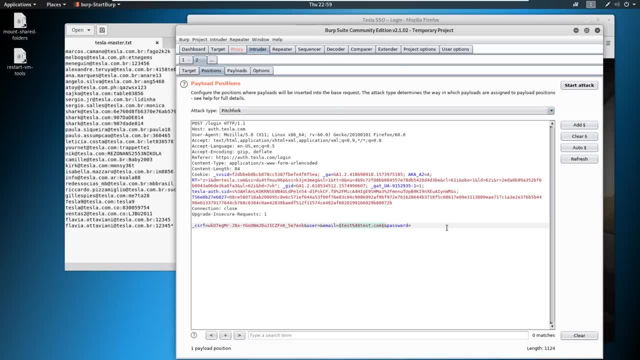 When you're attacking active directory accounts you want to be very careful because you could lock them out without even trying. So if you're doing a pen test, the best idea is to ask before you attack. say, hey, how many attempts do you have unsuccessfully before a logout happens or a lockout happens? 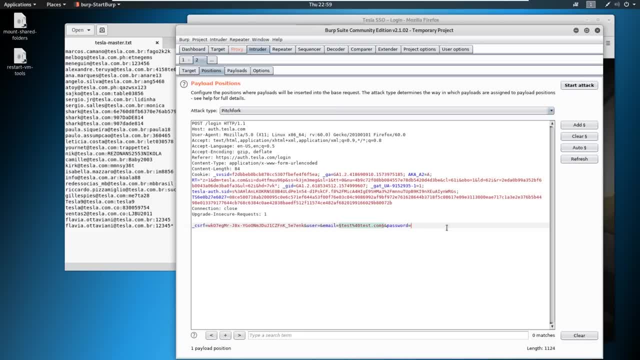 Because the worst thing you want to do is fire off 10 of these in a row, lock out a bunch of users and cause a denial of service. That is very, very possible and very, very easy to do, So make sure you're not just firing these. 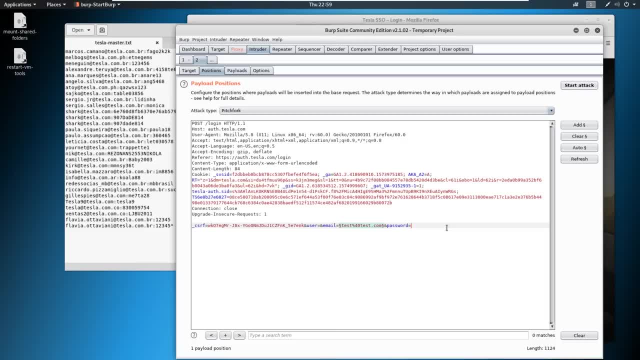 willy nilly that you have a good idea of the password policy, the lockout policy, etc. That'll really help you when you do these attacks. But you just want to do these kind of one or two at a time, wait a few hours, fire another one or two at a time and you should. 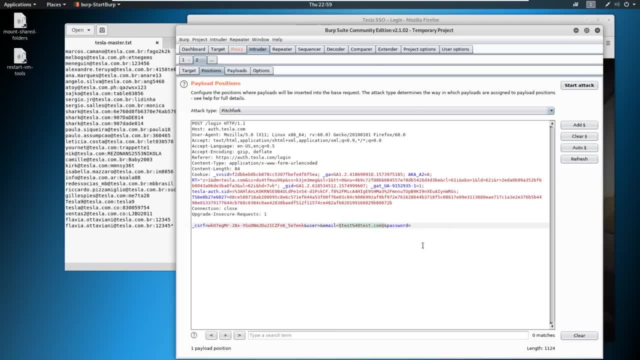 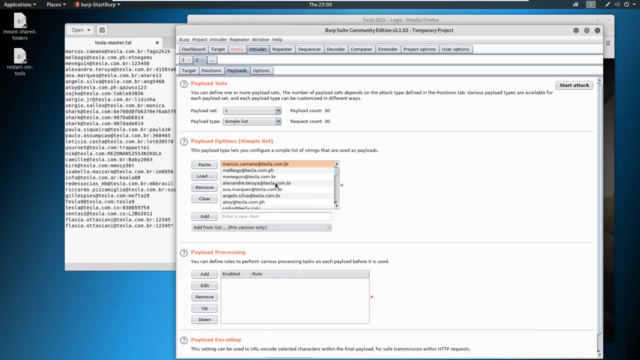 be good to go. Okay, so same deal here. we could fire this and we could just say: you know, I'll just say password 123. And we'll just switch this to sniper here. And if we come to the payloads you can see it just kept the emails. there is no payload to anymore. So what this? 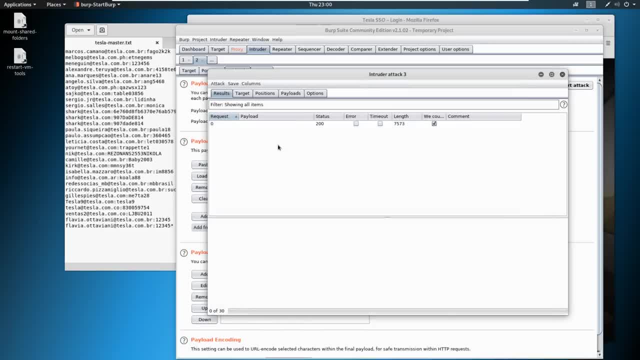 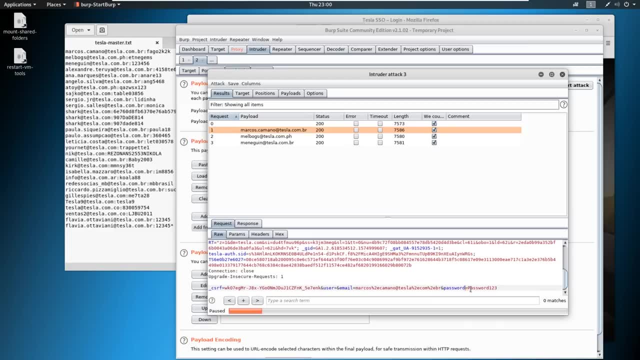 would do if we had start attack is it would start firing this against this email address with a password of 123. And then this one with this email address with the password of 123, it would just go down the list And that's all. password spraying is But the feature that I'm showing you here between 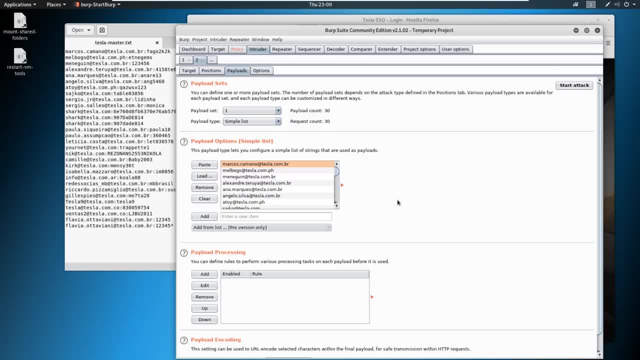 credential stuffing and password spraying is by far the most common way that we get in on external assessments, way, way more than you're ever going to see just an exploit out in the wild, where you're going to see this most likely. And second, you're probably going to see something like: 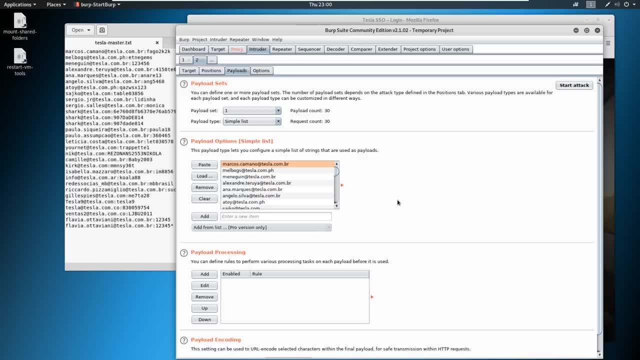 default credentials. So if you see a login page, always check default credentials because you never know, you're likely not going to see a exploit out there, Because the chances are. one is that if you see an exploit like that out there, who knows who? 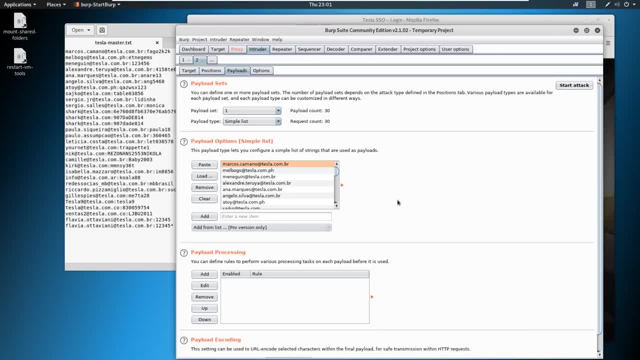 else has seen that already. What kind of bad actors? because bad actors are scanning the internet all the time for these sorts of things, And if they're seeing it, then guess what you know. if you're seeing it, then guess what they're probably have already seen it as well. So that's a bad situation. 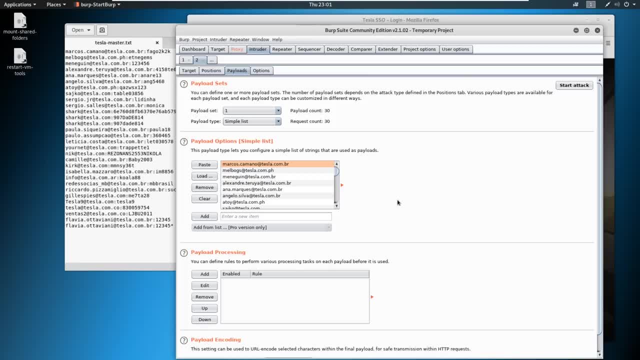 to. you got to think of protection And clients. just think of clients like a house When you talk about the external of your house, your external, your doors have really good locks on them. you might have two locks on your door. you might have good lighting, all this other stuff, right, like to try to keep bad guys out. 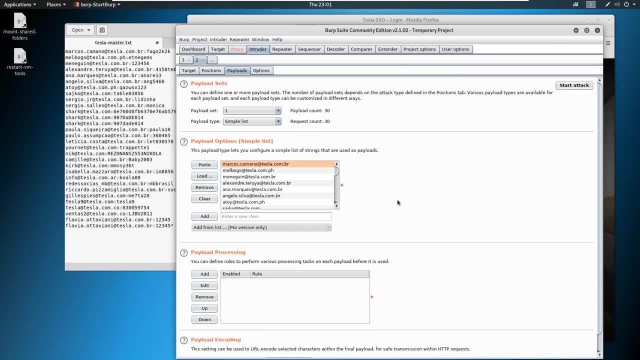 But on the inside some of your doors probably don't even lock, And that's really how you can treat an external assessment. The clients do a really good job of, you know, buffeting up their external, But when it comes to the internal it's not usually as good. So same thing with physical assessments as 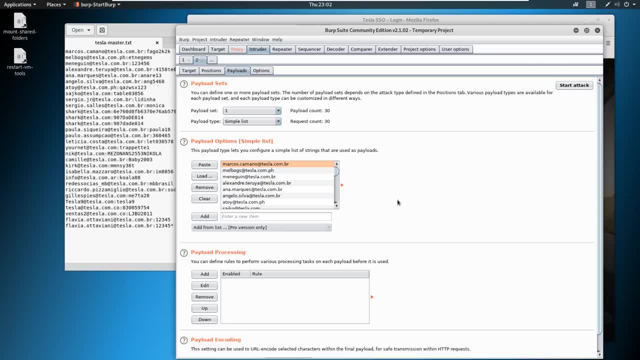 well, you just got to, you got to get inside. Once you're inside, it's kind of easy breezy for the most part. So take that lesson away. If anything you take from the course again, at least for the external side, take away that enumeration and information gathering- super important- because you 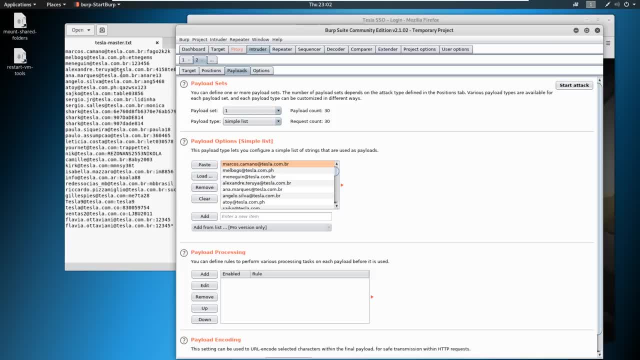 want to get to this stage here where you are doing these credential stuffing attacks And you can use burp suite for it. This is my favorite go to. There's other methods as well, But it's so easy just to grab any different website And, just you know, intercept the. 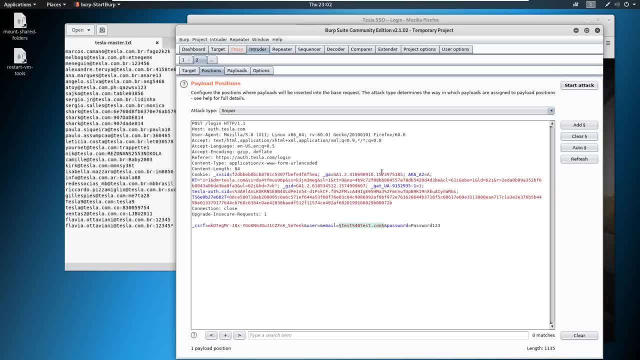 proxy, send it to intruder, make one modification and fire it off. So super, super simple. This is something you will come up in an interview as well, So make sure you're very aware of it And make sure you watch this again if you need. 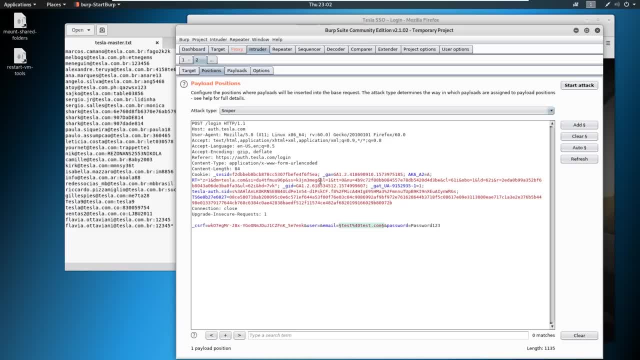 to understand the concepts. So from here we're going to go ahead and take a quick look at our notes in the next video, just kind of where I want you to be with your notes, And then we're going to get into what I call that mid. 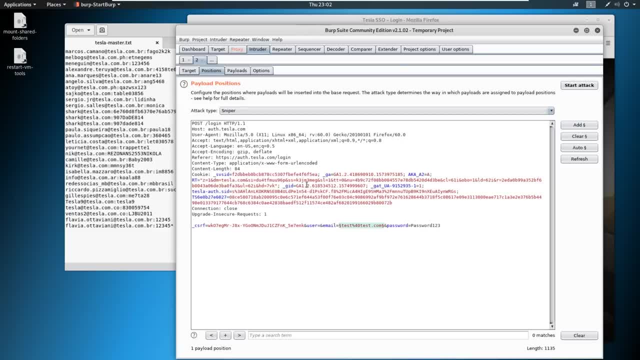 point course, capstone, where I'm going to show you a bunch of different hacks and just my thought process and theories in thinking when I go into a scan and looking at results And just so you can kind of get into the mind of an attacker and how we 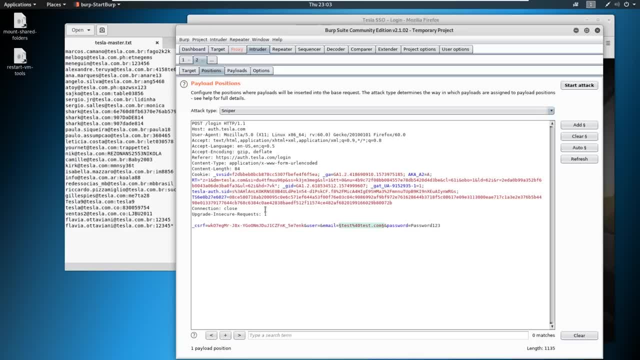 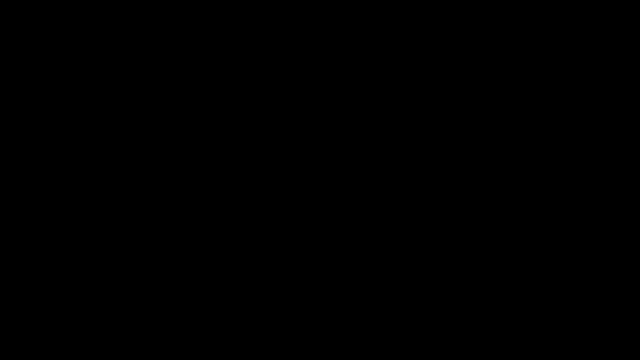 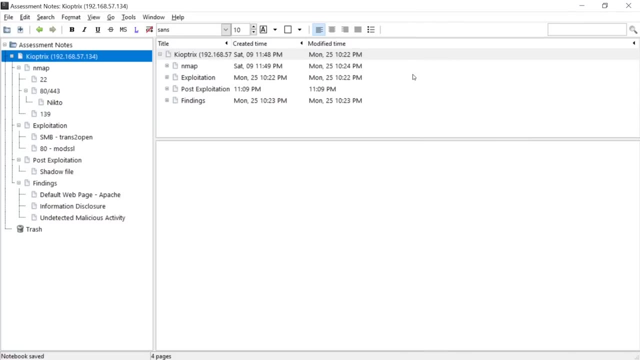 think, And then we'll start moving on to exploit development and my favorite, the Active Directory exploitation. So I look forward to seeing you in the next video. Let's briefly cover our notes so far. So we have covered a little bit of this. right, we covered the fact that we have our end map in here and what we saw in. 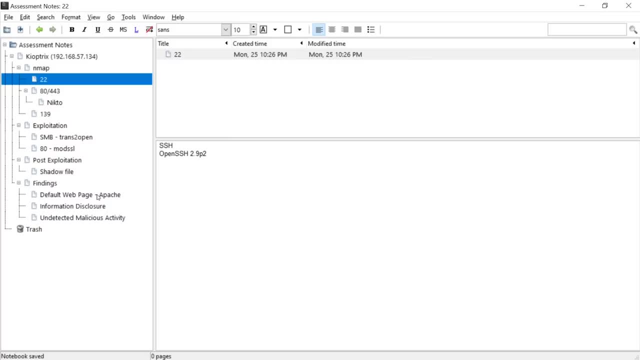 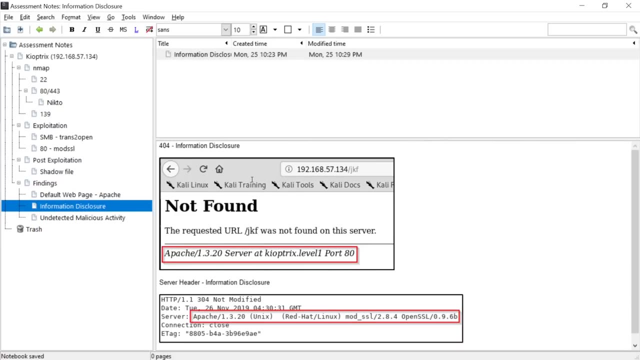 port 22,, port 80, etc. And we had a couple of findings from before. we had default web page on Apache and we had this information disclosure as well. Now we've done some exploiting, So I've gone ahead and just put in here- I put the SMB exploit, So I put an. 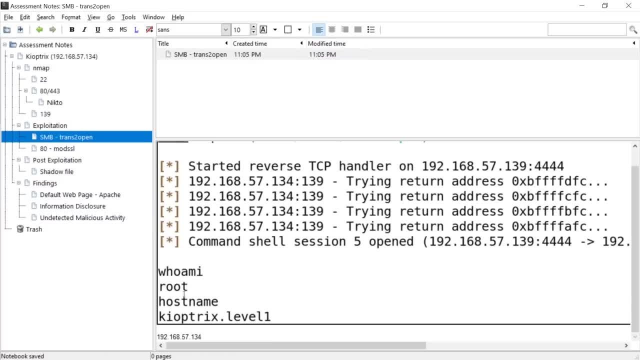 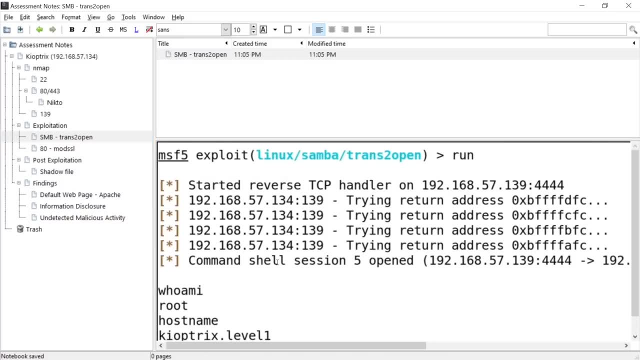 example of what it looks like when we run it And you could see that the Who am I and the host names in there, And then I've got the IP address. this is just for my notes. you can make this as detailed as you want. By the way, you could say: 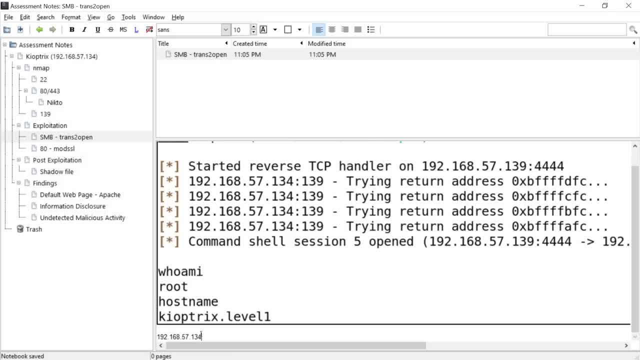 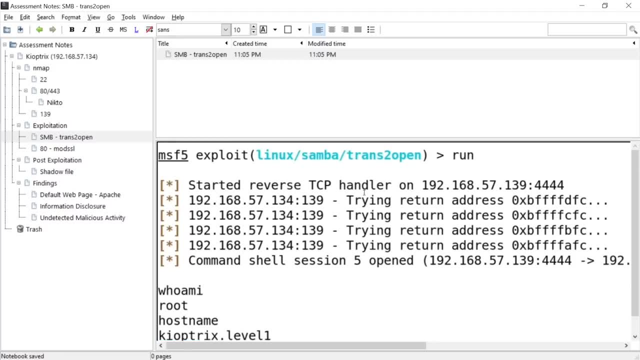 hey, I ran this at this specific time And I ran it against this host And here was the attack I ran, etc. And we'll get more into what your report should look like, But as long as you know- at least for me, as long as I know, or I have a screenshot of proof that I did it and I have the IP address- 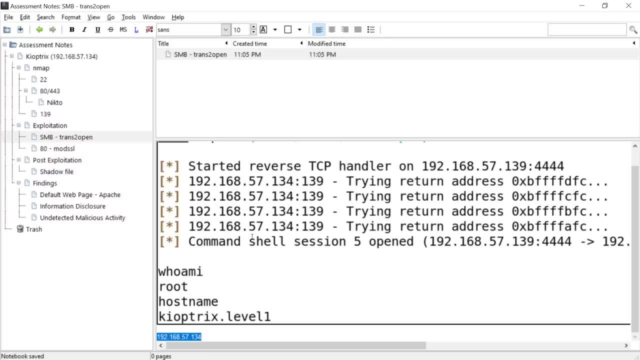 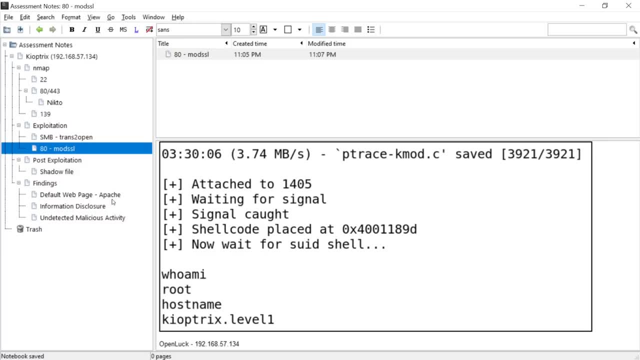 that I ran it against. that's pretty much enough. I can remember the rest and then type out the report. And same here with the mod: SSL attack on port 80. And 443.. And I don't have a copy of it right now, But the shadow file. we did uncover the shadow file as being a root user, So this: 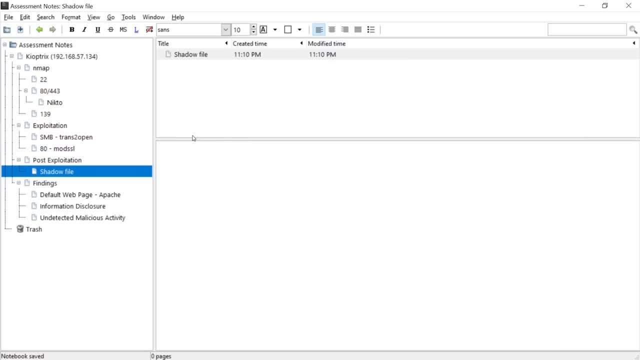 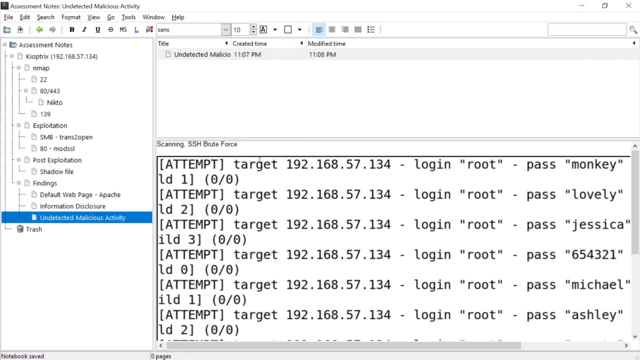 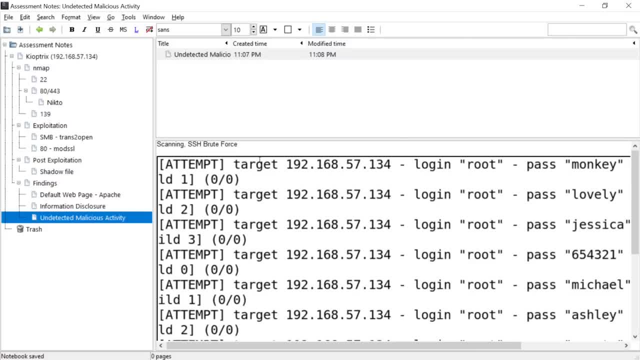 to see on a report And we talked about in the- the brute forcing video, where if we're doing any kind of brute forcing, we're doing it not only to see if we can get in with a bad password but to see if the client catches us. So in this example I'm just going to say, hey, they didn't catch us. 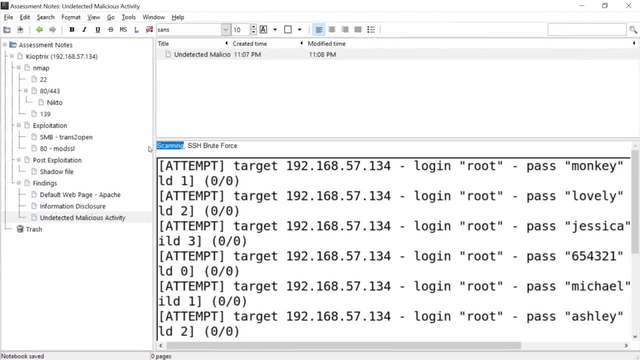 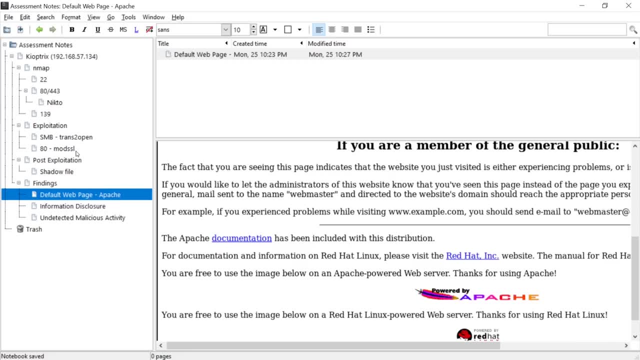 Here's an example of what we did, Also scanning in there as well. If you're not seeing a scan, that's something that we're going to report back, So this would be typically a low finding. these would also be low findings Anytime we get access to a machine. this is obviously critical. 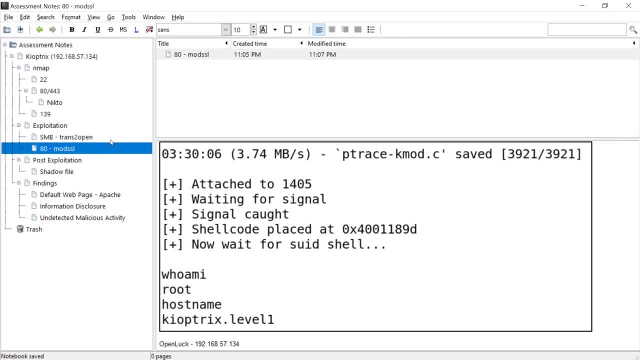 finding. So we just want to keep note of you know what kind of things we're finding, take good pictures, etc. So I'm hoping that you are getting the gist now of what your notes should look like again. make these your own However it feels good to you. This is just how I kind of do it. I don't 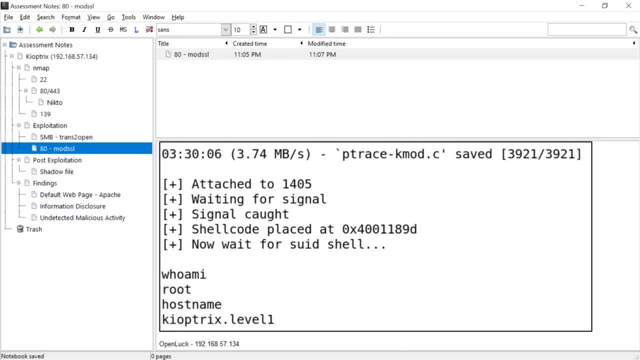 have to put a ton of information in there for me to remember, as long as I have my screenshots, which are most important because that's your proof that you were actually there and you did it. Otherwise, it's just: he said, she said, kind of thing. So that is it for this video. That is it for this section. 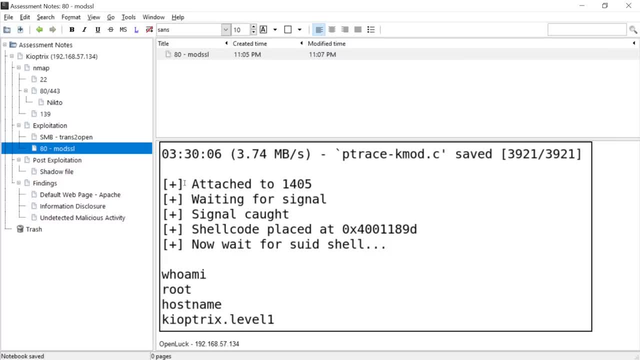 congratulations again for making it this far. Now we're going to move into some of the fun stuff where we get to look at a bunch of different attacks and gradually just get a little bit more complex and learn some new things along the way. And I like to call this a capstone because 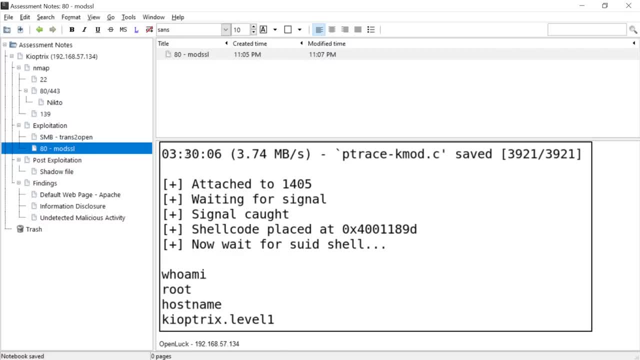 we're capping off where all the things we learned so far we're gonna actually build upon it. So you're gonna learn a bunch of new little techniques as we do this little mid course capstone And then we're gonna get into really fun stuff Once we get into Active Directory. I'm really excited for that. 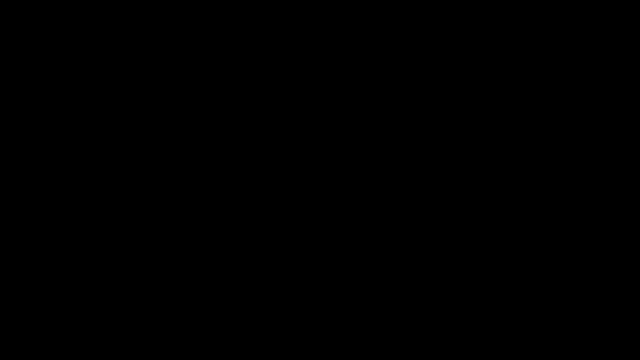 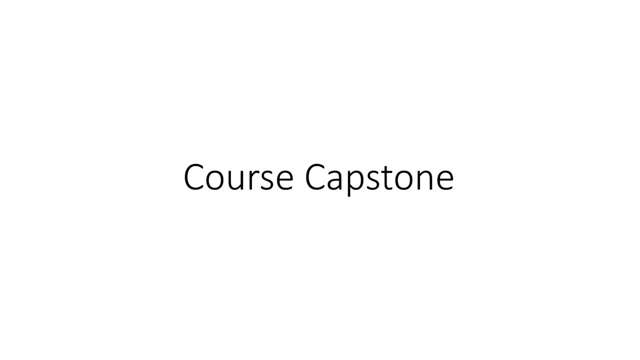 So I will catch you over in the next section. Welcome to the course capstone. This is the 2021 edition of the course capstone And we'll get into the old capstone, the new capstone and what the differences are, But the course capstone. 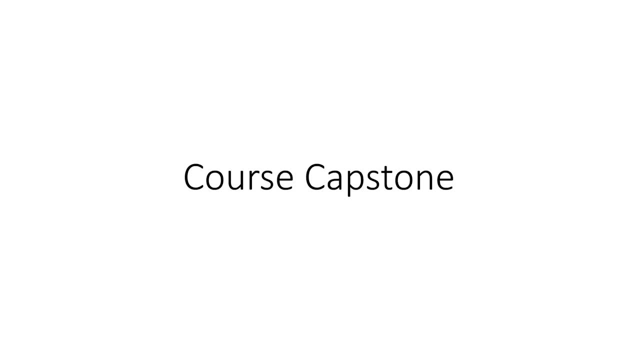 is meant to challenge you and test your skills and knowledge up to what you've learned so far. Now, not everything is cut and dry. These boxes are not meant to be particularly easy. They're actually meant to be learning experiences. So what that means is you are welcome to go through these machines on your own. 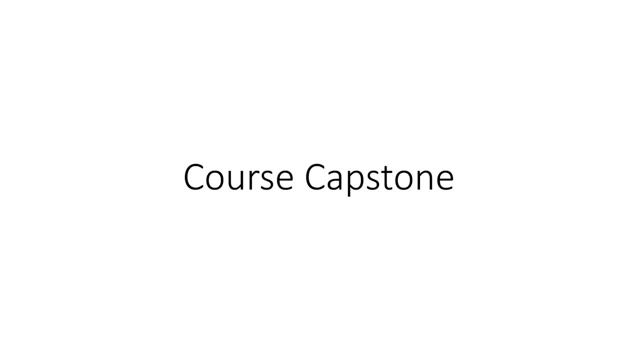 give them a try. I realized that we have not talked whatsoever about privilege escalation. We have not talked about a lot of the tools that you're going to see, And this is by design. hacking is not going to be able to show you. a course on hacking is not gonna show you everything. 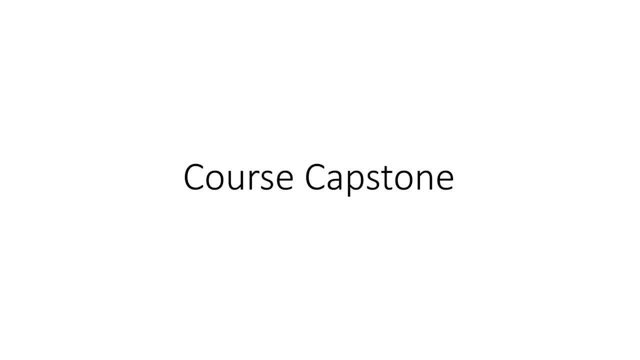 but you're going to get to pick up some ideas and a little bit of Googling and a little bit of frustration and really just getting in there getting your hands dirty and seeing what you can come up with. So I encourage you to try these on your own, in the order that they're listed: 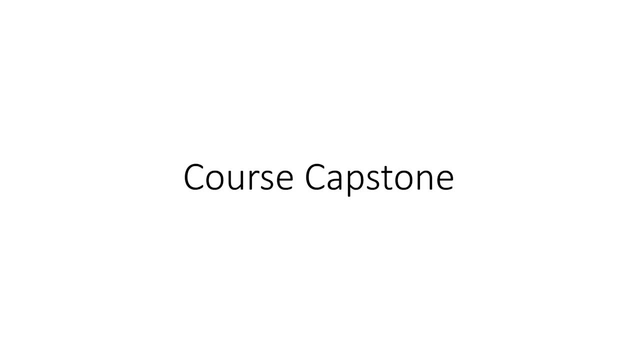 However, if you want to just watch and follow along, that's absolutely okay as well. Now I mentioned privilege escalation, but we'll talk about that here in a second. I want to show you the old course capstone, and where the new course capstone is, So I have uploaded the new course. 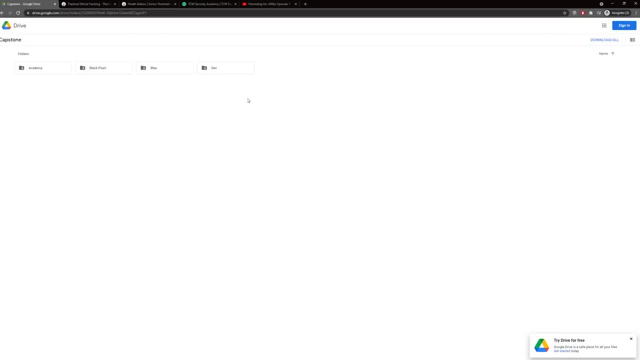 capstone. This is not all the machines yet. This is just the ones that I started uploading. All you got to do is go in here and download these machines. You can run them with VMware or virtual box. I've got set up instructions for a couple of the machines. Once you've seen one, 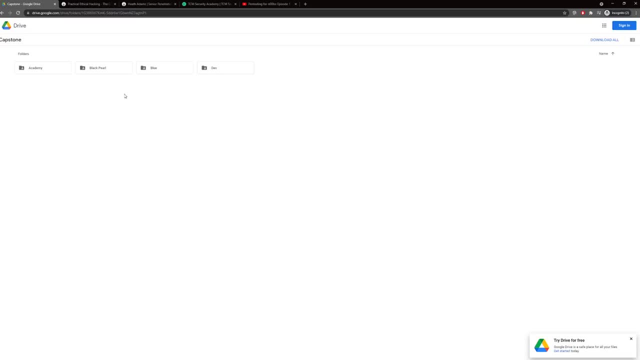 windows or one Linux. you can see them all and how to how to download them and run them. So that's pretty straightforward. The link will be provided in the resources or you can download them from the link that's in the description. So if you want to download them, 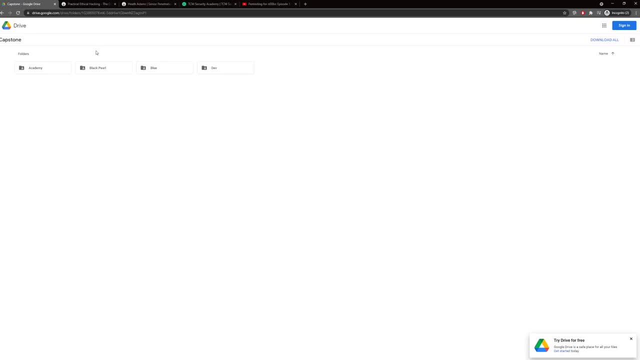 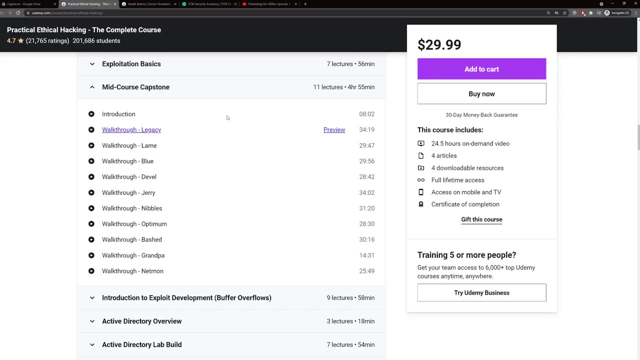 you can download them from the link that's in the description. So if you want to download them from the below the video, depending on what platform you're on Now the old capstone. here's the old capstone. I have not pushed the new update yet, So this is what the old capstone looks like. 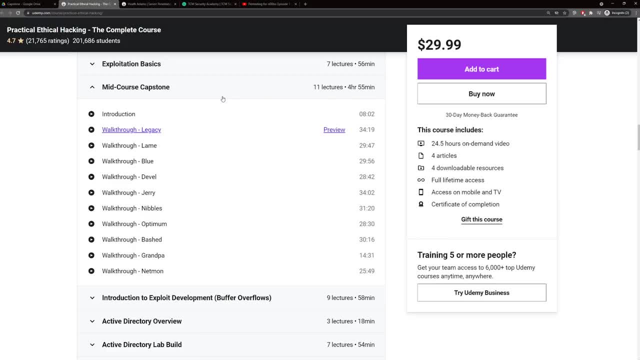 You could see there are 10 boxes. There were five hours of material, or was five hours of material? The issue with the old capstone was that we were relying on a platform called hack the box. hack the box was a paid subscription platform. It costs anywhere from 10 to $15 a month. I'm not 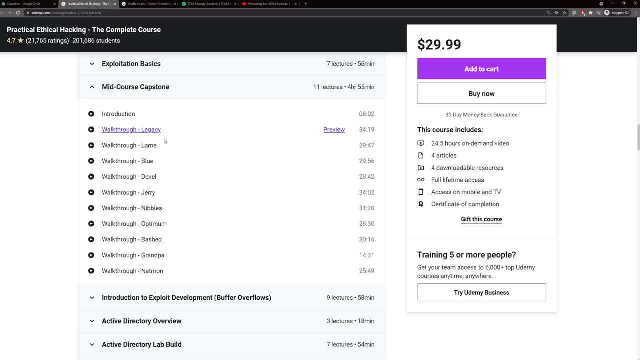 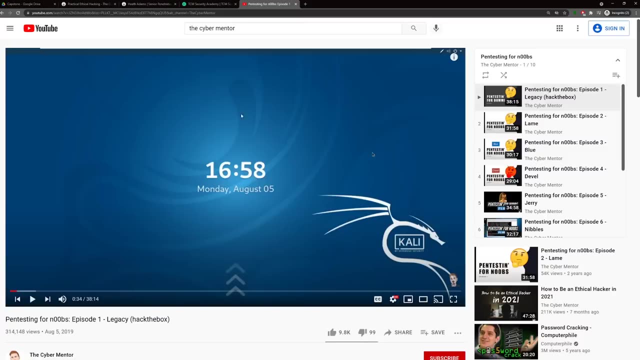 sure exactly of the true costs, But I realized not everybody can pay additional funds to go and use this platform to walk through these machines. So what we have done is we have made these machines available via YouTube. So I'm going to put this down below as well. But there is a series. 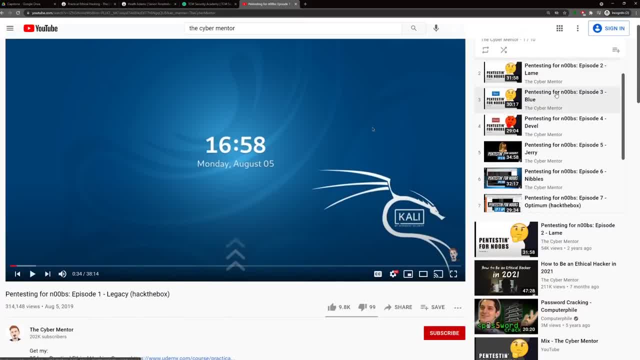 originally released, called pen testing for noobs. If you look, all 10 of those machines are going to be here as well, So you're welcome to come to the YouTube channel and watch these videos, And I'll see you in the next video. Bye. 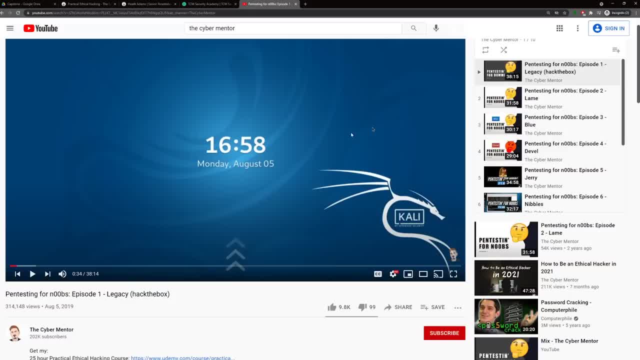 extra content, extra walkthroughs in, more of the practice and more of the capstone. you're welcome to go sign up for, hack the box, do all that, But we are removing that dependency from the course. Now these machines are going to require what is called privilege. 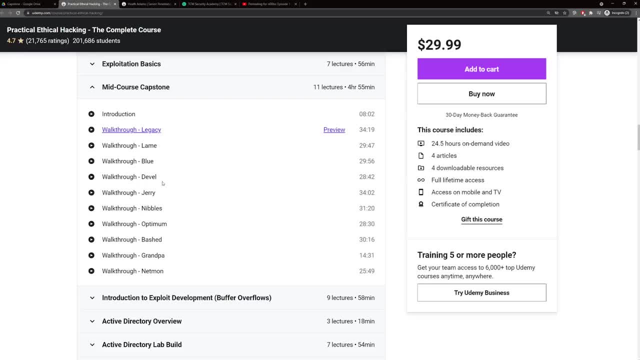 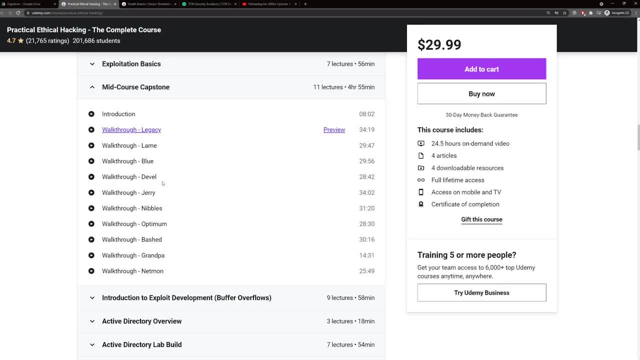 our privileges to the highest level that we can. So all of these machines, except for one at the time of this recording, are going to have some sort of privilege escalation involved. Now you're going to get to see some cool tooling, some different techniques and tactics, But it's not. 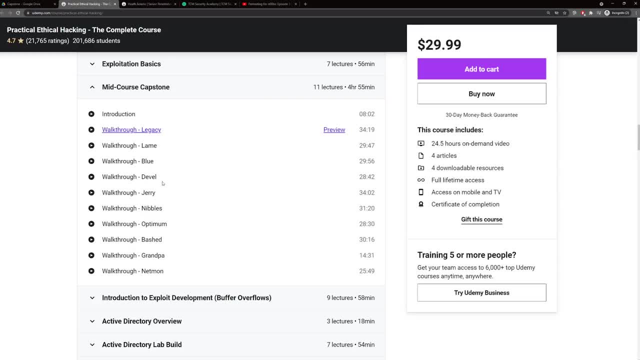 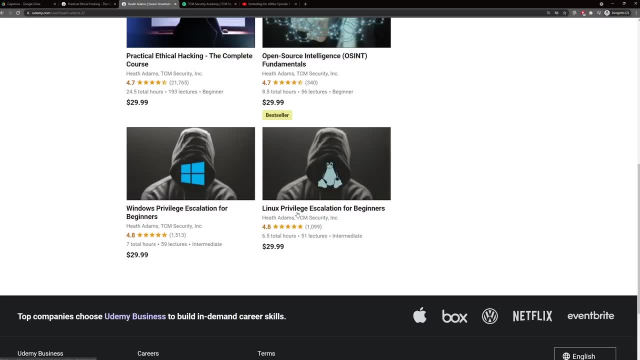 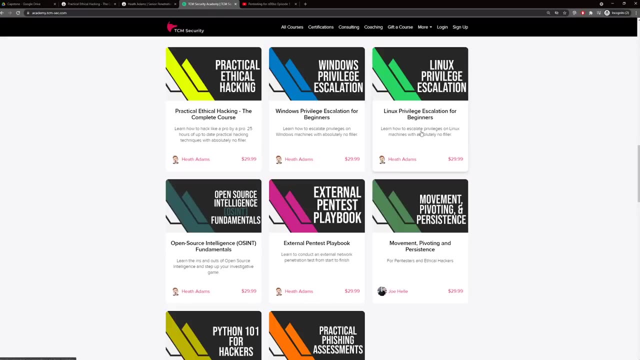 going to go into super depth on this. There are courses out there that we have created. We have two here: the Windows privilege escalation for beginners and Linux privilege escalation for beginners If you are on Udemy, if you are on the Academy. same concept: Windows and Linux. 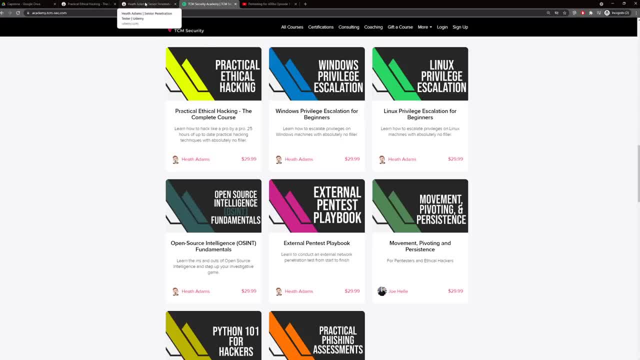 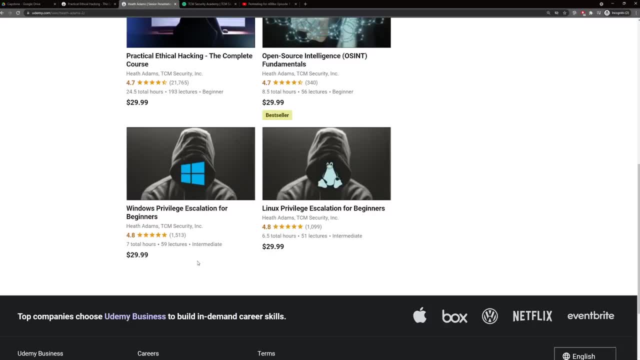 just depending on the platform you're on and which one you you prefer. So if you're interested in going after any sort of certifications, if you're interested in doing any sort of capture the flag or getting better at just escalation, in general highly recommend these courses If you're looking. 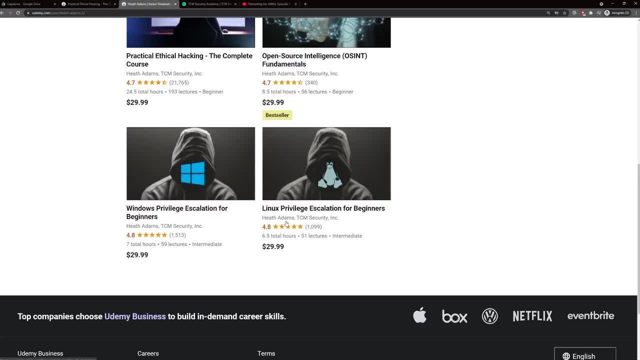 to stay kind of on that practical path, then these aren't really necessary. It's really based on chasing certifications in the hacking realm, like your OSCP or some of the other certifications that might be out there. they use a lot of privilege escalation to test on. But again, it's not really. 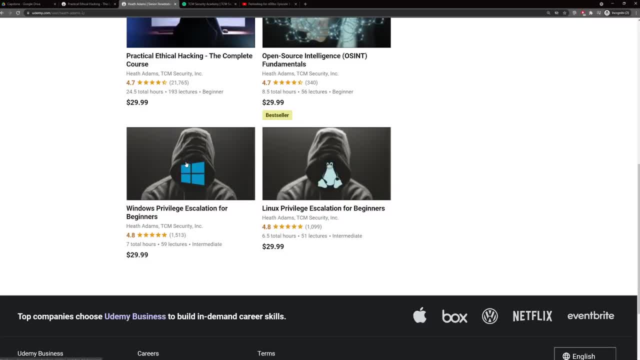 on the practical side of things. So, depending on what your motivations are and reasoning. however, we are going to show them in this course only because they are a good introduction to hacking. it's good to see the other side. it's good to see some of the exploits that are out. 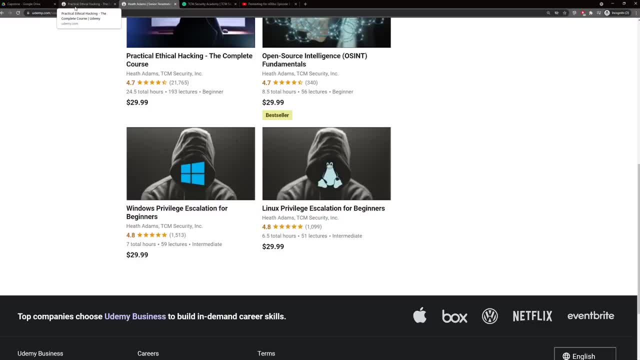 there some of the thought processes that are out there And then, once we get into the active course, we're going to take off from a practical standpoint And we're really going to start hacking like we are hacking in a real network and it's going to get really fun. It's my favorite. 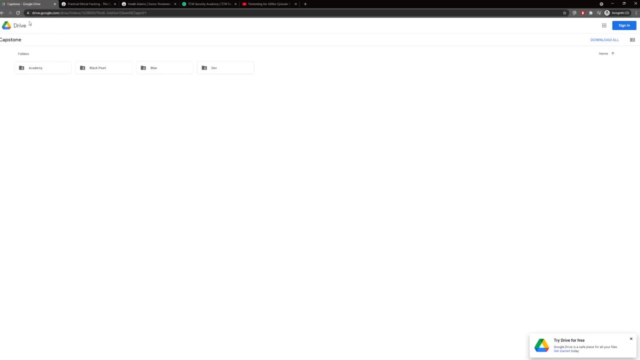 section in the whole course. So, with that being said, go through the courses again in order as you see them. So, however, you see them in the list, go ahead and go through them. We're going to add more courses over time. As of right now, the dependency is that you download these and install. 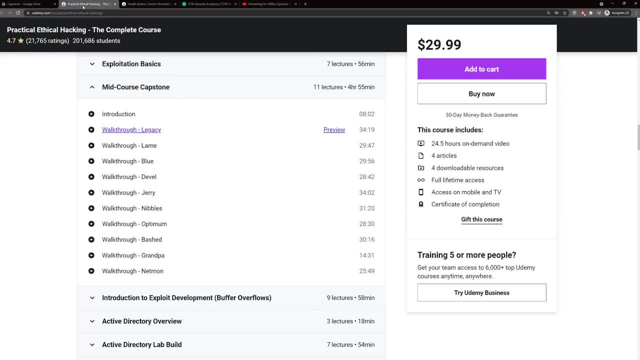 these for your lab. Again, there will be instructions for those. In later attempts we're hoping to offload these to an online lab. Unfortunately, we won't be able to do that with Udemy, But with the academy platform we should be able to do that. So we're working on getting that, but for now, 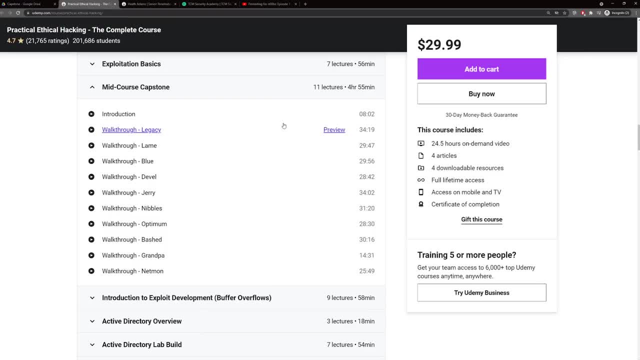 the Google Drive link that you see attached to the introduction video. this video will have all the files that you need to download in order to complete this section. So, with that being said, go ahead and complete the next box. I'll see you in the next video, and hopefully you rooted it. 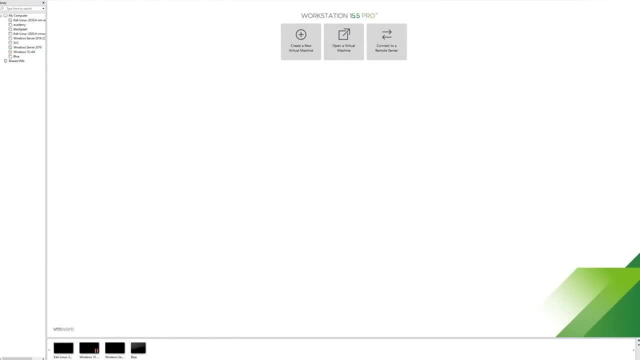 in. So, before we begin the capstone, I want to show you how to import a machine, And I'm going to show you, starting with blue, how to import blue, which is a Windows machine, And then we're going to go ahead and import a Linux machine and a later video, So that way you should know how to do both. 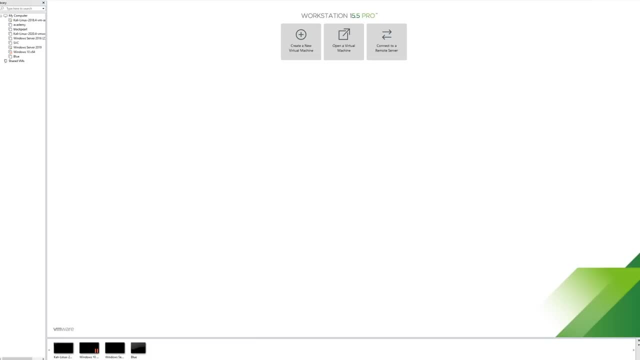 though the process is exactly the same. So for blue, what we're going to do is we're going to come into VMware here and I'm going to show you VirtualBox as well. We're going to go open virtual machine And you're just going to select the file that should be available to you here, which is: 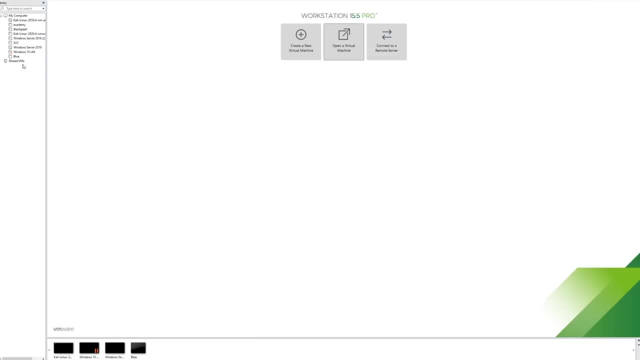 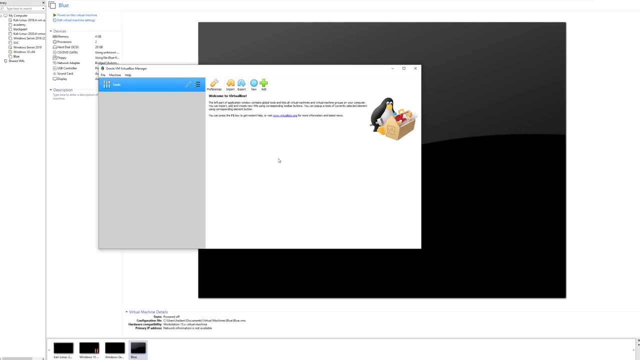 blue. I've already done that through the magic of editing, So it's already here And I'm just going to go up here and show you that we'll get to settings here in a second. For VirtualBox, same exact process. I'm going to go ahead and just go to import. I'm just going to paste the location in. 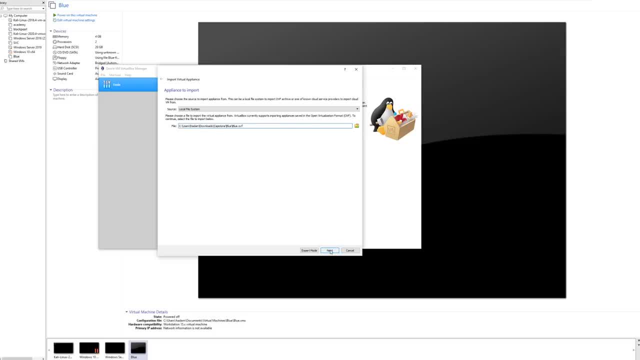 here. you can also use this to go find your file And I'm going to hit next and import. Okay, and it should start importing this file. So I'm going to go ahead and import this file And I'm going to paste this file. So here we go. it's importing. it'll take 50 seconds. that's fine, gives me time. 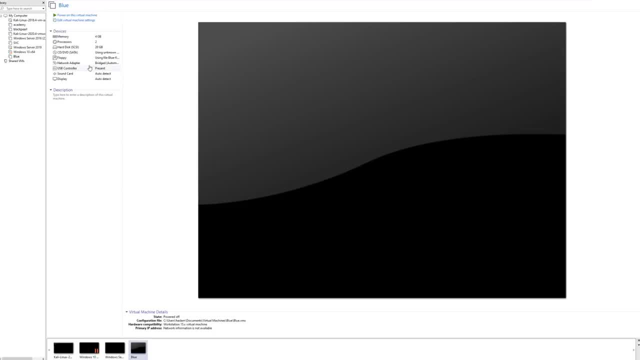 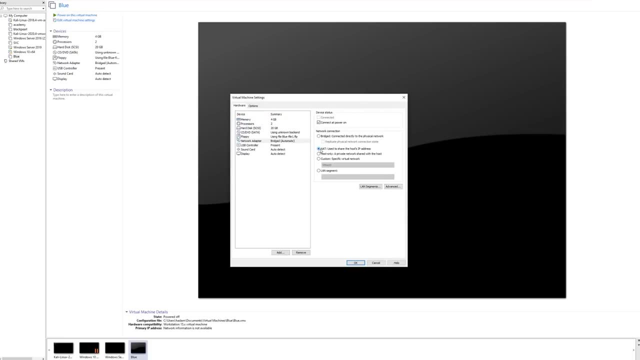 to talk about the settings. So you can see here that we are in bridged mode. Okay, we don't want to be in bridge mode. let's go ahead and edit this, go to bridge And we're going to turn this into actually just net. Now you can choose how much memory you want to use here. mindset to four. 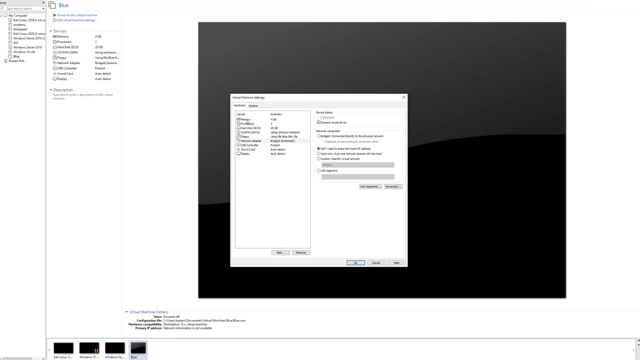 gigs. that's fine. I've got a lot of RAM. if you do not, then go ahead and maybe turn this down to two gigs will be absolutely fine. Okay, so I'm going to hit OK here, And then I'm going to hit. 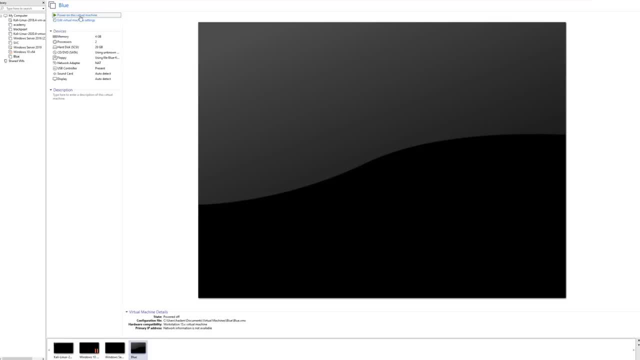 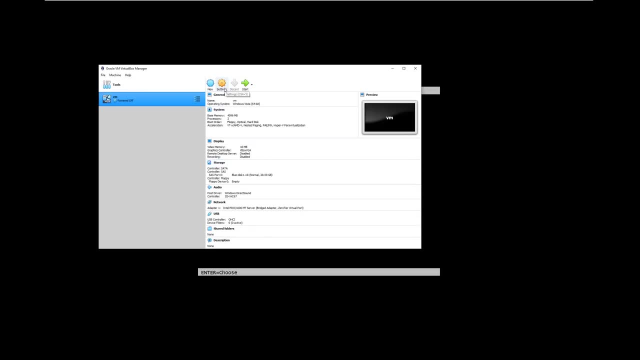 here. Now I'm going to power on this virtual machine And then we're going to wait for the other one to finish importing which it has. So here, while we're waiting on this, go ahead and go to settings, And you're going to want to do the same thing. So, network, no bridge, don't do bridge. 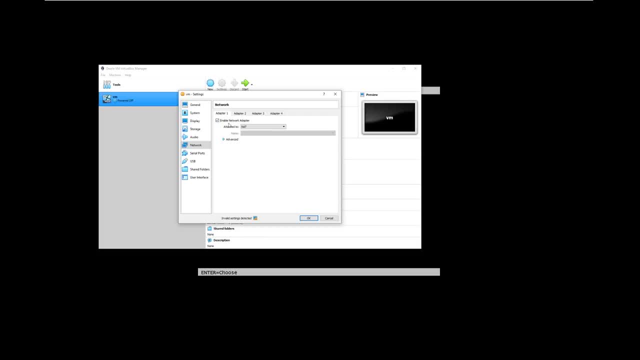 we're going to do net, Okay, And then we're going to just enable the network adapter here, So you should have your net network set up. Remember that when you you did that originally with our settings. if you need to, you can go ahead and hit import And then we're going to wait for the 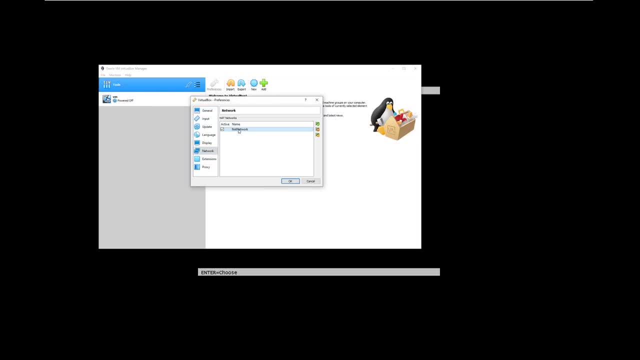 network adapter, And then we're going to go back to tools. you can go to preferences. come in your network, make sure your net network is set up. Anyway, come in here. you can go to your settings And again make sure that this is on NAT. So, or NAT network, I apologize, NAT network, right here. 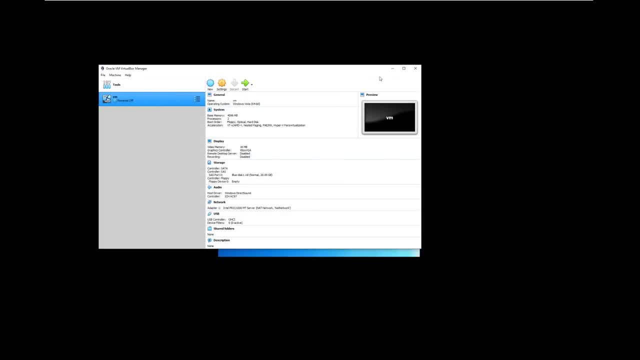 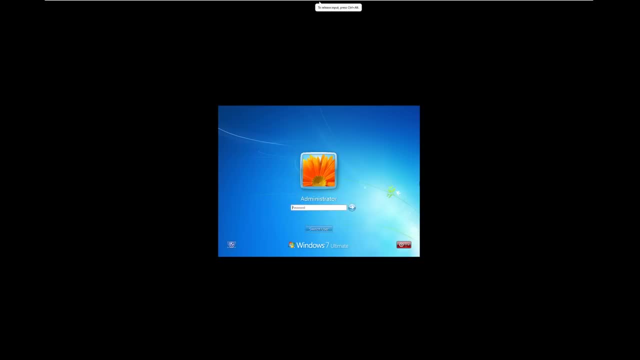 Okay, And then I'm going to hit OK, And then all you need to do is power this on. I'm going to show you with the virtual or the VMware, it's going to be the same process. Now you can log in as the. 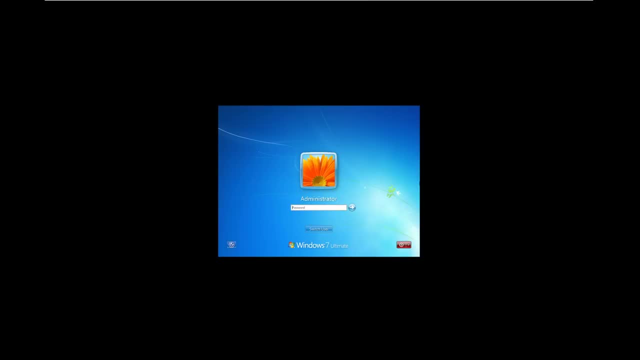 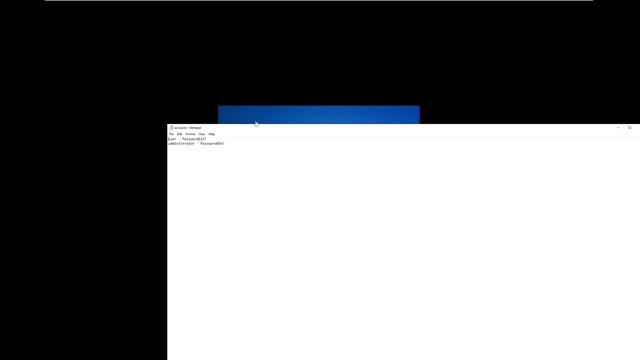 administrator, you're going to get all the credentials for every box. that is for the sole purpose that you can access the IP configuration and find the IP of this machine. Okay, just to make it a little bit easier, So there will be an accounts file in here And here you can see the administrator password is password. 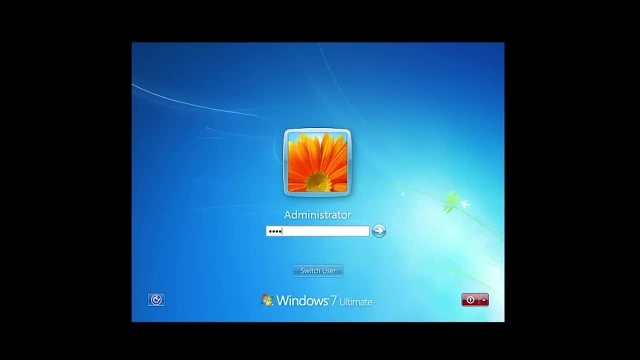 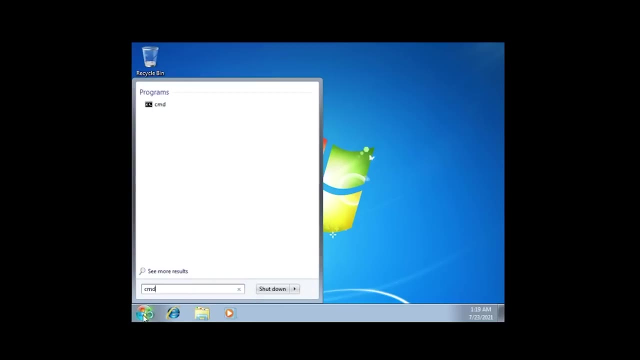 456, exclamation. So we're just going to do that And we're going to make sure that this box is online and that we can communicate. So I'm going to quickly go to command And you can install VMware on here. But if you want to, you can install VMware on here and then we'll see what you want. 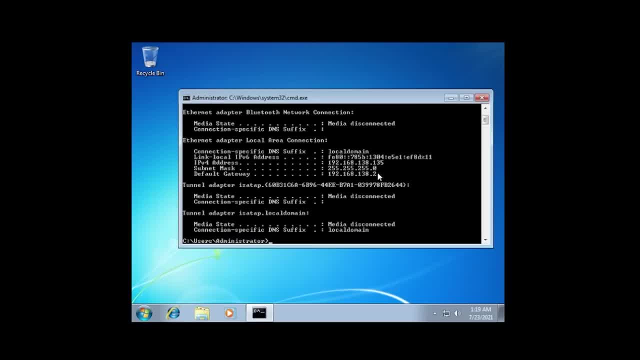 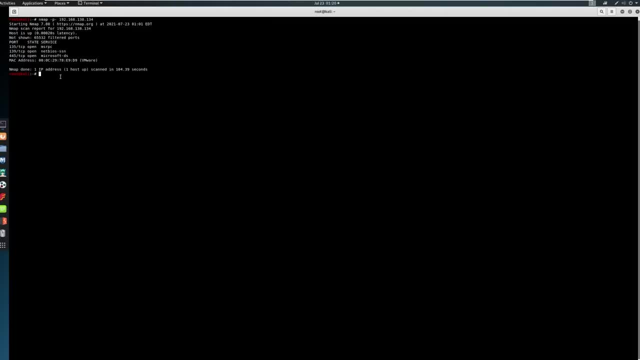 Make this pretty, all that jazz. I'm not going to do that here. I'm just going to quickly figure out what's what's what you can see: 192, 168138, 135.. I'm going to come over to Kali Linux. I've got a scan. 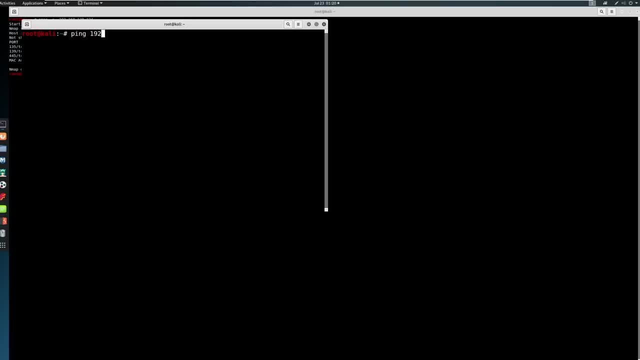 that we did for 134 up. that's okay. I'm just going to ping 192: 168138.. 135.. Okay, and you can, And that's it. you need to make sure that you can communicate with your machine, So if you're. 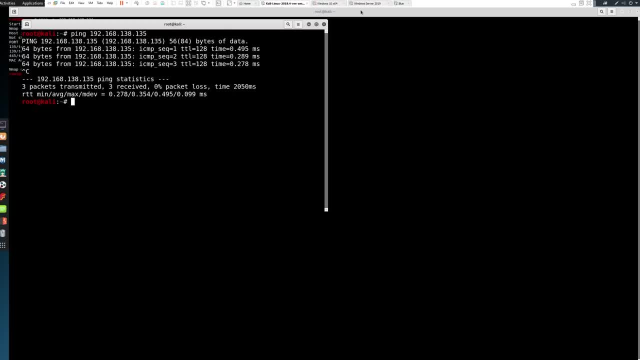 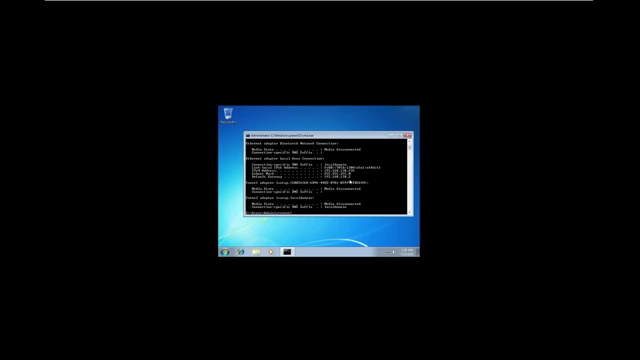 running VirtualBox. make sure you spin it up, you log in, you figure out what it is that your IP address is and go from there Very, very straightforward. So that is it for this video. go ahead and attempt to attack blue. see if you can figure out what the deal is and where you can. 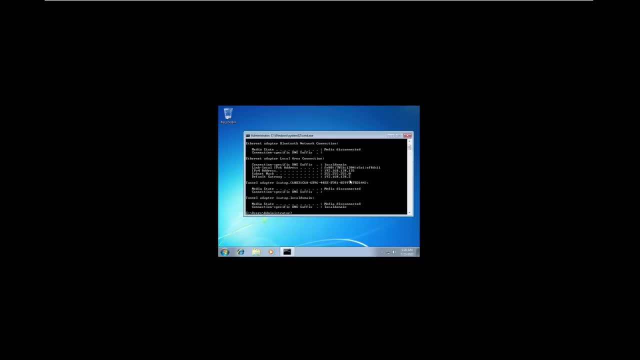 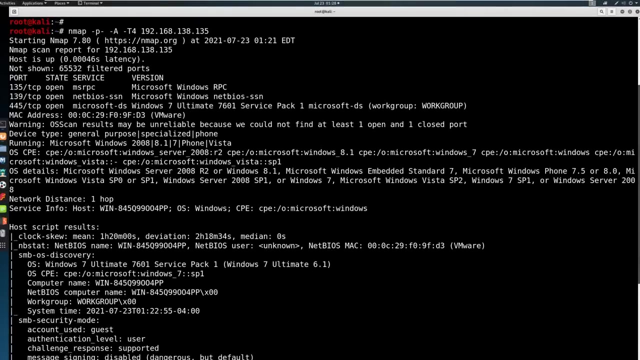 go and how you can exploit it and meet me in the next video And, once you've attempted it, to see if you were able to successfully route or system this machine. Thank you, So let's start by taking a look at our nmap scan Now. the IP address I got was 192.168.138.135. 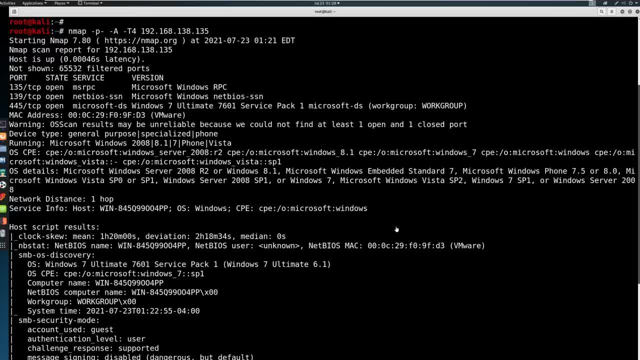 And not a lot of ports came back. So we got 445 back And we can scroll through, get a little bit of information Like we see a net BIOS name on this machine. We see that it's running Windows seven ultimate 7601 service pack. one doesn't appear to be part of a domain, just a work group. Same thing, work. 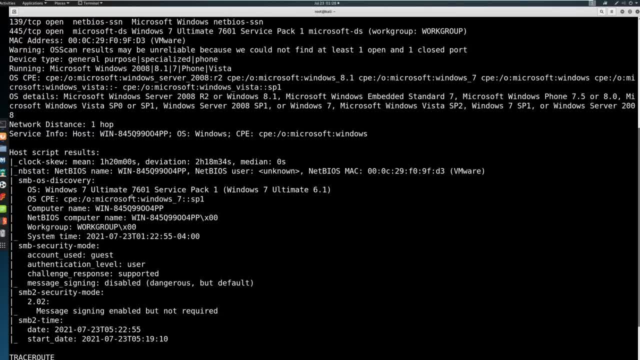 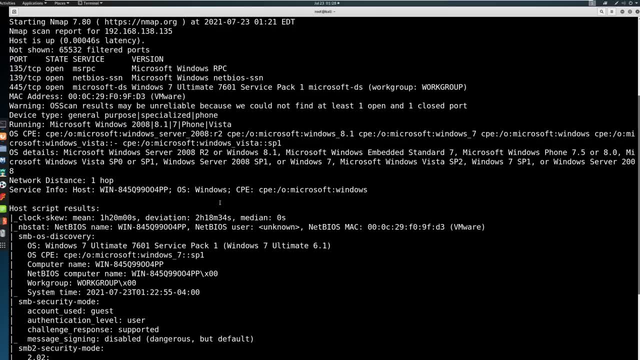 group authentication level user And really there's nothing here that is a big indication as to what this could be. So when we have this, as we discussed before, when we're looking at SMB specific vulnerabilities- because that would be my guess here would be the vulnerability would be SMB related- we need to 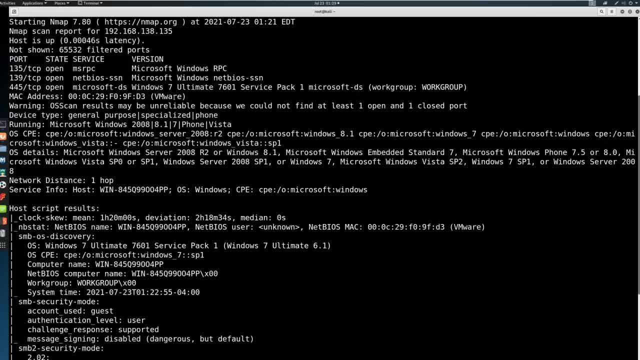 enumerate SMB in one of two ways, really. The first of that being well, can we search based on version information that we see here? Can we search on this and see if there's anything vulnerable that could be there? Second of all, if we can't find anything right off the bat, for this, maybe 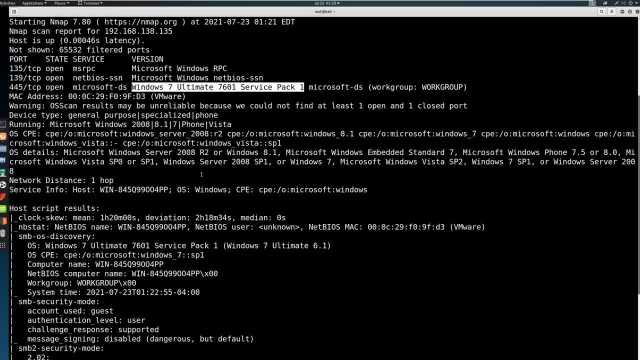 then we can go and use something like SMB client, do some research and see if there's anything that's vulnerable that could be there. Then we can do some enumeration. maybe there's a null session we can connect to, maybe there's a. 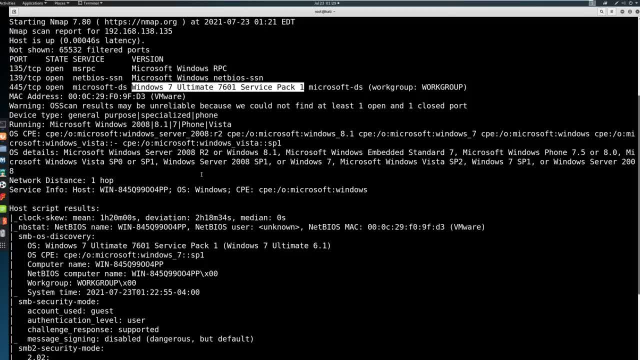 file or something, some sort of information with a username or password or something along those lines that gets us into this machine. Otherwise, we're pretty much stuck with version information. Okay, so we're going to go ahead and just copy this, And there's a reason that this is the first. 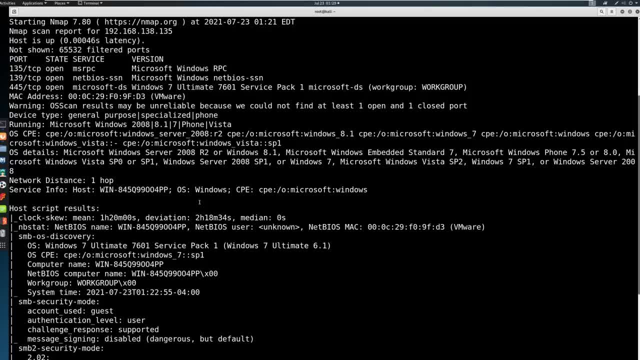 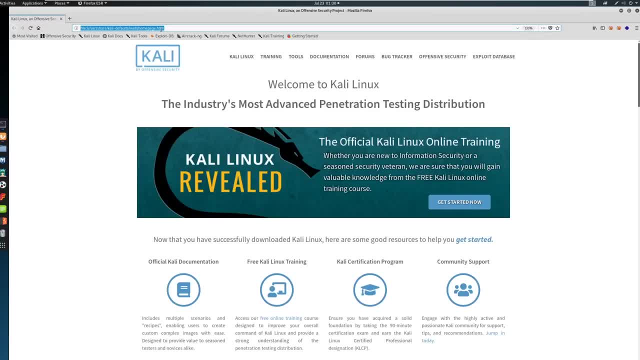 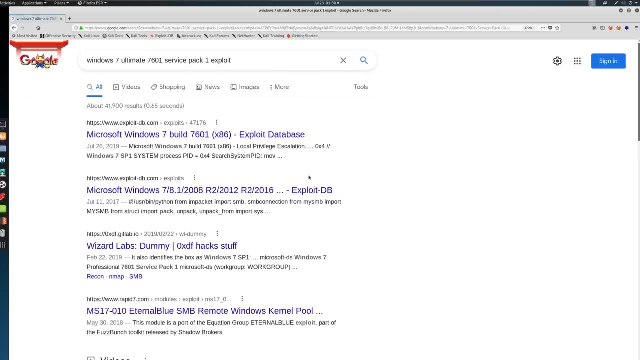 machine in our run through the capstone because this is the easiest, or should be the easiest. So we're gonna go ahead and go out to Firefox and I'm just gonna go googlecom come in here, we're gonna search for this and I'm gonna search for exploit. it already knows me and we can. 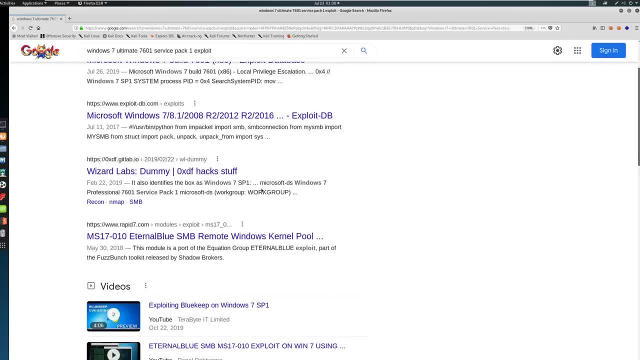 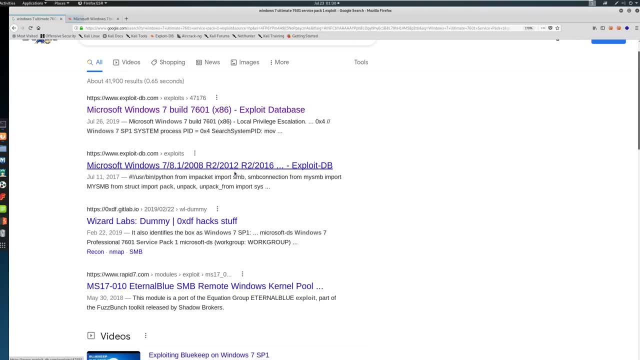 look through some of these and see if there's anything here that really stands out. first thing for me: we've got got a few. we got one here, one here. these just kind of say they don't necessarily say what they are, so we might need to click. 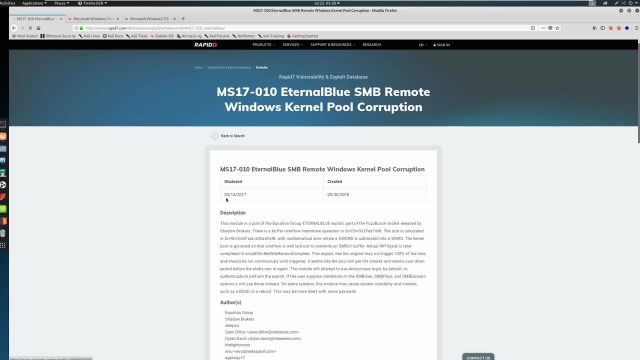 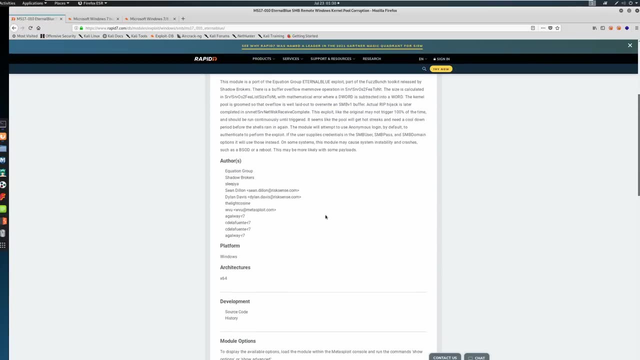 into them. ms-17 0 1 0 keeps popping up quite a bit. let's see if it tells us anything here about architecture. really doesn't just shows up as this, so we'll have to do some reading into this. this is a local privilege escalation doesn't. 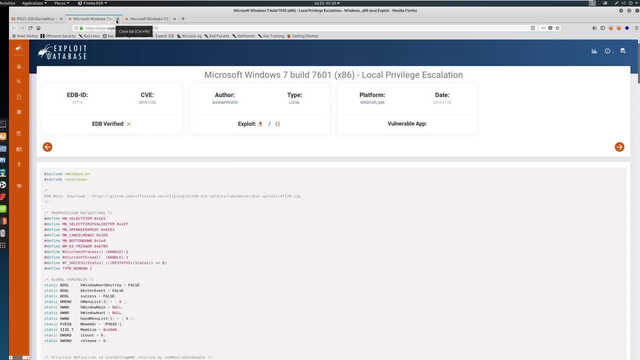 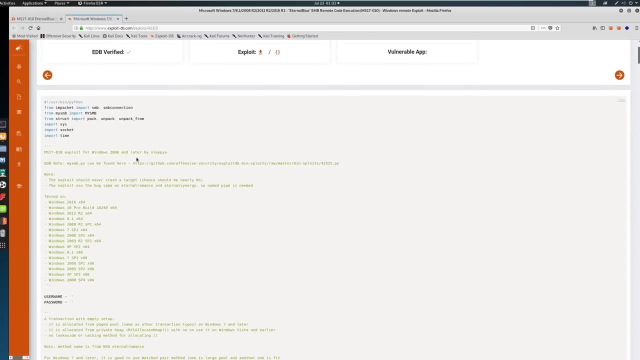 really help us, because we're not doing privilege escalation at this point. we're just looking to see if we can even get on this machine. okay, this shows us. hey, ms-17, 0, 1, 0. this is you a exploit, for it, written in Python, it looks like and it says: hey, okay, this. 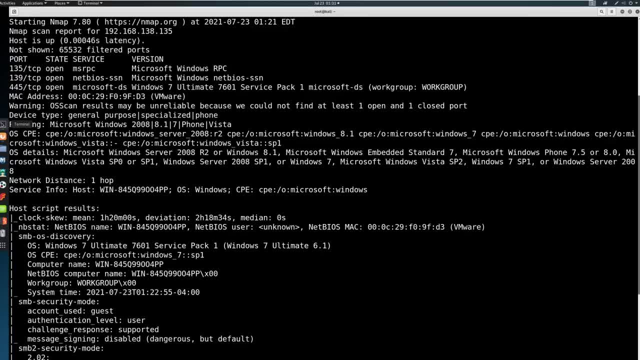 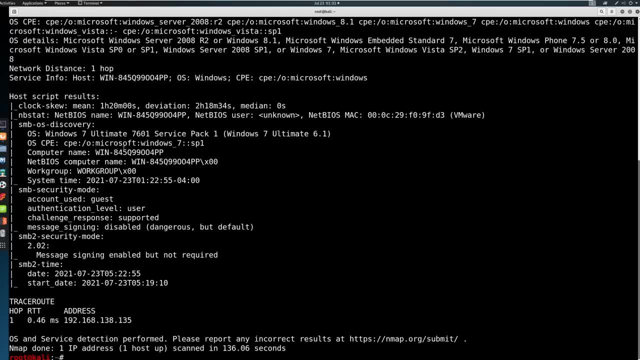 could be our, our target. so we're gonna take two different paths here. we're gonna look at it first in Metasploit and then we're gonna take it from a manual path and we're gonna see if this is indeed what we're after. so let's go. 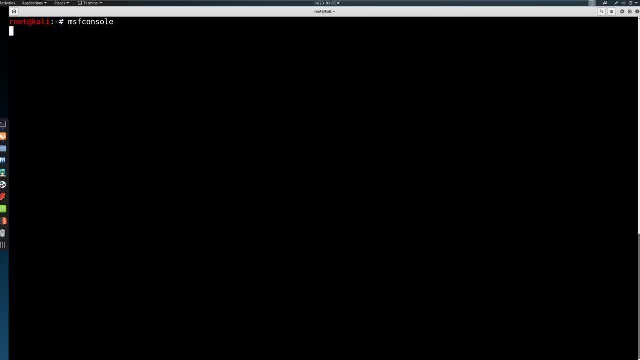 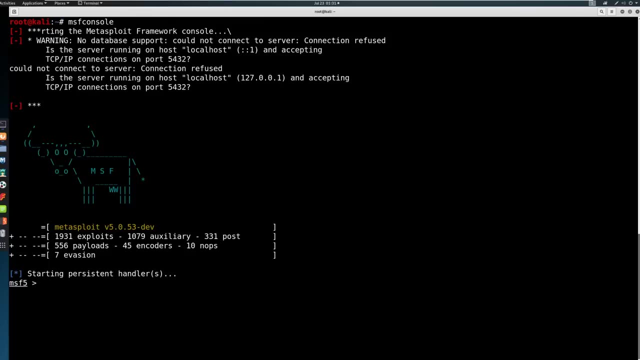 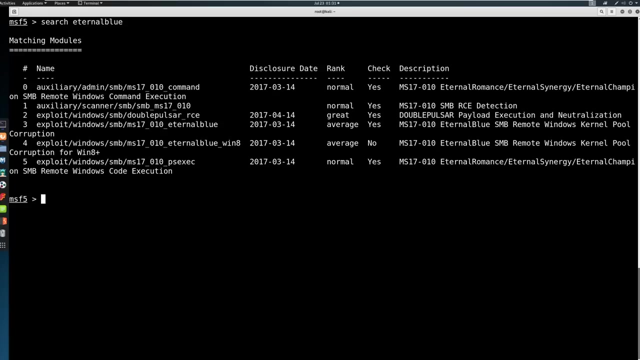 ahead and just go to MSF console and yours might look a little bit different than mine depending on what version of Cali you're on, but the process should be the same. I'm on msf5, so we're gonna go ahead and just search eternal blue, and I do know recently they 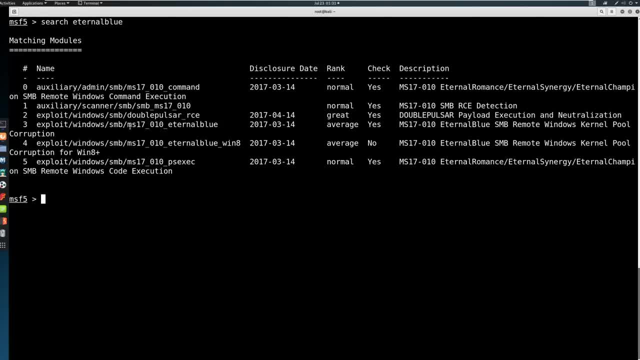 combined all the eternal blues into one. so, again, yours might be a little bit different than mine, but it should be the same processor concept. now the first thing we want to do is we want to look up this SMB scanner. right, want to do an auxiliary. our auxiliary modules are gonna tell us what is there. it's gonna. 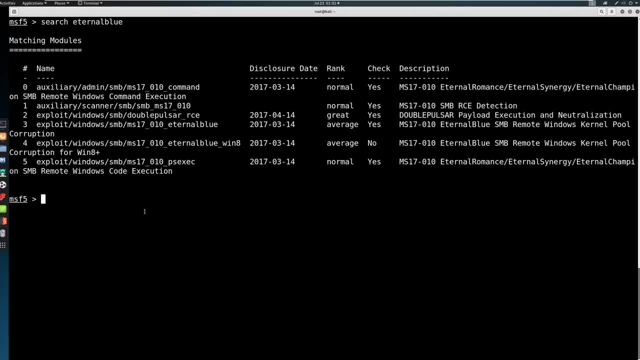 be a check. it's not gonna be so much an attack, it's more of scanning than anything else. then there are some attacks and auxiliary modules, but they're not full on exploitation. So let's go ahead and just say: use one And we're gonna go options in here And all it's going to do for us. 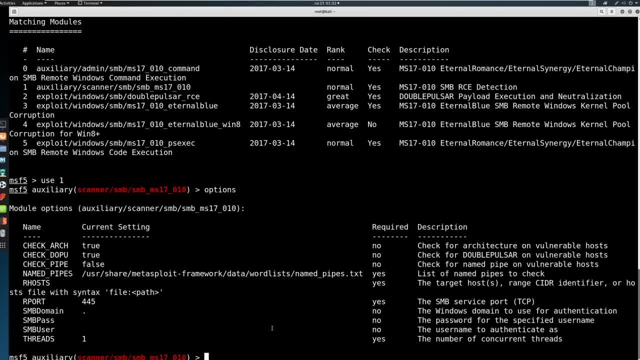 is. it's going to come in here, we're going to provide it with an R host, we're going to run it and it's going to provide a check. Okay, so we can just say: set our host to 192, 168, 138, 135,. 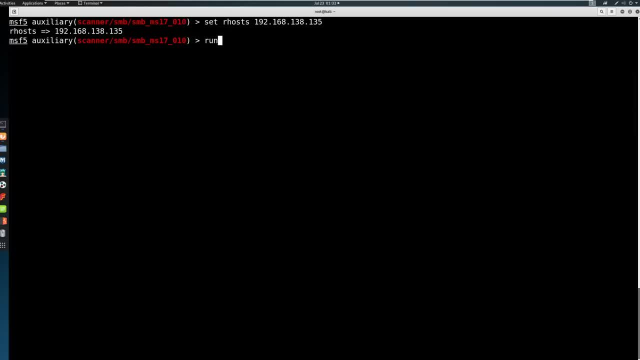 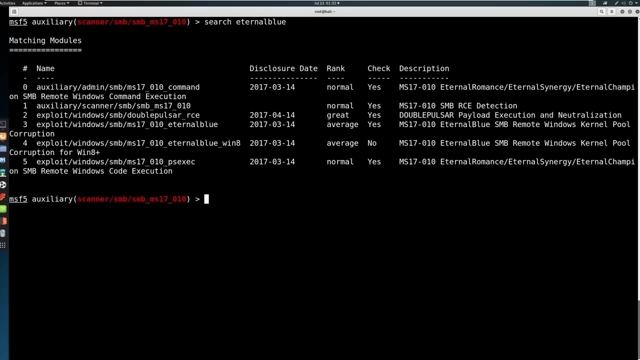 whatever your IP address is. And then I'm going to say run And it says: host is likely vulnerable to Ms 17 010.. Okay, there's a second way to do this. So let's go ahead and just search eternal blue again. You can also search Ms 17 dash 010.. Or however you want to do this, it should all show. 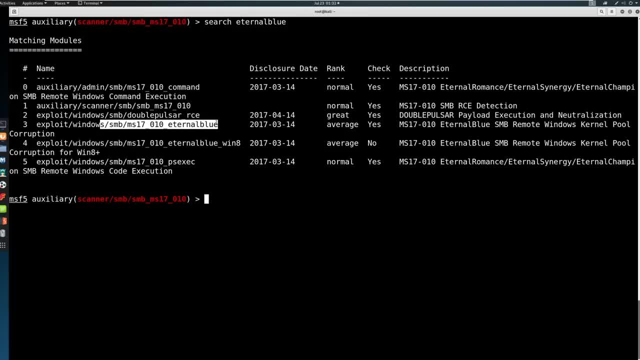 up. I'm going to use this number three here, the eternal blue one, We don't know. we do know that we're on Windows seven, so the Windows eight won't work for us And PS exec we could run, but I'm going to go ahead and just use the one that is. 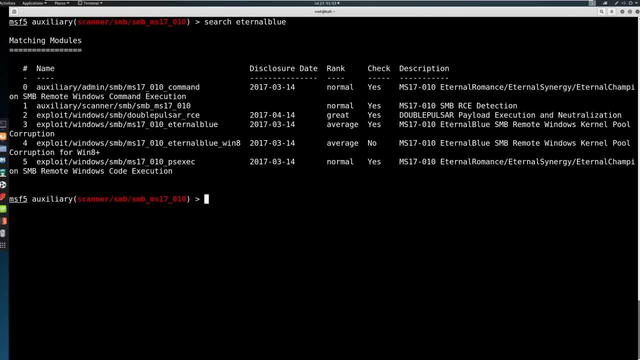 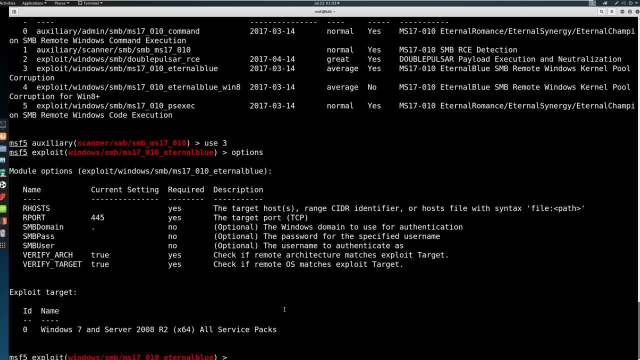 most popular and works usually out of the box. So I'm gonna go ahead and just say use three and type in options, And in here we have a verify option, which means we should have a check option here. So I'm gonna again just say: set our host, I'm gonna show you the check feature. 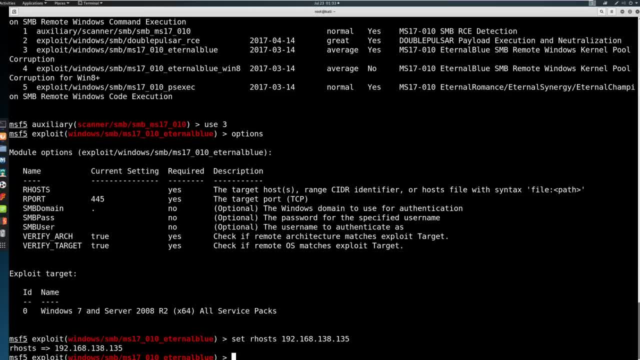 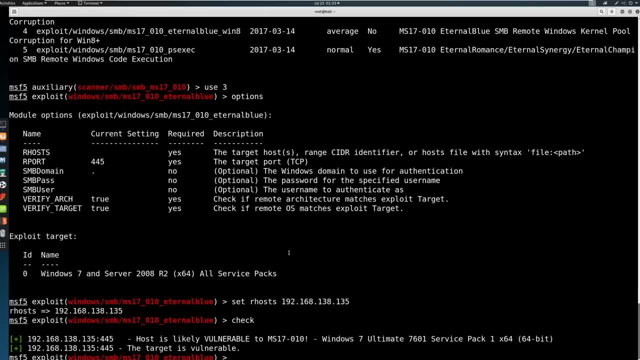 So this is basically what the auxiliary module did for us. it says, Hey, it's, it's vulnerable. okay, are likely vulnerable. So what we need to do is we need to set a payload here. Now, something that you might not know yet at this point is that payloads are by default, they are set to 32 bit. 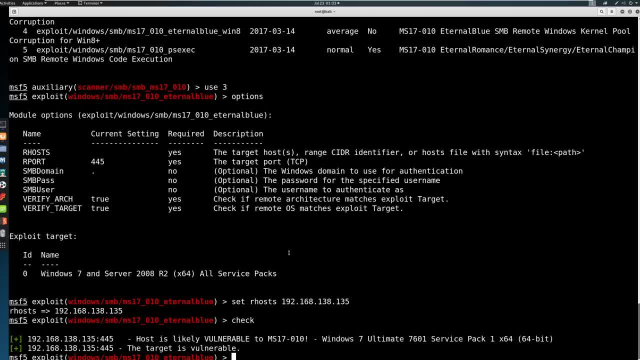 at least in this, this example, because there could be a 32 bit exploit in here. Actually this says 64 bits. I could be lying to some. some payloads are set to a 32 bit to start, because we know that this is a 64 bit machine, or at least should be, given that it's enterprise. 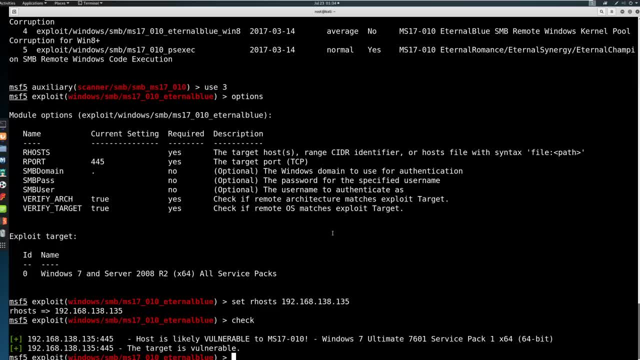 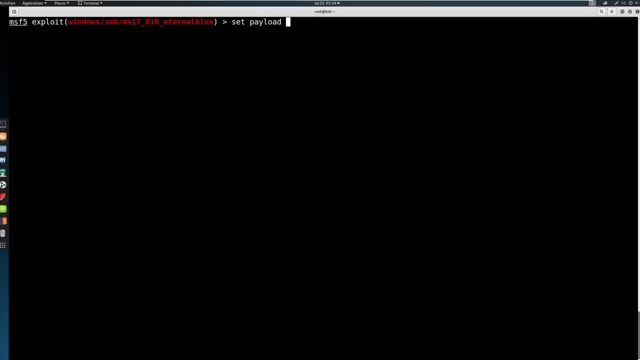 we're going to go ahead and set this to 64 bits, just to be safe. so this is a practice that i take on. if i know the architecture of the machine, i'm going to go in here and set my payload for myself. now this should be 64 bit, but just to be safe, we're going to type in windows and hit tab. 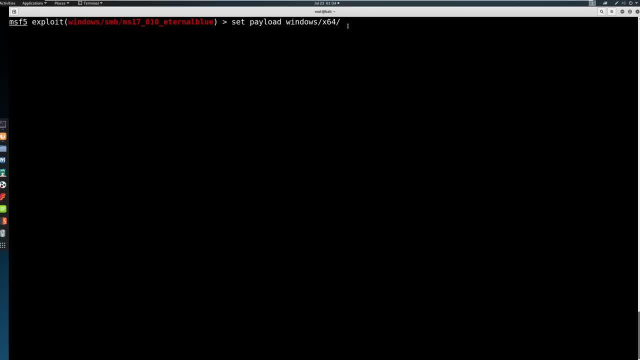 because it only auto completes to 64 bit. this is perfect now, i think. where my mind was going is that i want this to be a meterpreter shell, and i don't know if it defaults to meterpreter. um, it might default to a reverse tcp of some sort, so we're going to go ahead and use a. 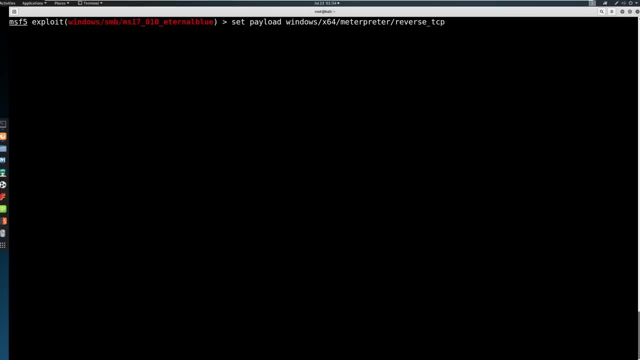 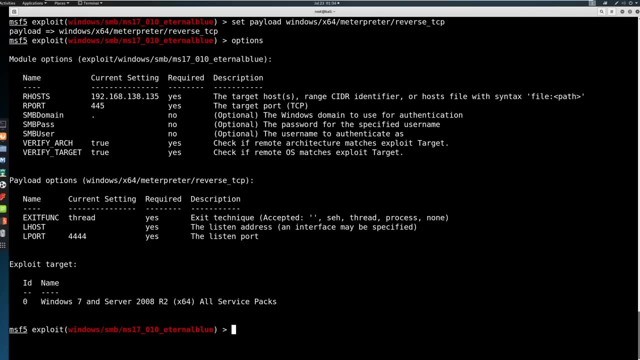 meterpreter shell because we want a nice interface um to to have. so i'm going to go ahead and set that options one time and i'm going to look at the l host here and we could just say: set l host over to. we could just call it eat zero or you could set your ip address in here again you. 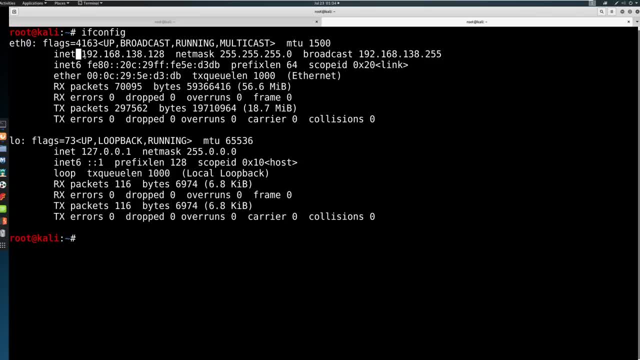 could set your ip address in here, and you could set your ip address in here and you could set your ip address in here and you can ipa or if config, and whatever your ip address is, i'm running on eat zero. so whatever your um, whatever you choose, you could place here as well. so i'm going to go. 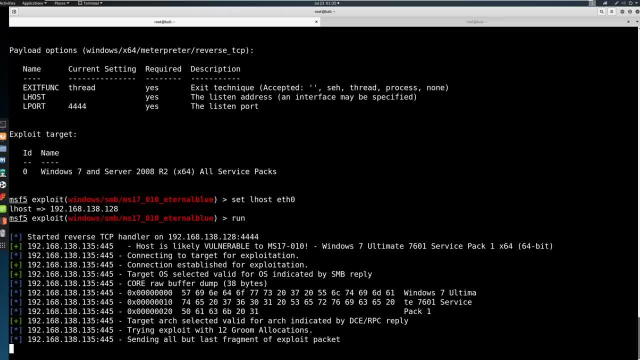 ahead and run this now while this runs. this might not work on the first go. it might not work on the first few goes. this is going to try, uh, going through what are called different sets of grooms on here and it looks like it worked right away. but sometimes this doesn't work right away and 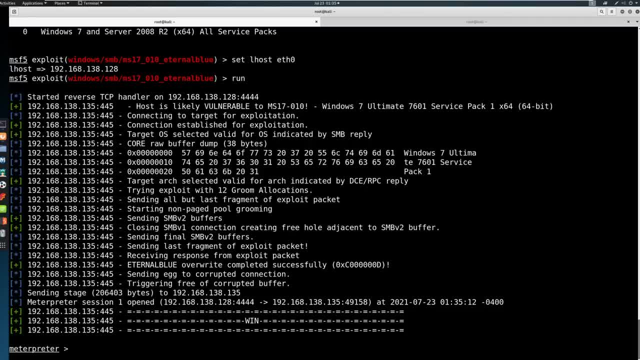 if yours doesn't work right away, that's okay. it might take a few attempts through this first process and you might have to hit run a few times for this to go. now i have chosen using blue or eternal blue for this course because it's so relevant. this is a 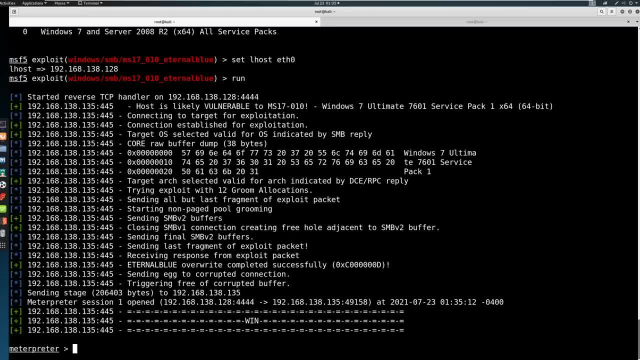 four-year-old exploit now and i see it on so many internal penetration tests. it's not even funny like i wish it would just go away, but it is this easy to run and just get on a machine and gain access and it's incredibly easy and incredibly prominent in environments. think about environments where they have systems. 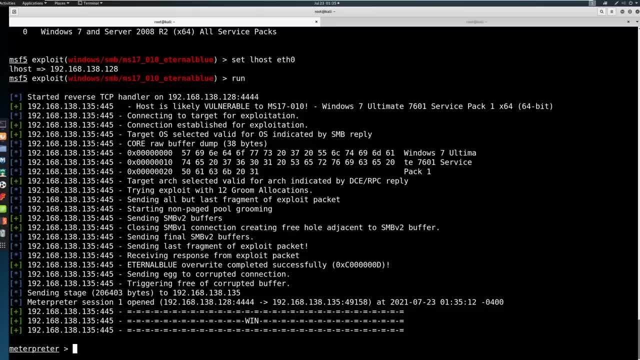 running that they can't update or do anything with, and you have this. or they just have poor patch management and you have this. it's so easy to get on a machine and then you come in here and you say hash dump, and you dump out the hash and now we've got administrator hash. we can go try. 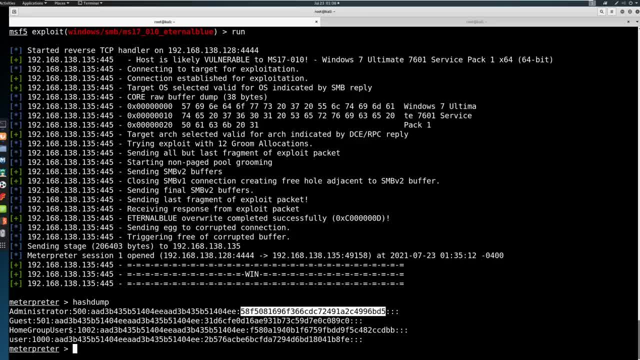 to crack. that we can do. pass the hash which we're not there yet. we're going to get there in the active directory section. you're going to see what the differences are on this kind of stuff. but you can utilize these hashes to our advantage and we're going to play around with that a little. 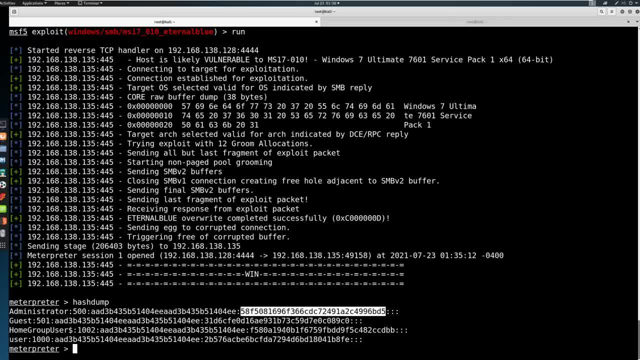 bit later in the course. so, with that being said, this is something that you will likely see if you do become a pen tester. you'll see this in an environment and it is really this easy to get into a machine like this. so we have used this now to come through here and gain access. we're going 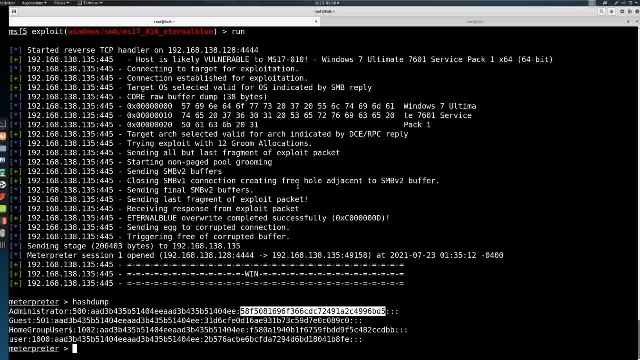 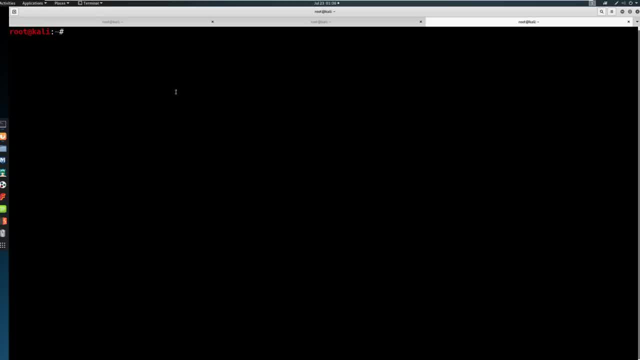 to go ahead and go back and we're going to try doing it again, but we're going to do it through um, through a manual method. so i'm going to open up a new tab, all right, and we're going to come in here and i'm going to search google now if we want to go. 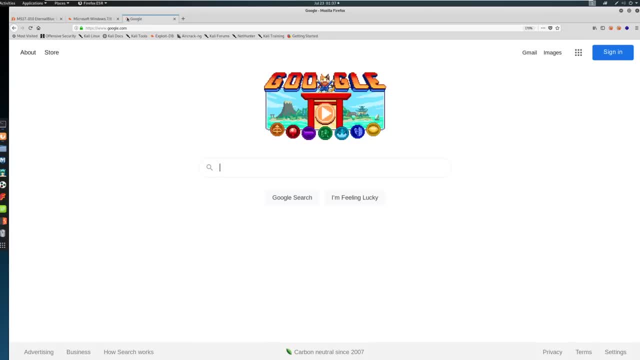 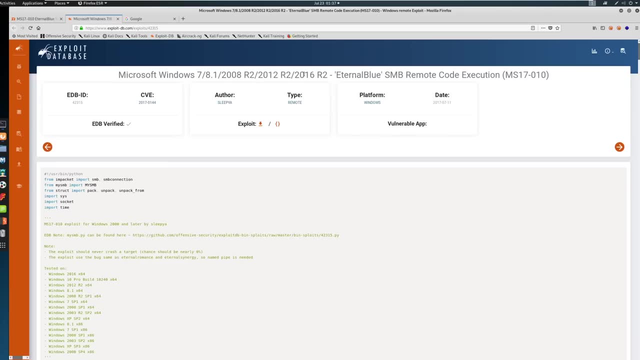 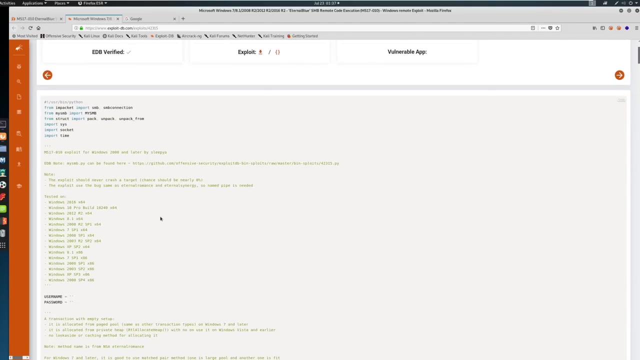 look for manual methods of exploiting a system. we're likely going to use github, perhaps exploit database. now, this exploit database- one i'm not going to use, only because it gets a little tricky with eternal blue. there's a few things that we have to do. i don't believe this one is just one. 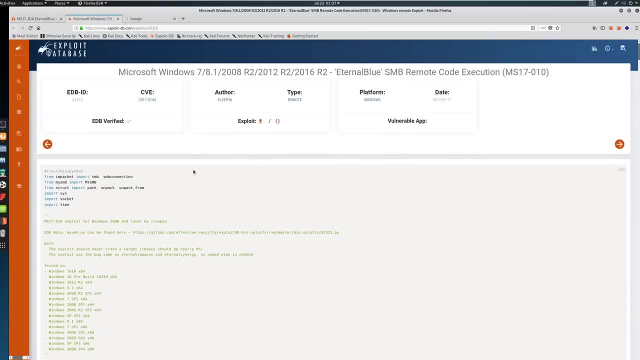 thing that we have to do. i don't believe this one is just one thing that we have to do. i don't believe this one that runs right out of the box. it has a little bit more information here than what's leading on now. we might need to reboot this machine. by the way, we'll- we'll give it a. 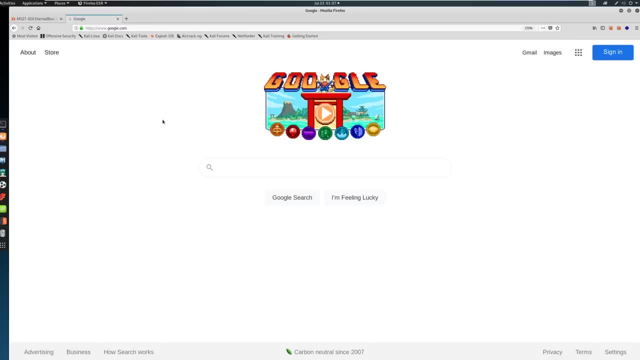 go and see if it works. it might not work out of the box because we've already exploited the system, but we'll try anyway. so what we might want to do is something like eternal blue and we might want to say: github, okay, and we can come through here and look through different ones. 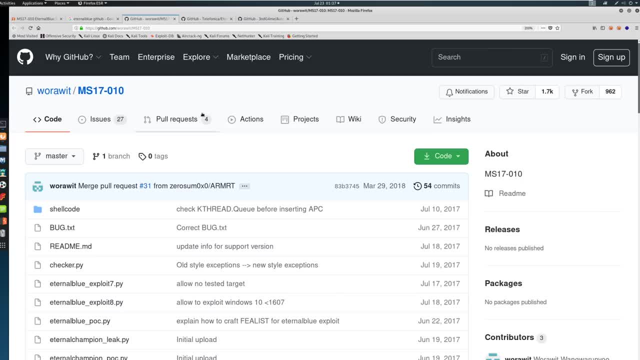 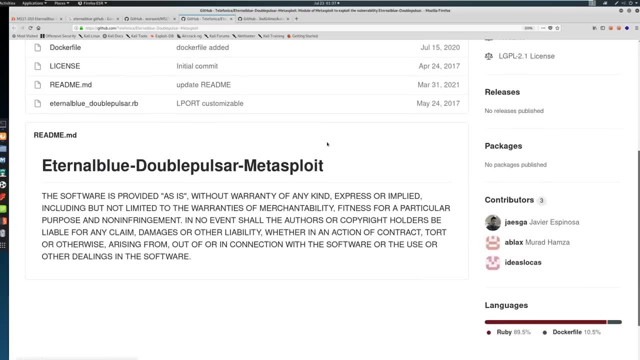 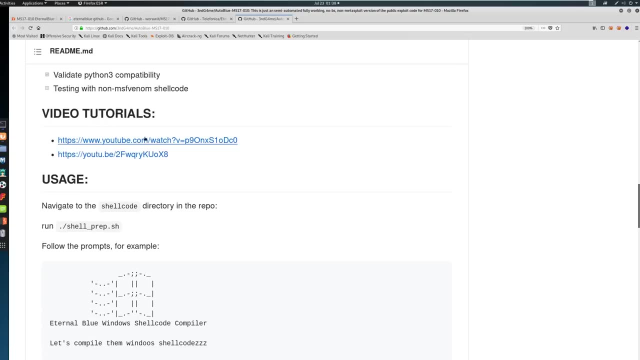 i like to open a few and i like to look at them and read the the amount of stars that they have. read the descriptions that they have detailed walkthroughs. you know all these have decent stars. this one doesn't have a great walkthrough. this one has a very good kind of detailed walkthrough, has video tutorials. 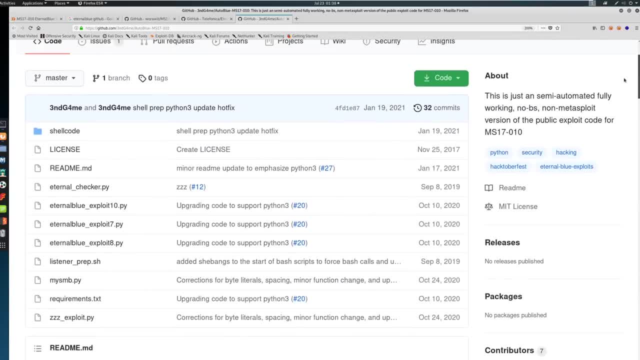 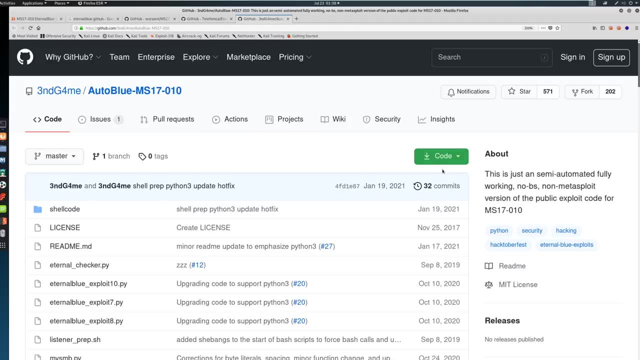 has a decent amount of stars and i i honestly like it. so we're gonna go ahead and just get the auto blue one from endgame. so go ahead and find that and get to this. we're gonna go ahead and copy this code. we're gonna go ahead and copy this code. we're gonna go ahead and copy this code. 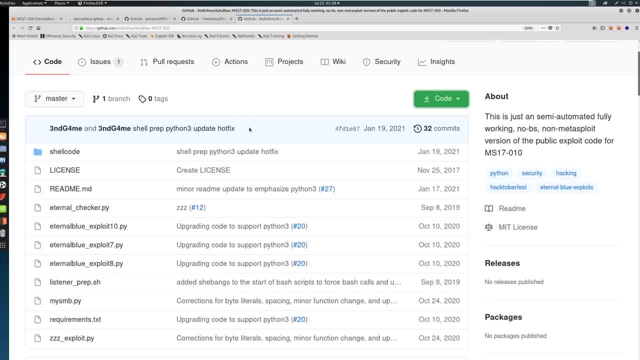 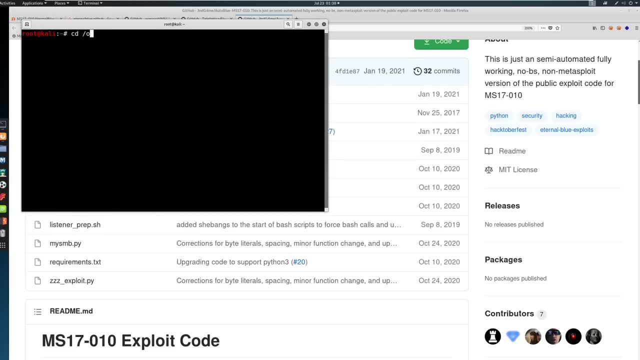 and there have been commits since 2021, so that's great. there's recent commits to this, which is awesome, so i'm going to go ahead and go into um, i'm going to cd in the opt and i'm going to get clone. this and that's not what i should have been copying. uh, should have copied. 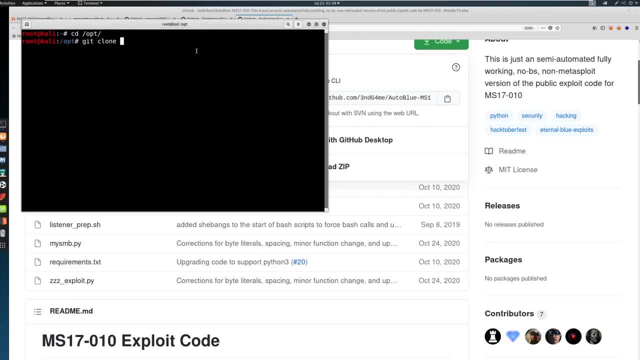 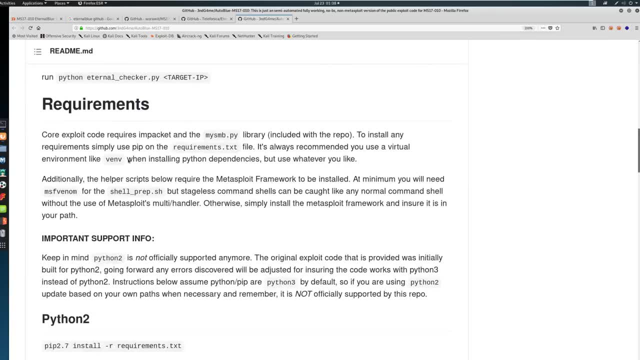 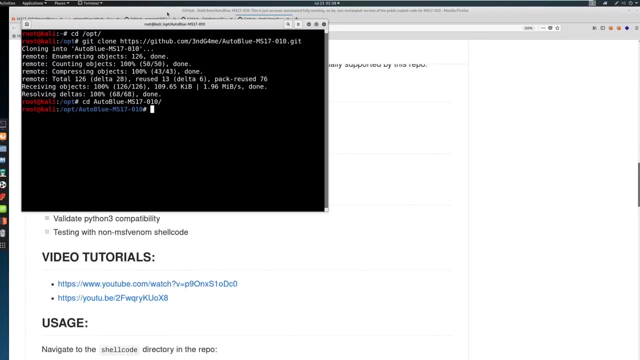 this, but we'll try it one more time and paste here. all right, and i'm going to cd into auto blue and it gave instructions in here somewhere about how to uh, how to install this. let's go to installation. pip install requirements for python 3, which we 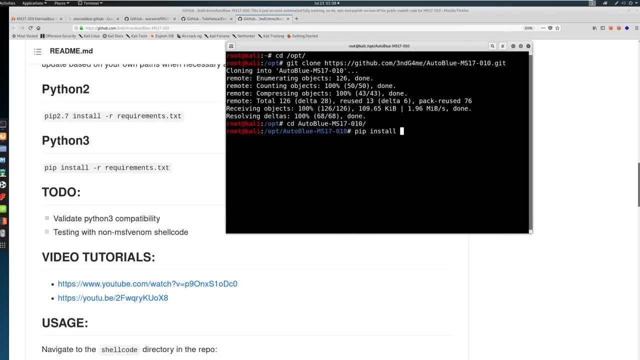 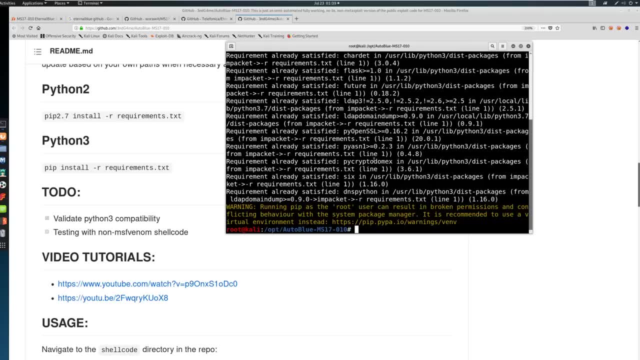 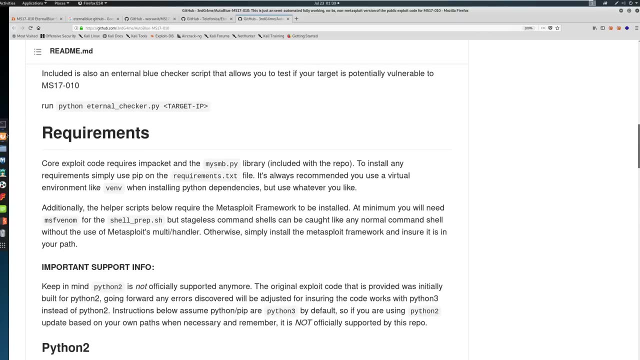 should be on at this point. so we're going to do pip install, dash r requirements, just like that. let that install. looks like everything is satisfied or installed, so that's good. um, from here we're going to go ahead and do the usage. now there was a checker in here, so we can. 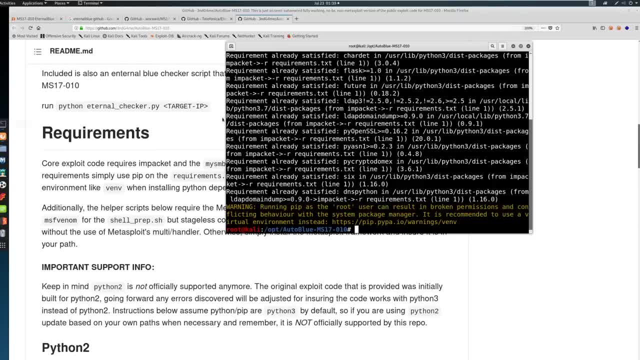 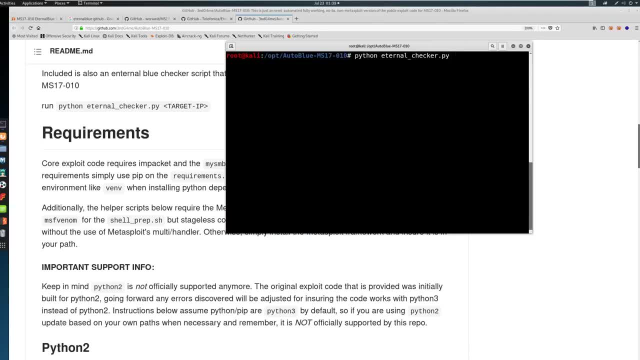 run python with the checker, so i don't know. it says python 2, so let's go ahead and run python 2 with it. it could be python 3 too, so we might run into an issue. checkerpi 192, 168, 138, 135. 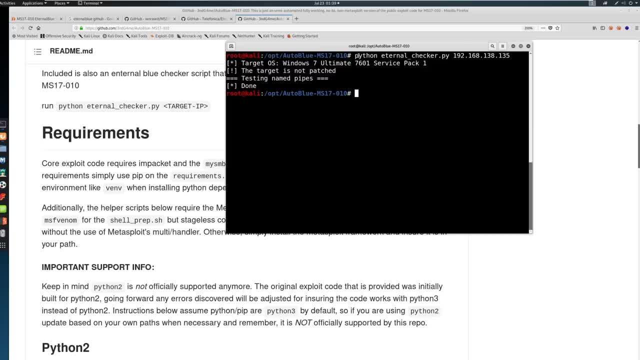 target is not patch testing name pipes. okay, so this is something that i actually use on an assessment, regardless if it's this or the, the metasploit version. i will take a screenshot of this. uh, there are reasons sometimes where we won't run the exploit if the environment has critical. 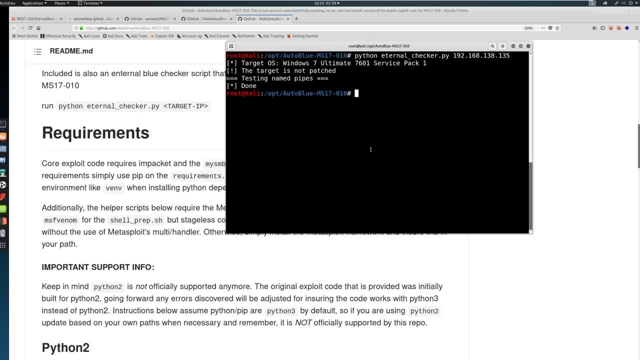 um, critical machines running, for example, like in a hospital. i might not run this exploit because this can take down a machine, and if i don't know what machine i'm taking down, who knows in a hospital? right, you don't want to make that mistake, so it's always better to play it on the safe side. 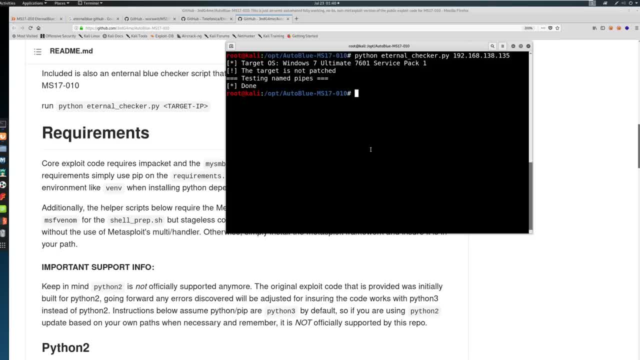 when we're running these exploits, if you're, if you don't know, you can always ask. your client say: hey, i've got this machine, here's the ip address. i want to run this exploit, is that okay? and get permission first. now there's a lot of ways which you'll see in some of my other videos, but i'll just go ahead and 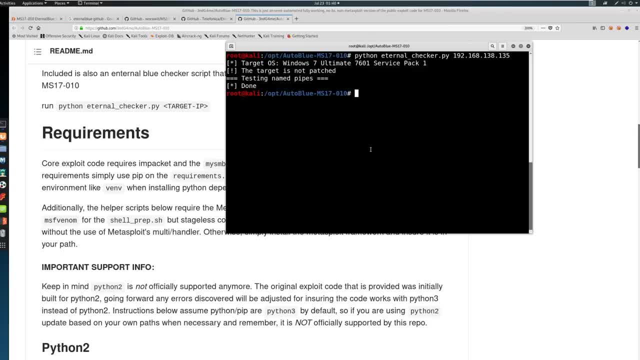 when we get into the active directory, exploitation part of the course that we can compromise the domain and we can run all kinds of exploitation, own the whole domain controller and not worry about tipping over the server by any means. this can tip over a server, So you want to be safe with. 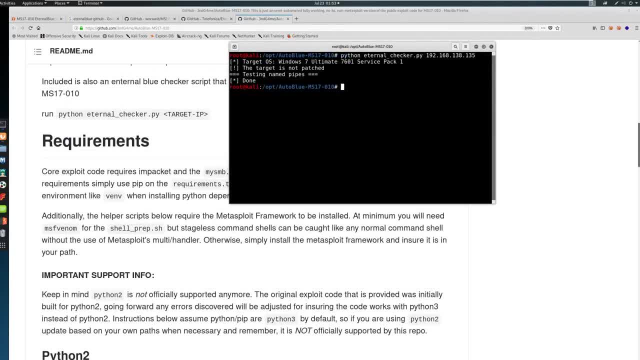 these kinds of things. So, with that said, I'm going to show you how to run this manually, but it's going to. it's going to tip your box over. I'm going to give the secret away. it's going to tip your box over And this is going to be the lesson learned from running this exploit. I'm 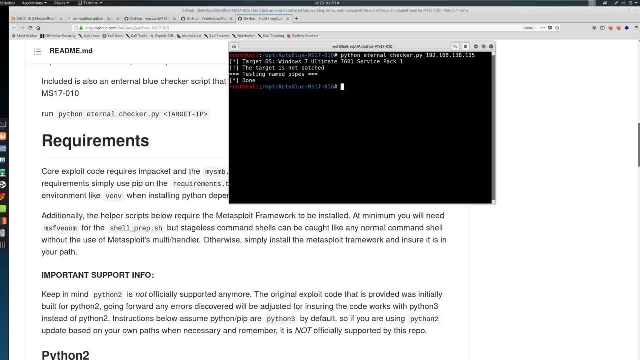 going to show you the proper way to do it manually With the version we have. it's not super easy to get a shell from the manual method. we could go around and play around and find one that works. But I'm going to show you this from a. here's how you would run it manually, But also here's the. 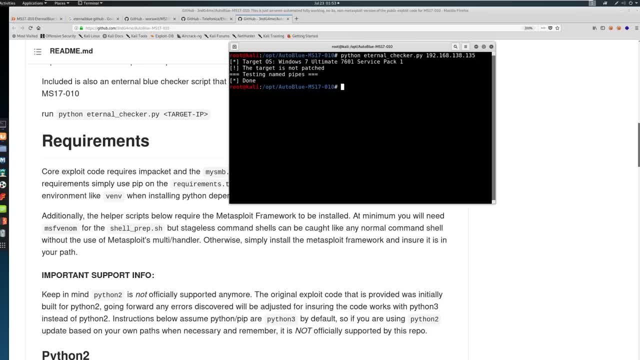 dangers of running this in an environment, And this is a perfect box to show you why we don't just don't go run remote code execution on machines in an environment, because this can take down a machine. So let's go ahead and run through the process. I'm going to show you. 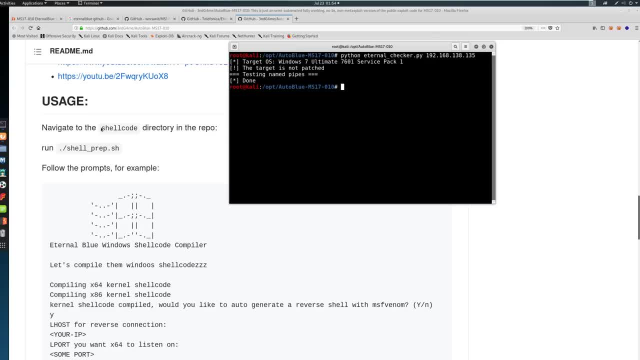 the process And then we're going to knock this machine over. So first thing we're going to do is we're going to cd to the shell code directory And we're going to run shell prep And I'll say this now and watch. the exploit will work fine. So, oops, we're going to go ahead and just hit Yes. 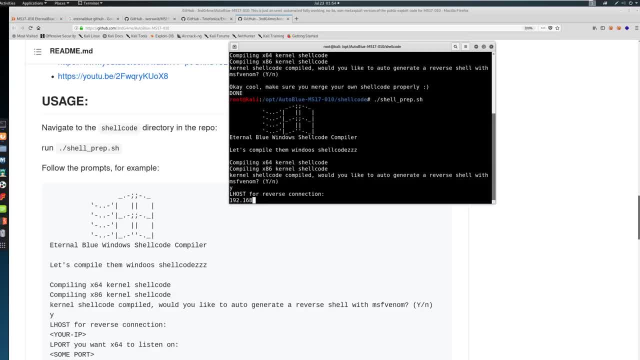 here And then we're going to enter in our reverse connection. 12168138128 is mine. I'm going to say 9999 for this. we can do 2222 for x86, we're not going to use it. Now we have the opportunity to. 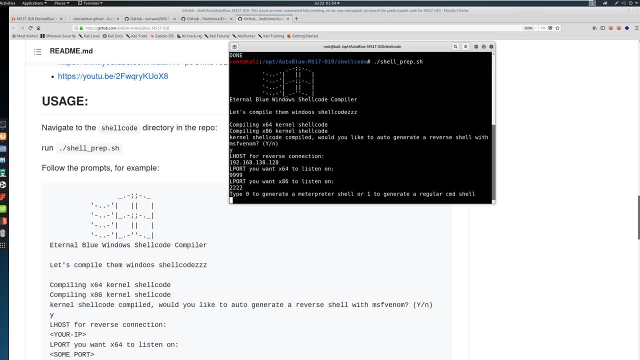 use a meterpreter shell or generate a regular command shell. If we do the meterpreter shell, we can go into meterpreter And we can actually run it in the sense that we use a multi handler and pull down. it's basically a listener. it is a listener and it's going to pull down a 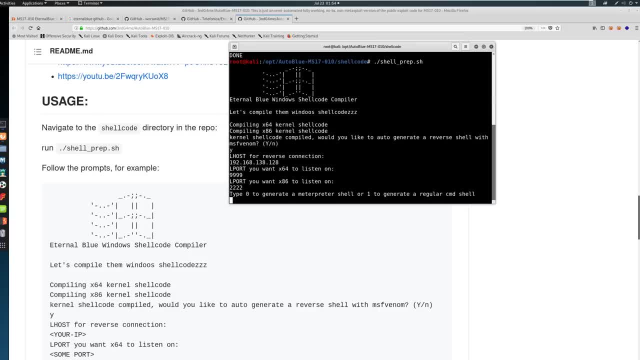 meterpreter shell for it. So it's just a shell code that we're generating. we already use the meterpreter shell to get the first shell on this. So now we're going to go back and we're going to go ahead and try to do this with a regular command shell, So you can press zero if you want to try. 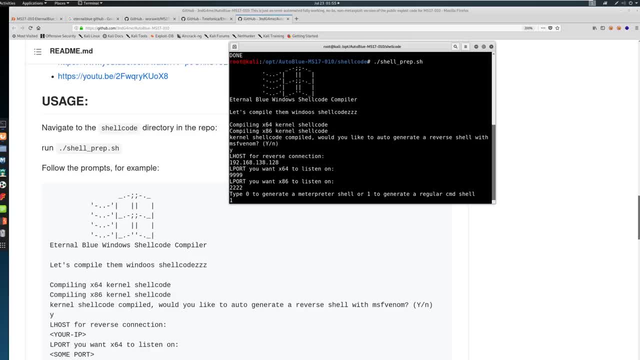 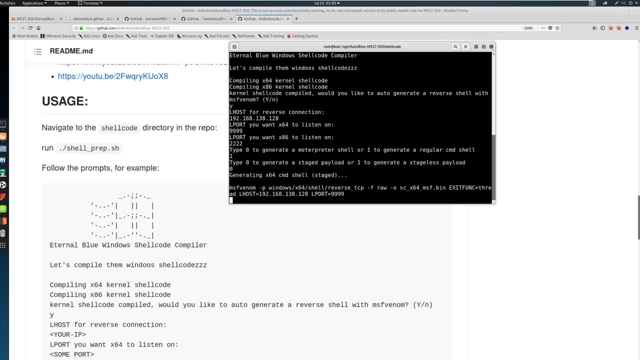 the meterpreter shell method. you can also press one to generate the regular command shell method. we're gonna go ahead and just do the regular command shell. we're going to generate a stage, payload, stage or stages. here should crash the crash this machine. The other thing we're going. 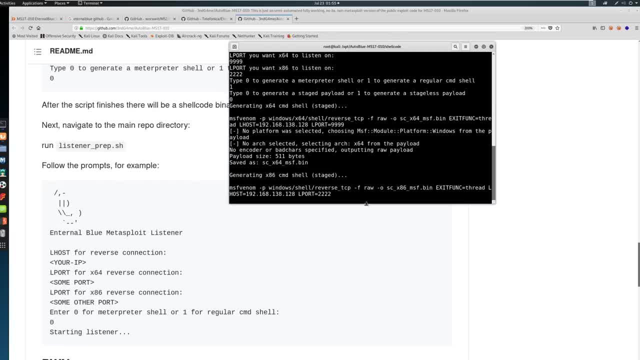 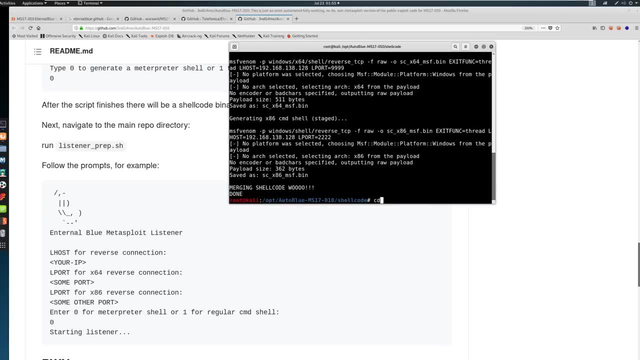 to do is we're going to run this listener prep once this is all done. So it's doing this for us. we're gonna go ahead and CD back in a second once this is done. Alright, now I'm going to CD back. 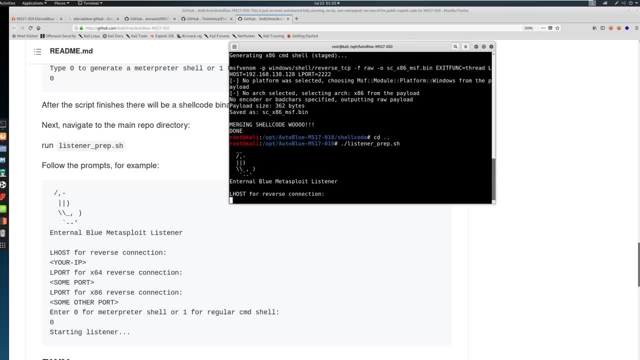 and we're going to do listener prep And this is going to run a listener in Metasplay for us, which is nice. we could just as easily run this with Netcat. we can just say NC and VLP, like we. 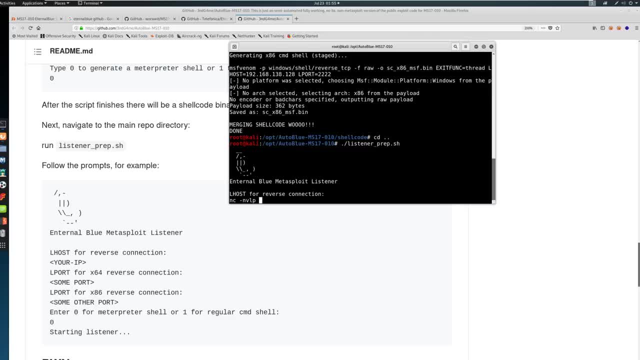 have before and see dash in vLP like this and whatever port we're listening on all nines before. So we're gonna go ahead and just let this run its course as in ended And we're going to do 9999.. We did 2222 here And we're going to go ahead and say regular. 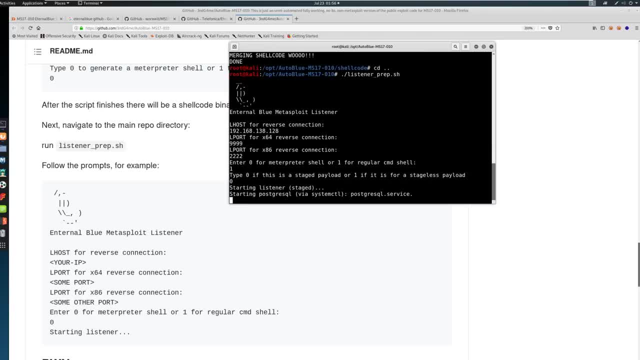 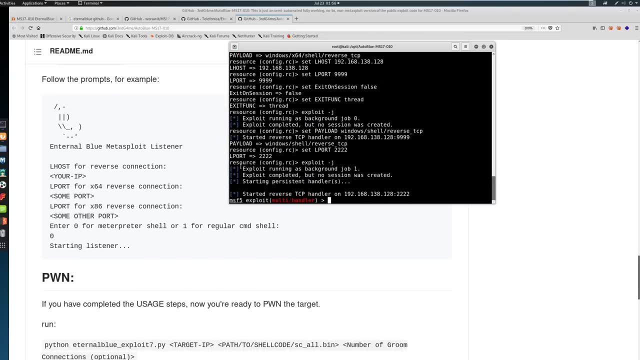 command shell, all the same things we did before: stage payload, And it's going to start this up for us, hopefully start up some listeners, and you should see a lot of work. just go in. Okay, it's got all those listening is waiting for any sort of connection to come through. So the next. 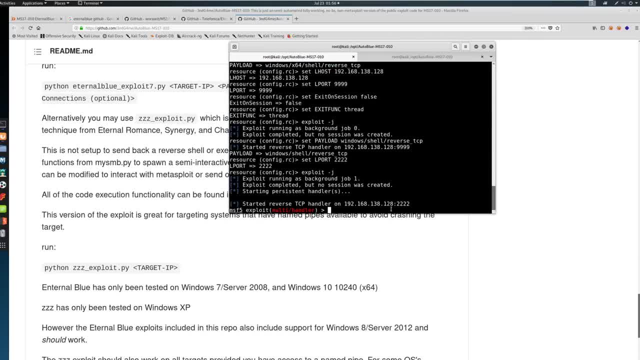 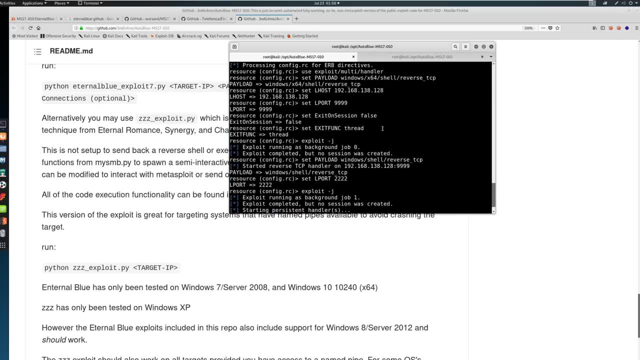 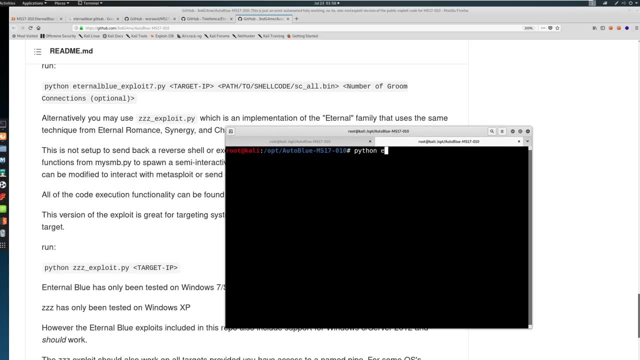 thing we're going to do is- and it is using the multi handler for us already- It's just using a shell: reverse TCP instead of a meterpreter- reverse TCP here. So last thing we're going to do is run the exploit. So we're just going to say: Python, eternal blue, like this exploit, and we're on seven. 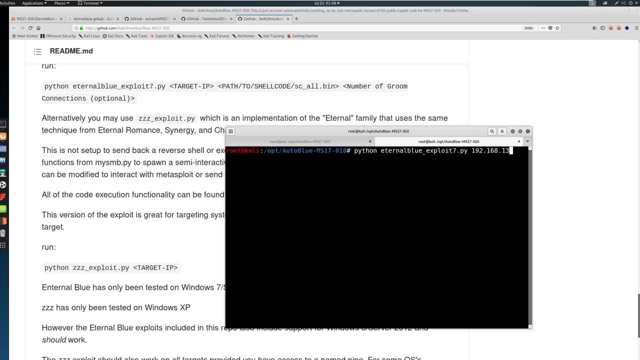 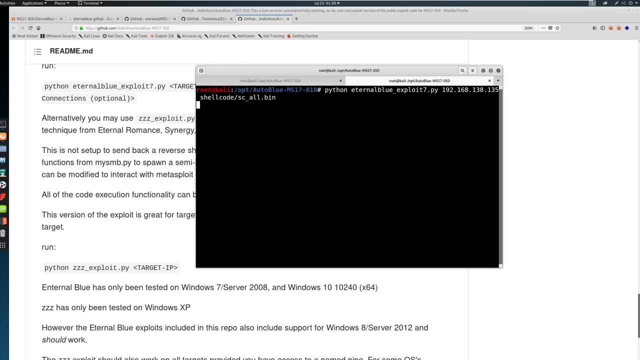 dot pi. Our target is 192.168.138.135.. Path to shellcode is just shellcode and then sc all dot bin And we do not have to provide a number of room connections. that's optional. We're going to run this and we'll cross our fingers. you never know, might work. 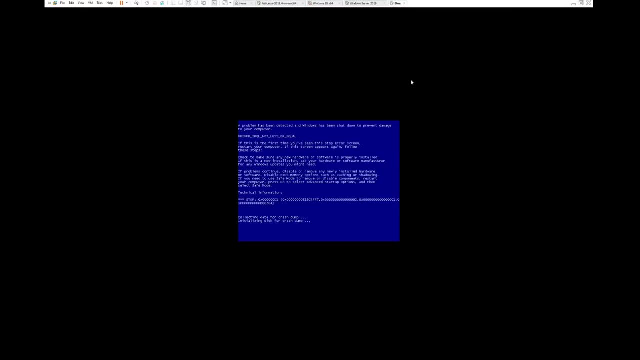 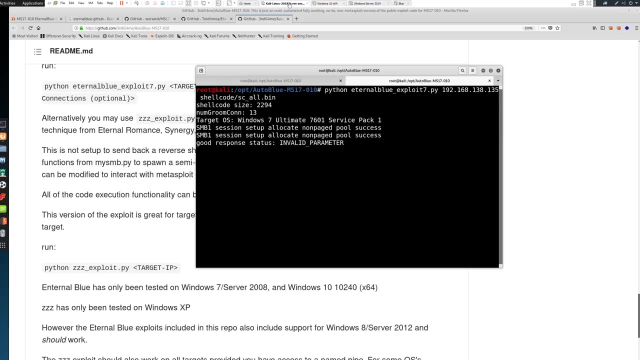 doesn't look it's working. We blue screen the machine. So this, this is a perfect example of why you just don't willy nilly run this in an environment. Okay, So a good lesson learned, honestly, because if you're in a critical environment, you have no. 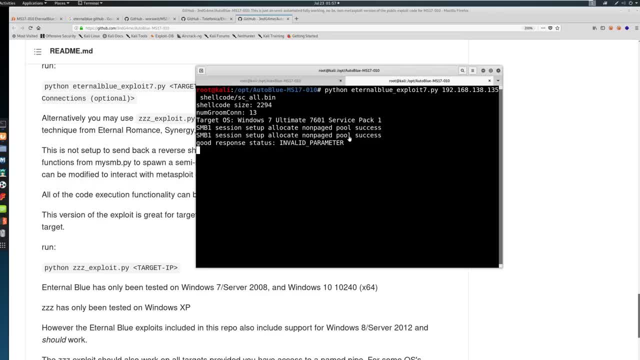 idea what that machine does. Imagine that this was something in a hospital controlling equipment that was being used during surgery. Who knows, if you took that down could be very, very, very bad. So it's good to see the other side of it Again. get permission before running something like this. 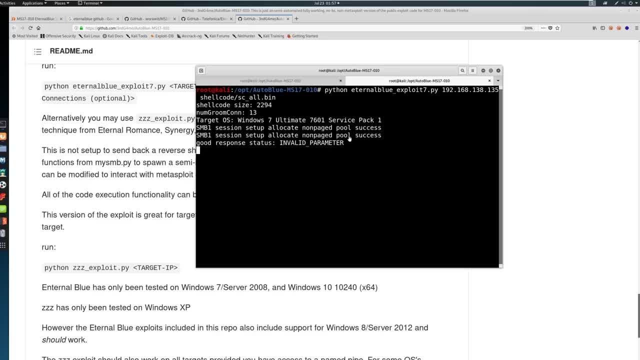 unless you know that your environment safe, it's okay to take down some machines etc. But usually that's not the case. So with that we're going to go ahead and move on to the next machine. Hopefully you got this in through the walkthrough just fine, So I'll see in the next machine as we walk through that and 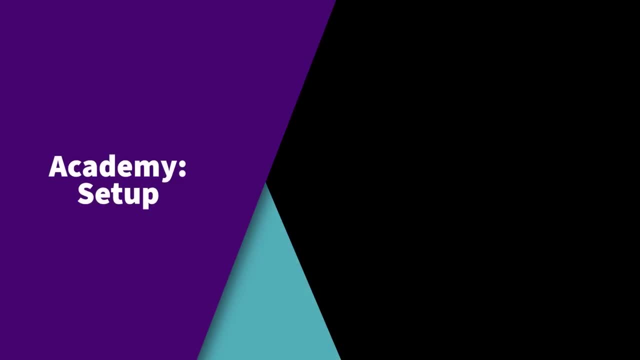 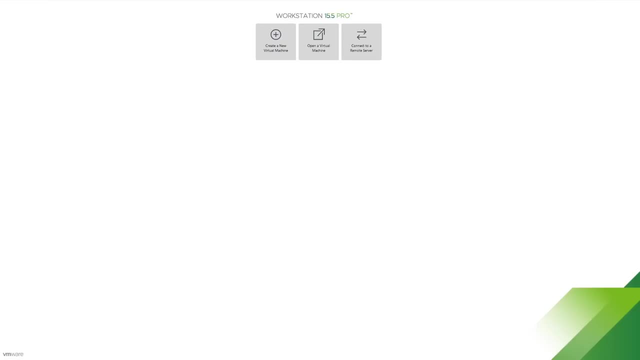 hopefully take down another box. Okay, in this video, I'm going to show you how to quickly open up the academy machine in both VMware and VirtualBox, and how to set it up. After this, you should have seen a Linux setup and a Windows setup, So you should have. 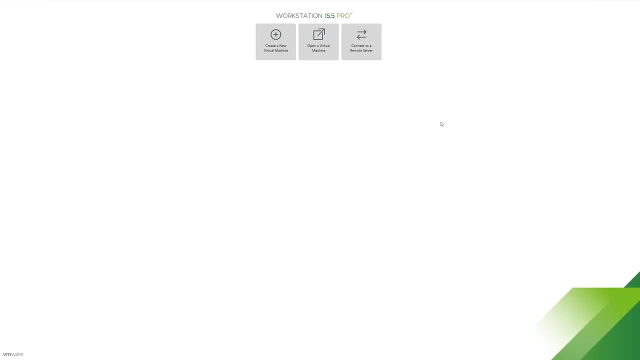 no more issues setting these up. I have full faith in you beyond this, So repeat the process. If you need to go back watch the video, just come back and watch one of these. Anyways, we're going to open a virtual machine. if you are in VMware, I'm going to go into my folder. 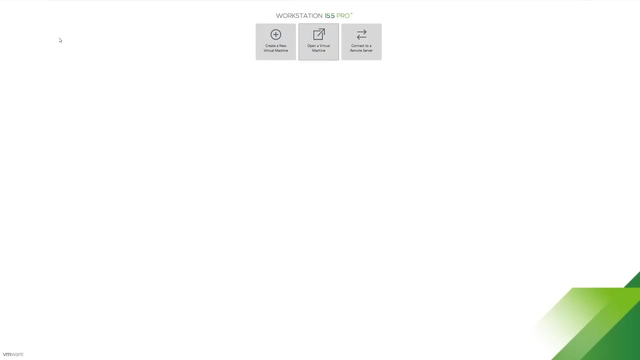 that has it capstone, and I'm going to go to academy and just double click open that up. It's going to ask me where I want to put it. I'm going to go default settings. you can choose wherever you want. I'm just going to hit import. It's going to take a minute to import. while that's happening, 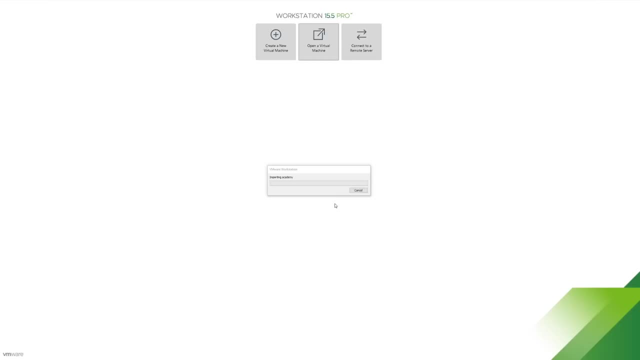 I'm going to show you and you might see a retry. Just go ahead and hit retry on. that should work. While we're waiting, I'm going to go ahead and show you the other side of things, which is VirtualBox. Go ahead and hit file. Go ahead and hit import. 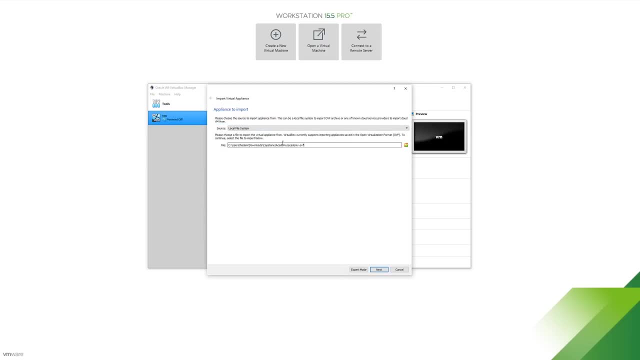 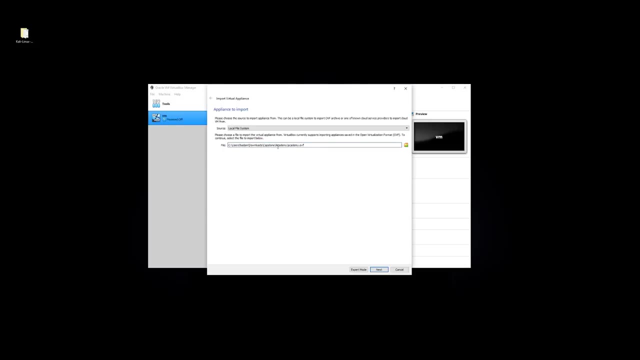 appliance And then just go select your file. I've got it for copy paste purposes. It's a lot easier And VMware thinks it can just take over. It's wrong. So in here, make sure you just have your OVF file that you downloaded, hit next And then come in here And you're going to see. 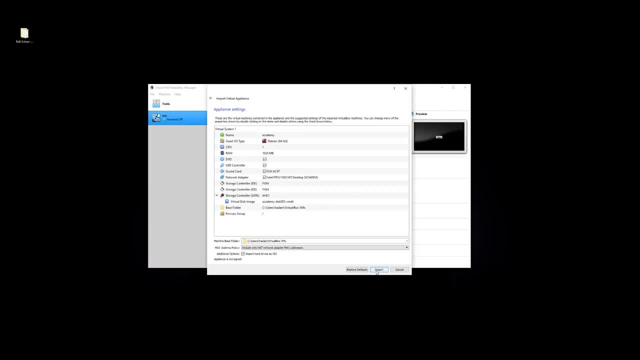 these settings. you can go ahead and just run the default settings for now And just import will be the default settings once we have it imported. So go ahead and import that. On VMware, we're just going to ping pong back and forth real quick Under the settings for the academy. go ahead and 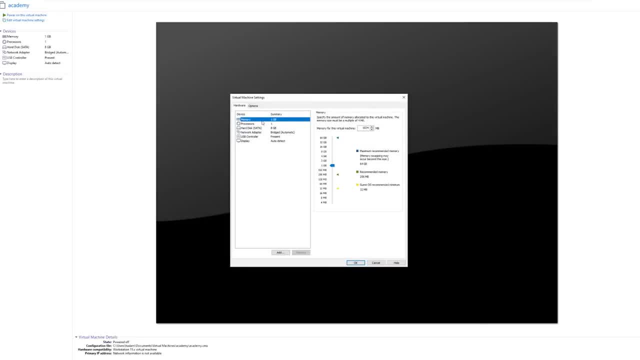 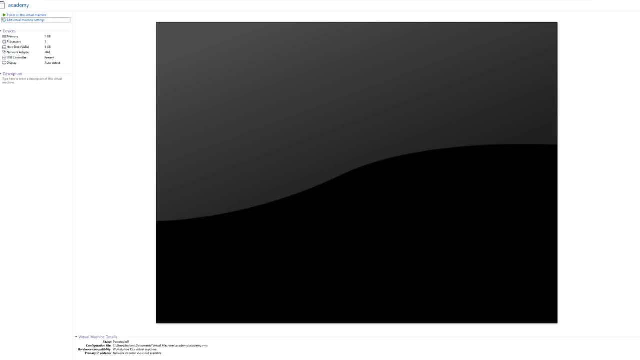 just hit edit virtual machine settings In here. this is a Linux machine, So one gigabyte of memory is fine. we don't need a lot. Come to your network, adapt adapter and make sure that it says nat and not bridged. Hit OK, Go ahead and log in. Now you can power on this virtual machine. get that going. 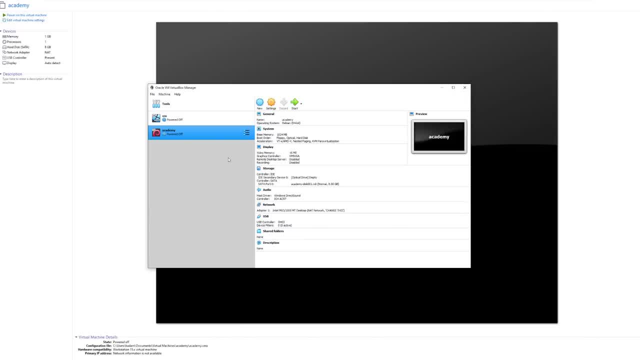 I'm going to show you the password, which is just a root TCM. Same thing here on the academy. go ahead and go to settings. We're going to go to network. Make sure your NAT network is selected. Remember, we created a NAT network. make sure your NAT network is selected and that you're on the. 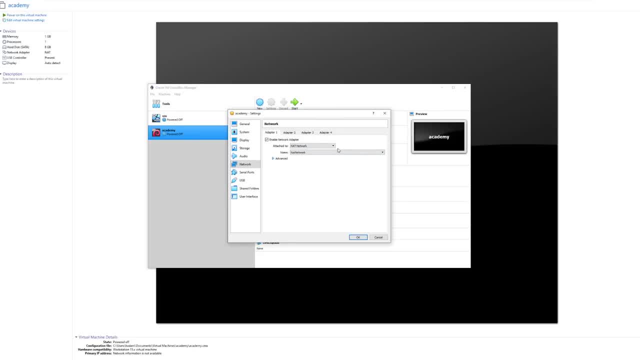 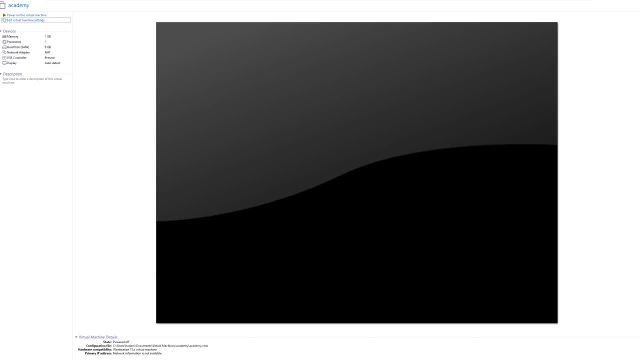 same network as your Kali Linux machine or you will not be able to communicate with it. So with that out of the way, you can go ahead and power this on, depending which one you're on. Catch me in the next video when we will talk about logging in, And I'll see you in the next video. 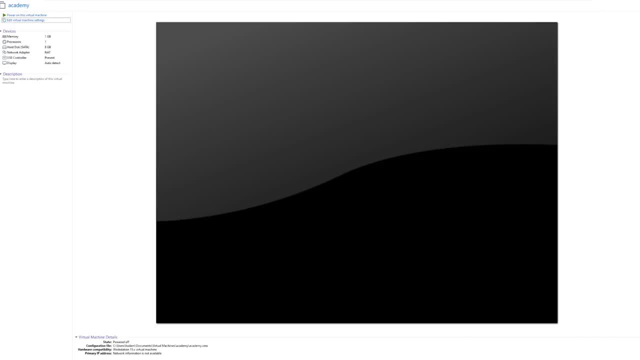 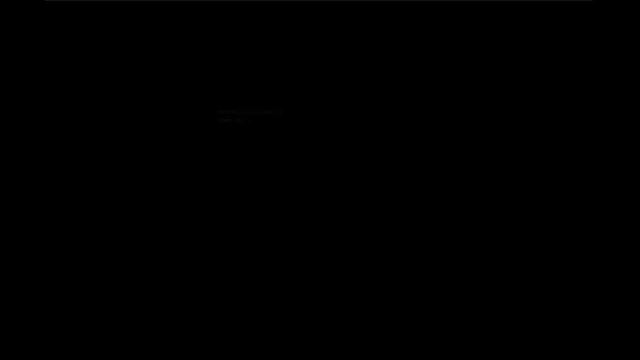 Finding the IP address and getting started with attacking this machine. I'll catch you over in the next video. All right on to the next machine. This one is called Academy And this was created by Alec especially for us. Now we're going to attack this machine And we're going to get a low. 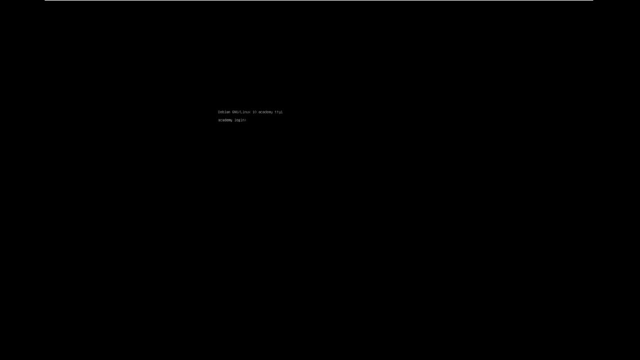 level user, we're going to pivot into a second low level user And then we're going to root this machine. If you did not root this machine, do not stress about it. These boxes are meant to be hard if you are a beginner And you are meant to walk through with us and see all these different. 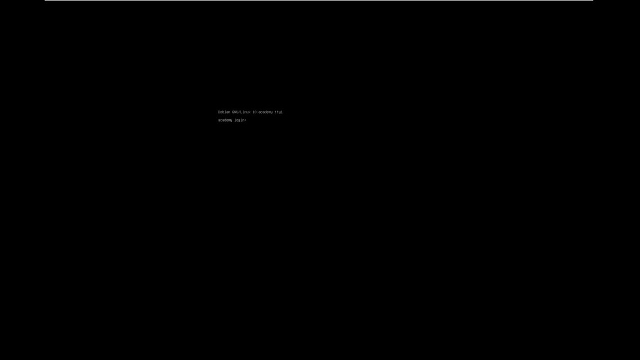 techniques, tips and tricks, and just the idea and mindset as well. So do not stress. if you're having issues trying this on your own, That's 100% Okay. So I have imported the machine. you should be familiar with this. At this point. all I'm going to show you is how to log into the machine. similar 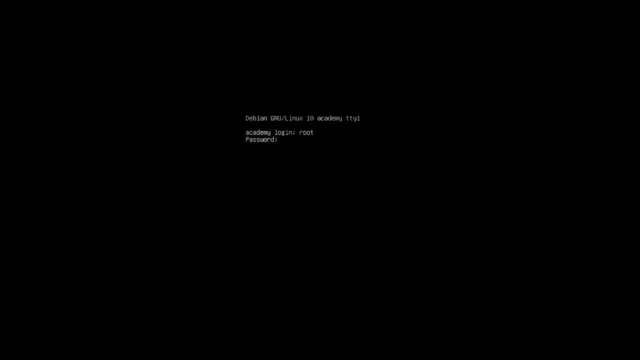 to what we did with the Windows box. Now the password here, the username, is root, the password is TCM Tango, Charlie. Mike, okay, we come in. we're going to run dh client. dh client: hit enter. Okay, mine says file exists. That's because I already ran this. you go ahead and run it. 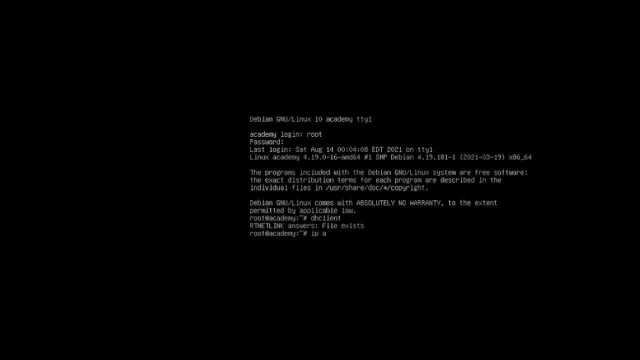 it should take a second to load. Once that loads, go ahead and type IPA And you should get an IP address back: Okay, 292-168-138-129.. Yours might say something incredibly different, But go ahead and go with. 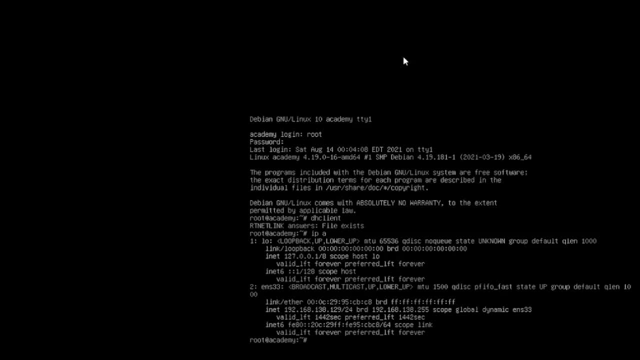 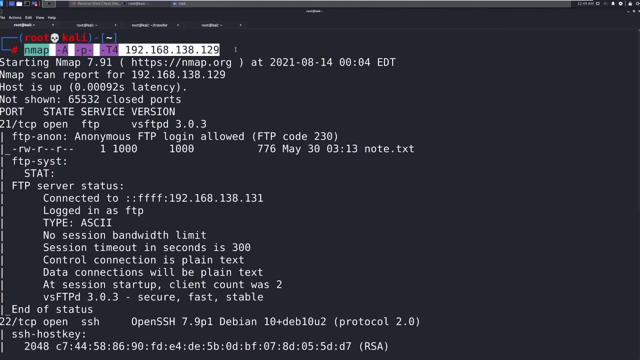 whatever the IP address says here, because that's what you're going to use Now. with that out of the way, I went ahead through the magic of editing and ran a n map scan. you're welcome to do this as well. dash capital A, dash p, dash, dash t for IP address. Nothing new at this point, Okay. 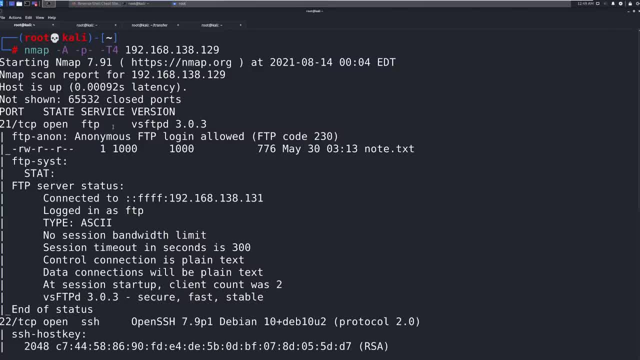 What came back for us was a few different things. here We have port 21 open And we have a VSF TPD. say that three times fast: 3.0, point three. And it says anonymous FTP login is allowed. Okay, it says hey, there's a notetxt. 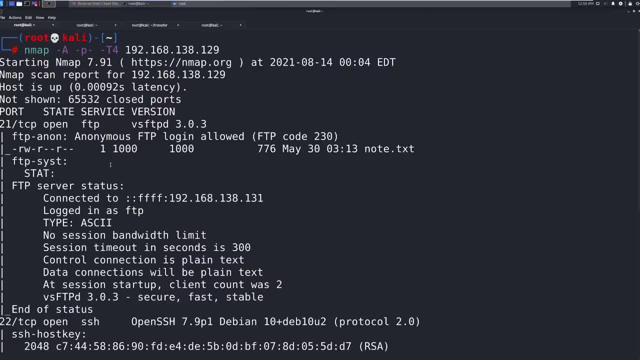 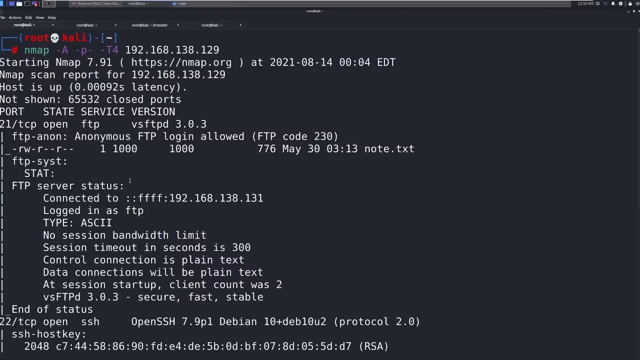 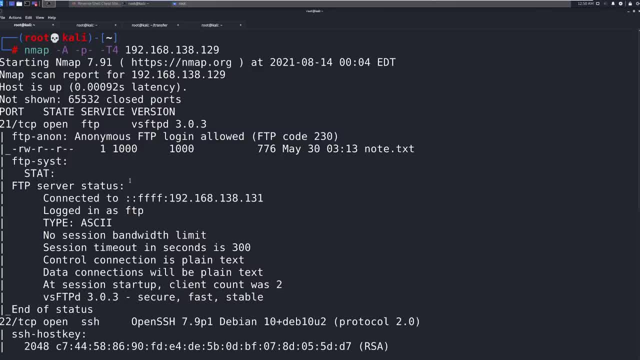 directory- pen testing section. we're really just trying to focus on some of the basic concepts and some of the things that you'll see if you go do any CTF events or you go on to any other certifications or anything like that. So this is a good introduction, kind of jump into the pool. 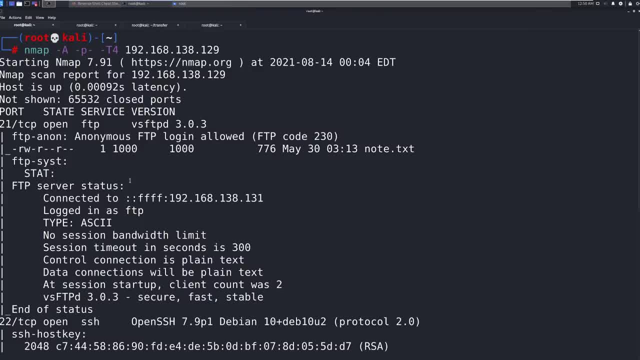 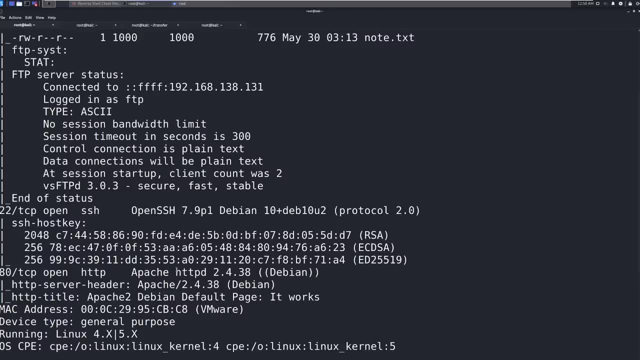 maybe get your feet wet first into hacking. So this is a good introduction, kind of jump into the pool, maybe get your feet wet first into hacking. So with this in mind, we've got port 21,, we've got port 22,, we've got port 80. Now 80 is a web server. 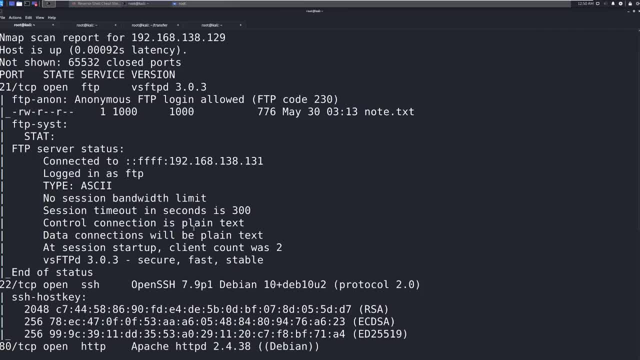 22 is SSH. My strategy here: when I see port 22, I immediately erase it off the board. Now, that's not to say that it couldn't have an option of attack here. you could brute force it. you could go in there and try, like a root username, Or if you knew other usernames, you can go in there and just try to brute force it. You could go in there and try like a root username. Or if you knew other usernames, you could go in there and try like a root username. Or if you knew other usernames, you could go in there and try like a root username. 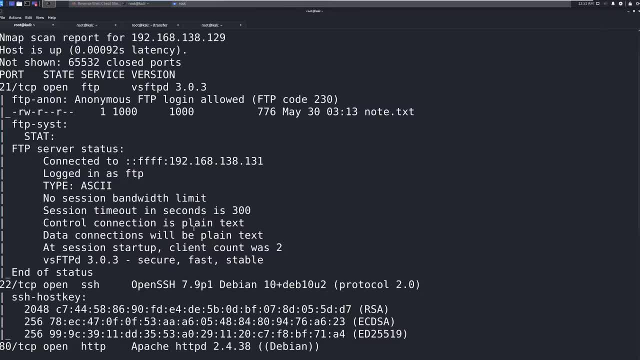 And maybe you get lucky and log in, Usually on CTS. that is not the intended route Now for things like, say example, a pen test. you might want to brute force SSH because there's a couple reasons. One is: is there a weak password? Can I log in with a root user on a weak password for this machine? 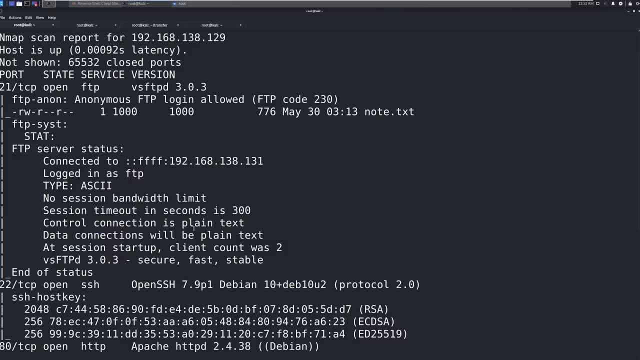 If so, that's bad. You tell your client: hey, this is bad, you're using weak passwords. Number two: you want to see if your client can pick you up Meaning. do they detect you when you are running brute force scans? If you have 500 attempts against an SSH login and you're still able to go? 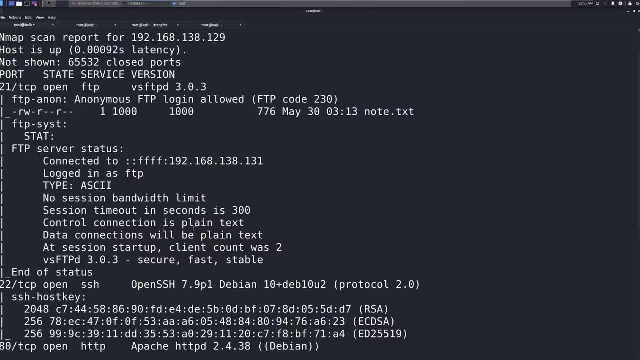 attempt after attempt and nothing has been detected, you have not been prevented on that network, then that's an issue. You should probably bring that up to the client. say, hey, I ran a brute force against this login And you didn't detect me. you didn't see me, you didn't. 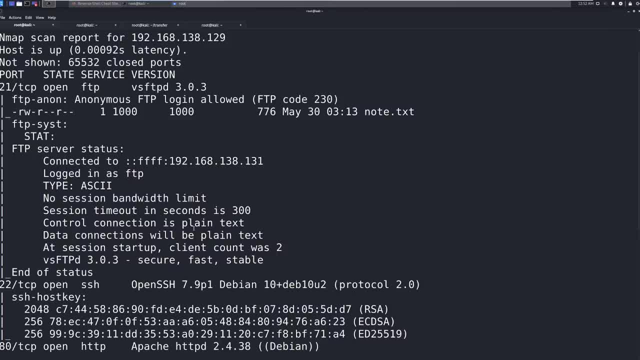 see me do anything. We'll talk about that more in the report writing section, And some of the things that you might want to do is: you might want to do a test, So you want to do a test to see if you're detected. You're testing detection throughout an entire pen test, So you want to say hey. 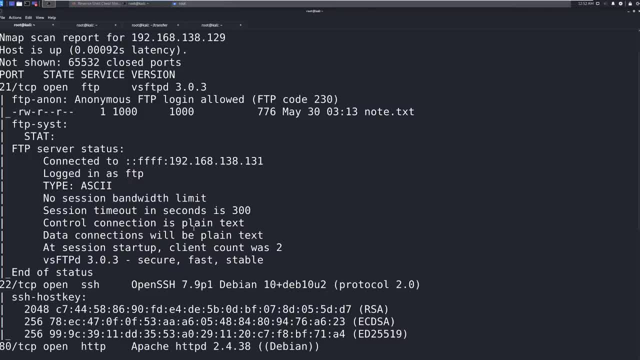 did you see me scanning? Did you see me brute forcing? Did you see me running exploits? Did your antivirus pick me up? Where was I caught during this pen test And where can you improve? So something about SSH. a little tangent there, But with that out of the way, port 21 is open. 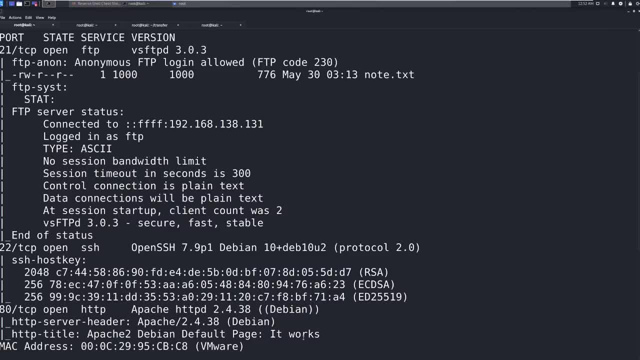 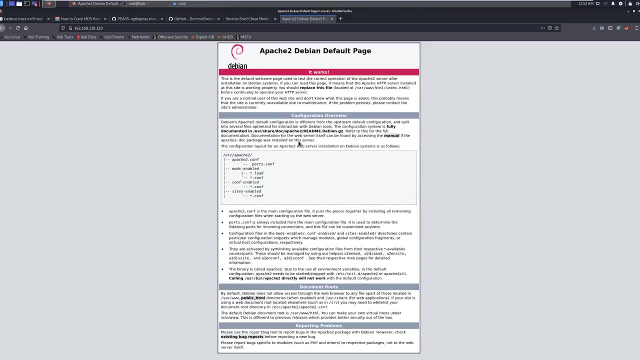 port 80 is open. Now we see down here that it says hey, we're getting an it works page, which means that it's just a default Apache to web server. we can go out to this web server And just take a look: 192, 168, 138, 129.. You can see this is just a basic Hey, it. 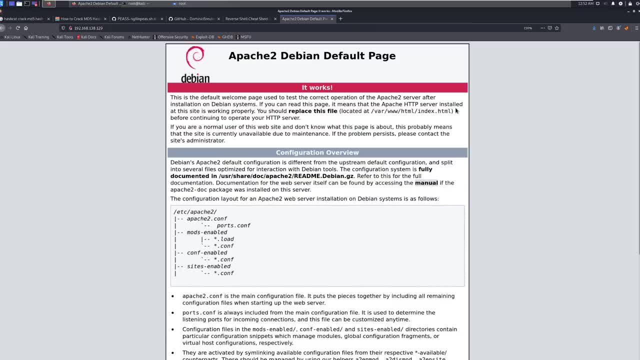 works. Apache to Debian page. That tells me that we're likely running on PHP on the back end, though that doesn't mean that entirely. this is just kind of an indicator. when we see Apache, I'm assuming PHP on the back end. So let's go back here. 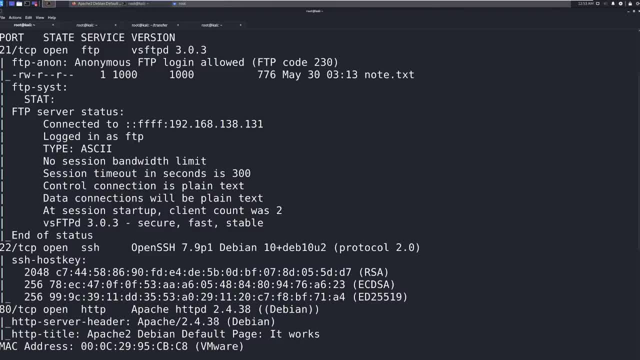 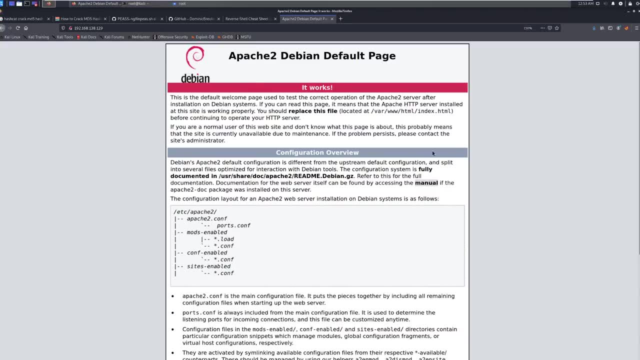 Now we could do a couple things. we need to identify what's going on behind the scenes, because all we're seeing is a default web page which, by the way, this is a finding on a pen test. So you would say, hey, this is just revealing too much information. Why do you even have this? 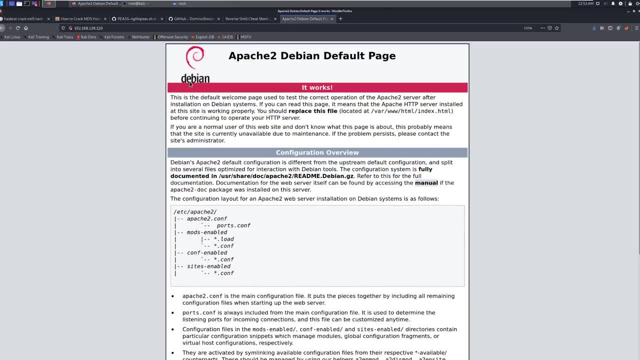 out there. Is this web server meant to be up? If it is, then take away this default web page. make it, you know. make it, say hey, if you're not supposed to be here, then don't be here. 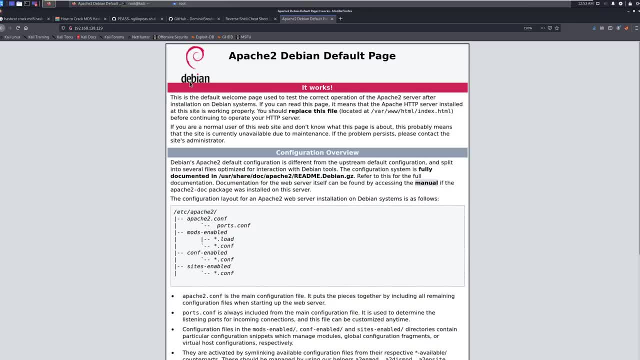 Anything but a default web page, because all we're seeing is architecture here If it's not supposed to be there. from a hackers perspective, this means poor hygiene. you're just leaving ports open, you're just throwing computers on the network and on the internet willy nilly, And this just means that. 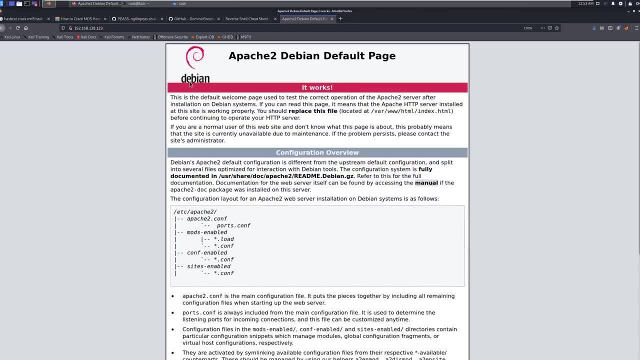 you likely have poor hygiene And we want to look into you further Because if this is something you're doing, you might be using bad passwords or not patching, etc. etc. So anyway, off that tangent. going back to the scan, I'm curious to know what the note says. We'll go check that out. 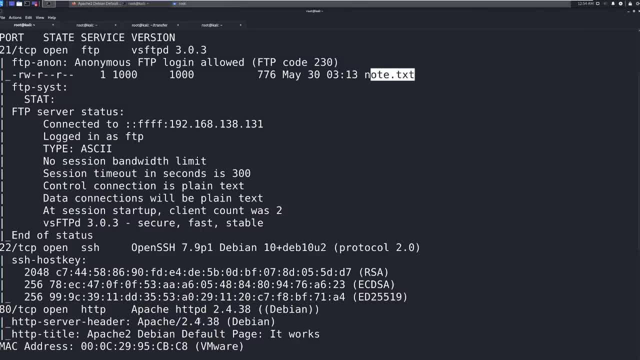 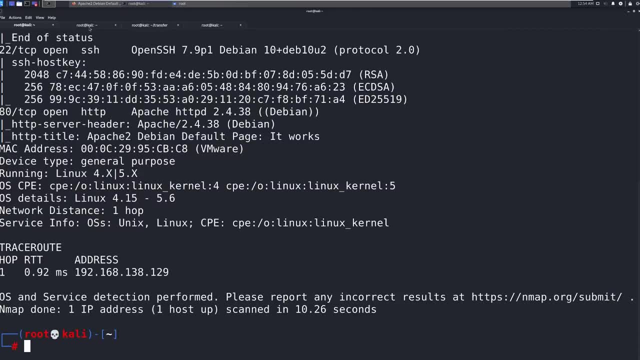 we have anonymous login, So we'll start there, And then we're going to go ahead and take a look at the different pages that could be hiding behind the default page. So I'm going to leave this up And now we're gonna go take a look first at the FTP. So in here I'm going to make this bigger, Okay, 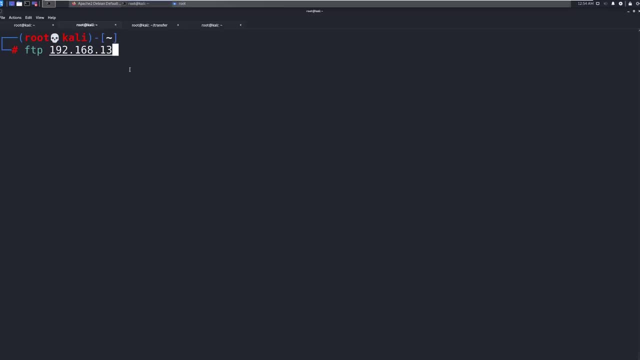 so FTP. all you gotta do is 192, 168, 138, 129, or whatever your IP addresses. And then I like to just type anonymous twice. Okay, we get an anonymous login. we are successful, we can come in here and 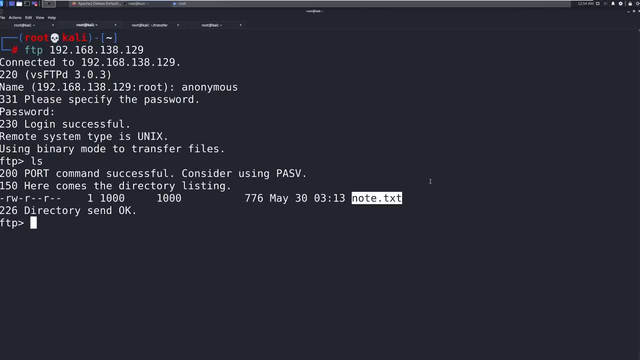 we can see that we have a notetxt in here, So all we need to do is type in get notetxt. That's it, And we're pretty much done. So the option here is: we have FTP open. Now there's a possibility that we could utilize this, So we have the ability, with FTP, to put files and get. 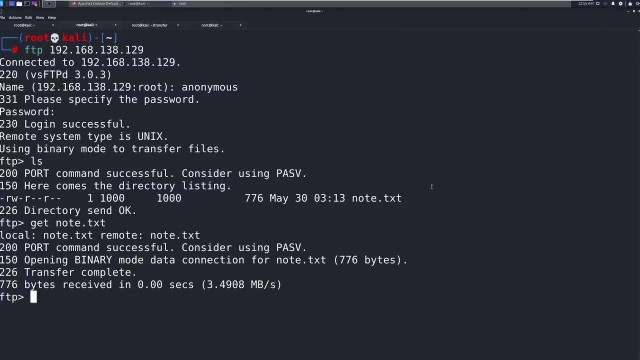 files. we just got a file. we can come put something on here. The only issue is we don't know where on this machine that this notetxt is. So we're going to go ahead and type in a notetxt And notetxt is stored. If, for some reason, this note file was stored in like the, I don't know this. 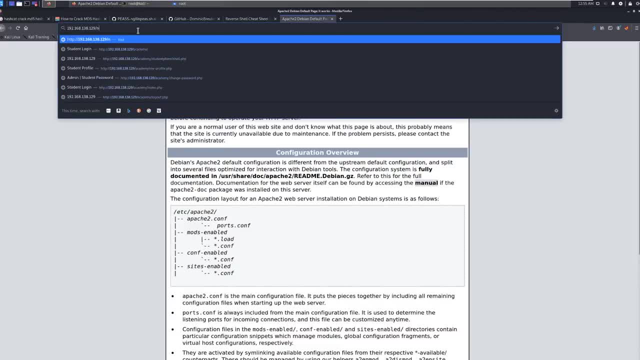 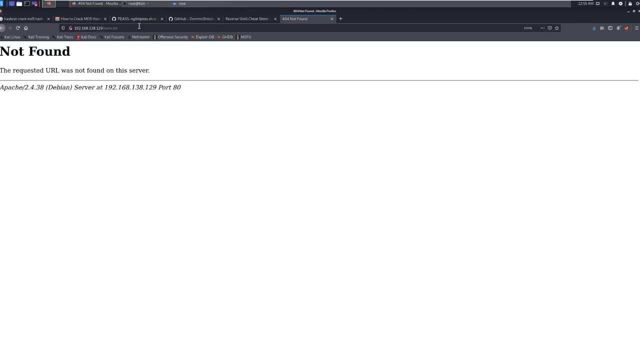 Apache server. we came in here and we just went like forward slash, notetxt And we saw it All right. then that could be of interest because we know the directory that we're in. we can come in here just upload malware, come up here, execute the malware, because we have execution, And then 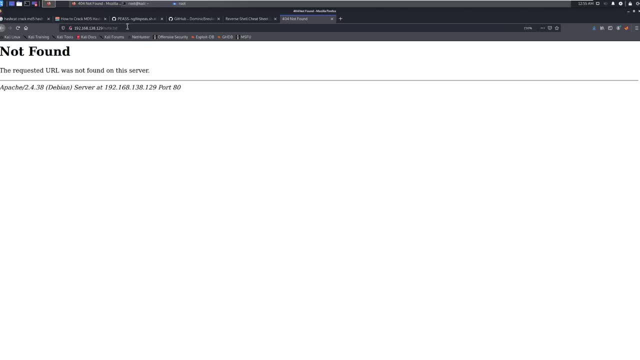 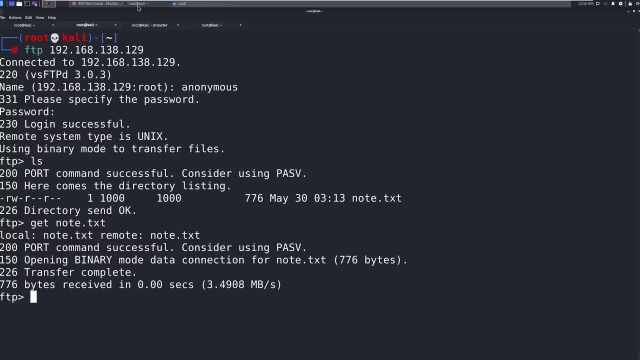 we could get a shell and keep pushing forward, But in this instance we don't know where it is. It's there's a good chance it's not even in the web server. If for some reason it wasn't the web server, we could use that to execute, And that is a strategy that we might see at some point. But 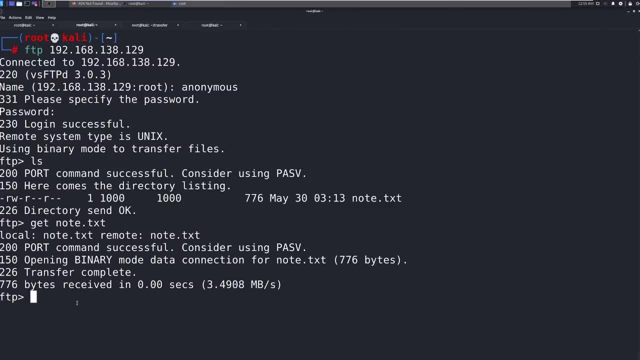 here in this instance, unless I know where this is, the ability to put files in here does nothing for me In a real world scenario maybe. maybe we can go look at getting social engineering or getting somebody to open a file or something along those lines. But for here, for this capture. 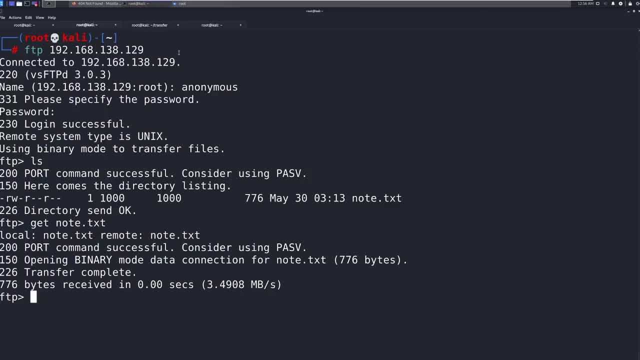 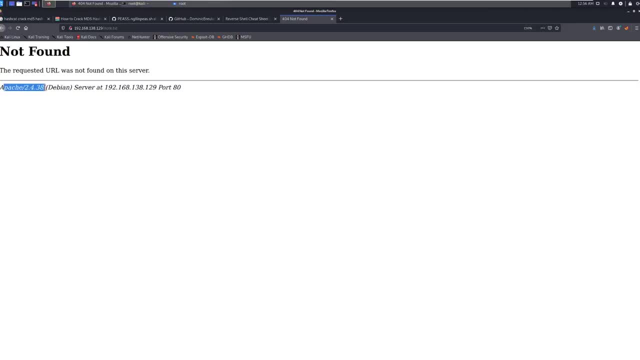 the flag type style. we are only focused on getting this notetxt And then we can go ahead and click on this note And that's pretty much it. Also, secondary finding on a pen test would be this: because we see Apache 2.4, point 38. It's telling us it's running a Debian server which 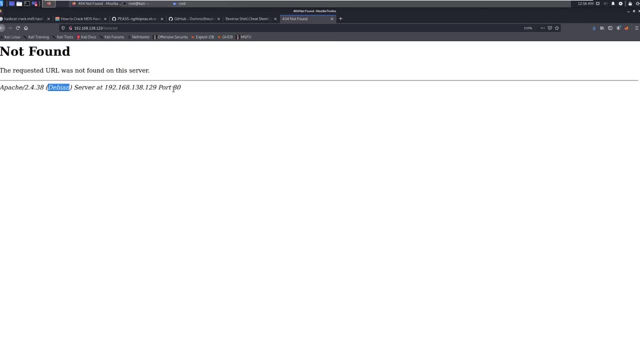 means we're attacking Linux. So if we were doing this blind, didn't know that. now we know. we know the Apache version, we know Debian. we're getting a little bit of information And we're just compiling that information right now: Debian server, Apache, PHP most likely. okay, all of. 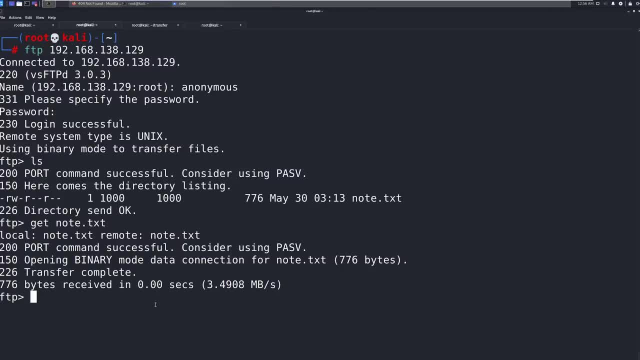 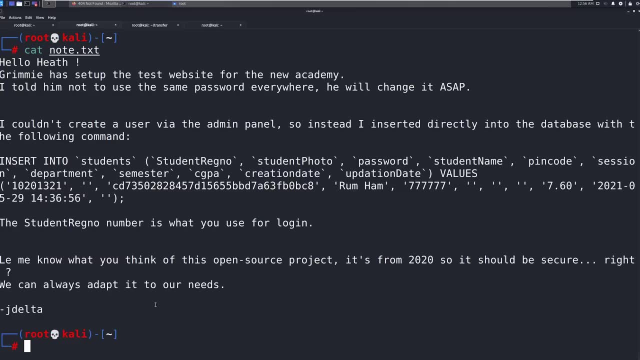 this is information gathering, And that's all we want to do- is gather as much information as possible. Now let's go ahead and exit out, And I want to just cut out this note about txt: Okay, so it says: Hello, Heath Grimmie has set up the test website for the new academy. 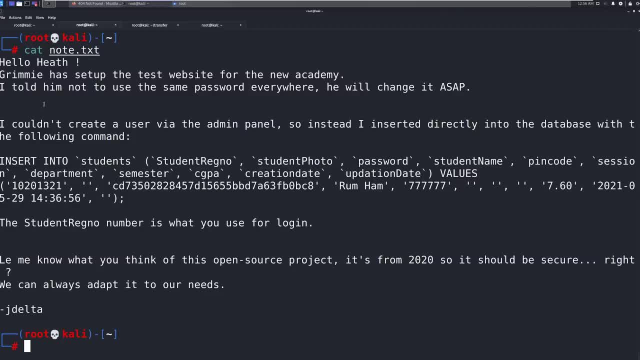 I told him not to use the same password everywhere. he will change it ASAP. I couldn't create a user via the admin panel, So instead I inserted directly into the database with the following command: Alright, so we get the looks like a database information. 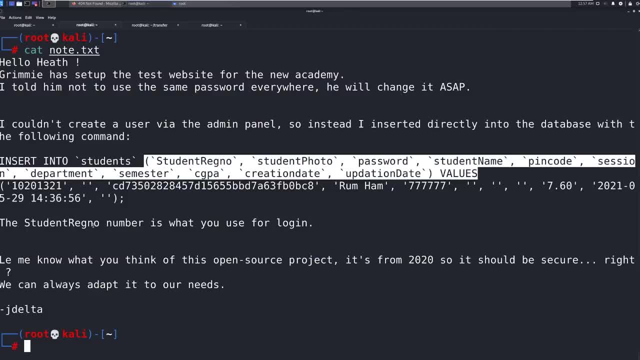 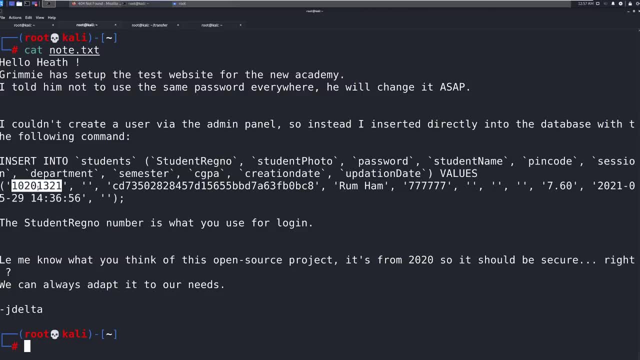 here with values. Now it says the student reg no number is what you use for login. So student reg: no. here you see this ties up to the first and then we see student photo And there's nothing in for the student photo. We see password. then we get password here. student name: okay, pin. 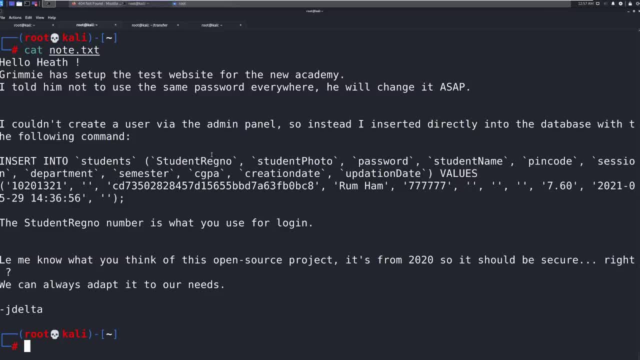 code going on. So this is pretty sensitive information If this were on a pen test, which I've actually seen something similar to this. I've been on pen tests where I have seen open FTP. I've seen open web directories where they had backups of their entire website on there with 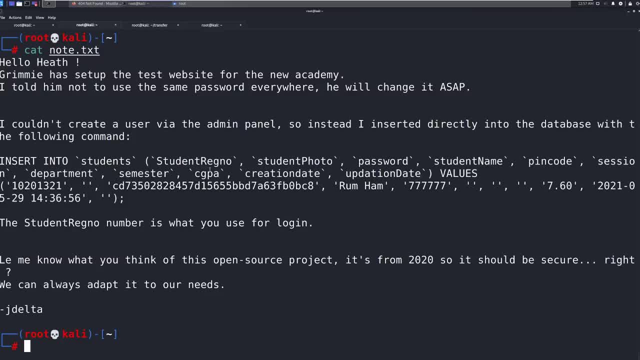 database passwords and everything It is. it's realistic in a sense that you could run into something like this. it would be pretty, pretty bad. So, anyway, this is coming from our friend j delta, And we're going to go ahead and just grab this password here. we've got this. we've got this. 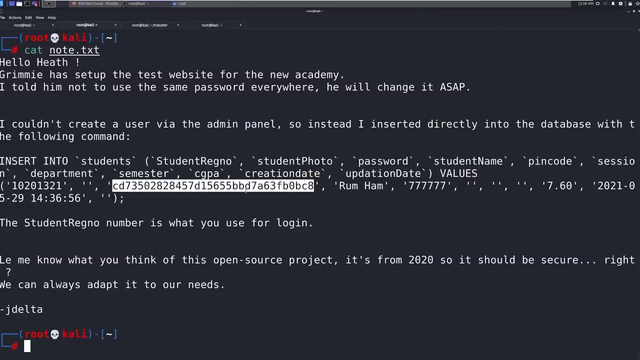 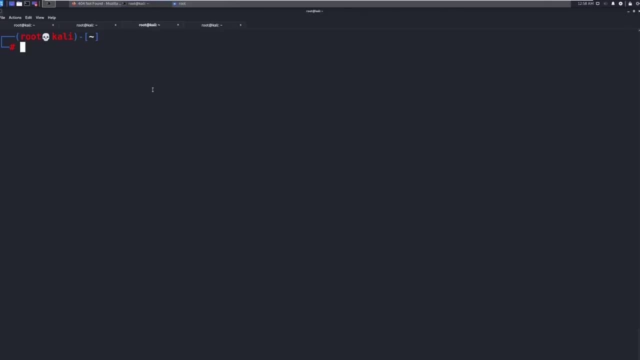 now the issue is: this is likely not a password, This is likely a hash And we can copy this and see first before we go down that route. This might be a password, but we can copy and let's just take a quick look. we can go, let me see the back out of this. Here we can do something like: 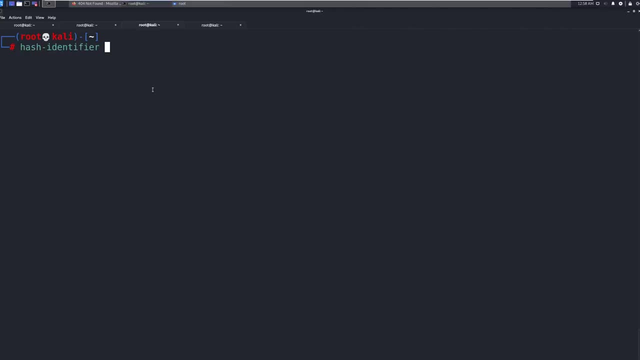 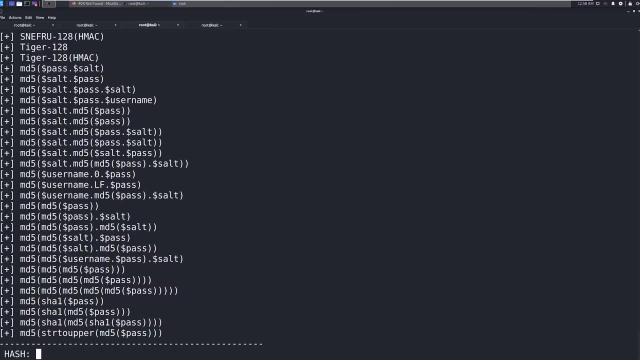 this: we can type in hash identifier like this and just hit enter. Okay, this is built into Kali Linux. you just go ahead and paste selection, hit enter And this will tell you all the things that it thinks it is. this is saying hey, most likely. 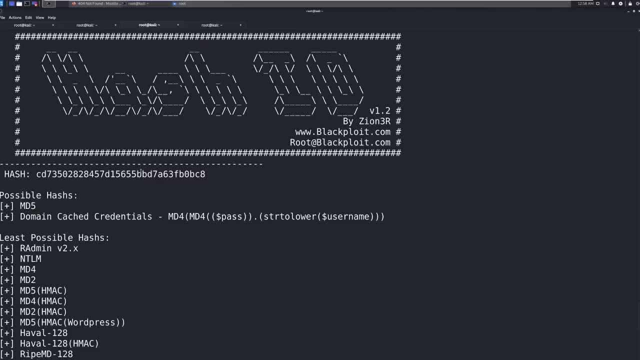 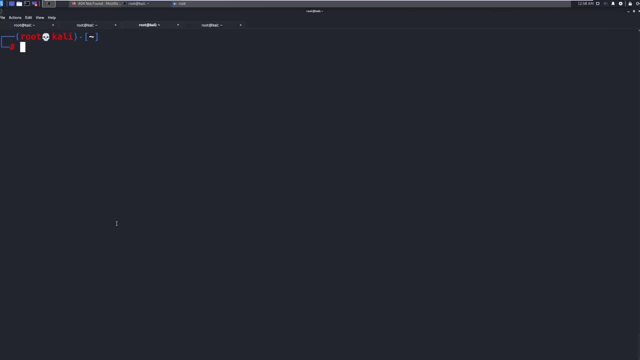 it's md5 hash. Okay, so we have an md5 hash. guess what we can crack that hash. I'm going to go ahead and exit out of here with Ctrl C And if we go to Google and do a quick Google search. so 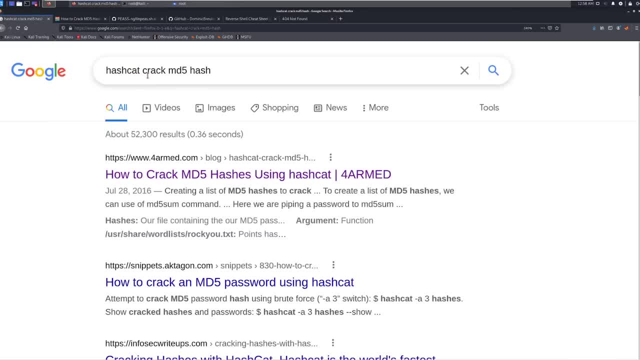 I'll give you time to go to a go do a Google search, But all you have to do is say hash cat, which is the tool we're going to use to crack this password. crack md5 hash. Here we get a. 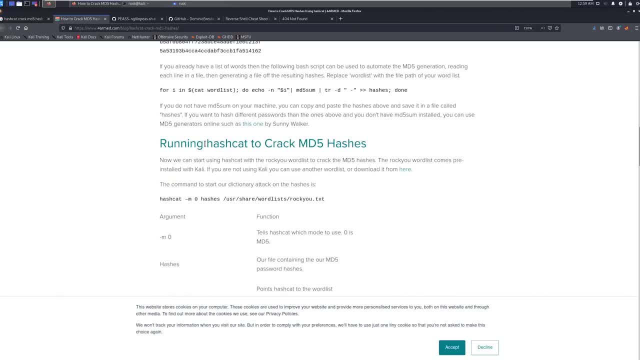 a blog. this is how to crack md5 hashes. you go into that And it says Hey, in order to do that you need to run hash cat, dash m for module and zero with your hashes file and then a password list like rock youtxt. So we haven't gotten much into hash cracking in this course And we're going. 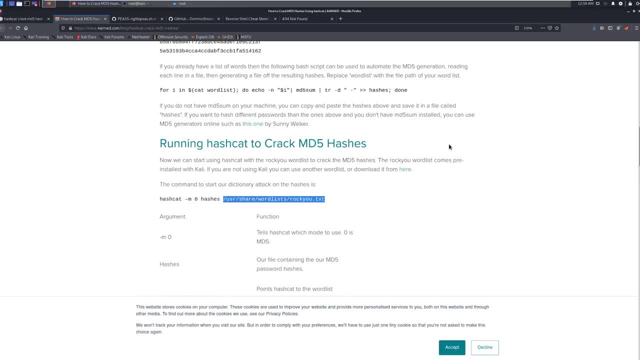 to talk about a little bit. we'll talk about it a lot more. when we get into the actual active directory, hacking- because we start cracking passwords there- becomes a lot more important. So I'm just going to play around with it a little bit. So I'm going to show you this, Only this one. 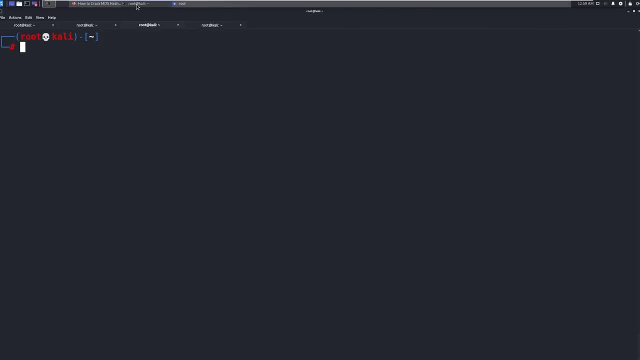 time. I'm going to show you this on on a Linux machine. This is running in a virtual machine here. Okay, so we're running hash cat. we're about to run hash cat in a virtual machine. Typically, we do not want to do this, because hash cat is going to be running off of our CPU. 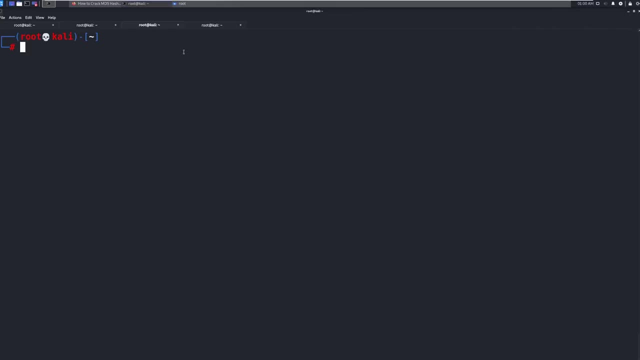 Okay, it's going to be running off our CPU inside a virtual machine. That's going to make it run a lot slower. hash cracking runs off of GPUs. Okay, so we're running off of the graphics card, not our CPU, So we want to do that. So when I run hash cracking in the real 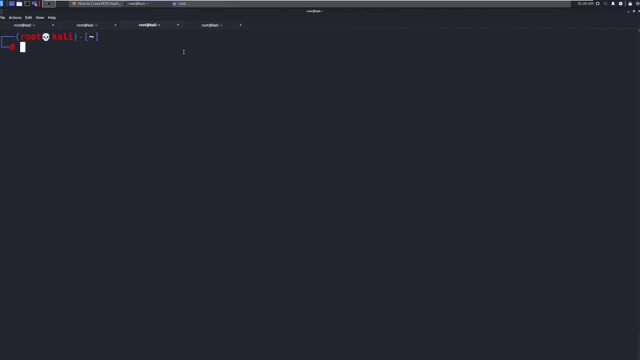 world or even later in this course. you're going to see me running it on Windows, because that is my base operating system. I will take that. I'll run it off there, because it's going to use my GPU, it's going to use my graphics card And that's what I want. So in this instance it's going to. 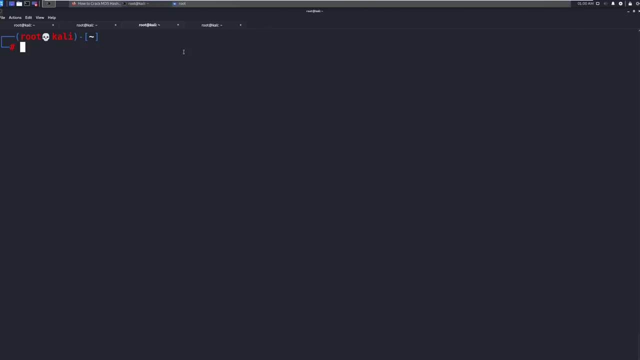 run a lot slower, But because it's going to be an easy password to crack, we don't have to worry about it too much. But if you want to be good at cracking passwords and practice that, definitely make sure you're using it on your base OS, regardless of what it is, because some crack a lot. 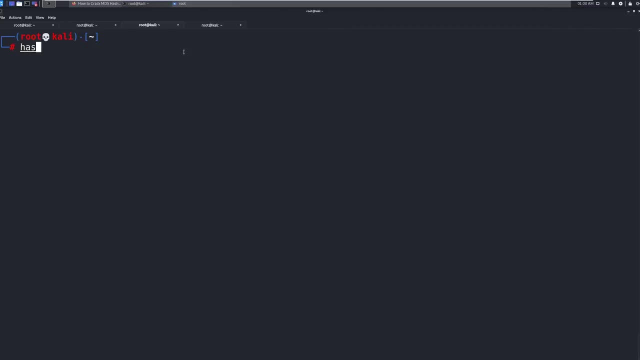 faster than running it in your virtual machine. So we're going to do a hash cat. Actually, before we do that, go ahead and type in locate rock you dot txt. you should have it somewhere. Okay, you might have a tarred version of it or a G zip version of it. you can. 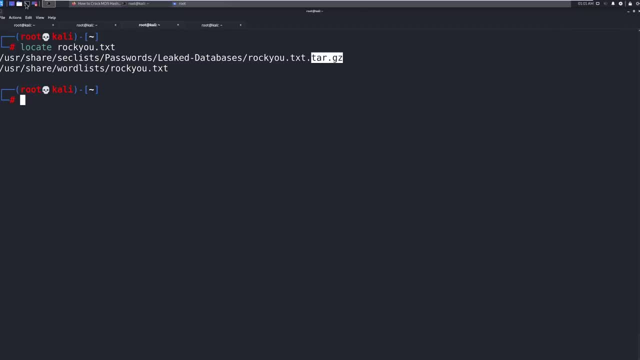 that if you navigate to this folder like user share, come in here to your folder like, literally go into browse network or file system and go into user share etc. You can get there. if for some reason, you do not have rocky dot txt in the later version of Kali, they already have it here, So I'm 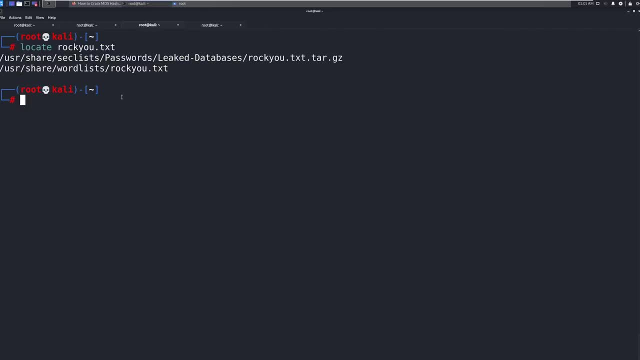 assuming that it's here. If not, if all you see is a G zip, go ahead and just unzip that. Now, what we're going to do is we're going to say actually, one more thing I forgot. you can go ahead and do a. 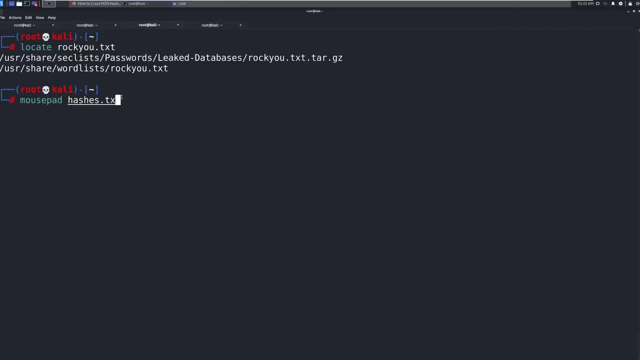 mouse pad or G edit or whatever You want. you can do a hashes dot txt. copy and paste the hash. it's a little small probably for your screen From what you can see here. copy and paste the hash into this hashes dot txt, the one we got. 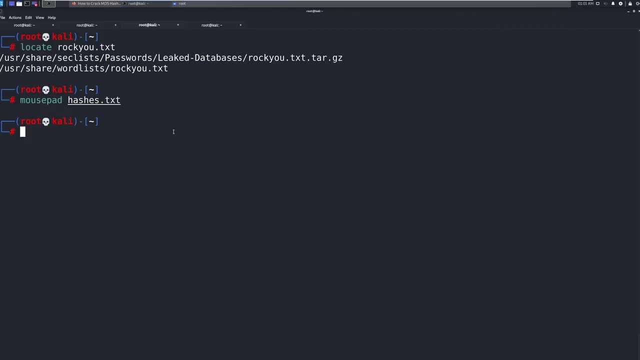 right here. Okay, make sure it's in a file. So once we've done that, go ahead and run hash cat with a dash m of zero. that's a module. So we're going to be attacking the module of zero, which correlates. 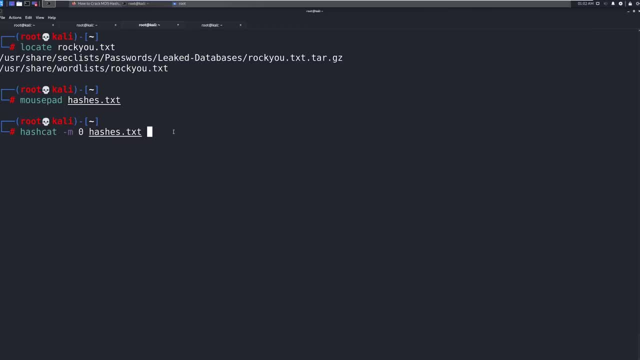 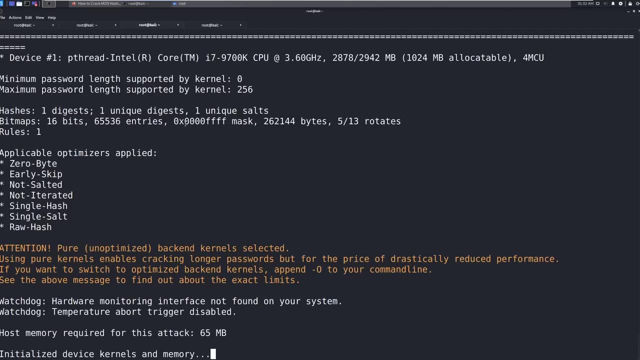 to MD five: hashing. we're going to give it the file of hashes dot txt And we're going to give it a word list to run through of rock you dot txt. Okay, and I'm gonna scroll up just so you can see this. It's going to run. it might take a minute to run. took me a. 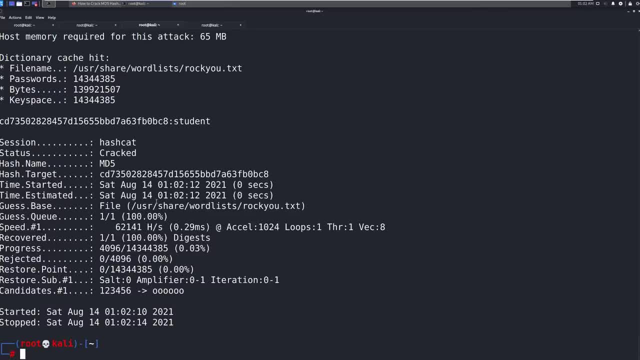 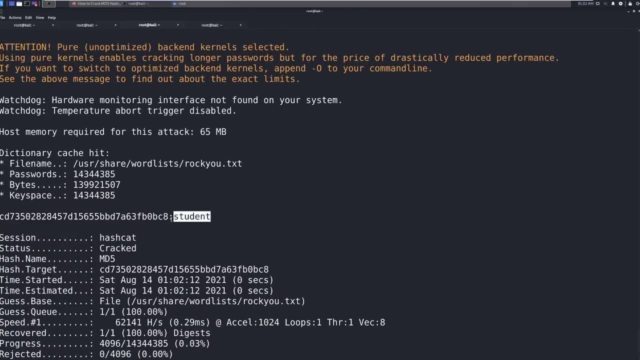 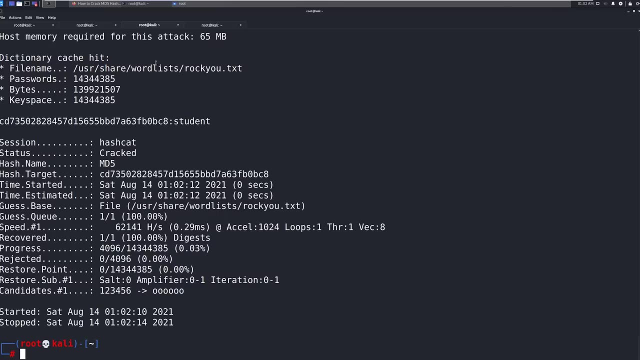 couple seconds here gets there pretty quick. Rocky runs fairly fast on a VM And this one picked it up pretty quick. So the password of what's coming up is student. password of student. not very great password. weak password policy. Okay, so we have a username, we have a user ID, we have a password of student, but we have no idea how we're. 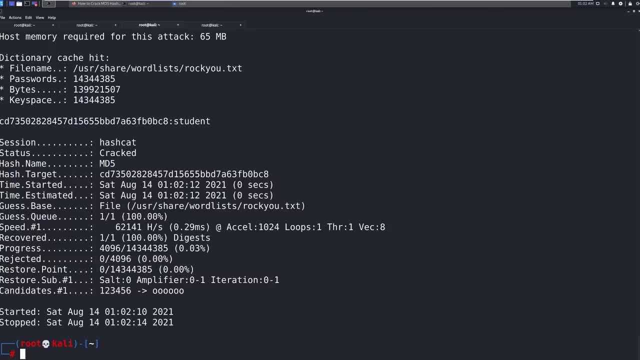 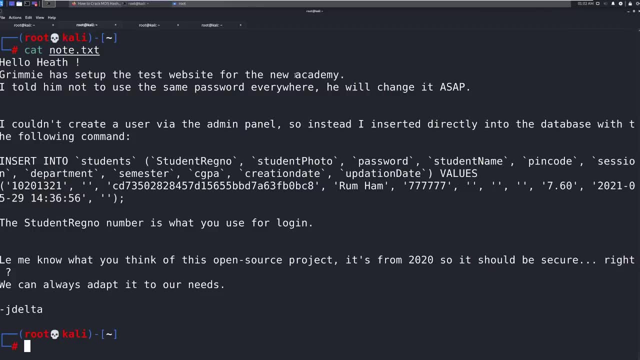 going to do this. Okay, where are we going now? I can take some educated guesses here, Like, for example: they're saying: hey, this is for the new Academy and this box is called Academy, And there's a good likelihood that if you were to do a 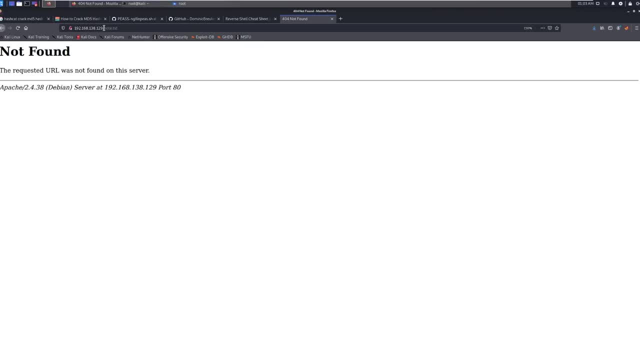 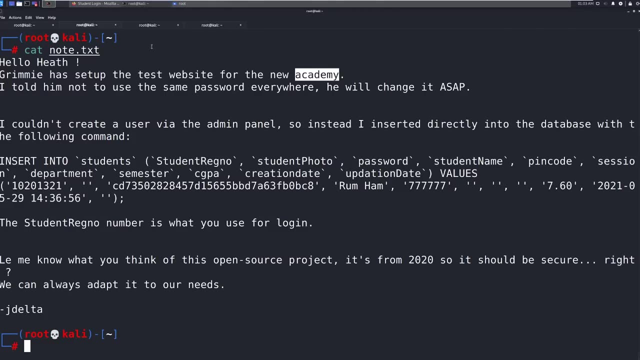 forward slash Academy on the web page that maybe you it right and we can go academy and go find it. but i don't want to just show you and cheat, so let's go back and we're going to walk through it. we talked about directory busting with dir. 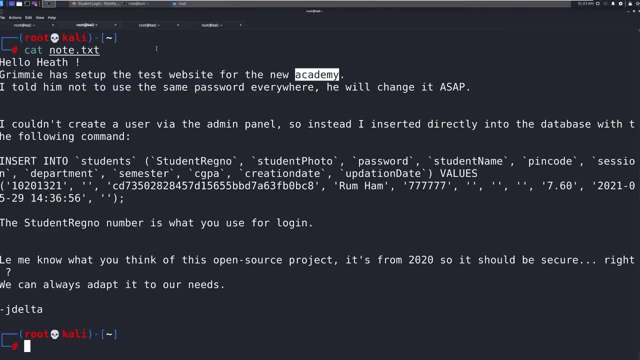 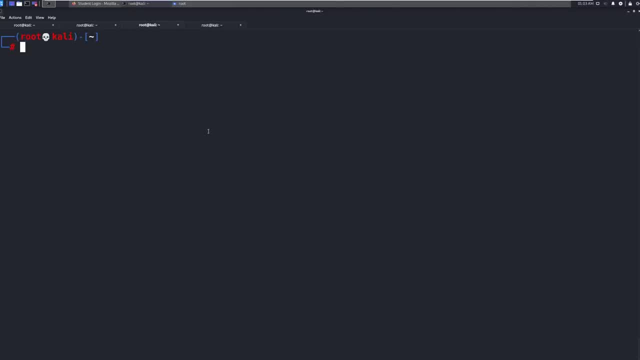 buster, i want to show you a couple other tools that we can use and show you the pros and cons of both of them. so open up a new tab, make sure we're going to use two different tools. so i want to show you both. go ahead and use a tool called dirb, d-i-r-b and for derb, all we have to do. 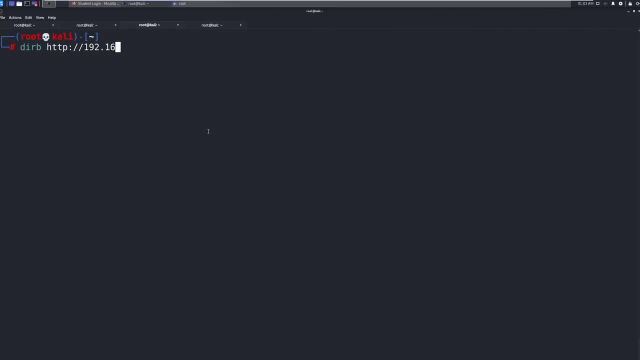 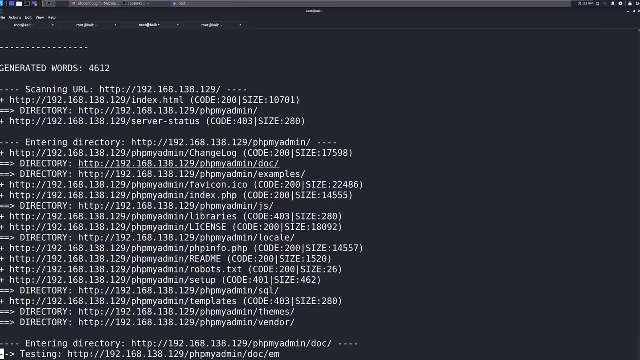 i do believe is just type in 192, 168, 138, 129 and hit enter. so this is going to go off of the website. it's going to run on its own word list. it's going to go in here and try to find stuff immediately. i found php, my admin. the issue is with this. it's just going to go in and start like: 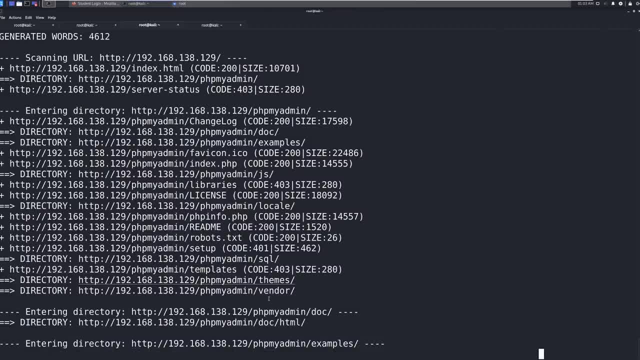 going in and going into the phpmyadmin and looking for directories and it's finding all kinds of directories and this is going to take a minute. so this is one way of doing it. another way of doing it is you're going to go to your directory and you're going to go to your directory and you're. 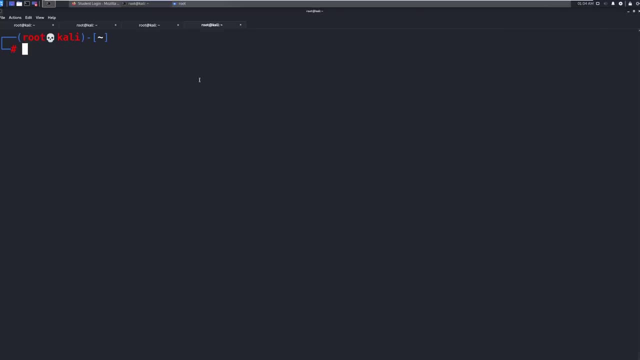 it is using a tool called FF. I don't know how you say it. FF, uh, whatever. Everybody's got their own pronunciation. If you do an app install of FF UF like this, you hit enter. I already have it, but yours should pick it up. Okay, We're going to run the tool just like this. So we're going to. 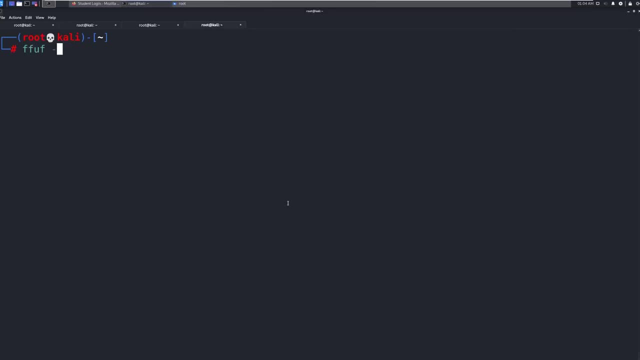 say FF, UF, Once yours is installed, do a dash W. that is for word list, and your word list should be in user share word lists. but we can do Durabuster, That's fine. This is where all the word lists are, And then I just like to double tab or tab around, and we're going to use the. 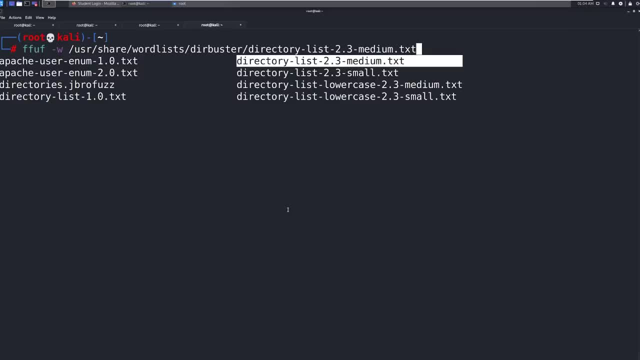 medium word list. That's my, my go-to for most cases. We could use the lowercase if we wanted to. Um, I think either are fine. Okay, From here I'm going to go ahead and, um, we're gonna go. 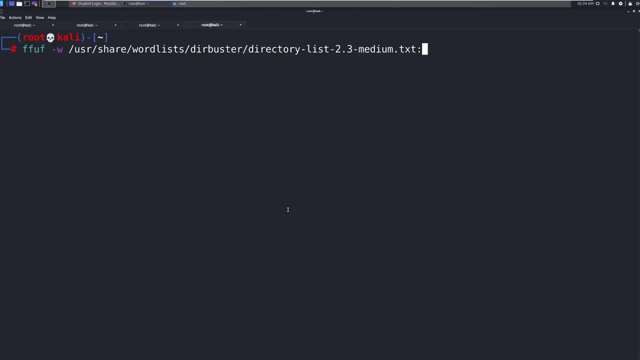 ahead and back up. And now what I'm going to do is I'm going to put a colon here And I'm going to type in: fuzz. Okay, This is what we're going to fuzz, We're going to do a dash U. 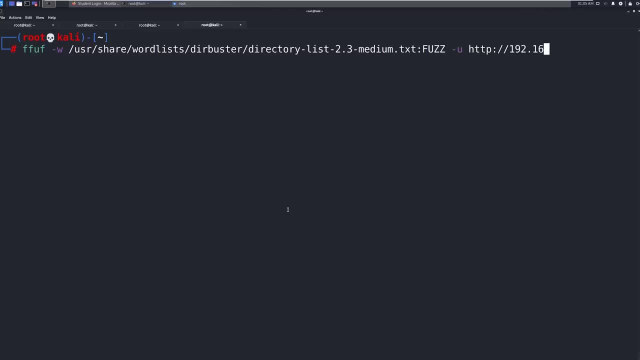 and we're going to do HTTP 1 9, 2, 1, 6, 8, 1, 3, 8, 1, 2, 9.. And we're going to say forward slash, fuzz. So we're telling this is Hey, with this word list, we're going to be fuzzing with this word. 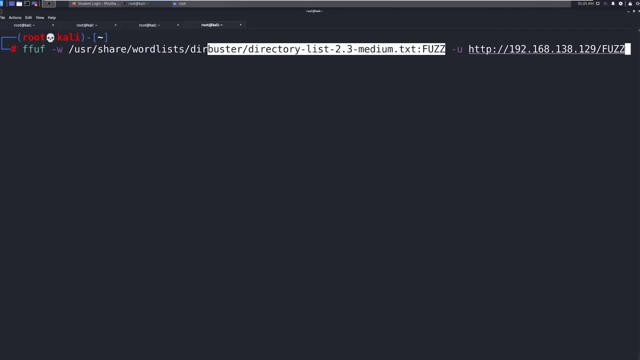 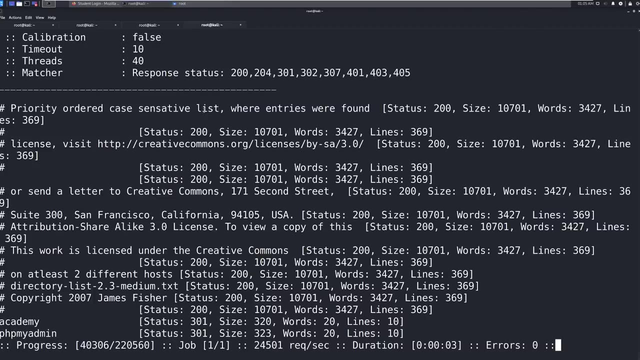 list. We're going to fuzz this parameter right here is exactly what we're doing. Okay, We're going to hit enter and this is immediately going in and just Doing all that we want to do. I found Academy right away, PHP Miami right away, And this is: 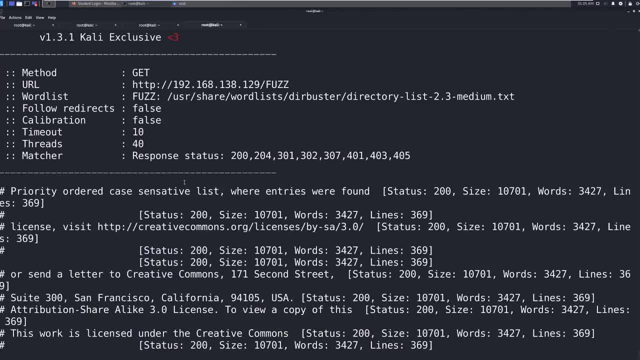 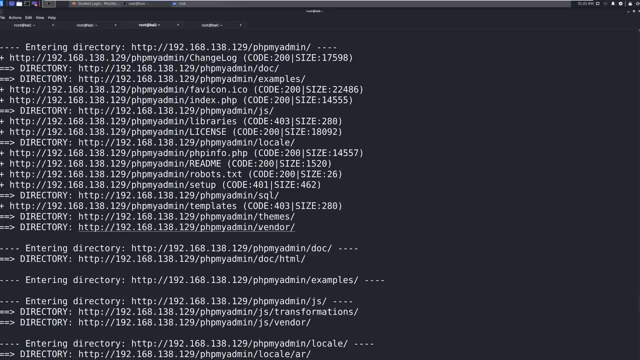 very fast Found a server status and all it's doing is looking one thread deep, So it's not doing what DERB is doing. DERB is going and saying, Hey, I found PHP, my admin. Now I'm going to go through and find every single directory inside of that, And every single. 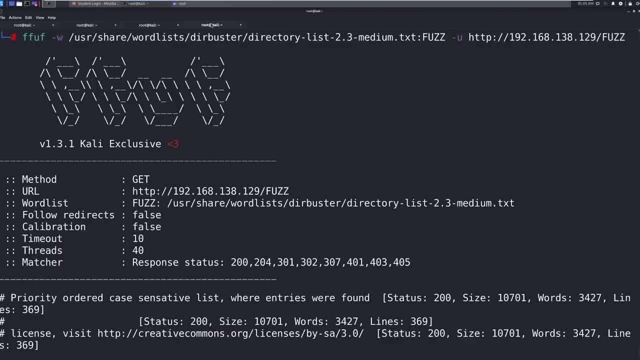 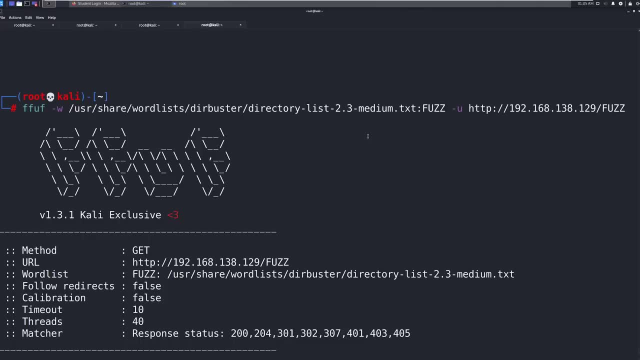 directory, inside of those directories, which can take a while. Uh, this one is saying: I'll find all the first level directories And if you want to go search those, you can. like we can type in: Academy slash fuzz. There's commands in here that we can use And then we're going to go ahead and 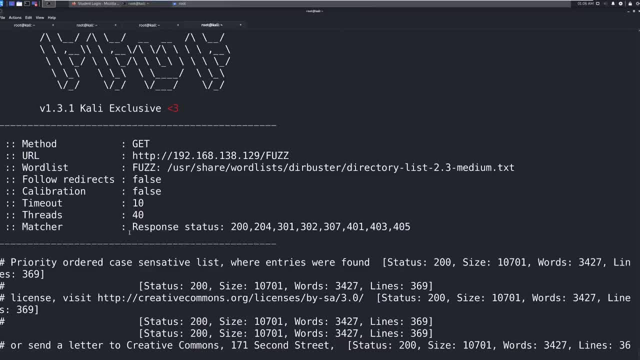 type in academy slash fuzz. There's commands in here that we can use. And then we're going to type in academy slash fuzz. There's commands in here that we can do. to take this further, We can limit which response statuses we want. Maybe we only want 200s, or maybe we want 302s, depending on this. 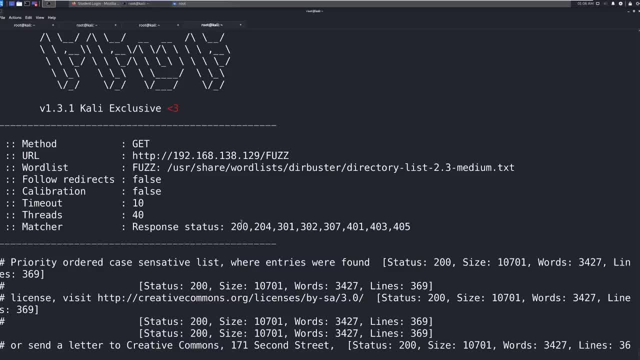 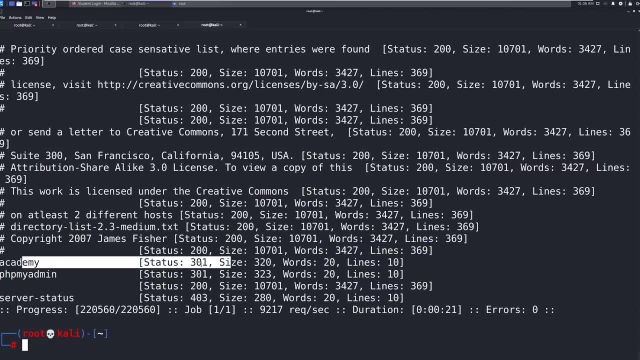 So maybe we don't want any 401s or 403s or 405s, We only want the ones that come back as 200 guaranteed. So, um, in this case we're looking like we got a 301 from Academy, So there's a. 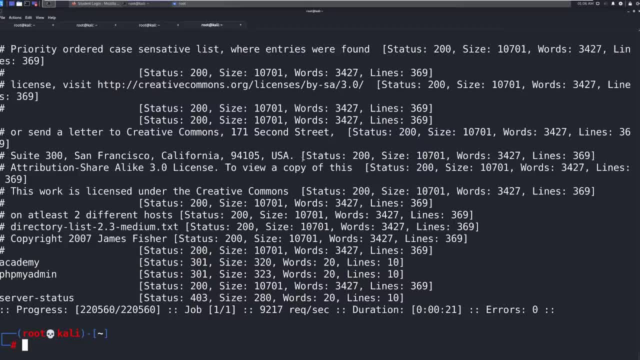 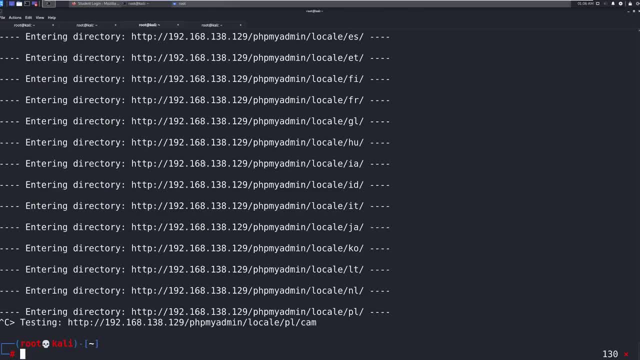 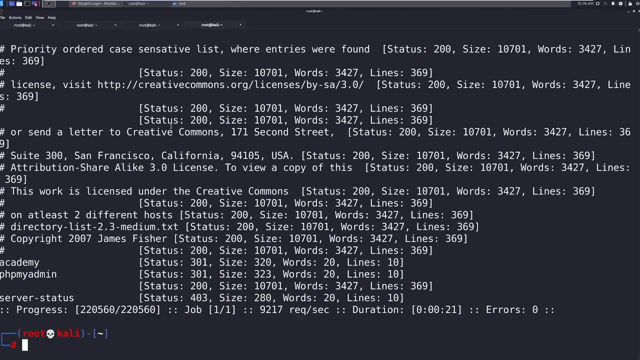 redirect there. Same with the PHP, my admin, All right. So with that in mind, this is how you can find it. Found it quick. This one's still going. There's different strategies, different tools, everything else. This one's pretty nice. There's a lot of tools that come out for directory busting all the time. 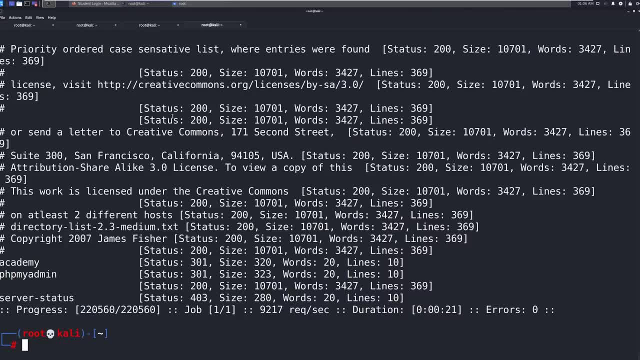 Latest ones are being built in rust, which is interesting because rust is really fast. There's ones built in go because go is really fast. So you pick your poison on a directory busting tool and you just run with it. So, anyway, we're going to go ahead and enter in that registration number. 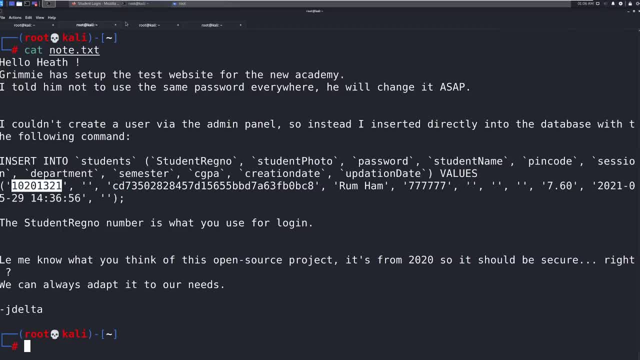 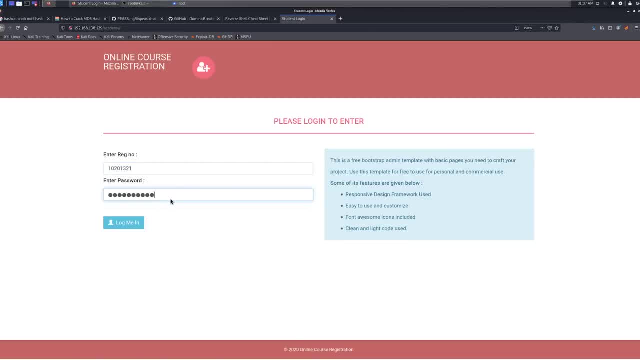 So you can go ahead and just come copy it from here, And then you're going to go ahead and paste that And then the password is student For me. I've changed the password in here because I've already gone through this box, but you'll be brought to a change. 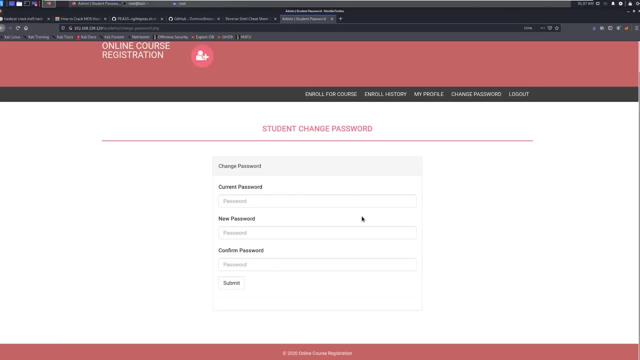 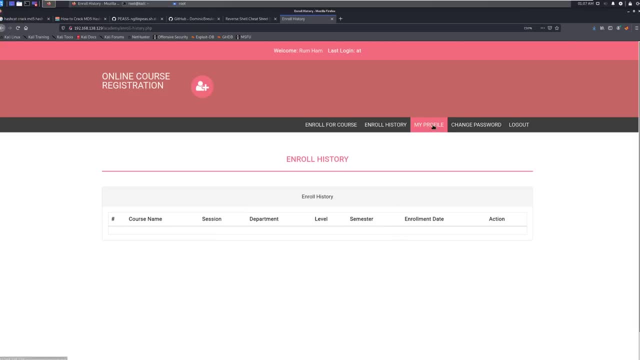 password screen So you could type in student, change it. If you want to- you really don't have to- you can come in here and start clicking through: Hey, I want to enroll in a course, enroll history, my profile, change password, et cetera. Um, so this is really what we have. Now the interesting thing is that you can go ahead and type in student and then you can go ahead and enter this code to join the course And then you're going to find that change password or ID that you've sent in. you can type in that in here and that'll show up, And then, when you open, 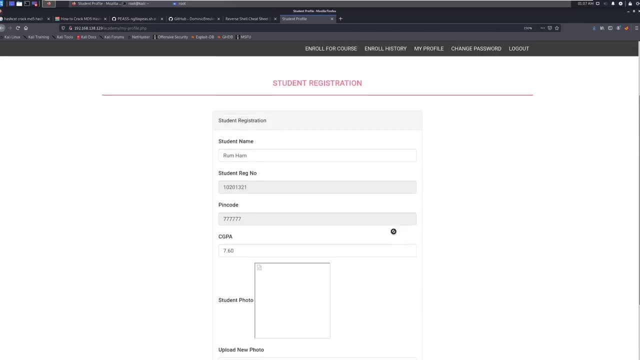 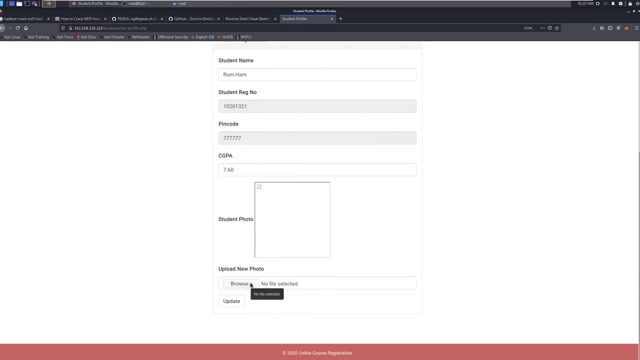 the next page you can see in here. So the interesting thing in here is that we have this um upload photo feature. So if we look at this, we can come in here and say, okay, how do we want to attack a website? What are some ways that we can get code execution? 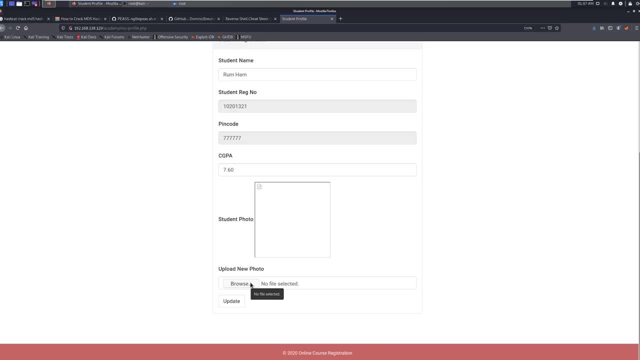 Um, we might be able to perform like LFI, RFI attacks on this and pull down information or execute code. Maybe there's SQL injection somewhere in here, or we can pull down and dump the database. We did see a PHP, my admin. Maybe there's more behind this, behind the 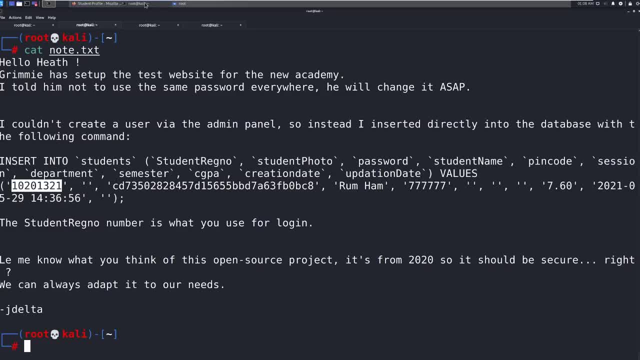 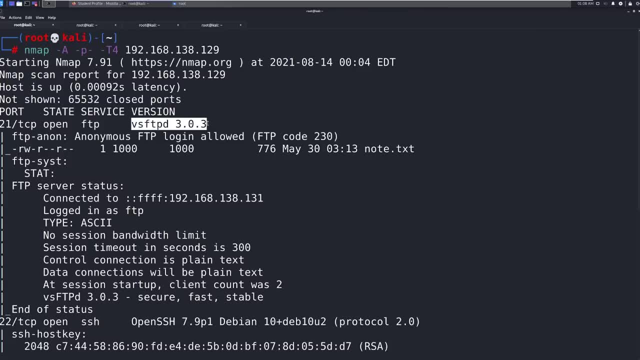 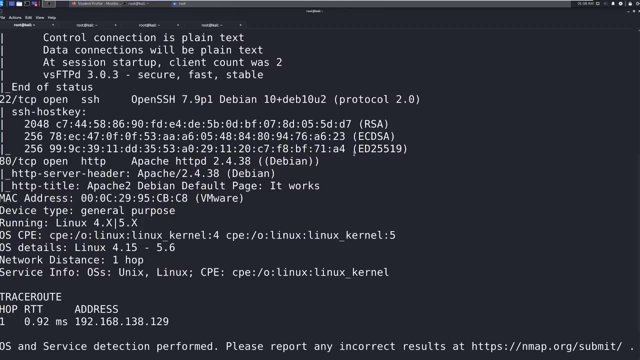 scenes that we can do. we can also go out, and something that we didn't really look at on the first scan is we can do a version check- like we didn't check on this version- to see if there's a vulnerability there. that would be something you can do. same with the open sh, same with the apache. you can go and do those. i'm only 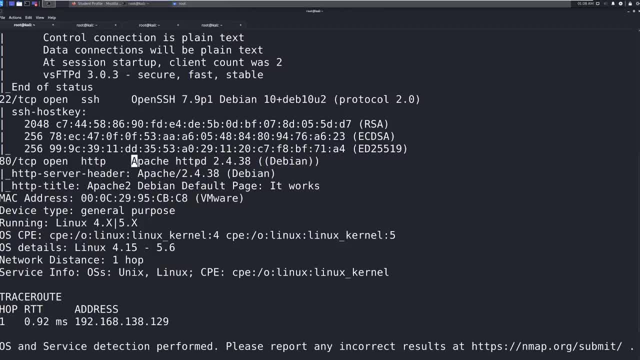 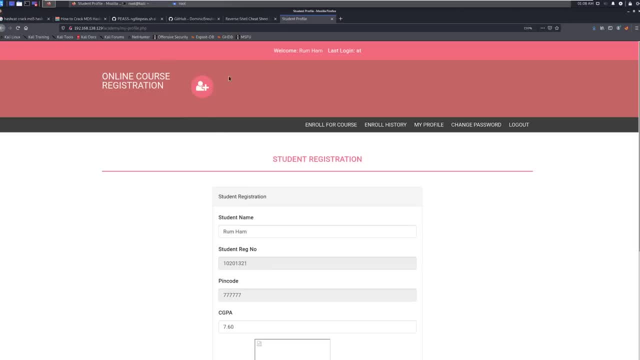 not showing you that because i'm saving time here, but the correct methodology would definitely be to go check these as well to see if there's any vulnerabilities. now there is in here a uh, this is a online registration. you can look and see if there's any way to pull down, like viewing the 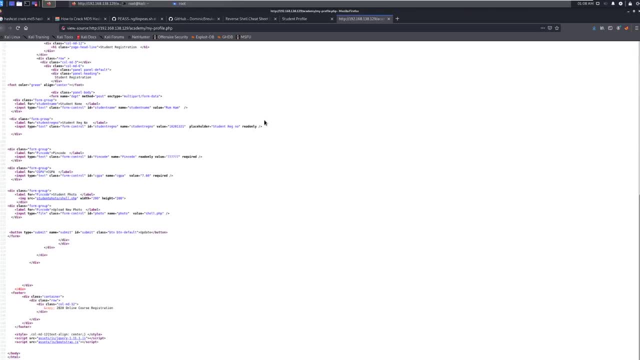 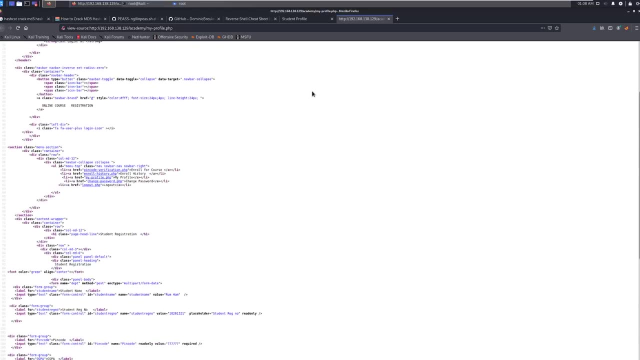 source and see if maybe anything in here would tell you, hey, what cms is this, what is this built off of? because clearly this is a cms of some sort that they've used. now, with that in mind, we can go back and we can kind of just look and see if we can find anything. the first thing we might want 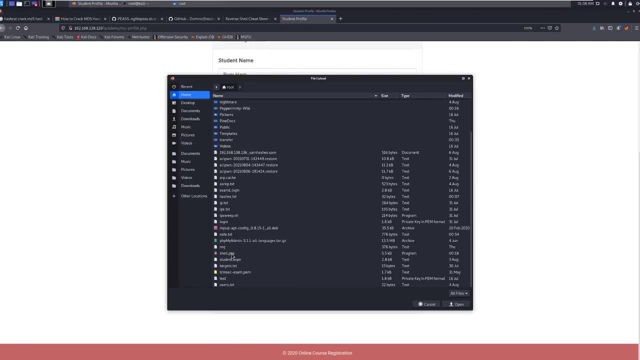 to do is just come in here and do a browse and come and say, okay, i'm going to upload. uh, let me go to my my desktop. i'm going to upload a picture of a dog. you can see that it's the same as the version that we did in the earlier version of the apache. 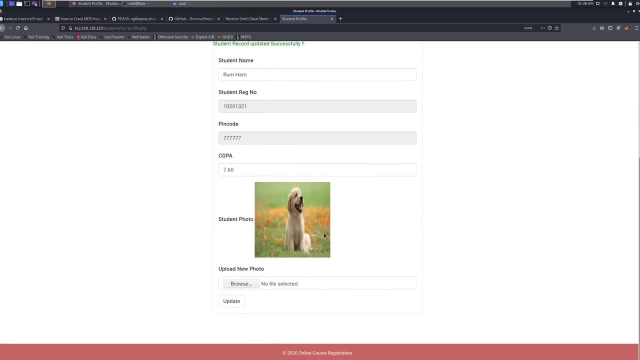 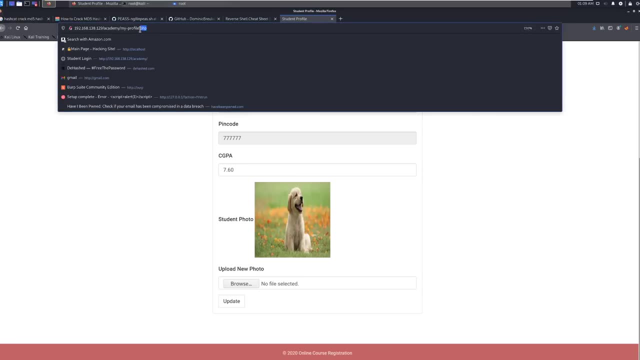 don't have to do this, i just want to see if it works, okay. so i uploaded a picture of a dog, perfect. now the question here is- and, by the way, we can see up here that php is in use. i'm gonna make this a little bit bigger, by the way, but php is in use, such as, say, my dash profilephp. 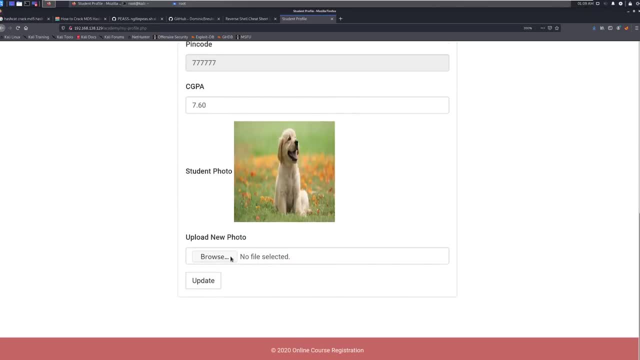 um, what we want to do is we want to see if we can upload a file that is not not- not a dog, okay, like not a jpeg, not a gif, not a, not whatever png. we want to see if we can upload something that's not a photo and abuse the file upload system if they're doing no checks here. 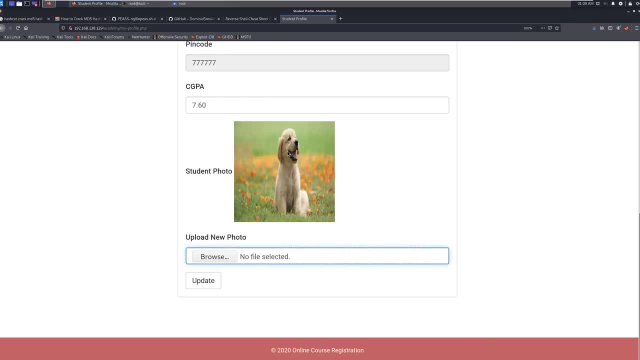 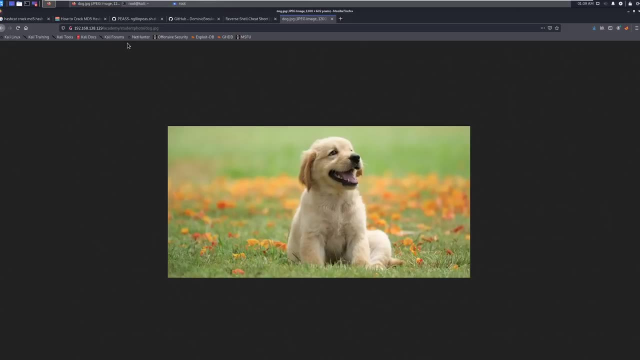 and we can just upload this. they are in big trouble. so what we can do is we can right click and go um, we can view image which will tell us kind of where the the image is stored. so it's stored in academy student photo forward slash and this is dogjpg. 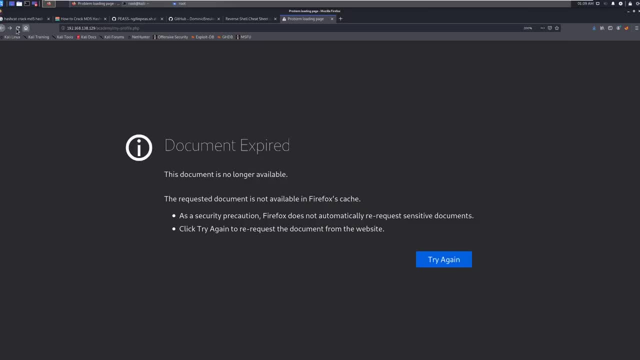 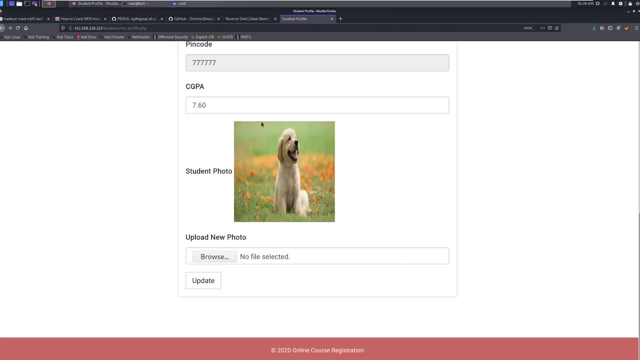 jpg, which is what i uploaded. so what we can do- let me refresh this- what we can do is try to upload a reverse shell here and see if we can't get a connection back by viewing this. let's see if we can upload something malicious. now we know this is apache, so we're going to upload via php. 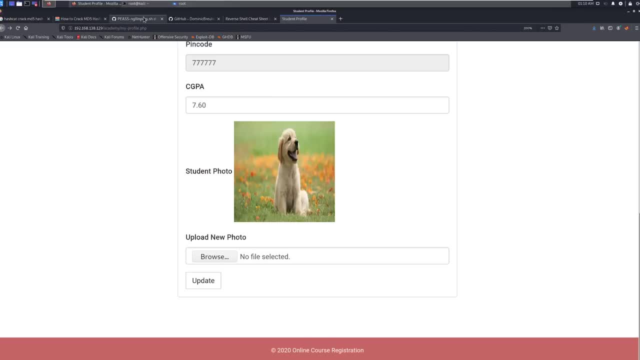 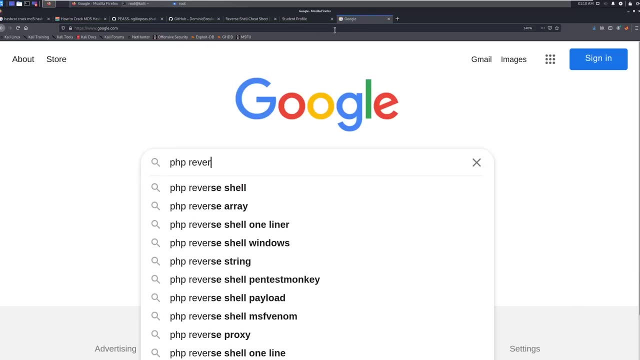 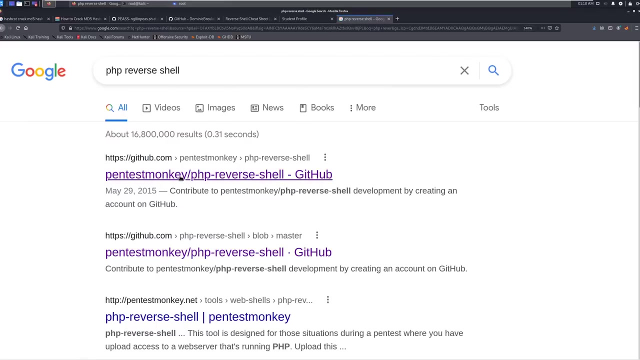 so i'm going to go ahead and do that. what i want to do is go out and we're going to do a quick search. we're going to go to google and we're going to say php, reverse shell, and there is a great one out there from pen test monkey. okay, first hit should be up here. there's. 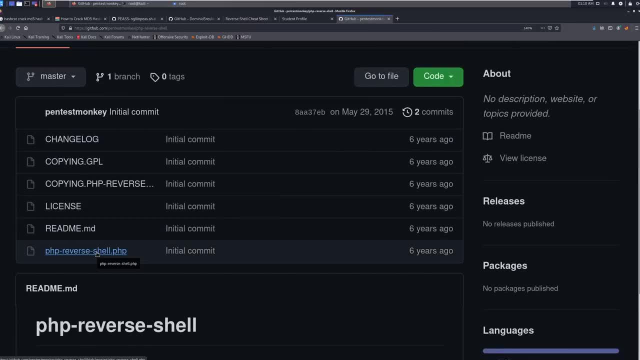 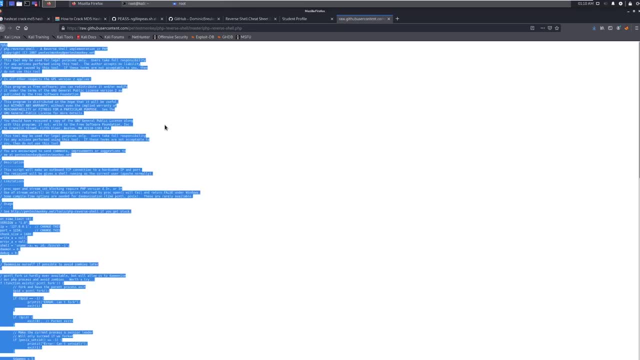 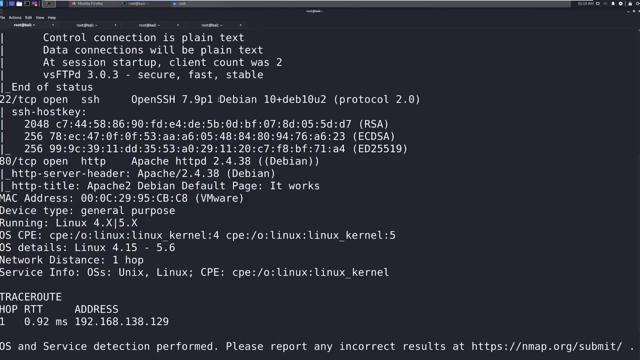 other ones that you can use. people have their preferences and their favorites. this one is six years old and still works perfectly, so all we're going to do is go raw here and copy this control a, control c- very quick, and what i did was i went ahead and put this into a um a file here. so let's. 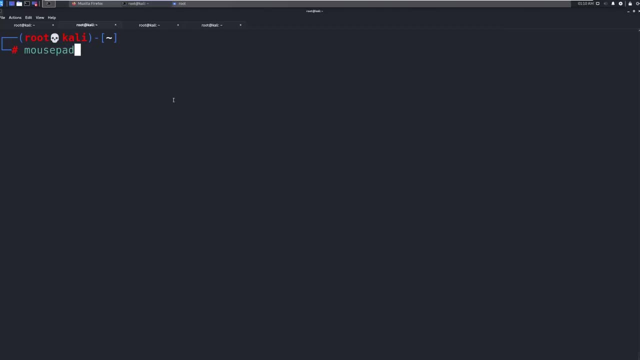 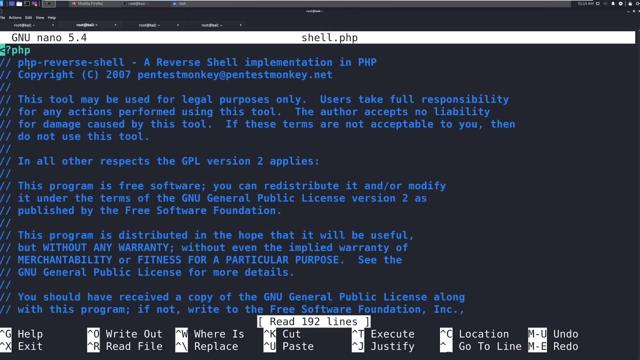 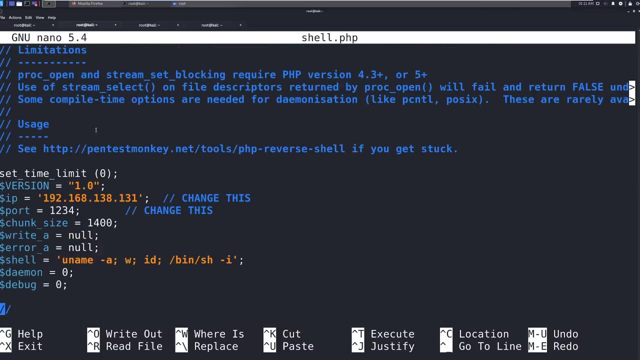 go here and copy this, and so what we're going to do is go embedded here and copy this. make that documents to a new file, and this is where it's going to be the format. what we're going to do is we're going to select a file and i'm going to fill the variable and paste it to the file in the 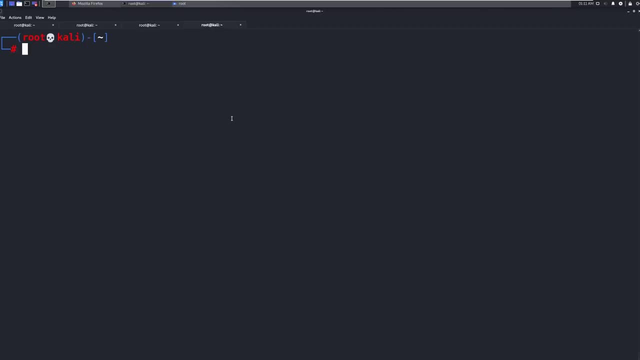 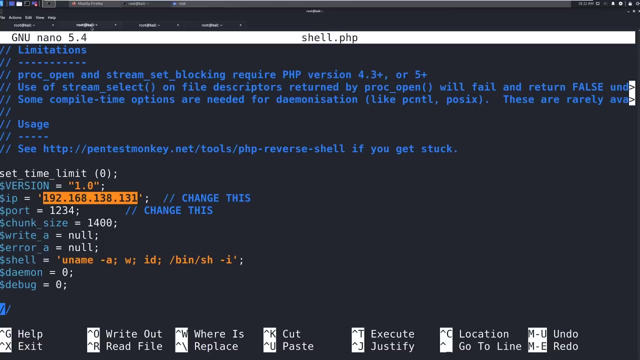 needs to go here. So if you need to open up a new tab, come in here, do IPA, or if config 192, 168, 138, 131.. Come back. that matches what I've got. 1234,, in my opinion, is fine, you can. 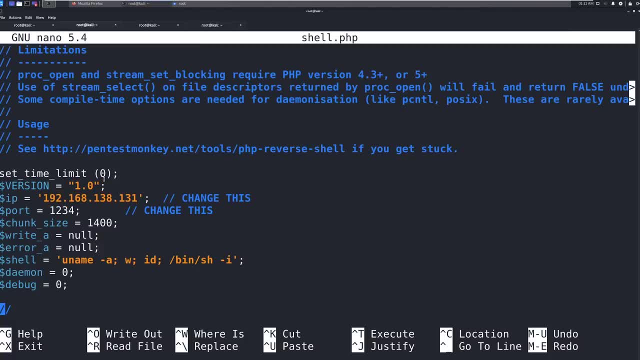 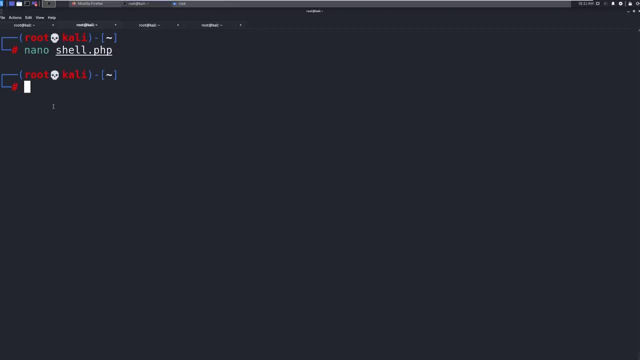 leave it as is for this machine. So Ctrl X. This is fine. You can hit Yes, save. if it asks you to just hit Y and enter, And that will save your shellphp. So we have shellphp. we need a listener. we're going to do a reverse shell here, So 1234 on. 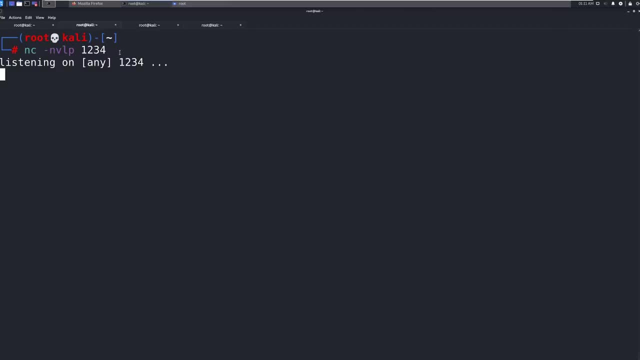 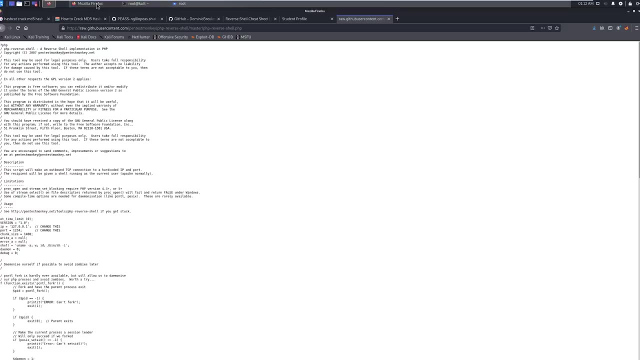 the NBLP on netcat. This should not be unfamiliar to you. should already be aware of this. So we're gonna go here. And now we've got this listening, we're waiting for something to happen, So we're gonna go back into this and we're going to upload. 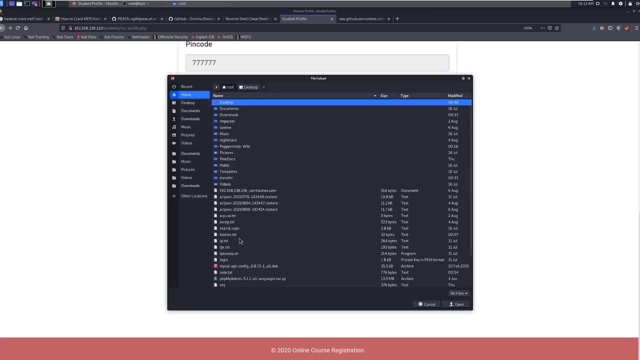 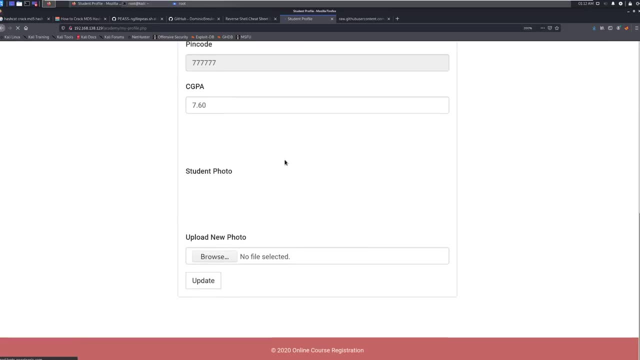 this malicious file. So I put this in my root folder: shellphp- click update. come in here. you can see nothing's happened. Let's see if it tries to execute already executed. So we don't even have to go to like we don't have to right click and go to that. that. 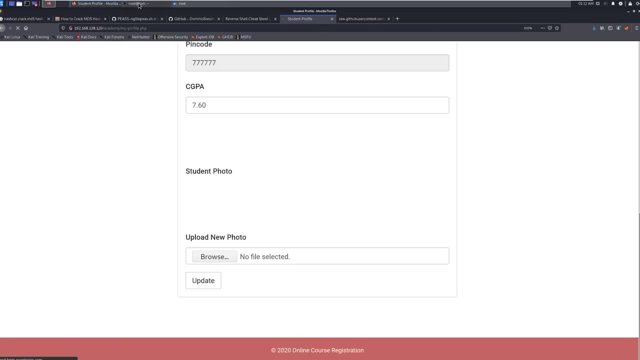 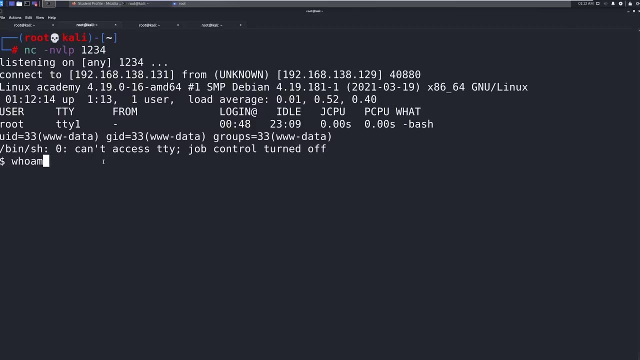 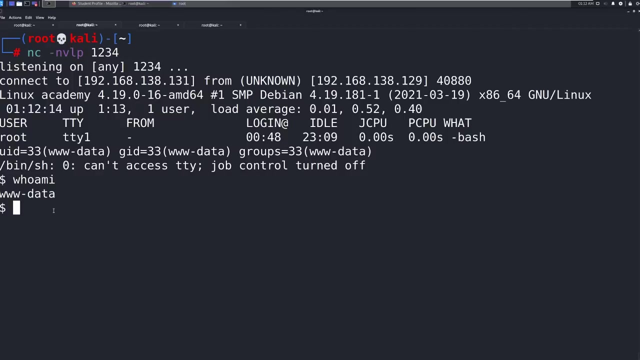 location. it already executed that file when it loaded this page, which is crazy. So we have a. we have a shell here, which is great. So if we do a, Who am I? you can see: we are the WWW dash data user. So we are not. we are not an admin. We are an admin. 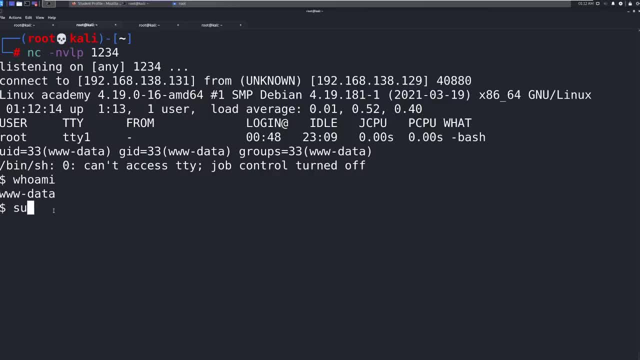 on this machine. We are not root. we can do a pseudo, dash L- But they rudely took away pseudo. we could type in which pseudo and see if it's there: locate pseudo. maybe they put it somewhere else. Locate- not found either. So they're playing a. 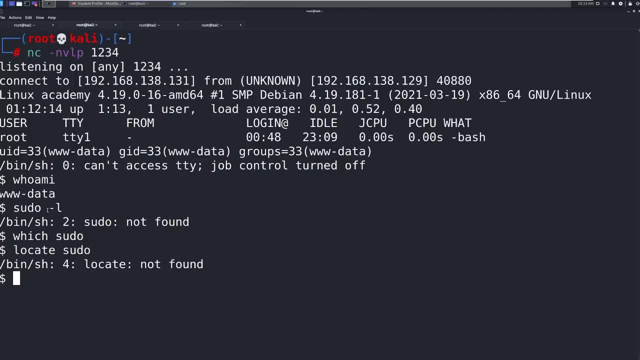 little bit of games with us, just a little bit, because we should be able to run and see, hey, what privileges do we have? a pseudo, but it's not there. That's okay, though. we still, we're still going to be fine. 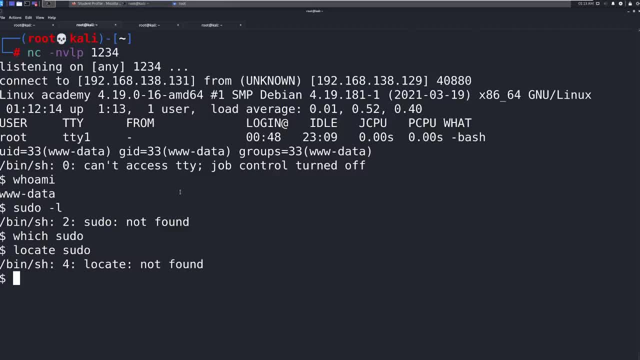 So what I want to do next is: we land on a machine. we're not a root user. we need to perform privilege escalation. this is where things get fun And this is where we're going to take a bunch of winding roads to. 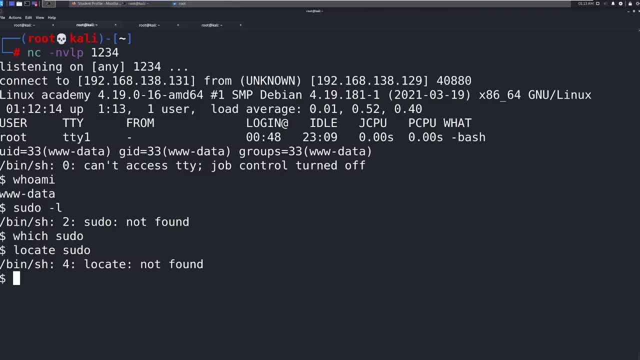 get to where we're getting. So what we're going to do now is we're going to use a tool called Lynn peas And we're going to utilize that to do some searching. Lynn peas is a automated tool that goes out and does basically hunting for any 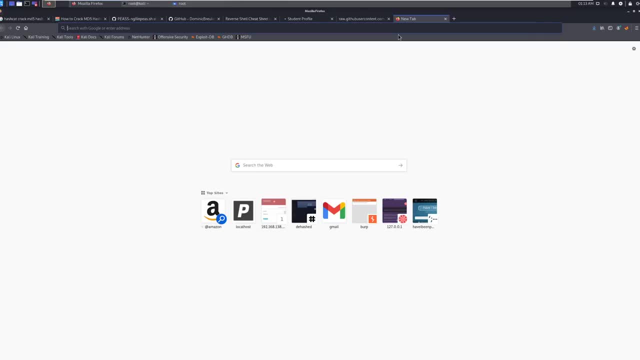 sort of privilege escalation And I kind of cheated a little bit. let me go to Google and just type in literally l i n like Linux, p e a s like the food peas. Hit Enter, you'll see it here in GitHub And you see a. 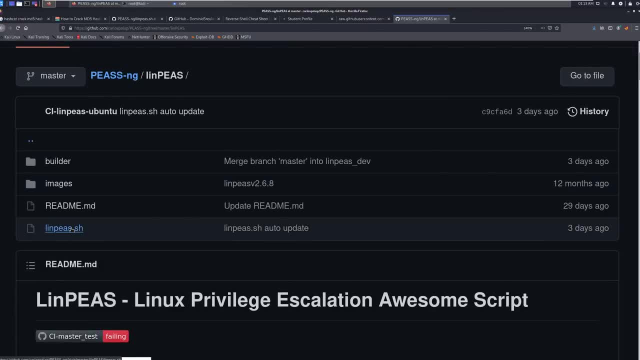 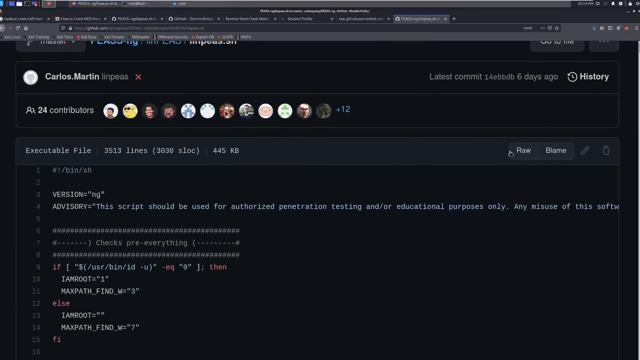 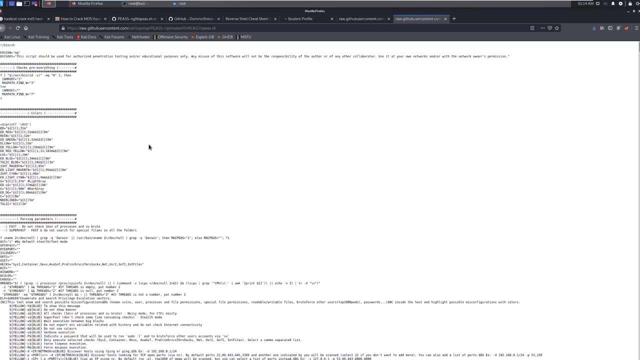 Lynn peassh. updated three days ago: Nice, All right, And this is going to go through and perform all kinds of checks to see if there are any escalation privileges or privilege escalation or paths for us with privilege escalation, what I should say, So you can go in here and you can see that we're 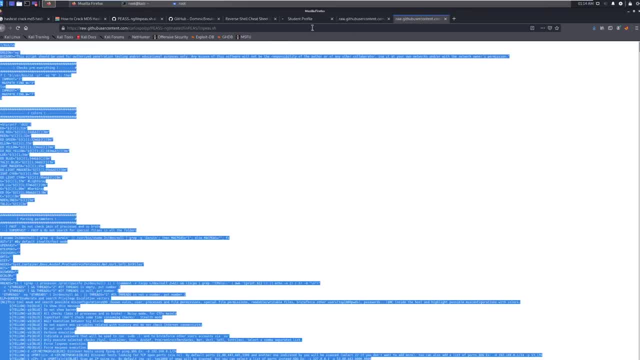 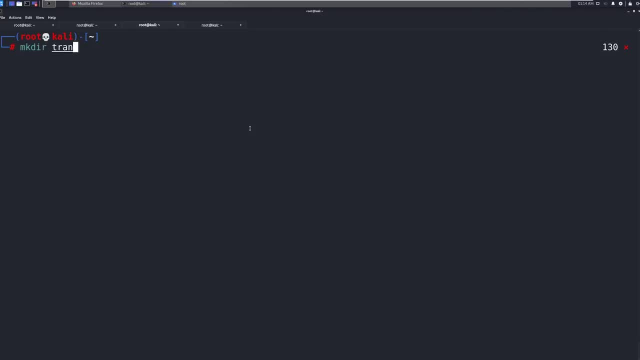 going to have a couple of different functions So we can go in here again: raw control, a control C, And what I like to do- and this is how I actually operate- is I like to make dirt on a transfers folder. I call it transfers And I've already got. 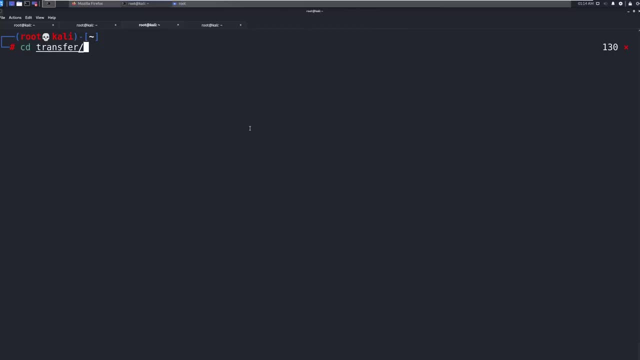 one, So I'm just going to CD into transfers- Or transfer is fine as well. LS in here and Lynn peas sh is already in here, So you can nano limpies sh- Same thing. Just go ahead and get it into this folder. 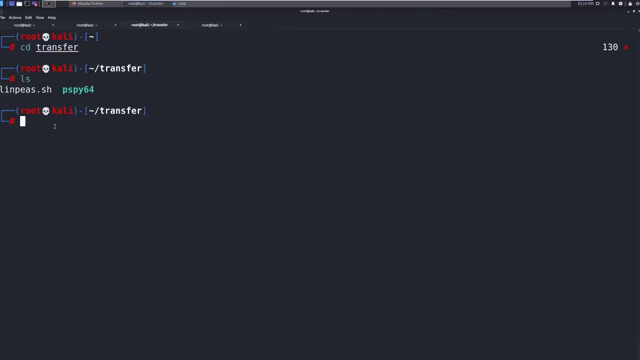 make sure you copy paste it, put it into a file and have it ready to roll. So what we're going to do is we're going to host up a web server. So we're going to say Python three, dash m for module And we're going to type in HTTP, dash, server 80.. 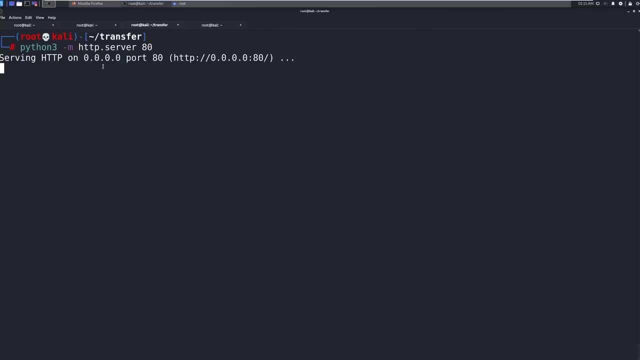 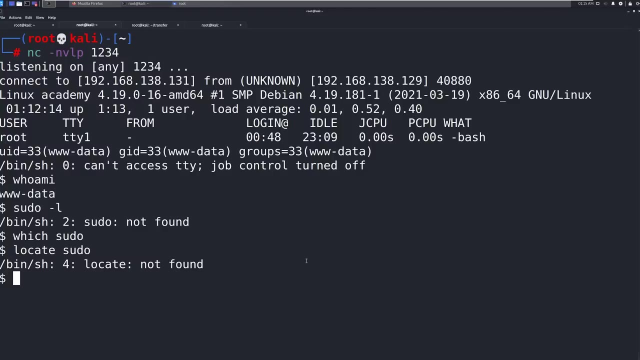 Okay, and this is going to host up a web server In this folder. we're going to go and grab this file on this machine. So a good place to put a file that we want to. we want to dump on this machine, So we're going to go and grab this file on this. 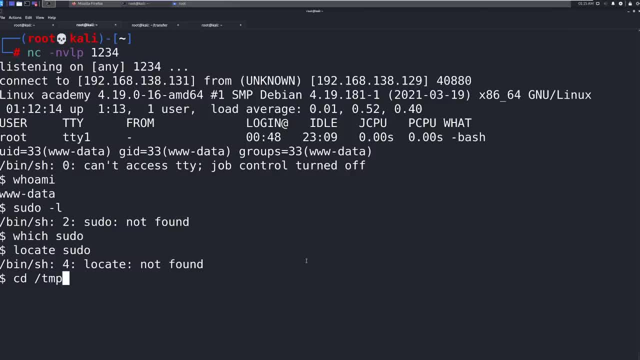 machine is. we're just going to put it right into the temp folder, So CD, into temp Print working directory. We're in forward slash tmp, Okay. so what we're going to do now is we're going to do a w get HTTP your attacker machine IP. So I'm at. 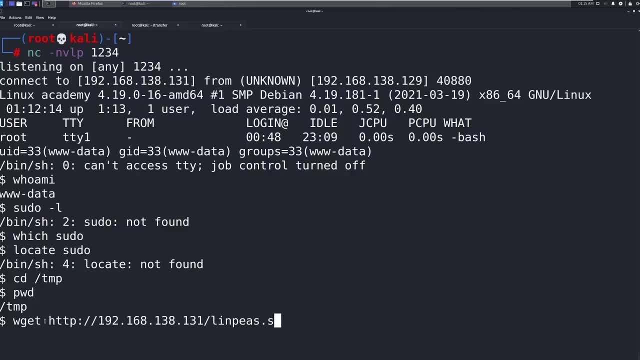 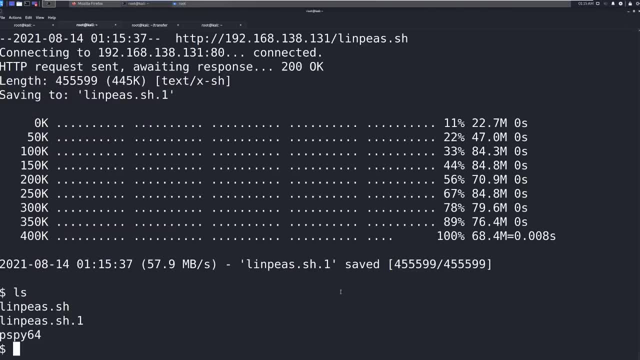 131 forward. slash Lynn peas: sh. hit Enter. It should copy over. you could see it coming through. Do a quick LS. I already had Lynn peas on here because I was running through this box earlier, but I'm going to use the original, in peace. So. 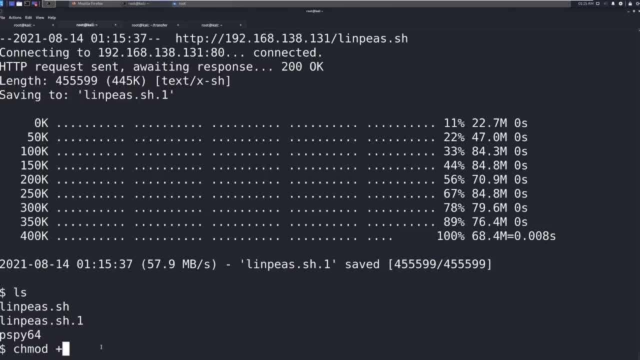 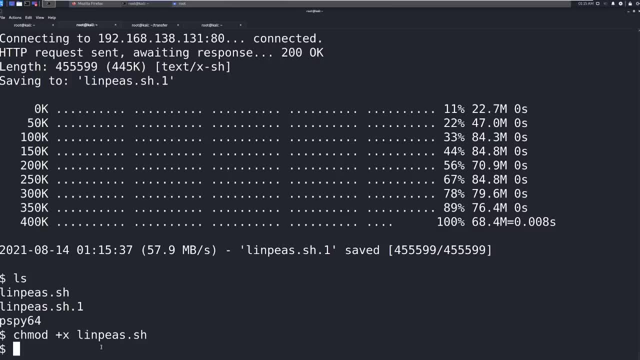 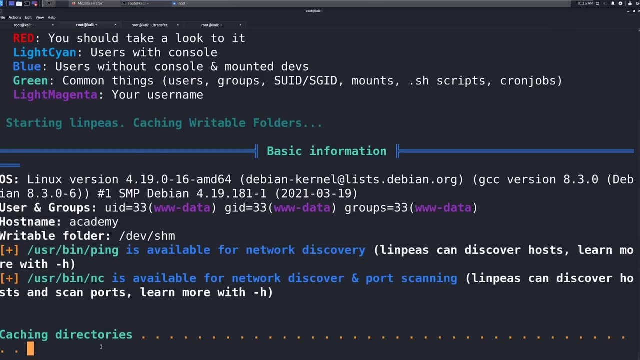 pretend with me. we need to make it executable: ch mod plus x or change mode: Lynn peas sh. Okay, Now we're going to run it dot forward: slash Lynn peas sh, just like that. Hit Enter, It's going to start just flying across the screen. 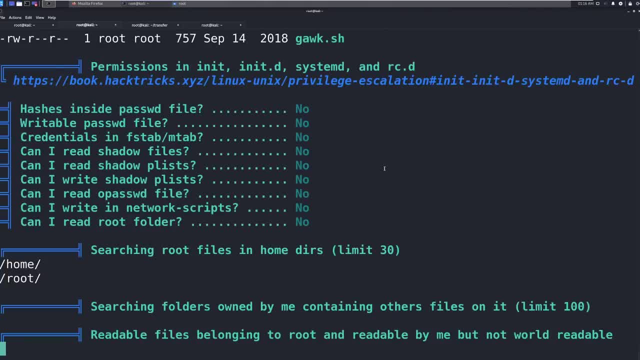 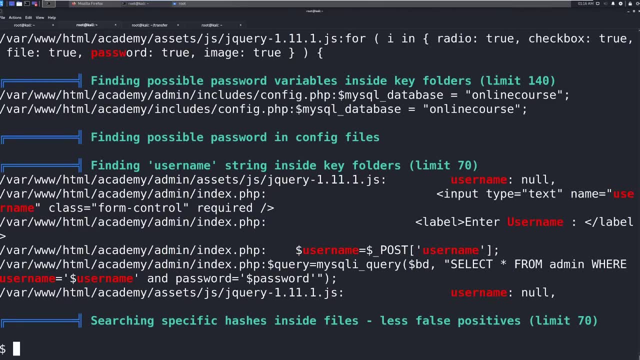 it might take a minute to go through. We're going to go through some of this, But I'm going to give you the general gist of what you're looking for and the things that you want to look for in here. So I'm going to take this and scroll back up to the 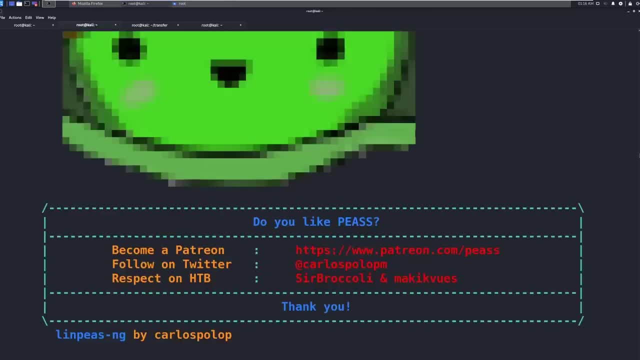 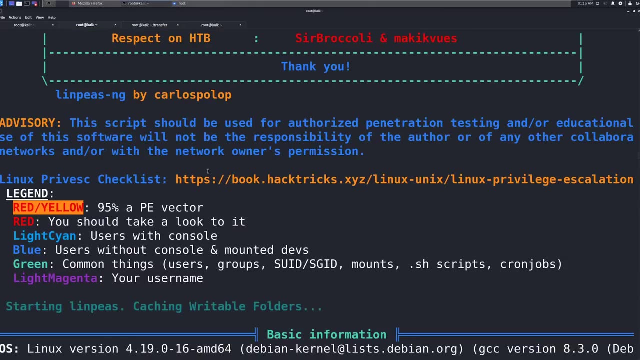 top. If yours isn't done running yet, that's fine. I kind of just want you to watch anyway on this one. So we run it, we get a nice little Ninja Turtle- cute- And you go through and it tells you the legend on here, Okay. And it says: Hey, red, yellow means 95%. 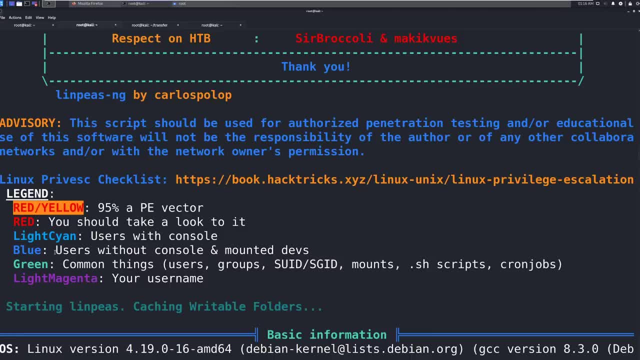 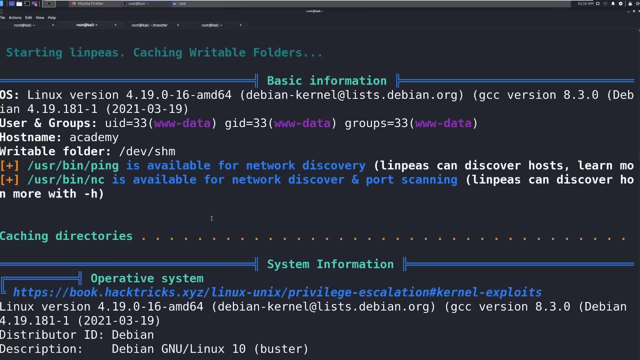 could be a privilege escalation vector, red. you should look into it And then it gives you different ones. So really we're looking for red And we're just trying to see if we can find anything in here that could be of interest for us Now as we're scrolling through. 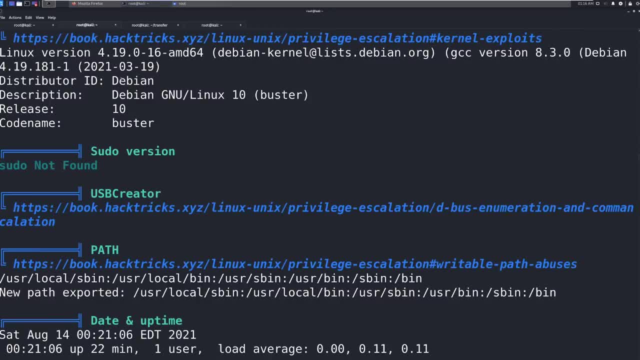 it gives us information about the, you know, the Linux distribution, the release, all that that could be useful If we have some sort of escalation against this. there are different types of escalation that we could use And the release information could be important to us, though it is not for this. 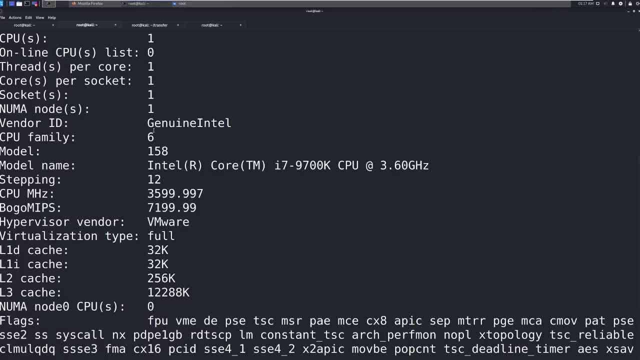 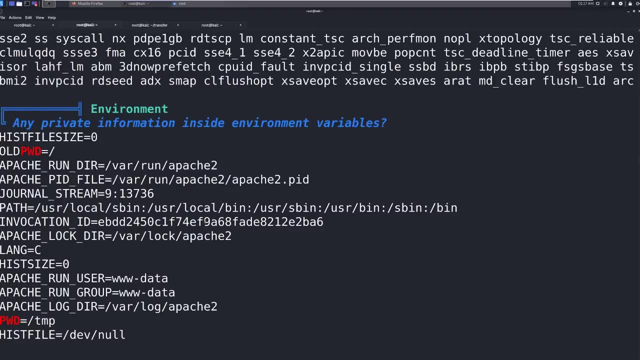 machine, So we're going to skip over it for now. Now you go through, it tells you all kinds of stuff about the all the operating system, what's running on it, and it's looking for anything that could be of interest. Now it's telling you: hey, what do? 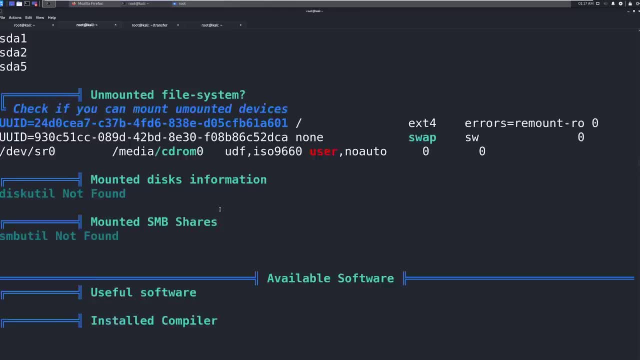 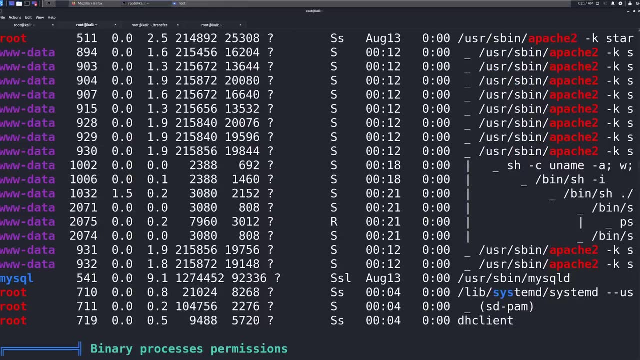 we have that we can run. This just says yes, this is a virtual machine. Keep going through, keep going through. This is looking at cron jobs, which we'll talk about in a little bit. This is looking for any sort of system, D timers or cron jobs. We have no cron jobs running. 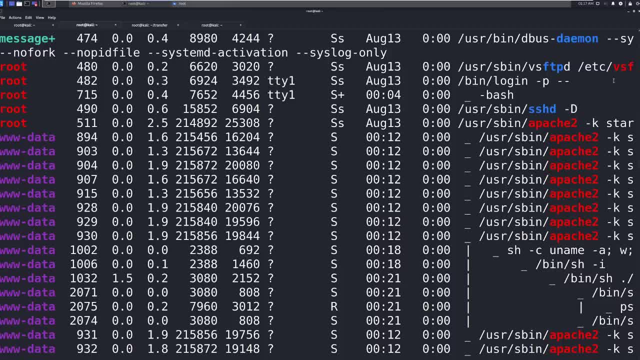 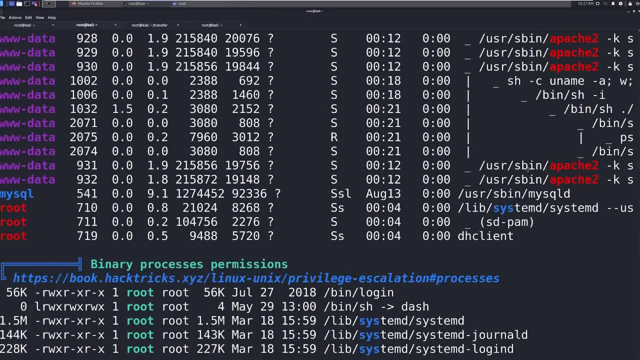 that look relevant to us. This is just running Apache two, This is running a and this actually looks like it could just be the processes running, not even the cron jobs. So these are just the processes running, Nothing of interest to us right now. 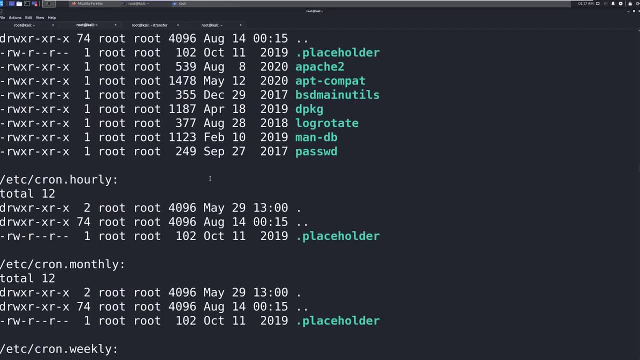 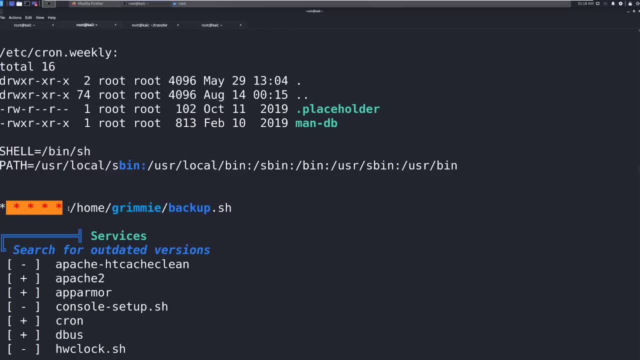 Scrolling through here. we're just going to look and see if we find anything of interest. Now there is a highlighted red and yellow here with home grimy, backupsh. We're going to copy that bad boy, see what, what it is. And then from here you're going to go ahead and just keep. 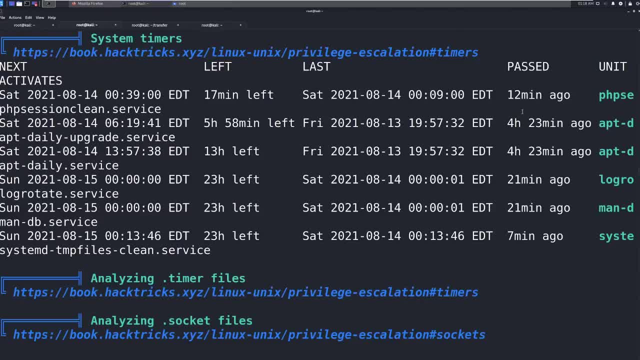 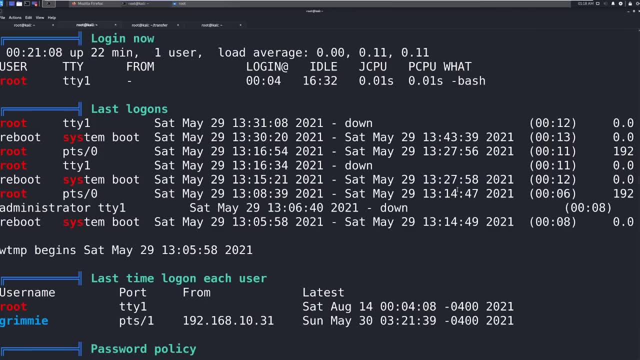 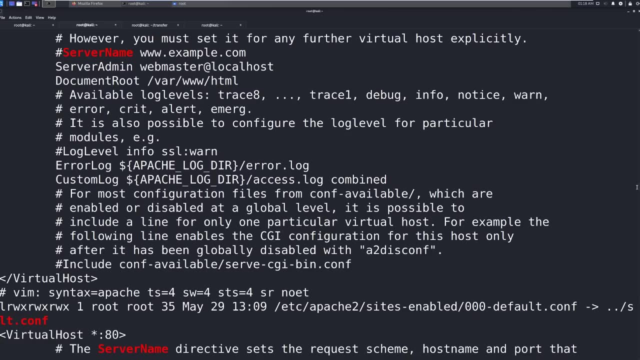 scrolling, So we come through, keep scrolling, keep scrolling, And a lot of this is just information that is provided with us. what is of interest and for this machine? Now, you're welcome to read through this. There's a lot of data to read through. I. 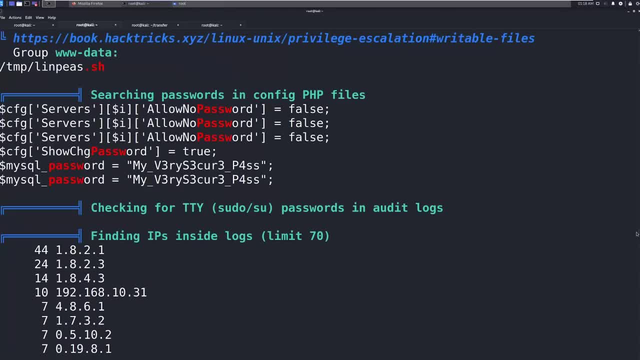 like to scroll through kind of really quick and just see if anything stands out, not at this pace, But like right here. look, we're scrolling through and we see, Hey, there is a MySQL password of my very secure pass That is of interest to us. It looks for passwords And we're going to. 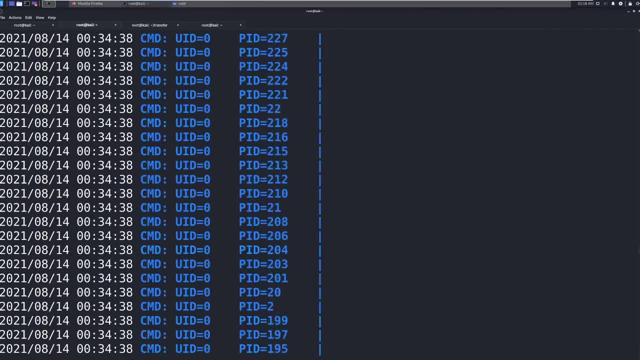 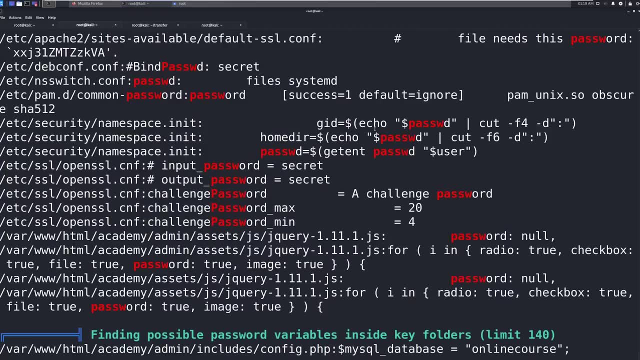 scroll down to the bottom, I'll show you kind of what it looks like. So if we scroll all the way down, we start scrolling up a little bit, you'll see that the my very secure pass shows up again. it shows up right here And it tells you: hey, this is in. 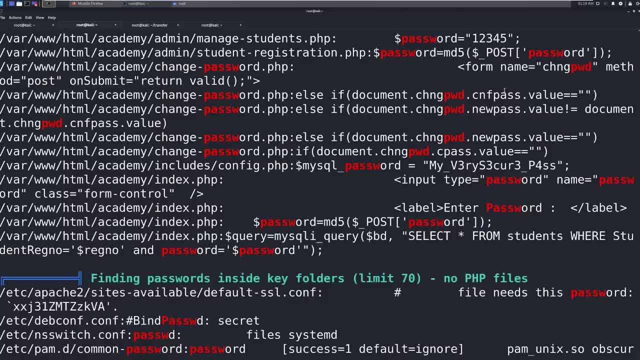 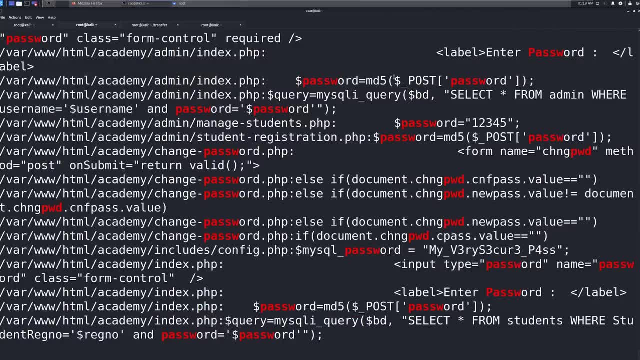 this includes config dot PHP file. So that's really what we're looking for. We've got a password up here: manage students at 12345.. So we can go look at that if we wanted to, And some things in here that we want to. 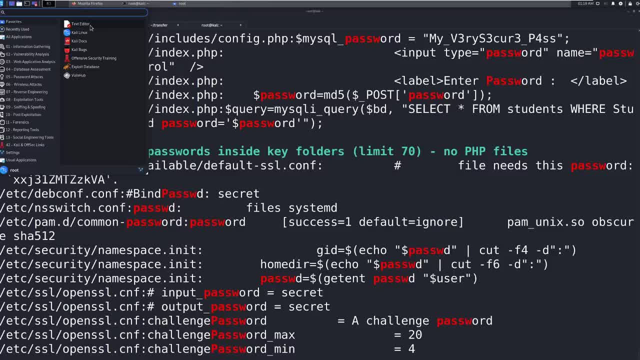 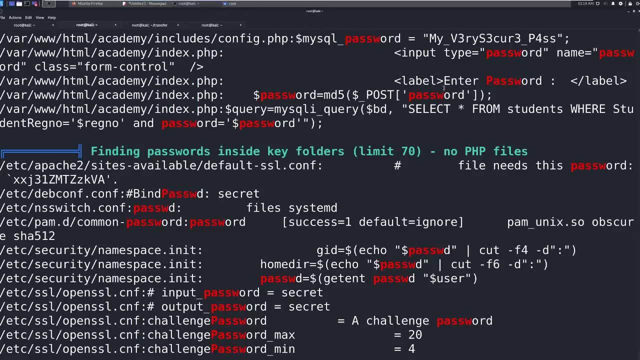 make note of. So maybe we open up a notepad Like we come into, we come into a text editor, we just do a paste here, because the Grammys of interest, we found the password, my very secure pass, which maybe we want to just copy this whole thing out. 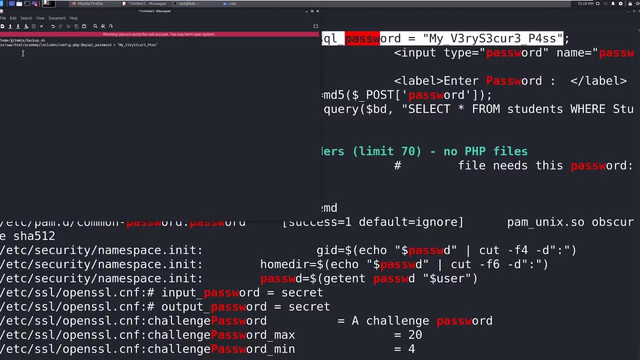 Okay, and I might put that into my little, my little notes as well, And maybe I want to read this, this document, and see what's in here as well. So this is of interest. we want to go through and just see anything of. 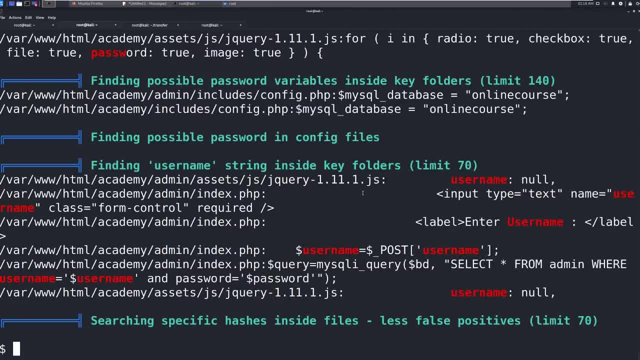 interest. Now I am skipping ahead just a little bit only because to save time for the video. there will be other opportunities to learn privilege escalation, And again we have the privilege escalation course. if you want to go through this in more detail, This is again just trying to get your feet. 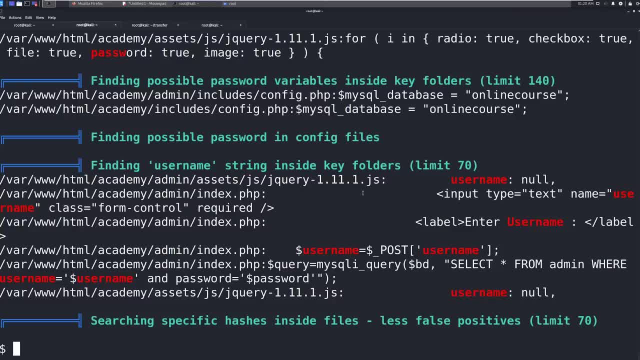 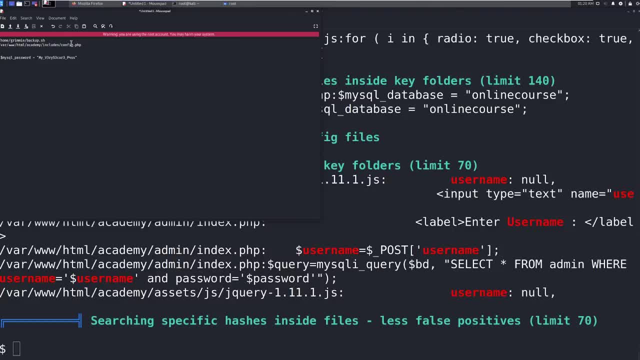 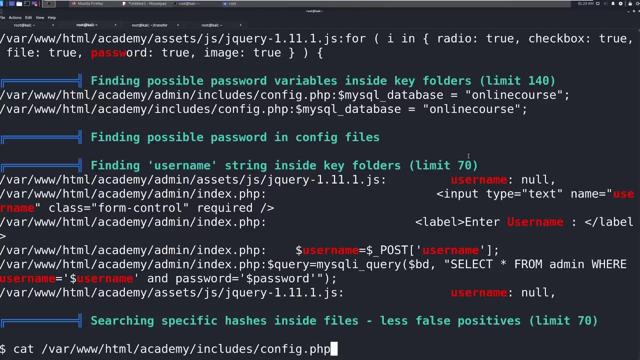 wet introduced to the idea and understanding what we're doing here. So now let's go ahead and let's look at the file that we just found first. We'll wait on the Grammy file. Let's go ahead and just cap this out. Okay, so if we cat out this, 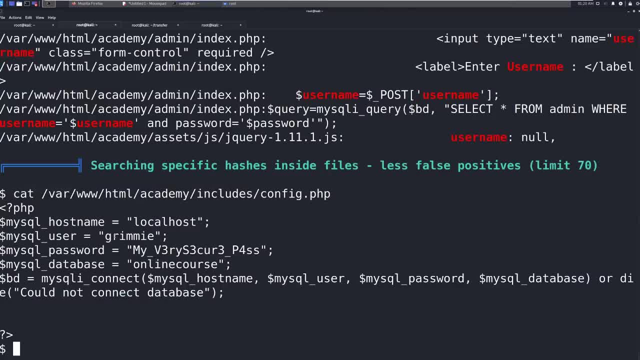 config that PHP. we see that we get a SQL user of Grammy. we get my very secure pass. Okay, we get some information there, So we can maybe try to see if the this works for us anywhere. It's a SQL user database, maybe we. 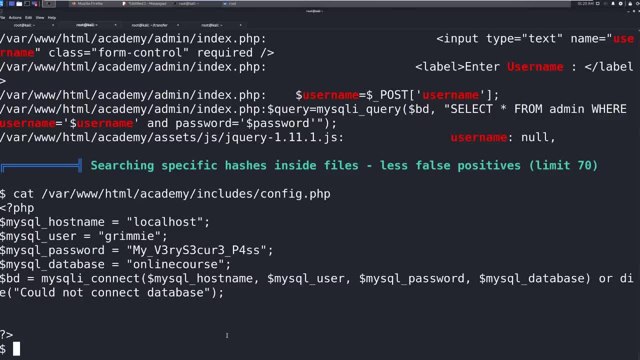 can get into the SQL database and find some information. That is one option, though I did not see any sort of information for SQL unless we could log into PHP my admin with this on that web panel that we're looking for. So that's something that. 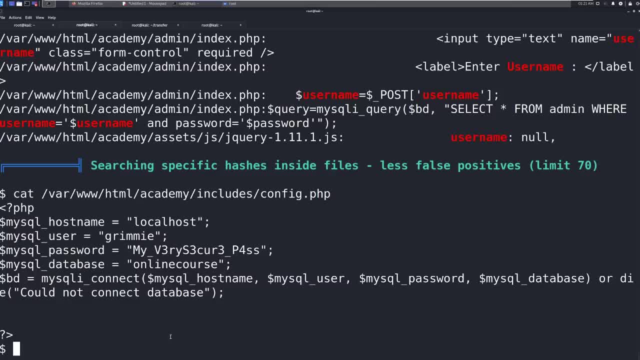 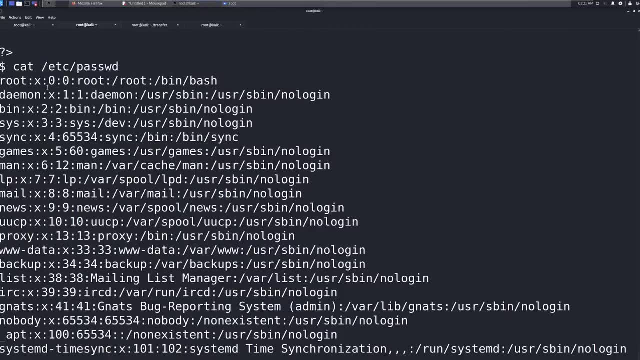 could work. We also want to see if there's anything. maybe we go cat Etsy password see if that works for us. Okay, so Etsy password is showing us all the users on the machine I've interests. we'd like to scroll down to the bottom and we 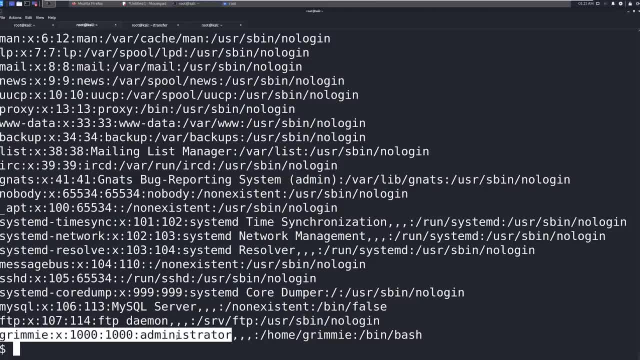 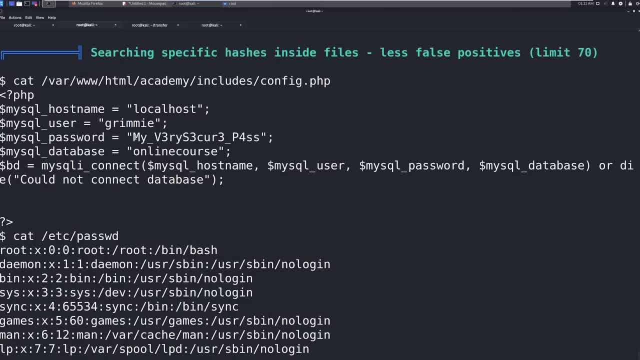 see a user of Grammy And it says Grammy is an administrator, which is interesting. So it's pointing to Grammy being a user on this machine. So it doesn't hurt to just copy this password and see what we can do with Grammy, So what we can do here. 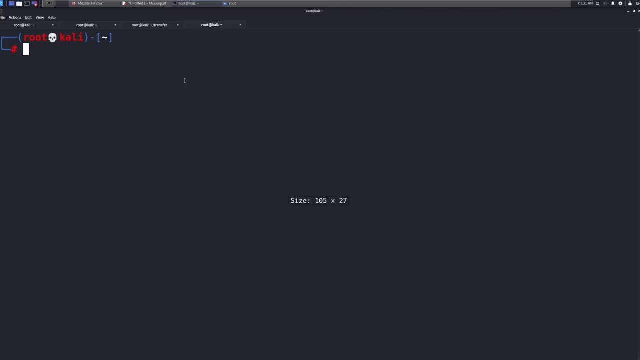 is. I'm going to go ahead and just go to a new tab And I'm going to cat. and, by the way, we should have known that anyway, because there was a folder called home Grammy, backup sh or home Grammy. So Grammy would have been an indicator anyway that. 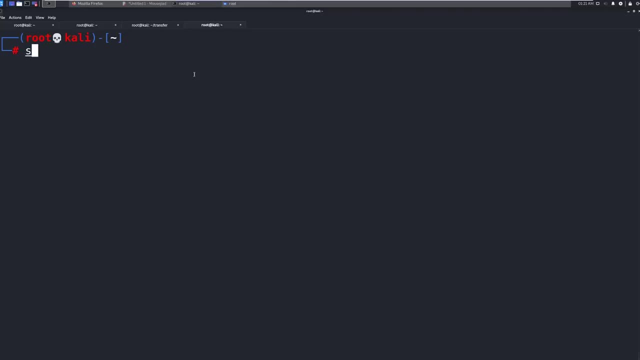 that we were up against a username, Grammy. So we do SSH, we can do Grammy at, and this machine is 192 168, 138, 129.. For me, go ahead and hit enter once you got it in there, And it should ask you your first time about a fingerprint. just type. 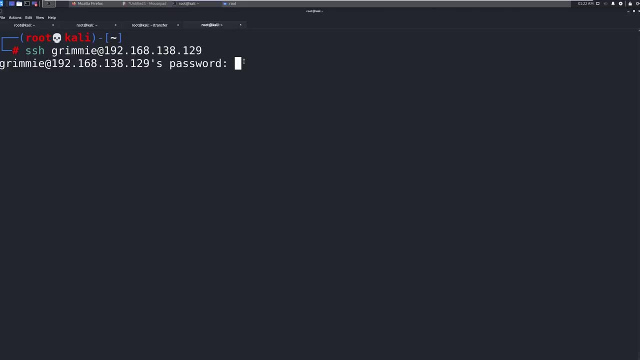 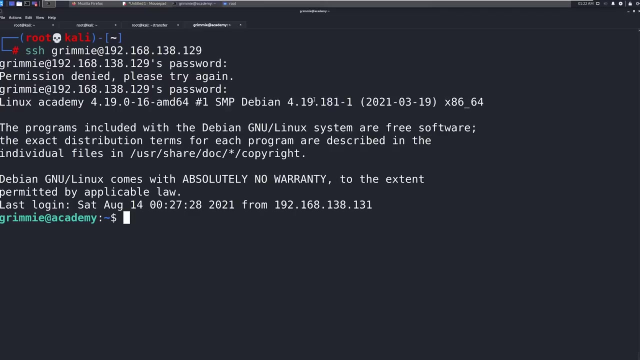 in Yes, hit enter And then go ahead, and you can see that it's in that password that we just got, And maybe I copied it wrong, So I'm gonna go copy that one more time. Okay, and here we go. So now we are in this machine, We don't. 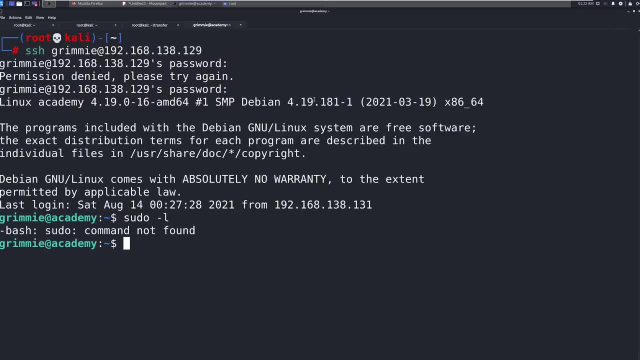 have sudo access. I don't believe sudo dash l. again it says sudo not found. it could be that we have a broken version of bash or they intentionally removed it because it's just C2.. Yeah, that's one of the first checks I do. History is another. 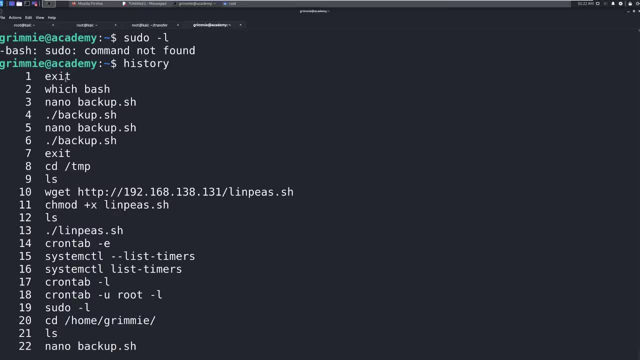 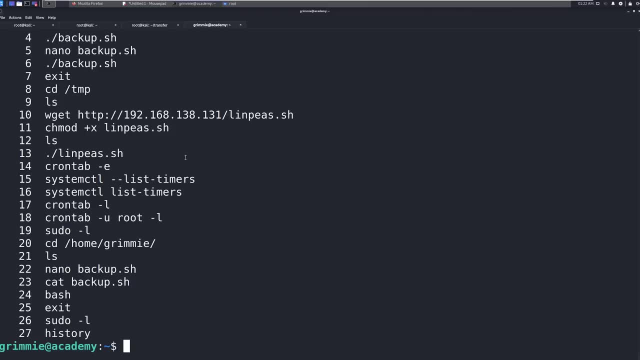 check, though, I have some history in here from myself, So you might not have any history when you come in here. This is just all me doing this. Now, one thing that I do again is I like to come in and I like to download Lin peas. run it again. 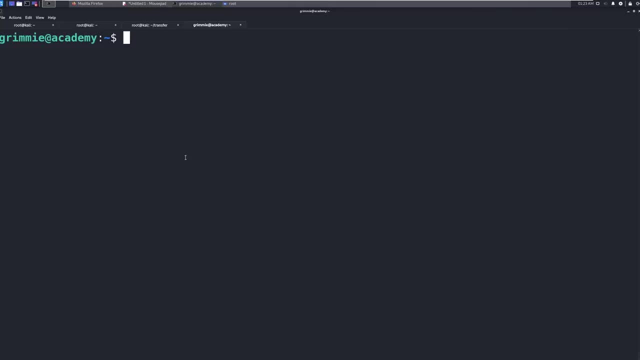 see if anything's changed. I'm going to skip over that process, But I'm just telling you for the process, what we want to do is we want to make sure we look at the file that's of interest. Okay, so that file when we went and saw was in the home- grimy. 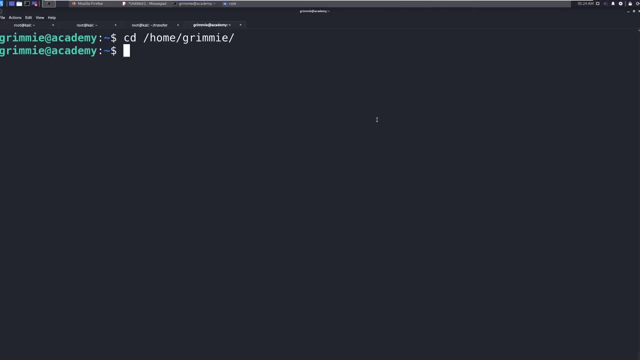 folders. let's just go ahead and cd the home Grammy, And we're gonna LS in here and all we have is backupsh. So let's run cat backupsh. So what we have is looks like it's removing a temp backup file. it dot zip. it's zipping up a backup, dot zip. 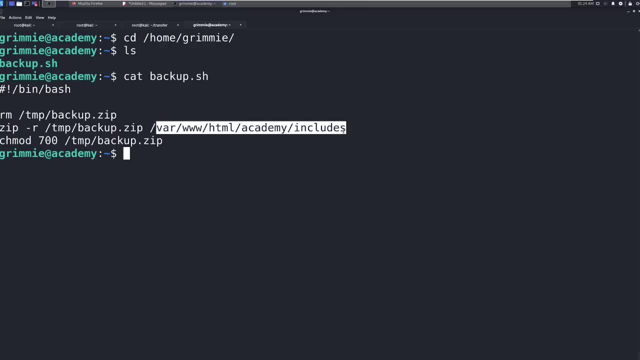 from this HTML Academy includes. So it looks like it's doing a backup of the Academy And then it's changing the permissions of the temp file. So if we look at temp, there may or may not be a backup zip sitting in there. So what this is telling me is this is probably going out there and doing 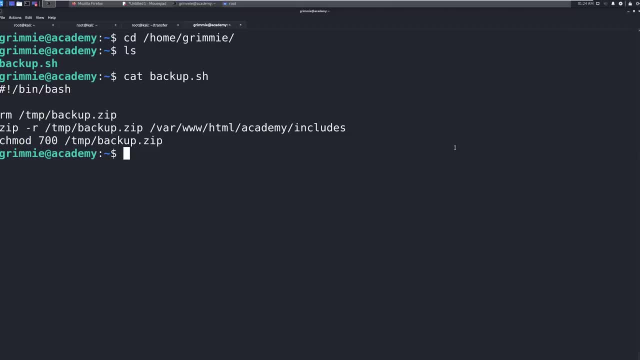 periodic checks or a script is running periodically to see if or to perform this backup. So it could be running every hour, every day, every week. we don't know what is running. Now we can see if, by chance, we have access to that information. When we were looking at the 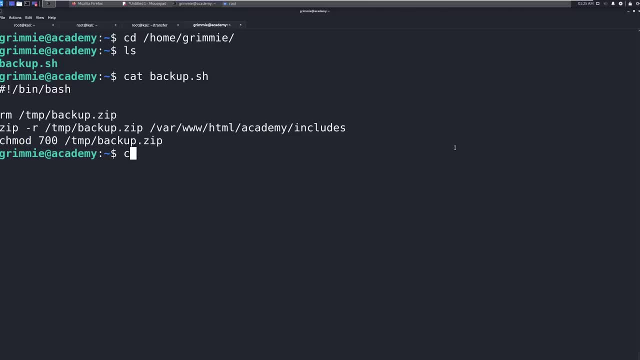 cron information from Lynn peas. I didn't see it in there. we could also do a cron tab. dash L to see Here. we have no cron tab for Grimmy, So what's happening possibly is that Grimmy doesn't have the cron tab. we can try to see if we can cron tab. 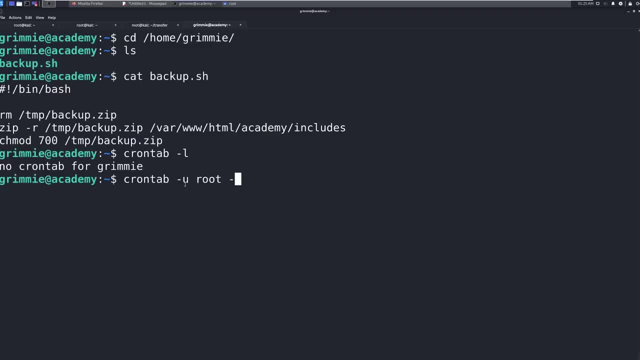 Of a user, look at route and just do it a dash list. But it says you must be privileged. So we have to run pseudo. but we don't have pseudo. So we won't be able to switch into route to use that as well. We don't have privileges to that. So, without having any cron tab information or seeing 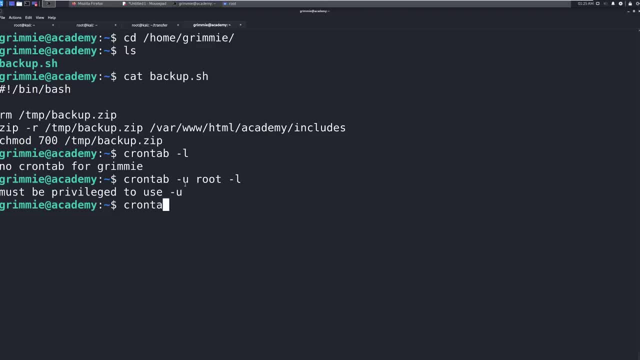 it running. when we looked at the cron, we could do a cron tab dash E as well. I just don't. I mean, there's nothing. there's nothing in here, So this isn't giving us any indicator And a cron job is. 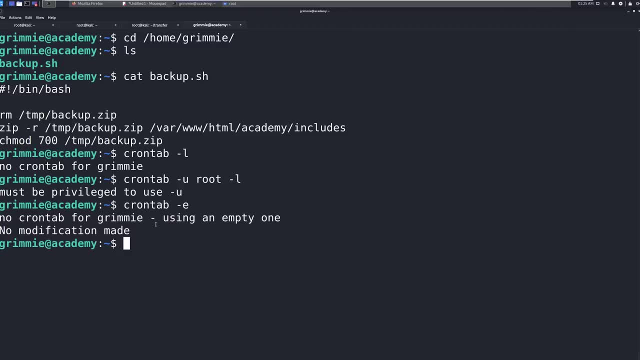 something that will run for us, by the way, And we tell it: hey, I want to run this, this script, every hour, every minute, every day, every week. we could tell it when, when we want it to run. So this is a realistic scenario in that sense that cron jobs are used in administration. So, from 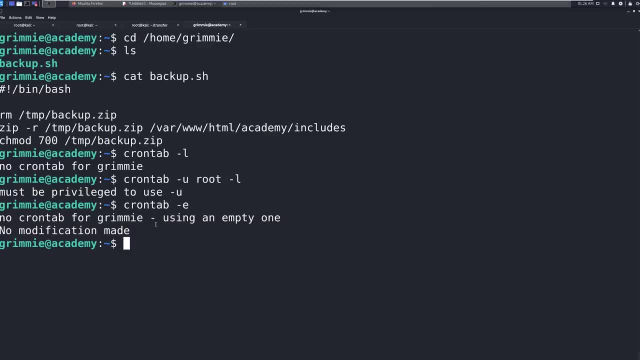 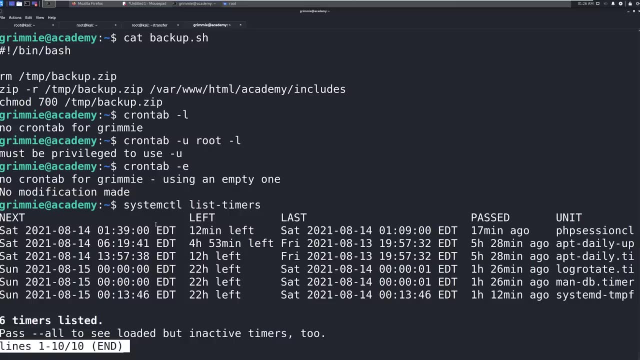 here. if we don't have that, there's something else called a system D timer. we can look at that from system CTL and just say list timers And let's go through like this and see if there's any script in here running that's in a timer And I 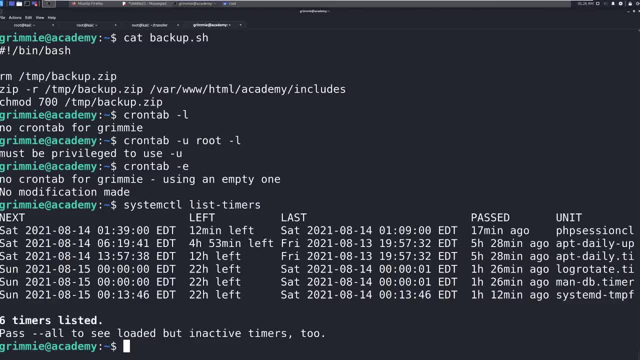 actually don't see anything here. you can hit Q for quit And that'll that'll exit this. So when we have this situation, there's a tool that we can use out there that will actually give us more information of what's running with the processes than what is leading on. Remember we ran a PS. 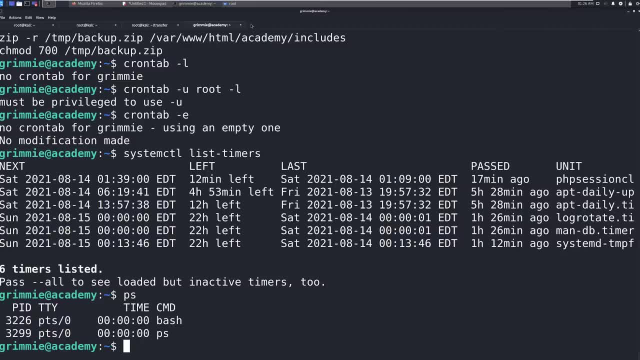 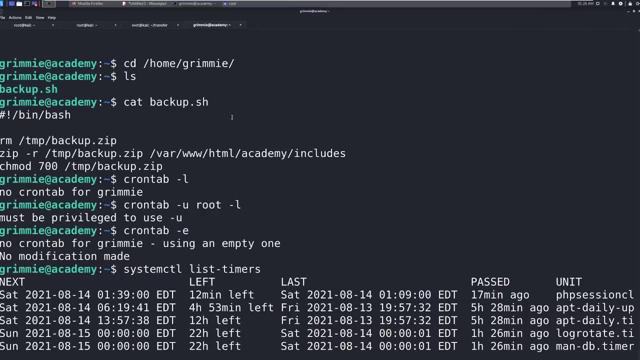 with the. we ran PS for everybody with the, the script, the Lin peas. we saw it, we didn't see it running And there was a tool out there. So that's a good example And you can see it's a very good tool And 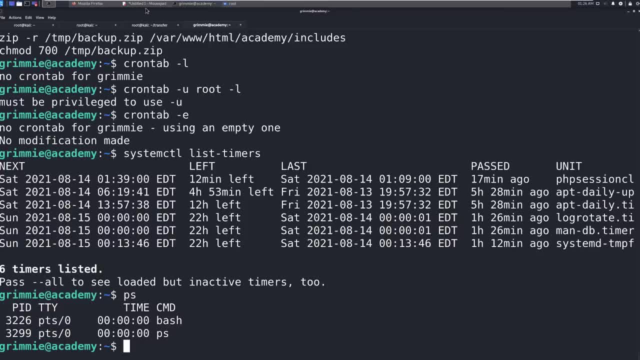 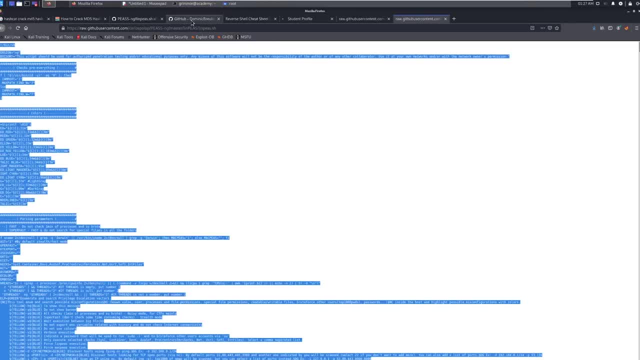 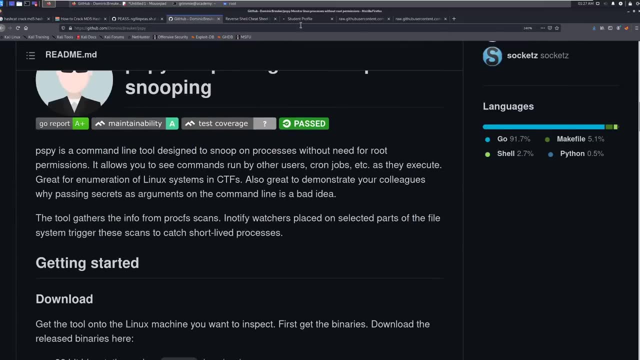 you can see anything in there that was any indication of this backupsh. So if we want validation and confirmation that this is running on a timer, we can go ahead and go out, And there's a tool out there that is pretty neat. It's called PS pi, PSP Y, And all you have to do- literally I have to do- Google this, by the way, just I'm. 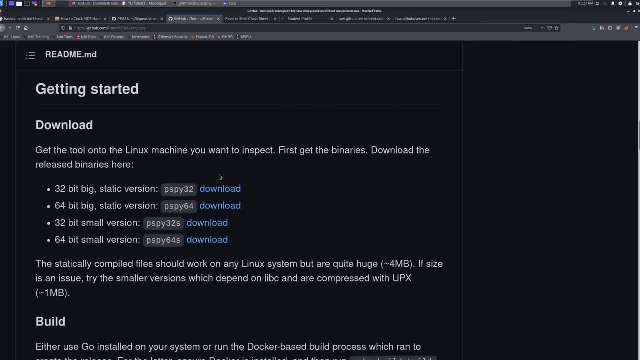 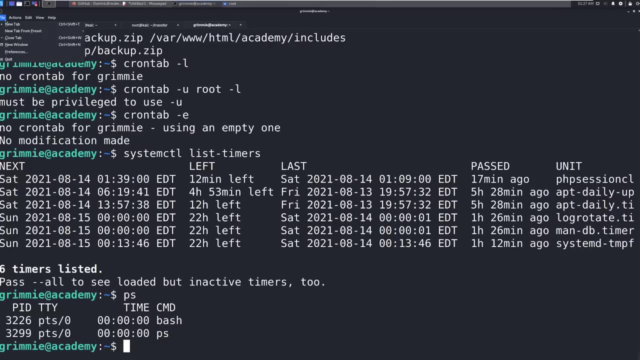 gonna do it, Just so we can say we did it So in here. what you want to do is go ahead and download the 64-bit static version, And when you download that you might get put into your downloads folder. All you have to do is we'll open a new tab here real quick. 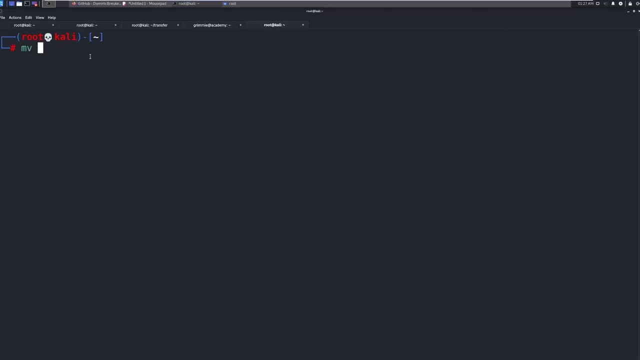 All you have to do is do a move command if you don't remember. So move downloads PSPi and just put that in your transfer slash PSPi. okay, PSPi 64 is actually what it's called. I'm just winging it here. 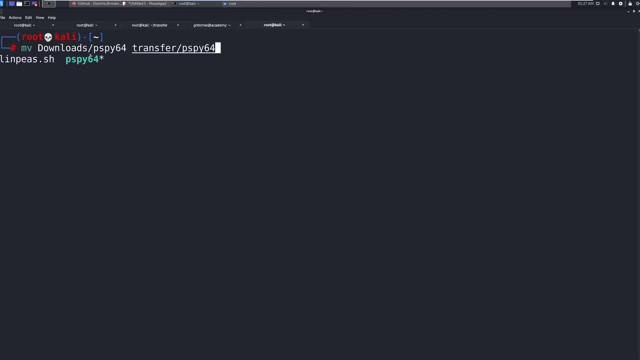 I've already got it in my folder, but make sure you move it over to your folder. Or if you want to keep it in downloads and run from there, that's fine as well. Just note that I already have this in my folder here. 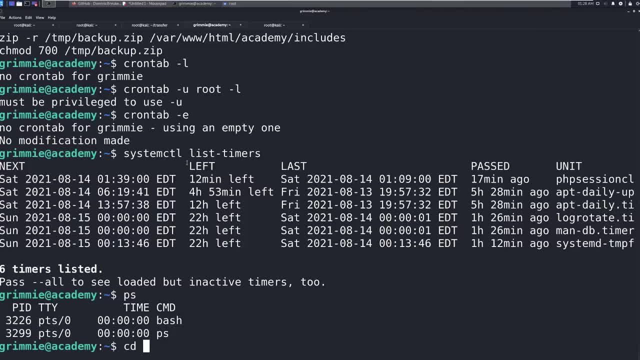 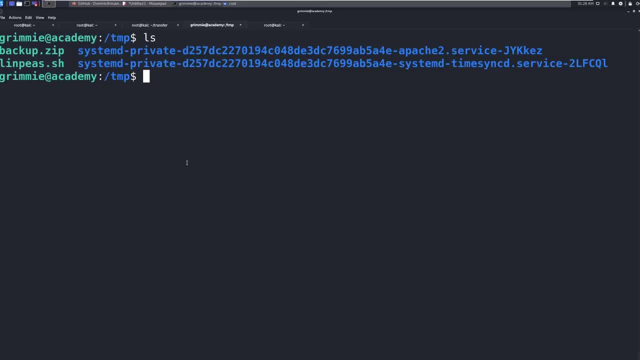 So all you have to do now is cd over to your temp folder. If ILS- I've already- I've got some stuff in here- Looks like linp's backupzip is sitting in here. What I'm going to put in here is this PSPi and we're going to run it. 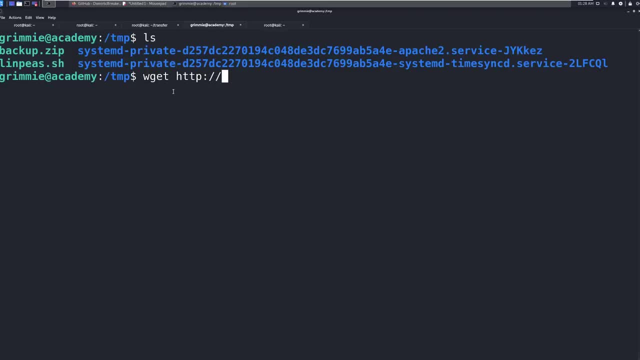 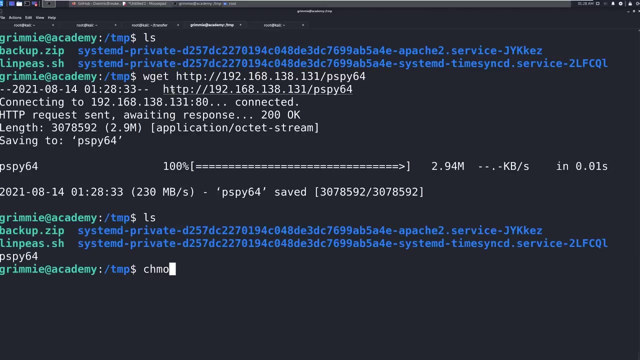 So I'm going to do a wget And remember I already have my listener for my web server running from earlier. So this is just going to be a simple grab and go, and this is PSPi 64.. Grab this, All right. ls chmod plus x on PSPi 64, and we're going to run it. 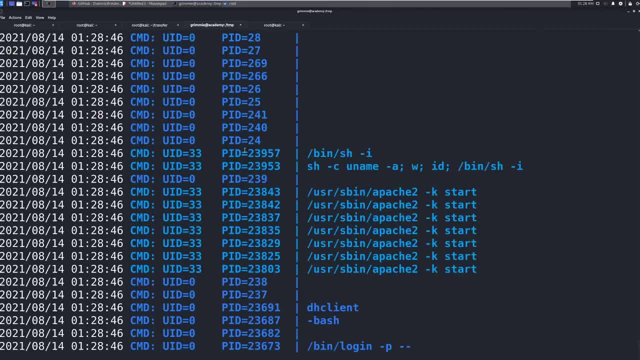 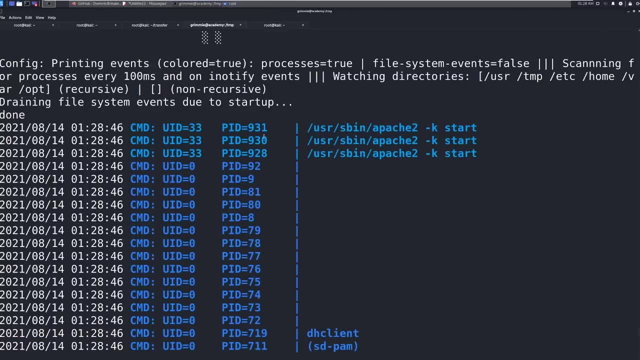 Now, what this is doing is showing us all the processes. This is running on the machine, all of them, And we can scroll through this and kind of see, and yours is going to look different than mine, Don't worry about the PID numbers. 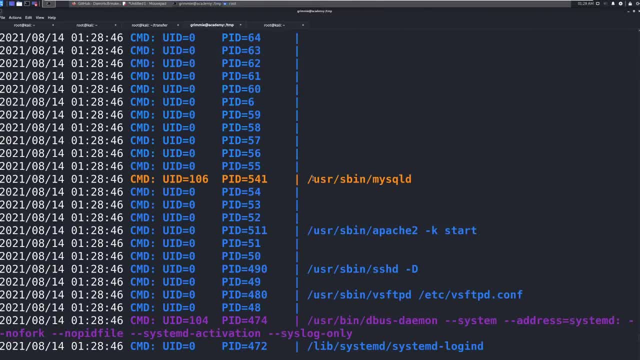 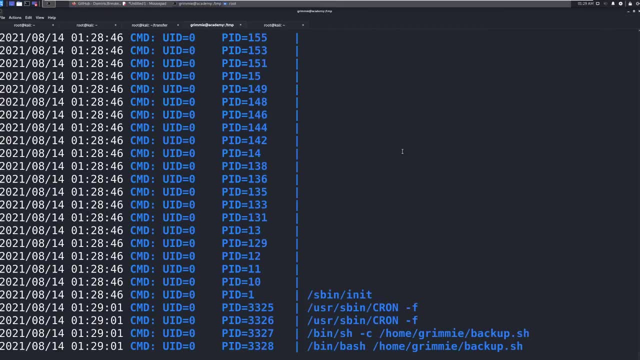 Don't worry about the timing, Don't worry about anything like that. All you got to do is scroll through here and see if we can see that backupsh running, And we can come through see if there's anything in here And look, now it showed up, backupsh. 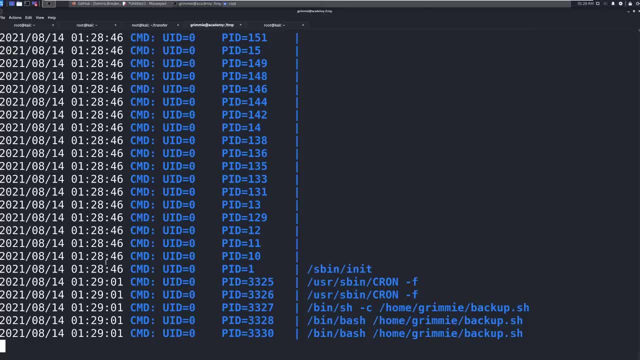 I don't think that was there before. So what happens is it just waits for this to run And then, when it runs, we're seeing it come through here, So that looked Like it just ran. If we wanted true confirmation, we could sit here and wait another minute and see if this runs. 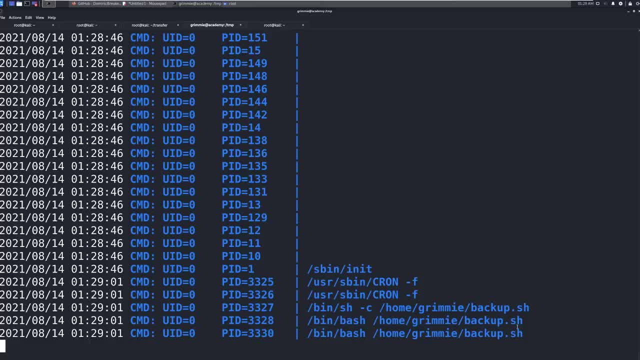 because my punch is just running every minute, because this is capture the flag box, So we could do that. I'm going to tell you that it is running every minute, so we don't have to do that, Just to save a little bit of time. 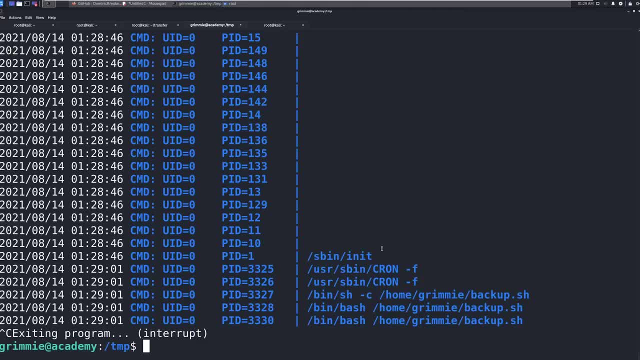 So control C, get back into your Grimmy at Academy. And now we are going to abuse this in our favor. Let's go ahead and go to CD home Grimmy. We're going to go back. Make sure you have your backupsh in there. 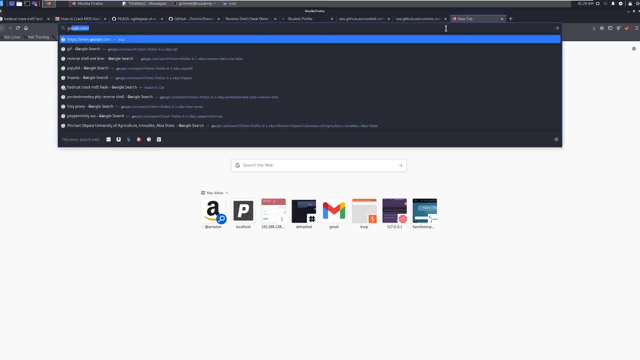 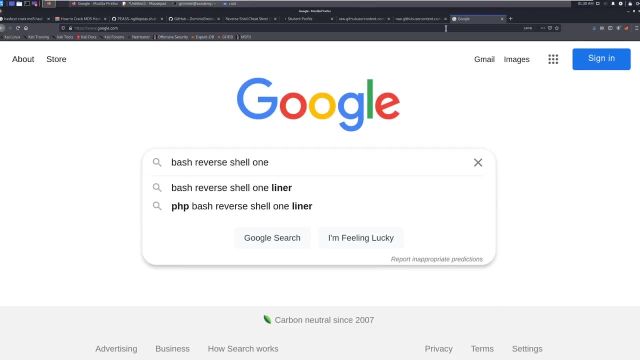 And now what we're going to do is I want you to Google. Go to Google And you go and say: bash, reverse shell one-liner. Okay, And there is a reverse shell cheat sheet from Pentest Monkey. You could also type that in. 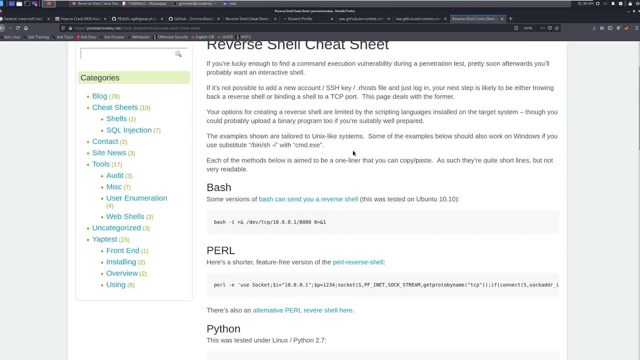 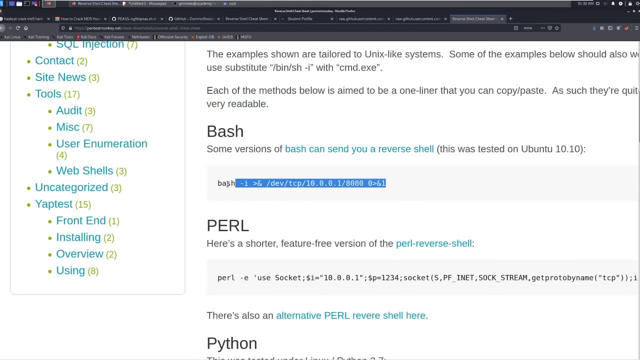 Click on that Here you will see right up front. you will see bash-i. You're going to see this right here. This is a one-line reverse shell. This is awesome. All we're going to do is put this into a shell script, which we already have. 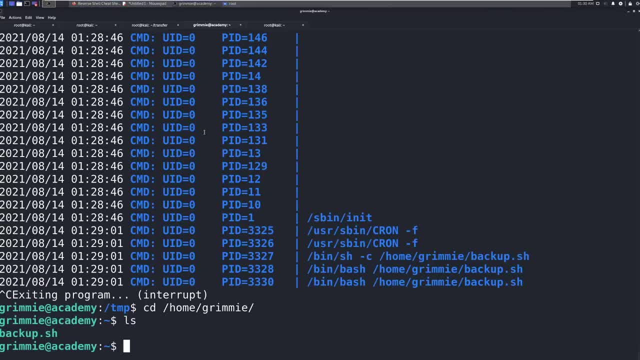 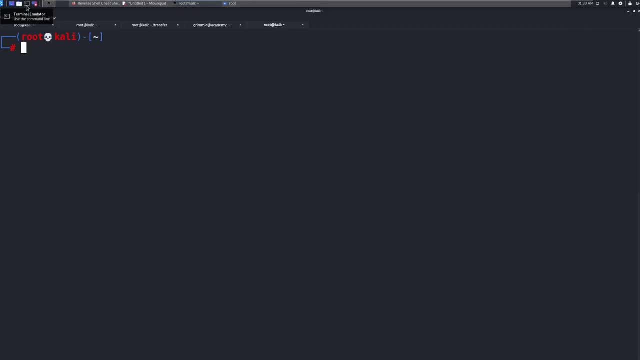 We have it right here, We're going to put that in there and when it executes, it's going to perform reverse shell. So what we want to do is we want to modify this a little bit. So let's go ahead and open up a notepad real quick. 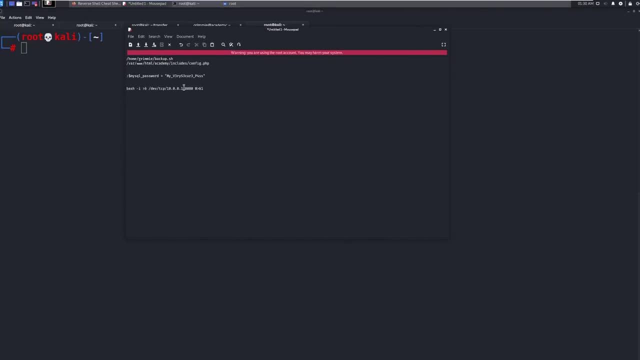 It might be a little bit small on your screen for you, but what I'm doing is I'm putting in where it says 10.0.0.1.. Okay, I'm putting 192.168.138.131,, which is my attacker machine. 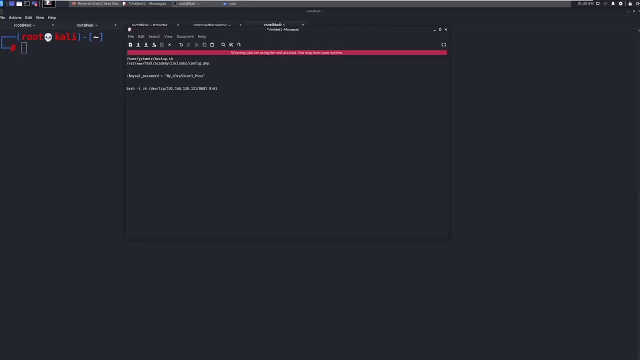 And I'm going to change the IP address to 80.81 or to the port to 80.81.. You are more than welcome to keep it at 80.80.. I'm just doing this because I ran through this once earlier and there's a. 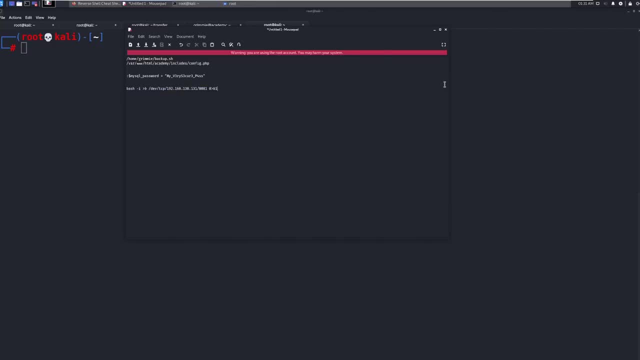 possibility that port is still out there lingering. So just for the video purpose, I'm changing it to 80.81.. So what does that mean I have to do? net cat and VLP, set up that reverse shell listener And here's what's going to happen. 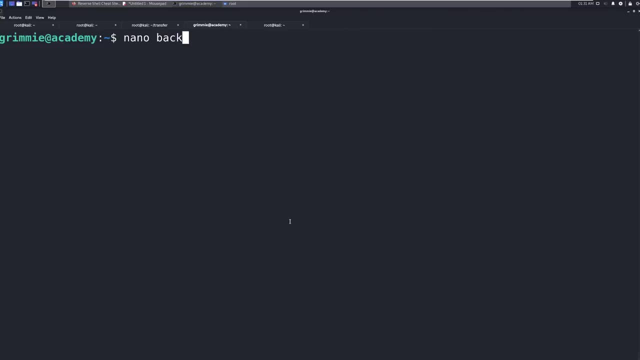 We're going to come in here and we're going to say: nano backupsh. You can come in here, tab down a couple of times And if you hit control K it deletes a line. That's the magic, If you didn't know it, and you can come right, click paste selection, maybe. 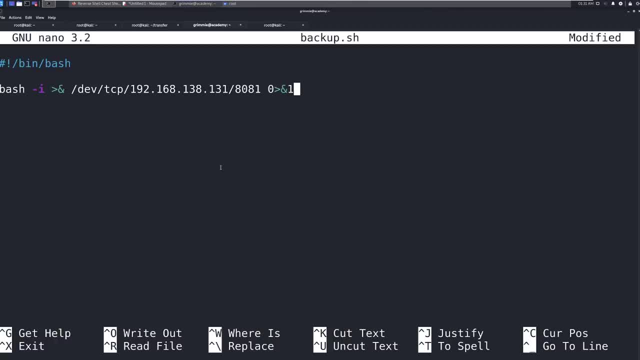 paste clipboard. Okay, Uh, and what we're going to do is this is going to execute bash dash I dev TCP when I two and six, eight. it's going to call out to our IP address with this And, if our hunch is correct that this is running as the root user, we're 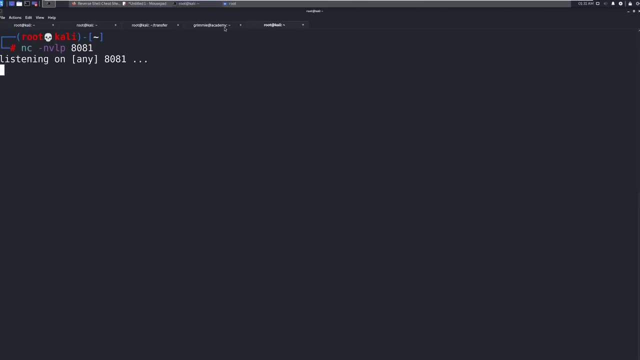 going to get a root shell on this. So what's happening is this: cron job is out there, It's running as root, it's executing as root And when it executes that script, it's going to execute as a root shell, which it just did. you could see root at Academy. 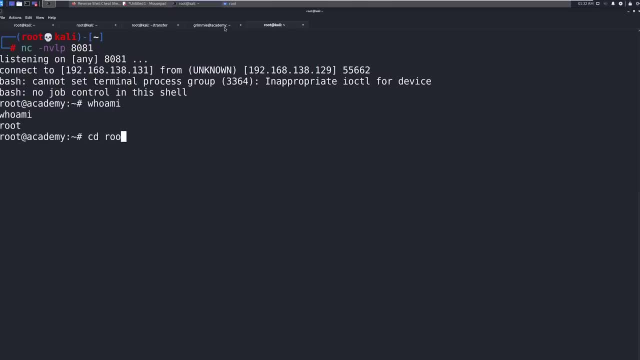 Who am I? Okay, So let's CD to root, just for the fun of the game. Uh, maybe CD root LS. Okay, And then cat flag dot TXT Says: congrats, You rooted this box. Looks like this CMS isn't so secure. 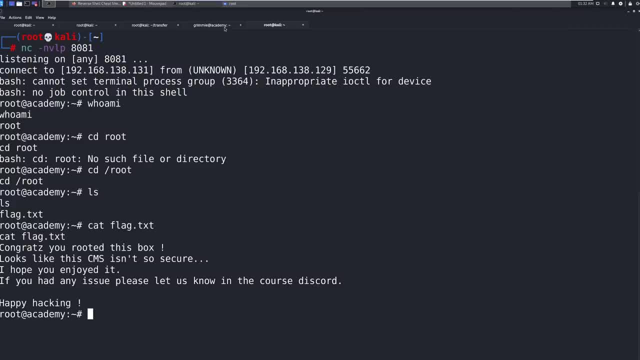 I hope you enjoyed it. If you have any issues, please let us know. in the course, discord, happy, hacking, Great. That was a example of a box with a couple of pivots, a couple of different privilege escalations and very gamified, very capture the flag. 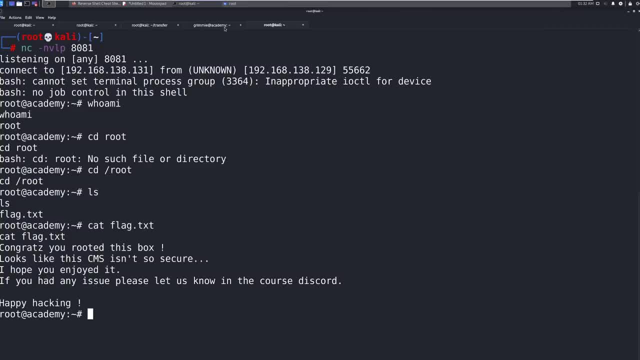 You will likely never do most of this on a pen test ever in your life, but it's still important to learn from the hacking process as we build up into this And then as we get into More of the active Directory stuff. So that is it for this video. 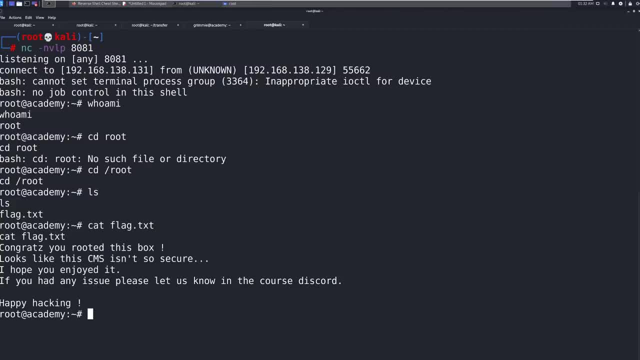 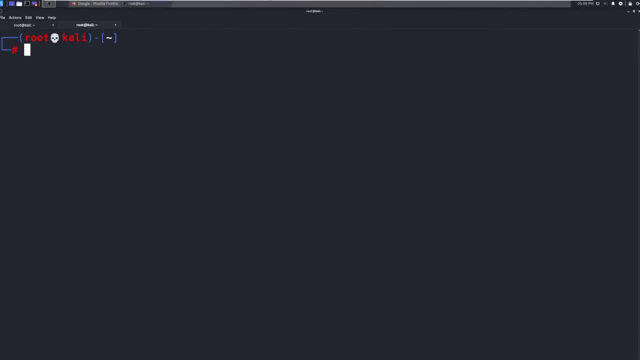 We're going to go ahead and call it here And I'm going to go ahead and catch you in the next one. Okay, Onto the box, dev. Now let me preface this with: it is raining pretty bad here, So if you hear thunderstorms or anything in the back, consider it part of the ambiance. 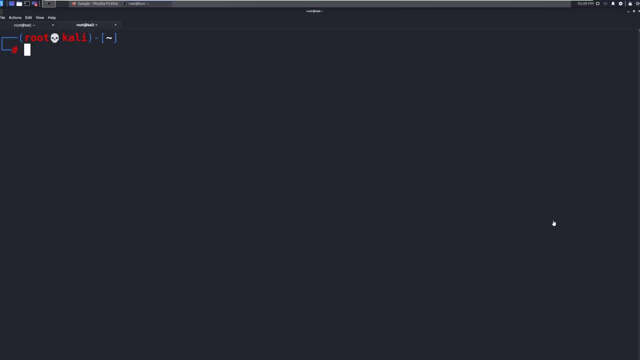 Uh, but we're going to do another box from Alec. Thank you, Alec, for creating this wonderful machine, And this box is a Linux machine, so you should already have it, uh, set up. We're past the setup stage. 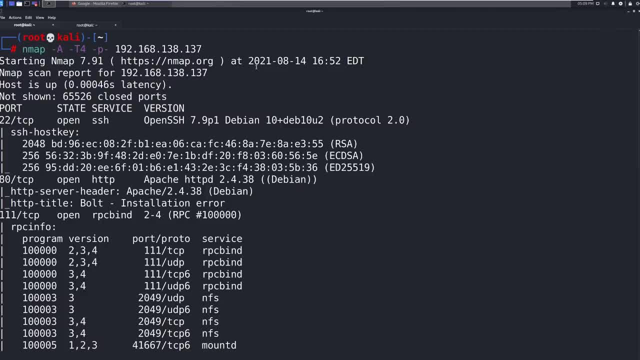 You should know how to set it up. come in here. I already have an MAP scan ran against it, So if you do not have an MAP scan ran against it, you should go ahead and do that Pause if you need to, Otherwise you could just follow along. 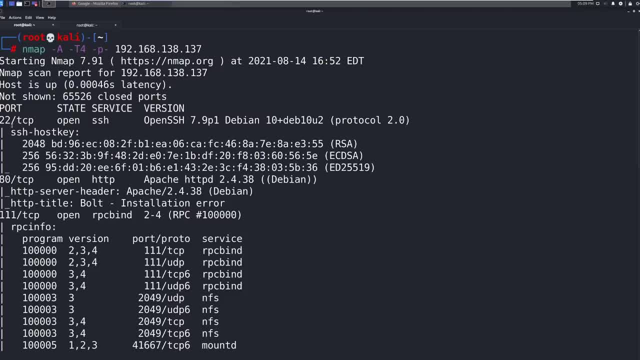 So running the MAP scan, we could see that we have port 22 SSH. And remember what we said about SSH man, we're not going to look at it right now. It's nothing- That's at least in my experience- I've ever found an exploit for. 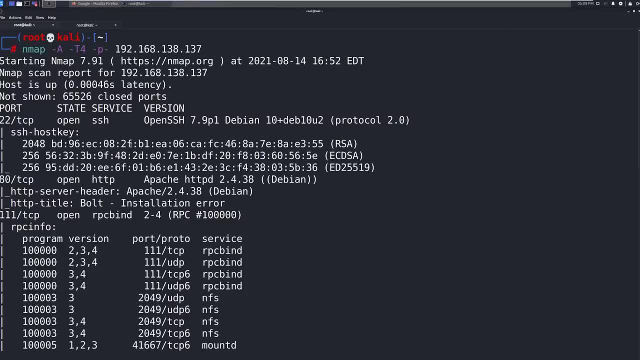 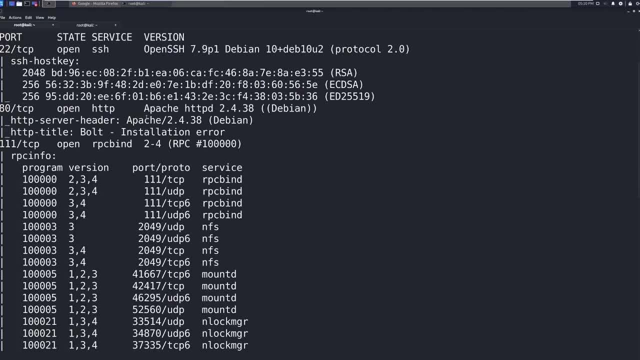 So unless we have credentials or something for that, we're not going to get into SSH. We have something on port 80 called bolt installation air for Apache web server. Okay, That's an indicator. This might be a Linux machine already, Cause we're seeing Debian. 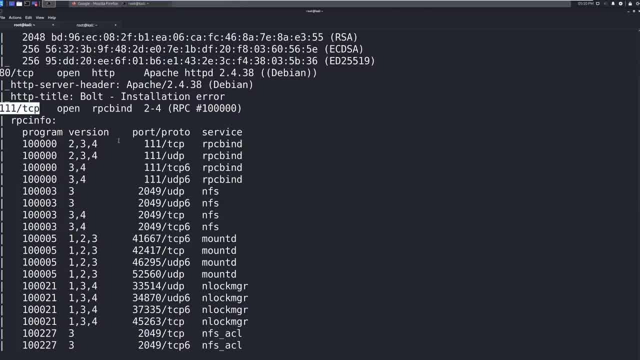 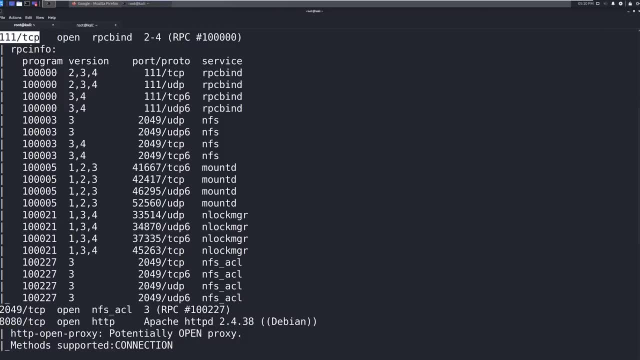 That's a nice indication. We have RPC bind which we can enumerate RPC, though It's not that advantageous for us right This instant that gets into more advanced stuff. Honestly, As a beginner, we're going to leave RPC alone, though. 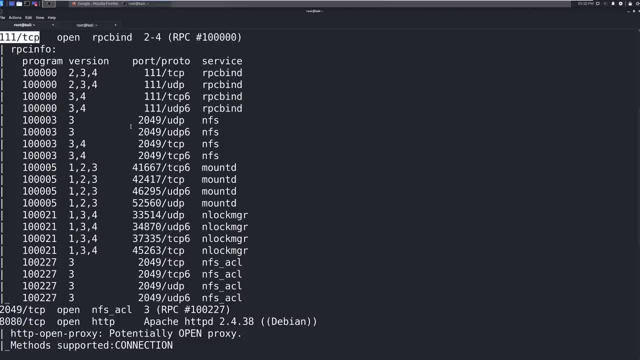 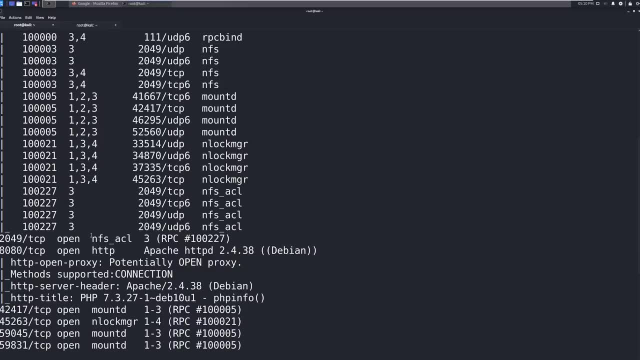 There is some information gathering that you can get out of RPC. as of right now We're going to just kind of push it to the side, Cause we've got more important things to focus on and more common things to focus on. So we have 2049 NFS, which is a network file share. 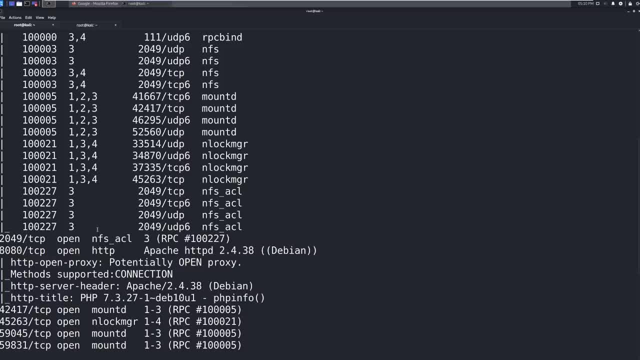 Think of it like almost like SMB, like a Samba for file sharing. This is a network file share. We can potentially Mount to a file share here, So that might be of interest for us. We also have HTTP here for 80,, 80.. 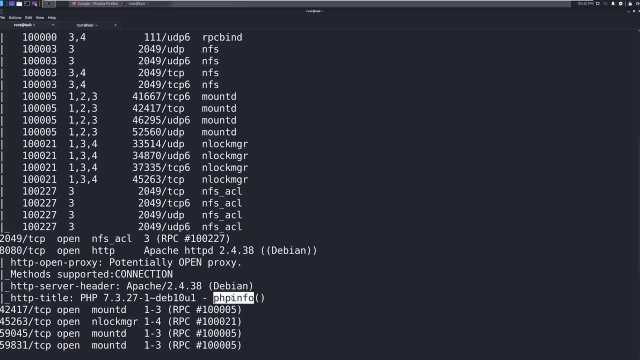 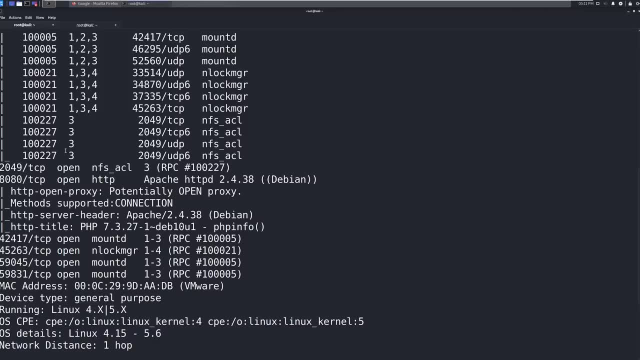 It just says: uh, connection Apache Debian PHP info page. Uh, we've got some mountain D and lock manager. We're not going to worry about any of these. ports which stand out to me are 80, 80,, 20,, 49 and 80.. 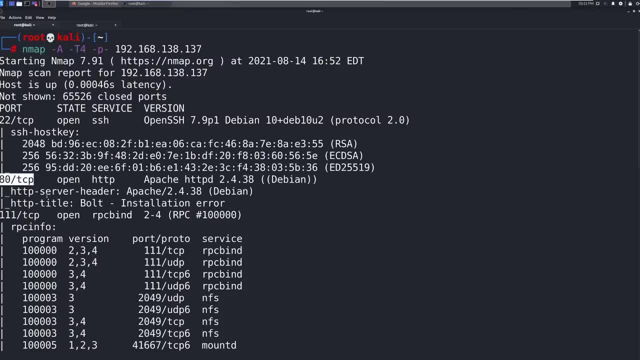 Okay, So keep those in mind as you go through these more, as you get better at this, it'll be easier for you to understand which ports you're looking for, which ports you can kind of just throw to the side for now. So 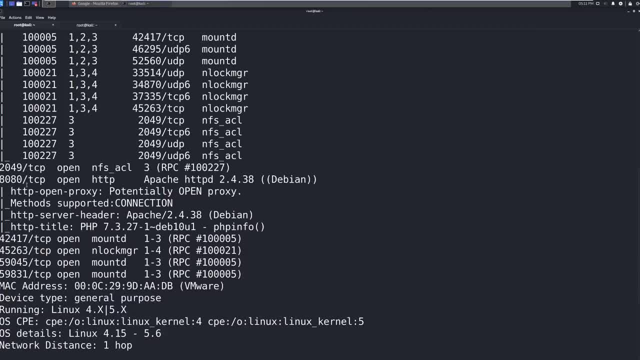 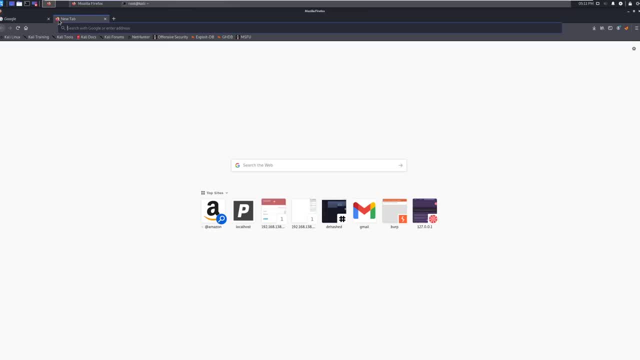 With that, we're going to go ahead and take a look at 80.. We're going to take a look at 80, 80. Then we'll take a look at the network file share. So, going out to the webpage, I have Google open. 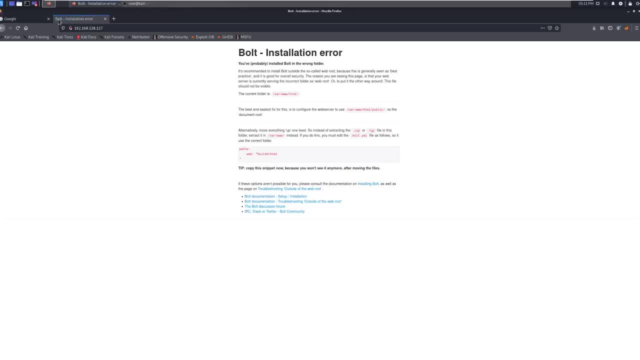 I'm just gonna go: 1 9, 2, 1, 6, 8, 1 3, 8, 1, 3, 7.. Go here And I'm also going to copy this and take this out to port 80, 80.. 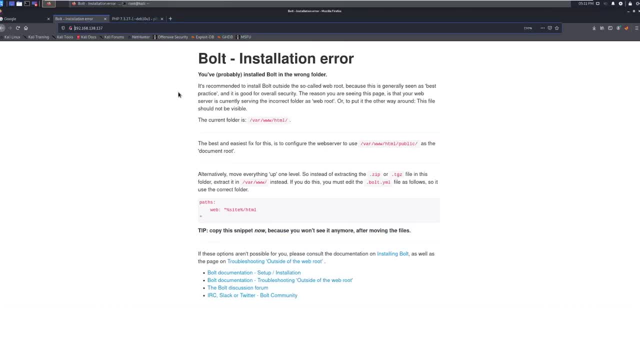 And you could see that we have a couple of pages. One is a bolt installation error page, which is interesting. We can come out and look at This. it looks like there's something called bolt. We can actually go to the real webpage here and see what's running. uh bolt CMS. 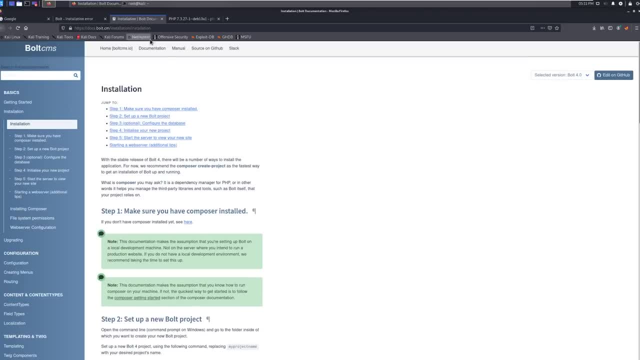 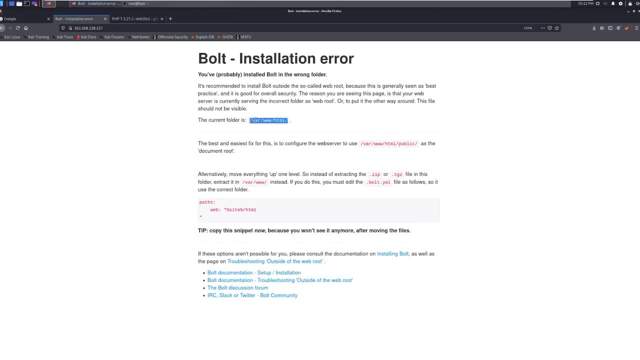 So we'll keep that in mind. Maybe they're running bolt CMS. We could put that in our back pocket in our notes. It looks like there's an installation error. It's talking about the folder that should be installed, in which these are Linux folders. 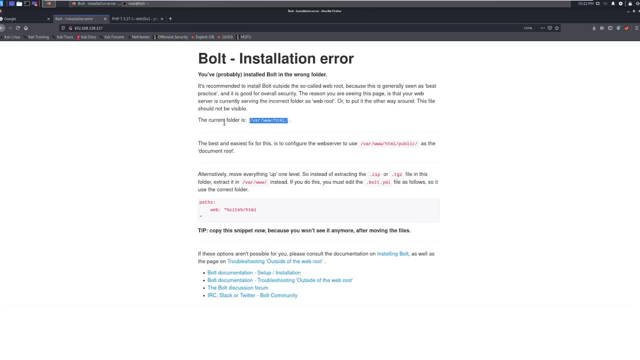 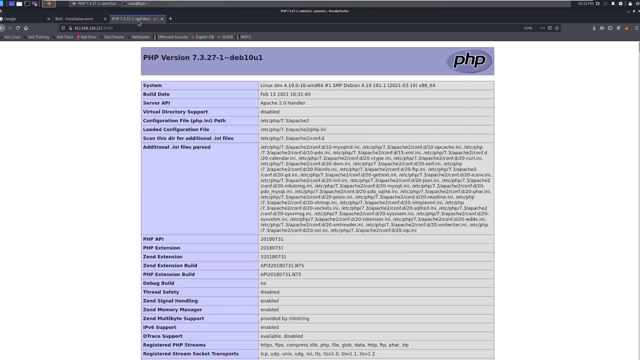 So this is more indication that we're likely attacking a Linux machine here. so we can do some research on this, but let's put that in our back pocket for now. Um other website here is Um port 80: 80,. we're getting a PHP info page, which is nice. 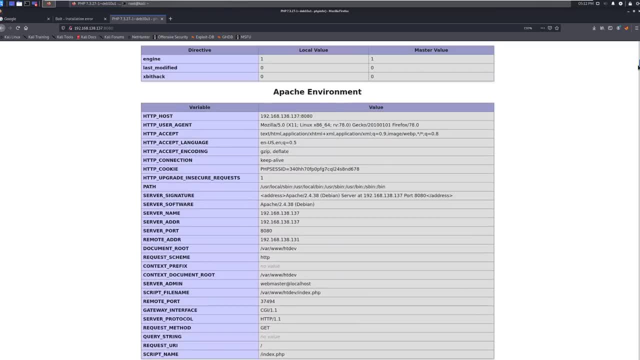 Uh, sometimes this can disclose some information. You can actually read through this and see um like: here's the path, here's like the webmaster, here's the IP address that we're we're pointing at. Uh, so there's some different things in here that we can, we can, look at. 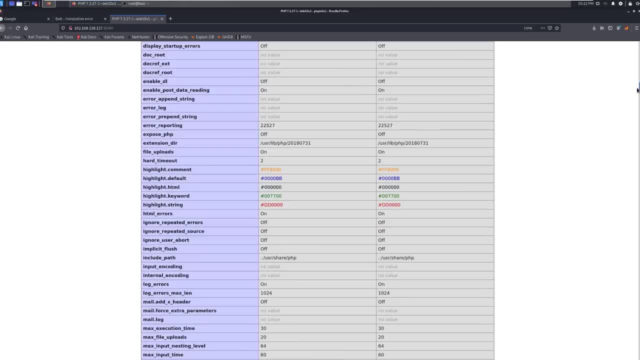 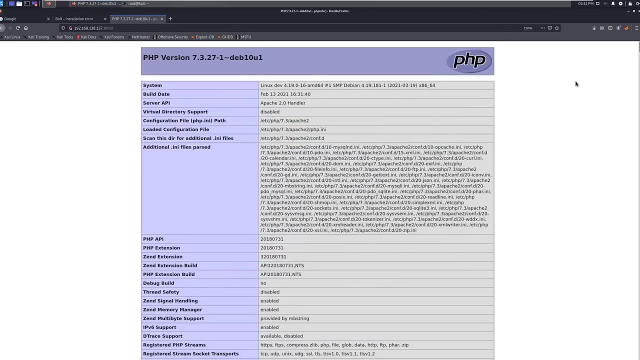 And possibly, if we were attacking this page, there can be some information disclosure in here that could tell us what the setup is of this PHP page, Um, and That could tell us like, Hey, maybe there's file inclusion, Maybe there's uh, uploading allowed a different attacks that might be enabled because of a setting that is configured or misconfigured in this PHP: my info type page. 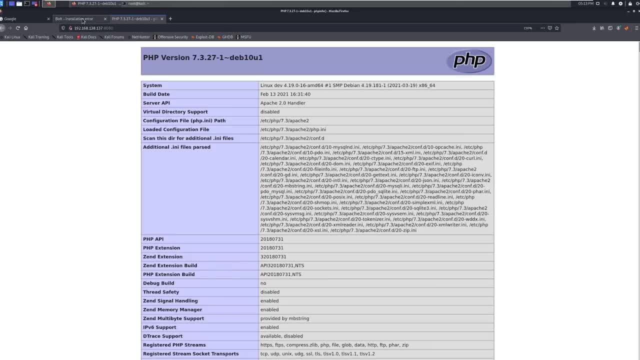 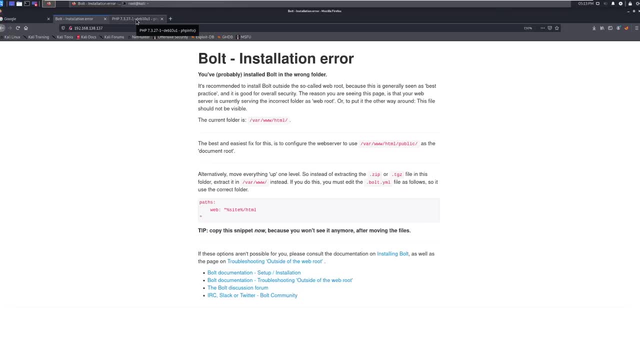 So our PHP info page, So We have two pages here that are, I mean, there's nothing really there. It's it's like: Hey, PHP info, bolt installation air. So we kind of want to look under the hood. This is just common. 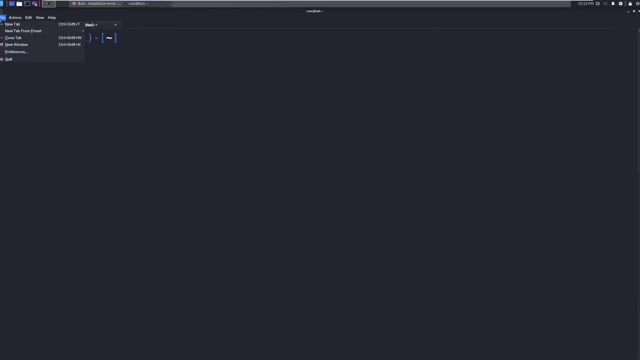 Common tactic here that we're going to open up a new tab. I'm going to open up two of them and we're really just going to uh, enumerate this a little bit further. I just want to see how, how far we can take this. 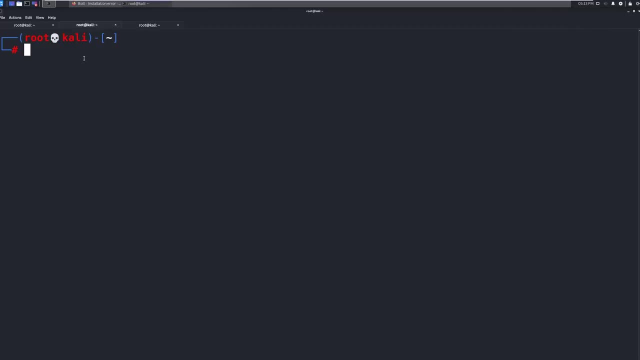 If, if it is what it is like, port 80 is literally just a bolt installation area page, That's fine, but we need to confirm that. So we're going to use uh F, F, whatever you want to call it. 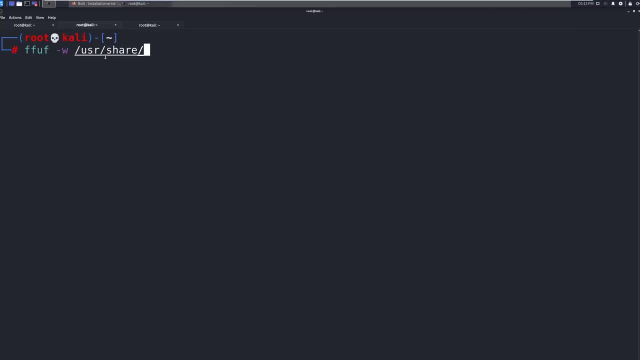 And we're going to do a quick scan on this and we're going to do a user share- uh, wordless. And then I go to dirt buster and, just like before, you can just tab and I use the medium word list. I put a colon. 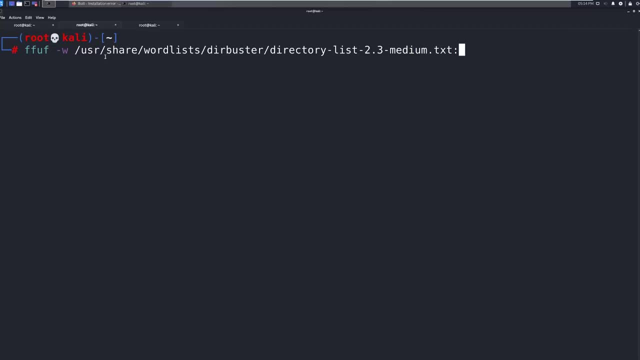 I don't know how to you know the trick of getting it to line up immediately after you. let me know. Otherwise, just go delete that one space. We can fuzz here And then we can do a URL of HTTP: 1, 9, 2, 1, 6, 8, 1, 3, 8, 1, 3, 7 for this machine forward slash, fuzz. 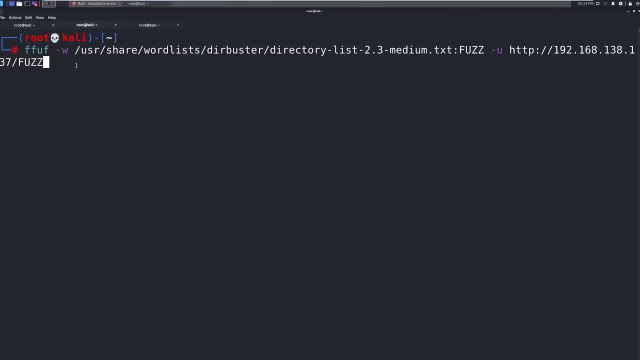 Now, before you hit enter, go ahead and copy this. We'll make life easier. hit, enter, Let that bad boy run. come in here, paste again. And all we're going to do on this one is we're going to put 80- 80 at the end of it. 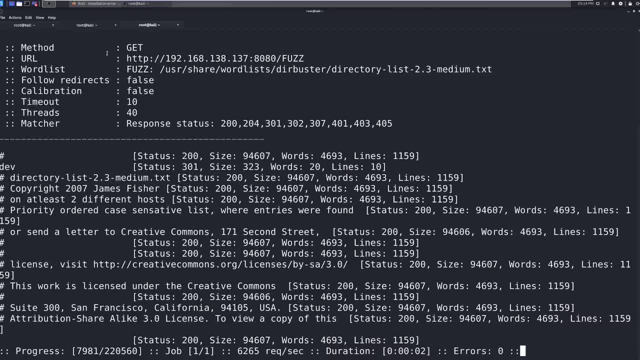 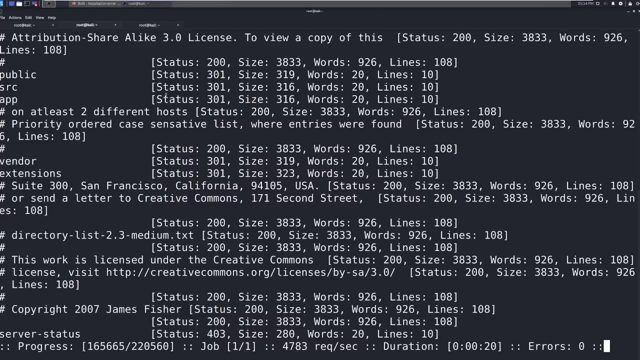 So we're going to fuzz against 80, 80 and port 80, and we're going to let these run a little bit. Okay, So we'll let these run, perhaps finish, see if we can get anything of interest out here. 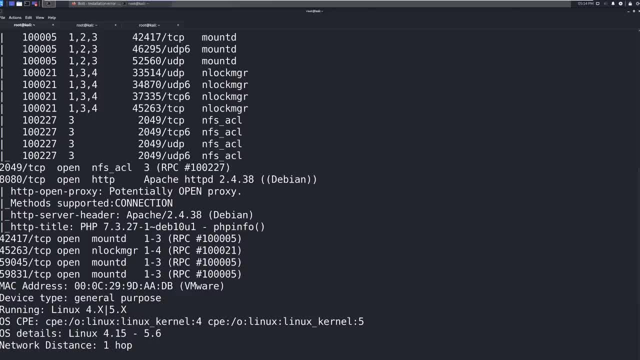 Um, while they're running, we can multitask. This is part of the process, by the way, as, As a, as an ethical hacker, or hacker in general, multitasking is important because you- uh, if you're on an engagement like a pen test, you're going to be doing a lot of things at once, because imagine a situation where you have a thousand IP addresses and you have a week to go against them. 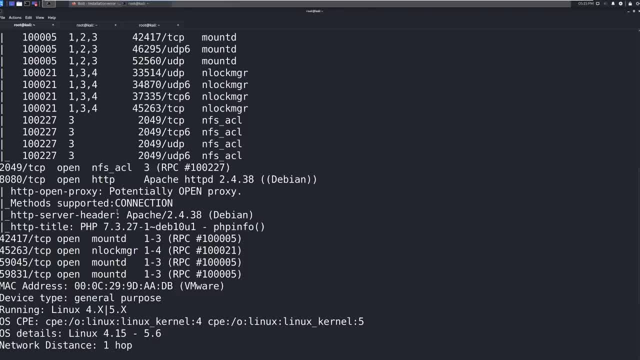 If you only have a week to do, a thousand IP addresses you're talking like a few minutes per IP address to look at. So you really have to identify and scan for low hanging fruit. figure out which IP addresses are the most advantageous. Go touch on those more. 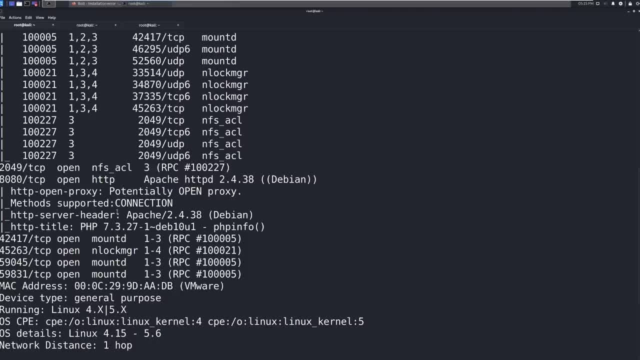 And, um, you know, perhaps be spending a couple minutes on each at the same time while you're doing this. So it's advantageous to look at multiple things, have scans running and be bouncing back and forth. uh, from an ethical hacking perspective, 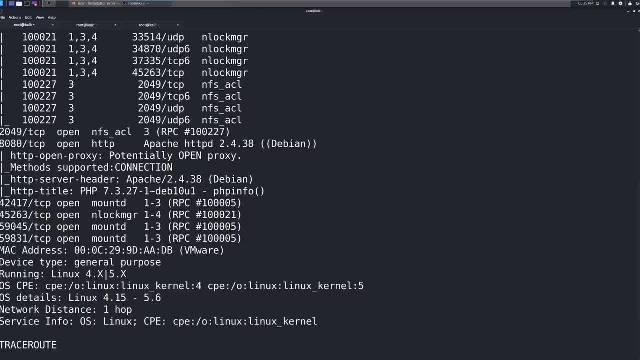 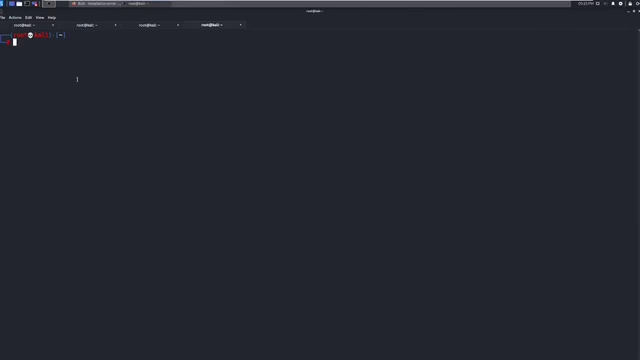 And you pick up the ability to multitask over time. So, anyway, we have this NFS, this network file share, and I'm curious if there's anything there. So what we can do, I'm going to go ahead and just open up a new tab. make this a little bit bigger. 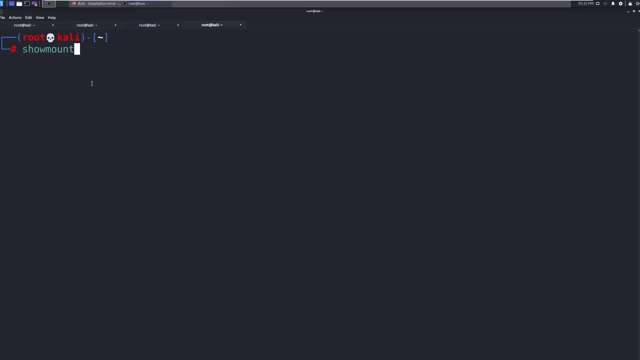 What we can do is we can say Show mount. This is a command already built into your machine. If you're familiar with Linux, you probably know this. but either we're just going to list out the directory, That's here the mounted file share. 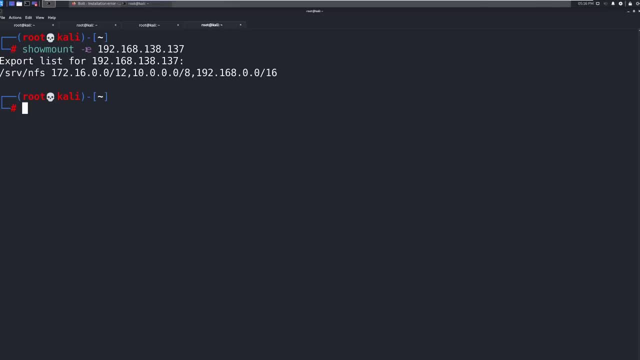 Hopefully that there's one. Okay, And we're exporting from here This. okay, This is the file share that's offered up. So we've got it looks like server NFS network file share. So what we're going to do with this is we're going to go ahead. 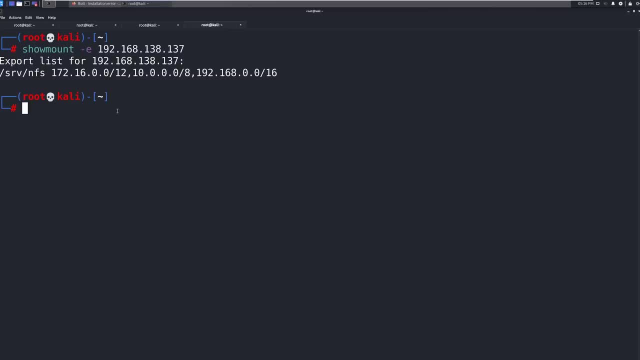 And utilize this uh from to our advantage. we're going to Mount and see what we can see in this share. So in order to do that, we need to make a directory to Mount too. So I'm just going to make a directory called Mount MNT. 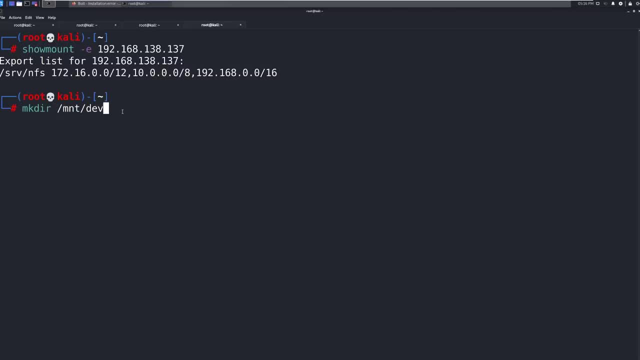 We have an MNT folder by default, and then I'm just going to call this dev, since that's the name of the machine, All right. And then we're going to Mount this. So we're going to say: Mount tack T, NFS. 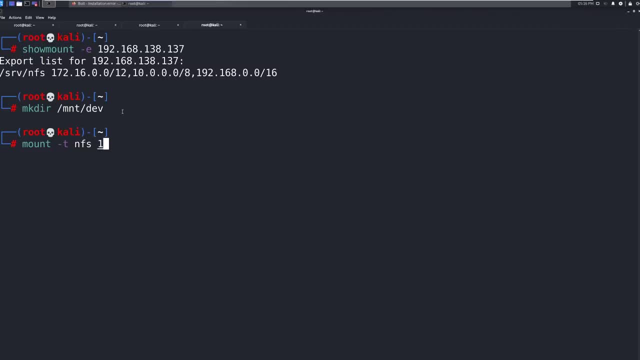 So this is the type is NFS, And we're going to say 1, 9, 2, 1, 6, 8, 1, 3, 8, 1, 3, 7.. And then we're going to do server NFS. Okay. 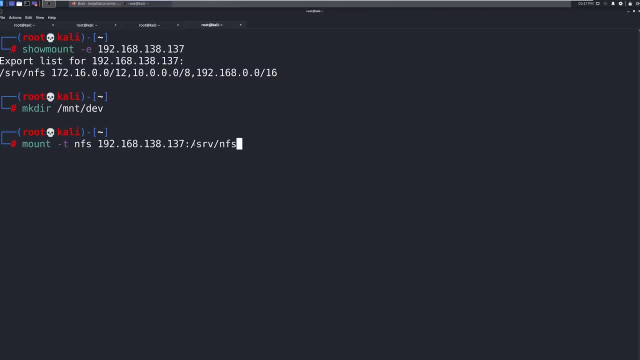 So we're calling out on this machine: is this server NFS or SRV NFS? And then we're going to put it in Mount dev, just like that. All right, So now we can go CD into Mount dev LS and you can see that there is a file in there. 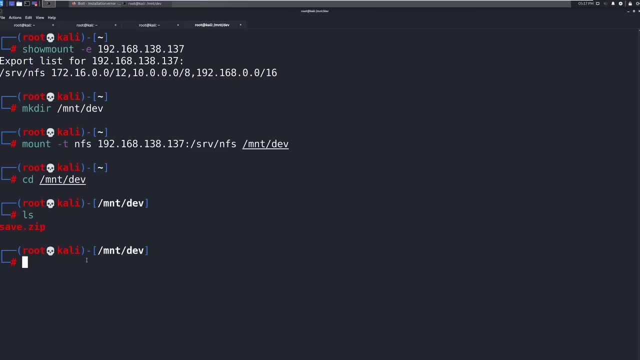 That file is called save dot zip, So I'm going to go ahead and try to unzip that And it says: Hey, we need a password to unzip this ID RSA file. Uh, I have no idea what the what the password is. 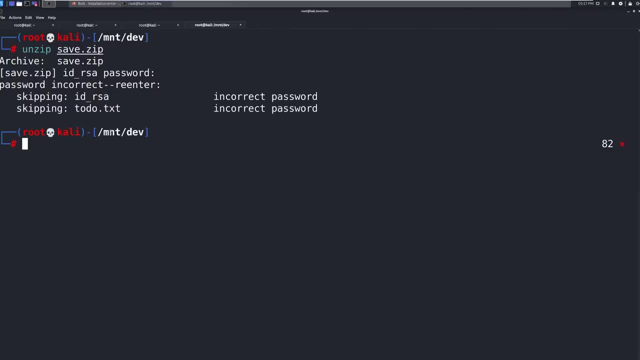 So it looks like there's an ID RSA in here and a to do that TXT, And we don't have the password for either of these. Now there's a possibility that we go online, We look through some of these- uh, these folders. maybe something comes back. 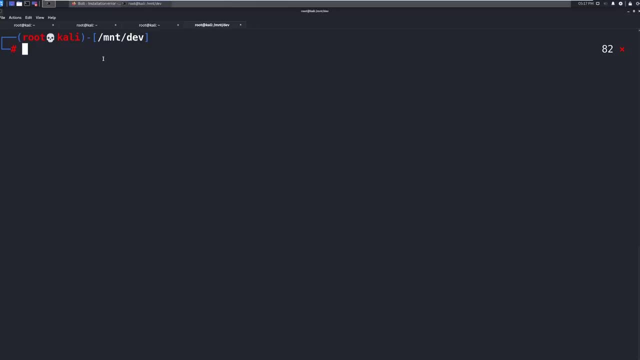 There's a password in there. That's the path to go. The other thing that we can do is see if we can crack this very quickly. If we can crack it, then maybe we can get in there, And there's a tool out there called F crack zip. 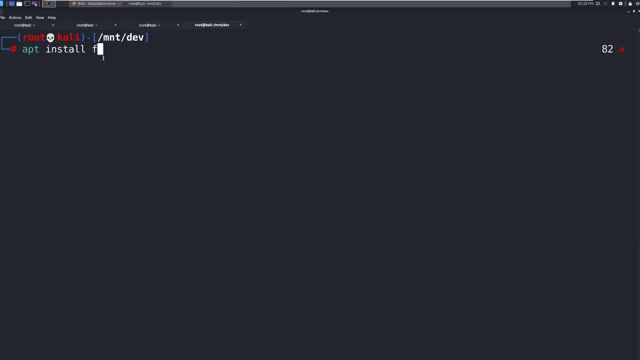 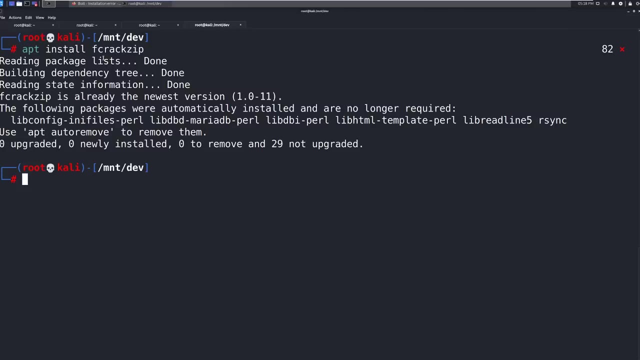 So we can do something called like app install, F, crack, zip, just like this: And I've already got it installed, but you should not. it doesn't come by default. Okay, Go ahead, Let that install. should only take a second. 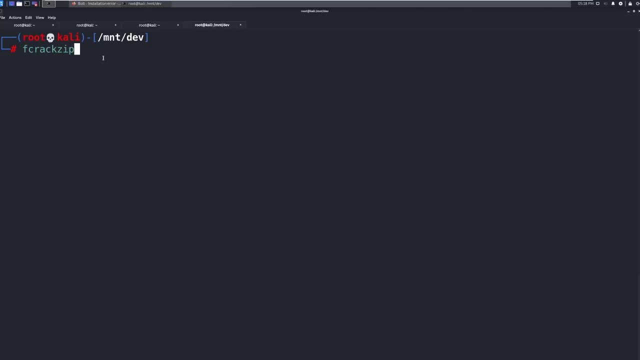 And then come back And now we're going to do F crack zip, just like that. Yours might not auto tab, You might just have to type it out. That's okay. Uh, dash V for verbose. We want to have verbosity here. 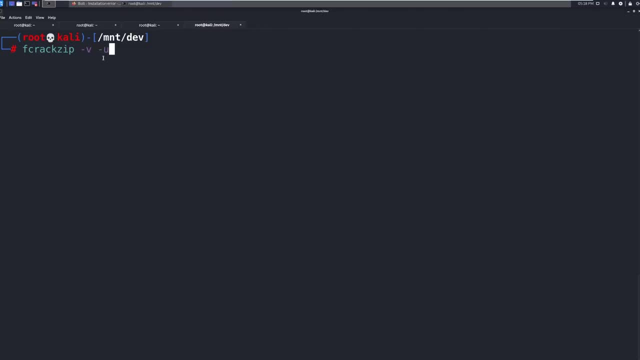 See all the output. uh. dash U just means we're going to be unzipping, So we're going to unzip the, uh, the files here. And a dash capital D means we're going to be using a dictionary attack and a dash P means we're going to be using a file in order to 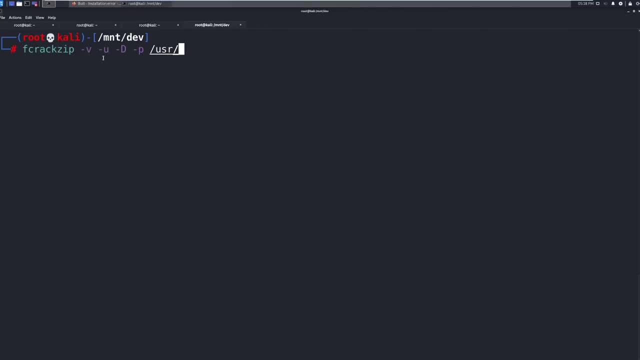 uh attack, So um, the dictionary attack we're using is the user share word lists and then we're going to use rock you, Okay, And on this other part, for the dash P, we're going to go ahead and use this savezip. 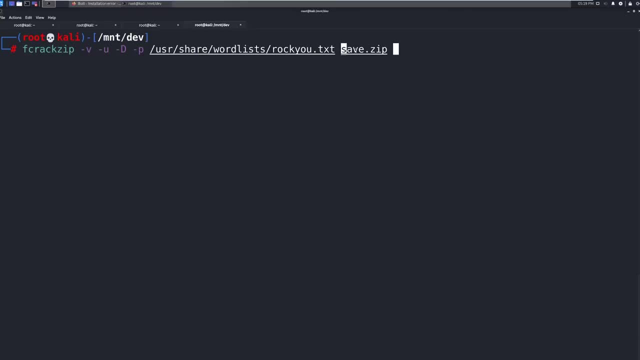 So we're using a string here as the initial password file, which is what we're doing. If we didn't have this here, it would just start attacking uh via the files inside. So we're going to, we're calling out specifically, and then here we're. 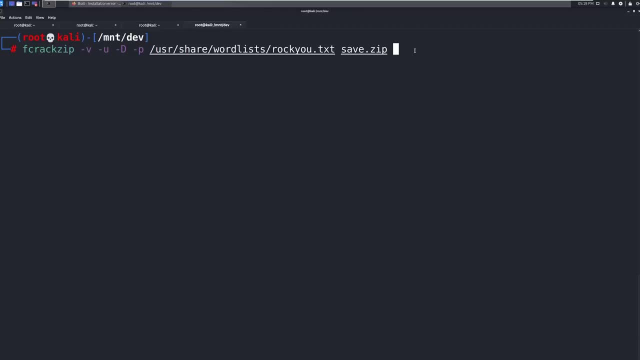 saying we're using a word list, Here's the word list we're using. So we go ahead and run that. Hit enter Okay, And you can see that we have found password is equal to Java one Oh one. So now if we go to unzip, save that zip type in Java one Oh one. hit enter. 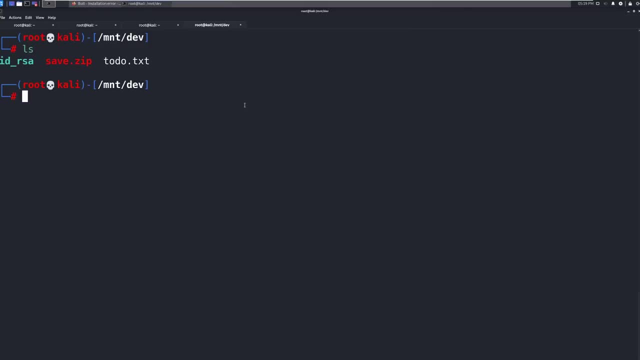 Okay, We Ls. they should be here now. So let's cat out the to do dot TXT. It says: figure out how to install the main website properly. The config file seems correct. Update development website. keep coding in Java, because it's awesome. 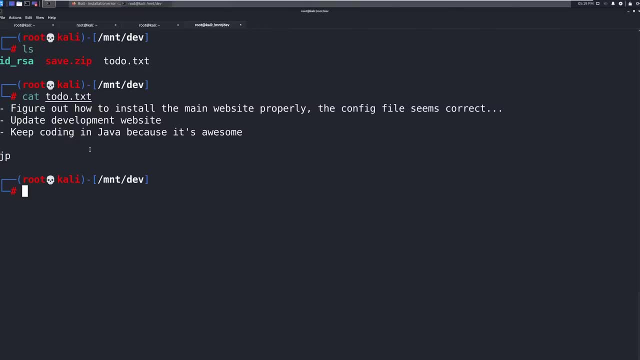 And then we're going to run it And then we get a signature from JP- Uh, we don't know who JP is, but we do get an ID RSA file, So that ID RSA file can be used in order to connect via SSH. 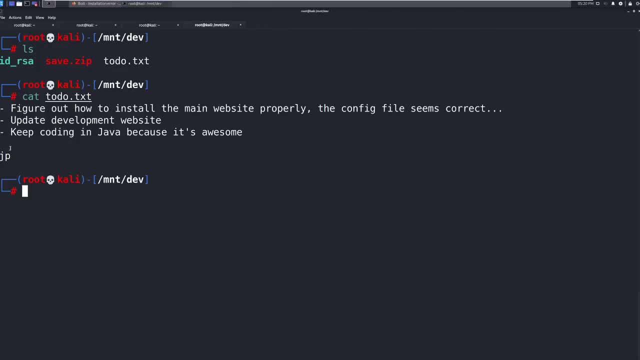 Now we don't know who the user is. There's a chance that the user might be, uh, JP, So we can do something like SSH dash I. I'm not sure if the permission settings here are going to be correct in this ID RSA file. 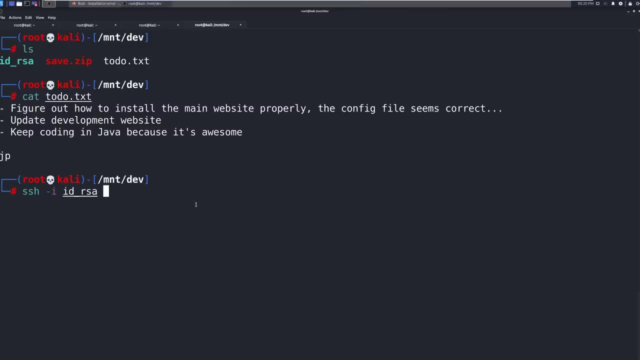 We'll see here in a quick second. And then we come in here and we say something, Something like JP at 1, 9, 2, 1, 6, 8, 1, 3, 8, 1, 3, 7, cross your fingers type. 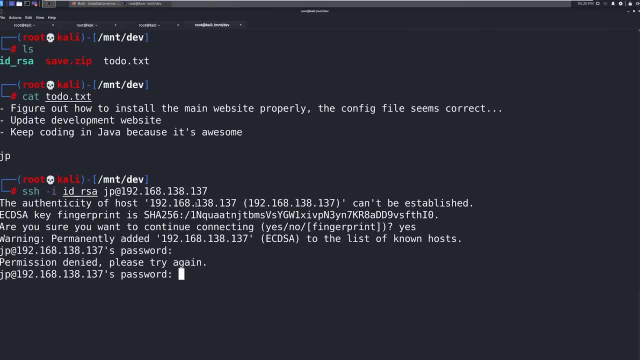 Yes, It asks for his password. Uh, we don't. we don't know a password. Um, so we're not even sure if that's that's working. We're not sure. It didn't even look like it took the ID RSA. 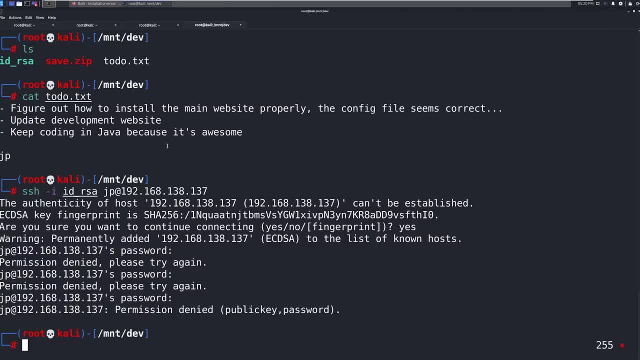 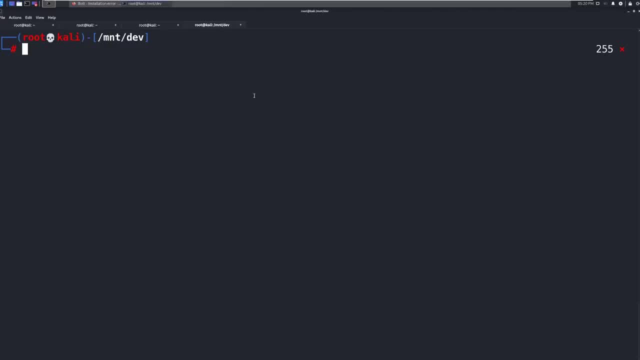 Uh, so we're not sure if this guy's even a user. So let's, let's keep this information in our back pocket for now. Uh, we have this, We're going to clear screen, We have this ID RSA file and we have some information. hopefully. 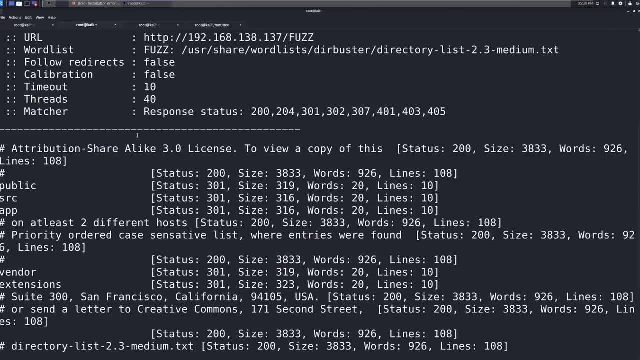 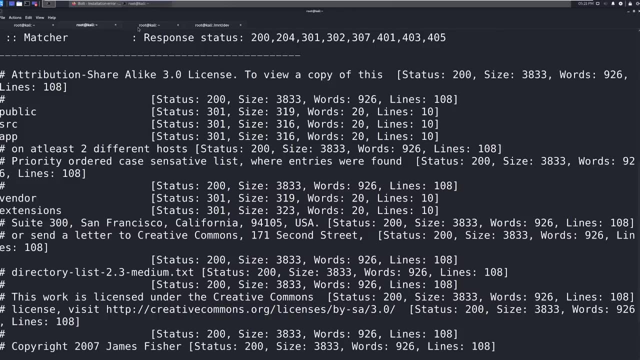 sitting here waiting for us. Um. so on the port 80 side we have a public three Oh one, We have a source- three Oh one, We have an app- three Oh one. um, vendor extensions. Okay, So maybe we come in here and we take a look at that. 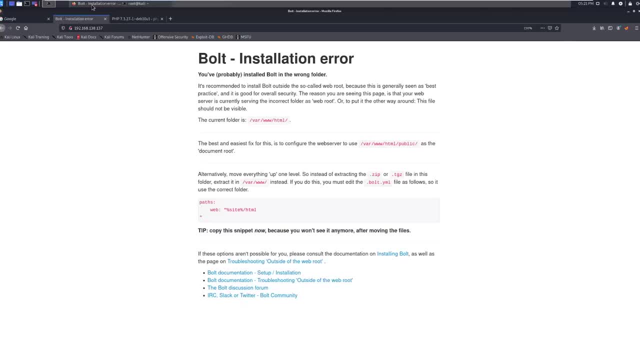 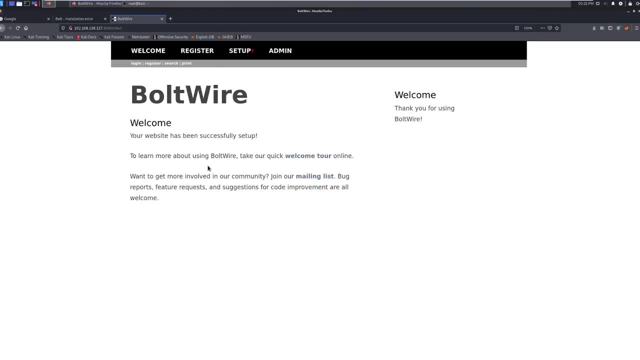 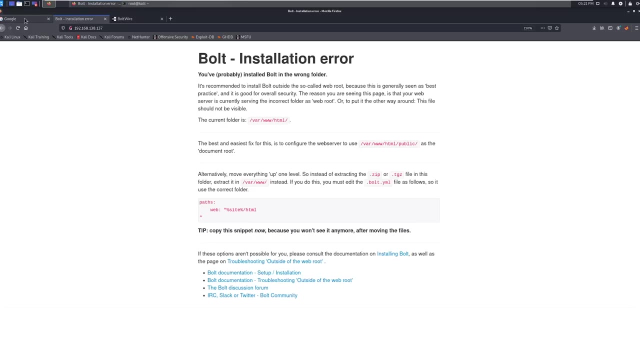 Also, on this side we have a dev directory. So if we go in here and we just Forward slash dev, we are brought to this bolt wire application, which is cool. Um, on here we have a few different. uh, we have a few. 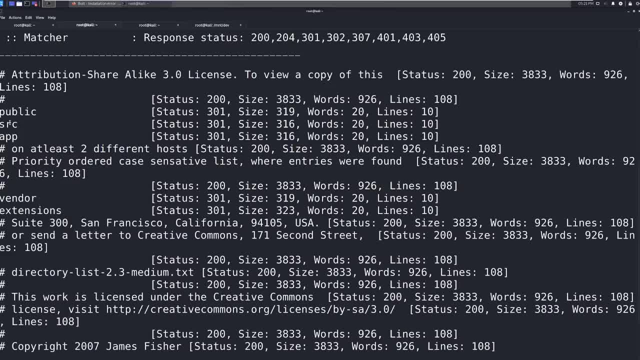 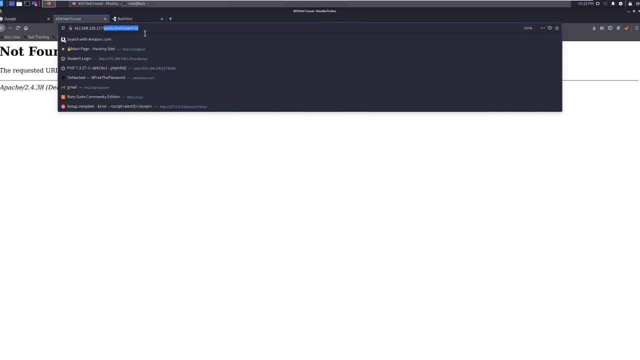 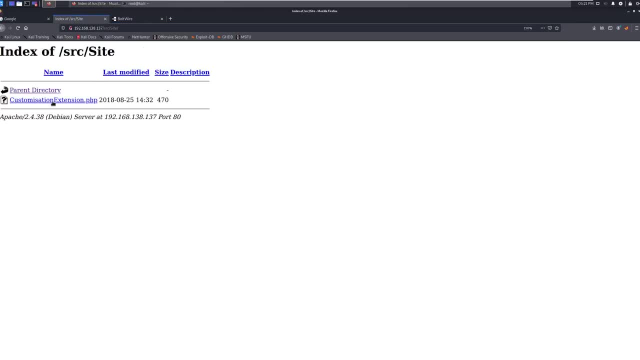 different directories that came back. Let's see, we have public source app so we can kind of go through those manually. just public, see what's there, Nothing's there. bolt user first. It says um source site. Uh, we get a customization extension PHP. 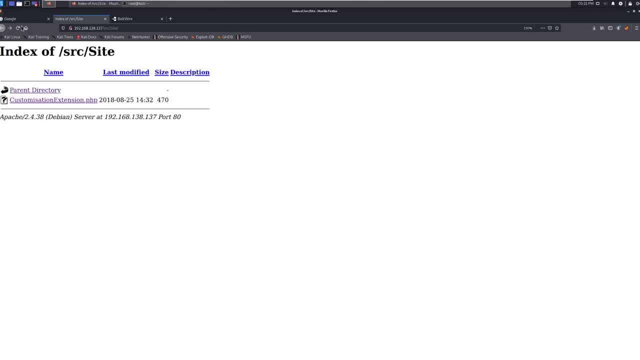 I don't know if there's anything in there You could open that It doesn't look like it's going to go anywhere. Um, next we go to app, kind of come through here, And this is where we find a directory, And I think I said in one of the past videos that it's kind of realistic. 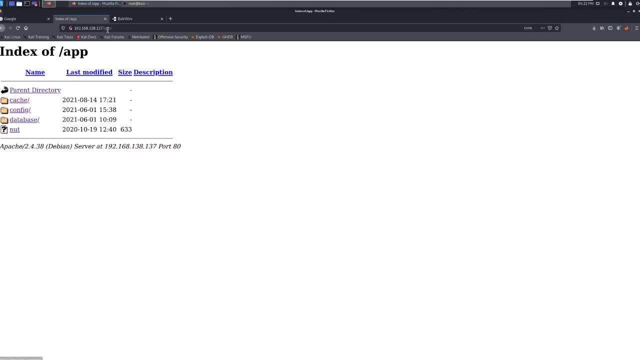 I have seen this actually on a pen test before, where you come across a directory and this directory listing can be a finding. Um, one time I literally came in here and the first thing sitting at the top of the directory was SQL database. Okay, 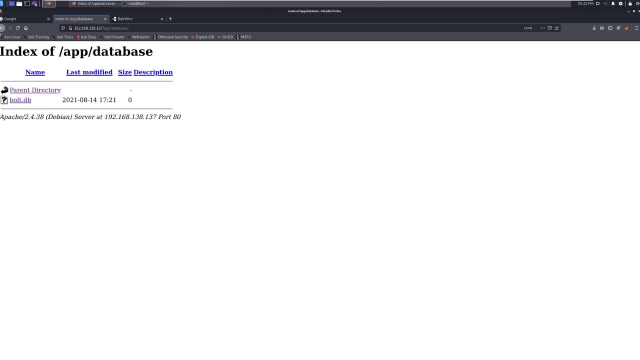 With all the passwords and information in here, So it looks like there's a bolt database in here, though The size is zero. Um, I clicked through here earlier, trying to click around see if I could find anything. um, cash is interesting, but config would probably be more. 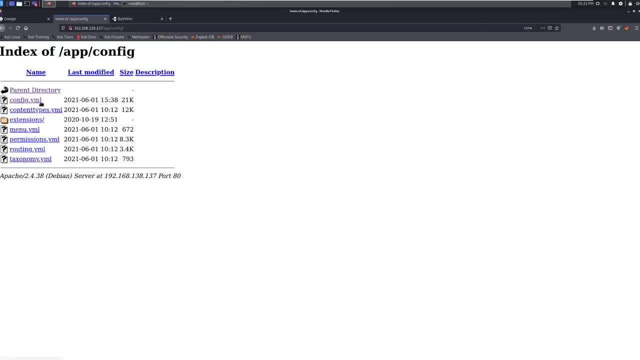 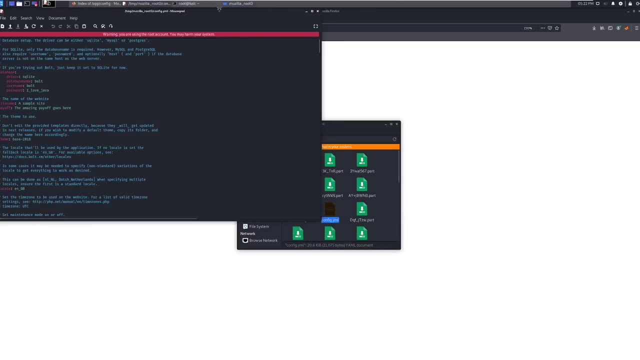 interesting, especially a config dot YAML file. So, um, I went ahead and just downloaded that and then I have it stored here. I'm going to go ahead and just open that up and I encourage you to do the same. Open with mouse pad, open with whatever you like here. 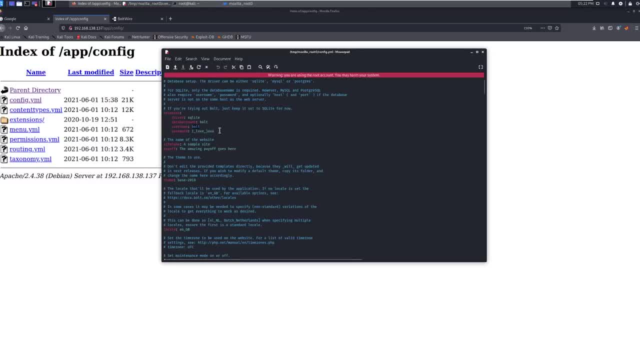 You can see that it says: Hey, the username is bolt and the password is. I love Java, So I'm going to copy this. We don't know where this works, If this works, if this pays off for anything anywhere, uh, but we're going to. 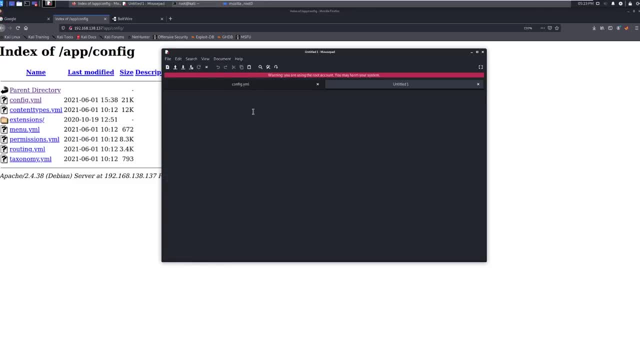 save this information kind of in our back pocket. So I'm going to do a new tab in here and just paste that Um cause, that's some information that we got. So the other side of things is that we also have Okay. 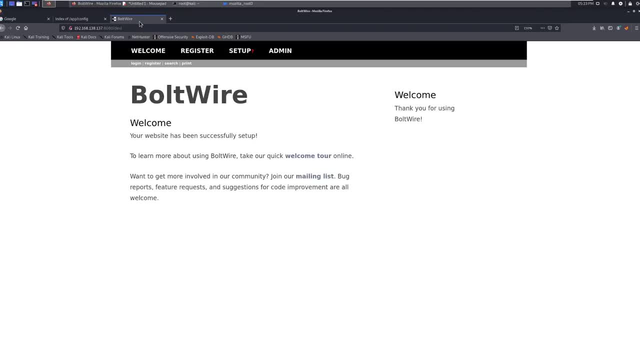 A bolt wire application and we can come in here and look around. It looks like there's a registration page. Um might be able to register like uh hacker and password hacker. come in here And uh, it doesn't look like it's letting us do anything else. 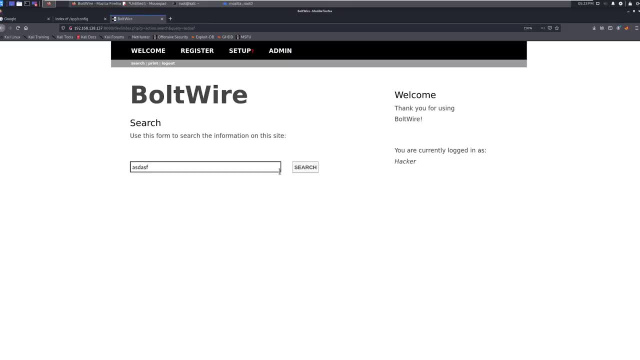 So we're clicking around. we've got some search features. Uh, it doesn't look like it's doing anything. print can print some information on the site, So it's best to click around and see if there's anything of interest in here. 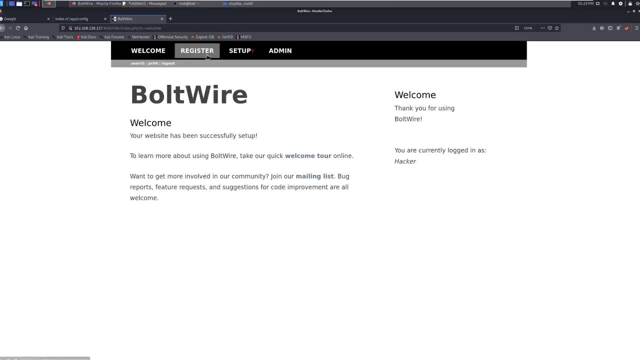 But I'm not seeing anything at this point in time of interest. Uh, so, as of right now, I'm curious as to this bolt wire, if there's anything, um any, any vulnerabilities that exist So we can go out to Google, um actually have Google open right here and we can. 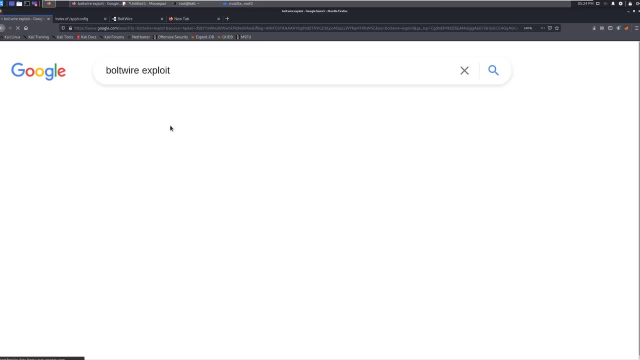 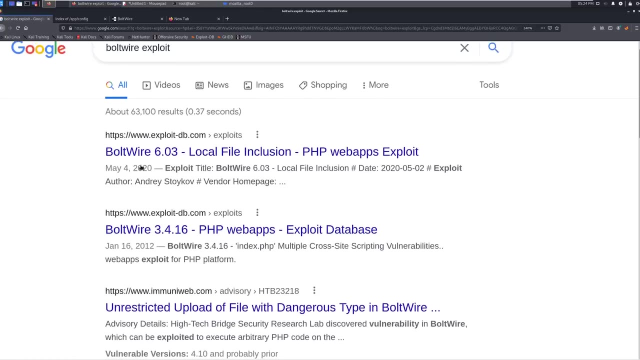 just say like bolt wire exploit and see what comes up. now there's one from 2020.. Uh, there's one from 2012.. I'm going to use the more recent one, this local file inclusion. We could also search this on our Cali machine, by the way. we can go in and 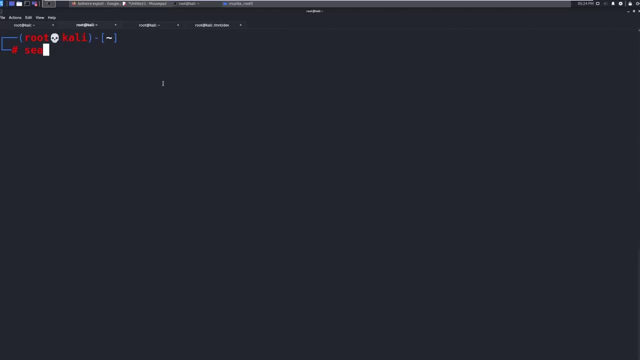 just do like a um, let's see we can do a search split and just do bolt wire and see what comes back, And you can see that all that shows up are multiple cross-site scripting, which cross-site scripting is not going to have any any effect for us. 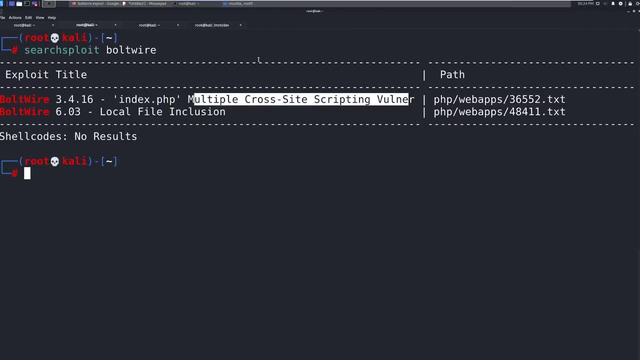 Like putting cross-site scripting here Isn't going to do anything on a box like this, unless they are, uh, from a from a CTF standpoint, unless there is somebody mimicking a user Going in and and actually navigating the website. 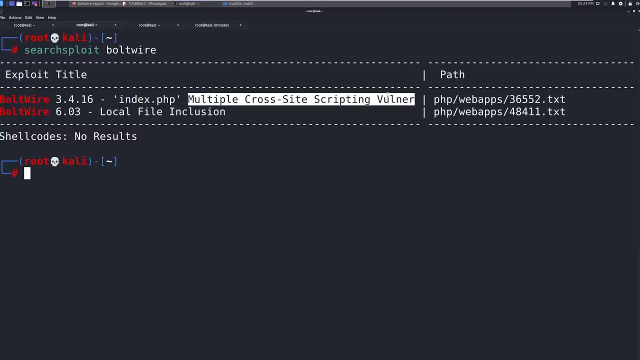 There's no use for even attacking cross-site scripting. That's not to say that this is not a great vulnerability And this is something that you you would see in the real world. You absolutely do, but we attack real users with this. 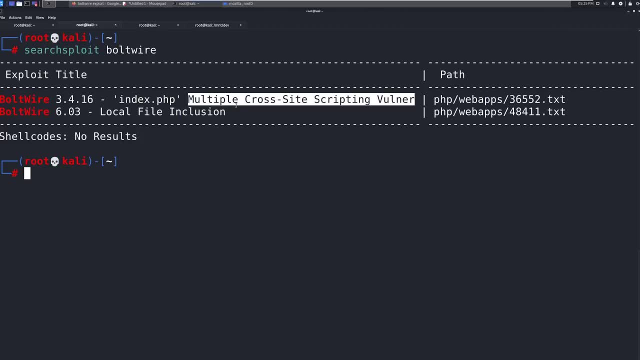 That's part of it, because you store cross-site scripting or you store JavaScript, or, and you attack users that we're not attacking any users, We're just attacking this box at this time. So what we're going to do then is probably really focused on. 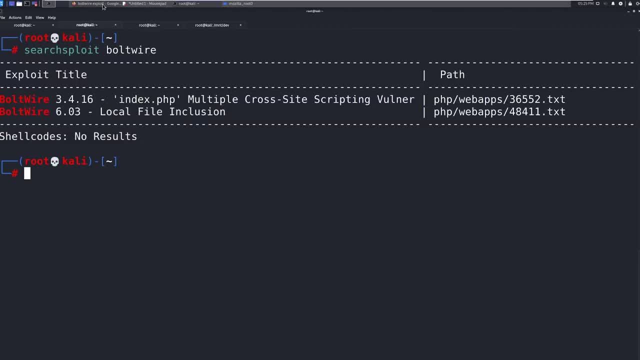 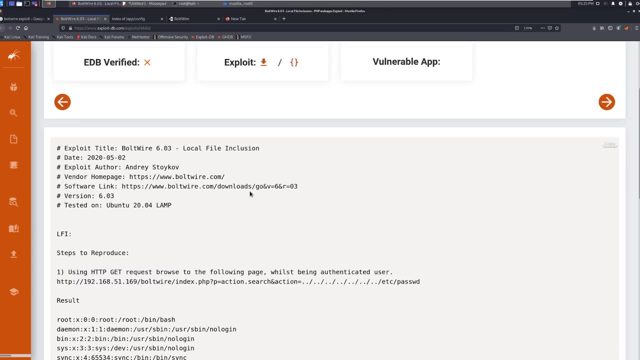 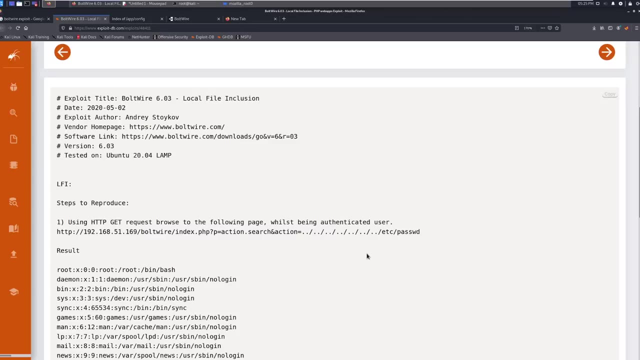 this local file inclusion. So Let's take a look at it And open this up. We'll talk about local file inclusion, what that is, what it might be. So, really quickly, Local file inclusion allows us to potentially expose files that are running on a server. 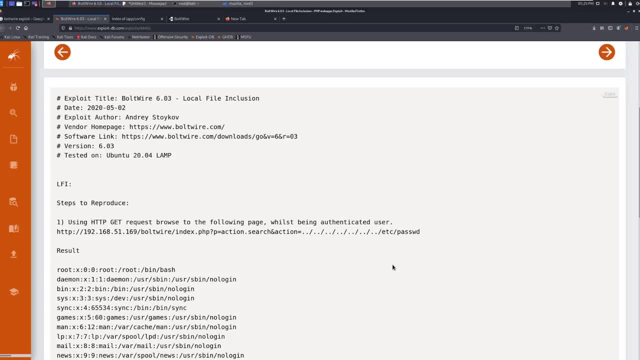 Um- and this can lead to information disclosure, as you're going to see here- remote code execution um cross-site scripting. There's a lot of things that it can do. So, basically, what's happening is it is accepting this path here. 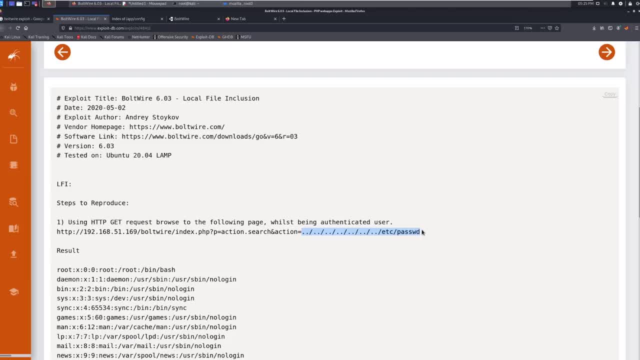 It has input. It's a coding error on the development side. So we're able to input this. and what we're doing? dot dot slash, dot dot slash. Imagine you're in a Linux machine. We're literally just saying: Hey, I want to go back as far as 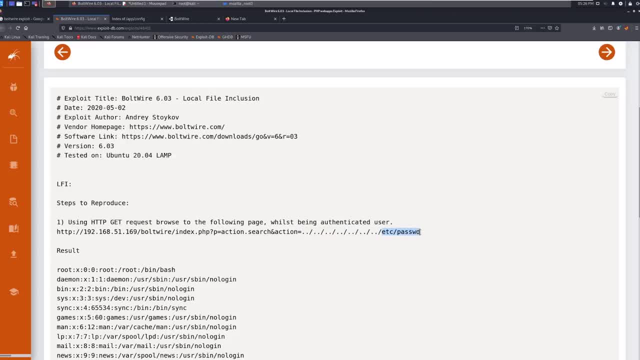 possible, to a base directory and then Etsy password. Okay, Um, so this could be as many directories as needed. You could throw in 10 of these and it might work. Um, and then we're trying to get the Etsy password, because this will allow us to. 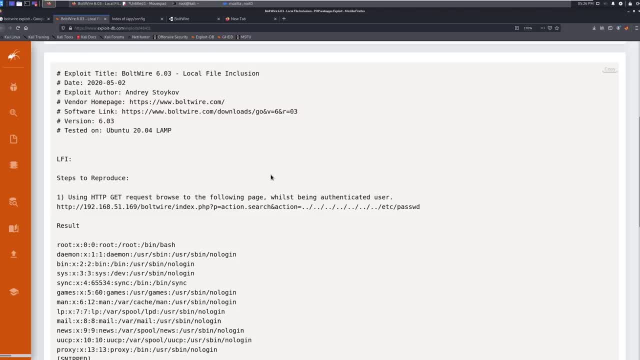 see who's on the machine running. Now, if this is running as a, as a um root user, then guess what? We can run this as a Etsy shadow and go grab the hash, And maybe we have even more sensitive information. but this attack by 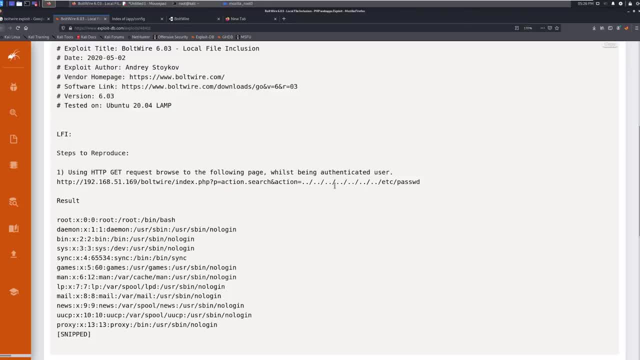 itself is pretty cool and is um. it's not seen in the wild as much, but it is definitely out there, So it's something we test for on every web application. So what we're going to do here is we're looking for local files. 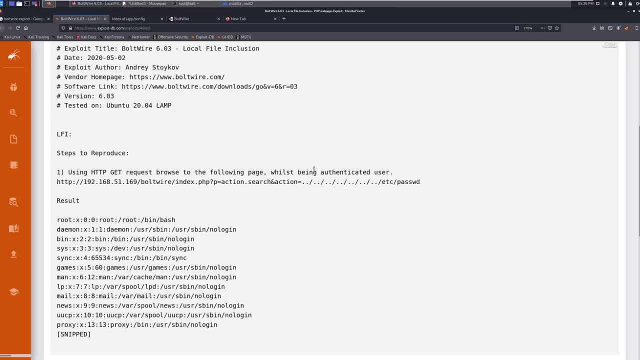 Remember this is local file inclusion, so, um, no remote files, which is Okay. The different type of attack: LFI here, not RFI. So it looks like we're using action, search action and then this attack frame here. 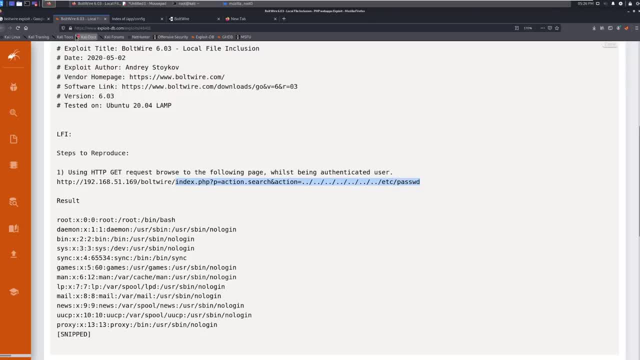 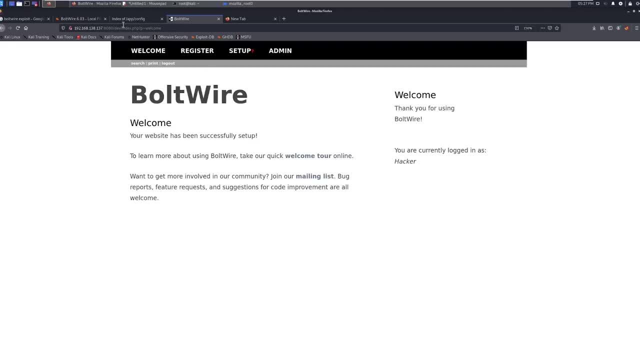 So I'm going to go ahead and just copy this. I'll show you why, Cause I was looking at the application and you can see that. here's the index that PHP: P equals. welcome in here. It's very similar: P equals action dot search. 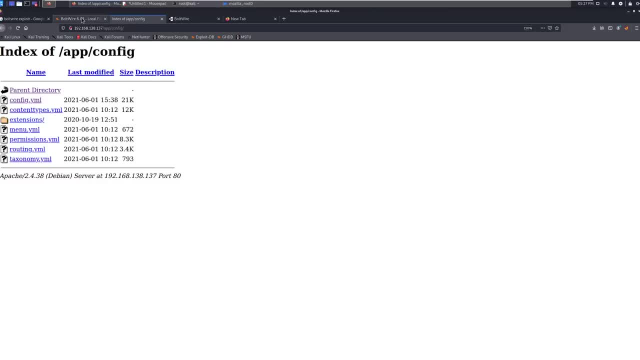 So this is on the search feature. It looks like it's happening um or on the action parameter, So we're going to go ahead and paste that in here. Make sure you've created an account, by the way, if you do not have an account. 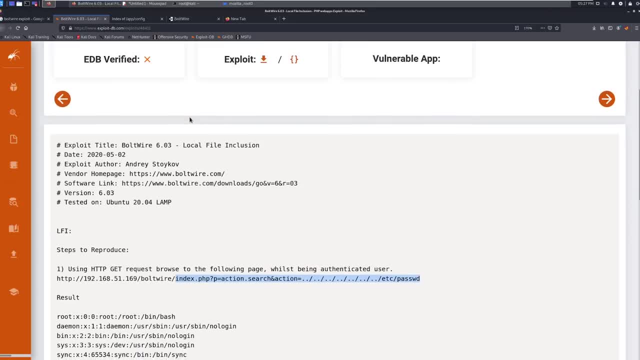 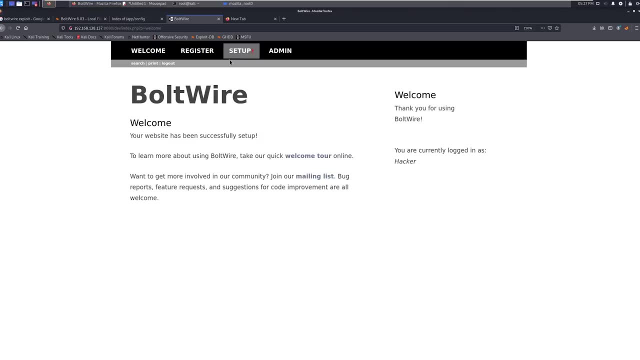 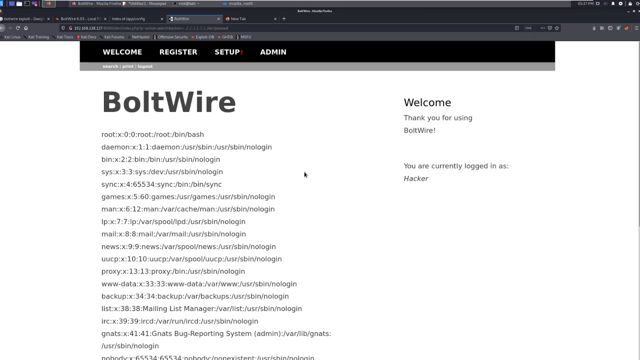 created for this, then it is not going to work. I don't know if that says that in here, that you need to be authenticated or not. Oh, it does being authenticated. So if you're not authenticated, it will not work. So you can come in here, just come over here and paste, cross your fingers and it works. 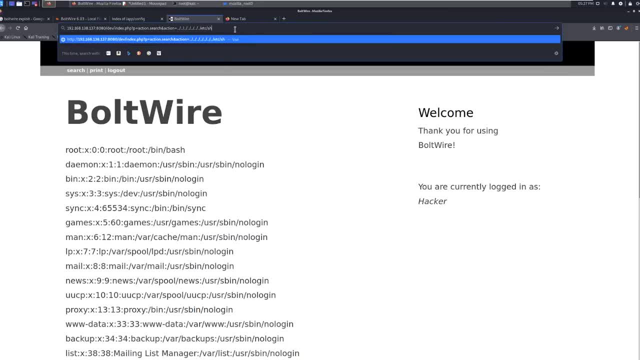 So one thing I want to try real quick is like Etsy shadow: nothing, It was worth a shot, You never know. So we're not running as a user that can read the Etsy shadow file, Um, so in this instance we're just looking at a user that can read the Etsy password. 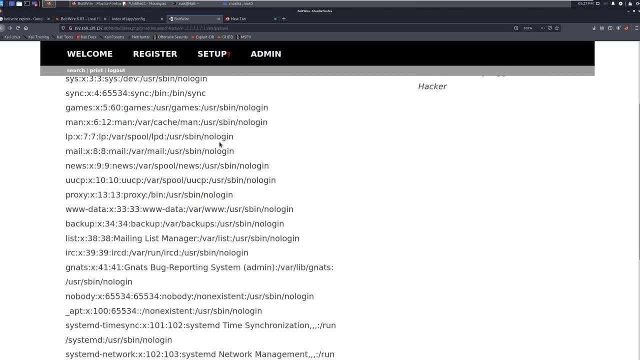 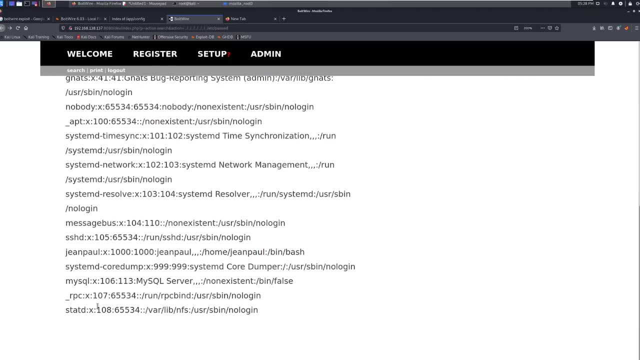 That's okay. We're not a high level user here And what we can do is we scroll down to the bottom. We always know roots at the top. scroll down the bottom to see who your users might be And out of anything that stands out in here, there's only one user. 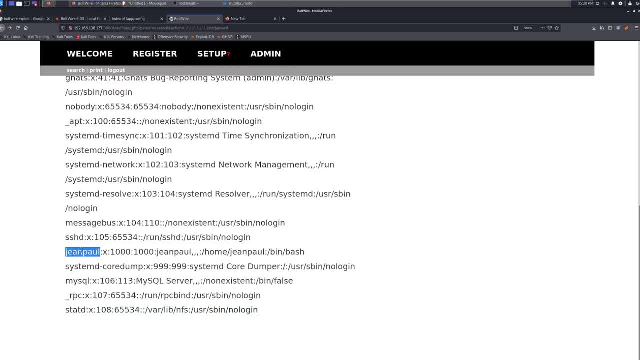 And that is our friend JP, who looks like his name is Jean Paul. Uh, so I think we have a user here. So this explains why the JP didn't work for us before when we tried logging in on the machine, because John Paul was the user that we had. 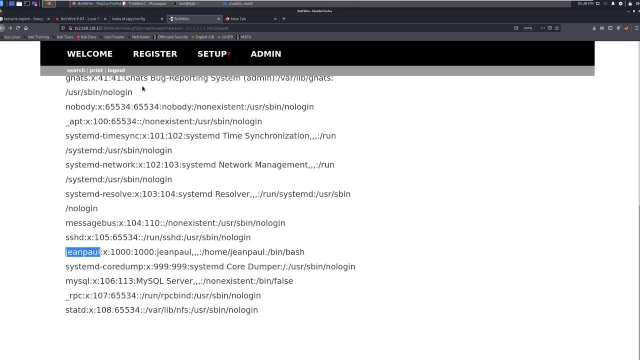 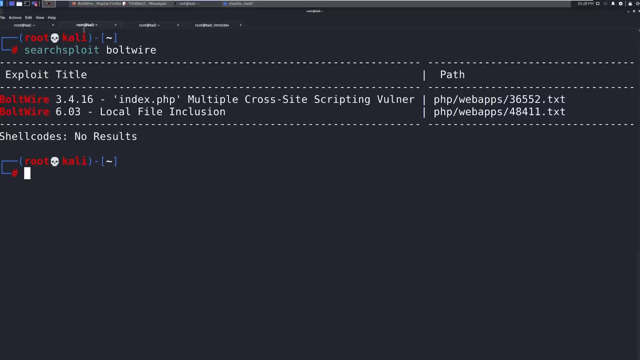 Um, and he wasn't on that machine, So we were looking for John Paul. So now we found a little bit more information and we can tie this all together, hopefully, and actually exploit this machine. So I'm going to go back. 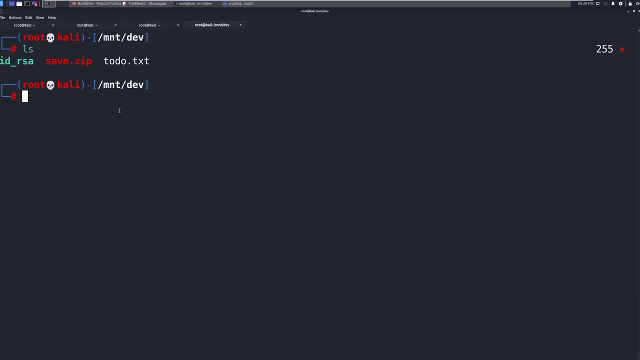 Where was the Mount that I had? Um, I'm going to go back in here and try SSH again with this file And do a John Paul And it's asking for a password key phrase. Okay, So there are two options that we can do here. 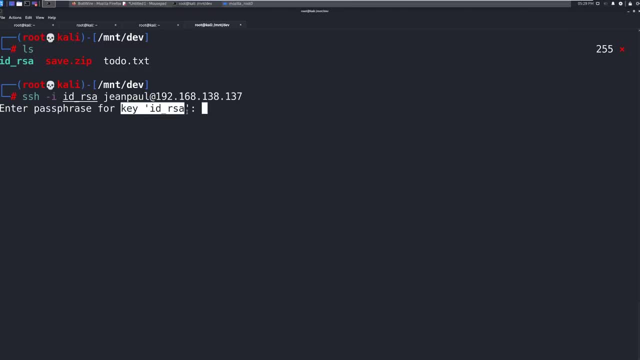 Option number one is: you are capable of brute forcing this uh key ID RSA. John the ripper can take this and push it through. The issue is, if the password doesn't show up in your word list or the password is uh too strong, for example, then it's a good idea to have a key ID. 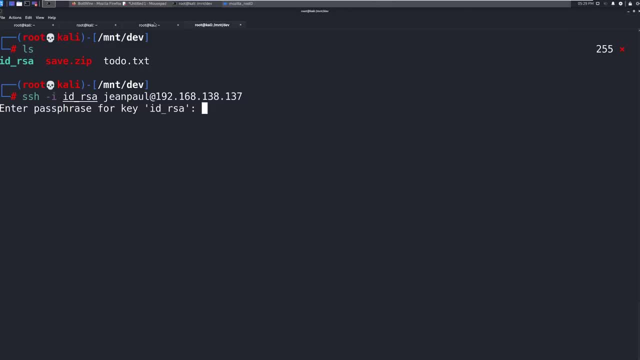 So let's show them. Okay, it's not going to work. We also have some information that we found before that might work out for us. We already know that john paul, or JP, said in his to do that he is a lover of what? 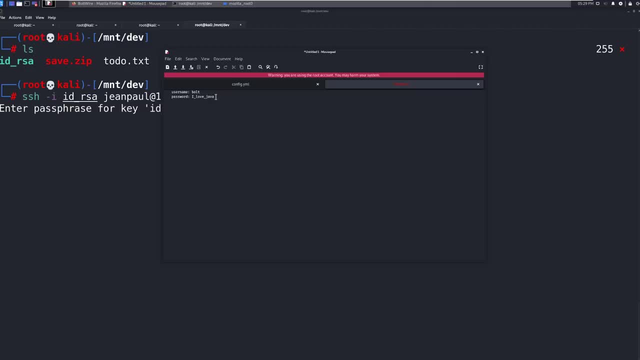 Java and he comes in here and we have a password saying I love Java. Now my hunch is: this probably doesn't show up in in rock you and we can do a quick check on that actually. So let's just do a cat user share word lists, rock you like this And you can just watch, and then we're just going to. 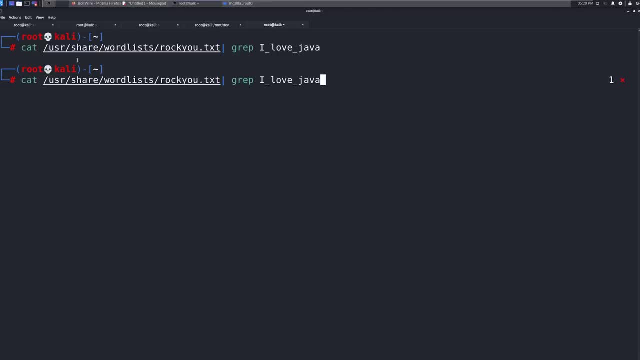 grip on this password, It doesn't show up like where. if you wanted to grip on like pasta, You can see all the different times pasta shows up in this, in this word list, So that if we were to run rock you against this with the word list, it wouldn't have worked. Now if we would had a 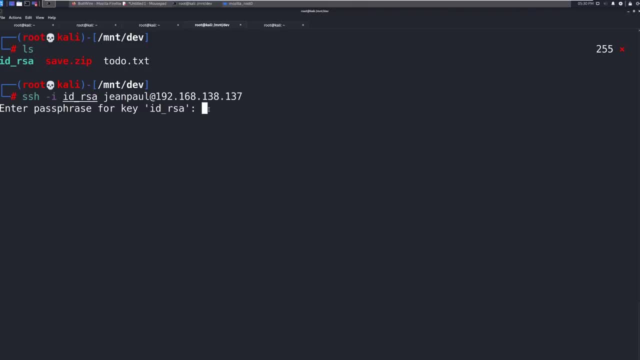 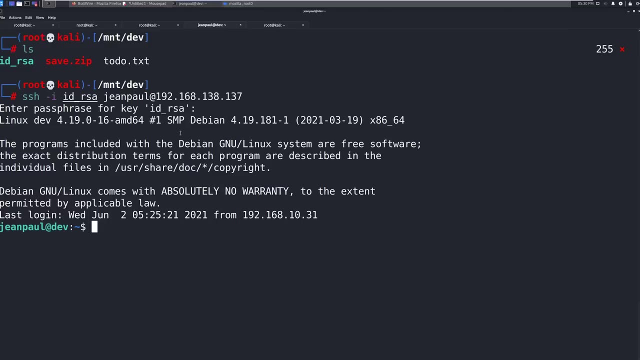 really good word list. possibly it shows up, But we already know a little bit about him. we're going to go ahead And try pacing that in And of course it works. john paul really loves Java, So john paul at dev. 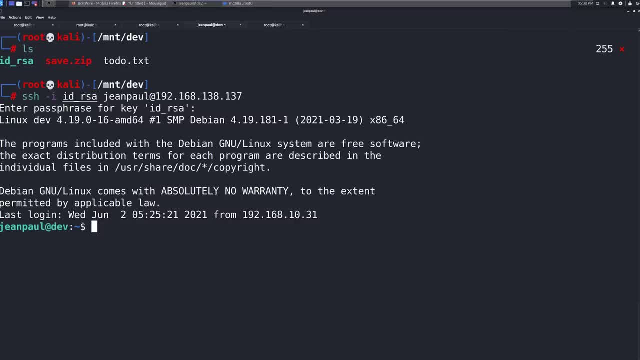 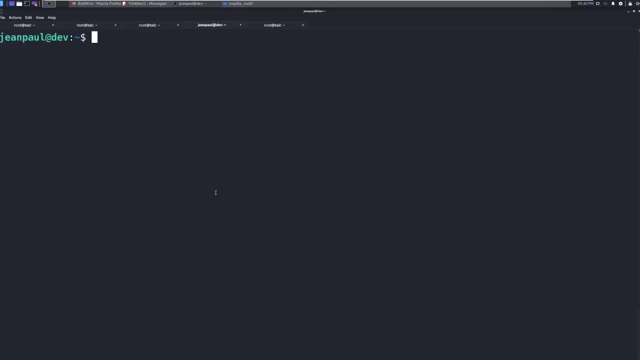 has logged in, And now we are. we are the low level user, So do a quick LS print: working directory. we're in his home folder. there's nothing here. Some things that I like to do immediately: history check. Okay, it looks like somebody cleared out the history. Somebody ran. 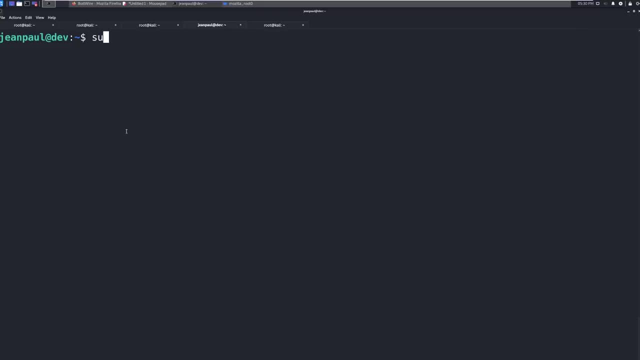 a sudo dash L in here exited. sudo dash L is the second check that I like to do, or even first check like do, because it tells us what we can run as sudo without a password. Okay, so sudo, remember, is what we can run as elevated privileges. 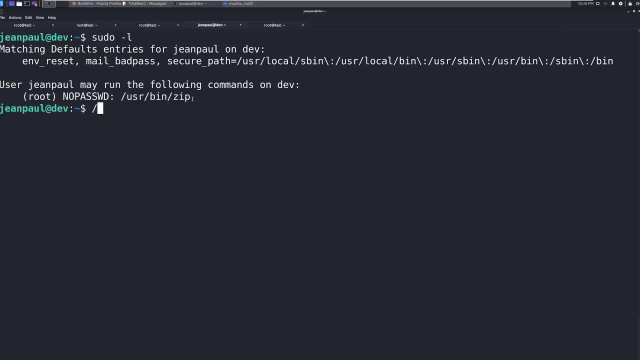 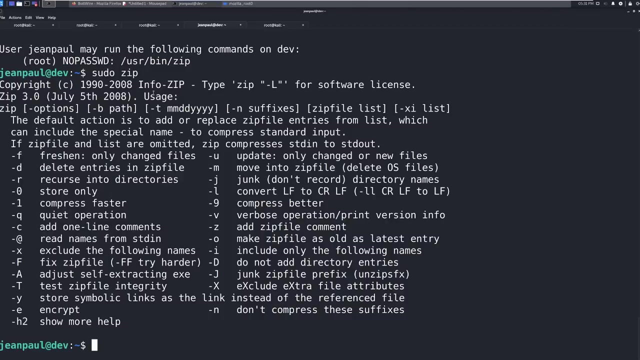 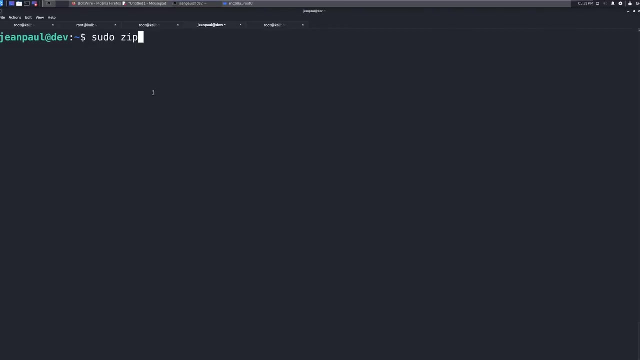 So in this instance we can run the zip feature with with no password. So we can literally run sudo zip and should work. Okay, so it's not requiring a password. Awesome Issue here. Wow, how can we take sudo zip and abuse that feature for us to be able to? 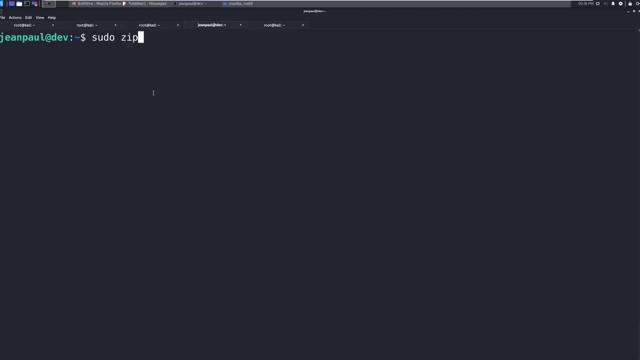 escalate into root. That is the question. if we have a no password- which this comes up a lot in boxes like this, like CTF style boxes- If we have a no password, how can we do this? So we need to go take 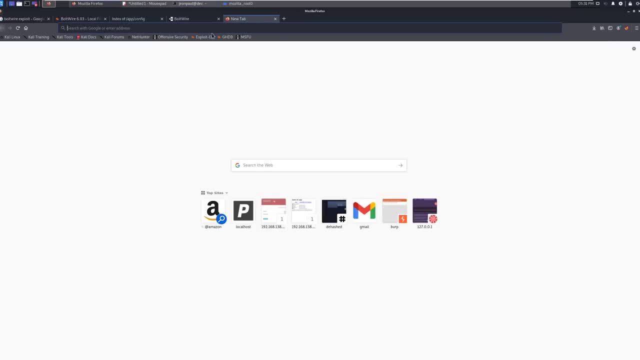 a look at that. We come over here. I got a site for you. go out to the Google machine, Okay, and you're going to type in GTFO bin, just like that. It's really GTFO bins, but we took what showed up first. 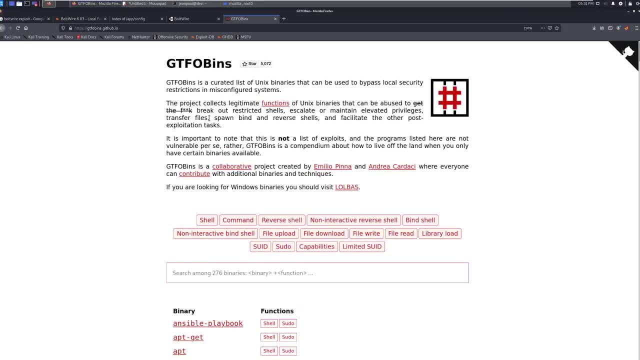 Okay, GTFO bins- Great website, Let's make it bigger. Great, great website. you come in here you can look for the different type of escalations that you want. We have a sudo escalation- Okay, sudo escalation. And we come in here we say, okay, we've got sudo, And then we're looking for Zip. we 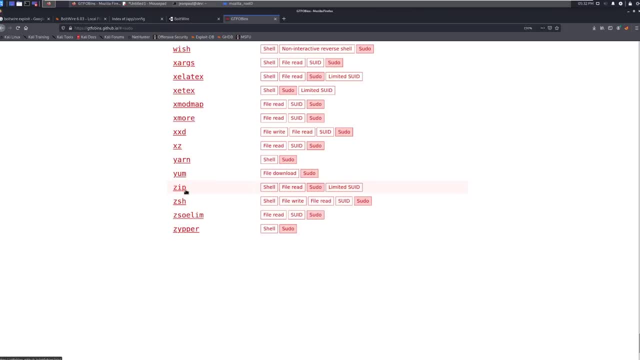 can come. we could type in here at the top and you'll be able to scroll down. So why don't we go there and zip in the search bar? but we also have zip right here. so if we want to do a pseudo zip, we 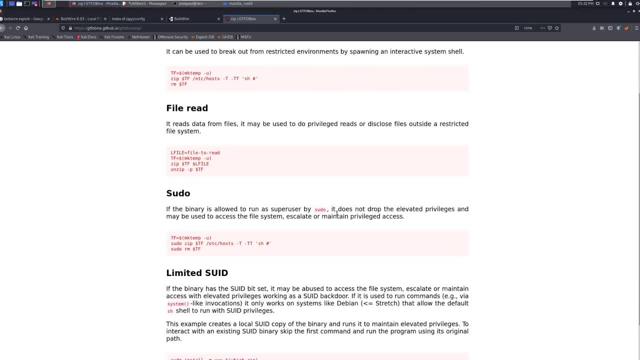 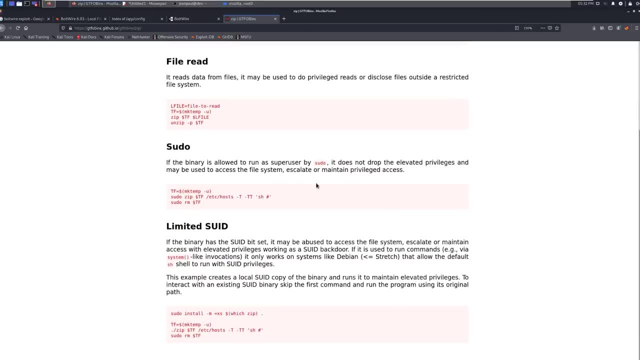 go into zip, look for sudo, and it says here's how you use sudo as a zip in order to get a, in order to get root privileges, okay. and so it says in here: if the binary is allowed to run as a super user by sudo, it does not drop the elevated privileges and may be used to access the file. 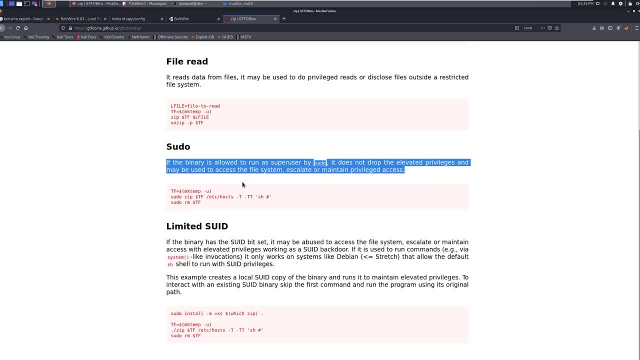 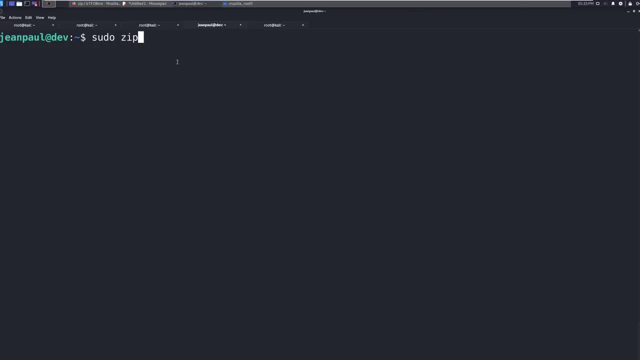 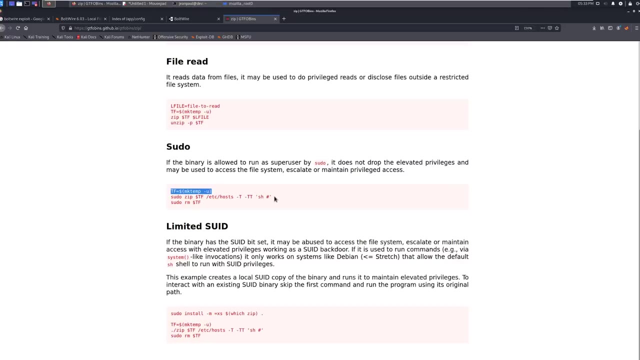 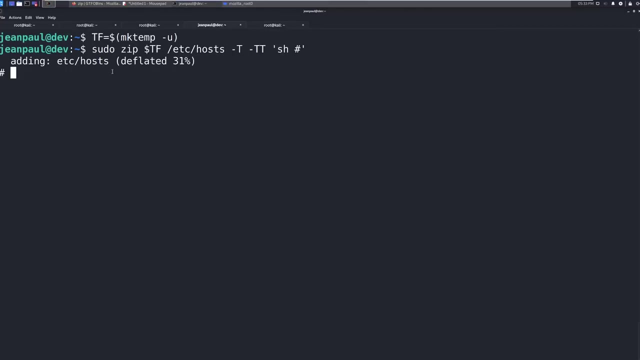 system, escalate or maintain privilege access. it's telling us what it's doing. all we have to do here is copy this. come over, paste this. okay, come back, copy this. this should drop us into a shell. this should drop us into a shell. let's see what happens. all right, we have been dropped into a shell here as sudo. 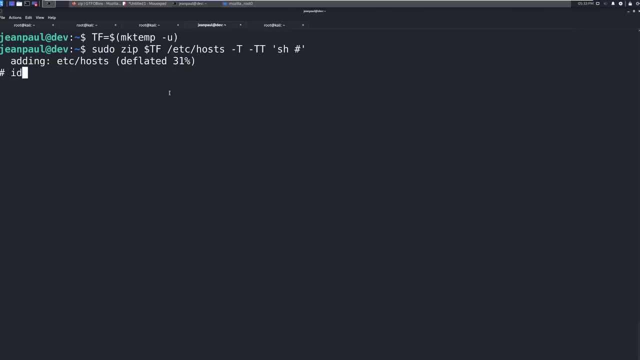 we dropped into a shell. so with that we type in id. we are now root. why? because sudo runs elevated. we said, okay, as elevated user, we want to go ahead and drop into a shell here. we did this. now we can go cd to root ls- cat out our flag. 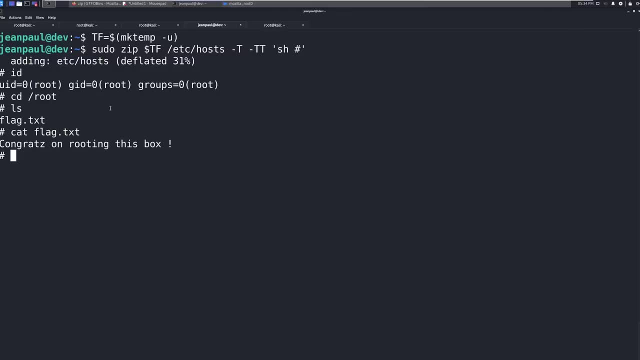 congrats on rooting this box and that's it so. hopefully that was informative for you. this was a fast-paced video. we'll rapidly get to more bugs and tests as I approaching future glitch times. if you have any questions, please press the subscribe button. be sure you are subscribed. 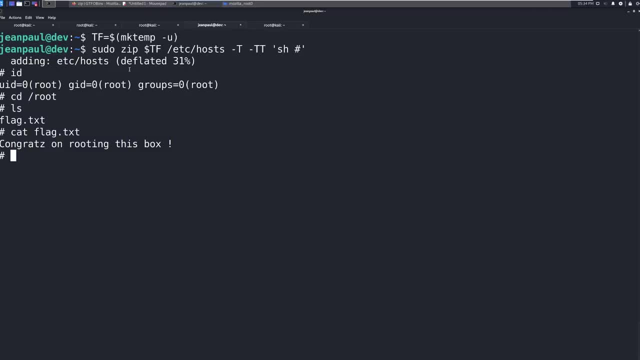 i think that goes a long way. so thanks for continuing to watch this video. leave a thumbs up, click, select, comment and nonebutton and i'll see you next time. next time, all right. so let's get started with test on the, i would say, easier side of the machines. we're 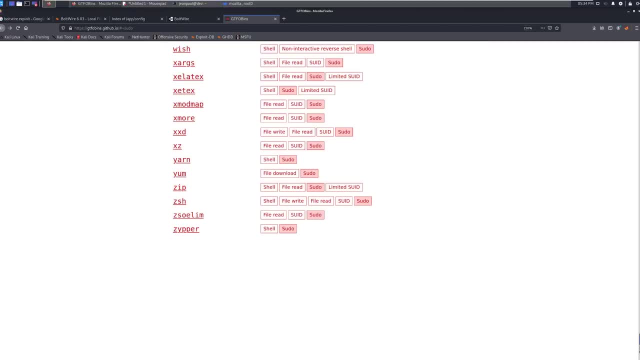 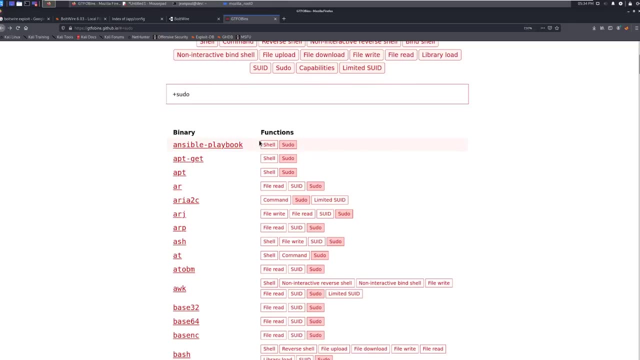 trying to go in order of difficulty. this one is something that you you get a few different options, escalations, if pseudo privileges are enabled- in order to get into, to go from low level to root. So it's quite fun and quite common, by the way. So that's it for this video. I will go ahead and 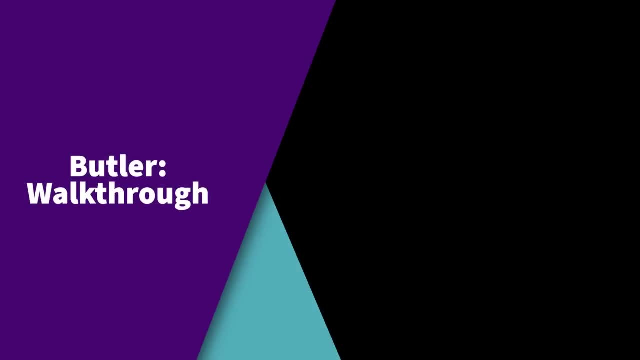 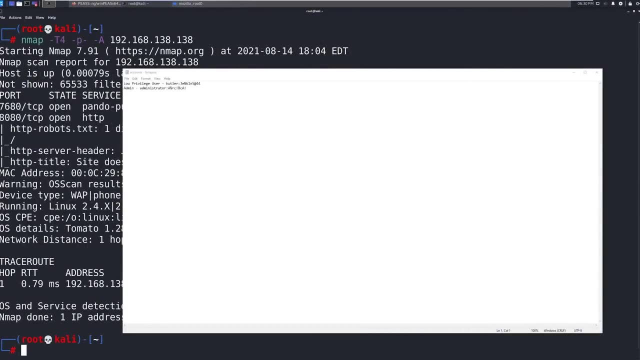 see you in the next one. On to the next machine, which is Butler. Now, Butler was created by Joe Helley, aka the mayor. Thank you so much, Joe, for creating this machine for us, And this machine is going to be a Windows based machine that is going to allow us to explore privilege escalation, since 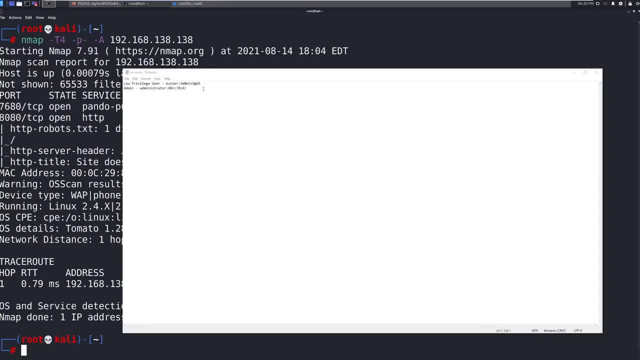 when we first used blue, blue went right to root for us, So this one's going to give us some experience with privilege escalation. Now I have this accountstxt file open, just to show you that the administrator password for this one's a little bit different than the other Windows machine. 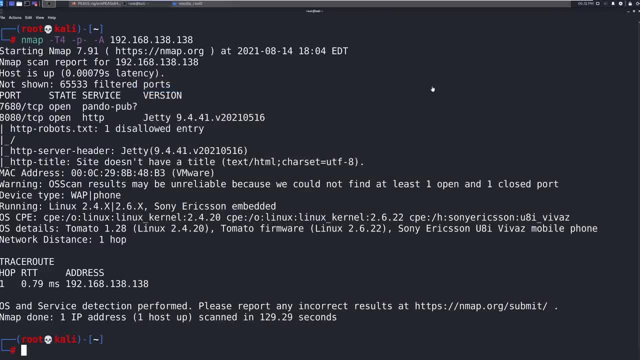 This file is included in your, your download. So if you downloaded this, you've installed it. you should have found the accounts. That way you can go and get the IP address that was pulled from this machine. So with that out of the way, I went ahead and ran and map again. 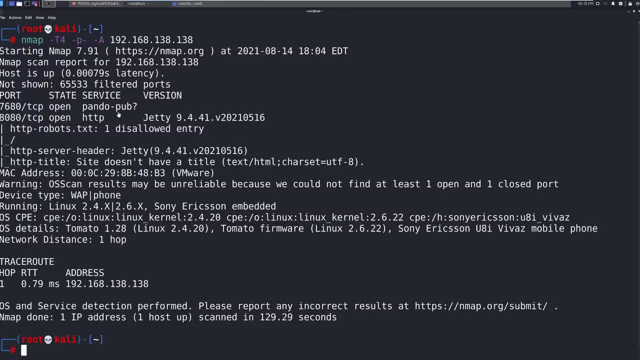 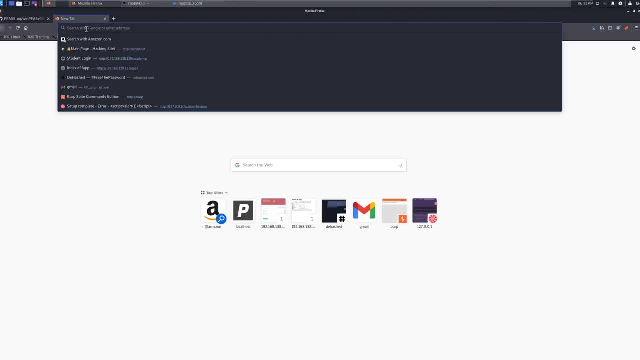 similar process. Now here we have 7680 open and 8080 open. I'm going to go ahead and you can ignore that for now. I'm gonna go ahead and go out to the website 168138.138.. And we're going to see. 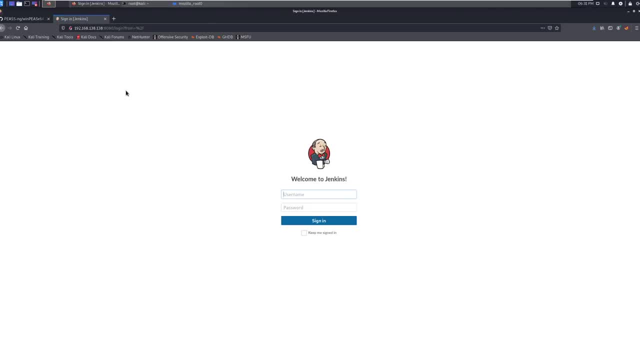 if it would help if I put 8080 on the end of it. we're going to see what's there. Okay, all that's there. And if we go ahead and click on the download, we can see that we're going to see. 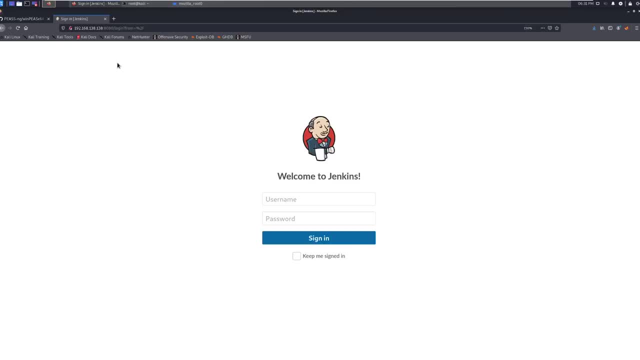 that we've got the same page for Jenkins. So we don't we don't have much here yet. There are a few things that we can do here. we can try to do some brute forcing. we can look for directory busting. we could try to do a view page source real quick and see if there's any information in. 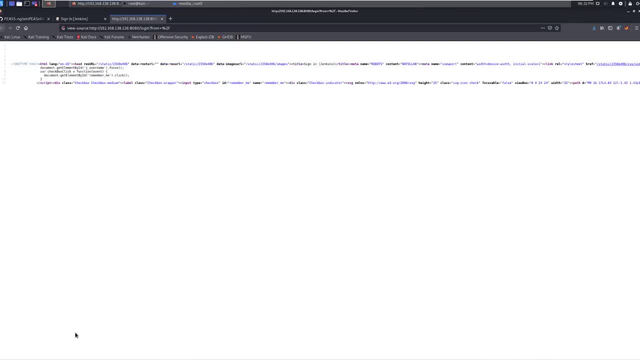 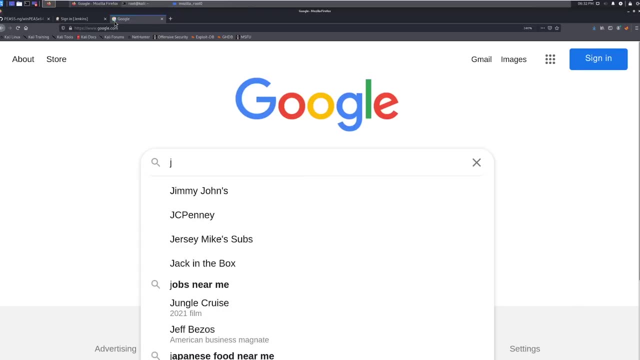 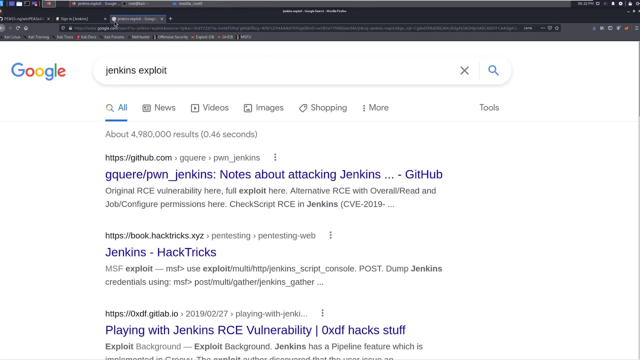 here that might indicate what version we're running on and see if there's anything in here that we can get maybe an exploit off of, And really there's not going to be much. we could go to Google and do a quick Jenkins exploit and see if we can find any sort of Jenkins exploits. And there's this here about. 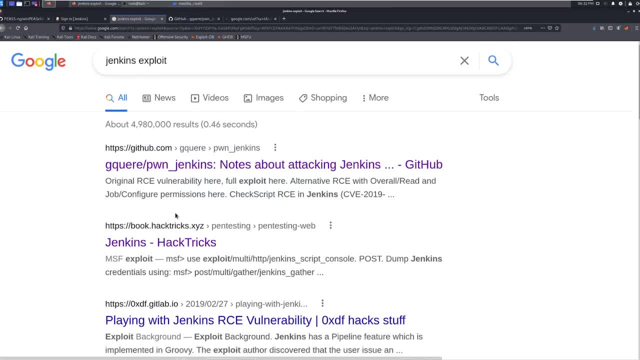 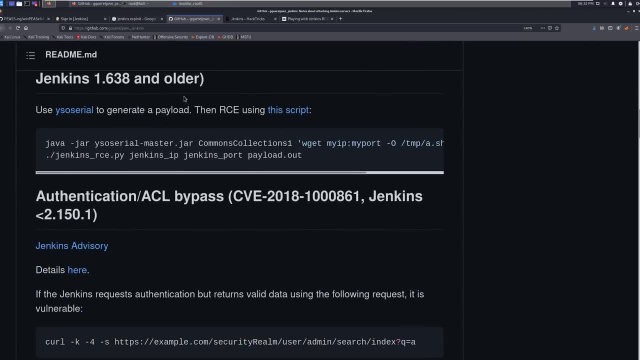 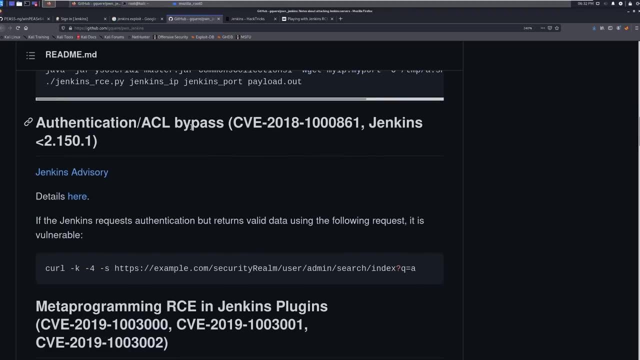 attacking Jenkins. there's one here about attacking Jenkins. this one has remote code execution And we got to click through these and see what we're looking at for this. So it looks like 2015 Jenkins has some deserialization attacks. 2018 had authentication bypassing. 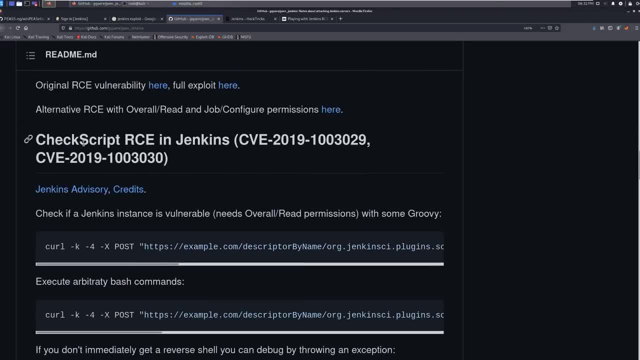 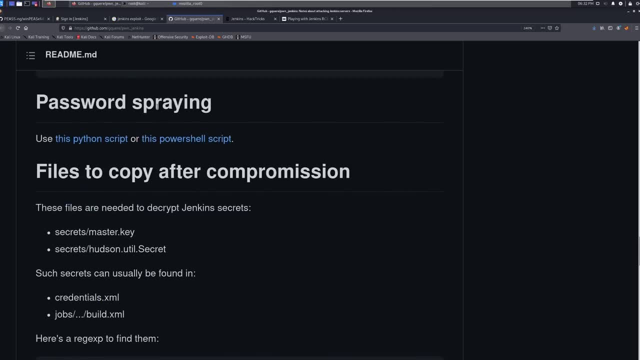 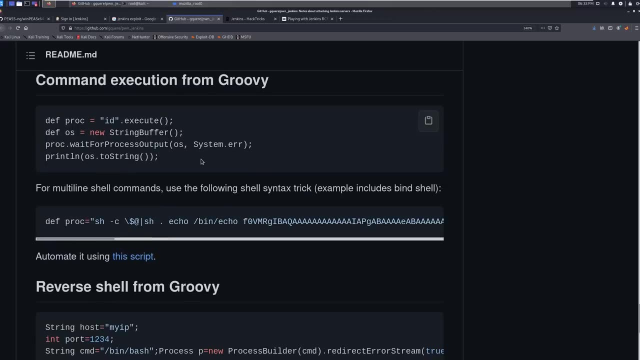 And it looks like. let's see, we've got check script, remote code execution. there's a lot of different looks like attacks in here. there's some password spraying that you can do against this, which we'll talk about here in a minute- dumping secrets, groovy scripts, reverse shells. 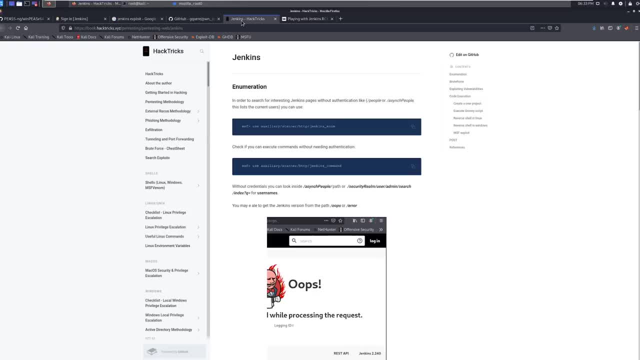 with Groovy. Okay, so there's quite a bit in here. This one is a little bit. let's see if it's the same or not. This is saying: hey, here's how you can create run indexes on heures. Let's see what this thing says. there's a lot of stuff to do with this. This is saying: any event manager needs a design. 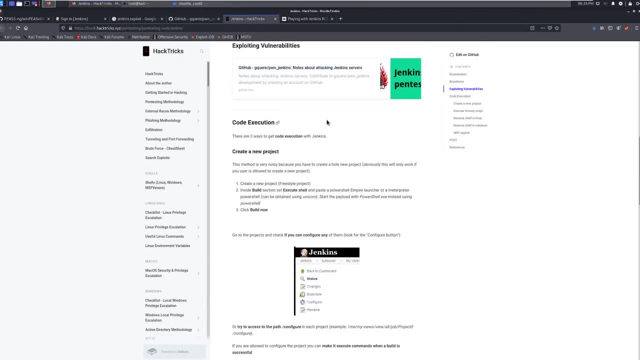 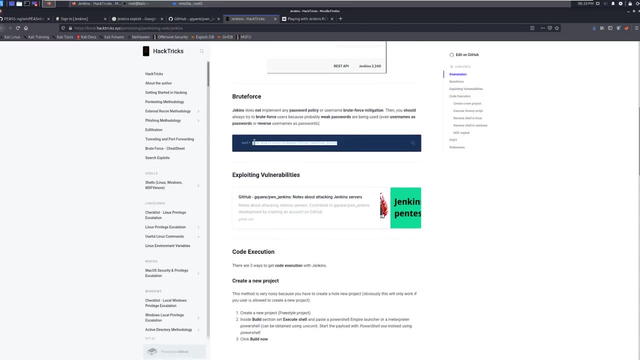 the same or not. This is saying: hey, here's how you get code execution. there's three ways to get code execution, which, ideally, we want code execution. we could do some brute forcing here, but I'm going to show you a way to do brute forcing without having to do this. 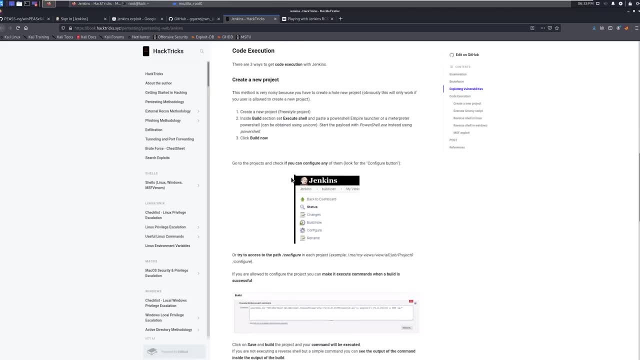 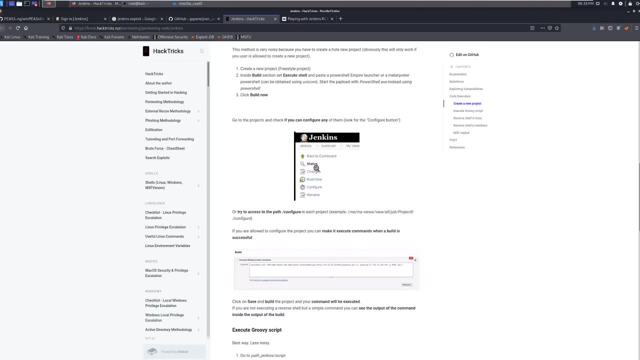 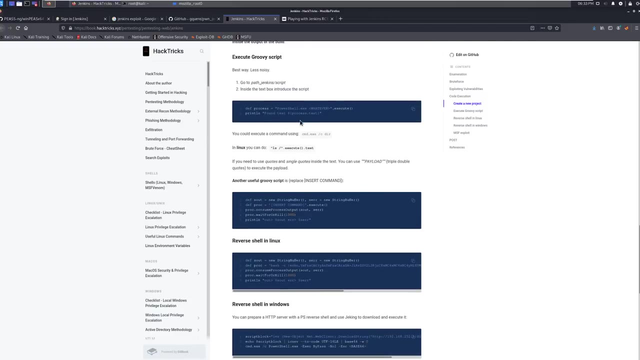 We can do some remote code execution And it shows: hey, there's a few different ways to do it. In this instance, we're going to need authentication. There's no way around this for using Jenkins. we need authentication to get in here, So it's it's pretty neat. 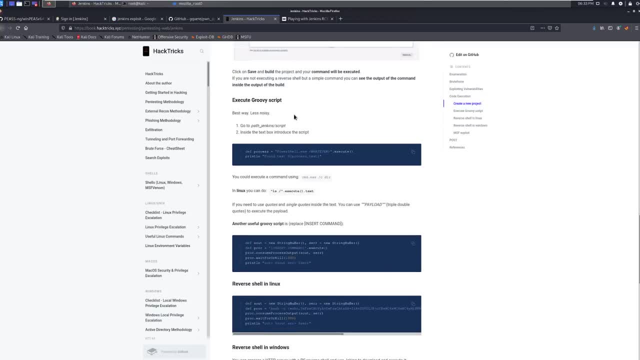 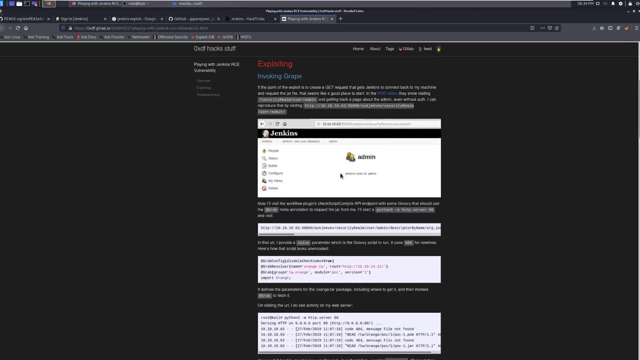 They're show you a few different ways to get this exploit, And everything's pointing back to groovy, or it looks like there's a PowerShell way of doing it, which is neat. This article here tells you: hey, when you're logged in, you can log in, and it shows you how to attack this. this looks a little. 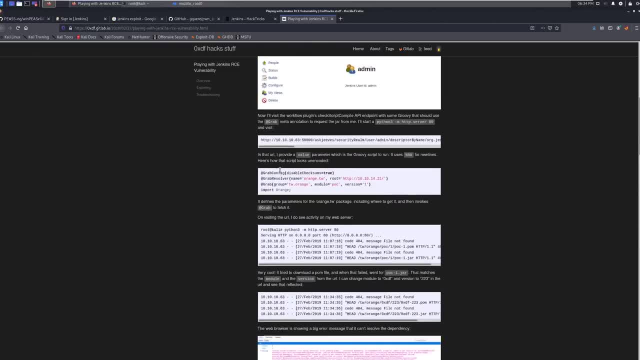 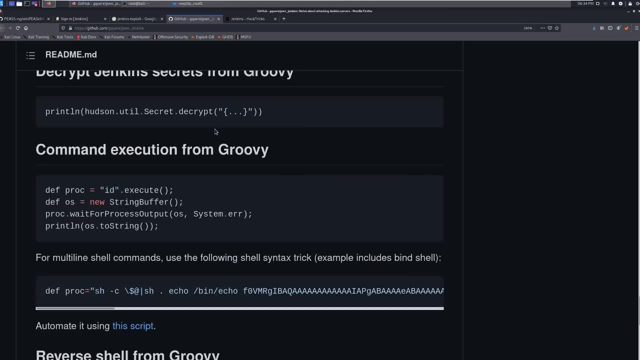 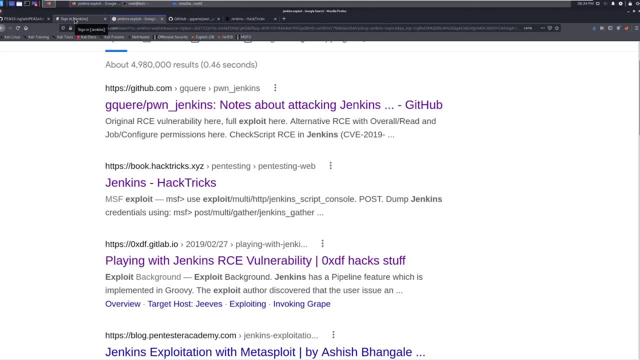 All signs so far are really pointing to authenticated attacks. There are some here that are older that looks like they're bypassing authentication Just to save time and skip ahead. we're going to go ahead and avoid those, though it's not out of the realm of possibility that you explore those. 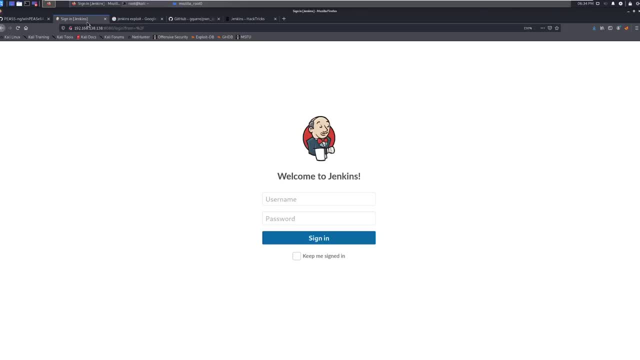 go down these rabbit holes, check it out, see if there's any sort of attack that you can exploit here. So our main focus is: how do we log into this application? we haven't found any sort of version yet, So we're going to go ahead and log into this application And we're going to go ahead. 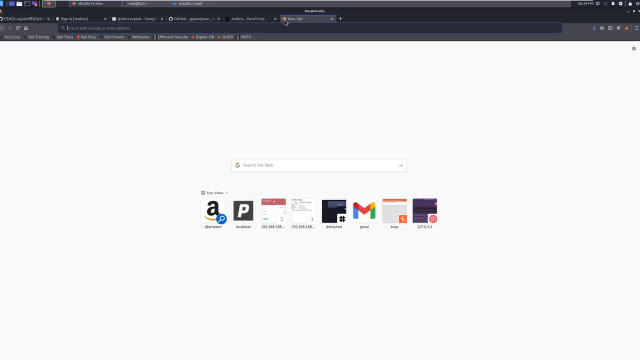 and log into this application. we haven't found any sort of version yet, So we're going to go ahead and click on update, And then we're going to click on also new, but we're going to go ahead, and The other thing that we can do is we can go to Google and we could say: Jenkins default password. 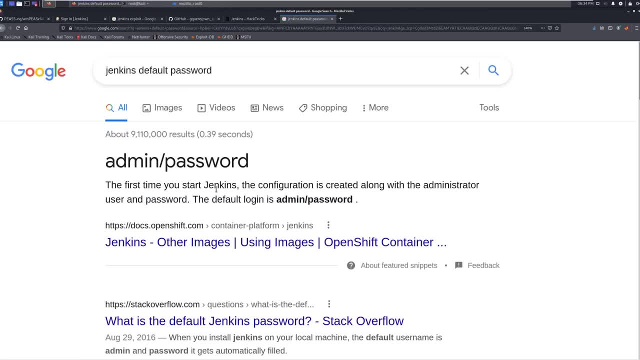 And it says the default password is admin password, which is what's created the very, very first time you log in. I think it asks you to change it once you log in, though I am not 100% confident on that- And we can come in here and try admin password. And we're gonna see that doesn't work. So we're gonna go ahead and do that And we're gonna take our password and we're going to go ahead and go on and we're going to click on add password And we're going to go ahead and do that And we're going to click on update password. 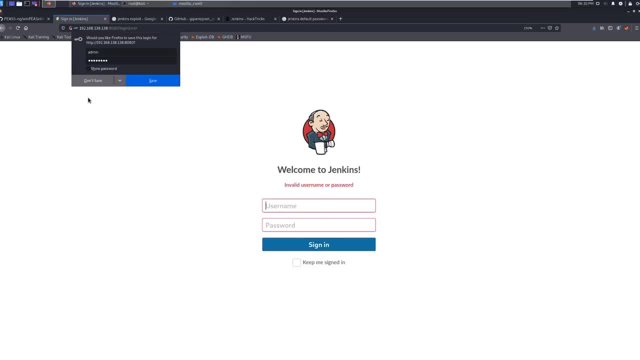 and we're going to see that doesn't work. unfortunately, we don't have default credentials here, so uh, we do have. we have the possibility of doing some brute force directory busting on this. maybe there's a configuration file or something sitting on the back end that we can get access to. 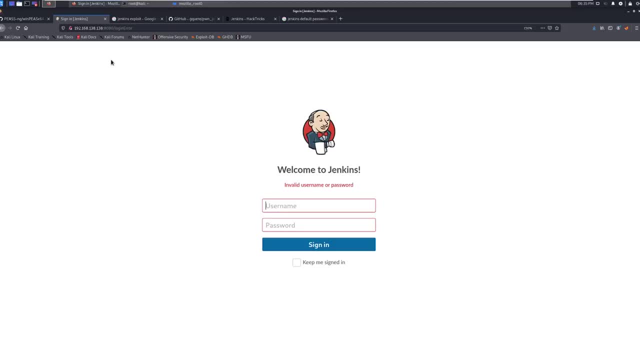 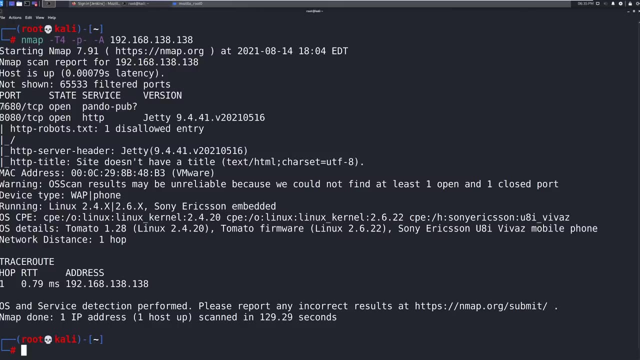 i'm going to tell you just to save time. that is not the case, though. if you're thinking through that methodology or that mindset, that's fine. i think that's okay. the other option is this port here, this 7680. we could try connecting to this. you can use netcat, you can use telnet- there's. 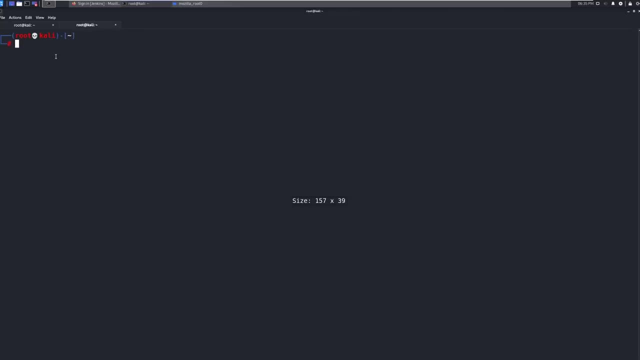 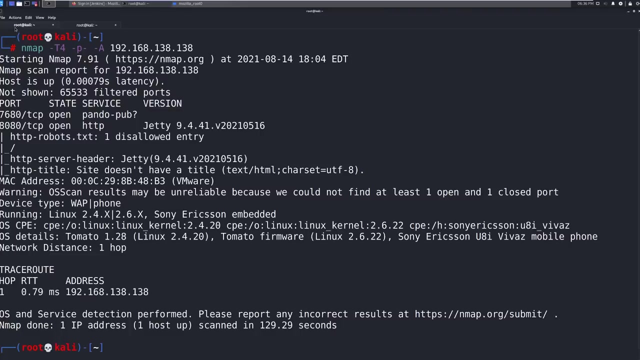 options here where you can try. for example, you could try telnetting, but you could do apt install telnet, because it doesn't come by default anymore, and then you would just go telnet ip address: 138, 138 and then that port number, which would be 7680, and you could see what's listening on there. 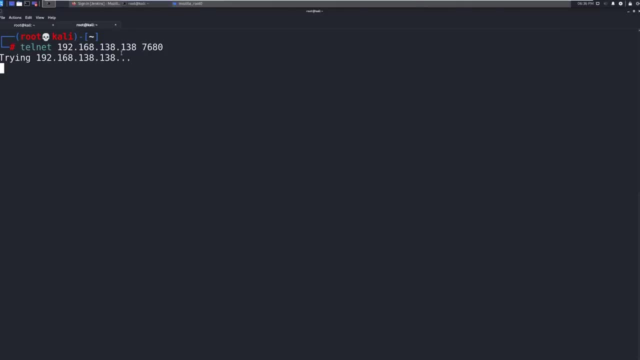 this is a. this is a. this is a port. it's trying, it's not connecting. it's one of those weird ones that you don't really see that often and i'm telling you from my experience, i don't see that often. you can go out and google. 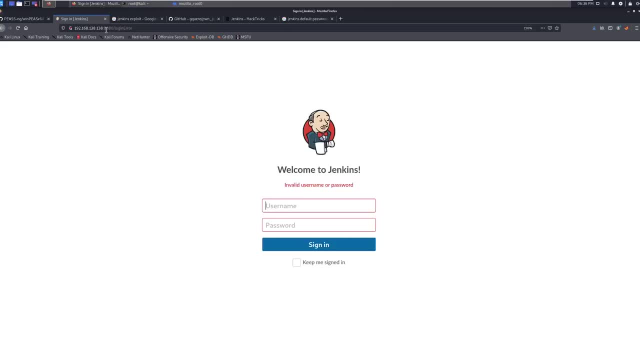 hey, what does this port do? you could also go and say: hey, i know this port's open, so i'm going to go ahead and just try 7680 here. that's going to stall out. it's not a web address either, so we're running out of options on how to actually connect to that. that could be a false positive that it. 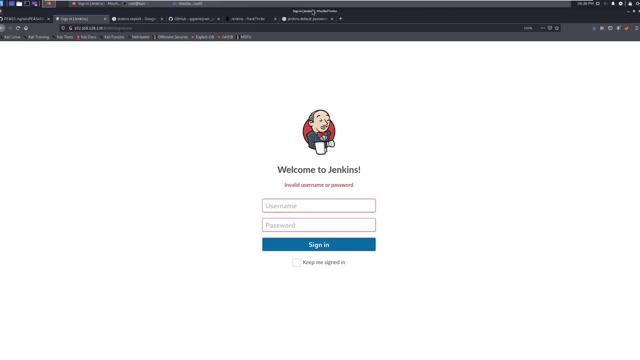 could be a false positive that it could be a false positive that it could be connecting into that machine. so, with that being said, we need to brute force. jenkins, now you saw metasploit had a module. somebody showed that in one of these we're going to do it, the burp suite method, because that's my 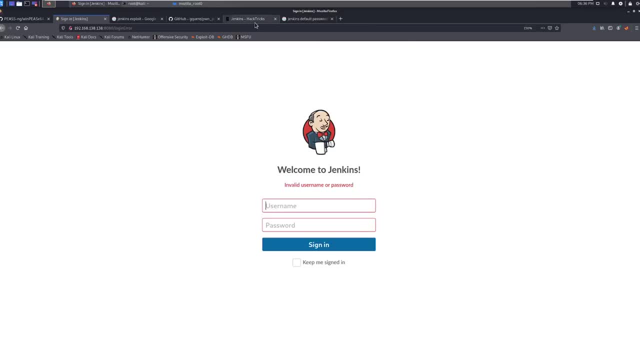 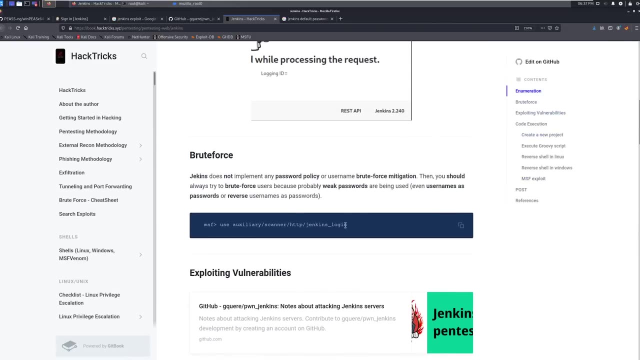 favorite go-to and i'll show you the burp suite method. if you want to play around with some of these other methods like that's shown in here- sorry, i'll make this bigger, but that's shown in here- feel free to go use this and metasploit and see if you can. you can brute force passwords. 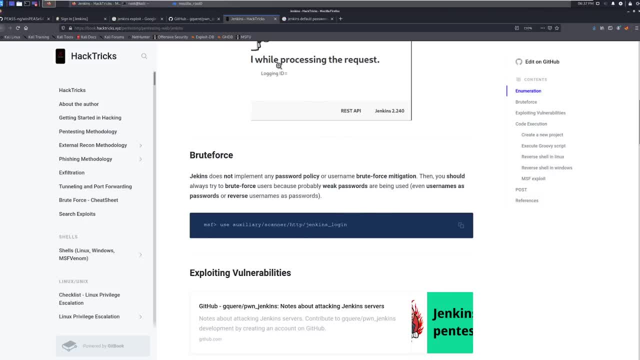 usernames, etc. but from here, what we're going to do is we're going to do a couple of things here. at do is we're going to use burp suite. So I'm going to use a tool called foxy proxy, Since we're in 2021, I'm going to go. 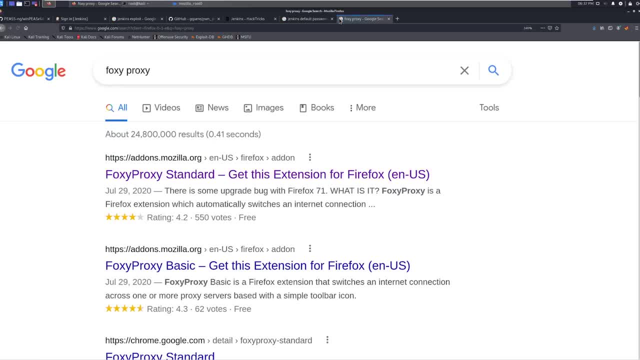 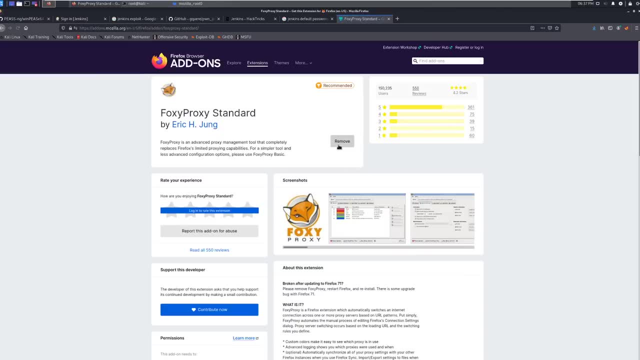 ahead and show you how to install this. Just to get this up and running, If you just type in foxy proxy, literally go the first link you get with standard, go in here, hit install. mine's already installed, So it's going to ask. 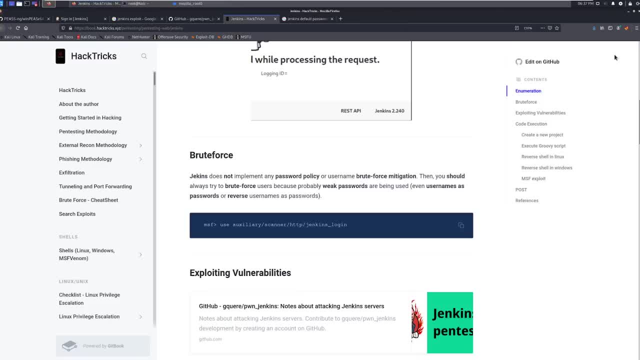 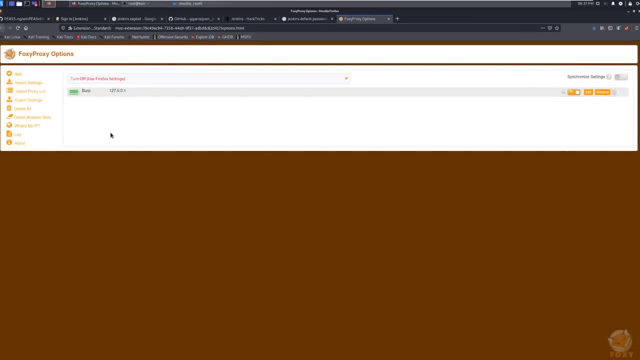 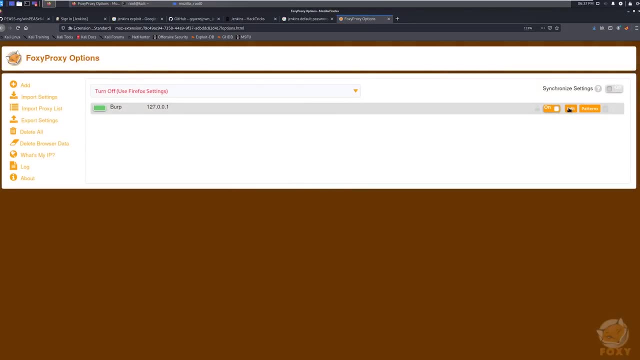 me to remove it. All you gotta do is install it. It should show up right here in the corner, Little Fox, okay, go to options for your first time setting it up, And in here all you want to do is hit add And then I'm going to cancel this. Let's edit. 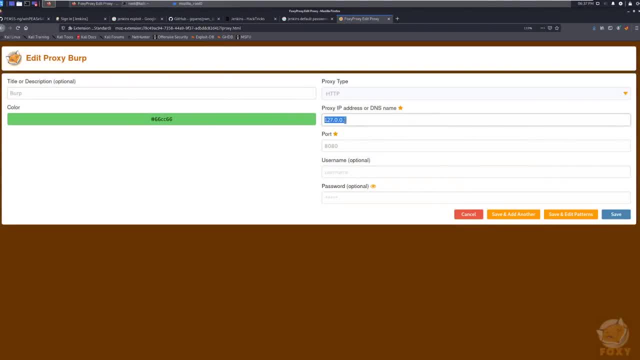 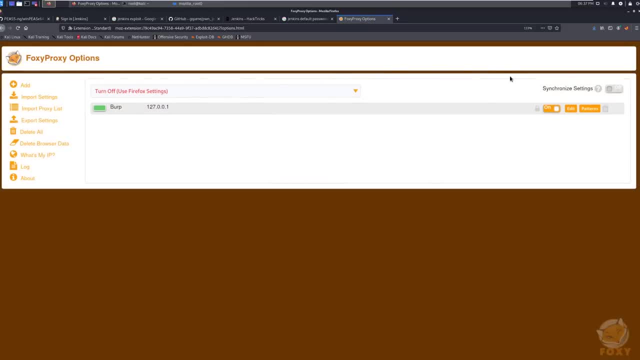 this so you can see what my settings are. I just named it burp 127001, our local host and our port of 8080.. What this does is we use burp suite once in the course And we had to go in and 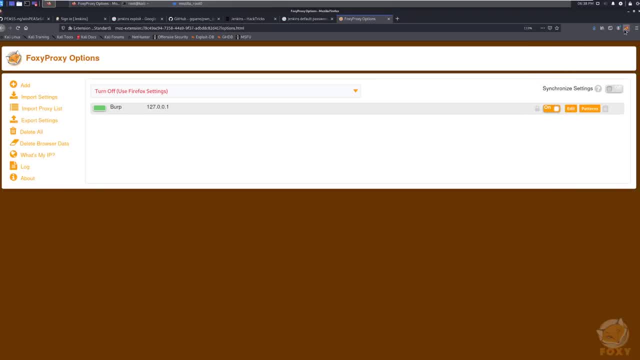 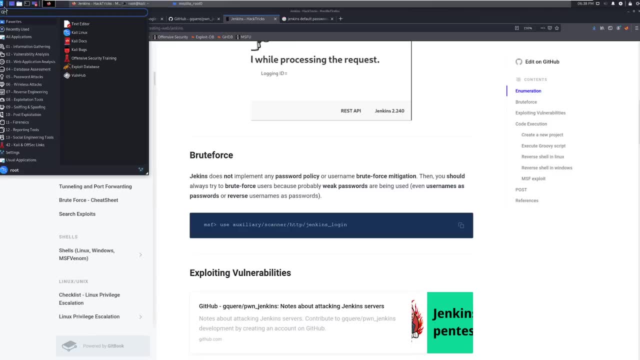 change our settings and our preferences and come in here. This just does it for us automatically with like the flip of a switch. So when we open up burp suite, let's go ahead and do that. You can just type in burp up at the top and open up burp suite. So 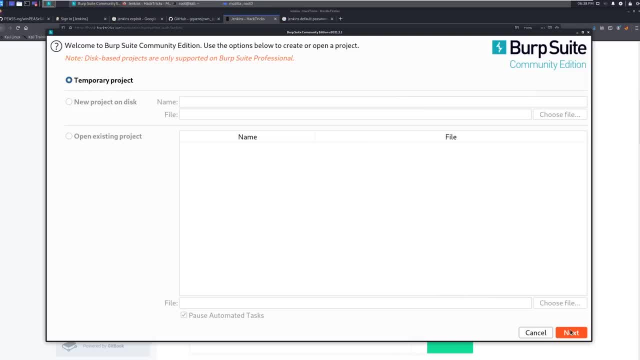 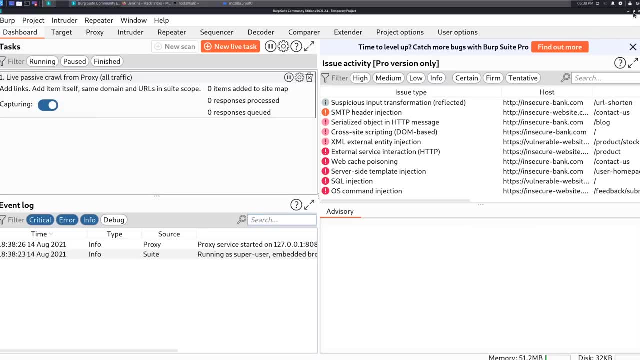 we're going to use this proxy, right, we're going to proxy through this. I'm going to cancel any requests for updates. we're just going to use what's in here. This is 2021 2.1, which is new enough for me. I've made my font size really big, So 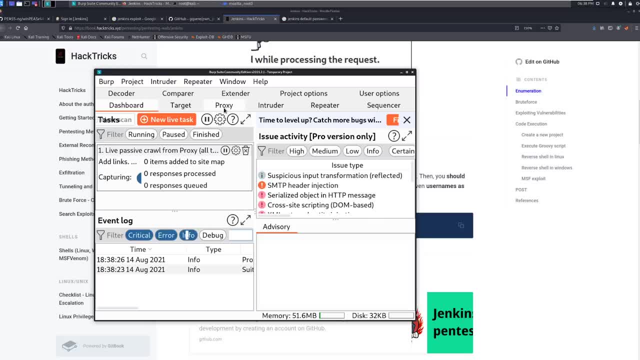 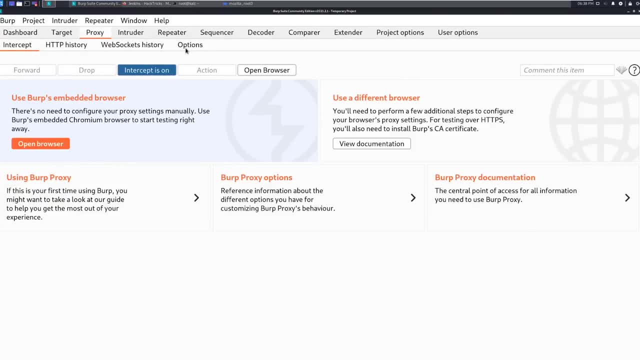 yours might look a little bit different. This is just for video recording purposes, But in here we have a proxy, So we're going to use this proxy. Okay, this is what we're going to be listening on. we're intercepting some traffic. we showed this a. 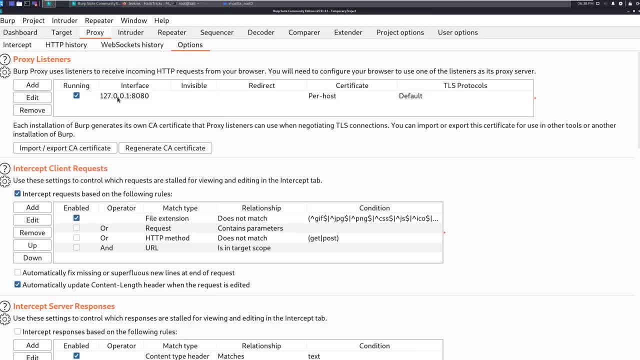 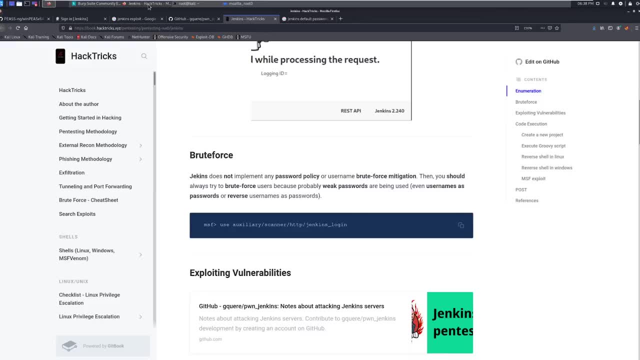 little bit in the last, the enumeration section, But here you can see 127 001. 8080 is where the traffic is flowing through And I'm going to go ahead and intercept traffic. So like I'm going to come in here And I'm going to say admin. 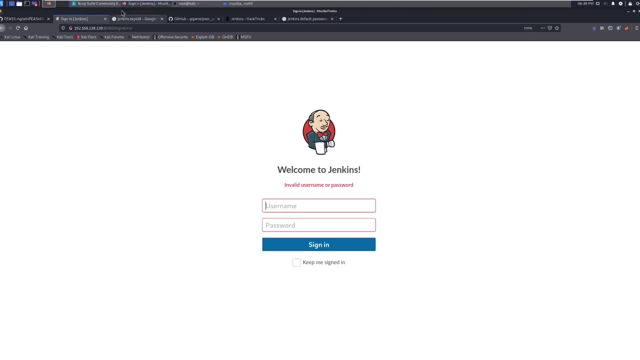 password on this attempt, which I know is not going to work, But we have the traffic now intercepted, hopefully, in our burp suite. I'm going to go ahead and hit enter. Okay, now it comes up, So you can see the request comes through. in this inspector, we're. 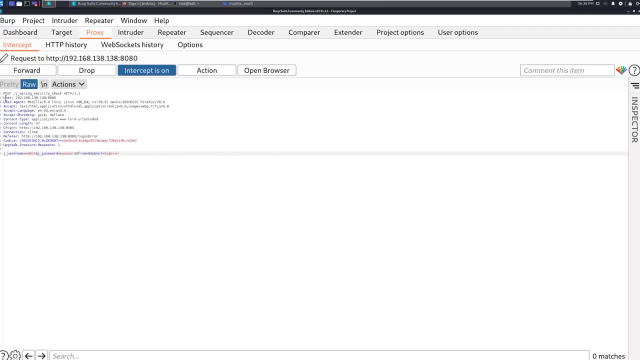 getting a post request. we're trying to pass this password through admin password sign in form. Okay, what I'm going to do is we can send this to repeater. I'll send it to repeater first, then I'm going to send this to intruder, So just right click. 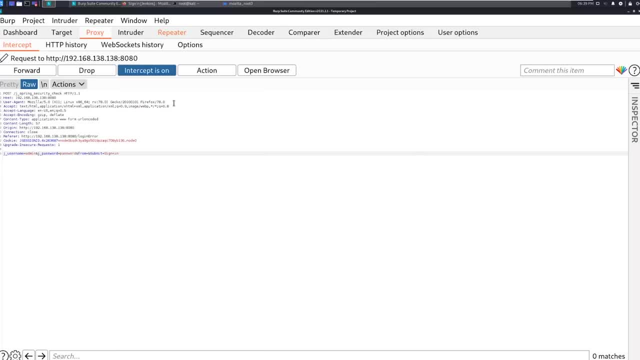 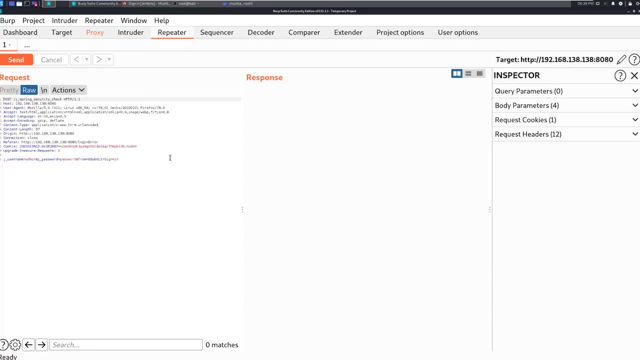 You can do Ctrl R, Ctrl I. both are going to be in the same folder. Okay work. Ctrl R to send repeater, Ctrl I to send to intruder. But in this instance we can just push this request, hit send And. 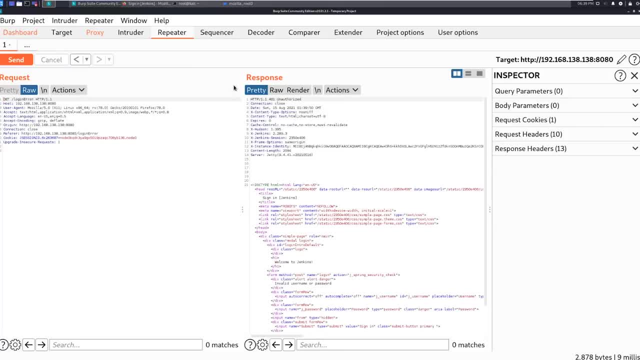 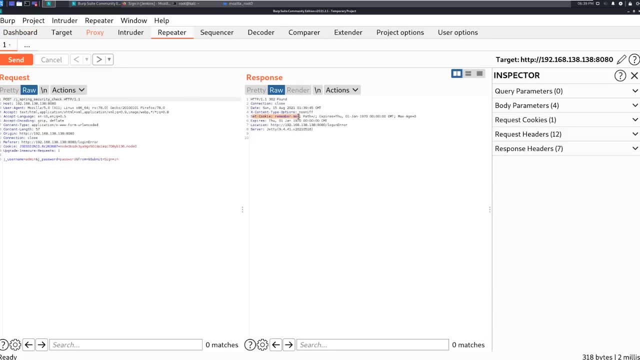 this will just say: hey, 302 found. you can follow the redirection. it's going to say 401, unauthorized. Alright, so that's one thing we could see in here, that the set cookie comes, remember me, equals. and there's nothing in here So that could. 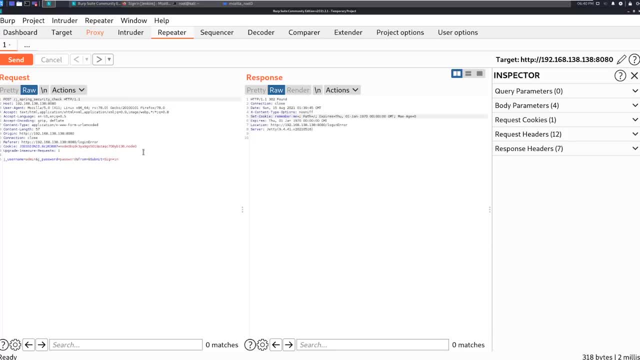 be something to look forward to a little bit later, But what we want to do is we want to come in and we could technically brute for us. we could be like password, password, one, go, send that one and keep coming through until we can find, follow the redirection and find an actual login Doing. 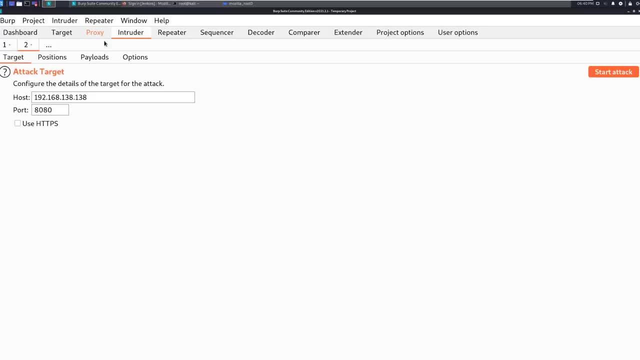 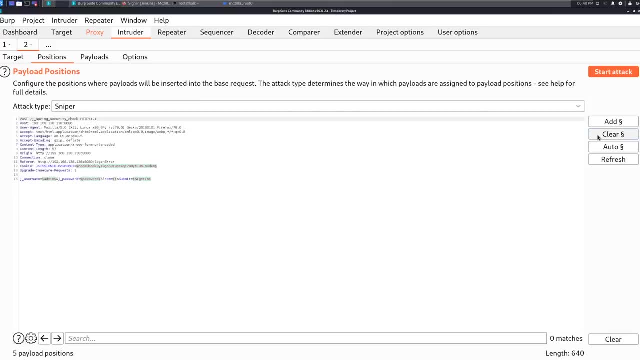 this with repeater will take forever. Good thing is we have something called intruder. So if you come in here and you go into the positions tab right here, go ahead and hit clear. What we're going to do is set a couple of positions. we're going to come. 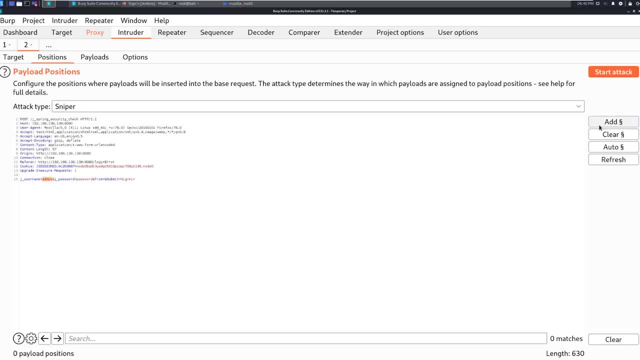 in here and we're going to say, okay, admin, I see you. I'm going to go ahead and say: add double click on admin. hit add. double click on password: hit add. We are basically setting up our parameters or our variables. that. 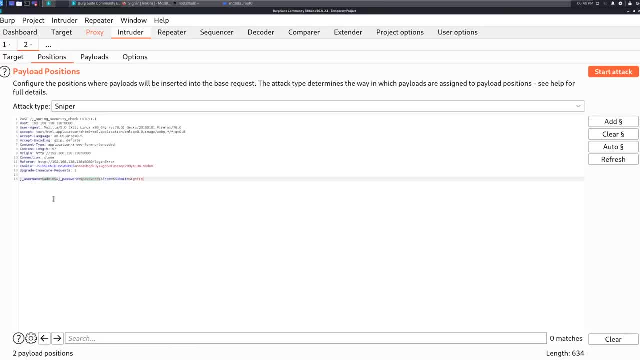 we're going to use. So we're going to perform an attack where we give usernames and we give passwords and it's going to try those in combination. So really, when we use multiple facets here, we're either going to be using pitchfork or cluster bomb. So 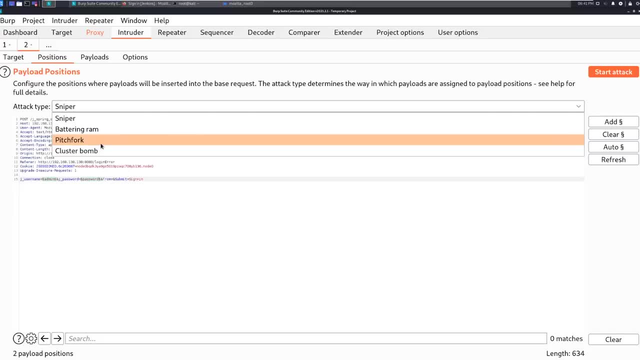 pitchfork is great for what is credential stuffing which we're going to be trying. hey, I know this user has this password, So we'll say admin has the password, a password, and we may have found that in a breach. Okay, 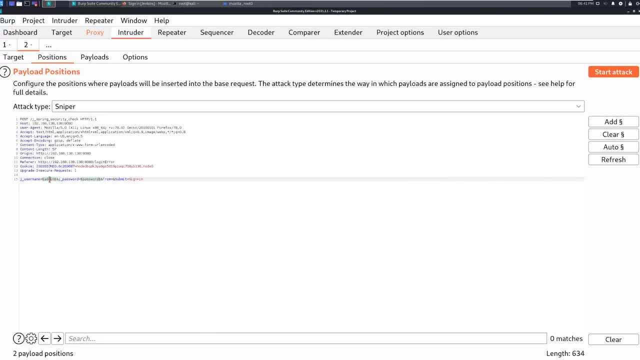 so we'll try admin to password and then we'll try next user with that password. So it's one to one. Now battering or sorry, cluster bomb is I'm going to try every single user with every single password in the list. So if I've got five users in 10, 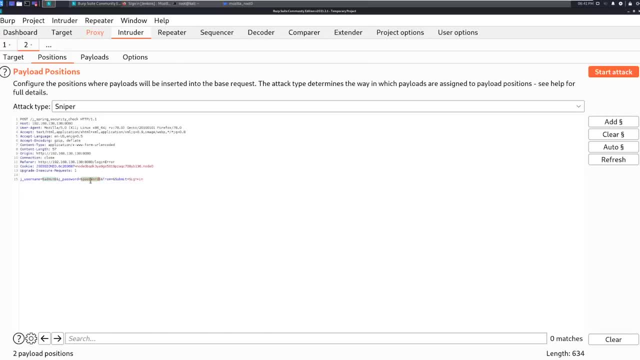 different passwords. that's going to be 50 different attempts because it's going to try user one with all 10 passwords, user two with all 10 passwords and so forth. So we're going to use a cluster bomb attack because we have no idea what the username or 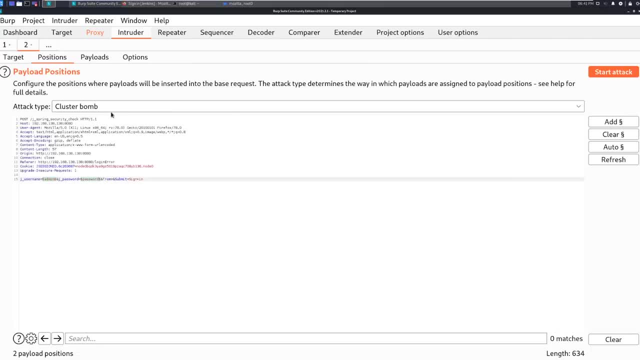 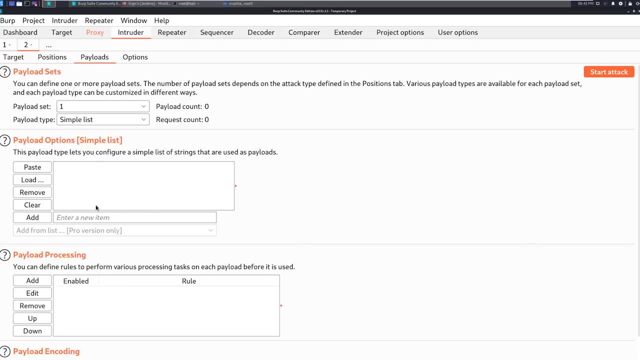 the password is Now. in order to save time, I'm going to just type in a few different payloads here. Realistically, we would guess some different usernames that would go in here, like, for example, admin, administrator, Jenkins- Okay, if we knew like an IT person or 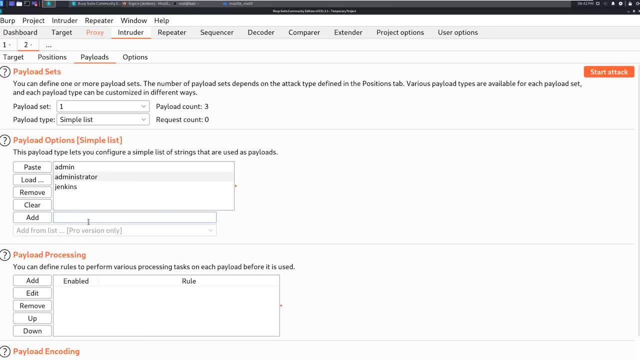 somebody who might be running this we might put in their name. But in this instance we might just want to run with these three And then on a bad password list we might just go copy like the worst 100 passwords or worst 500. 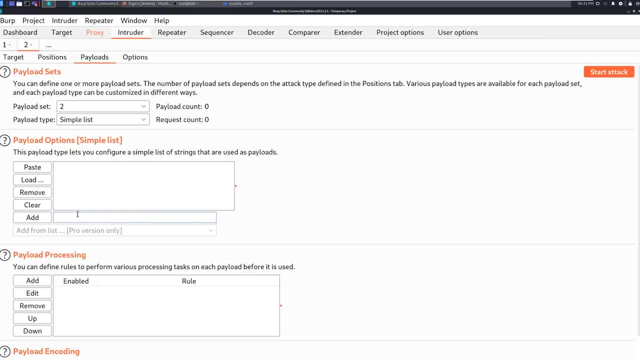 passwords and then just hit paste and paste it in here. In this instance, I'm going to type out some bad passwords. So maybe password Jenkins? how about password with a capital P? Jenkins with a capital J? Okay, you know something like password one, etc. Now we have three different. 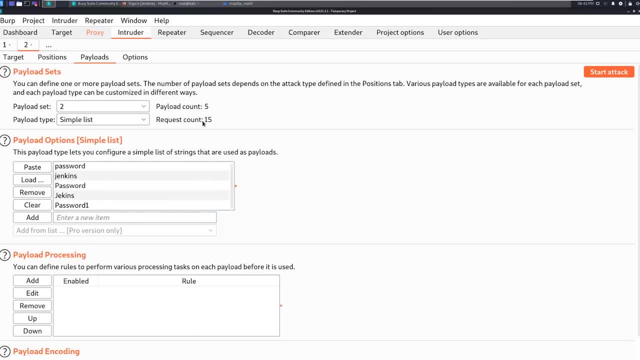 users, five different passwords, 15 different attacks. three times five is 15.. So we're going to try admin first, with all these passwords, then it's going to go through and try administrator with all these passwords, then it's going to try Jenkins with all these passwords. Okay, 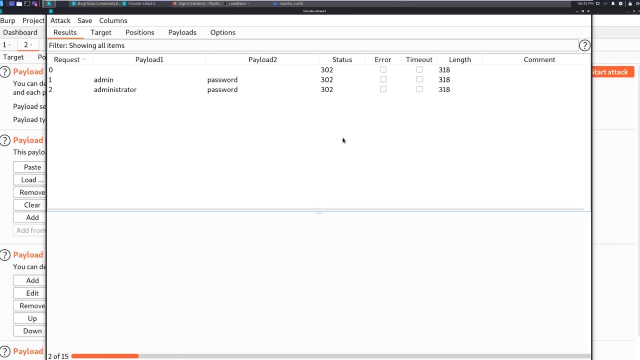 so we're going to hit, start attack, And what's going to happen is it's going to start pushing through And we have to be very cognizant and watch this and watch for any sort of changes that might happen in this. Okay, it's very, very subtle. Okay, when we're looking through this, 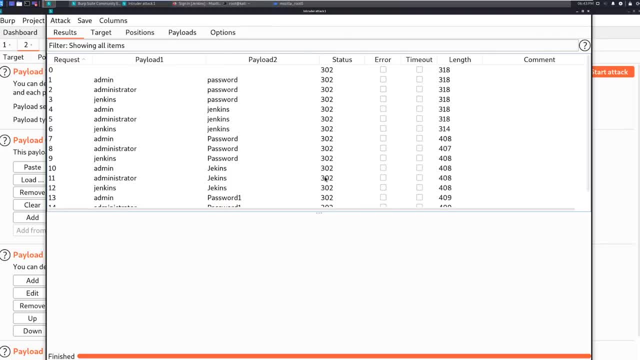 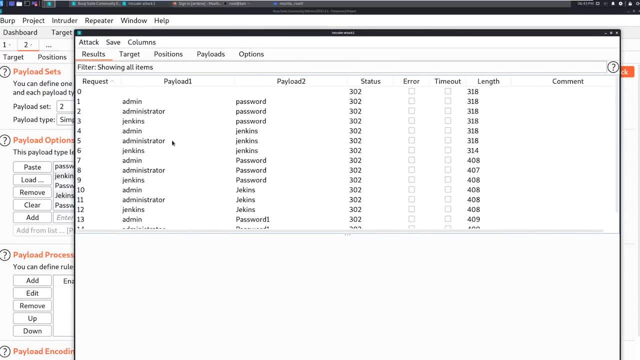 if there's a status change, sometimes these will go like 401.. Or we could follow the redirection in the settings. By the way, we could select that. There's also advanced stuff that we'll get into with, like we can use grep to look for different changes in here. We'll talk about that. 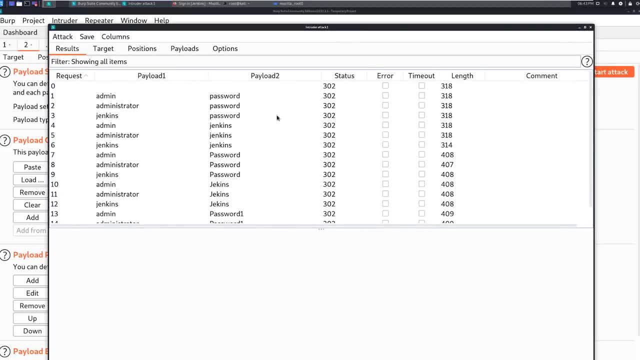 a little bit later, But we also cover that in the external pen test playbook course, because that is something that we do when we're doing password spraying attacks Here. in this instance, we are looking for subtle changes like the length that is here, If you. 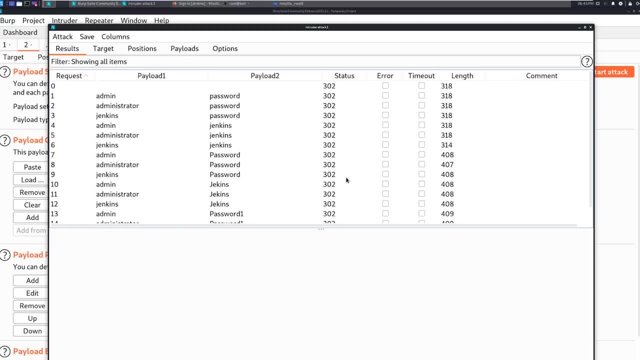 notice, everything's 302.. So there's no difference in status changes. There's no difference in, like error codes or anything. What we're seeing, though, is 318, 318, 318, 318.. All of a sudden, there's a 314 on Jenkins, Jenkins. What changes here? What is the response? that changes compared. 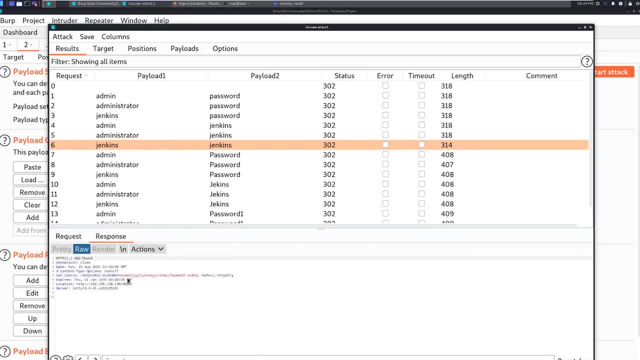 to this: Okay, here we get a J session ID Cookie, where here before we did not have that. Here we get a cookie. And then what changes? Here we already have a J session ID cookie And we're getting a login error Because we have more data. 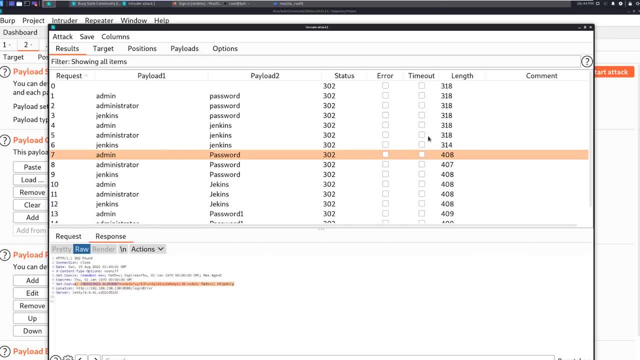 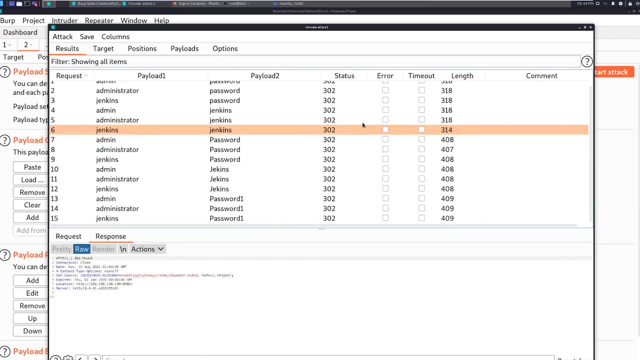 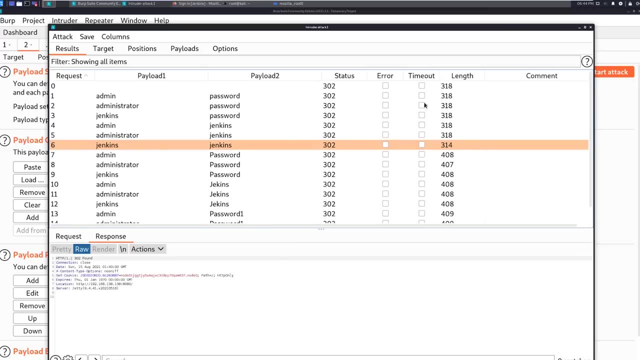 that we're storing in here. we're already authenticated, So now it's gone from 318 down to 314 for this one request into a bunch of 408 to 409 range. So this one small, tiny little request indicator that there's something different. So you have to really scroll through this. Use your 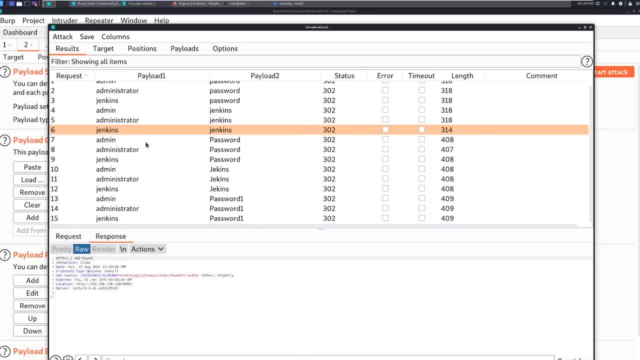 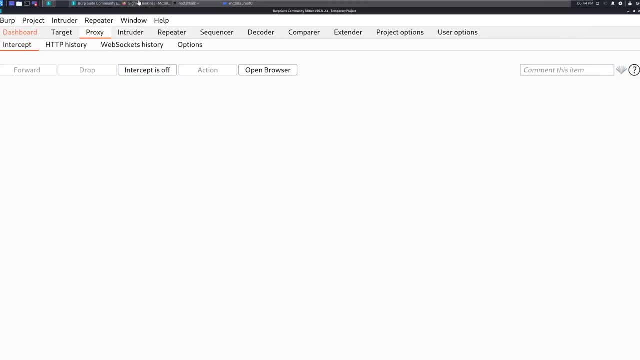 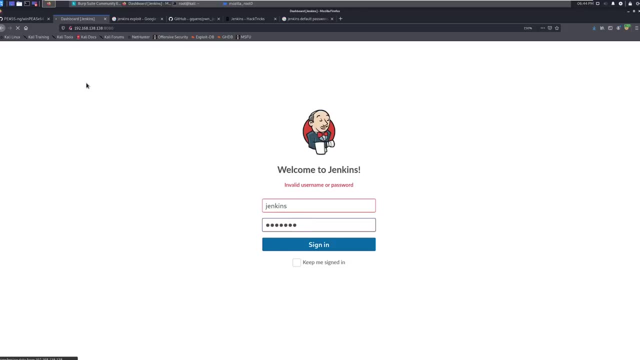 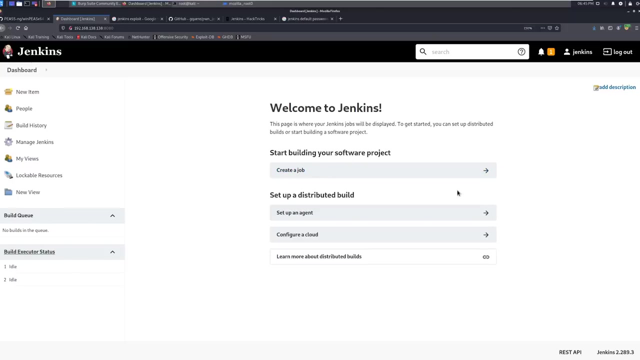 eagle eyes and make sure that you are looking through this with a fine tooth comb. Here I'm seeing Jenkins Jenkins as a valid login And we're going to go attempt that and turn this off. We're gonna go attempt to log in with Jenkins Jenkins And hopefully we get it. Okay, We do get it, So. 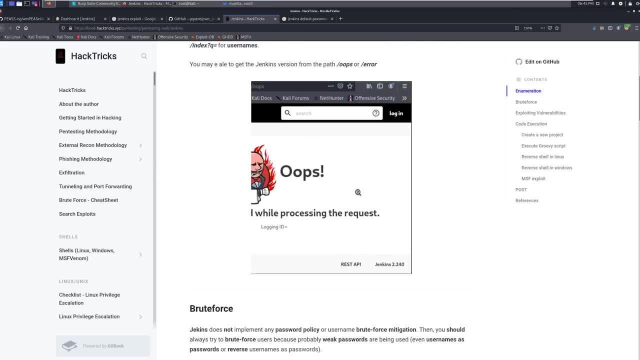 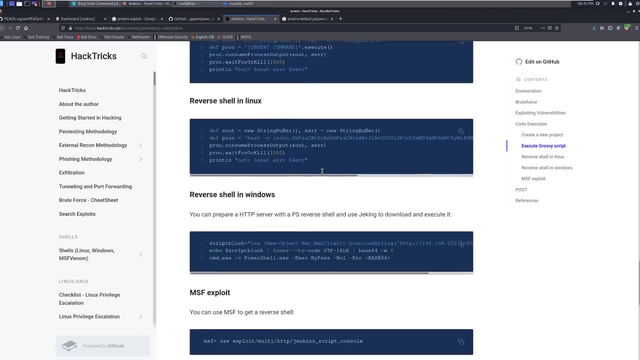 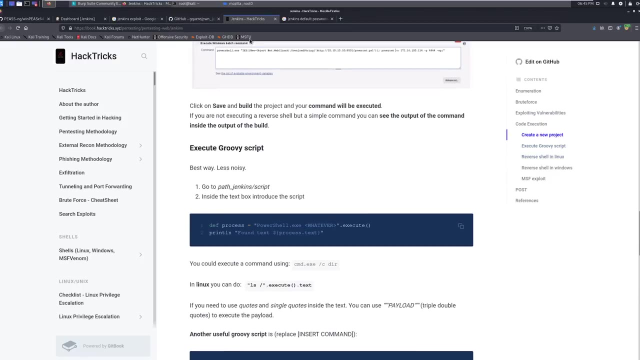 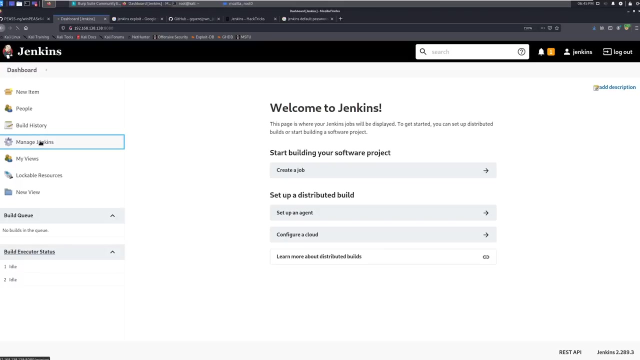 from here have the ability to run code execution. let's see what they say. so we need to find a place to execute this code. this is okay. i've seen better write-ups on this. so going around and doing some research, you will find places to to execute code in here. if you go into manage jenkins, there should. 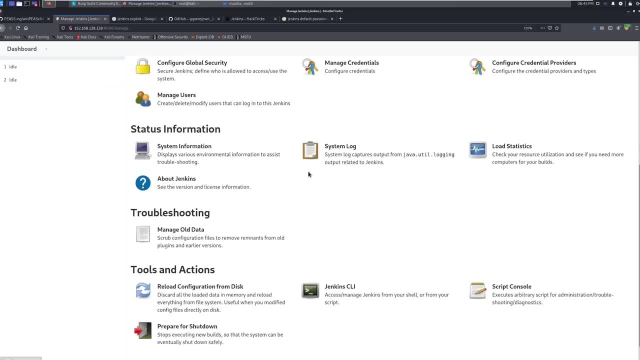 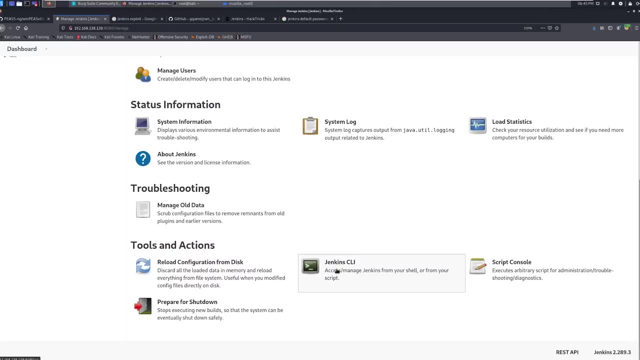 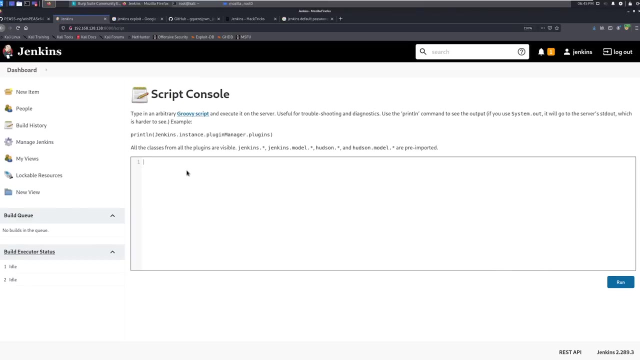 be a bunch of different tools that are in here. um, scrolling through, there is a command line here that you can run from a shell, which seems pretty interesting. it's just getting into a shell on this machine from a script. there's also a script console here. okay, the script console is interesting. 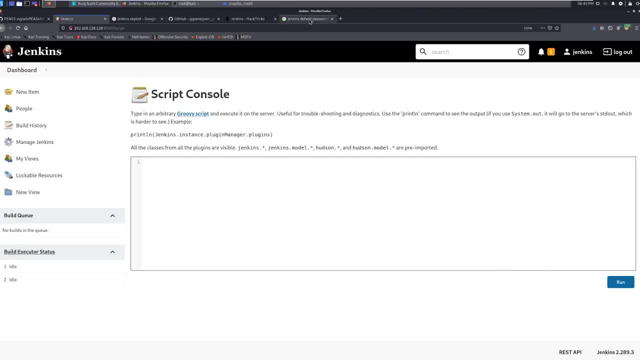 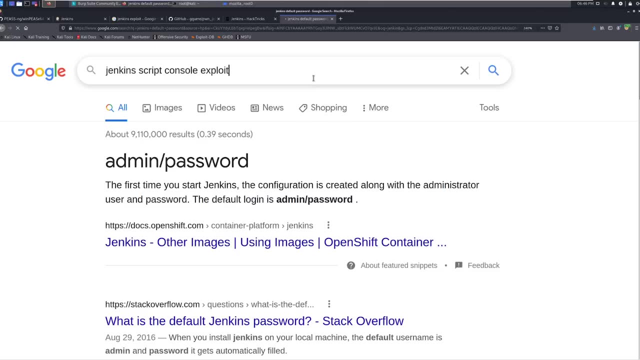 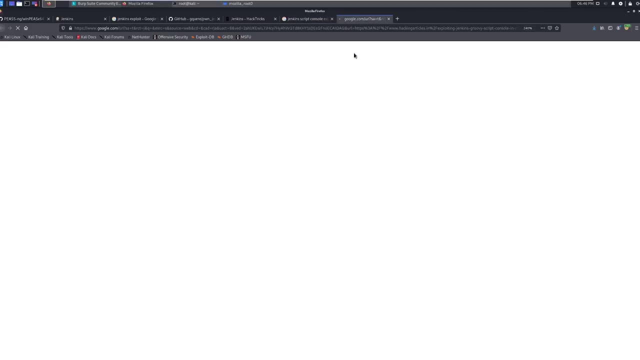 because it's in groovy. we've seen groovy a few times. you might even type something like jenkins script console um exploit something like that, and you can see exploiting jenkins groovy script console in multiple ways. so this is somebody that came in here and did this. um. another thing that you can just read through and see: they're 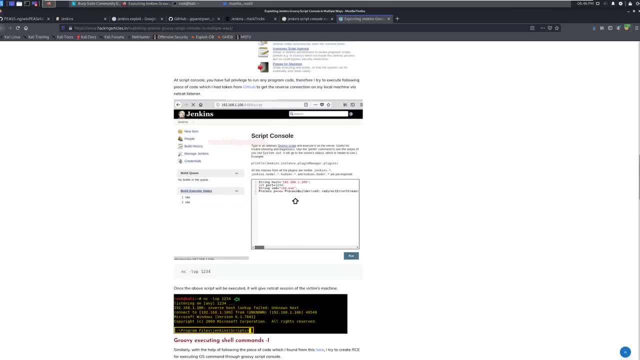 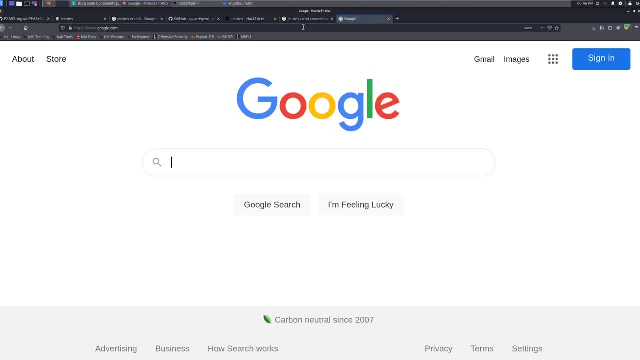 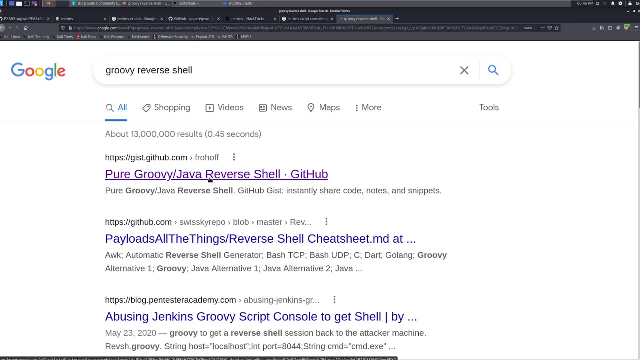 using metasploit, we can use manual methodology, which is right here. there's a github reverse shell which? um? honestly, if you just go to google and you just type in groovy reverse shell, the first thing that comes up should be your ideal, one, which looks like that's the same one they had too. 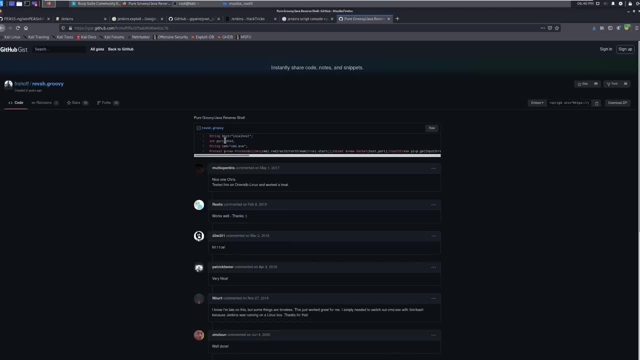 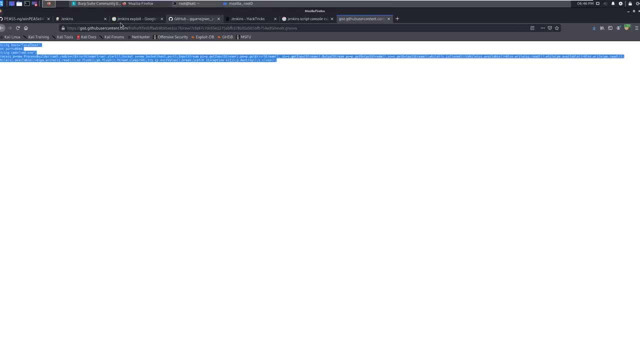 but this is a good way to do that. so i'm going to go ahead and type in groovy, and this is what i like to use. you can come in here, make this a little bit bigger. you can just go raw, copy this and then we'll paste it and we'll talk about it. so copy that, paste it in here. 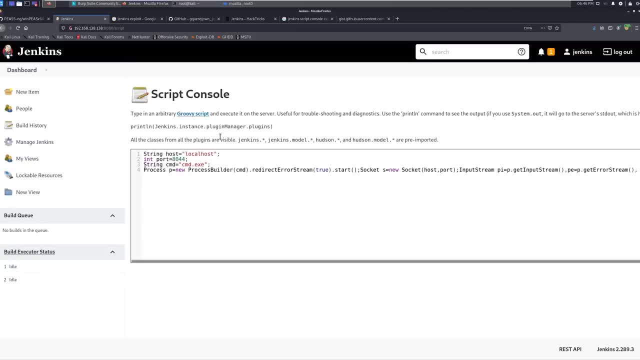 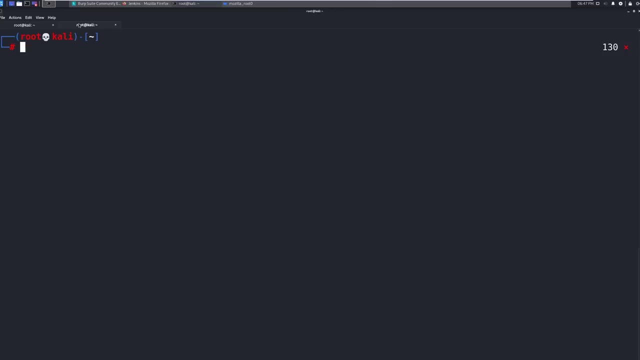 so we need to utilize this for a reverse shell. this is using commandexe to perform the reverse shell. it's giving the port of 8044. you can choose whatever port you want here, but i'm going to keep it the same. why not keep it simple? okay, so i'm going to go ahead and type in groovy reverse shell. 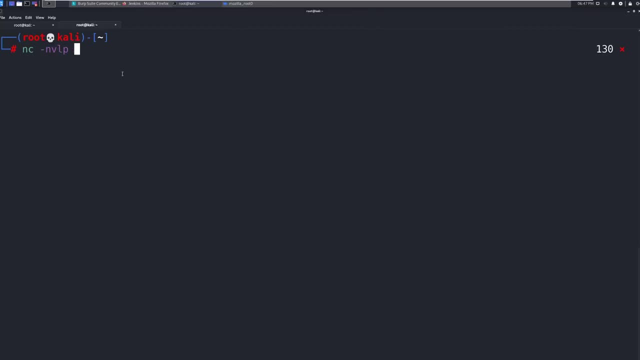 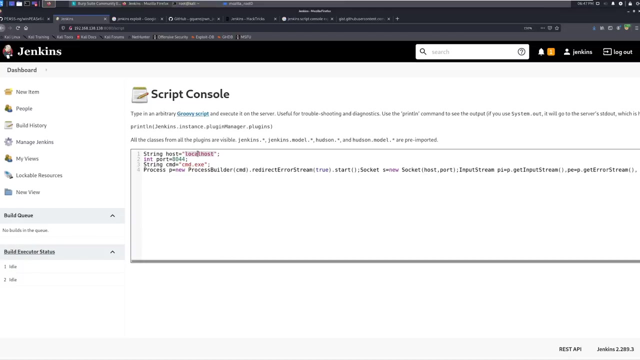 so i'm going to make this bigger. netcat: mvlp 8044. we'll set up a listener on here. we have local host. we're not running local host. okay, we're gonna give it 192.168.138.131 or whatever your attacker ip is. so, whatever your ip of your kali linux machine is, this is what you want to get. 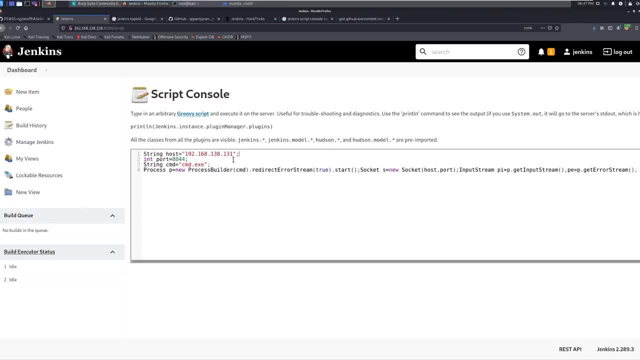 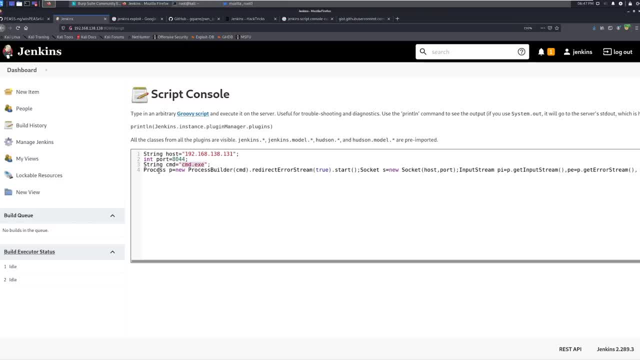 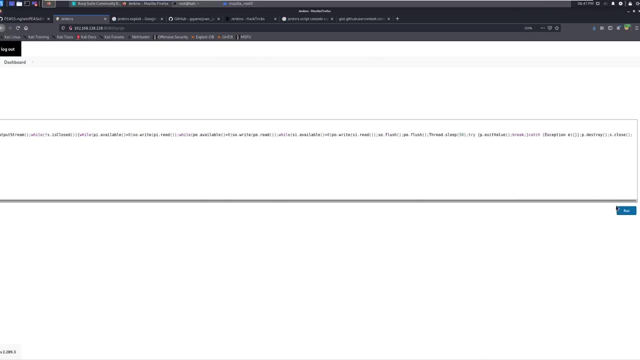 on this port and when it reaches out to us, it's going to execute commandexe. here is the whole process of that code. all we have to do is execute this, which i might need to make this a little bit smaller to actually see that. see, we'll just go all the way over the right and i'll just run this. 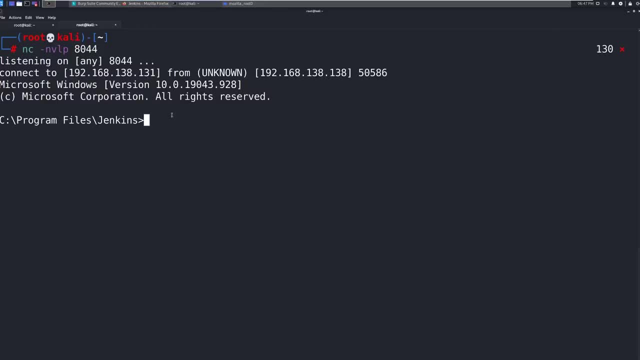 okay and it's stalling, which is usually a good sign, meaning that we are likely getting in and we do have a shell here. so we are now: who am i? we are now butler on butler. we are not system, we're not authority system. so we need to take this a little bit further and see if we can elevate privileges. 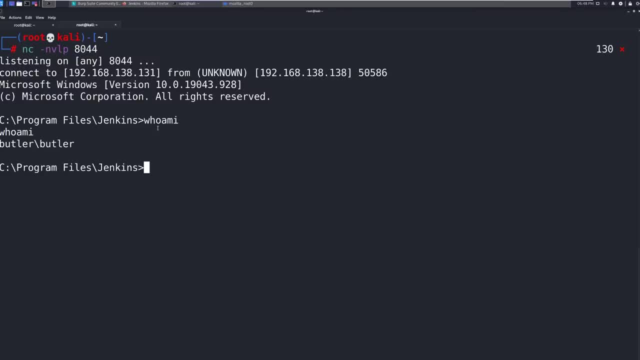 now there are several tools and methods that we can utilize. we are going to look at a classic form of privilege escalation on this machine. if i were going through this machine, the first thing that i would do is i'd look at system info. i would want to know what the system is all about, and i would 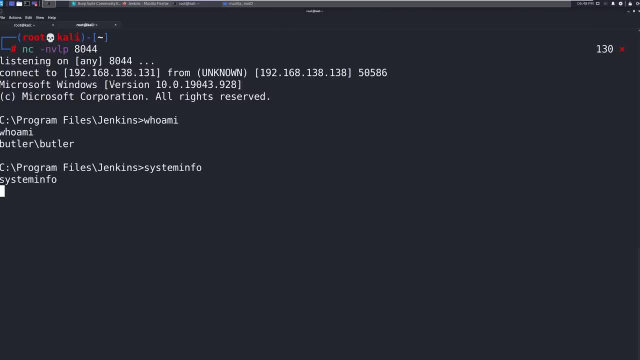 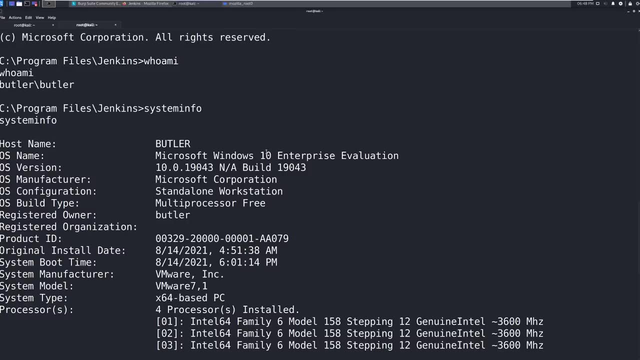 want to know what the system is all about, and i would want to know what the system is all about and machine. this is what the build is. you can see we're running on windows 10.. if this was running on an older edition, this is a windows 10 enterprise, which is nice. um, we're running on windows 10, so 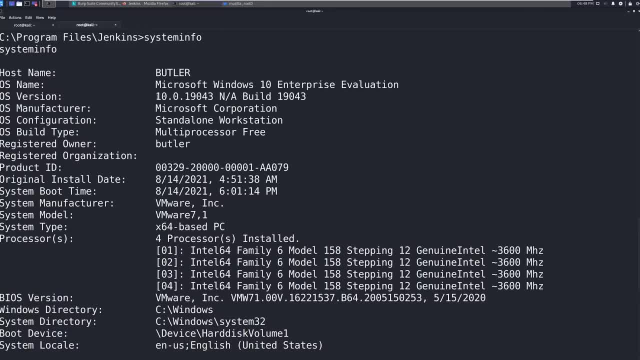 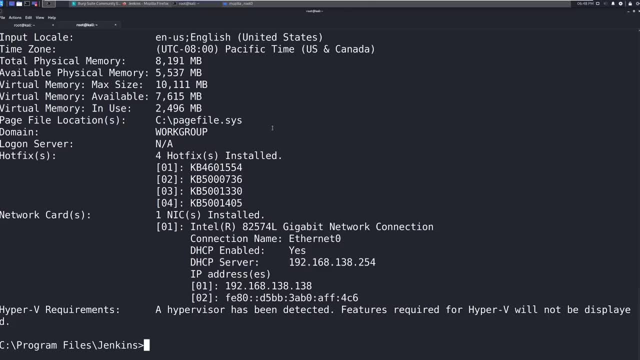 the chances of there being an exploit for this build may be pretty low. i would look at this build, see if there's anything there that we can use or abuse in order to get escalation, but the intended path on this as of right now is a different method. so we're going to look through that and i'm going 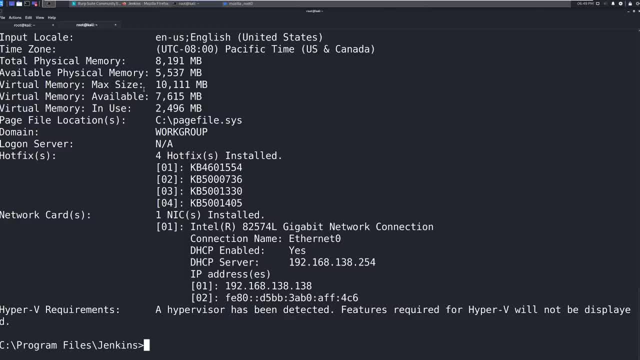 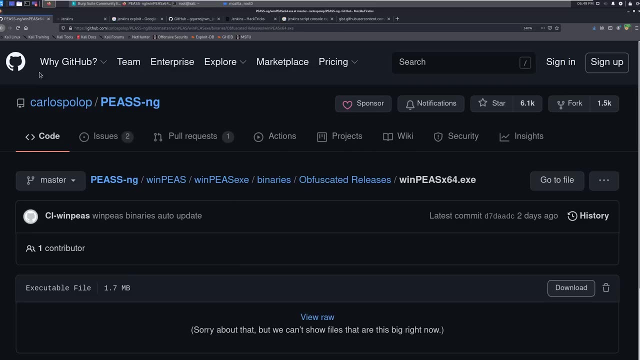 to show you kind of the basic enumeration process that we can use again. if you're curious and seeing this in way more detail, you are welcome to join us in the windows privilege escalation course and go through this a little bit more. so, um, with that out of the way, there is a tool out there called winps, so i'm going to go. 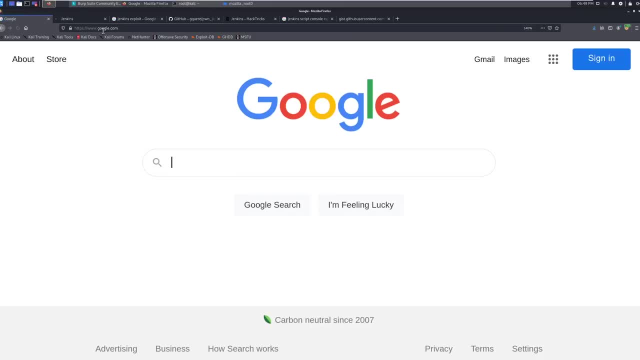 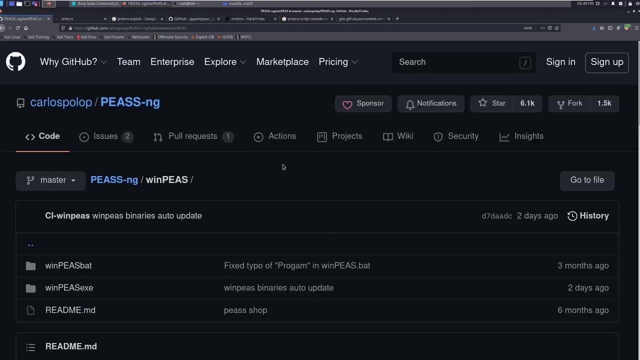 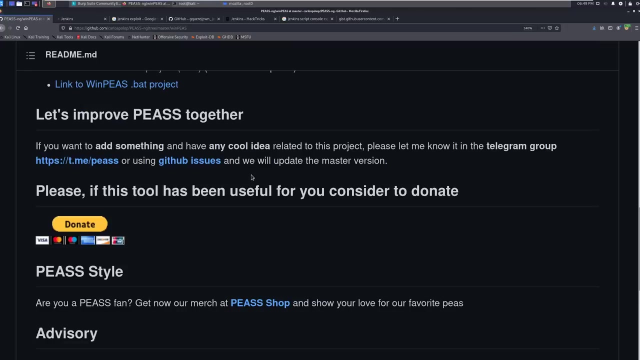 back. i'm kind of already cheating and going ahead because i downloaded this earlier, but if you search winps, remember linps. this is the windows version of linps. so just go to the first thing that you see now in here. if you scroll down a little bit, they have the different. um, they'll have different. 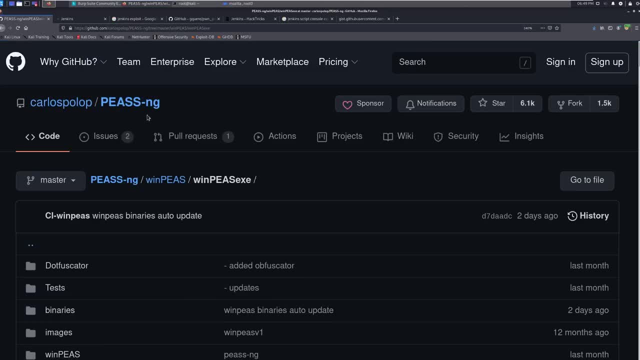 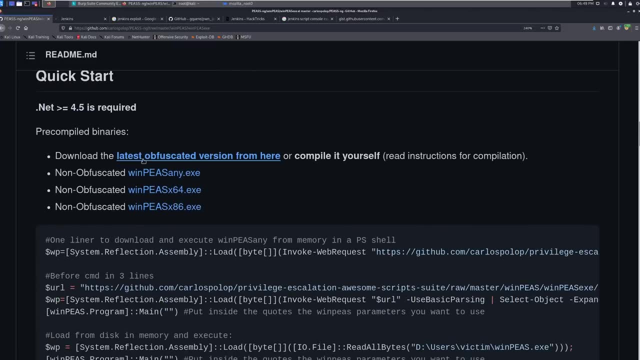 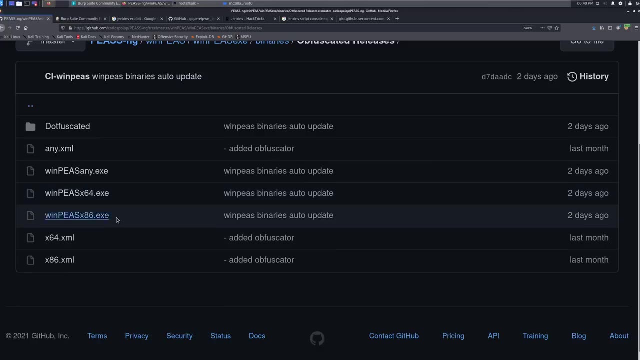 downloads so we can go into the exe. here, winps exe and you'll see an sln. we don't want the sln, we just want to be able to download the latest. so go into download the latest version. we're not going to compile this, we're just going to trust what they've got. so come in here, download winps x64.exe. 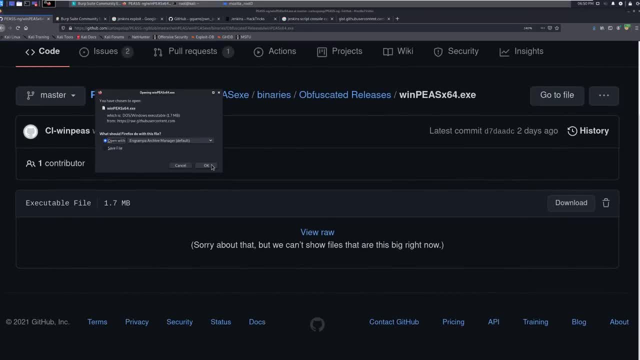 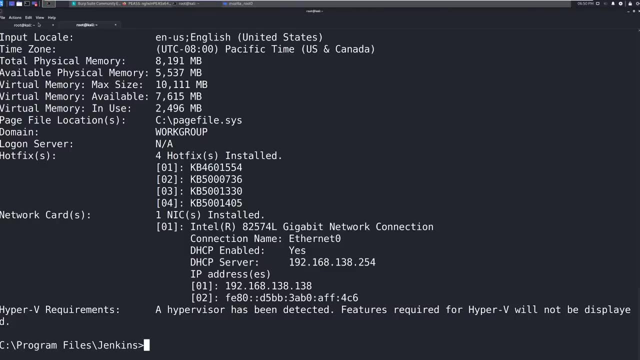 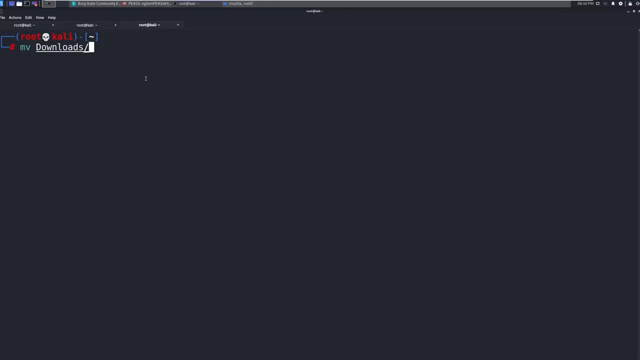 right here. all right, i'm going to. i'll say okay on this because i want to show you again what i do. if you come into root and you open a new tab, make sure you move this. so i moved. i don't know if i actually downloaded it. let's see um winps. i didn't download it, but 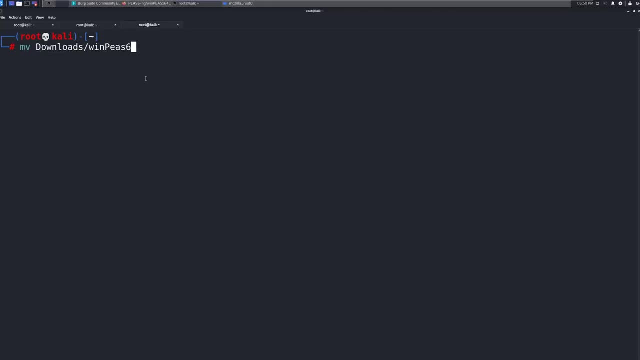 i moved winps, whatever it's called winps 64.. make sure you do that, move that into your transfer folder or ensure that you're going to have it um, where you, where you want to host it. i actually just moved it and i renamed it winpsexe, because it's a lot easier to just type that out on. 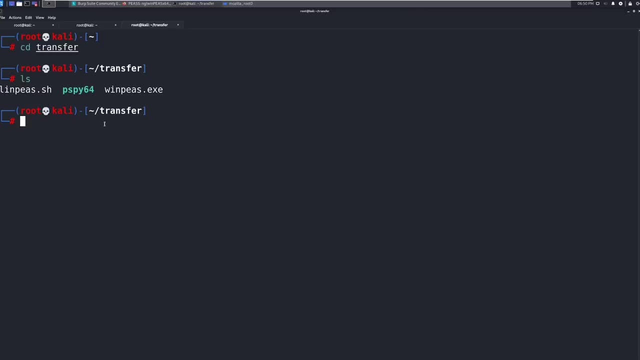 a machine and so a little bit, uh, keeping it simple. so with that, i'm going to go ahead and just do this, which is python3, m4 module, httpserver and port 80.. so we're going to host up this transfer folder in here, i'm going to go ahead and go to my shell and i want to go to my user folder. 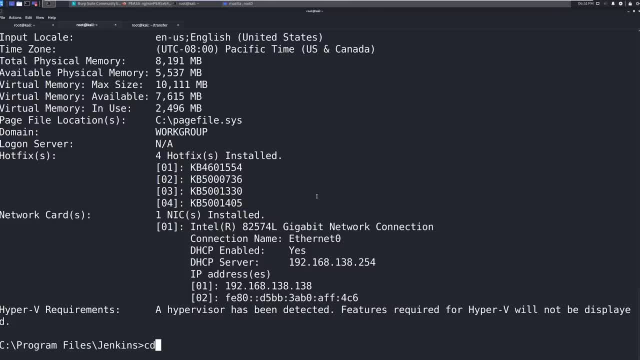 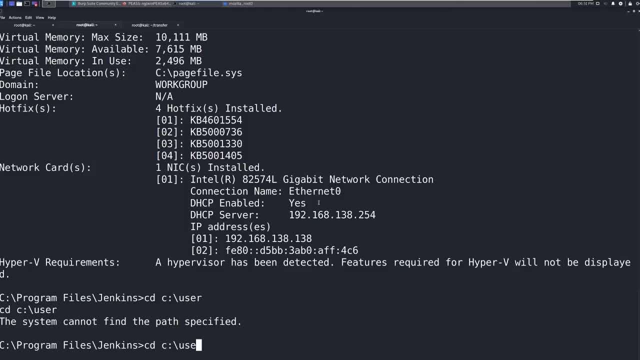 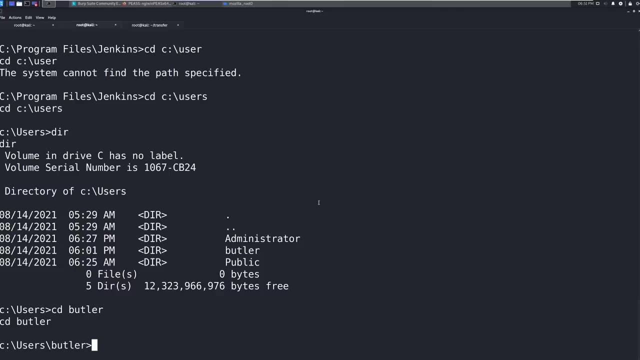 that i can write. it looks like i'm in the jenkins folder, but i like to go first of all. cdc user: okay, um, actually cdc users do a dir in here. um, butler should have read access or read write access, so we're gonna go there first. um, what we might do, too, is see if there's anything in here. 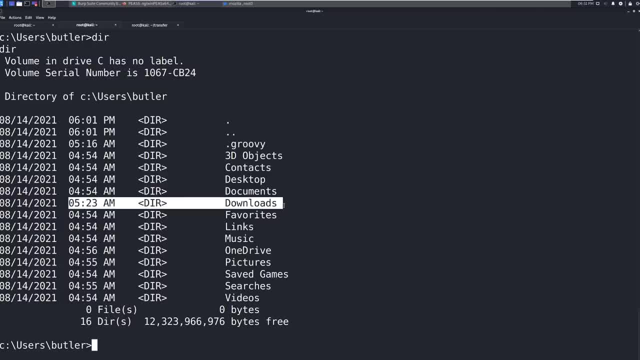 like we might. we might look at like the well, he's got some downloads in the downloads folder. it looks like: uh, an indicator in here is looking at the different times sometimes when you're doing these ctf machines, like what was the last time this is updated. so there might be something in. 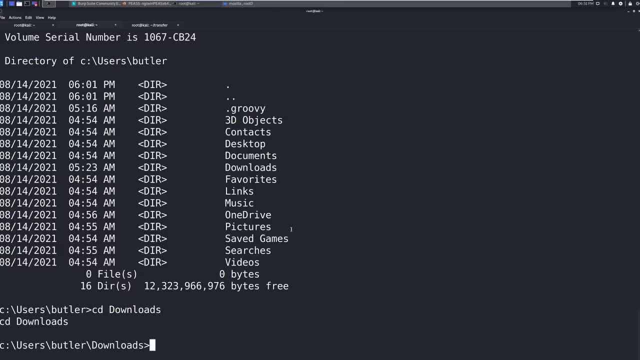 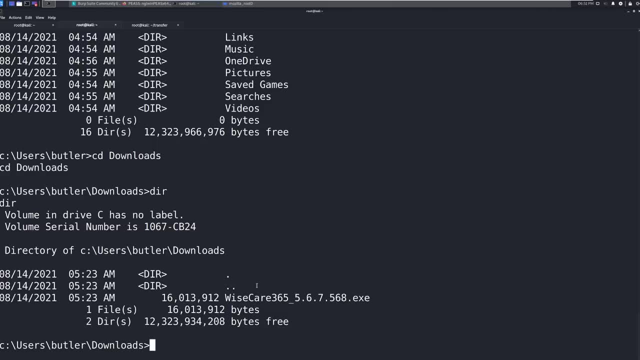 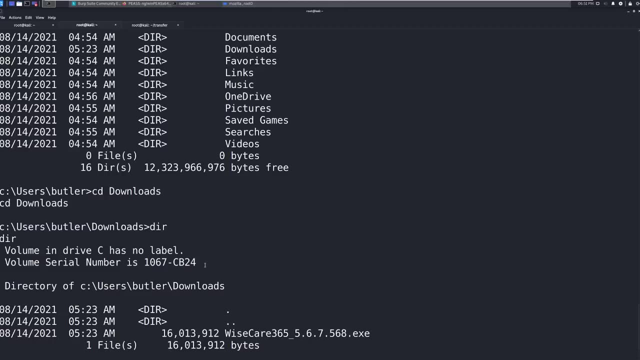 the downloads folder. that could be of interest. like cd downloads go der real quick. it looks like wise care 365 was installed. who knows what that is. that could be something of value to us later. but that is not um, that is. that is information. it's just not exactly what we're looking for at. 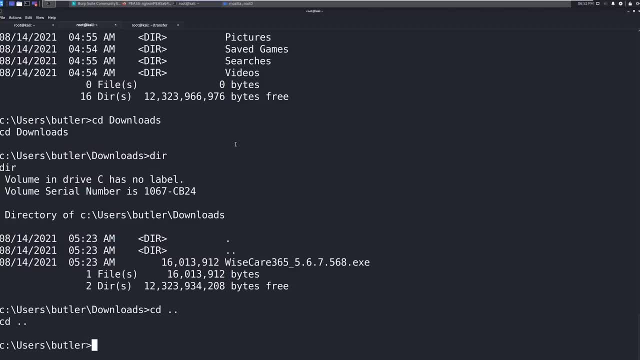 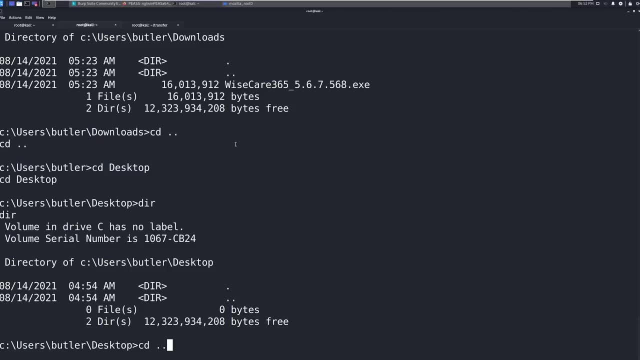 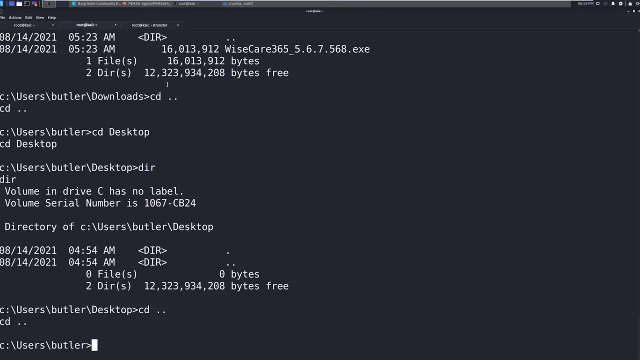 this again, exact second. um, we can go around, maybe cd to the desktop, see if there's anything there. um, nothing there either. okay, so we just want to be able to put a file somewhere that's writable. so i'm going to put, i'm going to put win piece here in butler's folder, just his base folder. 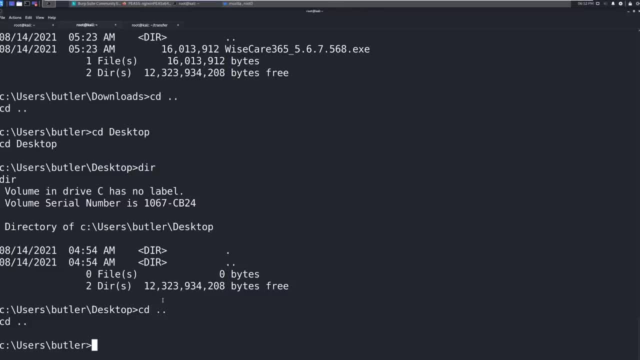 here for his user, and all we're going to do is use a tool called certutil to transfer this over. so, certutilexe, we're going to do a dash url cache like this: dash f for file, and then we're going to grab the 192, 168, 138, 131, slash win pc. we're going to call it. 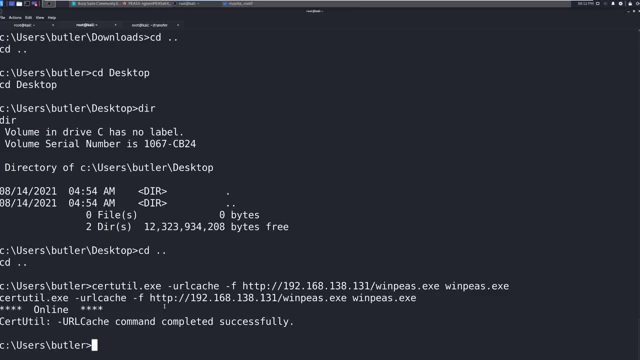 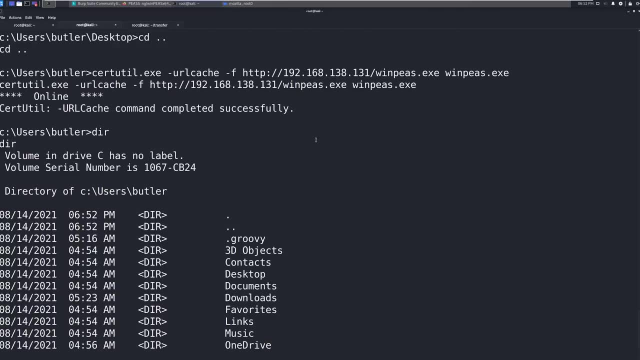 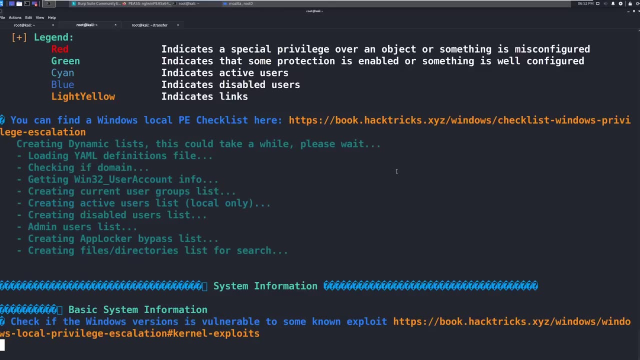 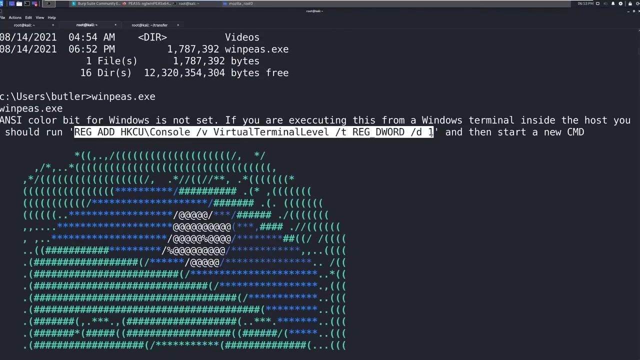 win piece. okay, we should do a dir and it should exist right here. so you need a second ketchup. go ahead and catch up, otherwise we're going to go ahead and move on. so now we just run winpsexe and special note: yours might not be in color. You can run this reg, add command or should be able. 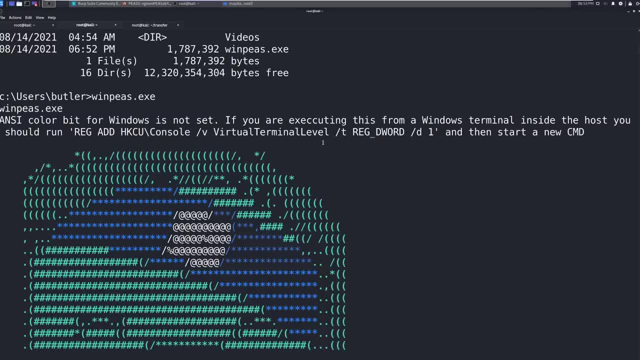 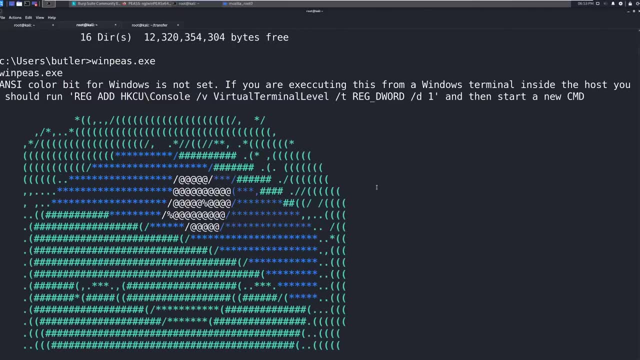 to run this, I'm not sure as a lower level user actually, So you might have to suffer through the first time with seeing it not in color. But just follow along on my screen. If you can't run this, reg add, but you're going to have to run this and then run this again. Otherwise we're just going. 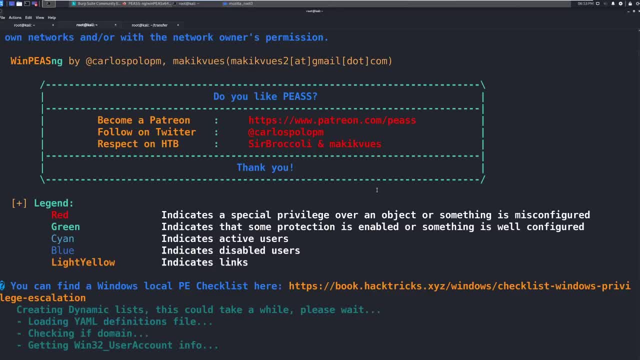 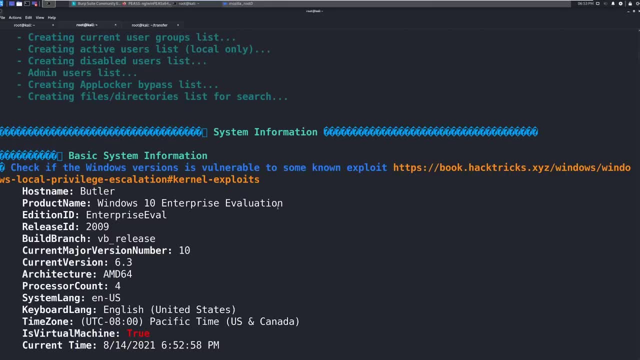 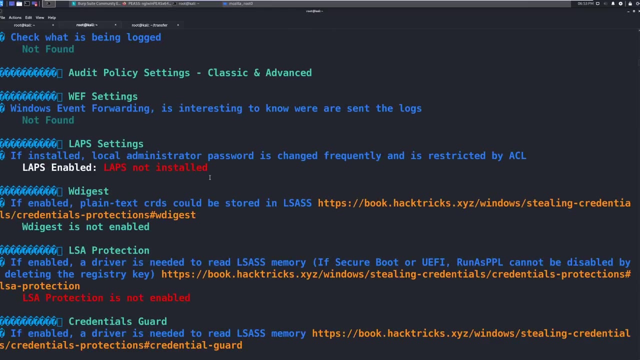 to kind of scroll through this and see this is similar to what we saw with Lynn peas. Red means something we want to look at and kind of scroll through. Okay, so we're just going to scroll through this. There's a lot of output on this machine. I'm looking for anything that quickly. 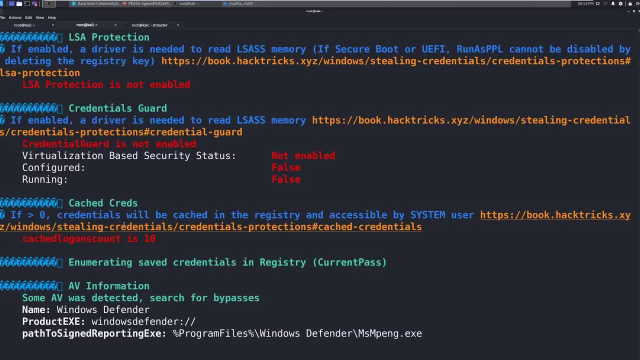 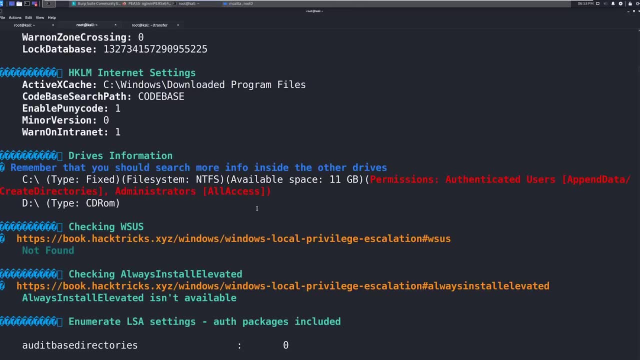 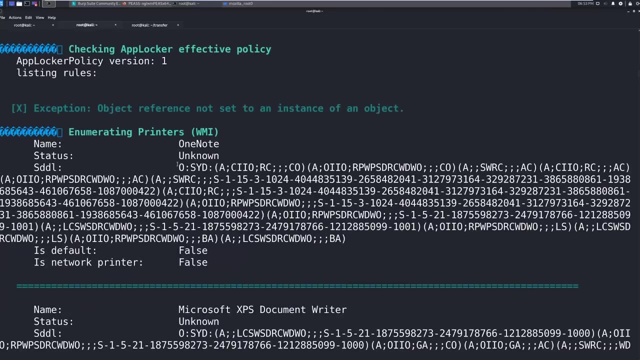 stands out for me, These protection enabled. they really don't matter to me at this moment. I'm looking for something that might just like: hey, this immediately stands out. So it's giving us drive information. Most of this is just disk enumeration at this point, Nothing of value. 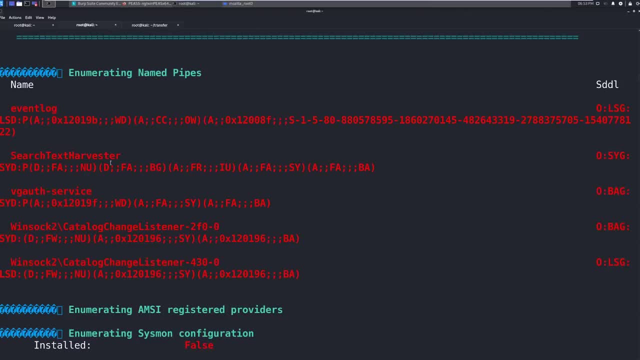 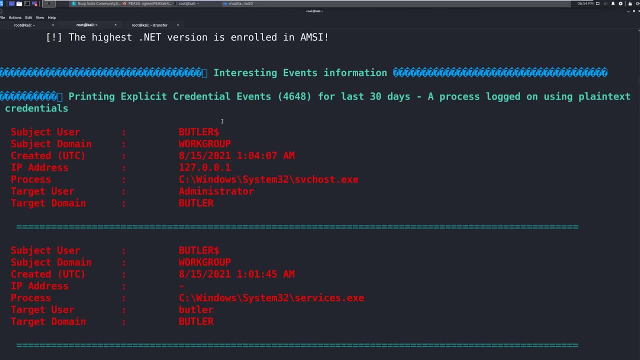 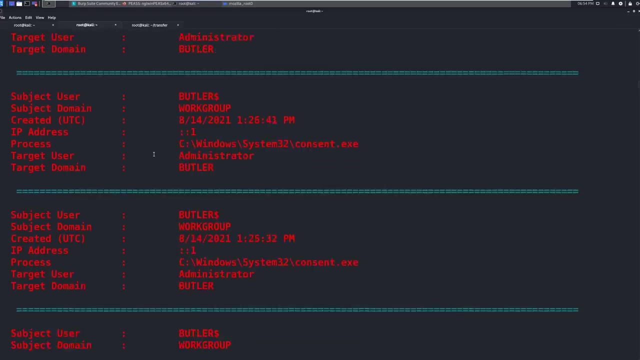 here So far. it's looking up printers, tells printers is looking up name pipes, which is fine. Going through this is telling us explicit credential events, which these are plain text credentials, If we have them. I'm not seeing anything here, So we'll scroll through these keep. 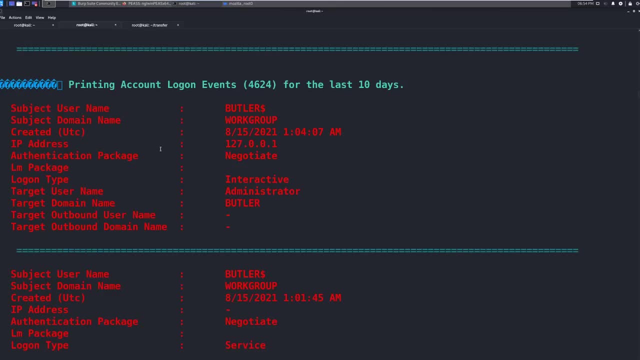 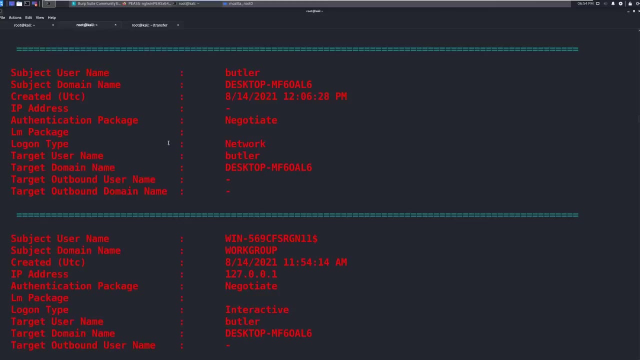 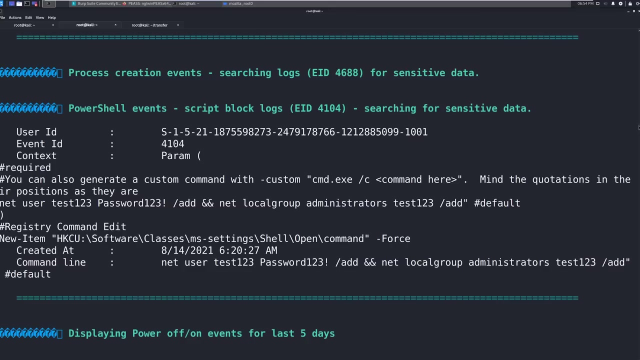 going Printing account logon events. These are just events again. So when piece has gotten beefier over the years, it used to be pretty quick to scroll through. I'm going to actually cheat a little bit and scroll down. PowerShell script blocks. Let's keep going here. Okay, users information. It's telling. 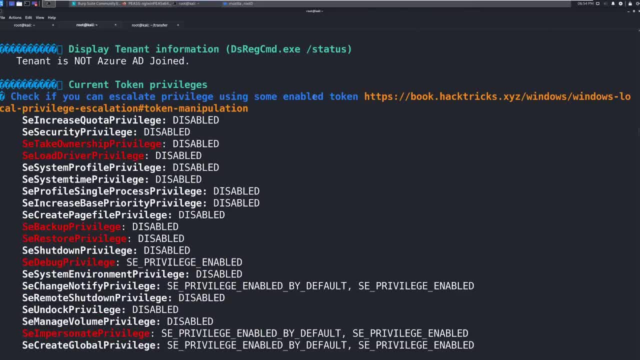 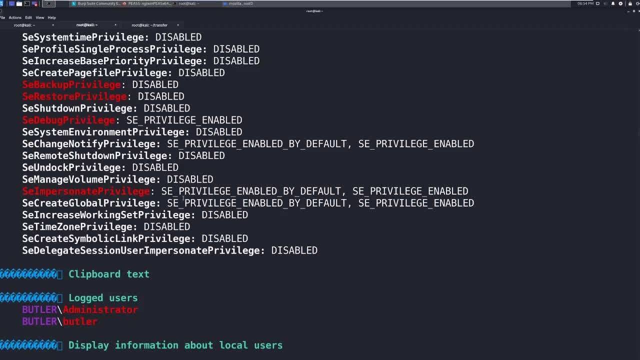 us, the users on this machine. And again, this is all different kinds of enumeration. Now, the se impersonate privilege could be good for a potato attack, But that's a different type of attack. We're not looking for that at the moment, But that could be something. that's why it's. 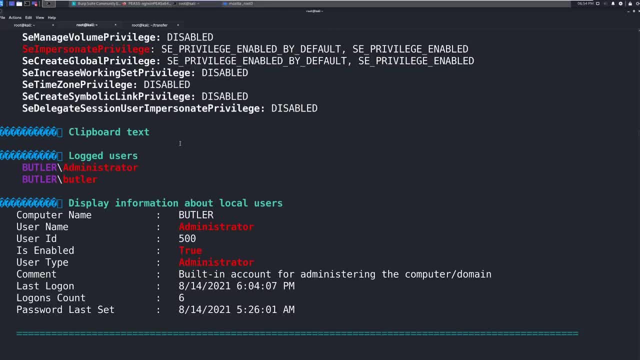 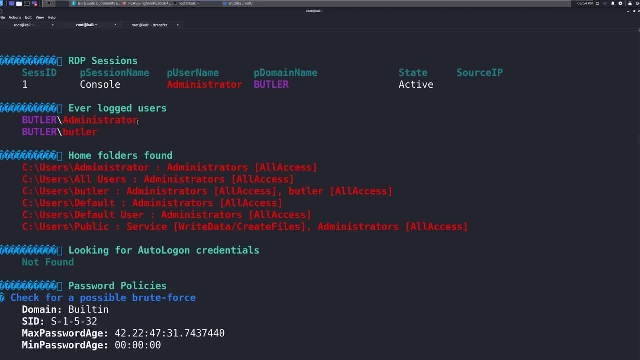 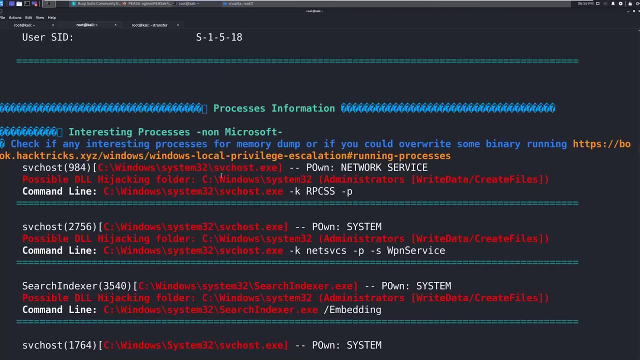 highlighted in red, something we do cover in the the escalation course. So it's telling us more about user accounts that are on this machine, any sort of RDP sessions that might exist, any sort of folders- heavy, heavy, heavy enumeration to scroll through. Okay, we're in process. information. 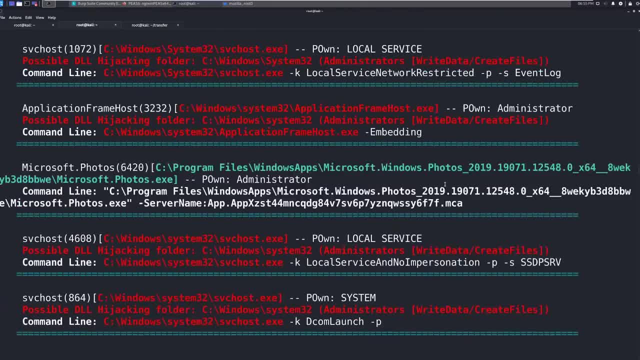 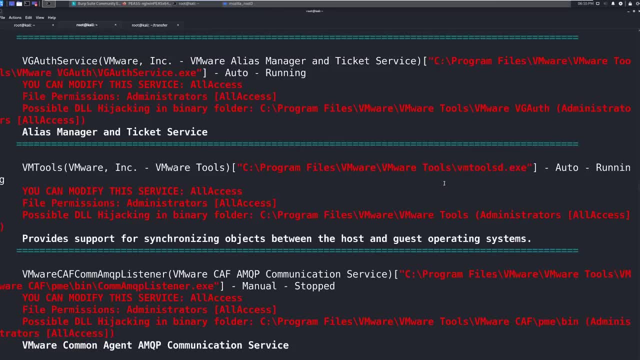 I'm going to skip past processes. I'm not too concerned about what processes are running. That could take a long time to scroll through. When we're doing privilege escalation, we are looking for quick wins. So we got some service information And in here, there there are. 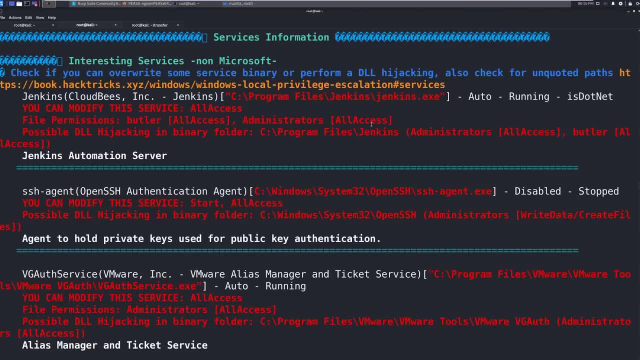 some. okay, there something does show up And this is all lighting up red. So I'm looking and reading through: here we have the ability to modify services, like we have the ability to modify Jenkins dot exe. perhaps we can modify that and write a shellcode here and get a shell. 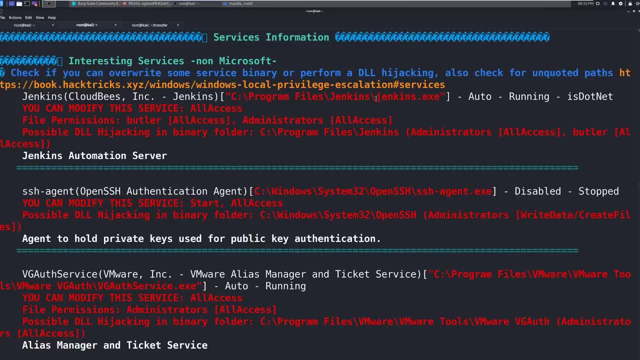 since we're running as this user, But I'm not sure that that's going to run as as administrator. it looks like file permissions here. we'd have to be able to hijack that binary, So I'm going to scroll through Again. this is disabled. we might be able to enable this. 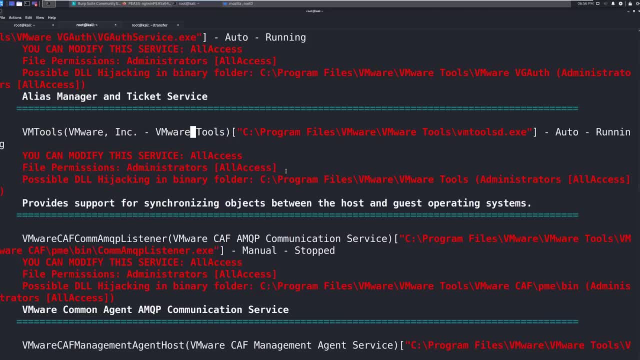 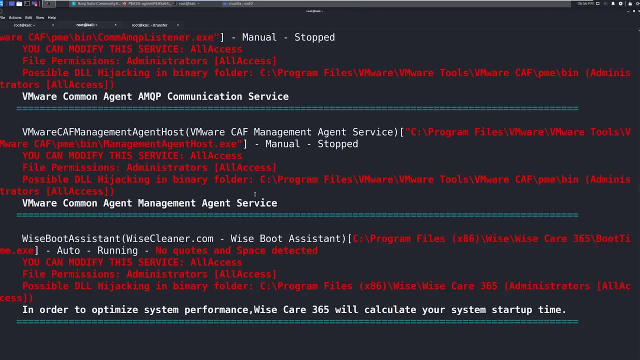 VMware. I don't ever attack. I don't know if that's really truly an attack method, even though it shows up a lot. The other one that showed up that's interesting is: here we have this wise boot assistance, which was that wise care that we saw downloaded. So 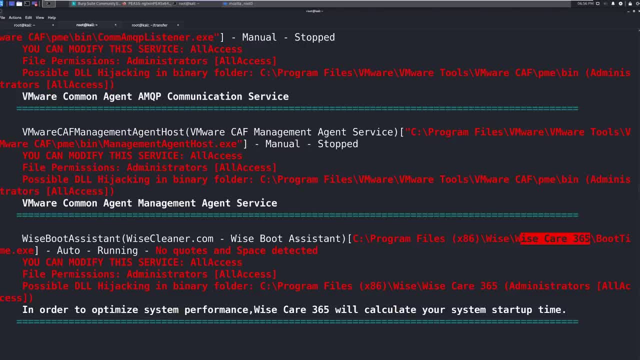 that's of interest, because we did see that downloaded. we do see this running And what's weird is: okay, it's running, it's auto running And it says no quotes in space detected. It said you can modify the service all. 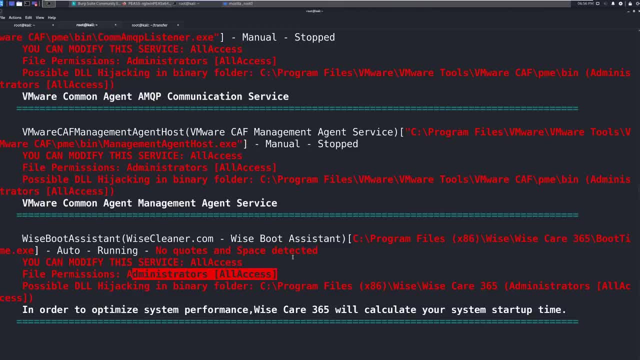 access file permission is run as administrator. That's very, very interesting. So let's talk about what we're seeing- And I know this could be a little bit overwhelming because this is just kind of throwing privilege escalation in your face from a Windows perspective, And that can get. 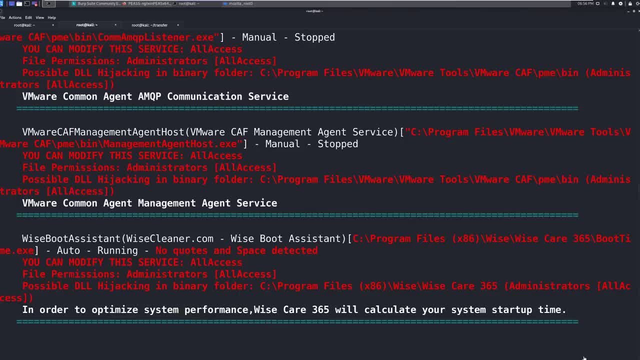 pretty messy, pretty quick, depending on what you're looking for. What we're looking at here, and why this is important, is we're looking at a privilege escalation that will allow us to to get system on this machine, And this is called unquoted service paths. I'm going to show you what. 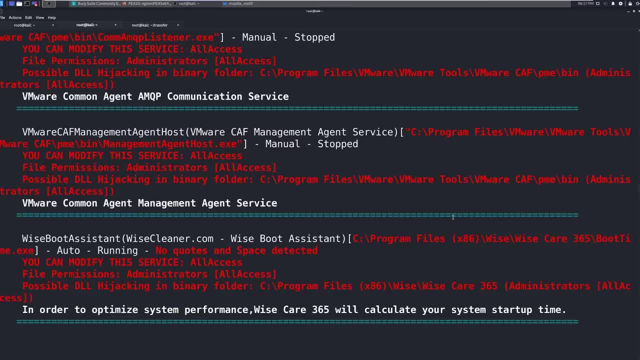 this looks like on the Windows machine, But basically what's happening is the service executable. that is here the service executable. it is located in a path that is not enclosed in quotes. okay, so you see no quotes And there's a service executable that is located in a path that. 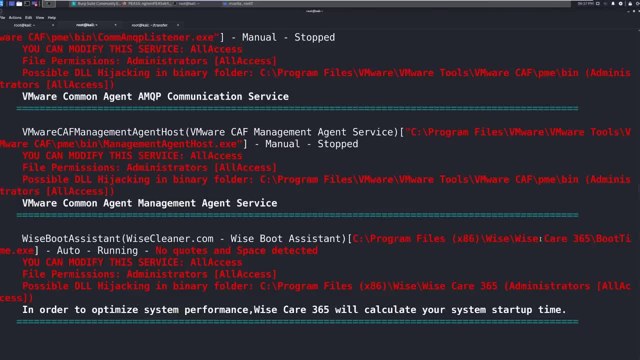 is not enclosed in quotes And there's a space detected. So you see a space. you see a space. Okay, the issue here is that when we're running this, when Windows runs this and it looks for this service, when you start the service up, it's literally looking for every instance. 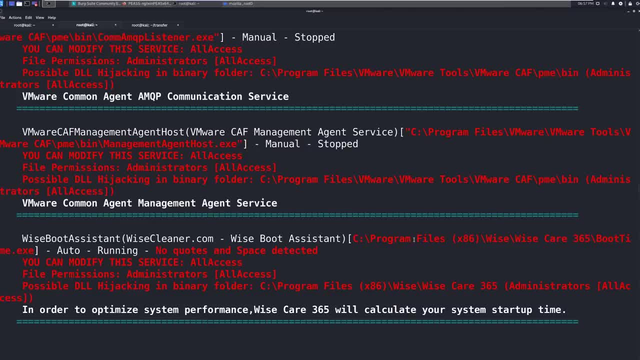 that exists before the space and trying to add dot exe. So it first tries C program, dot exe, then C program files, that exe, Okay, keeps going on And got chin cap Now. So this is actually kind of going like G bunun, not use him. 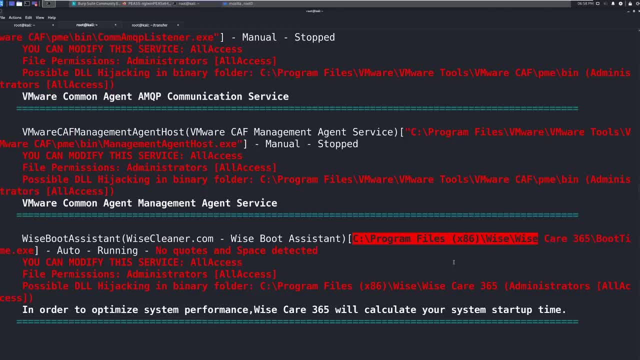 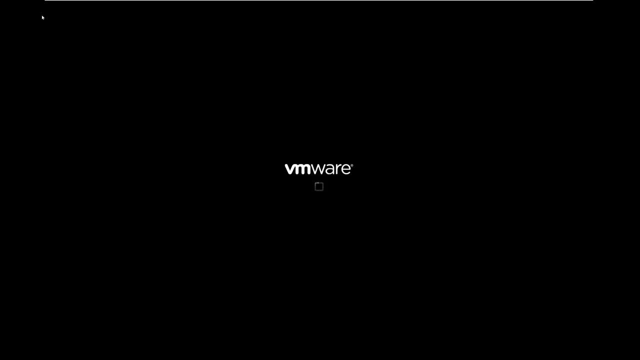 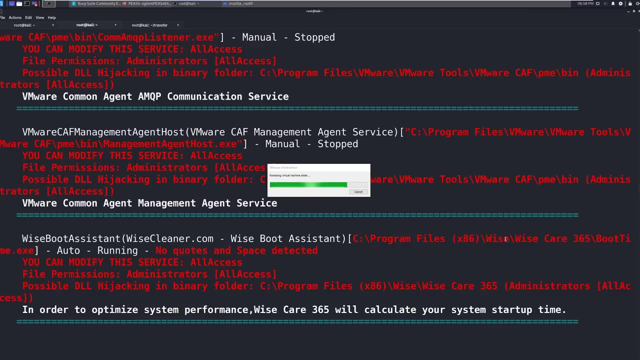 But it is going by the��GoV, Doesn't it? We need to add an exe variable over here. consider: nice can come um, I don't what happens here. So yeah, from here, C wise dot exe, or wise forward slash, wise dot exe, wise care. you see, okay, and what's happening is, I think, my machine. might have just shut down on me. I'm going to go ahead and turn this back on, as I was going to show you. what's happening is we can take an executable- malicious executable, basically malware- and we can upload it to this mach high value, replace it in one of these folders. we don't have to overwrite this, by the way, not the boot average. 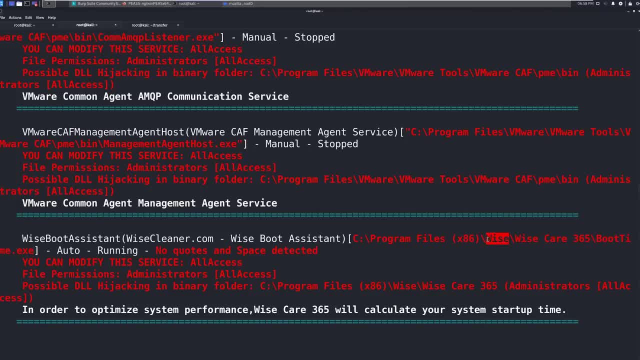 Run back to our built from habnet exe. we can literally just write something called wiseexe. As long as we have permission to write into this folder, we can do that- And then we can run it and hopefully we can get a shell out of that, because the system is going down and it's looking for wiseexe. 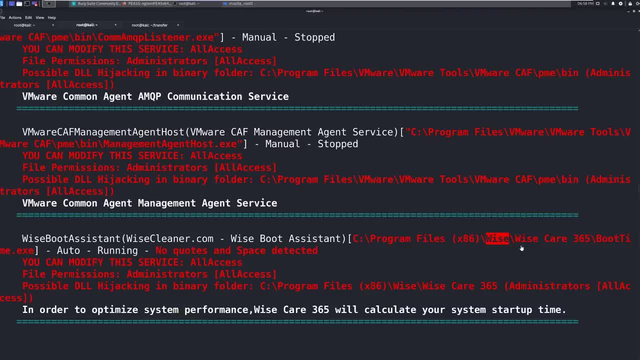 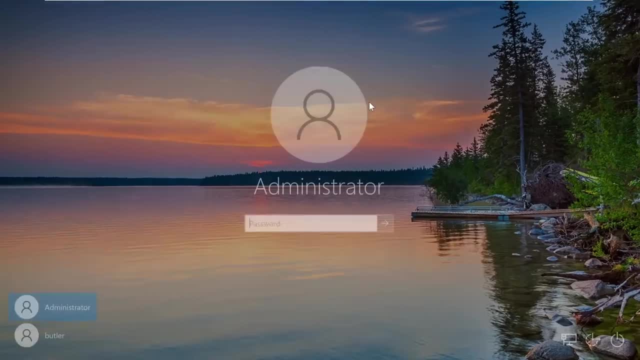 And when it finds it, it will run that first And then it's going to. we're going to attack it based on this. So I want to show you really quick on the windows side of the things. Um, of course, I am locked out of the administrator account as well. Okay, So what I've done in. 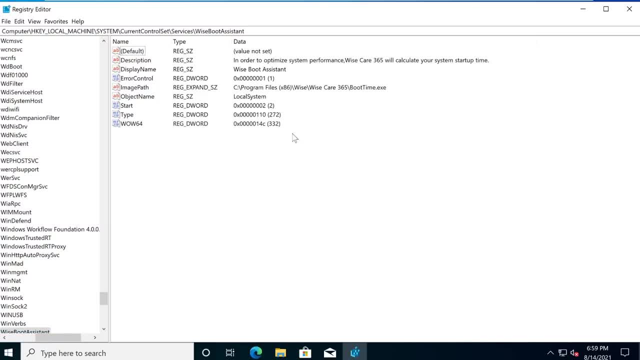 here is. I've gone out and I've looked for this um service in the reg edit. You don't have to follow along Um, but this is an H key, local machine system, current control set services and then the wise boot assistant. When we say unquoted service path, if we look. 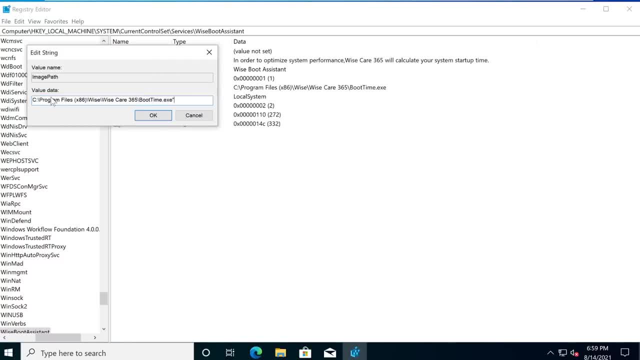 at this image path here there should be to prevent this attack from happening. There are no quotes around this. There are not quotes around this, So this is called an unquoted service path, meaning we're not taking the literal path of this. Thus, when 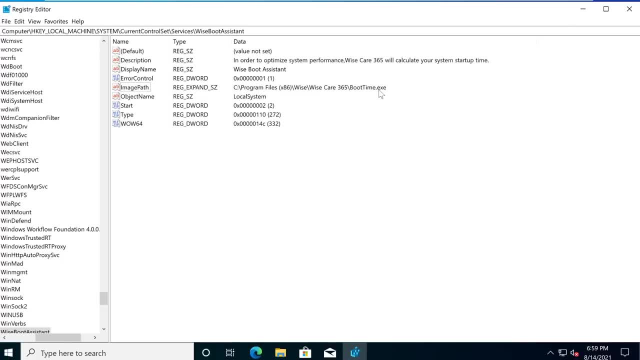 we run C program files X 86 wise all the way through for this boot time. it's going to do those checks Now. I don't know if we have right permissions to the C program files folder as a user, but we certainly should have right permissions here since we installed. 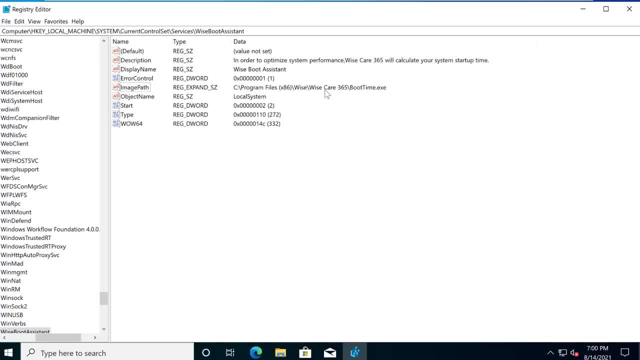 this. it looks like as the user Um. so if we have right permissions to this wise folder, we can go ahead and just drop a file in there called wiseexe And it will try to run wiseexe in that folder. Okay, so it'll go see program files: wise wiseexe is going to. 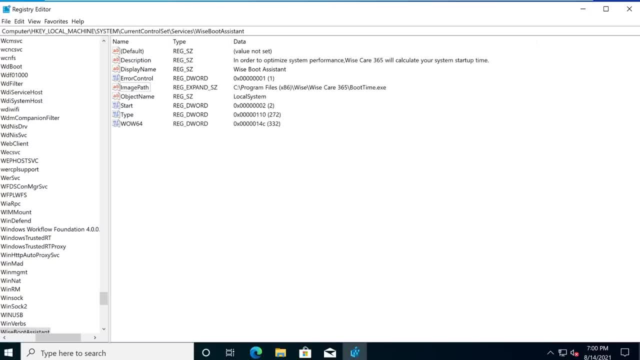 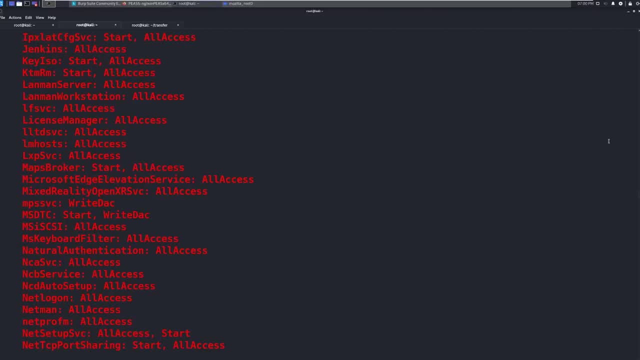 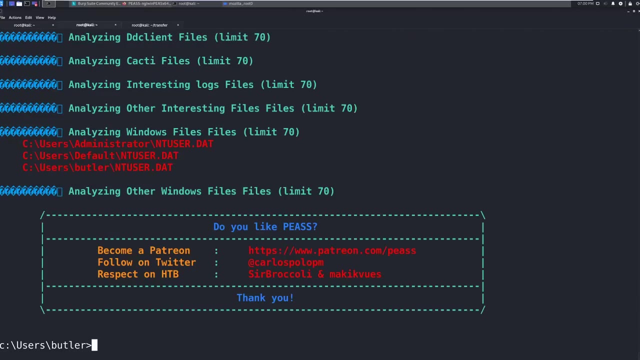 exploit this situation here, And hopefully we will get a shell out of this. So let's go ahead and give this a try. What I'm going to do is I'm going to scroll all the way down here and look at all this mess. There's a lot. Now there are other tools that can easily identify this. by the way, 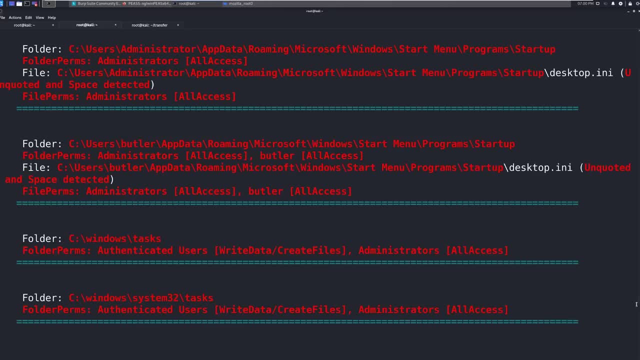 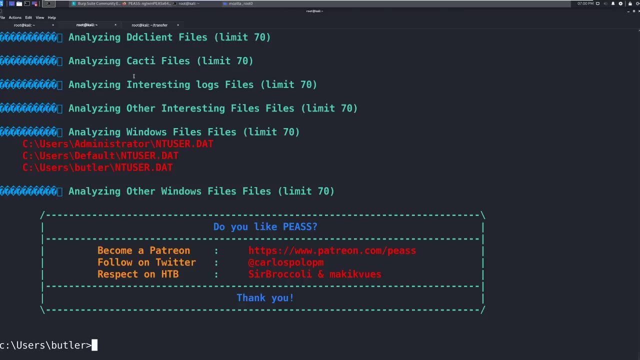 like this. tool is probably the most comprehensive And that's why I showed it to you. But there are tools called power up which will do this. there are exploit checkers that will do this. There are other ways to run through machines like this and do escalation checks. I'm showing you the most. 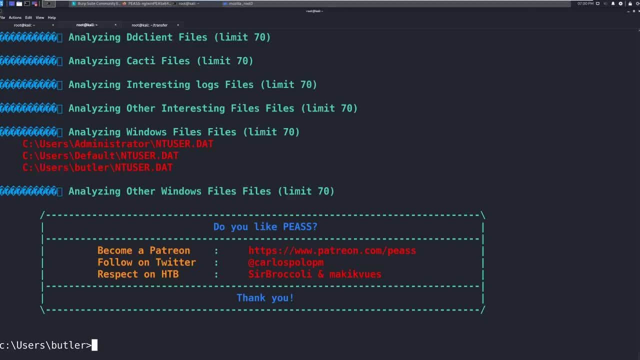 probably popular tool, but it is the most comprehensive and it can be overwhelming. So please don't feel overwhelmed. You will with probably popular tool, but it is the most comprehensive and it can be overwhelming. So practice and, over time, learn how to decipher this. read through it really fast and know kind. 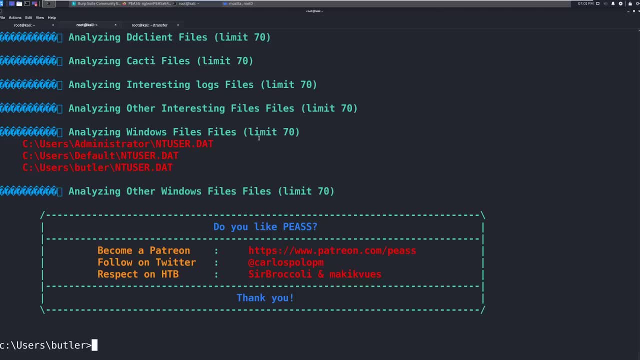 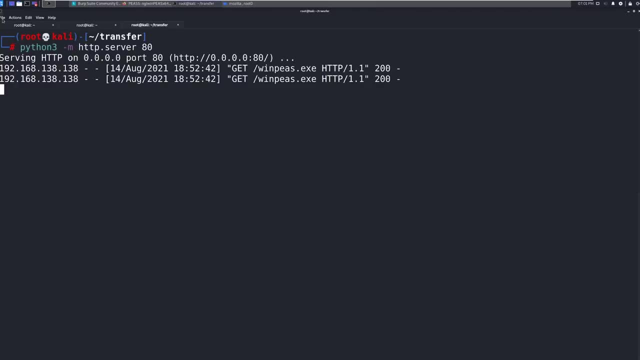 of what you're looking for. train your eyes for those things. Again, this is just introductory, ground level type stuff. So what we want to do is we want to generate some malware. I'm going to go ahead and stop sharing this folder real quick, because I'm going to put malware into this. So 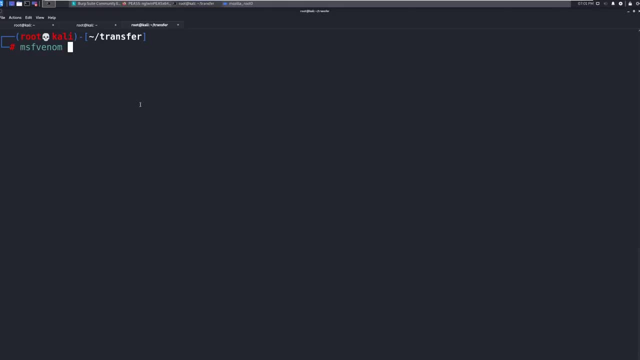 we're going to use MSF venom And we're going to use this to generate some some shellcode here. Okay, so we're going to do a payload of Windows x 64.. We're going to do a shell reverse TCP And if you wanted to do this with Metasploit you could do like interpreter, go down. 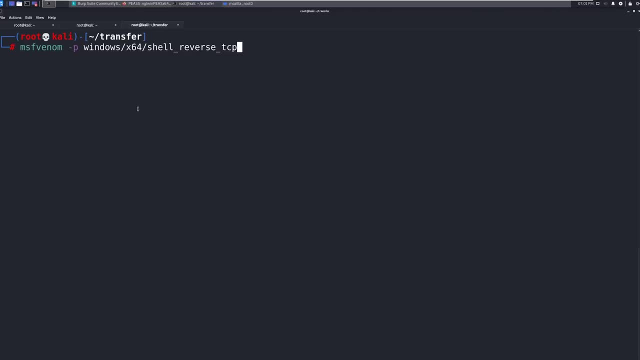 that path, etc. For this instance, we're going to use no Metasploit. We're just going to do this all manually. We're going to give our listening host, which is us 192.168.138.131.. This is your attacker machine. We're going to give a listening port. I'm going to call this. 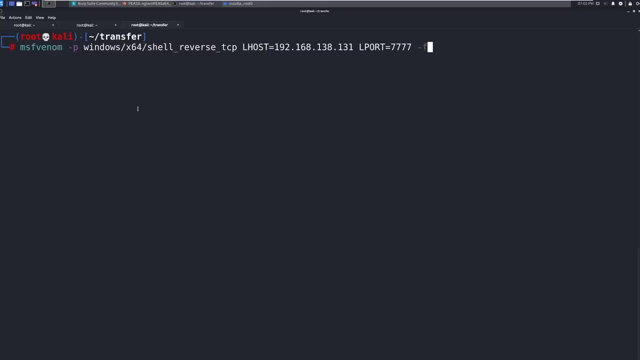 7777.. Do a file type of executable in an output of wiseexe. You could also do this as wiseexe, just like that, All right. So we're going to go drop this once it generates into the wise folder. So I'm going to go ahead and put this back up as a transfer. So my transfer folders back up and 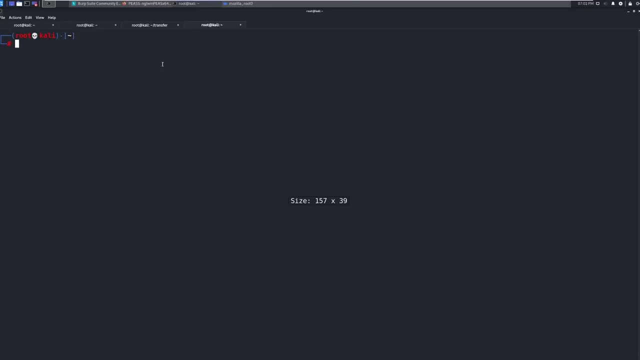 running. I'm also going to open a new tab And I'm going to net cat and the LP And we're going to listen on all sevens, because that's where we said that this is going to work. So we know this is 64 bit architecture. We saw that. by the way, when we were running system info, we saw that. 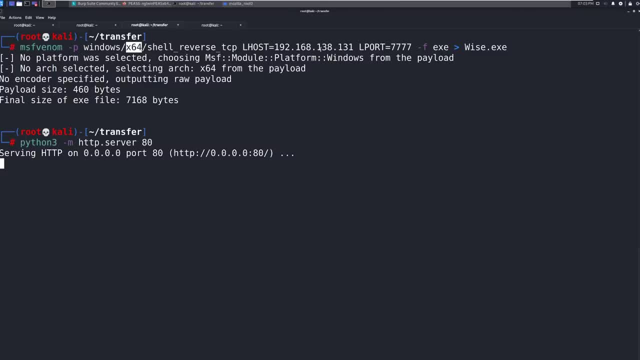 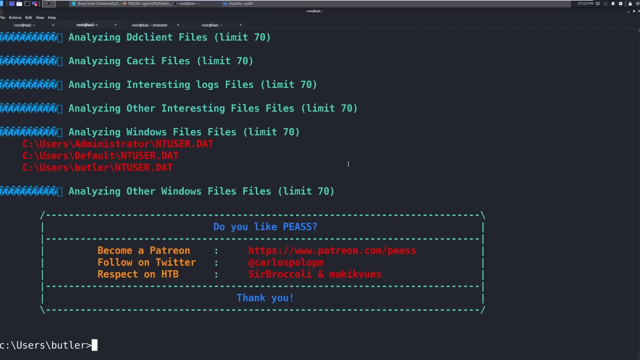 this is Windows 10 64 bit architecture. So this is all all from our little bit of a enumeration that we did. Going back to this machine, we need to go ahead and get into that folder. So that folder was in C, So we're going to CDC And we're going to go ahead and do a quick. 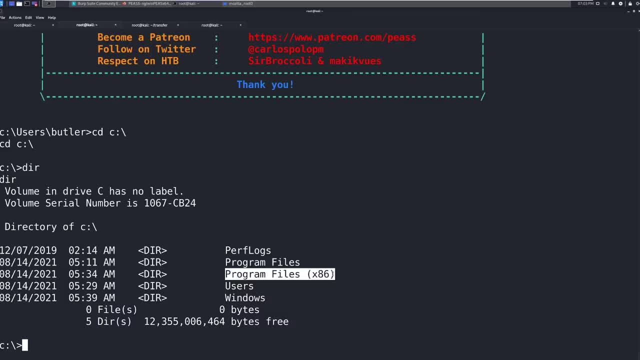 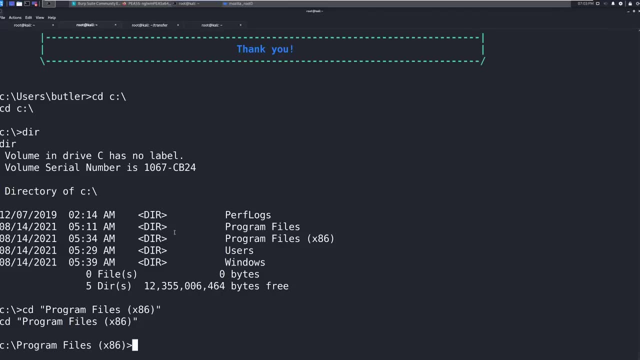 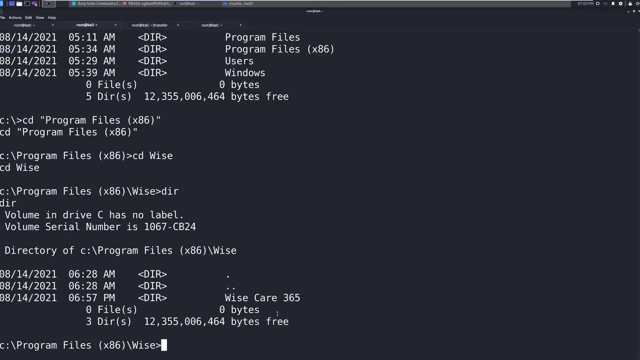 dir And it's easier for me to just copy like this And then do a CD, paste like that. get you in there. CD into wise. Okay, and now we're in the folder that we want to be in. So if we type in dir, we got wise care 365.. So we're. 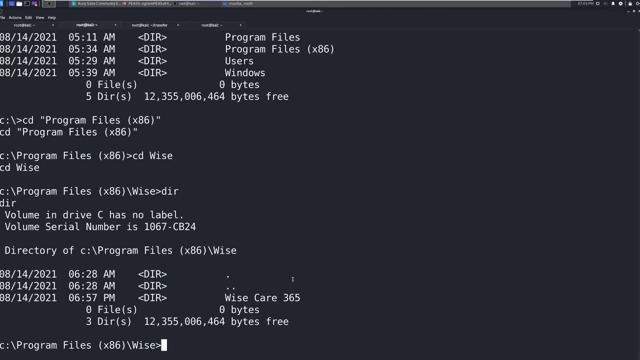 going to put wise in here. it's going to try to run wiseexe And we should be good to go, So we'll see how this works. What we need to do is run cert util one more time. Same way we're going to use. 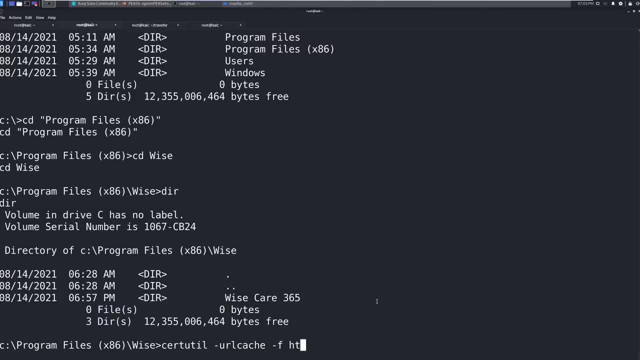 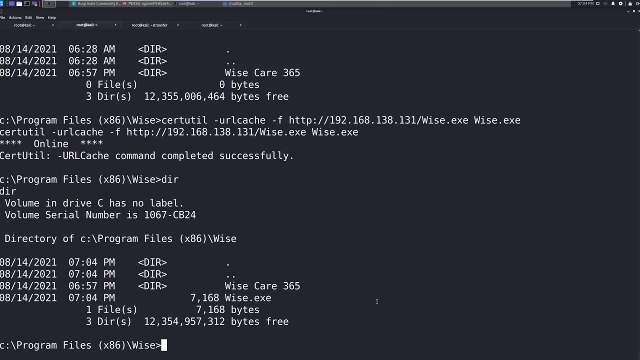 this to transfer a file over, which is nice. HTTP, just like this: 192, 168138131, forward slash wiseexe. Just like that. Hopefully it comes over to a dir. Okay, it's sitting in here, That's great. Now the 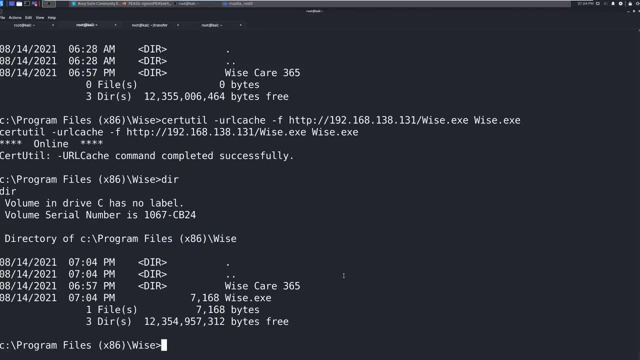 question is: how do we run this? If we just do a dot forward slash or if we just go wiseexe, don't hit enter. If we do wiseexe, that is going to run this as the regular user. It's going to run it as. 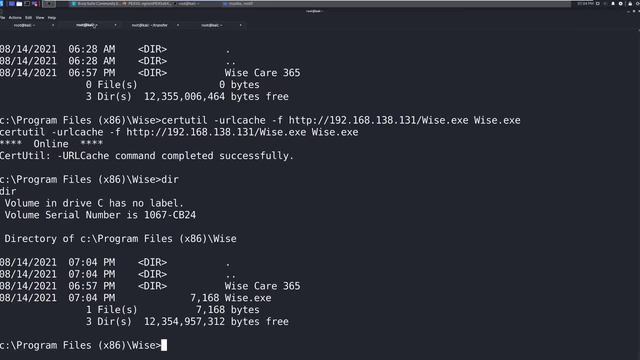 Butler, you will pop a shell back here as Butler and we will have the game: no ground whatsoever. So what we need to do is we need to stop the service that's running. Now the the service that's running is the wise boot assistant. Okay, we can query that to find that out. I'm just 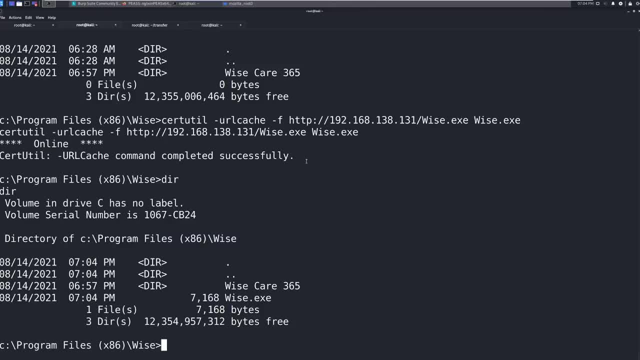 telling you how to do it Just a little bit easier. You can go Google what the what the running service is called. You could look through winps And it'll tell you as well. I'm just just guiding you along, giving you a little bit of information, So I'm just going to go ahead and go ahead, and go ahead and 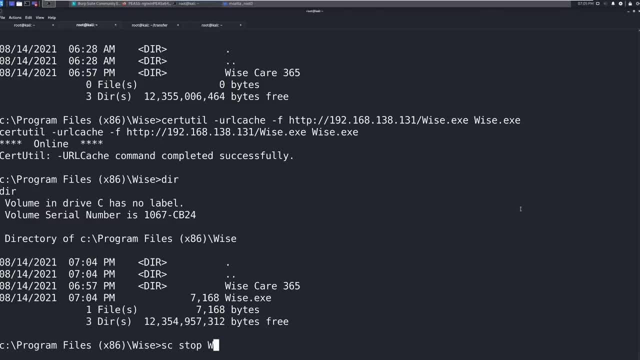 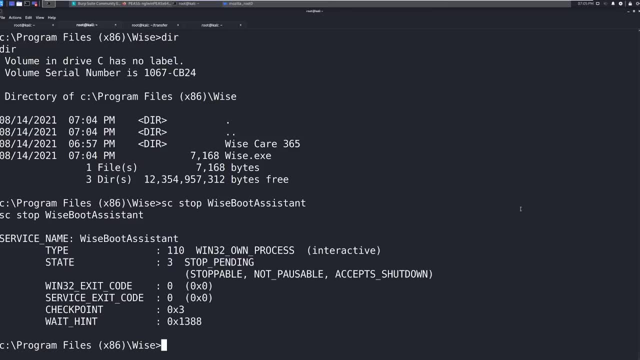 you a quick step ahead here. So we're going to do a service, stop on wise boot assistant. It's all one word like this: Okay, Okay. so it's saying stop pending. it's going to go ahead and stop. that we can do, I believe. SC. query of wise boot assistant. Okay, and you can see that this is. 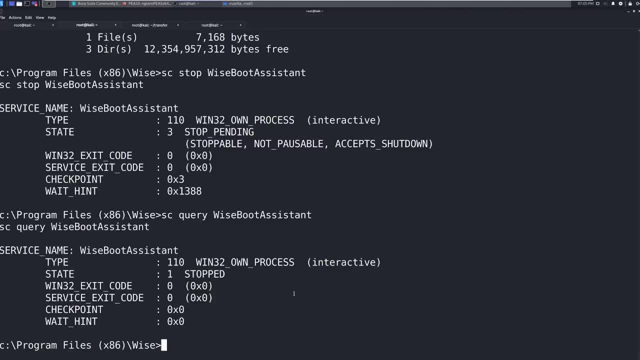 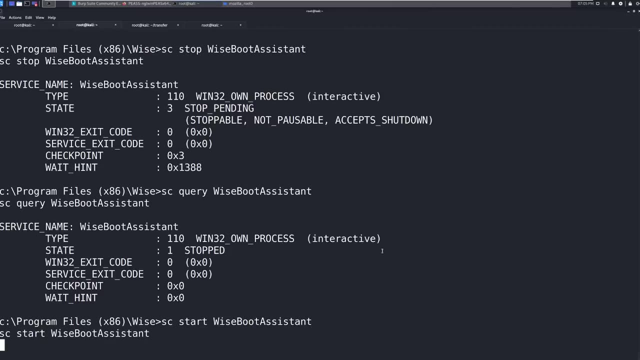 stopped. So now that it's stopped, what we're going to do is we're going to start it. When we start it, it's going to execute as the system. It's going to run that shell code as system and hopefully we get a shell back as system. So you see, the shell came through. We say: who am I? 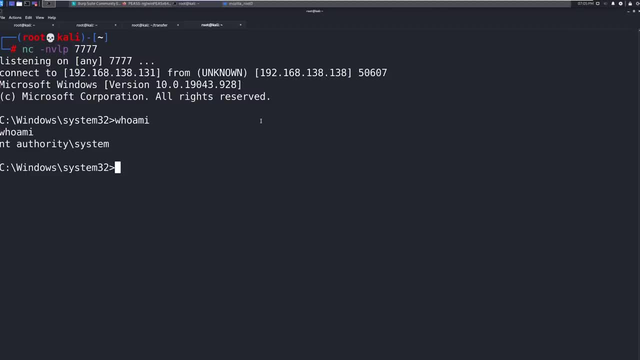 authority system. And that is it. So this is a very, very classic, absolutely classic way of exploiting a machine. So I'm looking through the printout of win piece Again. there are other tools out there that do this. there's actually even a check that will do this from a one liner. There are privilege escalation. 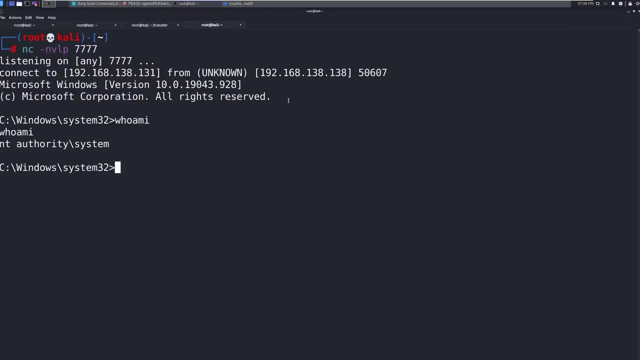 checklists and guides that you can go through. So when you get on a machine you say, Hey, I'm going to check this first, then I'm gonna check this next, and you go through the checklist and make sure you leave no stone unturned. You kind of get your low hanging fruit, like you saw with the Linux. 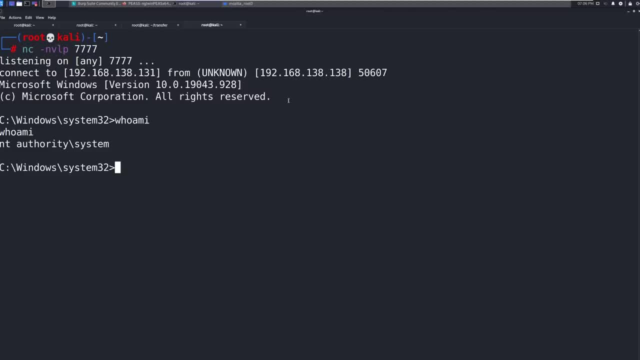 like we'll check history first, because maybe there's a password stored in history. then we'll check sudo and see if we have a problem. Okay, so we're going to go ahead and go ahead and do that. So we're going to go ahead and do that. 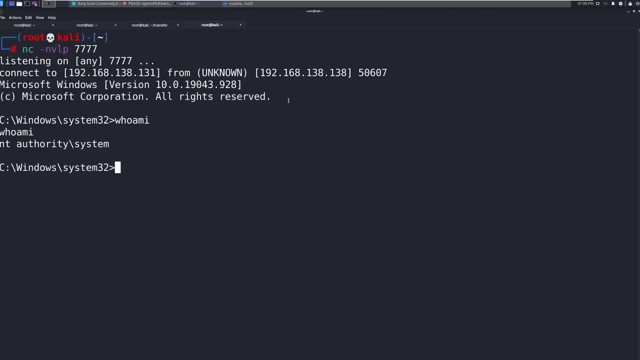 If you have any privileges and and kind of go down the easy list. Same thing with system info. I want to see what the build is- if I can recognize the build- there's something there from trained eyes- and then kind of just go down the list as to what we need to do. Running win piece. 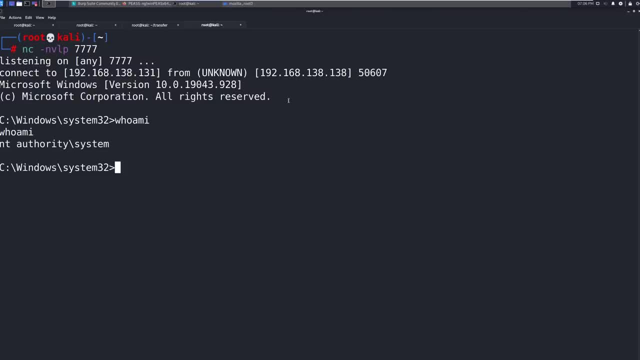 is something that we can execute fairly easy. run through it- Same thing with power up or other tools like that- And we can go through and find issues like this, And this one is a classic. If you do any CTF machines, I guarantee you will see this in the future, So this is a good one to show. 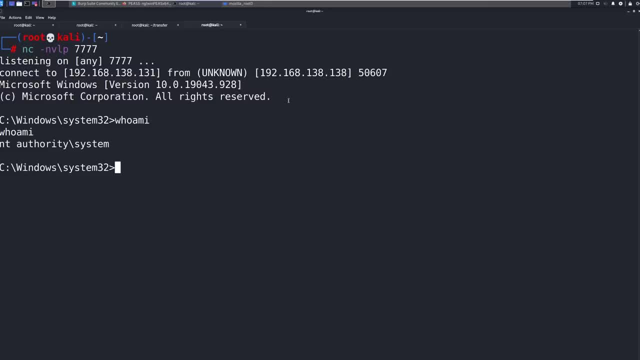 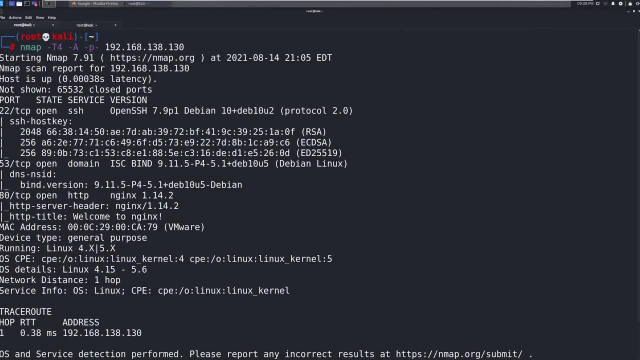 you as an example And build you up into privilege escalation and get you kind of get your feet wet in the game. So that's it for this machine. We're going to go ahead and move on to the next one. Welcome to this box titled black pearl. This box was created by Alec and is a Linux machine. Thank, 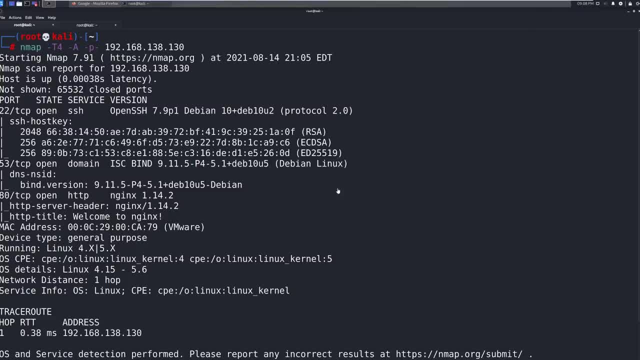 you, Alec, for creating this machine. We're going to go ahead and start off with our nmap scan, As always. if you haven't found your IP address, go do that. get your nmap scan going, If you just want to follow and watch. 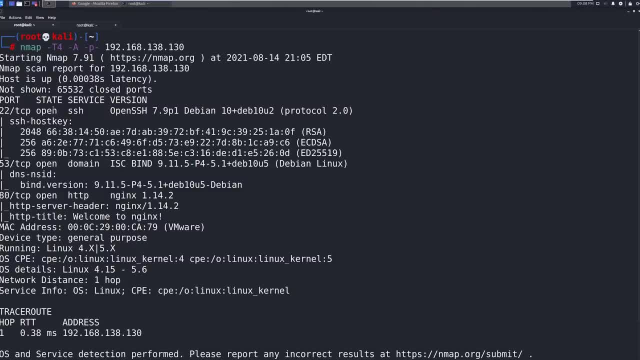 along and continue from here. that's fine too. Now our nmap scan only shows us here with port 22, DNS 53 and port 80.. As discussed in the past, 22 likely not the option. So that really leaves us with 80, because 53 is likely not the option either, though it does come into play a little bit now. we. 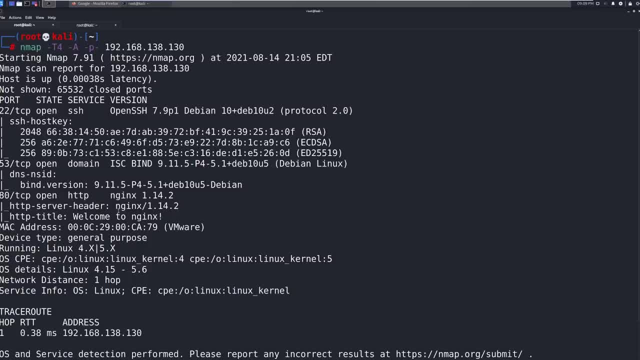 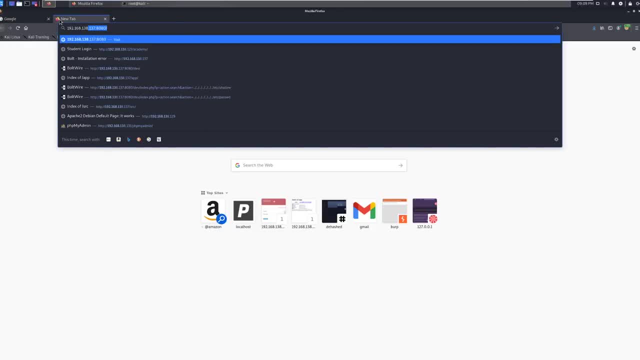 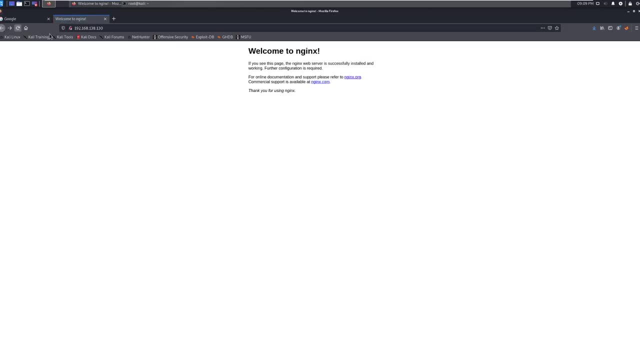 can see we have a default web page Here just by looking at the the title: this nginx. we have a welcome to nginx. meaning if we go out to this website, we go 192.168.138.130. uh, and i turn off my proxy and refresh. oops, and refresh, we get. 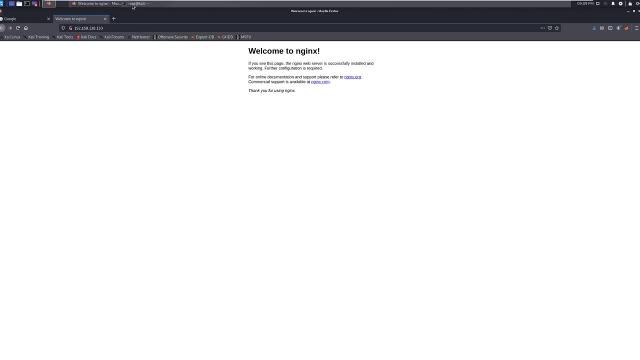 a welcome to nginx page. so what do we need to do? we probably need to fuzz this and see where we can get with this information. um, so we're going to do a quick fuzz on this. uh, something else that's, i think, hidden in here. let me view the page source. it always helps to define the page source in here. 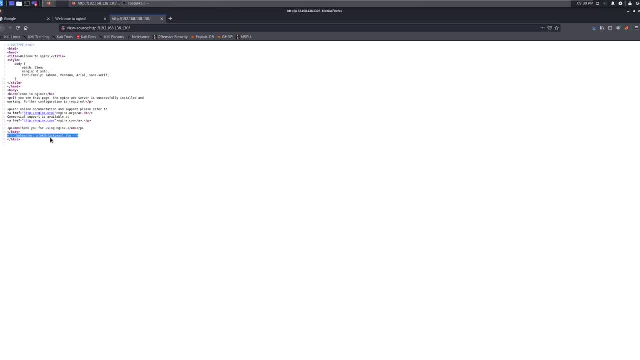 you can see that there has been a little nice thing added in where it says alec at blackpearltcm. so that's your webmaster. let me make it a little bit bigger: alec at blackpearltcm. this is a big hint giveaway, something we haven't covered quite yet, and we're just going to keep that in the back. 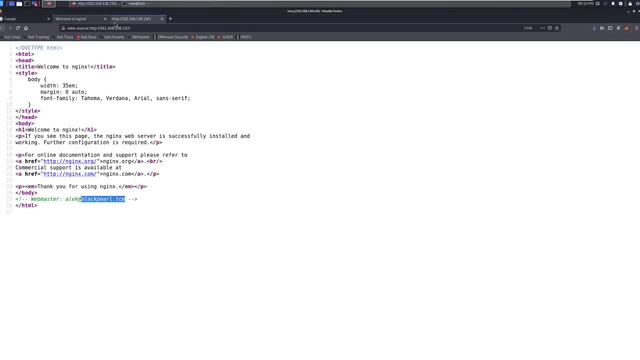 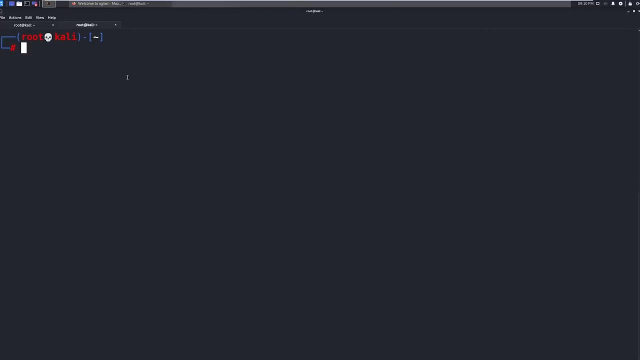 of our mind, but we know that we need to access this web page. we're going to go ahead and try to do some directory busting first and see if we can't get there with that. so let's go ahead and take a look at the directory busting and then we'll go from there. so new tab we're going to do. uh, do dash w user share. 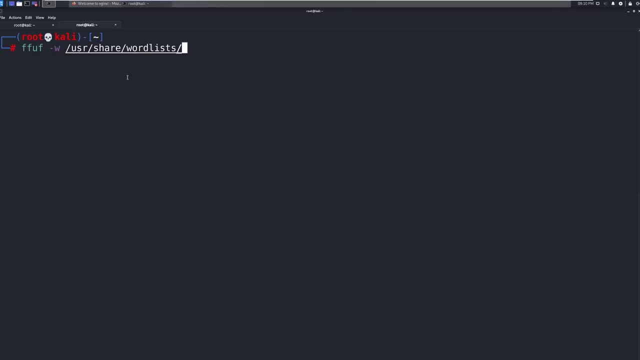 word list. this should be starting to feel a little bit familiar, right? uh, dir buster for me. and then just tab through to get to the medium list and then go ahead and say fuzz. and then we're just going to run this with the ip address- for me it's 130, slash fuzz. run that and see if we can't find. 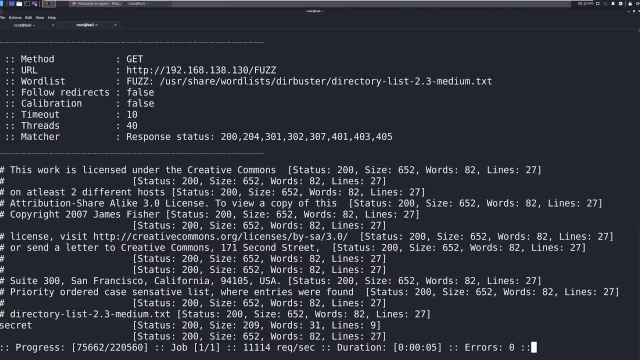 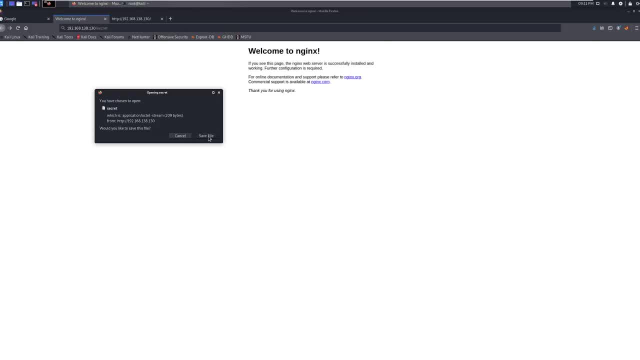 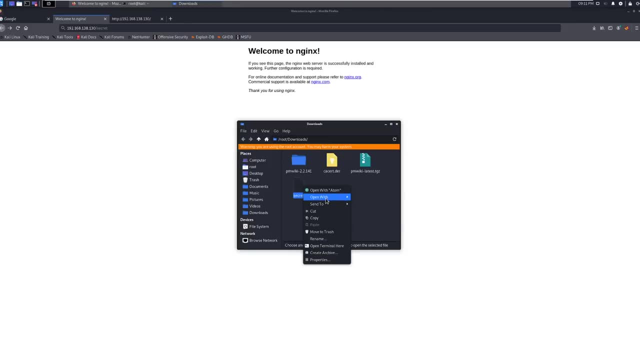 anything and immediately we get something called secret. so let's go ahead and go over to forward slash secret. uh, it's a file, let's go ahead and save that. let's uh open the containing folder and let's just open this, if we can open up with. 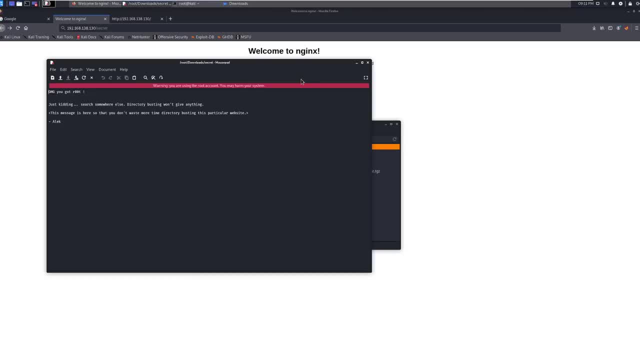 mouse pad And it said: Oh my God, you got root. Just kidding, Search somewhere else. Directory busting won't give anything. This message is here so that you don't waste time directory busting this particular website, Alec. Okay. So what he's telling us is: you're not going to find. 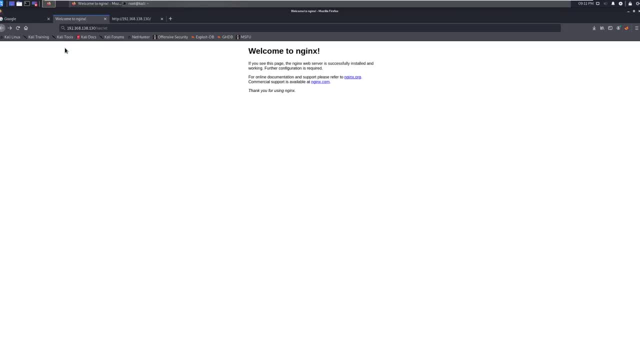 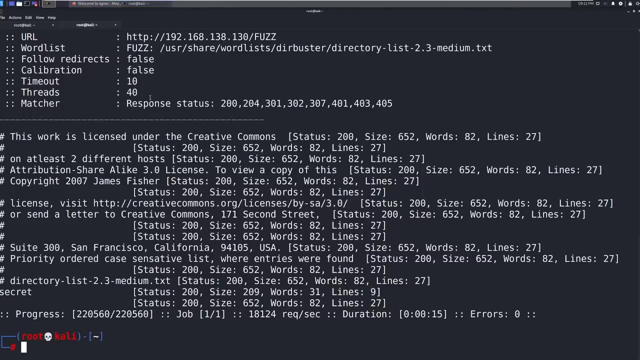 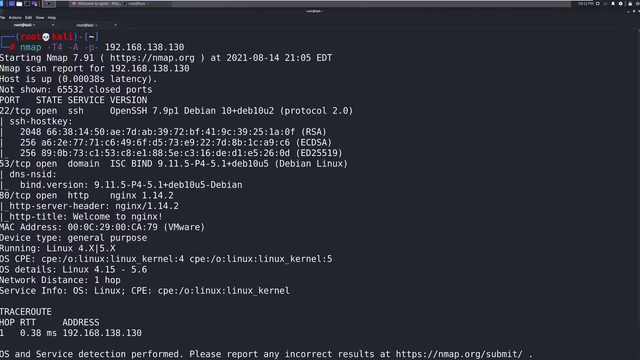 anything on this directory. Well, we're likely not going to find anything hunting down port 22.. Uh, we're likely. I mean we could attack maybe Alec at 22 with some weak passwords and see what we find. Um, but that's not the entry port And here we have 53, which means that this is running. 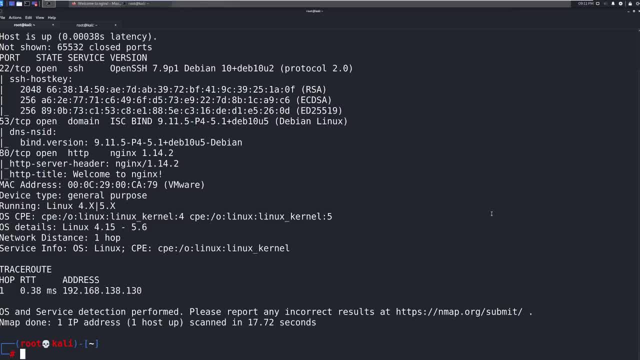 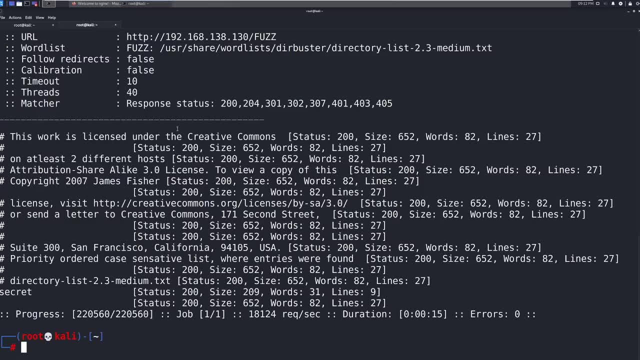 DNS and it's running DNS for a reason. So we're going to do some recon on this. Um, what we're going to do is we're going to just say- and I'm actually going to run it over here- We're just 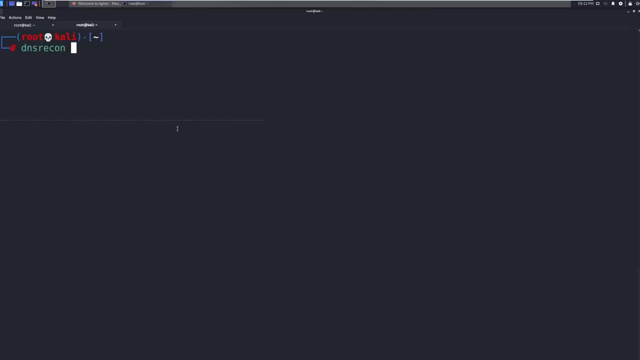 going to use a tool called DNS recon and we're going to say dash R And that is for our range of 1, 2, 7, 0, 0, 0 slash 24.. We're just scanning the local host. 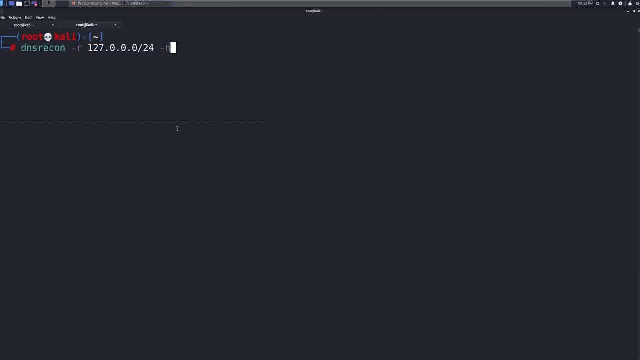 because that's where our machine is. And then we're going to provide the IP address of the box that we're actually looking for, which is one 30. And then, for D, you can literally type in whatever you want. We can just type in: blah, D is just needed there for a dictionary, but we're 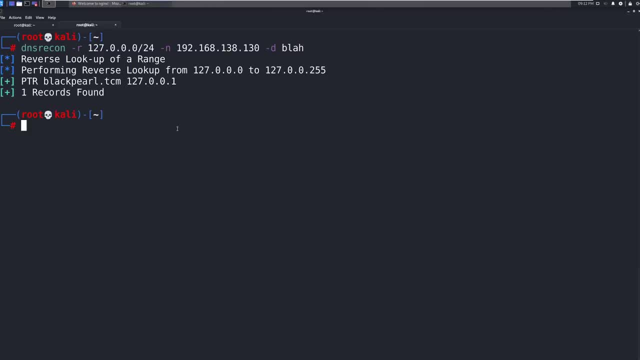 not going to use it And it's still gonna be able to find it. If we take it out, it won't work, which I'll show you. Or D for domain- I'm sorry, not dictionary. D for domain. Um, it's we're. we're providing a domain. 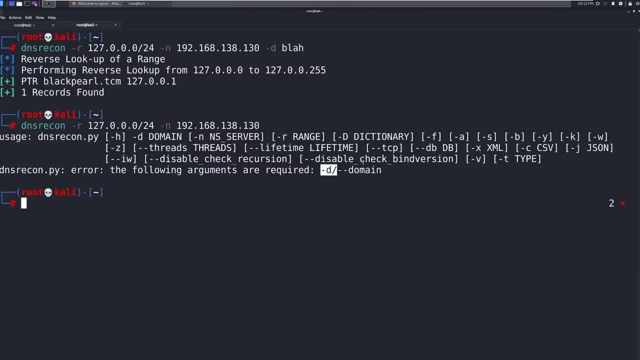 but it's going to look for that domain. But if we don't provide it it won't search, So it requires the domain. even though we don't have the domain or don't know the domain, it's still able to find it. So what I found was 1, 2, 7, 0, 0, 1 at black pearltcm, which means that there's DNS pointer. 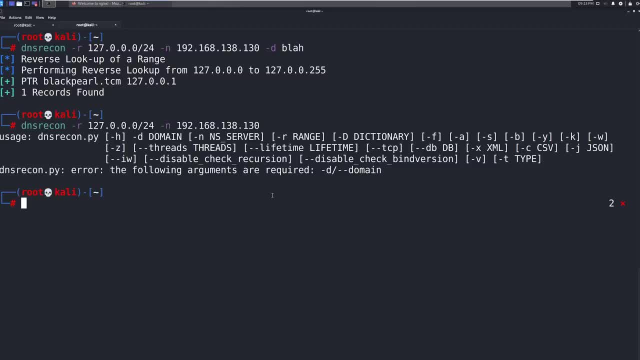 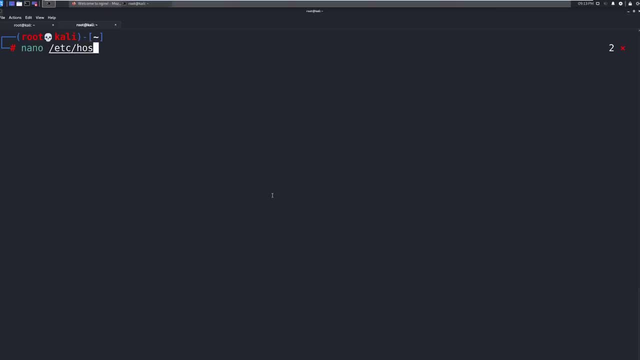 record here to this webpage. We need to go ahead and add that to our DNS. Okay, So what we can do is just nano Etsy hosts, and in here you can see that we have our 1,, 2,, 7,, 0,, 0, 1. 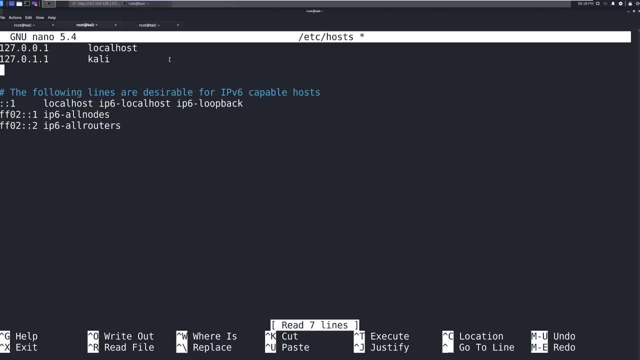 for local hosts and 1, 2, 7, 0, 1 1 for Cali. We need to add in the IP address: 1, 6, 8, 1, 3, 8, 1, 30.. We're just creating a DNS record here. 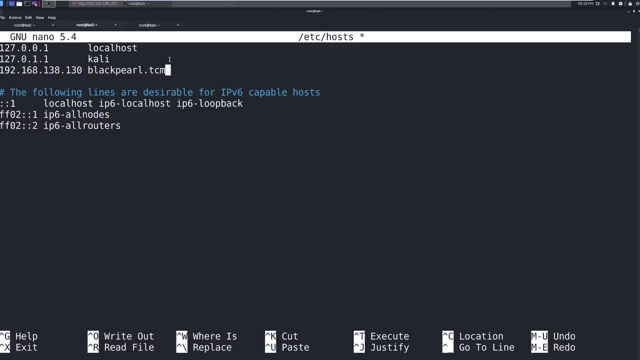 For black Pearl dot TCM. So now we're going to say, Hey, black Pearl dot TCM allocates to this IP address, And DNS is going to do its magic. So we're going to Ctrl X, hit y, hit, enter And then 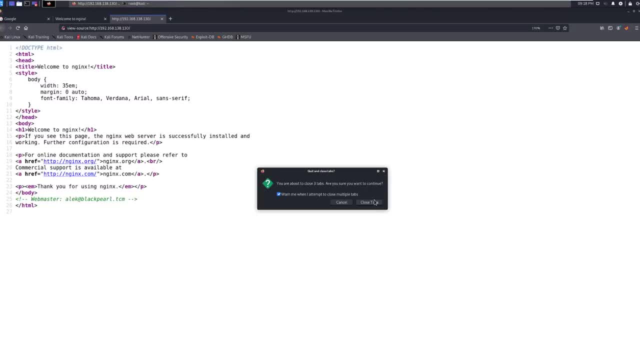 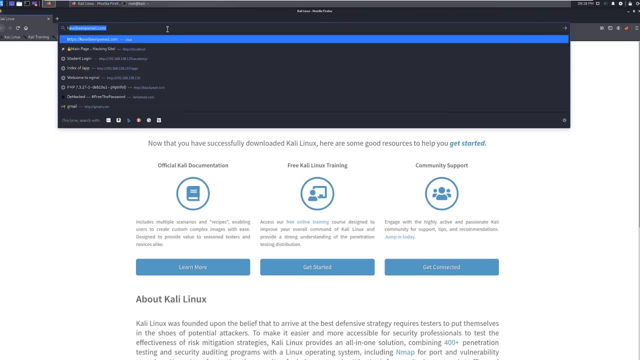 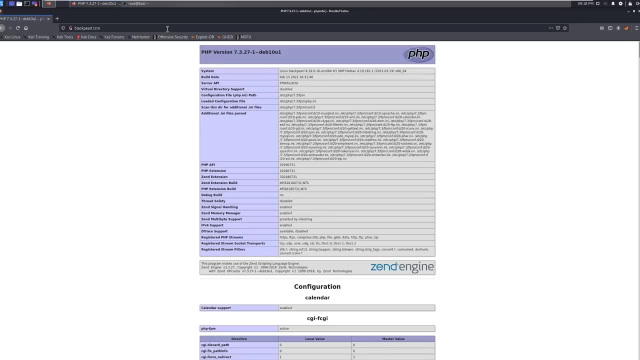 in your web browser, go ahead and close it completely. If you had one open and then we're going to go back, open it up And hopefully this will work, first go so: HTTP double dot slash, slash black pearl dot TCM. Okay, and if this happened correctly, you should see this page. Okay, if for? 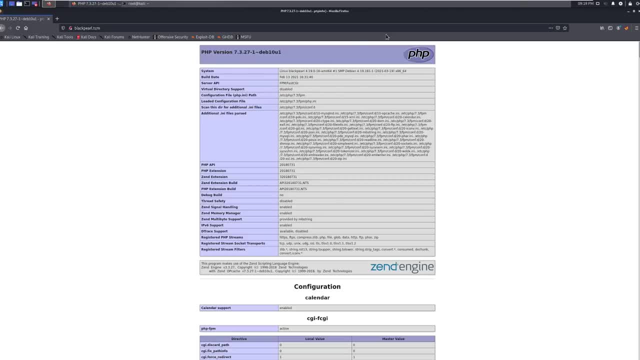 some reason it did not load for you. go ahead and go back, close this out again, give it a second, let it, let it repopulate. So here we are, brought to this, my info page. Now, we have seen this before. 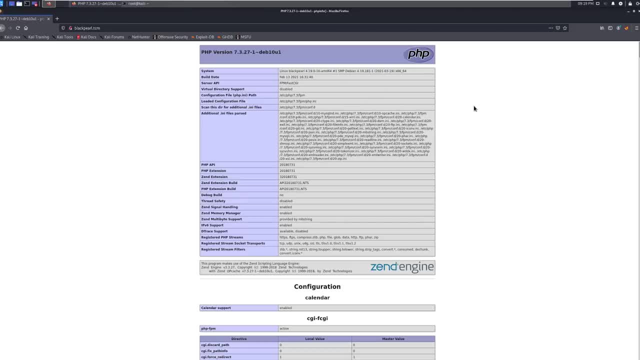 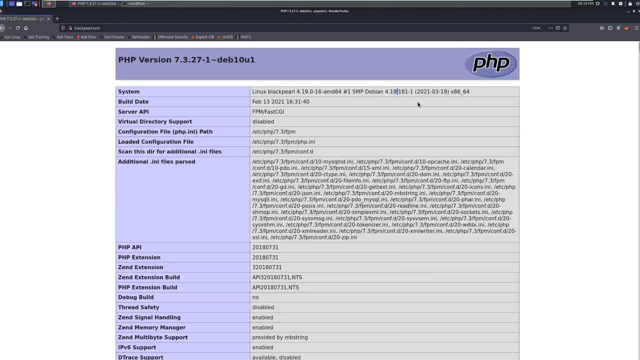 And again we can get some information disclosure here We can see that we're up against the Linux box. We can see the name of the box: Debian, system type. there might be some sort of execution we can run against this, But again, when we're up against a directory like this, we want to do some directory. 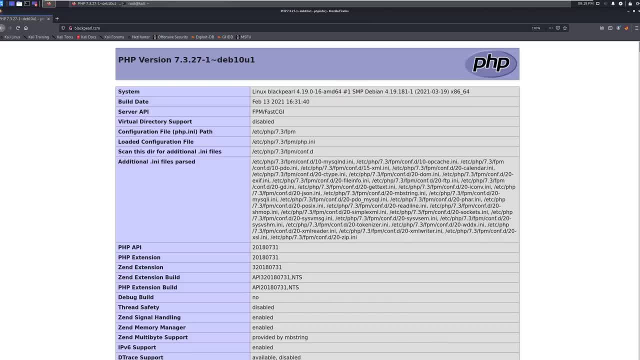 brute forcing and see if maybe we can get access to this machine or get access any further than what we are. So we're just going to want to fuzz the directory one more time and see if that leads to anything. As of right now, this info page is giving us info, yes, but there might be more hiding under. 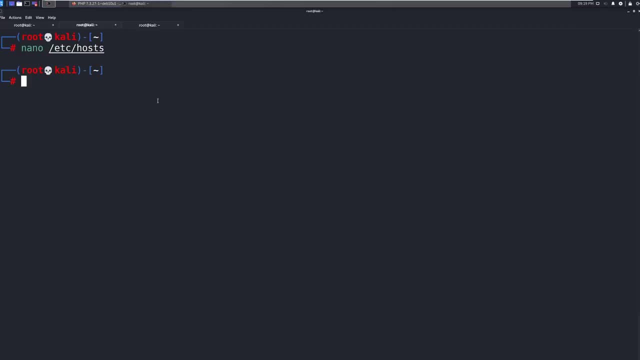 the covers. So we're going to go ahead and go back And we're going to just use fuff, fuff one more time. User share, wordless. And I'm never going to get tired of saying that, der buster, I can type and then do my. 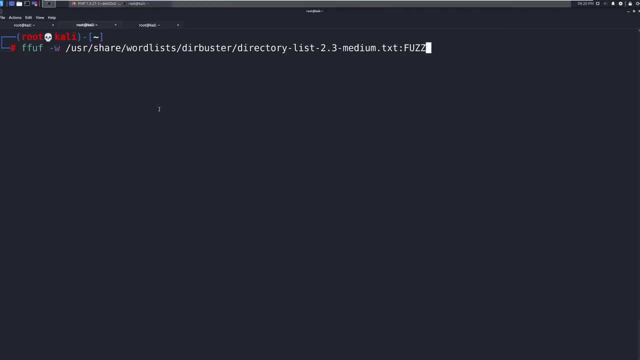 tabby thing. Alright, so we're going to fuzz here And then, this time around, we're gonna do a dash you, and we're going to do black pearl dot TCM, not the IP address, black pearl- And we're going to say: 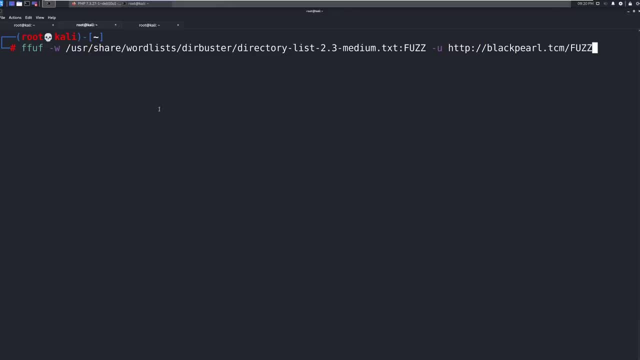 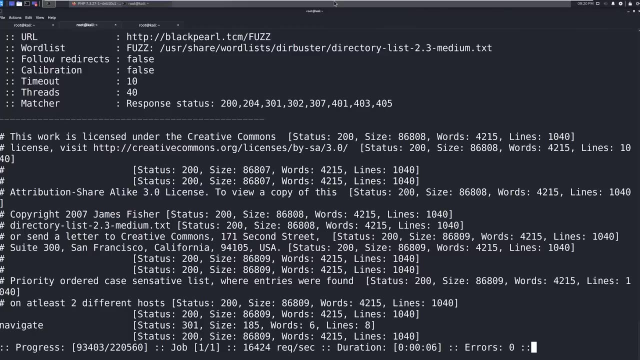 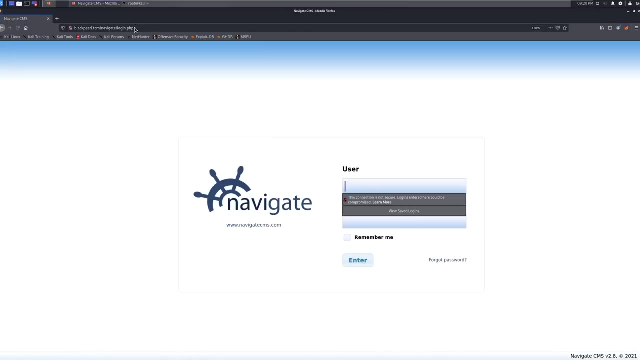 fuzz. Okay, And we're gonna let this go through. we're going to look for anything that might show up and immediately navigate shows up for us. So that's interesting. Let's go ahead and just navigate to navigate, shall we? Okay, we've got navigate CMS, version 2.8.. Copyright 2021.. And we're gonna go. 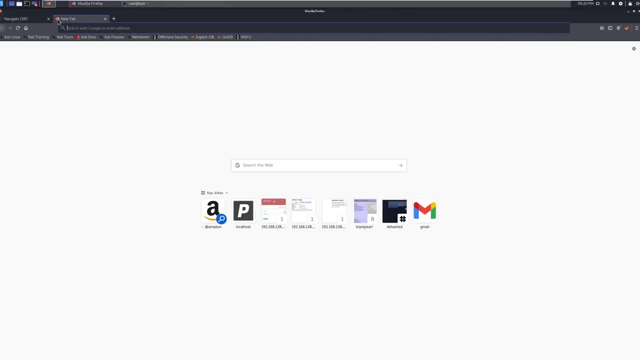 ahead and just dig a little bit further into this. So my go to is always Google, right? So we're going to always Google. just Hey, navigate CMS. we could look for exploit. we could also look for default credentials, if there are any. see if we can go in there. But look at this, we've got unauthenticated. 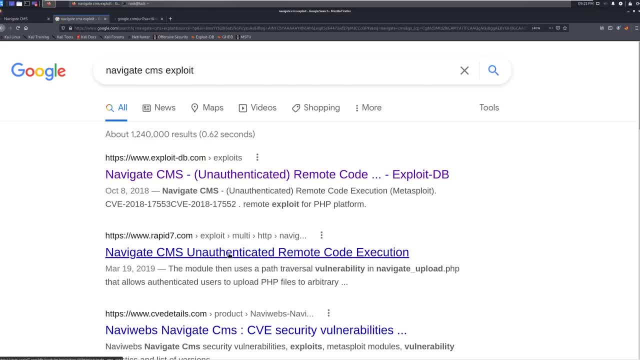 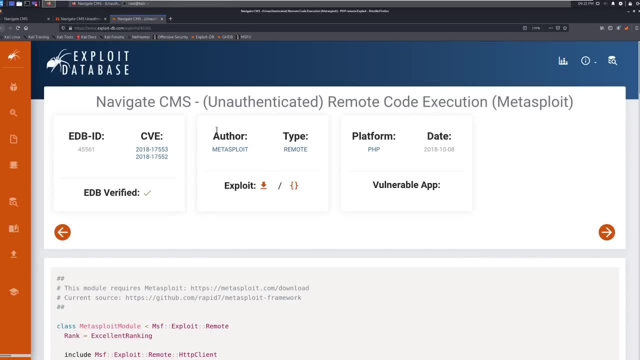 remote code execution from exploit database. we can run it manually or we can run it with Metasploit. So that's nice, We have options. So actually an exploit database is with Metasploit as well. I'm sure there is manual code out there, But for this one, since we haven't run Metasploit, 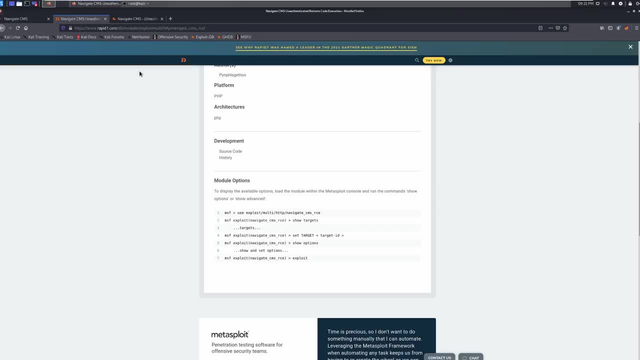 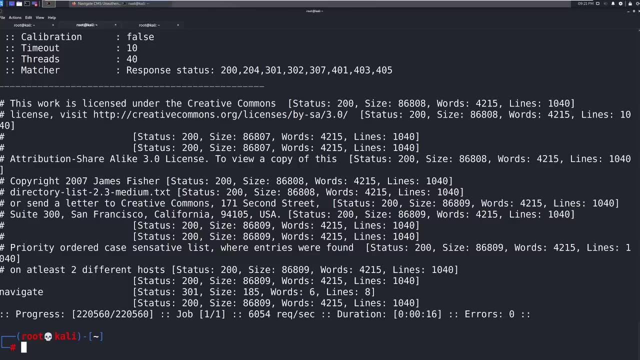 much in the capstone. we're going to go ahead and mix it up and use a little bit of Metasploit here. Otherwise I encourage you to go back and try this manually as well. But we're going to go ahead and open up Metasploit and see what it's got to offer for us. So MSF console- Let this load real quick. 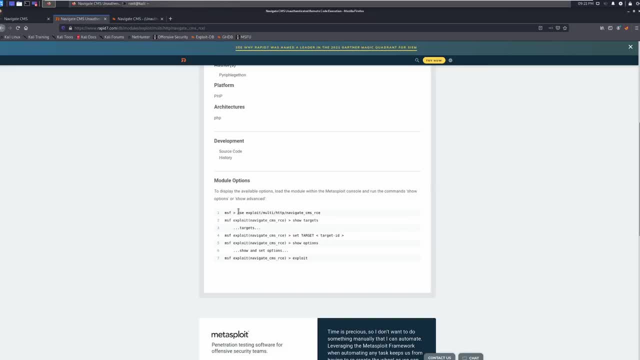 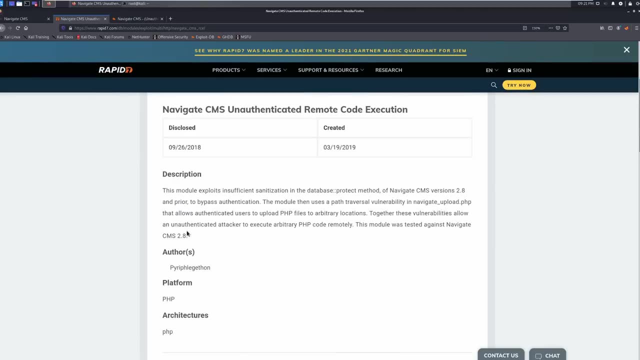 And this gives us the module in here. I mean we could search for it, but it's easier to just like, honestly, just copy this And we should probably verify. Okay, so this is tested against navigate module. exploits insufficient sanitization in the database protect method and allows us to bypass 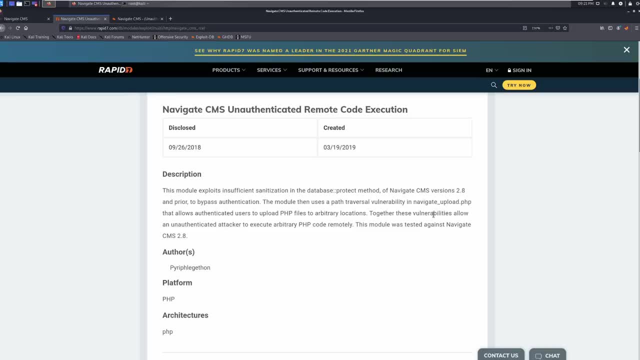 authentication. The module then uses path traversal vulnerability that allows authenticated users to upload PHP files. Together we can get remote code execution. So it's chaining attacks here. First it's going and it's bypassing authentication. It's then uploading malware. 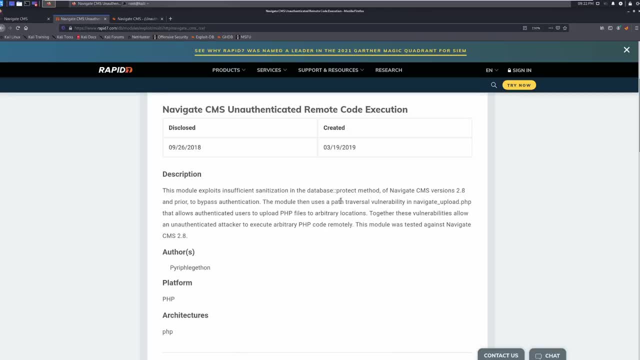 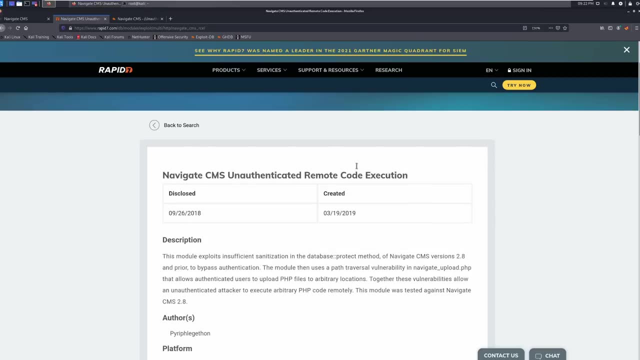 which uses a path traversal vulnerability to do that via the authenticated user And then uses that to do remote code execution. So this is a chained attack here. This is pretty, pretty unique, So we're going to go ahead and go in here and just paste. Hopefully this works This. 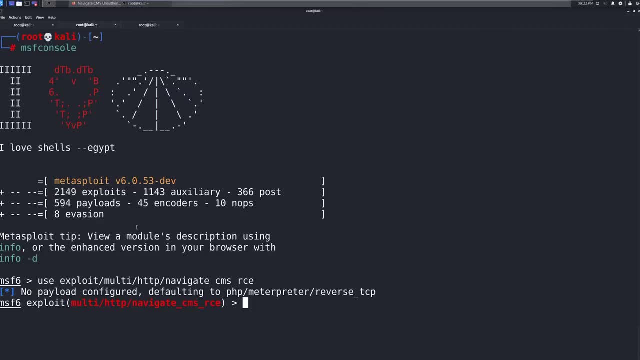 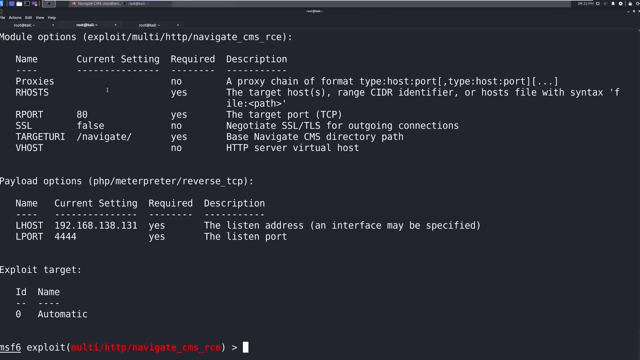 is Metasploit six. I'm on And it does Okay. so when we're in here we get to say options And we're asked for an our host, we're asked for our port. we have our our port, we're asked for. our L hosts, which is fine, I think. And then our host, we're asked for our L host, which is fine, I think. And then our host, we're asked for our L host, which is fine, I think. And then our host. 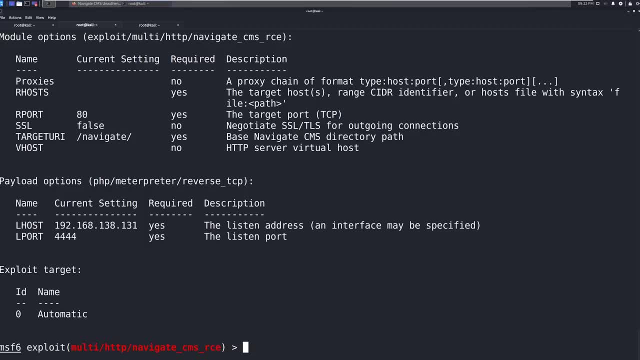 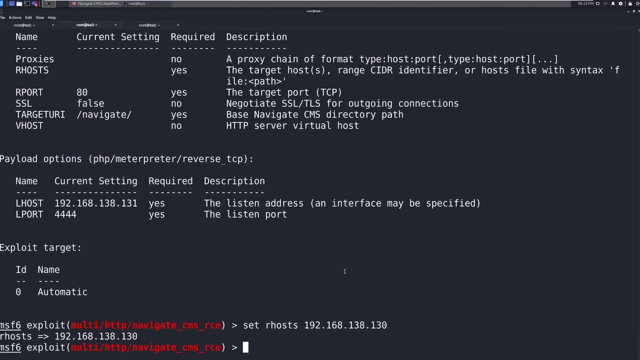 we're that. pH, benim interpreter, Everse TCP looks good. I think all we're going to do is just make sure we set our our our host here, which is going to be 192, 168, 138, 130.. But we also need to set the server virtual host, So we're. 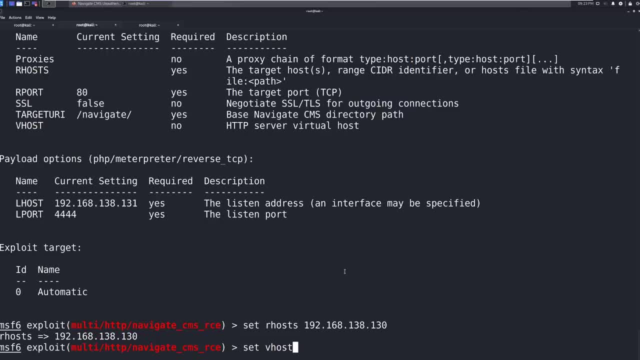 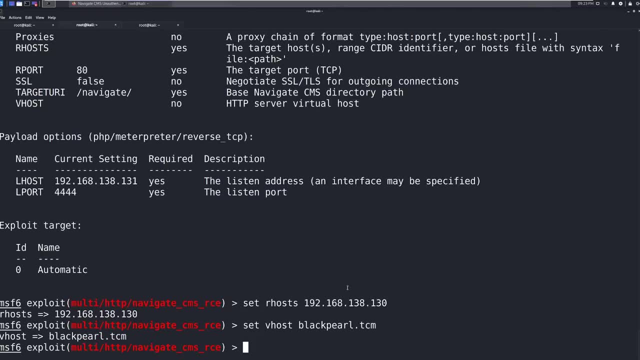 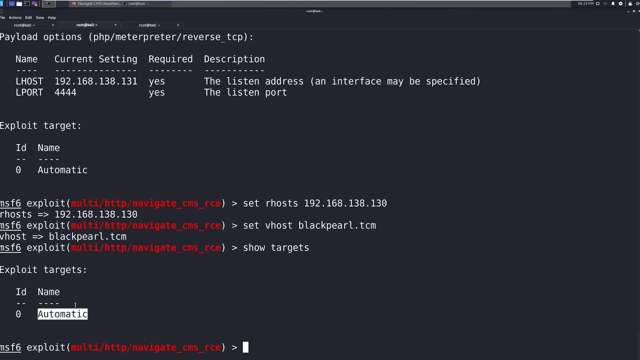 gonna say: set the host to black pearl dot TCM. Okay, everything else looks good. This is automatic target. We could do a show targets real quick and see if there's any other targets. There's not just automatic. This is our attacker IP address. That's fine. All ports fine. Forward slash. navigate as. 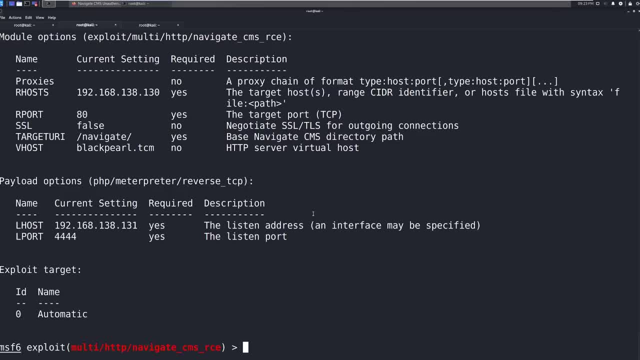 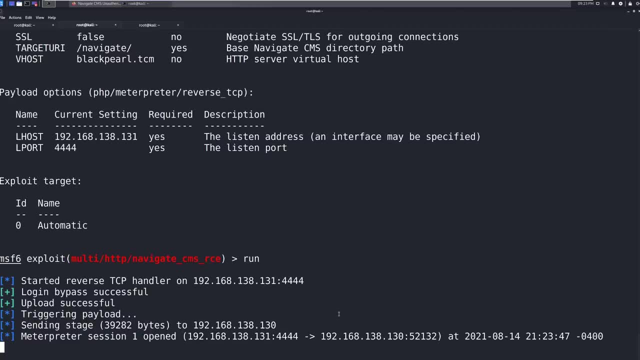 the target URI looks fine. I always like to do options one more time, just get the visual of it. Everything looks good to me, So I'm going to go ahead and just hit, run, cross my fingers, Hope and pray. Looks like we're getting a meterpreter session back, So let's hit enter. 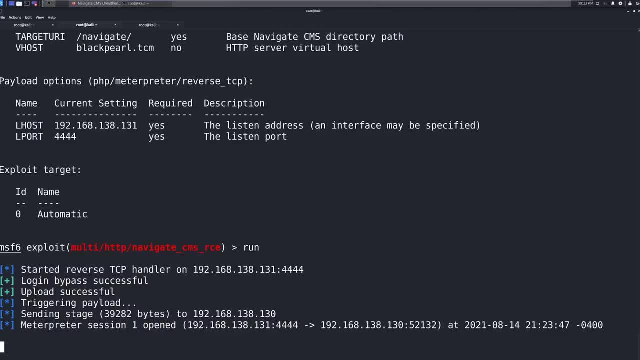 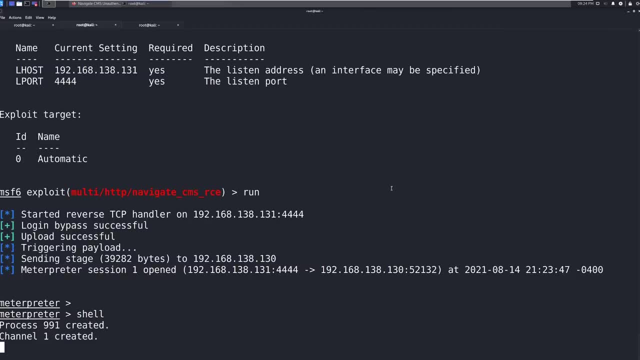 might be rushing the process here a little bit. We'll see if it works. Might take just a second to load. Okay, and from here we have a shell, so we can jump into a shell by typing shell And in here we don't see anything. But if we do, Who am I? 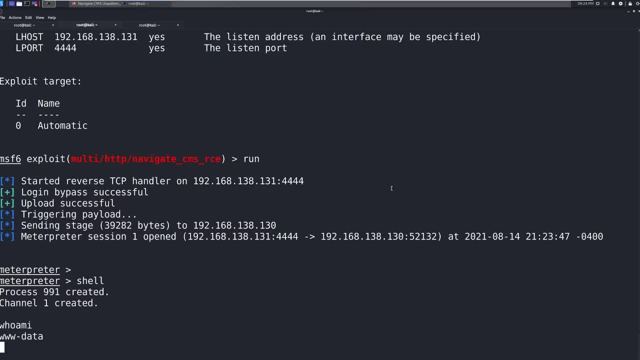 you can see www dash data, which means we're going to have to do privilege escalation again. Now we are in this funky little area. we don't see like a shell, normal shell type, right. We don't see like hey user at machine name. So we need to generate a TTY shell And there's easy way to do that If 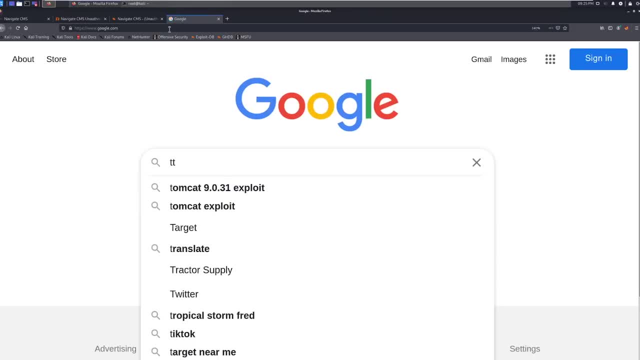 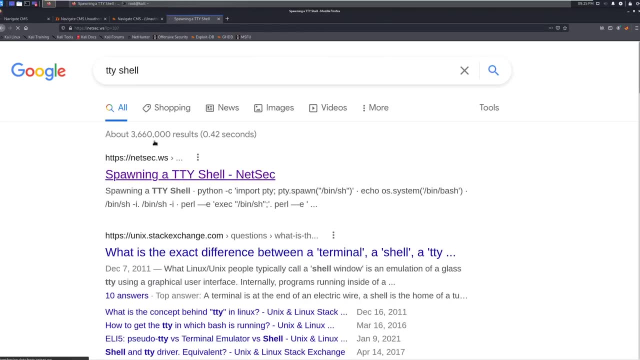 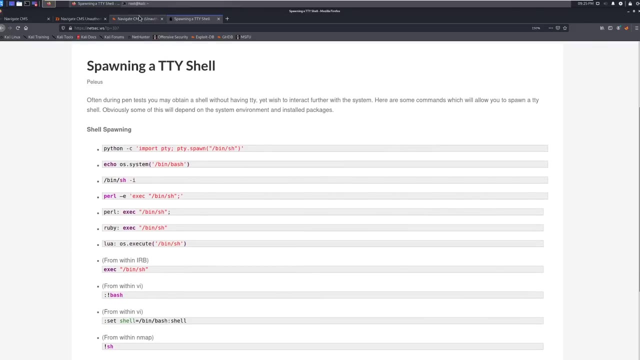 you go out to Google TTY shell. if you just Google that, you'll see spawning a TTY shell. Now my favorite method of doing this is using Python, But we need to have Python on the machine, So you'll see what this does here in a second. But there's other ways to do it. Python's quick way. 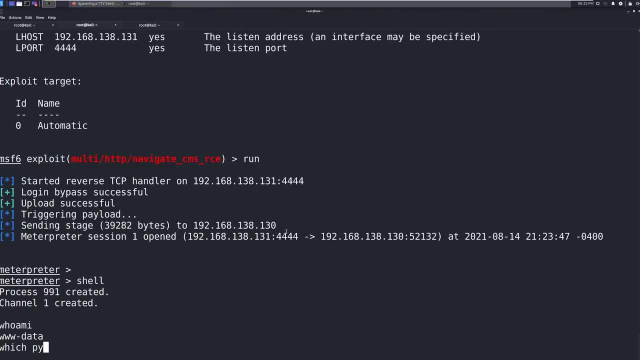 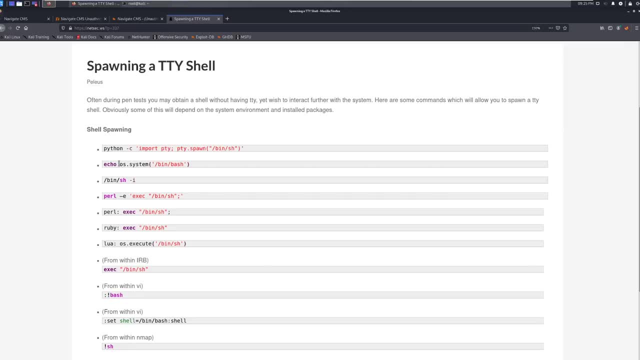 if Python is on the machine. So what we're going to do is just say which Python And you can see user bin Python exists on this machine. So that's where it's calling out. We're going to go ahead and just copy this, And I'm going to modify this a little bit. I like bin bash over just sh, So I'm. 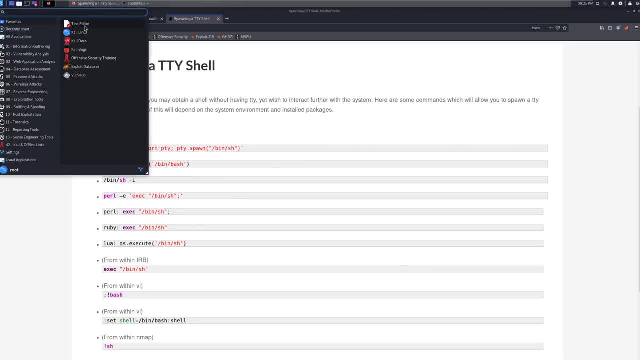 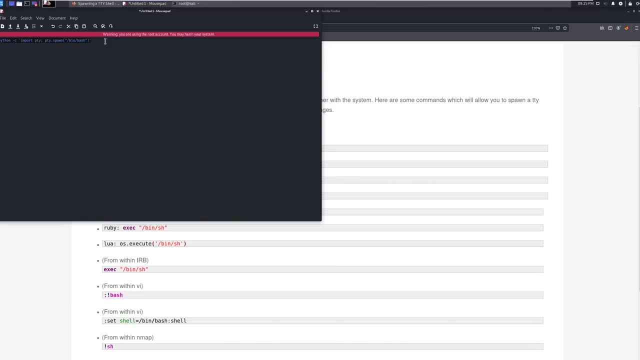 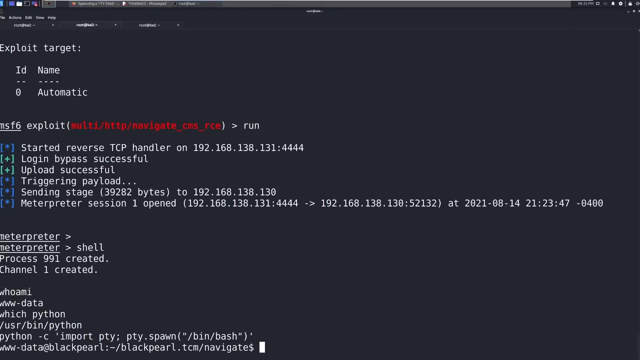 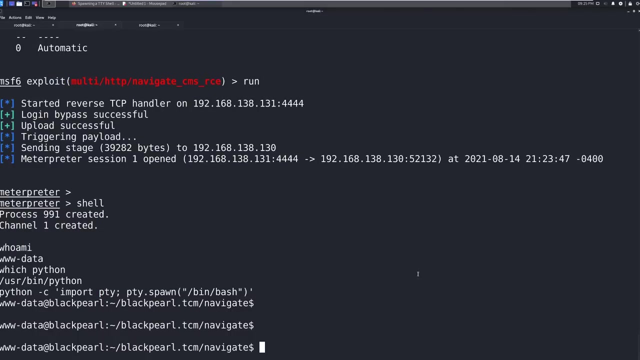 going to open this up in a notepad or a text editor, paste this in here, add a BA in front of that for me, And then we're going to go paste this into this shell. Okay, now that looks a little bit better. Now. we have an actual shell here. So what we need to do is we need to again go through our 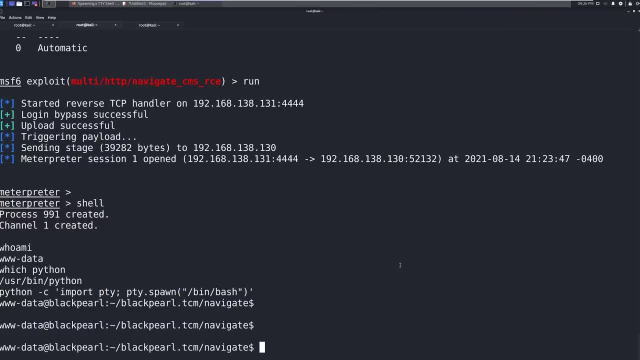 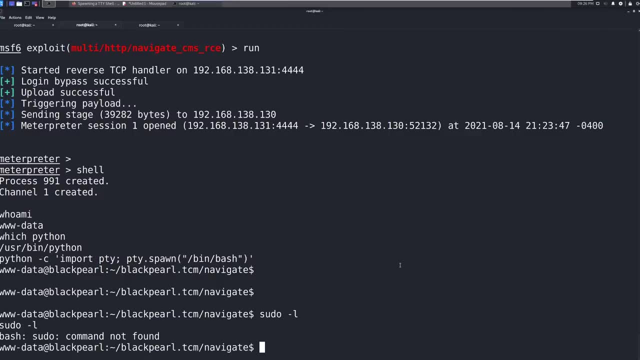 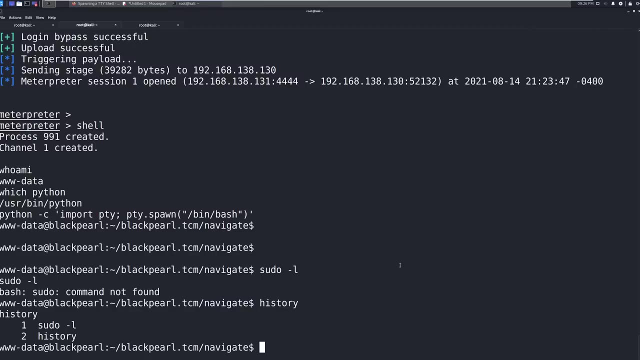 privilege escalation capabilities. In this instance, running sudo dash L, we can try see what's there. sudo command not found. Running history we could see that it's not found. So we're going to see if anything's there- Nothing Great. So we need to check for privilege escalation And we can do. 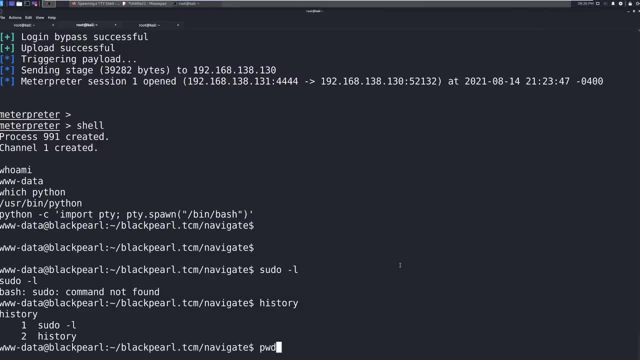 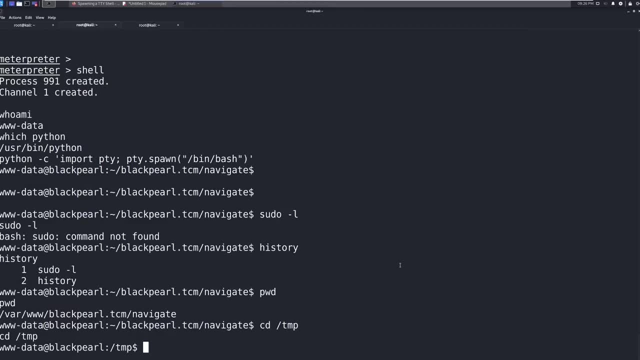 that using something like Lin peas- right, This should be familiar. Now we're going to do print working directory. I'm going to go ahead and CD over to temp, because that's where I like to move things. We are in temp And now what we're going to do is I'm just going to upload this, this file. 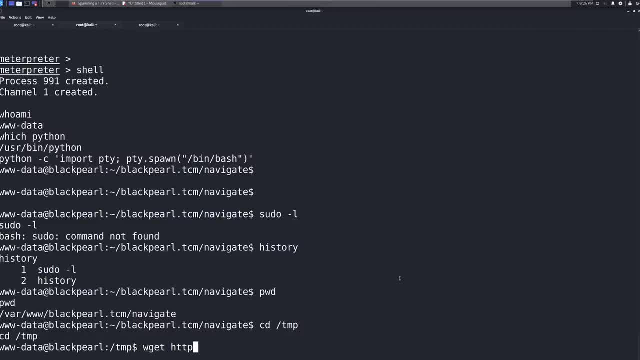 So we're going to do a w get And I don't have it Hosted yet, but I'm just preparing it. So 192, 168, 138, 131 attacker IP address forward slash: Lynn peassh And then Lynn peassh. This should be familiar. Now we're gonna come in here And 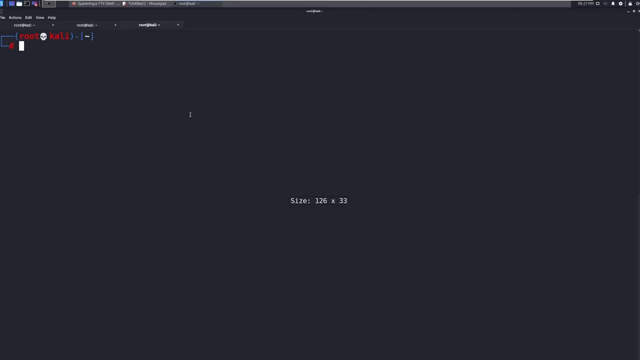 we're going to a control plus here, we're going to go ahead and we're going to CD to transfer. you should have one of these by now. Yes, Lynn P should be in there. So all we're going to do is Python three, dash m, simple, Sorry, HTTP. 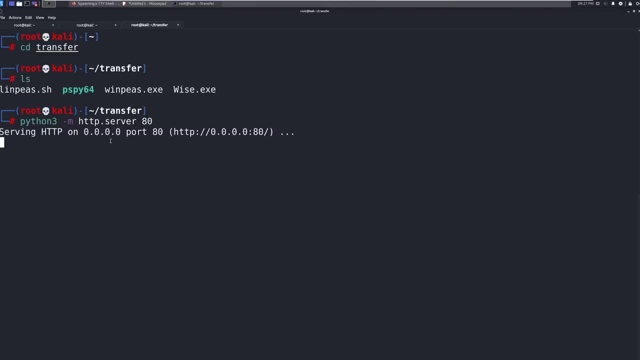 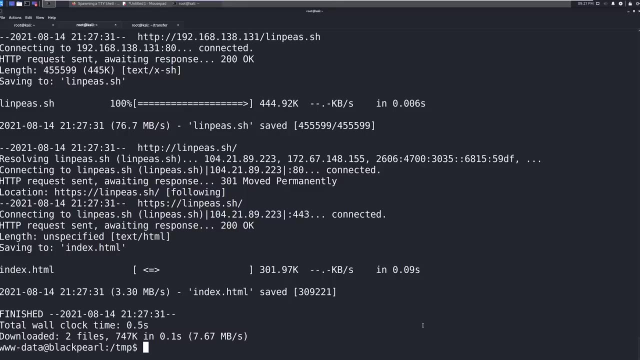 server. I'm thinking my Python two days and port 80. Now we should be able to run this. Okay, Let's go ahead and let's see if it actually generated. Did I call out Lynn peas? I did. Let's see ls Lynn. 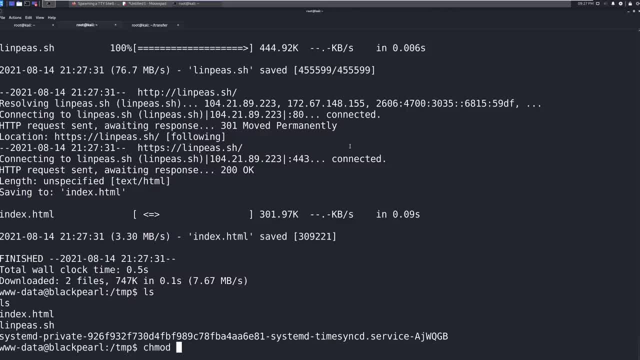 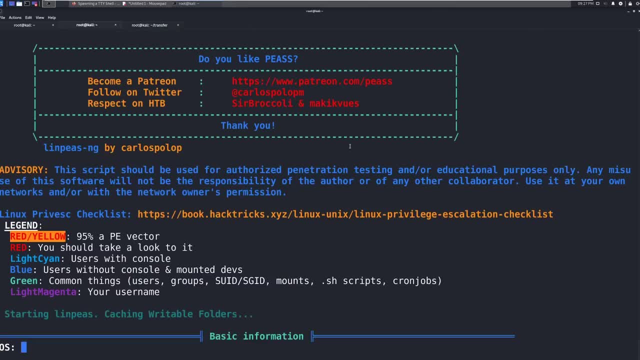 peassh. So I'm going to go ahead And just ch mod plus x- Lynn peassh. Ford slash Lynn peassh. Okay, now that's gonna run. So let's let this run for a second. I'm going to pause the video, let it run through, and then we're going to come. 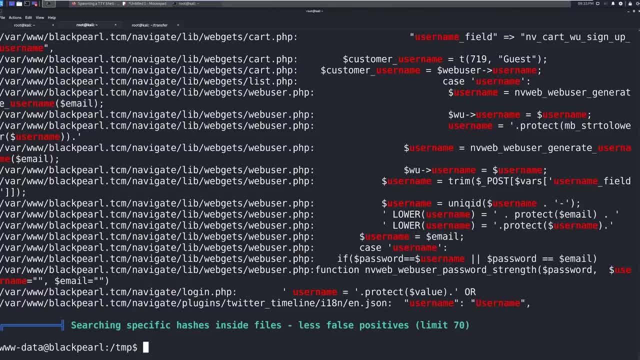 back and look at the results. Okay, so the results have come back And we're going to look at it from the bottom up this time only, because last time we took it from top down, We're gonna go bottom up. the top section is: 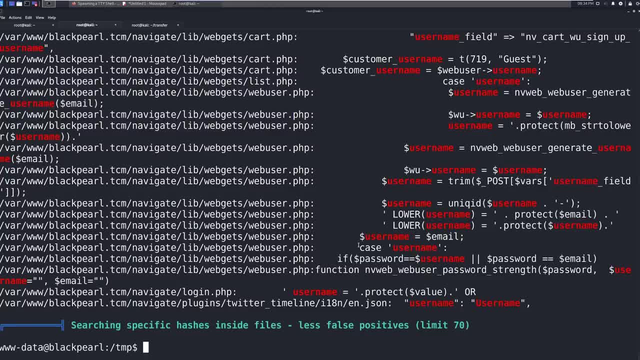 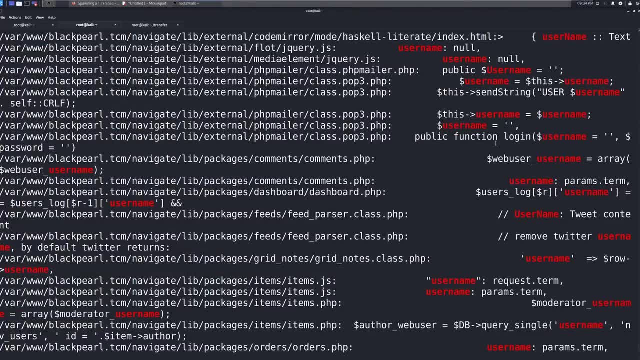 really very system and what users are there, and it's a lot of good information. but at the same time we can kind of just skip down to the bottom and scroll up like here: we're looking for usernames or passwords that might exist and we're just kind of going. 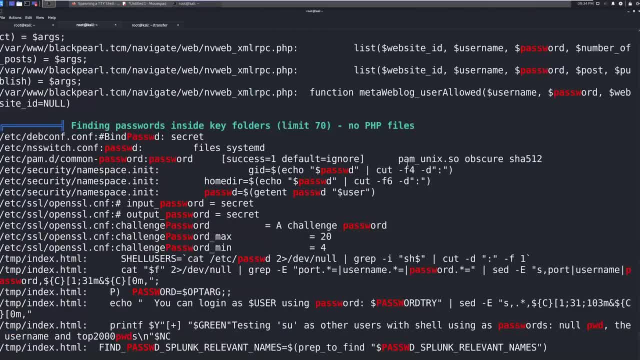 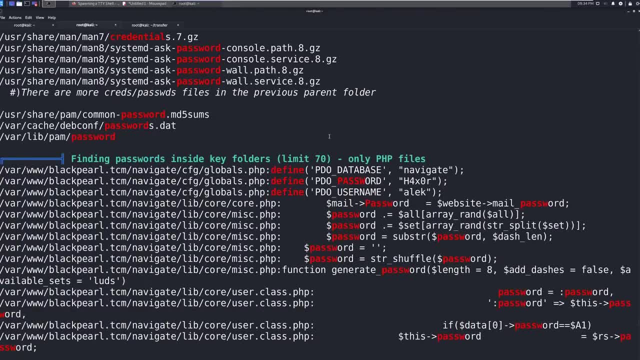 through and trying to see if there's anything in here where we could find that would be relevant. remember, we're looking for red and we're looking for red, yellow, specifically. that would be good. I'm gonna skip over some of this and I'm looking for, in particular, some different things. now, if there's any sort, 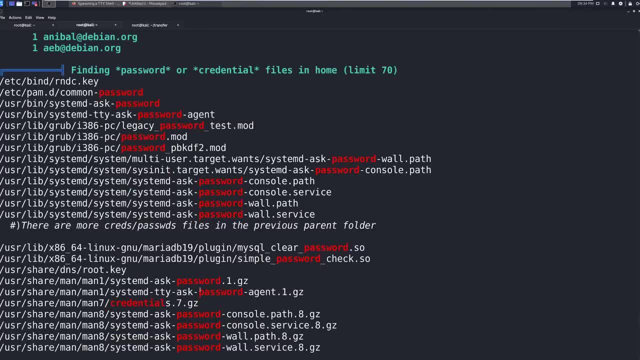 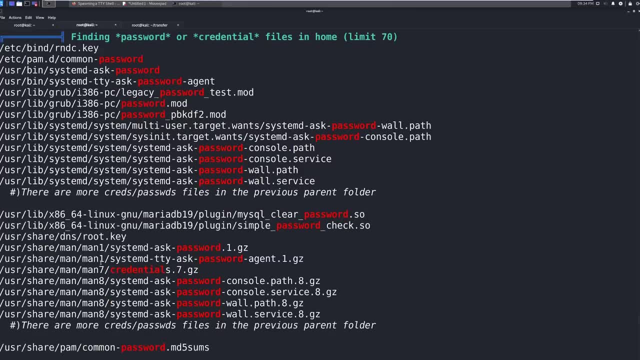 of password or credential here. that could be interesting. if there's like a file named password or password, credential and you kind of learn what these are, you're really looking for something to stand out. none of these really stand out. these are all common, kind of just pads on the system and 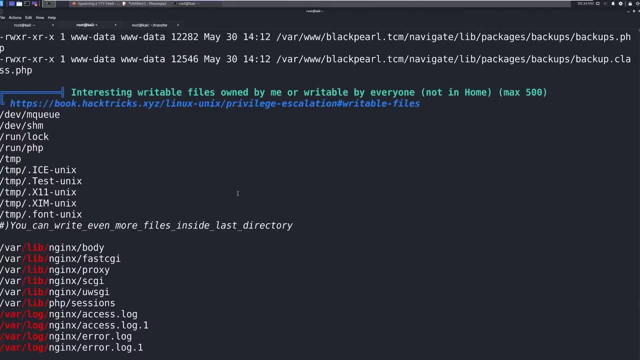 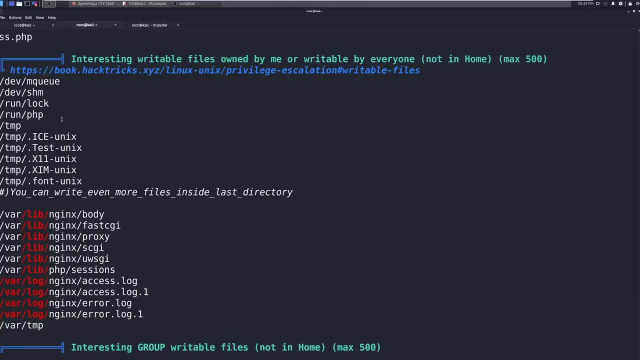 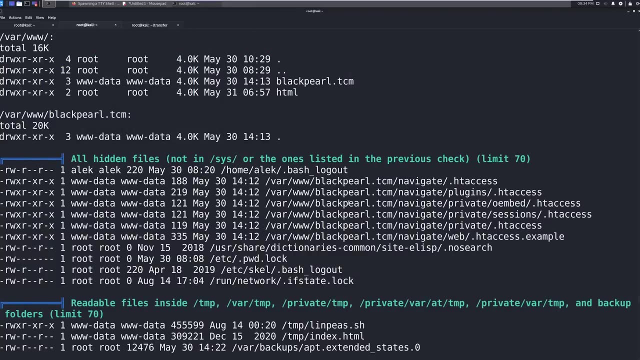 common files on the system. now, if we keep scrolling up, what I'm looking for are any sort of interesting writable files like here: run PHP, run lock, but there's like we need to be able to have something that we can abuse. the feature of it has to be more than just writable. so, again, this is providing 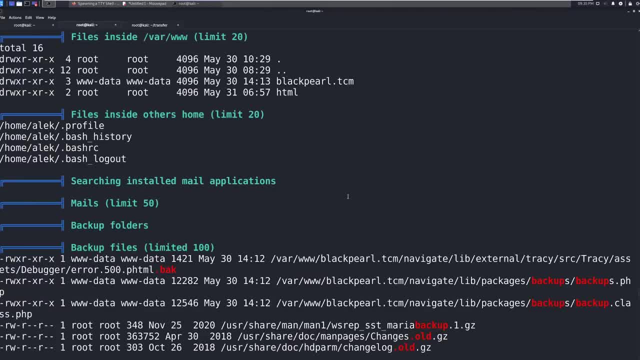 information, but it's not always going to be one specific thing. now, backup could be interesting, like there's backup files. it looks like this is specifically to the bar WWW navigate. there could be information in this backup folder, like there could be perhaps like passwords or something in here, so this could be an. 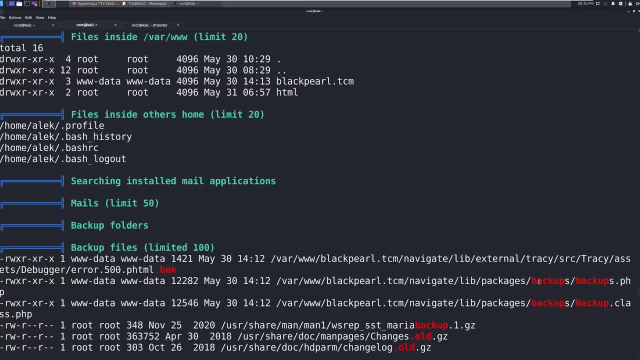 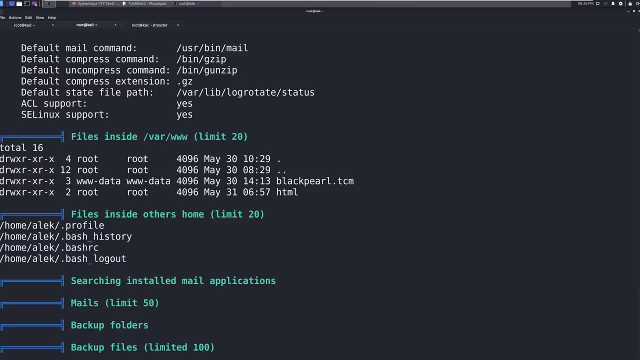 area where we might want to look at, just because there might be a password for a user, that user might be the root account password. we have no idea, so we kind of want to look at that. we do want to know what other users are on this computer, so starting at the top is not a bad idea. we could also just cap. 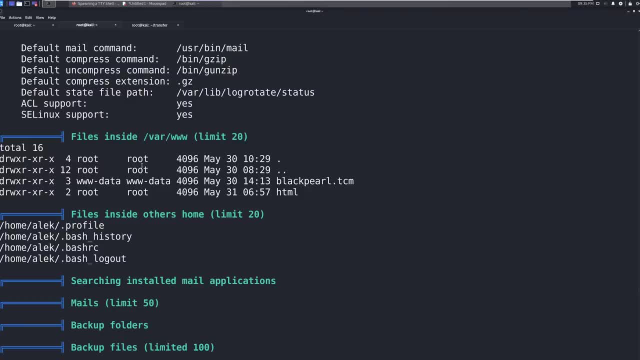 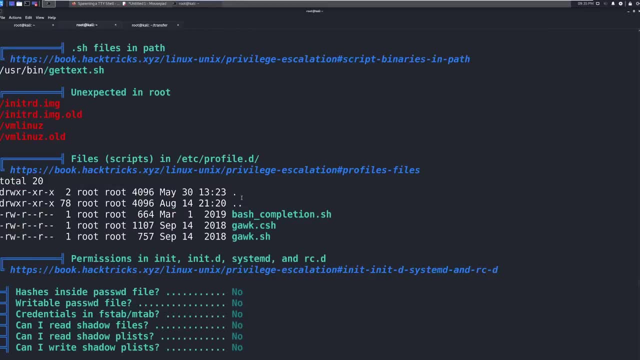 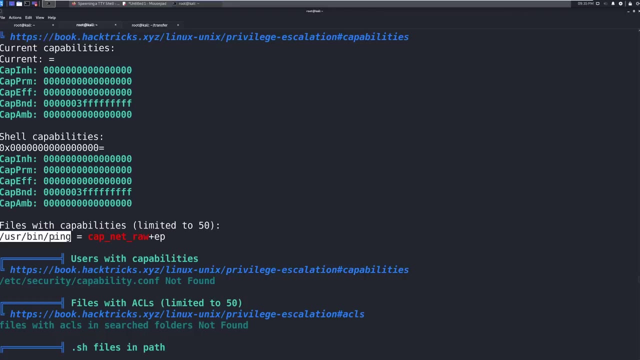 the Etsy password file and see what's going on there. in this instance we see root. we see WWW dash data. there might be more users, we're not sure quite yet. keep scrolling up, let's see if there's anything in here capabilities could be a possibility for us to look through. we'd have to look at GTFO bins and see this. 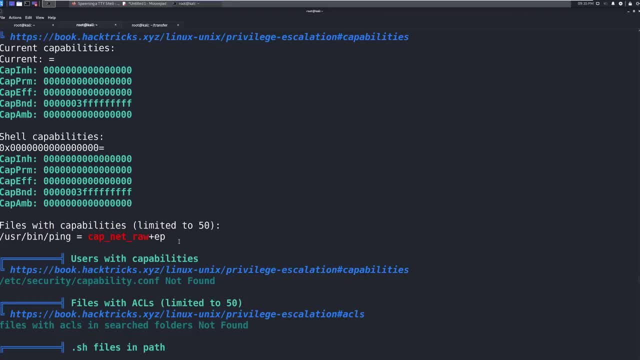 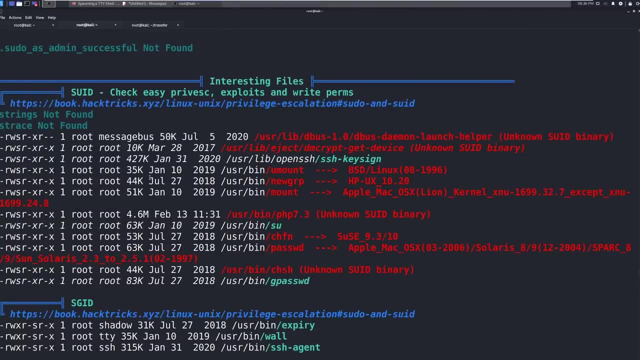 is something that's a little bit beyond the scope of this course, but it is covered in the previous courses and we're gonna keep scrolling up, and this is where this gets a little bit interesting, especially when I start seeing unknown su ID binaries. so let's talk through the su ID. 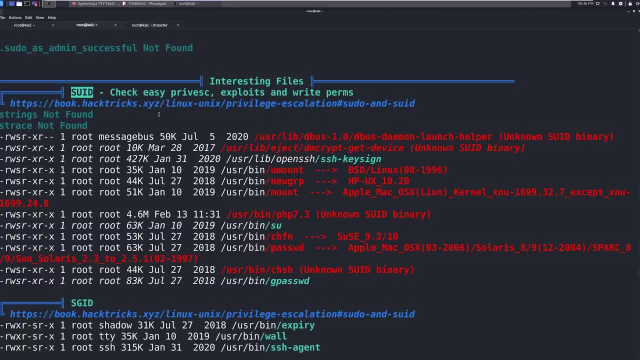 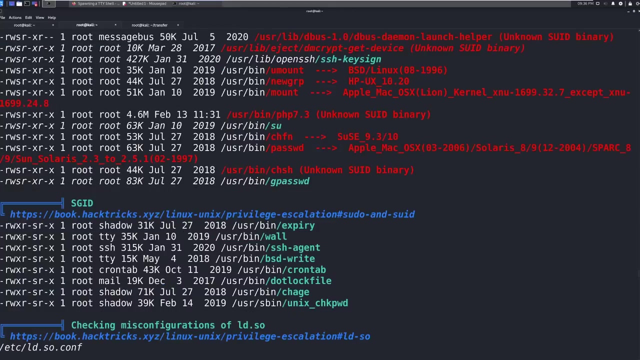 and the, the sticky bits and all that good stuff real quick. so this is actually a great example. so we're looking in here and we have what is called an su ID set. now, if you remember, recall from our early Linux lessons, we have file permissions. we have read, write, execute. let's go down a little bit like right. 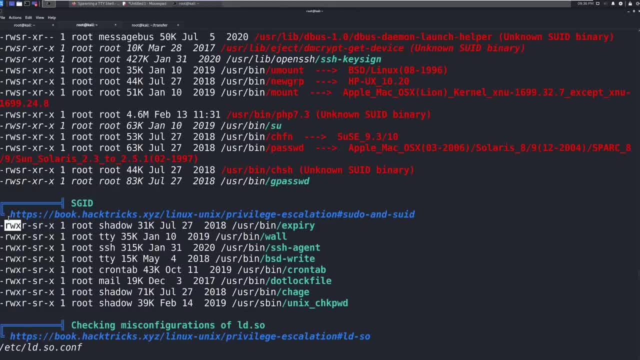 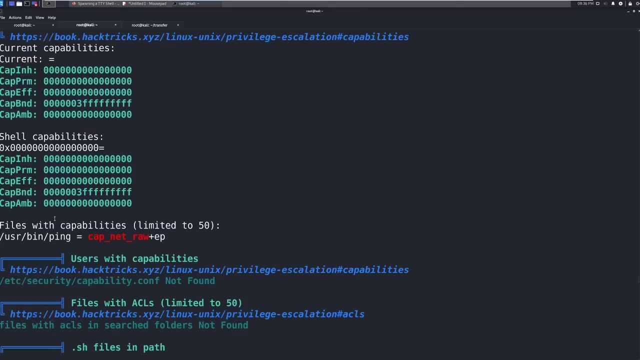 here: read: write: execute. this is the root setting. okay, this is the owner setting. I should say owner of the file. this is the setting. read blank s: okay, this is actually SG ID. this is okay. we're gonna. let's pretend this says. let's pretend this says: execute. like this right here, read blank: 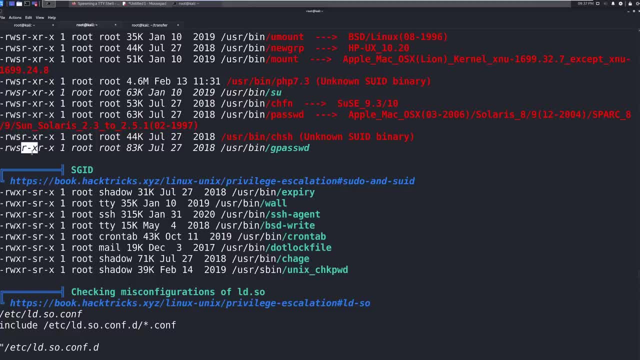 execute. so this is a group setting. anybody belonging to this group has read and execute permissions. they do not have right permissions, anybody in this one. okay, this is global. this is uh, read, execute again. so we see here who's the owner of the file. when we're looking at all of 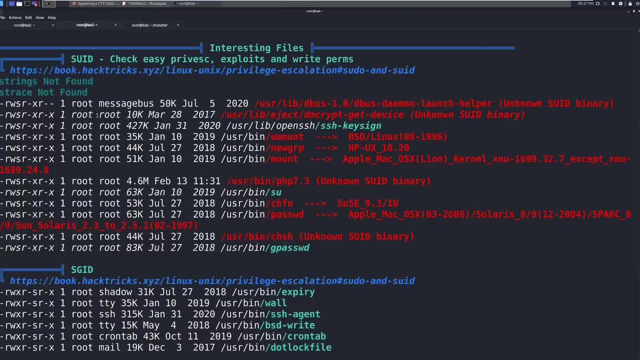 these. we see, root owns all of these different binaries here. okay, now let's talk about su ID. you see, instead of read write execute, we have read write s. okay, s is our su ID. this means that we can run this, and whenever we run this, here we have the. 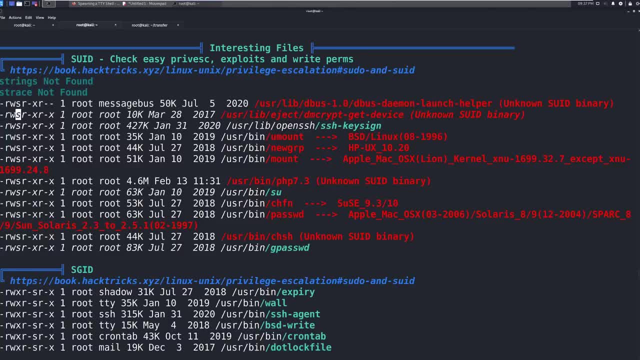 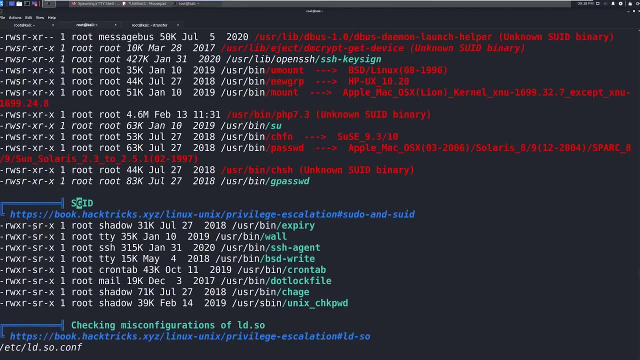 ability to run this as the user that owns it. this is a uh and the su ID. we're on the root here- or the owner. sorry, we're on the owner, so we can run this as the person that owns it, which is root. now you see down here what is called an SG ID, which means we can run as the 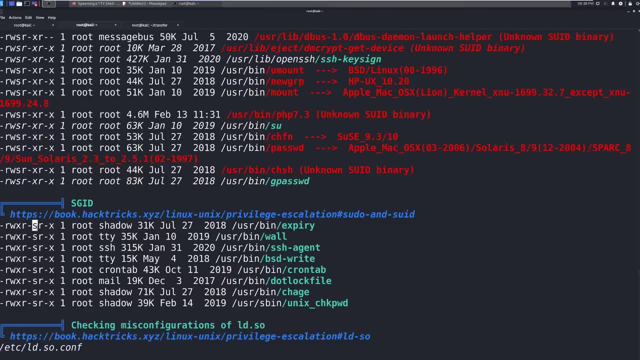 group and that's sticky right here or it's an s right here. I keep calling it sticky. the sticky bit is when it's in this. when you see an S in this area, right here for everybody else that's called. the sticky bit. here is SG ID and in this group setting it's an su ID. when we look at su ID, 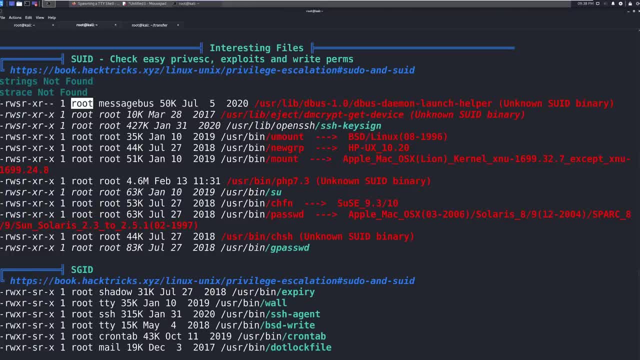 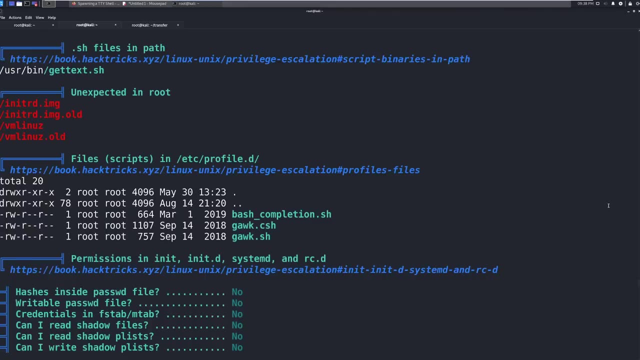 it's very interesting because we have root ownership. we could run this binary as root and abuse that feature. now there is a quick way to do this and I can show you how the script is running this. but this is really just looking for permission settings so we can come through and 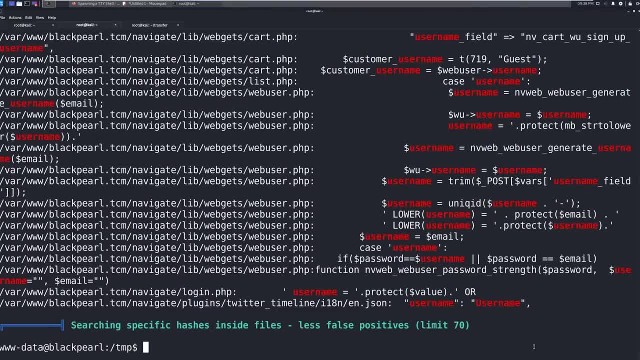 look and if you ever go through a, a checklist, you'll see something like this where it's just doing a quick find command and it's looking to see if it can find the permission settings on these. okay, so permission is going to be four, zero, zero, zero, and this is looking specifically. 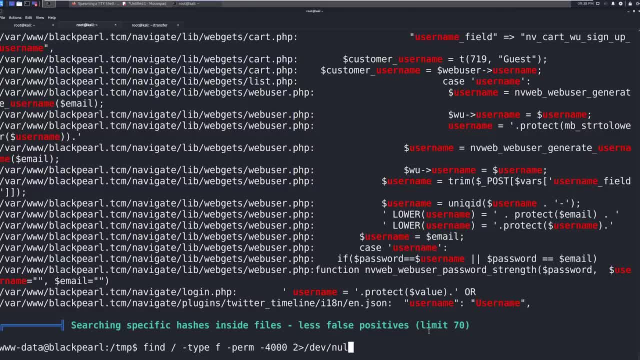 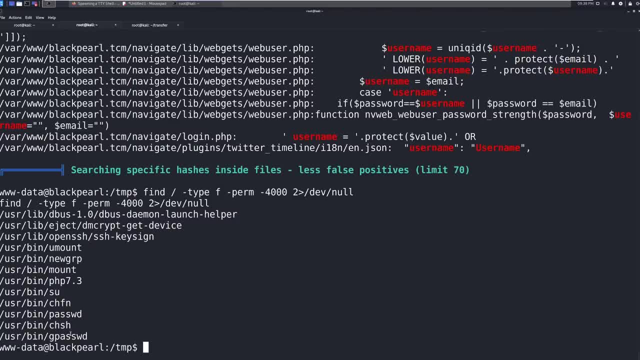 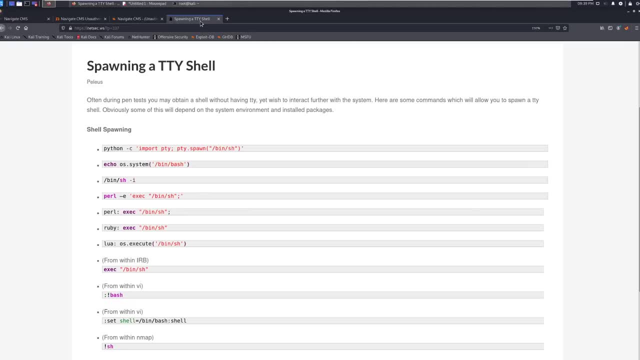 for that su ID, and we're just going to put this to dev null. here and now you find all these in a much cleaner setting. so, from our perspective, what we want to do is look at this, because not having the suid enabled does not necessarily make it vulnerable, but we have a great website that we looked at earlier. 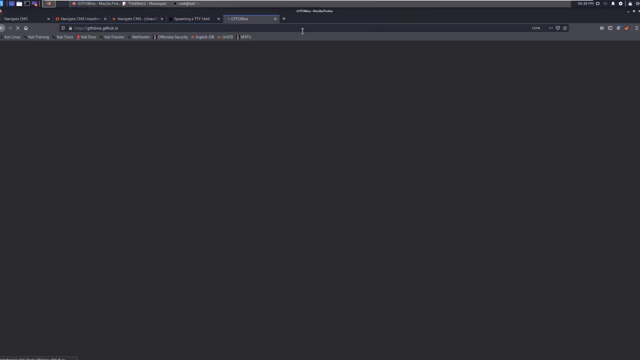 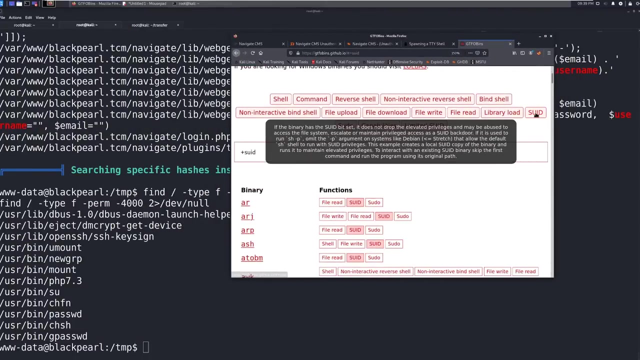 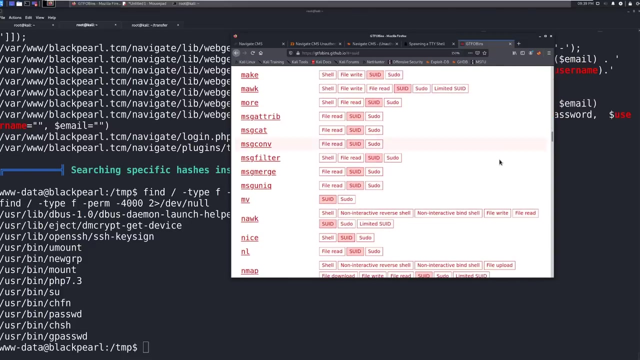 gtfo bins. okay, dot githubio, and we can do something like this. we can come in here and say, okay, we've got suid, and then maybe we want to start looking through some of these, like maybe like I don't know- mount, for example, if we can come through, see if mounts in here mount what. I'm looking right here. 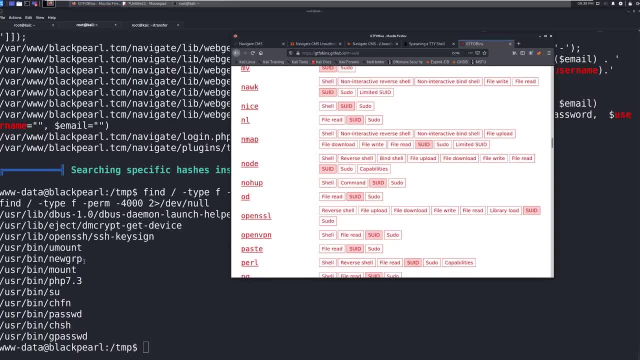 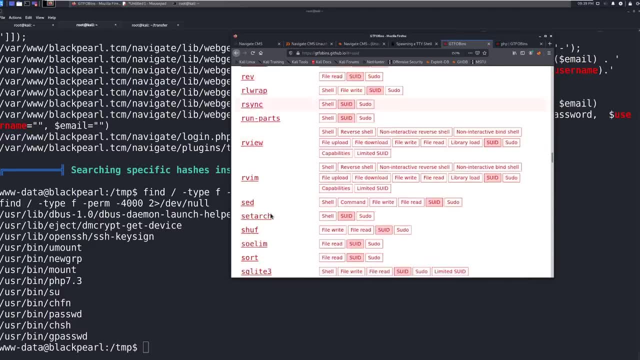 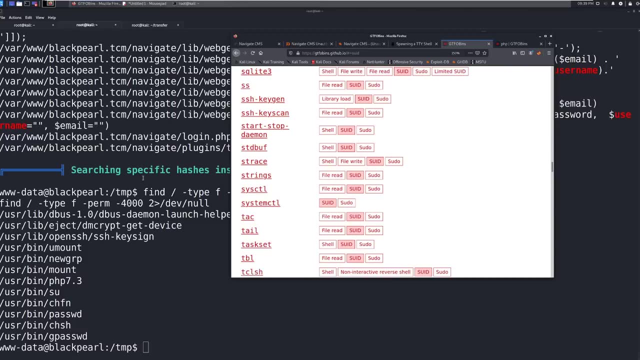 not there. um, this new grp not there. uh, php is there, even though it's 7.3. php is there, so maybe we want to open that like: uh, switch user su. I don't see it in here and you would just go through this list and say, okay, does anything on this list? 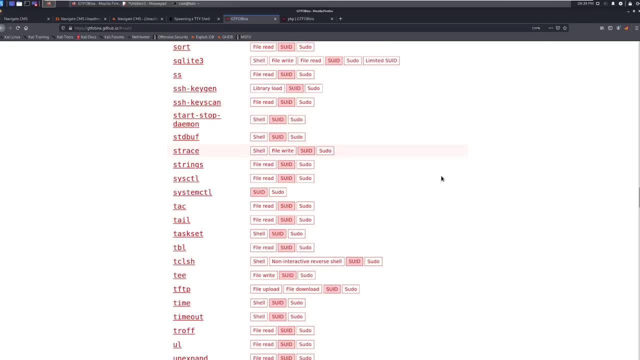 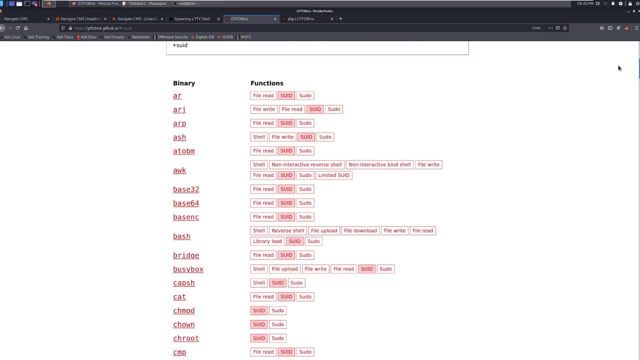 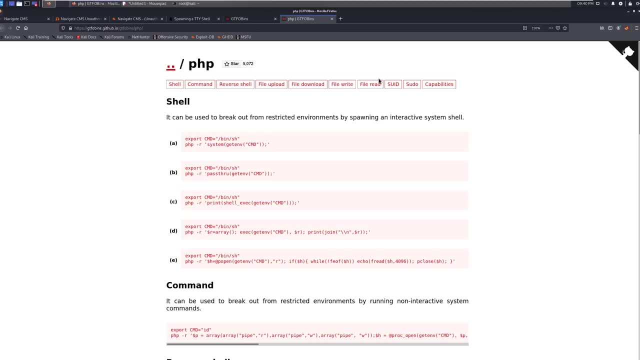 stand out as um, as being a privilege escalation. now, you are not expected to remember all these. there are some that you will see and it will stand out because you've done it time and time again, but for this situation, this is absolutely what the gtfo bins is built for, so we can scroll down. 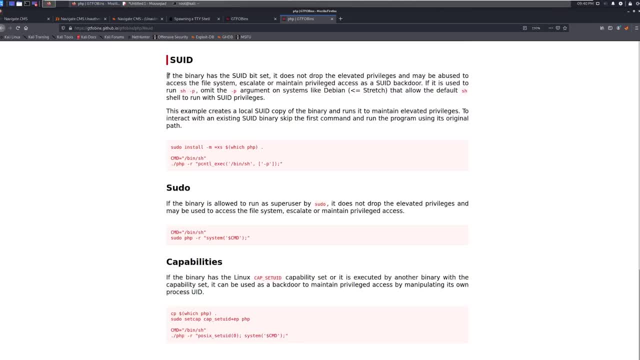 over to suid and click on it and it says: if the binary has the suid bit set, it does not drop the elevated privileges. it may be abused to access the file system, escalate or maintain privilege. access to the backdoor: okay if it is used to run sh-p. omit the dash P argument on systems like debian that. 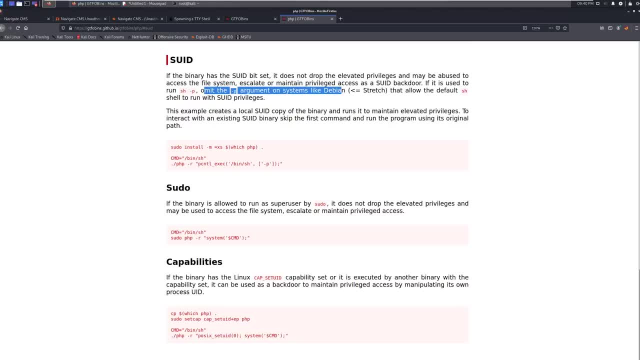 allow the default sh shell to run. so it's giving us some instruction here. okay, so all we need to do on this is we just need to run the php and we need to run it with this rest of this setting here. okay, that's, that's really it, and we're going to call out that binary specifically, so you copy this: 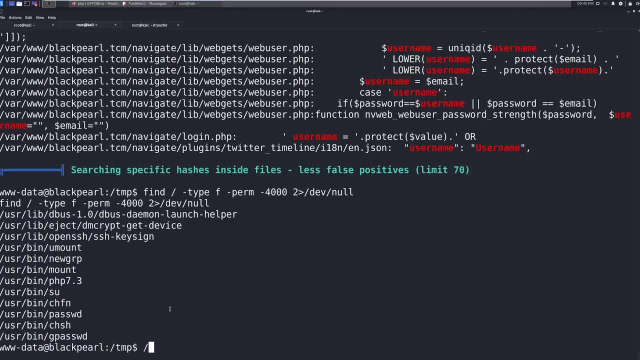 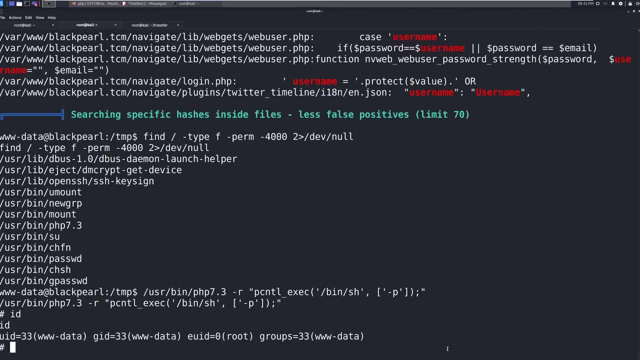 come back in here, we see the binary is sitting in user bin php 7.3, and it shouldn't matter that it's php 7.3, just paste the selection. okay, this is going to execute bin sh as the root user, giving us, hopefully, a root shell which it gives us the euid of root. okay. 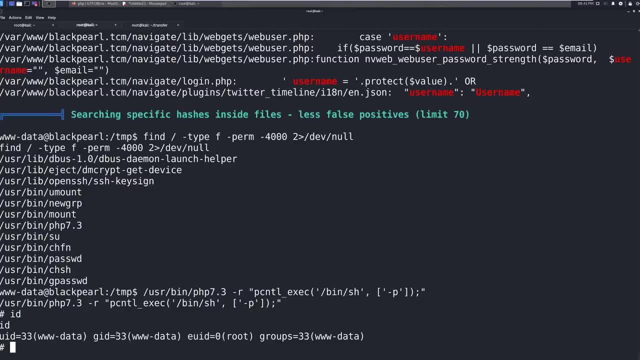 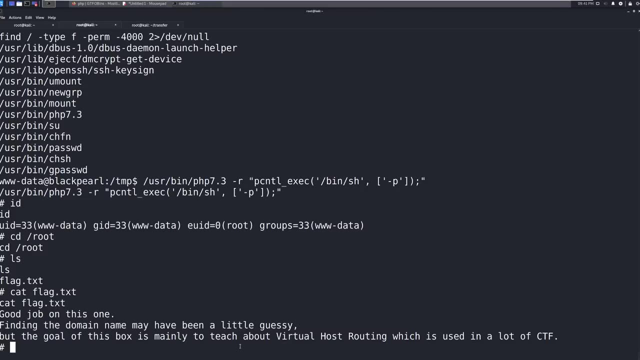 which means, even though it says we are uid of ww data and a group ID of uh wddata. look at this, euid. what we can do with this is cd 2 root ls cat flag dot txt. we are staying as the root user, but we're running in a shell that is executed by route. 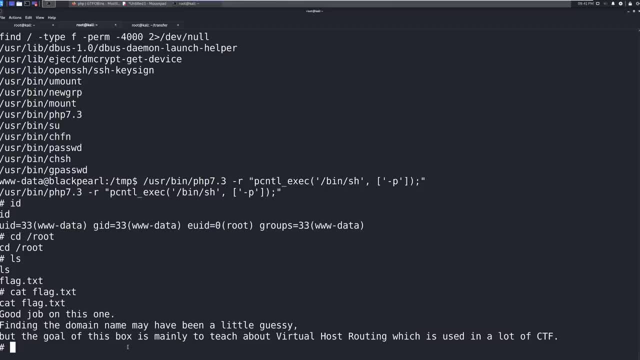 Okay, so it's a good job on this one. finding the domain name may have been a little Guessy, but the this box is to teach about virtual host routing, which is used a lot on CTS, which is true. So, and proof of concept here: 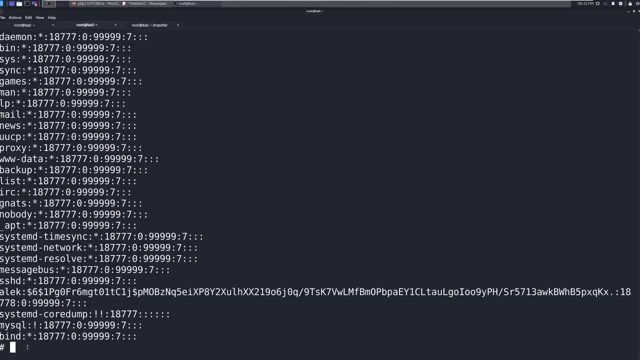 is, you should be able to cap the Etsy shadow file. Okay, Prior to this we would not have been able to do that. doesn't matter that when we write Who am I? Oh, we're actually showing his route, but our ID is still staying as WW data. Okay, but we are. 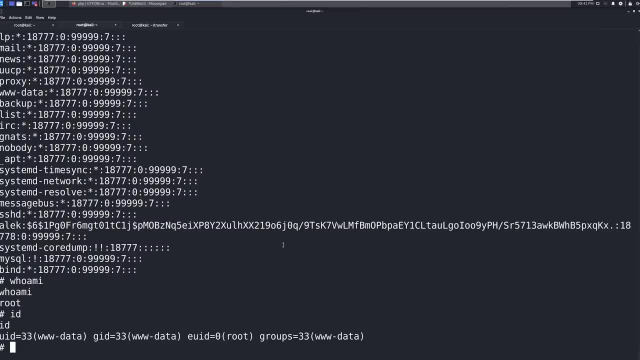 executing as root right now. So keep that in mind. We are the root user, we have owned this machine as the root user, And that's it. So su ID is a new lesson for you. Again, if you like this concept of privilege escalation we are scratching. 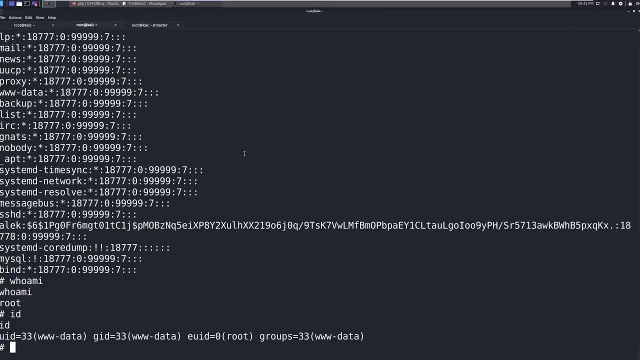 the surface. there's so much to learn. There's always new tips and techniques out there. I encourage you, if you're interested in the CTF path again to check out the escalation courses. If not, we're going to start moving into. 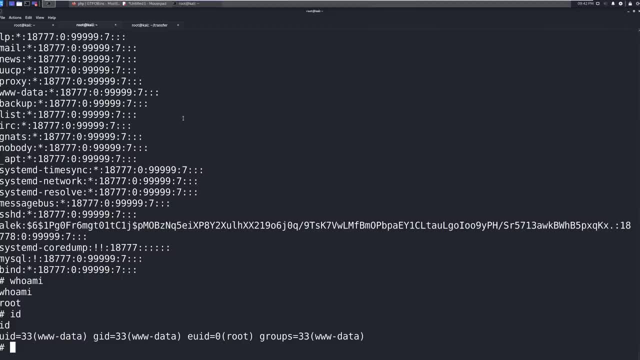 exploit development. we're gonna start moving into exploit development. we're gonna start start moving into exploit development. we're gonna start moving into some of the other stuff that's out there with the Active Directory, pen testing and get more into the realistic stuff. So this is good foundational lessons, but I look